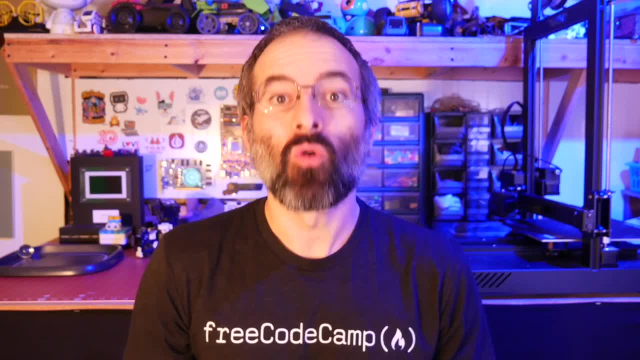 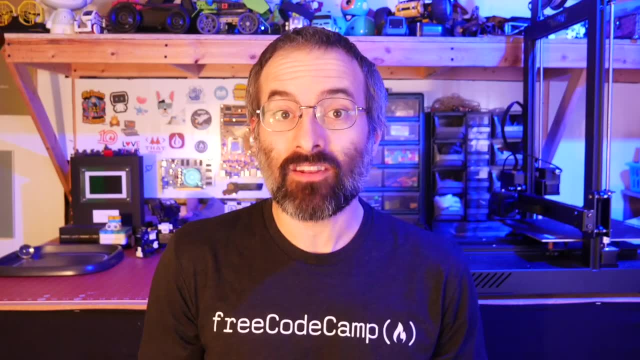 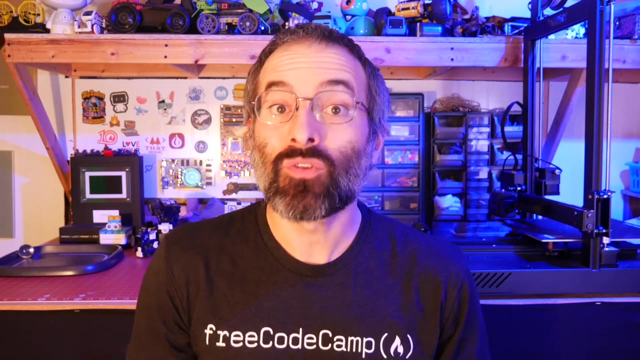 This course will teach you to build real world apps with react router six. you will master essential react router features, such as layout and index routes, nested routes, search parameters, route protection and the new remix inspired data router API's. Bob's role teaches this course. 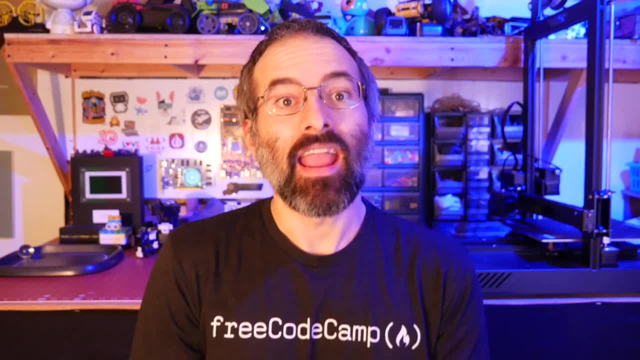 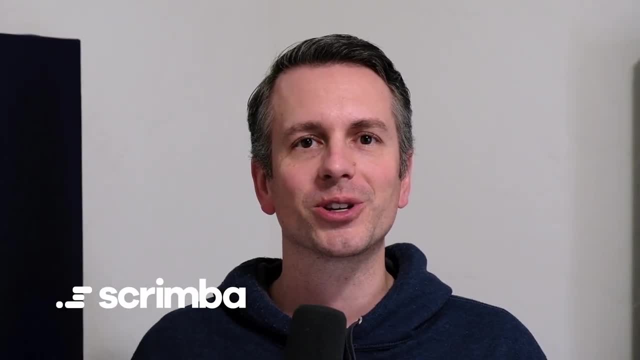 He is one of the most popular react instructors ever and is also the head of education at scrimba. Hi there, free code campers, and welcome to this interactive scrimba course where you are going to learn how to use the react router library to build single page applications in. 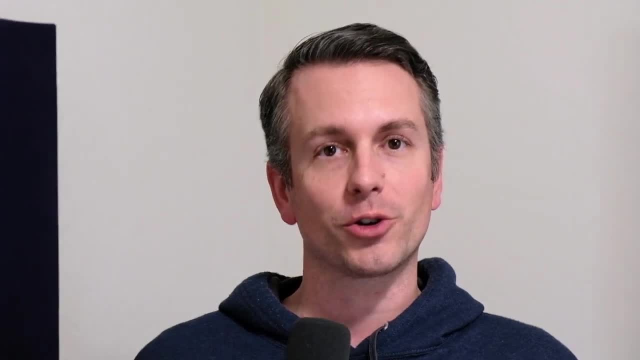 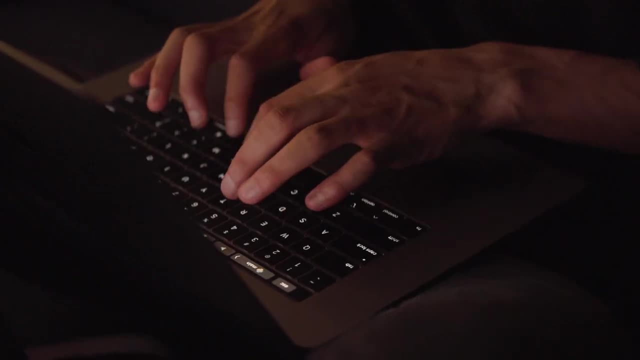 react. Since this is a course dedicated to a specific third party react package, it's going to be pretty important that you already know react. If you haven't yet learned react or you just need a refresher, I've got you covered. I've got another free course here on free code camp and 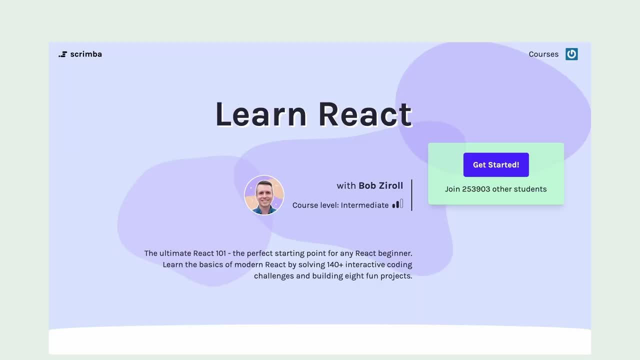 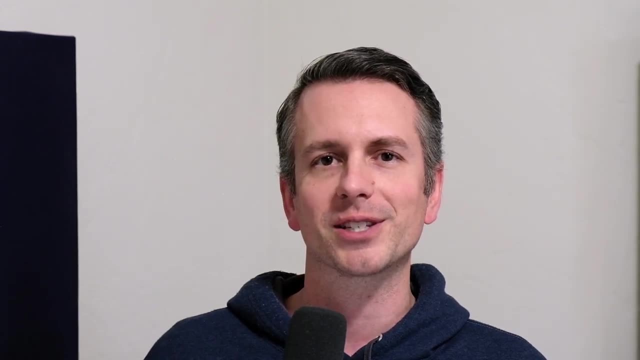 on scrimba. That's a complete introduction to react. you can check the video description below for a link to that course And then, when you're ready, you can come back to this course. it'll still be here for you, I promise. Now, the special thing about this course is that it is fully challenge based. 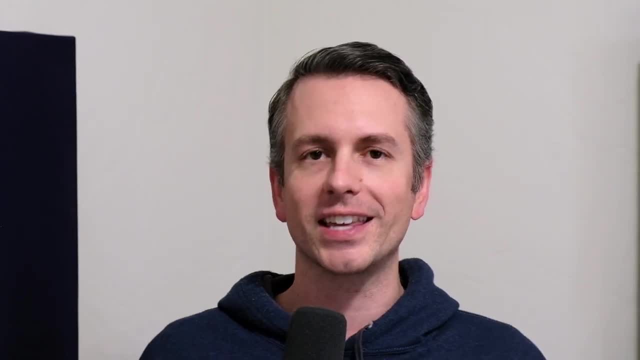 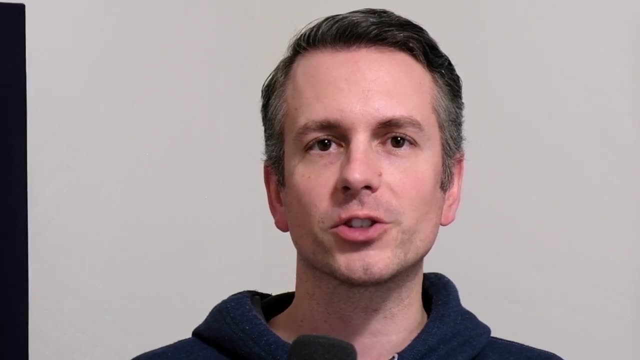 which means you, as a student, are going to get your hands on the keyboard again and again to really practice the topics that we're learning And if you're feeling a little bit concerned at all about following the challenges of this course on your local development environment. 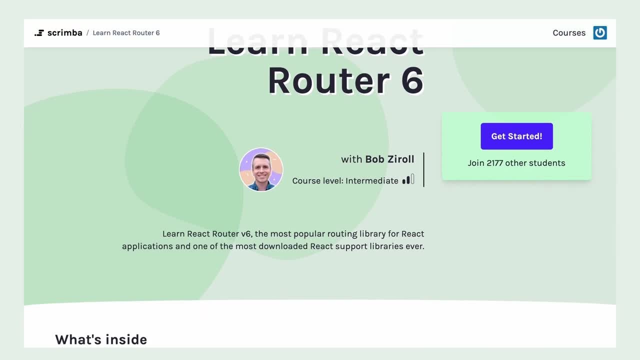 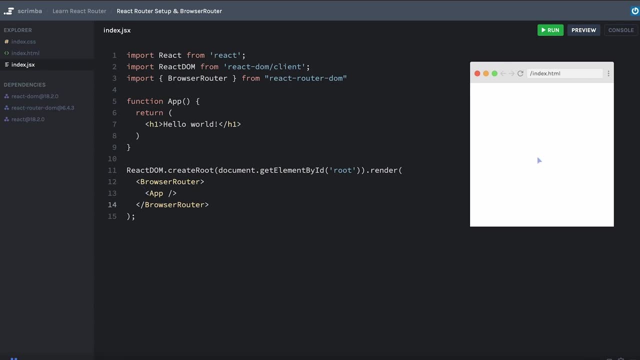 don't worry. That's why we've created an interactive version of this course over on scrimbacom. There, you can solve all of the challenges directly in your browser without having to worry about anything with your local environment. If, instead, you do want to follow all of the challenges on your own local environment, that's great too. 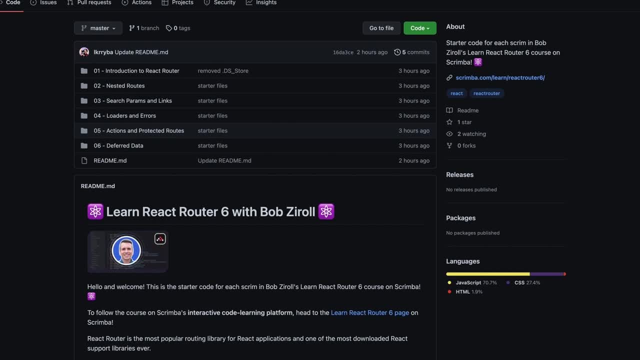 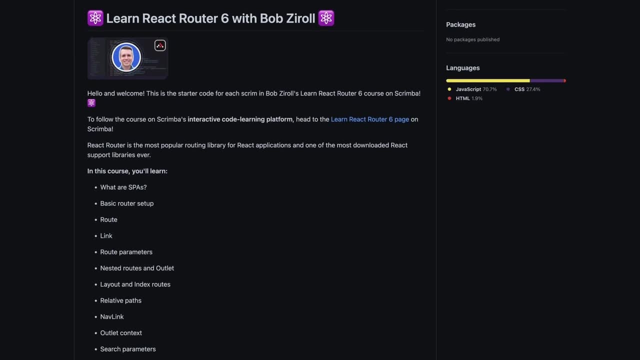 I've got a GitHub repository with all of the code that you'll need in order to follow any of the challenges that we have throughout the course. Again, check the video description below in order to get links to that GitHub repository. One final thing, if you are enjoying this course, 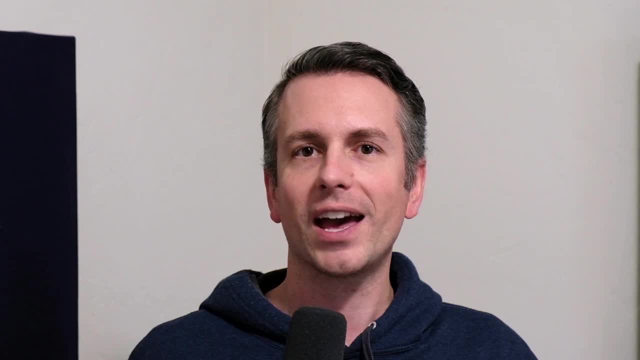 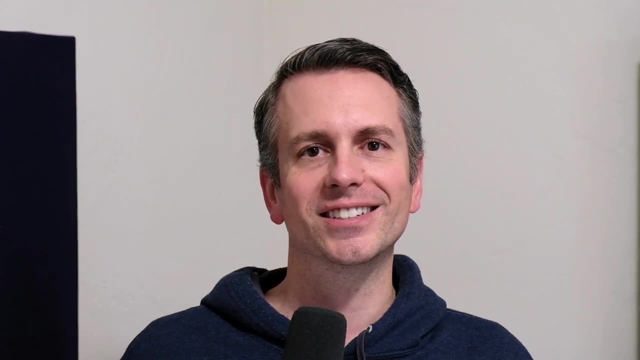 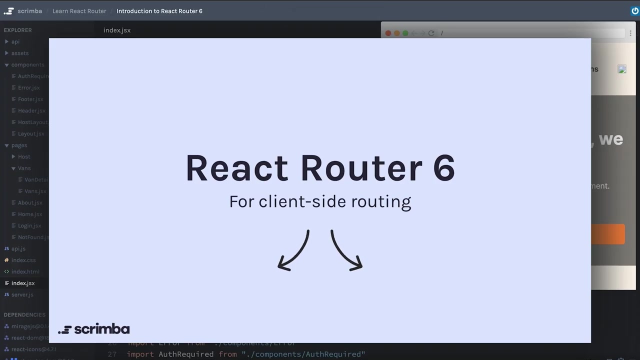 I ask that you please give it a thumbs up here on YouTube, And if you have any feedback for me, you can always reach me on Twitter at Bob's role. So, with all that said, let's get started. Welcome to this course on React Router 6.. I am so excited to guide you through one of the most 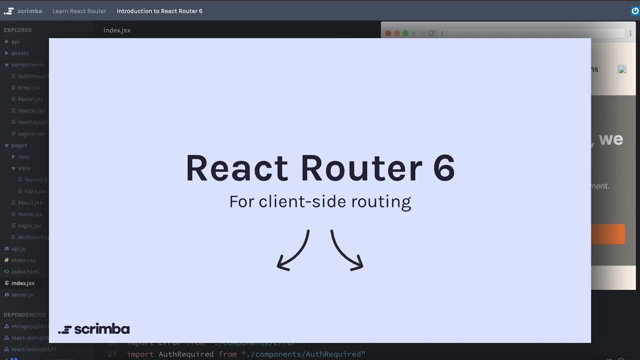 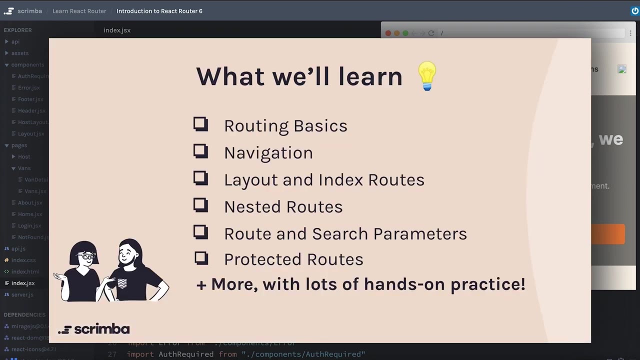 popular and impactful libraries that exists in the React ecosystem. Now React Router is a library used for enabling something called client-side routing, And understanding what client-side routing even means is just one of the many things that we're going to learn in this course From a really high 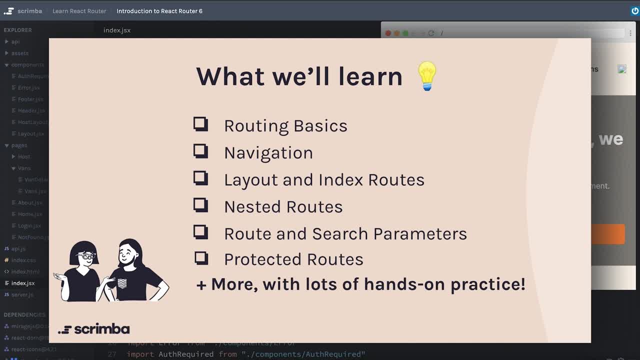 level. we're going to be learning about the basics of using routes and how to use them. We're going to learn about how to navigate between our routes. We'll learn about layout and index routes- nested routes. We'll dive pretty deep into learning about search params and how to 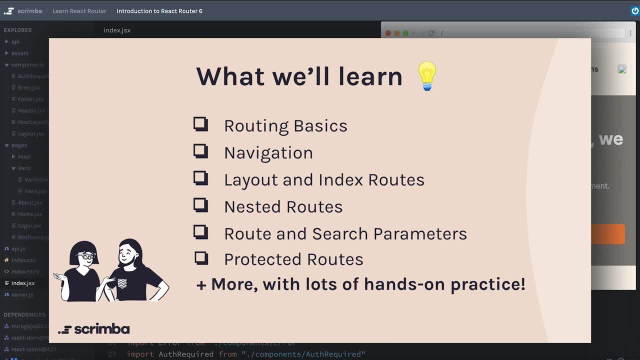 filter results, And we'll be creating protected routes so that you can allow only authenticated users to visit certain parts of your page. Along with those, there's a ton more that we're going to be learning And, of course, in the typical Scrimba fashion, we'll be doing tons of hands-on. 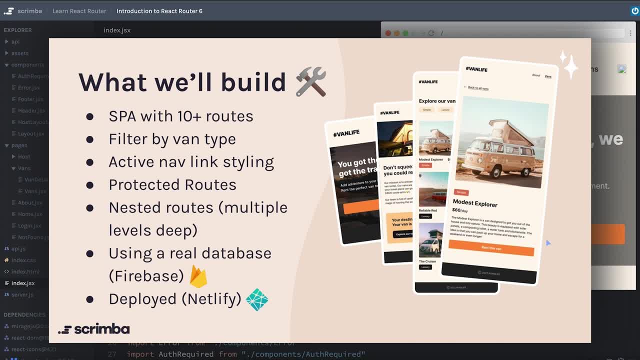 practice. In order to drive the curriculum forward, we're going to be building a really cool app called Vanlife, And we're going to be building a really cool app called Vanlife, Which is a way for people to rent out camper vans for their next road trip adventure. 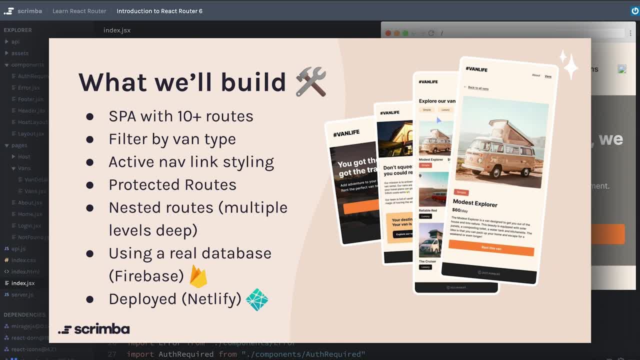 This app will have over 10 routes. We'll be able to filter the vans by their type. We'll learn about active nav link styling so we can very easily tell in the user interface where we are. in the current app, As I mentioned, we'll be including protected routes so that certain pages 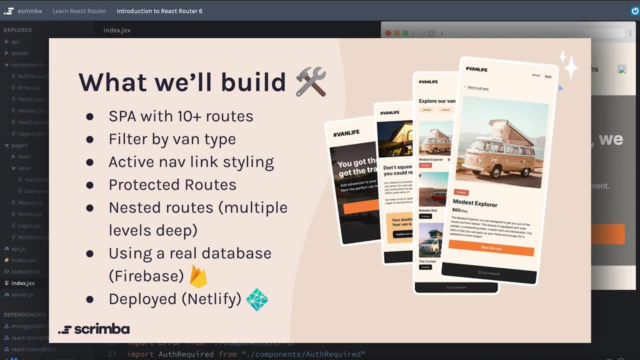 will only be accessible if you're logged in And we'll be hitting hard the concept of nested routes, because this app goes multiple levels deep into nested routes. Then, towards the end of the course, we're going to be shifting focus briefly to learn about how we can migrate our fake data into a real 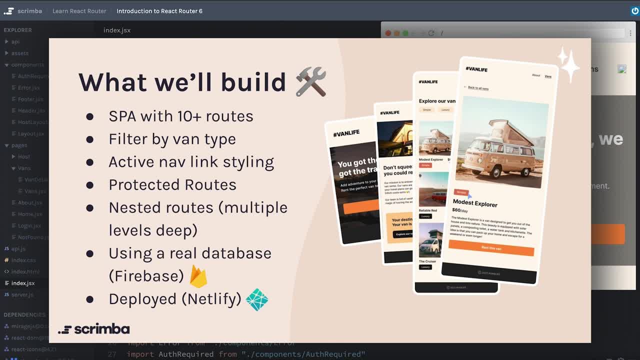 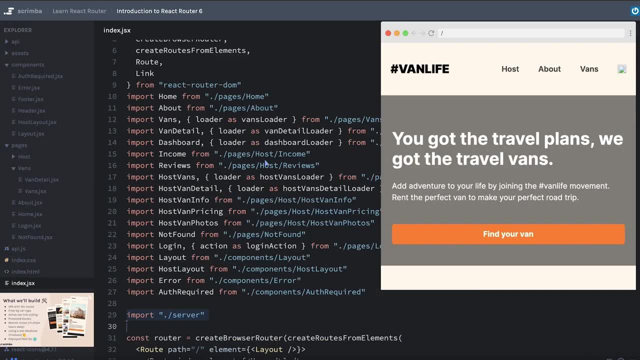 database using Firebase And periodically throughout the course, we're going to update a live version of our site by deploying it to Netlify Here on the Scrim. I do have the final version of the code for the app that we'll be building, So you're welcome to poke around the app. 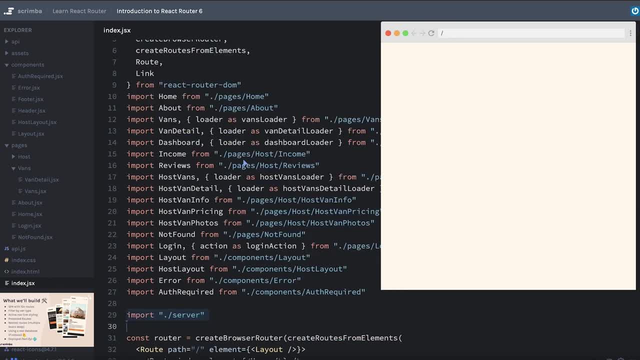 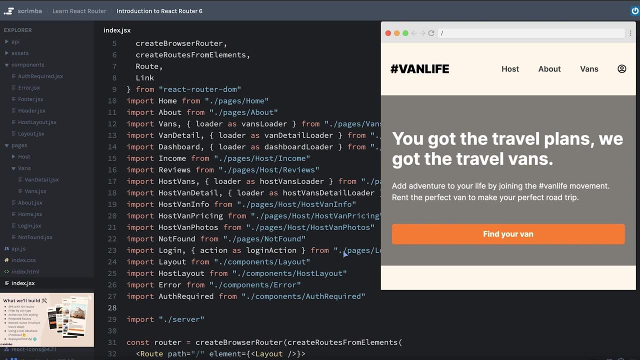 get a feel for it. You, of course, are also welcome to look around the code. Don't let it be intimidating, because jumping into a new code base is always a bit intimidating. Instead, be excited about learning everything you see here. Now, this should be relatively self explanatory, But the 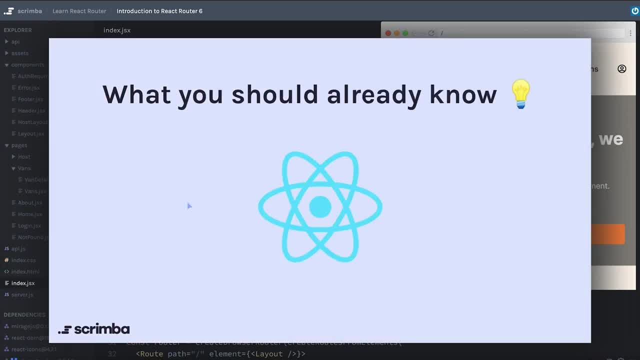 things you should know before starting this course are, of course, react. I would expect, before you start this course, that you have a pretty solid foundation in react. If you are feeling rusty or you have not yet had a chance to really learn react, this course will not be a good starting. 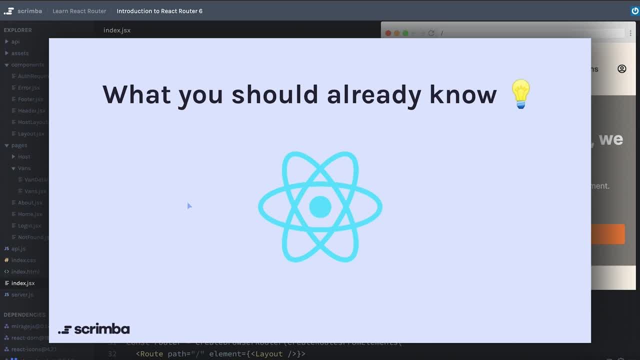 point. for that it will assume that you already have the basics in your tool belt. So if you do need to spend some time learning, react or just brushing up on certain topics, I have a free course that's over 12 hours long, It's got tons of practice, tons of projects and is completely free. 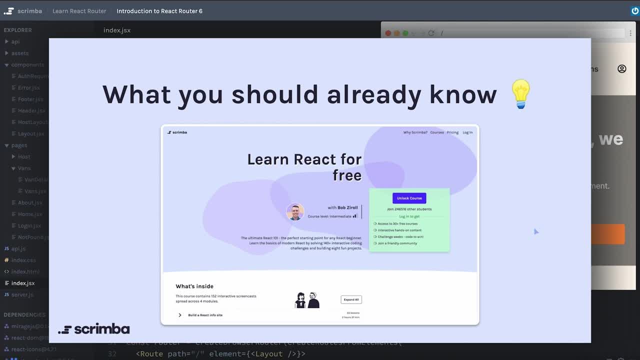 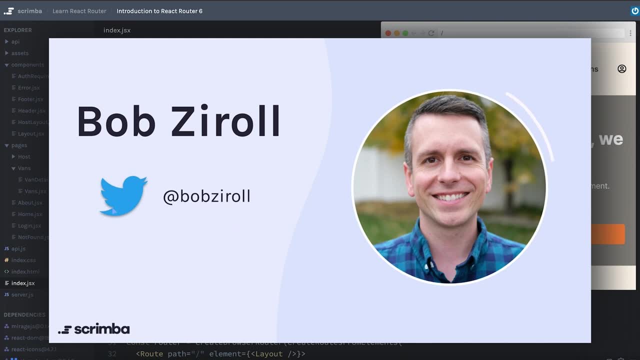 You can click the screenshot here, which will take you to that course on scrimba, If you'd like. My name is Bob's role. I'm going to be the course instructor for this entire course. the most active place you can find me online these days is on Twitter. you can click this little Twitter icon. 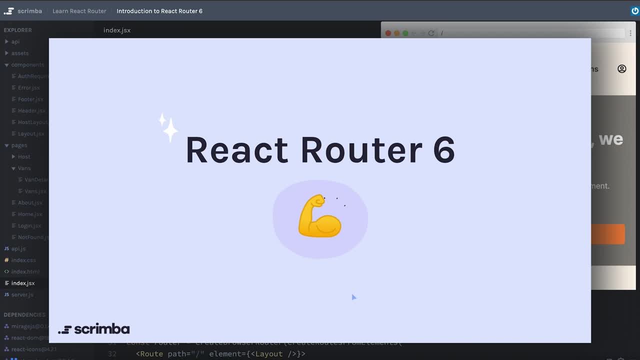 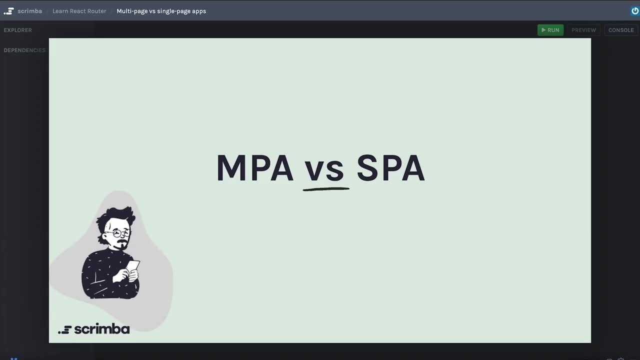 to go to my profile page on Twitter And, without any further delay, let's jump in and start learning about react router version six. That react router enables us to do something called client side routing. However, that might not make a whole lot of sense on its face if you're not familiar with the history of multi. 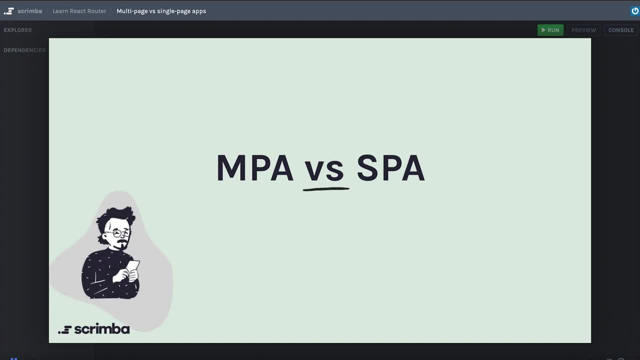 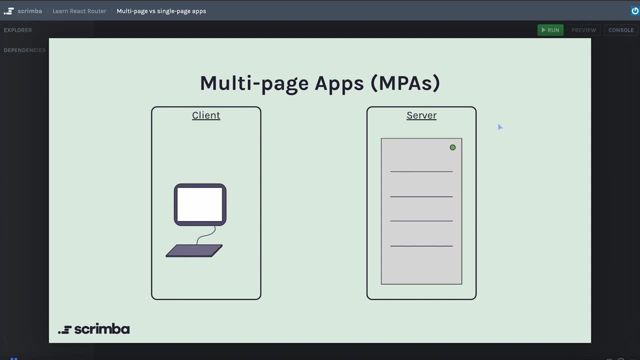 page applications versus single page applications, So let's spend a second talking about the difference between these two. In a more traditional website, you have multi page applications, or MPAs. On the left side of this diagram we have a client. it's showing a computer, but more accurately. 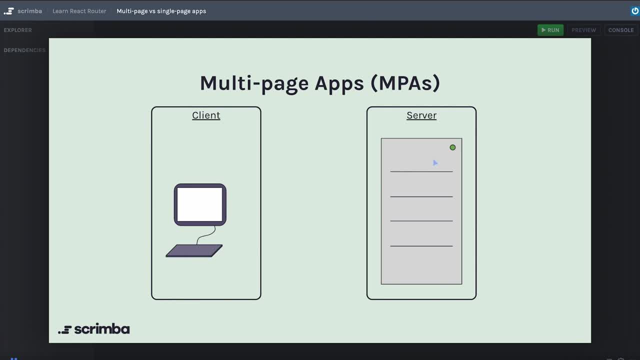 the client is really the browser in our case, And on the right side we have a server which really is just a computer that lives off site, usually somewhere else. So when you go to your browser and you navigate to a website, let's say my sitecom. 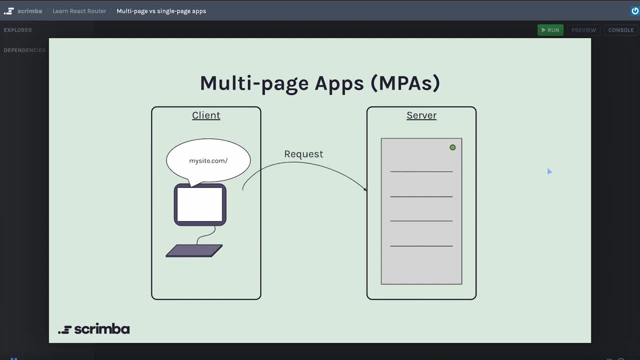 a simplified version of what happens is a request is made to the server that's associated with the domain of my sitecom And it's requesting the HTML page that is needed to display the web page. At that point the server will do some processing. it will grab the HTML page. 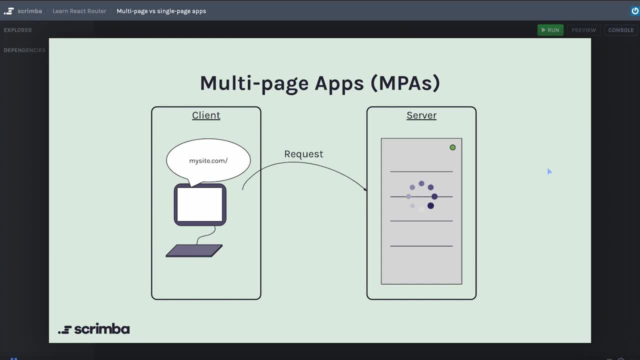 but it also might be evaluating some CSS or some JavaScript. It could potentially be reaching out to a database or making API calls to other servers, In the end with the ultimate goal of putting together a completed homepage to send back to the browser in the form of an HTML file. 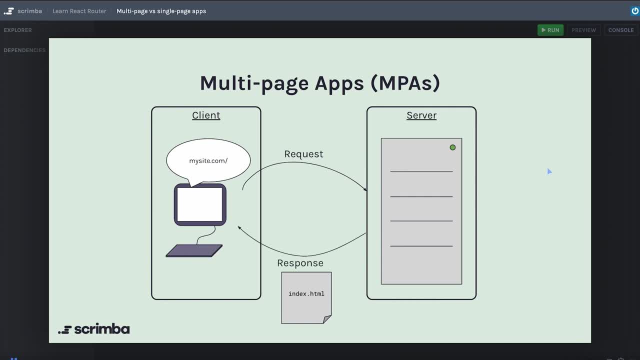 That HTML file is then sent back as a response from the server to your browser, and your browser then loads that page for you to view. So then, once you're looking at that homepage, you might go ahead and click on the About page. The URL for this would be: my sitecom, slash about. 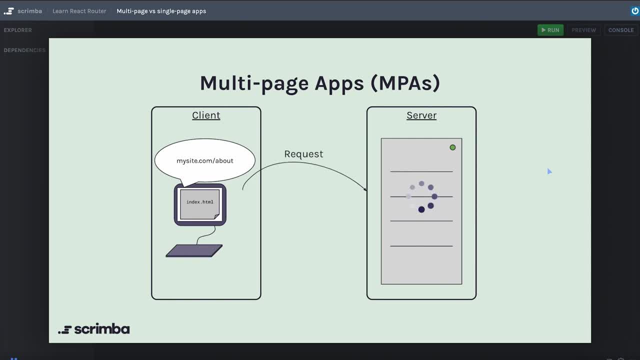 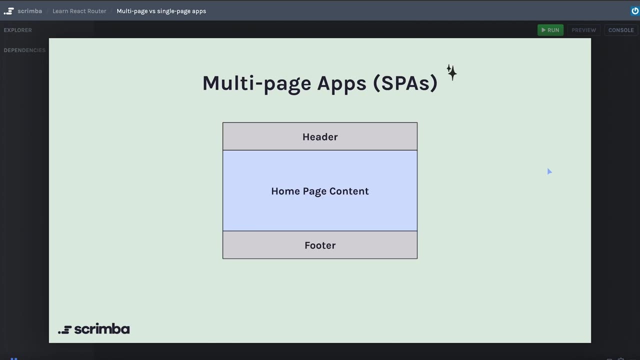 which would then perform another request to the server. The server again would go through similar processes where it would be searching for the About page to then deliver up to the browser. Your browser would then replace the old homepage with the new About page. From the browser's point of view, it might look something more or less like this: 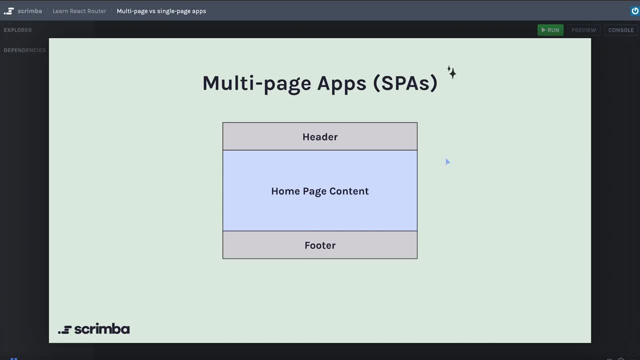 not including this actual animation. When you're on the homepage, you can see all of the homepage content, including a header, let's say, and a footer, And when you click on the About page, the entirety of that page is discarded. 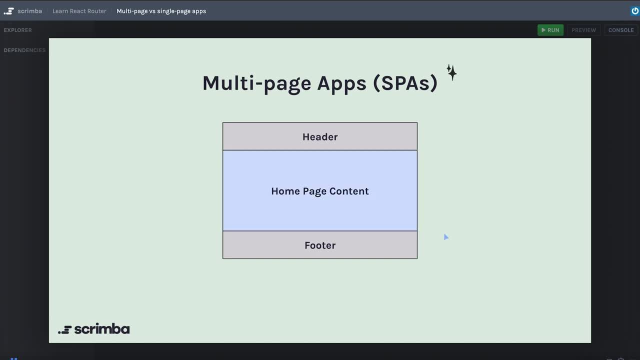 and replaced with the entirety of the new page. Of course, it's usually not a sliding motion like this. Instead, it will appear more like a flicker, And that telltale flicker is a good way to know that you are currently looking at a multi-page application. 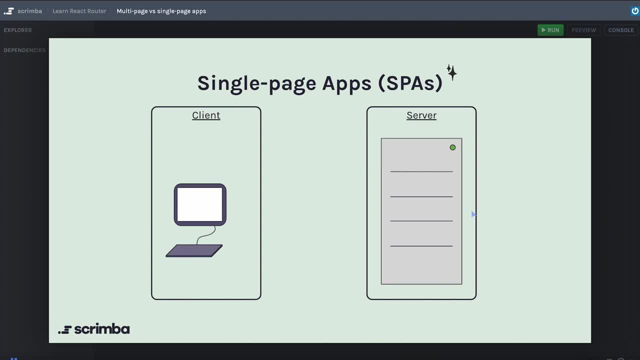 So how does a single-page application differ? Well, don't be confused by the name single-page application. It doesn't actually mean you can only have one page on your website, but instead it means that your browser is only loading a single web document one time. 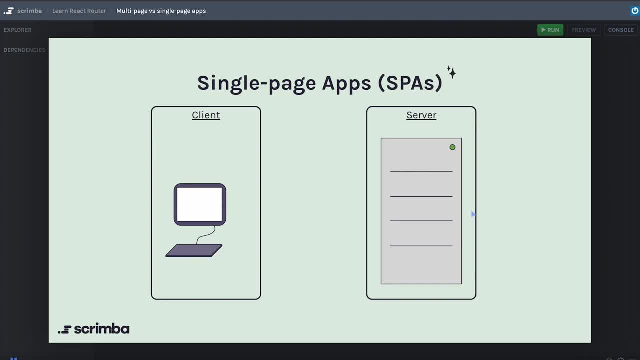 and then your app will make incremental updates to that existing document through different methods like internal React, state changes or fetch requests to an API. It all starts in a very similar fashion. In your browser you navigate to mysitecom That makes a request to the server. 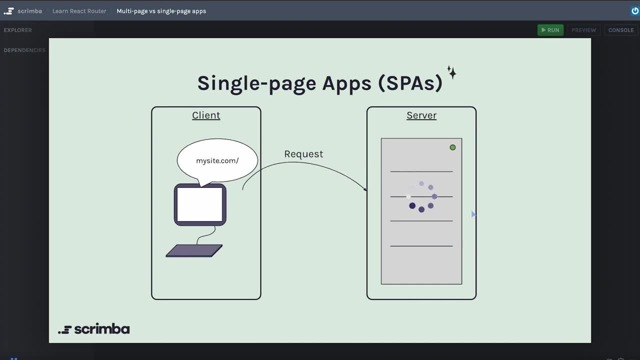 The server will then process a few things, but this time, instead of its job being to process and build an HTML file, it's going to send back an entire React application. So that application is sent back to the browser. It's loaded into the browser. 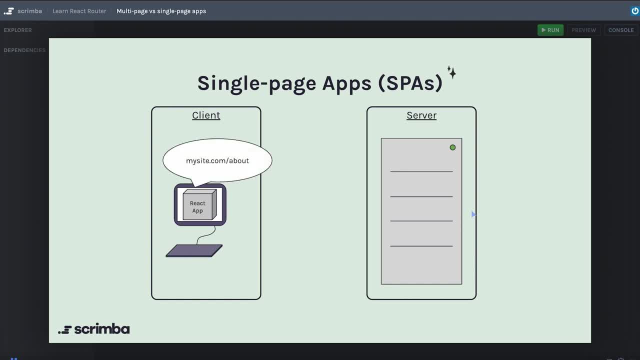 and when new requests, like going to the About page, are made. oftentimes portions of that new page are able to load directly inside of the React app without any new requests being made out to the server. That said, the About page might still need some extra information or data. 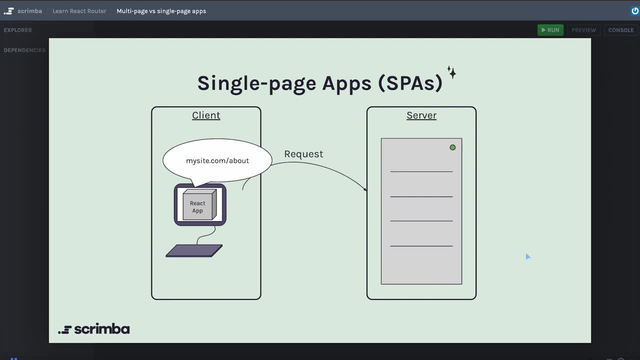 from a server or an API, and so a request could still be made out to a server, at which point it would do its job, and this time, instead of sending a new page back, because, remember, that view already exists inside of the React app itself. 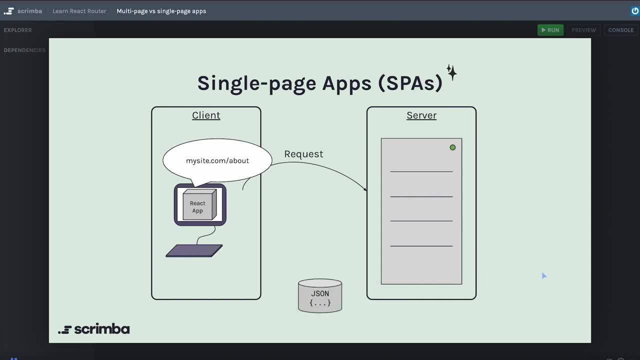 it's likely only going to be handling sending back something like JSON data. That JSON data gets sent back to your React app, which then loads into the React app, gets consumed by it and changes whatever view you're looking at to include the new JSON data that you just loaded from the server. 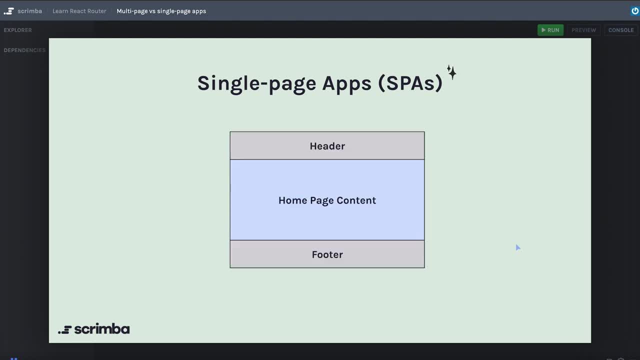 All that said on the client side, the real difference that you'll see is there won't be the same flicker of the entire page when you're going from one page to the next, Because, remember, we're not reloading the entire document. 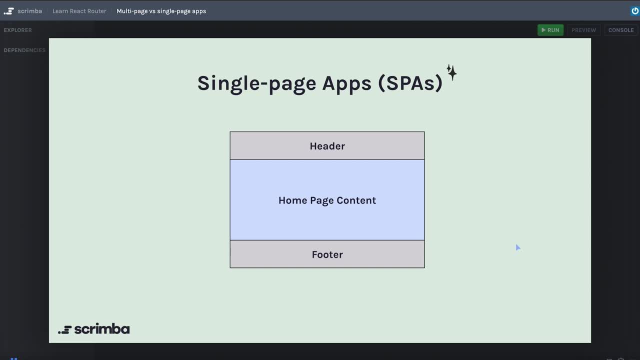 It's just one data, One document, One page, But the content on that page might change. In essence, what that does is it might swap out the home page content for the About page content, Because the React app was loaded on the initial render of your website. 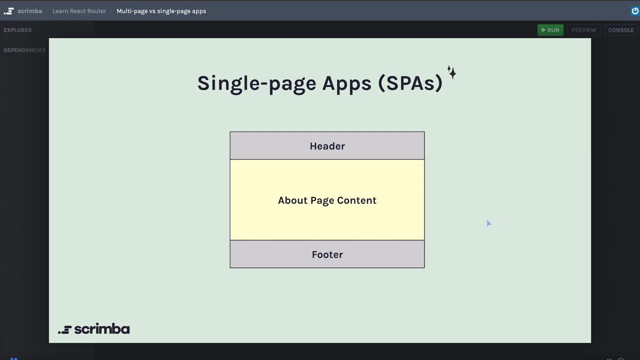 it already knew what content the About page was going to contain, and it may or may not have had to reach out to a server to get some additional data. In fact, in our van life app we're going to see this, where we can transition to the About page without any delay. 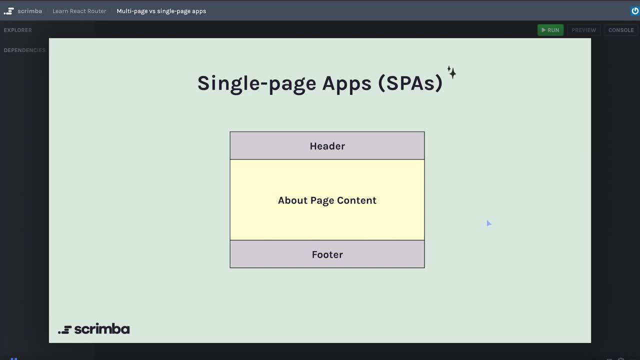 without any of that flicker. that happens with the multi-page application, And the About page doesn't request any additional resources or JSON data from the server. Instead, it's already loaded on the initial render of our site. However, when we go to the Vans list page, 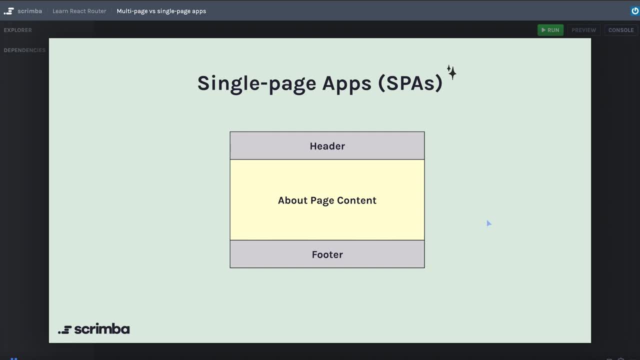 the beginnings of that page will load in sort of a skeleton UI, you could say, while in the background a request is being made to the server to ask for the specific data about the vans that we need to list. Then, once that data comes in, 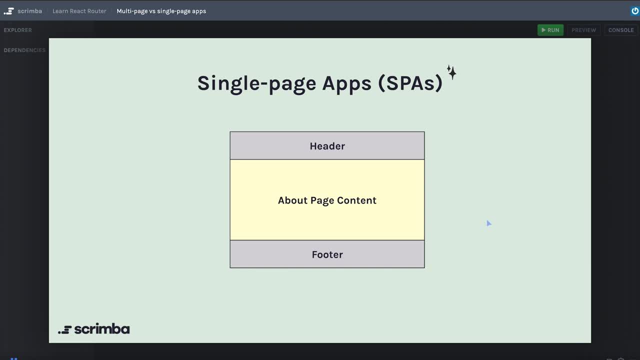 it will update the page to display the vans. This will make a bunch more sense once we actually start developing it. So that's a very high level overview of what will be happening, as we're building a single page application using React Router. Now it's time for us to actually dive in and start learning the code. 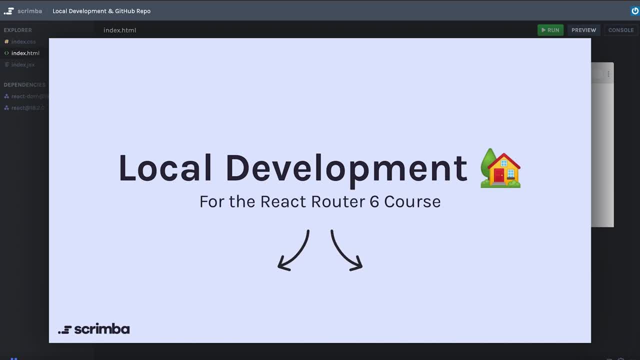 Hey, free code campers, This is a special message just for those of you that are taking this course on YouTube. When you're following this course on YouTube, you likely will want to complete the challenges and write the code alongside me in your own local browser. 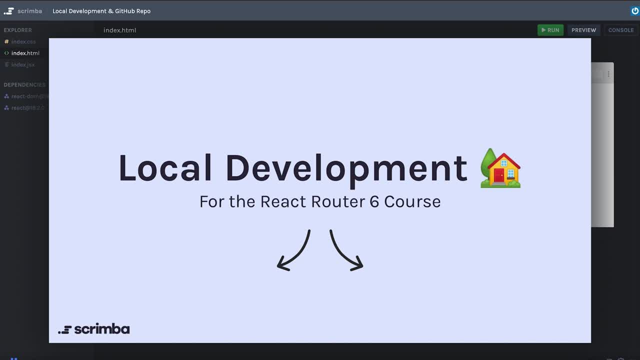 Local environment, And so I wanted to make a quick note about developing through this course locally. At this point in your learning journey, I assume you're already familiar with some kind of editor like VS code and at least know your way around the program in order to create new files. 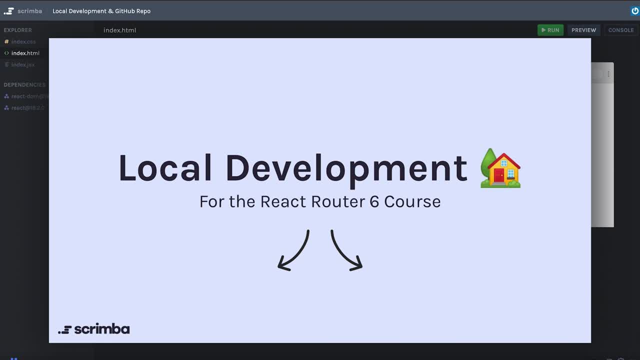 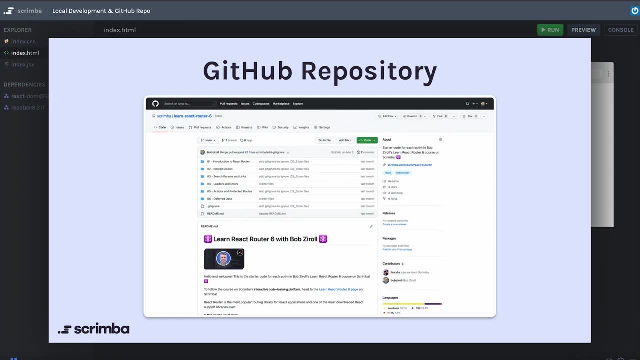 and open a new project, and so forth. Well, the code for every lesson in this course exists inside of a GitHub repository that I really want to encourage you to go follow. Using this GitHub repository will give you the starting code for every single lesson in this course. 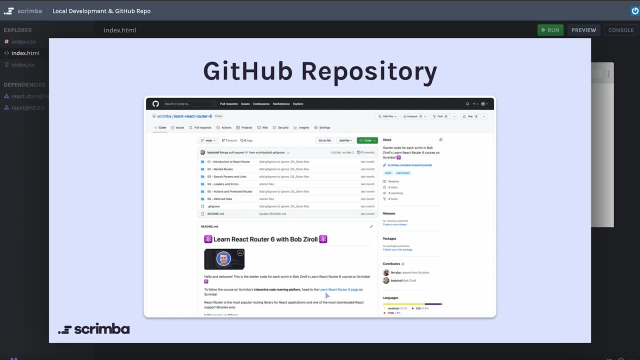 Not only that, but it will have a really important readme down here that will give you specific instructions for how to set this up on your local machine and any gotchas that you might run into while you're developing locally, as well as any updates to this course. 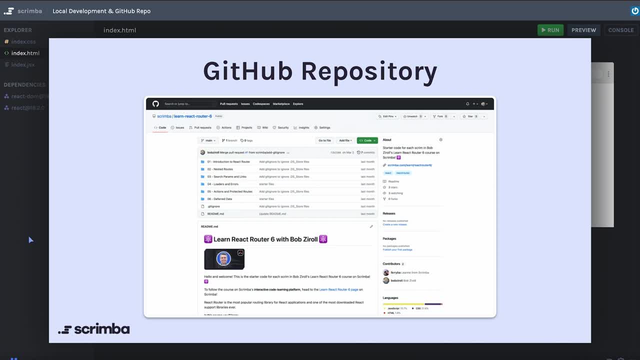 that you might need to be aware of. Inside of scrimba, I have the power to record new lessons and insert them anywhere inside the course that I want, But with the course being here on YouTube I don't have that same capability. So this GitHub repository and the readme therein is going to be a little bit different. 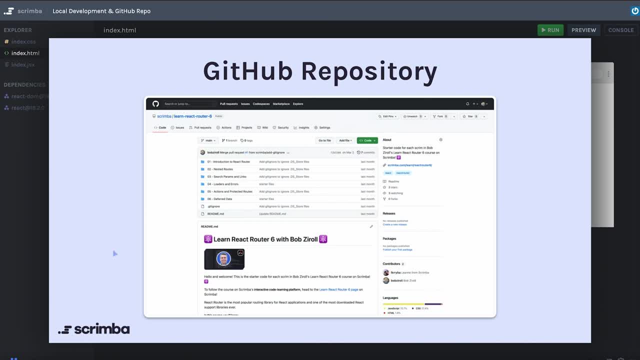 It's going to be a really important tool for you as you work through this course, to make sure that you're getting the most up to date information. So, even if you don't plan to use the code from this GitHub repo and you just are going- 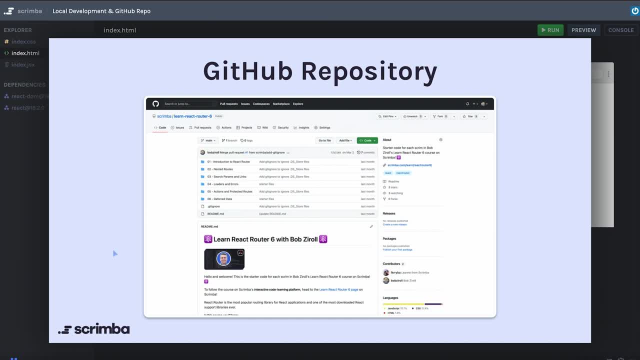 to start the project up completely from scratch on your own. still, make sure that you come to this GitHub repository, star it, watch it, bookmark it. whatever you need to do, and make sure to check it regularly in case there are any updates. that will be important. 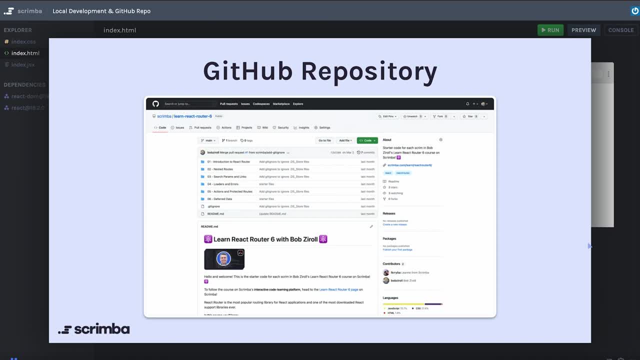 to you as you learn React Router in this course. The link to this GitHub repository should be readily available in the description down below If, for whatever reason, you get stuck developing locally. while it is a great experience to debug those local development issues, I don't want that to become a demotivator for you and 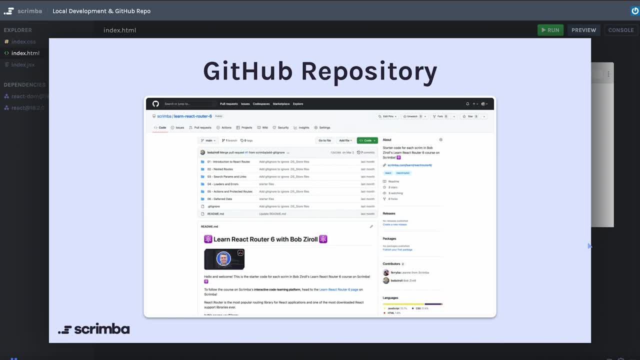 stop you from your progress in the course. So if at any point you do feel like you're getting stuck, you are of course always welcome to head over to the scrimba platform and just pick up where you left off in the React Router 6 course. 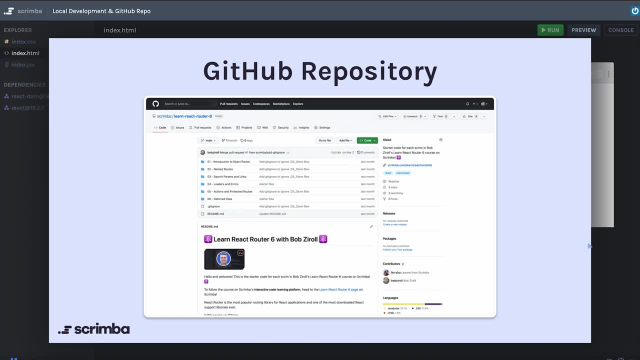 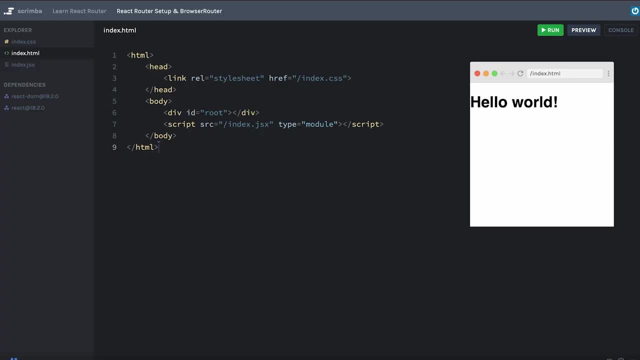 Okay, that's all I have to say about this for now. Let's keep moving forward in the course. Okay, we're going to start this app from the almost bare bones. We have a very basic React project here. You can see that all we really have is a simple hello world. 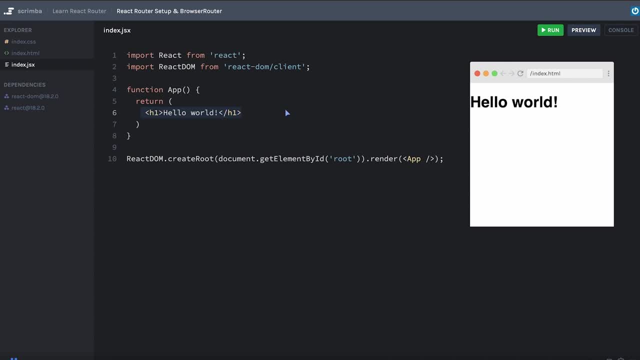 There's one thing I do want to point out, and that's something that I haven't really talked much about before, And you might have noticed it real quick over here in the indexhtml, You'll see that our script tag is pointing to indexjsx. 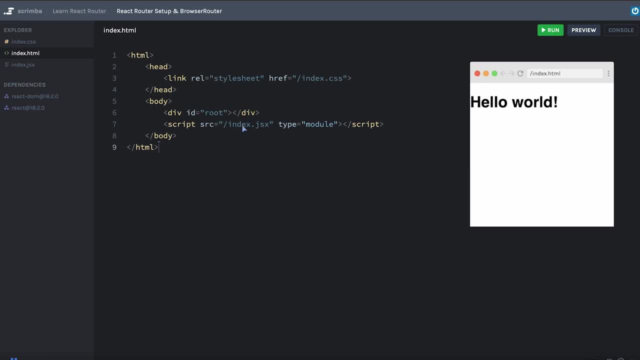 When you're working in a React project, you can specify any files that have React components in them, specifically ones that are using the JSX syntax, as having a jsx extension. Now, under the hood in scrimba, we've made it so that it's using veet. 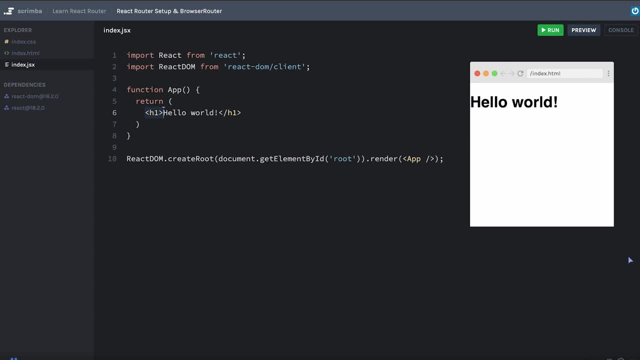 in order to compile the language. if you were to download this onto your local machine and run it, Veet expects any components you make in the JSX syntax are using the jsx file extension. Now, here on scrimba it's going to work just fine if you decide to make these as js files. 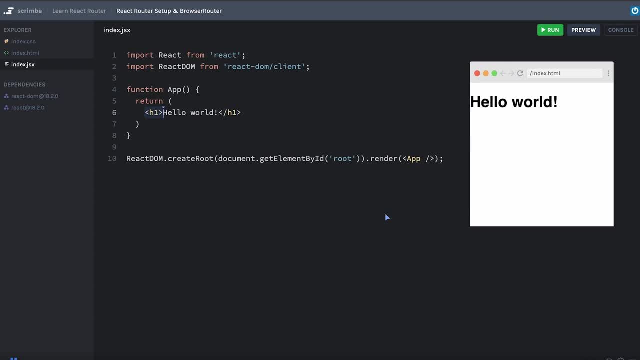 but I did want to introduce you to that in case you had never seen it before. Okay, so if you're a Ha génér, Throughout this section and this project we are going to be using JSX files when there's a React component involved. Okay, let's move on to React Router Setup. You can see I have React and React. 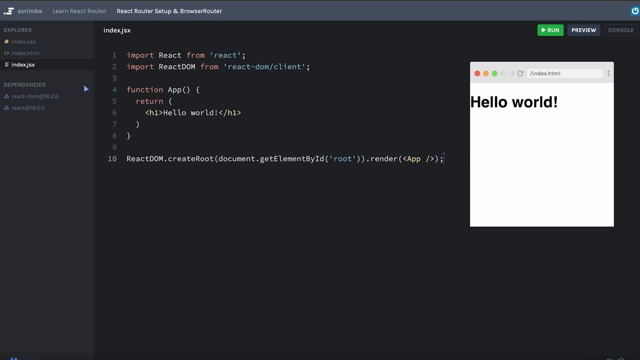 DOM included as dependencies. I need to include another module called React Router DOM and that's React-Router-DOM, So I'll add that here. You can see the current version is 6.4.3.. Now for a little extra information. React Router DOM 6.4 introduced a whole new set of tools that you can use in React. 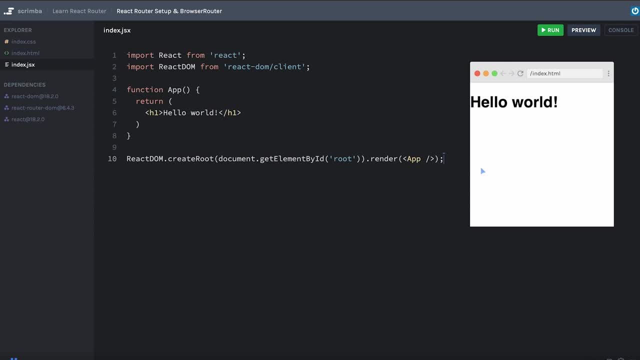 Router. I'm planning on touching on those new additions to 6.4 a bit later in the course. However, in this section, I'm only going to be focusing on the basics that come with version 6.. We will not be going into the data layer APIs that come with 6.4.. Okay, let's start out with the 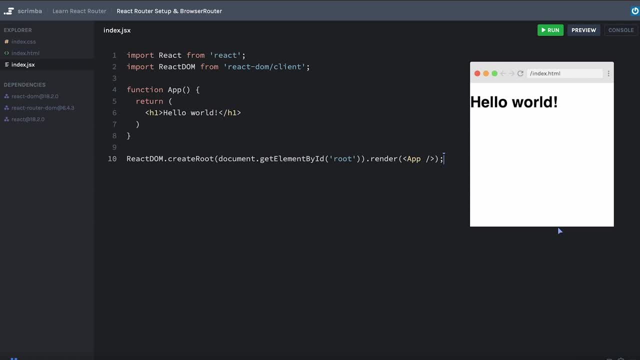 most basic thing, In order to set our project up as a single page application with routing using React Router. we need to set up a single page application with routing using React Router, We need to import a few things And, in this screencast, the only thing we're going to be. 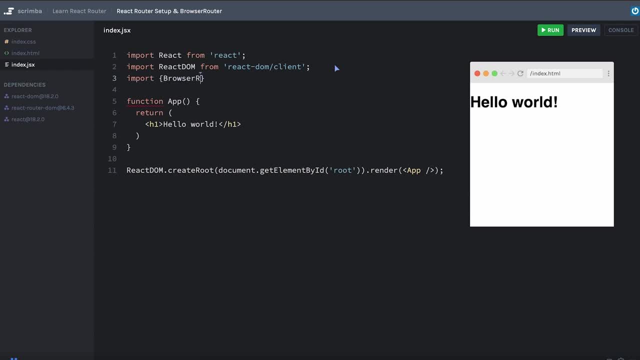 worried about is importing something called Browser Router, And that comes from React Router DOM. Now, we just learned about context recently in this course, So I think this will be interesting to you. What Browser Router is doing under the hood is it is a context provider, And so, in order. 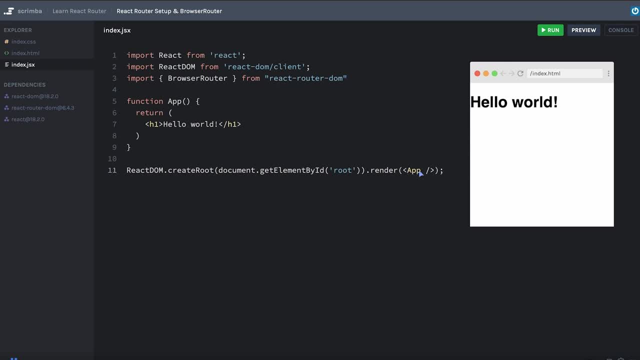 to give our app the power to include routing in its functionality, we need to wrap our entire app with this context provider. And so, in order to give our app the power to include routing in its functionality, we need to wrap our entire app with this context provider. And so, in order to give our 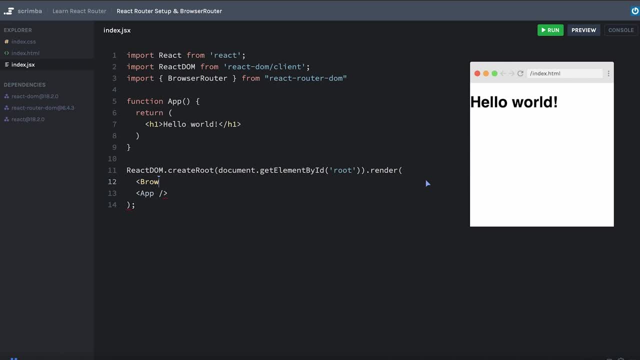 app the power to include routing in its functionality. we need to wrap our entire app with this Browser Router. So I'm going to put Browser Router around the app like this. We'll hit save and nothing much should have changed. we should still get our Hello World text right there, But by 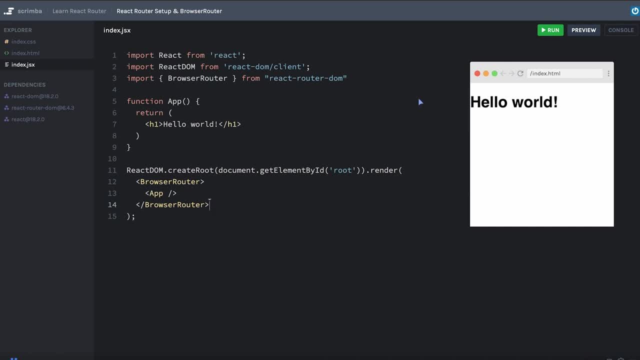 simply adding Browser Router. we now have a whole suite of tools that come with React Router DOM that we can use to control our app. Now, just in case you see this in the wild, sometimes people will rename Browser Router since it's a bit of a mouthful, And so they'll import Browser Router. 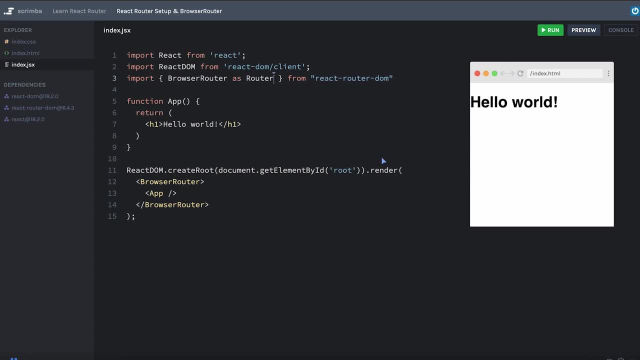 but then rename it to something else. And so we're going to import Browser Router but then rename it to something else. And so we're going to import Browser Router but then rename it to something else like router. Now we're also going to be seeing that there is a routes component and a route. 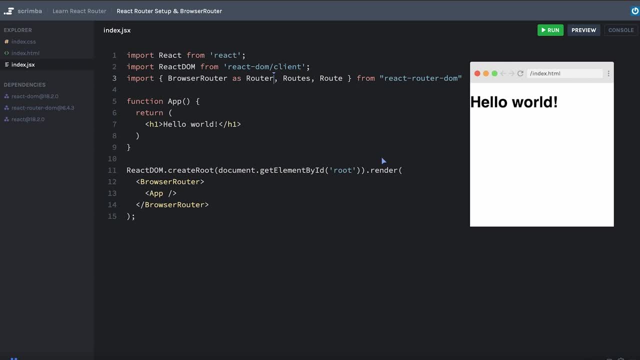 component, So I'm not going to rename it as router, because those are all very similar, So we'll just call it Browser Router for now. Awesome, This is a great start. Like I mentioned, there's a few other components we're going to be importing, So that's what we'll be working on next. 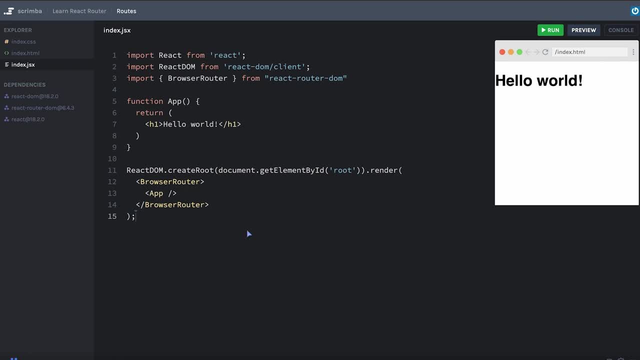 As we mentioned, Browser Router is a context provider and it provides context to all of its children components, very similar to what we were doing in our reusability section. So Browser Router is the provider we need to set up a way to define the routes that we want in our application. 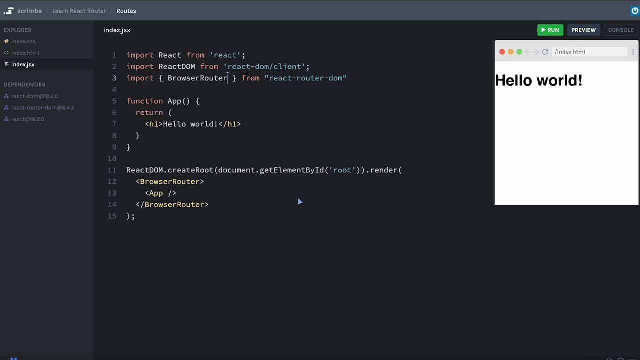 we're going to start with a really simple home route and an about route, And there's two components I need to pull in in order to start setting that up. The first one is one called routes. The routes component goes as the first child inside the browser router, So I'll set up. 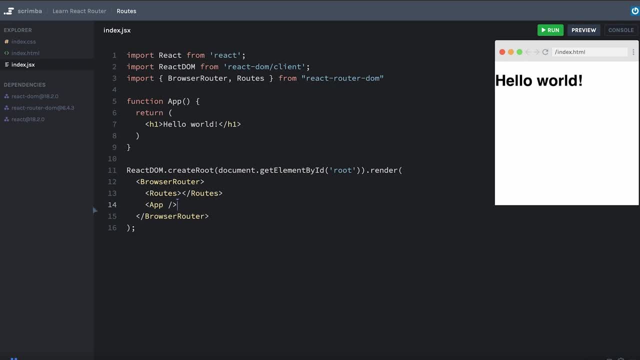 routes here And I think, to avoid that, I'm going to go ahead and set up a new component called routes And I think, to avoid that, I'm going to set up a new component called routes. And I think, to avoid confusion, I'm actually going to stop rendering our app component, So we just have the browser. 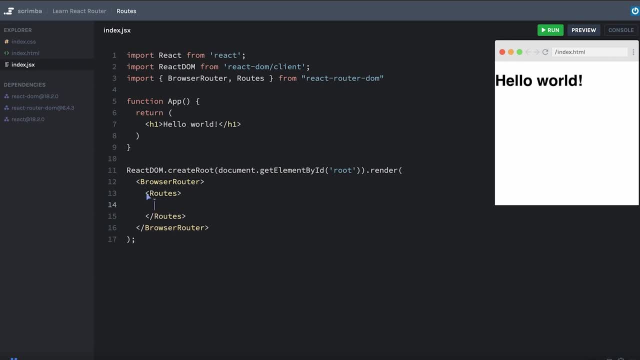 router and this empty routes element. Notice here it has a separate closing tag And that's because inside of routes will need to go a series of new components. that is just called route. Now, just in case you don't know, a route is just part of your URL that specifies where on your website. 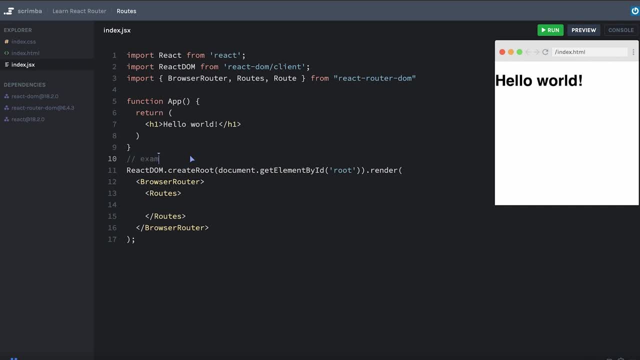 you are. So let's say you have a website like examplecom. Examplecom would be your homepage and oftentimes it has a trailing slash, So that route might just be called the slash route. But if you wanted to create an about page on examplecom, you would maybe have a route called slash about. 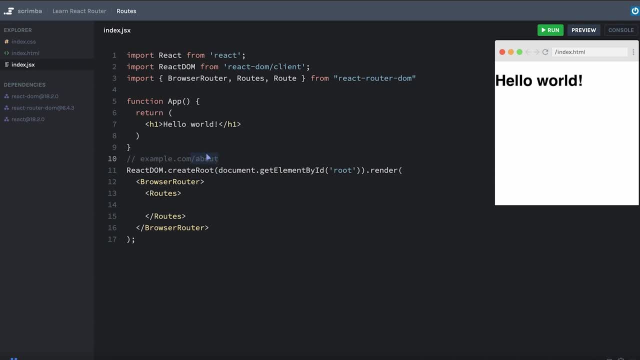 And then this part of your URL is the route for your site. Maybe you have a contact page- that would be slash contact. Or maybe you have a blog page- slash blog. Now, routes can be nested And we're going to cover nested routes later, But if you had a blog, you might want to specify that you. 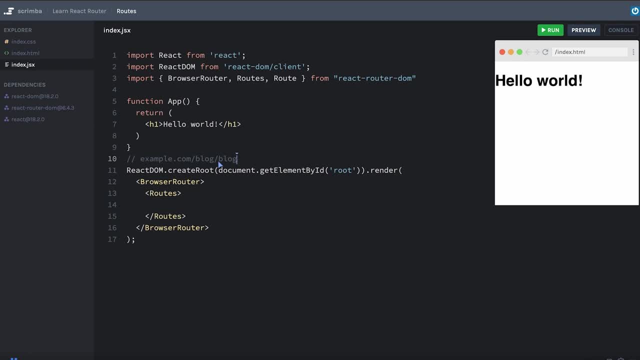 have another route as part of your site, And then you can also have a contact page as part of your URL that leads you to blog article one. you hopefully have more interesting titles than that. Oftentimes, blogs will use the title of the blog as this part of the URL, Although you might see. 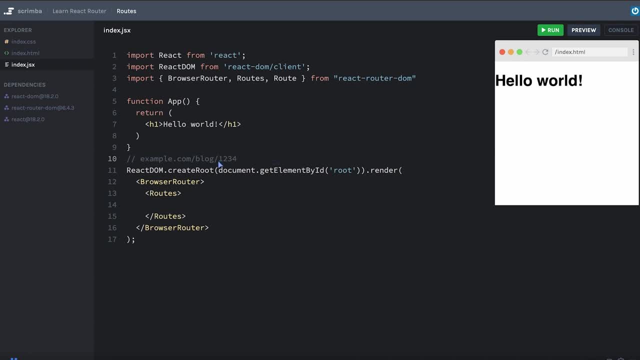 sometimes it's just an ID number, where it specifies for the database under the hood which blog ID number it should be looking for Currently. over here in the mini browser you can see that it says slash index dot HTML, And when we're just serving up a single HTML file, that might be true. 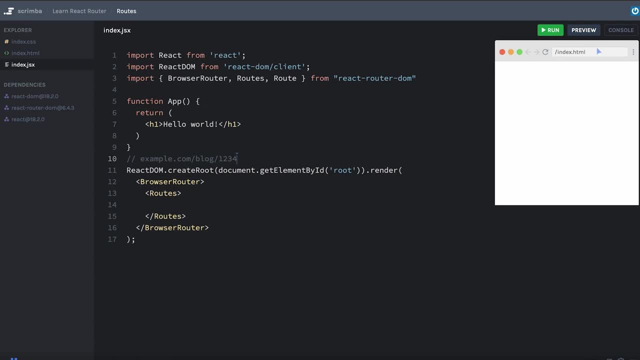 But once we set up our routes, we're going to need to create a new route, So we're going to just see the route portion of our mini browser. it's not going to say something like examplecom is just going to say slash, or, in our case, slash about. it'll also say in the app we're building, it'll be. 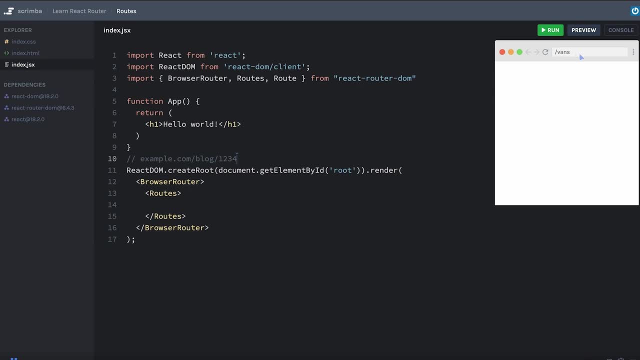 slash vans, it'll be a vans route And then we're also going to have vans slash and then some ID number for the van. Okay, we're getting a little ahead of ourselves. we don't have any routes to find, So now we have a place to put our routes. we need to start using this route component to 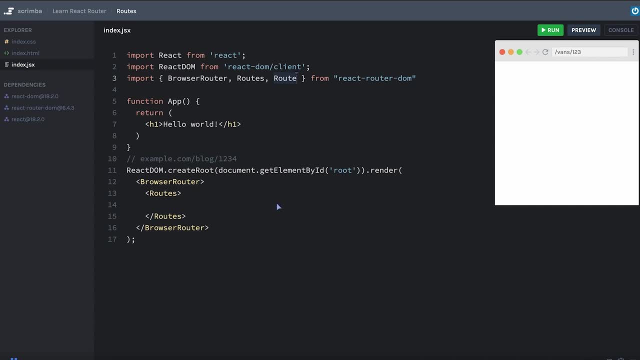 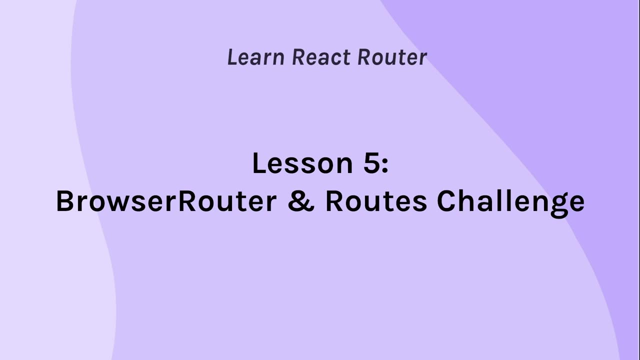 actually define our routes, And actually we've covered a lot of routes in this video, but we're going to have a quick challenge before we move on, Before we get too far. I want to make sure that you are practicing some of this, So you're basically starting from scratch. I've actually 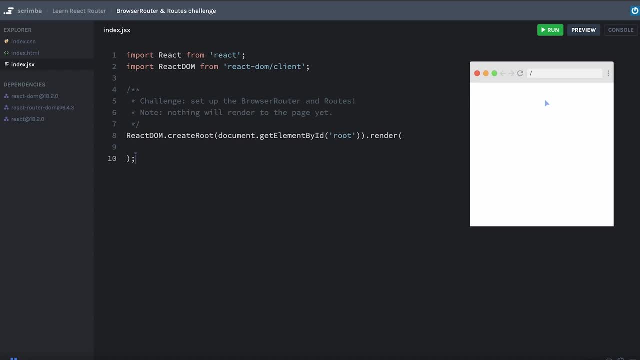 removed the app component because in this case we're not actually going to render anything to the page yet And I've already included the React router DOM dependency over here. So all you need to do is to render our browser router with a routes component inside of it. So pause here and 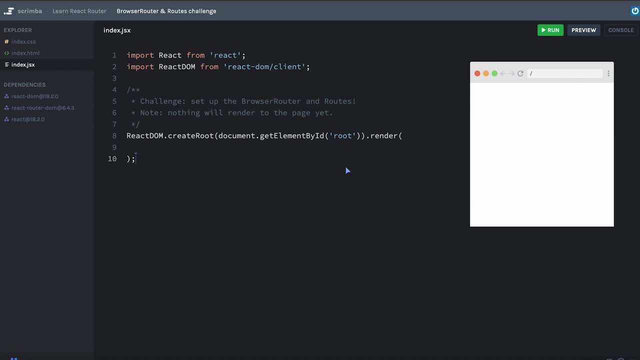 enjoy this challenge. Okay, first things first. let's make sure we import the browser router and the routes components from React router DOM. Again, the browser router is a context provider, So we are going to wrap everything that we have below in the browser router And for now we're. 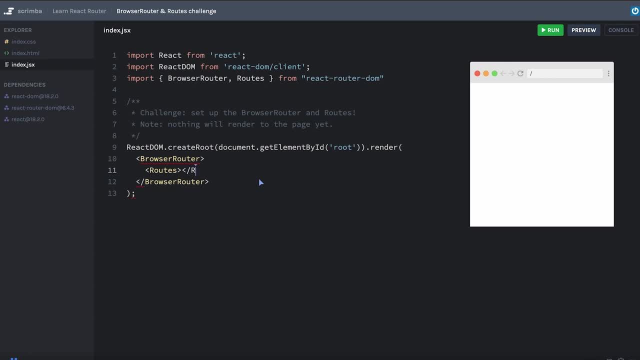 just going to put one nested child component in there And that's going to be the routes component. So we're going to put one nested child component in there And that's going to be the routes component. All of the rest of our work with React router is going to happen inside of this. 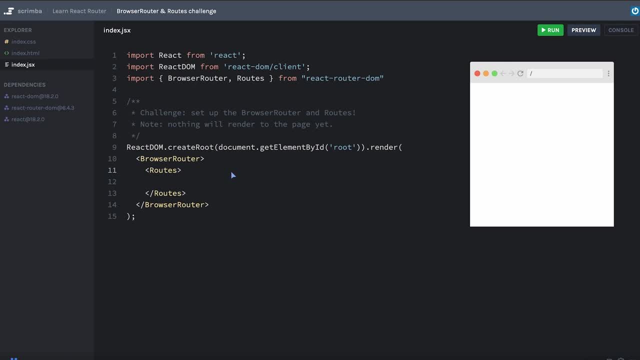 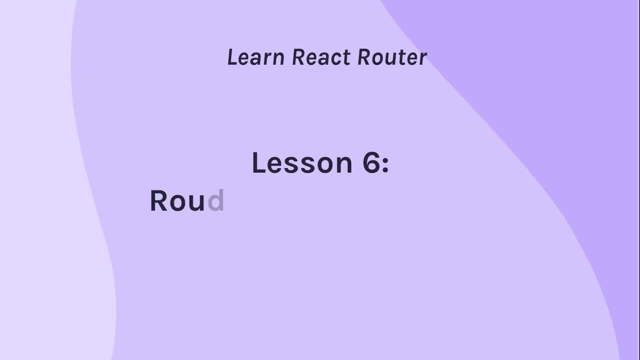 routes component. Okay, hopefully everything has made sense so far. we haven't gotten too deep yet, So when you're comfortable with what we've done here, we'll move on next to creating our route definitions. The next component we'll talk about is the route component, which we also need to. 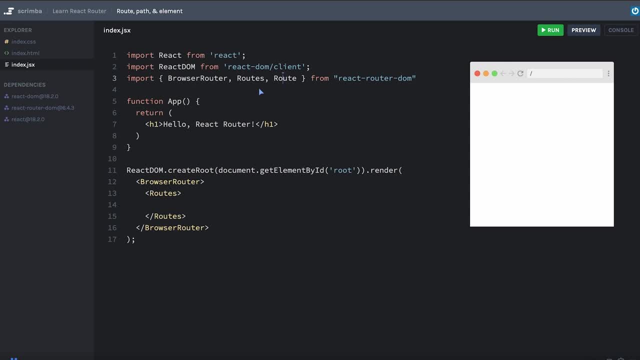 import from React router DOM, And this is really where the meat of what you'll be working on will happen. It's within these route components. The most important thing is that we're going to be using a route component And that's going to take a few different props. The most basic way to use a 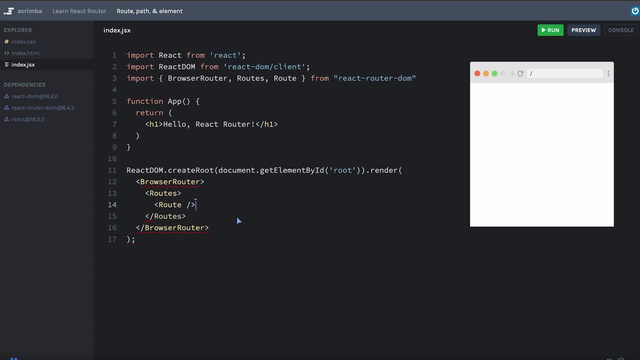 route component is to render it as a self closing element here, And the route component can take a few different props, the most common of which are the two that we're going to learn now. And that is path, which is where we specify what the path to this route should be. Remember, I mentioned that. 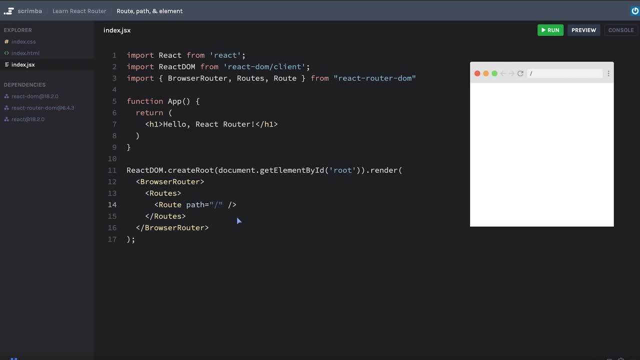 the home route is going to be called just slash. Well, that's what we're talking about here. we're talking about the route path. If I wanted to create an about page, I would make this: slash about, or a contact page, slash contact, And that's what we're going to be doing here. So we're going to be. 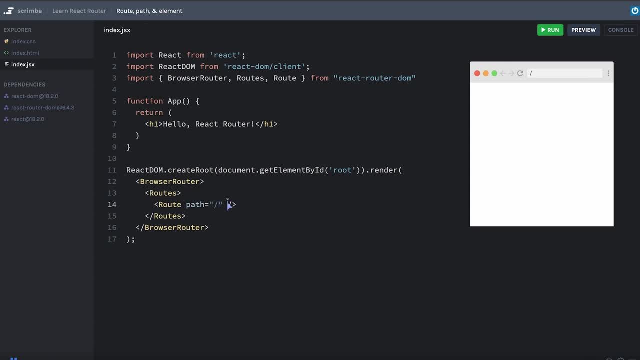 going to create a home page And secondly, we need to tell it which react element we want to render, if the path in the URL bar matches the path that is defined here on this route component. Now you'll see that I put a set of curly braces. that's because inside the curly braces I need to. 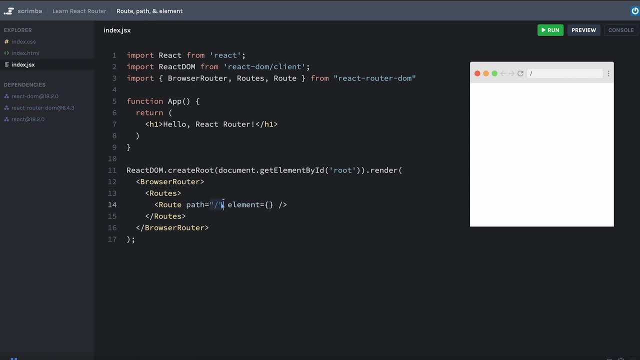 render some kind of JSX. In this case we'll say when the home page is loaded, or rather when the path is just a plain old slash. we want to render our app component that we have up here Now. I haven't quite done that yet, But we're going to do that in a second. So we're going to do that in. 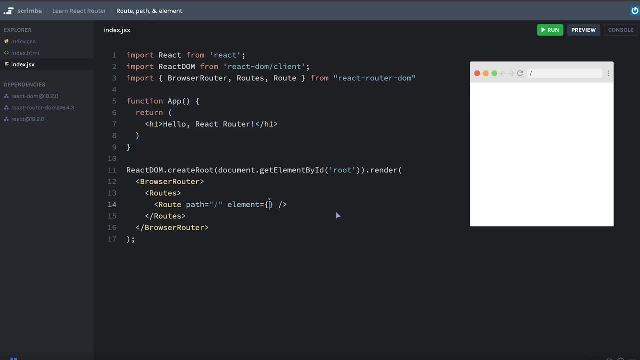 a second So you can see that the app component is rendered inside the state. Now I want you to see if you can figure out what we need to put here. I mentioned that we need to render our app component. see if you can read between the lines and figure out what it is that's going to happen. 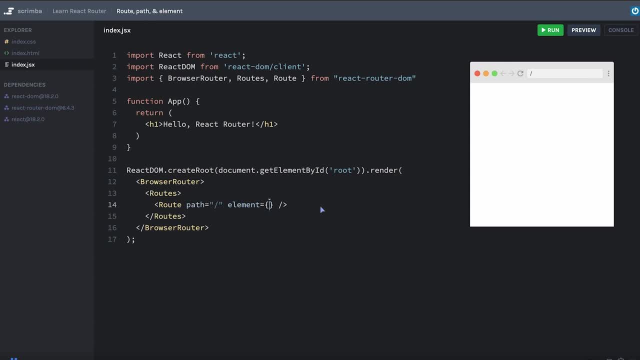 inside my curly braces here. This is the kind of thing that's fun, just to play around. If it doesn't work, that's completely fine. You're not breaking anything that can't be undone. So notice that our mini browser is currently at slash. see if you can make it so that when you fill in this element, 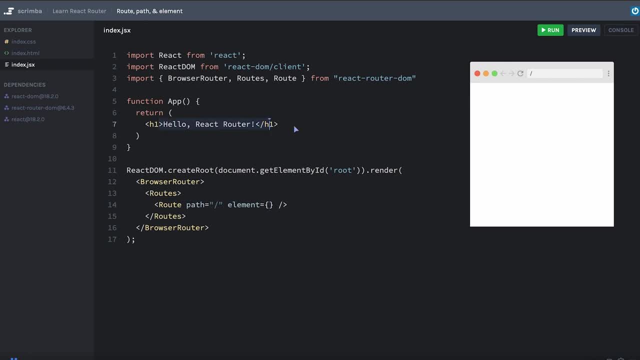 and then hit save, that your Hello React router h1 will show up here on the page. Pause now and see if you can get that to work. One thing you may have tried was to pass a component as a function like this, and actually in past versions of React Router you actually could do something very similar to that. 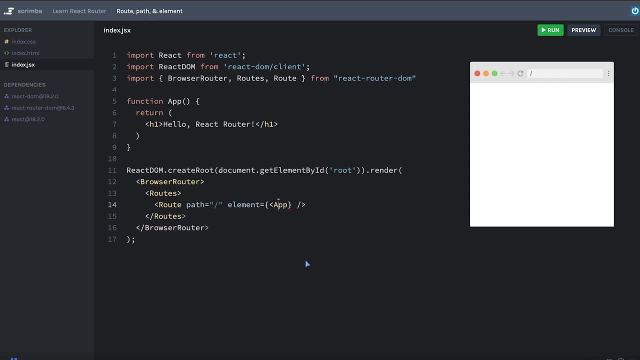 However, I did mention that we need to render the app, so I'm going to surround it with the angle brackets, like we see here. Okay, let's hit save, and there we go. We are at the slash route and we're rendering the app component when we're at the slash route. 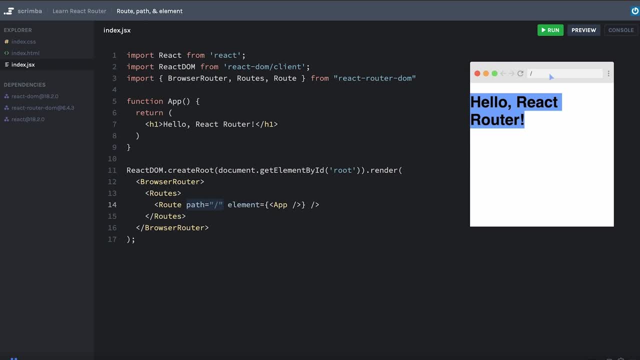 Out of curiosity, let's see what happens if I add slash about here and hit enter. Okay, it sends us to the slash about page, but there is no slash about path, and so nothing is showing up. This seems like a great place for another challenge. 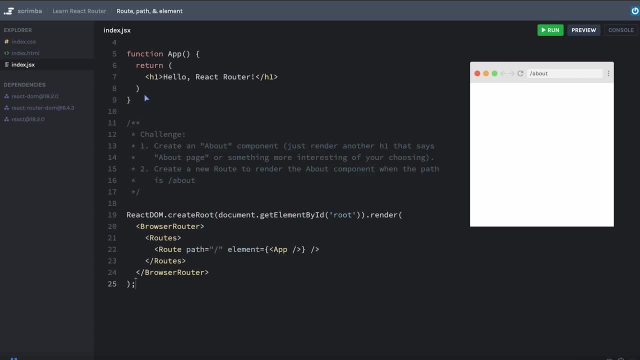 Okay, your task is to create an about component just right here underneath our app component, and it can render whatever you want. I mentioned an H1 that says about page, but then I realized that's probably pretty boring, so choose whatever you want to render there. 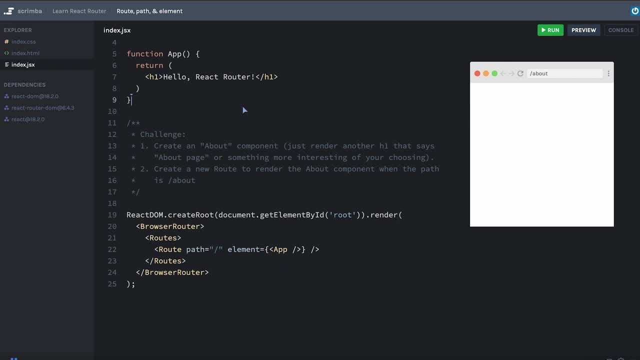 And then you need to create a new route so that it will render the about component when the path is slash about. I've already put it here at slash about, so you will know that this worked. when you hit save or refresh over here and your H1 or whatever it is you render in, your about component is rendered to the page. 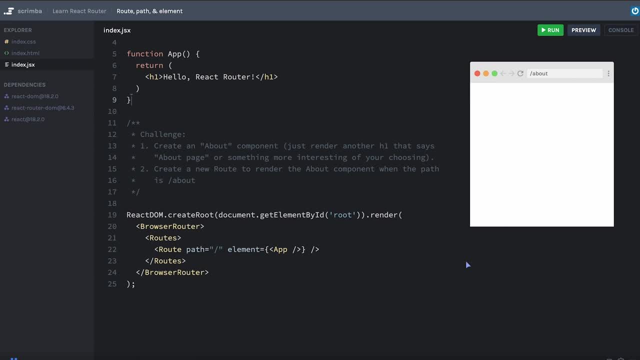 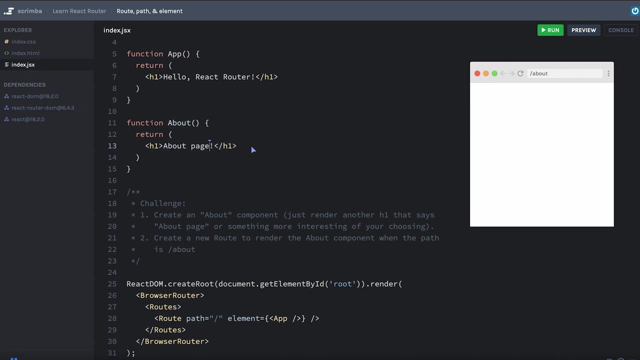 Pause now and work on this challenge. I'm feeling a little bit boring, so I'm not going to be super creative and I'm just going to copy my app component and we'll put this as an about component and we'll just say about page goes here. 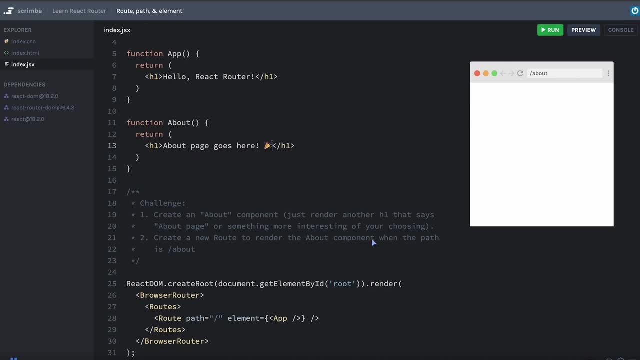 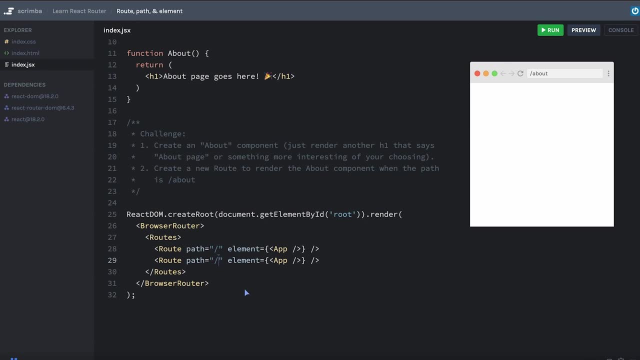 Okay, maybe we can make it a little more interesting. We'll put a little ta-da symbol there. Okay, now, down here where my route definitions live, I'm going to just copy my route. This path will be slash about and the element will be the about component getting rendered. 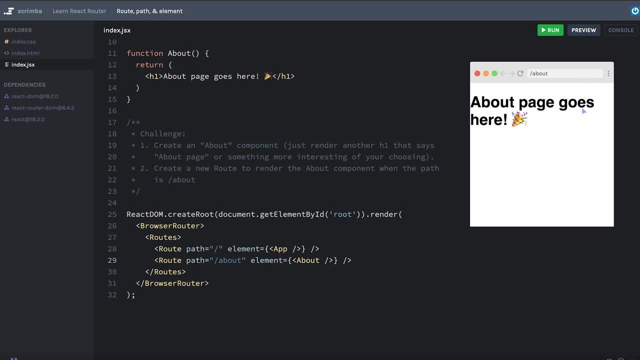 I'm already at slash about. Let's hit save And there we go. About page goes here, And if I get rid of slash about in the mini browser URL bar and hit enter, it sends us back to the homepage, or maybe more specifically, the slash route. 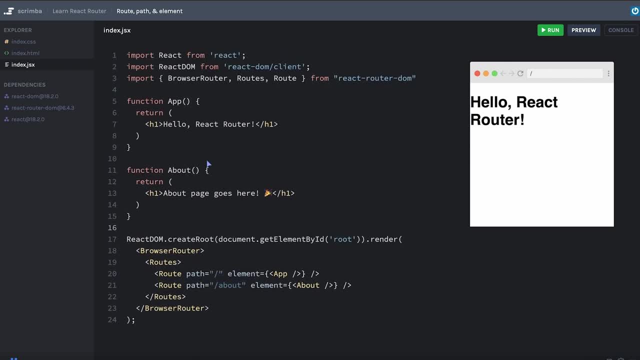 Let's clean this up so we can see a little bit more Awesome work. Now you might have noticed it's quite annoying to have to click up into the URL bar in the mini browser and type out slash about. Usually that's not how navigating around the website is going to work. 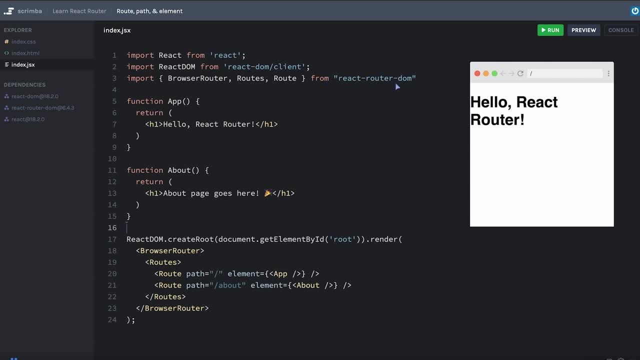 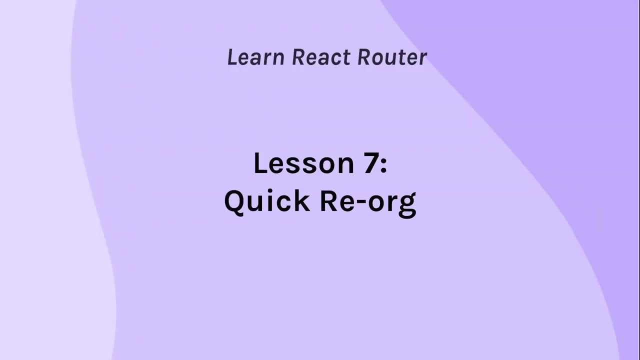 So in the next lesson we're going to briefly cover another component, React Router DOM, called link. that will help us navigate through our routes in a much easier way. Okay, before moving on, I actually want to do a very quick reorganization. 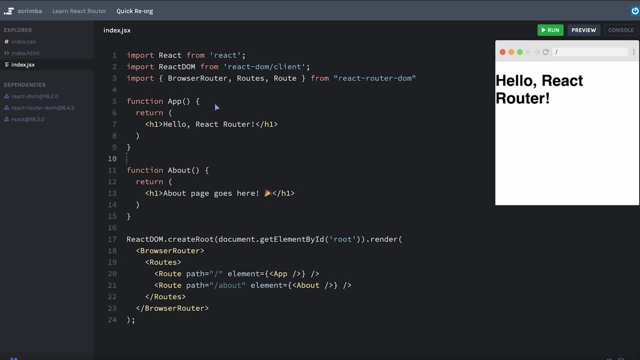 I didn't just want to do it behind the scenes, because I was worried that you might get a little jarred by me having changed the code so quickly. But right now it's, I guess, a little wonky. Maybe it's just me. 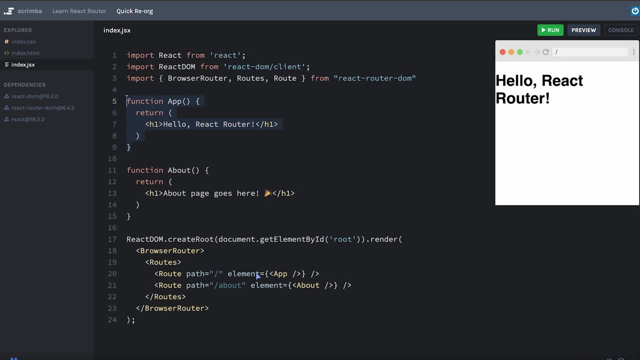 but I have this app function or app component that's being rendered as the homepage, but I have an about component that's being rendered as the about page. i feel like i'd rather keep the names a little bit different and then, instead of rendering the entire browser router inside of this render method, i think what i'm going to do is. 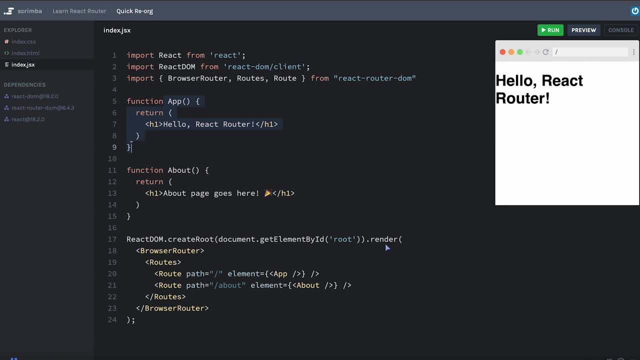 treat the app like the top level. so i'll just render app, and that means i'm going to take this entire browser router, put it inside of app and then i'll create a separate component, just called home, that represents the home page. then, instead of rendering the app as the home page, we'll render 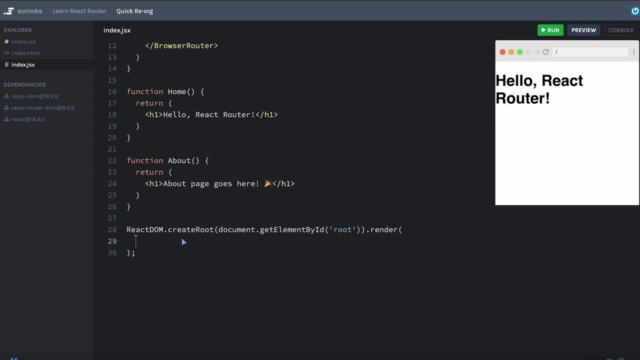 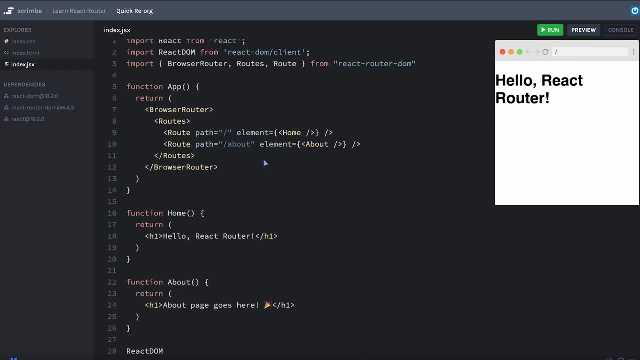 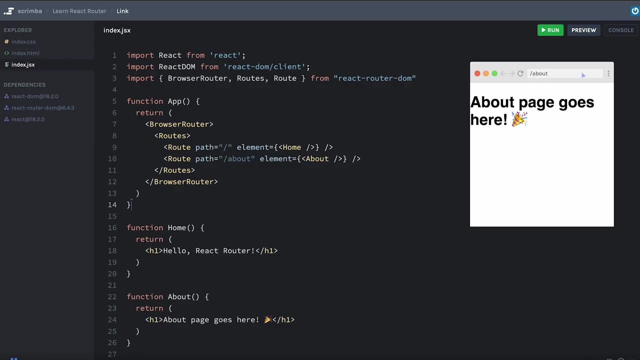 the home component that we just made, and down here we need to render our app and maybe let's move this onto its own line. okay, that feels a little better to me. let's move on. like i mentioned, it's a bit annoying to have to go up to our menu bar just to 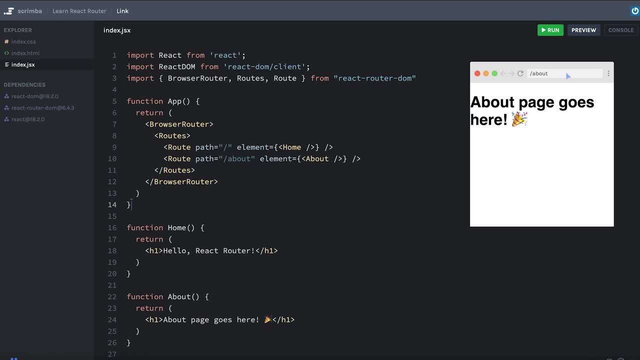 change which route we're in. so if i want to go back to the home page, i have to hit slash, and then if i want to go back to the about page, i have to type in slash about- we also can go back to the home page, and then if i want to go back to the about page, i have to type in slash about- we also can. 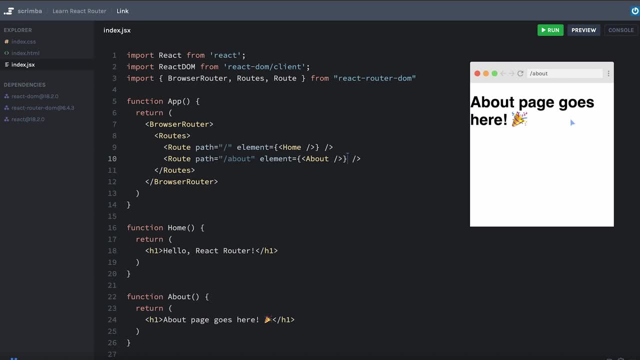 see that when i do that, the page is actually blinking, which means it's refreshing. it's doing a complete full page refresh. it's not that big of a deal when you only consider about the blink. but if you have any kind of state living in your app, that needs to be passed to the about page. 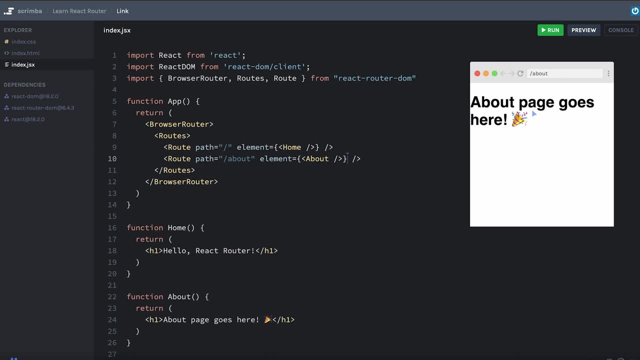 or well, really any state at all. doing that page refresh is going to completely wipe out any state that you were maintaining. if you really think about it, a react app is a little bit delicate when it comes to state, because if that page refresh happens, then all your state just completely. 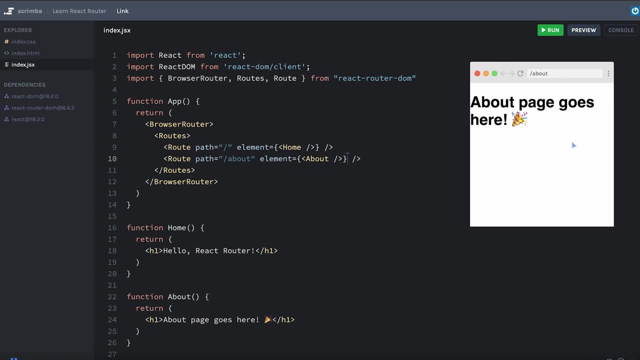 disappears, unless you're saving it in local storage or something like that. it will just completely reset. now the way to solve this problem in html is to have an anchor tag. the problem with an anchor tag is when you click it, it will do another page refresh. so we need some way to navigate between our different routes within the ecosystem of. 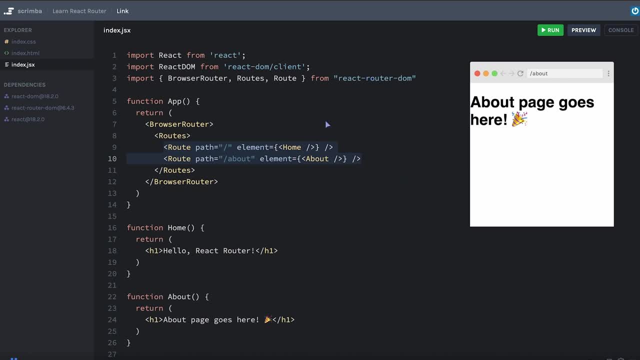 react router dom. unfortunately they give us a component to do that and it's called link. so i'm going to import the link component, capital l link. and if you actually look at your dev tools, when you render a link, it's just rendering an anchor tag but it's intercepting. 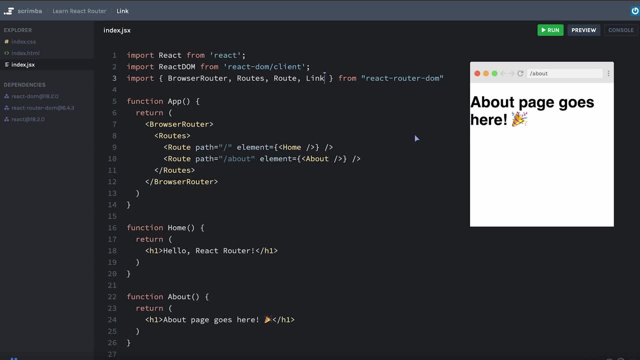 the path that the anchor is sending you to and making sure it doesn't do that page refresh so you can maintain your state. now, this isn't the real way that you would do this, but to avoid having to put links in both the home and about pages, i'm just going to stick a link element, right? 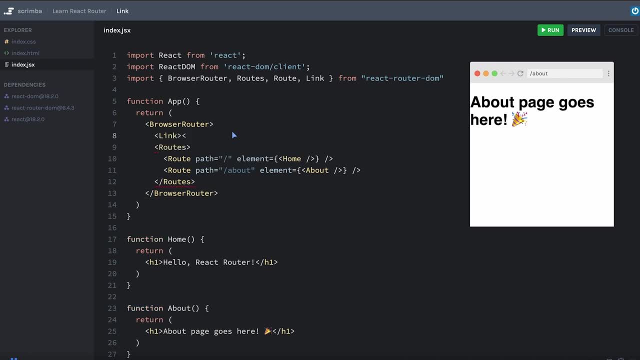 here, and the way that link works is very similar to an anchor tag, so it will have an opening and a closing portion to it. whatever you put inside is what will be the text element. so if you want to, that shows up on the page. But instead of an href property, a link takes a to property And this is. 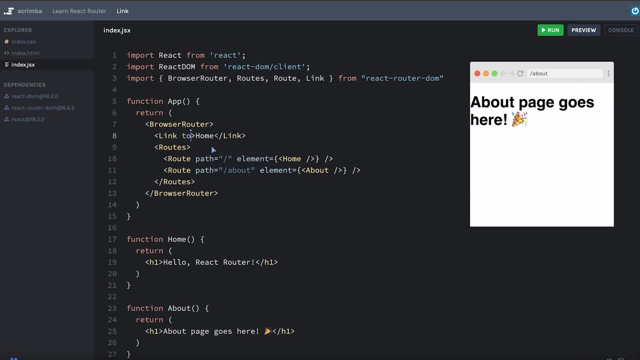 actually kind of nice because it reads like English: This is a link to the following route And so I'll say equals slash to go to home. We'll duplicate that and we'll say it goes to slash about to go to the about route. Again, you aren't going to usually stick your links just inside your 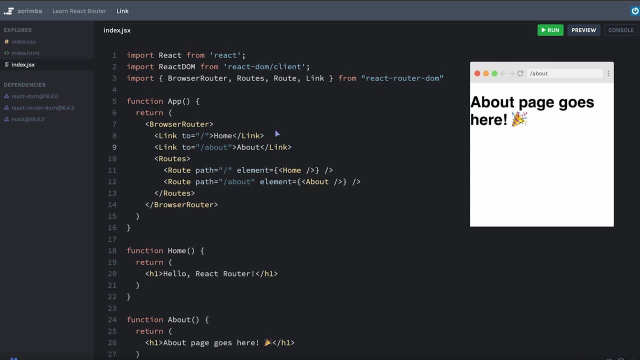 browser router like this. We're going to see a more robust way to have this navigation element. that will appear on every page later, But let me hit save. It's going to be poorly styled. It's just kind of shoved together because they're inline elements. But when I click the home button, 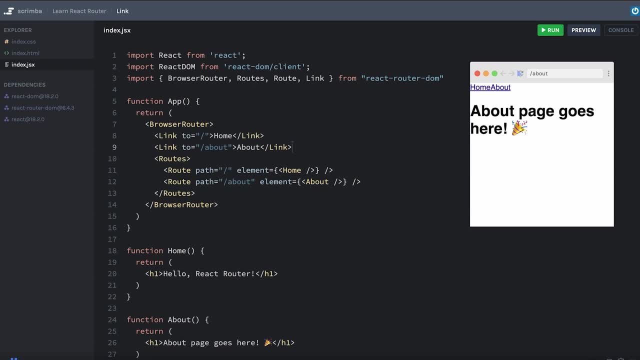 it takes me to the slash route And when I click about, it takes me to the about route And if you look closely, you'll see that there's no page refresh happening between the two. If I were to create some state in my app and pass that as props to my home and about components, 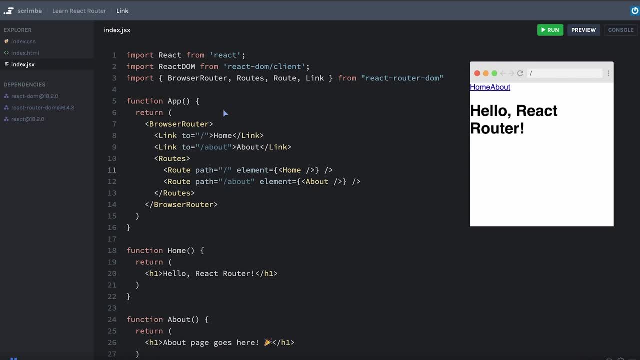 whatever state I created, even if I decided to change it, maybe like a counter- that I had a button that said increment and it counted up to 10.. When I go back and forth between the about page and the home page, both of those will still have that state of 10, as opposed to using an anchor tag or typing into. 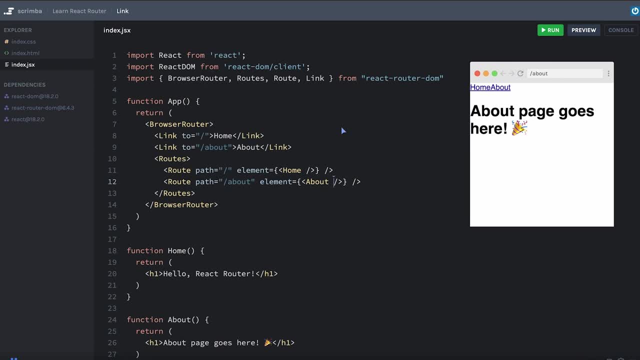 the URL bar because that would refresh the page and refresh my counter state back to zero, Because it would take quite a bit of code. I'm not going to bother actually showing that example. Hopefully it makes sense. If not, that's okay. The main thing to take away is that, if you want to, 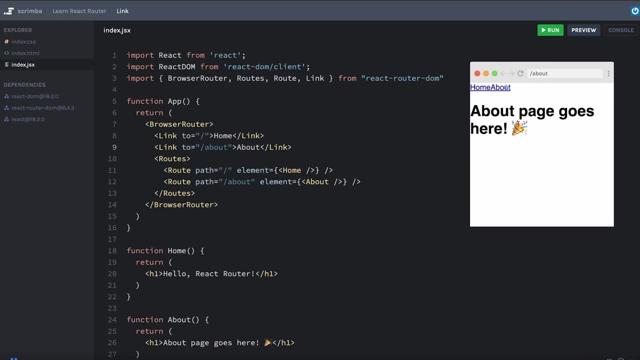 link from one place to another or navigate from one place to another inside your React app using link element. Now, if I want to style these links, I could either give each one of them a class name and select that class name in my CSS, or, if I need to use the element selector, then I can go into my 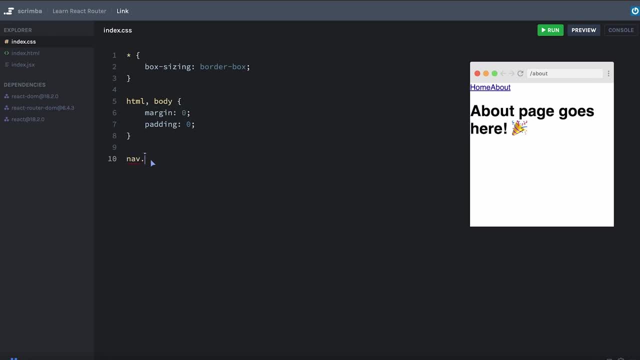 CSS. I can say select my nav, or maybe if I had some kind of class on my nav then I would put it there. But to select the element of the link, remember it's rendering an anchor tag, so I need to select the anchor. So maybe I don't like the underline. we would say text decoration: none. 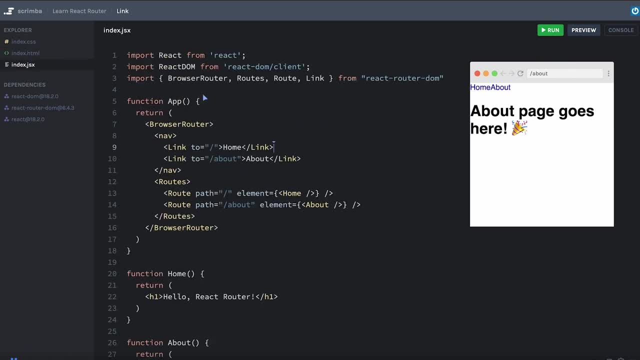 and there goes the underline. We are going to be revisiting the links a little bit later in this section, but for now this is good enough for us to more easily navigate around our app without having to type into the navigation bar or use these little back buttons and lose our state in the meantime. As always, feel free to play. 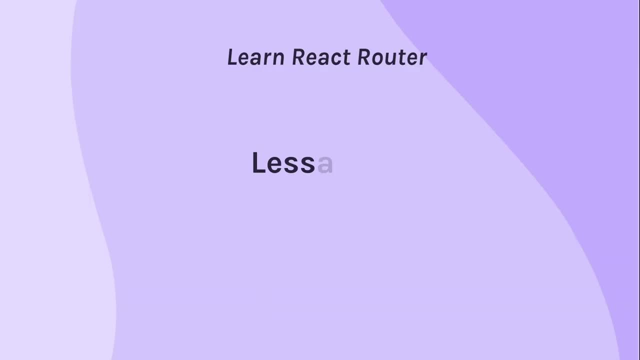 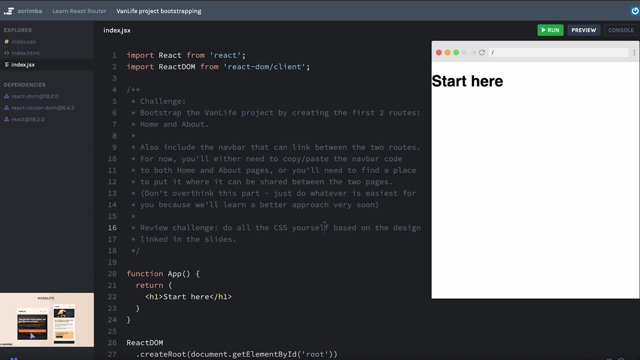 around with everything we've learned here and when you're ready we'll move forward. Before we move on, we're going to apply what we've learned so far by creating the first two pages of our van life project. So your challenge. 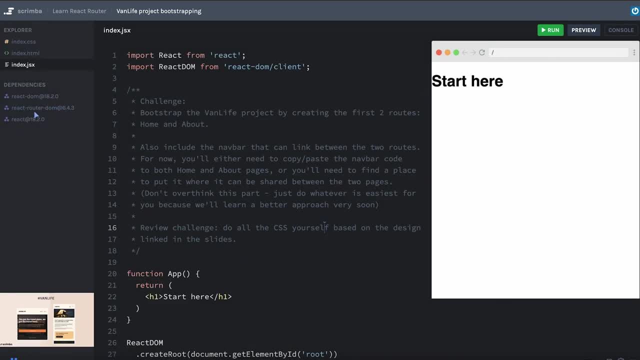 Is to do exactly that. I do have the React router Dom dependency already installed in this project, so you don't have to worry about adding the dependency. but you'll see that I have no imports. I'm not using anything with React router yet. 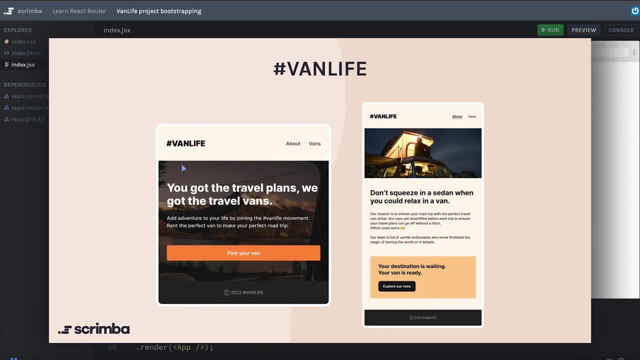 And so that's going to be your task. As a part of that, I want to make sure that you also include a navigation bar, so that you can at least get to the homepage by clicking this van life logo or the about page by clicking the about route. 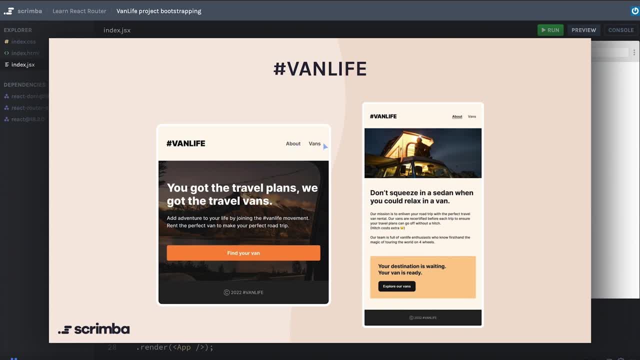 If you want, you can add a vans route, but we're not going to be dealing with that quite yet. As a part of that part of that, you'll notice that both the home page and the about page have the same navigation bar. we haven't learned sort of the official way to handle this. 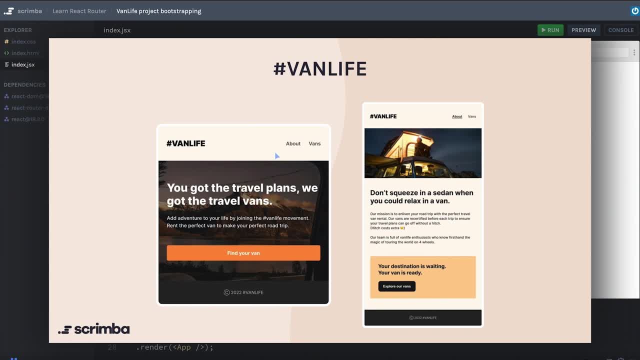 but I did show you one example in a recent scrim so I wouldn't worry too much about it. if you want to copy and paste the code you use for the nav bar on the two pages, that's totally fine if you find a way to use the same code on. 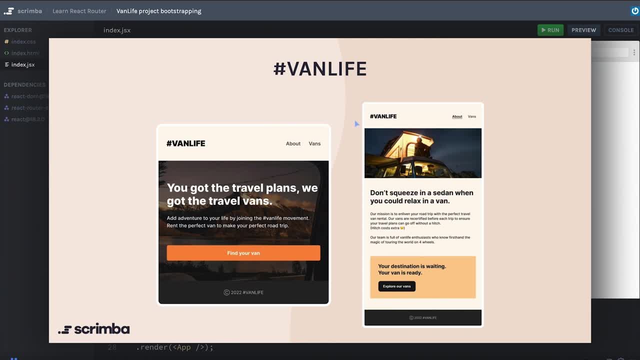 both pages. that's fine too. we're going to learn a more official way to handle that situation in an upcoming lesson. now, this isn't something I'll say super often, but I do trust you to know where your strengths and your weaknesses lie. if you do feel like you struggle with CSS, then I would encourage you to. 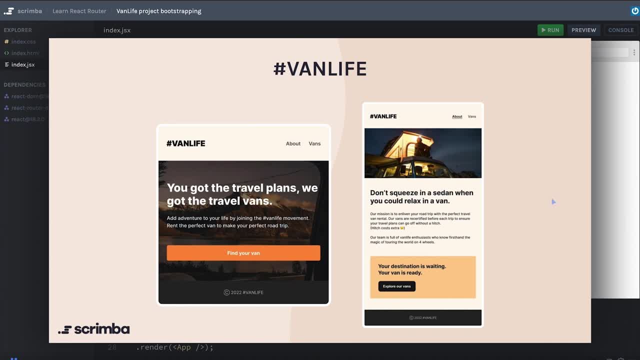 actually do all of the CSS by yourself. it's not an insignificant amount that you would be spending trying to get this designed this way, so I just wanted to give you a heads up, since I have already designed this on the side. we're not going to be spending our time actually thinking through and writing all the CSS. 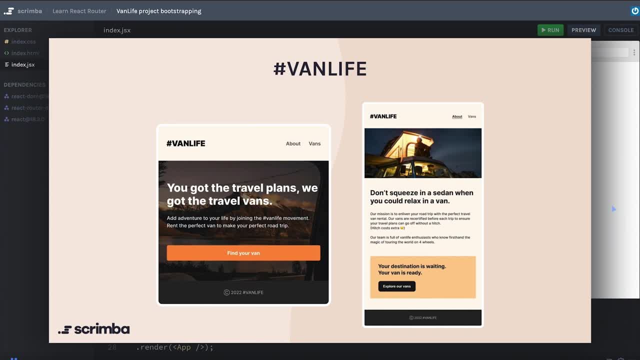 I'm just going to copy and paste what I already have, but since this isn't school, I'm not going to be giving you a grade. so if you have a weakness in CSS, then practice it, exercise it, actually, do this yourself. you can click on either of these screenshots, which will take you to: 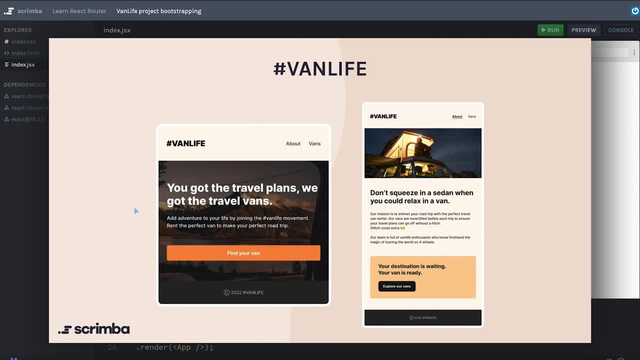 the figma design where you can grab all of the spacing and fonts and colors and everything you need. however, if you do feel pretty confident in CSS and you really are just here for the react, then I totally understand. if you just want to make a bare-bones white background, black text page that will link you between the 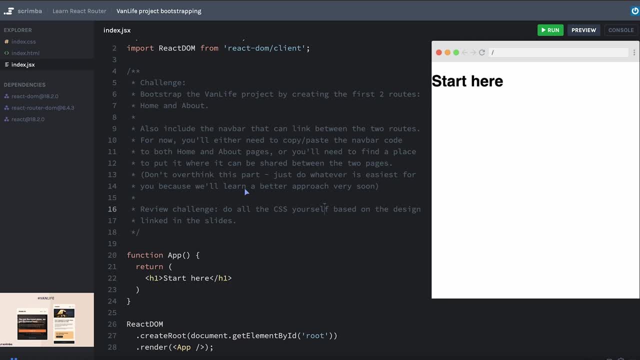 home and about page to practice react router specifically, and not necessarily to practice the CSS. so I'm just going to go ahead and do that and I'm going to practice the CSS. so I'll leave it up to you. just do whichever will be best for your own education. okay, that's enough of an intro. pause now and work on this. 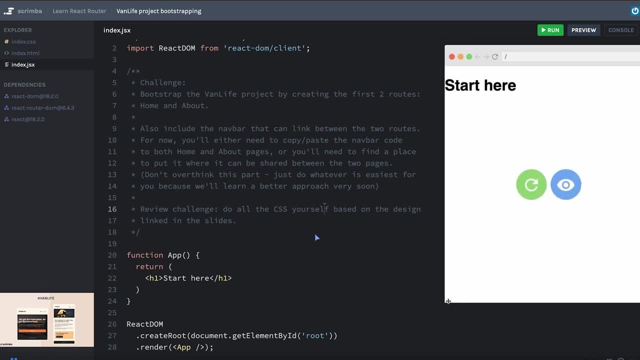 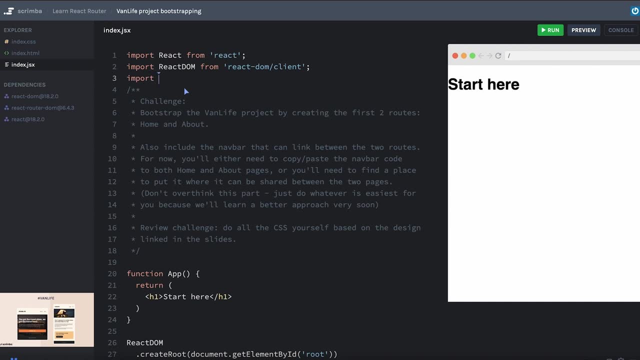 challenge. okay, let's import some of the things that we already know we are going to need. we know we need browser router. that's going to be the context provider that will set up everything with router. we'll need the routes component and some routes inside using the router. that's going to be the context provider that will set up everything with router. we'll need the routes component and some routes inside using the. 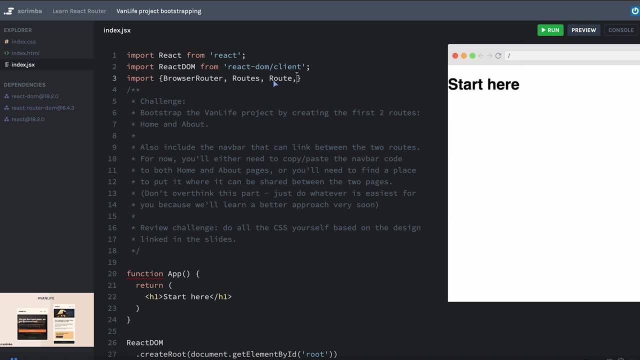 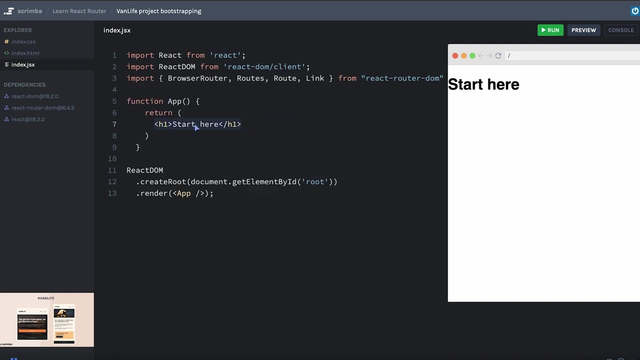 route component. the naming is a little confusing and we're going to need the link component and all of this will come from react router Dom. there's a few different ways that we can set this up. let me get by myself some space here. we could either put all of our react router stuff here inside of app, or we could put 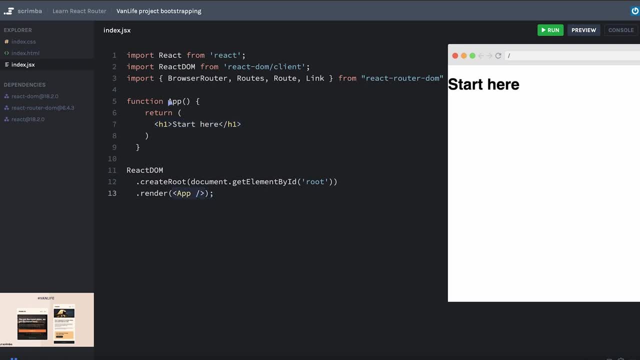 all of the react router stuff right here in the render. I'm going to prefer that my app act almost like a table of contents for my react router stuff, and so I'm going to verify that my app acts almost like a table of contents for my react router stuff, and so I'm going to 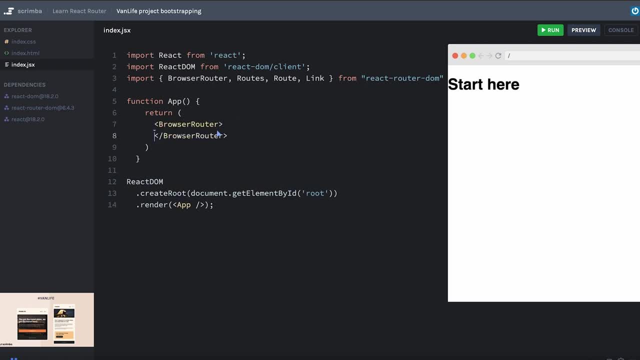 render the browser router. right here in my app we'll create our set of routes and inside there we will have a route. we'll have two routes and these are both going to have a path and the second one is going to be about, but we'll handle. 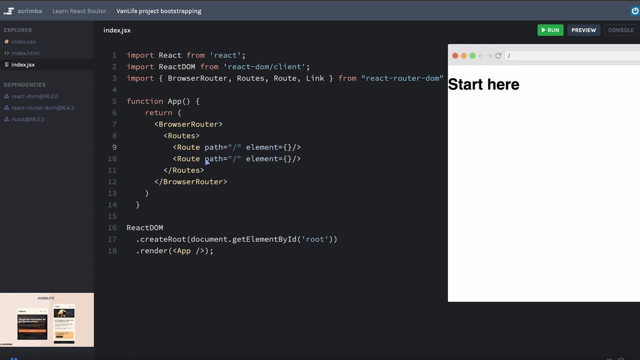 that in a second and then it will be rendering an element and let's have the first one, do a home element. the second one do an about element. this will be slash about and then that is going to lead us to some errors where we don't have a home or about elements. so let's import those even though they don't. 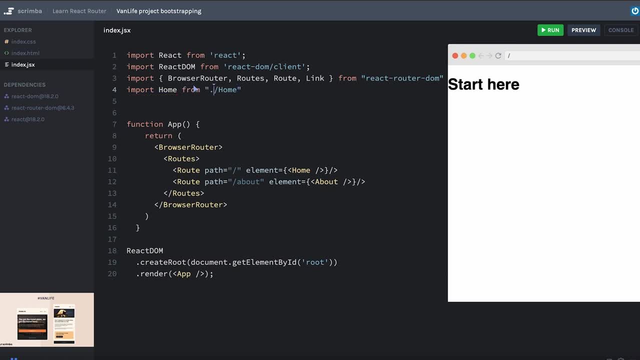 exist yet. and actually you know what I think? I'm going to put all of my pages into a folder called pages. so we'll say that I'm importing this from dot slash pages, slash home and about. okay, that means I'm going to have to create those. 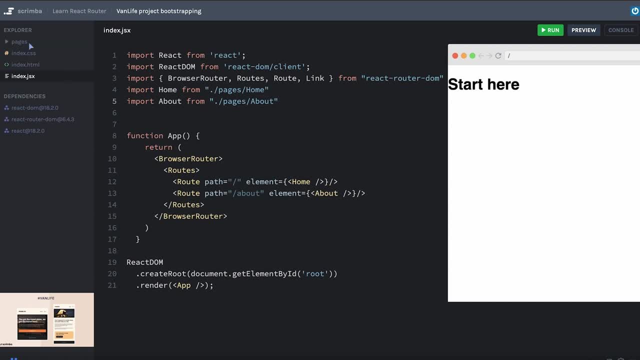 so we'll create a pages directory and I'll create a home, a home dot j let's see jsx, because i'm going to use jsx in this project, and we'll also create an aboutjsx. okay, import react from react. hopefully by now this has become kind of second nature, just being. 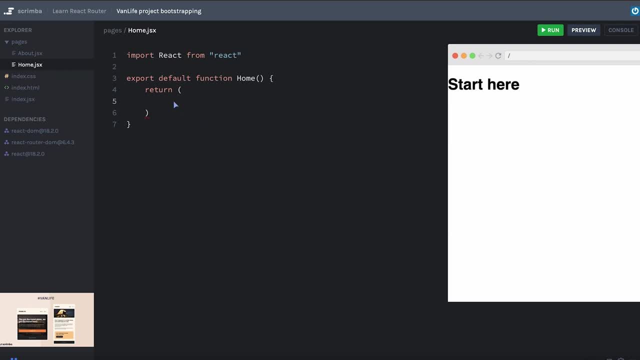 able to spin up a quick react opponent like this. let's do our classic h1 that says home page, and then i'm just going to copy this whole thing and put it in the about. we'll change this to say about page. okay, this is good. it's now displaying home page here. so let's go back to index and i guess 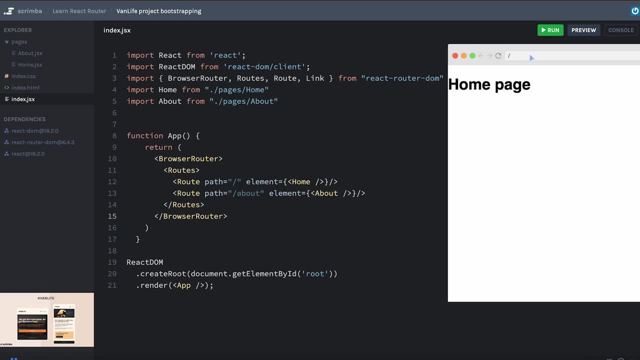 let's test to see if we have our different routes. so for now, because i don't have any links, we'll have to type in slash about. okay, we got to our about page. cool now. like i mentioned in the challenge, i didn't want you to spend too much time looking into how you would include the navigation. 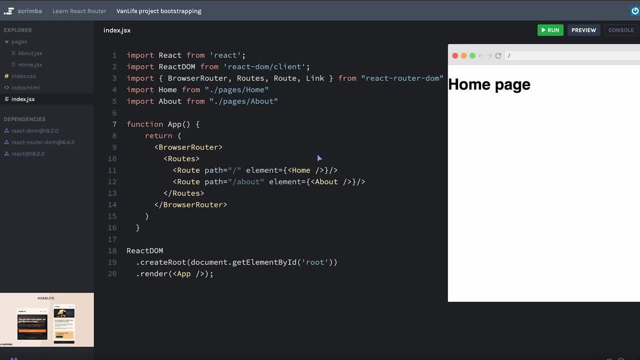 bar only because there's a sort of this designated real way to do this in react router and we haven't learned about that yet. obviously, when we have a site with a lot of different pages, it's not very maintainable to copy and paste the navigation bar into every one of our pages. if that's the way you solved this challenge of getting 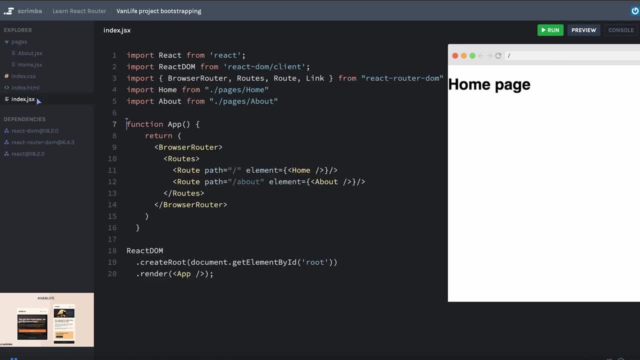 the navigation bar up there. that's completely okay. i specifically mentioned that that could be something that you do, but one other thing we could do is, before we start rendering our routes, i could stick the navigation bar right here under my browser router, above my routes. okay, so i'm going to go ahead and do that, and i'm going to go ahead and do that, and i'm going to. 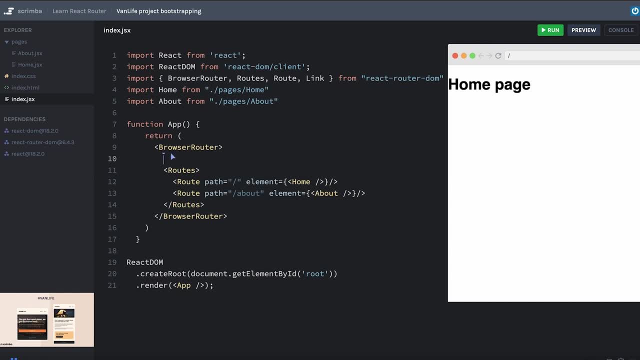 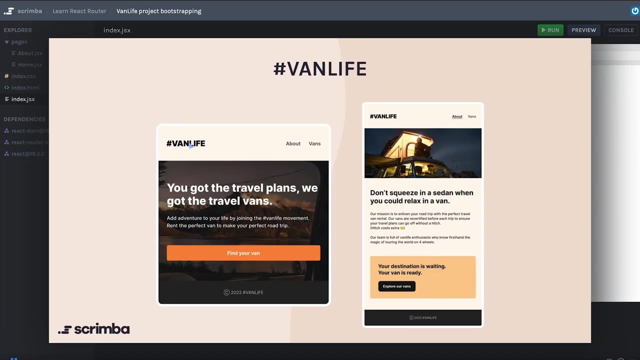 do that. so that's what i'm going to do for now, but we'll be learning the real way to do this very soon. so let's maybe put this all inside of a header element and that's where we will have our navigation and let's see. to be honest, i'm not sure if the logo that is clickable and sends you to the 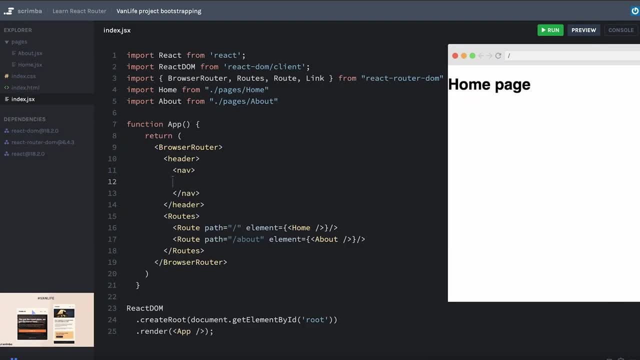 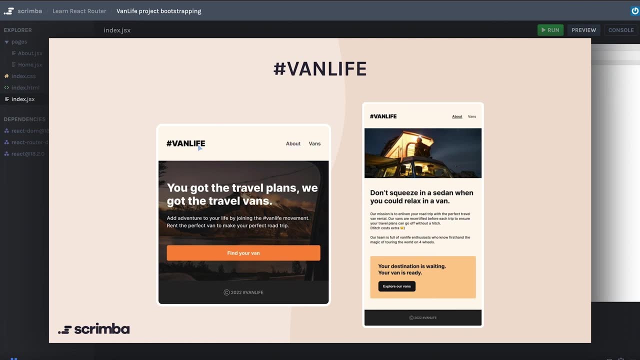 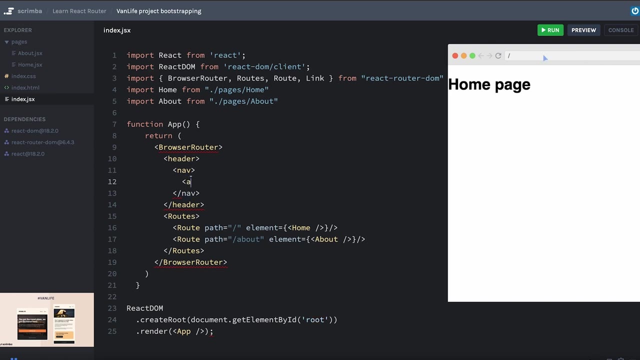 home page should be a part of this nav element because it's also kind of serving as the site logo. for now i think i'm going to just consider what's on the right here, part of the navigation, and i'll call this maybe its own link. so in the nav i'm not going to use an a tag, because that is not how we transition from one. 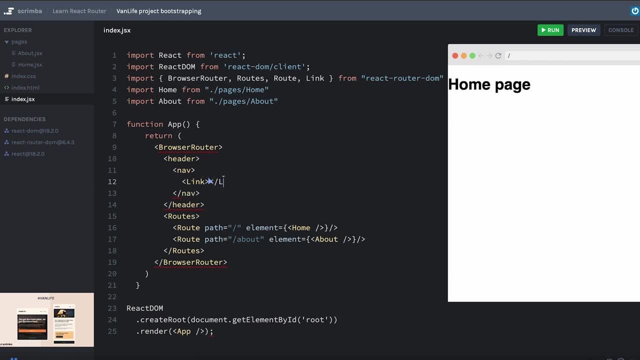 page to the next. in react router, i'm going to use a link element, but i need to import this. so, oh, i already did import it. okay, awesome. this one will lead us to the about page. i need a to prop that goes to slash about and then, as part of the header but not part of this nav, we'll say that we have. 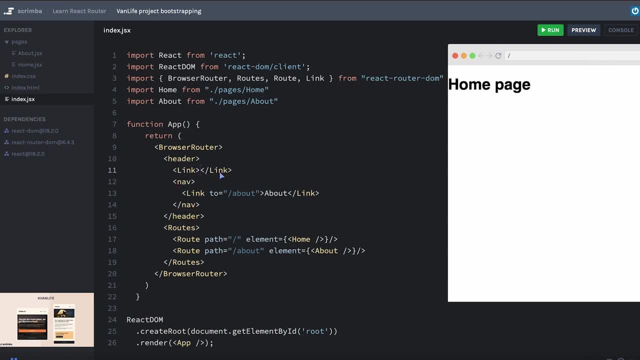 another link. this is the one that will say hashtag van life and this is going to send us to the home page or slash. okay, i'm sure this isn't going to be pretty, but let's see if it works. that takes us home, that takes us to about. okay, now this is kind. 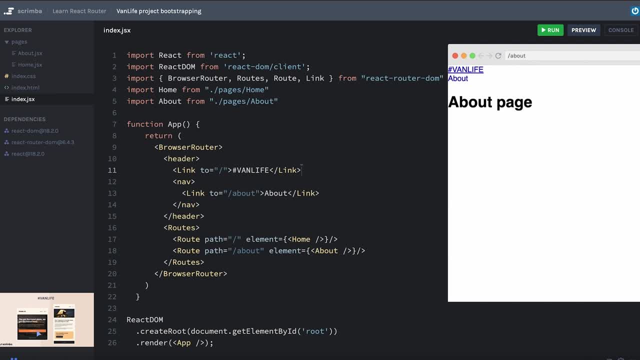 of what i was talking about. the rest of our efforts would really just be into putting some content on the page and then dealing with css. however, because we're learning about react router, i'm not going to spend our precious time making you watch me do css, so i'm going to snap my fingers and just like that. 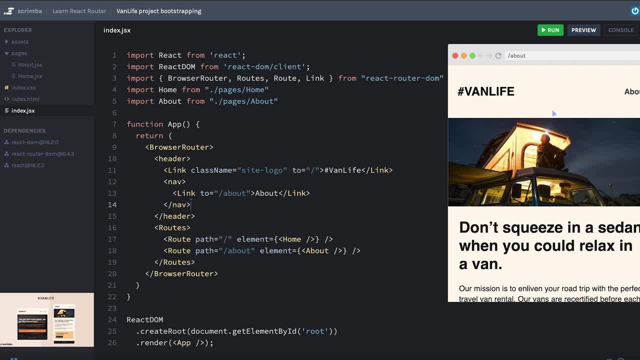 we have a project that is designed now. don't be thrown off. this is basically what we had before, just with a few changes, and i'll walk you through them so it's not so disorienting. our home page and about page: i've really just put in some css classes and some content. same with the about. 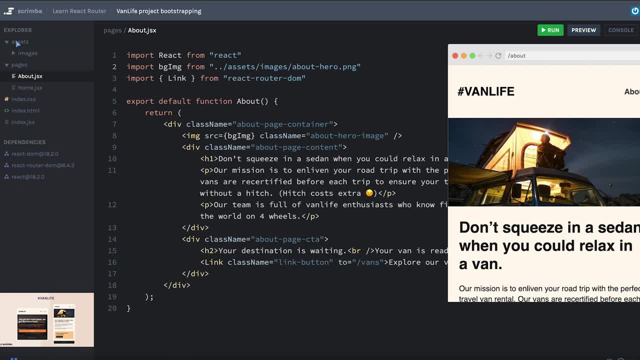 page over here. one thing you can see is that i also added these images. i put them inside of a folder called assets and then images, so we have the two heroes on the two pages. i have some styles that i plan to use throughout, like this button, and then i'm going to put in a little bit of 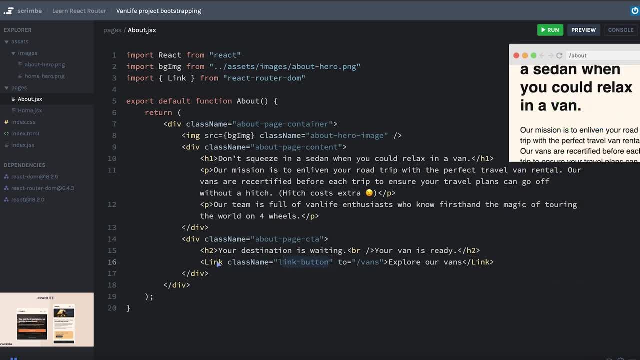 slack down here so that's a little bit easier for you to see that there are a few things i've done, that i wanted to get them created so we had this button right here. i called a link button just because it is actually a link, but i wanted it to look like a button and there's a few places where 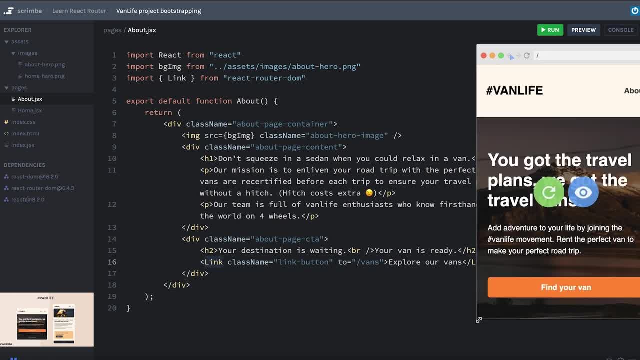 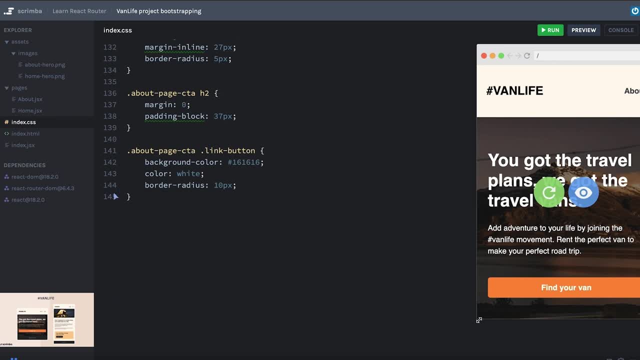 that exists, i think, over on our home page we also have this one, i think right now this might be sending to the vans route. yeah, but we don't have that yet. we're going to get there soon, so feel free to poke around the css if you'd like. it's really just 145 lines on top of what we already. 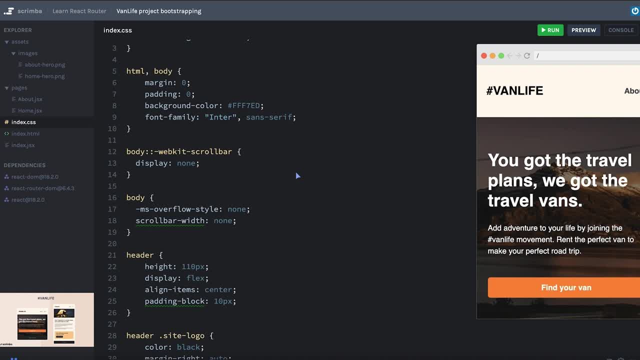 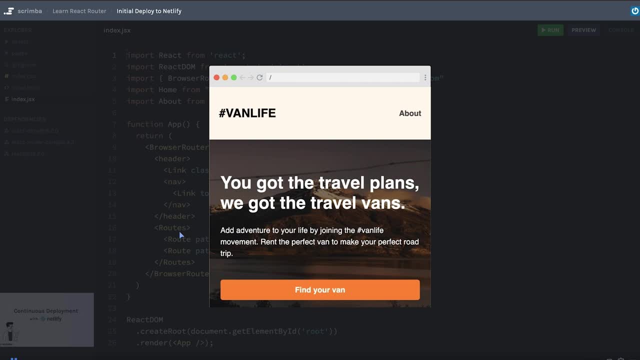 had, so it's really not too bad. so the next thing we're going to start learning about is something: Once you feel good about what we have here, let's move on. You know it may not look like much, but darn it, it is worth sharing. 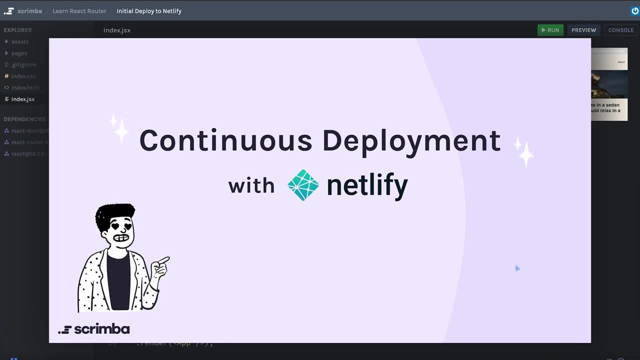 So let's talk about continuous deployment using Netlify. The terminology may sound complex, but I promise it's easier than it sounds. In this lesson we're going to walk through every step that you'll need to accomplish in order to get your project deployed up on Netlify and have an associated repository. 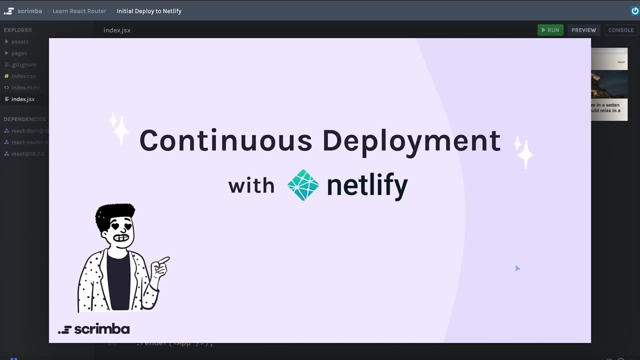 on GitHub. But once you go through all of these steps, as you'll see at the end of this lesson, it is dead simple to update your app and have that change automatically deploy to Netlify. So the idea behind continuous deployment is that as you make changes to your code, you 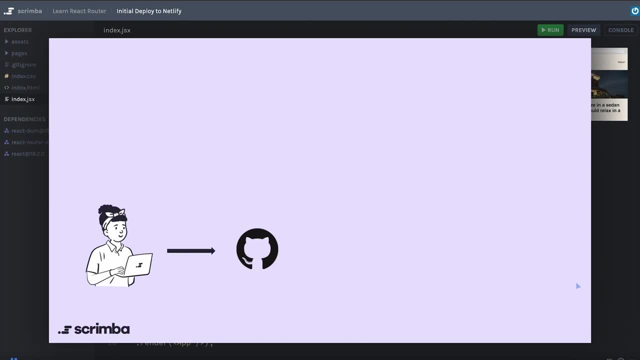 will push those changes to GitHub, which is an online place to hold your code, And when you push something to GitHub, it will automatically deploy to Netlify, And Netlify, being a web host, makes it so that people around the world can access your website. 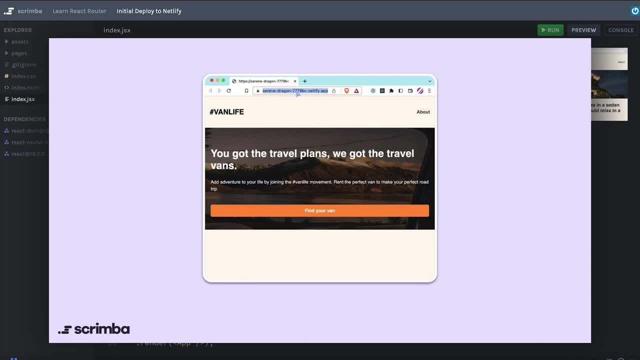 from their browser. In the end, the idea is we will be able to deploy your project to Netlify and Netlify will be able to have an actual URL that you could send to a friend, family member or post in a tweet and that person could go see the actual site that you have built and 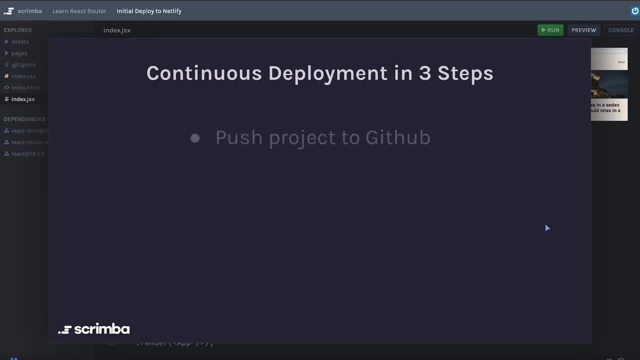 deployed Again. this will happen in three easy steps. First, we're going to push our project up to GitHub. Then we're going to tell Netlify which GitHub repository we want it to deploy and it will automatically watch for changes to that repository. 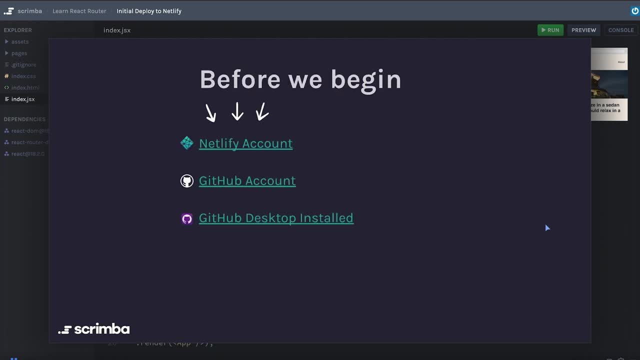 And the truth is it's only two steps. Then you're done. Now there's a few things we need to take care of before we begin, And actually I'm going to walk us through creating a Netlify account. So, in reality, you just need to make sure that you have a GitHub account and that you 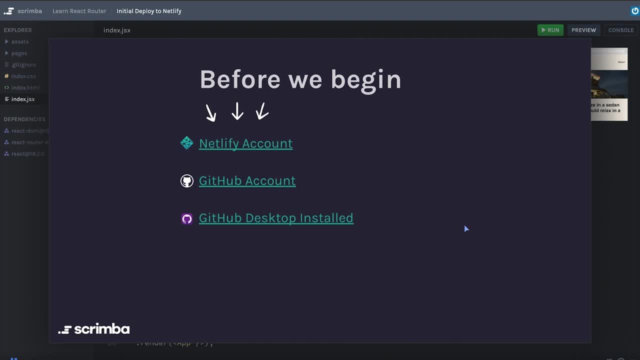 install GitHub Desktop. There's a bunch of different ways to use Git and GitHub, of course. I've found that for somebody first learning Git and GitHub, it's easiest just to use GitHub Desktop. If you are already familiar with using Git, then you don't have to do that at all. 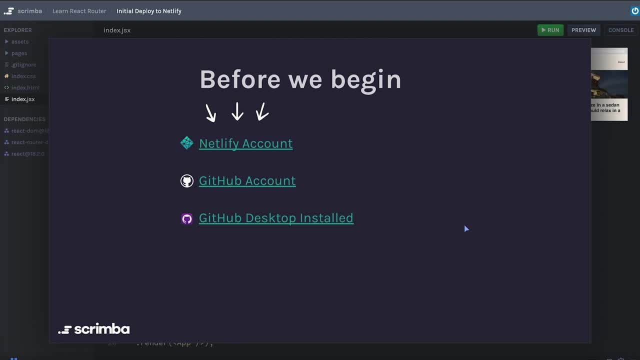 You can use command line, Git or whatever method you feel like using. So, before moving on, ensure that you have a GitHub account. Make sure that you have GitHub Desktop. If you don't have GitHub Desktop installed or you are already familiar with how you're, 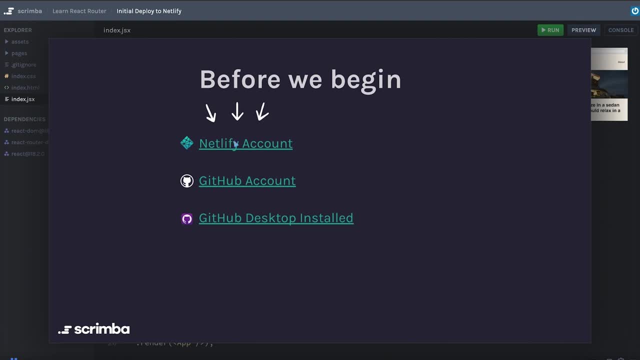 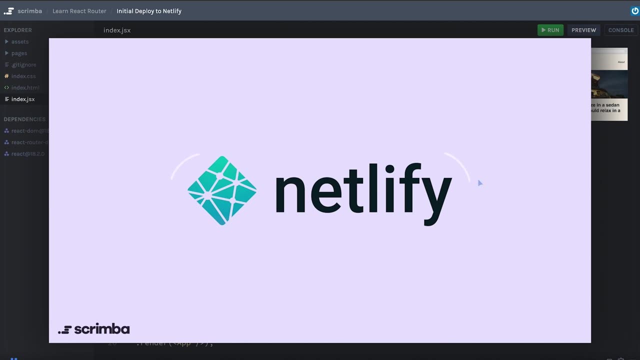 going to push your code up to GitHub. So, for creating a Netlify account, you can click Netlify account here and that will take you to the account page. or you can even click this logo here and you'll go through the steps of setting up an account just like you would anywhere else. 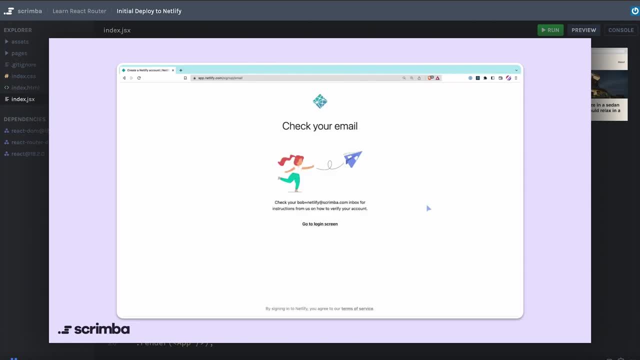 It'll ask for your email and password. You can hit sign up. That should send you a verification email. You'll go and you'll click that link. Clicking that link will take you to a sort of getting started page For me. 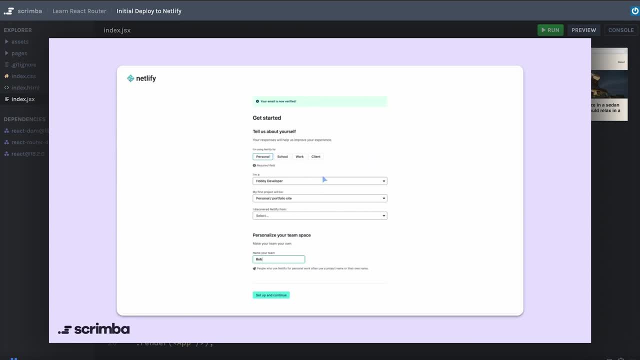 This would be primarily used as a personal account and I identified myself as a hobby developer. I don't think it matters much what you say your first project will be. I just put a personal slash portfolio site and for naming your team, because this is a. 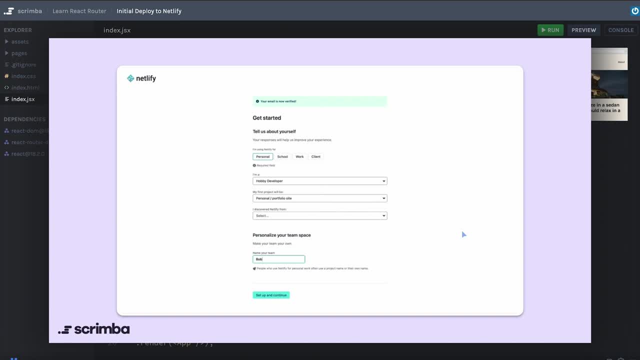 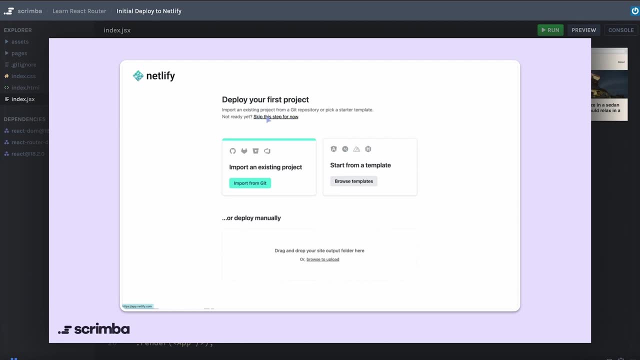 completely personal account. I just put my own first name as my team name. Then I hit set up and continue. We get to this page. For now I'm going to skip this step because we're going to come back to this later. 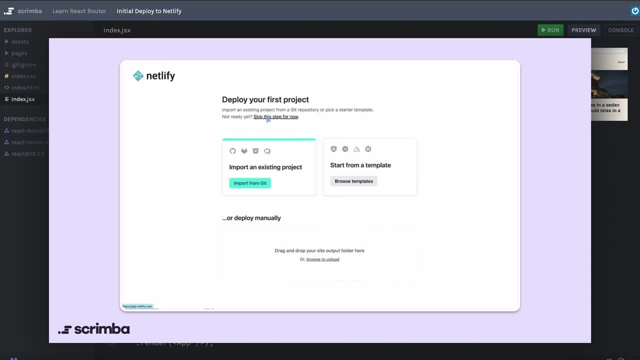 That said, if you're already familiar with Git and GitHub and you've already pushed your code to GitHub, then you can skip the next number of slides And, at this point, just say that you're going to import an existing project, for the sake. 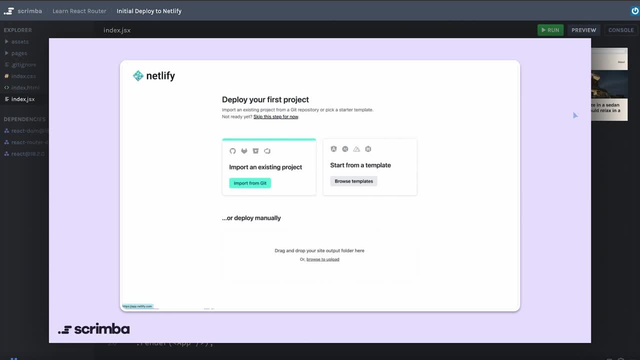 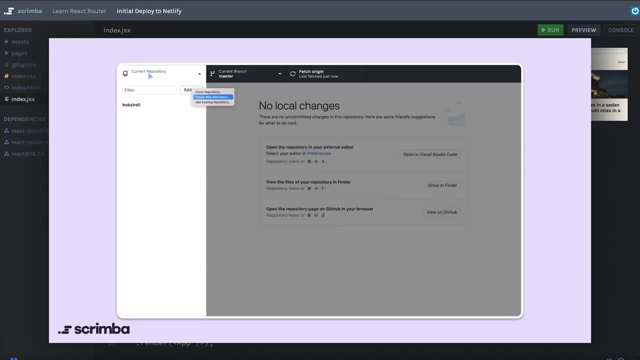 of completeness, I'm going to go through those steps and just skip this part for now. So that brings us over to GitHub desktop. I'm going to open GitHub desktop And in the upper left I see a dropdown for adding a new repository, and I'm going to create 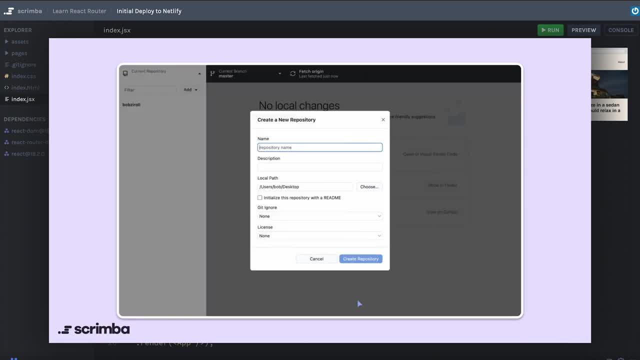 a new repository. Clicking create new repository will bring up a modal. I can give it a repository name. Everything else I'm just going to leave the same And for now I'm going to put it on my desktop. but I would recommend organizing it somewhere. 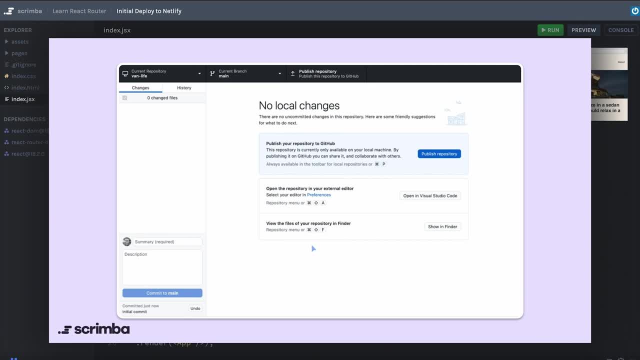 that you actually want to keep it. Then click create repository. That will bring you to the main page for your repository that you just created, And next we need to actually put some files inside of this folder. Now, depending on how you're following along, this next step will look a little bit different. 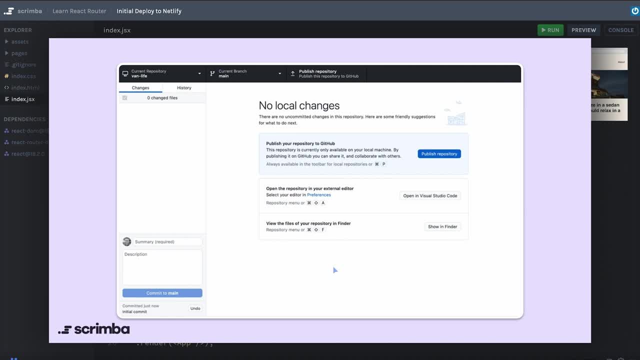 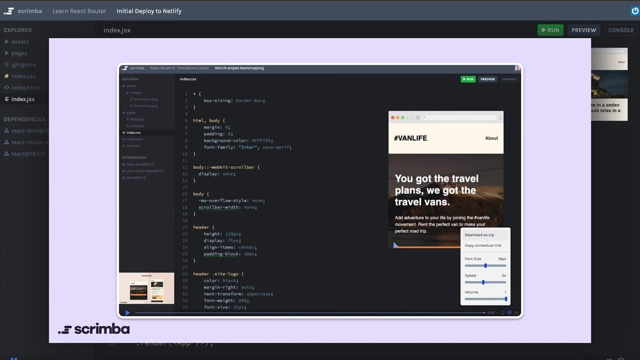 for you. I'm going to show you how you could do it directly from scrimba. in the current scrimba interface There's a little gear icon in the lower right that you can click and choose download as zip, And in fact you can do that right from the scrim here. 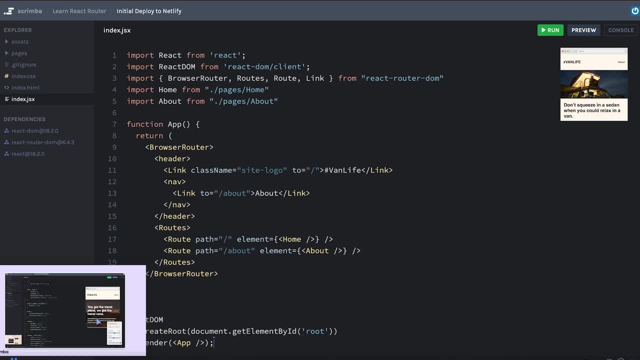 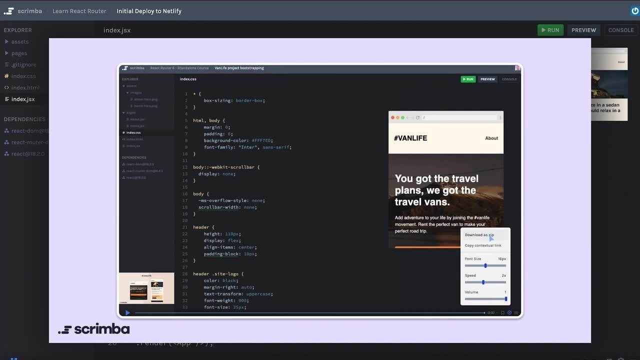 It basically has everything that we just saw where we left off in the last lesson. Do be aware that in the future, as the scrim interface changes, the location for this option to download the project as a zip may change. So just search around until you can find the option to download this project as a zip. 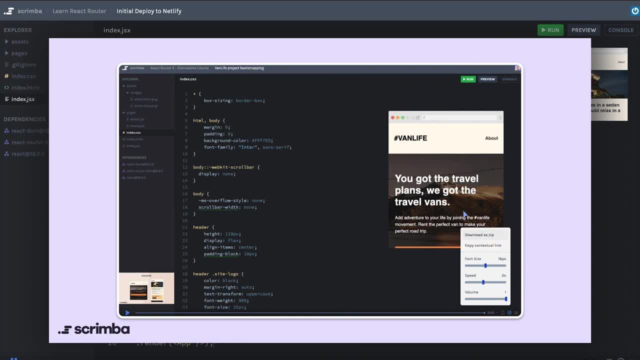 Now that will create a zip file. You'll have to unzip it- which will have a folder with your project files in it, And because we've already created a new folder that is a git repository, I've found that the simplest thing is just to take all of the files from the project that we just downloaded. 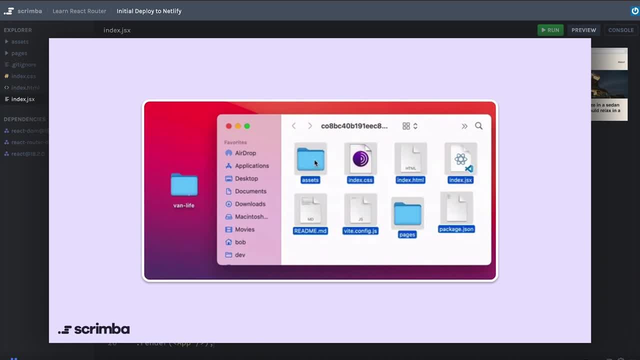 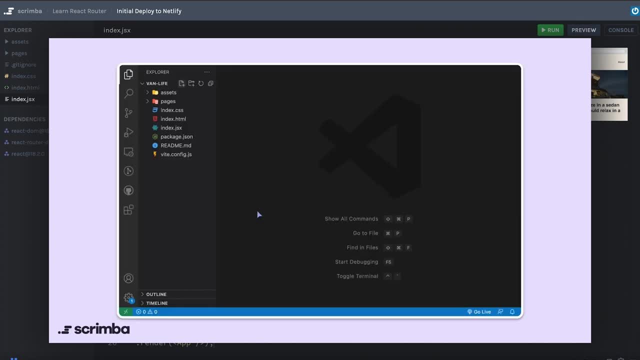 from scrimba and drag them over to the new folder that we just created with github desktop. Then you can take that vanlife folder and open it in vs code. Now this next step is going to be pretty important. We haven't yet run an npm install on this project. 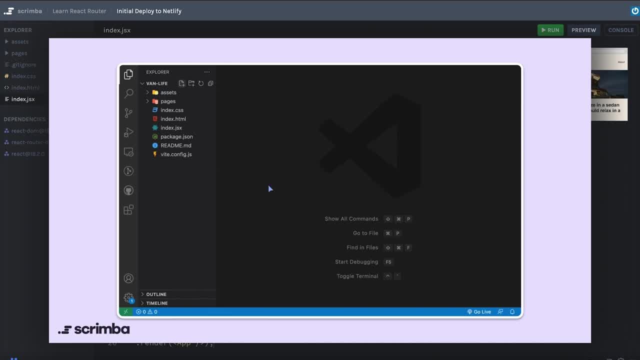 As you can see, we don't have a folder called node modules, But it's pretty imperative that we don't commit our node modules, along with a few other things that are really good to never commit to your github repository. So I would highly recommend at this point, immediately before doing anything else, to 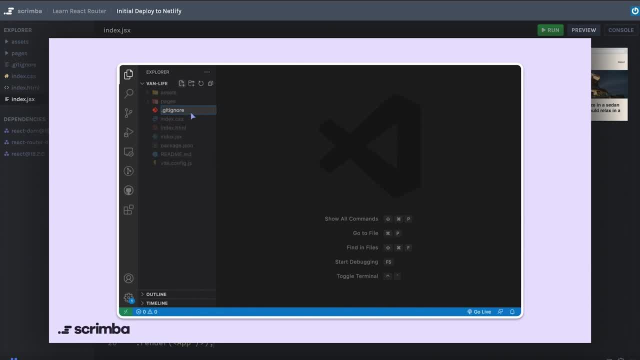 create a gitignore file. In this file, each line will contain a folder or a file or some kind of naming structure that you are telling git you don't want to ever include in any commits that you make. If that doesn't make a lot of sense, that's okay. 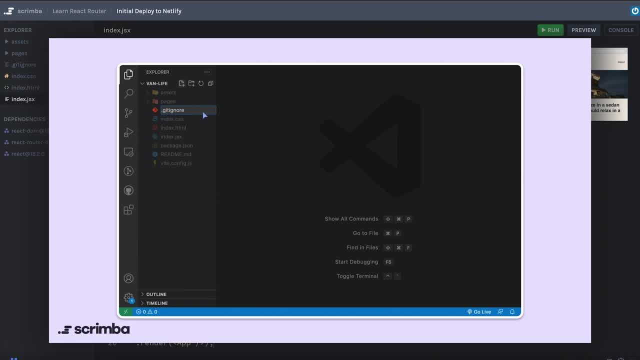 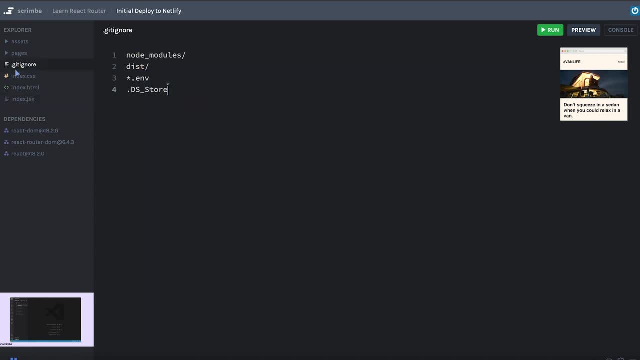 Just know that it's important to have a gitignore file And to include at least a few basic items. Now, if you were just following along and you downloaded this project, I did create a gitignore file already, mostly so that anybody who isn't downloading this can actually come in here. 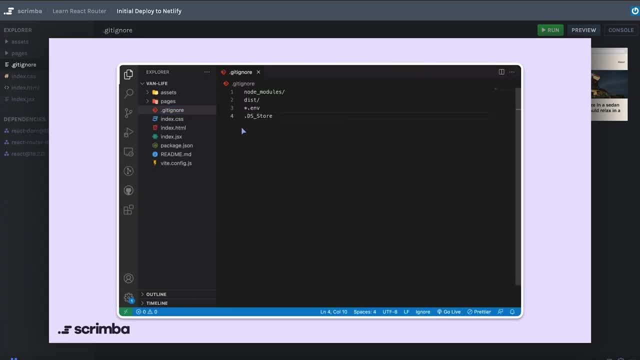 and copy the items that I have listed here and paste them into your gitignore file that you just created. I also made this a little bit larger, so it's a bit easier to see. Now that we've made a change to our project, we can go over to github desktop and we will. 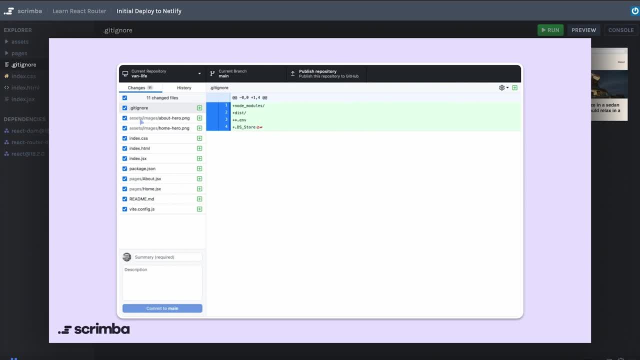 see that it is already tracking the changes that we've made, including dragging all those new files over and creating a new gitignore file manually. So let's go ahead and commit these changes. We can do that by adding a summary down here in the lower left. 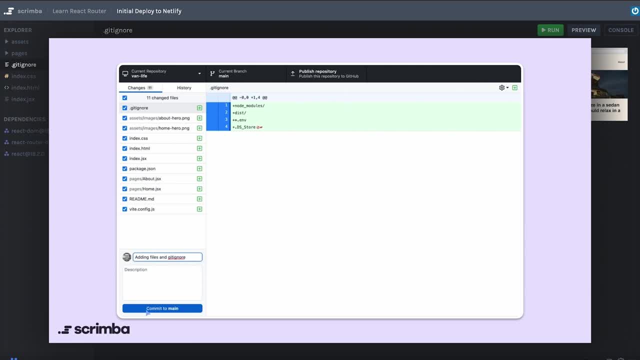 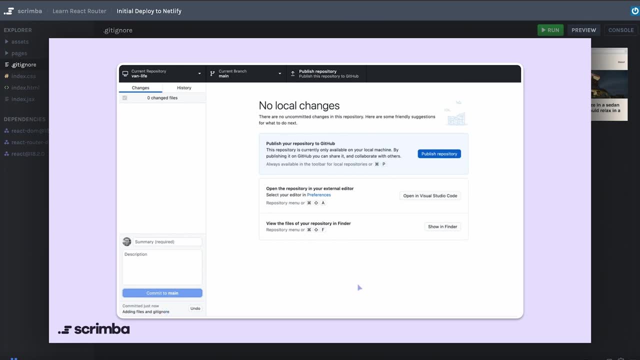 I'm just saying adding files and gitignore, And then I can say I want to commit these changes to the main branch. So I can click that button And after a few seconds that will be done. If you're relatively new to git and github, it might be important to note at this point. 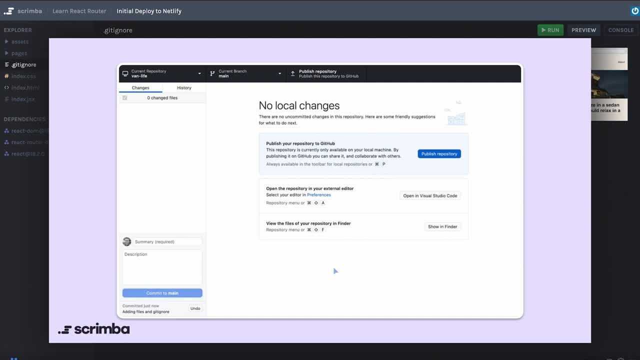 that you have only committed to gitignore, But you have not yet pushed anything up to your online github account. So that's what this publish repository button is for. We'll go ahead and click this at this time. We'll get a modal here. 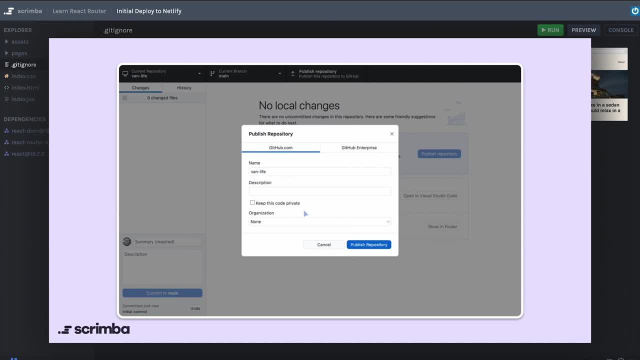 It should already have a name filled out. You don't necessarily need to change anything else unless you feel like adding a description or making this a private repository, And you can click publish repository And once that is done, it will send us back here to the github desktop dashboard. 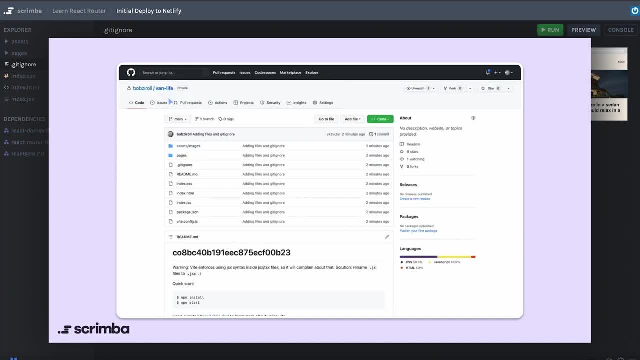 At this point, Click the button to view on github, which will show you that your code is now live online. The stock readme that we get from scrimpa is a little bit ugly, but that's okay for now. Okay, now that our project is live up on github, we are primed to go back to Netlify and sync. 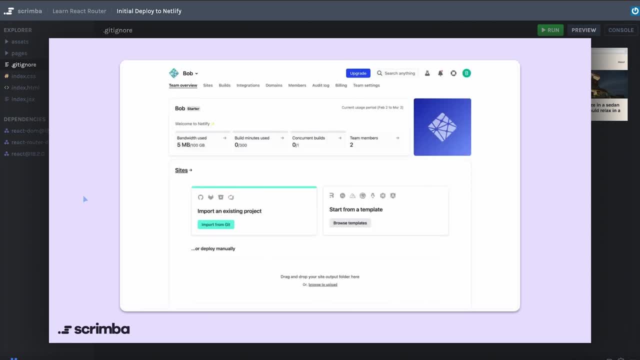 up our repository with our Netlify account. So back on Netlify, we are greeted with this dashboard page And we can click this button down here that says we want to import an existing project from git. When you click that button it will ask you to connect your git provider. 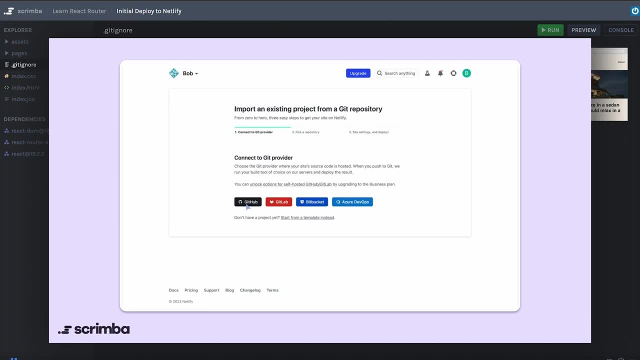 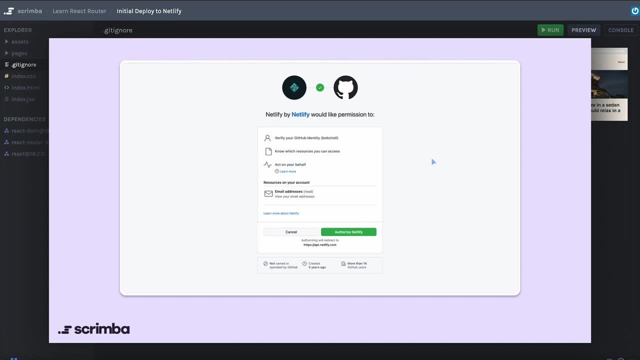 In our case, we're using github, So I'll click the github link, which will send me to an OAuth page where I can authorize Netlify to access information on my github page, And when I do that, I'll have the ability to search through my entire list of repositories. 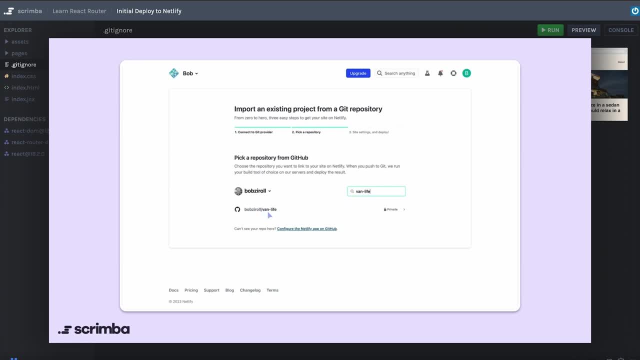 I've here searched for van dash life. that pulled up my new van life repository, So I'll select that repository. Doing that, Netlify will try to figure out the best way that it can deploy this project And it usually does a pretty good job. 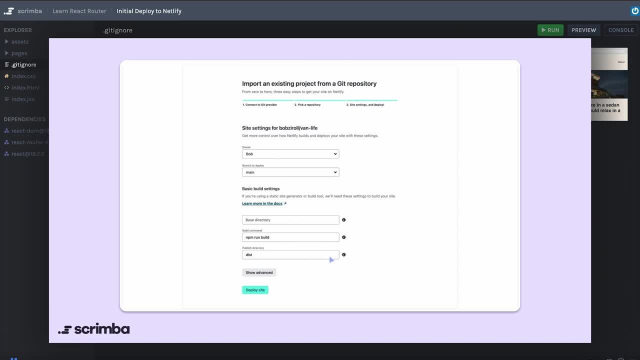 So for me, I was able to keep all of the stock options here exactly the way that they were. The most important thing is that we run npm, run build as the build command and that the publish directory is dist, unless you have gone out of your way to change the V config. 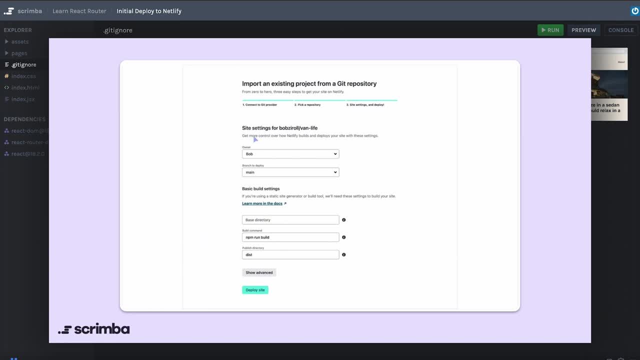 settings or the package dot JSON, so that this is different. So this is what popped up for me. I'm just going to keep it that way and hit deploy site. Doing that sends me back to a dashboard page for this specific site And we can see that it says it's building a new production build. 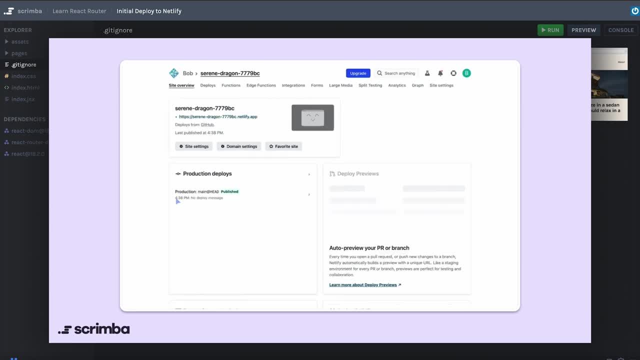 After a pretty short wait, we'll see that word building changed to published, And at this point it's just chosen a random URL which is going to be good enough for us for now that we can click on and see our site live on the web. 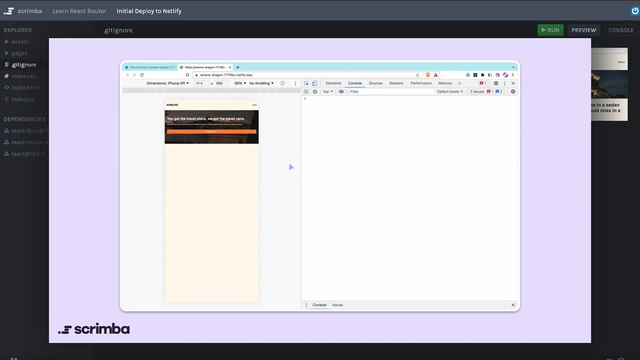 Super cool. Now, oops, it does look like we have a little bit of an issue Here on scrimba. Of course, we pretty much develop everything as a mobile style, But even when I turn on the mobile view in my developer tools, we can see that the styles 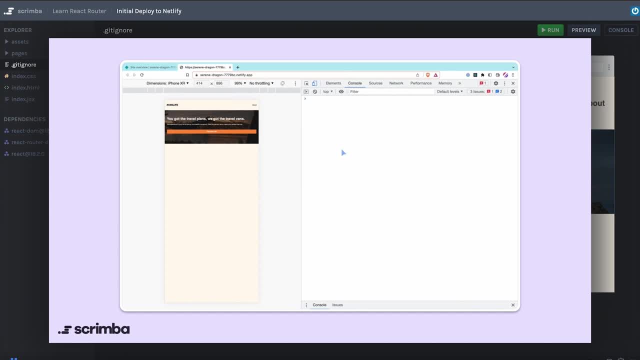 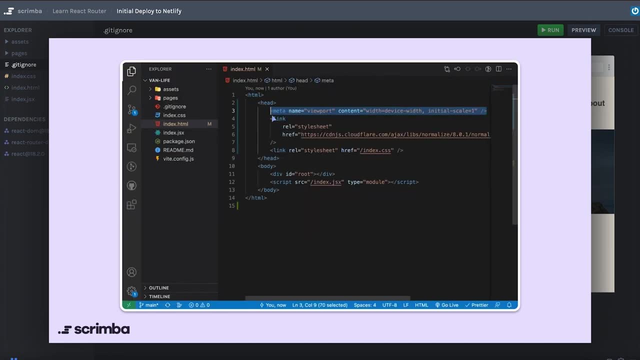 are not really looking like a mobile styled site. To be honest, this is something I almost always forget to include when I'm spinning up a new project completely from scratch, And that is to include this line of code, which is a viewport meta tag: 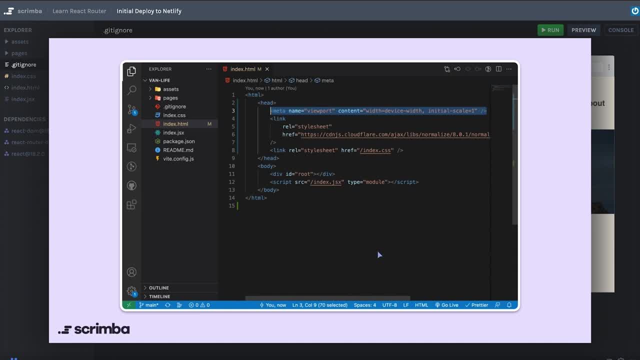 So the reason I'm showing you this process is not because I actually forgot to do this, But because I want to show you how, once you have deployed your site live, you can make changes and update the live version really, really easily. This is where the benefits of having continuous deployment setup really shine. 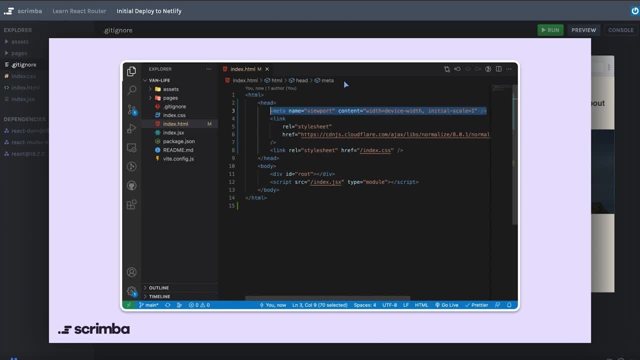 Now, if you are actually following along and you want to add this line of code, you can actually click this screenshot. it will take you to a page on MDN which has a quick way to copy this line of code and then you can paste it into your index HTML page right below. 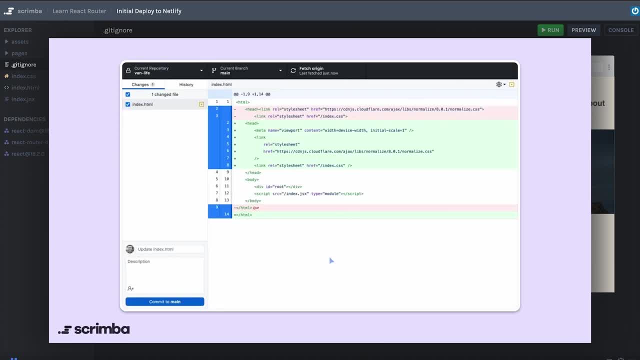 the start of the head tag, like I did here. Now, once I paste this in, we can go back to GitHub desktop and see that it is tracking some changes Here. I think my formatter might have changed the way that things were lining up, which. 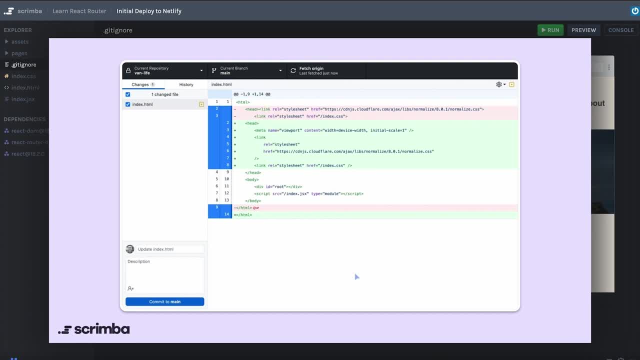 is why it's showing a little bit more green than what we actually added And, just like before, I can add a little summary up here. if I want, I can also add a description and hit commit to main Again. this is only committing to my local repository and doesn't automatically make 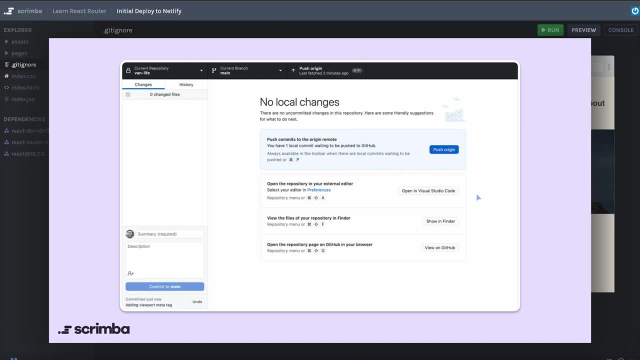 changes to my GitHub repository. In order to do that, I do need to remember to push these changes. this commit up to my origin, which is the repository that lives on GitHub And from GitHub desktop. I can do that by just clicking push origin. 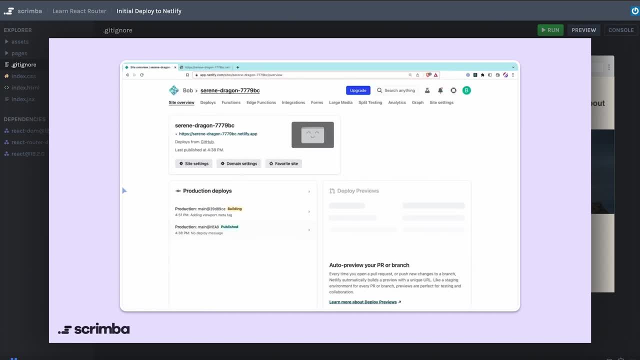 Then, without doing anything else, I can go over to Netlify and see that it has noticed a new commit to my main branch on my GitHub repository, So I can click on that. And now I can go back to my GitHub repository And so it starts rebuilding my site. 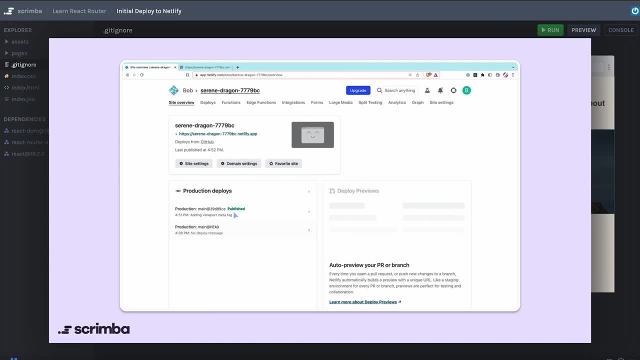 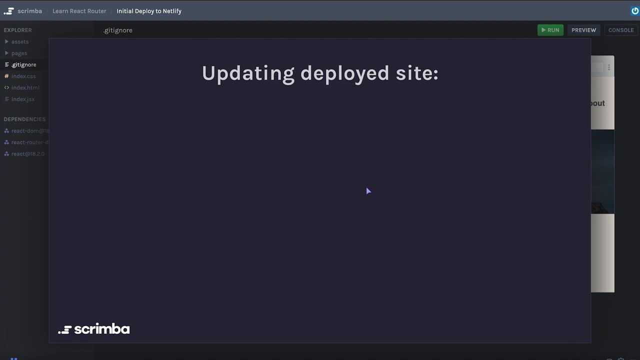 And after a few seconds again, it will have a new published site that includes my changes. Awesome. So again, the process for updating the deployed site in just three easy steps. One, we change our code. Two, we commit and push those changes to GitHub. 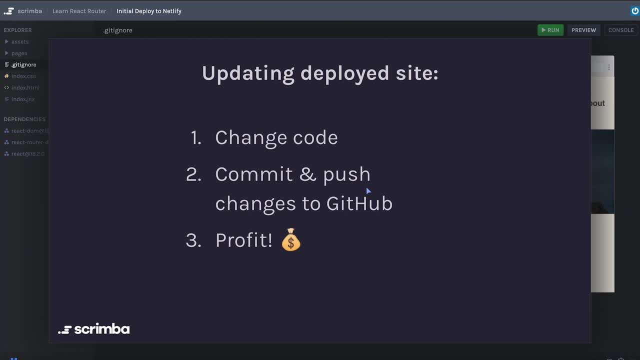 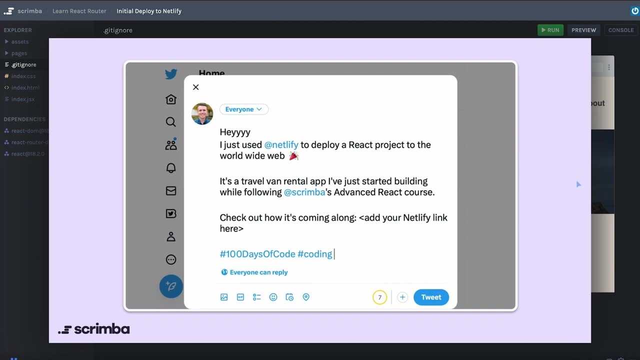 Again. it's just two steps. That's how simple it is. Now that you have a live site that you could share with family and friends, I'd recommend jumping in both feet with the build in public mentality. If you have a Twitter account, you can click this screenshot, which will pre-populate a 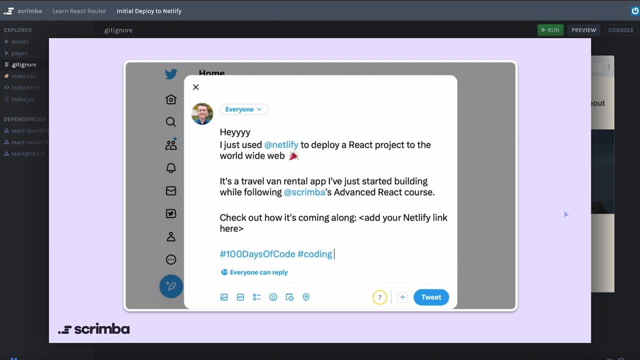 tweet that you could send out to the world and really show off the work that you're doing on your projects. Of course, make sure to add your actual Netlify link here at the bottom. One last important thing to mention is that, even though you've downloaded your code to 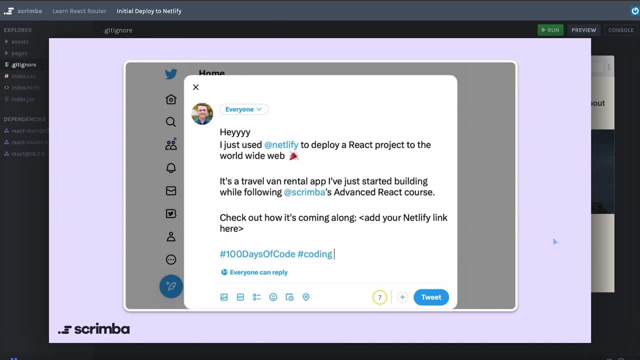 your local machine and pushed it up to GitHub. it will still be pretty important for you to follow here on Scrimba. Scrimba isn't intended to be the ultimate place that your code lives. You're not going to open Scrimba in order to write production level code, for example. 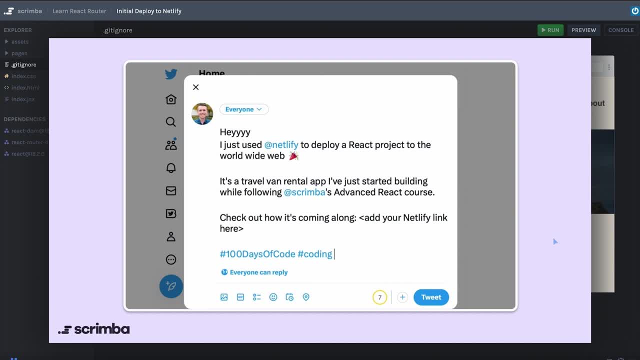 But for the most part, it's going to be the ultimate place that your code lives, that you're not going to open Scrimba in order to write production level code, for example, But for the sake of learning, Scrimba makes a lot of other things easier. 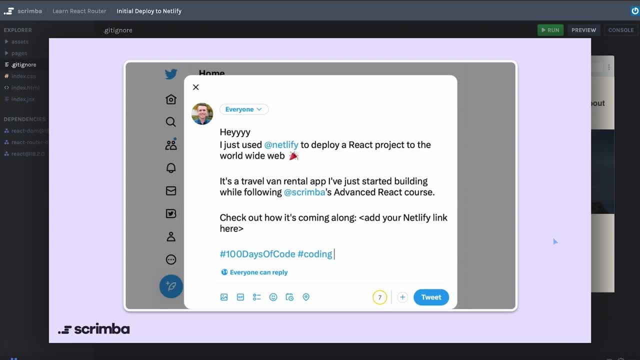 It lowers the barrier to get your hands on the keyboard and follow along. So in the future, when we talk about deployment again, we'll cover the steps on how to update the code that you just downloaded to your local machine so that you can deploy the most. 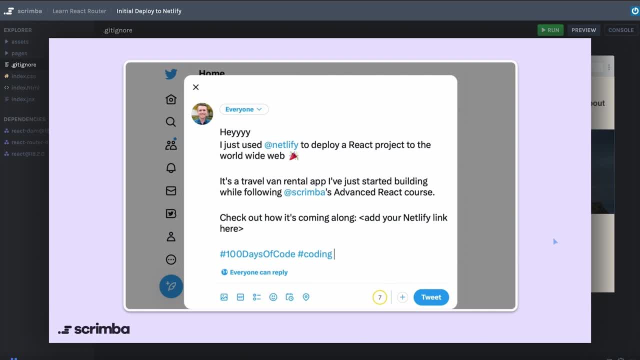 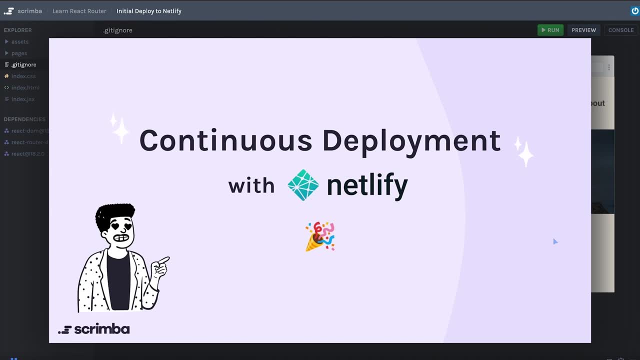 updated stuff, But for the best learning experience, just remember to keep following the course here on Scrimba. Okay, that's everything we have to touch on right now for continuous deployment using Netlify. So let's keep pushing forward and building our van life app. 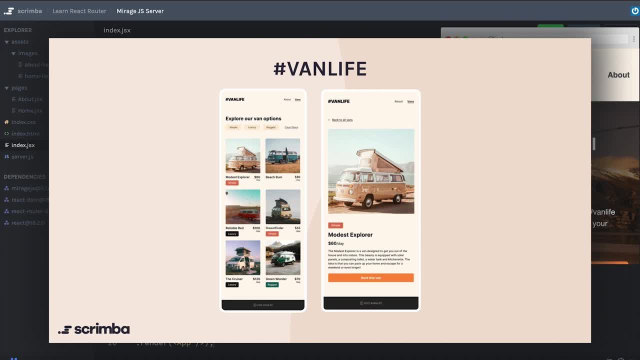 In these upcoming sections. we are going to be working on a vans list page and a van detail page And, as you can see, there's some data here that needs to be coming from somewhere. In the past, what I've done is created just a simple data dot j s file and kind of pushed 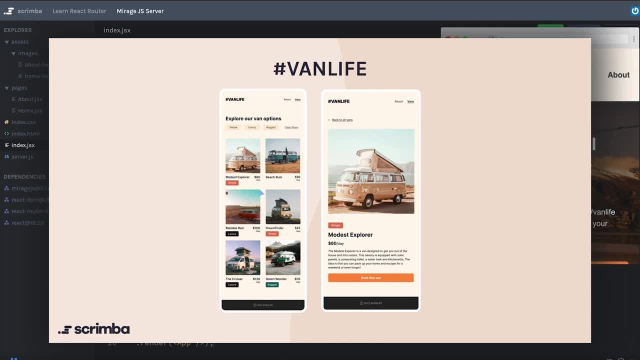 all the data in there, But that meant that we were just importing that file instead of actually doing a fetch request to a server and a database like you would in the real world. However, I also didn't want to create a real server and database. 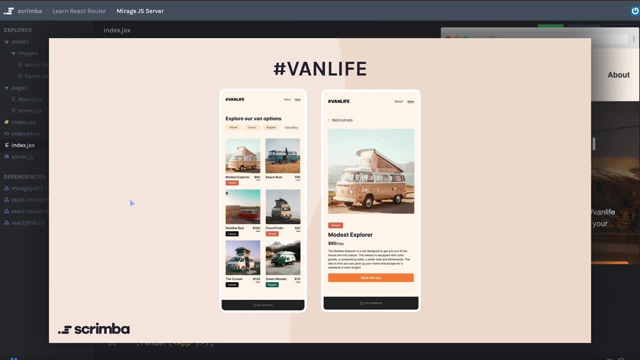 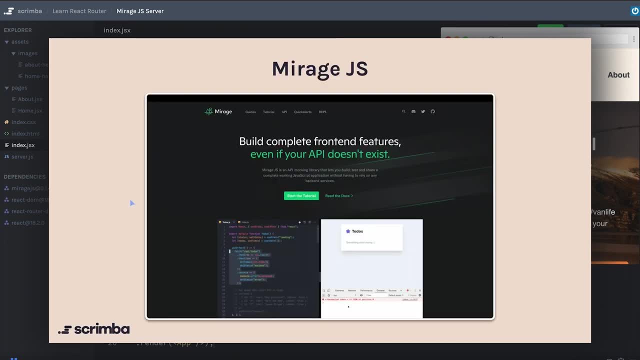 Just because of the maintenance problems that can happen over time. However, I found a solution that I think will be a really good compromise, and we're going to try it out in this project. There's an NPM package called Mirage JS. You can click on the screenshot here to go to their website if you want to learn more. 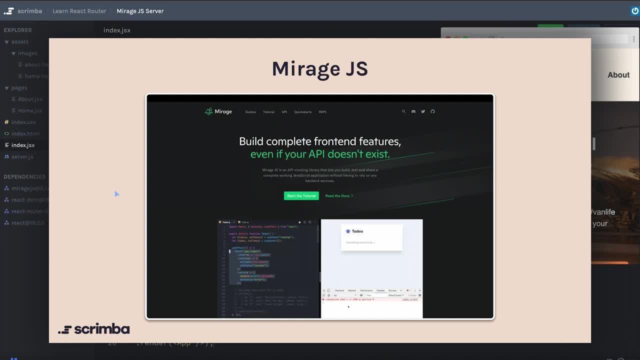 about it And it's a way to create a mock server that will intercept any API requests you make and it will return the data from your mock server instead of having to worry about reaching out to the real world. This isn't something you have to worry about. 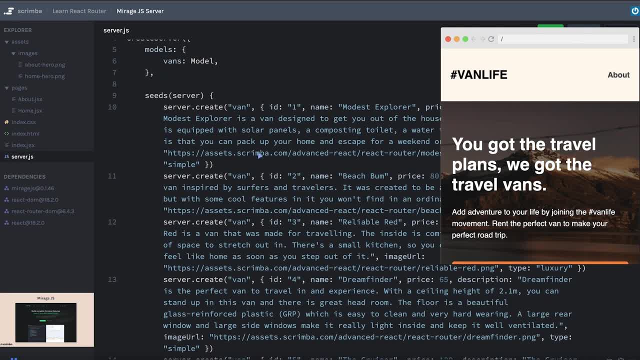 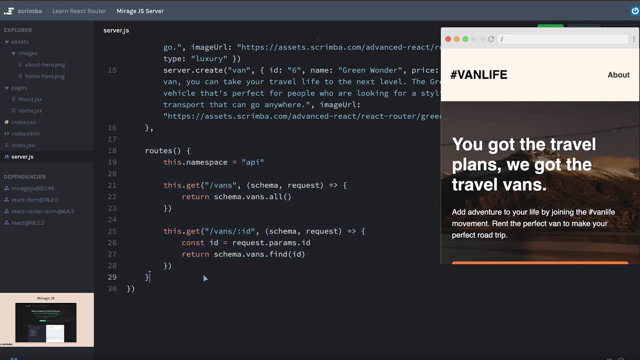 To look in this serverjs file that I created. you can see there's the data for our vans and down here at the bottom there's a simple routes section, which you can think of like the server code that will run whenever you make a request to slash vans or to slash vans. 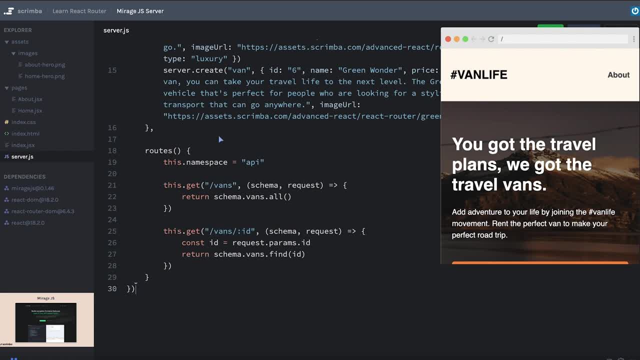 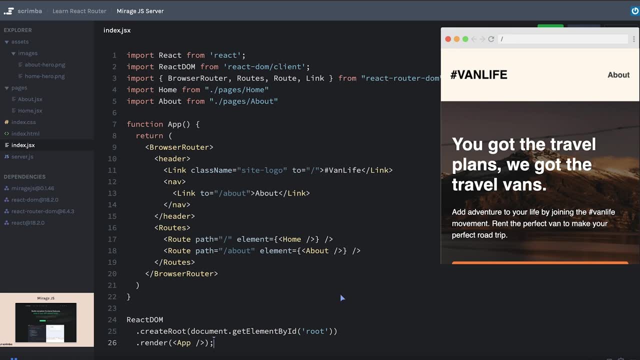 slash the ID number of the van Again. this doesn't have to make sense. In fact, you can think of it more like you are the front end developer on this project and a back end developer. one of your coworkers has already created the server and some endpoints. 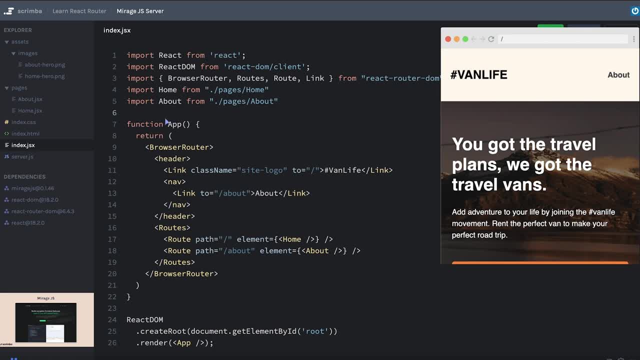 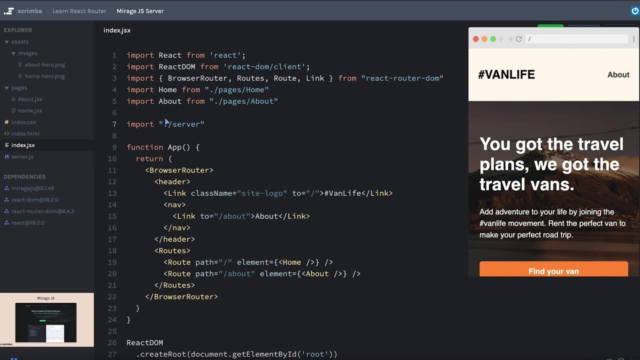 for you to get data from. What's nice about this is I don't have to pollute my code too much. The only thing I need to do is say import server. So import dot slash server and everything else will work out just fine. 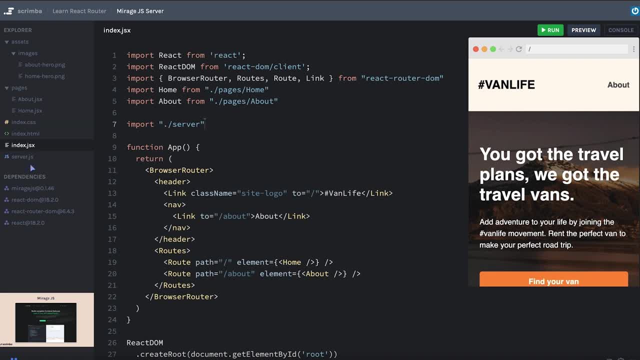 We'll get to see this in action in a little bit, but I just wanted to show you what I'm doing there with serverjs, so that didn't become confusing. Okay, that sets us up perfectly to now work on our vans page. So that's what we'll do next. 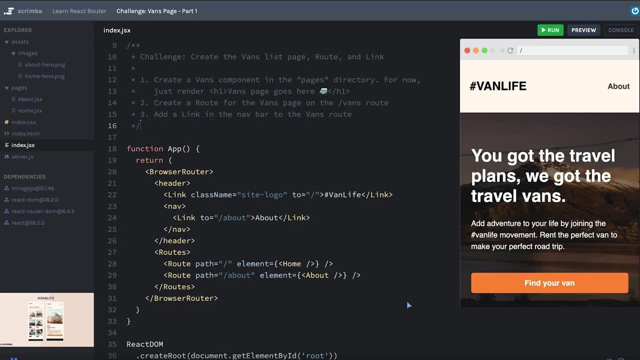 Okay, the next thing we're going to do is create the vans list page, And this won't really require you to do anything that you haven't learned yet. So I'm going to make this into a two part challenge. The first part is going to help you practice creating a new route: modifying the header. 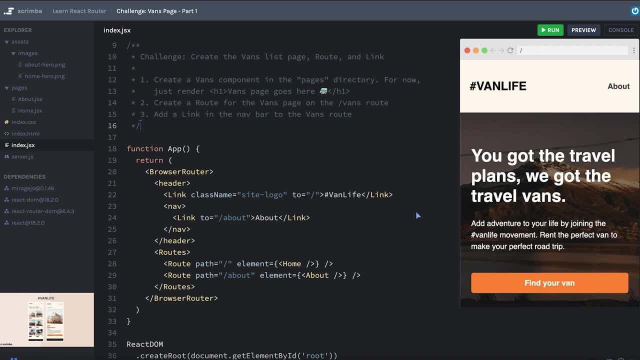 creating a new page, And the second part is going to require you to use a fetch request to get some data and use a map method to map over the data. All of this is kind of the introductory level react stuff that you should already know by 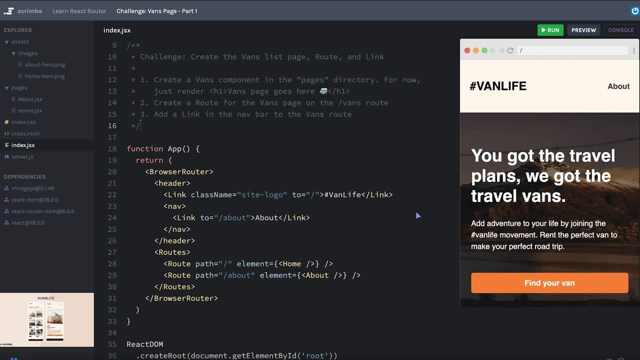 now, But let's not get too far ahead of ourselves. Let's start with part one. Again, your challenge is to create the vans list page that's going to be over in the pages directory, the route which is what will happen down here, and a link in the header so that 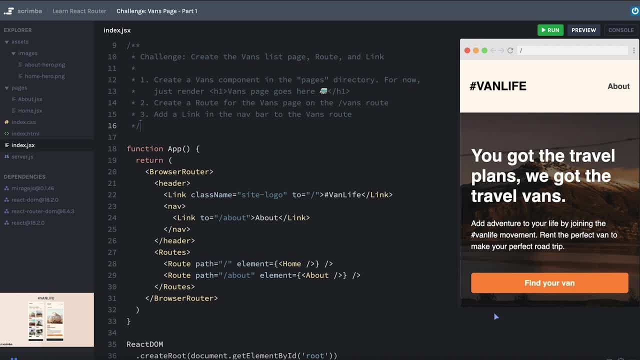 you can actually navigate to it Now, even though this is something that you have done recently. I really want you to practice this before just skipping ahead and watching me do it. However, if you get stuck, of course we will be going over this together. 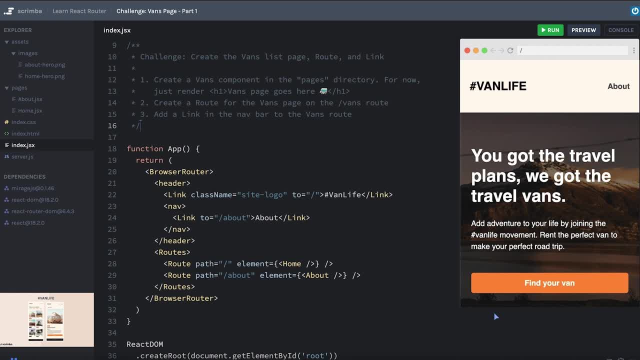 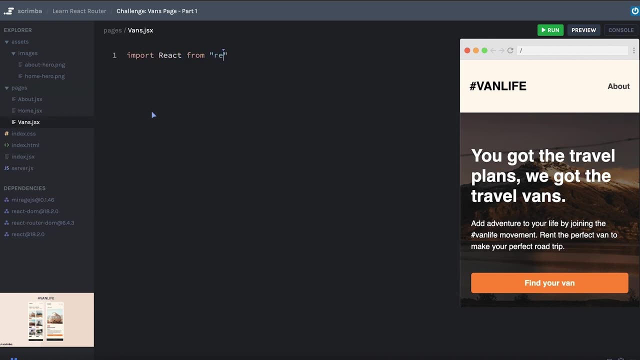 So pause now and work on this challenge. Let's start by creating the page. So I'll create a new file called vansjsx And we'll just do some of the regular setup stuff. Nothing fancy quite yet. We're going to get to that in the next challenge. 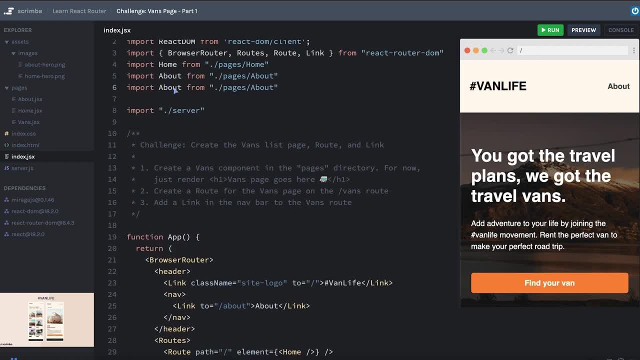 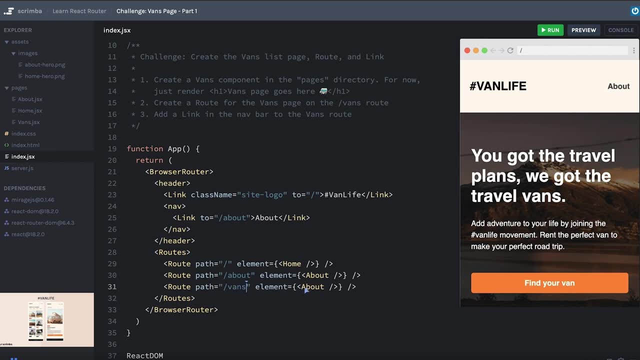 Then over here we need to import the vans page. We'll create a new route, So I'll just duplicate this line and change this to vans and this will render the vans element And then we will link to vans. so this will lead to slash vans vans, and I think that. 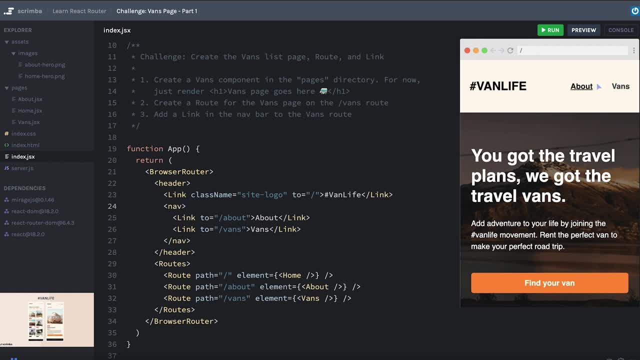 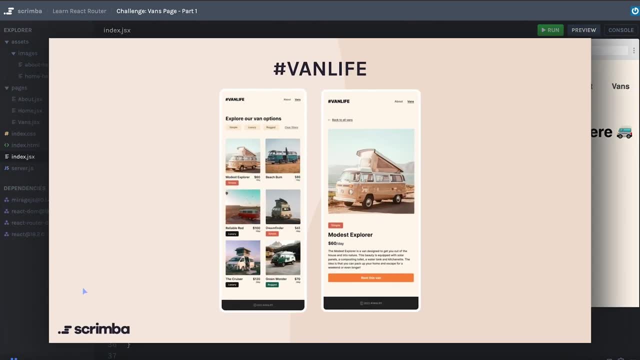 should be it. Let's hit save. Okay, we have our vans here and if we click it, vans page goes here. Awesome. Now comes the fun part. In the next challenge, we are going to actually pull in our data so that we can display the. 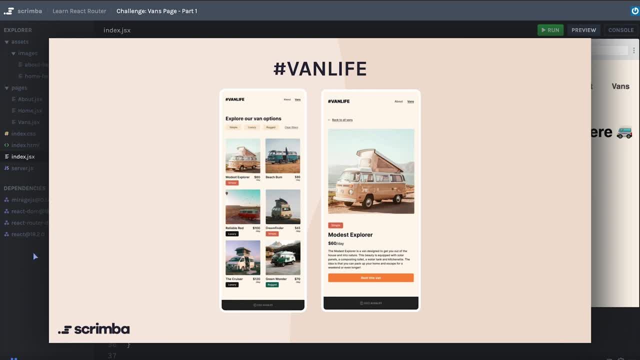 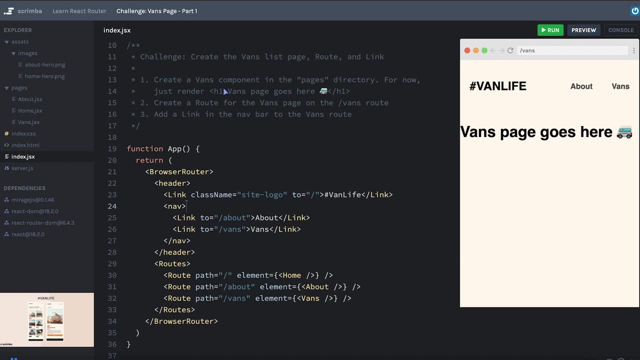 actual vans and the vans information. However, before plowing ahead, if you did struggle with this challenge, then just revert back to the video. If you're confused about these parts, then it will be more important that you kind of drill them in before you just plow ahead. 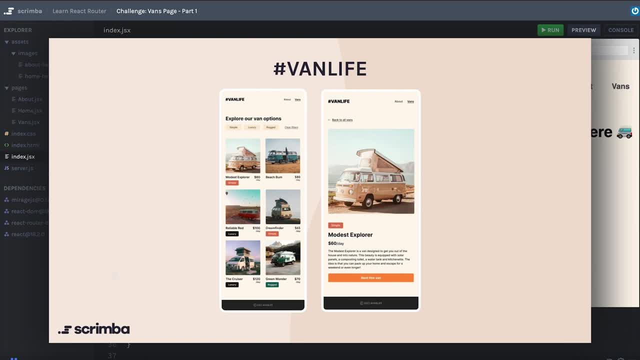 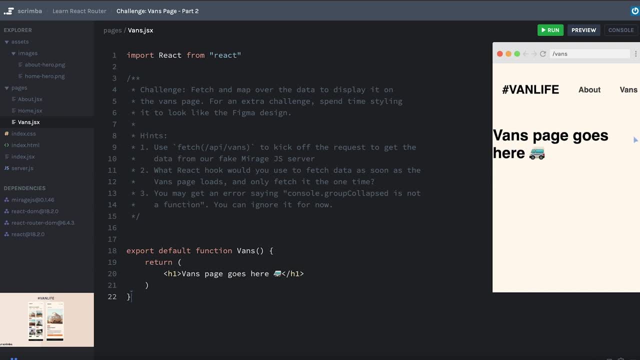 Okay, getting off my soapbox, let's work on part two of the challenge. Okay, this is the fun part of the challenge. This vans page goes here is nice and all, but we want to get the actual vans showing up on the page. 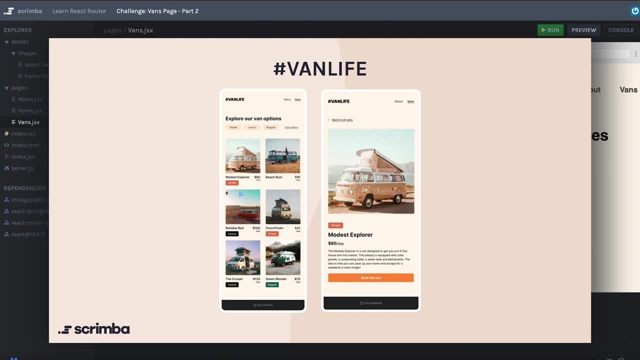 As per usual, you can click the design screenshots here to send you to the Figma design, in case you feel like spending the time Just like I did before. I'm not going to necessarily make you do that. I'm just going to do a magic snap of my fingers and we'll have the design already implemented. 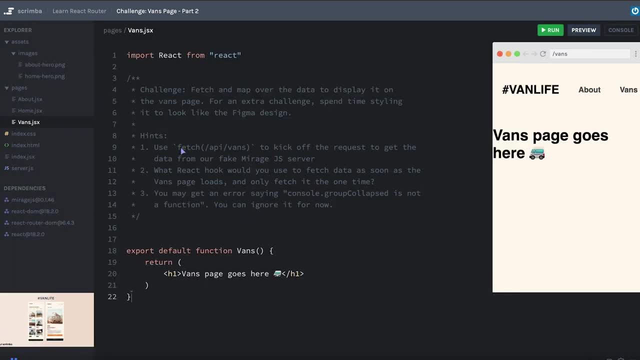 for us. So your challenge is written out here: You're going to use the fetch API from the web and you're going to fetch API vans. Let me put some quotes here, just to make sure that that's clear, that that's a string. 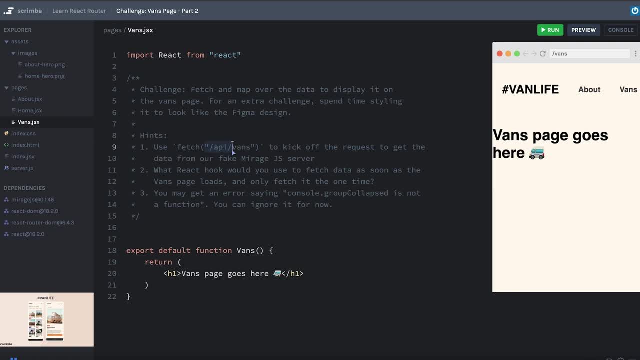 You're going to use the fetch API and you're going to fetch to slash API, slash vans. This might look a little strange. Yeah, doing your fetch requests to another server or another url somewhere, because usually you have something like https colon, slash, examplecom, slash api fans. but when you're fetching something, 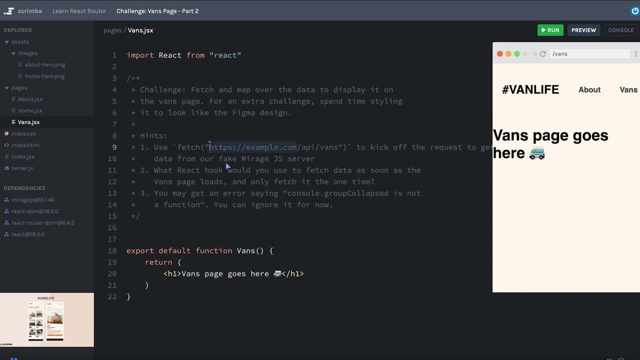 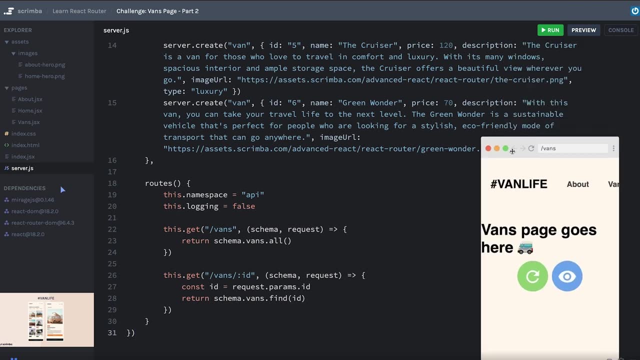 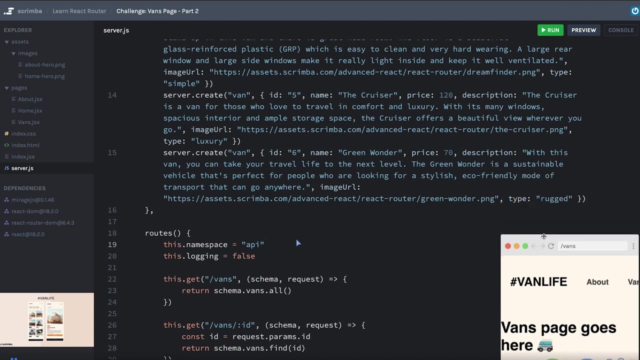 on the same domain as what your site is running on, then usually you only have to provide the relative path. now, remember, we have our kind of fake server running here with mirage js and you can see it says: thisnamespace is api. that means that all the requests are going to start with slash, api and then 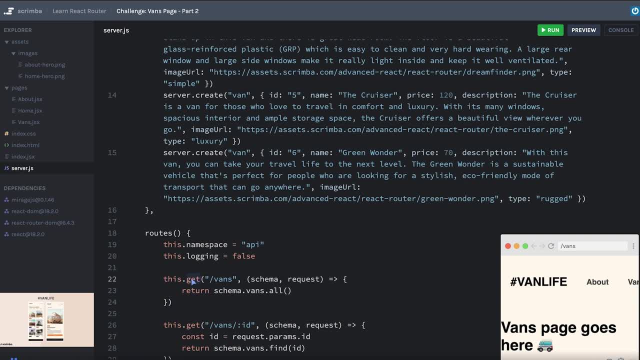 this function here is going to handle a get request to the slash api slash vans endpoint and all it does is return all the vans again. you don't need to understand this. this is not an important part for this course, but sometimes it's nice to poke around and see an inside look and hopefully that. 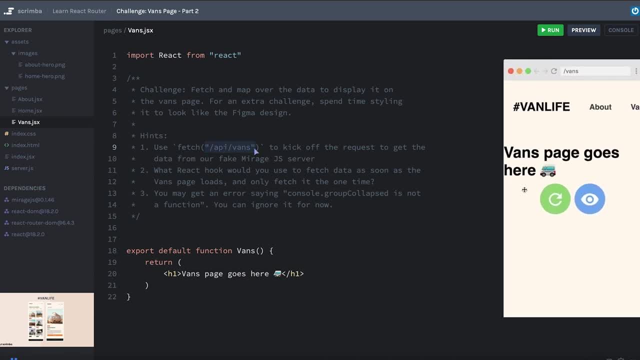 helps make sense of why this url- or what it doesn't really look like url, but why this url looks a little unique. so you'll kick off that request. you'll need to parse that json and turn it into data. you need to think about what react hook you would want to use to fetch the data as soon as the page. 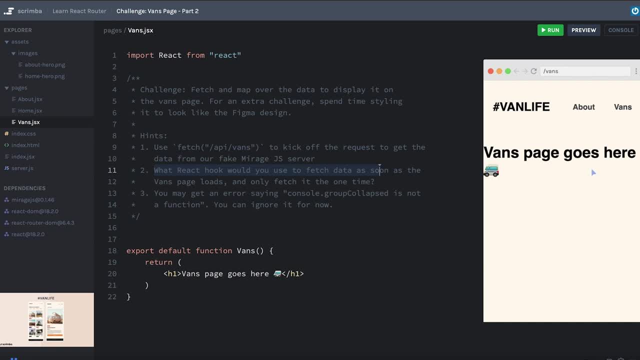 loads and how you would make it so that it only fetches it the one time and actually you know what. number three is no longer an issue, so i'm just gonna get rid of that now. parts of this challenge are going to require you to have prior knowledge in things like how to use the fetch api and where. 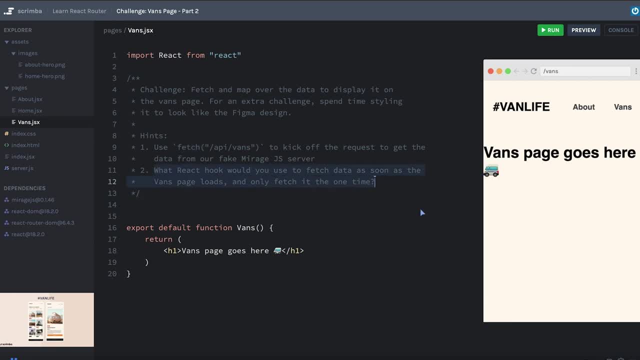 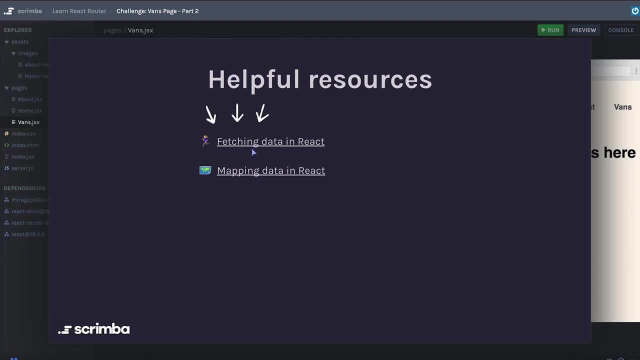 in react, you can kick off a request when the component mounts. if you're feeling a little rusty on that, that's completely okay. i've tried to include a couple helpful resources here. this is a link to the fetching data in react scrim that i taught in my introductory course, and the second one is how. 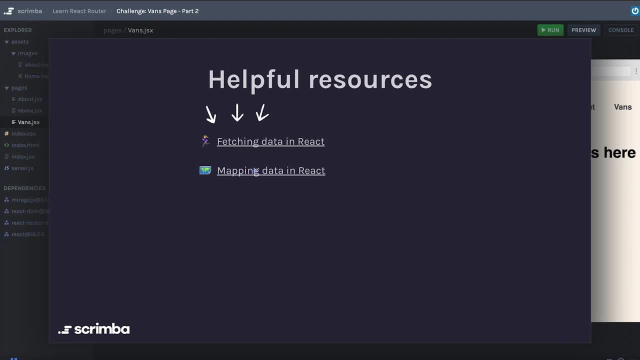 to take an array and to map over it using the dot map method and then how to actually display each of those as elements on the page. so feel free to check out those resources, brush up on some of those topics before trying to start this challenge here. okay, i think i've given you. 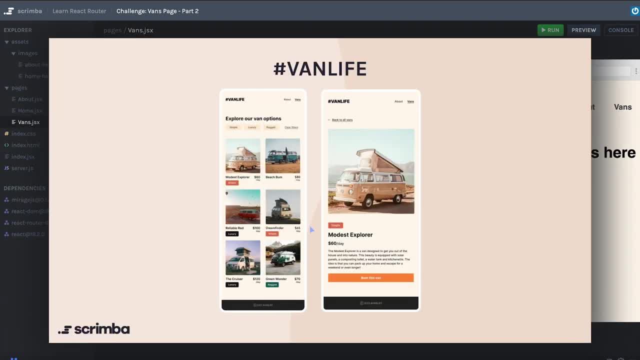 everything you need. again, if you don't necessarily feel like doing the css to make it all beautiful, i'm actually okay with that this time. just try to get each of the pieces of data displayed and if css is something that you feel rusty on or you want a little more practice with, then i would 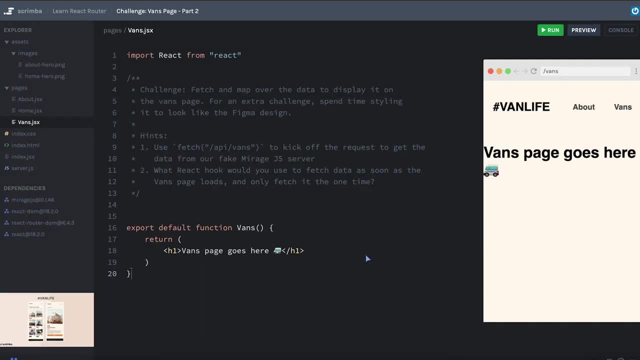 encourage you to do it. okay, enough of me talking. pause now and work on this challenge. i think i'm actually going to do these in backwards order. i'm going to start with number two, and the answer to this question is to use the use effect hook in react. now, the truth is, and this is something we're 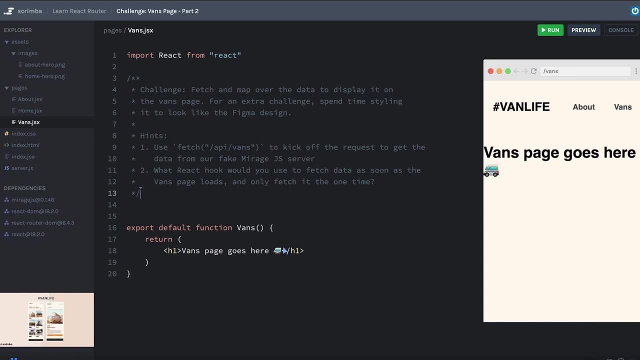 going to explore later on down the road or possibly in a different course. there's a bit of a movement away from trying to do your fetch requests for the data of a component in a use effect hook, but for now let's go ahead and use a react dot use effect. this takes two parameters. 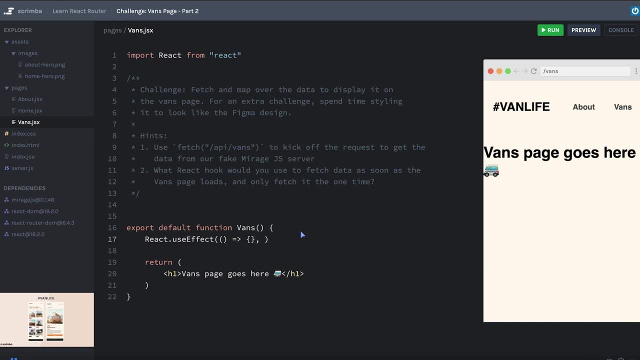 the first one is a function. the second parameter is an array of dependencies. in this case we have no dependencies, but it's important that i put this array here, otherwise our effect will run every single time. any state updates on our page at all inside the body of our function, we will. 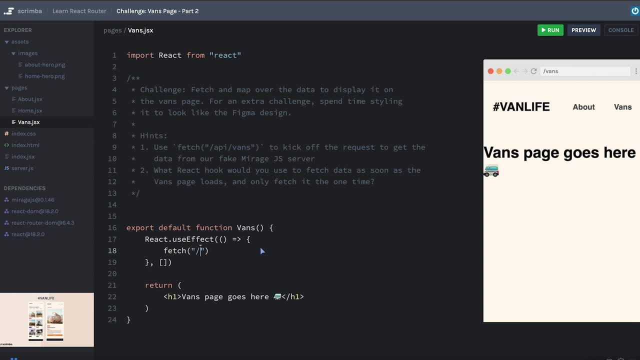 kick off our fetch request. so i'm going to say fetch, slash api, slash vans. and again, what our server is going to do, this fake server. it's going to intercept this fetch request instead of trying to actually make a fetch request out to some endpoint, probably here on scrimbacom. it's going. 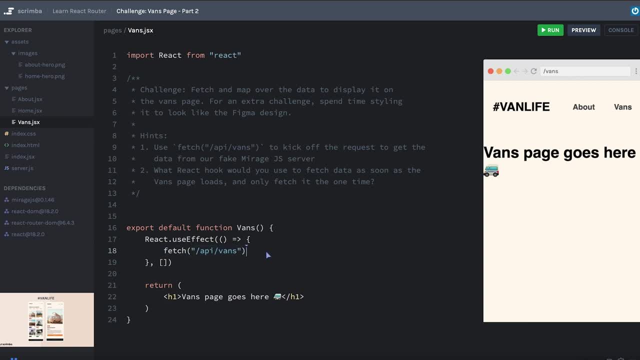 to intercept it and give back fake data. this fetch function: it returns a promise, and so i'm going to unpack that promise, which will come with a response, and we'll turn that into a javascript object or just regular javascript by taking the json part out of it. that returns a promise, so 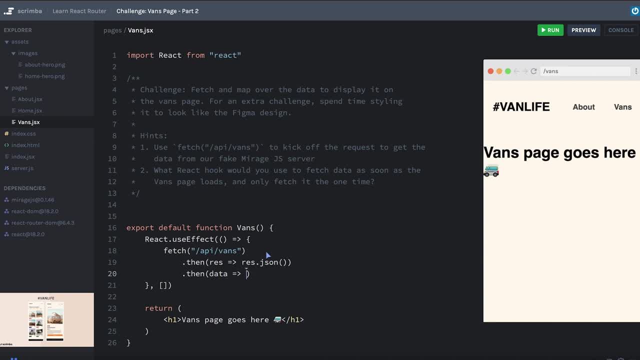 we will resolve that promise as well, and that is where we will finally have access to our data. i usually just like to console log our data for one, just to make sure things are working- we haven't made any mistakes along the way- but also to see the structure of the data. so we know. 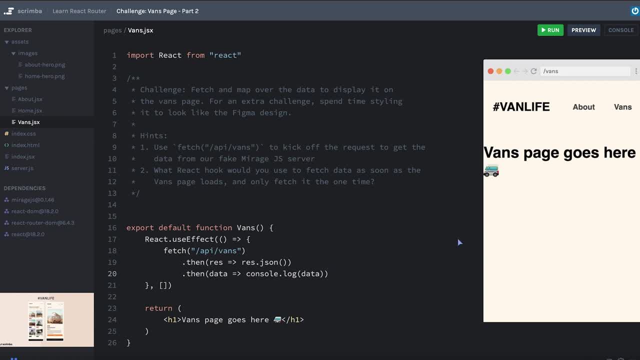 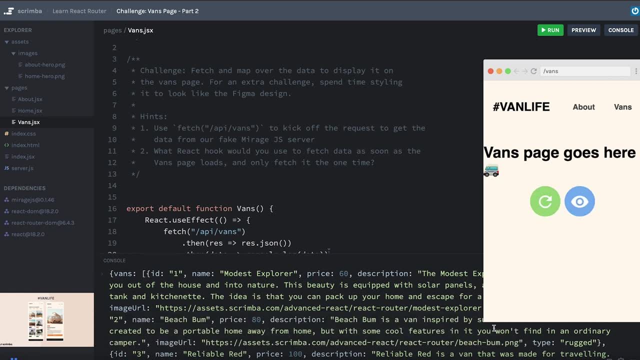 what it's going to look like, how we're going to access all the pieces of it. let's hit save and okay. well, we got something: console logging. it looks like it's an object with a vans property now, in this case, because we're choosing to kick off our request. 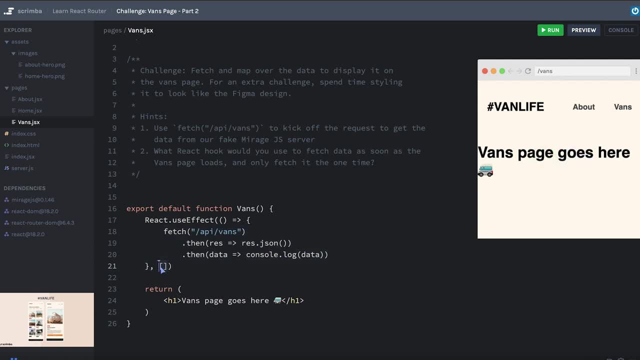 inside of a use effect and we're only kicking that request off one time, when the component first mounts. we need a place to save the data that we're pulling in, just so that, if anything were to change and this component got re-rendered, the data wouldn't just disappear. 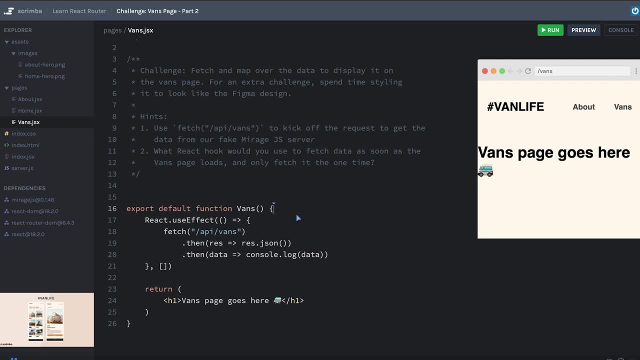 and you might remember that state is a place where data can survive the re-render cycle of a component. so we're going to create some state- let's call it maybe vans, and set vans is reactuse state. i'll start this as an empty array and then, instead of console logging, our 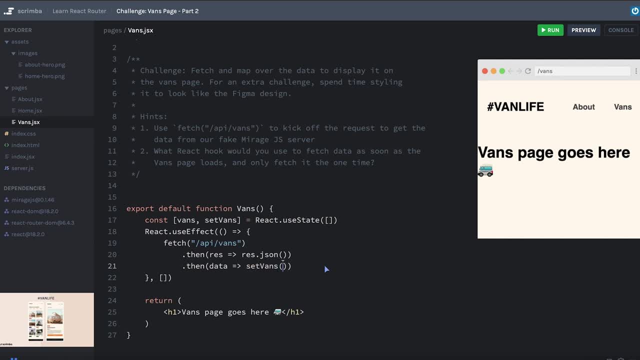 data. we will use set vans and we don't really care what it used to be, so i don't need the callback function. i'm just going to set it to data and then remember there's a property called dot vans. that's the one that actually has the array that we want. so if i console log vans. 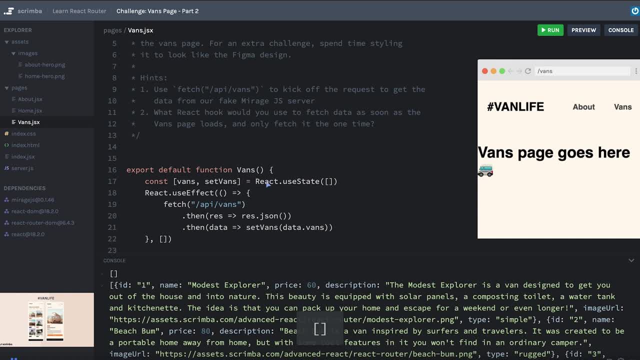 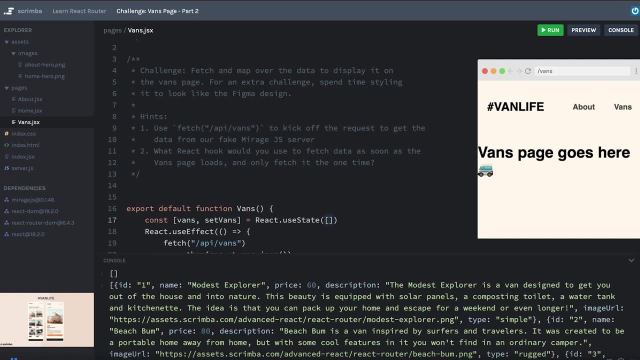 we'll hit save and first we get an empty array. that happens when the state is set as an empty array in the beginning, and then it turns into our array of van information from our fake server. awesome, actually, you know what. while we have this, still console logging, i'm going to grab. 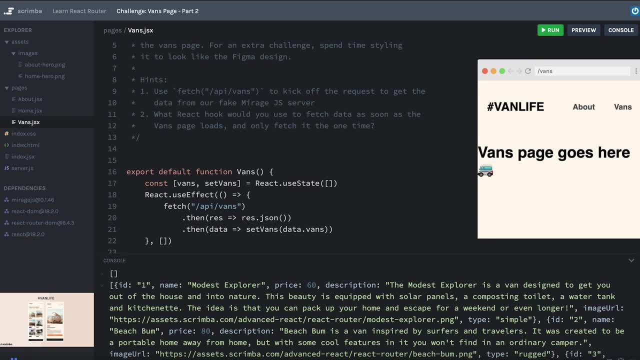 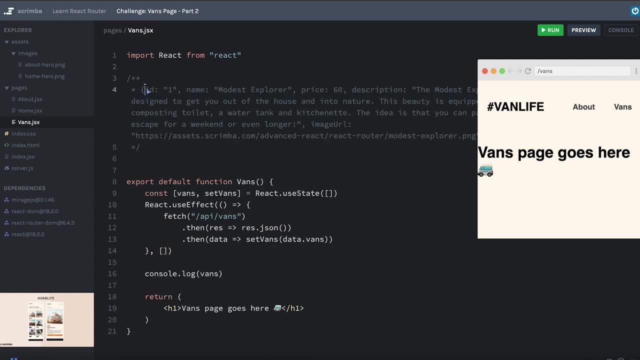 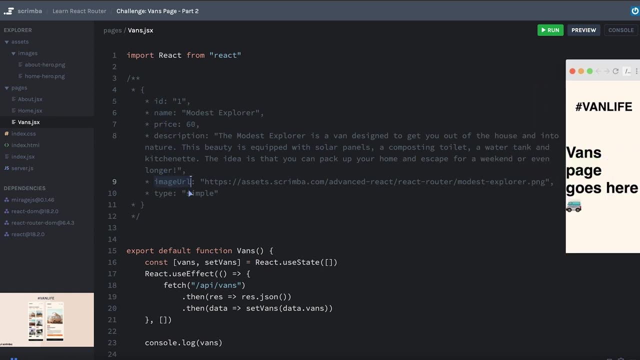 one of the objects of our vans, just so we know what properties it has. let me get rid of our challenge text. instead, i'm going to put in the properties of our van. okay, so our van has an id, a name, a price, a description, an image, url and a type. so i'm going to turn our array of raw data. 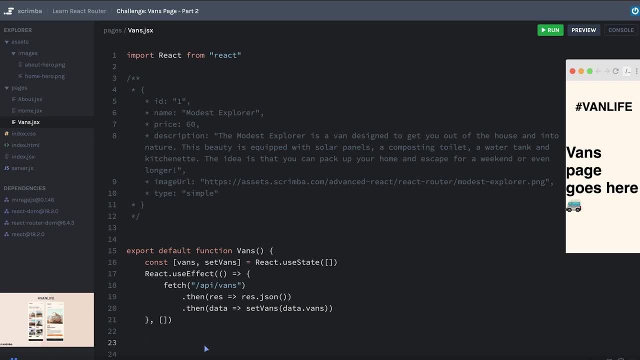 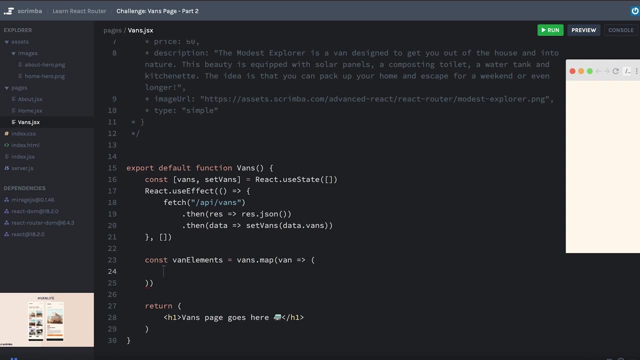 into an array of elements that we can display on the page by using the map methods, so maybe i'll call this van elements- is equal to vansmap, and for each van we are going to render- and you know what this is, where normally we would just start creating one van element that we want to show on. 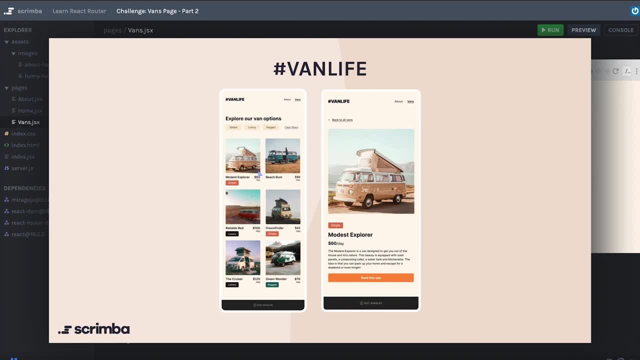 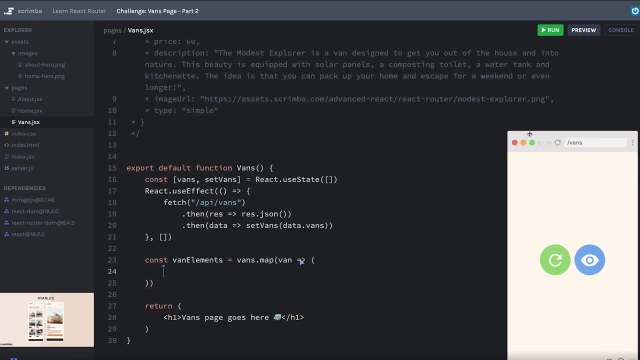 the page. so one of these lines here is going to be the van element, and then we're going to go ahead and create another one of these little sections here. for the sake of time, i'm going to paste in what i've already created, since it won't provide a whole lot to this lesson or challenge. 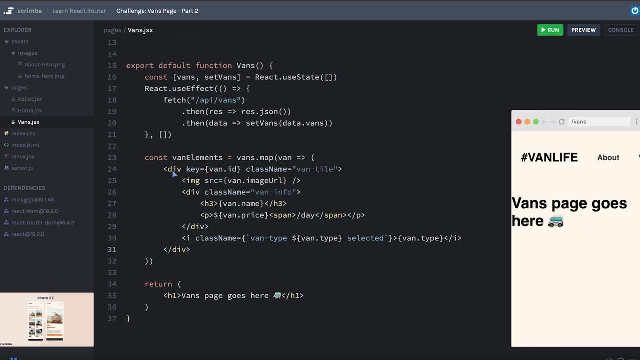 to have you watch me go through each little piece like that, okay, so what you can see is just a div that has the elements that we see in the tile of one of these vans, and since we're doing a map, it will end up being a tile for each one of the vans in our database and there's a couple class names. 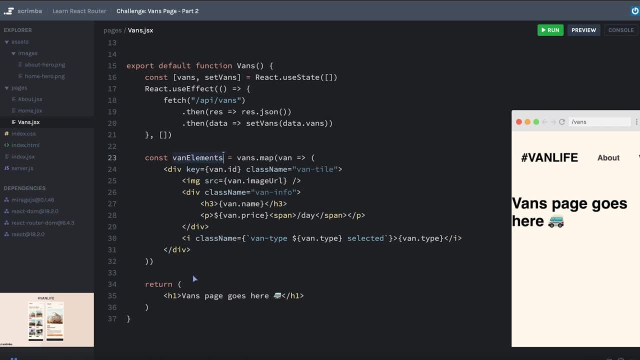 that are not here yet. let's actually put van elements onto our page first, and then we will go ahead and create another one for each one of these vans, and that's the css. so instead of our h1 that says vans page goes here. we'll have. in fact, let's use a fragment just because we don't. 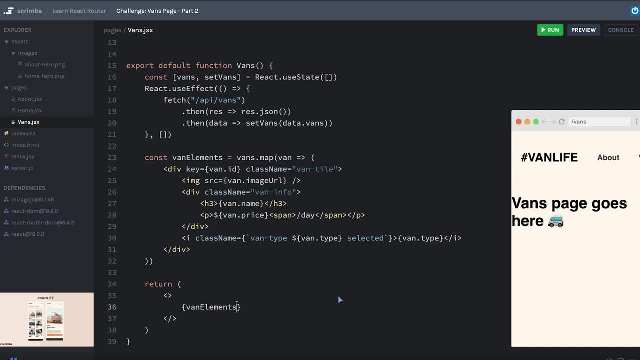 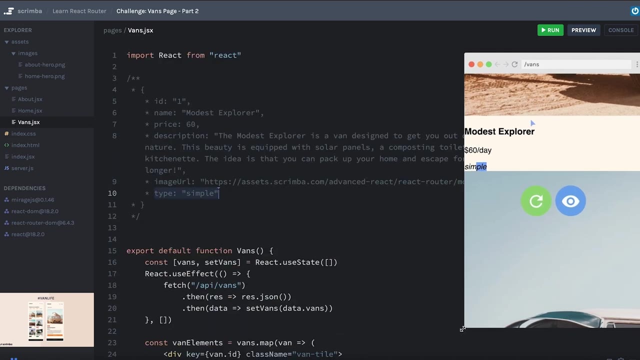 need to necessarily add a bunch of more elements and we will just put our van elements here and let's see where we end up. okay, well, that's a huge picture, but we've got our picture and it's got the name of the van, the price, and this is the style, or rather the type i think is what it was called. yeah, 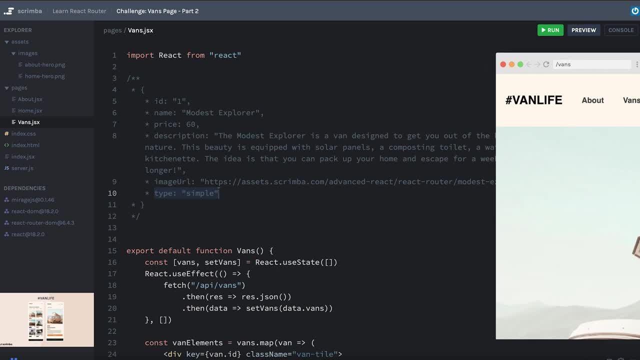 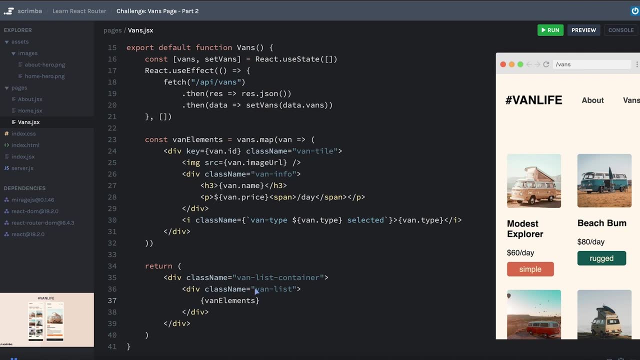 we have our vans- awesome. let me go ahead and just use the magic of editing to make this look a little nicer and just like that our css is applied. i had forgotten that we wanted a list container and then we have our list itself, just for styling purposes. so i got rid of our fragment and actually 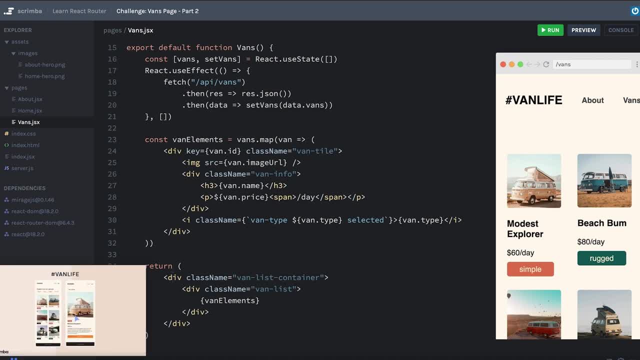 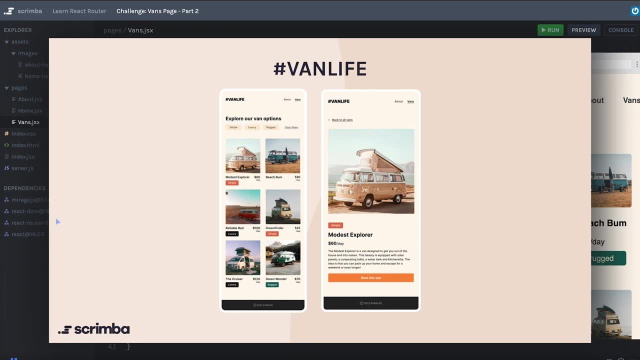 put in a div so that it could have a class name, and actually we're missing something from the. well, we're missing a few things from the design, but one that's really easy right now is this: looks like maybe an h1 that says explore our van options. so i'm going to 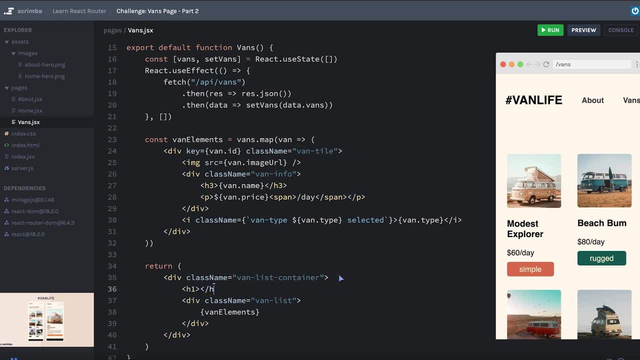 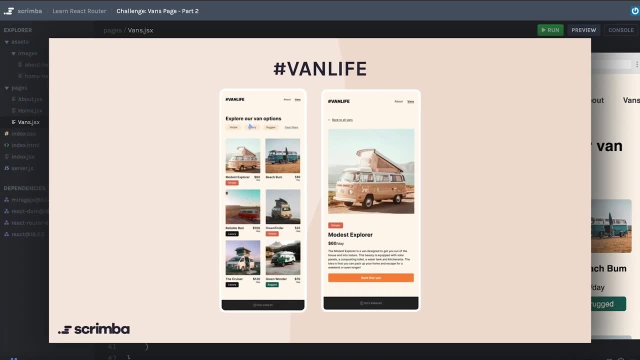 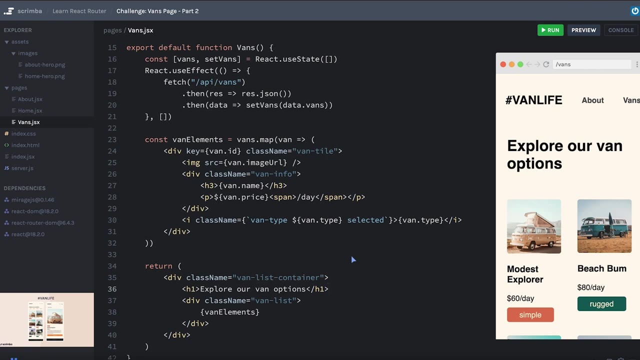 stuff that just right inside of our tile, here we'll have our h1 that says: explore our van options to save. okay, cool, a little step closer. we still have some other work to do, like these buttons, the footer and so forth, but we'll get to that. okay, man, that was a lot of work, but hopefully. 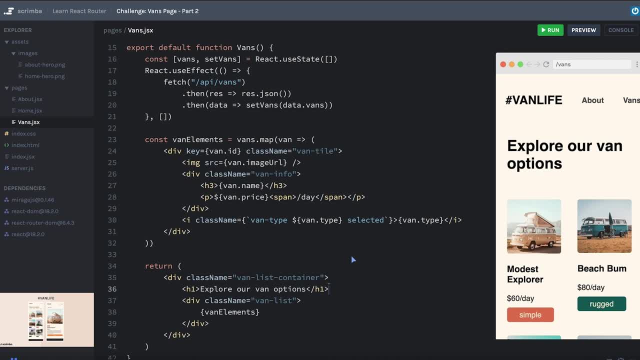 this is mostly just review from previous lessons that you have learned about react, but this does lead us to what we're going to learn next, and that has to do with nested routes, because what i want to do is i want to make sure that i have all of these tiles to be clickable basically anywhere. 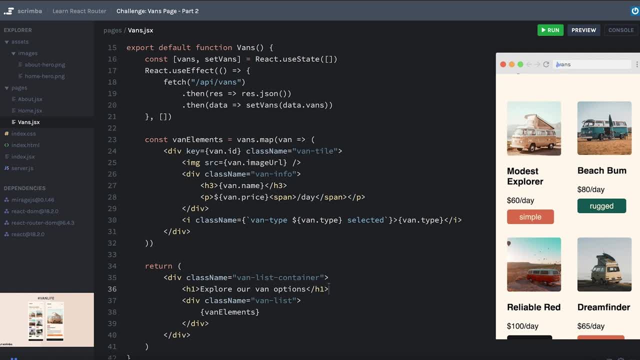 on this tile and i want clicking each one of these tiles to take me to a nested route. so it will be slash, vans, slash, and in our case we're going to keep it simple and just use the id of the van. so slash 1 will send us to a detail page of this modest explorer van, because that's the one with. 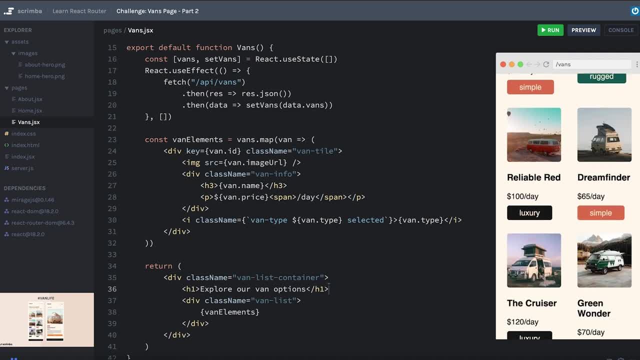 the id of 1.. slash 2 would take us to a detail page of the beach bum, van and so forth. there's a couple fun considerations to keep in mind when we're going to do that. so that's what we're going to tackle next. 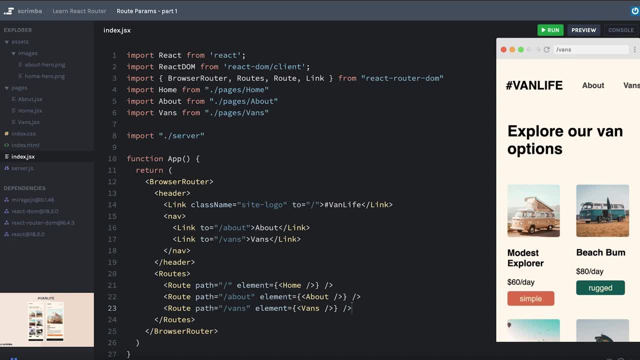 everything we've learned so far about react router, you could say, is like the meat of react router. what with the browser router, the routes, these individual routes that we have, and the link that allows you to navigate between one and the other. everything else that we'll learn is sort of the 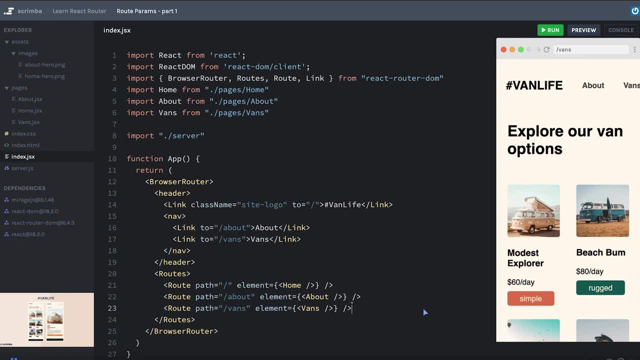 i guess you could call it the vegetables of this plate. they're really going to round out our experience and they're going to allow us to do some pretty cool things with react router. we'll spend the next couple lessons on how to use react router to do some pretty cool things with react. 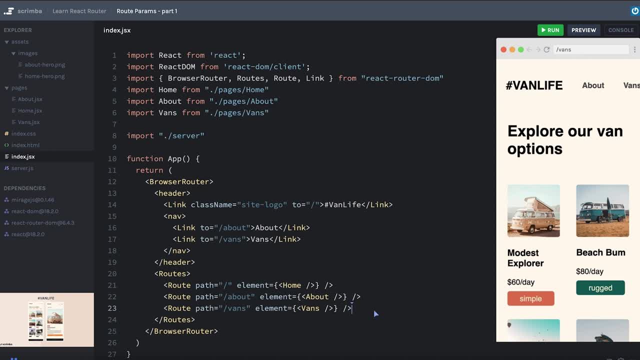 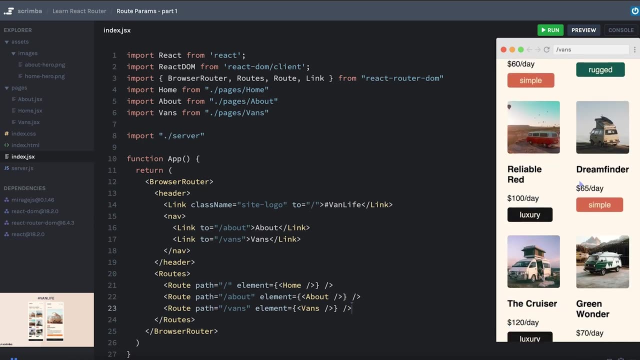 router. we'll spend the next couple lessons on how to use react router, to do some pretty cool ideas with react router, and then moving on, we'll focus on basic. here we have the list page: clicking on one of them sends us to the detail page And in 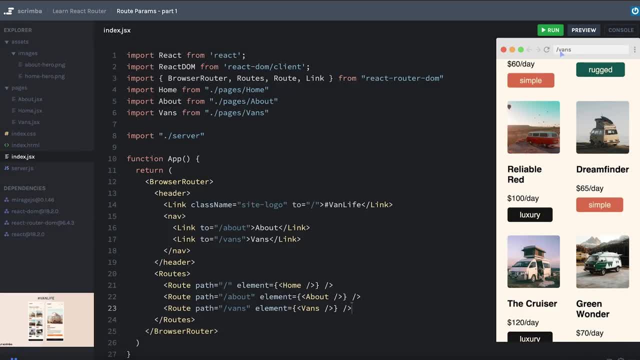 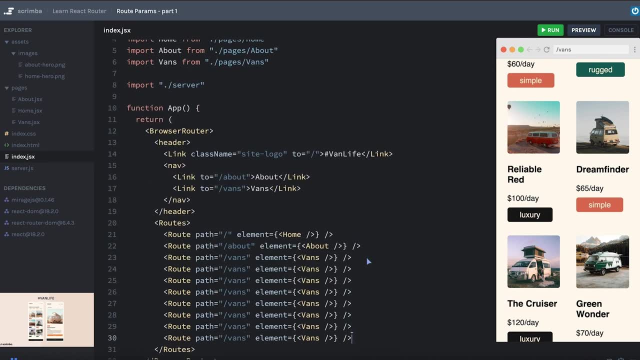 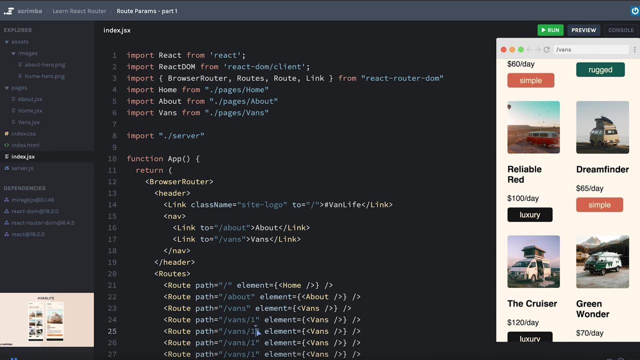 our case, we decided we want this detail page to have a route of slash vans, slash and then the ID number of the van. But we don't want to go through and create a new route for every one of the vans in our data and have something like slash vans, slash, and then slash one, slash. 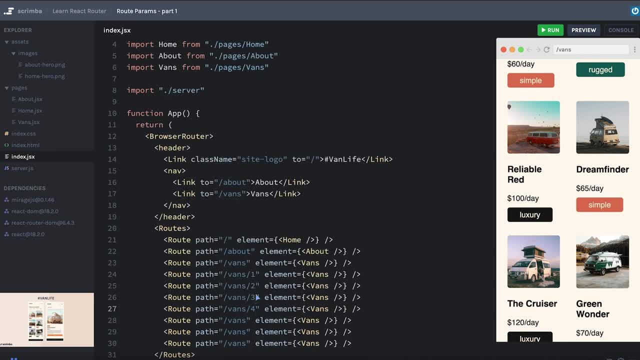 two slash three, slash four. we wouldn't want to manually create that because, well, it's just not maintainable. If we were to add more vans to our list, then we wouldn't also want to have to come in here and create new routes, create separate elements and so forth. So 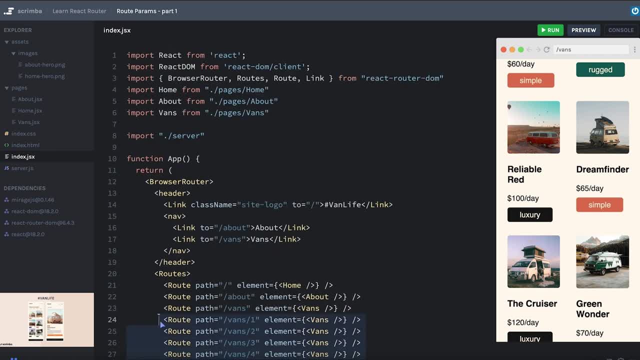 this is where route params come in. When we're defining our routes, we get rid of all these extra ones When we're defining our routes. I'm going to copy this one just as a starting point, And then, instead of saying, slash, vans, slash, and then a specific dedicated ID number, 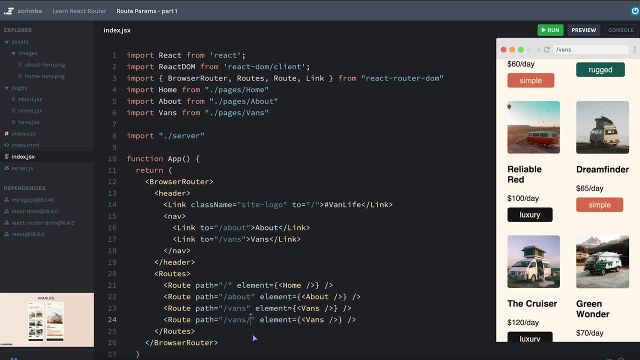 or some other kind of text. we're going to use a colon and then we're going to give it sort of a variable name. In this case let's call it ID. we get to choose whatever we want, But let's call it ID because we will put the ID of the fan in this spot, Because 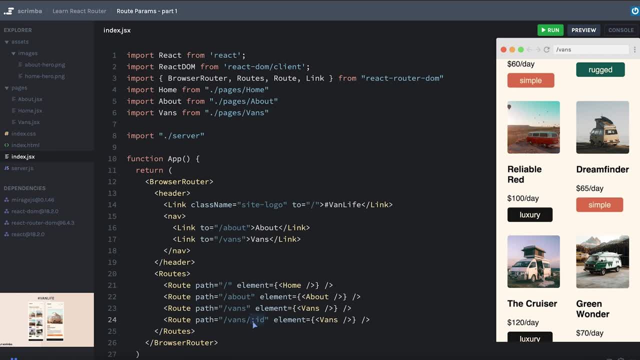 the colon sort of turns this into a variable. it means that we can reuse this one route definition for every detail page that we want to create, no matter what the ID is going to be. Now we need to change vans, because this right now is just leading us to the same vans. 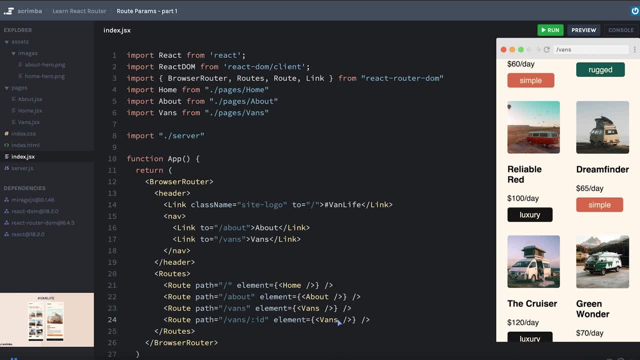 list page. So instead we're going to create a van detail page. So I'll whip that together really fast. we'll go to pages, create a new file, call it van detail dot JSX, And I'll just set this up really quick. Okay, like we did before, just. 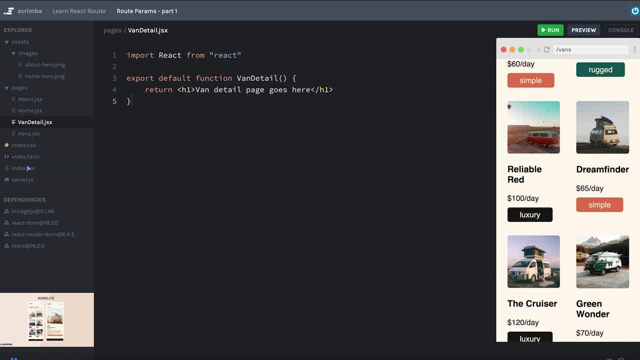 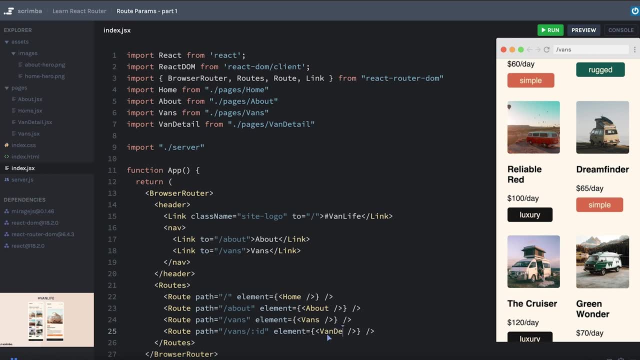 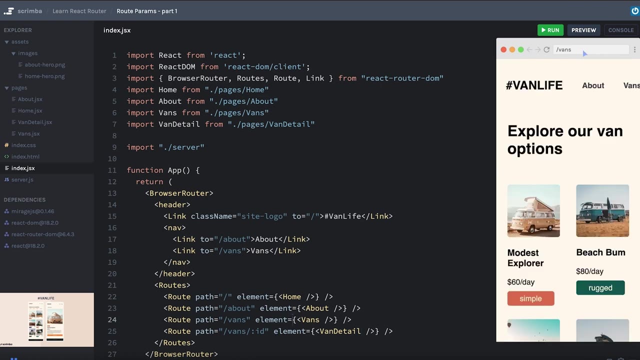 an h1 that says the van detail page goes here, we will go back to our index page, import it And instead of rendering the vans here, we will render van detail, And we don't have a link yet to send us there. So let me hit refresh And I'll just start by typing in: 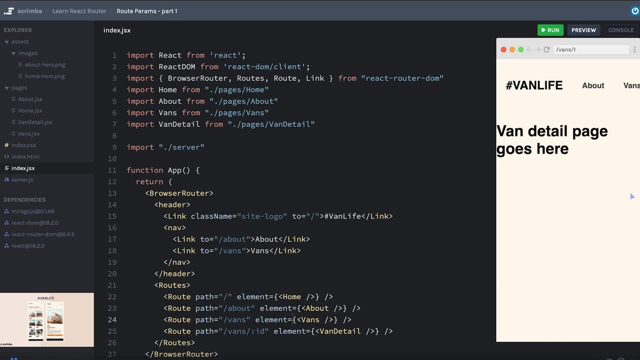 in the URL, slash one and hit enter And cool. that sent us to the van detail page. Now we'll notice that this doesn't say anything about one, it just says colon ID. So I could change this to slash 42. Even though we don't really have a van with an ID of 42, I could change. 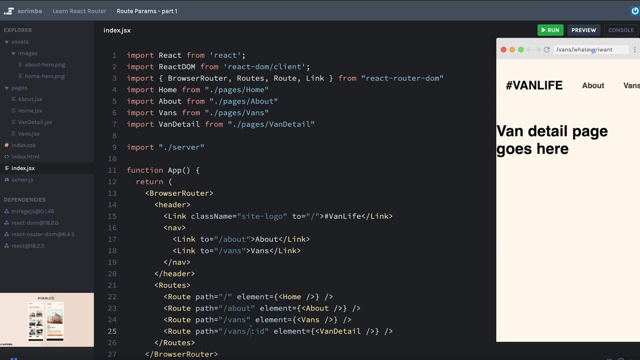 this to whatever I want and hit enter, and it really doesn't care. The colon is just saying there's going to be something here. I don't know what it is, but it's going to be something. So there's two more things that we need to do here. First of all, we need to create a 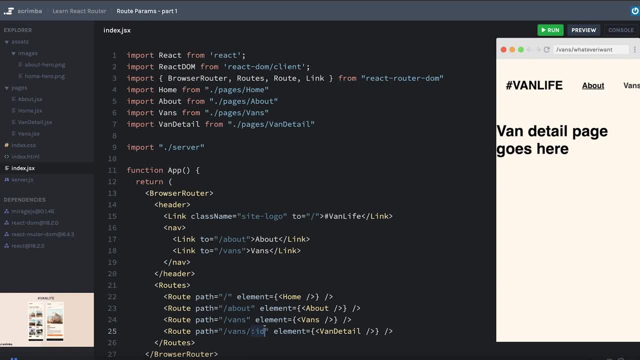 vans We need to hook together in order for this to work. The first is from my vans page. I want to have each of these vans send the user, when it gets clicked to slash vans, slash and then the ID of that specific van, And then in the van detail page: we want some. 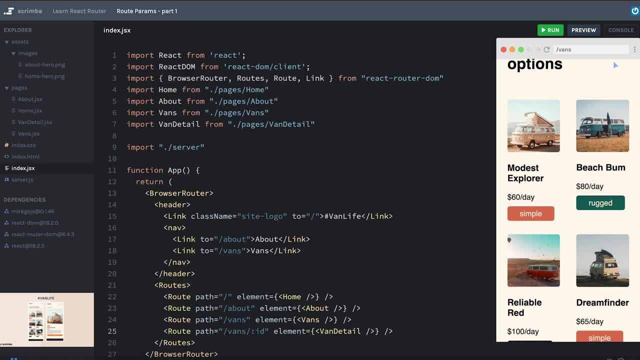 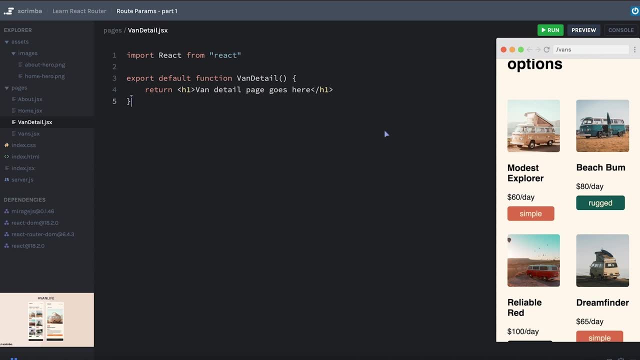 way that we can access the ID that is in the URL after slash vans And that way from the van detail page we can grab whatever the ID is from the URL. make a get request to our server to grab the vans And then we can go back to the vans page and we can create. 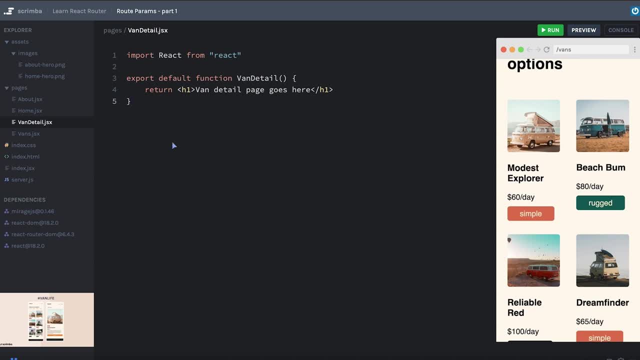 a get request to our server. to grab a get request to our server. to grab a get request to our server. So we're just going to grab the detailed information for that one specific van and then go through the process of displaying the detailed information for that one specific van, like you see here. 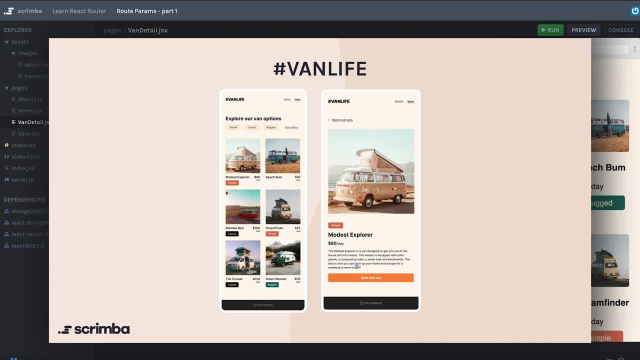 Really, I think the only information missing from the list page is this description down here. but still, for now, what we'll do is whole extra get requests to get the detailed information for this van. So for the sake of breaking this up a little bit, let's tackle. 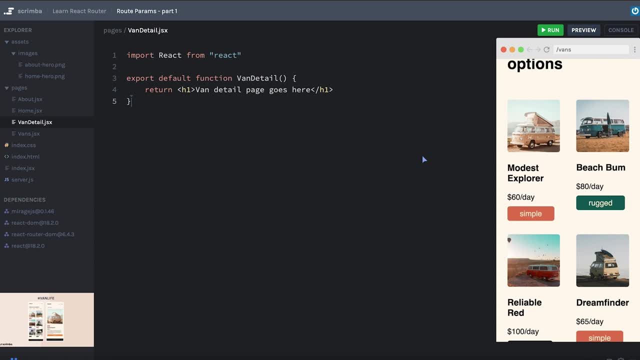 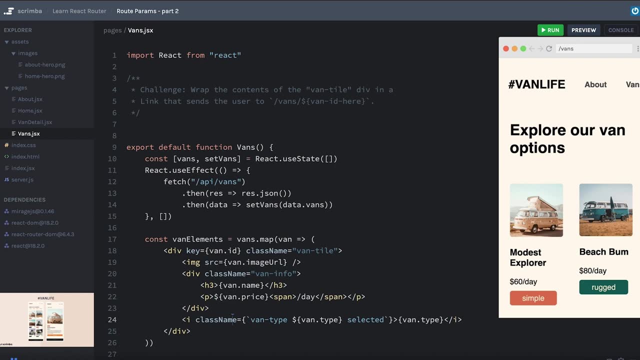 those two different parts in separate scripts, So that's what we'll start with next, The first part of this. This involves a challenge that you should already be able to complete without learning anything new. Each one of our vans is listed in what we're calling a van tile here on this div, and we 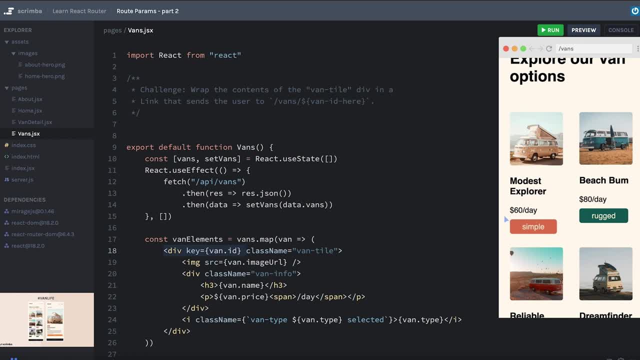 want to make it so that if the user clicks anywhere at all within the contents of this div, that they'll be sent to the vans slash and then the ID of the van. So your challenge is to wrap all of the contents of this div in a link from React Router DOM. 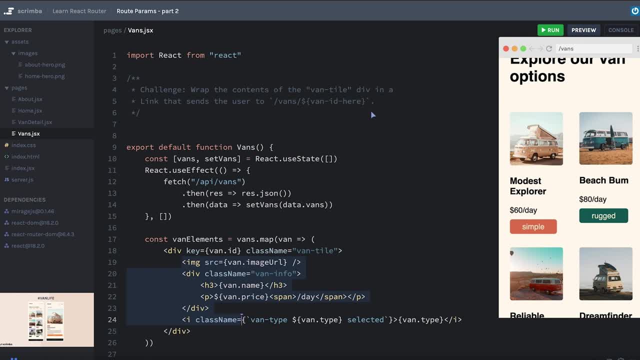 and have it send the user to that page. You'll know that you've completed it when it sends them to that van detail page goes here page. So pause now and work on this challenge. Okay, first we need to import link from React Router DOM and then we will just wrap everything. 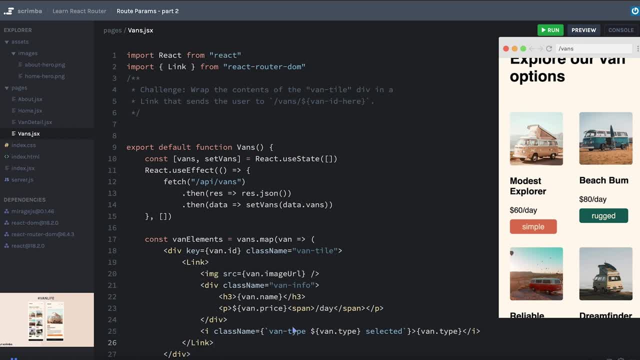 in a link. We'll indent that. And then the last thing is we need to send them to, And I'm going to use string interpolation here so I can say: slash, vans, slash. and then, because we're inside of the loop where we're mapping over the vans, we have access to each. 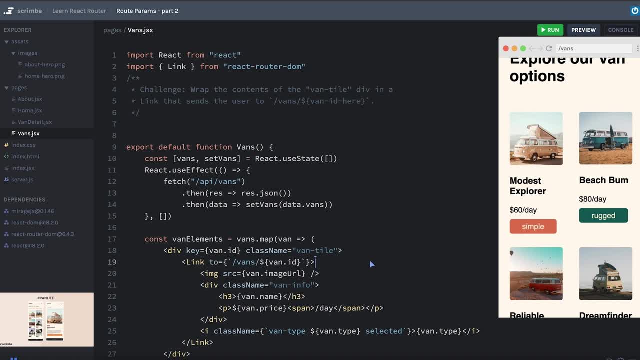 individual van and we'll say vanid, Okay, let's hit save, Let's click on reliable red, And of course it really doesn't matter. but we can see in the URL in the mini browser that it sent us to slash vans, slash three, because reliable red had an ID of three. 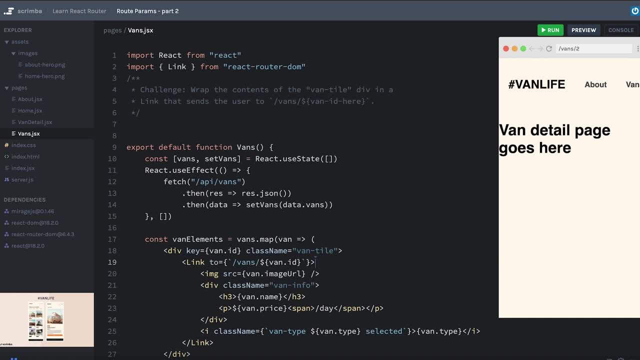 We can go back to beach bum, which should be two, and there it is Now. of course, This van detail page is not very descriptive. It's not really doing anything important. Next, we need to make it so that the detail page can grab information about that specific. 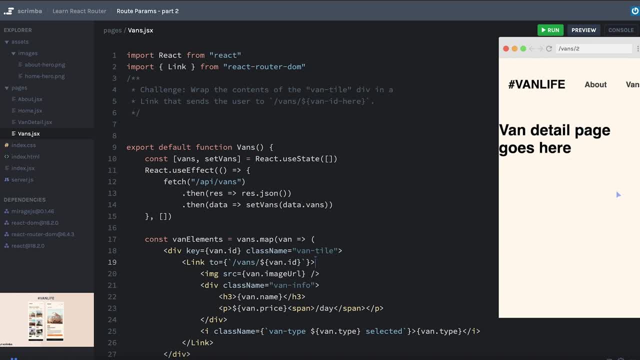 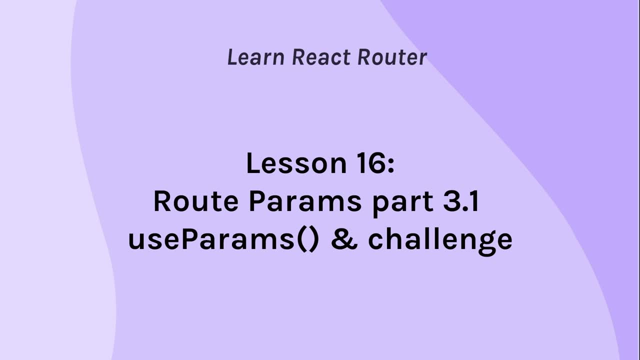 van that they clicked on, so we can display everything we need to display here. To do that, we need to learn about something called use params, So that's what we'll learn next. Let's take a second to look back at what we've done, just as a reminder before we move on. 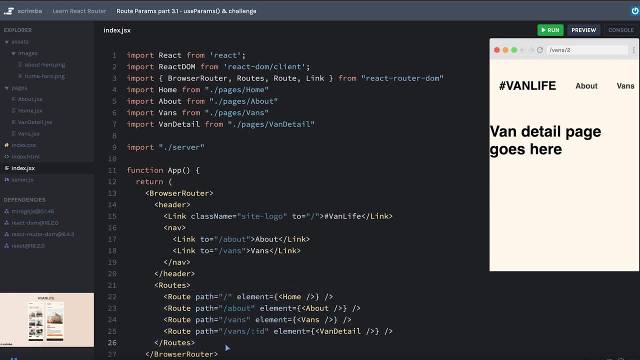 In our app component, where we have our route definitions, we created a route that has a parameter as part of its path that's identified by the colon in front of this part of the path. By putting a colon here, it tells React Router that this isn't going to be the literal text. 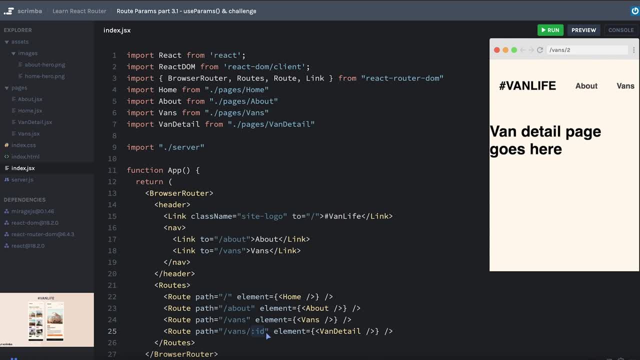 colon ID, but instead there's going to be something here in its place. I like to think of it as a variable inside of our path. So whenever slash vans slash anything is in the URL, then it will load the van detail element here. 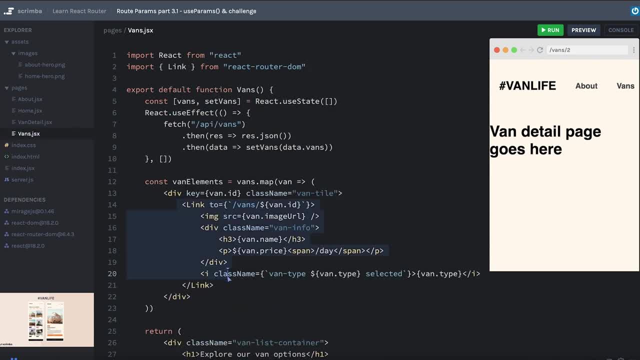 Then we set it up so that in our vans page We link to the Okay, Slash vans slash and then whatever the ID of that specific van that we clicked on in the vans page. By doing that it takes us over to slash vans, slash two, in this case, because we clicked 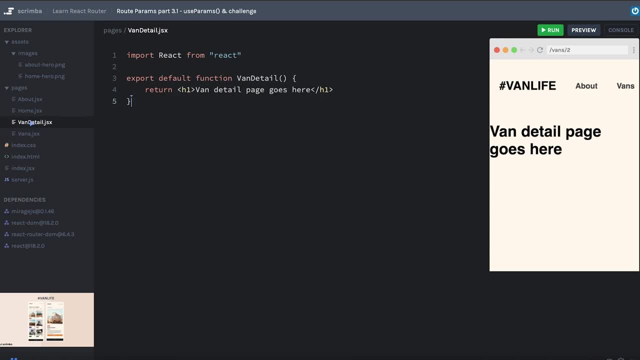 the van with the ID of two and our next task is to make it so that in the van detail page it's able to grab the two out of the URL and then go and get the specific information about this one van that we're supposed to be looking at. 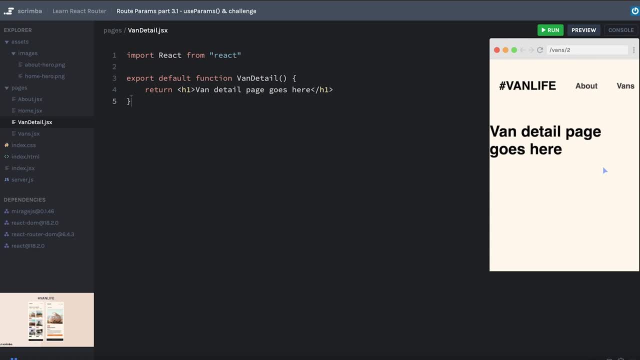 There's a bunch of different ways that we could do this and we're going to see some optimization that we can do. For example, right now, if we go to the vans page, you'll see it delays for a second because it's doing another fetch request, going to get all of the van information. 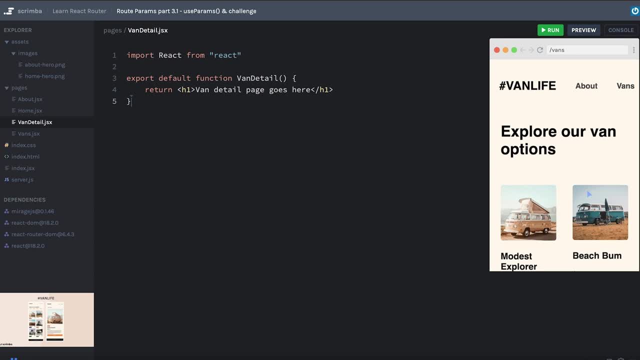 So really we should be caching that somewhere so that we can get that information much quicker, And then there's probably a better way that we can handle getting the detail information rather than always doing another get request, Since we have all the information when we get all the vans in the first place. the point: 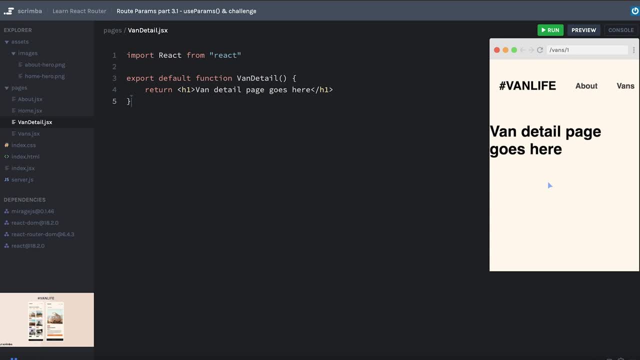 is. there's a lot of different ways to organize things to make it have better performance, But for the sake of focusing on our learning with React Router, we're going to keep it simple. React Router provides us a tool called use params, which allows us to grab any of the 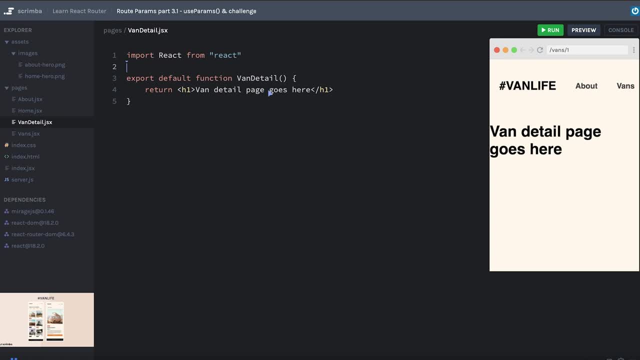 parameters that we have in our URL And that's a tool we will need to import. So I'm going to import use params from React Router DOM and inside the body of my component I'm going to grab the params. So we'll call it const params equals and then we'll call use params. 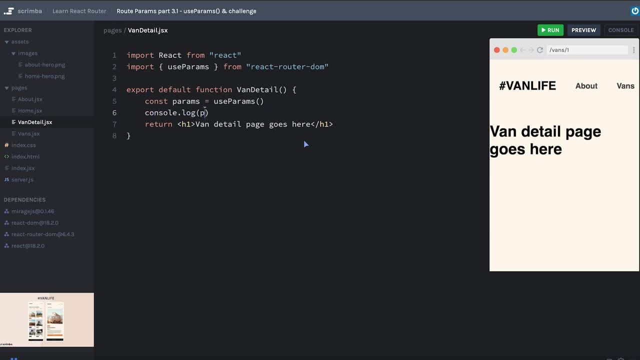 And let's go ahead and just console log the params. This function will run whenever the van detail component is mounted. So I'll open up the console, we'll hit save And cool. we see that we get an object that has an ID property. I want you to pause and. 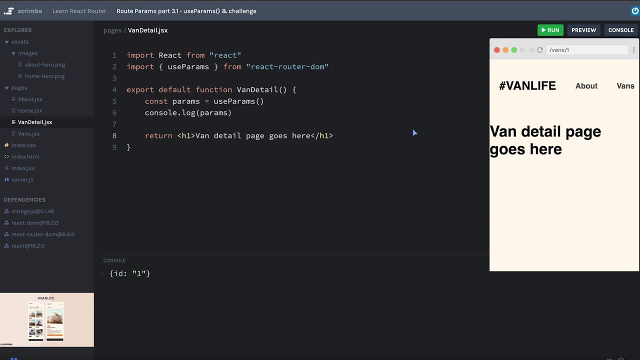 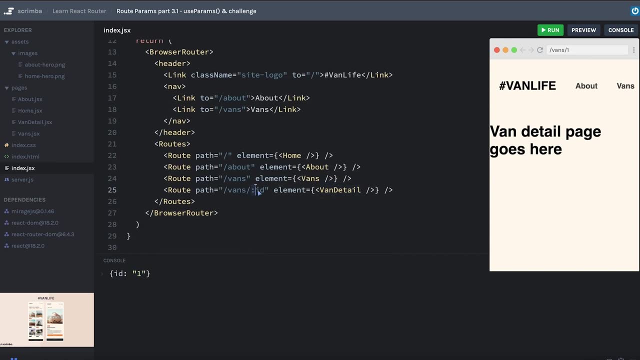 think for a second. where did ID come from? Remember, over in our index JS, after the colon, we put this colon, ID React Router will look at any sections of the path that have a colon before it And it will add that, And then we can see that it has the key in the key value pair in the object that we get. 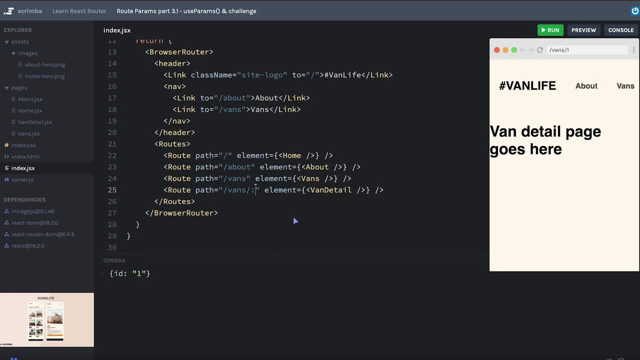 from use params. So if I were to change ID to blah blah and hit save, we'll see that now our object has a key of blah blah. That's too silly, Let's go back to ID. Also, it's important to note that the reason that React Router chose an object instead, 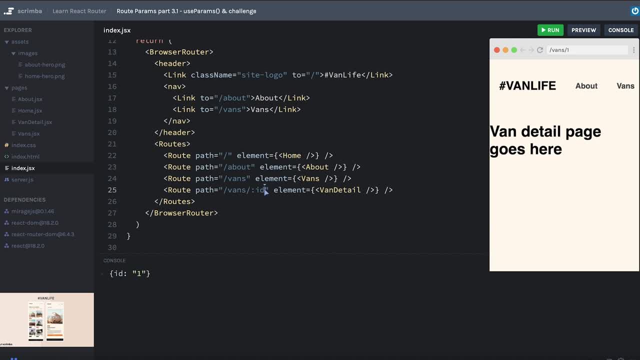 of just giving you the value of what's there. because you can have multiple params, there's nothing stopping me from using slash vans, slash ID, slash rent, maybe like a rent page that's nested inside of the detail page. Now, if I do this, my URL currently isn't going to match anymore. 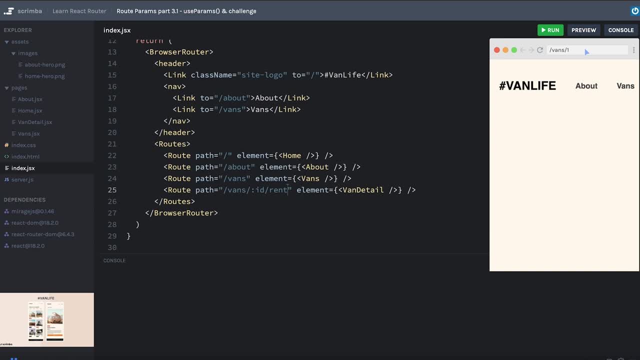 So I need to update it. we'll say slash van, slash one, slash rent. One really quick side note is there's nothing stopping us from having multiple params inside of our URL, So I could, after slash colon ID, I could add another slash and say colon. I don't know. 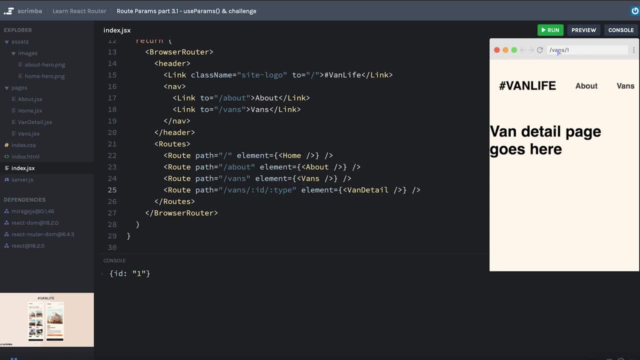 maybe type, And when I hit save, of course this path that we currently see isn't going to match anything on here, So it's going to disappear. But let's say we add to our URL slash rugged and hit enter, And now we can see the van detail pages back up, because this path is now matching again. 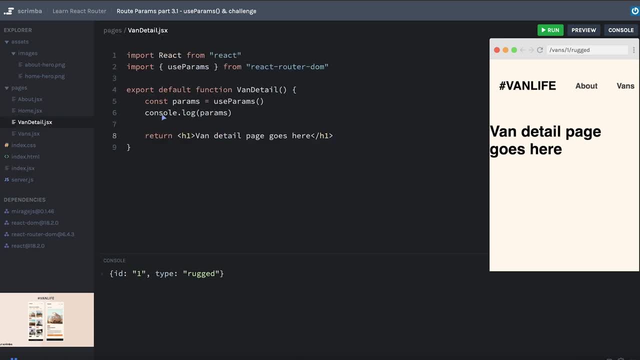 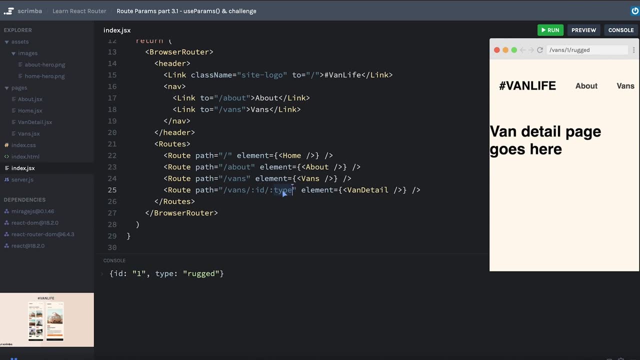 And also the params that we're pulling in the van detail page and we're console logging over here is now including both the ID and the type parameter. For our needs we won't be needing multiple parameters, But I just wanted to make that clear. 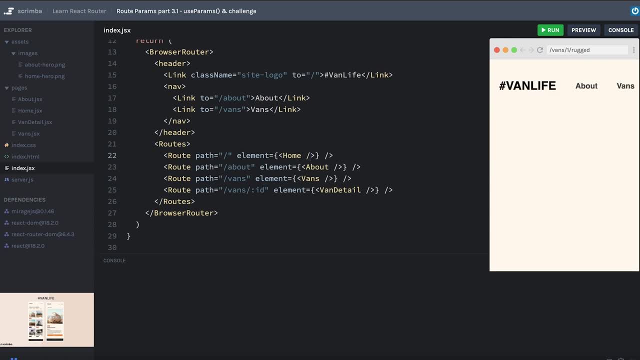 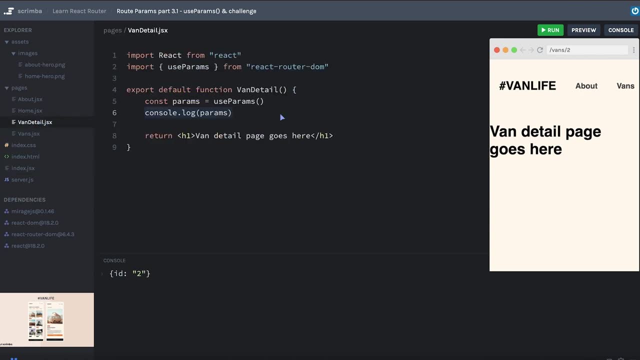 So let's go back, we'll go to. well, let's hit save, we'll go to vans. back to our vans. we'll do number two this time. And cool, our parameters are coming through, as we saw before, And now I think it's a good time to get your hands on the keyboard. 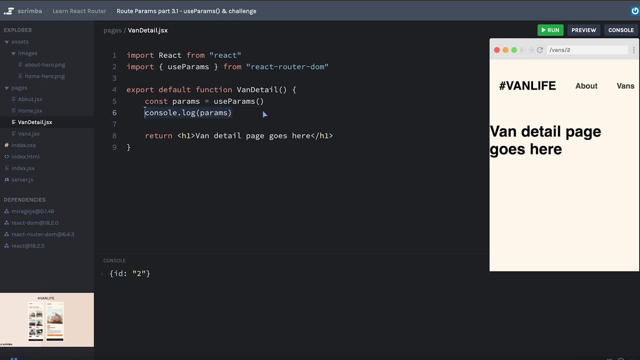 Instead of building a whole separate app to have you get practice with this. I'm actually just going to delete what we've done and have you do it from scratch, So I will write up part one of this two part challenge that we're going to do. 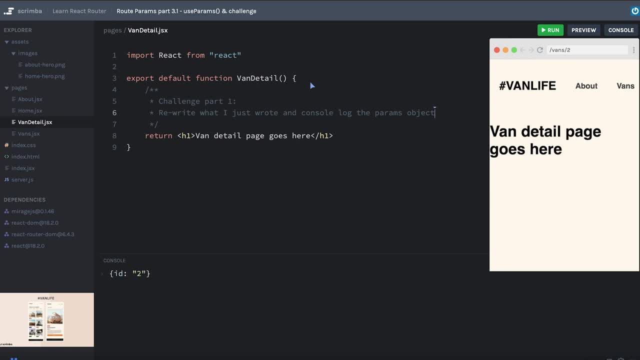 Okay, this will test if you were paying attention. of course, you can rewind to see exactly what it looks like, But I want you to be the one who's writing this out. So I want you to rewrote what we did And I want you to console log the params object, like we still see in the console from before. 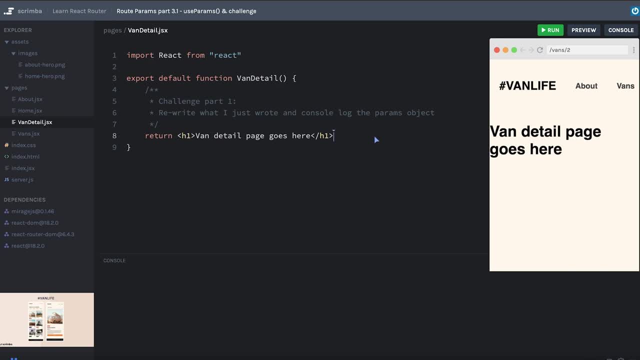 In fact, I'll hit save and that'll disappear. And now it's your turn. pause and work on this challenge. So we need to first import the use params hook from React router DOM, And then we will grab the params object by calling use params. 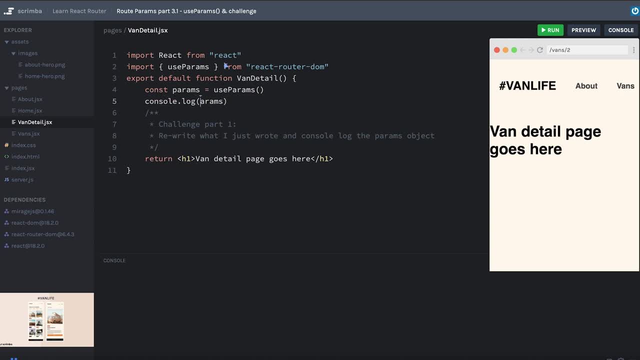 And then simply console log params, And that needs to be lowercase save. And there we are back to where we were. Okay, so now we're ready for part two, And this lesson is getting a little bit long, So we are going to do part two in the next scrim. 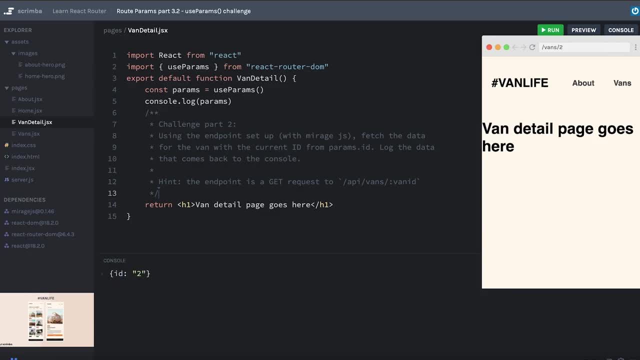 Okay, so in part two of the challenge, I want you to make a fetch request to get the data for the van that we're looking at on the van detail page based on the paramsid that comes in. So I'm going to press server, fake server again to get the data and the endpoint you will. 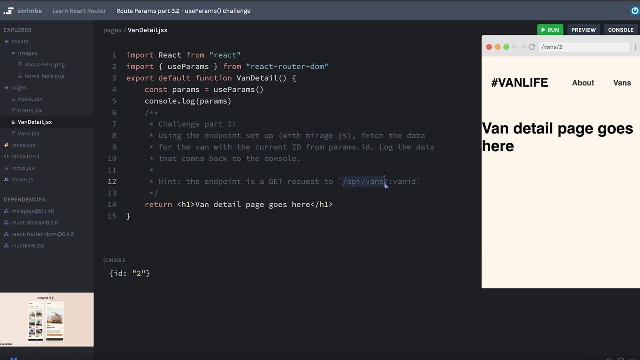 make a fetch request to is slash, API, slash, vans, slash and then the ID that comes from params. In this case, I'm just making this as a comment. van ID has no significant meaning or anything. I'm just saying that the ID of the van needs to go at this point in the URL. 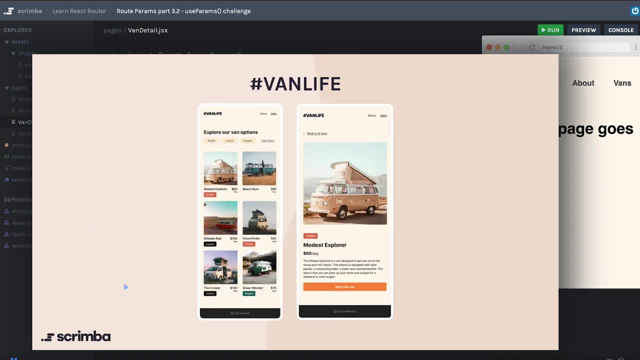 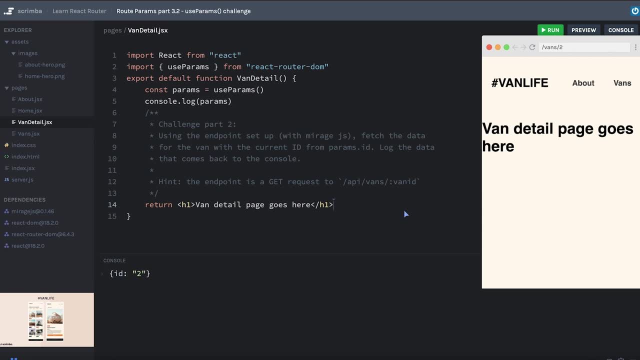 For now, you can just console log the data. we won't be worrying about designing up the page. I'm just going to give you all the markup that I use for that. Okay, pause now and work on this challenge. Okay, let's get ourselves some room by closing the console. 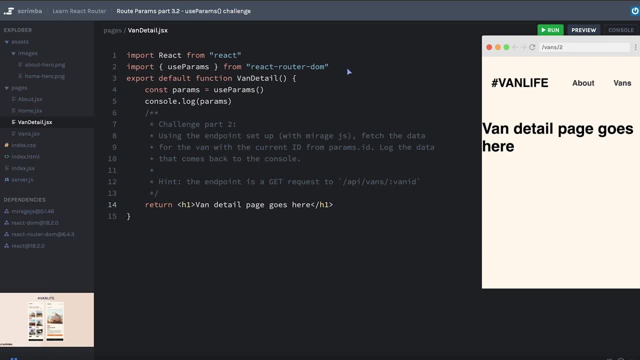 And, like we've done before, we're going to use react dot use effect to make a request when this component first loads. So let's go ahead and do that down here below this text we'll do react dot use effect. First parameter is the function, the effect function that we want to run. 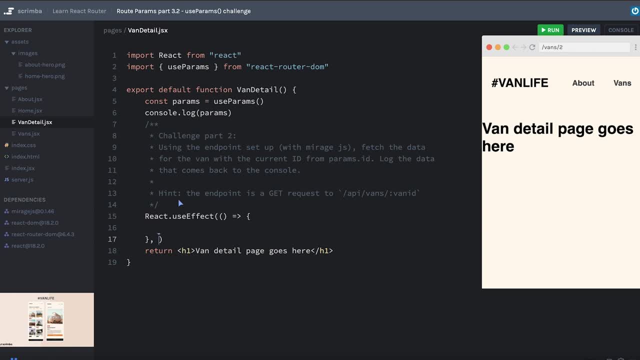 The second parameter is the array. The third parameter is the array of dependencies. Now, before, what we did was we used an empty array of dependencies, And that's because, well, the fetch request didn't rely on any other external piece of data to stay in sync with what we currently want to fetch. 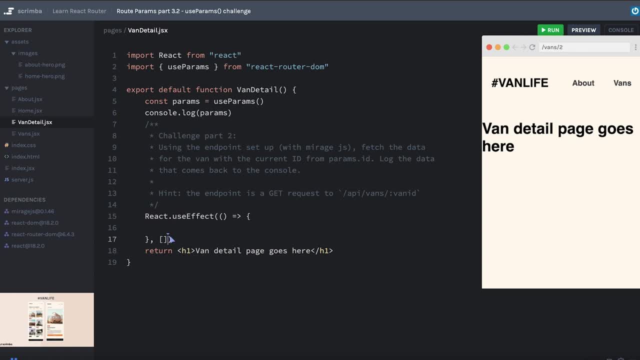 However, this time around we do want to rerun our effect. if somehow this component were still loaded but the params ID were to change. In our case, this probably isn't going to happen. The only way I can really think of this happening is if we had some link on this van ID. 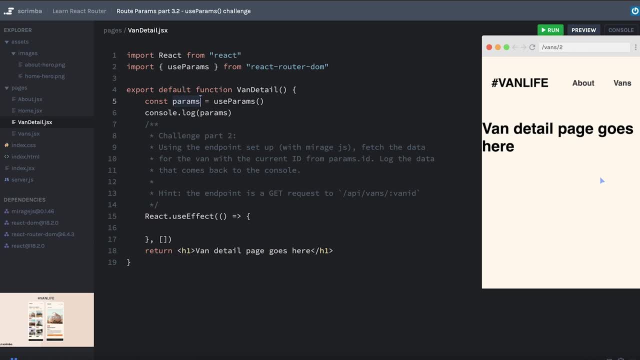 So let's go ahead and do that. Okay, So if we had a van detail page that links to another van detail page, in which case what would happen is the ID would change, but the component would not unmount and remount, it would just rerun the function with a new params dot ID. I suppose down the road maybe. 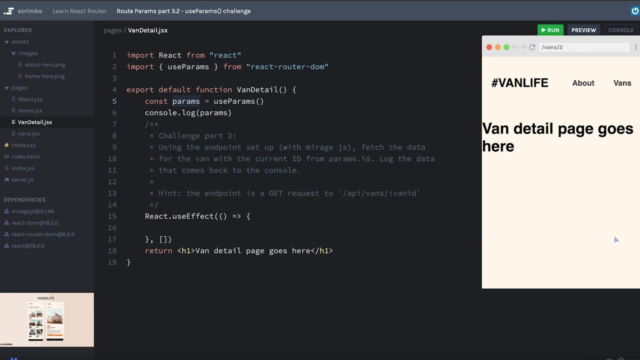 some feature that says here's some vans that are similar to the one that you're looking at could be implemented, in which case this would make a difference. If we left this as an empty array, it would not refetch when we moved to another van, like 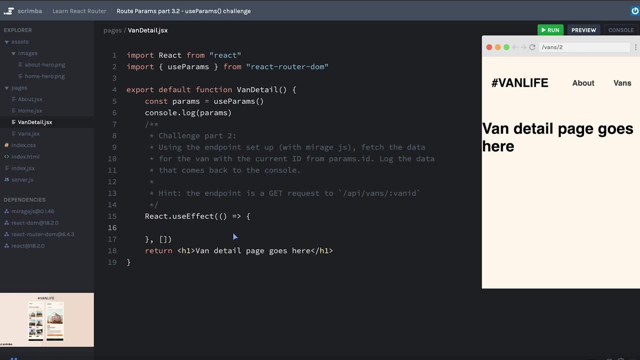 van slash three Instead of van slash two. it wouldn't run the effect, therefore it wouldn't run the fetch and therefore the page wouldn't change. That's not a feature we're worried about now, But since we know it could happen, we might as well put it in here. 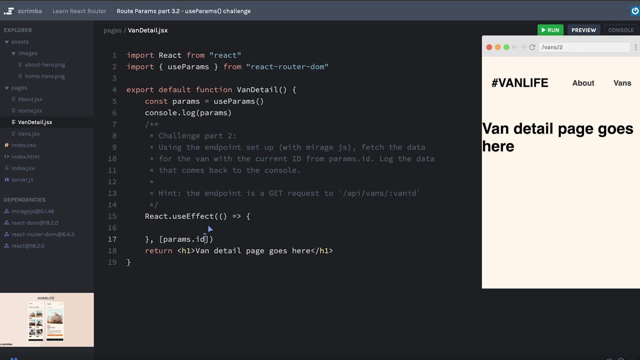 So I'm going to say I want you to rerun this effect if params dot ID were to ever change. Okay, so then we'll do our fetch request And we're fetching out to slash vans. no, slash API. slash vans, slash and then the van ID. 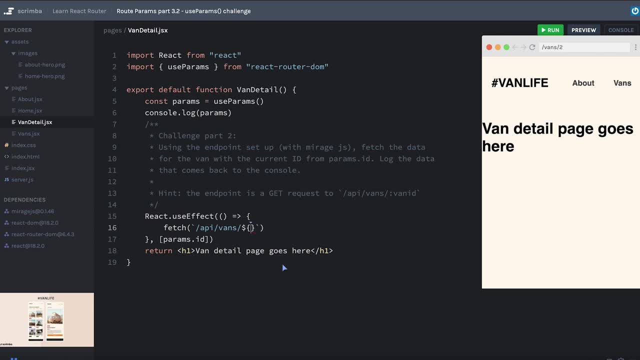 which we're getting from params that ID. So I'm going to use some string interpolation here And we'll say params dot ID. Then we will get the response and parse the JSON out of it like this: res dot JSON. That returns a promise that we will also resolve that we'll have the data and let's just console. 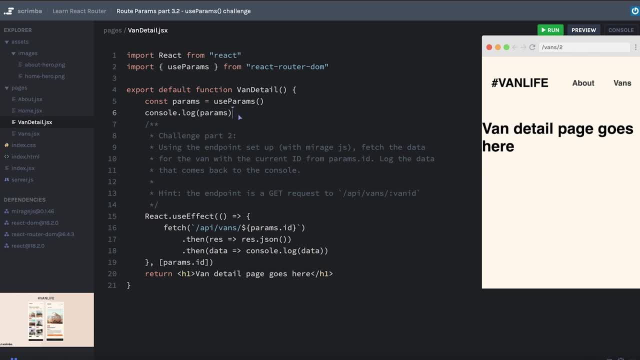 log our data And at this point I'll get rid of this console log And let's get rid of all the challenge text here, just to clean things up a little bit. We'll hit save and check our console. Okay, it took a second because it's doing a fetch request. Okay, it took a second because it's doing a fetch request And a day or two ago we were going to the database and it pulled the van ID of two. And a day or two ago we were going to the database. 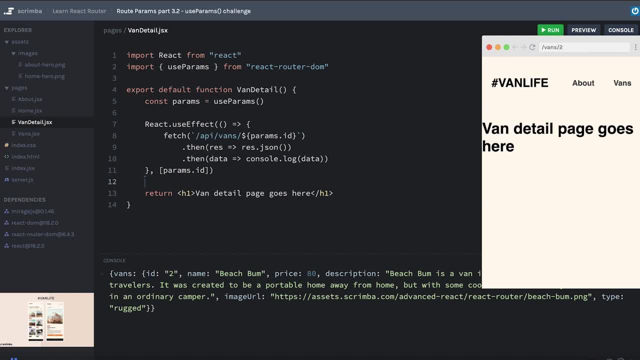 But it pulled in the van with the ID of two. In this case, we can see that there's this object that has a vans property And that's the only thing in here and the only thing we care about. And awesome, it has everything that we need. 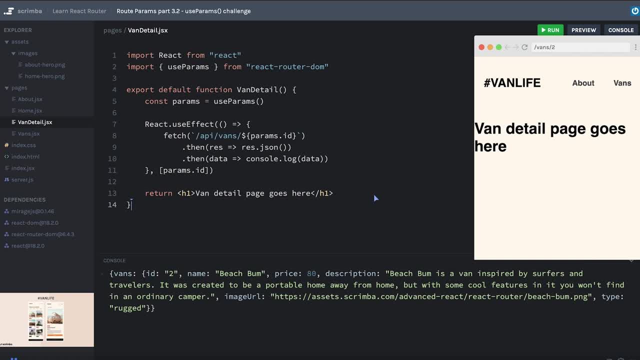 At this point, all of the next steps to get this page up and running actually looking good, with the data that we need is really something that you should be very familiar with by now. So once again, I'm going to snap my fingers. 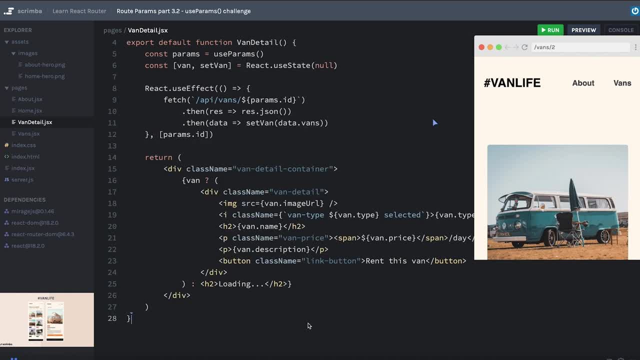 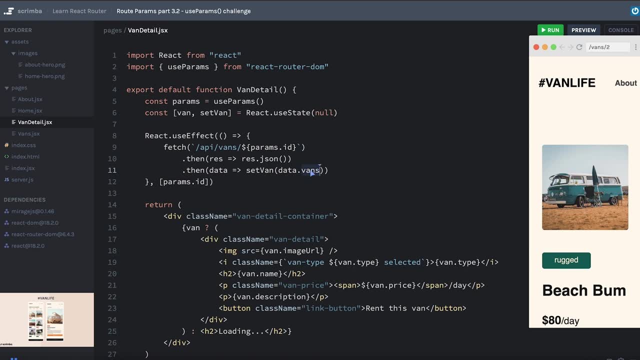 Really, all the changes that have changed are enormous. the changes that I made are: instead of console logging the data, I set that data into some localized state. You can see we used datavans because we had that vans property in the data that was coming in Up. here we're initializing that state. The rest of it is mostly just some. 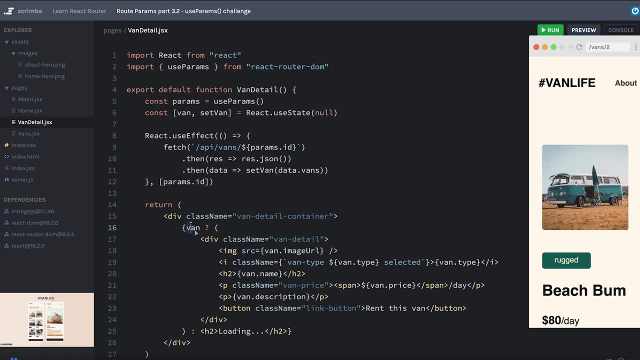 markup. You can see there's a little bit of conditional rendering happening here, because we're initializing our van state as null. If I try to access things like the image URL on null, then that's going to be a problem. So what I did was conditionally render if there's a van. 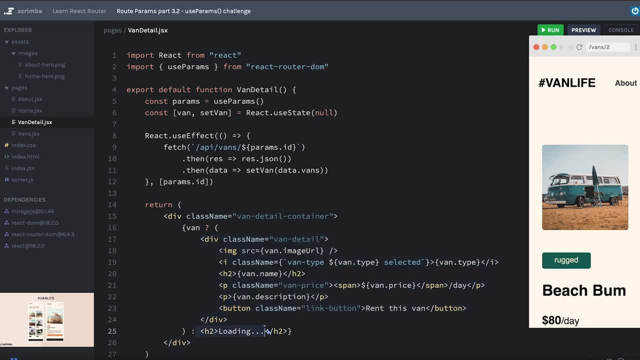 then I rendered all the markup, and if there isn't a van, then we just have this h2 that says loading. When I refresh the page you can see it. briefly it'll say loading and then it'll show the data. Everything else is really just some styling. There's nothing too special here. Clicking the. 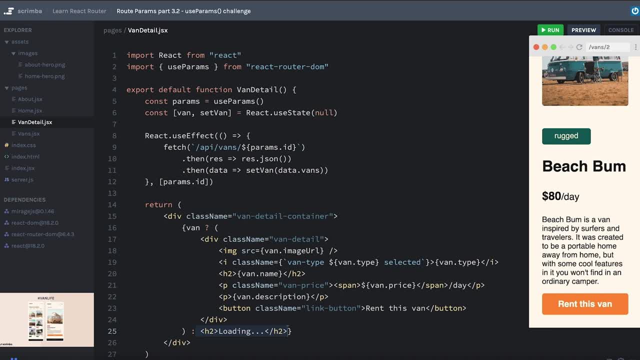 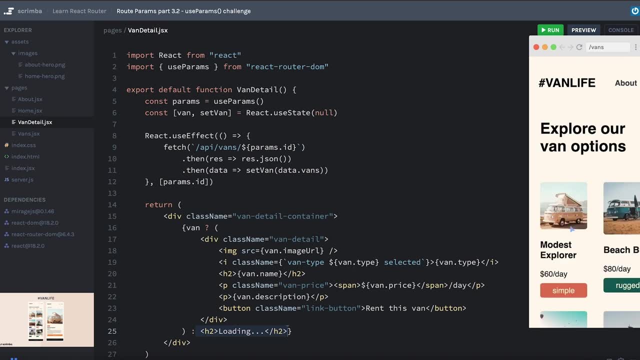 button at the bottom doesn't actually do anything, but what's awesome about this is because we're using a dynamic parameter in the path. we can go back to vans. We can click the modest explorer and we can go back to the vans. We can go back to the vans and we can go back to the vans. 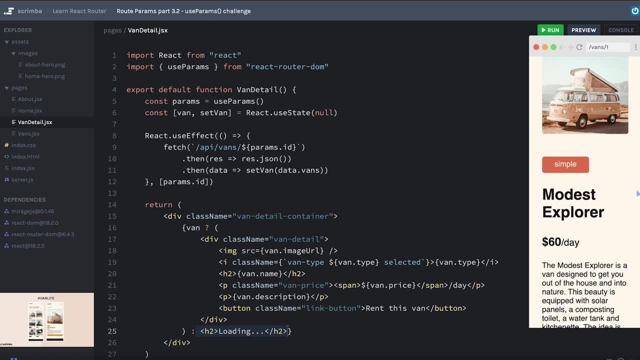 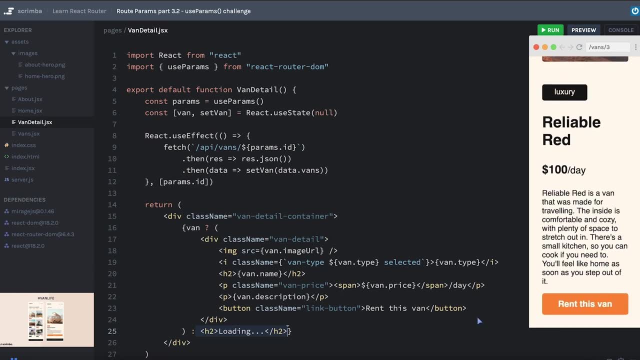 We can go back to the vans and we can go back to the vans and we can click the modest explorer And it's going to load the data from the van with the id of one. Go back to vans and choose something like reliable red, and we have that data as a separate piece of data. So, once again, as a 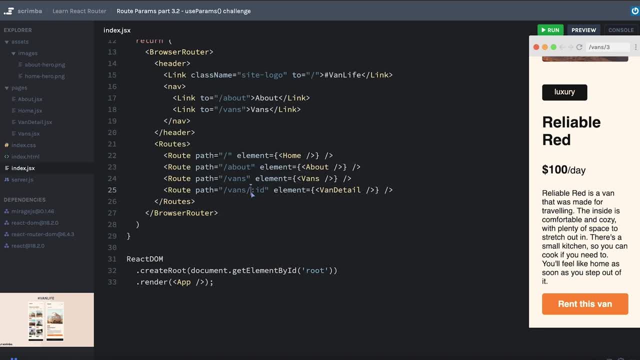 quick recap: over in index we created a route parameter that was dynamic by using the colon and part of the path that we have for our route definition. By using that colon we're setting it up so that react router will save whatever value gets put in the url when this page loads into a. 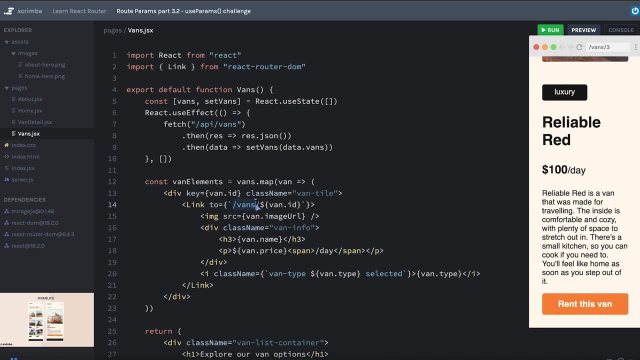 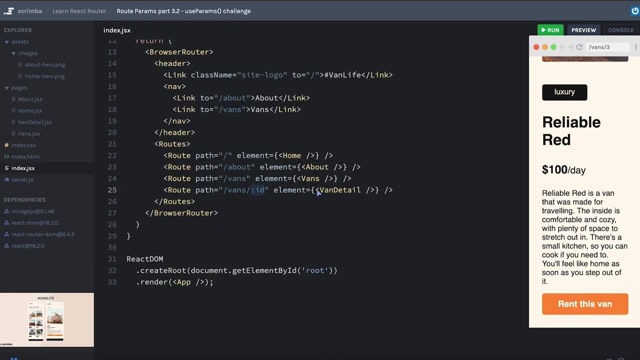 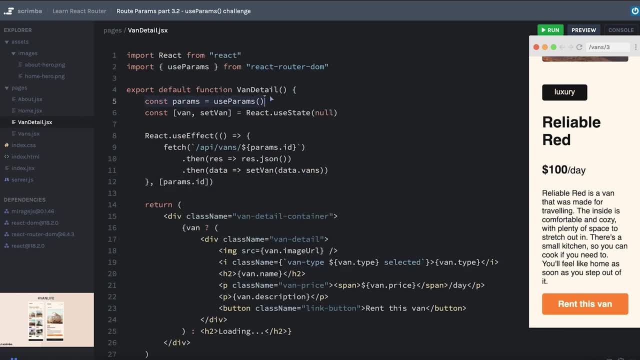 there because the element is set to go to the van detail page. when we get to the van detail page, very first thing we do is grab the parameters from the url so that we can make a fetch request to then get the van with that specific id. Again, we could definitely increase the performance of this. 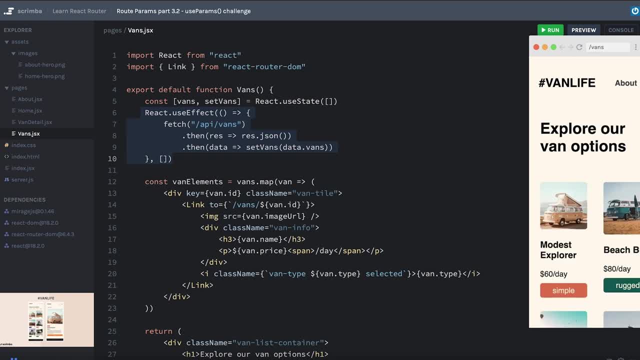 component loads or the vans component loads. We could probably save that maybe in local storage or do some kind of caching so that it can not have to make a request across the internet first but can just check our local cache And then, because this data that's coming in has all of the 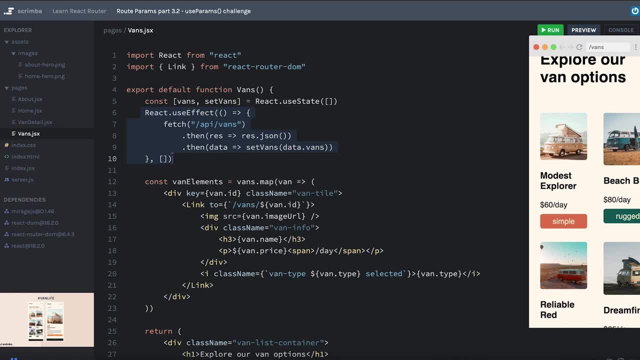 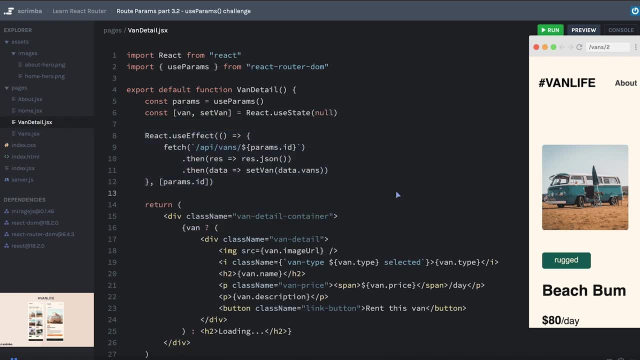 information for each van. we could theoretically just grab the piece of data that we need based on the url, instead of making a whole extra fetch request like we're doing in our van detail page. But at this point, with us learning react router, that's not really our. 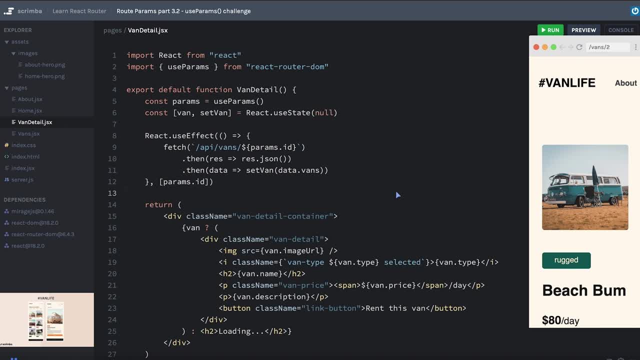 intent here. We're just trying to make this a very performant app, and just like that, we have a majority of our app built. at least the skeleton is all there. There's a few little details that we still need to fill in, so that's what we'll start working on next, As always, though, if there's anything that was confusing. 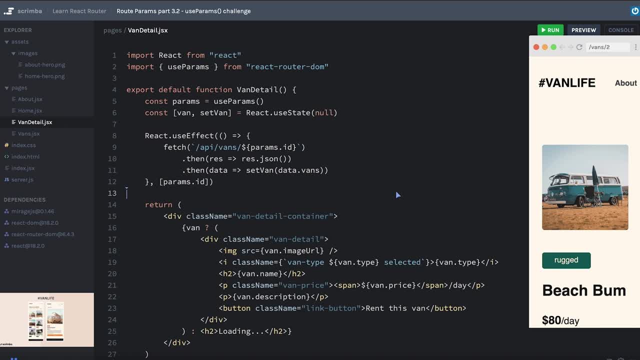 about this challenge series that we just completed. I don't want you to push forward, I want you to go back. I want you to practice, practice, practice, practice what we've done. That's going to be what helps you internalize what we've learned. If this were school, you might be cramming for a test just. 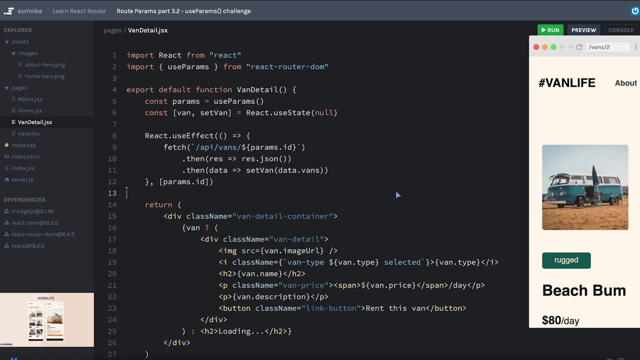 so you could pass the test and move on, but this isn't school. I want you to actually learn this stuff. Of course, it's always okay to use whatever resources you have. using Google is something that even the most senior developers do every single day, but getting the muscle memory. 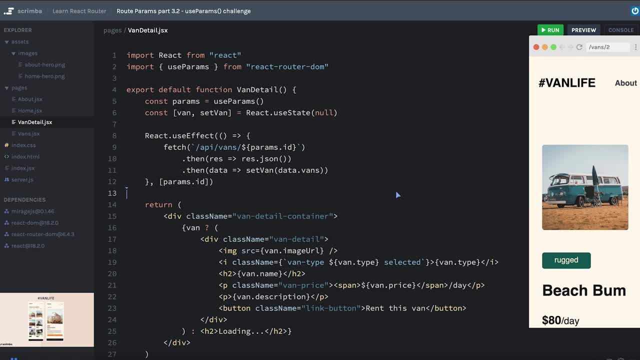 by practicing. this is what's going to help you truly, deeply understand what's going on, at least well enough to start building your own projects. So spend as much time as you need, Reach out to the scrim community and ask any questions that you might have and then, once you feel confident with the things that we've been learning, let's 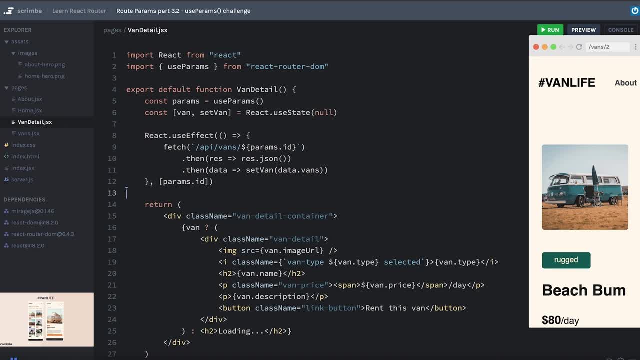 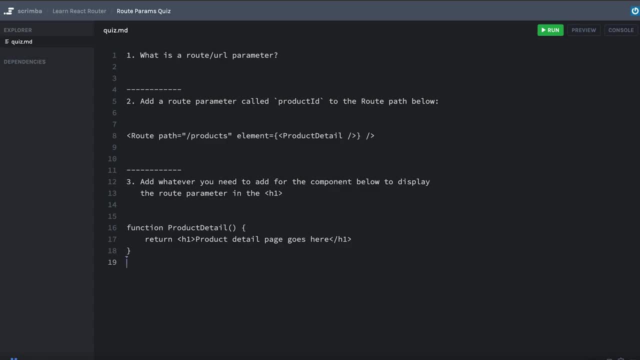 move on and we'll start learning some of the nuances about react Router. Let's run through a quick quiz on route parameters, just to make sure that you are understanding everything we've been talking about. again, I'll remind you that this isn't school. I'm not going to be giving you a grade on this. it will have no. 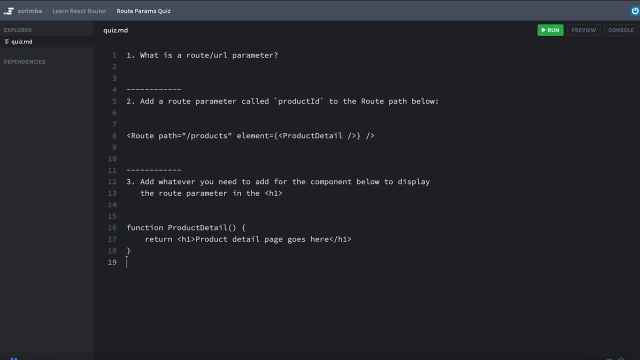 effect on how you do in this course. really, this quiz is a tool for you to assess your own understanding of what you've done. as such, I recommend you don't just skip ahead if you were to struggle with any of the questions here, but rather to maybe open a separate tab review the lesson. 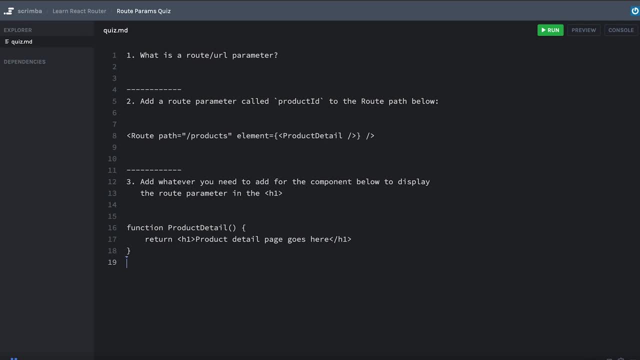 That's associated with each of these questions and then come back and see if you can answer them for yourself. Skipping ahead and just watching me answer it will maybe help you understand it a little better, but the understanding will be so much stronger if you're able to answer it by yourself. 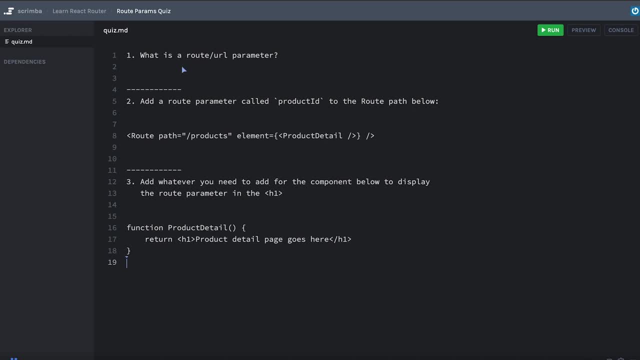 Okay, that's enough of a guilt trip now with these quizzes on scrim. but I do expect that you pause the screencast, just like we do with any other challenge, and physically type your answer down. I know when you hit play it's just going to erase your answers, but that's not the point. the point is to have that muscle memory. that's included. 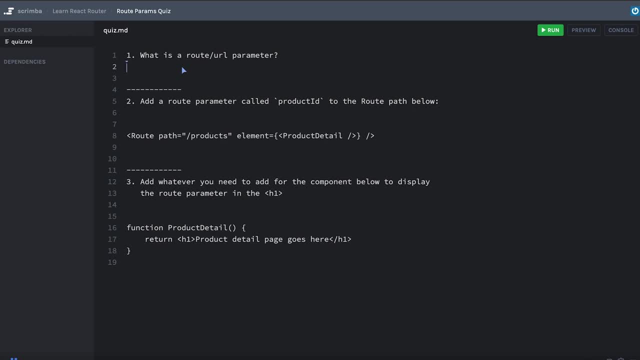 When you actually type on your keyboard. it will really help you retain the answers that you're writing down. okay, pause now and work on answering the quiz questions. Okay, number one: what is a route, or sometimes called a URL parameter? in our route definitions, we are able to tell it exactly what we want the URL to say when a certain component is loaded, or, more accurately, when a certain element is loaded. 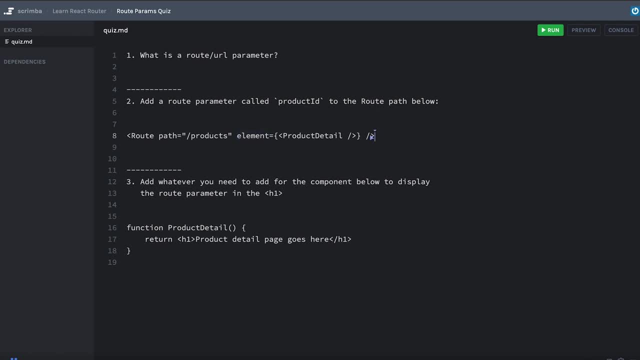 However, it's Pretty common for us to not know ahead of time, as the creators or the developers of these route definitions, what the actual URL will be. this is most common when you have some kind of detail page that displays specific information for one specific item in a whole group of items. 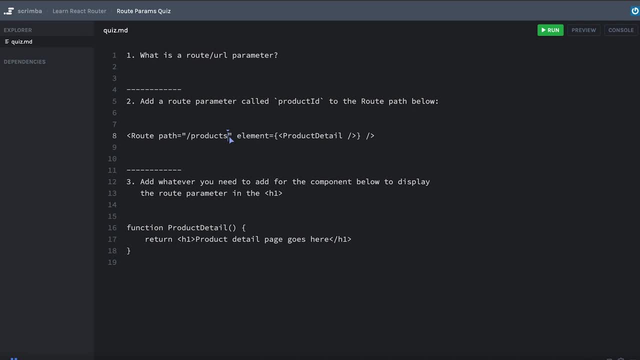 That sounds super specific, but if you think of basically any web app that you've been to, there's probably something like this. for example, any blog will probably have something like a slash blog route, but then after that you might want The detail for a specific blog entry, which case it would be slash blog slash, and then probably some kind of slug of the title of the blog. why I love react router, for example. the second portion would be a route. 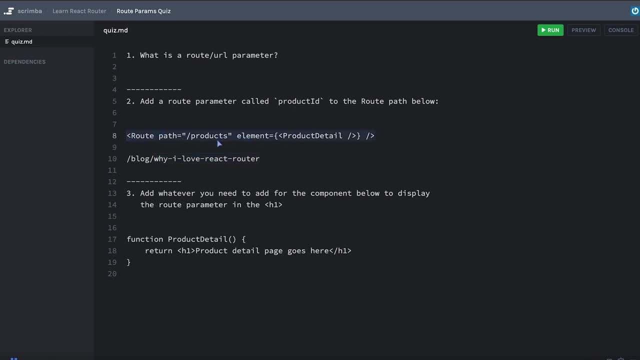 Param, instead of copying and pasting our route paths a billion times every time we want to add a new blog entry. instead, we can create a parameter inside of our route path that makes it a sort of placeholder for any part of the path that might be put in there. so 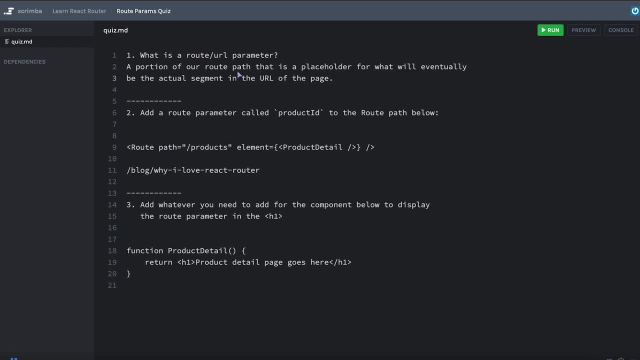 Let's, Let's. Let's try to summarize that in an answer here. This sounds a bit wordy, but I landed on a portion of our route path that is just a placeholder for what will eventually be the actual segment in the URL of the page. 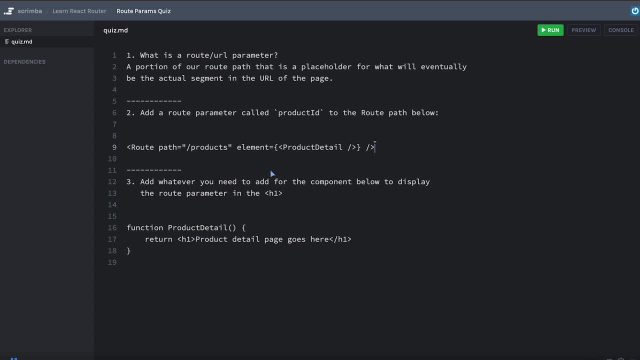 So let me clean this up. I'm already bleeding over into number two here, and let's work on number two. we need to add a route parameter called product ID. I'm going to copy that to the path below. we have a path that says slash products, but we are going to add a slash representing a new segment of our URL and then instead 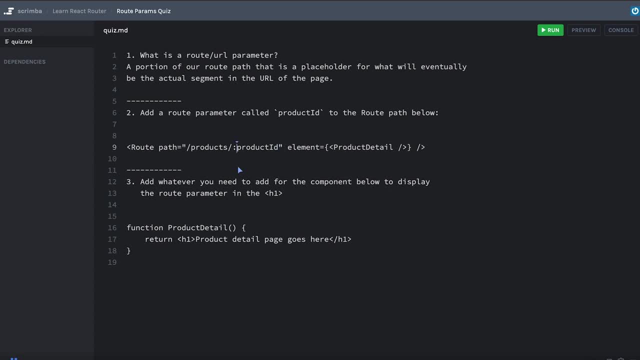 Let's, Let's. Let's simply pass fifth element to: okay, Let's just give it some역ata, Landis, seeing this is previously created in the scheesecast box in gebruic, because in e facts we've had some similar situations in the past. so instead of just putting product id, I'm going to put a colon in front of product ID. 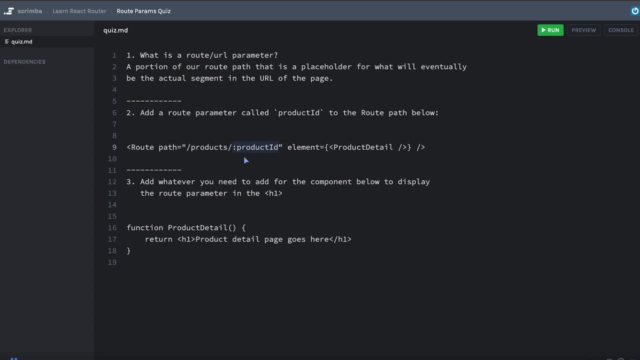 If I just had product ID, then it would be the literal text: slash products from product ID, with no deviation whatsoever in this. however, with the colon it says: by the way, this is just a placeholder for some other text. that will actually be the segment in the URL of our page. 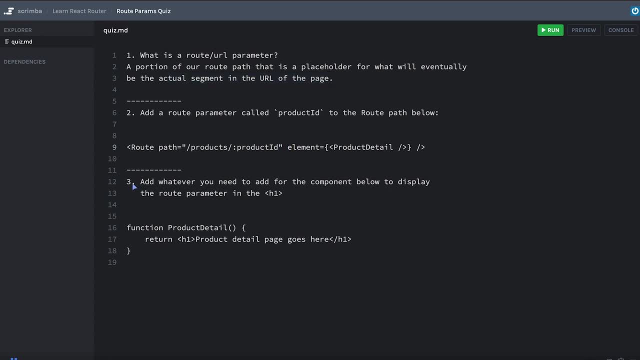 The ARR録 is got a picture, the page, so that we don't have which the textbar the email is using for Okay, and then for number three, we need to add some code below so that we can actually display whatever product ID gets put in the URL when it's displaying our product detail component. 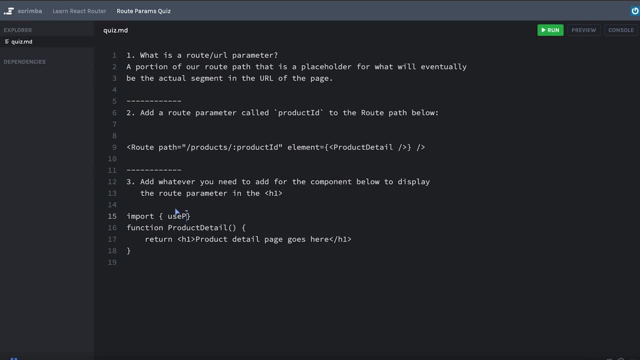 In this case, we would need to first import use params from react-router-dom, and then we can grab the specific parameter that we want. In our case there's going to be the one called product ID, and that will equal a call to use params. 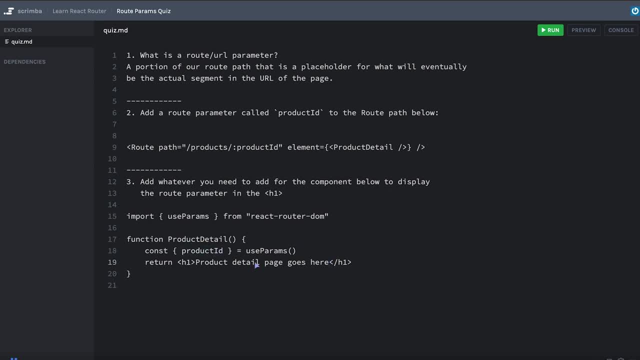 And now, with product ID in tow, we could say something like product ID is and then stick in our product ID. Okay, since this is just a markdown file, we can't really save this and double check that it works, but I feel pretty confident with my syntax here. 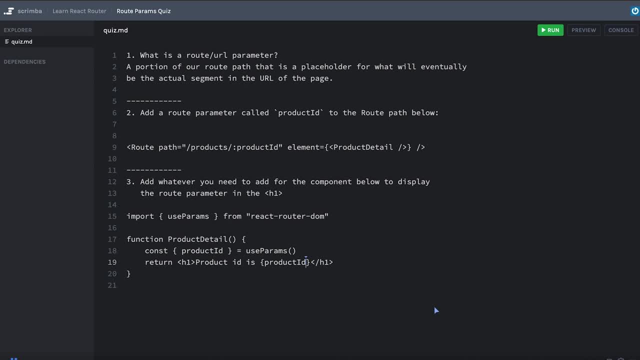 And more important than the specific syntax, is an understanding of the concepts behind it. Once again, if you feel like you need to review these things, then now is the time to do that, before we plow ahead, and when you are ready, we'll keep moving forward. 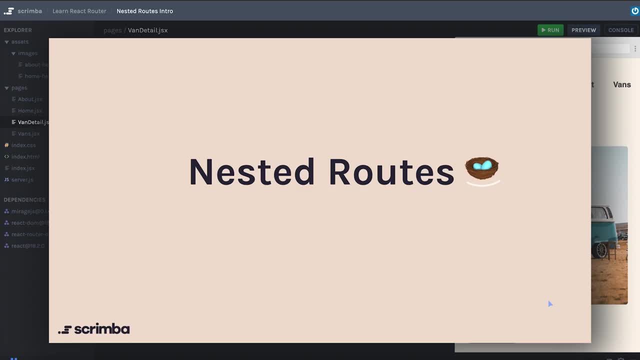 We are about to dive into what, at least for me, was one of the more complex topics about react-router. but that's okay, We're going to walk through it very much step by step and hopefully we can get to the end and you'll just completely understand it perfectly. 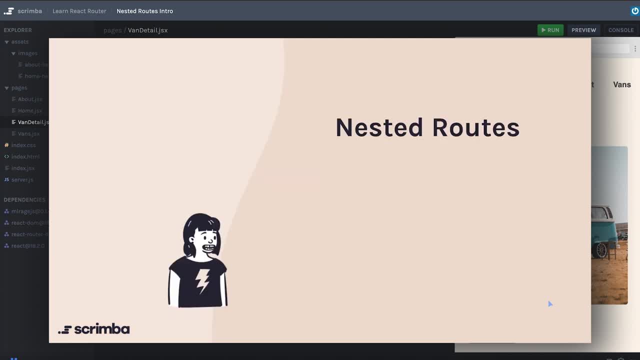 And that topic is nested routes. When we're talking about nested routes, we're oftentimes talking about actually a couple different things. First of all, we're talking about nesting pieces of the URL. So, for example, we've already seen something like this: 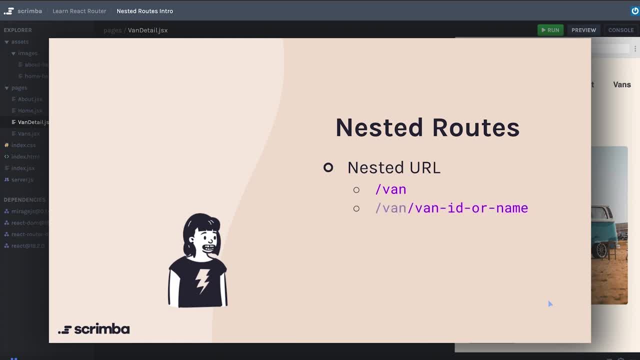 We have this Slash van route and a nested route that we have is the slash van slash and then the ID or the name of the van or whatever it is you want to be in the URL. But the URL is only a part of the story, because when we're talking about nested routes we're also talking about some shared user interface or parts of your page that need to remain on the page when you transition from one route to a child route or a nested route. 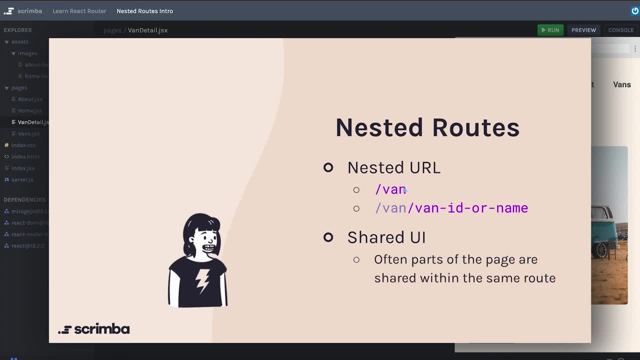 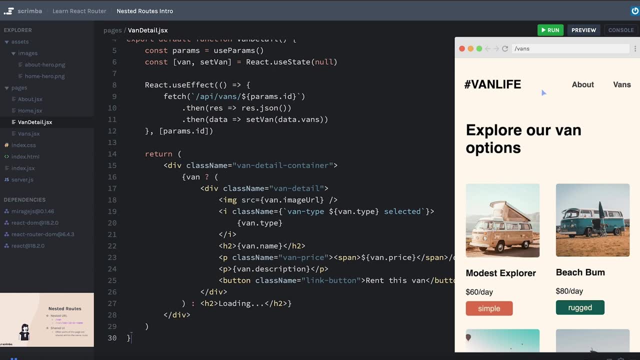 And that might happen more than you think With the example with the slash van and the slash vans Slash ID. over here we're not doing much of that because if I come to vans, I mean we're sharing our navigation bar across the entire site, but slash vans doesn't really have any shared UI with its child route of slash vans slash and then the ID of the van: slash, van slash one. 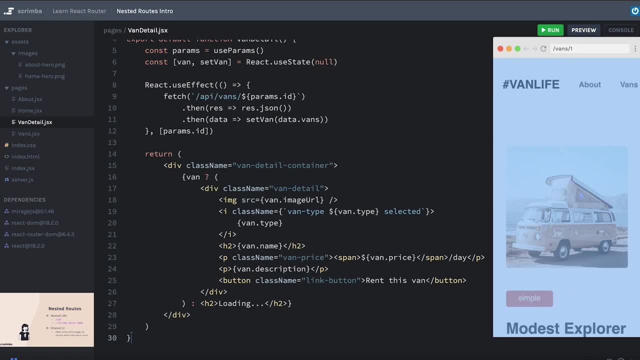 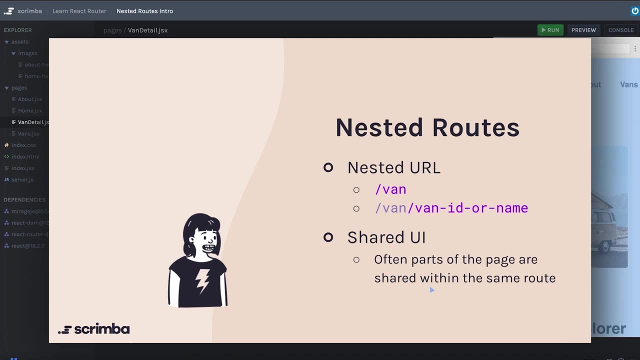 Even that little explore our van options wasn't part of this next page, And so this page isn't really sharing any user interface, but oftentimes you will want to do that. A really great visualization of this is over on The remix website. 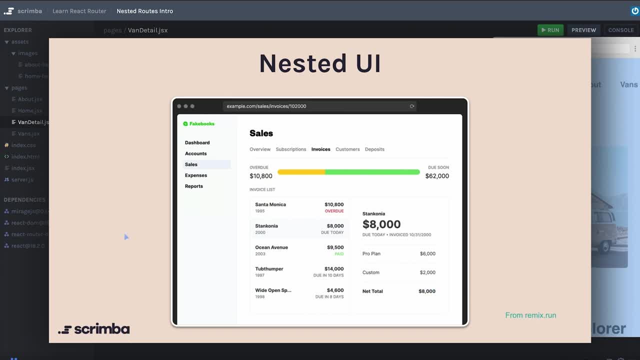 I included a link here if you wanted to see the live demo of this, And the reason it's over on remix is because react router is actually now a part of the remix package. Remix is just a full stack framework for the web. It uses react right now on the front end, although I think in the future they'll be supporting whatever front end framework you want to use. 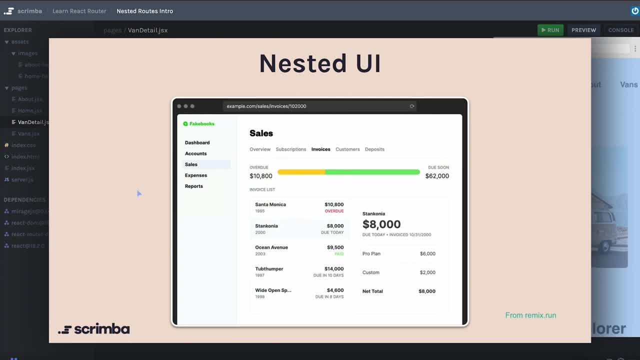 But a major part of remix is the way that it handles routes. So here we see an example app- They call it fake books- and we'll notice a few different things. First of all, we're inside Of a nested route. here we have example dot com, slash sales, slash invoices and then slash the number of one of the invoices and if we break this down, you'll see that example dot com is rendering everything that you see on the page. that includes the navigation bar over here on the left, the logo, everything else, as you might expect. as you navigate with this navigation bar on the left, it will probably go to example dot com: slash- maybe dashboard slash- accounts. we happen to be here at slash sales and so that's the next part of our URL: slash sales. 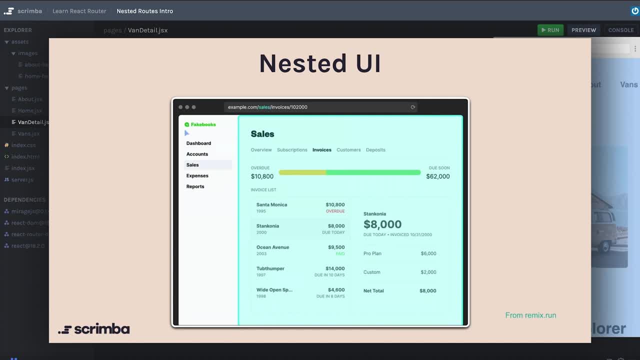 And We still have some shared UI here because we are maintaining the navigation bar on the left, the slash sales part of this URL is going to render everything else that you see here in this teal color. now, here we have yet another navigation bar. inside the sales portion of our website, we have an overview of our sales, subscriptions, invoices, customers and deposits again, presumably if we click on overview. well, that might just be the slash sales endpoint by itself, or maybe it's slash sales, slash overview. 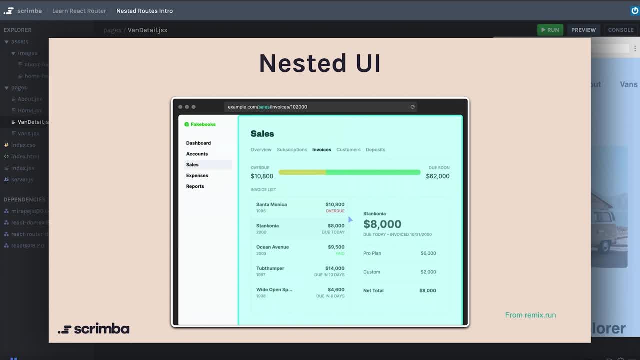 We click on Sales, Sales, Sales, Subscriptions. that's going to be slash sales, slash subscriptions. we're here at invoices, so we have slash sales, slash invoices. this top portion is going to be a shared UI or those other routes. so if we go to the next image, we see that invoices is rendering this part down here, but it's keeping everything from this kind of secondary navigation bar and then, of course, everything from the first navigation bar still exists to. over here we have a list of invoices and presumably this is one of those invoices. in fact it's the second one. 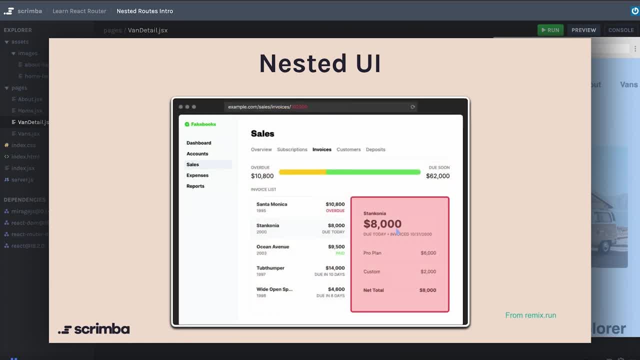 So the last part of our URL, which is the ID, is going to be rendered in this little portion over here on the right. so in this example, we see not just a nesting of the portions of our URL, but that those portions of the URL are mapping to nested content on our site. or another way to think of it is that there's quite a bit of shared user interface pieces on the site, even if you navigate to another route. so how do you actually create these nested routes? well, we know about the route component, but up until the end of this video, we're going to be talking about how to create these nested routes. 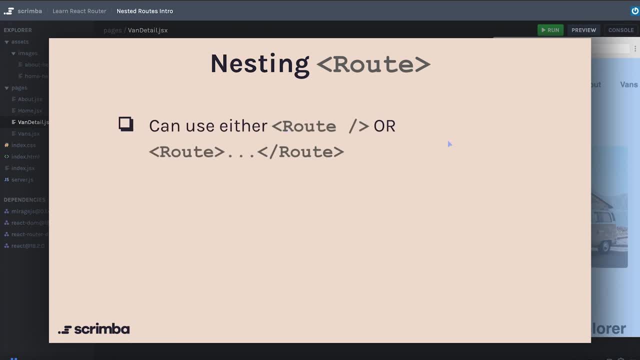 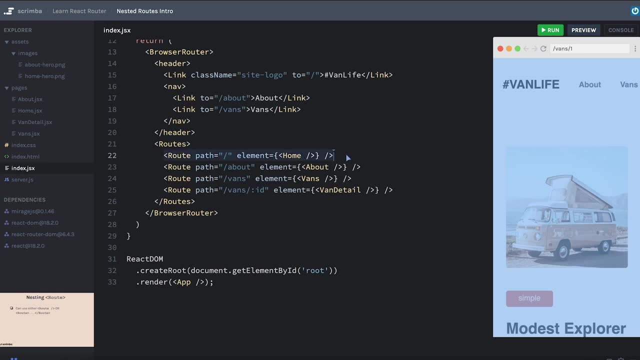 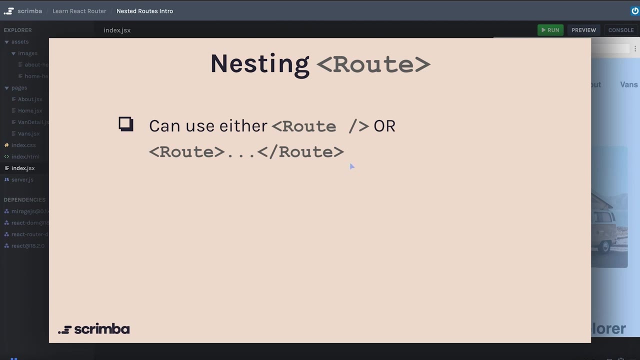 Now we've just been using it as a self closing component. if we look at the code that we've written so far- let's go to our index page- every one of our routes is closing itself. nothing is being nested. however, we can use route as a non self closing element, or rather something that has an opening and a closing tag. we're going to see exactly how that looks a little bit later, but it's one of the most crucial capabilities of the route component that allows us to nest our routes. now. we talked about there being a couple different reasons to do this. 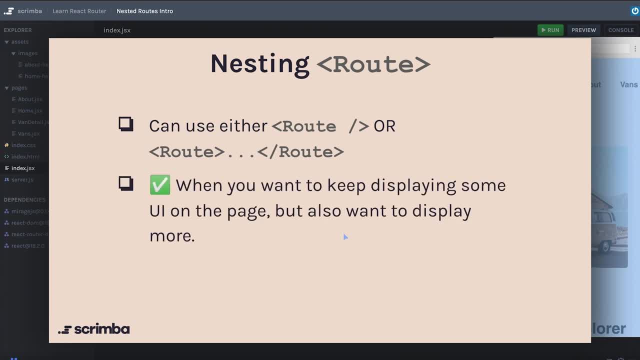 The first one is that you want to do nested routing, and I would like to propose that the primary reason that you would want to do it is whenever you want to keep some of the UI on your page, but you also want to display more. so you're linking to a new part of your website, but maybe that new part of your website is really just changing one small part on the page, or it could be a big part. to the point is, you have some things that you want to keep displaying, kind of like we showed with the navigation bar, or both of the navigation bars in that example, but you also want to display some of the things that you want to keep displaying. 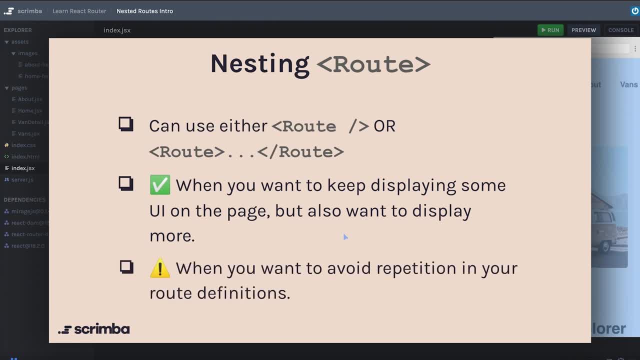 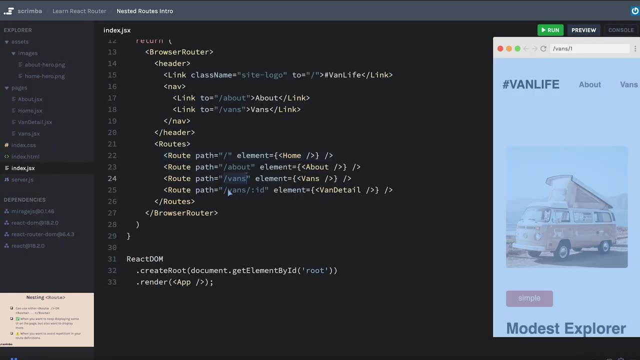 Another reason that you might want to do this is just so that you can avoid some repetition inside of your route definitions. I put a little caution sign here because sometimes that may end up being more work than it's really worth in the end. for example, over here we have a little bit of repetition where we're saying slash vans and slash vans, slash colon ID, but, as we mentioned, we're really not sharing that much user interface. actually, we're not sharing any user interface between the vans component and the van detail component, and so in this case you could choose to nest your routes. 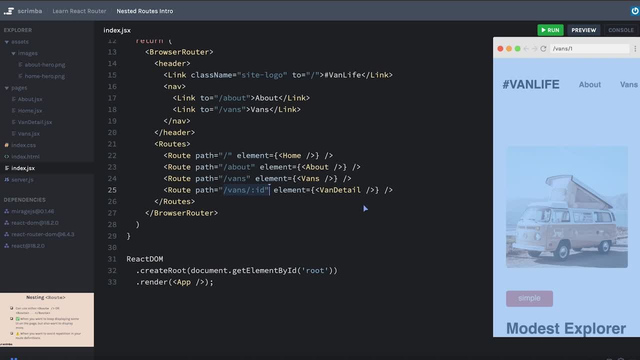 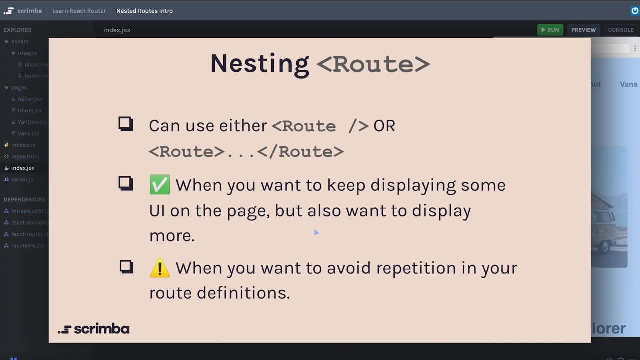 Or you could choose not to nest, and we're going to see what that actually looks like in a different scrim. but I wanted to lay the groundwork and say that the primary reason that I would suggest you actually considered nesting routes is when you have parts of your page that you want to keep, but also that you want to display some more stuff too. so this is really going to crack open our website, because we have a lot of pages that we're going to build so that we can really practice with nested routing and hopefully really solidify our understanding of nested routing. so let's take a quick look at what we will be adding to our site as of right now. 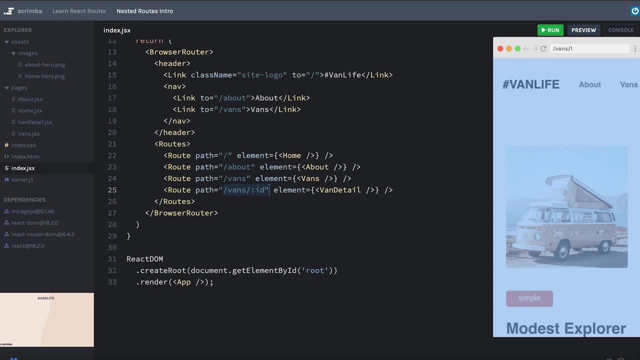 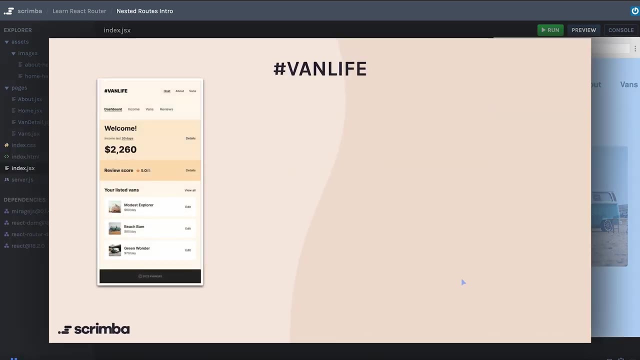 We are only consumers of our van life site. we can see the list of vans, we can see the details about one van. we can click this button that does nothing to rent the van, but on the other side of this equation are people who are renting out their vans. so we are going to be adding an entire host section to our website. hopefully it's not too small. you'll see in the navigation bar. we're adding a host link there and going to the host route is going to render a new navigation bar that we see here. that navigation bar will have a dashboard which is going to show us what we're going to be adding to our site. 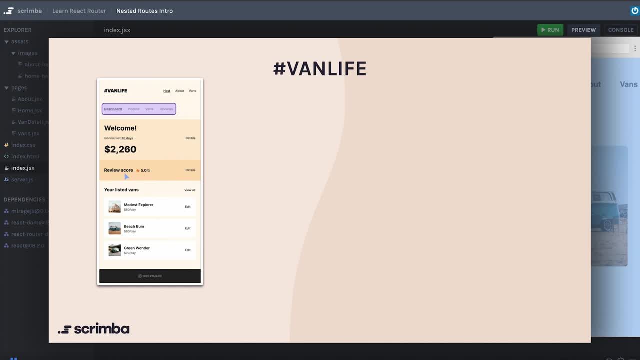 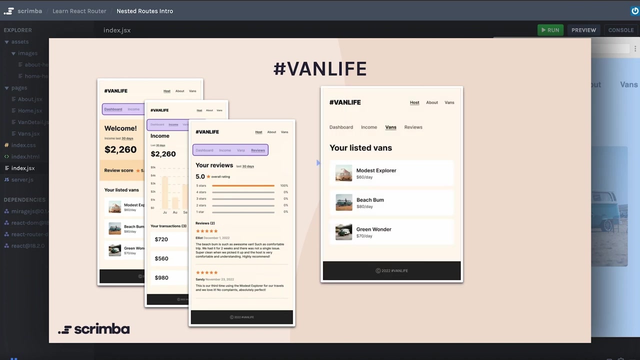 Which displays kind of a quick overview of the details the van host might want to know and also a list of the other information that the host would want to know, like a detailed view of the income. notice that it's also going to have this navigation bar. that's going to be a shared user interface- the reviews that their vans are receiving, again sharing the same user interface with that navigation bar, and then we have this section for vans. now I'm keeping this separate because this is going to go even another level deep on the slash host, slash vans route. we'll see. 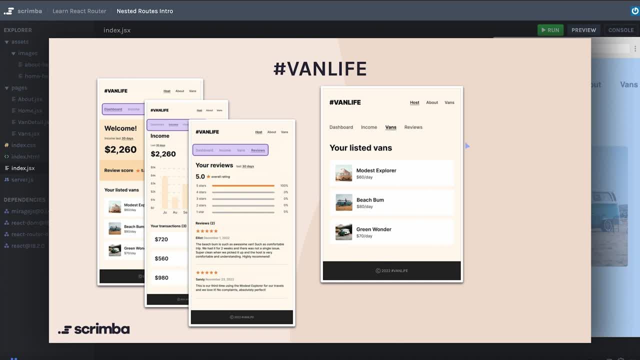 a list of all the vans that this host is hosting on our van life website. clicking on one of those vans will take you- and again it's got the shared interface here. but clicking on one of those is going to take you to a new page. there's still some shared interface, but this time we have yet another little navigation bar down here. this allows the host of this van to see the details, the pricing and the photos for this van. so the details will be kind of the default, and when you go to the pricing it will have both of those shared user interfaces too. and then 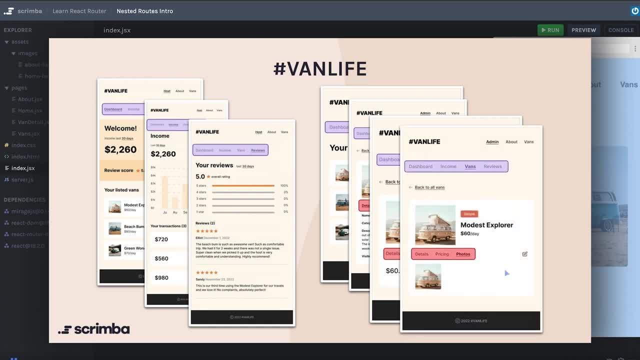 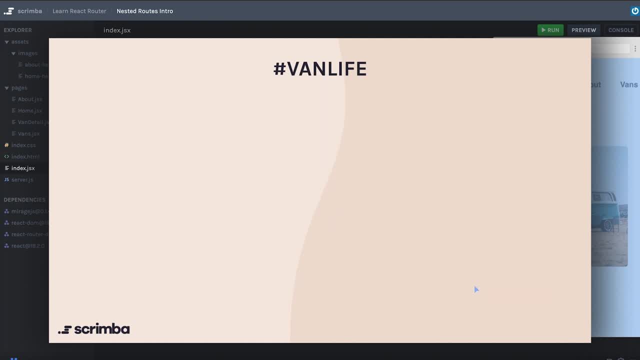 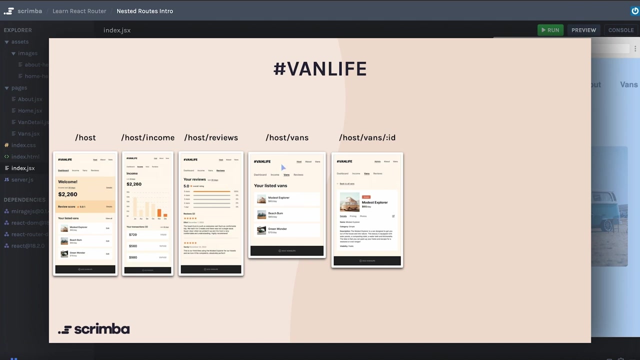 some new information that displays same with the photos. we'll have the photos of this van down here. theoretically, it would be where the host could then edit the photos. so to get an overview of the routes that we'll be adding, we will have the slash host route that's going to send us to the dashboard, then we'll have slash host, slash income, slash host, slash reviews, and then we'll dive into the slash host, slash vans. this is going to be the list page, but then we have yet another level of nesting where we'll have slash host, slash van, slash- the ID of the van that was clicked on. 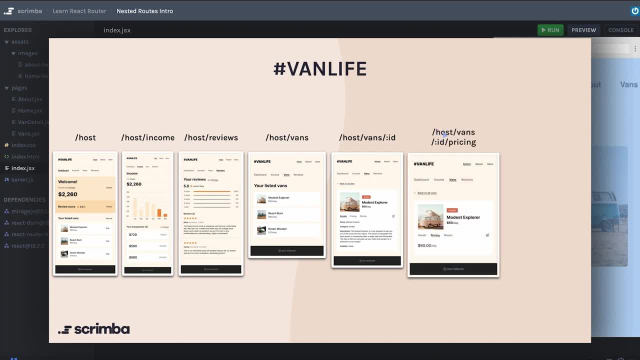 in slash host, slash vans, and then yet again we'll go down to slash host, slash vans, slash ID, and then slash pricing and slash photos. so this one here where it just ends in slash ID, that's going to sort of default to the details page. we also could choose to name this slash host, slash van, slash ID, slash details, if we really wanted to, but just making the executive decision to have that be the default view. okay, who, that is a lot. we have a lot on our plates, fortunately, kind of like before, because I really want to focus this course on. 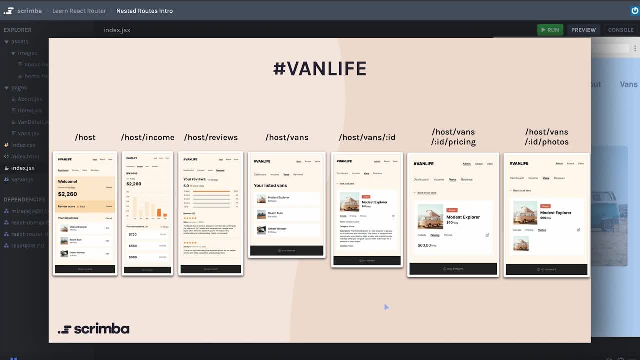 react router, and not necessarily on making a beautiful design. I will do you, the student, a solid and I will implement all of the styling and everything for you. I know that's not usually my style, but I do want to stay focused here on react router and, of course, that's not to say that you couldn't take the reins and actually design it yourself, if that's what you want to practice. so let's center ourselves, let's take some deep breaths if you need to, and we will jump right in. 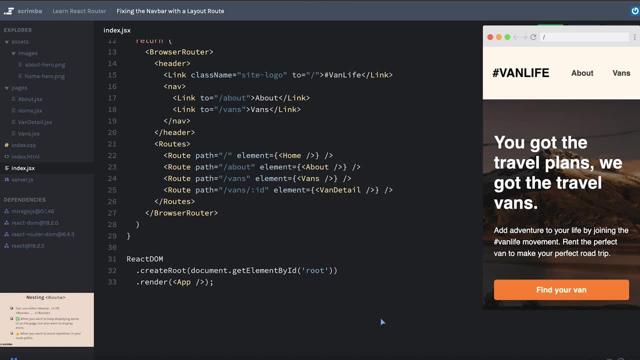 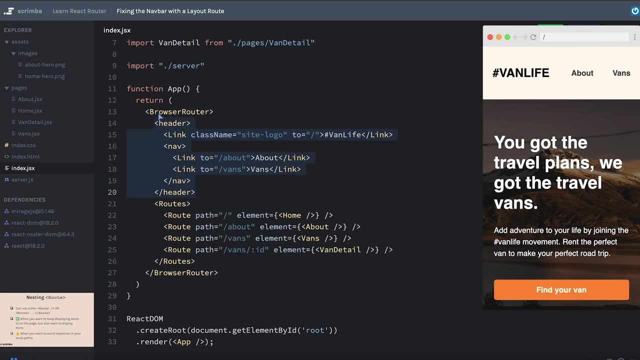 you. the first thing that I'd like to do to you- get our feet wet with this nested routing idea- is to really fix what we have going on with our header right now. we stuffed our header into our browser router just because it was outside of our routes, which means that it will display on every page. however, this really doesn't feel clean to me. in fact, if we had a header that was more complex, maybe it would take up 50 lines of code. it feels like a weird place to just stuff it into our browser router like this. I guess we could abstract it to a header component and then it would just say: header 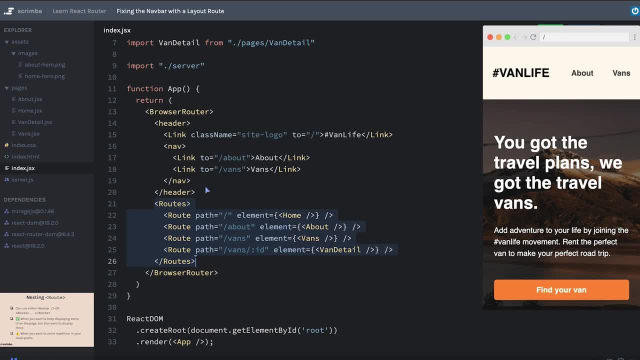 but still it doesn't feel good to me to put something that's unrelated to our routes inside of our browser router like this. So our introduction to nested routes is going to be through something called a layout route, And I wanted to remind you that the primary reason we are nesting our routes 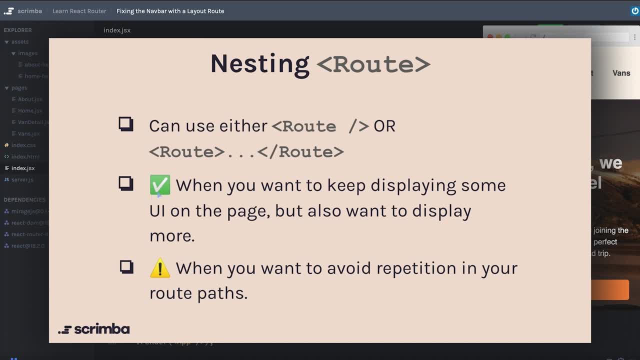 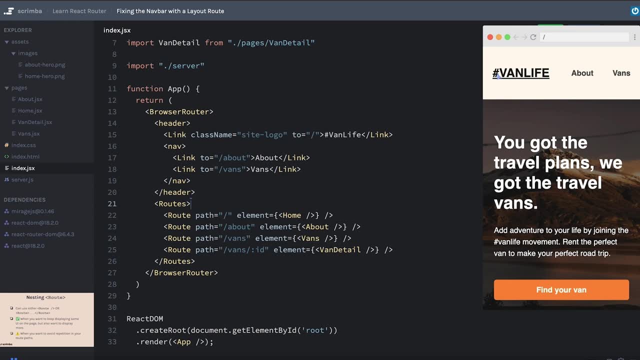 is so that we can hit this second bullet point here, when you want to keep displaying some information or some UI on the page, but you also want to display more stuff. That's exactly what we're doing with our navbar. We're keeping our navbar on the page And I think our design has. 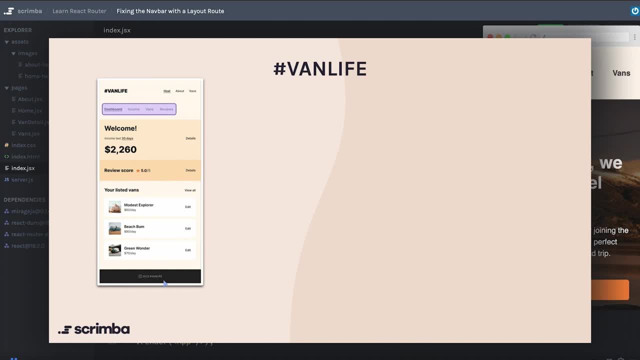 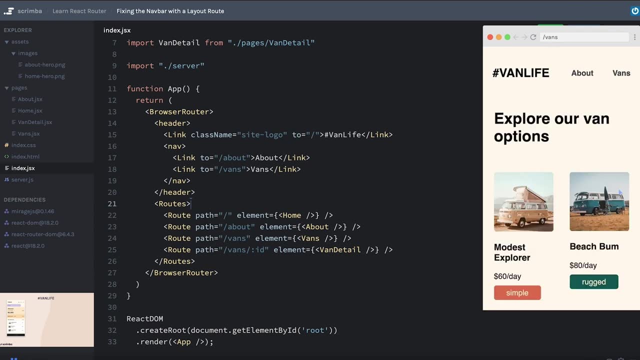 a footer too. Yeah, we've got a footer that we haven't implemented yet, But that would also be something that would just be on every page. But we also want the changing of our URL to display other things as well, So I added another slide to the end of this presentation. Let's bump forward. 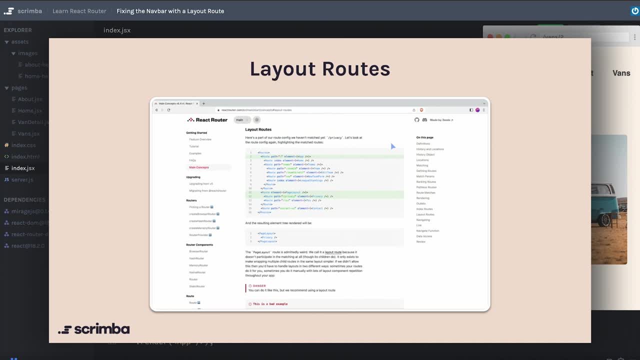 a little bit. This is an image taken from the documentation for React Router. It's specifically the spot that talks about layout routes. you can click the image you see here to go to the documentation. If you'd like, you can read through this whole main concept section, or at least parts. 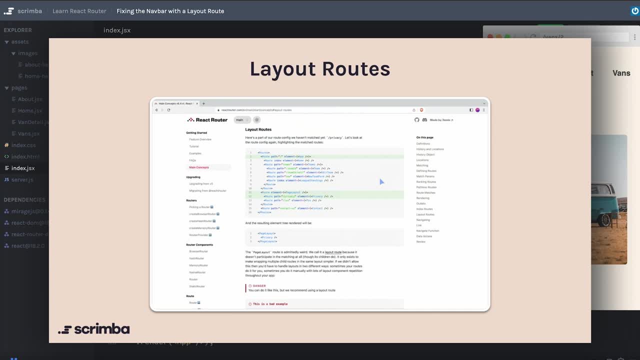 of it, And then you can see that it's a little bit more detailed, So I'm going to go ahead and skip through it. Maybe it might be a little hard to grasp if you haven't done React Router before, But it honestly has great information there. you might need to read it a couple times to make it. 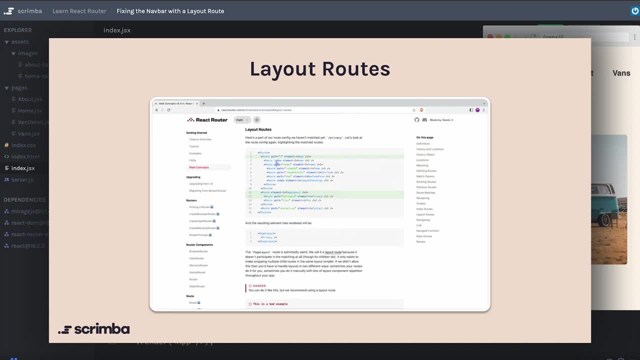 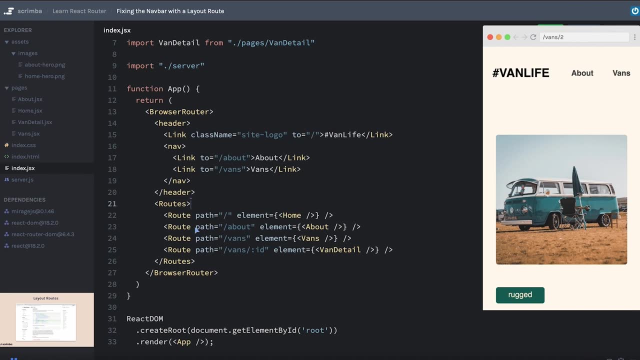 stick. So feel free to pause and go look at the documentation if you'd like, But I'm going to be talking about these layout routes. The idea of a layout route is that it doesn't have a path of its own per se, But instead its purpose is to lay out your page. we know that. we want every one of our 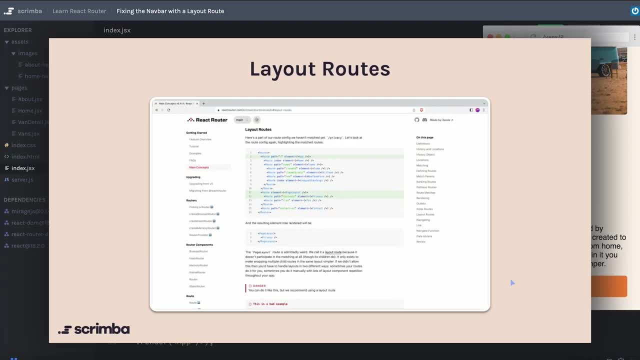 pages to have a header and a footer. If you want to have a header and a footer, you can do that If you go to that documentation. one of the things that they'll mention is how the concept of a route can be a little bit stretched, I guess, because in the case of a layout route you don't. 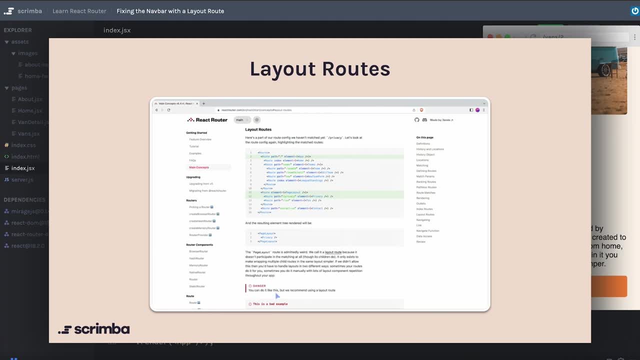 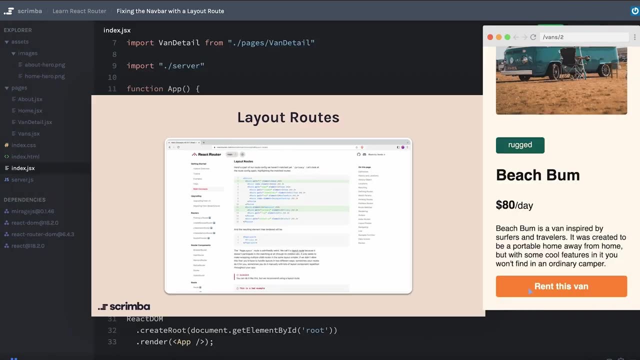 necessarily need to have a path. If you look really closely it's a little bit small in this image, but it says: this is a bad example And it says danger. basically, don't do this. What they talk about is how- if I didn't want my header here inside my browser router, but I did want to wrap- 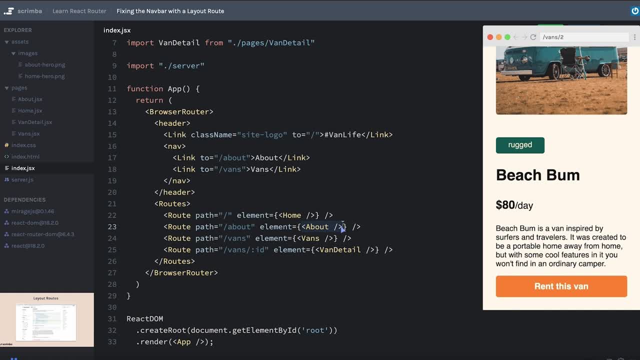 all of my pages without using what we're about to talk about, with layout routes, I would have to do something like this, And then I would have to do something like this, And then I would have to do this, And then I would have to do something like this, And then I would have to do something like this. 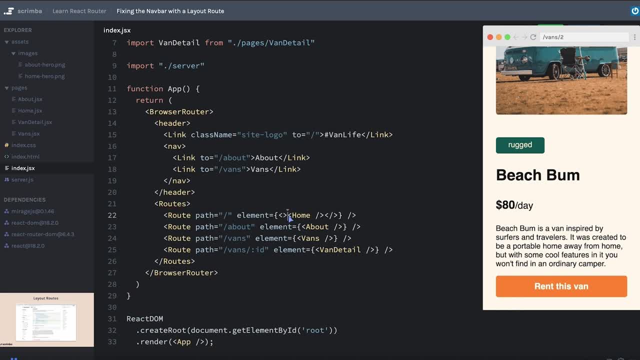 Take my home component and maybe wrap it in a fragment or a div and then start stuffing in all my header code just right here, And I would have to repeat that for every one of the elements that I want to have my header, And I would have to do that with my footer as well. This is obviously 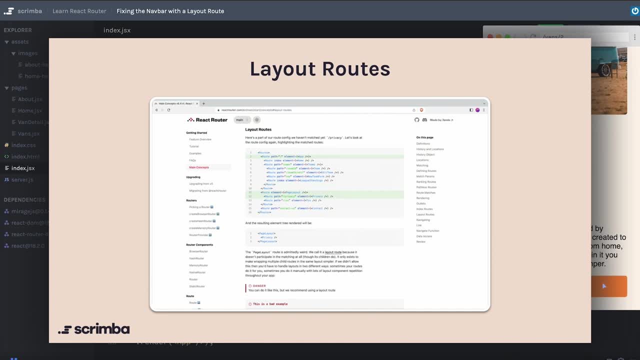 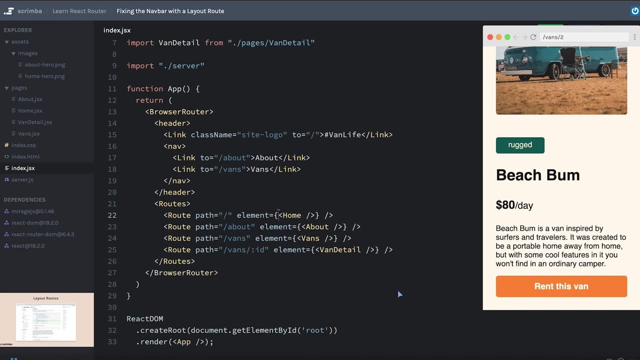 not a good example. Like it says in the documentation. don't do this. there's a much better way, And that is by using a layout route. So let me back this up to a reasonable spot Now. we do have a little bit of work before we throw the layout route together, So I'm actually 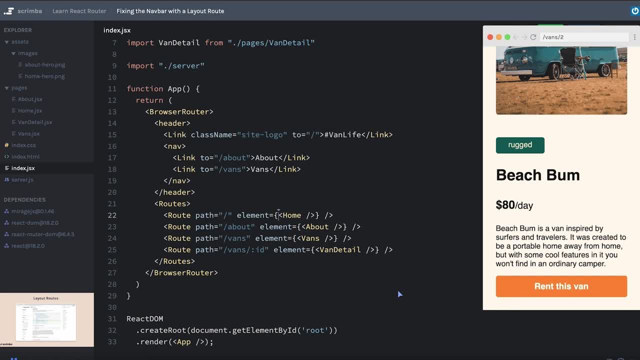 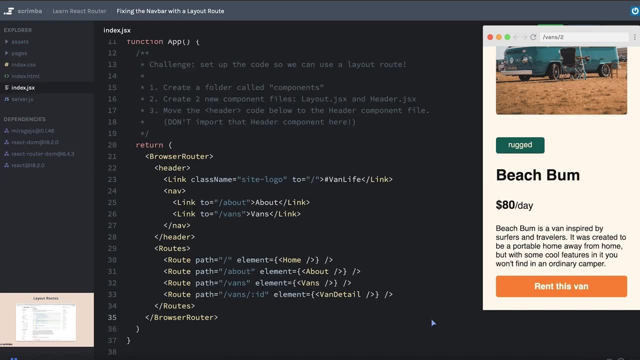 going to make a challenge. I'm going to give you the chance to do this hard work for me, And then we will actually implement the layout route in the next scrim. So let me type up a challenge for you. Okay, I'm sorry this is a bit administrative, But I want you to create a new folder called 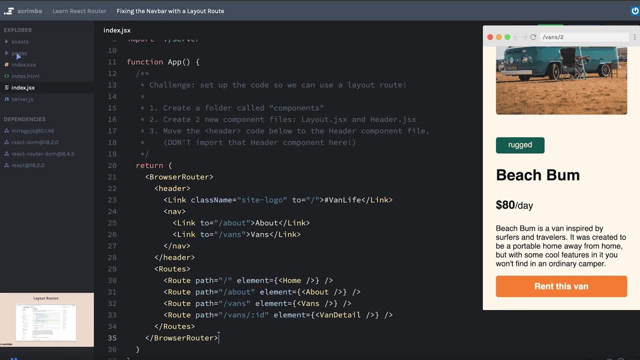 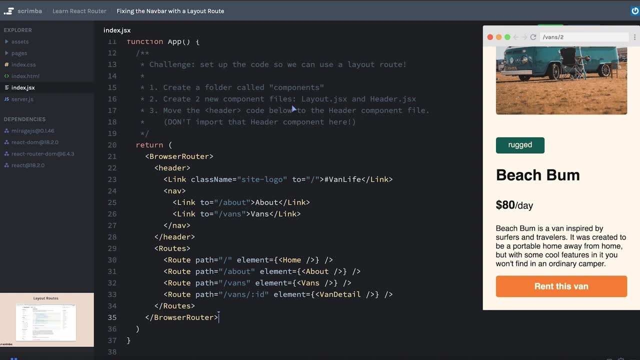 components. it's going to sit as a sibling to our assets and our pages folders, so not nested inside of them. And in that components folder I want you to create two new component files, layoutjsx and headerjsx, And then you will simply move the header code here into. 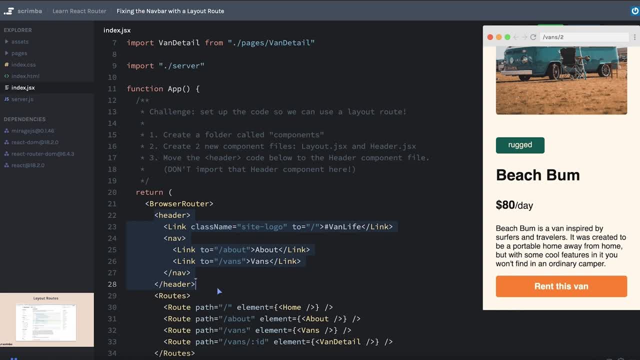 the headerjsx file. But I don't want you to necessarily go beyond that, because we will actually not end up importing it here and using it at all inside of our index file. So pause now and work on this challenge. Gosh, you know, I wish there were actually a way that I could just steal. 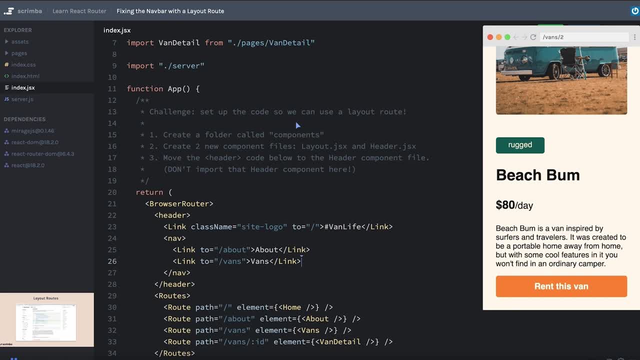 the code that you just wrote and use it in my recording here, But alas, that's not exactly how it works. So I will be doing this work. Let's go ahead and create a new folder called components, And inside I will create those two new files, header and layout, And then we will just steal. 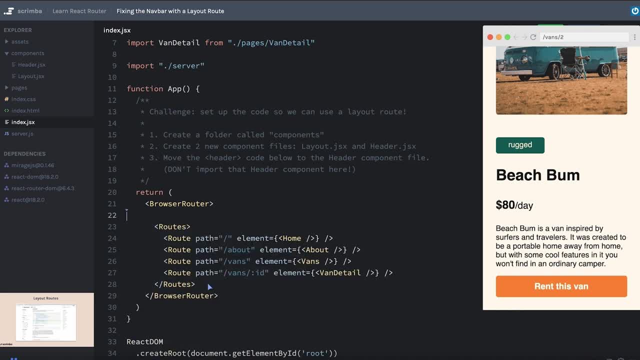 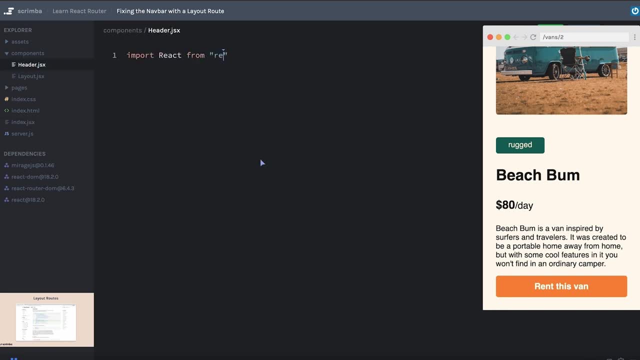 our header from the index page. we can actually just cut it. we're going to lose our header for a little while. So in the header we'll import react and we'll create our file, or rather our function, And we will return the header that we just copied. All right, let's hit refresh there. 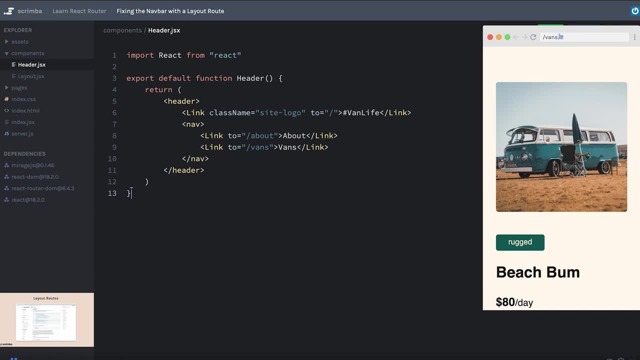 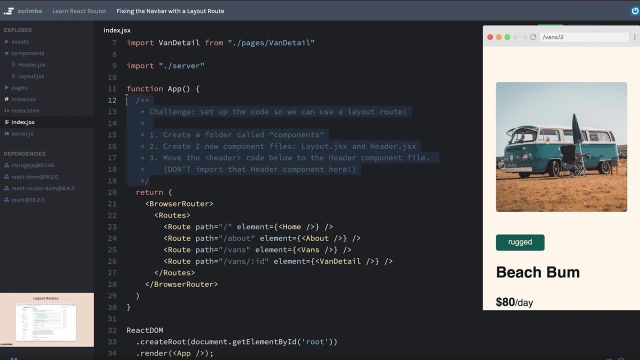 And okay. so yeah, our header is gone, which is a little bit inconvenient because we can't navigate our site anymore. But that's okay, we're going to fix that soon. Actually, we're going to fix that now because we've done the administrative stuff. we're ready to now just jump in and learn about. 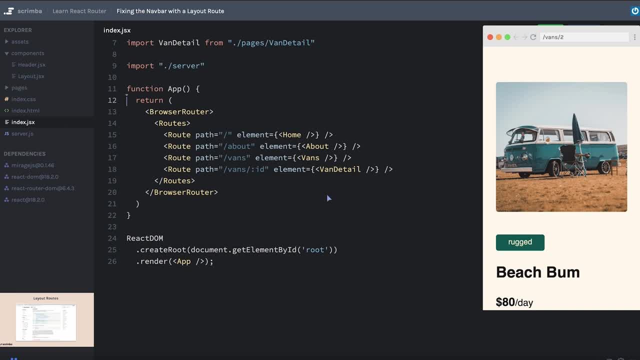 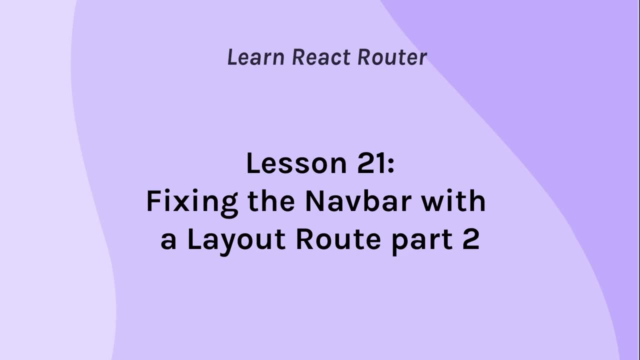 how we can implement this layout component so that we don't have to repeat ourselves by putting the header on every one of the elements that we're rendering at every path. Okay, so we mentioned how route is a self closing element, but it also can be an 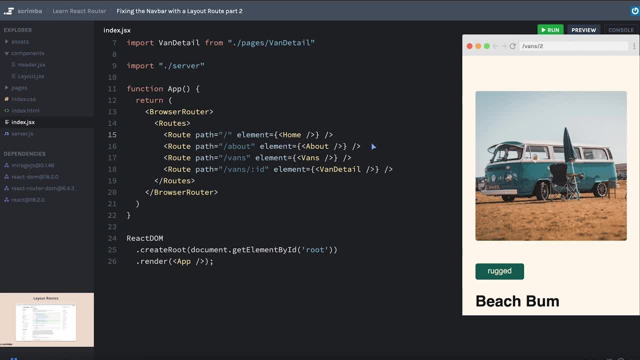 element that wraps around other elements And in fact, when the route component does take children, it needs to be other route components as its children. What I mean by that is, if I want to create another route up here and I want it to wrap around other elements, I can't just go ahead. 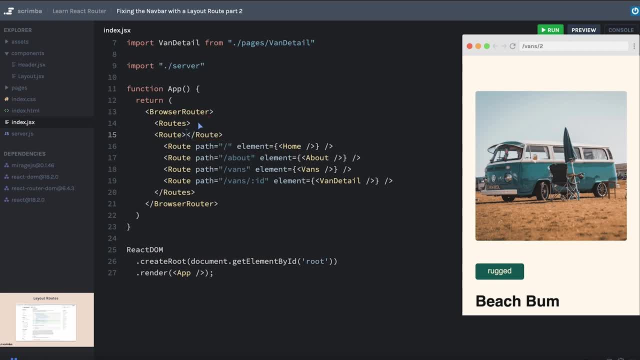 and start putting other things like an h1 in here. it needs it to be other route components as its children, So I'm going to move this closing tag down here. I want it to envelop or wrap around every part of my website that I want to be a part of, So I'm going to move this closing tag down here. 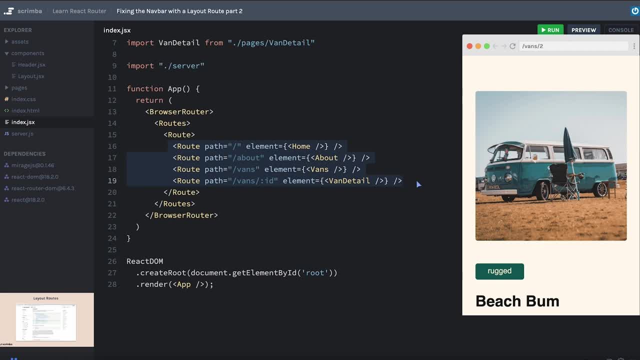 I want it to be anothersceneUads and I want to contain my navigation bar, which is everything. Now, assuming that you have dealt with React children, before you might start recognizing this pattern, this route component is going to essentially take whatever element we pass to it. So I can say an element, and this is where we're going to put our layout. 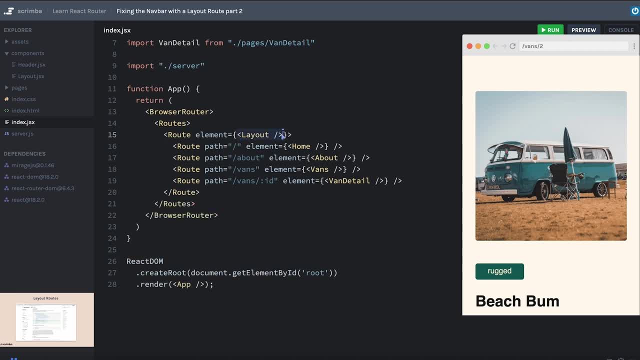 component And it's going to render the layout component and then it will also render whatever child route matches the URL that we're currently at. let's fix some of the bugs we have here. Let's fix here something we're not interested in doing, which isê. 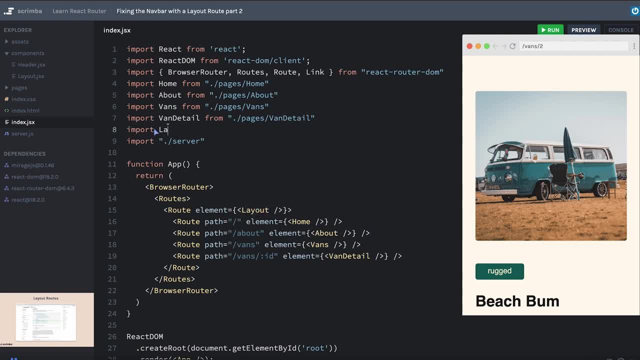 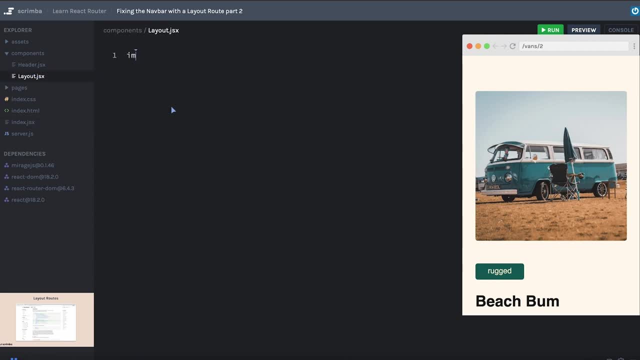 of all, we're not importing layout, So let's go ahead and import layout from our components folder slash layout, And then we need to actually create that, So we will get that set up. Okay, easy enough. This is obviously just a placeholder. Now I'm going to hit save. 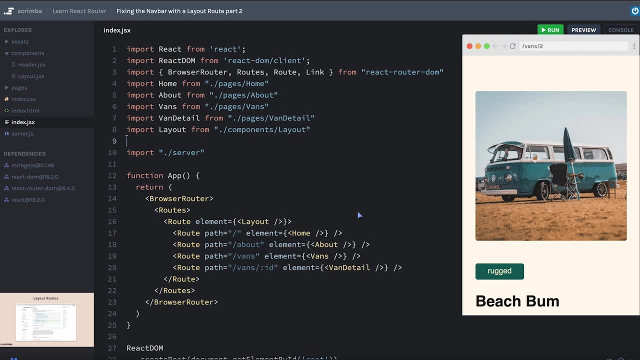 we're going to see what happens And then, well, yeah, let's just do that. I'm going to hit save. Okay, it's done. loading. This is everything that our site is now displaying at slash, van, slash two or, if I go to slash fans, also the same thing. Now, assuming you do have some experience using 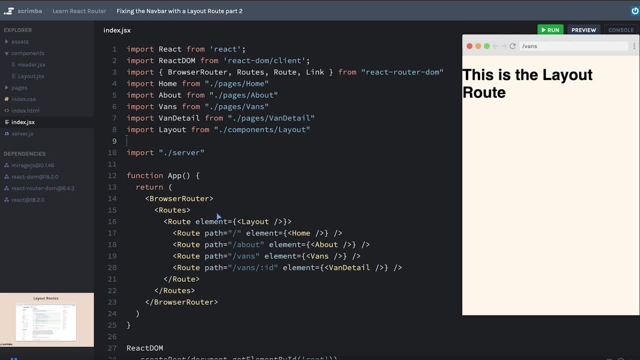 react children. I want you to think: why is it that this layout component has now completely taken over our app? it's the only thing being rendered here. If you'd like, you can pause for a minute to think about that. I wouldn't necessarily try to fix it quite yet, because 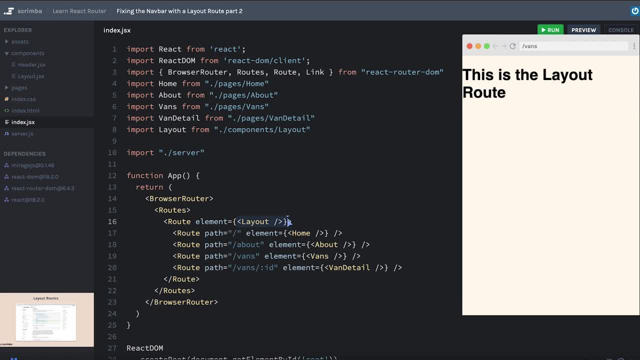 we haven't learned what we need to learn in order to fix it. If we were doing something like this, say, creating a layout component or actually rendering the layout component ourselves and wrapping it around, everything here like this, then we would have access to our route components inside of our 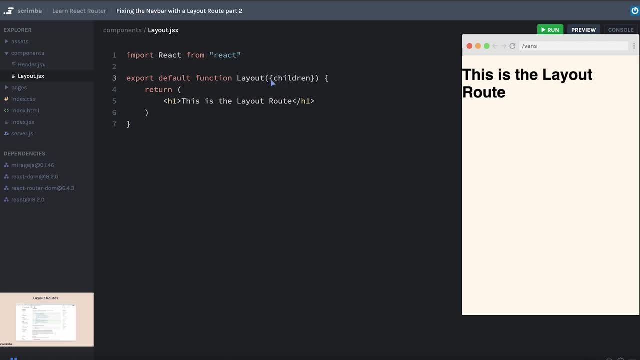 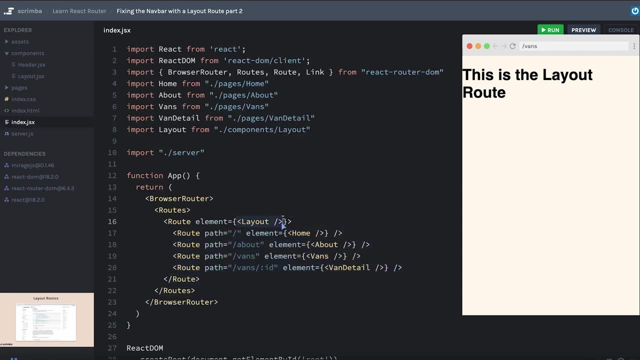 layout through the children prop. However, this isn't the right way to do it, because react router is not going to be able to render correctly if we do that. So when we have our layout as an element that we're passing to this route definition, there's a special tool that react router has. 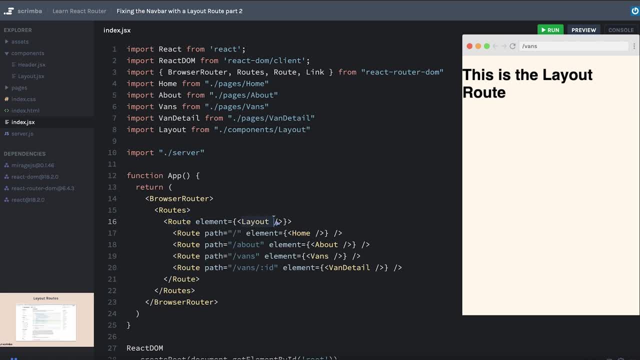 provided us so that we can render the layout, But then also tell it exactly where to render whichever route we're currently matching on the URL. For example, we're at the slash Vans route right now, so it should render the layout, and then we want it to render the Vans component that we're rendering here. 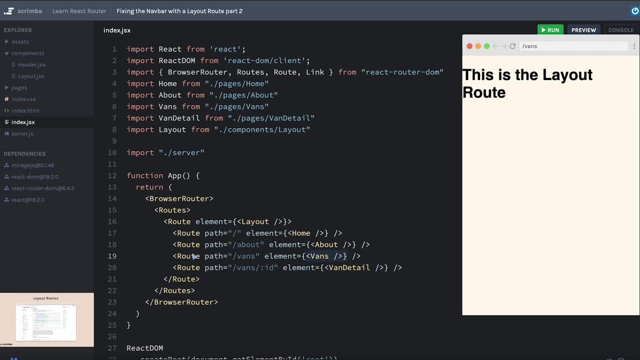 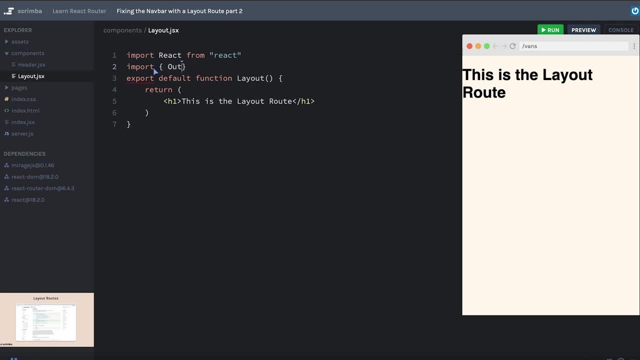 the element that we're rendering here or the element that we're passing to this route here. So let's go over to layout. and the tool that we're going to use is a component from react router, called outlet to spell it correctly. So we'll import that from react router, So we'll call this. 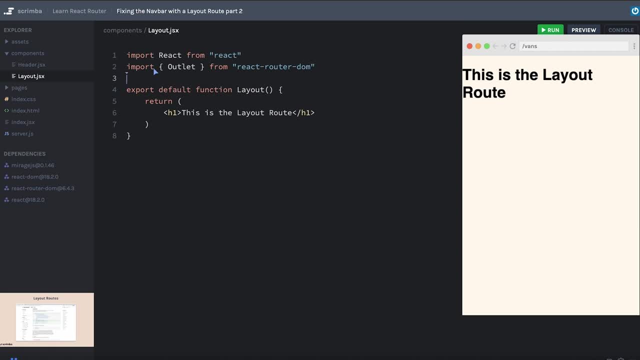 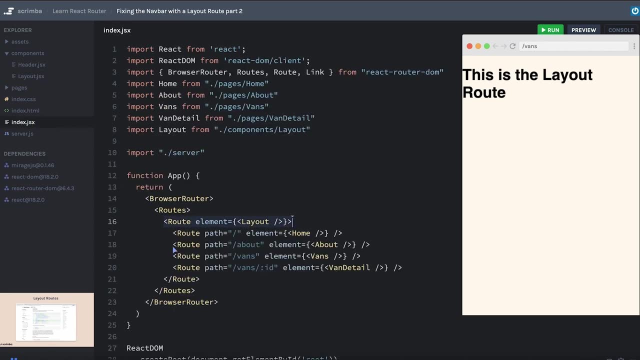 to router dom, And the outlet is basically our way to create a hole in whatever our component is, where the matching route that is, a child of the route that we're nesting here or the parent route. like this, the outlet creates a hole where the matching route can render. 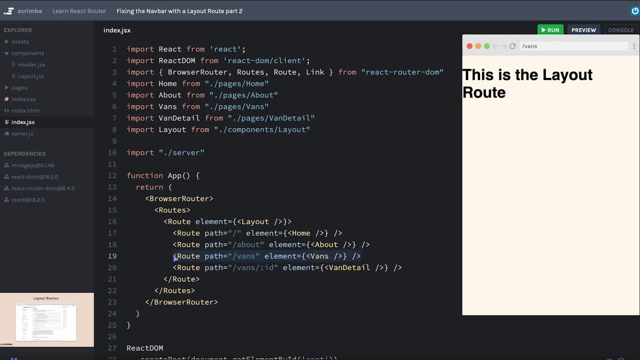 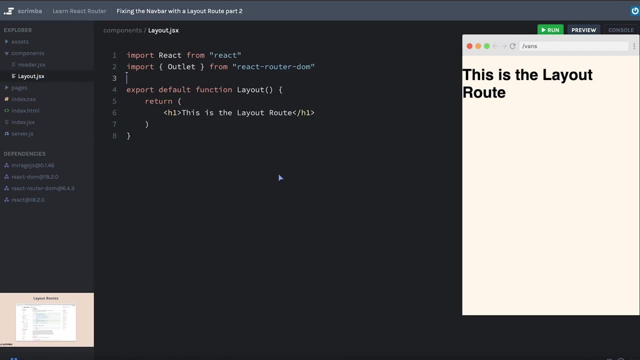 This took me a long time to wrap my head around, So don't feel bad if that doesn't make sense. Playing around with this is going to be the only way that it makes sense. if it didn't already, let's actually implement it, And then we'll go over it once again, So right. 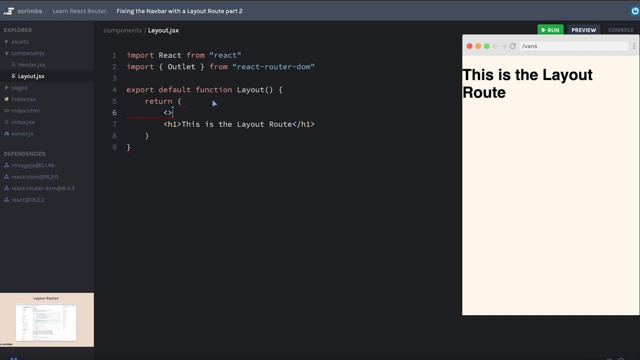 now I'm just rendering this h1, let's maybe put some fragments around this, just so we can actually render two things. And below my h1, I'm going to render the outlet as a component. So now I want you to think, when I hit Save, what is going to happen? Well, 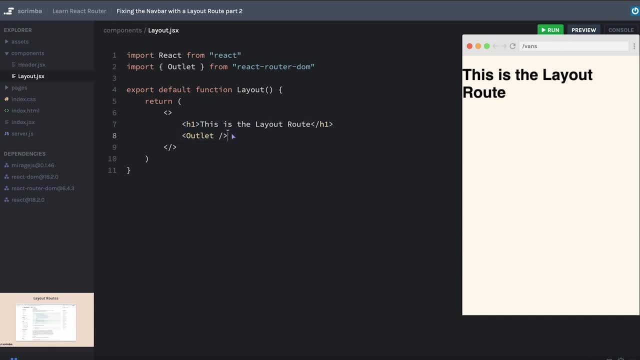 when I hit Save, I should get my h1 just like it is, But then I should also get the content that is supposed to display at slash fans. And sure enough, there we go. So this is the layout route. h1 up here is replacing our header, So we're going to fix that in. 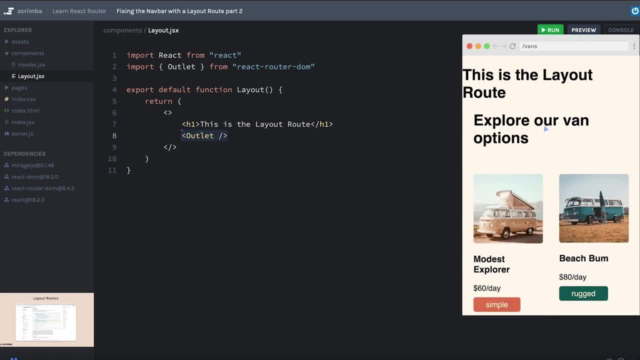 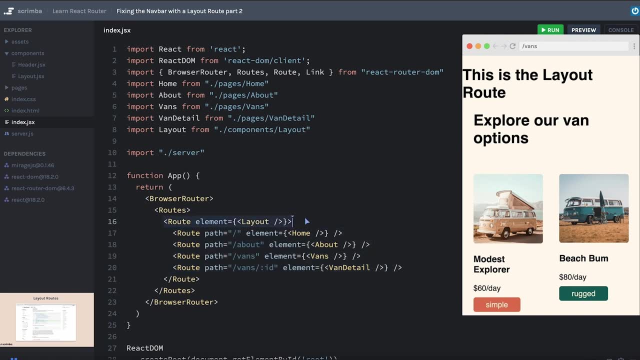 just a second. But now we have the rest of the slash bands page rendering below. So let's look at that once again, because we are nesting these routes inside of this parent route. React Router is going to notice that this route doesn't have a path, So it's always 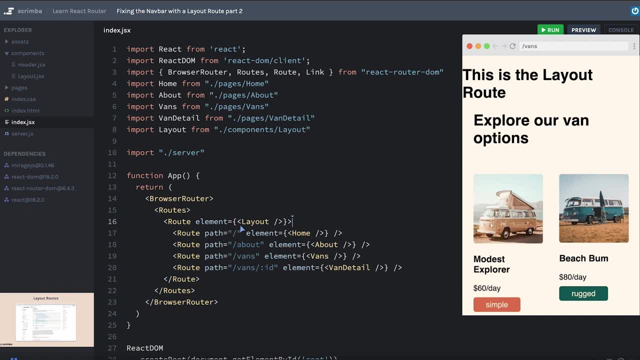 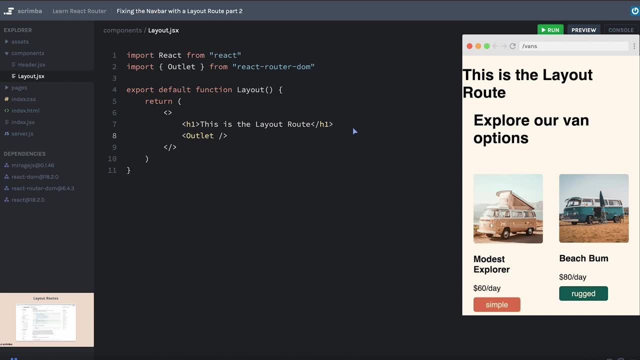 going to match whatever URL we're currently at And it's going to render our layout component. So when it renders our layout component, if we don't have some way to tell it, you know where to put the rest of the matching child routes, like we have currently slash Vans. 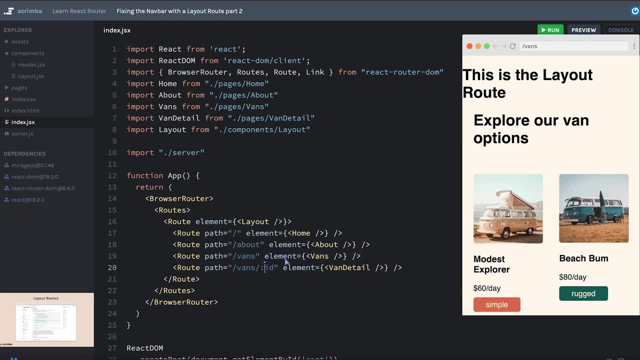 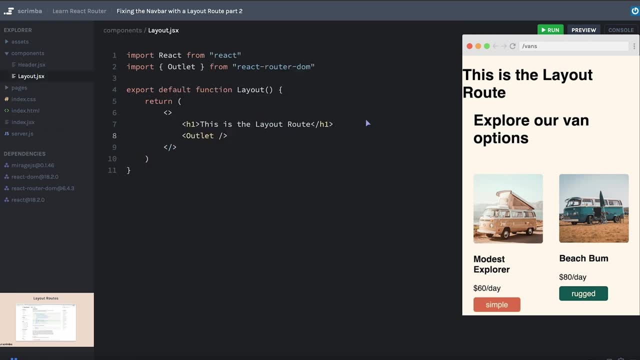 So this route path is going to match and we want to render this Vans element. we need to tell React Router inside the layout component where that Vans component should go, just like the children prop works in react children, where we get to tell it where the children 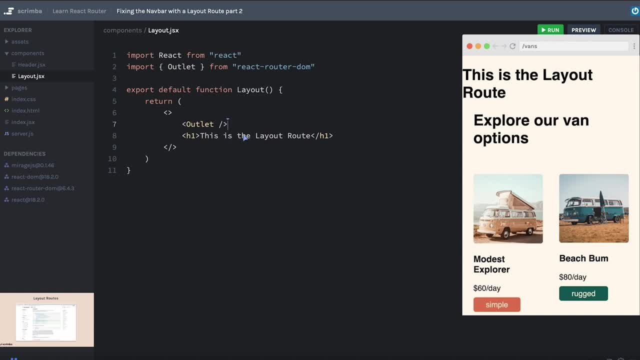 should be rendered. So I want you to think what is going to happen if I were to switch these two. I put the outlet on top and my h1 on bottom. you can pause the video. and you can pause if you want to think through it or if you want to run it and actually, 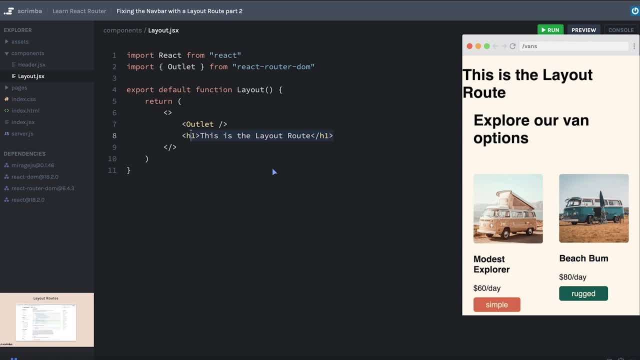 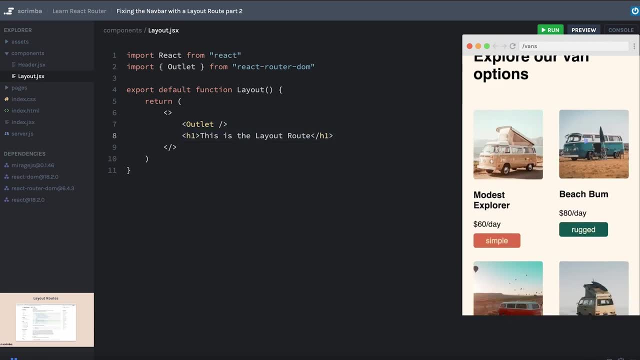 see what it does. Well, if I tell it that the content should be rendered first and then the h1 second, I'll hit save. we'll see that my content is first, and way down at the bottom we get our. this is the layout route h1.. Okay, now it's your time to shine. 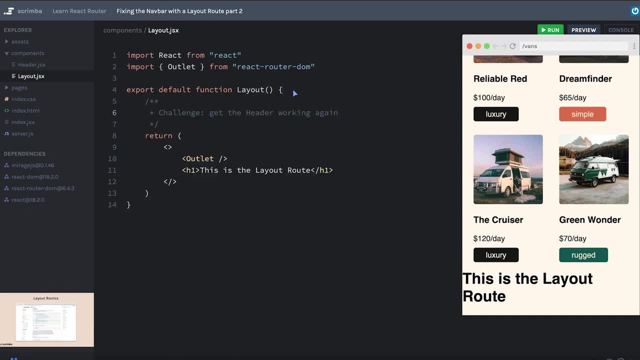 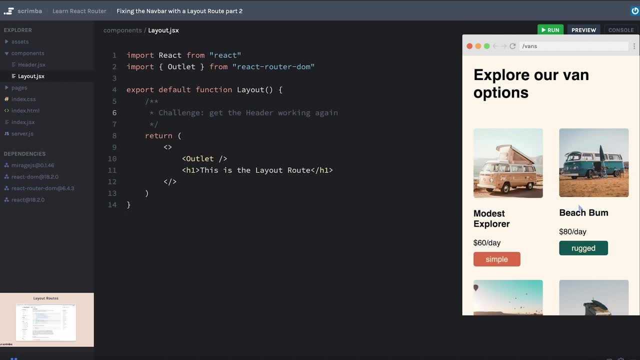 Let's do a challenge. I'll be a little bit vague. I want you to get the header working again. you'll know that it works. when you can go to the top of the page, you'll see our header. So let's go ahead and navigate between the pages again. pause now and fix our header. 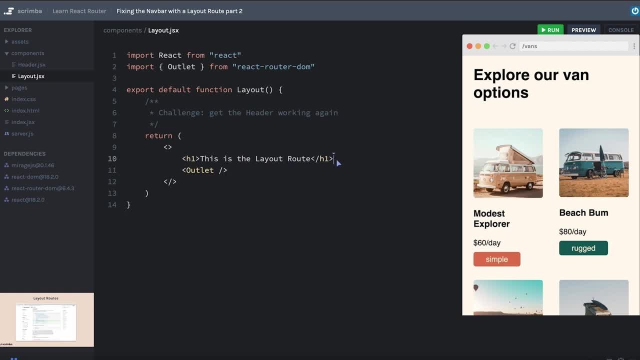 Well, everything should be set up for us. I'm going to move this outlet to the bottom And then, instead of using an h1, I'm going to simply import our header from, and let's see, it's inside the same folder. So I can just say dot, slash, header, and then I can render. 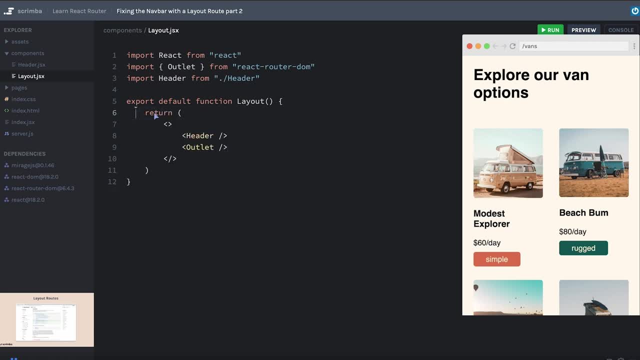 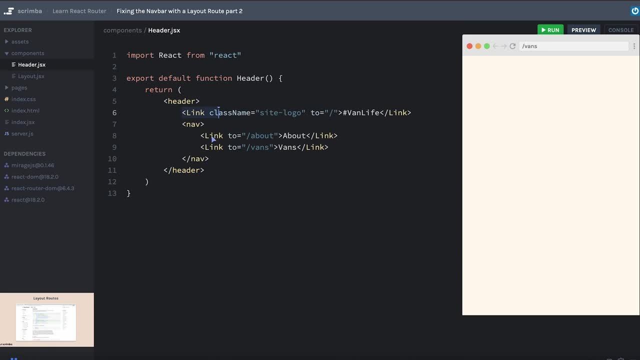 the header component And let's get rid of this challenge text. we'll cross our fingers and hit save. Ah, so close over in our header we're using the link component in a few places and I forgot to import that. Some of you were probably shouting at me about that And I 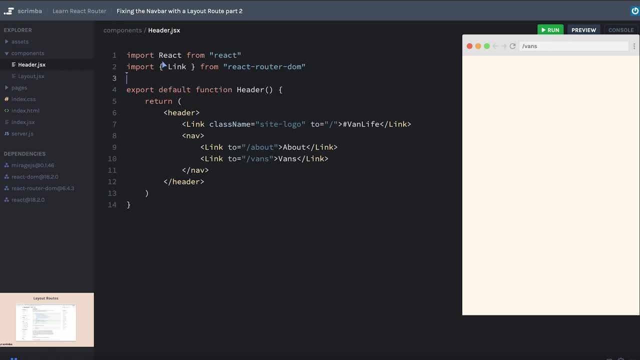 apologize, So react router DOM. Okay, let's hit save again. Awesome, I'm currently at the vans page. we see the list of vans. I can go into the vans detail page, go back to vans about the van lamp homepage. Now I know we're not working on nested routers. 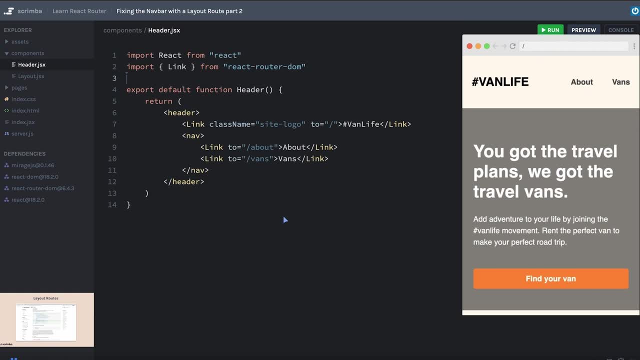 in the URL per se quite yet, but we are definitely going to get there. I think this is a great way to introduce the concept of nested routes And, most importantly, understanding how this outlet work. If it didn't totally make sense, that's okay. we're going to get a lot of practice. 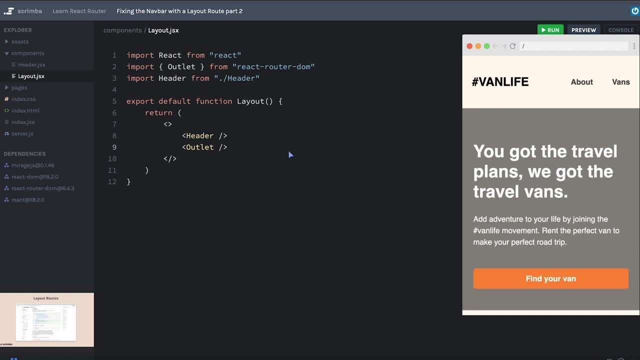 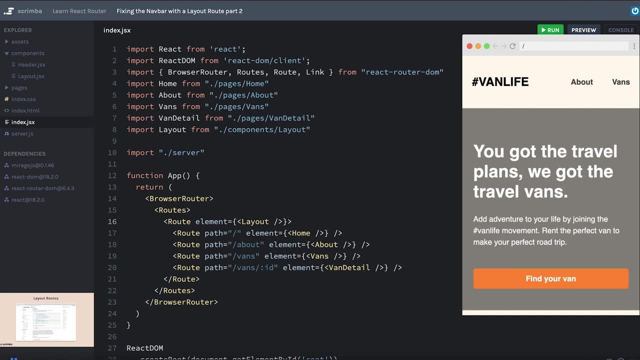 with it, But I've been blabbing on for a while. we've done a lot of good work here. we've got that ugly navbar pulled out of our browser router. the navbar wasn't ugly, but it felt ugly to have it here in the browser router. Now if, for some reason, I didn't want, let's. 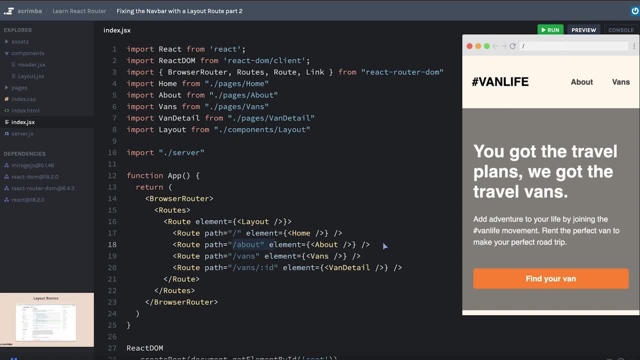 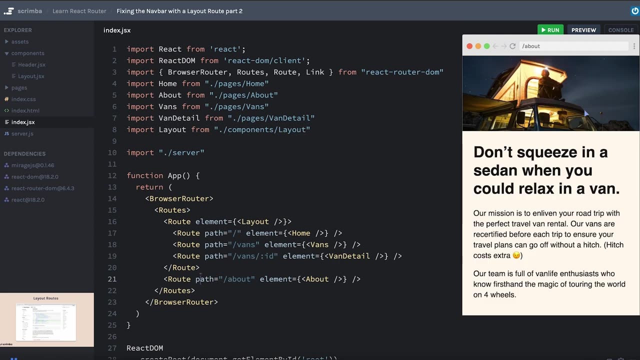 say the about page, to have access to the same navigation bar- and I wanted it to be completely different. I would need to move it outside of the children of this layout route, So that would just have to move down here And then I hit save. everything's working, But when I go to about, we lose our. 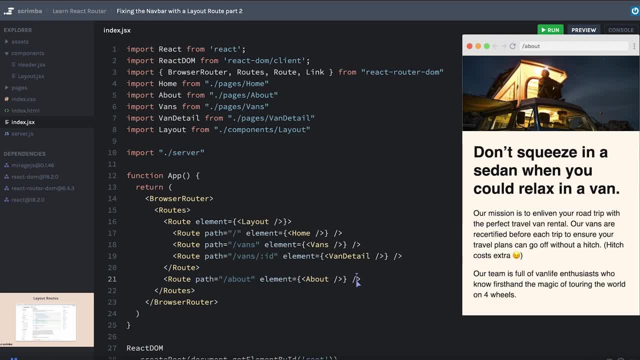 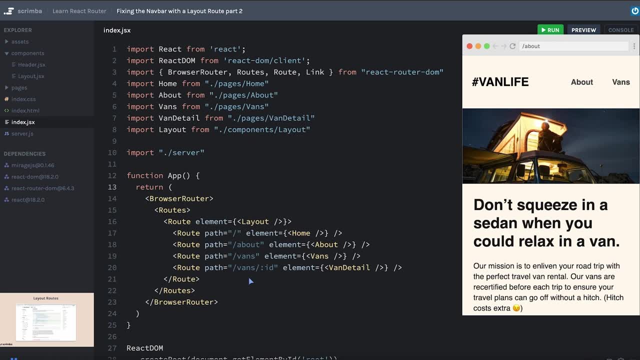 navigation bar. Hopefully that jives with your understanding of what we've been doing so far. Let's put it back in there So we can actually navigate back. Okay, with that under our belts, we're going to be bootstrapping out all of the host pages And remember there's 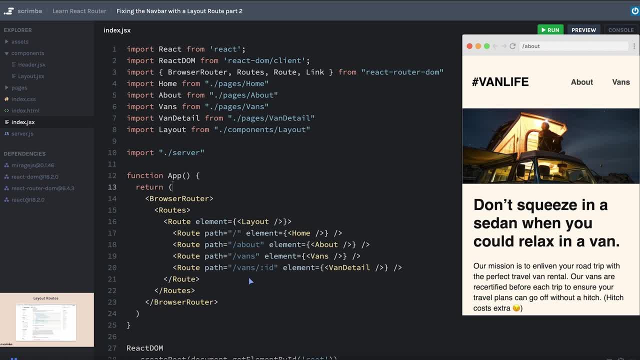 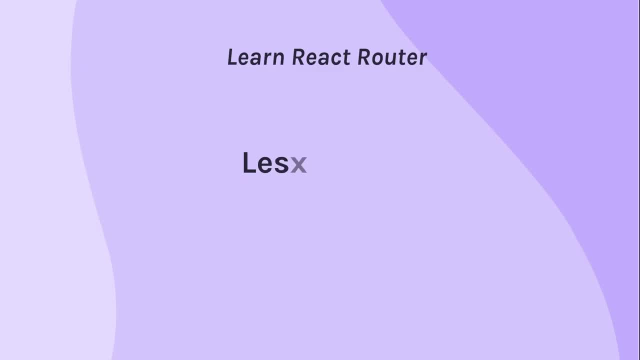 a lot of different cool shared user interface things that we're going to have to deal with with nesting. So we will get lots of practice with what we've talked about here. So when you're ready, that's what we'll start working on next. Okay, before we can dive into actually, 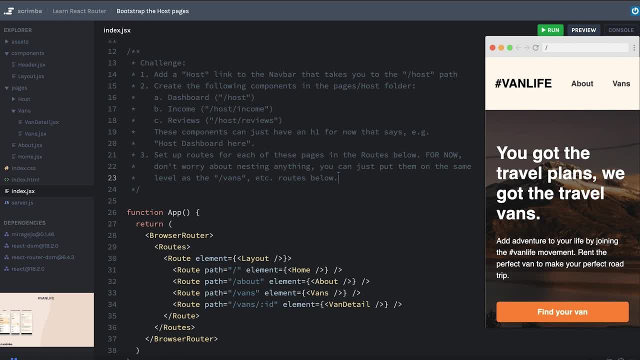 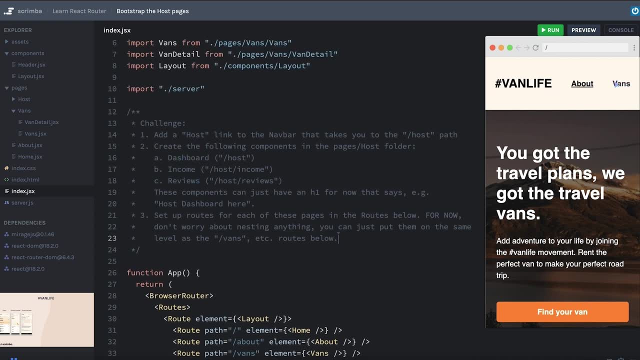 doing the nesting that we want to do. we're going to bootstrap out some of the pages that we need, And so that's going to be one of your first tasks. First of all, I want you to add a host link to the navbar. it should be before the about in vans, just over here. 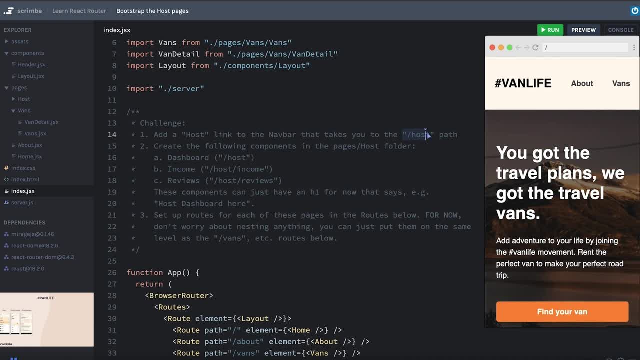 to the left And when it gets clicked it should take you to the slash host path, And of course, that won't happen until we set up the rest of this. But I want you to also create the following components that we see here: dashboard, income and reviews. I've organized things a little. 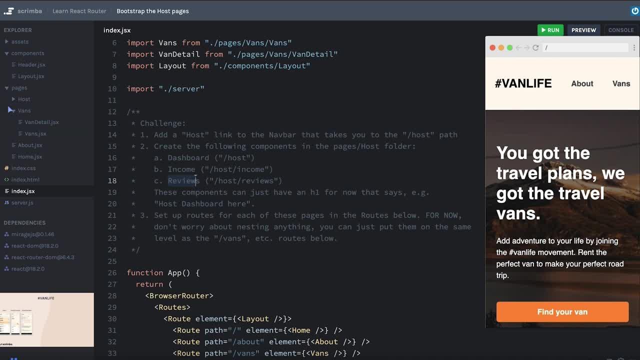 bit. I moved our van detail and vans pages into a dedicated vans folder, And so I've also created this host folder. Currently it's empty, And so you'll need to add these components there. I've also included the routes here, just in case you wanted a quick reference. 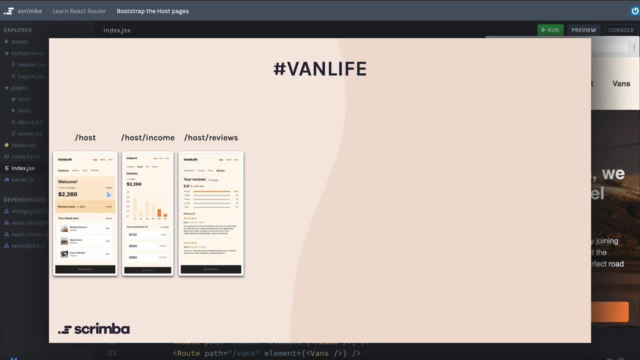 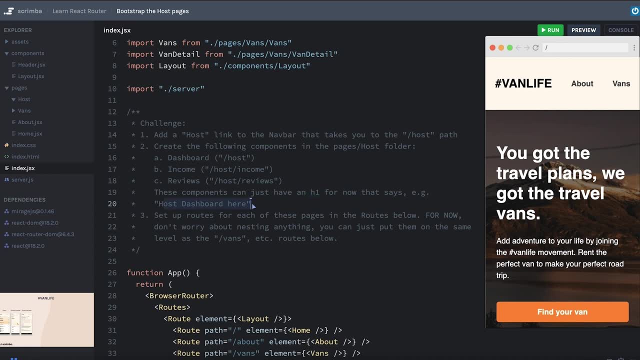 to them. I also pulled up the slide here in case, for some reason, this is better for visualizing it. And keep in mind, I don't need you to build the pages right now. I just want you to have maybe an h1 that says like post dashboard. 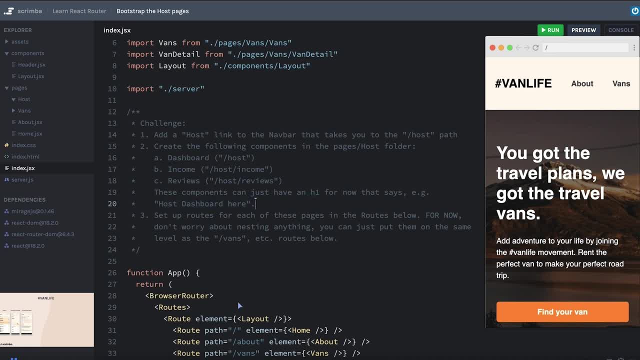 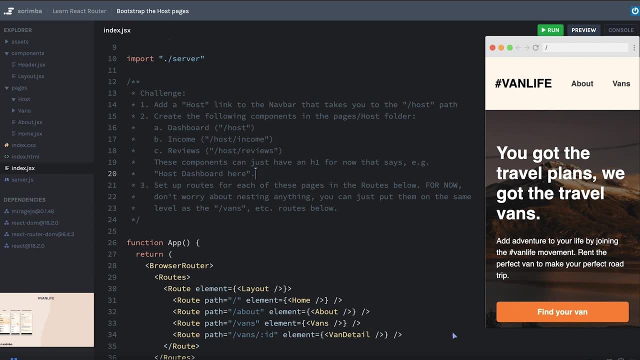 here And then, once you have those components ready, you'll need to import them And you'll set up the routes for each of those, Because we're just bootstrapping things, I don't want you to worry yet about doing any kind of nesting. you can just put everything as additional. 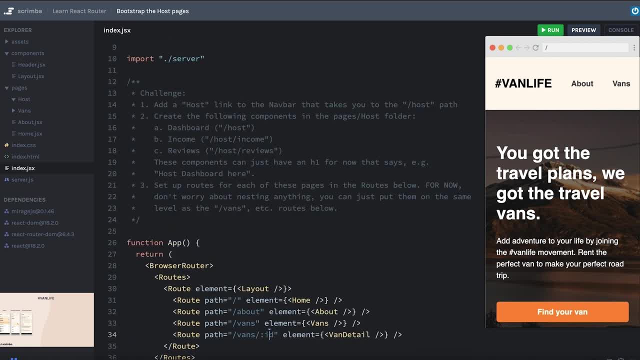 routes here, right on the same level as these other ones. All right, now it's your turn to get your hands on the keyboard. Pause now and work on the challenge. All right, let's get this done. So we'll first go to our header, which is where our 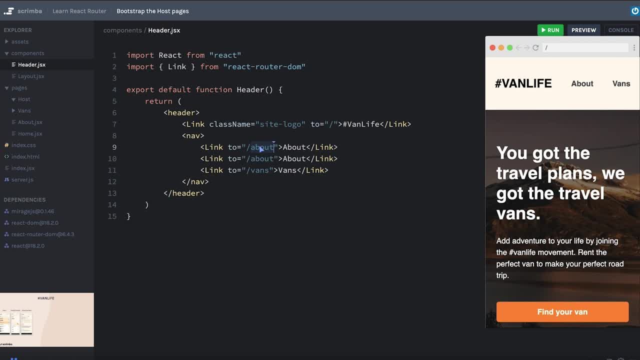 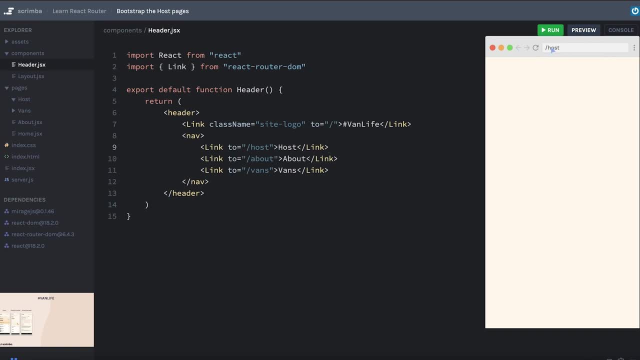 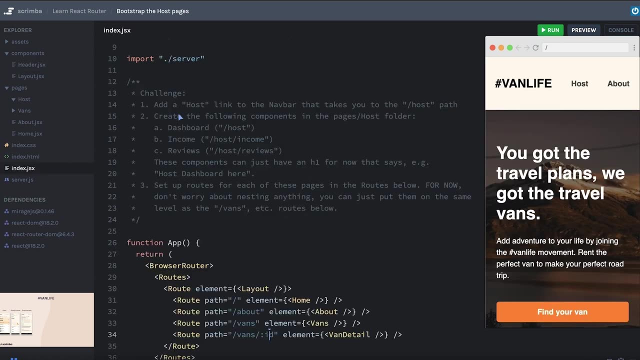 links are, we'll add another one that will take us to slash host Host. Awesome, Okay, easy start. If I go there, nothing's going to show up because we don't have any route that matches that. And oh no, I broke it. Okay, there we go, We're back. Okay, that's. 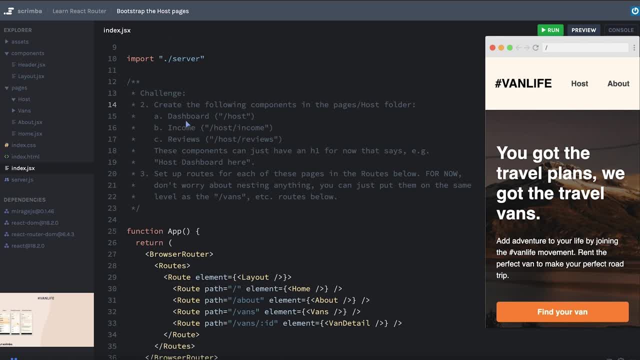 nice, Quick, easy win. We'll get rid of that. Okay, let's create some components here. So we're going to go to our header and we're going to add our links And then we're going to add another one that will take us to slash host. Awesome, Okay, easy start If I go there. let's go to our header. Okay, there we go. We're going to add another one that will take us to slash host. Awesome. Okay, there we go. We're going to add our links, And then we're going to add another one that will take us to slash host. Welcome to this new. 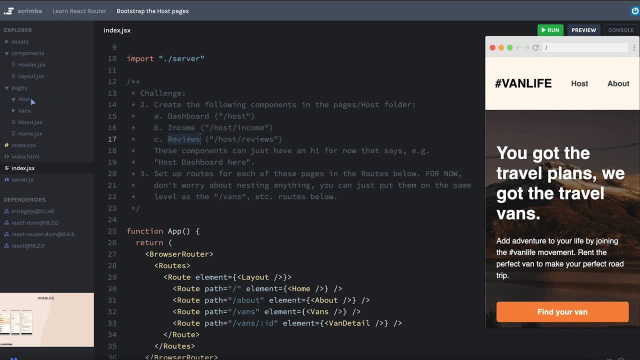 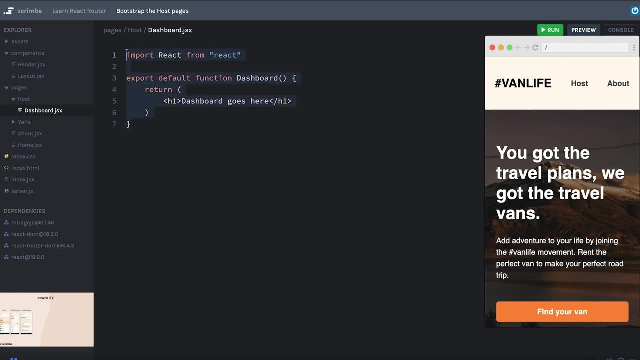 component: Dashboard, Income and Reviews. I won't bore you by making you watch me do all of this. So I just created a basic dashboard component and I'm going to do the exact same thing. In fact, I'm just going to copy this. 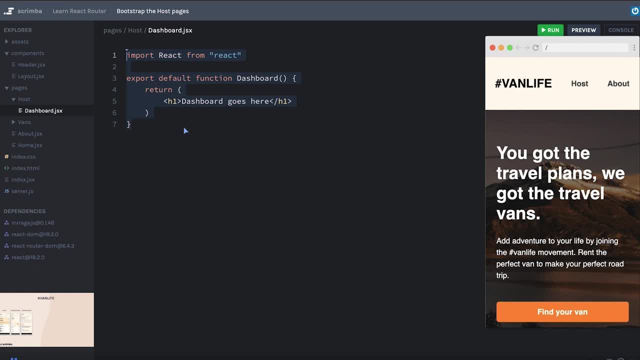 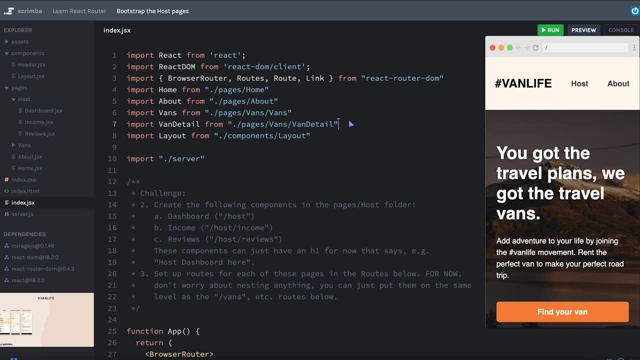 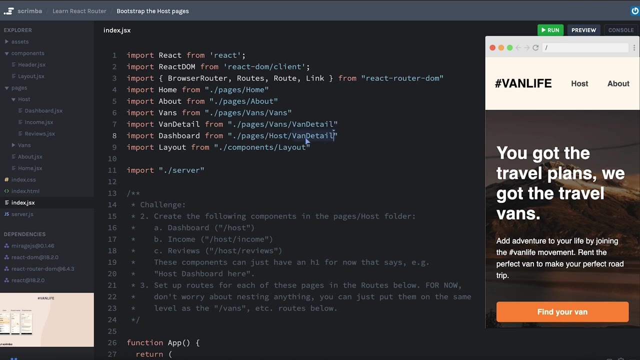 and paste it to some new components for the Income and the Reviews. Okay, so now we have the Income and Reviews done, Let's go to our index here and we will import those. We'll bring in. the Dashboard is going to be in the host folder and it's the dashboard component and then 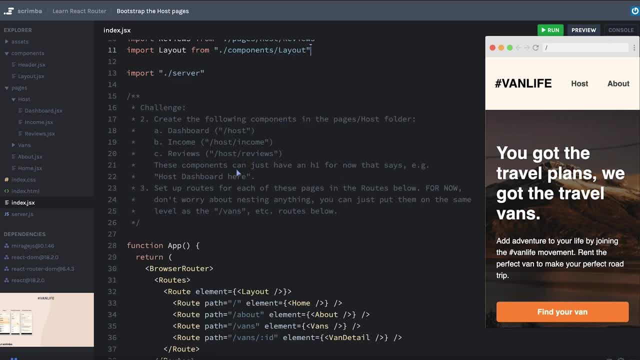 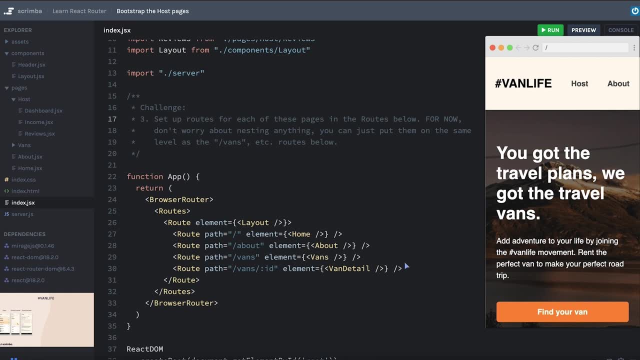 we'll just do that for the other two. okay, so challenge part number two is done and next we need to set up our routes. so I'm just going to take this vans route and see we need one, two, three of them, so we'll change vans to oh this. 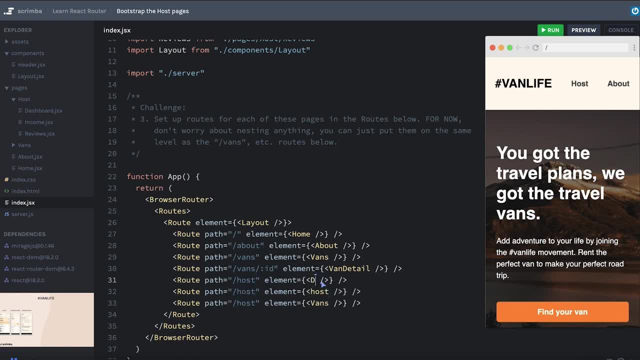 is wealth. that's okay. we'll change it to host and then I'm going to change this to the dashboard. I guess I could call this host dashboard or something if I wanted to be extra clear- and then this will be: slash host, slash income, that will be the income component and slash host, slash reviews, and that will be the. 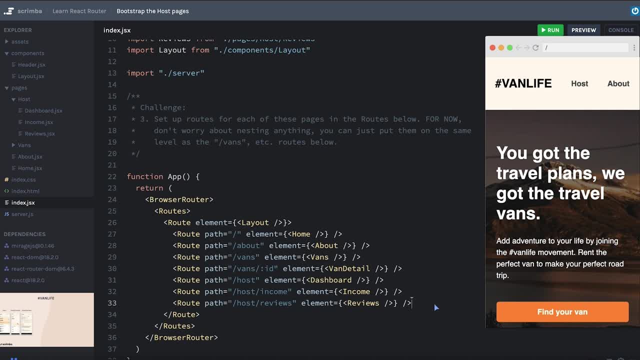 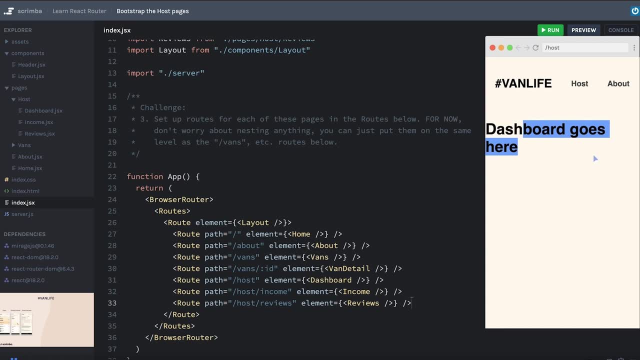 reviews component. okay, let's hit save. we're not broken. that's good news. I'm gonna go to the host and we'll see. dashboard goes here. that's good now. currently, we don't have any kind of navigation that will be able to take us to the income and reviews routes, so I'm just going to type it. 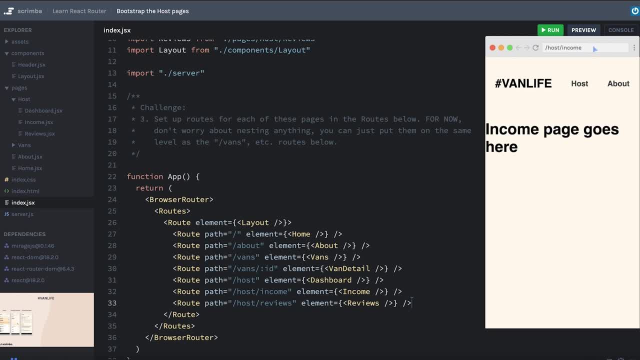 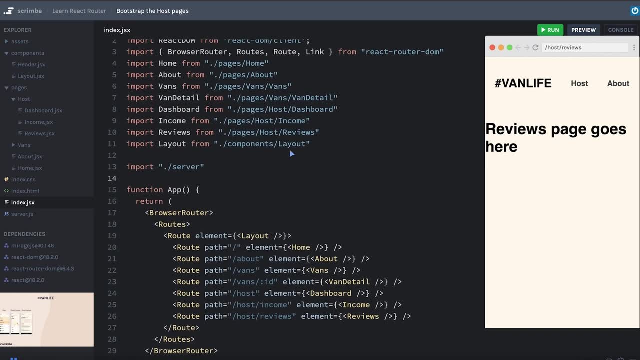 up here into the URL, we'll hit enter, okay. income page goes here. we'll do slash reviews- reviews page goes here. awesome. okay, that was all just some bootstrapping work, nothing too groundbreaking. but next we're going to see how we can actually, on our host page, have another navigation bar that will 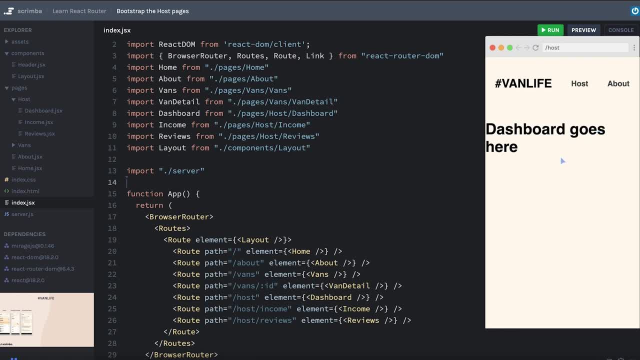 allow us to be a little more deeply nested so that we can navigate just through the different host pages. if anything that we did in this bootstrapping challenge here was difficult, then that's probably a good sign that it's time to get started, and I'll just go ahead and take a look at. 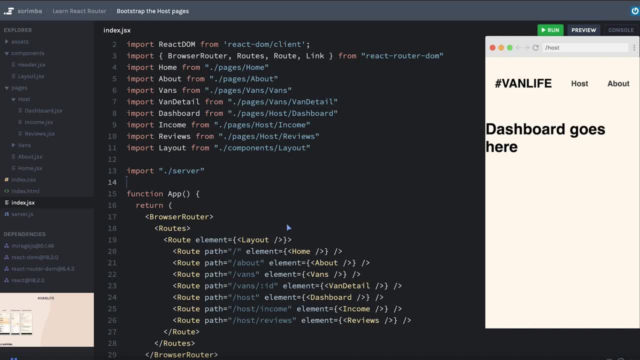 go back just review what you've learned. maybe it's been a little while since you've done it, but it really will be in your best interest to review what we've learned up until this point and try to catch yourself up. so, without further ado, let's start turning this into some more nested. 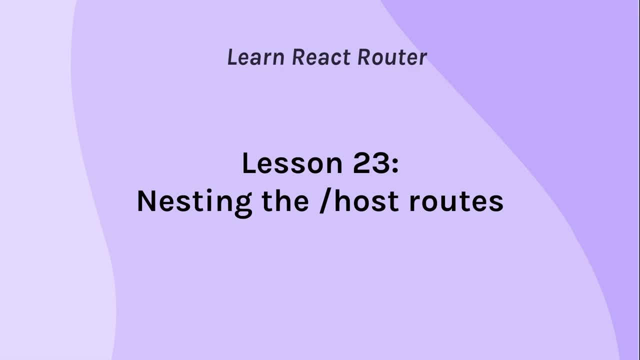 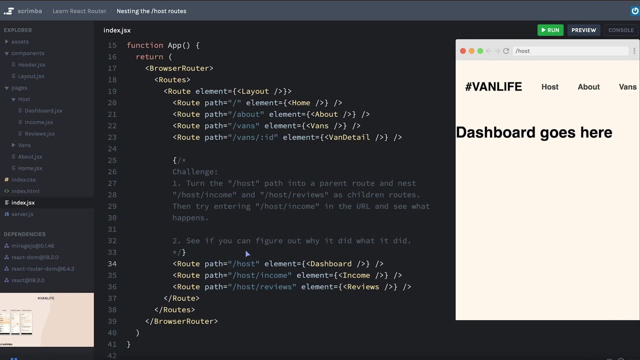 routes. okay, we are going to work on nesting these other routes inside of our slash host route and we're just going to take it one little step at a time. so your first challenge is to take this route that is for slash host and turn it into a parent route that surrounds the host income and 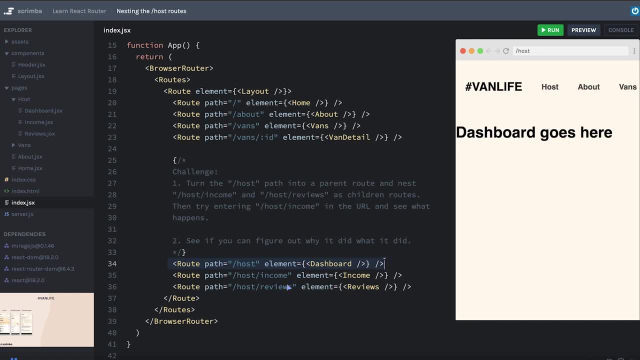 host, reviews- routes now, because we don't have a navigation bar to get to these other paths here. once you've done that, you'll go to the url and you'll type slash, host, income or reviews, it doesn't matter- hit enter and see what happens. once you've done that, i want you to pause and i want. 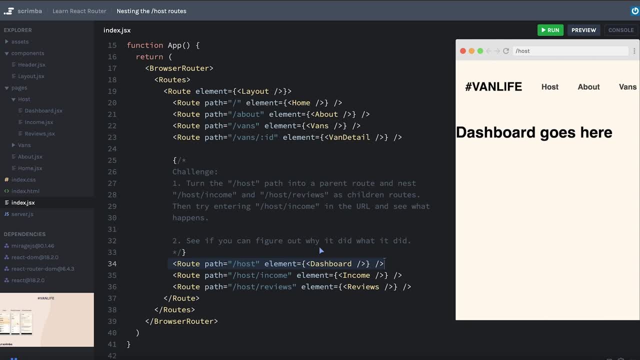 you to see if you can figure out why it did what it did. okay, so pause now and work on this challenge, okay. well, let's simply take this closing slash away so that we can turn this into a parent route here. we'll close it with a separate tag and move that down. we'll indent these nested ones now. okay. 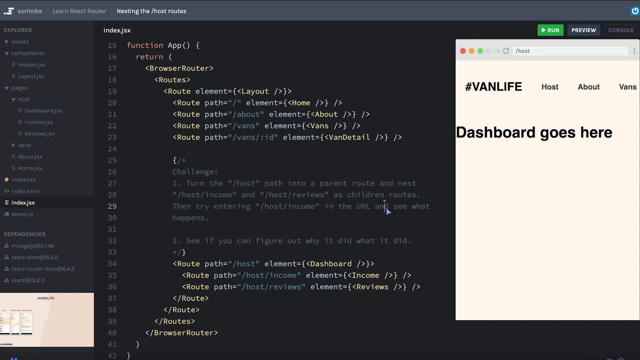 let's hit save again. we don't have any kind of navigation happening, so i'm going to type in slash income and hit enter and okay. well, here we are. it says we're at slash host income, but we're seeing that the dashboard goes here and we're not seeing the dashboard at any point. 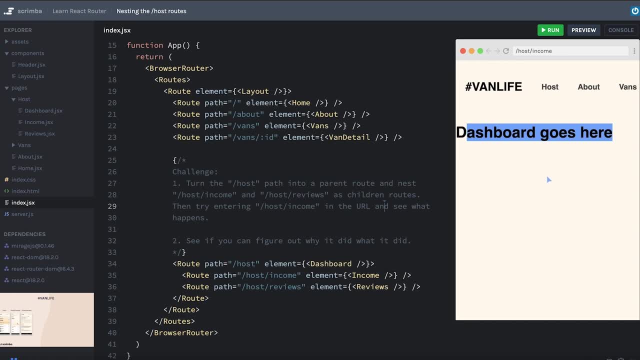 here seeing anything else, So maybe you figured it out. Kudos to you. if you did Remember, when we learned about layout routes, we learned that this route, as a parent to the other routes, needs to have some kind of hole inside of that layout so that React Router can know where to put the route. that 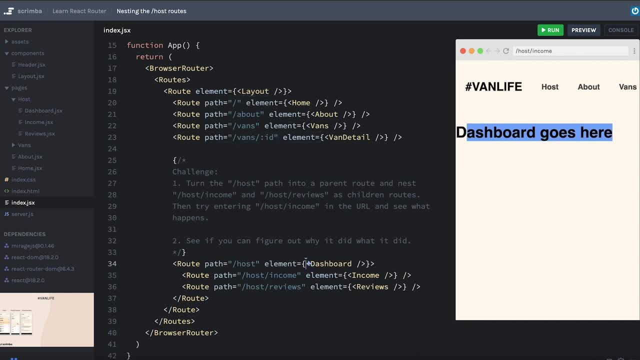 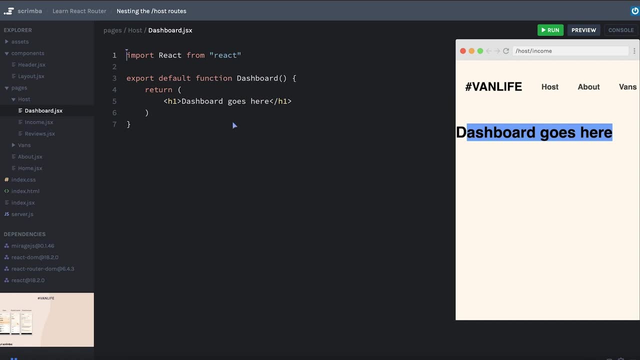 actually matches the URL. In this case, this dashboard element is acting like a layout route And if we go to our dashboard page, we don't have the outlet component here anywhere. So okay, let's say we go ahead and we import the outlet component from React Router DOM And let's just 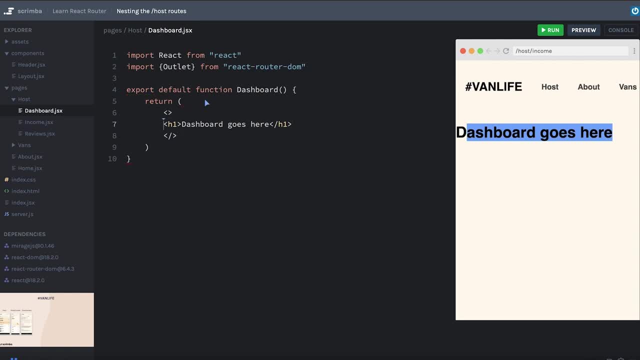 do a really quick fragment so that we can add our outlet. Let's save And look at that. we have our dashboard goes here. that's from this dashboard page, that's this h1. And then we have the outlet, which is the sort of placeholder for the route that's actually matching best to go. I guess the 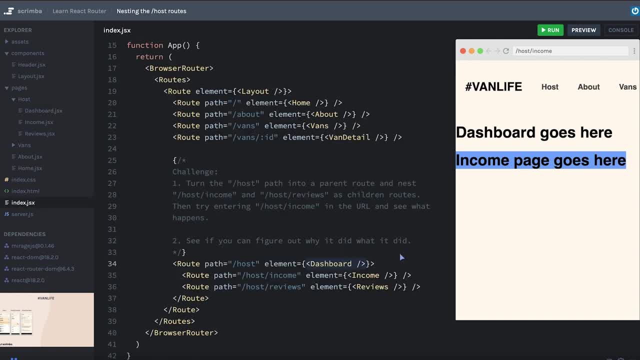 important thing to learn from this lesson is that the way React Router is working is that it's not just a placeholder. It's a placeholder that's actually matching best to go. It's matching multiple routes and deciding that multiple things can go on the page at one time. 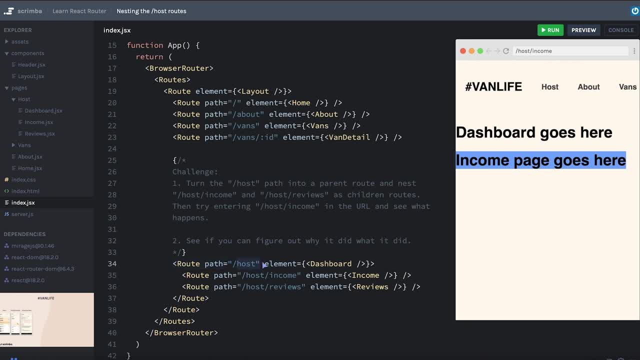 In this case, this route with the path of slash host is matching, And so it's displaying the dashboard, And, because our dashboard has an outlet, it's also matching this route here, And by matching I just mean that it's comparing our path in this route to what's actually in the 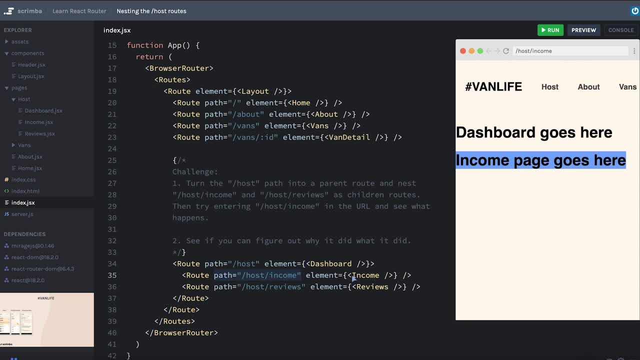 URL And because this route is matching, it's also displaying this income and it's putting it inside the outlet from its parent route. That's just a little bit of a tip there. It should have been review, but maybe seeing it in this slightly different context is helping. 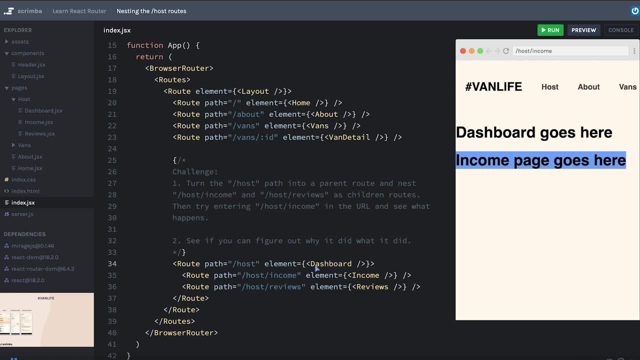 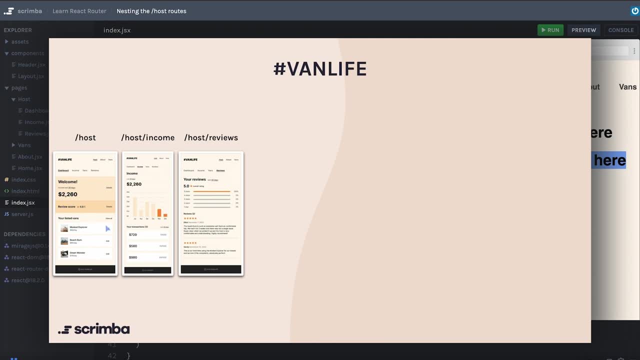 clarify that. Now, there's one major problem here, And that is that our dashboard is actually a different view altogether. It's going to have a summary of our earnings, our reviews, a quick summary of the vans that we're renting. So the dashboard isn't the shared user interface that 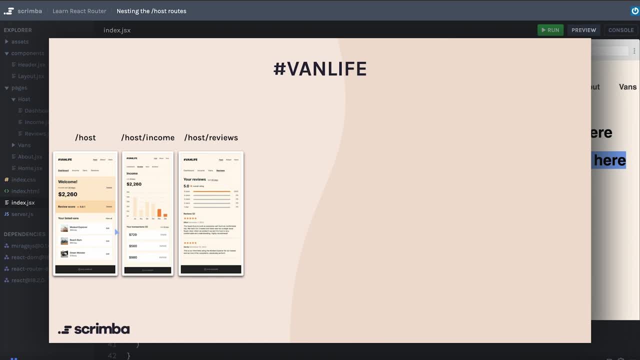 we want to share between these three routes. So think for a second: what is the shared interface that we want to share between these three routes? Well, it's this tiny little navigation bar at the top. So, in reality, what we need to create is: 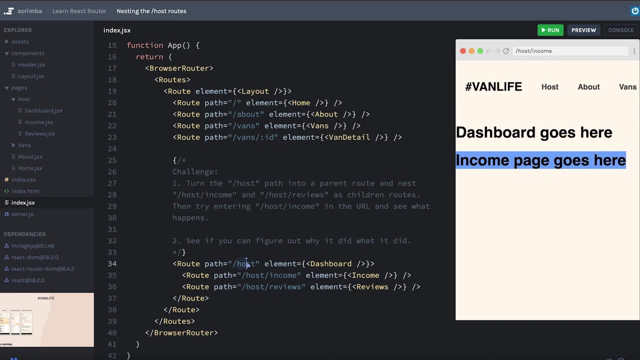 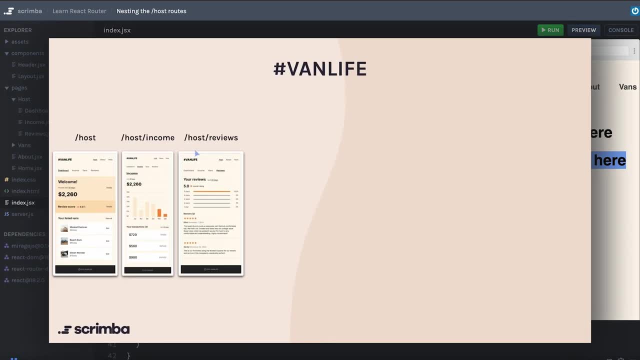 another layout route that is specific to the slash host route And this layout route is still going to be nested inside of our main layout route up here because we still want the top navigation and the footer. we don't have a footer but eventually the footer to exist. So in the next 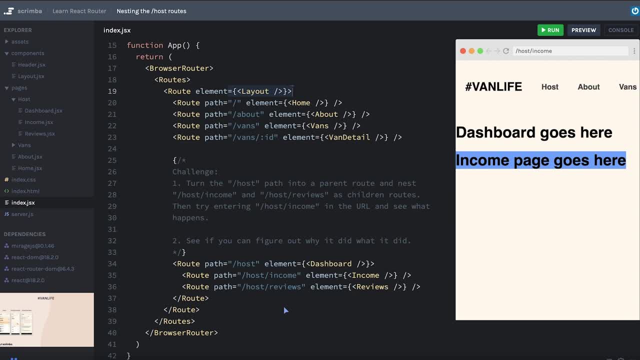 scrim. we'll have another challenge where we create another layout route- we'll call it the host layout- And we're going to create another challenge where we create another layout route and, thankfully, we'll create that little navigation so that we can actually navigate. 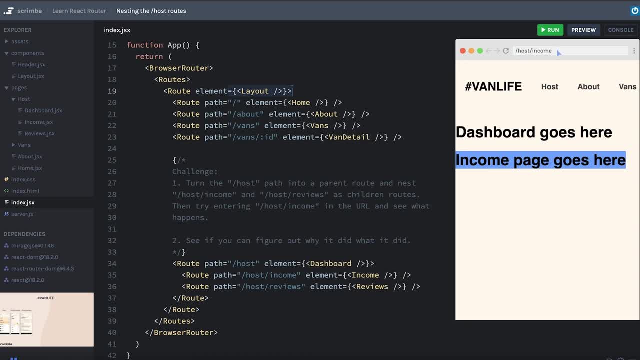 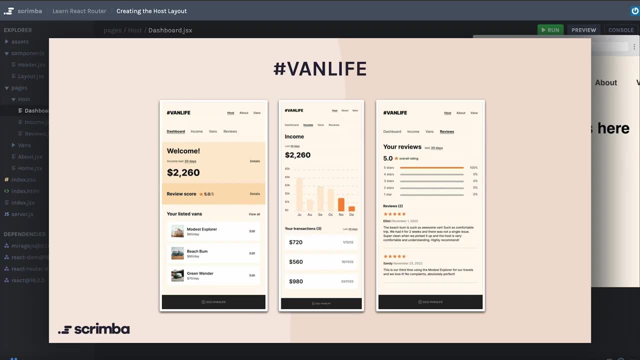 around this slash host nested routes without having to type anything in the URL. So that's what's coming up next. Before we jump into this challenge, we are going to backtrack on what we did on the dashboard file really quick. As you might remember, the dashboard itself is going to. 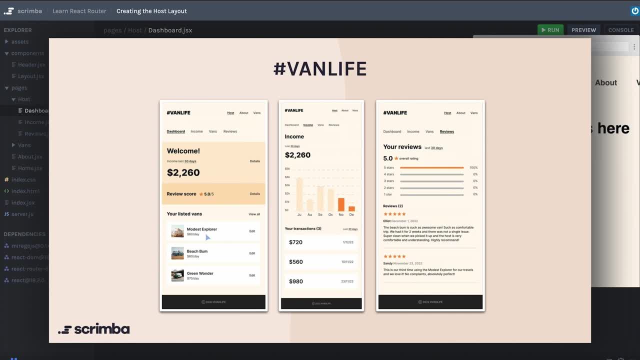 be the view that has sort of these summary stats And we also want it to include the navigation bar. but the navigation bar isn't really the dashboard, because if we navigate to another route, like the income or the reviews route, we want the navigation to stay, but we don't want the summary to stay. we want to switch. 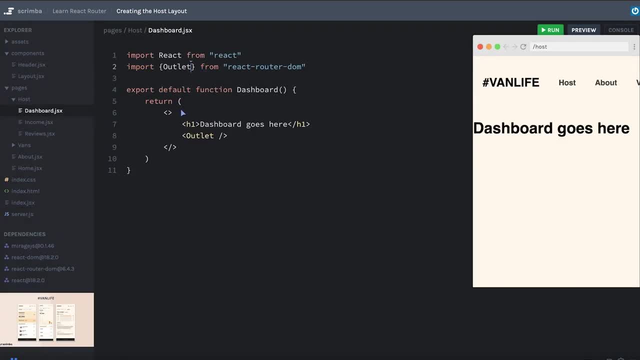 to those other routes. Currently, we set up our dashboard with this outlet, So we're just going to undo the changes that we made there so that we are all set to start now on the challenge for this scrim. So let me type that out. Okay, your challenge is to make the host layout component. 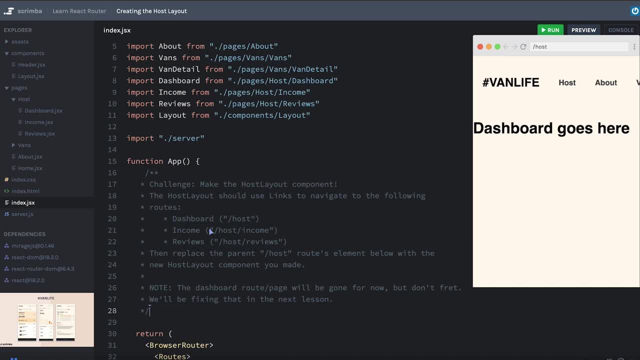 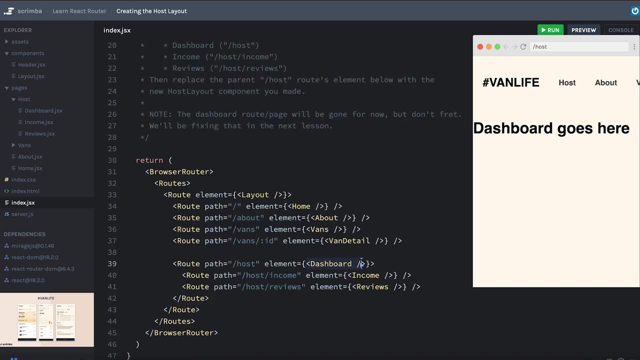 it's just going to have the navigation bar, but we don't want the summary to stay, So we're going to have the navigation bar for the dashboard, the income and the reviews, like it mentions here. once you have created that host layout component, you'll need to replace the dashboard being rendered here. 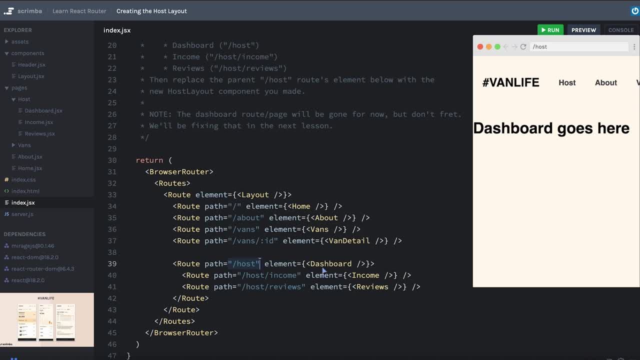 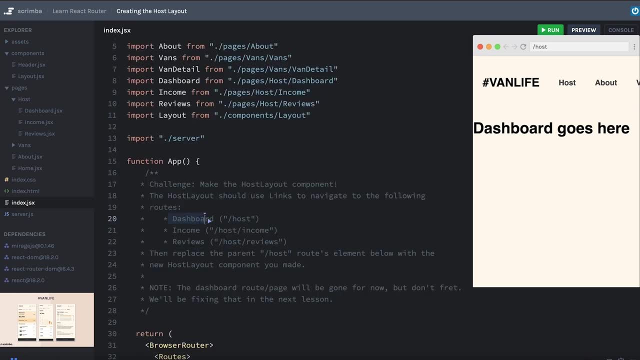 for our host route. As a caveat to this, it's going to make the dashboard disappear, But don't worry too much about that. we're going to fix that in the next lesson. So your navigation will include something called dashboard, but clicking it won't exactly show. dashboard. goes here the way that you 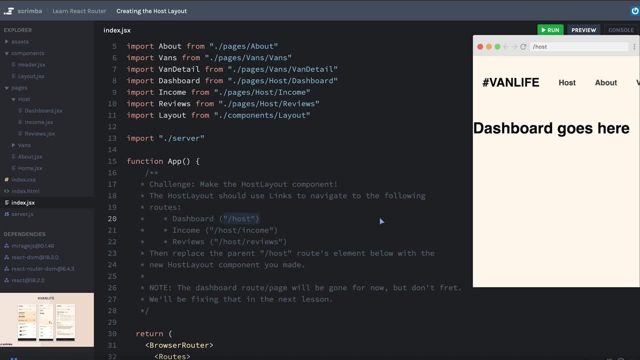 might think I've left out a couple of the steps that you'll need to take. So this is going to be a good challenge for you, And it will really test your knowledge and make sure that you've been following along with the challenges and understanding what we've been doing so far, especially regarding layout routes. So now it's your. 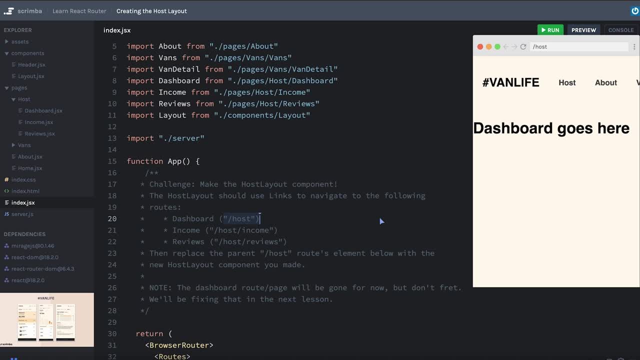 turn. pause now and work on the challenge. Okay, let's go over to components. I'm going to create my host layout in the components folder, not the pages folder. maybe there's an argument for doing it in the pages folder to me because, first of all, 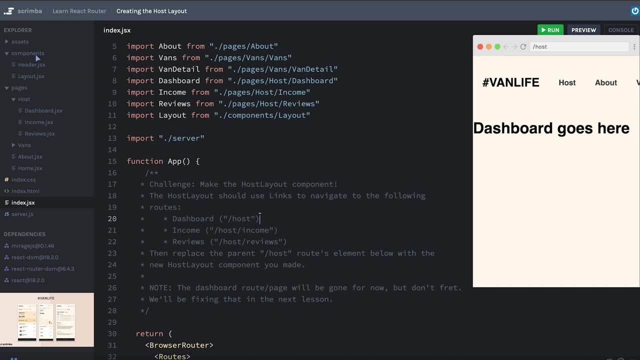 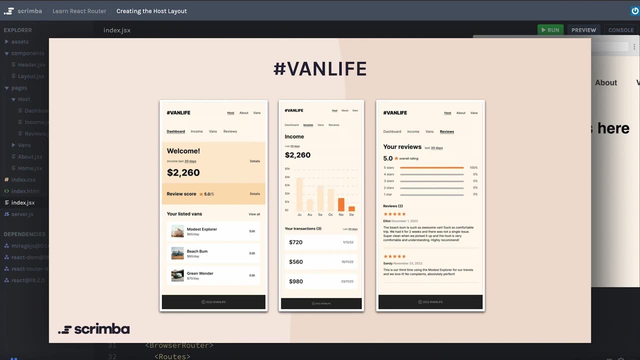 we have the layout component in the components folder. It makes sense to put the host layout component there. But secondly, this isn't really a full page per se. it's just this navigation bar that's going to be shared between the pages. So let's go ahead and create a new component. we'll call it. 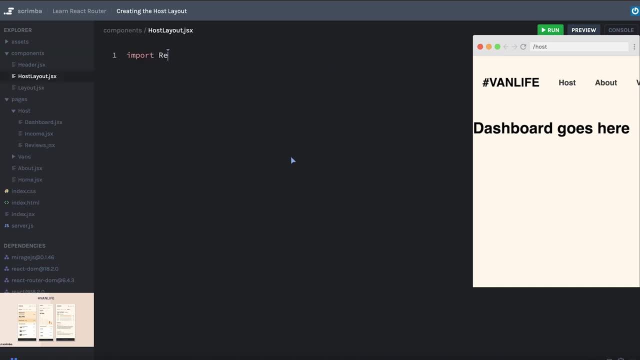 host layoutjsx And we'll just kind of get it set up like normal. For now we will just return an h1, just kind of do it one step at a time. We'll say host layout, then we need to make sure. 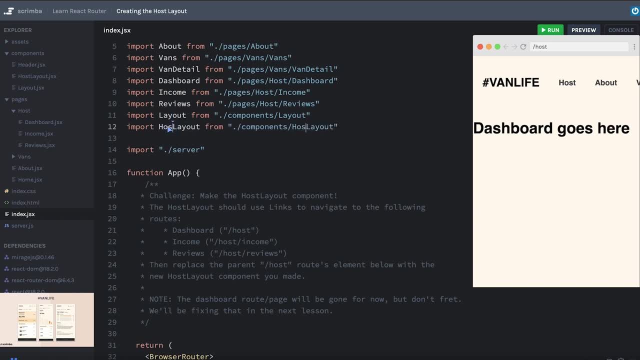 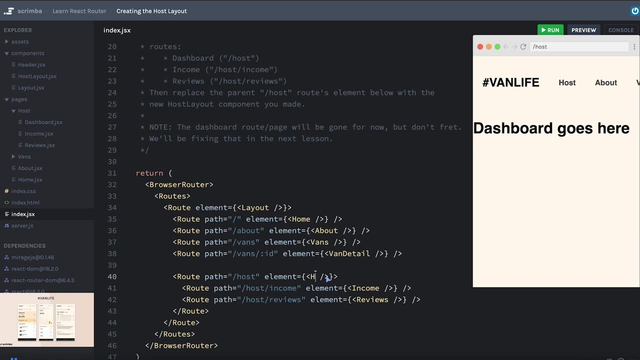 that we import that, So let's import it. import it at the top of this file: host layout. that was kind of a cool shortcut I could do there, and we'll replace the dashboard with host layout. We're at the slash host route. 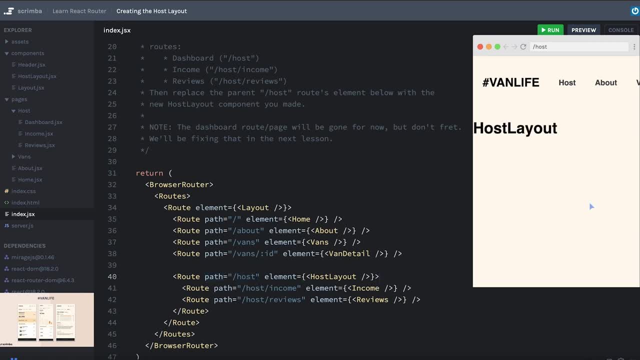 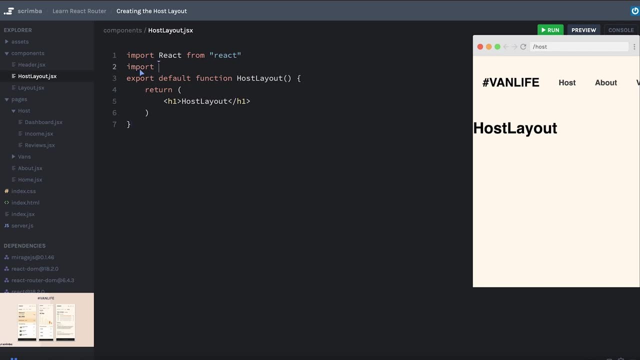 so going to that path should render the host layout and sure enough, there we are. Okay, let's go to the host layout. We know we need our navigation here and to navigate around we're going to use the link component from React Router DOM. 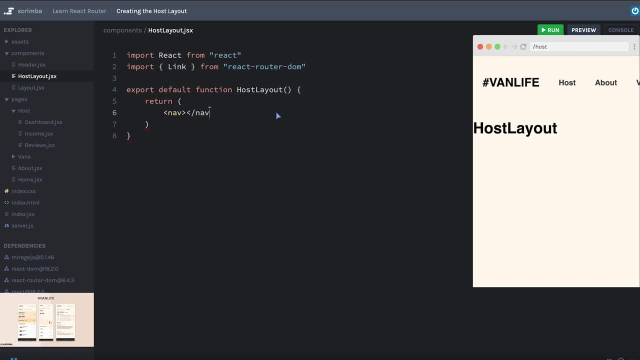 and let's use a nav element, since this is a navigation on the site, and we will create our links. So this is going to go to slash host. oh, not slash host, slash link. there we go. This will say dashboard. 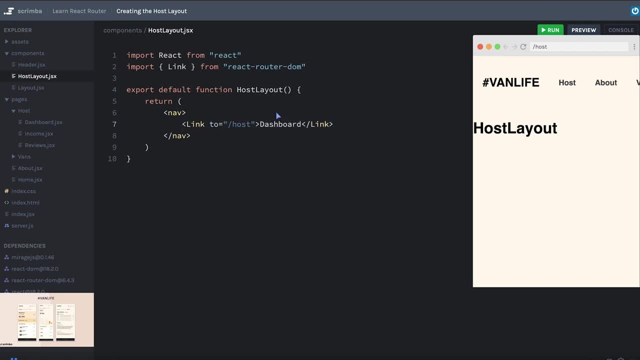 Again, this one's not going to be working the way that we think, but we'll fix that soon. Then we will create our other two. We're going to have slash. actually just here, let's see slash income, slash reviews. 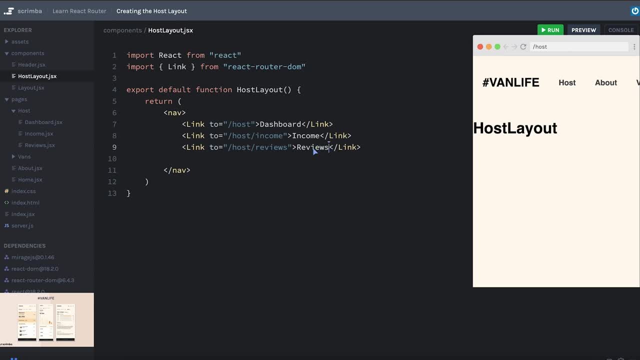 This will say income and this will say reviews. As a quick aside for anybody who may be already familiar a little bit with React Router, you might be screaming at me that I don't need these absolute paths, Even over here in our index. 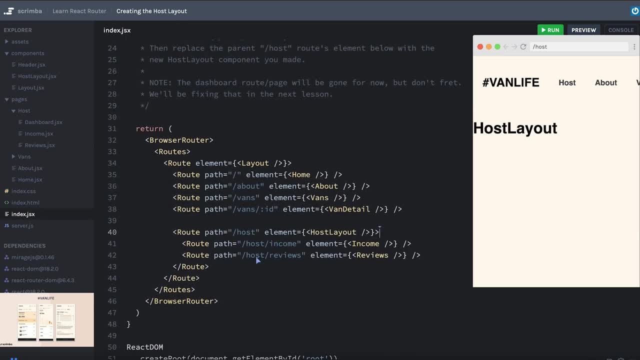 we have some repetition happening with slash host, slash host, slash host. so don't worry. If you know that there's a better way, I also know that there's a better way. We're going to learn about that very soon. If you have no idea what I'm talking about, 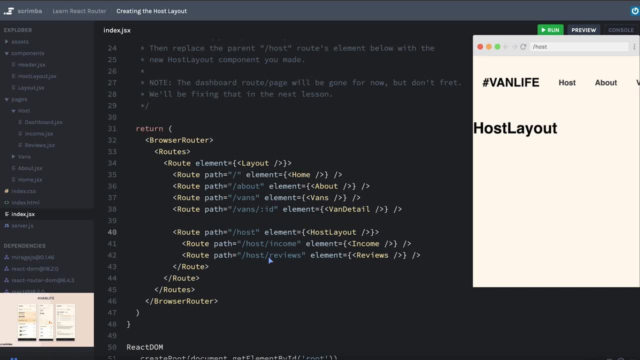 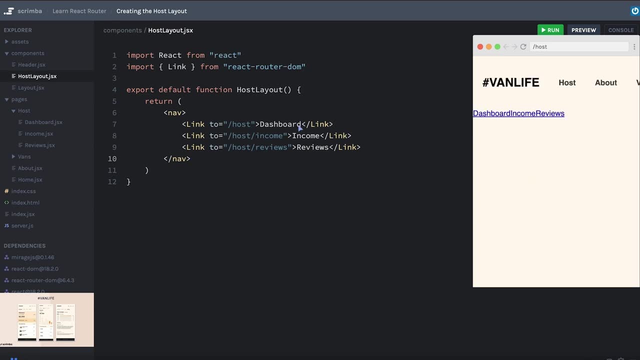 with relative paths or anything like that. don't worry about it, We will talk about it. Okay, let's go back to host layout. and well, let's go ahead and hit save. Okay, it's pretty ugly, so I'm going to call on my magic snap. 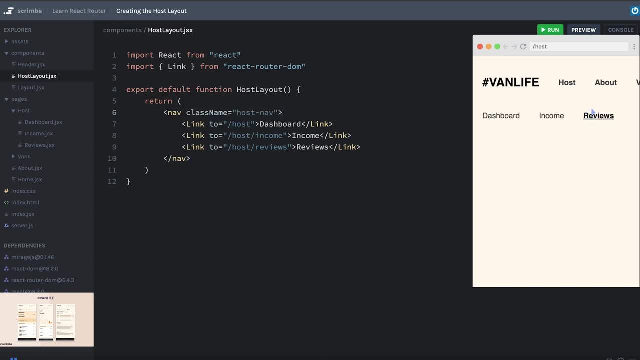 and here we are: perfect. It's a little basic, but the styling is there, so let's see if the functionality is there Now. we already talked about this dashboard. Well, we're at the dashboard. I'm clicking it. 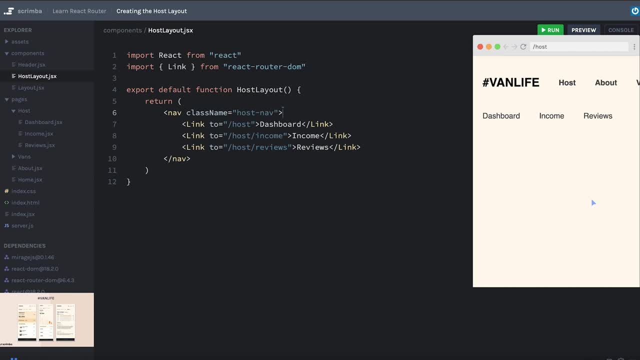 It's taking us to slash host, but nothing else is showing up, and well, actually, I'm getting ahead of myself. These will take us to slash reviews and slash income, but the part that I kind of left out was the fact that we would need the outlet. 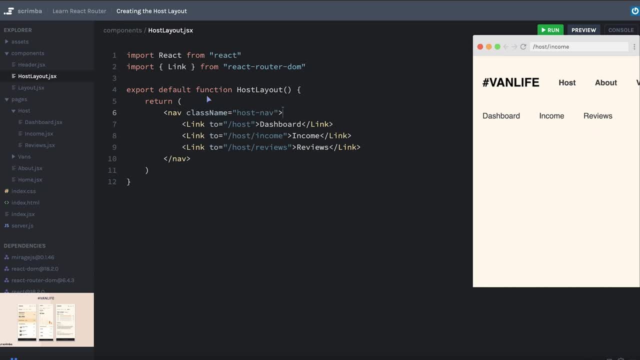 if we want to show any of the other parts of the page. so that's the next thing we need. Let's go ahead and import our outlet, and I will need to turn this into something a little different, so let's just wrap it in a fragment for now. 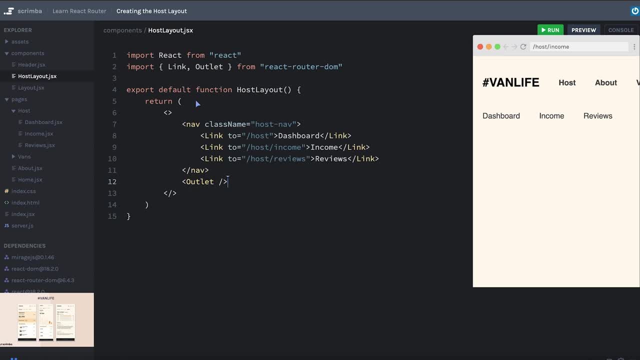 so that we can put more than one thing here and below our nav bar. we will render our outlet So let's save. Okay, awesome, We were at the slash host. slash income Income page goes here. That's, of course, where we would design. 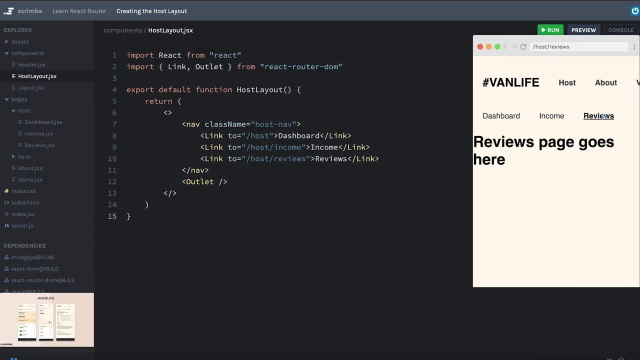 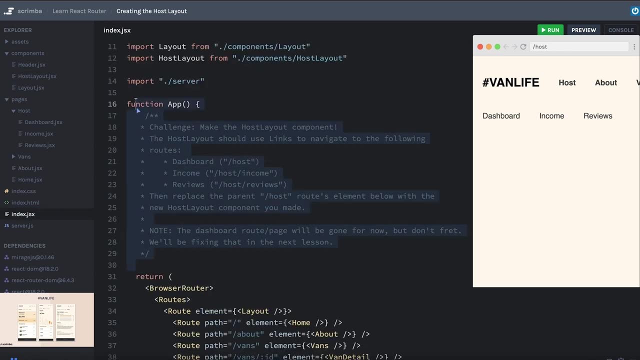 the actual income page. Okay, let's try reviews. Reviews page goes here. Awesome Dashboard- Uh-oh, nothing's there. Let's go look at our index and I'm gonna clean up this challenge here. I want you to look at this nested route setup. 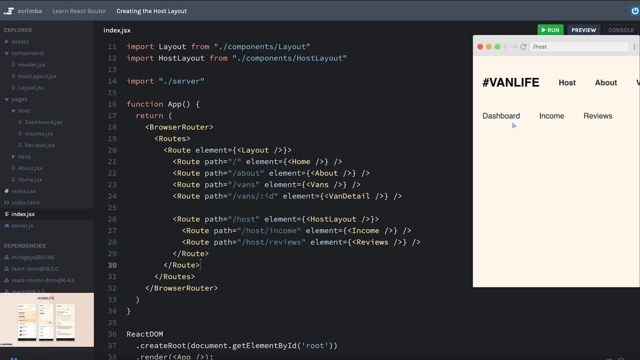 and see if you can figure out why it is that when we go to slash dashboard, our dashboard page is not actually showing up. In fact, you can even pause here if you need a little extra time. Well, one thing that might be obvious. 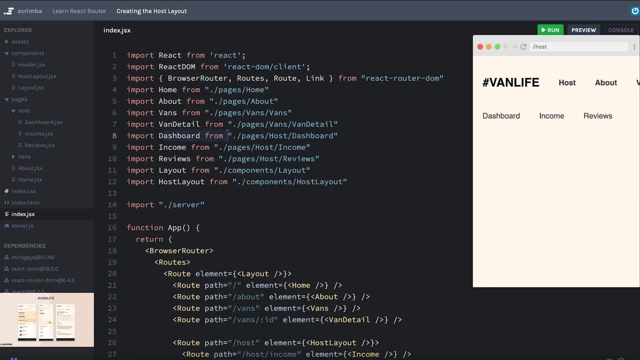 is that we are currently importing the dashboard but we're not using it anywhere, so the program has added absolutely no idea that we want the dashboard to be a part of this app. We had it right here with the host layout, but we needed to dedicate this parent route. 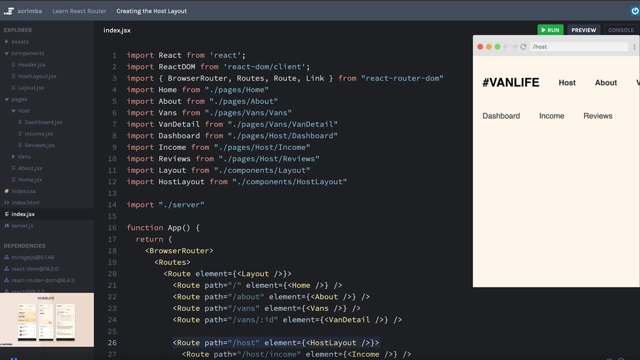 because the shared UI needs to be on the parent route to the host layout, so our dashboard is gone. Well, there's one way to fix this, but it's going to highlight what I was kind of alluding to a moment ago. 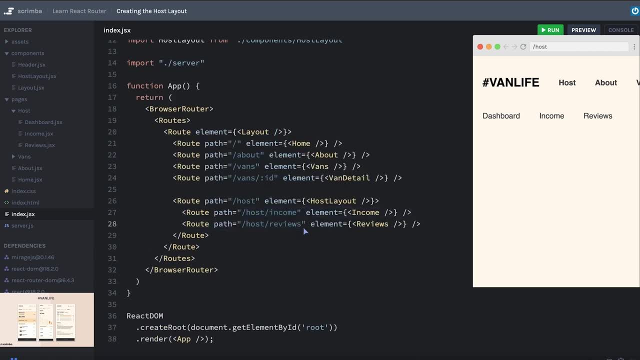 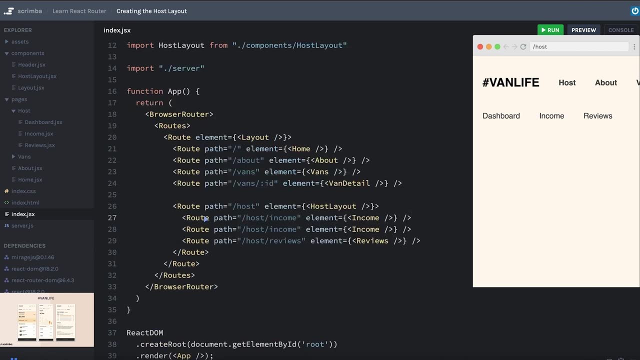 where I was saying that we have this kind of crazy nested repetition happening and we're going to eventually use relative routes to kind of fix this. So the workaround is, I could just, you know, repeat another path and say this one is also slash host. 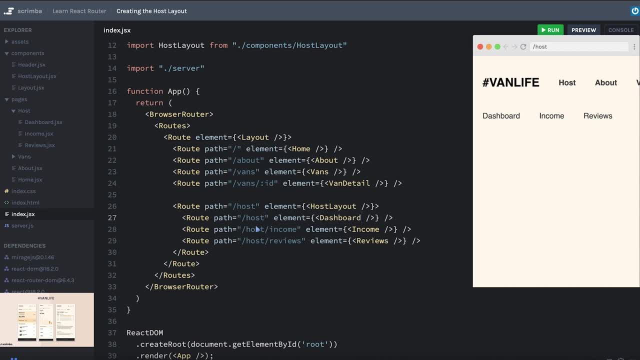 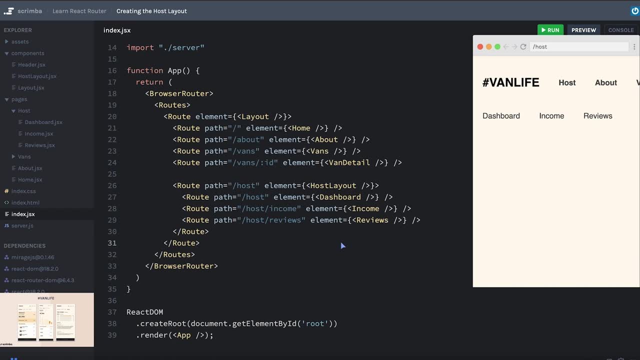 and the element should be dashboard. I want to make it very clear that you would never see this in production React Router 6 code, so I just want to make sure nobody takes this as their takeaway and decides this is how they want to do it. 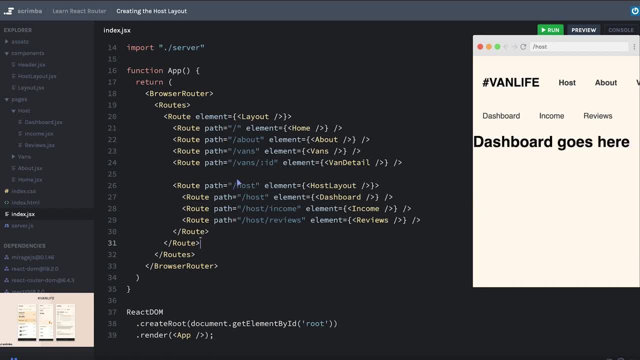 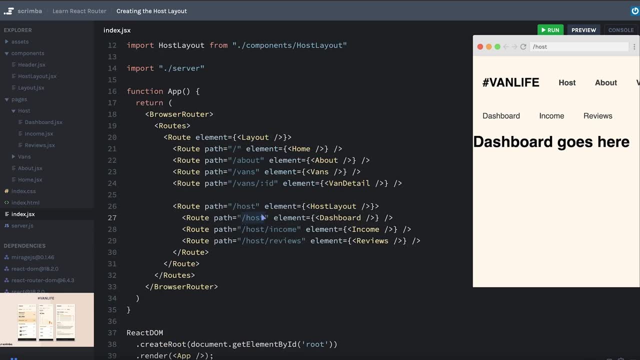 So let's hit save. Technically, our dashboard is showing up React Router is matching this route and it says the element is the host layout. and then it looks at this child route and it says: well, yeah, I already matched it. 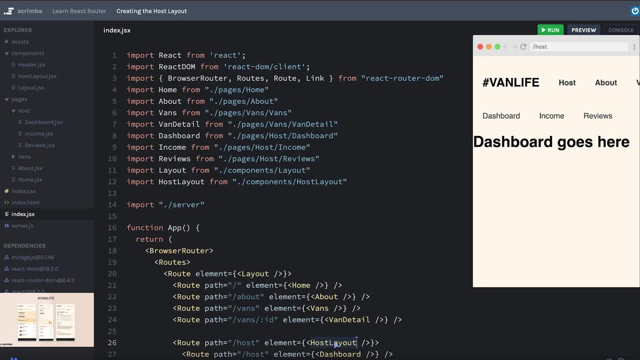 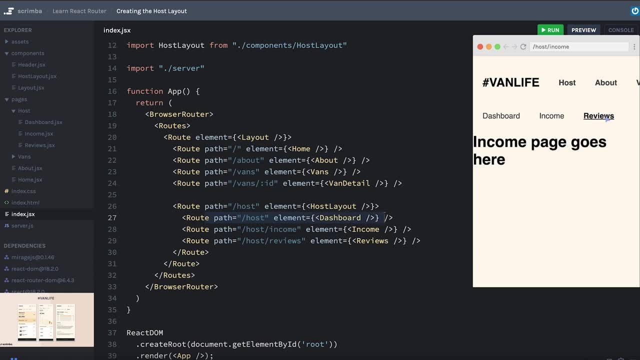 but I guess I can display this element too in the parent's output. So we have the host layout giving us this navigation bar and then the child route here displaying the dashboard as well. So technically this is working. but that leads us perfectly into the next topic. 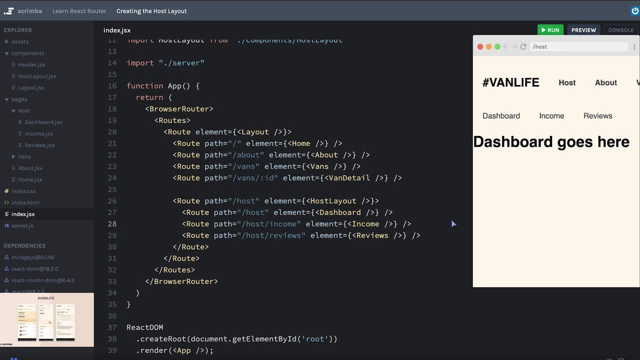 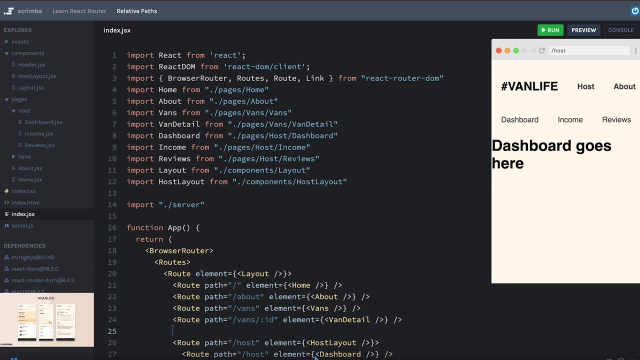 which is all about using relative routes. So that's what we'll learn about next. The way React Router works under the hood is when it is looking at a child route, like the ones we have here and here and, technically, this one here as well. 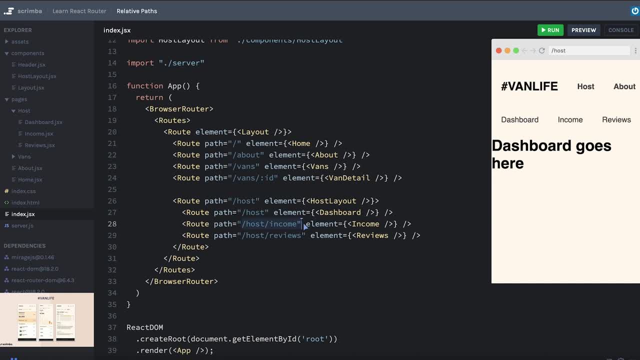 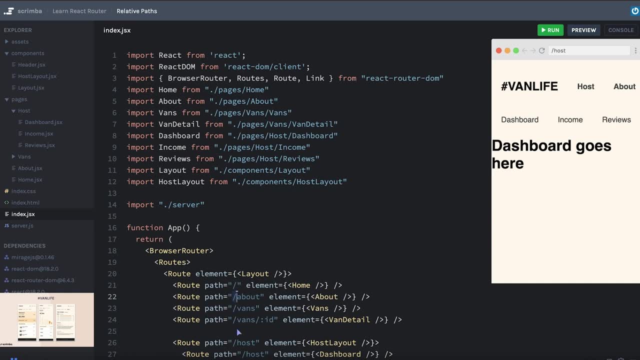 inside of the context of that route. it knows that this route is a child of the slash host route. Up until now, we've included a slash at the beginning of every one of our paths, but the truth is, we don't need to do that all the time. 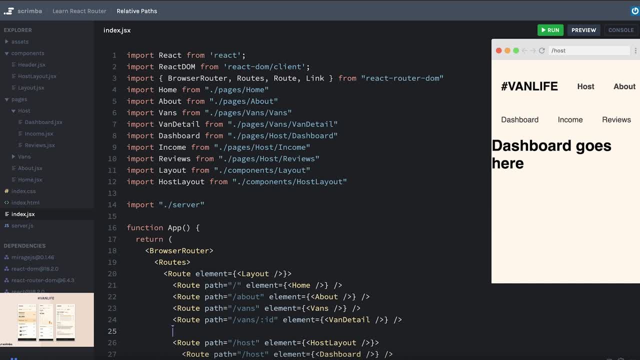 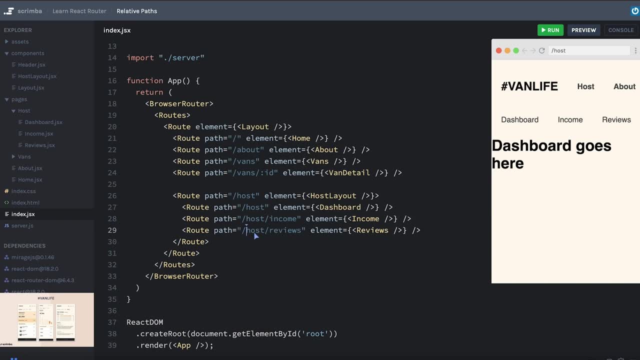 And in fact it's going to end up making our lives a lot easier to not have to have an absolute path like this every time. that gives us the complete view of the path from the very homepage at slash all the way to the end. That might not seem like a huge deal here. 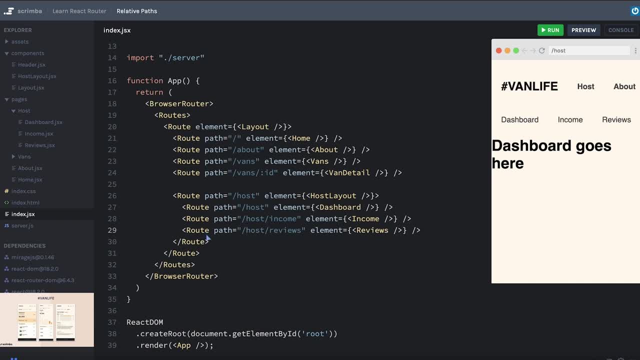 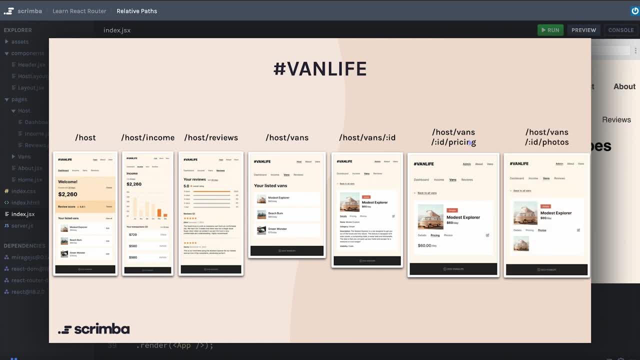 and we look at it, and we look at it, and we look at it. but if we look back at one of the pages we're going to be creating, we have slash host, slash vans, slash the ID of the van, slash pricing and slash photos. 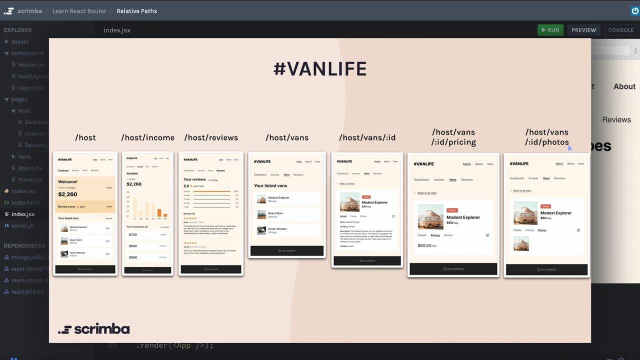 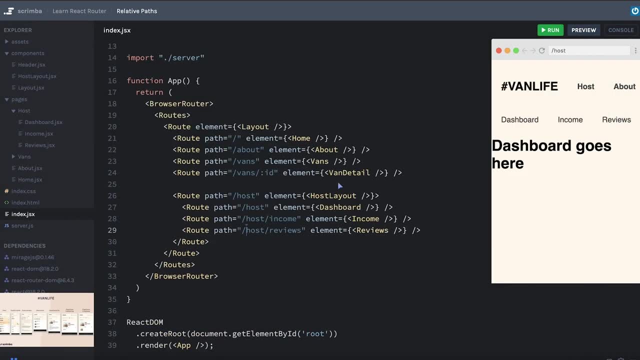 And that is going to start to get tedious. Plus, if this were to grow into a much bigger site, that might even get more and more and more nested and just become a little bit unmaintainable. Fortunately, there is a better way. 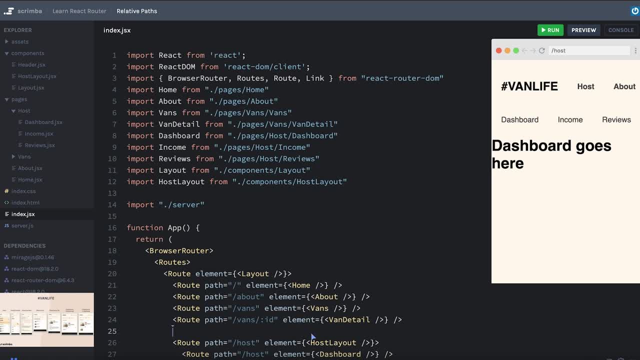 and, like I mentioned before, for anybody who already knows a thing or two about React Router, we can clean up what we have here and make it better, And the way we're gonna make it better is through the use of relative routes. Now, fair warning: by switching things to relative routes. 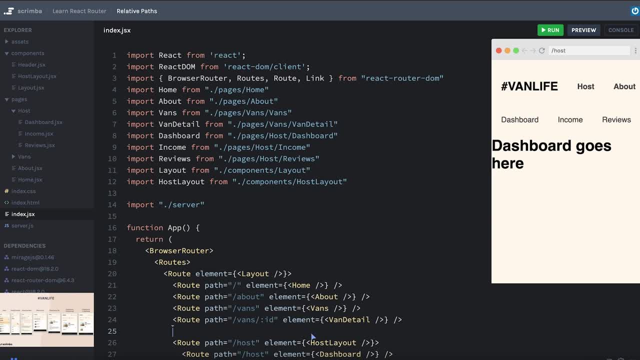 it is going to lead us into the next topic because we're gonna break a thing or two here, But that's okay. that's how progress is made right. The idea behind this is that the slash really should mean, and should be dedicated for the very initial homepage. 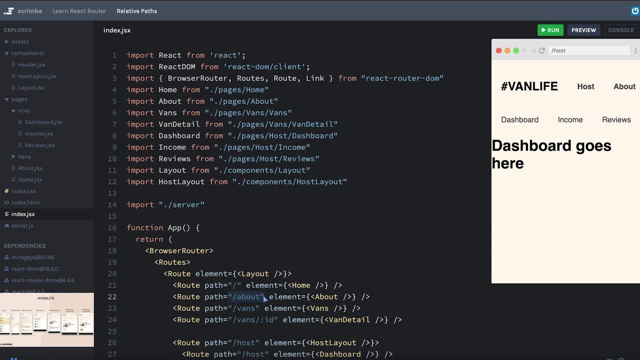 If I start my path with a slash, then React Router is going to treat it like an absolute path And technically, as we've seen, I can use that and I could just use that for the foreseeable future for my entire app and things would work. 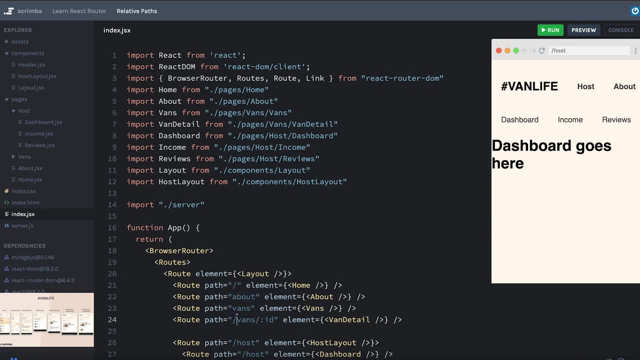 If I do not use a slash at the beginning, then it treats it as a relative route. And what is it relative to? Well, it's relative to its parent route. In this case, the parent route is not really determined. We have this path of slash, which is our homepage. 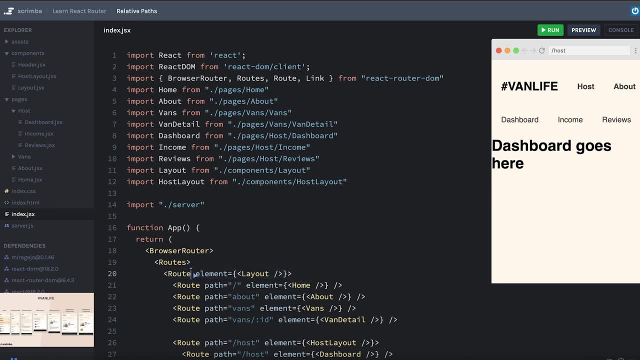 and the parent has no path. It's called a pathless route because, well, there's no path there. So it assumes, because there is no parent, that this is one of the first pages, like the first section of the URL here. 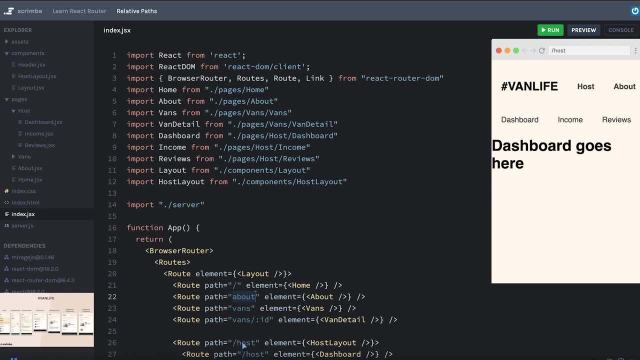 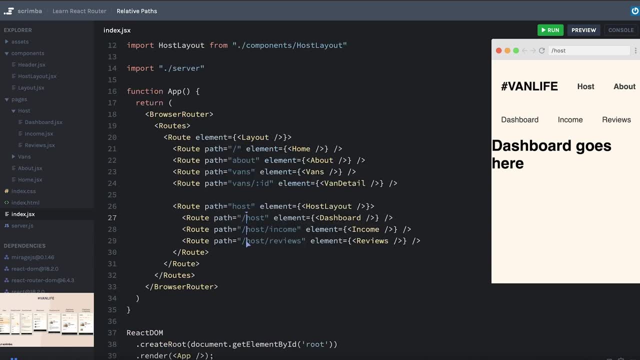 slash about slash vans, slash vans, slash ID. So I can do the same thing with my host here and just remove my slash, and maybe we decide we get a little carried away and we're going to just remove all of these initial slashes. 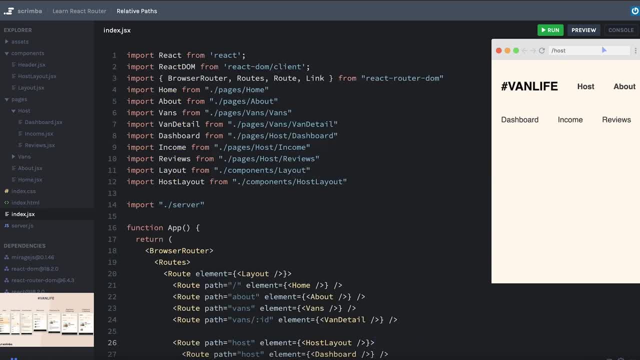 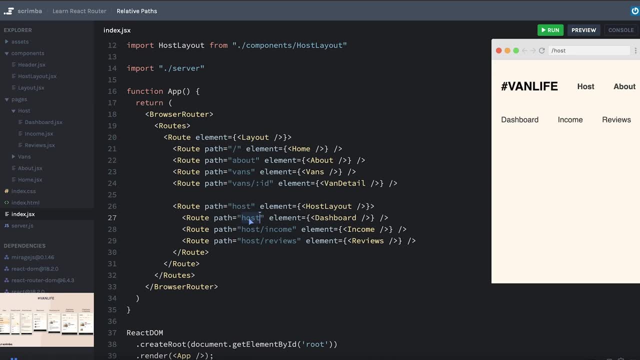 Well, let's hit save and we'll see what happens. Okay, I'm at the slash host route, but suddenly my dashboard is gone. But here it says that the host is the path. Well, what's happening is because I don't have a slash here. 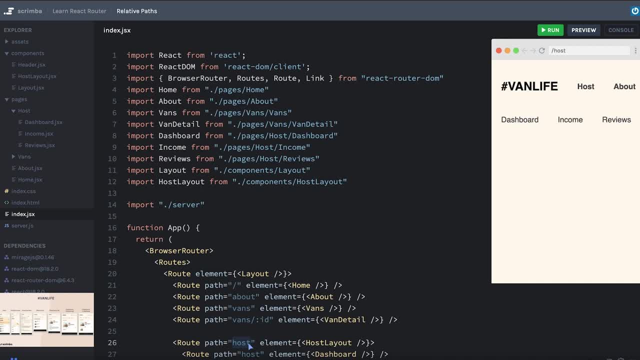 it is now relative to the parent route and the parent route is at slash host. It doesn't say slash, but that's because it's on the top level of our routes. So think for a second If this host is relative to the parent. 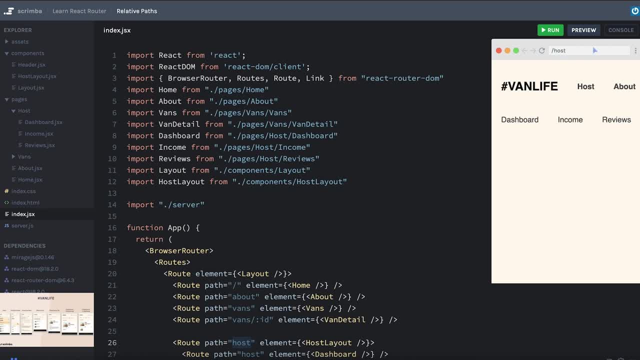 and the parent is host. what could I type into my navigation here, my URL, in order to get to the dashboard view? You can pause now and kind of play around with that or think about it, if you want. Well, what I'd have to type in is slash host, slash host. 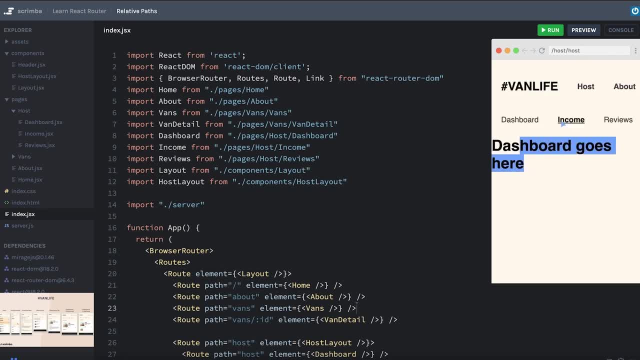 Hit enter and now I'm back to my dashboard. So that's not ideal. I go to income. Well, that route doesn't even exist anymore And you can see, actually none of it is matching because really we're defining slash host. 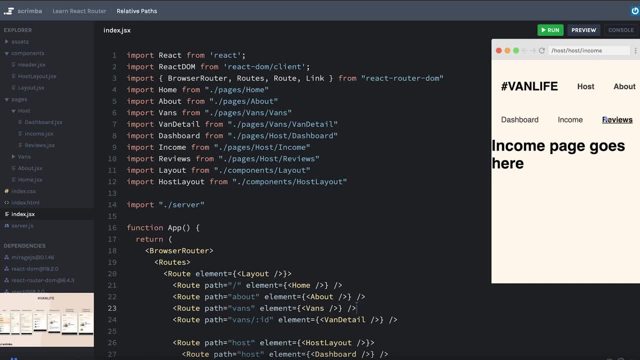 slash host, slash income. And now we're back to where we wanted to be. Of course, we set up these links as absolute paths to slash host, slash income, slash host, slash reviews, and so that's taking us to this unmatched blank page. 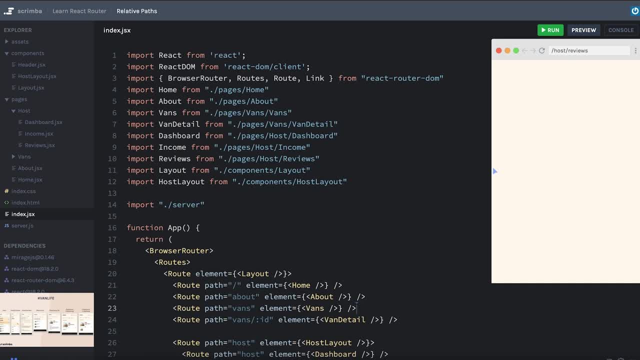 which we should actually put on our backlog, because we probably want some kind of 404, not found page to really soak up any routes that are not being matched in our route definitions over here. But that's for a future lesson, Let's go back. 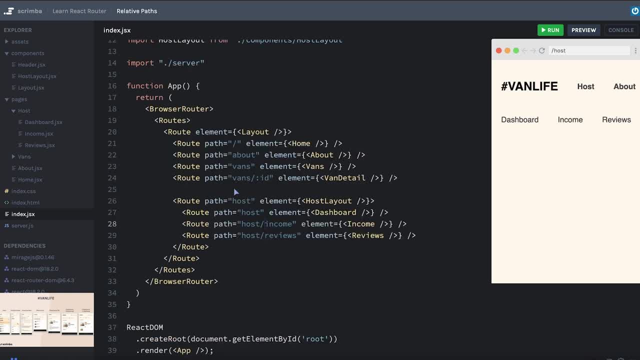 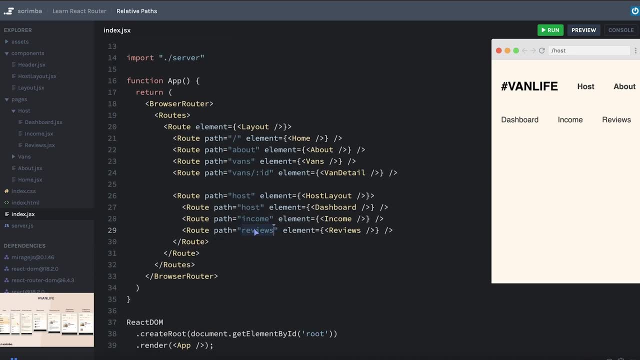 Okay. well, how could I fix this? Well, if these routes are relative to the parent, then I don't need to specify host again. I can just say: this is the path of income, this is the path of reviews, because, in the context of these nested routes, 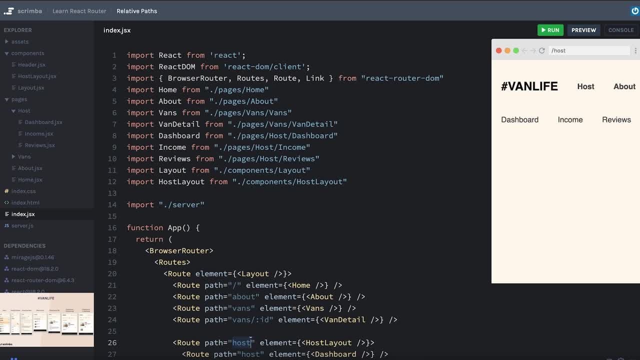 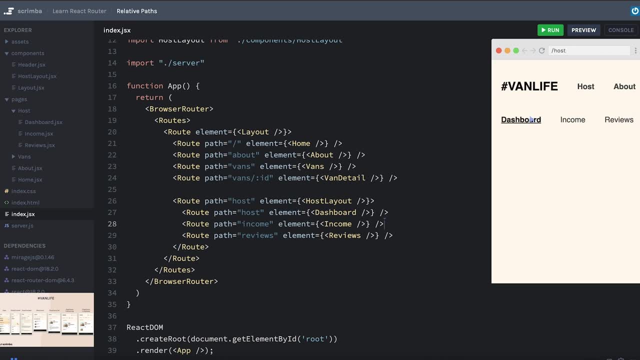 it already knows that the parent is host, slash host, So that should fix income and reviews. Let's hit save, go to income and awesome. Our income page is back, reviews page is back. the dashboard is still broken Now at this point. there's a couple small caveats. 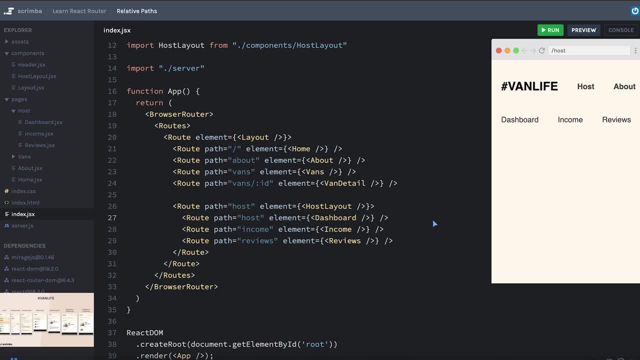 that I wanna talk about, and I think that will probably be best served by doing it in the next lesson. So before just moving on, if you want, you can play around with everything we've done here. You can scrub back to the beginning of the video. 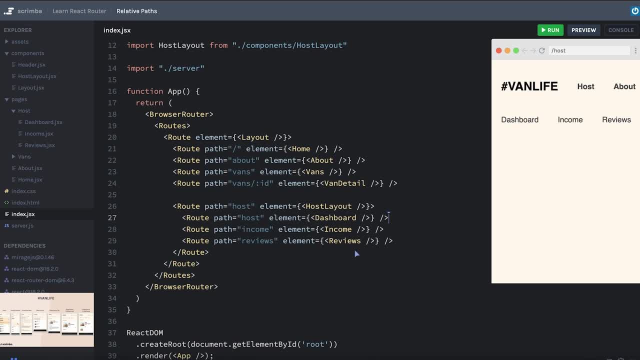 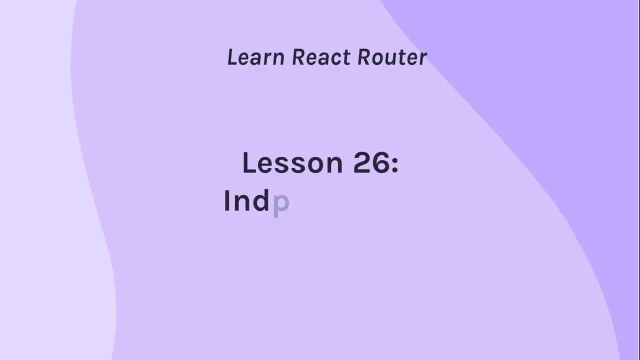 and see if you can recreate this relative path setup that I have here, And when you're ready, let's go to the next lesson. We'll learn how to fix dashboard and a couple other minor things as well. Okay, let's fix this weird conundrum. 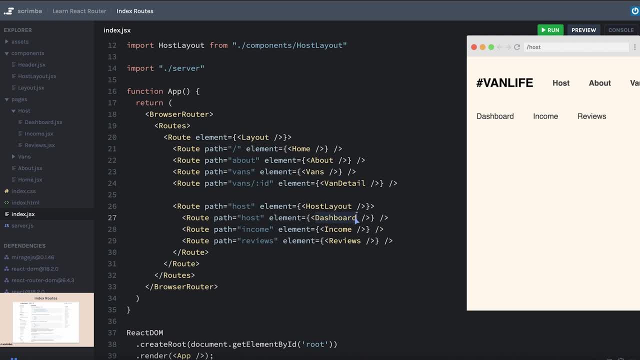 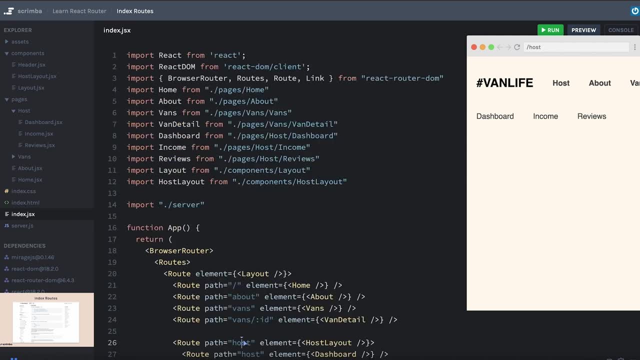 where we have slash host, slash host and that's where our dashboard lives. We've already seen that the income and reviews are working, because we do want them to be at: slash host- slash income and slash host, slash reviews. It's pretty common when you're creating 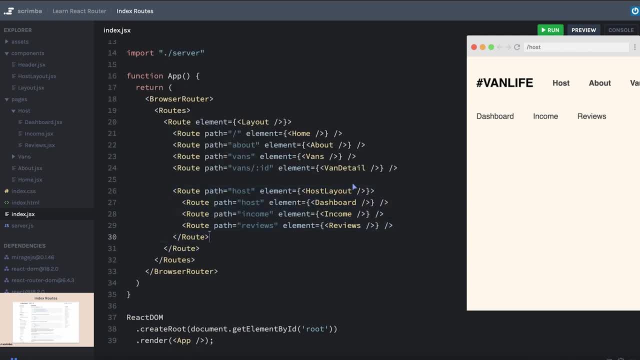 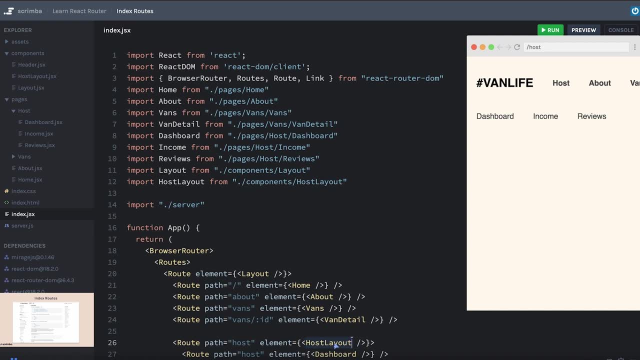 a nested route scenario like we have here, to put some sort of layout element at the parent of that nested route series that you're creating. This layout element is, of course, as we've learned, the one where all of the shared user interface. 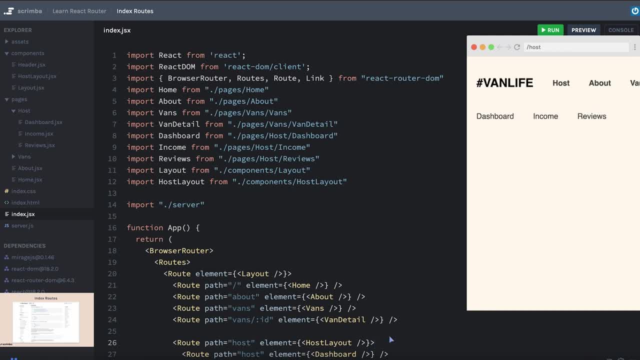 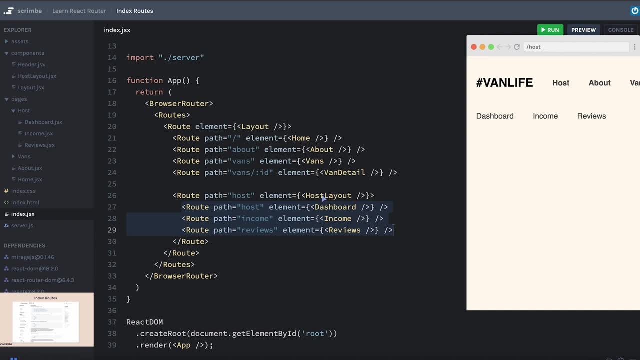 in our case, just this simple little navigation bar where that's going to be exposed, and then everything else that matches more nested inside of will just go into the outlet of the parent layout component, Because this is a pretty common setup in React Router. there's a way for us to say: 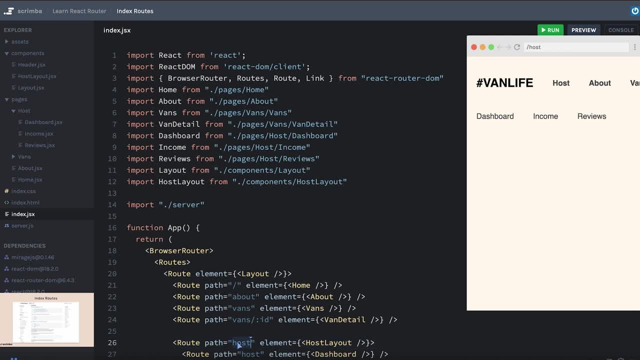 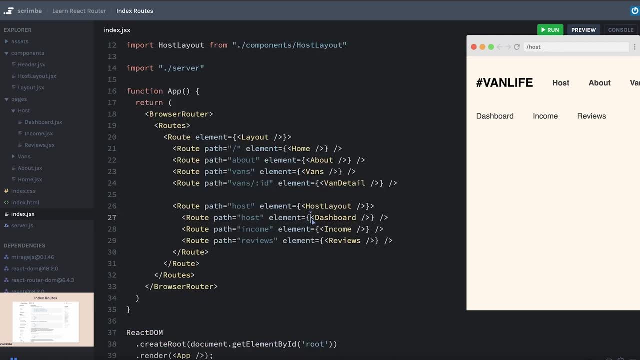 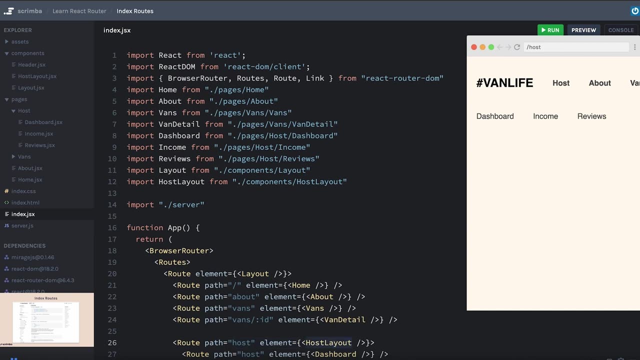 okay, this is the layout element, and this layout should exist on every route that starts with host or slash host. but when you go there, I also have a component that I want to render in the outlet of this host layout component and not at some further nested URL path. 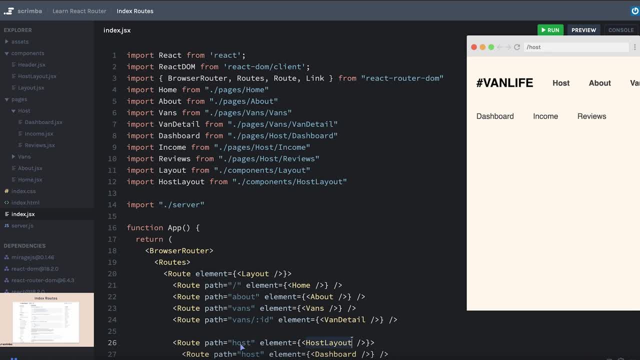 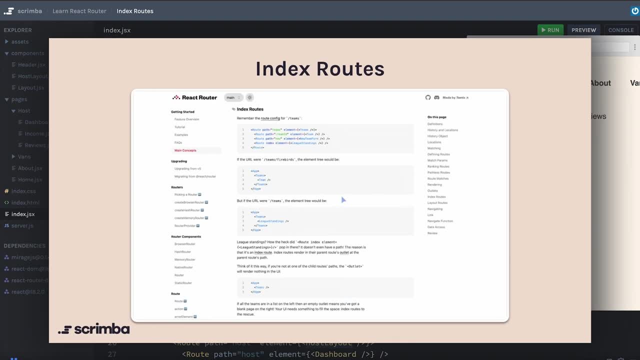 like slash host- slash host, just at slash host, And the way that you do that is with something called an index route. You can click this screenshot, which will take you to the React Router docs, which talks a little bit more in detail about index routes. 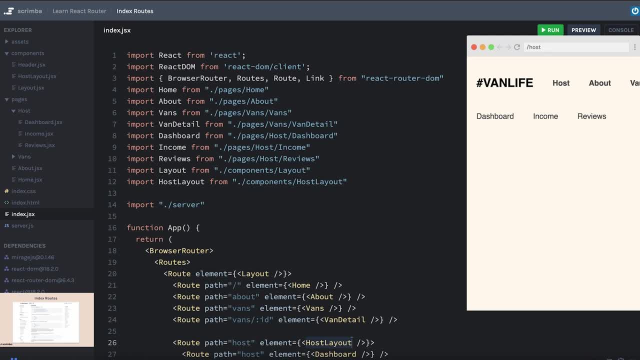 But the main takeaway to remember that was at least most helpful for me is to know that if I have an element that I want to display in the outlet of the layout component, but I want it to be at the same route as what the layout component is defined at, 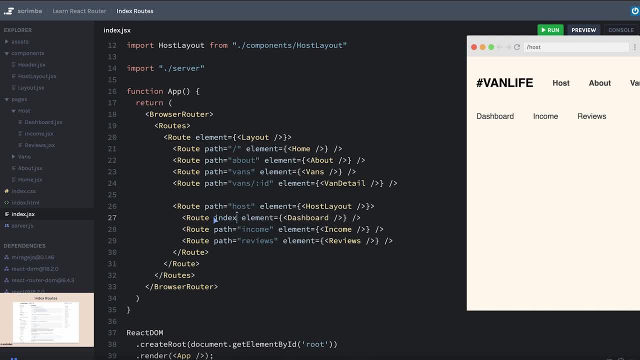 then I can simply replace my path with the prop called index. A way that I tried to understand this for a long time was to imagine it being like: path equals slash, but the problem is, when a path starts with a slash, it's an absolute path. 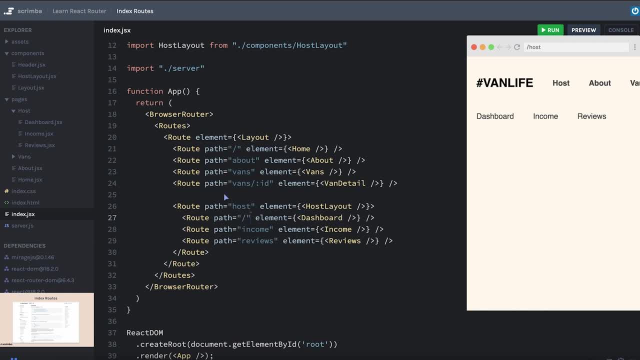 So doing this means that this would only display at the top level slash path up here. It's like it would be the homepage. So the slash isn't going to work for us because that's an indicator to React Router that it's an absolute path. 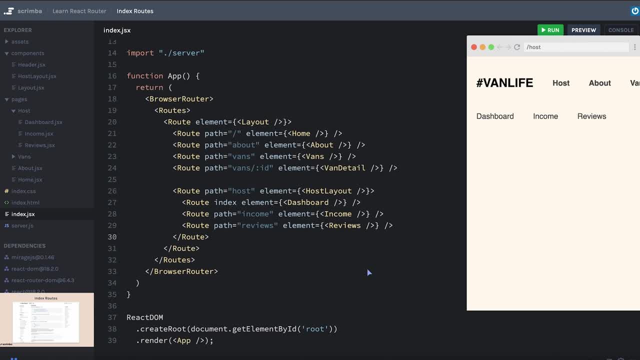 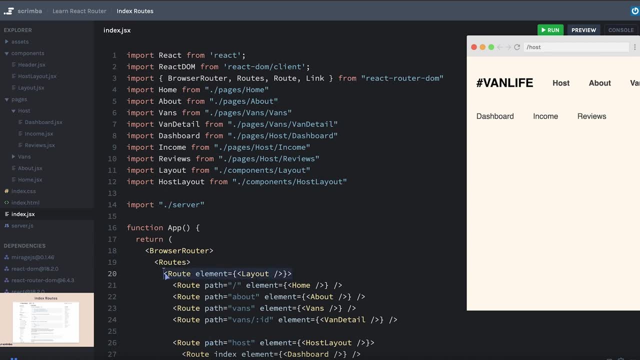 So their workaround for that is to say, index. Now there's a nuanced difference between the layout route that we have here that does include a path and the layout route we have above that does not include a path. In this case, the layout component will apply to. 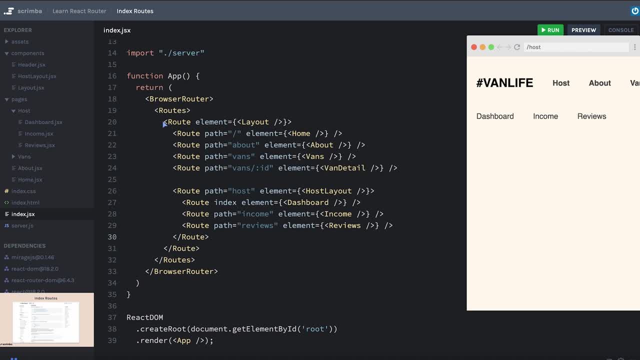 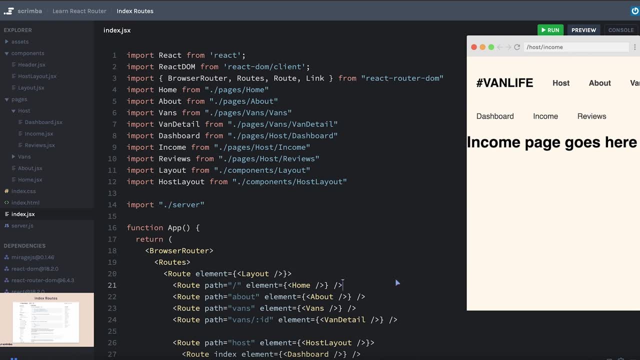 well, everything, because everything is a child of that layout route, And that's why we still see a navigation bar, even though we're inside of our more deeply nested routes here. Now, in fact, I could switch this definition here so that it does include a path. 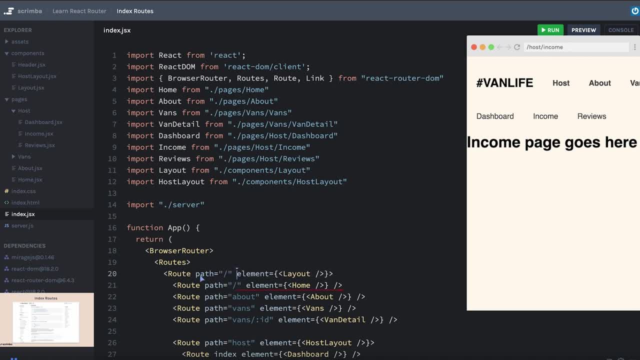 and the path would be: path equals slash. But if I do that, I want you to think to yourself: what tool did we just learn about that I would then have to use in order to maybe update my route so that they looked a little bit more consistent and clean? 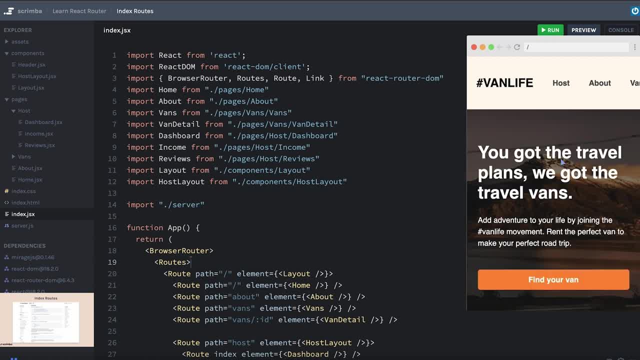 Well, let me hit save, Let's go to our homepage and everything seems to be working just fine. That's very specific because of the way that the slash works and this being an absolute path, But the point is, we could also replace this path- equals slash- with index. 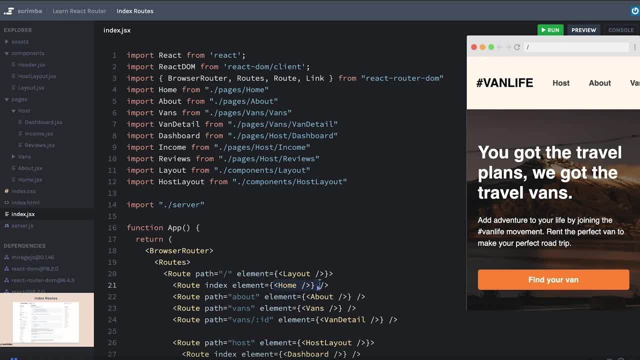 Because once again, index is saying: I want you to put this element, the home component, inside the outlet of my parent route when it matches, So when the path is just slash, then first render the layout and then inside the outlet. 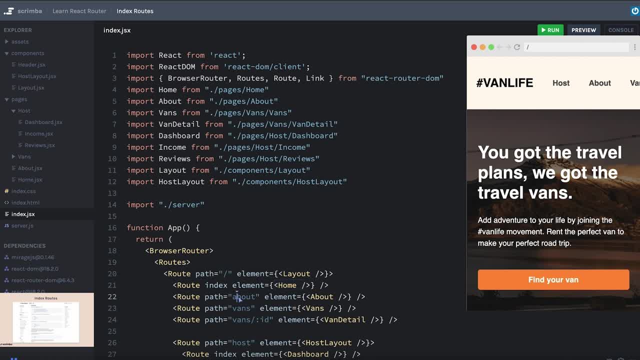 stick in the home element When it changes to slash about. then I don't want you to render the home anymore, because it's not the index anymore, it's slash about, And so you should render this element inside of the outlet of the parent. 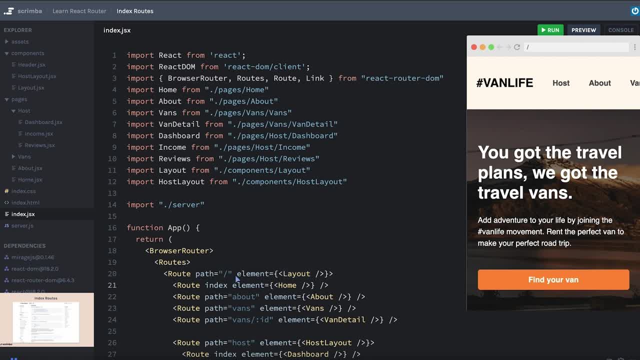 I think, for the sake of more closely matching what the documentation shows, I'm going to leave it this way, But it's helpful to point out that it was working before and it would continue to work the other way as well. Okay, there's one other little caveat. 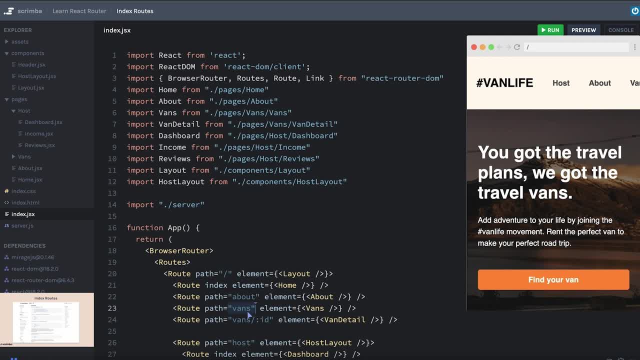 that you might be asking yourself about. and that's right. here We have this vans path and then we're explicitly saying vans slash colon ID. So what gives with that? How come we're not using nested routing there? Well, that's a great question if you were asking that. 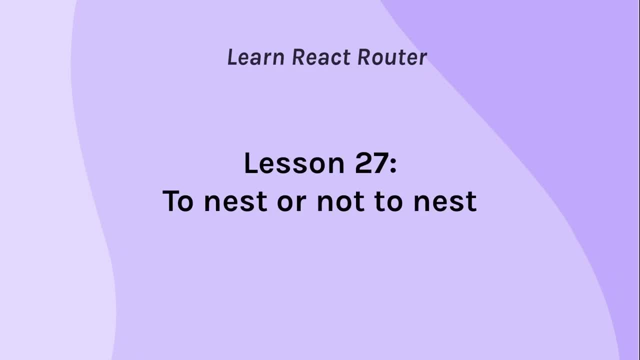 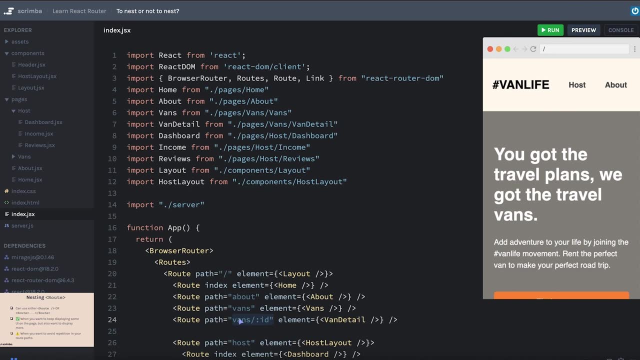 and we're going to talk about it in the next lesson. Okay, so what gives with having this vans slash colon ID here if we were just talking about how we can nest the route so that we don't have to include these nested route definitions in our paths? 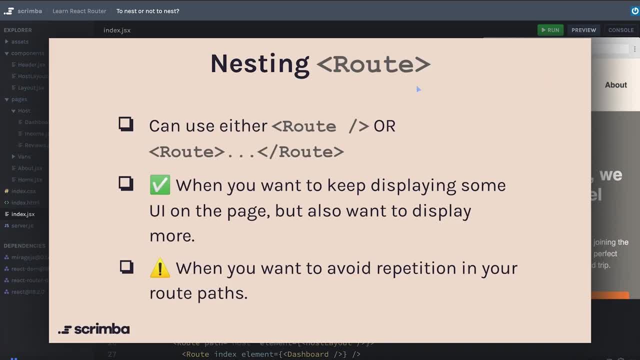 Well, I want to refer you back to when we first started talking about nesting the route component. The primary reason you would want to do that is when you want to keep displaying some user interface on the page. some part of your page will stay the same. 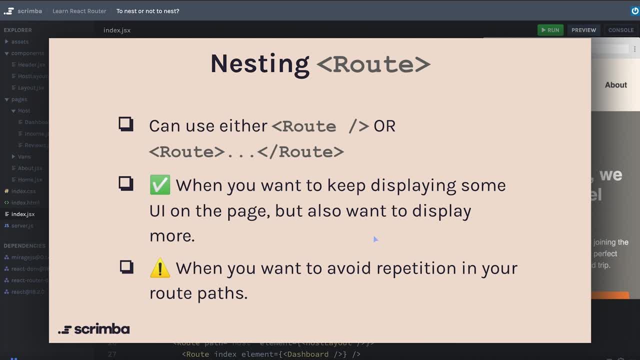 while other parts will display differently, or new things will display on the page when you're changing from one route to the next. And then we talked about how there's kind of this caution sign when the only reason you want to nest routes is because you want to avoid some kind of repetition. 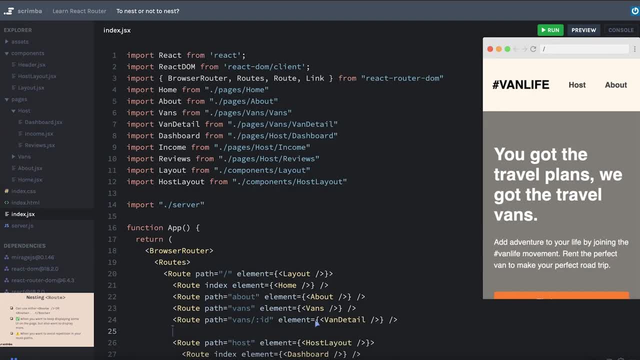 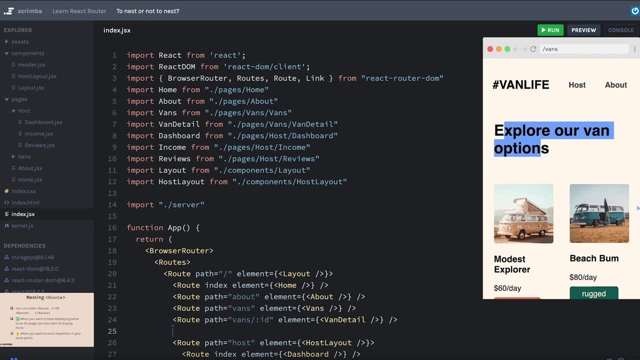 in your route paths. Let's take a look at that. So the vans and vans ID: we have this slash vans page And it starts with vans as in the canal and vansexe and so on, And it starts with explore our vans And then we click on one of these and nothing has remained. 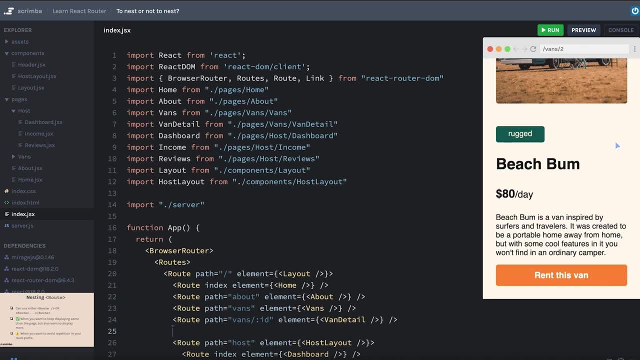 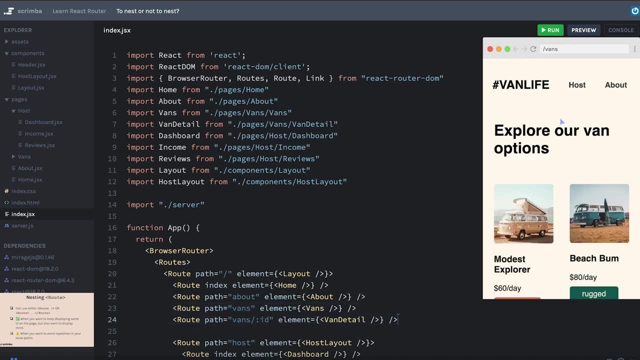 the same. I mean our navigation bar and our eventual footer will remain the same, But that's outside the purview of these paths here, these routes here. So, looking at these two pages, because none of it is sharing the same UI, there isn't necessarily a reason for us to nest a route. 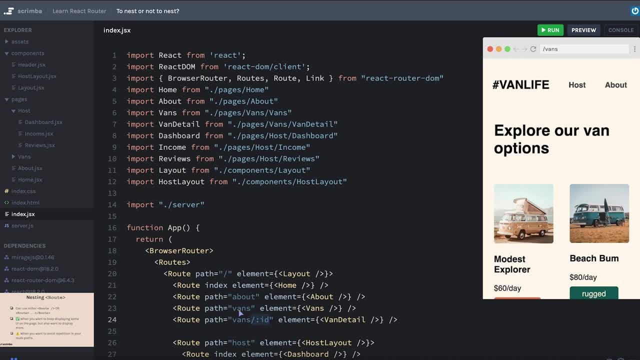 for just the colon ID portion inside of a nested route for vans. In fact, doing so would make us create a route that has a path but no element, because as soon as we put an element in a parent route, we have to include an outlet for that parent route, And because we're not sharing any. 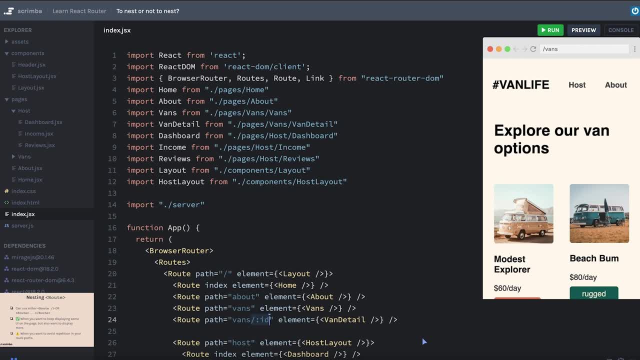 UI. that parent component would be a layout route that only has an outlet in it And we end up with a whole extra component that's not really doing anything, In fact, maybe just for kicks and giggles. it could be fun for you, as part of a challenge, to see what that would look like. So 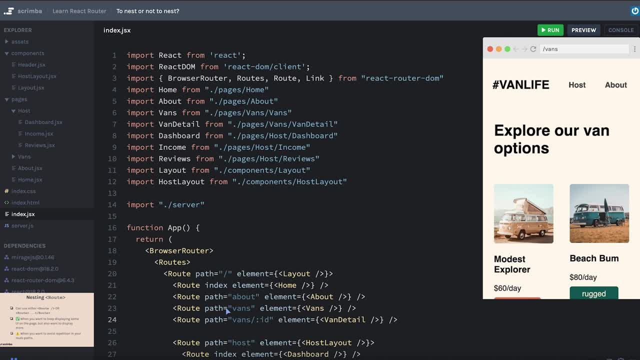 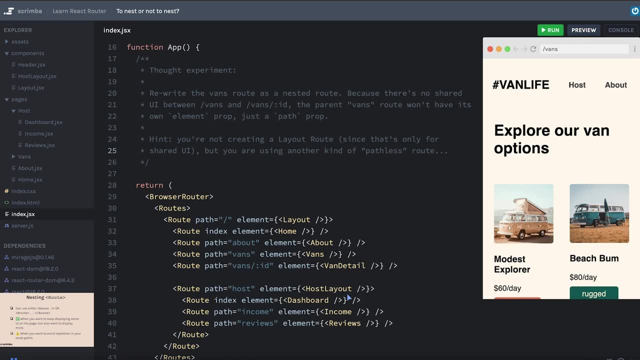 we can nest this van slash colon ID route inside of a vans route. Let me actually type that up as a challenge. Okay, I'm going to call this one a thought experiment, because I personally don't believe that the way we're going to write this is going to be an improvement per se, But it could be a. 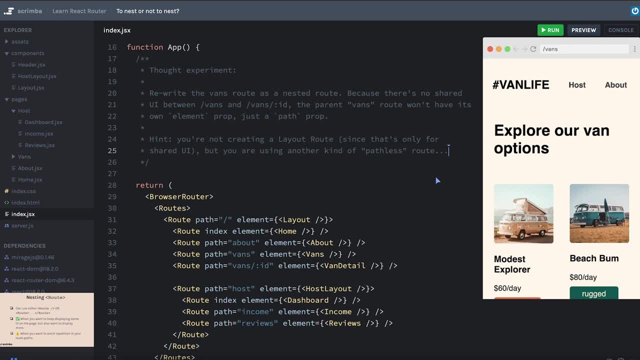 good way to practice what we have recently learned and kind of better understand how these routes and these paths work with each other. So I want you to rewrite the vans route- let me actually put this as a little separation- So you know what you're working with. you're working with these two routes. 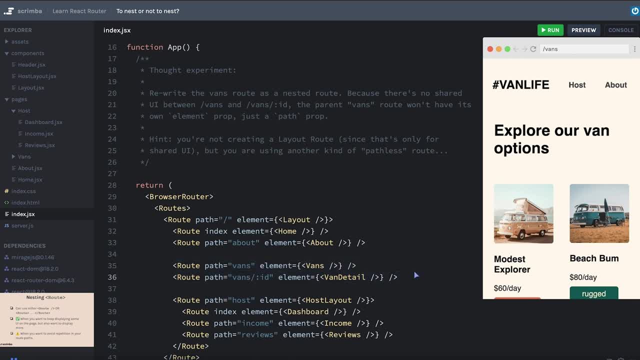 here. I want you to rewrite them so that they are nested In this case, because there's no shared user interface between the slash vans and the slash fan slash ID route. the parent vans route that you create won't have its own element prop. it's only going to have a path prop. 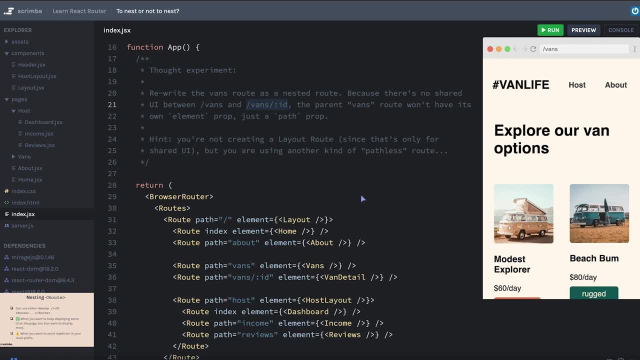 And that does mean that as part of this thought experiment, you're going to have to figure out how to render something at the slash vans route If the parent route here in the definition won't have its own element. you can read the hint here, which should help a little bit. So pause now and 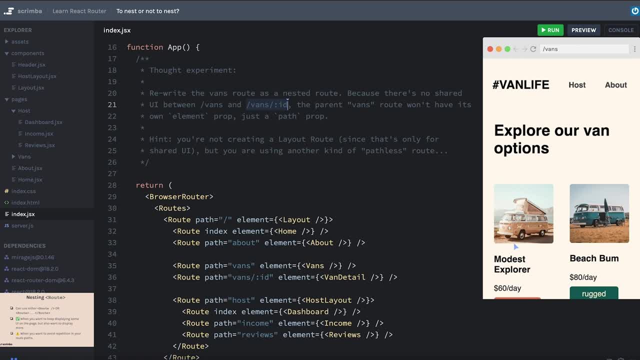 work on. Well, hey, it's not a challenge. Let's maybe say: work through this thought experiment. Okay, let's go ahead and create a parent route that's actually wrapping these other routes Go like that And in this case, we need to move our path of vans up to the parent route. 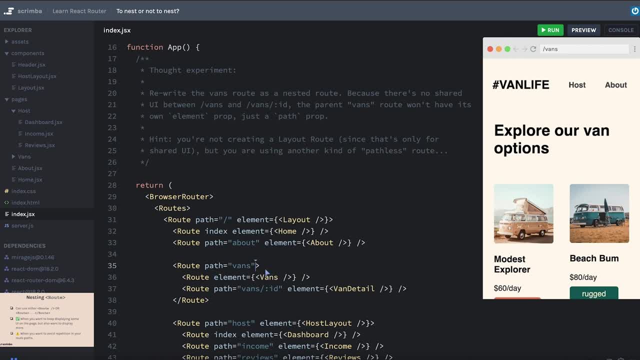 But because there's no shared user interface, I'm not going to put an element here. Again, putting an element at the parent route would mean that I would need some kind of outlet inside the parent route. So I'm going to put an element here and then I'm going to put an. 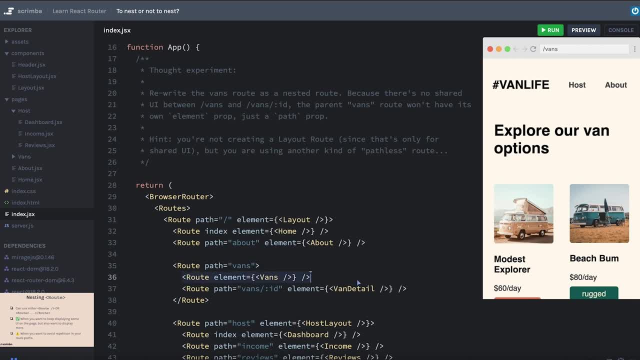 element inside that element so that it had a place to display the children routes. But because we have no shared user interface, I would just be creating a layout route that had nothing but an outlet in it, which is totally extraneous. that's not necessary at all. So for this first, 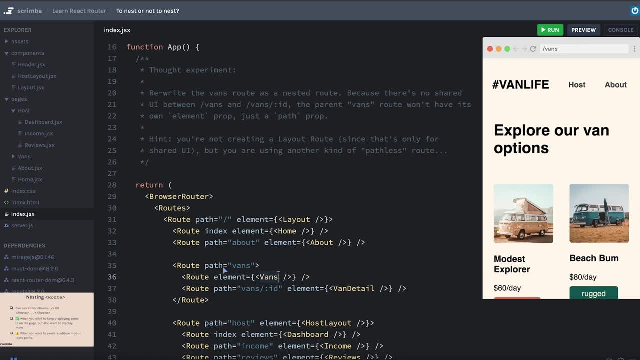 child the vans page. I do want that to render when it's at the slash vans route. Well, we just learned about the index prop where I tell this route to render this element at the parents path. technically speaking, it usually wants some kind of outlet in the parent route. So I'm going to. 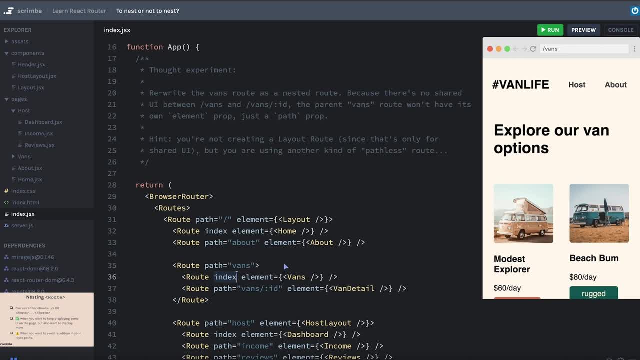 put an element at the parent route and then I'm going to put an element at the parent route, So outlet in the parent element, but in this case, because we have no parent element, it's just going to render the vans page, with no shared user interface between all of these children routes. 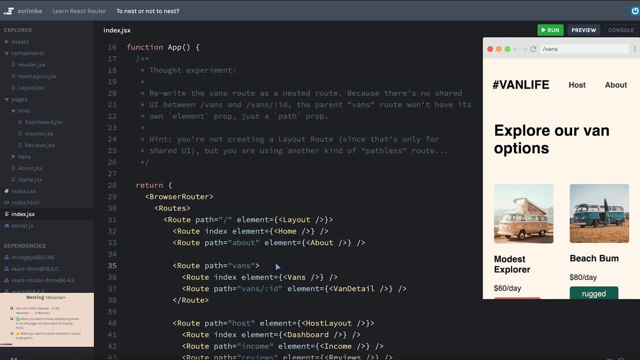 And that's exactly what we want. So that should work out. Okay, then, the only other thing I need to change- because we're already nested inside of this path equals vans- is: I don't need to repeat the vans and the slash here, I can just say that the path is colon ID. So let's hit save And things. 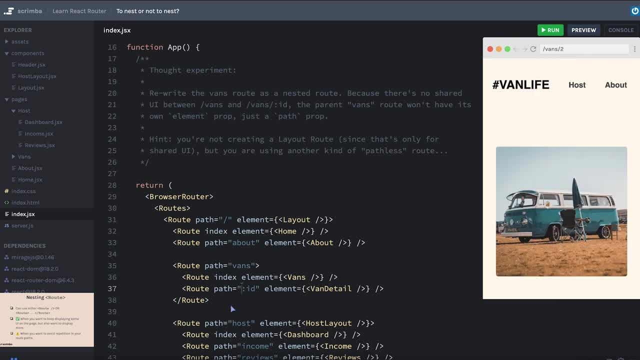 seem to be working the way that they were, which is good. That's what we'd expect. Again, we're now using four lines instead of two lines, which, of course, isn't that big of a deal, But it is doing some weird things, like we have a route which has no element And now we have to specify another. 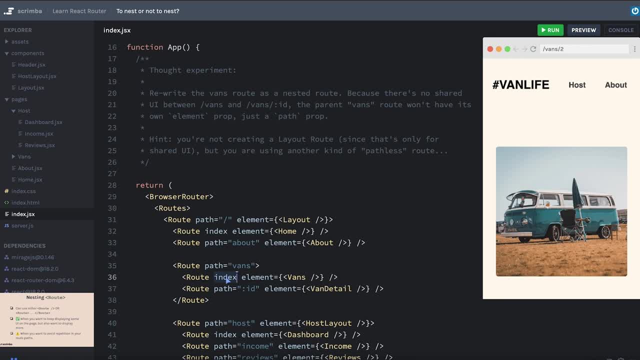 child route using the index route. So, again as a thought experiment, I wouldn't necessarily recommend doing this. maybe there's a scenario where it makes sense, But when there's no shared user interface between these routes, there's really no reason to do a nested route setup like. 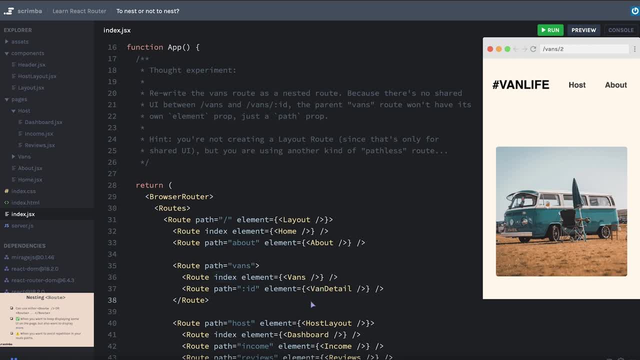 this. So while that was fun to play around and get some practice under our belts, let's go ahead and undo everything we just did. Honestly, that's a really great part about practicing, especially in an environment like we have here on scrimba. You can mess with the code and maybe even get. 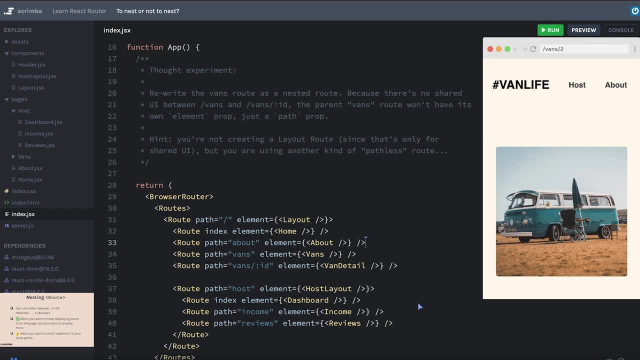 something completely, completely wrong And it's not going to break anything. If you're anything like me, I suffer from some severe perfectionism sometimes And it can be really liberating to realize that it's okay. when I'm just practicing, I can mess everything up and then just go back. 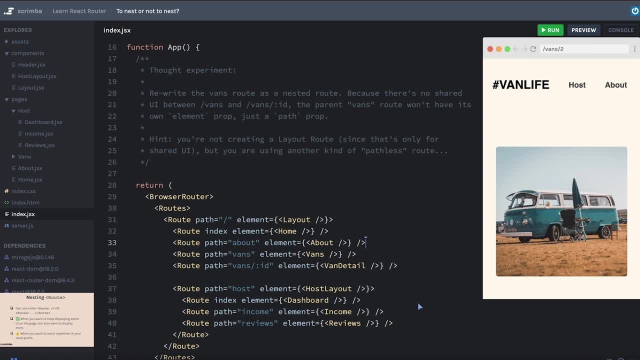 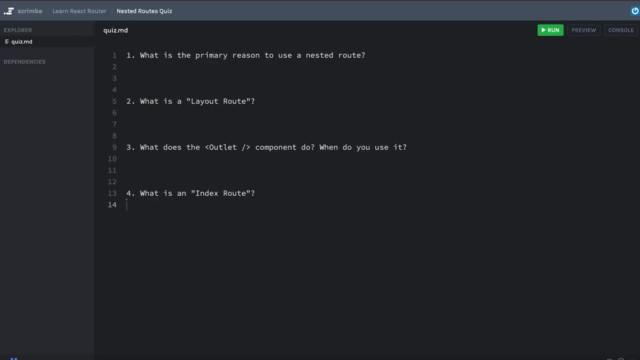 to where I was before. I think that's pretty cool, But now it's time for us to move forward. We've talked quite a bit about nested routes, So let's pause for a minute on the curriculum And let's go over a quick quiz dealing with nested routes, Just like before. I do actually want you. 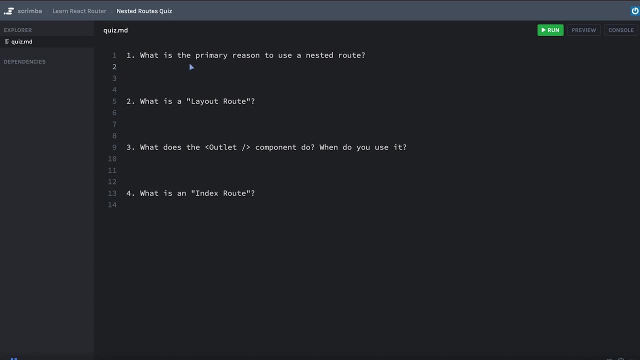 to click into the editor here and type down your actual answers to this quiz. And again, of course, I'm not going to give you any kind of grade or anything like that. The purpose is to help you reflect on what we just talked about and hopefully wake you up a little bit, just in case you've been 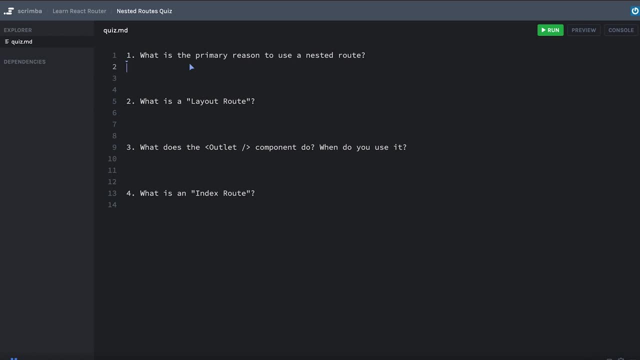 in a bit of a dream state. I know sometimes when I'm watching a course, I will tune out a little bit and I'm hoping this will help you a little bit. So let's go ahead and get started. So let's go ahead and. 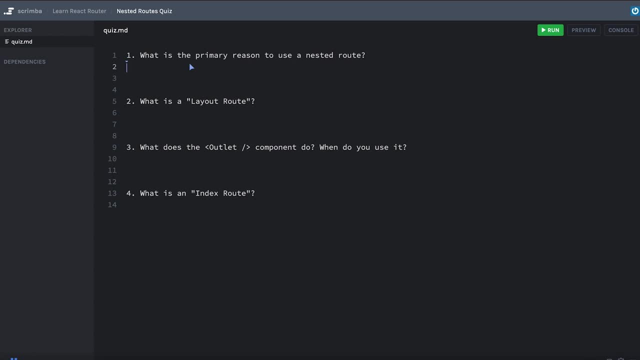 get started. This will help combat that. So pause now, answer the questions in this quiz, and then we'll go through it together. Okay, what is the primary reason that we would ever want to use a nested route? we saw two possible reasons, but one of them is much preferable, or rather: 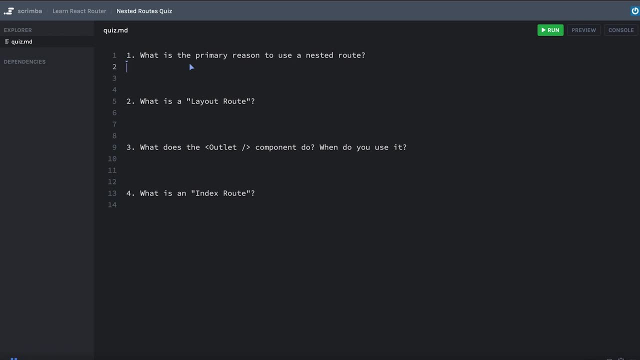 one of them is much more important than the other one, And that is whenever we want to use some kind of shared user interface amongst multiple different routes. So I'll type that down for reference If you have a larger app and there are a lot of nested routes that are all sharing the same name. 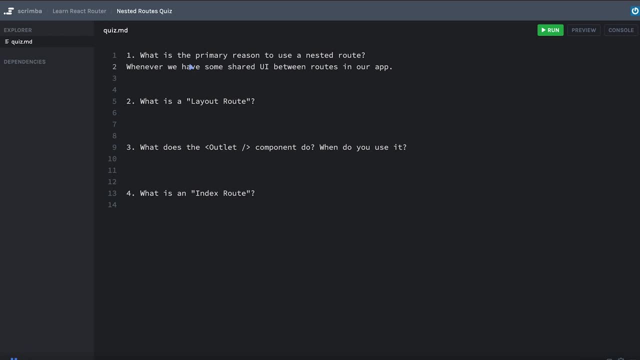 in its path. I suppose there could be an argument made that using a nested route could help avoid some of that. More often than not, we'll focus on this primary reason, which is when we want to share user interface between the routes. So what is a layout route? Well, a layout route is the 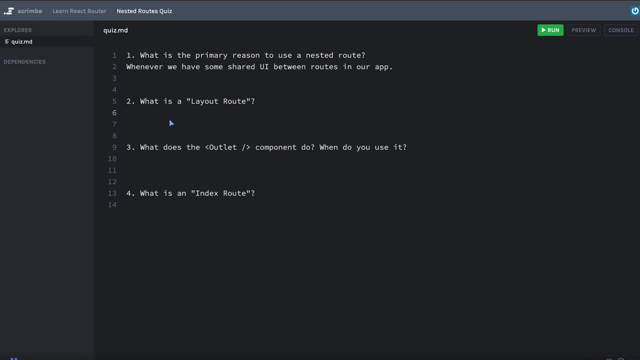 actual route that hosts or contains the shared user interface portion of the nested routes. So its job isn't to display the primary content from the nested routes or the routes from which you're trying to display content. Its primary job is to display just the shared portion that you don't want changing when. 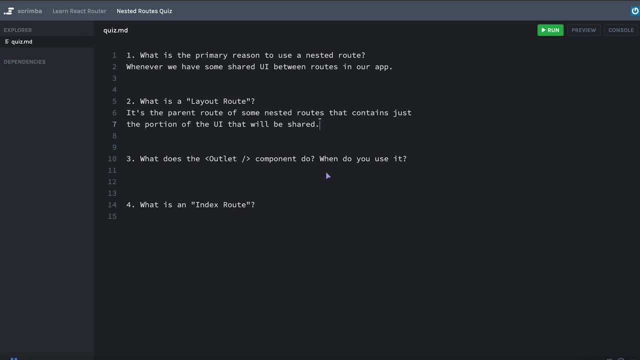 you go from one nested route to another nested route? As a segue into the next question, another important aspect of a layout route is that it will use an outlet component. I'm not going to go too much more into detail about that in this question, because that is what the next question is. So what? 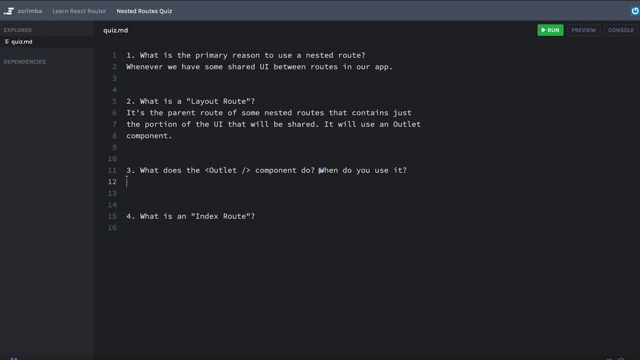 does the outlet component do and when do you use it? Well, to answer the when do you use it part, first, you use it inside of some kind of layout route where that route is the parent to some nested routes. So maybe even more specifically, rather than referring to the term layout route, 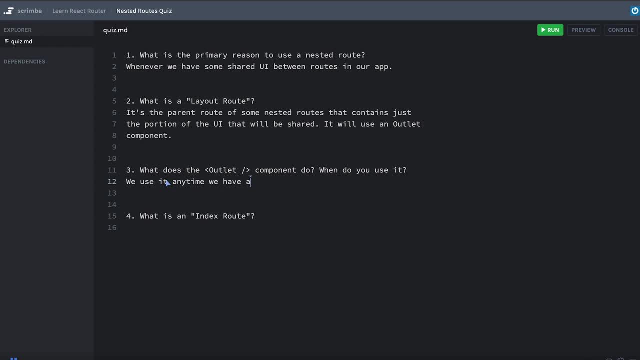 we would say that we use it anytime we have a parent route. that's, I guess, by definition, wrapping children routes. And what does the outlet component do? Well, it's an outlet or a placeholder that represents the place in your parent route where the matching child 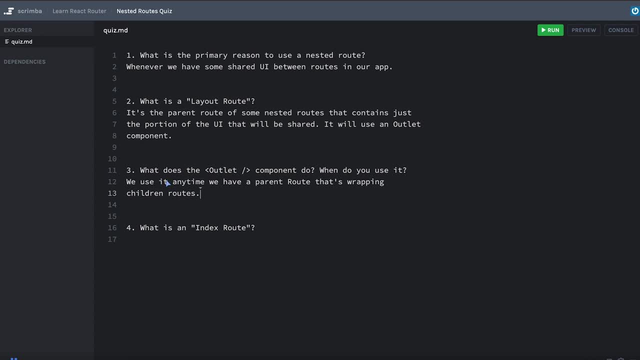 route will render its contents. So the parent route will oftentimes have the shared user interface, like we talked about with a layout route And so that parent route elements will contain the contents that you want shared across every child route And then the outlet is sort of. 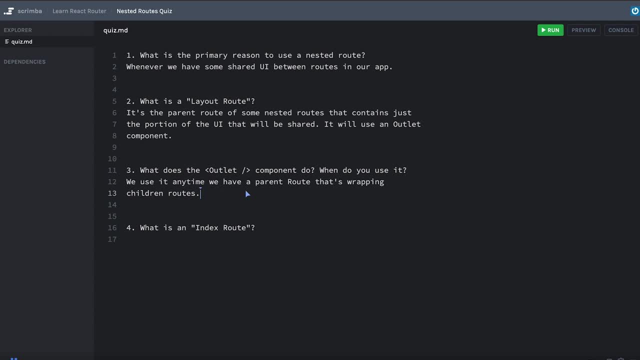 like the concept of children. if you have used compound components and react before, where it's a placeholder, where the children route, elements will render. I think I just said the same thing two times, So hopefully it's starting to sink in. Let me write up a summary. 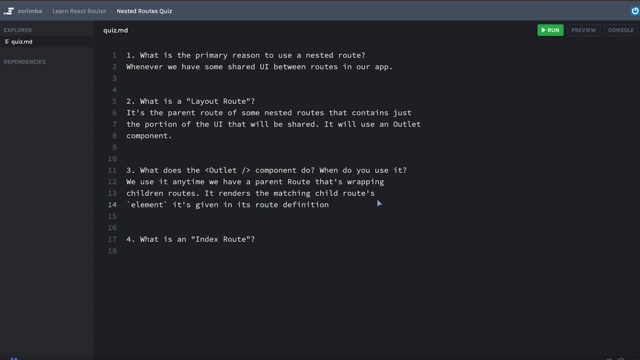 This is worded a little bit differently, but it renders the matching child routes element prop, and we'll say prop- given in its route definition. Okay, so then, what is an index route? Well, an index route is a child route that will match the path of the parent route if the parent route 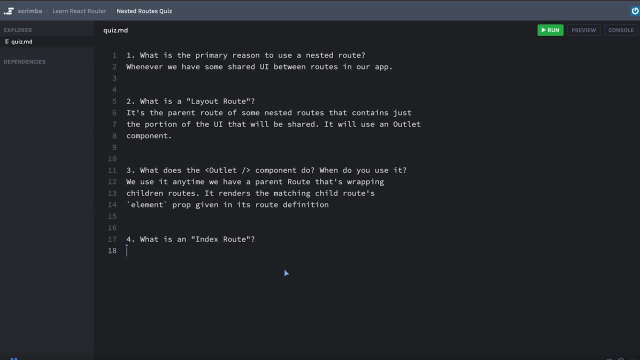 has a path defined. That definition might be something you have to really think about a lot, but I promise the more you use it, the more it'll make sense. So let's go ahead and get started. So let's go ahead and get started. So let's go ahead and get started. But remember we might have 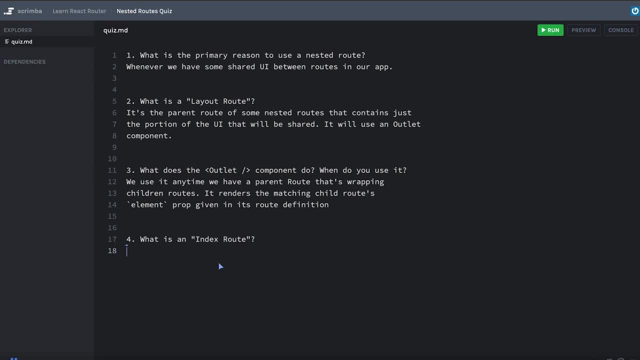 a layout route as a parent which is containing any shared user interface you want amongst all the children routes. But you might also want another element beyond just the layout component to be rendered when the path of the parent route is matching or is rendered. So a good way to think. 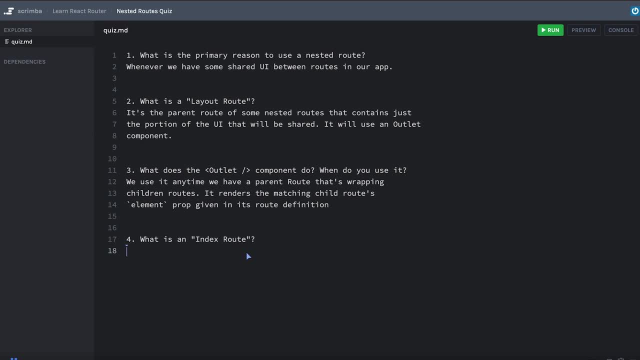 of an index route is like the default element that should render in the parents outlet when the path matches the parent and nothing else. I think that's a good one that we could write down. I don't have the slides for the vanlife app right now, but a good example of this is how, on our host page, 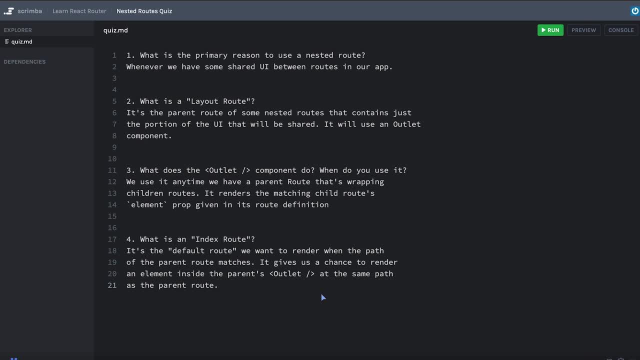 we have the route slash host and we want it to display both the little navigation bar for just the hosts that navigates us between the dashboard, reviews, vans and income, But we also want to display all of the information from the dashboard. We could have made the dashboard display at: 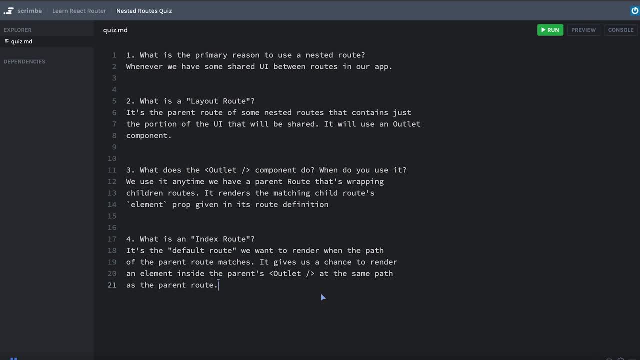 slash host, slash dashboard. But just to keep things simple, we wanted slash host to display both the shared user interface of that little secondary navigation bar, So we could have made the dashboard display at slash host- slash dashboard, But also all of the information from the dashboard. Okay, that wraps up this quiz. Feel free to go back and review some of 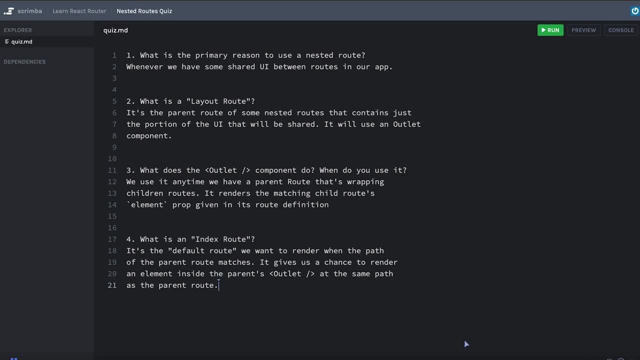 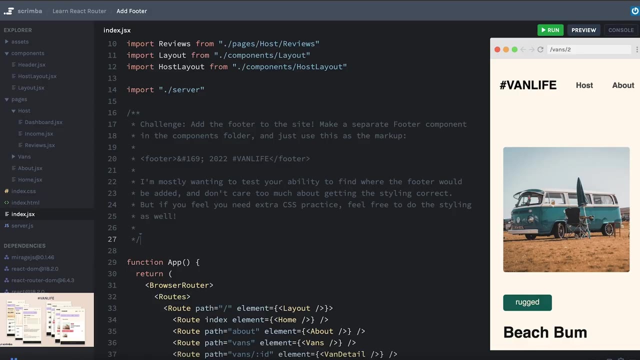 these answers. if you'd like, You can, of course, go back and re-answer them from scratch. Might be a good way to really help it sink in. And, as always, when you're ready, we'll keep moving forward with our vanlife app. This challenge is a bit off the beaten path for what we've just been working on. 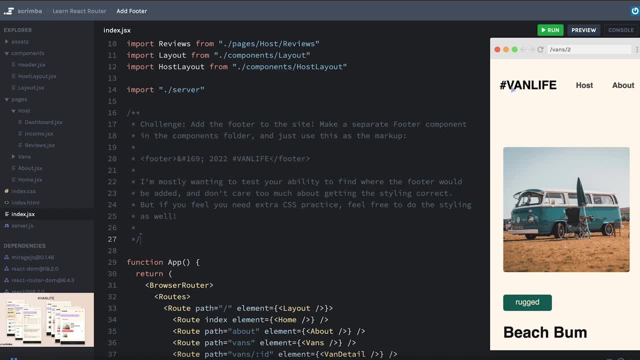 but I wanted to put a little bit of space between when we added the head header from before and now what your challenge is: to add the footer. That's just a way to test yourself and your abilities from what we learned prior. So your challenge is to add the footer to. 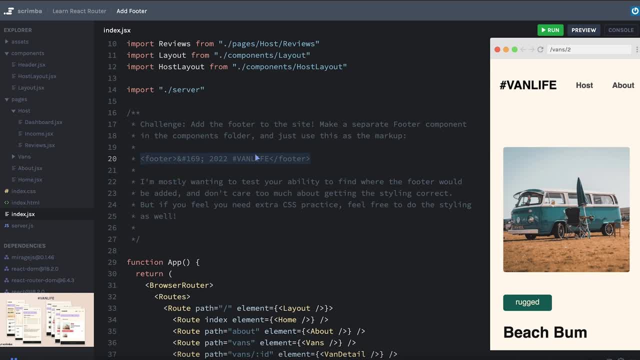 the site. I've even given you the markup here So you can use that in a new footer component that you create in the components folder. And mostly I'm wanting to test your ability to see if you know where the footer would be added. So I don't care too much about you getting the styling, just 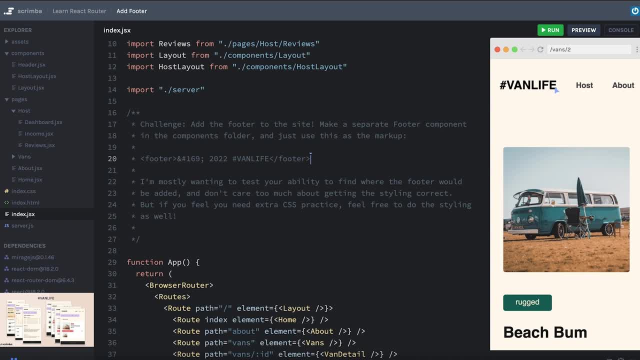 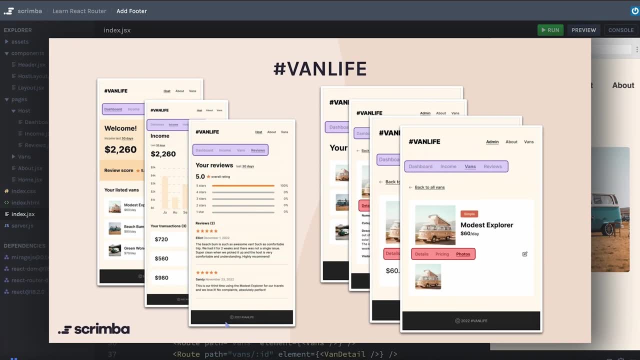 right. However, you'll be the best judge for your abilities in CSS. If it's been a little while, you're feeling rusty or you're not sure if you're going to be able to do it, So I'm going to give you a little extra practice. you're more than welcome to add the styled footer. you can. 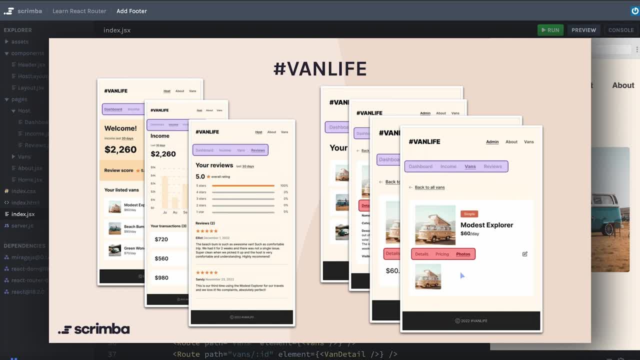 click on any of these multiple screenshots to take you to the Figma design file for that, if you wanted to get the details on it. But otherwise I will just be handling the styling behind the scenes And mostly what I'm looking for is that on your app, any page you go to will have the 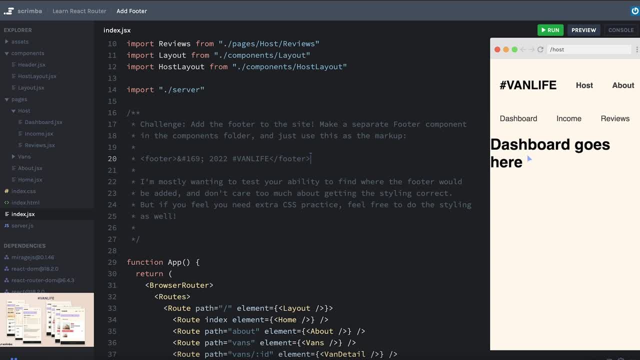 footer just tacked to the bottom of the page. So if you're not going to be doing the styling, it will just appear, maybe on this really short page like this right here below dashboard goes here On a longer page. it's going to be on the bottom of the page, So if you're not going to be 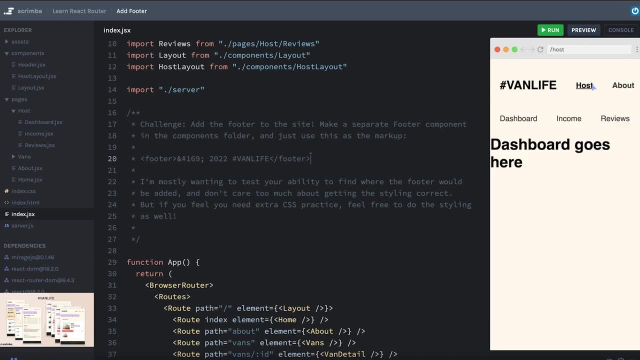 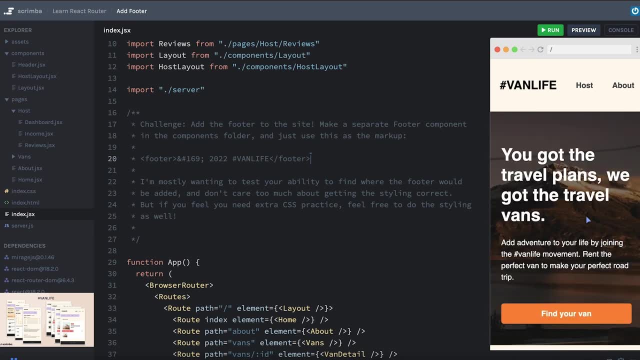 on the bottom of the page. it would show up at the bottom. you'd have to scroll down to see it. If you are working on the styling, then the idea is that the footer will always be at the bottom of the content, Even if you have to scroll to see the bottom. then you would have an extra section. 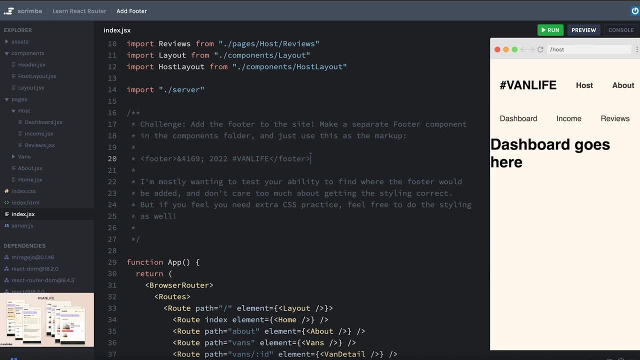 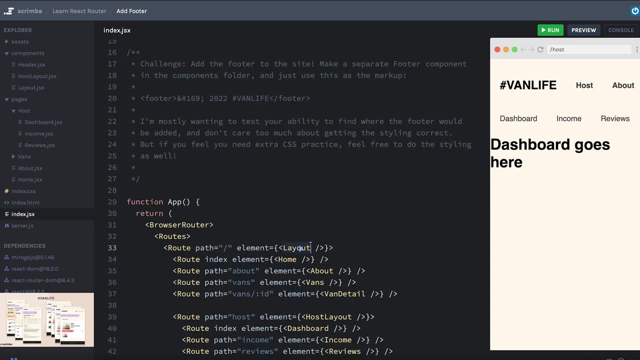 where the footer sits. If it's a small section like this, then the footer would still be at the bottom of the page. Okay, I think that should all make sense. Pause now and add the footer to our site. Okay, you might remember that the layout component is going to be on the bottom of the 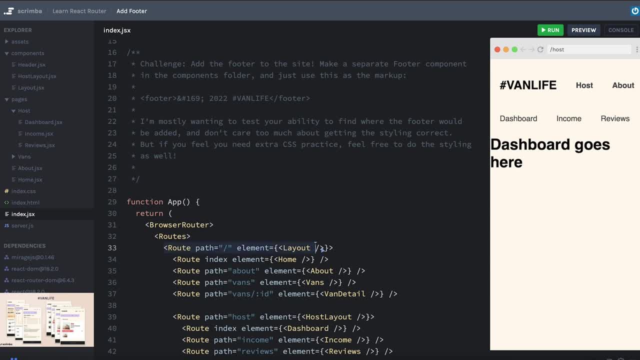 page and the layout component is where we are including our header. And because this route, that's using the layout component, is wrapping every single route in our route definitions here inside of our router, that means that the header is going to show up on every single page And 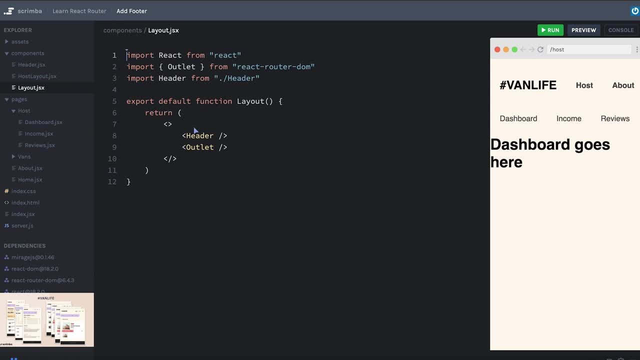 since that's what we want to do with the footer. that's what we're going to do. we're going to put the footer inside of our layout route here, or rather our layout component, So below our outlet. remember, the outlet represents whatever content will go below the header. we're going to say we 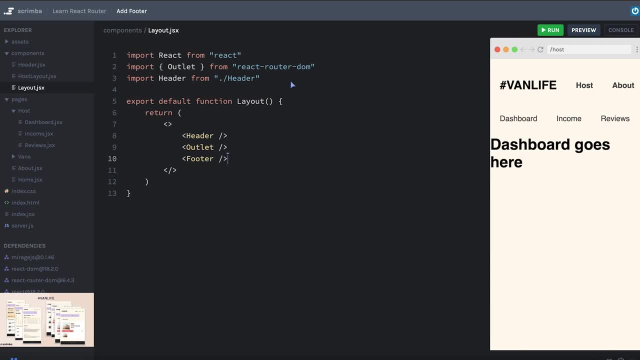 also want a footer in here And that's going to be at the bottom of the outlet to import our footer even though we don't have it yet created footer Let's save. Okay, unknown error, That's because footers undefined, So let's go ahead and create footer dot JSX And we'll set this up like normal. 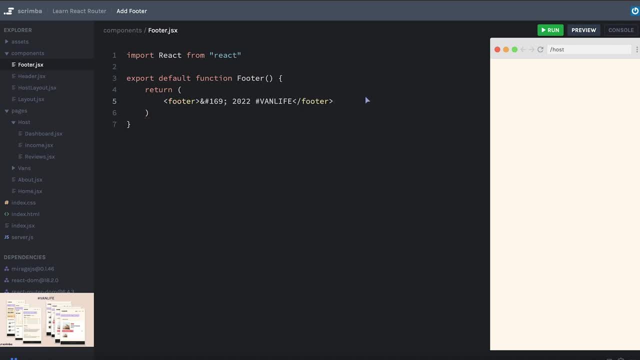 And, fortunately for you, I was so kind as to just give you the markup that you need to include. Let's hit save And great, there's our footer, And now we're going to go ahead and create a footer. So let's go ahead and create our footer. as basic as it is, And it should be showing up at the bottom. 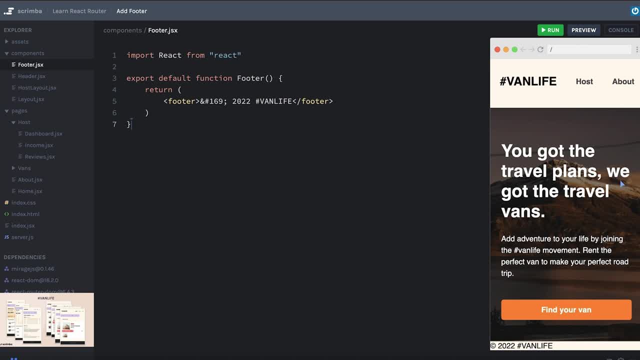 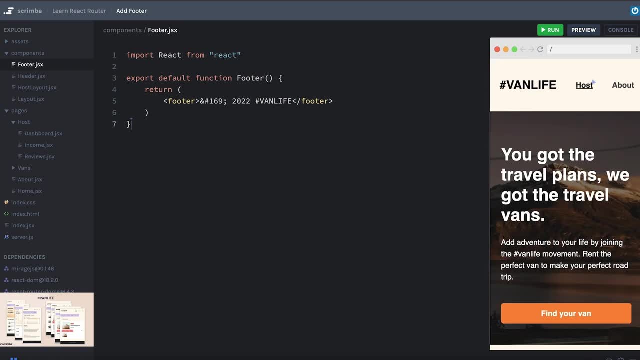 of every page. There we go. Like I said, I'm going to handle the styling for you, So I'll use the magic snap of my fingers And there we are. So we can see that if we go to a shorter page, here we 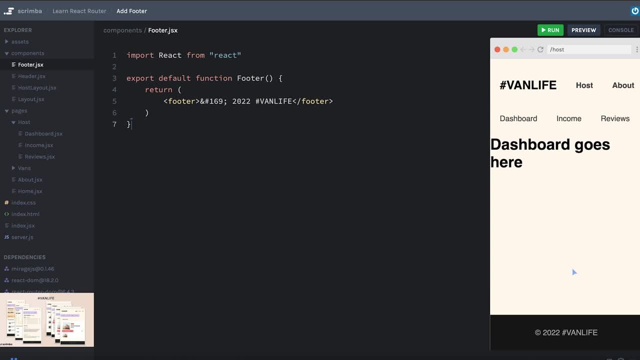 have our van life footer down at the bottom. the main point isn't about the CSS. the main point is about this layout file. you can see I've made a few changes here to make it so that everything laid out correctly. Great work. Hopefully that wasn't too much of a challenge. 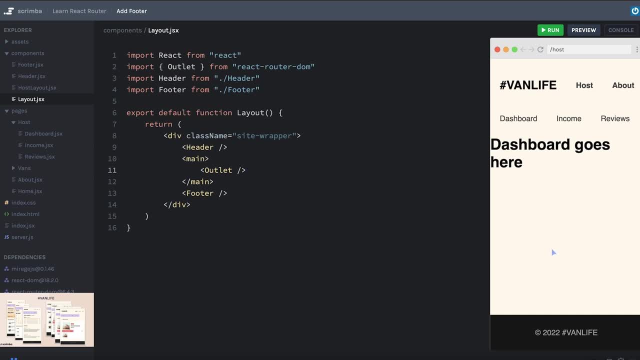 I think the CSS was a lot harder than actually getting the footer to show up on every page, And hopefully that was the same case for you. Okay, it's time for us to jump back into some new material, So let's do that next. Let's bring things back to a much simpler time than the 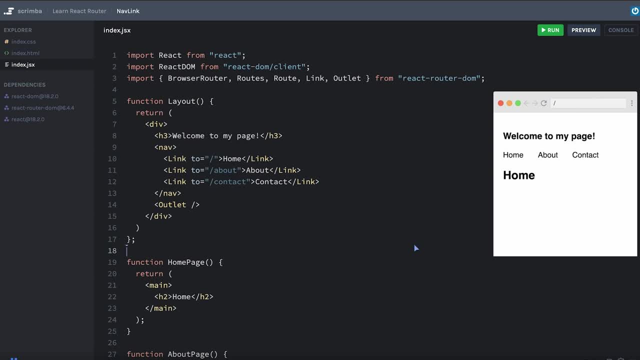 more complicated app that we've been working on. This is actually the current default react and react router scrim that scrim but produces when you tell it to create a new scrim with react router. I've made a couple styling changes, but that's about it Currently. 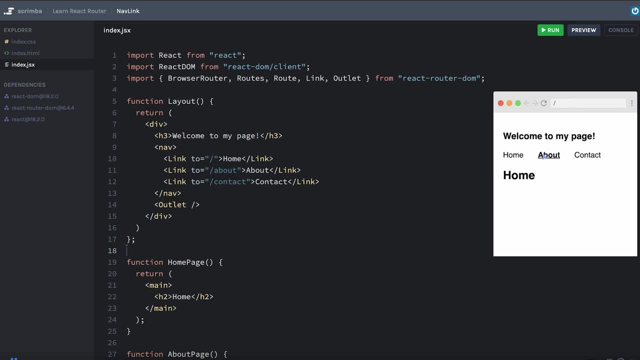 I have it set up so that when you hover over one of these links, it makes the link bold and underlines it. this is actually going to be pretty similar to what we do in the van life app. However, navigating around, there really isn't any visual feedback as to where I am, other than what's. 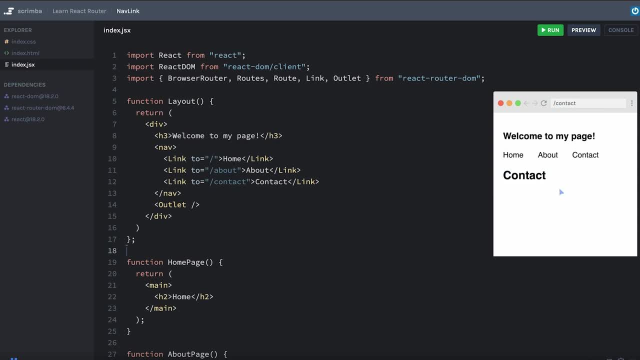 actually on the URL bar And, of course, the actual content on the page. a really common practice is to have the navigation bar highlight the item that represents the page that we're currently on. So if I click about and hover off of it, maybe I want to keep this hover style. 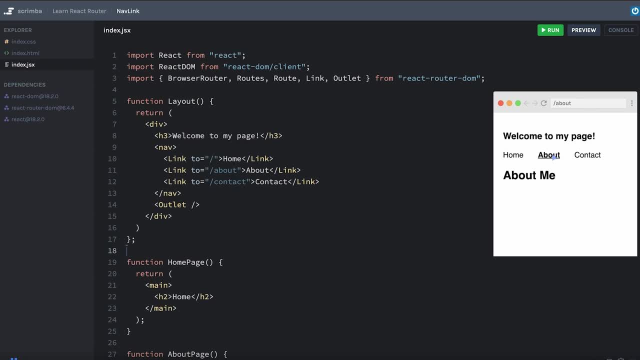 to be always applied to this link here. Fortunately, react router makes this fairly easy, And it uses something called render props, which, if you're taking this course as part of the full advanced react course, you have already learned about. So let's see how this is done. 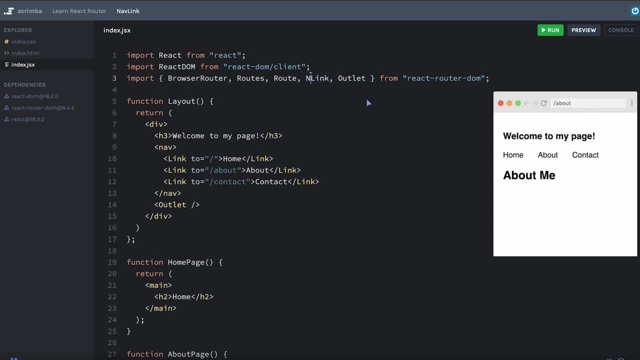 I'm going to replace the link import with something called nav link. Nav link is basically the same as link, except the style prop and the class name prop can both take a function as its value. Let me show you what I mean. First of all, I'm going to change: 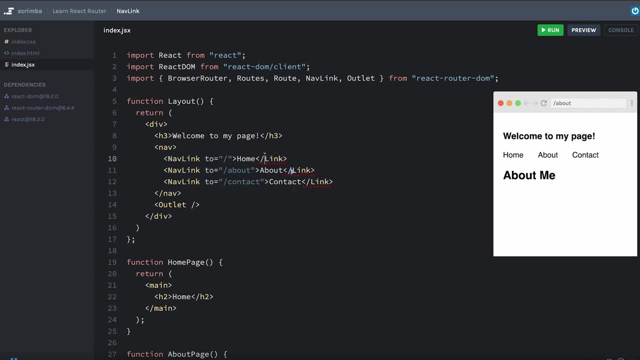 link to nav link everywhere, And of course, I have to do that here as well- And, as it stands, I can hit save. everything will work exactly the same as it was before- And it's, of course, not working the way that we want it to. yet where it keeps some visual feedback about what page? 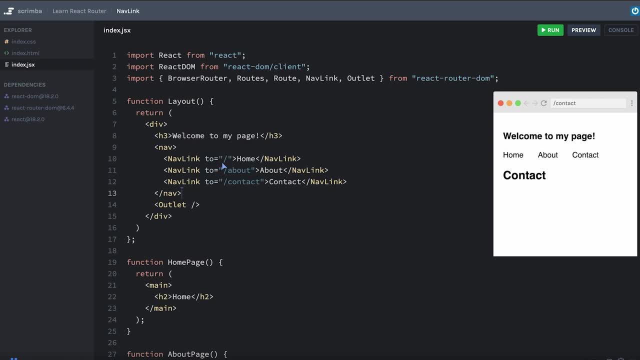 we're currently on, But that's where the difference comes with nav link. Let me actually put each one of these on their own lines. Okay, this might look like overkill, since it's got so few characters in each one. spreading them across five different lines is a little bit crazy, But we're going to. 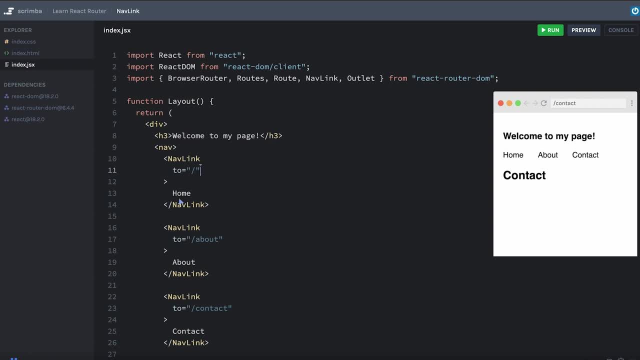 add to this. This will help make it look a little more visually distinct from one another. Let's start with this slash about link. here, As I mentioned, the nav link can take a regular class name, just like you might expect, And I could give this a string value, like I don't know. 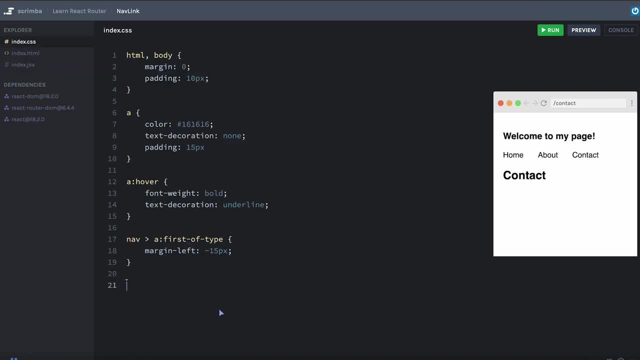 my link. then I can save that, I can go into my CSS, I can target my dash link. I can maybe say: the color is red. of course that's going to add that class name. no matter what route I'm currently on, you'll see them at the slash contact route. But just like we would expect in regular 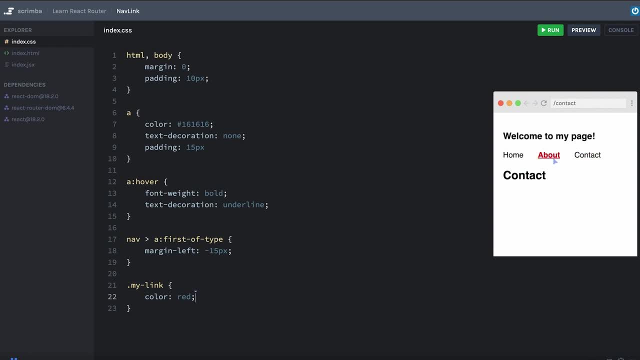 CSS. this is styling my about text here, my about link, as red. Well, with nav link, we can do this programmatically. Let's go over to where we're using our nav link And, instead of providing a string as my class name, nav link allows us to pass a function. Because I'm going into JavaScript. 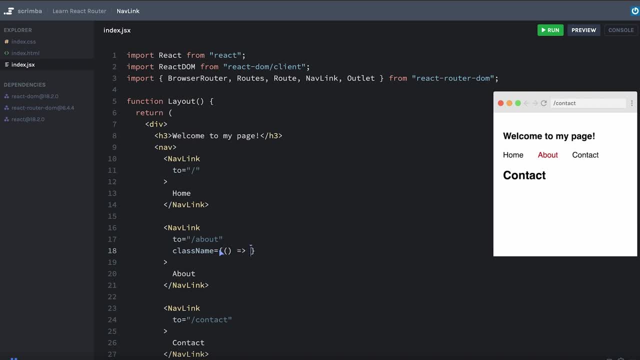 I need to use my curly braces And then I can provide a function, And whatever that function returns will be the class name that gets applied to my nav link. The reason this is beneficial is because React Router will pass this function an object and that object will have a property. 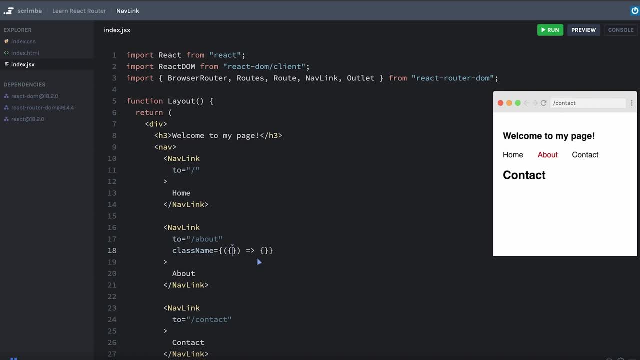 called is active. So right in line here I'm just going to destructure it. this looks a little bit crazy with the curly braces- parentheses, curly braces. But just know this is getting me into JavaScript. this is my function And it's an arrow function, So it's just parentheses, arrow. 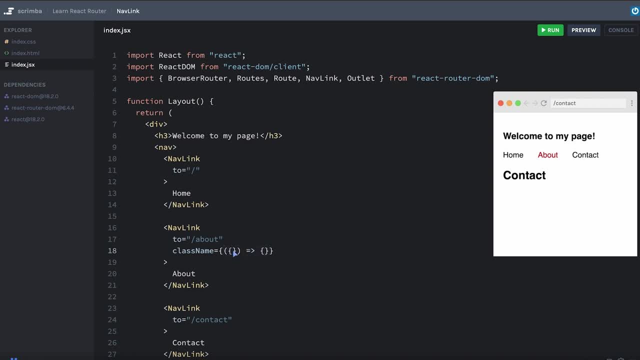 curly braces, And then inside of that function parameter, I'm immediately destructuring it. I guess I could say something like object, and then I would have to use the object dot syntax in order to do that. So I'm going to use the object dot syntax in order to do that. So I'm going to. 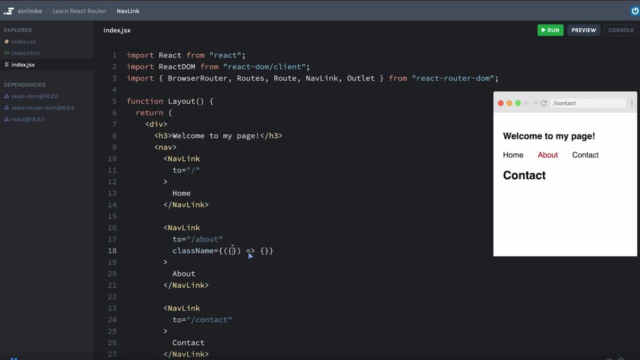 use the object dot syntax in order to access the property. In this case, I'm just going to destructure it And the property that I care about in this object is called is active. the is active property will be a Boolean And it describes whether or not this route, the slash about route. 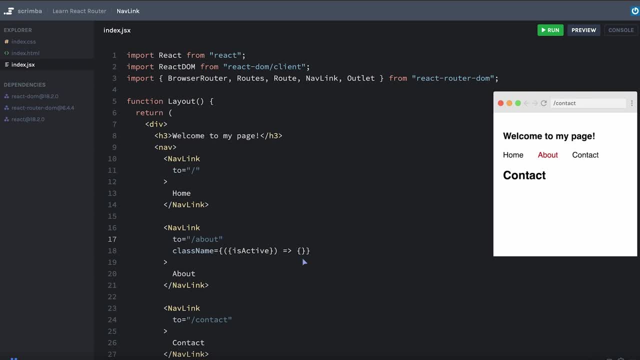 is the current active route. So this is nice because I can use it to determine what my class name should be. So inside my function I'm just going to use an implicit return. So instead of using curly braces and then having to use the return keyword, we're going to implicitly return. 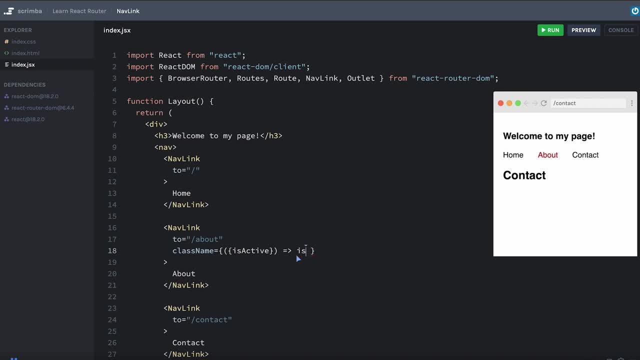 still need that last curly brace there And we're going to say, if is active is true, So it's a Boolean. I'll just say if is active, then I want it to be the class my link, But otherwise we'll just have an empty class or an empty string representing the class we might also be able. 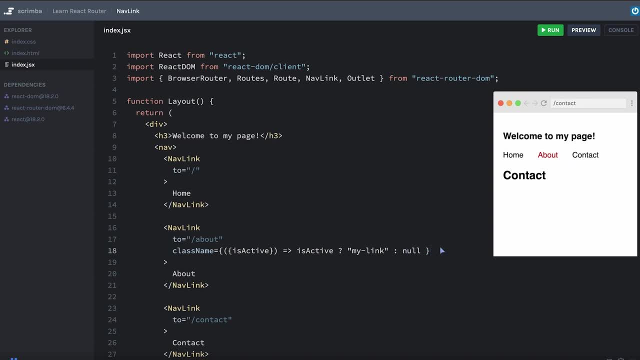 to do something like: no, let's see how this works, So I'll hit Save. Okay, we're on the slash contact route. Remember, we've only put this class name on the about link, So when I go to about, it turns. 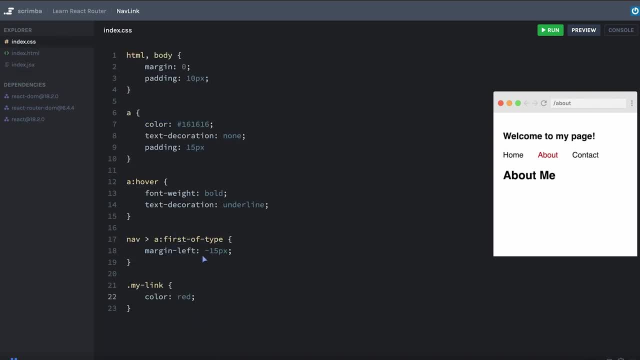 red and it stays red. Awesome. So it's not just on hover right here. this hover CSS rule is making it a font weight bold and a text decoration of underline, But the my link class is what's making it actually read. So I will make a copy of this and move it up to my home nav link. Then we'll do. 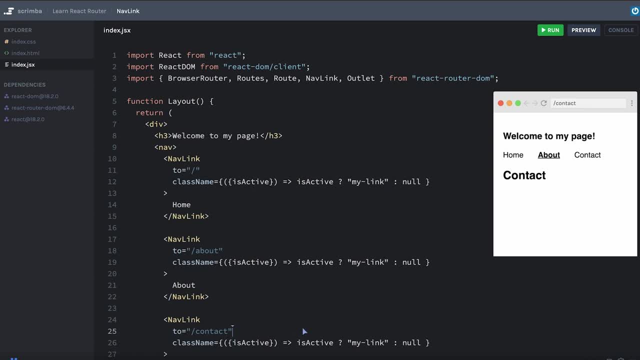 the same down to contact, And I want you to think for a second: when I hit Save, what is going to change on our page? Well, we're on the slash contact route And we just added this active style class name to the link that is for slash contact. So when I hit Save, it should turn red, Hopefully. 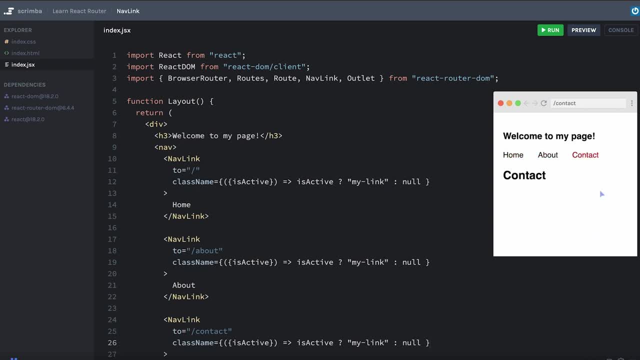 perfect, Okay, so now everything seems to be working. You might remember I mentioned that nav link allows us to either use class name or the inline style prop, And that is allowed to be a value of a function. So if I didn't want to define a separate style in my CSS, I could. 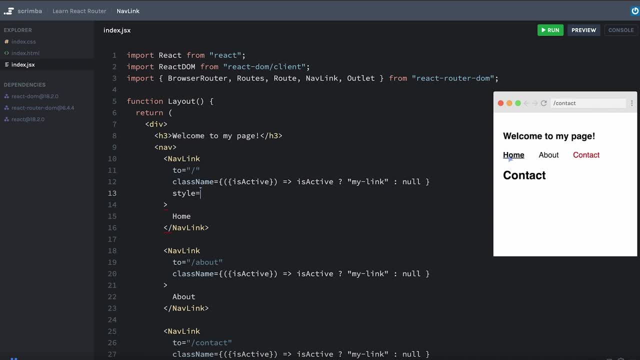 an inline style directly here Let's actually combine our hover state and our selected or our active state into one set of styles. So inside my layout I'm just going to create a styles object. we'll say this is maybe active style And we will have our font weight of. 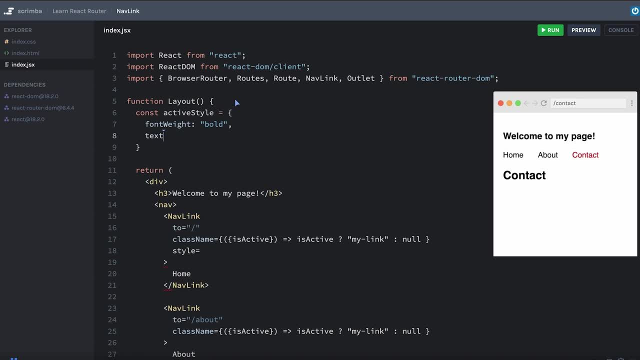 bold our text, decoration of underline, and we'll say: our color is red. Now the only thing left we have to do is to actually use this active style And we will just take exactly what we had with our class name, But instead of applying the last name of the string, my. 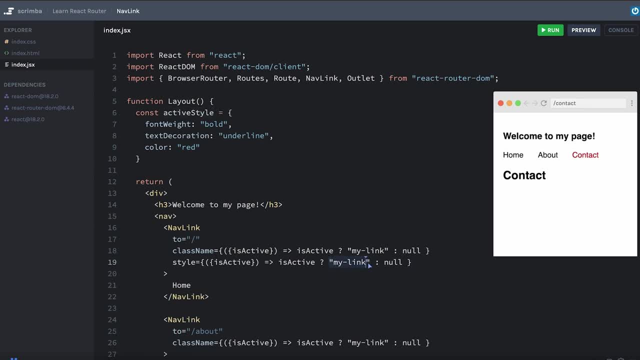 link, we will include our style of active style. So we'll just say if it's active, then the style should be this object of active style And otherwise. well, I think we can just keep. No, let's get rid of our class name And I will just copy these down here and clean. 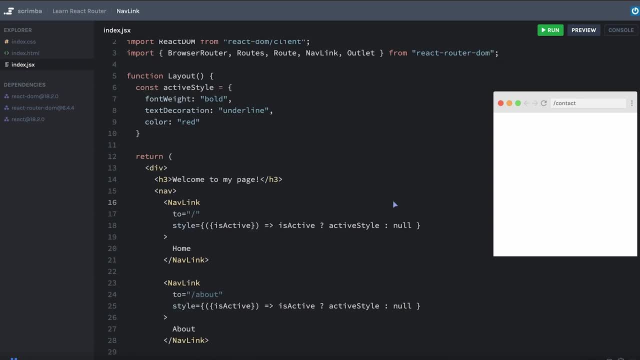 up our class names there And this should have the same effect, Although now our active style includes the underline and the bold, so it'll keep it kind of the way that it is on Hover State, except our Hover State is not red, So we would have to go over here. 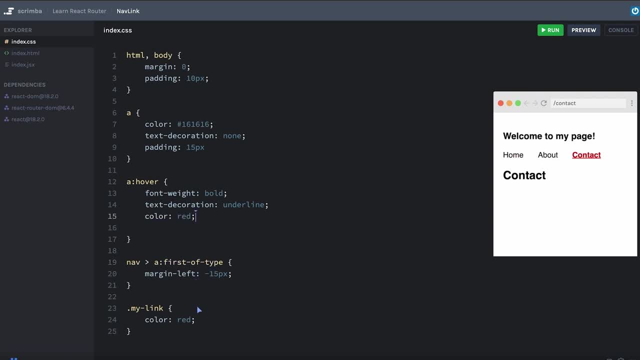 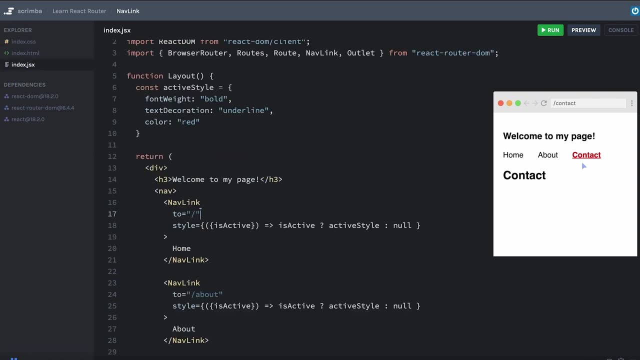 and say that the color is red, can get rid of this style here. Well, I'll leave it there for educational purposes, I guess, if you're looking through this later, Okay, so hit save Now. the hover state is the same as the active. 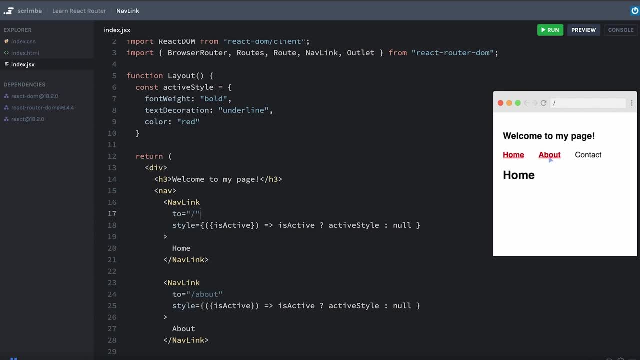 state And when we click over to home, that becomes the active state there. Awesome. Whether you use the nav link style prop or the class name prop is completely up to you. If you're working in a team, there will probably be some kind of standard or norm that you should be following, So just stick. 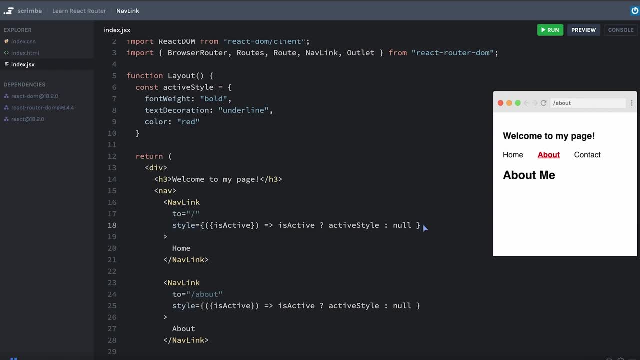 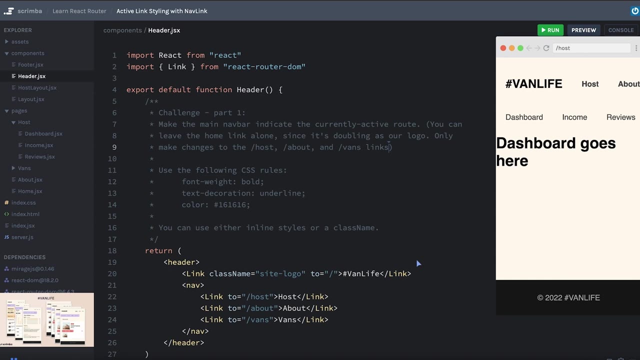 to whatever makes the most sense for that project in that team. Okay, now that we've got the basic idea of nav link down, we're going to back into the van life project and apply it over there. Let's apply what we just learned about the nav link elements to our van life app. We have a few. 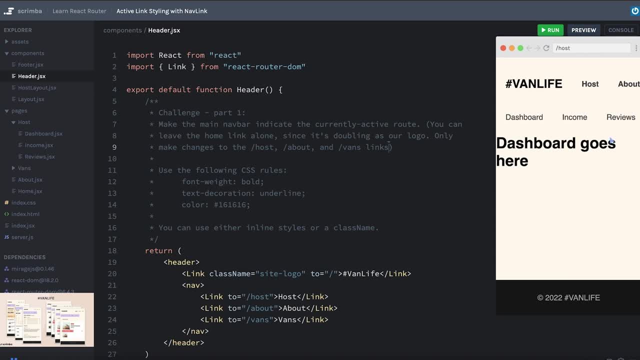 different places throughout our app because we have multiple navigation bars in these nested routes. So we're going to work on those one at a time, And there's going to be an extra thing or two that we learn along the way. To start, we'll do this easiest one, And that is for us to style the main navigation header up here. I've 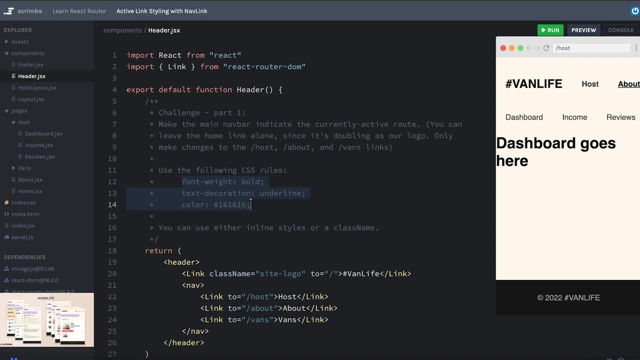 given you the CSS rules that you should apply to the link. if that's the currently active route that the application is on- And I made a little note to that- we don't need to style this link that goes to the homepage, mostly because that's kind of our logo right now. In fact, I should probably get 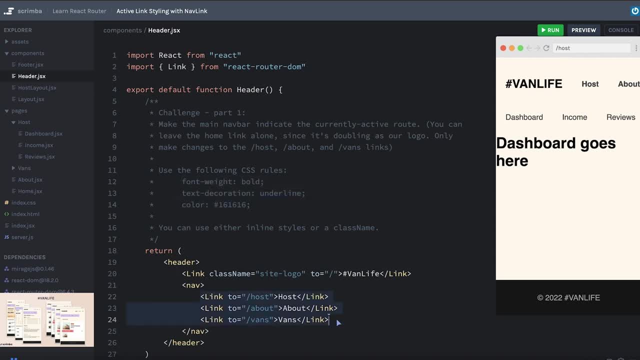 rid of this underline. that's happening. So only worry about these three links here, Don't worry about this link here. With that said, make sure you read through the challenge. I think you should have everything that you need to know To complete this challenge. So pause now and work on this challenge. 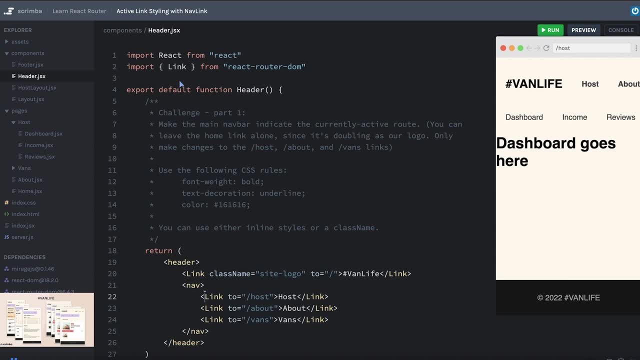 Okay, well, we know that we need to change our links to nav links. I do want to keep this link here, So I'm not just going to change my import, But instead I will also bring in nav link, And then I will change all of these to nav link As it stands. 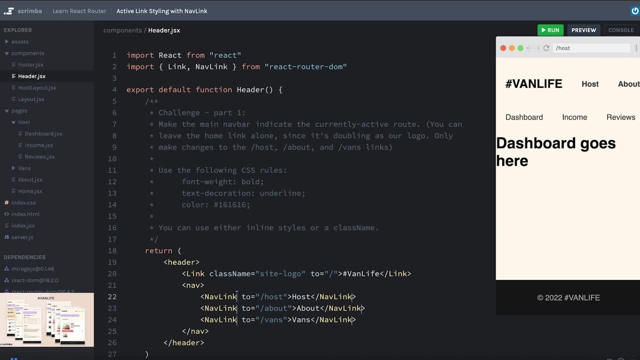 everything should work exactly the same. There's nothing different about nav link in its functionality, But it does add the capability of adding that active class or the active style. this is going to get a bit long vertically, So I'm going to separate things onto their own lines. 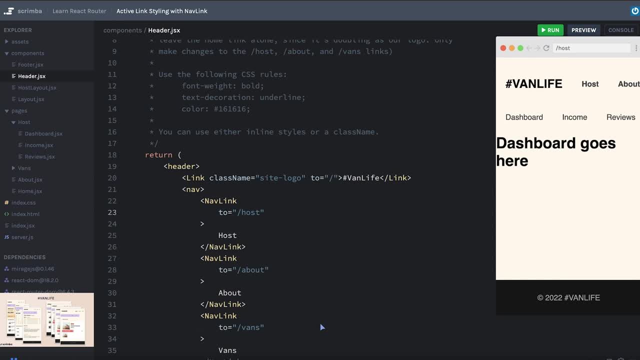 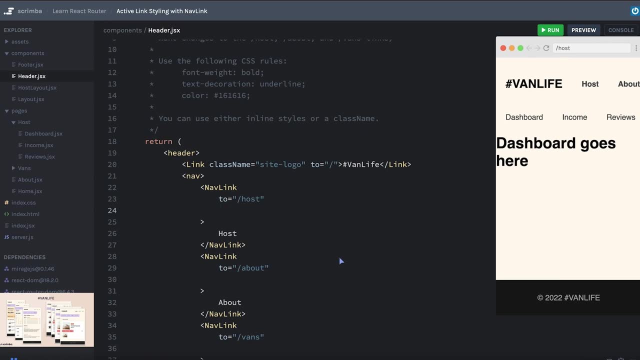 And since these are going to be repeating themselves quite a bit, I'm just going to keep my three cursors up here. And as it mentions, you could either use inline styles or you could use a class name. maybe just for the sake of seeing both ways, I will start with. 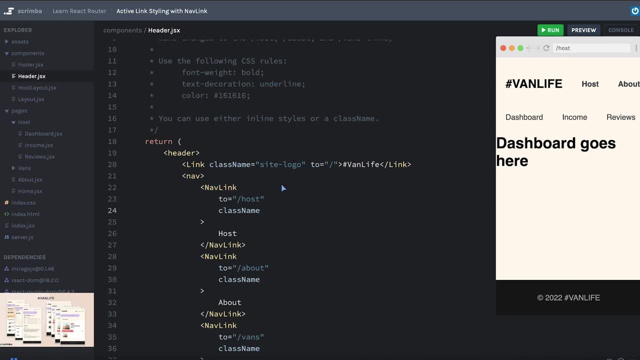 a class name, And the thing that's special about the nav link component is that I can provide not just a string as my class name, but I can pass a function. This is an example of nav link using a render props pattern, where we pass a function And when that function gets called. 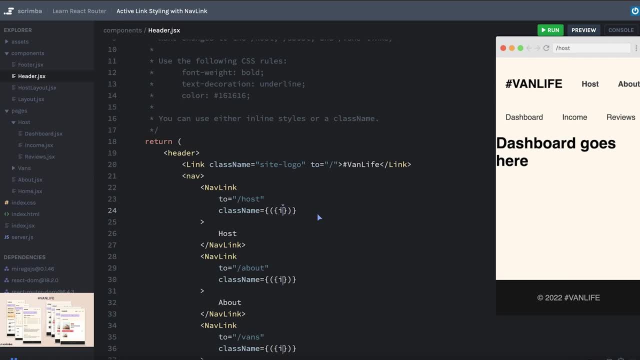 by the nav link component. it's going to call it with an is active property on an object. So it's going to call it with an object. there's also an is loading property on this object, But we're destructuring it to just make use of the is active property on that object And that way we know that. 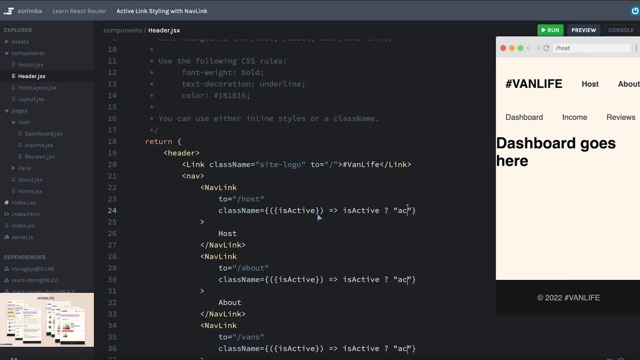 the is active is true, then I want to provide- maybe we'll call it active. link will be the class name. we haven't created that yet, But we'll get there And otherwise I don't know, we could say no, or maybe empty string is better. I'm honestly not sure. Last but not least, let's go Actually. 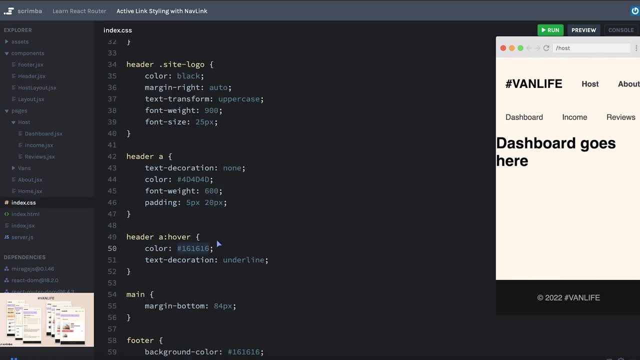 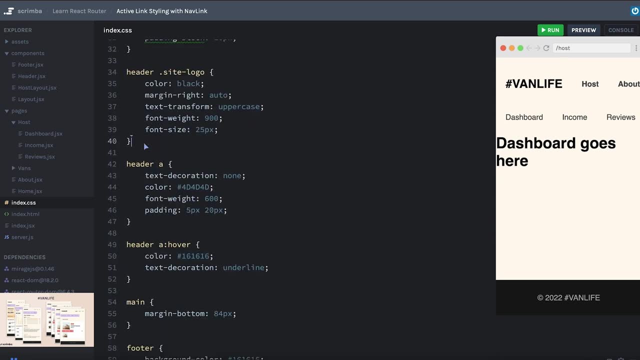 let's copy these styles here And we'll go over to our CSS And actually maybe closer to the top is where we'll define this Here. we're accessing some header anchors. let's just style all anchors class of active link. We'll give it those CSS styles. Let's get rid of these comment stars. 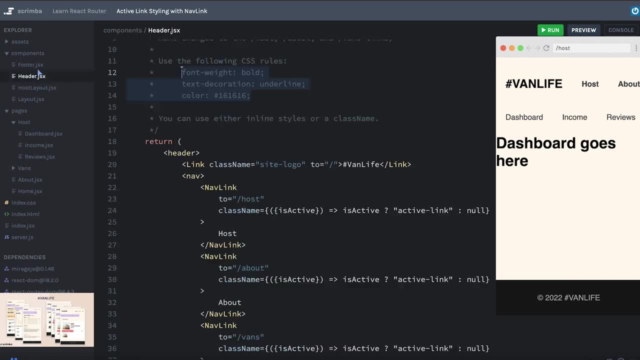 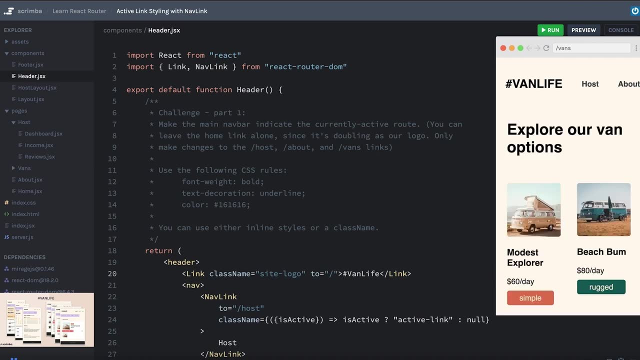 here And I need to make sure. let's see up in the header. I hit Save And okay, well, host is highlighted. That's good news. I click this and about is highlighted. Vans is working And this one is not, of course, because we left it as a link. This is really cool, because without a 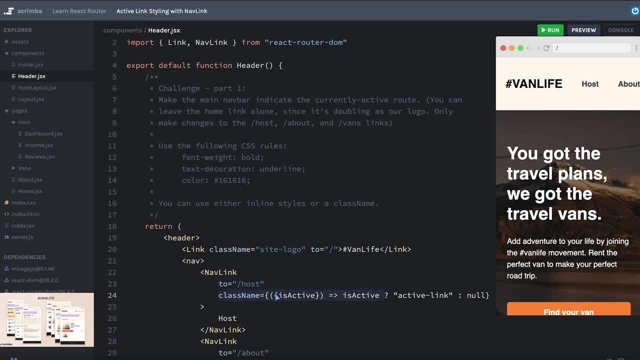 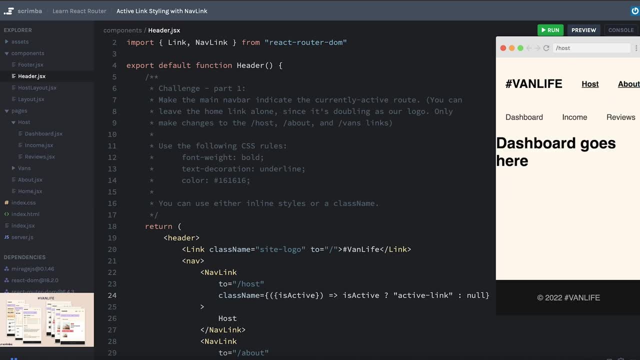 whole lot of extra knowledge under our belts just understanding this render prop pattern for class name. we were able to add something to our app that really does help quite a bit with the user experience in understanding exactly visually where they are without having to look up in the navigation bar, Especially because these days the URL bar 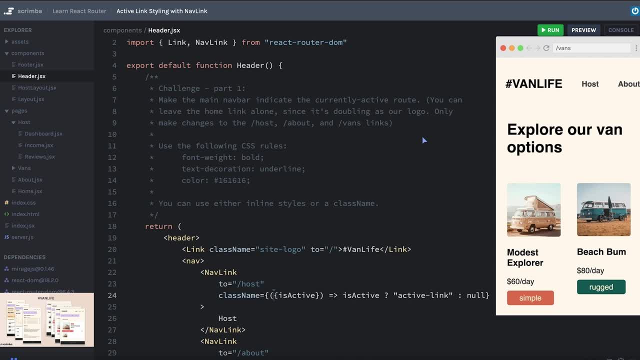 kind of obfuscates what path you're actually on in a lot of browsers. Awesome work. Hopefully you were able to complete that challenge. If not, feel free to go back and try it again. Next, we're going to go to this nested navigation bar that we have inside of our 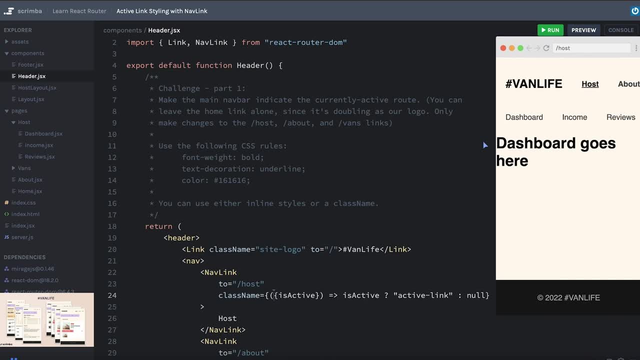 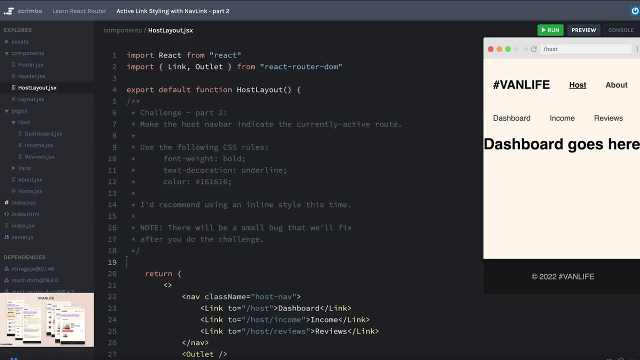 host routes And we're going to do the same thing. There's going to be a small caveat, but we'll get to that in the next challenge. Okay, we're going to do more of the same thing inside of our nested host view dashboard here. 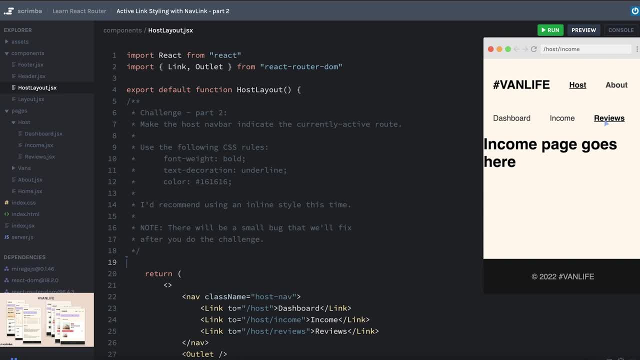 or navigation bar. here we have our dashboard, our income view and our reviews view, And none of them are really giving us a good indication as to which one is currently selected. So your challenge is to do the same thing here. you should know that there's a little caveat. I included it. 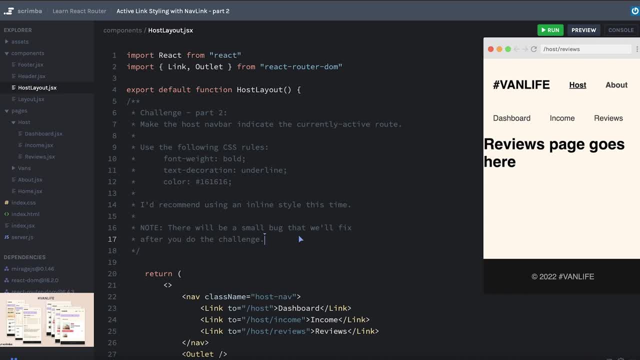 in my previous note. here there's a little bug that you're going to run into- It's nothing to worry about- while you're doing the challenge, But we'll be fixing it right after we do the challenge. This time around, I'd recommend using an inline style And instead of using a class name. 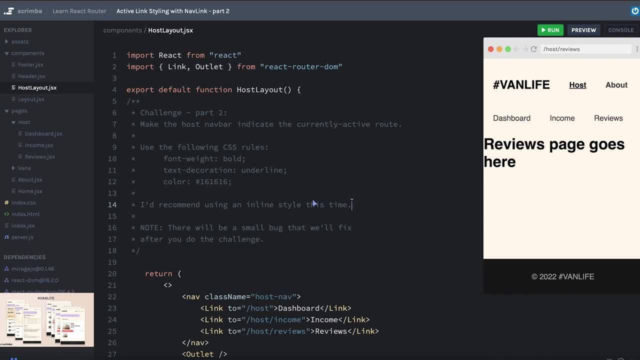 and I'll tell you why, after we do the challenge. but let's get your hands on the keyboard. pause now and add the nav links to our host layout navigation bar here. This time around we will not be keeping any of our links, So I'm just going to go ahead and hitik. 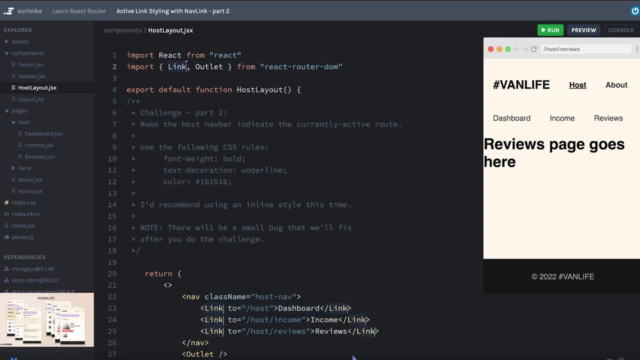 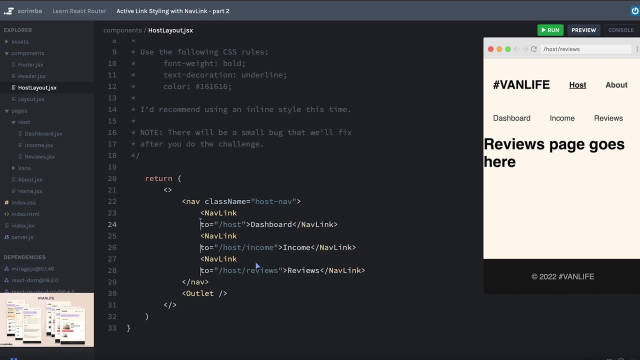 to replace my link import and I'll select all of these links while I'm at it. We'll replace it with nav link. That gets us a fair amount of the way there. Then I'm going to- because there's some repeated code and it's going to get a bit long- I'm going to put some of this stuff on its own. 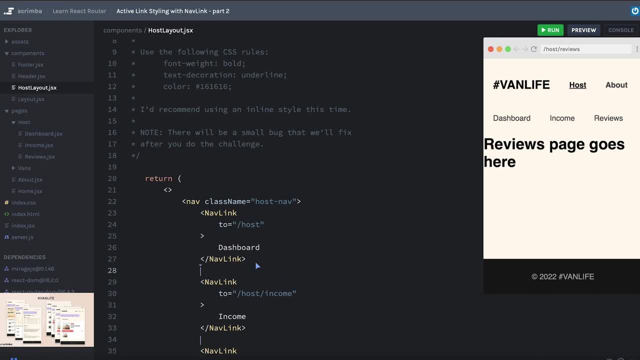 lines, just like before, And let's go up to this to line. And on the next line we're going to add a style prop instead of a class name. Again, the value is not going to be a string or anything like that, or even just a plain object. It's going to be a function, And that function will return the. 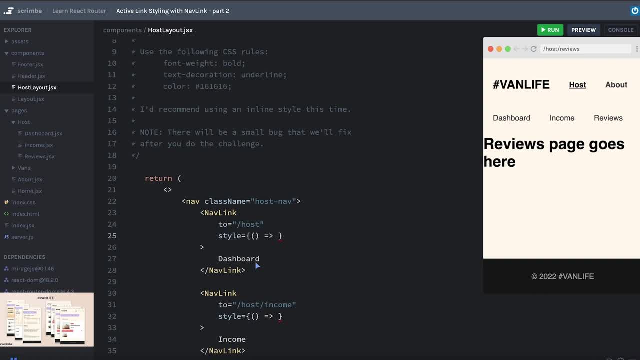 object that we want And we will receive in that function an object with an is active property. We'll use that to determine if we want the active styles- We haven't created that yet, but we will- Or if we don't want any additional styles applied, Let's go ahead and create this active styles. 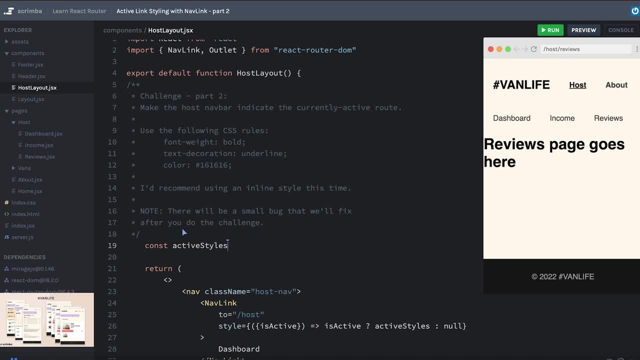 Just put it right here: Say: const Active styles is an object And let's pull in these properties Now, because this is an object and not just a CSS string. get rid of this stuff. We're going to have some syntax errors if we try. 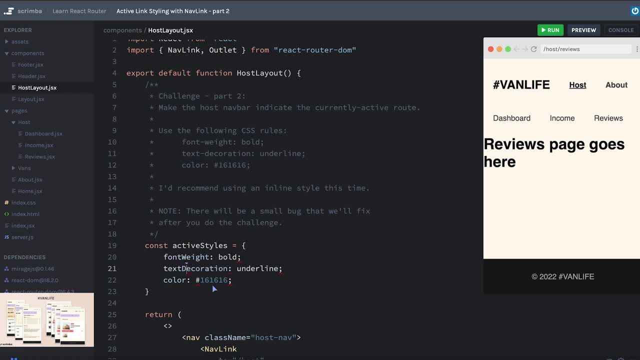 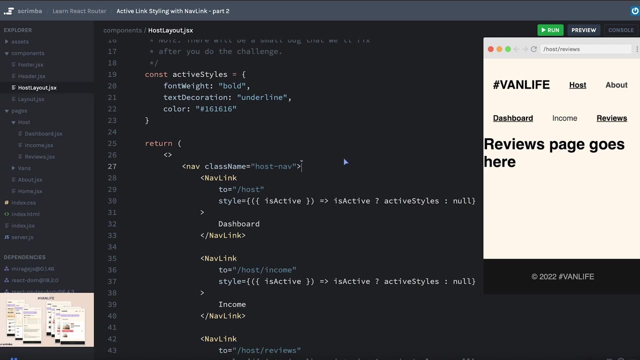 to just copy over the CSS, So we will use the regular inline styles in React. where we need that to be camel cased, These will need to be strings, And instead of semicolons we'll use commas. Easy enough, Everything is set up. let's hit save. Okay, we can see the bug here. we have both our dashboard and our. 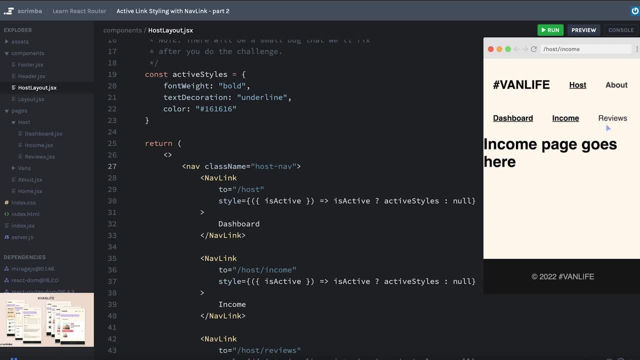 reviews showing as the active links. But we can see that for the most part it's working. we have income and reviews working, And then if we go to dashboard, neither income nor reviews are highlighted or have the active styles on them. So why exactly is it matching both the dashboard and the reviews? Well, an. 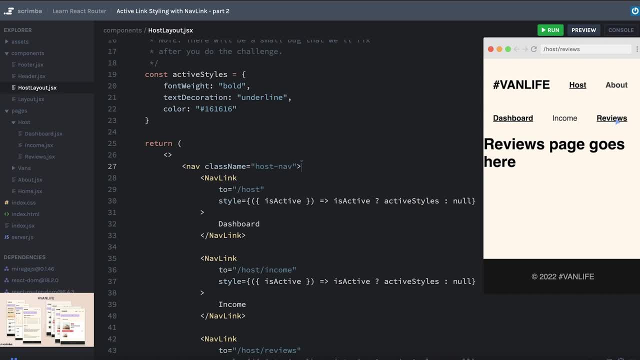 important thing to understand about react router under the hood is that it is not just matching a single route, it's matching multiple routes. Whenever you have a nested route like this. what I mean by that is under the hood, react router is matching Actually, I think. 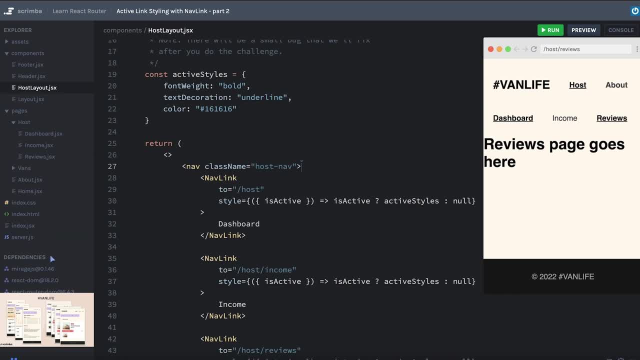 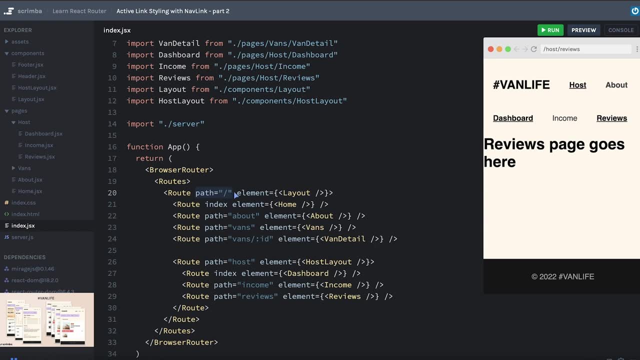 three routes here. The first one is the slash route. we go to our index here. as you might remember, we have this parent route that has the path of slash and that one is getting matched. In other words, react router is considering this an active route And that's really good for us because we want it to render this layout. Secondly, 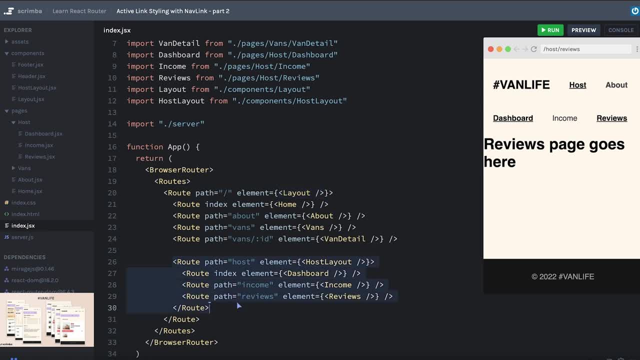 it's matching the host route, And that's again really good, Because we want it to render our host layout route. So when we're at slash host, it's matching both the slash route and the host route And therefore the link for the slash host route is being matched, or rather the nav link is showing as this being an active. 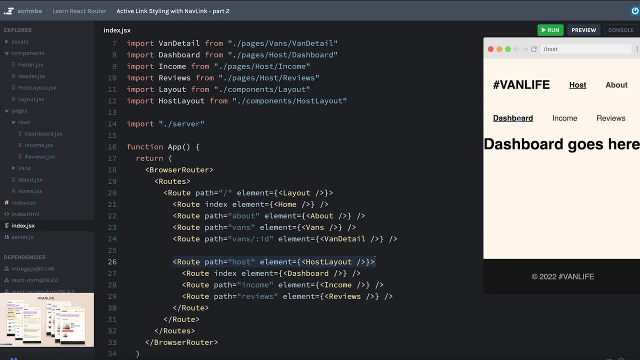 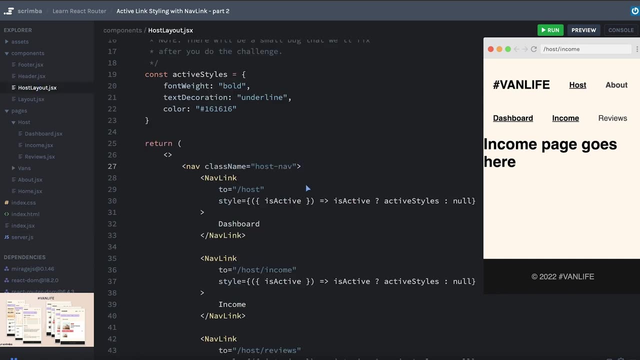 route. Now, when we go to income at the dashboard, it was matching two of these routes: this slash and this host. when we're at income, it's matching three routes: the slash, the host and the income route. Because one of those matches is the host route, this one. here our nav link is considering this host link as an active link. 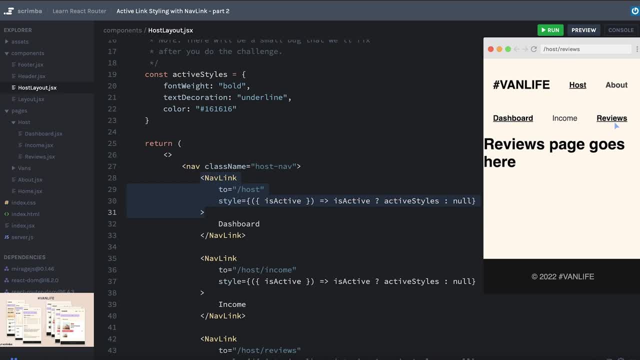 And therefore we get the dashboard being highlighted, even when we know that it's really the reviews page or the income page that is the active page. We didn't see that problem up with our main navigation bar because we decided not to change our logo here to the nav link. 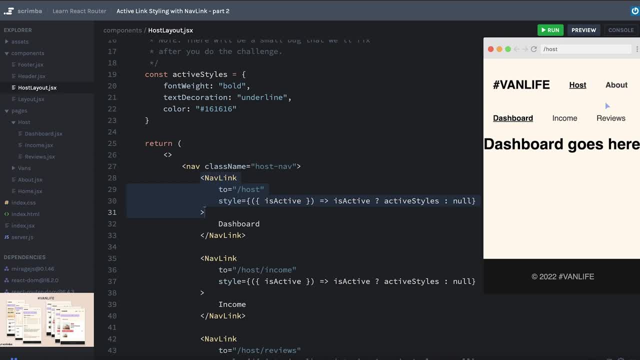 We kept it as the original link So we didn't run into this problem. But I think we would have if we had changed this van life logo to a nav link, because it is slash and host is slash, host. Anyway, I think you get the idea. 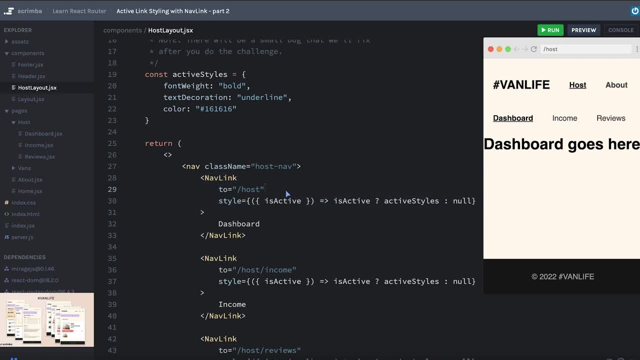 How do we fix it? Well, it's really easy. There's a prop that we can add to our nav link that's just called end, And what end does is it tells React Router to end the matching here. So if a more nested route matches, it won't also match this link on this route. 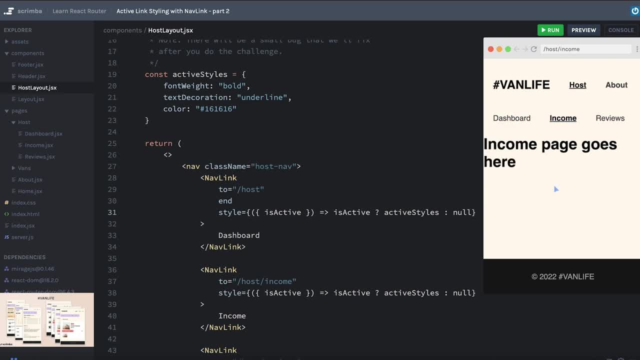 So we hit save, We'll go Over to income and now dashboard is no longer highlighted. This might look a little funny if you're not terribly familiar with it. When you just provide a prop name and not set it equal to something, it considers it a boolean. 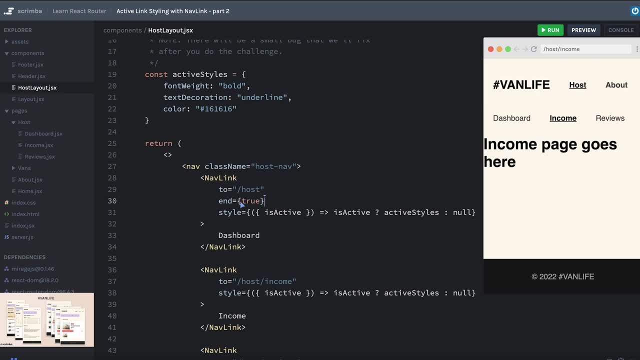 This would be equivalent to saying end equals true, or at least it would be functionally equivalent. in the documentation They just use end, So I'm going to stick with the way that they do it in the React Router docs. Awesome work, Let's keep moving forward. 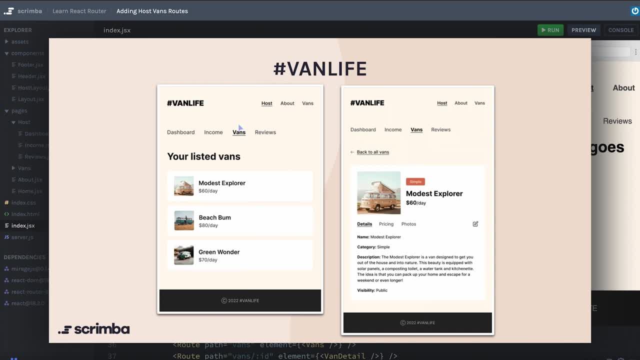 The next thing we'll be working on is the Host vans page. This is different than the vans page that we have in the nav bar- the main nav bar up here- because that lists all the vans on our entire van life site Going into the host kind of sub menu. the vans page here just is supposed to list the vans that this particular host is the owner of. 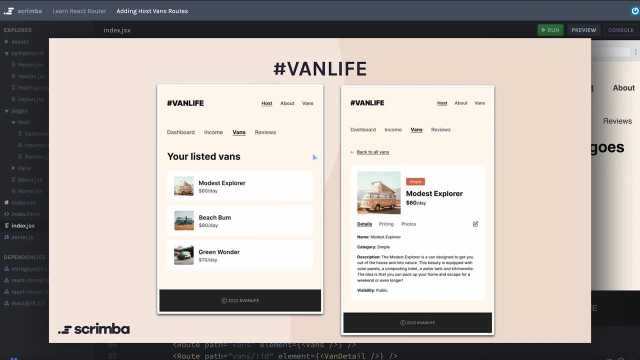 Keep in mind, we don't have any kind of authentication, so this is all a bit contrived, but the idea is the host would only see this host link when they're actually logged in, if they're a host, and they would only then be able to get to the host. 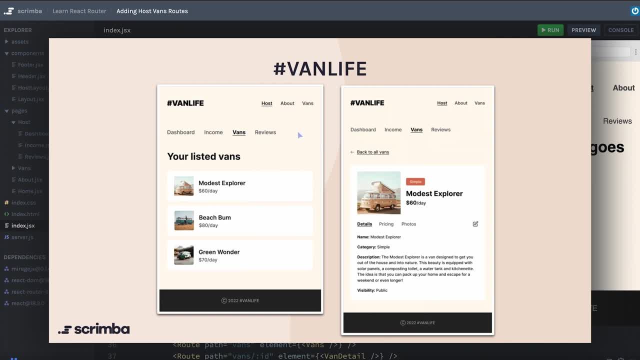 So this is all a bit contrived, This dashboard and navigation for hosts, but that's beside the point. Your challenge is to start off by creating these first two pages. You'll see there's a van list page, Again, the vans that this host owns. clicking on one of those will send you to the van detail page, and that van detail page has details, pricing and photos. 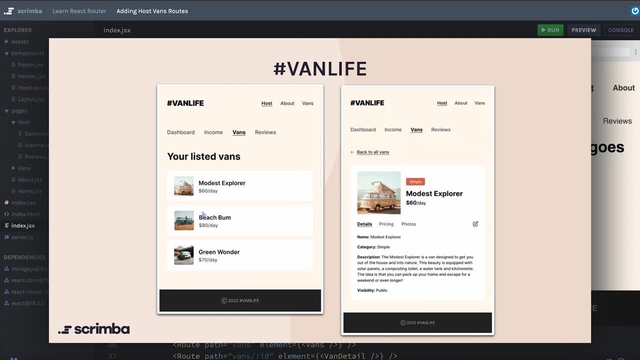 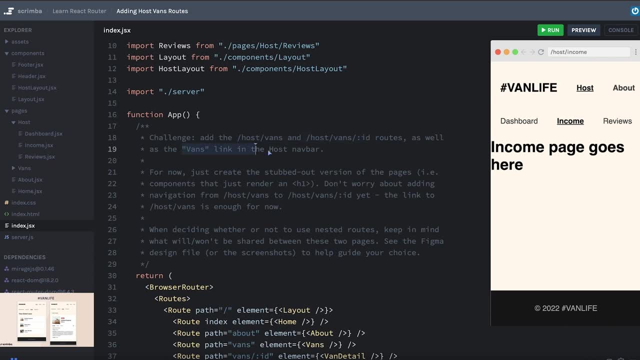 We're not going to worry about pricing and photos. We're actually not going to worry about any of the user interface that you see here, because the challenge is to add those routes and to add the vans link in the Host Navbar. right now we just have dashboard, income and reviews. 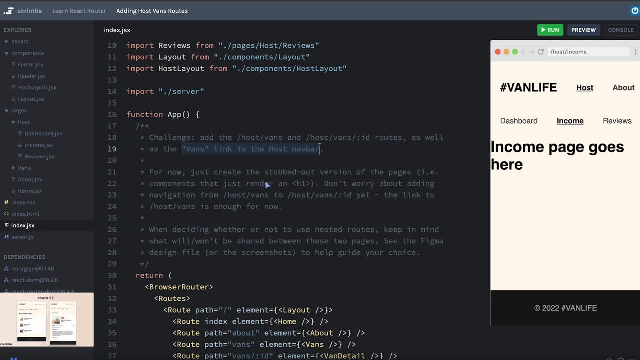 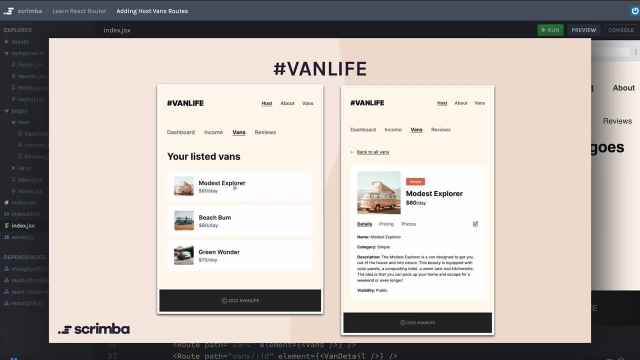 We need to add the vans link there, like it says. just create a stubbed out version of the pages that return an H1 for now and don't worry about adding the navigation from host vans to the host vans detail. In other words, because you're just going to have an H1 that says host fans page here, there isn't going to be a way to have a link to the individual vans quite yet. 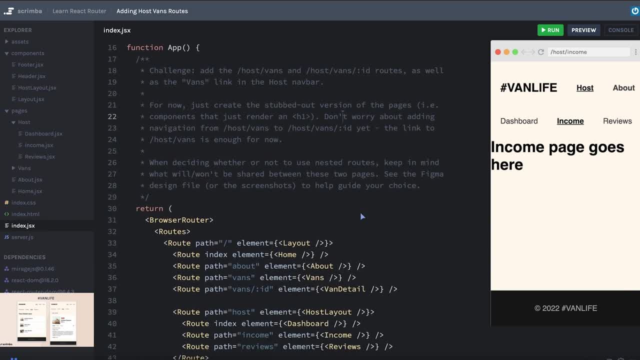 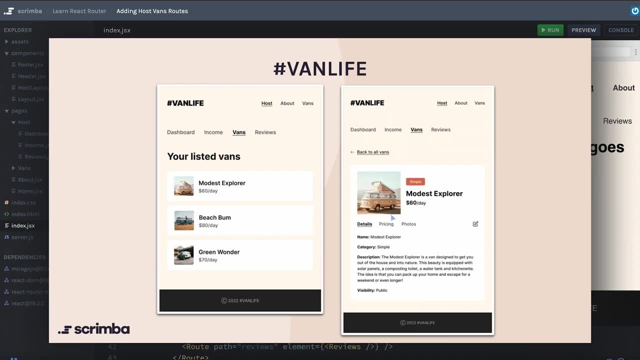 Don't worry, we'll get there soon. as a part of this challenge, you'll need to decide whether or not you'll be using nested routes, And I want You to keep in mind what will or won't be shared between these two pages. you can take a look here. remember that the navigation bar is being provided by the host layout component, not the host vans component, so I'll leave that up to you, and I think that's all the primary you need. 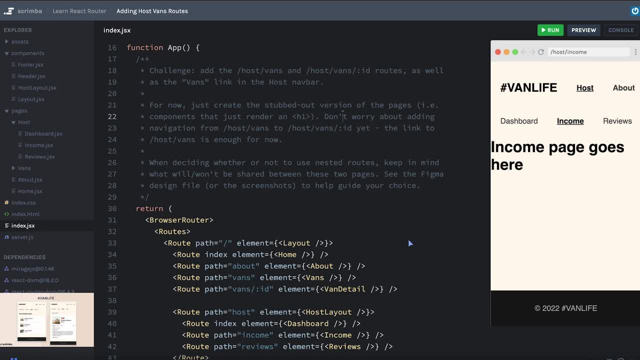 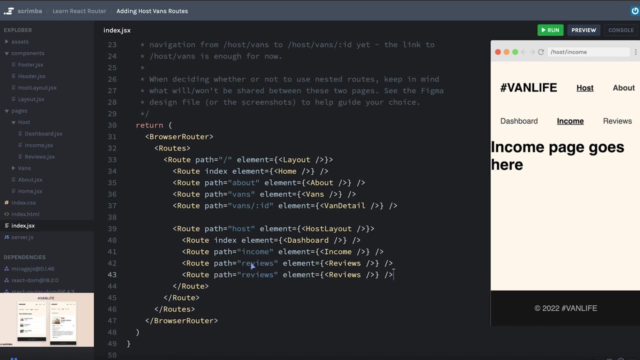 So pause now and work on this challenge. We already have the slash host, slash host slash income and the slash host slash reviews pages, So all We need To do is create another route here or slash host slash vans. when that page is reached, let's create an element that will call maybe host fans and for now we'll just create that component in our host folder here will call it host fans dot JSX. in will set it up like normal. 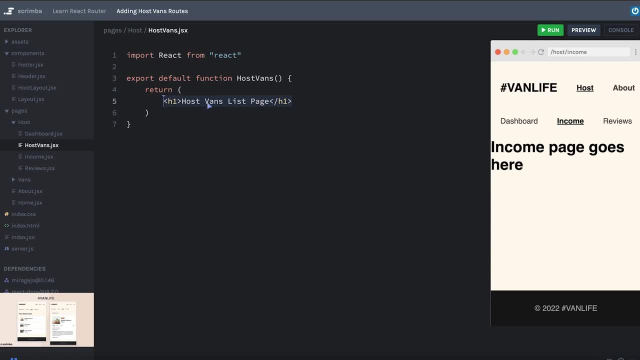 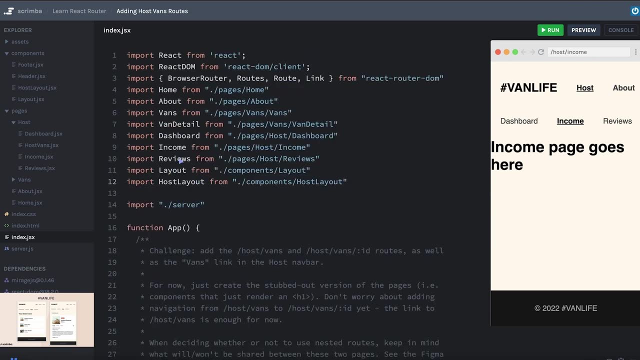 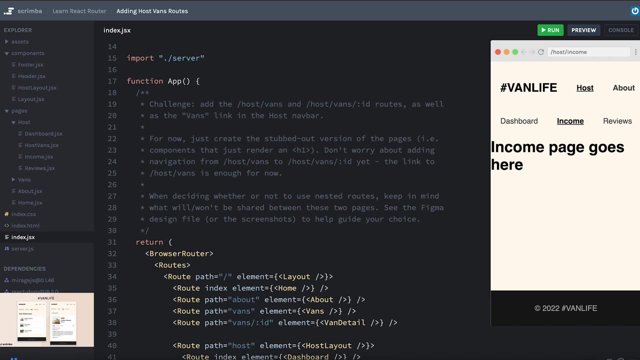 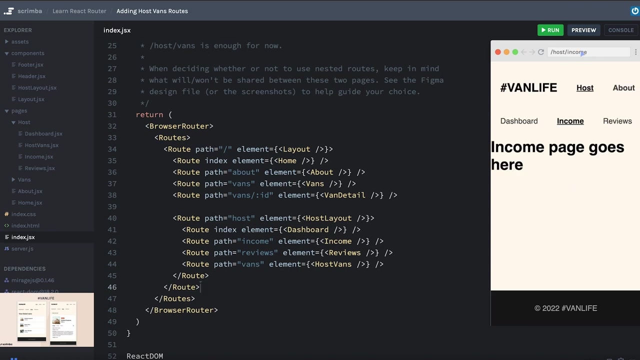 As I mentioned, for now it's just going to return an H1 will have its a host vans list page. let's go ahead And Import that over here so we don't get that broken, and actually let's copy this reviews one and we'll just make the change. there will say host vans and that's the same name we already chose for our element. so well we can hit save. we don't have any kind of navigation there, but I should be able to change the URL to say slash host, slash vans, and we're at the host vans list page. awesome. 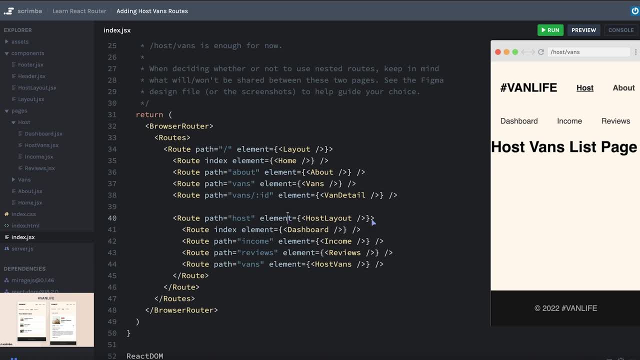 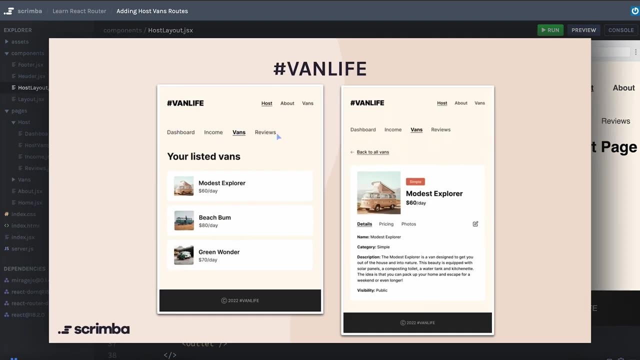 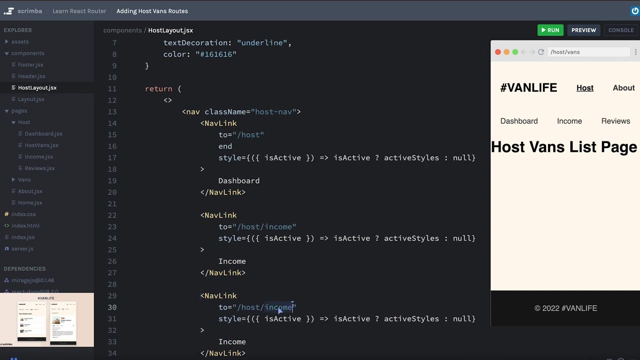 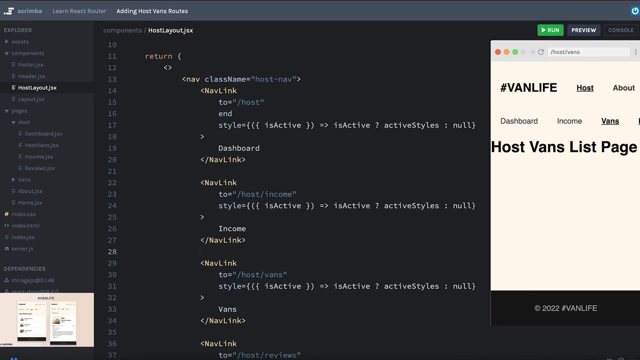 Let's add that to our host navigation before we worry about the host vans ID page Or the host vans detail page. you could say this navigation bar, if you remember, is under host layout, and I will simply: well, let's look at the design. design has dashboard income, then vans, then reviews, so let's just follow that. that means I will copy this income and put one right below it, will change it to slash host, slash vans, and will change this to say vans save. awesome, now we can actually navigate between these pages now. I imagine the biggest struggle was trying to figure out how to do this. 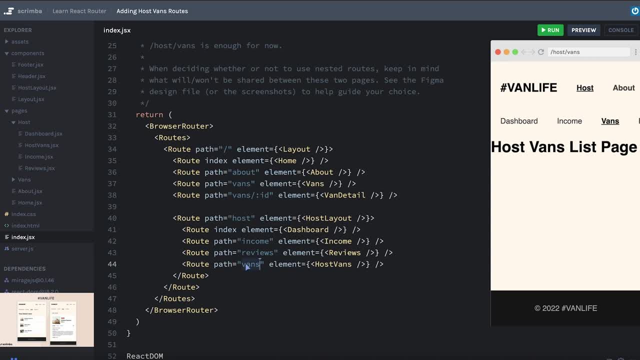 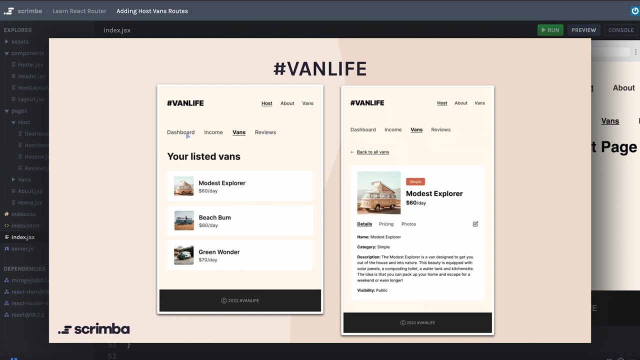 Was Trying to figure out how to do this. Trying to figure out how to do this, Trying to figure out if you should nest the vans, or rather host vans slash ID, as a child of this route or if it should just be a sibling route like this. and if you remember, our decision up here in not nesting was because they didn't share any user interface, and that's actually the case here as well. we look at these two. there's nothing that shared between these two that isn't already being shared from a layout route above, in which case it would be a lot more trouble to try and nest these two. 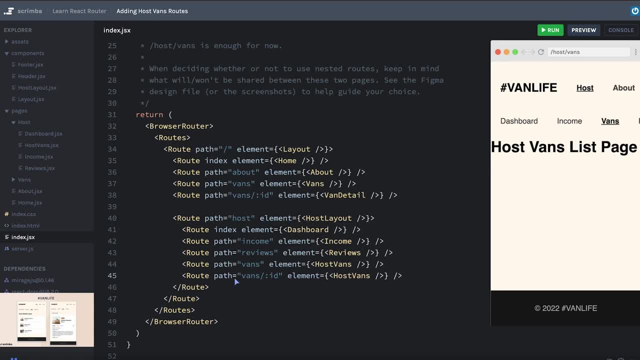 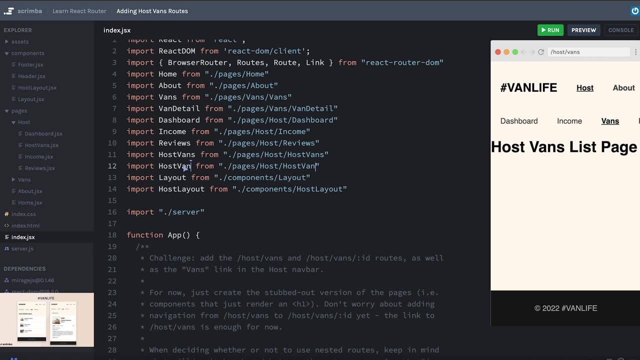 So in my opinion, I'm just going to say: going to have a van slash, call an ID and that will be a sibling route to the vans route and we will call this host. then detail doesn't exist yet but will create it, will copy this host fans and change it to host and detail and then create this component in our host pages. so we'll say host and detail dot JSX. 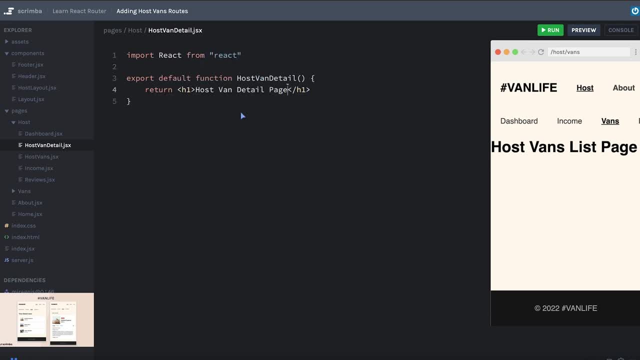 Import act from react and get everything else set up like. All right, let's hit. save no errors. that's good. again, we don't have a way to link over there quite yet, so in the navigation bar I'm just going to say: host van slash one. 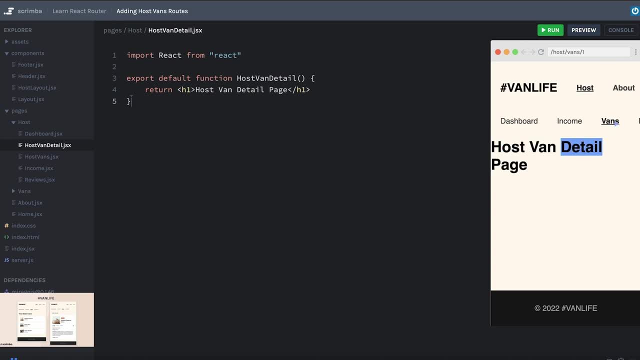 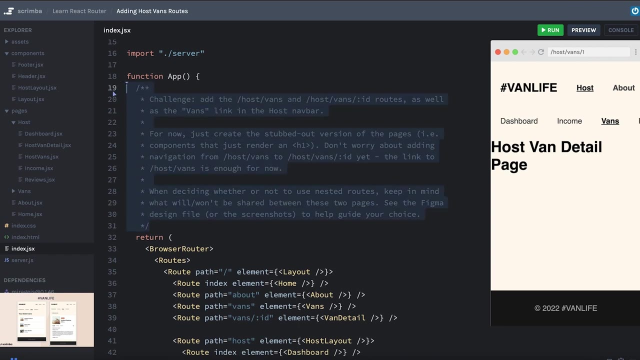 And there we go: host van detail page. it was a little bit subtle between the two, because this one says vans list page and this one at slash one says vans. nope, that didn't work. slash one, then detail page, and that just about does it for the whole challenge. yeah, we finished everything here. 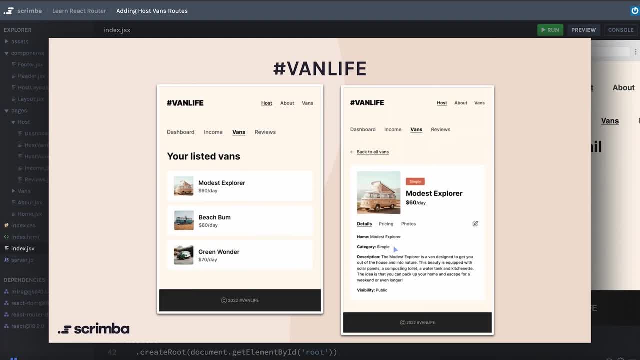 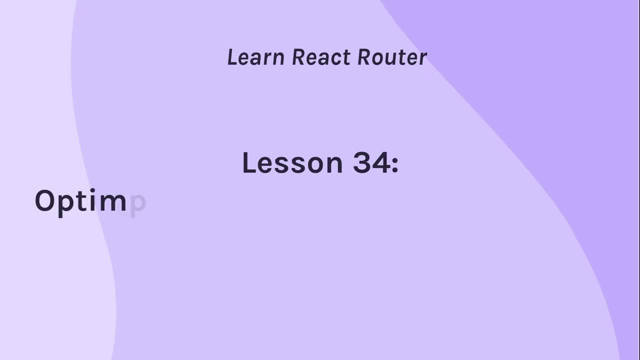 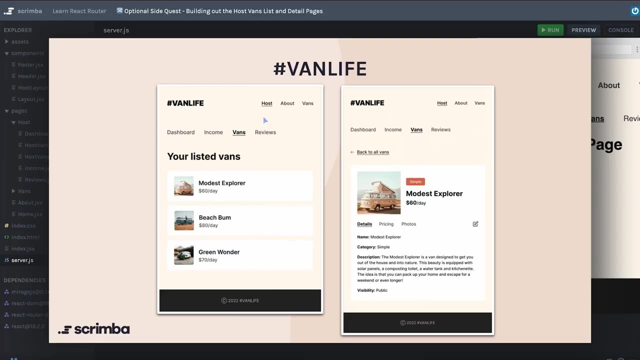 Awesome, it's clean this up. all right, this gives us a good start. the next thing we'll be working on is getting these nested routes implemented as well, so that's what we'll jump into next, Because we need a way to get from our van list page, or rather our host van list page, to the host and detail page. we do need to build out this page here. however, that doesn't have a whole lot to do with react router, so I'm making it an optional challenge for anyone that needs to use a react router. 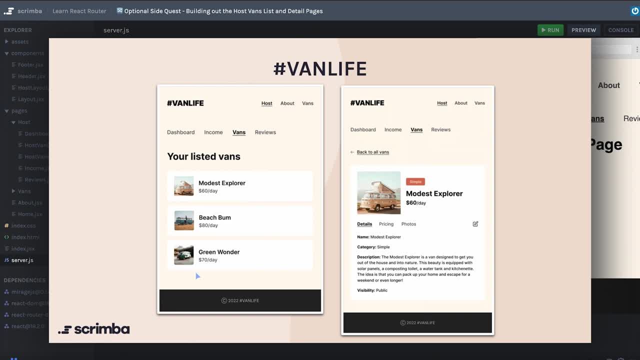 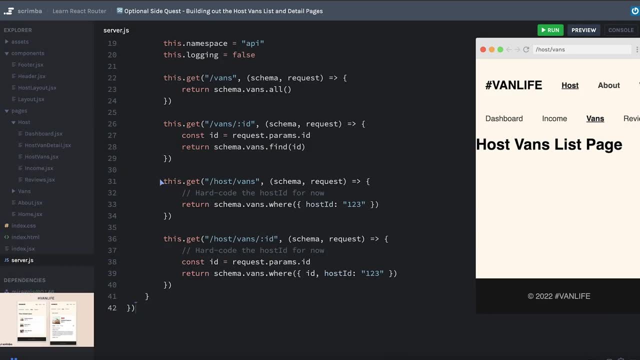 who wants to really flex their React skills and exercise what they've learned in React in general. to build out this page, To make that a little more possible, I've added some endpoints to our server: the slash host, slash vans endpoint, specifically. that will return only the vans that are owned by. 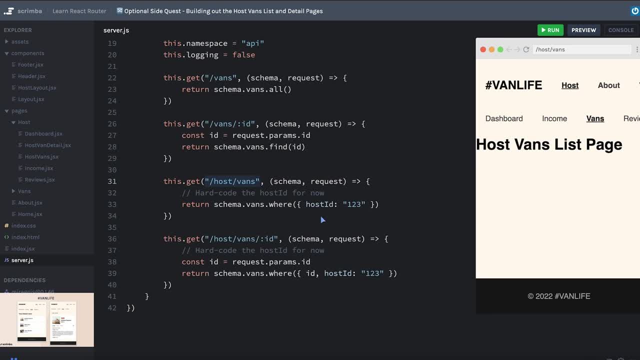 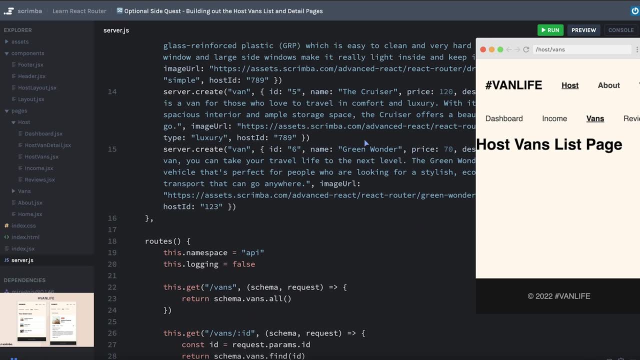 the specific host that we're pretending to be logged in. as You can see that it's searching all the vans where the host ID property is equal to 123.. That's not something that used to exist, but up here I've added a host ID to a number of these vans, some of them including 123.. I think 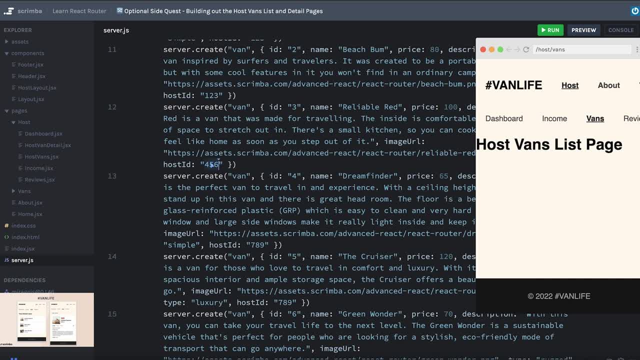 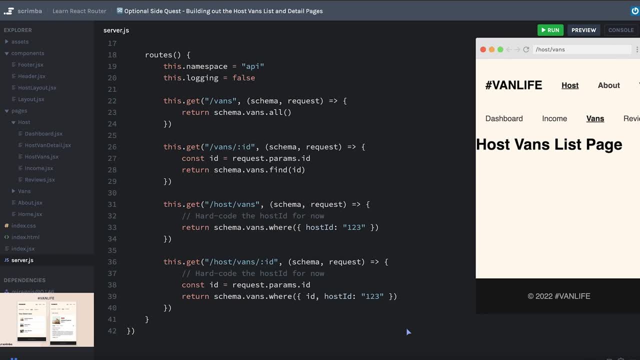 three of them have the host ID of 123, and the others have just random other host IDs that are not owned by the currently logged in host. air quotes around: currently logged in. Remember, all of these requests are implied to start with slash API. so when you make the fetch request, 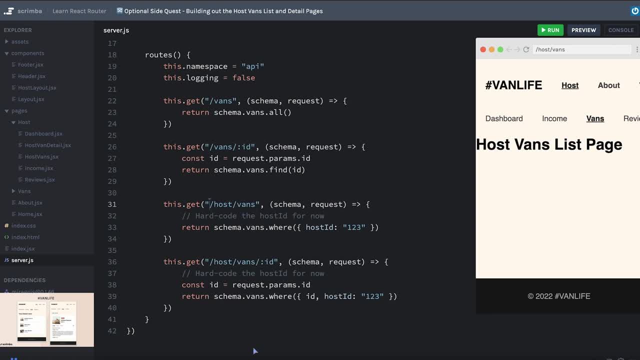 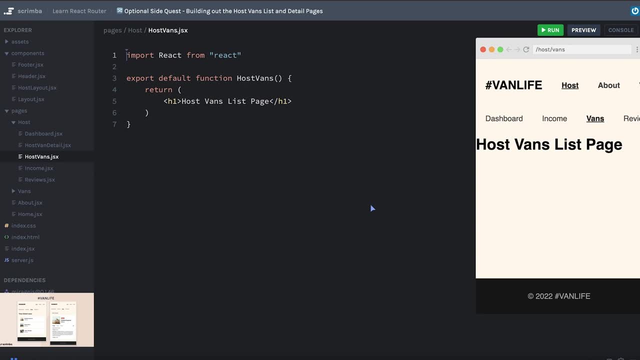 you'll make it to slash API, slash host, slash vans. What actually gets displayed will be here in the host vans list page. Again, this is an optional challenge. I'm not going to be walking through the actual creation of this because it's a fair amount of work, but this is the time to pause if you do want to work on that. 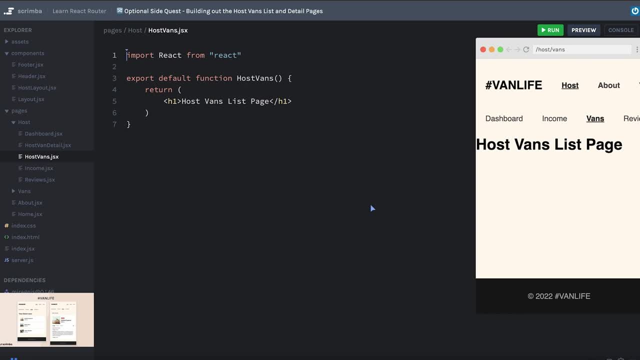 optional challenge. If you know anything about me, you know I don't do this very often, making these challenges optional, So I'll nudge you once again. if you are feeling a bit shaky on your React skills, then once again, I really implore you to go back and to do this optional challenge. 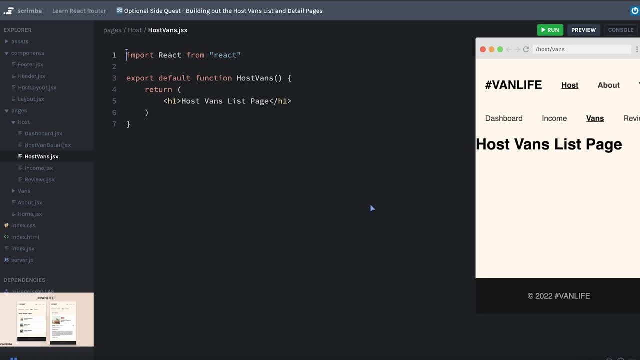 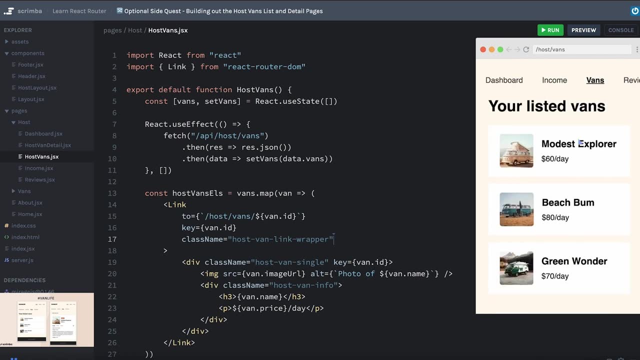 But otherwise I'm just going to pull out my magic wand, snap my fingers and just like that we have our vans list page built. As I mentioned, there were three that had the ID of this particular host or the host ID of 123, and that is these. 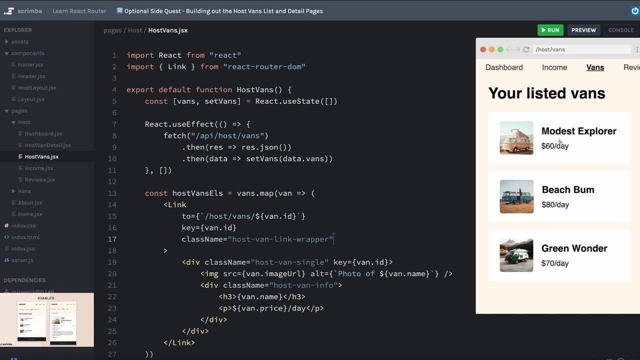 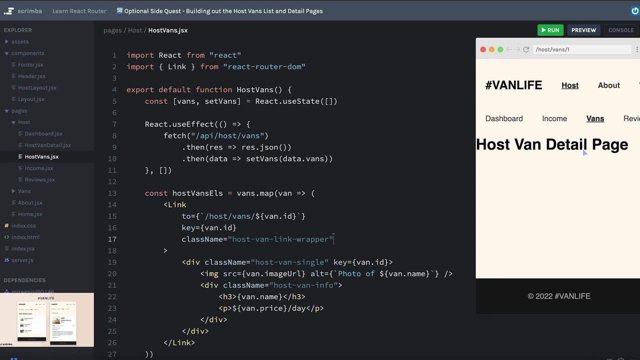 three vans that you see here. We have not yet built out the detail page. We're going to work on that next. If you click it, it does take us successfully to the host van detail page, but of course there's nothing specific to this one van here. A few key things to note is that when we're 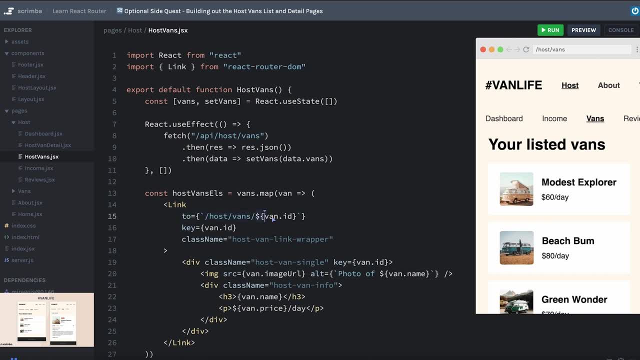 creating a link to the host vans slash colon ID and we make sure to dynamically fill in the ID of the currently looping over van or the van that we're currently looping over in our use effect. you're seeing that we are creating our fetch request to slash API, slash host, slash vans. We're. 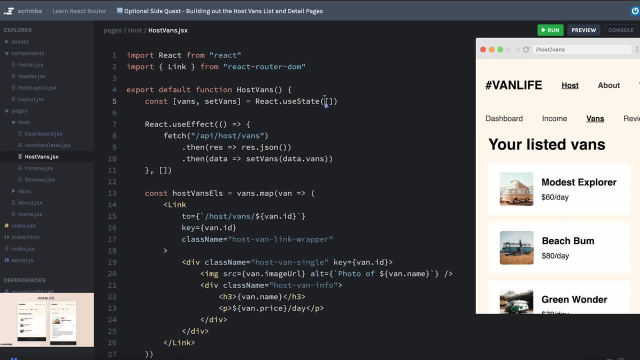 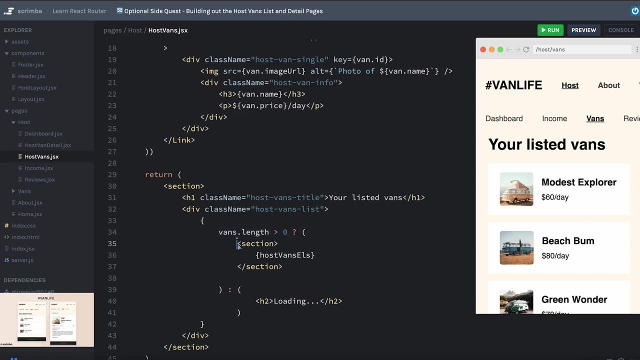 setting that into the van state, and because we're initializing our state with an empty array, we're checking if the van's length is greater than zero and if it is, then we're displaying the van that we created above, but otherwise we're just creating this loading element here. Now that I 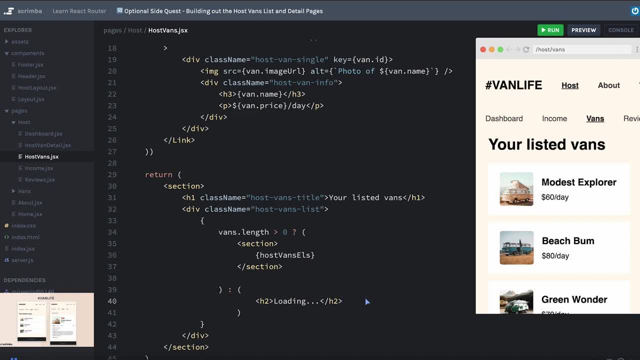 look at this. this isn't going to be a problem, but there could be a little bug where if the currently logged in host has no vans, it's just going to say loading forever. So I've used kind of a cheater's method here of getting whether or not it's loading. Usually we would look for some. 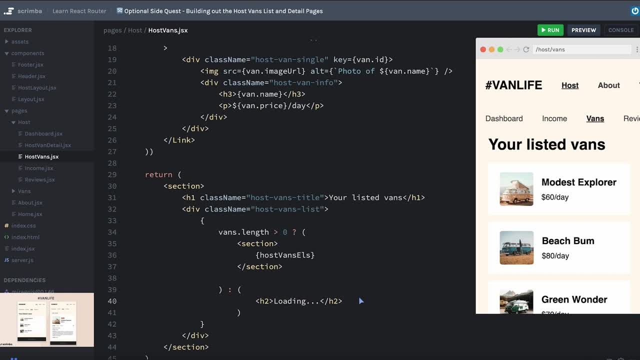 kind of loading state, but that's a topic for a completely different lesson. Okay, if you did this challenge, hopefully it wasn't too hard. If you didn't do this challenge, I know for a fact that it wasn't too hard for you. but now we're primed. 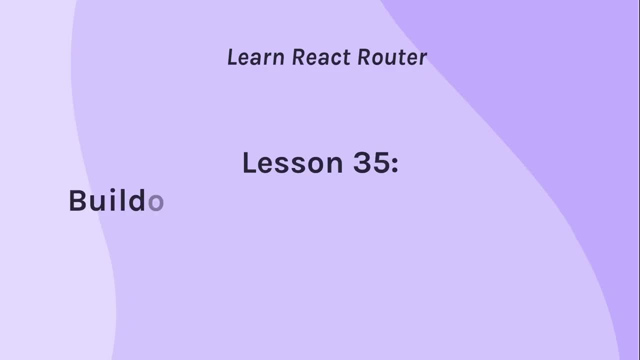 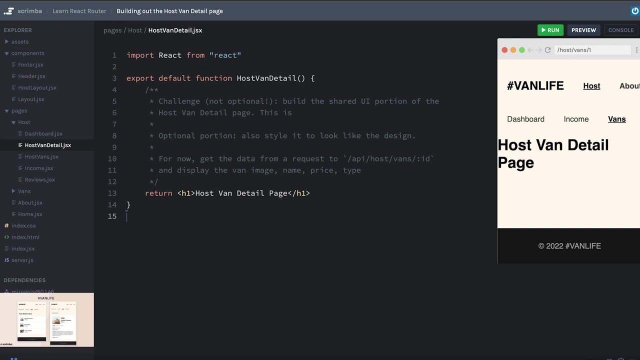 to work on the detail page, so that's what we'll be doing next. This challenge marks the start of embarking on, I think, the most complicated part of this app, so we're just going to take it one little step at a time. That said, most of the things that 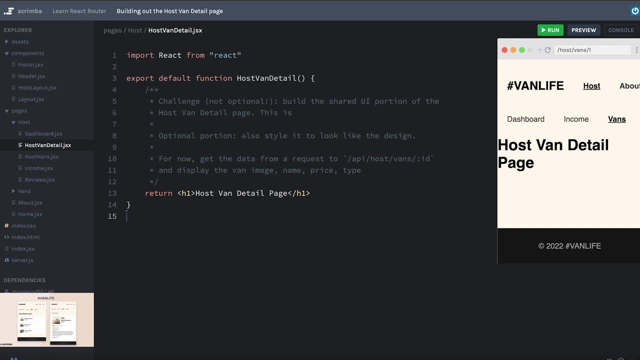 we'll be covering should be things that you already know. We're going to add some new knowledge along the way, but in the meantime, most of this should be doable, and if it is a really big struggle for you, that's a good indication that it's time to go back and just 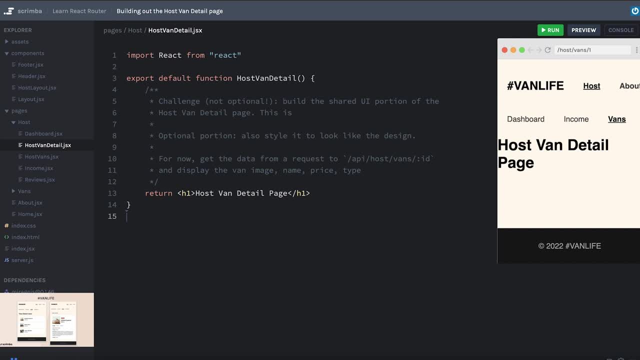 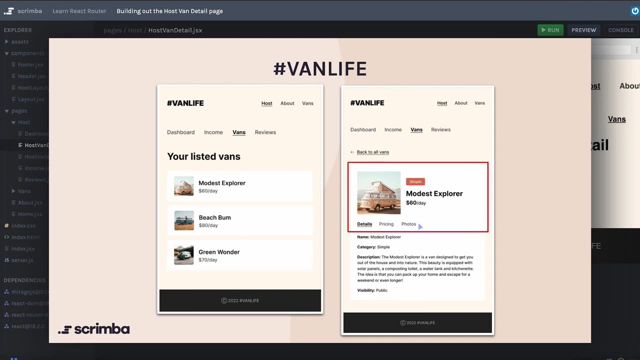 to review some of the things that we've learned. The challenge here is to start building out the shared UI portion of the host van detail page. so that's this section right here at the top, and if you remember from, let's see one of these past slides here: 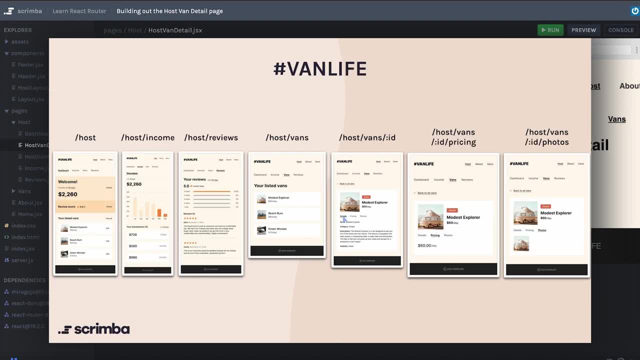 these last three pages are really all we have left to build This one. it's a little hard to see because it's so small, but this one is the detail page that we're working on in this challenge, or rather just this top portion, and that top portion is what's going to remain constant through the host van's ID. 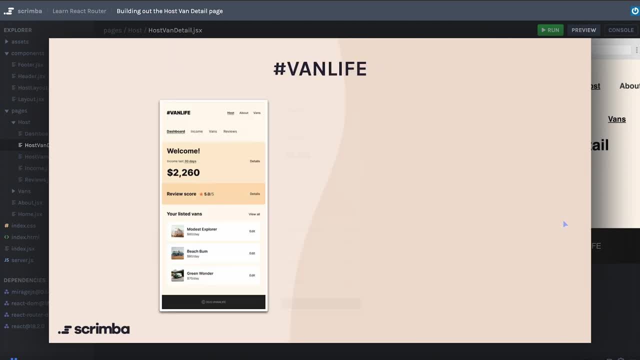 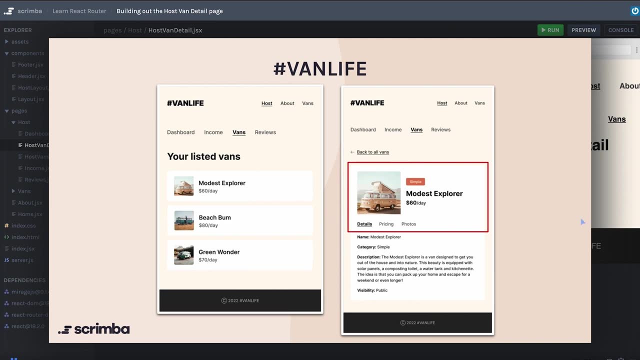 pricing and the host van's ID photos page. Let's go back here to a little bit better of a view. Hopefully it rings a bell that because this is going to be some shared user interface between those pages- the pricing and the photos page and the details page- you'll remember that we will end up using a layout route for this. 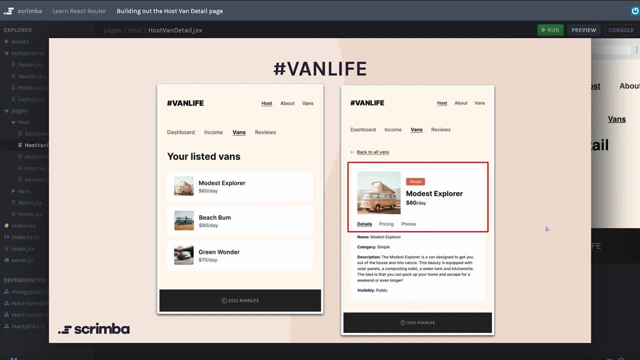 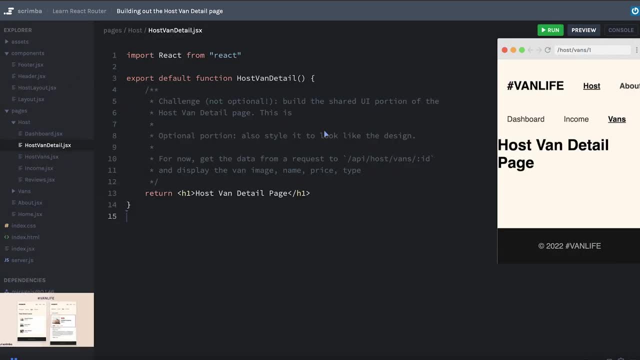 So eventually we'll have an outlet that we need to use For this challenge. don't really worry too much about that. You'll make it so that this appears when you're on the what is it host vans and then the ID of the van. So building this page out is not the optional part of this challenge, but there's a lot of things you can do to make sure that you're able to do that. So if you're able to do that, you can go ahead and start building out the page. 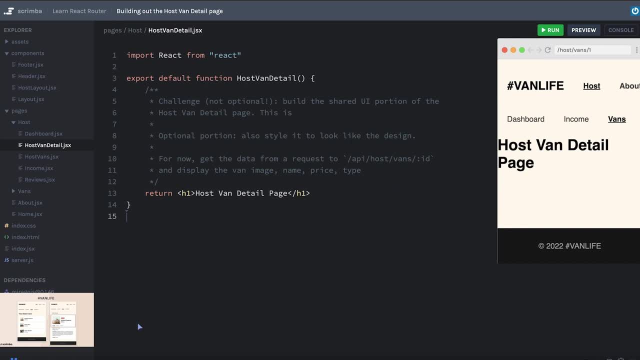 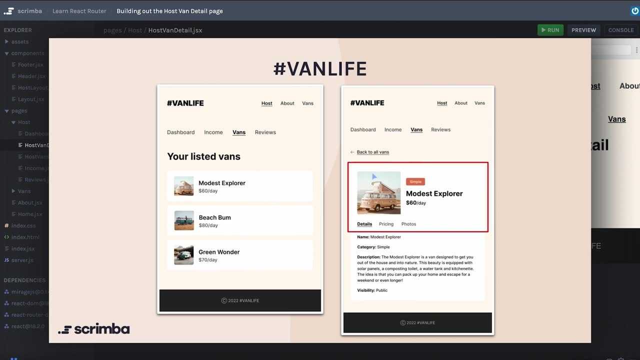 So building this page out is not the optional part of this challenge, but there is an optional portion, and that's to style it so that it looks just like this. If you don't feel like you need to practice your CSS at this time, then you can just get all of this information displaying on the page, and then I'm gonna handle the CSS part on my end. 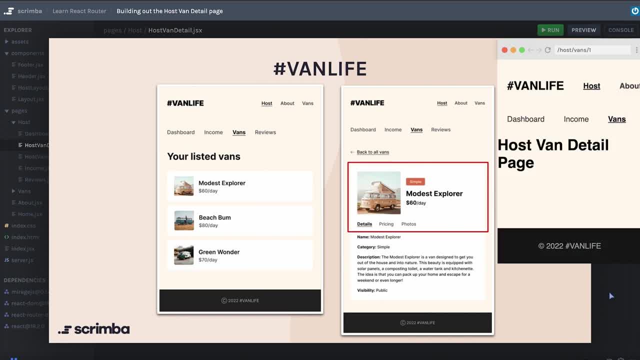 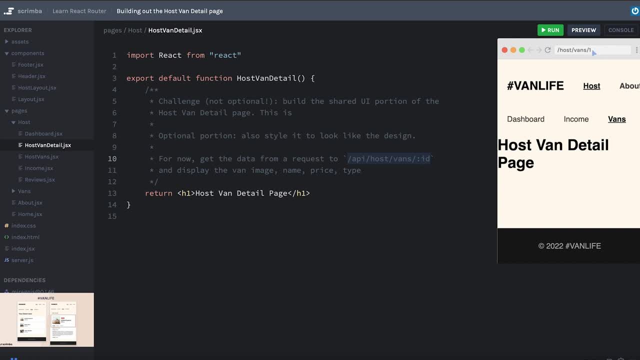 We're going to fine tune how the data gets into this page, but for now just make a request to slash API, slash, host, slash, vans, slash, and then whatever the ID is in the URL. So the ID of this van The server is hard coded just to organize it. 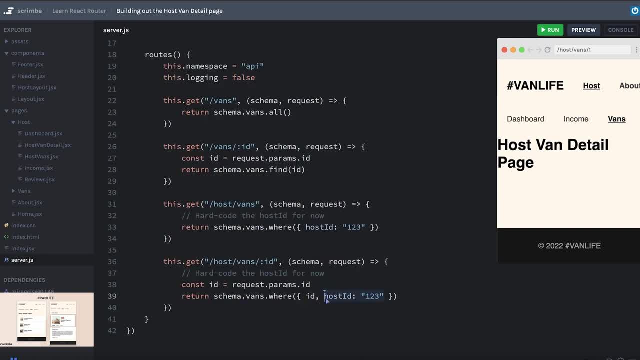 So it's all set up And then we can run this only pull when the ID is equal to the ID you pass in and the host ID is 123.. So that's really already handled for you. This is obviously not exactly how it would work in the real world. 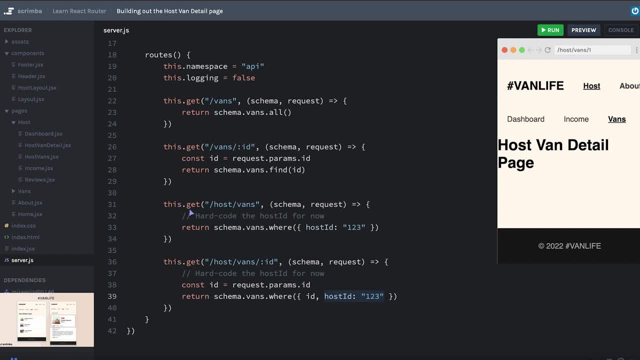 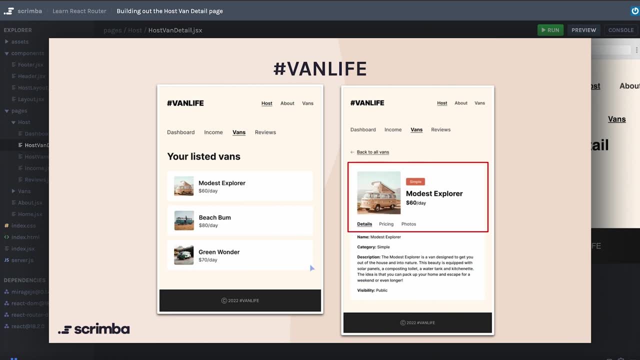 but it's close enough for our purposes in learning React Router. So again, you will just be building this top portion. Don't worry about changing the routes we have in our index or anything to set up for this bottom portion. That's what we'll be working on in the next challenge. Okay, it's. 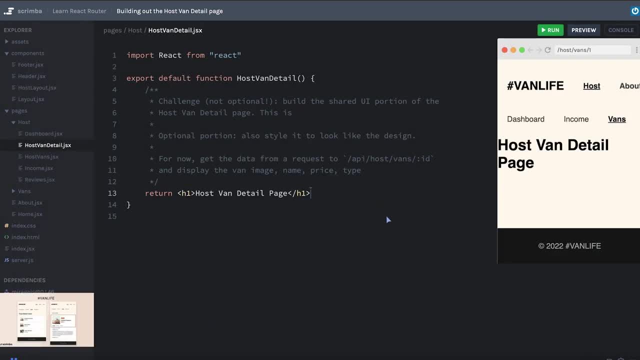 your turn to get your hands on the keyboard. Pause now and work on the challenge. Okay, let's set up some state for holding the current van. So we'll say current van and set current van is reactuseState And until that data comes in, we could initialize it as null. 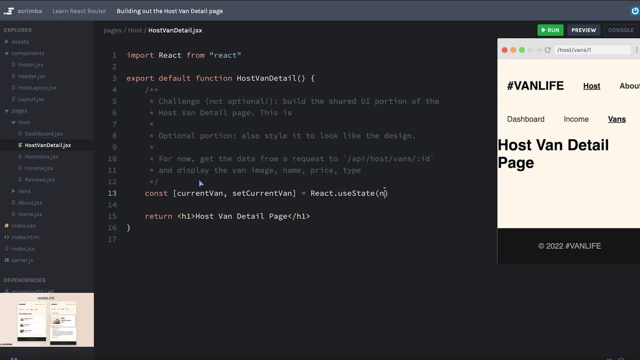 or I suppose we could initialize it as an empty object. Let's go ahead and do null for now. Then we will do a useEffect, which is where we will grab our data. We'll set up the dependency array and we'll leave it empty for now. just saying, if this component ever loads, then we want you to. 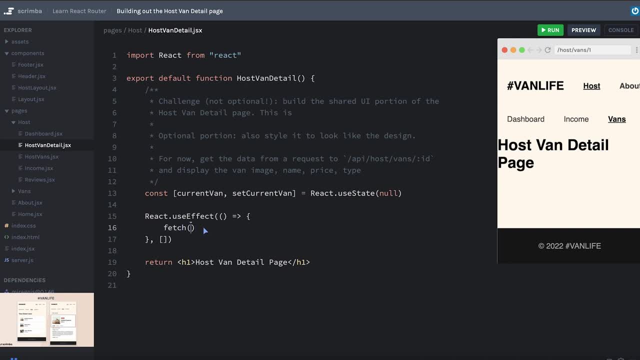 run this effect And we will send out our fetch request. So this will be to. let's see, I'm going to use a template string because I know that I need a dynamic access to the ID on the current URL. So that's going to. 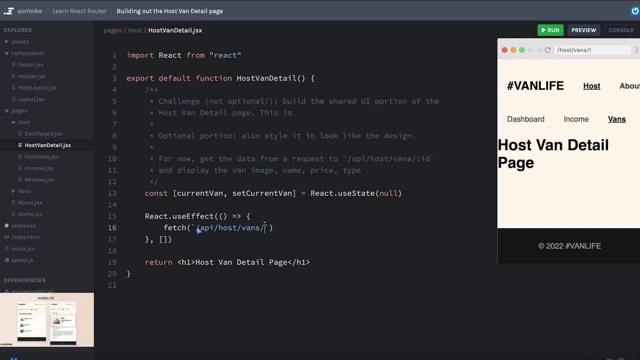 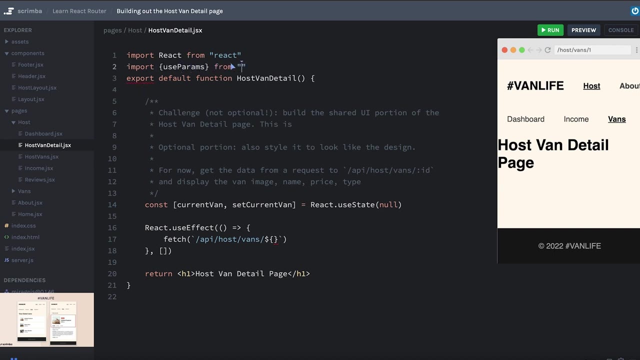 be actually. let me just copy this part right here. Okay, and then I will use a template string to inject some JavaScript. Now I need to figure out what the current URL is And if you remember way back, we can get that from the params. So I need to import use params from React Router. 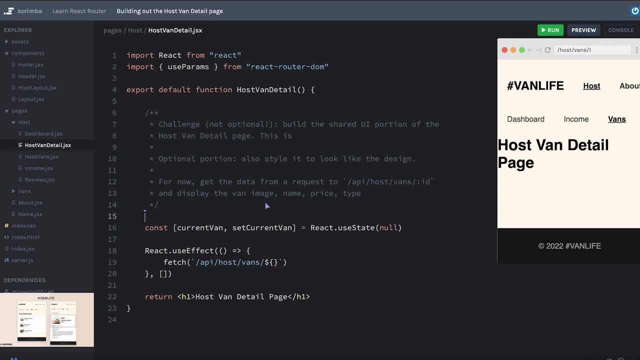 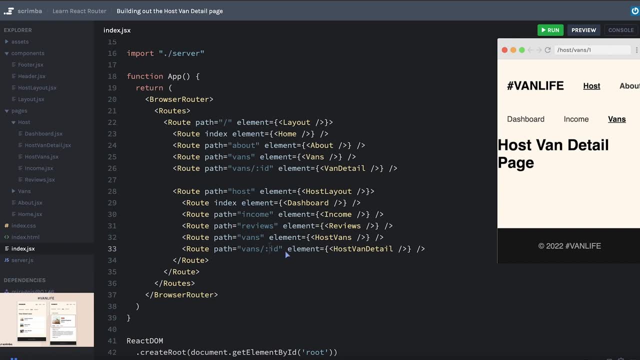 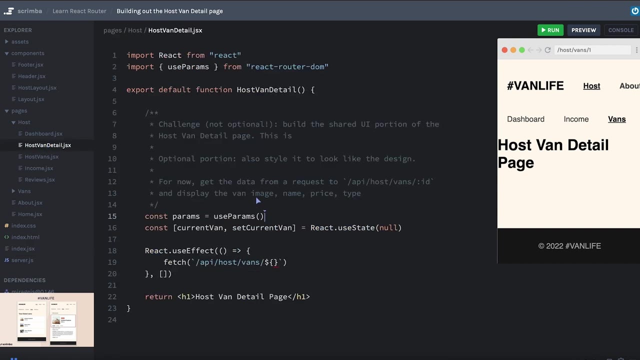 DOM And then I can grab the params by calling use params. And let's see in our indexjs I think we've called everything ID, Yep, So whatever. I guess you could call it variable name we put here. if I said this were colon, whatever, then over in our host and detail page params would have 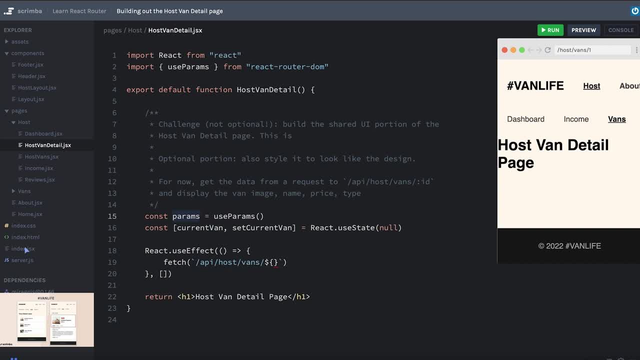 a property called whatever, So it'd be params dot whatever. that's too silly, So let's take that back And this will be params dot ID. Or if I wanted to, I could just destructure it when I pull it in, And then I can grab the params by calling: use params. And then I can grab the params by calling: 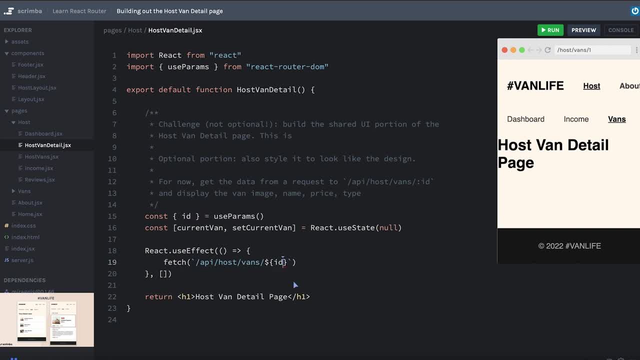 it in and say: I only care about the ID property. So then we could just say ID here, Okay, and then we will get the response and get the JSON turned into a JavaScript object And then we will have access to the data And, if you know me, I'm going to console log this data before we get too far. 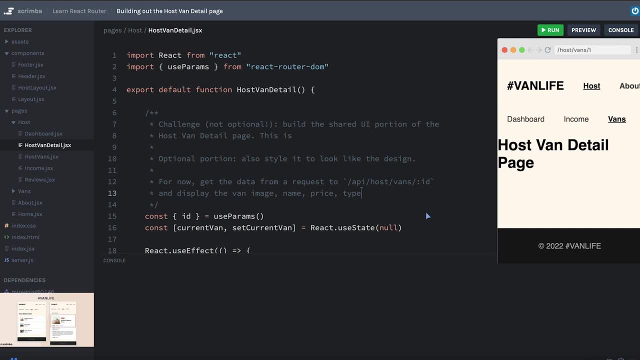 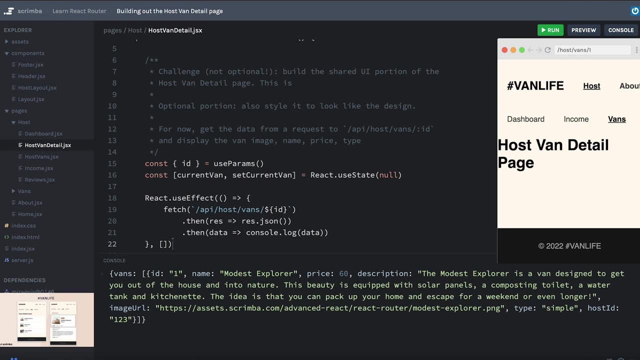 down this rabbit hole. So let's hit save- open up our console. not JSON parentheses, we need res dot JSON Cool. Okay, so we get an object with a Vans property And oh, this is interesting. I guess this is the way that the server is returning the data. the Vans property is an. 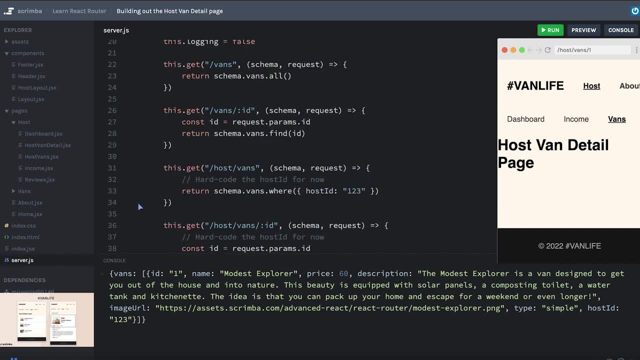 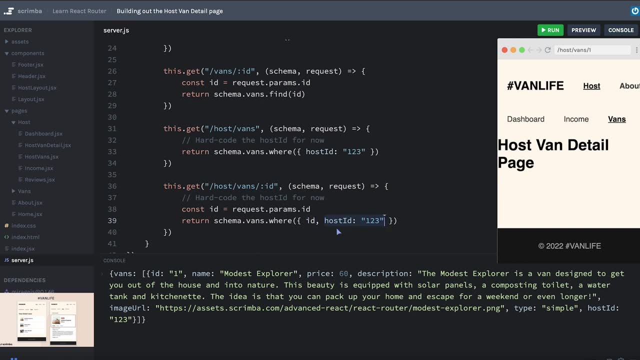 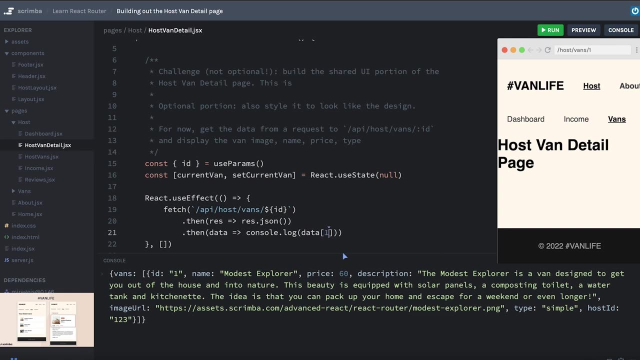 array, But because of the way that I wrote this server endpoint, it's always going to return only one item, just because the IDs are unique, and especially when you take into regard the host ID. So in that case I guess I could just always console log, let's say data, oops at no, that's. 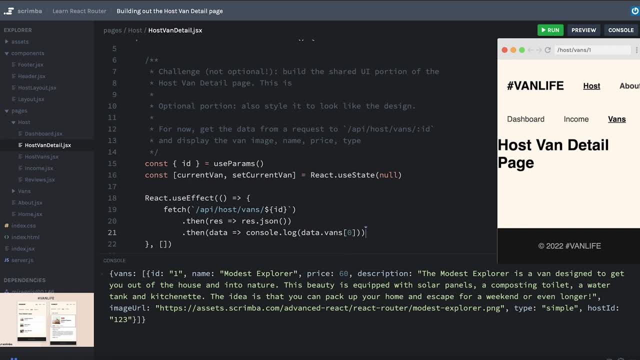 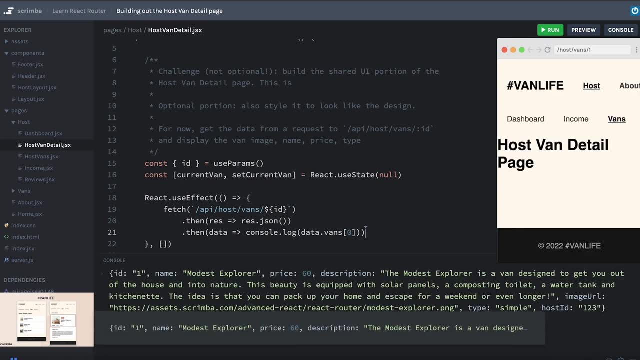 zero dot Vans at the index of zero, which would always be the first object, because I just know that it's always going to be one object. Let's just see what that looks like. Okay, so that is the van that we care about, And hopefully you were able to figure that part out, because I am the 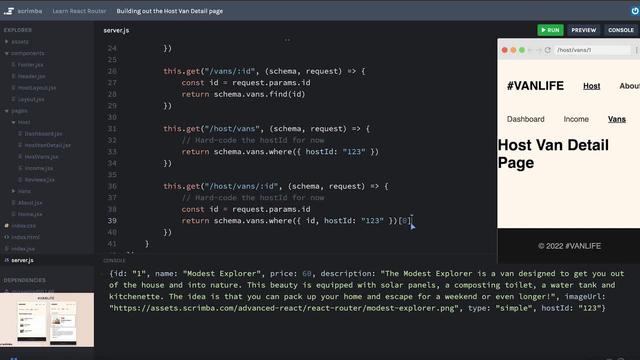 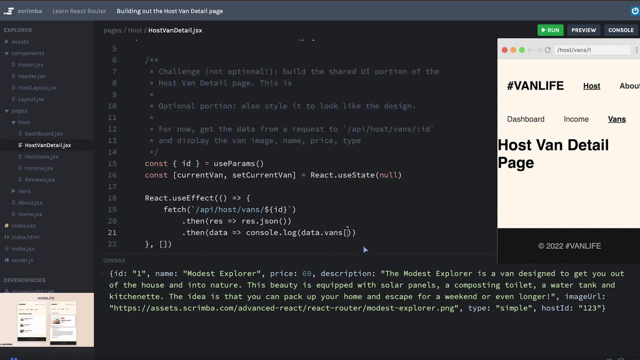 creator of the server And I'm just going to cheat. So I'm just going to put my index of zero on the server Because, to be frank, I probably should have done that in the first place. So let's take off the index of zero here, because now data dot Vans, oops, nope, that's gonna be see, it's gonna. 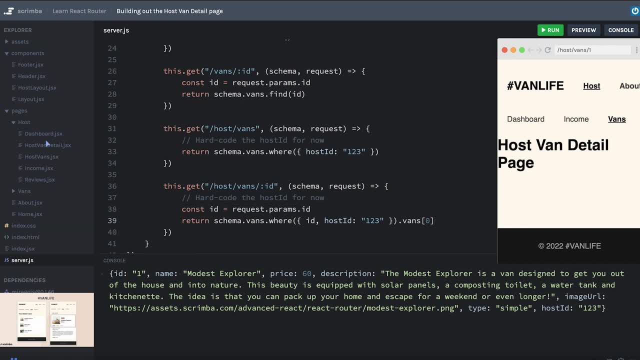 be that dot Vans at the index of zero. Okay, let's see if this even works. This might not even work. Data Nope, that's not gonna work. Okay, bear with me. here I'm actually going to change this. 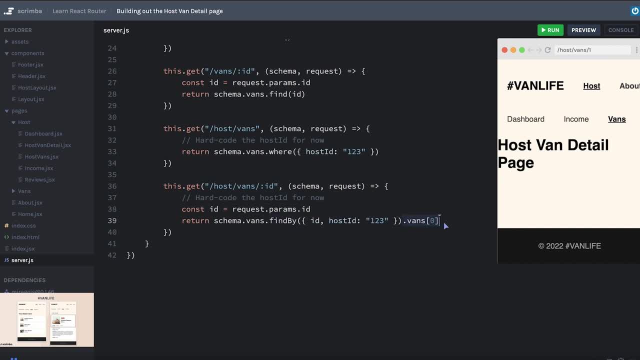 from dot where to something called find by, and then we'll take this out. The find by method allows me to pass in an object with a bunch of key value pairs that it will find and return the first instance in our quote unquote database that matches these parameters. So let's go back to host. 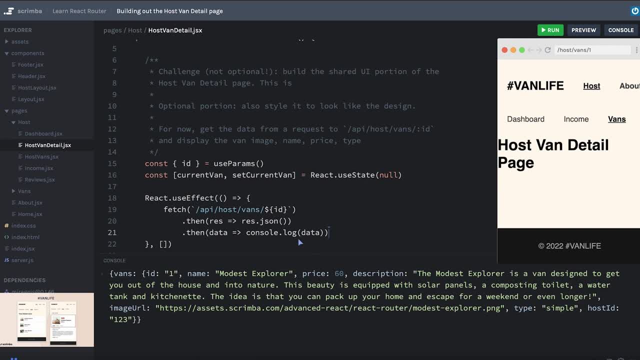 van detail. And now let's see what comes in. Okay, cool, That's pretty much what we wanted. It's pretty simple. So we'll just say: dot Vans, Cool, Okay again, because I hadn't made that change. 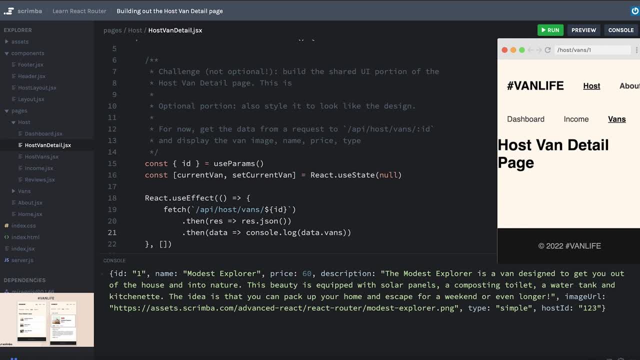 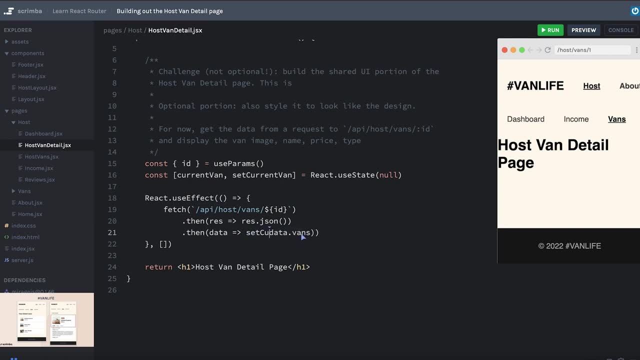 before you did the challenge. This is, I guess, outside of the purview of what we did for the challenge. This makes a little more sense to me, though. Okay, well, we don't want to console log data dot Vans. we want to set the current van to data dot Vans And then, in our markup, the 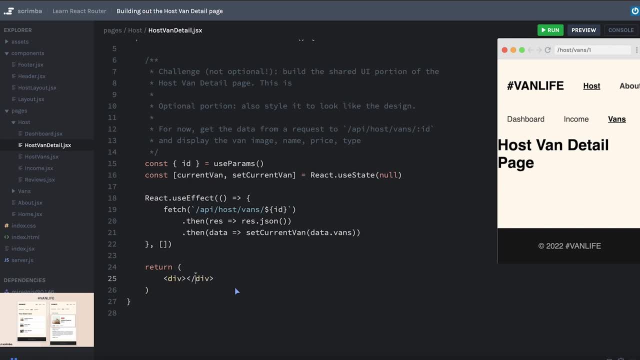 challenge just says that we need to display all the data. So let's just stuff it into a div for now, And then I'm just going to paste in the CSS and the markup that I used, And then I'm going to create this myself to speed up our process here. So let's get an image. we'll set the source equal. 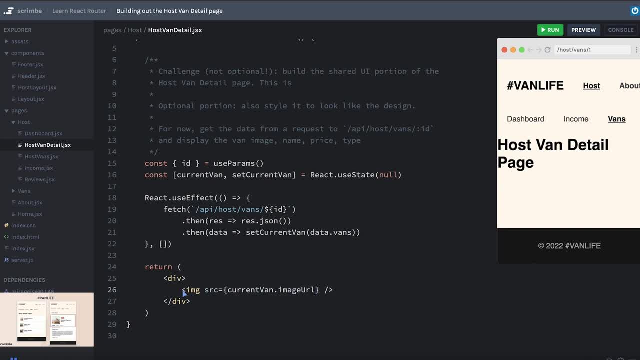 to current van dot image URL, And I can already see that there's going to be a problem here, because we're initializing our current van state as null And so null dot image URL or trying to access the image URL property on null is going to throw an error. So again hit save And we'll see. 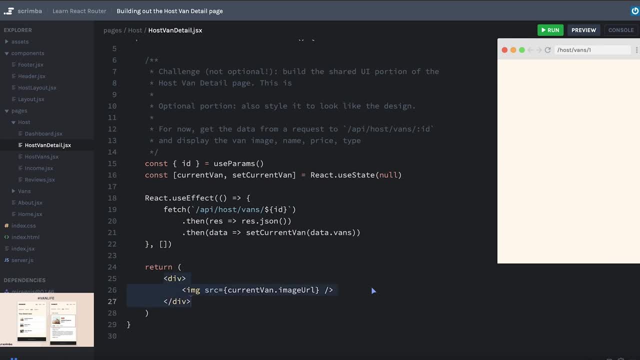 I cannot read properties of null. A quick kind of bandaid for this would be to conditionally render everything, or maybe even better is just to say if there isn't a current van, then we'll early return and we'll say return h1, that just says loading. Like I mentioned before, we probably 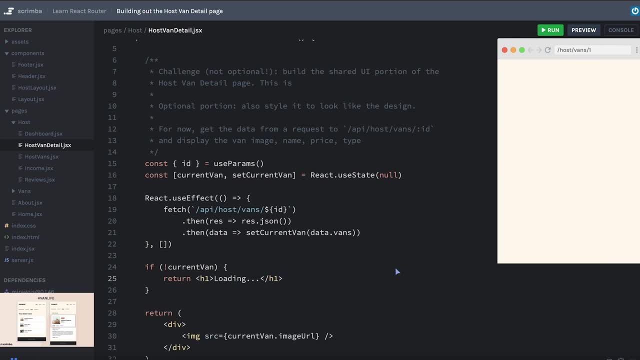 would want a real loading state to include here, instead of just assuming that if there isn't a current van it's because it's loading and not because there's some kind of network error or some other problem. But we're taking a few happy path shortcuts here, So this will work for now. 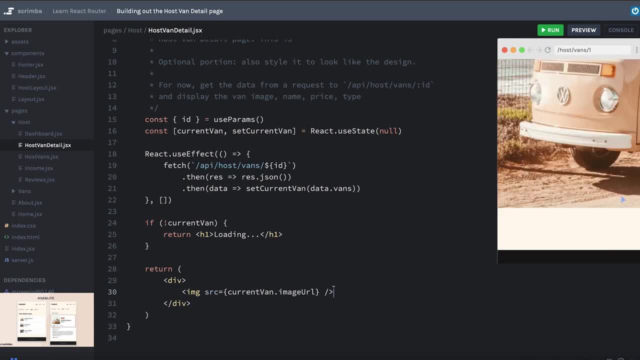 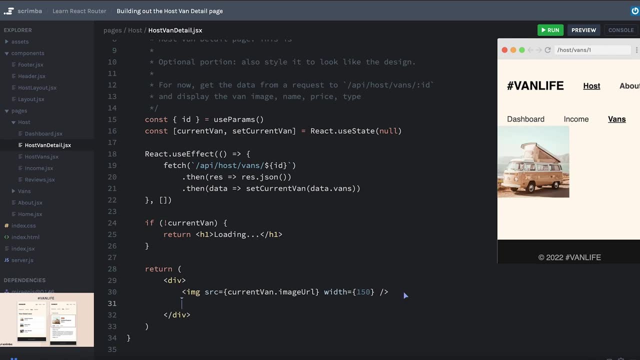 Okay, let's try this again loading and then we get this massive image. Okay, we're going to fix that. In fact, I'll just throw a bandaid on it and say that the width is equal to I don't know 150.. Okay, let's see what else it said. display the van image. 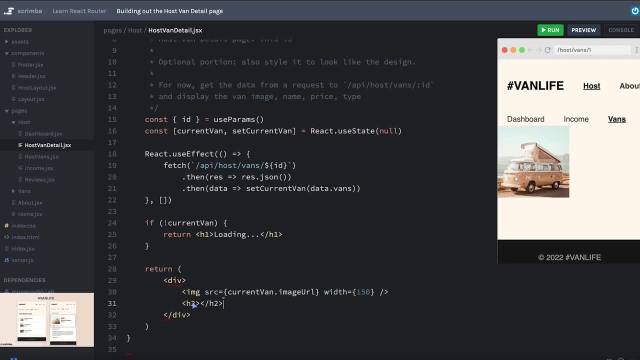 name, price and type. So we should be able to just kind of throw those in. we'll say: current van dot Z, Is it name? Yeah, there, it is Okay name. And let's just stuff these into a paragraph for now. 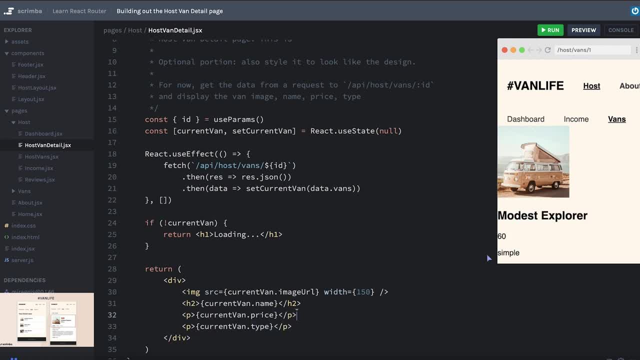 Current van dot price And we'll say current van dot type. Okay, it's obviously not the form factor that we want, But that is a great start for us. If you weren't able to get to this point, then I would recommend pausing and going back, reviewing what we've done here, Honestly everything we've. 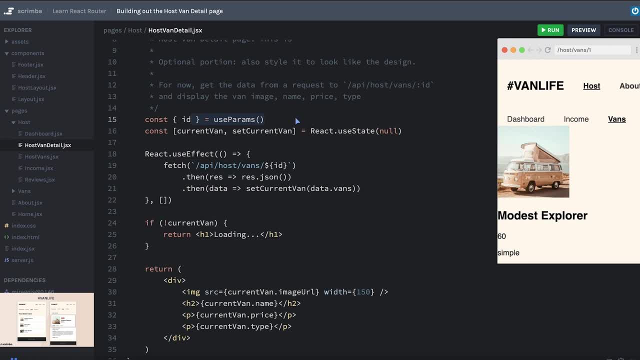 done so far, except for the use params, should not really be too new to you. in React, This might be a good time to mention that there's kind of a shift away from using use effects to do your fetches these days. There's other methods that we're actually going to cover a little bit later in. 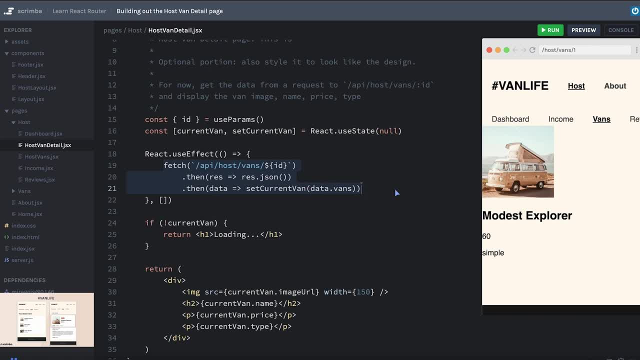 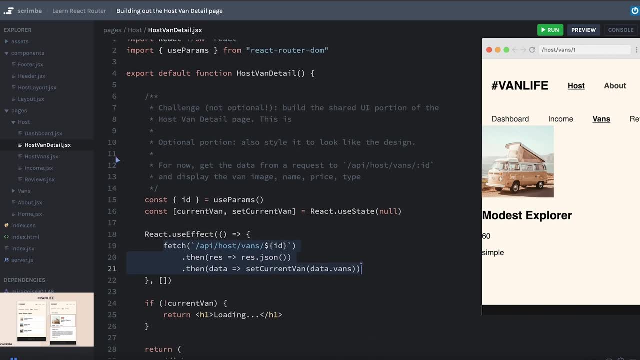 this course and some new, really cool React APIs that are coming out in the near future That will make this a lot easier to write and to reason about. And you know what? because this has actually been a bit of a challenge already. it's taken a fair amount of time, I think this last 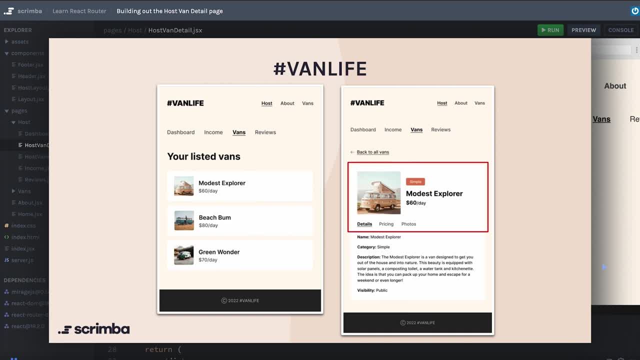 portion. what we'll do right here is actually going to be something we work on in the next challenge. If you were able to do this little navigation bar, then that's perfect. That's really really good. We're going to do that in the next challenge If, again, you already did it. 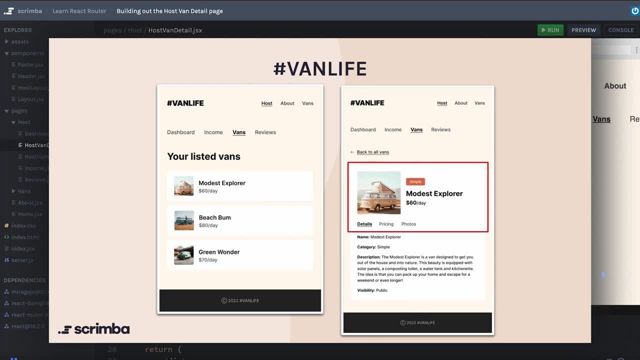 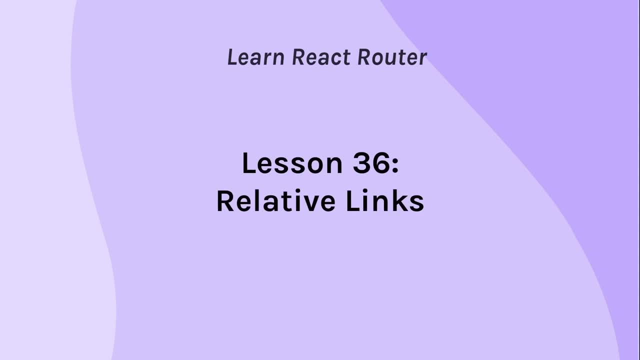 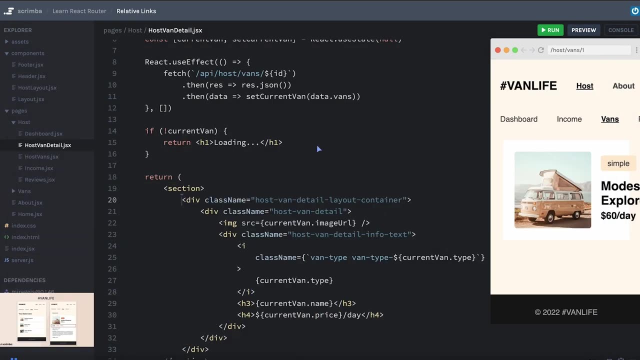 then you can skip doing that challenge And you can just watch me do it over there in that lesson. Okay, great work. Hopefully that went okay And if not, you know what to do. Let's move on. Okay, I lied. Before we get to doing this nested navigation bar, we need to spend a minute to talk. 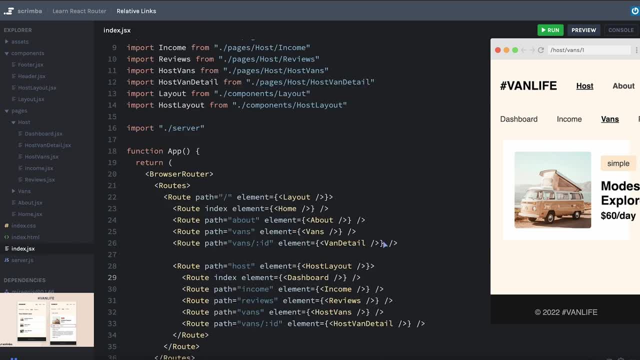 about relative links. We've covered relative route paths. For example, here we have our main route, which is the path of slash, which enables us to put all of its nested routes as just about, instead of specifying slash about because its parent is slash, the slash is sort of assumed A more. 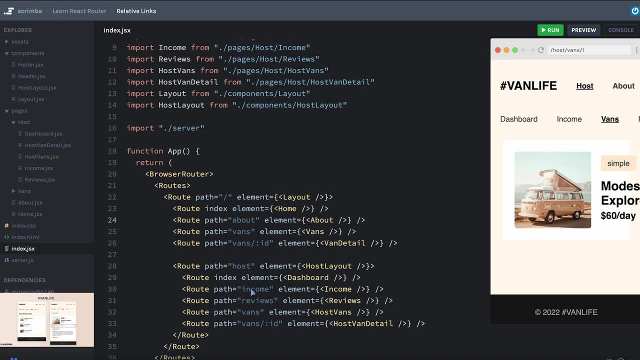 obvious way to do this is to put all of its nested routes as just about, instead of specifying slash. about This version of this is when we come down to the host ones, where we have the path just as income. but this is not slash income. it's slash host, slash income. These are relative paths. 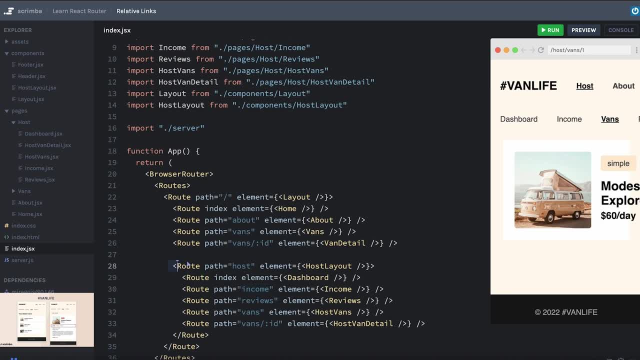 because this is a nested route inside of its parent route, it assumes a known path leading to all of the parents above it. Or rather, it's assumed that when we say income here, it's referring to the absolute path of slash host, slash income Down. here we had to specify. 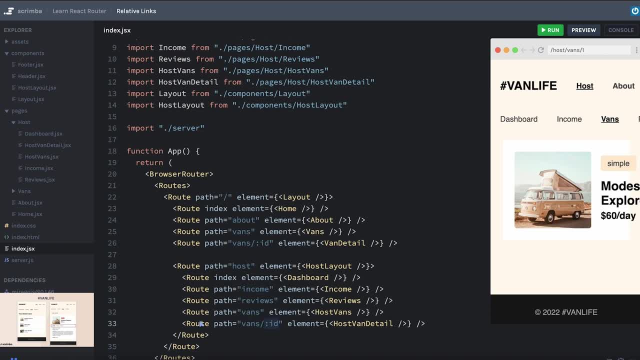 vans and not just colon ID, because we did not nest this route as a child of this route And therefore we need to be a little bit more explicit in the path leading up to it. However, it's still relative because the URL is not slash vans slash ID, it's slash host, slash vans slash ID, So that 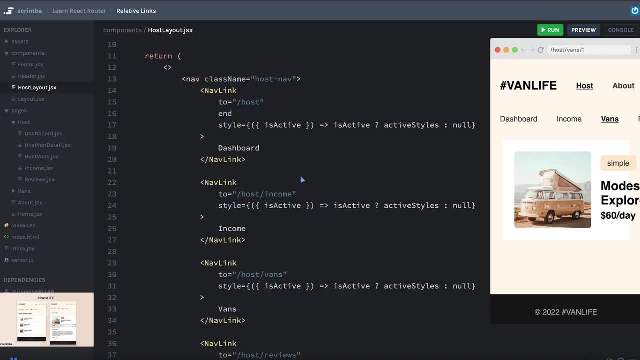 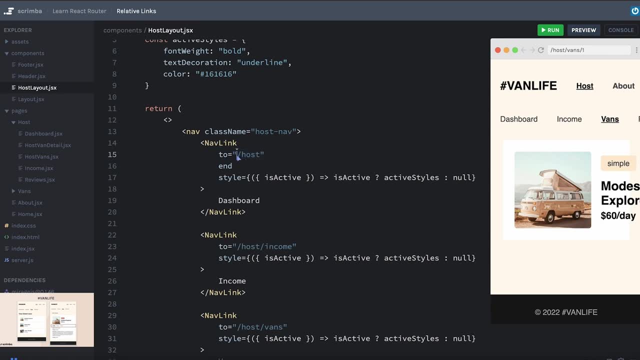 brings me to what I actually wanted to talk about, And that's over in our host layout. When we created these nav links, we created them as absolute paths. we said that this path, this nav link, goes to slash host, slash host, slash income, slash host, slash vans, and so forth. However, the truth, 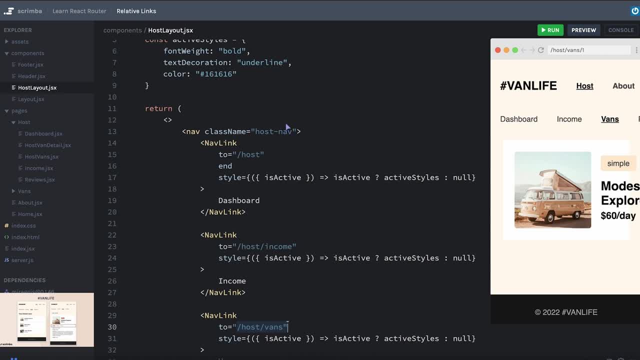 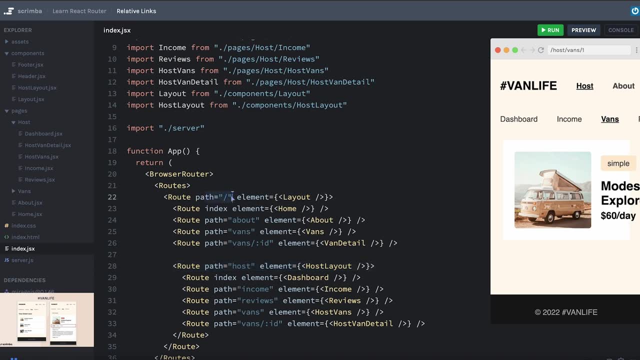 is we actually don't need to do this, And that's because this host layout is getting rendered right here in this route, And this route is already a child of the slash route. Because our element is part of the route for path of host, the element can assume the path of host in all of its links. 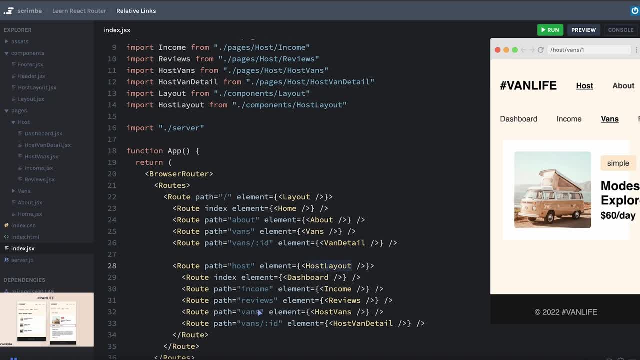 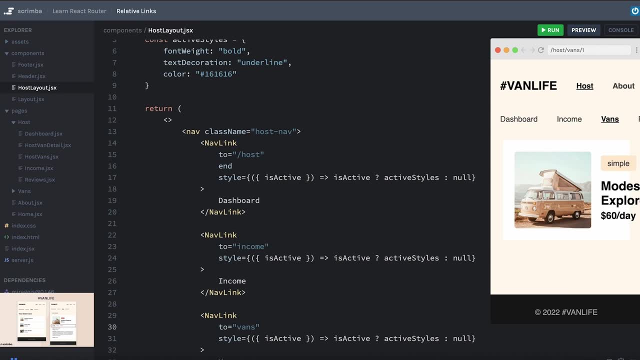 So if I come back to my host layout element- this one that's being rendered on the slash host route, and I'm going to go back to my host layout element, and I'm going to go back to my host layout- I can change these to just say income bands and reviews. I'm going to talk about this. 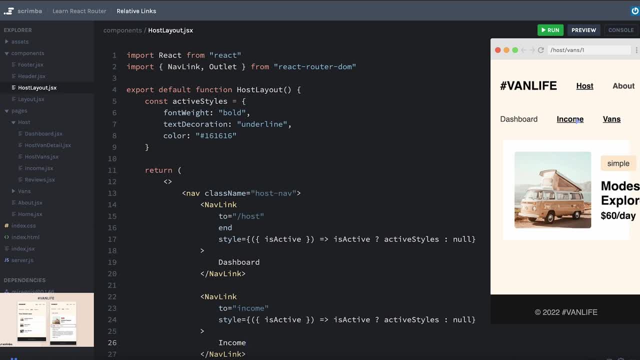 top one in just a second. But let's go ahead and hit save, And I can see that this is going to take me to. well, this is the one that we didn't change, because that's our dashboard. Let's go to income. 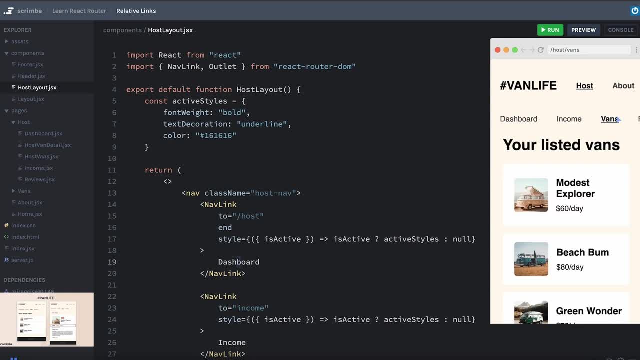 Okay, the link is still working. slash host- slash income. slash host, slash vans. slash host- slash reviews. And, once again, the reason that's working is because this host layout is rendered or nested inside of the slash host path. So if I go back to my host layout- and I'm going to go back to my host- 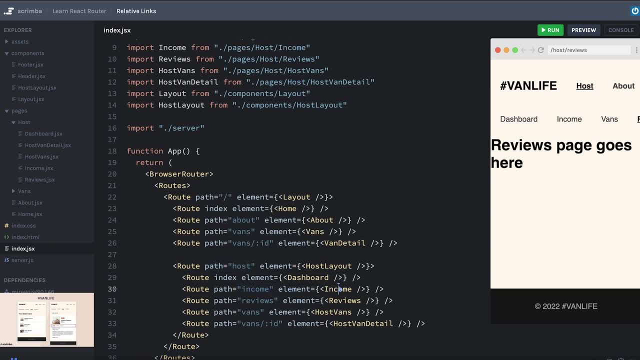 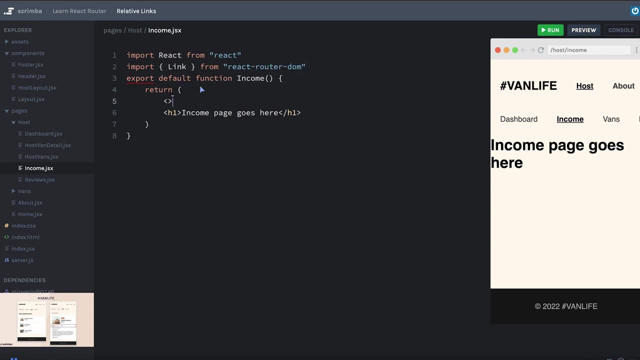 path. this means that if we have links inside of the income component here we don't need to specify the whole path leading up to income slash host, slash income. In fact, let's see that, just for the sake of learning, I'm going to import a link from react router DOM And let's say that we 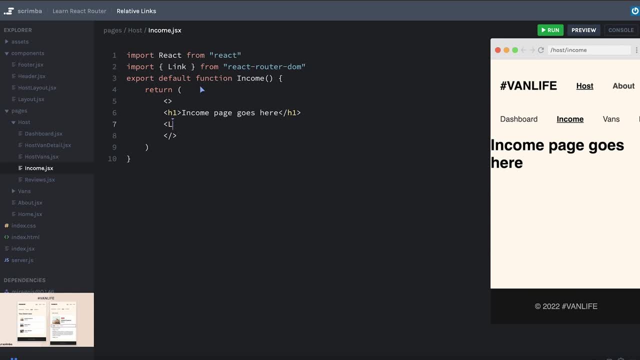 are rendering both an h1 and a link. Let's see what happens if we put: I don't know just something here, Let's hit save. we have our click me. I want you to think for a second: where is this route actually going to take me to? in the URL Again, if we look at the route hierarchy, we have this: 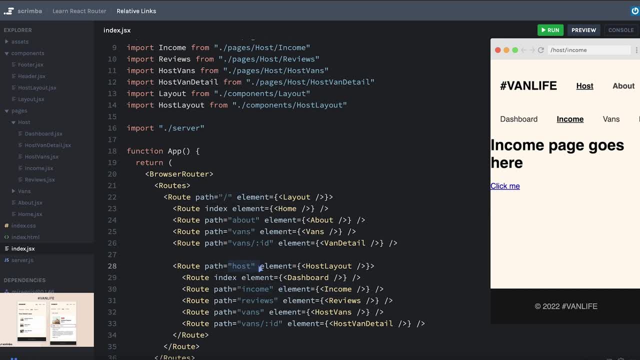 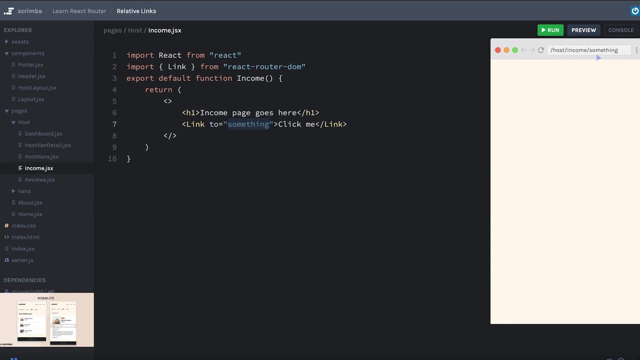 income is nested inside of slash, also inside of host, and it's already rendering on the income sub route. So slash host, slash income. So if I just say that the link is going to take me to this string of something, it's going to take me to slash host, slash income, slash something. So 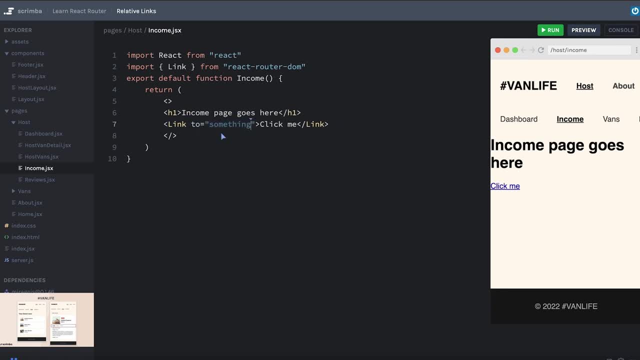 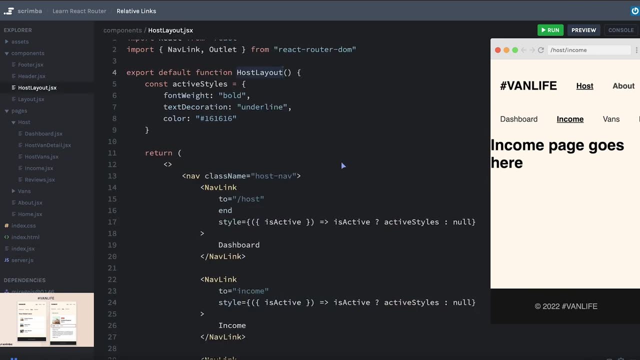 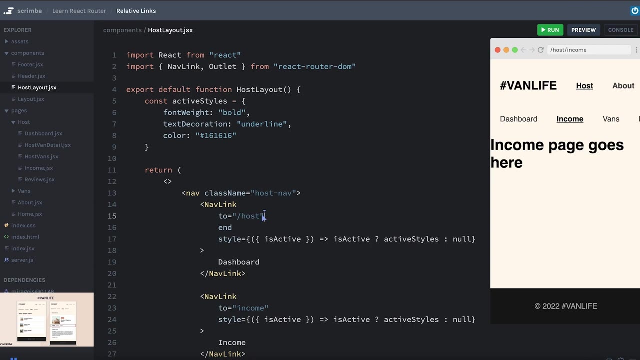 that's the idea behind relative routes. Let's get rid of these changes, Okay, and we'll come back to our host layout file. So this is why all of these relative paths are working. Something that's pretty pertinent to what we're about to work on is how to handle this nav link here that takes us to: 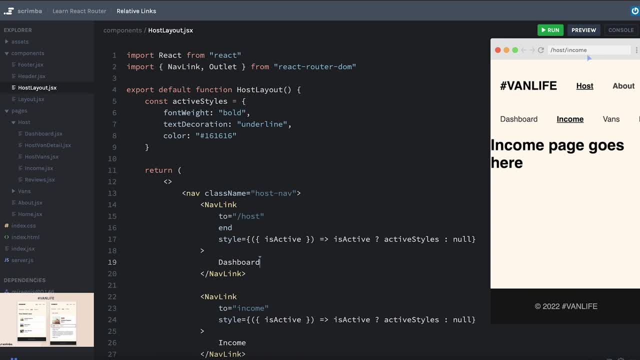 the dashboard, because our route is not slash host. slash dashboard, it's just slash host, whereas these other ones- the routes- are actually nested as one layer deeper in the URL. we need to do something different. Well, I guess we don't need to. I could just leave this as slash host. 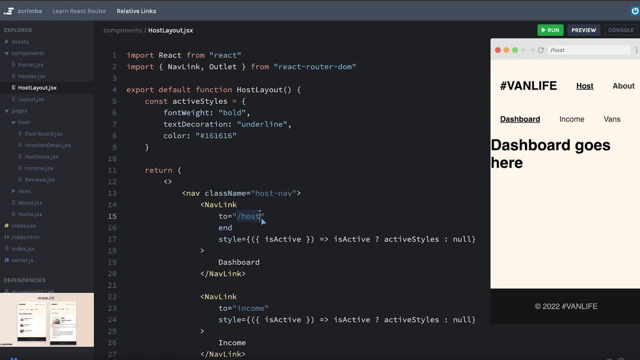 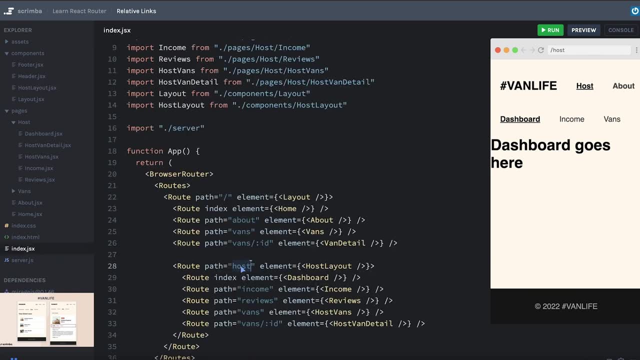 but one of the benefits of using relative routes and relative links is if, for whatever reason, I decided I wanted to change what this was called maybe I don't want it to say host, I want it to say admin. let me navigate to, maybe the about page and then hit save. I'll click on host. Well, 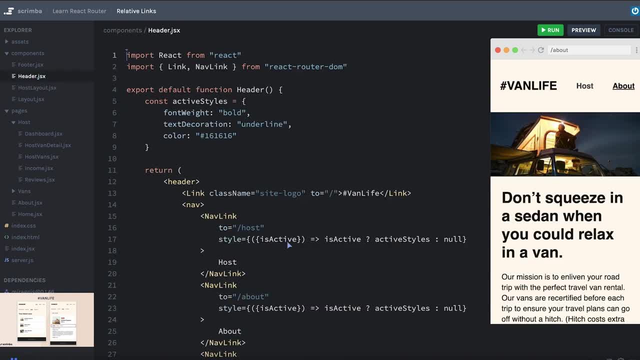 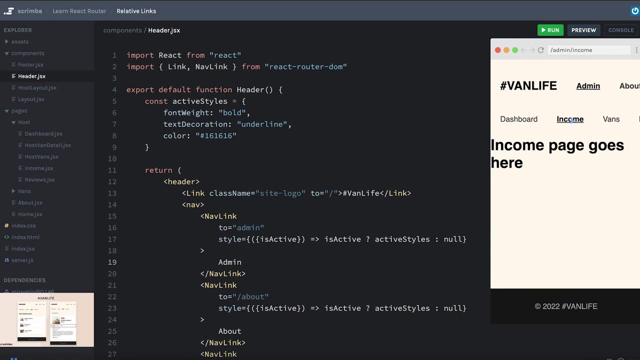 actually that one. we didn't fix me, fix that in the header. this one is: Oh, these are also using absolute paths. So let's say this is going to admin and this will say admin. Okay, so I click income. my link isn't broken because it's a relative path. I only had to make a couple small. 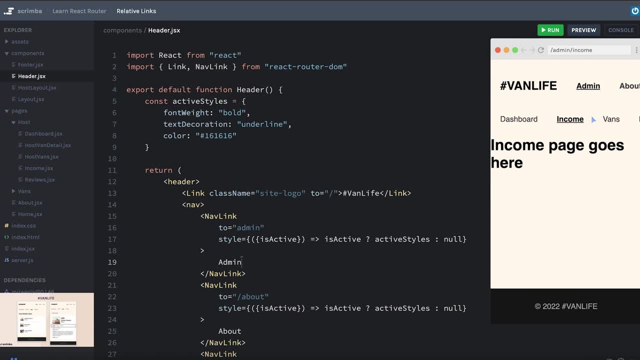 changes. I didn't have to make a change on every link that leads to slash admin. slash something else. However, my dashboard is still broken because it's linked to an absolute path of slash host. So let's undo these changes, because I don't want to name it slash admin And we'll come back. 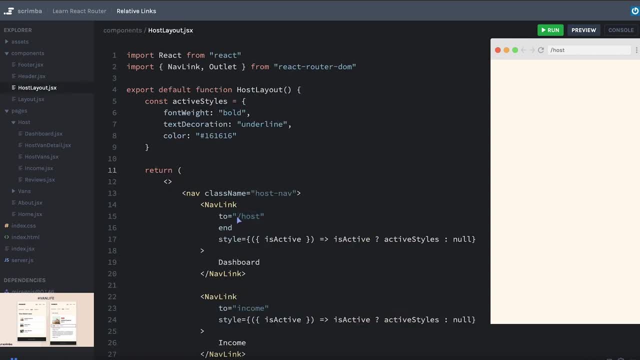 to our host layout. These nav links are all fine, So what exactly should we put here when, basically, what we want to say is: I want to link to this route, the route you're currently on, just slash host. Well, if you've had a chance to, 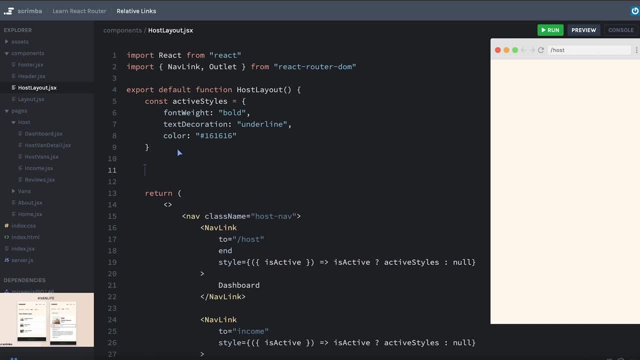 practice using your terminal on your computer. if you want to reference the prior directory, you can use something like dot dot. it's a shorthand for the parent directory of the directory you're currently in using your terminal. For example, if I wanted to change directory to 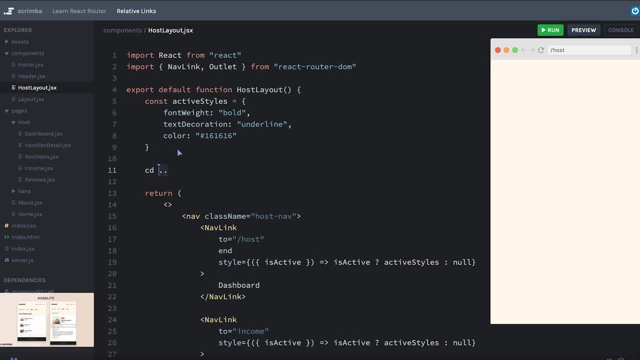 the previous directory. I would say cd space and then dot, dot, which represents the parent directory. Well, in a Unix terminal you also can say cd space dot, And that represents the current directory. cd space dot does absolutely nothing, it changes. 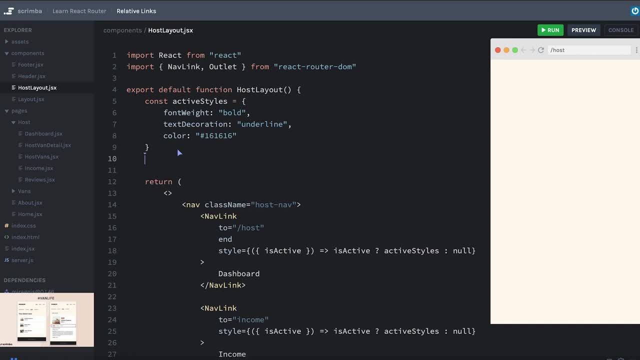 directory into your current directory. But that little history can hopefully help you understand what I'm about to teach, which is, if we just want to link to the route that we're currently inside of, I can just say dot. this isn't by mistake or really has anything to do with the directory. 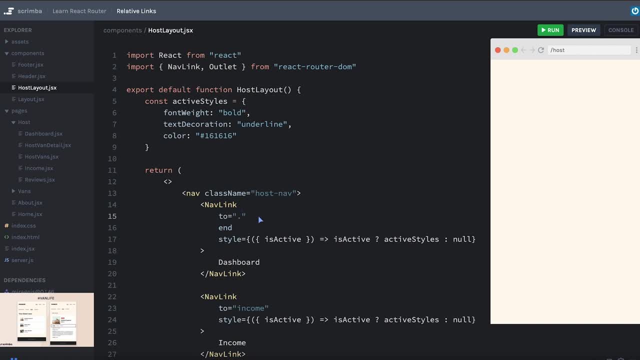 hierarchy. It's just something that React Router has implemented into the React Router package And, as a sneak peek, very soon we're going to see when we might want to use dot dot, But that's for the next lesson. So for now we're going to say: I want the dashboard to link me to the current. 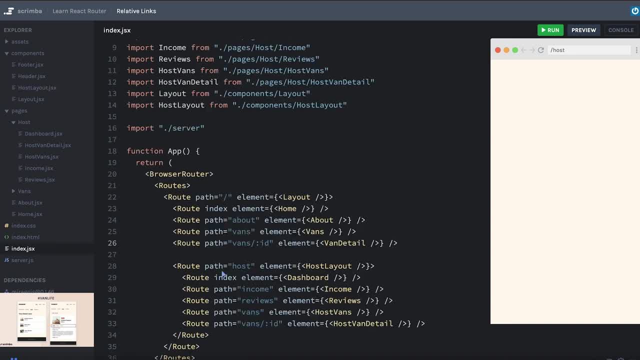 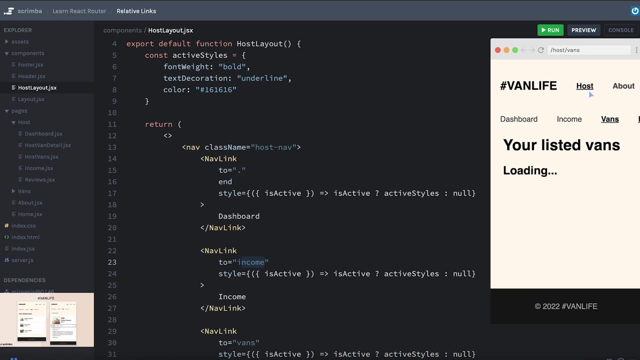 route where the host layout is being rendered. And again, the host layout is being rendered on the path of slash host. So let's go ahead and hit refresh. I can hit income. that takes me to host income. let me come back out here to the host layout. So income is a relative path, vans is a 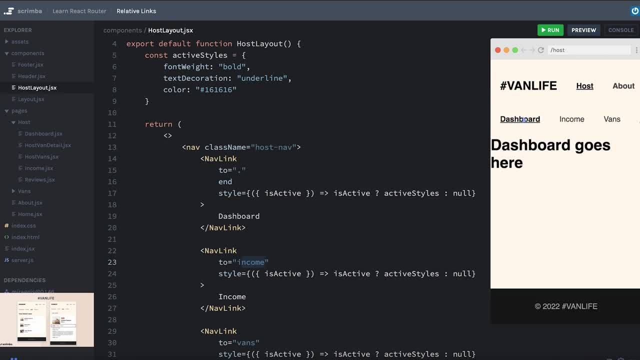 relative path, reviews as a relative path And now dashboard is a relative path to slash host. if I were to go back and change host to say admin, I would really just have to change it here in this top navigation And in the path. 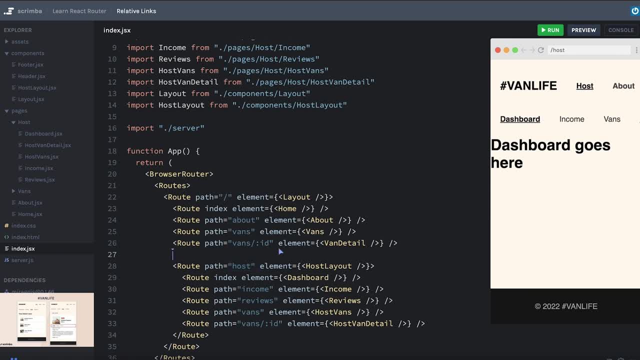 right here. Other than that, all of my relative links would still be working. Hopefully you can see that there's a benefit in doing that, And I've spent a lot longer talking about this than I originally planned, But hopefully that gives us a quick primer into the next thing we're going to. 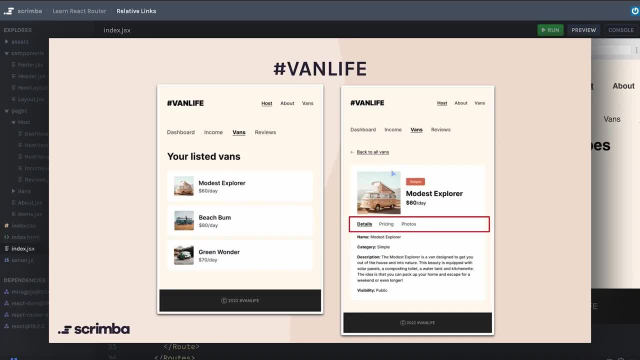 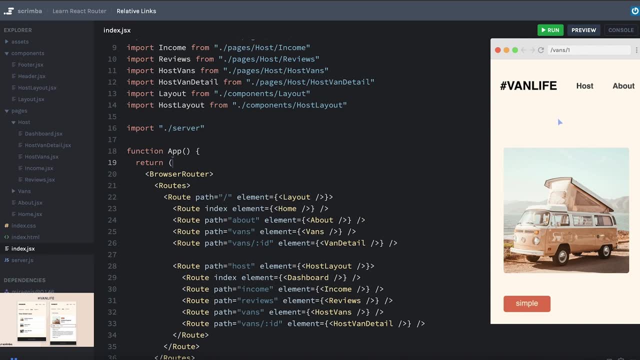 work on which I know I said would be this navigation bar, But it's actually going to be this: back to all vans button. I purposefully didn't teach this when we were doing these vans list here, because there's a little bit more we need to learn, But when it comes to this, 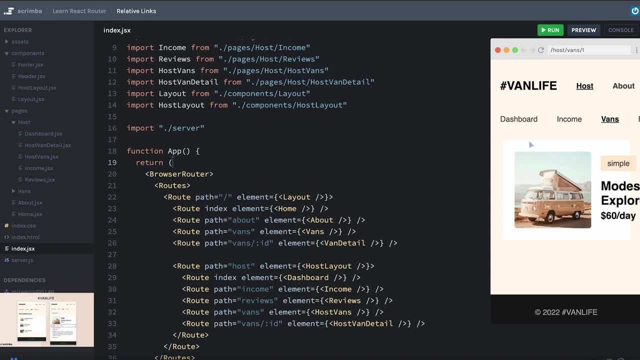 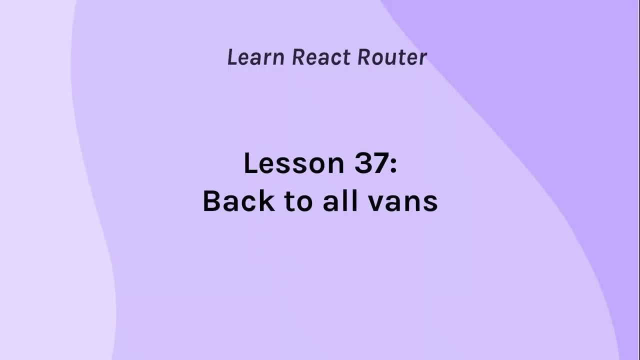 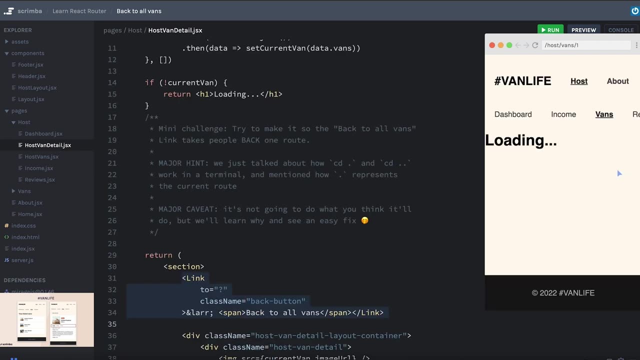 vans right here. adding a little back to all vans button is something we now are capable of doing, So buckle up. that's where we're going next. Okay, I even did some heavy lifting here and added this link for you, And of course, you can tell that I added all the styling to our van list detail page. 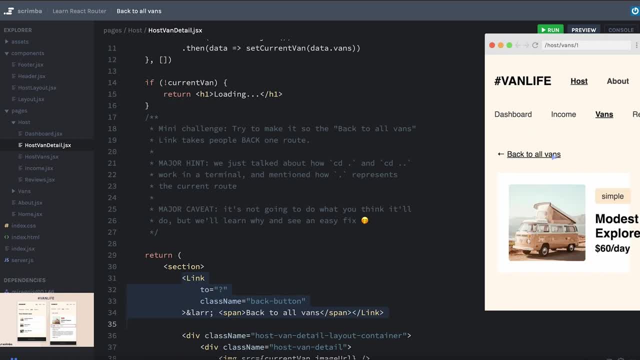 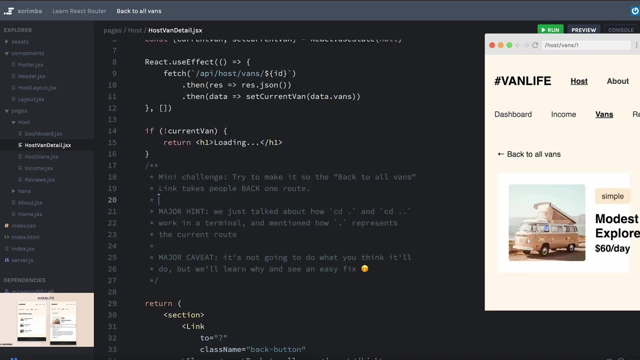 at least the beginnings of it. So we have this back to all fans link And this is supposed to take us back to this page: slash host, slash fans. So let me click on this. we have a quick review of this And we're going to do a quick mini challenge for you. I want you to change the two so that it goes. 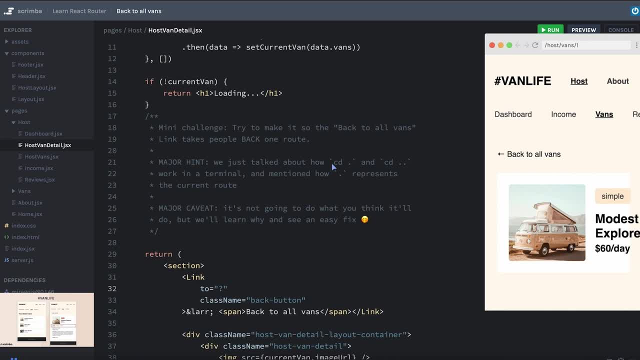 back to all vans. A major hint is how we just talked about the difference between saying cd space dot and cd space dot dot in Unix terminal or in a terminal, And we mentioned how dot represents the current route when we're talking about react router, relative links. But before you get started, a major 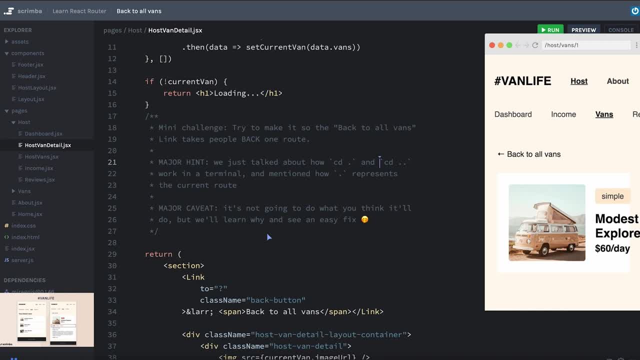 caveat on this is that it's probably not going to do what you think it'll do, But I do want you to give it a shot. See if you can figure out what I want you to put here, And if you don't, you can. 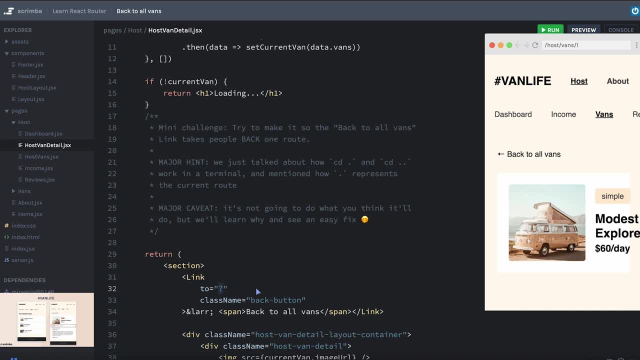 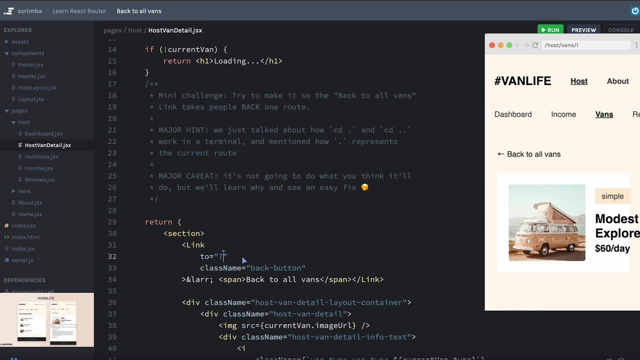 put it in the chat And then we're going to learn one little extra tweak so that it will fix the problem that you're about to see. Okay, pause now and work on this mini challenge. Hopefully your thought was to say: Well, if I don't want the current route. in fact, let's see what happens. 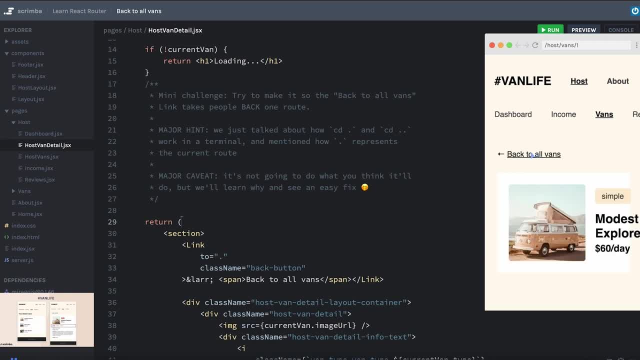 I'll hit save, I'll click back to all vans And well, nothing changes. And that's because dot means the current route, which is slash host, slash fan, slash one. So theoretically I should be able to say, Well, let's go back a route, dot, dot, I'll hit save And what happens is well. 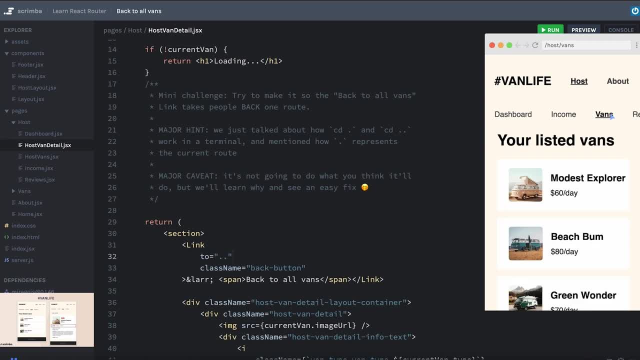 it takes us too far back. we go to slash host. we wanted to be at slash host, slash fans, this page here, So why did it do that? Well, something that I mentioned but didn't really dive deep into is the fact that when we're using relative links, what it's relative to is the route hierarchy here. 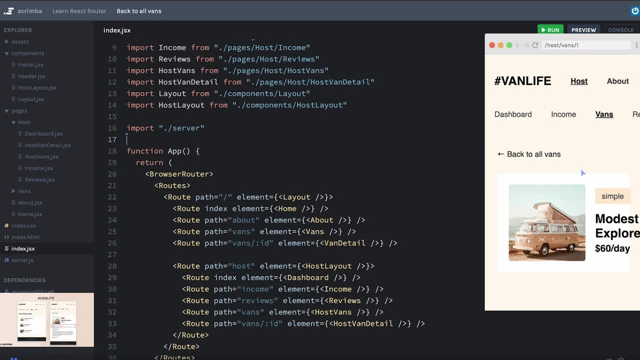 it's not necessarily relative to the path that we currently see in the URL. Why does that matter? Well, when we're here in this route, slash fan slash ID or, in this case, slash fan slash one, sorry, slash host, slash van slash one, to be more specific, When I use the dot dot, relative path. 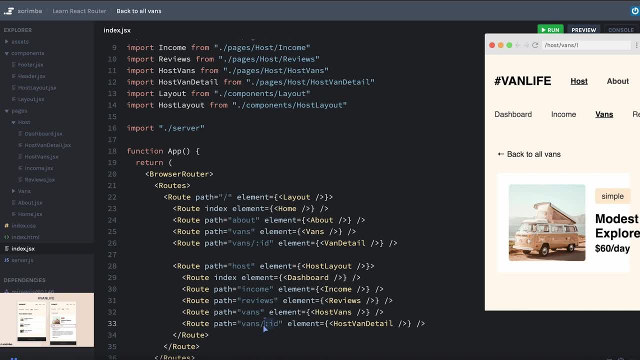 the default in react router is not to go back exactly one route, which would be slash vans, but it's to go up one level into the parent route, And our parent route is host or slash host, which is why currently clicking back to all vans takes us to slash host. Remember, we realized that 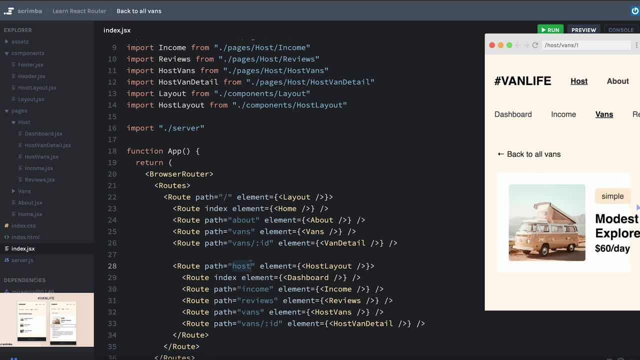 the vans list page and the vans detail page here didn't share any user interface, And so we chose not to have a nested route for vans like we might have otherwise. In fact, just for fun, I'm going to show you what it might look like And we'll see how. it's a little bit ridiculous if we 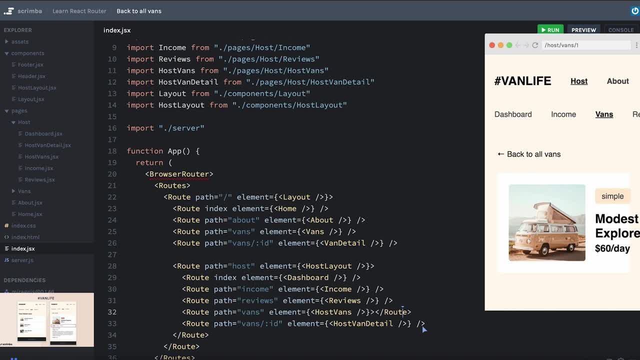 were to nest this route. So I'll create a closing element rather for the route. we'll stick our vans colon ID in there And now, because we want this host vans to show up and the index of slash vans, we'll have to create another route. that's going to be actually know what when we put some space around. 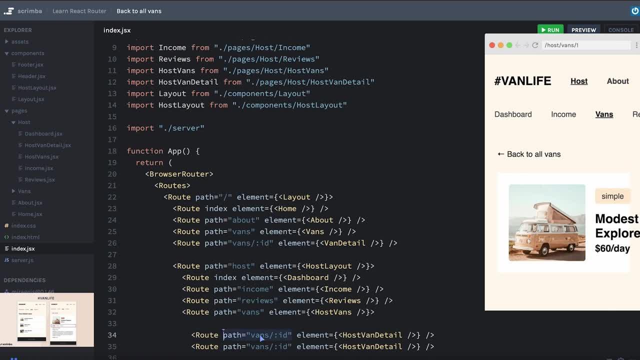 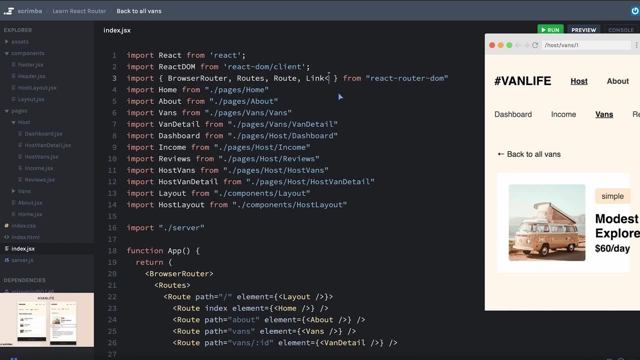 just so we can see it a little easier. This one is going to be the index, In other words, the host vans is what we want to show up in the outlet of the parent route here. Well, we don't have an outlet in host fans, So we would need to just render an outlet. Let's bring in outlet from. 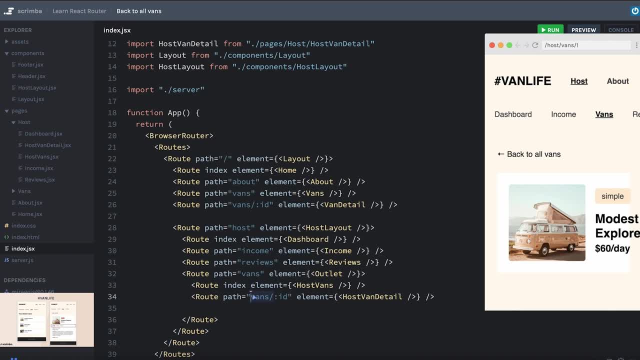 react router DOM. Now, because I'm nested, I don't need to specify vans slash colon ID. In fact, it would be wrong to specify van slash colon ID because that would mean slash host, slash vans, slash vans slash ID. So let's get rid of the van slash part. Okay, that was a bit of work And we. 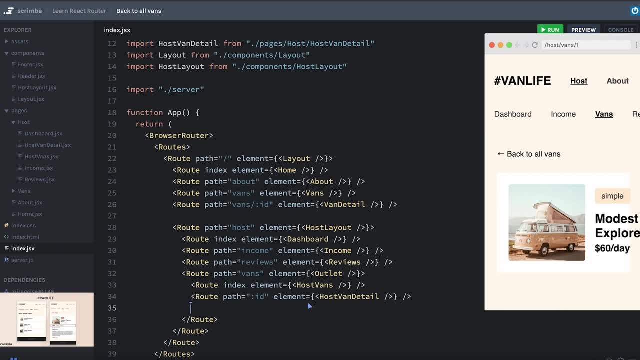 have this kind of ridiculous just rendering an outlet in the parent here. But let's hit save. everything seems to be working. And now that the parent of my slash ID route is slash vans, the dot dot should work. Let's cross our fingers, we'll hit back to all vans And sure enough. 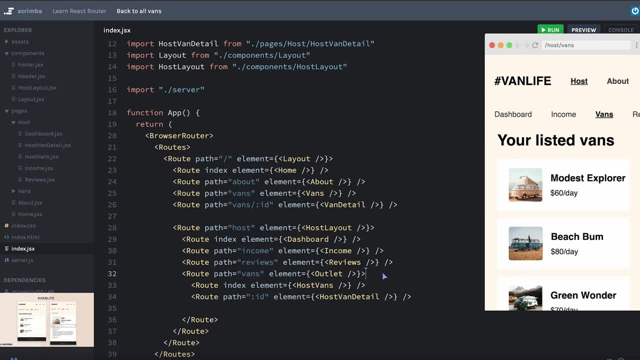 that takes us back there. Now, the reason I was mentioning this is a bit ridiculous is because this is a lot of work just to get that back button to work. So I'm going to undo all of that. go back to the way we were. 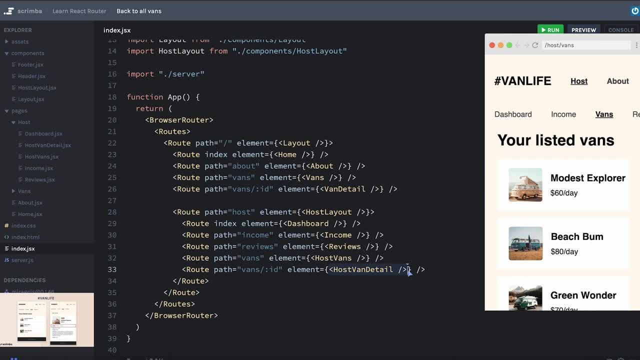 we have no shared user interface between these two, So there's not a really compelling reason to have a nested route scenario like we just saw. So how do we fix this problem? Well, react router has us covered If we go to the host layout. no, the host van detail. 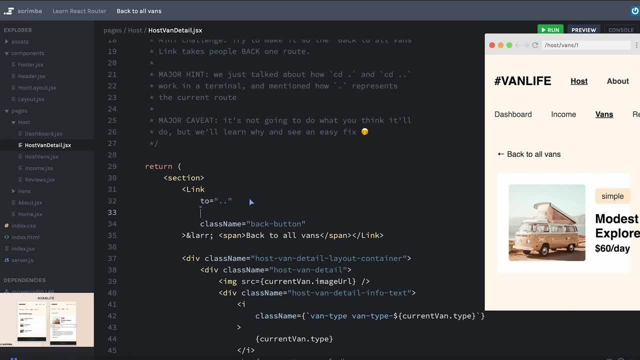 our link. one option for a prop that we can pass is something called relative. And we're going to go to the host van detail And we're going to go to the host van detail. What we can tell it is to be relative to the path, not the routes. This means that when we say we're 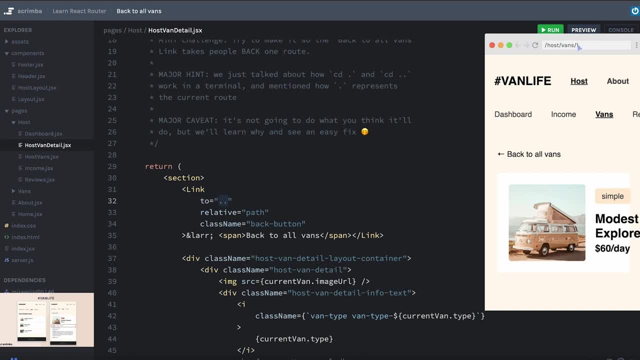 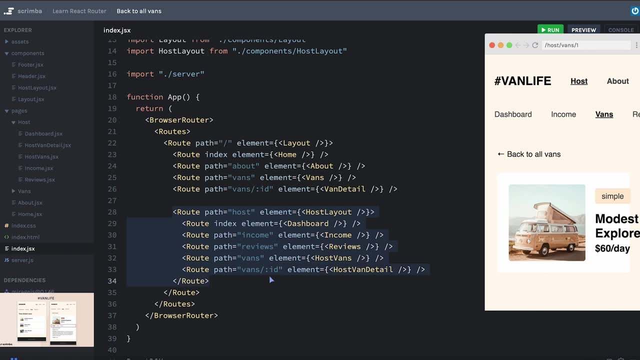 going back a route. we mean that we're going back one level in our routing structure, in our path structure, not up a level in our routing hierarchy. With this setup, react router knows that there's a slash here And it knows that we're just going to go back one little path segment, which would 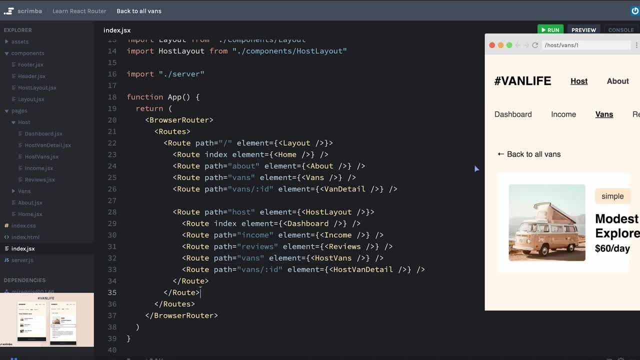 be this host vans path. So let me put my money where my mouth is. let's hit save Back to all vans. now successfully takes us just back to the parent path, not the parent route. That might have been a lot to take in. I know we went kind of quickly. If you need to watch this, 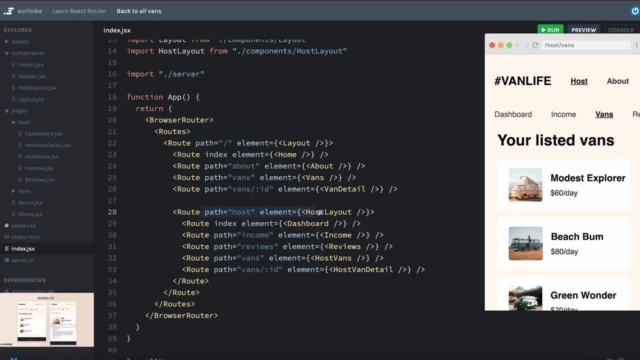 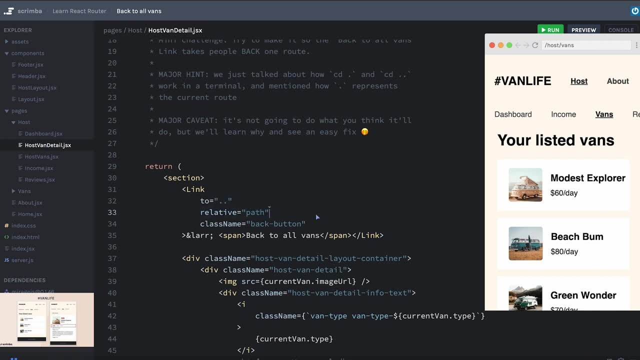 again, that's okay. Understanding this relative path thing took me a while to fully grasp, But I am grateful that react router introduced this relative equals path prop because that wasn't always there And it really helps us out in scenarios like this. Okay, I promise we're. 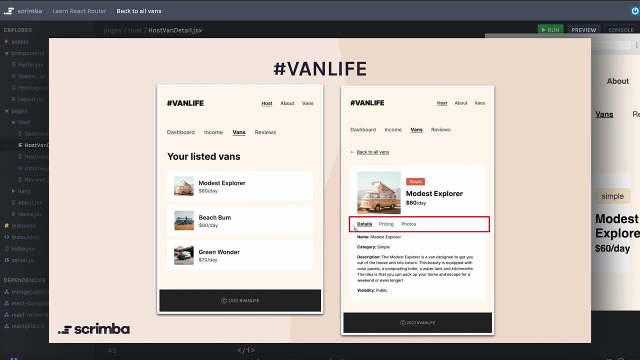 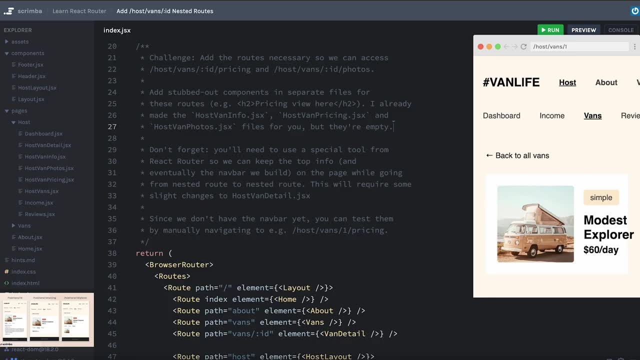 done. talking about relative links, Let's get back to what we were working on, which is getting this navigation bar working All right. this challenge is going to be a little bit of a doozy, So I've tried to give you the hints and the preparation you might need just to make this a 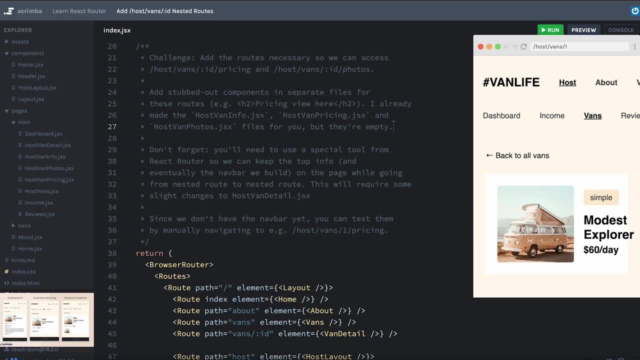 little bit easier for you. That being said, just because it's a more difficult challenge, it doesn't mean that you're not prepared for it. Assuming you've been following along and doing all the challenges, you should have all the tools and knowledge you need to complete this. 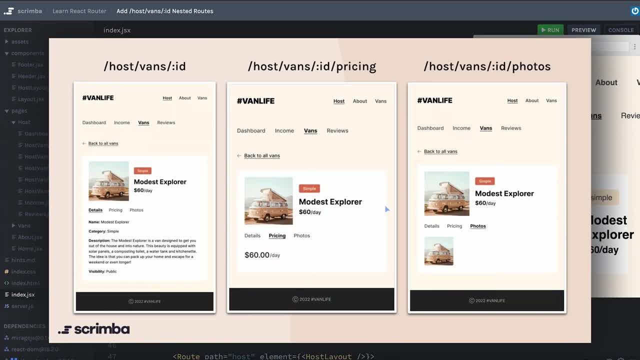 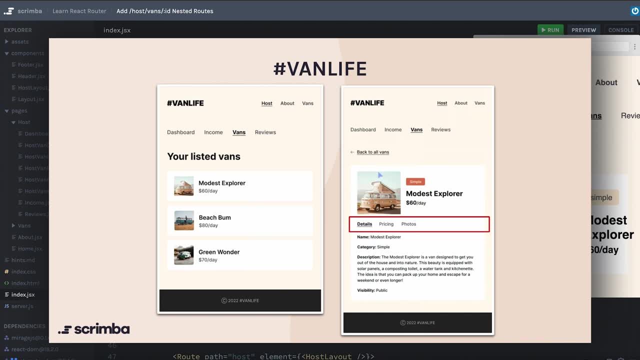 challenge. So what exactly are we doing? We're not yet working on the navigation bar. Instead, we're going to create a route, or the routes that we need, for these views, underneath what we've already created, to display. So this view over here shows you the three different. 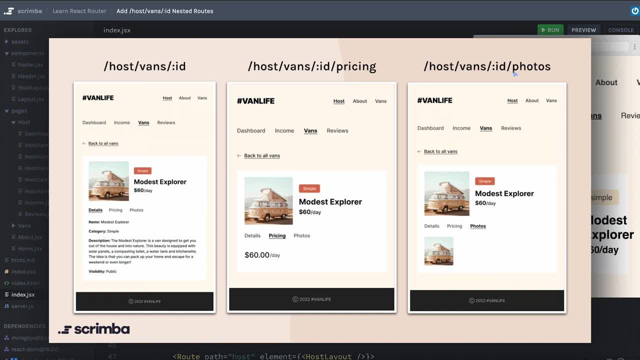 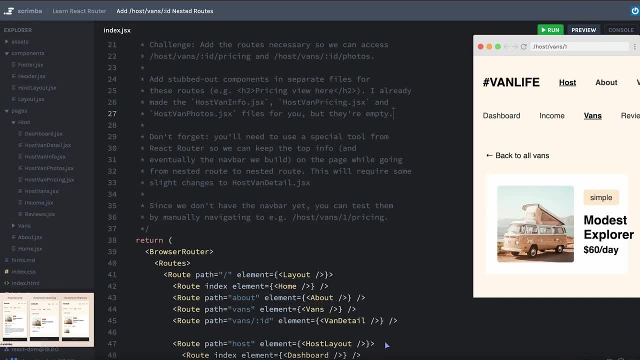 views that we're creating. side by side, Up at top, you can see the three different routes that we're expecting to use in order to see these views, And so that's what your challenge is: It's to set up the routes that you need here in our index file that are necessary so that we can 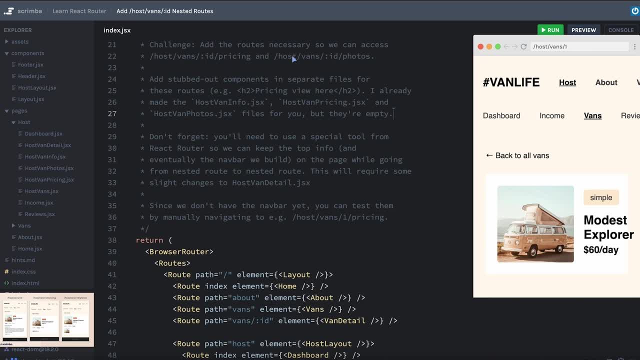 access the host vans ID pricing and the host vans ID photos view. Part of this challenge will be for you to add some stubbed out components in separate files. I've already created these files for you. We have the host van info, the host van photos in the host van pricing components. They're just empty files right now. 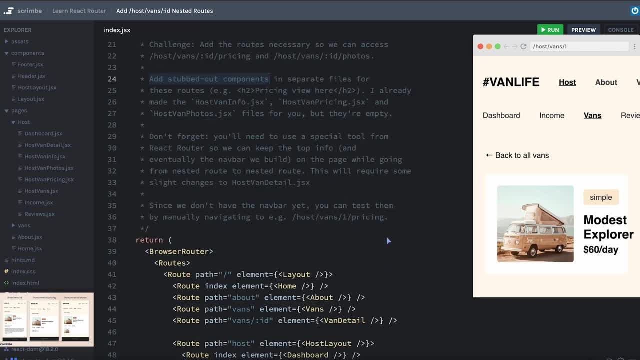 so that's part of your challenge is to fill those out, But they can just be stubbed out. Like I said, you just maybe add an HD that says pricing view goes here, or whatever. My first tip that I'll give you is that you need to use a special tool from react router. so that we can keep all of this top info that you see over here in view over here, And that's exactly what I'm going to need right now. So I'm going to certain plug this down to an undrafted source leader. If you see all of this pop up here and then ever comes out just typical new items, it's going to. 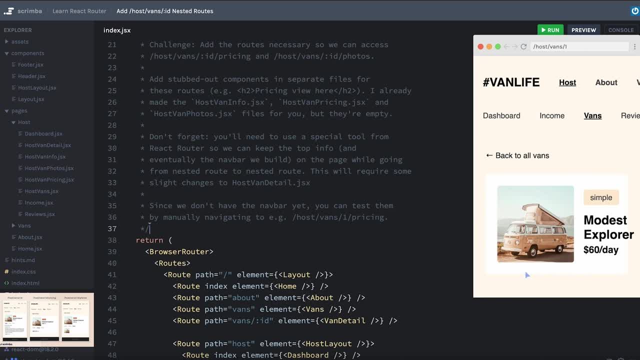 here in view while we navigate between the different sub views or sub routes that we are going to be creating. This is going to require some slight changes in the host van detail page, And I've tried to indicate where that will be exactly in that component. 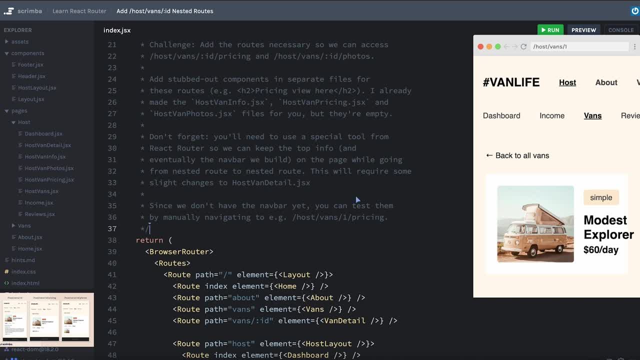 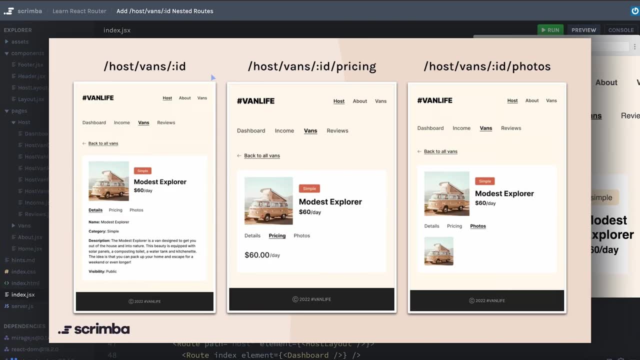 Now, since we don't have the navbar yet, you can test them manually by navigating in the URL bar, by actually just typing in the path that you want to go to And actually, as you might have noticed, the slash host, slash van slash, ID, view or path. 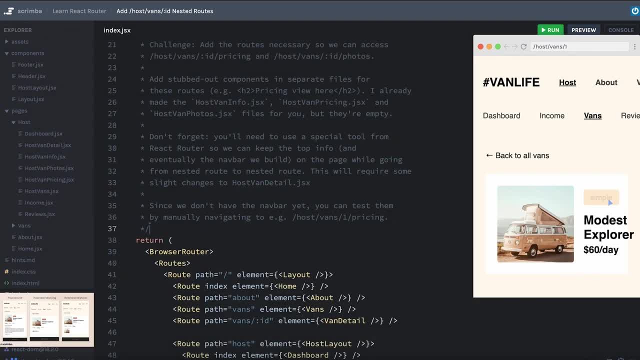 will display the information down here at the bottom. Currently we're not doing that, but we are at that path, So you should be able to start out by just adding what you need in order to display the information or, more importantly for this challenge, just a stubbed out version of that. 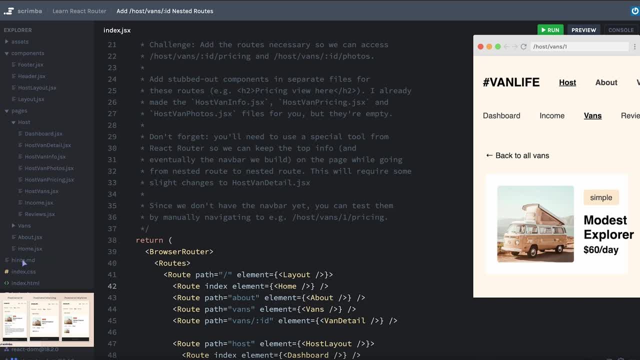 Because this is a little bit more of an involved challenge. I did include a hintsmd file. I'm not going to click on it here because it'll give away the first hint. Try not to go there if you don't need it, But if you do start feeling stuck, then feel free to go to the hints. 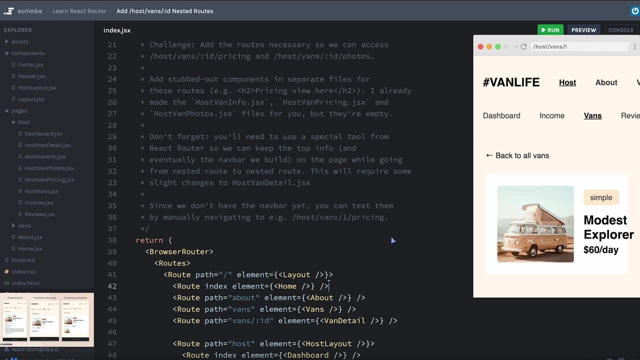 I have two hints that are separated by a lot of space, so you have to scroll to see hint number two. Okay, lean on your instinct. remember what you've learned. rely on the community. if you're really feeling stuck, turn to the hints if you need them, but I believe in you. 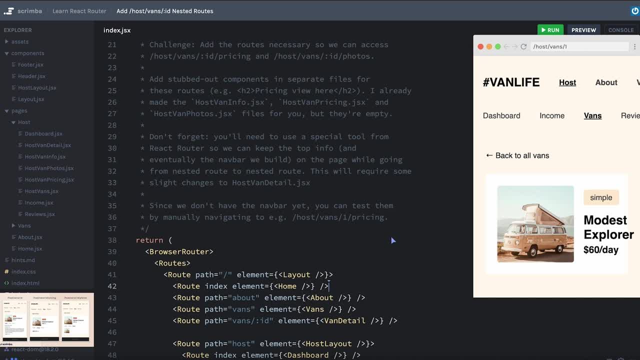 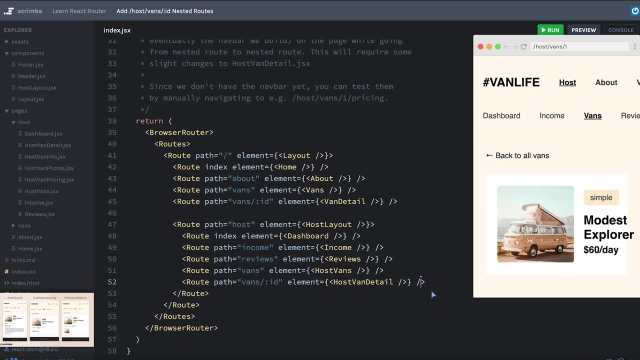 You've got this. Pause now and work on this challenge, Okay. well, the first thing I'm going to do is take this route here and turn it into a parent route to other routes. Currently it's self-closing. Let's go ahead and not make it self-closing and we will add a closing route element, or? 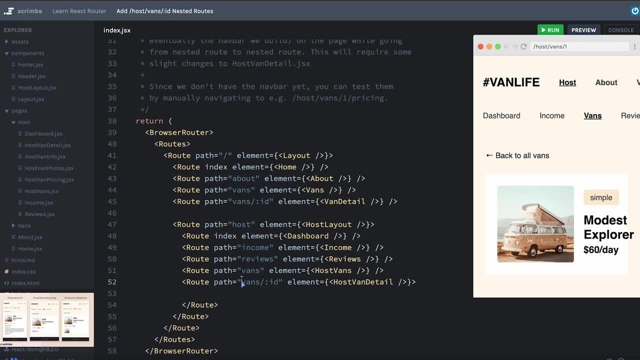 tag here Now. the reason I'm doing that here again is because this van slash id, or rather slash host, slash van slash id, is going to essentially become a layout route for the children routes that I'm going to create. We're starting to sort of conflate what we're actually referring to when we talk about a. 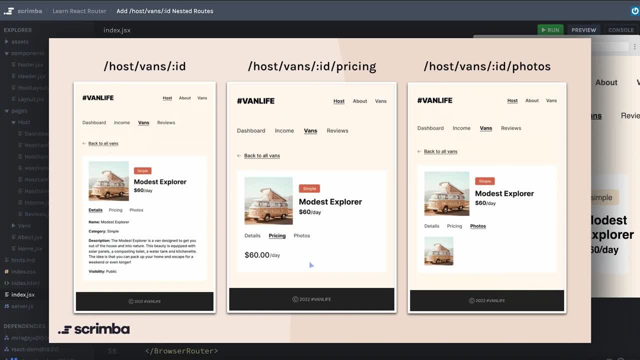 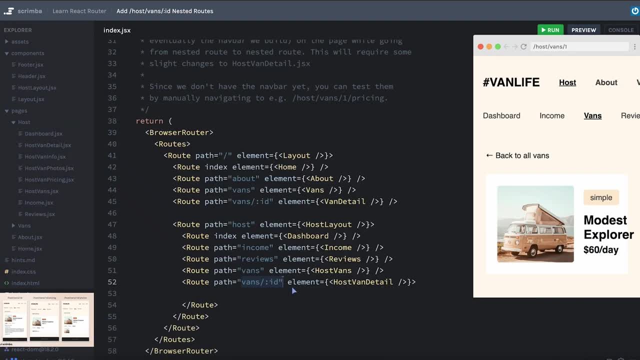 page Because, if you think about it, we're not really creating new pages here per se. we're just swapping out, We're creating a small portion of our UI, But for the time being we're calling it pages. Maybe this is where a good refactor of our folder structure would make a lot of sense. 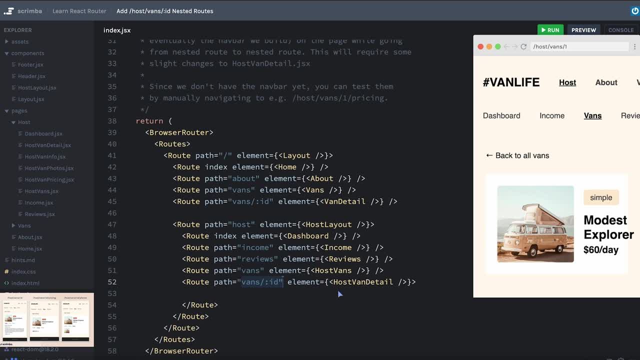 I'm not going to do that now because it's outside the scope of what this challenge is. But by doing this I'm turning this element, this host van detail element, what we see here- into sort of a layout route or a layout component. 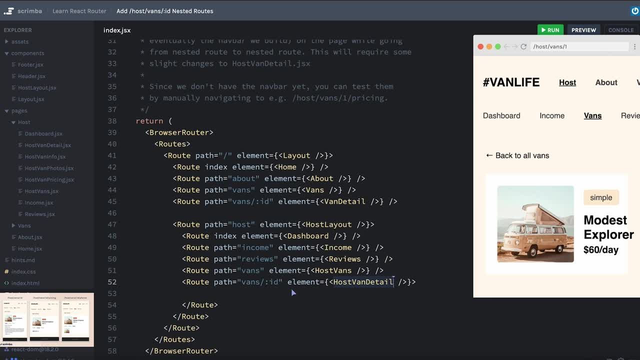 And when I have a layout component where I have child routes that need to be displayed, I need to use the outlet component. So before we even work on creating the layout component, I'm going to go ahead and create a child component And that's where I'm going to be creating these nested routes. 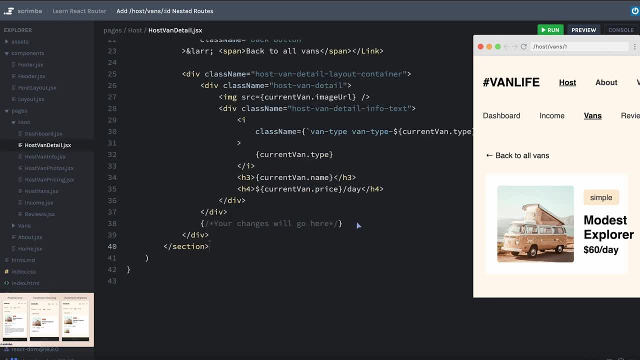 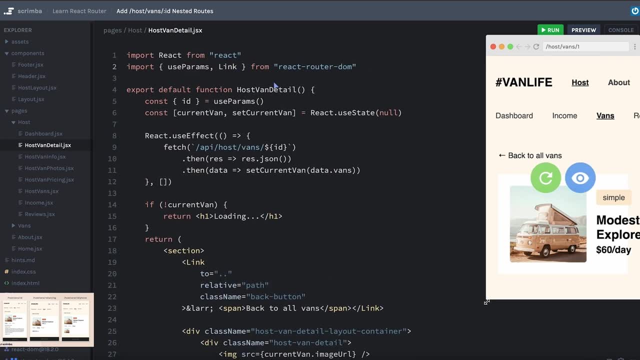 Let's go over to the host van detail component, and my changes are going to go here. This is where I'm going to include an outlet component. I need to make sure that I import that from React router dom. So we'll import the outlet. 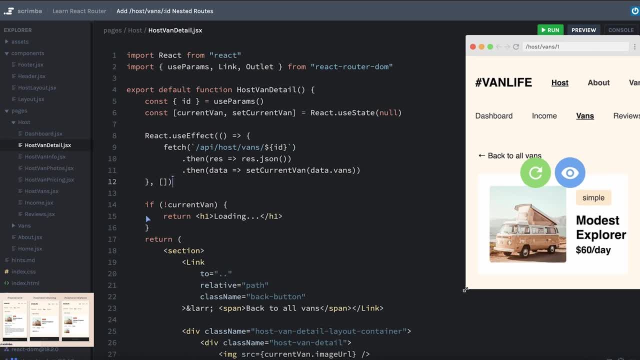 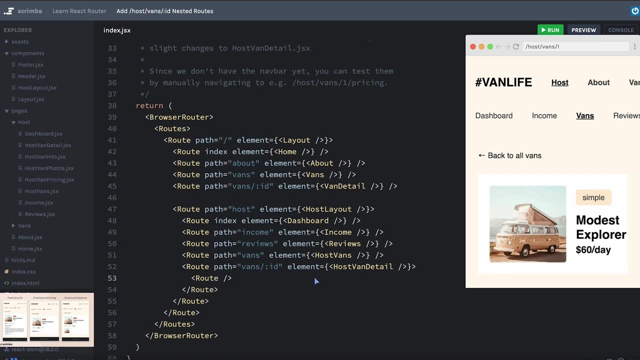 I think hitting save should change nothing at this point. Now let's go back to our index and let's create our child route. This one will be self closing for the time being. we're not going to have any more children nested, which hopefully makes you a little bit happy. 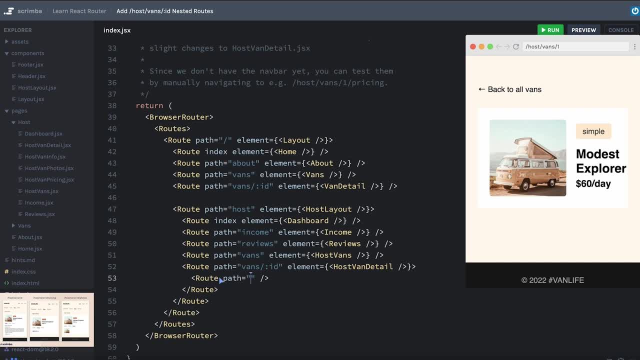 about getting closer to the end here. we're going to say that the path is equal to- and actually you know what? this is not going to have a path. instead, this is going to be the index route. as i mentioned, the slash host, slash van slash id route should automatically and by default display this. 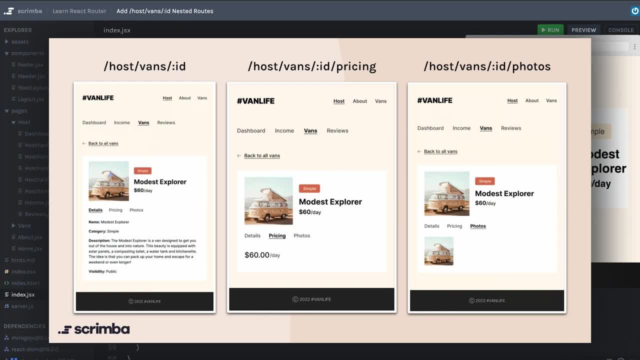 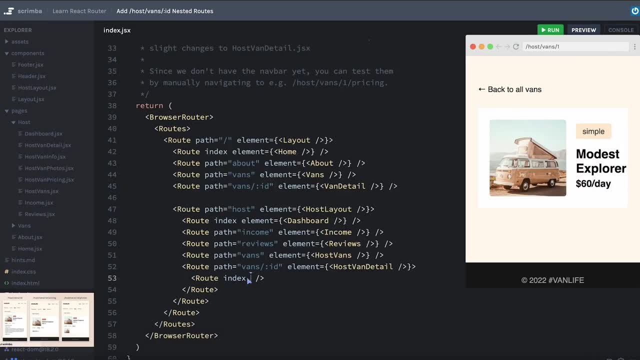 information. so we're not saying it's slash host, slash van slash id, slash details or anything like that. it's just what will automatically be displayed on this route. so that's when i would use an index. we'll say the element is going to be well, you know what? instead of going down the whole path of 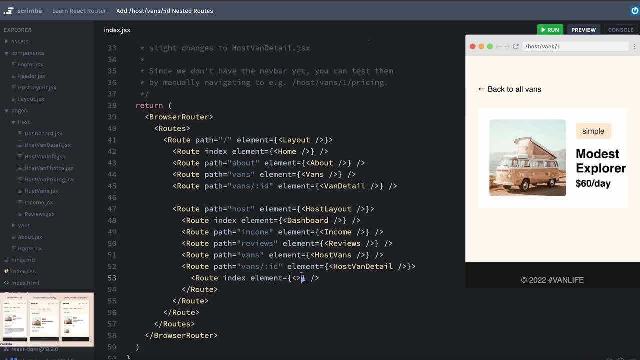 creating the stubbed out version here and importing it. let me just kind of skip that for just a second and we will just render, let's say, an h2 that says the detailed info goes here. assuming we have this set up correctly, it's not probably going to be pretty, but let's hit save and look. 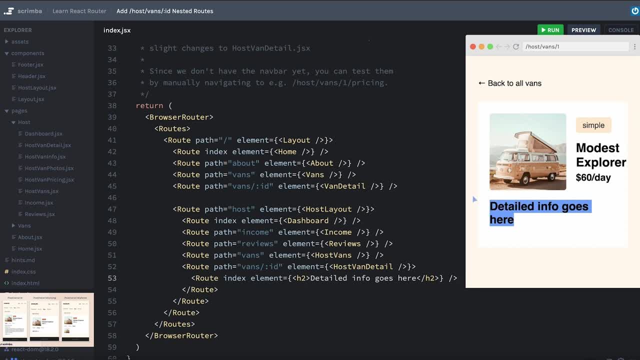 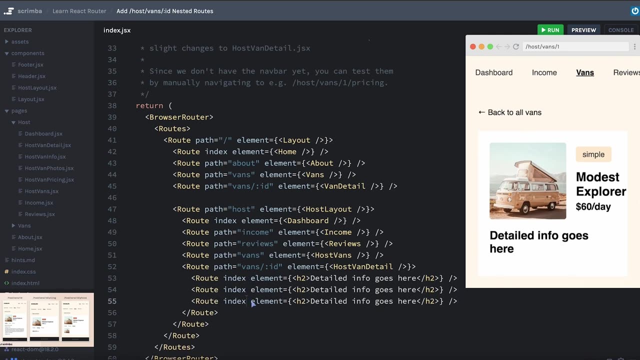 at that we have inside of the layout here. the detailed info goes here, perfect. but if i navigate to slash host, slash van slash one, slash photos, well, because that route doesn't exist, it's just going to give us a blank page. so we're not quite there. fortunately, i can just make copies of this we'll. 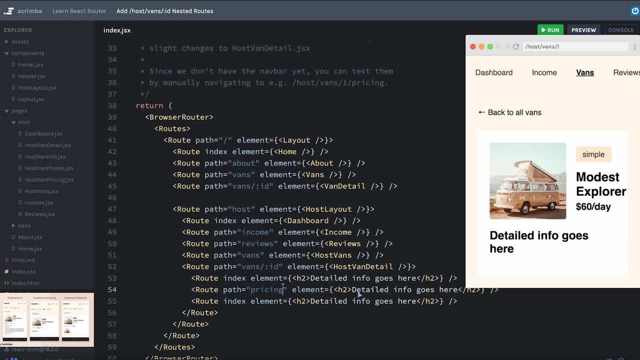 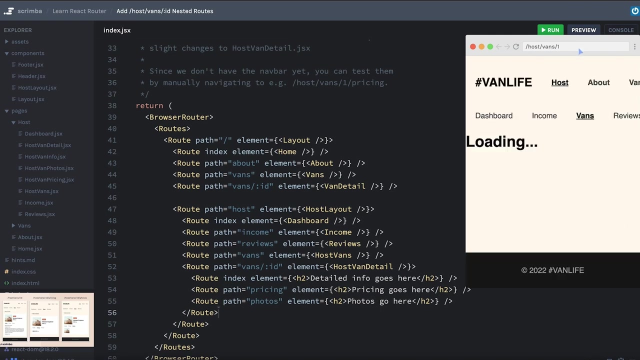 change this one to have a path of pricing and let's say the pricing goes here and we'll change this to a path of photos or foots, no photos. and we'll say that the photos that'll be go here. all right, let's cross our fingers. hit, save. detailed info goes here. we'll manually go to slash photos. hit. 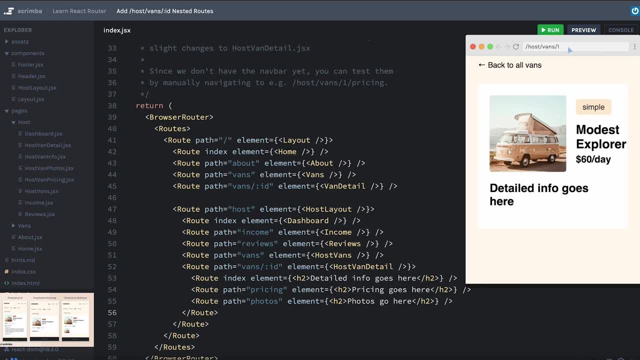 enter. oh, and for some reason the url did not listen to me. sometimes this can be a little bit tricky, i don't know. let's try a refresh. okay, that took a minute, but here we go. we have photos. go here. this has been quite a bit. the rest of this is just kind of procedural, so i'm going to import. 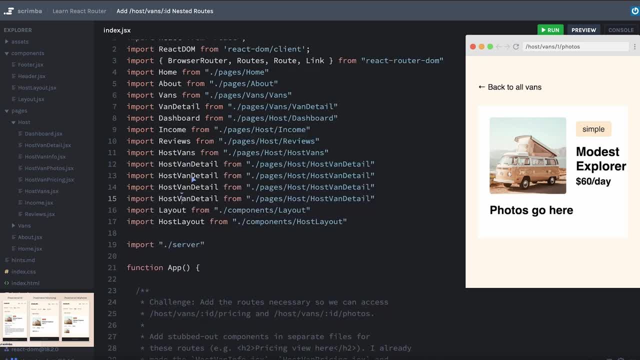 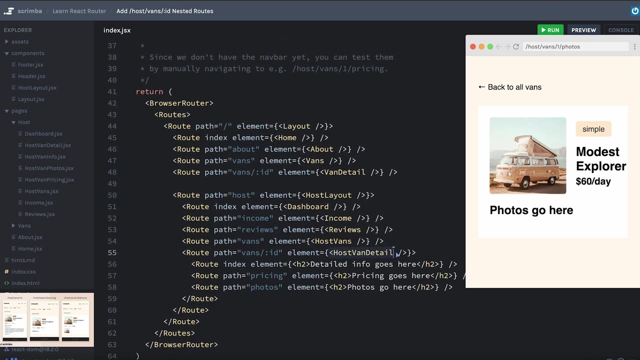 let's see, i'll just copy this one, since that's most closely related. the third one: so we'll bring in the host and info, host van pricing and host van photos, components, okay, and then i'll just, uh, let's just copy this and replace each one of these. okay, those components have nothing in them, so we need. 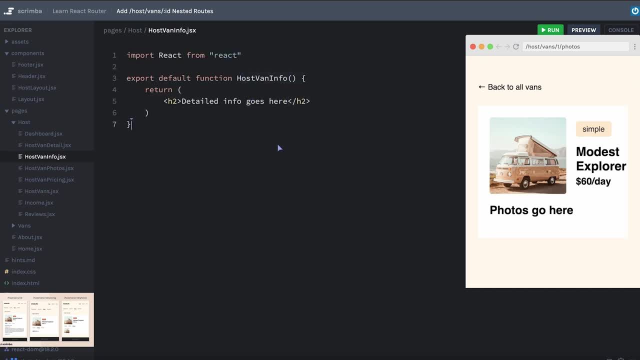 to fill them out. okay, so i created this one for the hostman info and we will cheat and copy this over to the host van. what is this one? photos, photos go here, say, pricing info goes here, and i think we should essentially be where we were before. 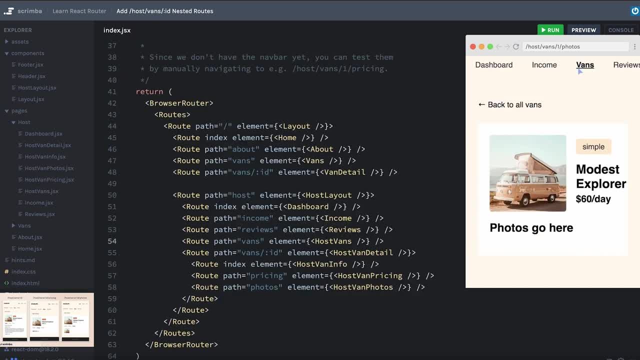 so let's go ahead and hit save okay, photos go. yeah, because we're at the photos route. let's see if this even works. pricing: hit enter okay. that takes me to the pricing page. and then, if i just go back to slash one and hit enter, detailed info goes here now because i'm entering. 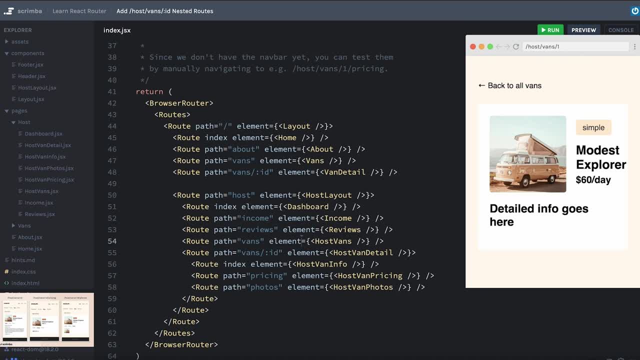 this in the url bar and hitting enter it's actually doing a full page refresh. but in the next challenge where we add our navigation bar, that will take us from one page to the next without the whole full page refresh and flicker happening. Okay, take a deep breath. Hopefully that was okay. I completely understand if it wasn't. 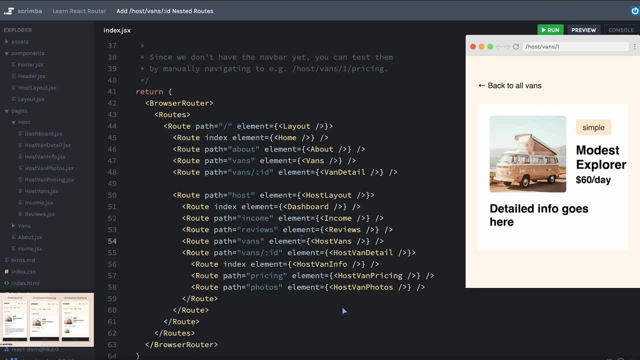 even if you have been doing all the challenges. I think this is probably the most involved challenge that we've had so far. If you were able to do it, pat yourself on the back. That's a big congratulations. If not, again that's completely okay. At this point I would scrub. 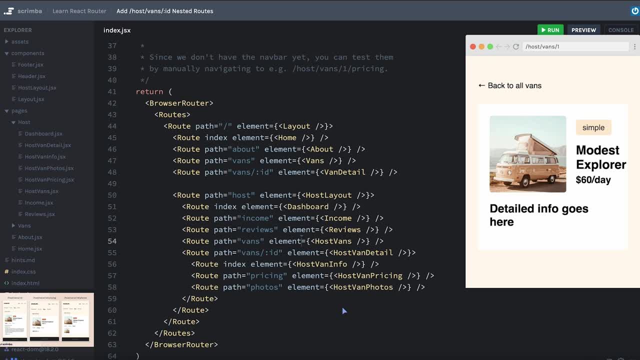 back to the beginning of this scrim and try doing it again from scratch. As always, that muscle memory is only going to set in if you are actually typing with your hands on the keyboard, working through it in your mind, trying your very best to get it done, No matter what happened. 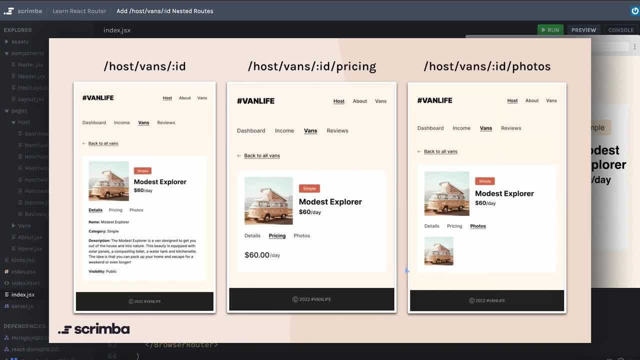 great job or good effort, And now it's time to really tidy everything up by putting this navigation bar in, And next we'll be working on adding the navigation bar and then figuring out how to make the actual information show up instead of these silly little stubbed out versions. 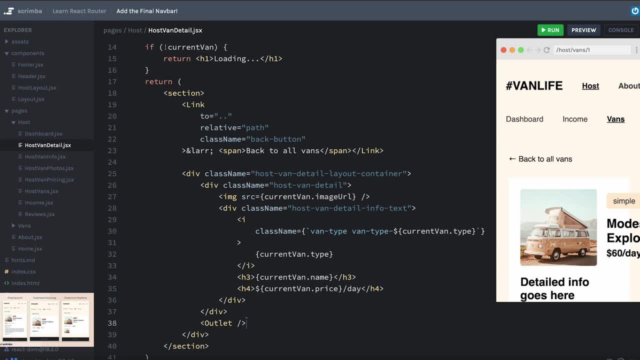 Before we even jump into the real challenge on this scrim, I want you to think for just a second. We have here our host van detail page. Where on this page are we going to start writing our nav bar code? Take a look at what we currently. 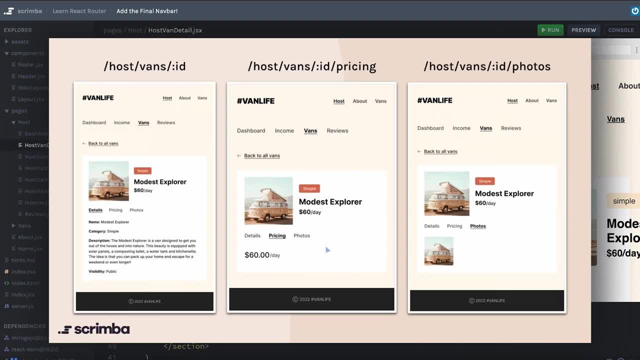 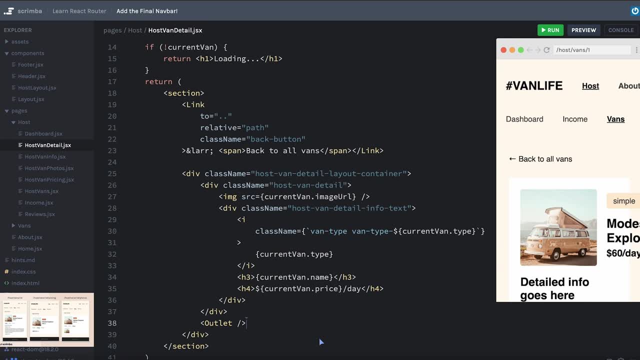 have where the outlet currently sits and what it's supposed to look like. Here we have the nav bar and then the information. So if you need to, you can pause and think about it. Otherwise, I'm just going to be quiet for five or seven seconds and let you answer the question. 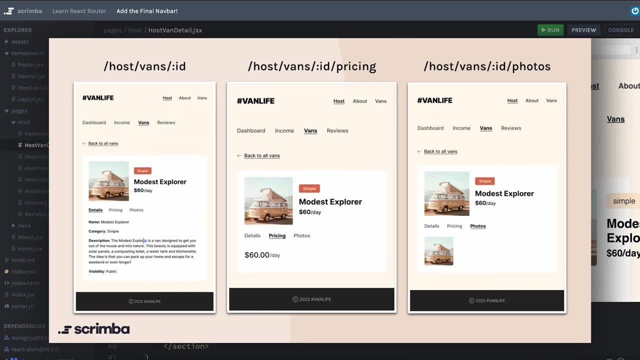 Well, the outlet represents the switching out views or the user interface that we're going to be changing from one route to the next And we show that our navigation bar is above that switching out view. So we're going to add our nav bar code above our outlet here, right here. Okay. 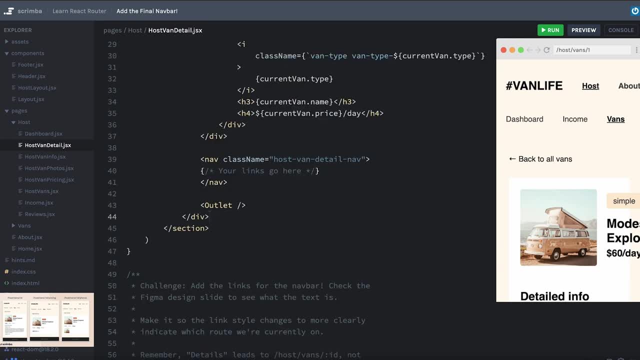 that sets us up for the challenge. Let me type that out. Okay, this is fun. The challenge text is actually here below, where you're going to be writing your code. Now I did add the nav element with the correct class name and the CSS styles that you need, just to make sure that everything. 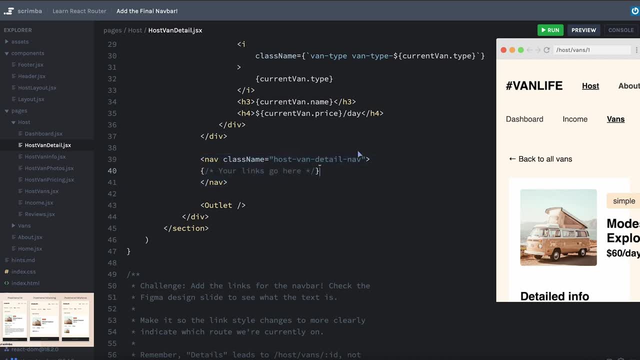 looks okay. So you should be able to just add your links as part of the challenge and the style should kind of work out okay. So the challenge is to add the links to the nav bar. that's going to be above this information. that's showing it below here. that swaps out from one view. 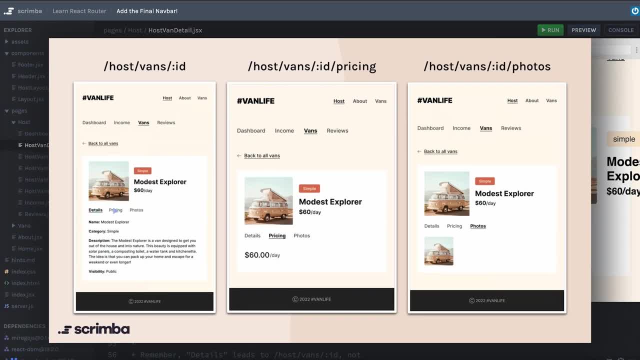 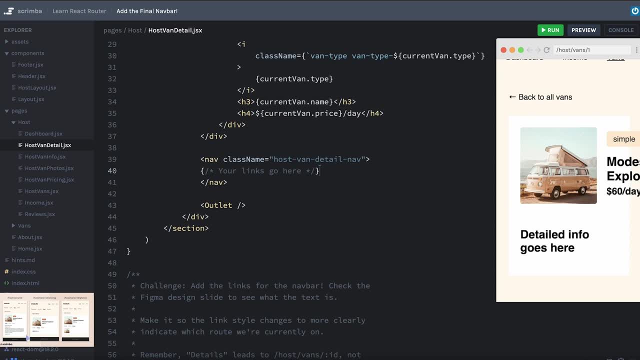 to the next And if you need to check it out, I mean it just says details, pricing and photos. So that's really what I mean by check out the Figma design to see what the text of the links should be. We also, as you might notice, want to make it so that there's a clear indication as to which 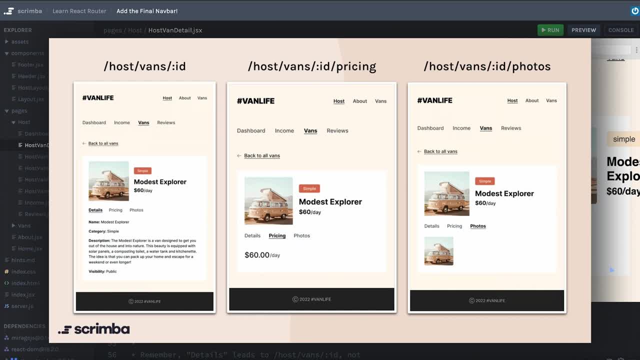 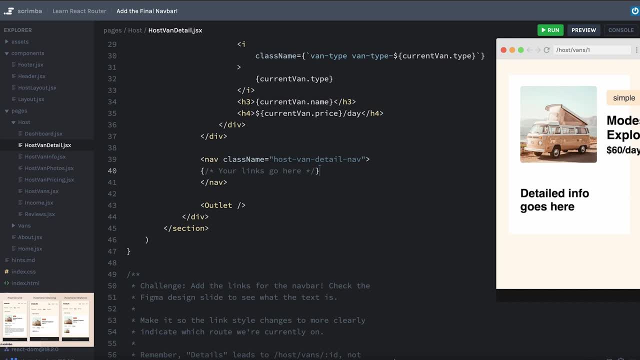 route we're currently on, So you'll have to remember how you can do that, And if you're going to do that, you're going to have to click on the details link And, of course, you can look at the other parts of the code base where we're doing that. we're already doing that in this nav bar and 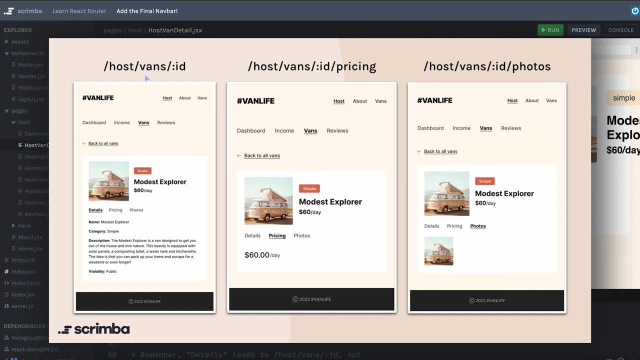 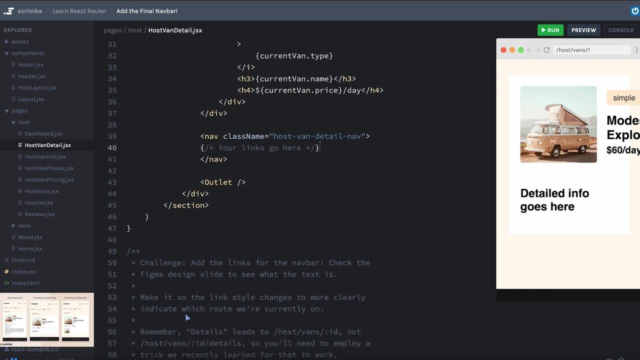 this nav bar And remember the details link. here is just leading you back to host vans ID. it doesn't go to host vans ID, slash details or anything like that, So you'll have to remember the little trick we recently learned so that clicking the details link will take you to that route. 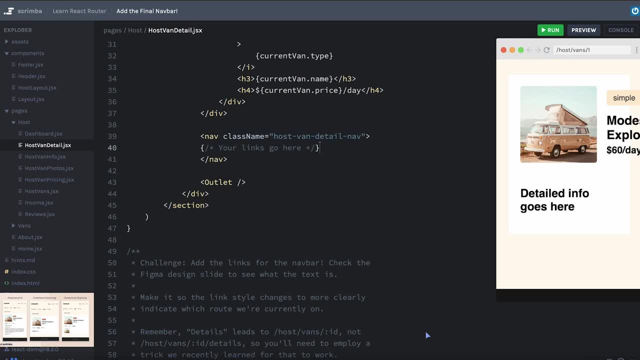 instead of one of the other nested routes. Okay, that's enough of me talking. Pause now and add our links. Thank goodness, It's our final navbar, Am I right? Okay, let's go to add our links here Now, because we want to indicate, based on the current route, a different kind of style for each link. 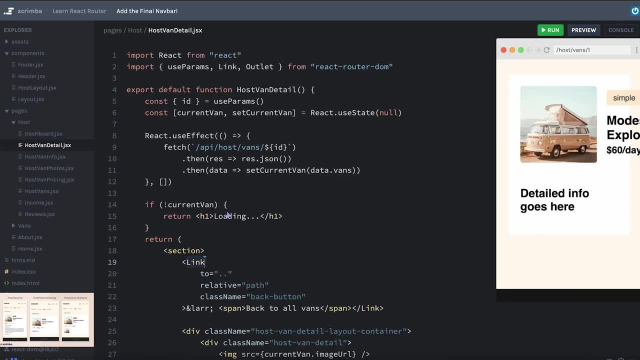 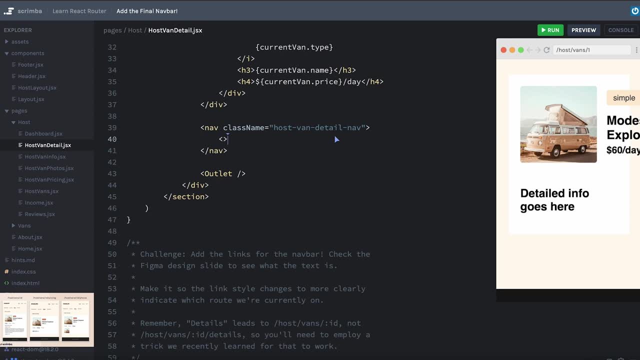 we're not just going to use the link we're going to, which we're already importing, we're going to also use nav link. So we need to make sure we import that, then get rid of this And we'll say we're going to add a nav link And we're going to have three of them for details, pricing and 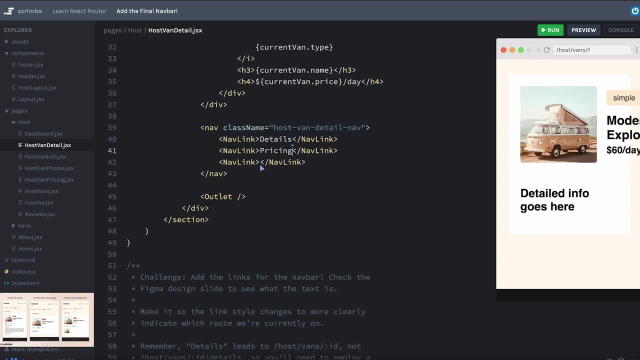 photos. So let's just type in that text And we're going to add a nav link And we're going to add a text here: details, pricing, photos. Now I do know that I'm going to be adding a few other things here, So I'm just going to split things out onto their own lines right now And we'll put a little. 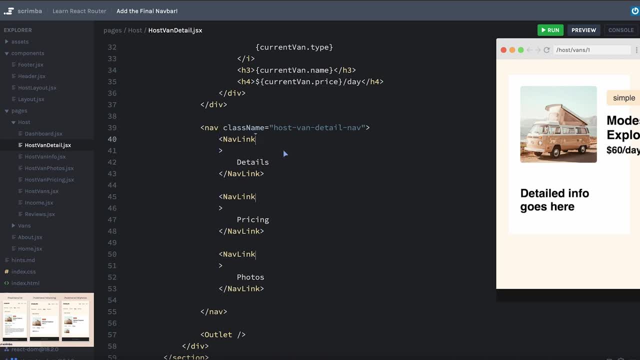 space, just so it's a little easier to understand what's going on here. Okay, first of all I need the two path, So we'll say two equals And let's work on getting these right. So hopefully the pricing and the photos was fairly easy Because I'm inside of my nested route. I can just say: 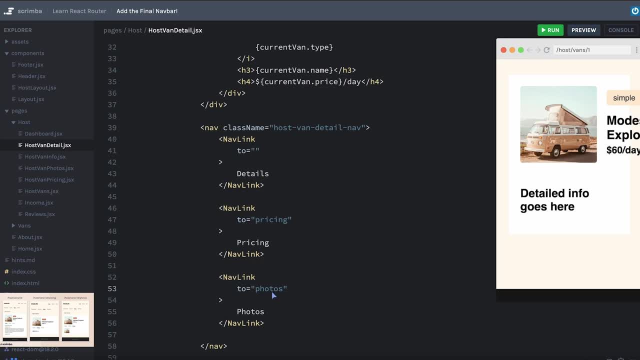 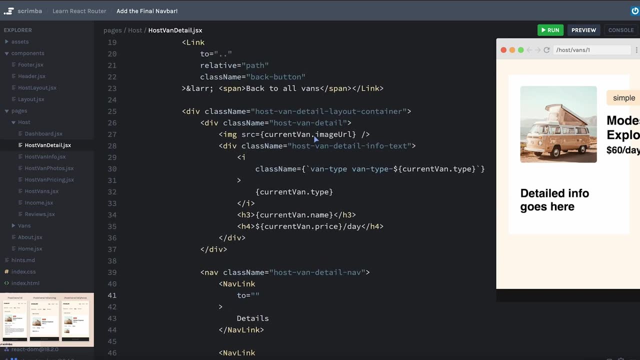 pricing and photos And I'm going to add a new path. And I'm going to add a new path And I'm going to say pricing and photos. I don't need to specify the entire absolute path leading up to this. this one is the tricky one because the details should lead us kind of back to the route. 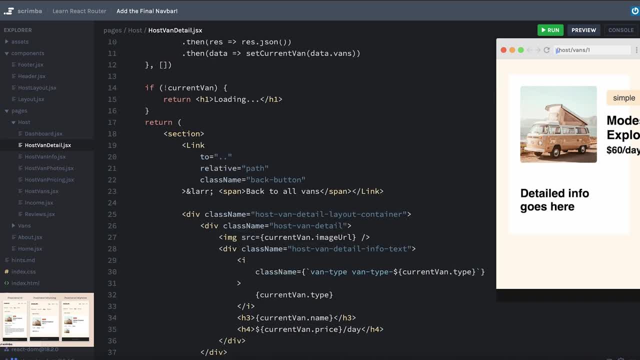 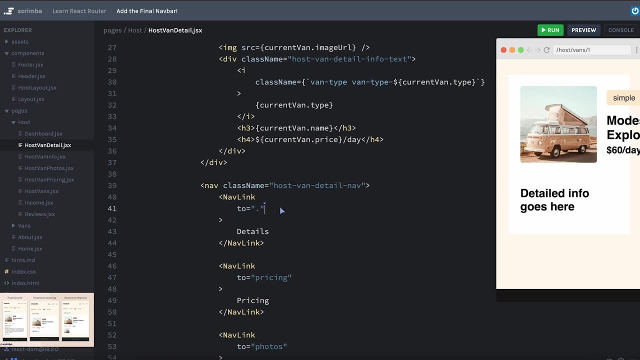 where we're currently writing this code. In other words, all this code is living at slash. host slash van slash, and then the ID I'm going to use, just a dot, And that represents the current path. Remember, this host van detail is being rendered at the ID path or endpoint here: host vans ID. 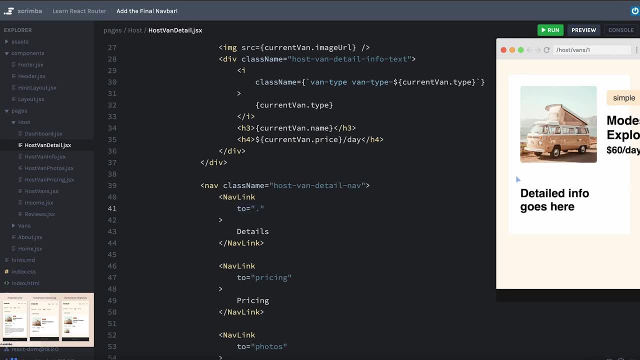 And so when I say to dot, that means just go back to host man's ID, And actually I think this is a majority of what we're trying to do. So let's hit save. we're going to see a little bug here. Oh, actually. 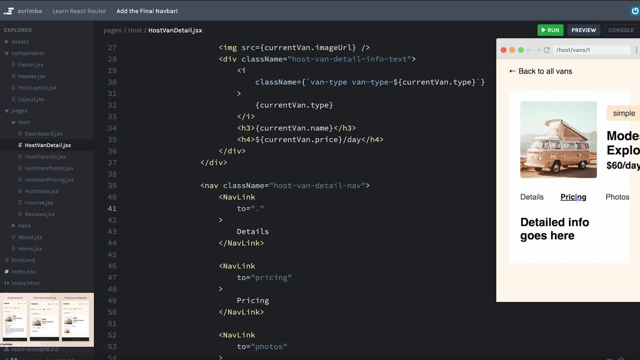 we're not going to see that little bug till we get the styling in, But I, hopefully, can navigate. let's hit pricing- Awesome. This is so cool. photos details- that takes us back to detailed info goes here. Perfect. Now let's add the actual active class that we need by using the style And. 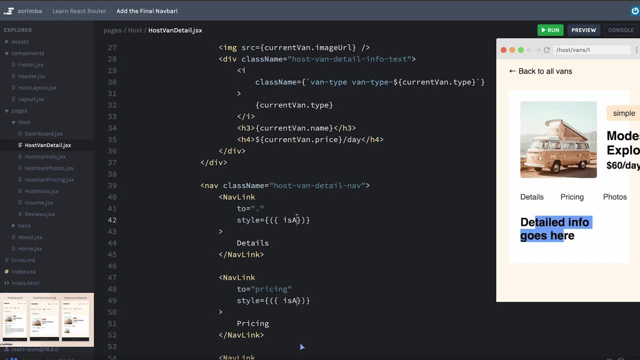 again, this is going to be a function that takes an is active prop or parameter and we want it to return. if is active is true, we'll return. we haven't created this yet, But we'll create some active styles And yikes, this is starting to bleed off the page here. So, active styles or 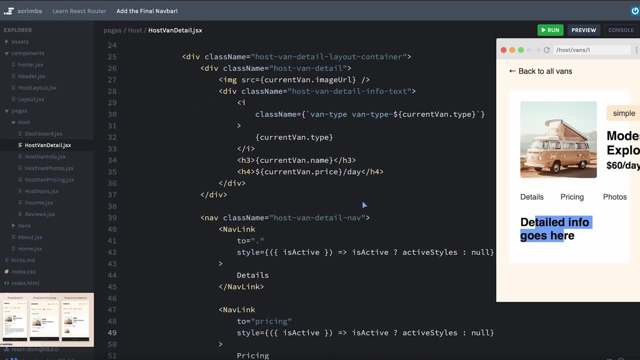 no, Okay, sorry that that's being covered up there, Because I can scroll up and we can see. that's the same. I could make this a little bit smaller, a little too small, Okay, Oh, that wasn't me. There we go. Good enough for now. Okay, these are working. No, I have to hit save And we have. 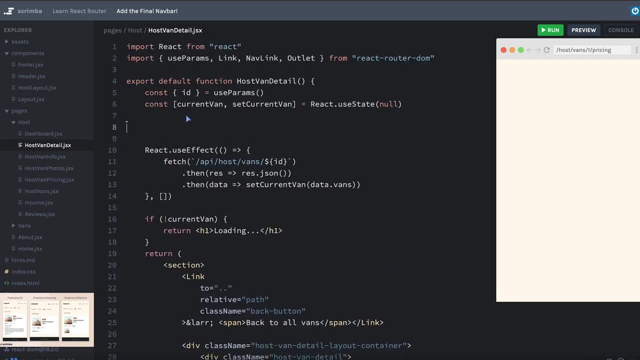 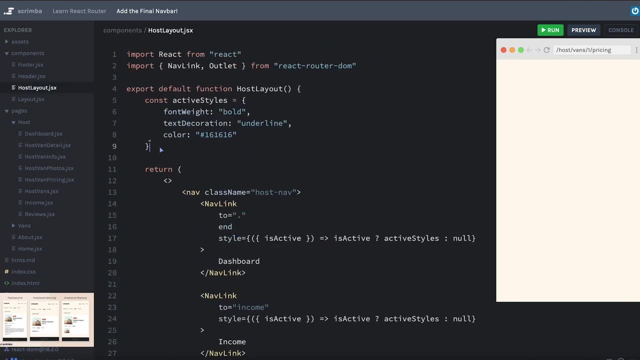 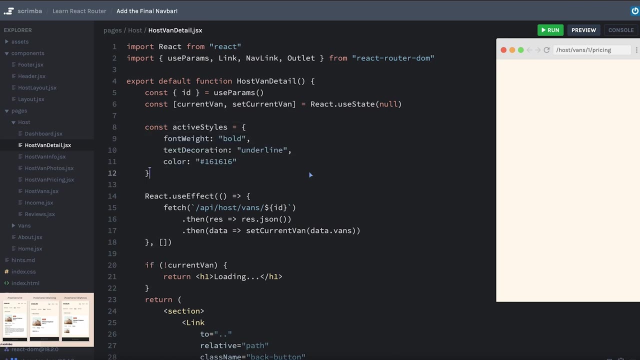 to create active styles. So let's go up here, maybe just before our use effect, we'll create an active style. So that's an object And you know what? I'm going to steal it from my other ones. So we'll just come back, spend detail, put it right there. Oops, let's replace this whole thing and 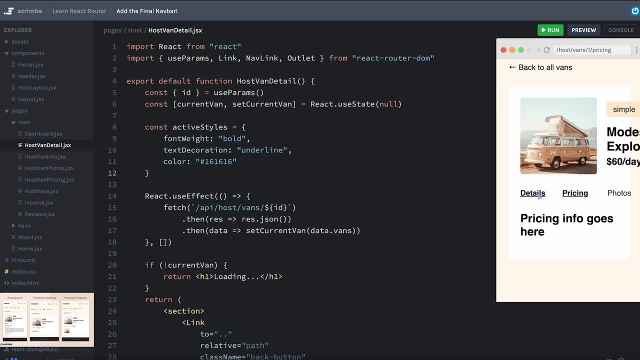 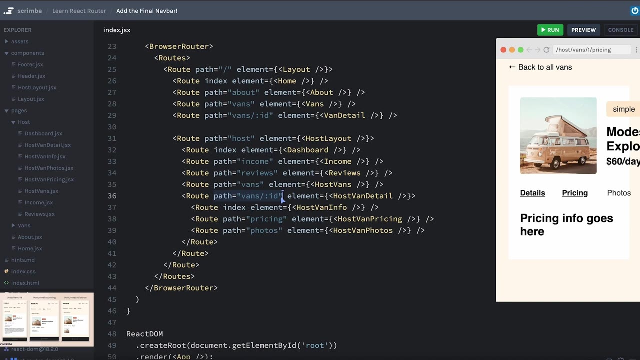 hit save. Okay, this is where we see the little bug. Remember we have both of these matching because details. This is not a sibling route per se to pricing and photos. we look here once again: the host van info is being displayed at as an index route, which means it's at this path And that means that this 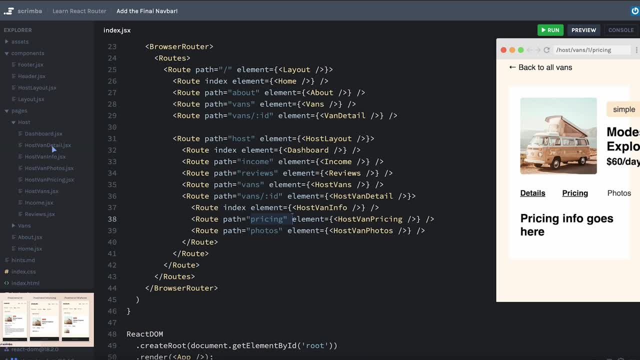 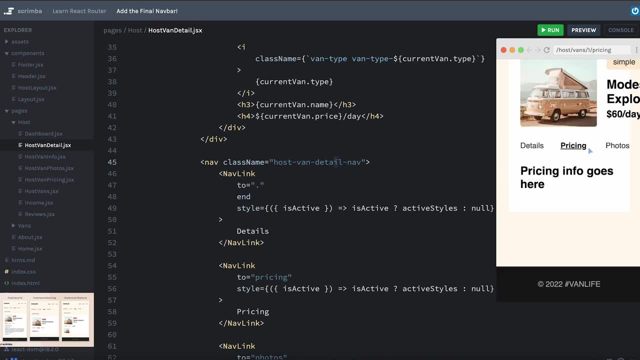 is matching currently, even when I'm in pricing. So to fix that I simply need to add: let's go back down the end prop, So I can say and we'll hit save And there we go. Okay, so now details is the only. 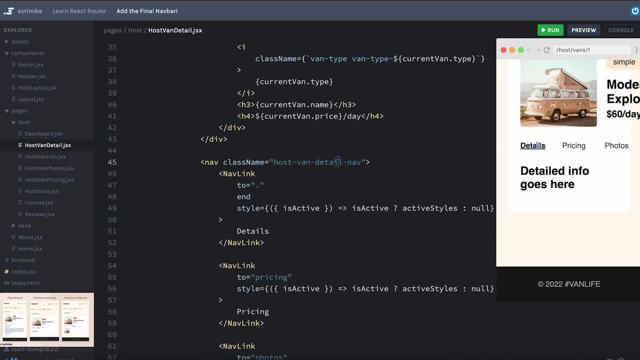 nav link being displayed or being highlighted, rather pricing. So I'm going to hit save, And then I'm going to hit save, And then I'm going to hit save, And then I'm going to hit save. Perfect, I hope everything went well. One of the final major pieces that we're going to be working on. 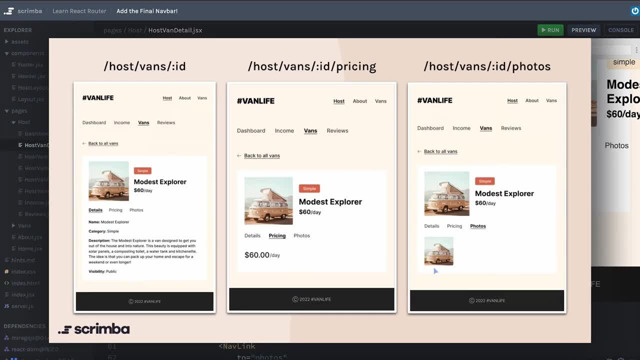 is actually getting the correct information displaying here inside of our nested routes. At first glance it might seem like it's easy because, well, we've already got this information, why not be able to display it down there? But remember, we only have an outlet here, we're not actually coding. 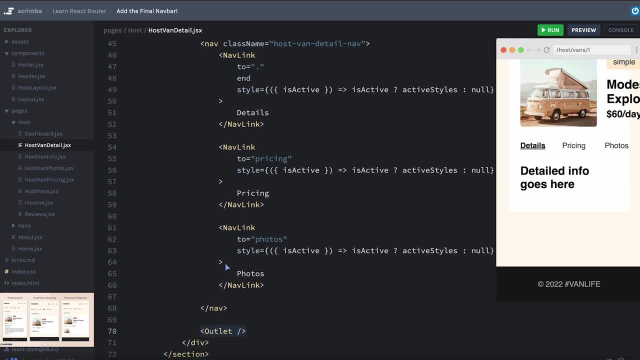 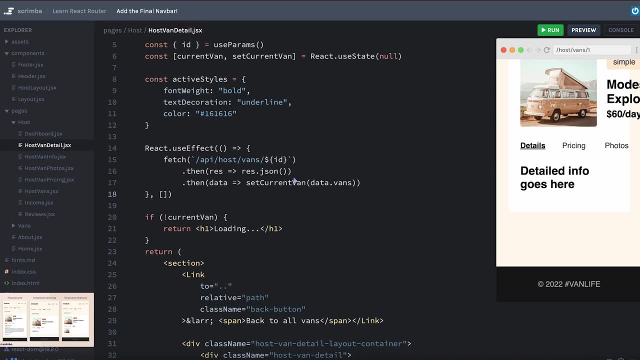 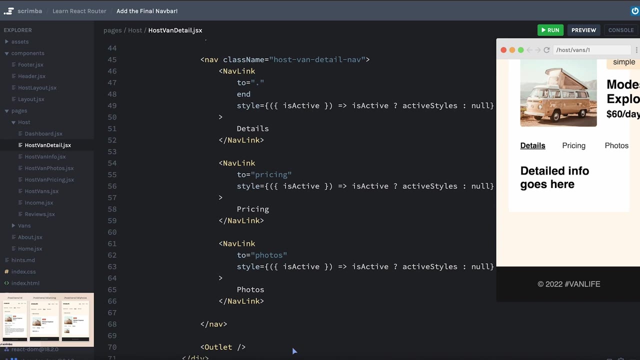 out the detailed info or the pricing or the photos here in this file where we have the information from our fetch request. So we have a little bit of work to pass the information that we've gathered to the child routes so that they have access to that information in order to display it correctly. Fortunately, react router has made this fairly easy. 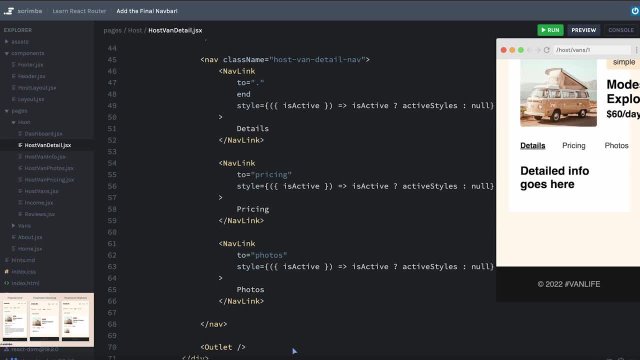 So we'll be able to do that pretty quickly. For now, start to get excited. We're almost done with the majority of our app. we have a couple loose ends to tie off, But those things are fairly minor in comparison to all the amazing work. 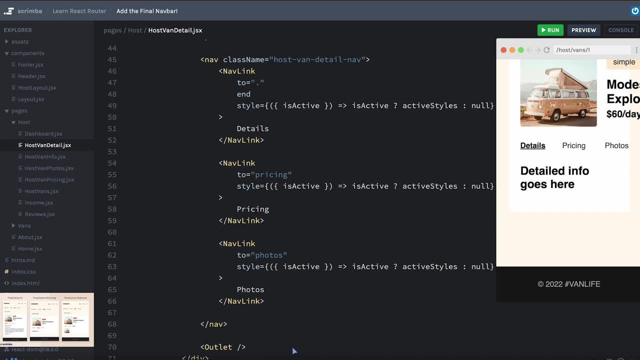 that you've done so far on this project. Once you're done with your little happy dance and maybe doing a lap around your house or something, Let's get back to work And we will figure out how to get the information into our child routes. 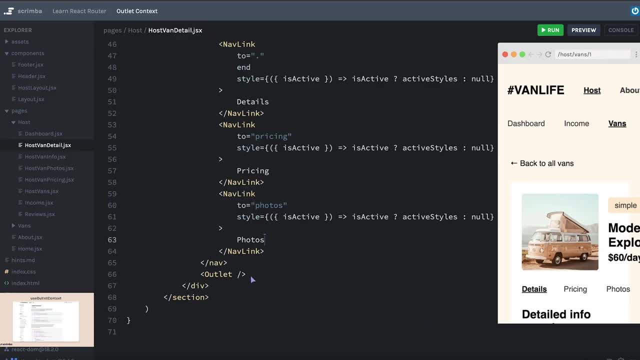 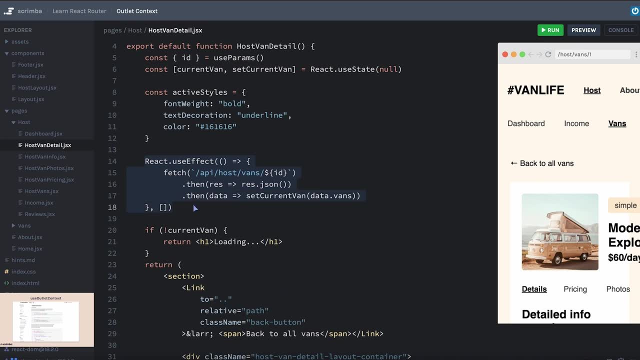 Okay, so here we are. we have our navigation bar, we have our outlet, And the place where our navigation bar lives is also the place where we're getting our information from the server. It's saved into state locally on this component, And if we were just rendering a 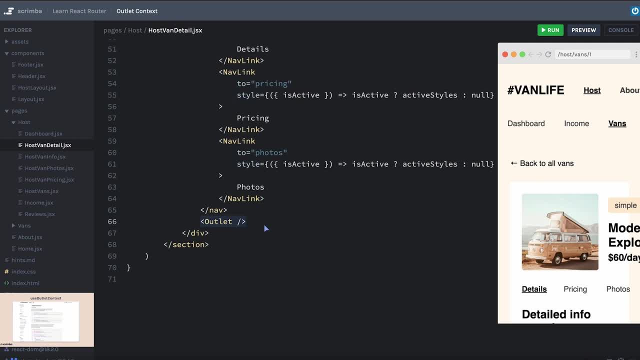 child component, we could pass this information down through props to that component. In this case, we're not rendering the host band info, photos or pricing because we don't know which one of those is going to appear in the place of this outlet. 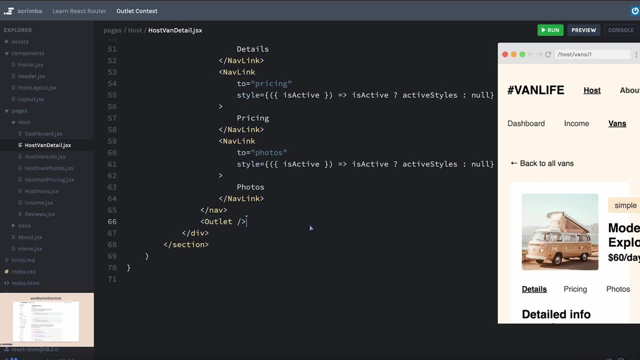 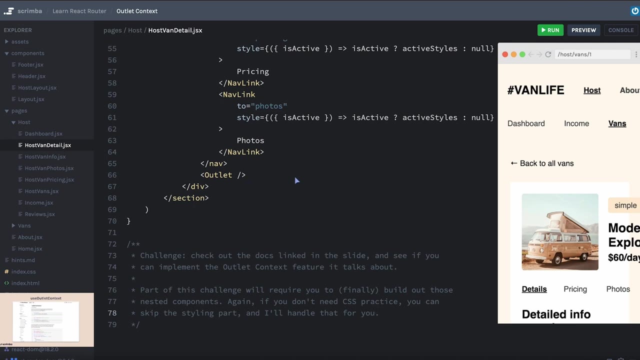 Fortunately, react router makes it really easy for us to get information into the components that are rendered as part of this outlet, And so this challenge is actually going to be a bit different than what I usually do. Let me go ahead and type it out. The reason this is different is because I'm not going to teach you how to do this before I ask you to try and do it as part of the challenge. Instead, I've linked the documentation to this. 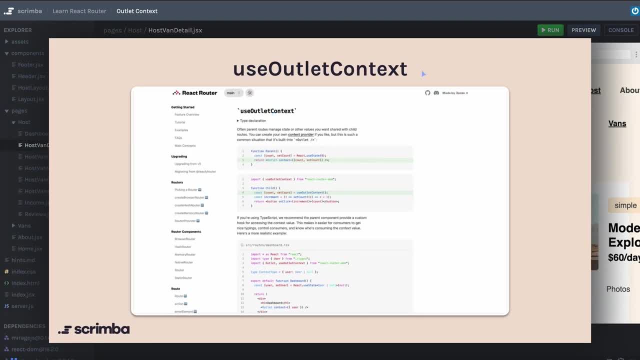 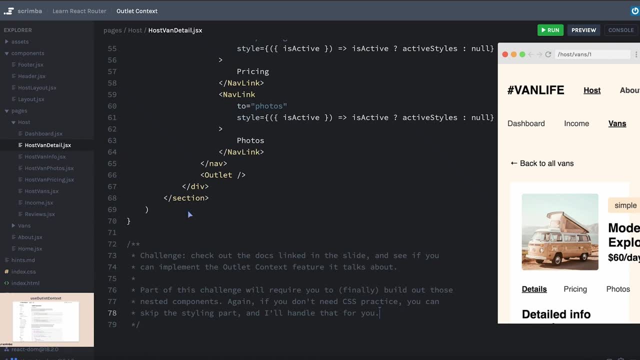 instead, I've linked the documentation to this. instead, I've linked the documentation to this documentation, to this documentation, to this documentation. to use原成用: 距離 MyButtitjpg. conversation conversation process process, process, process process process script users. Okay, pause, now go to the docs and work on this challenge. This makes a lot more. 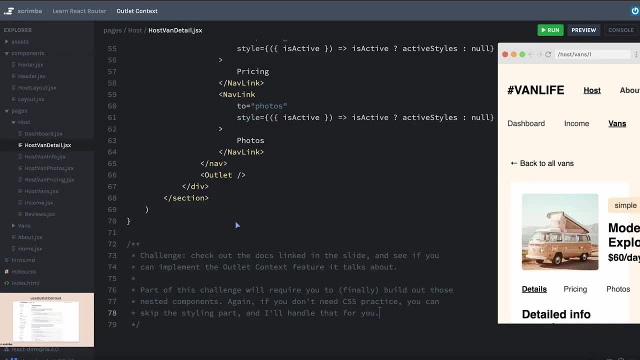 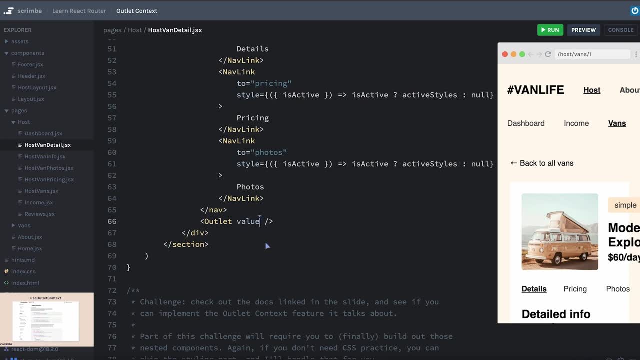 sense if you already have some experience using context in React, because in this case essentially Outlet is just a context provider In React. if I were creating this, I would create a value prop, but the way that they've defined it, I create a context prop And whatever value I pass to my 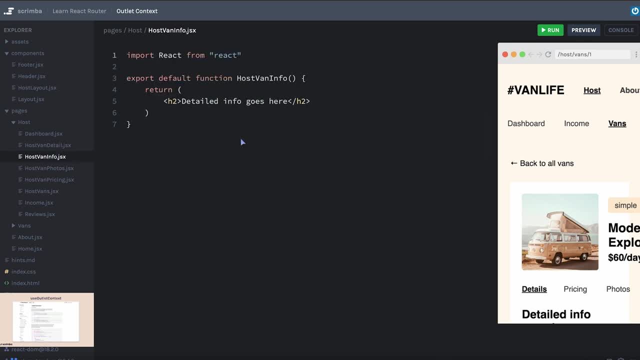 context prop will be receivable in my other components using a hook called use Outlet context. So we'll just go ahead and import that here for now, And I guess, while I'm at it, I'll put this into my other components as well, since I'm going to need the Outlet context in each one. 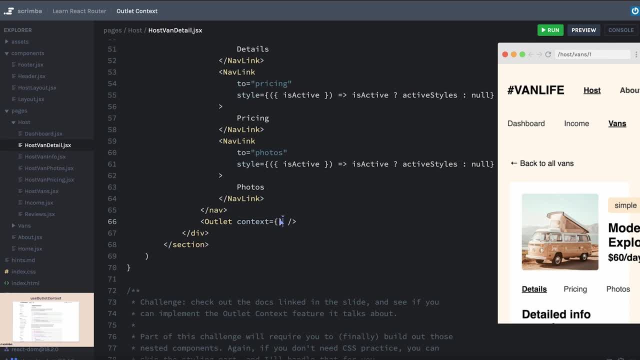 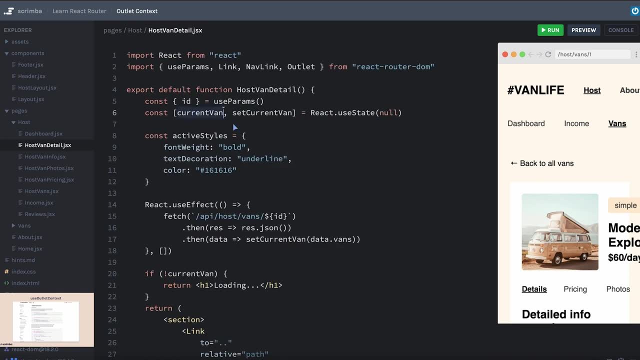 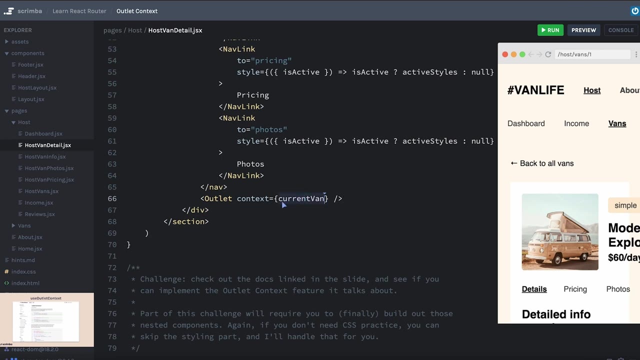 of these. Okay, let's actually pass something to our context before we go too far down that route. As I mentioned, we have the information in state called current van, So let's go ahead and just pass the context. So in this case, we're passing the van object as the entire context value. I guess what I could do. 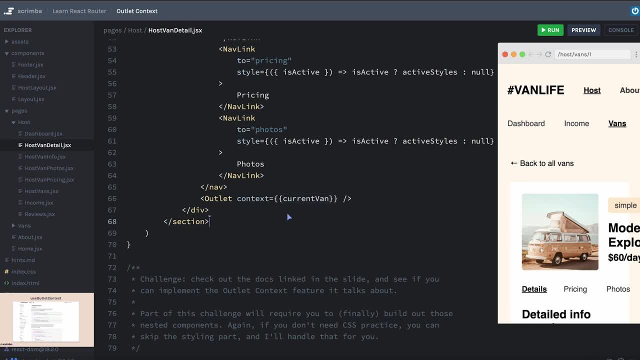 is surround this in another set of curly braces, which in this case means I'm going to pass an object and it will have a current van property whose value is the current van object. So this is the shorthand of saying this. I do tend to see something like this a little more frequently than 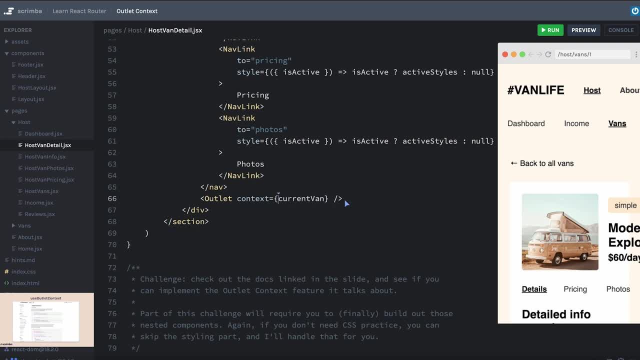 just passing the entire object by itself, with nothing else. So I think, just for the sake of sticking with the example that the documentation gave, I'll do it this way, which means when I'm receiving it in the host van info, we'll go ahead and say my const. 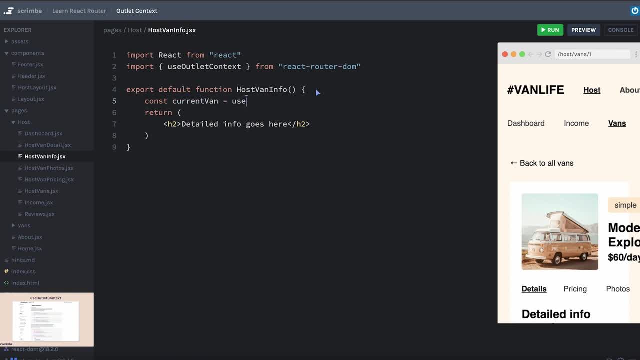 And I can't just say the current van is equal to use Outlet context, because current van is an object that has the current van property, So I can just destructure that right in line. while I'm doing that, Again, we'll go ahead and copy this into our other components. And now I 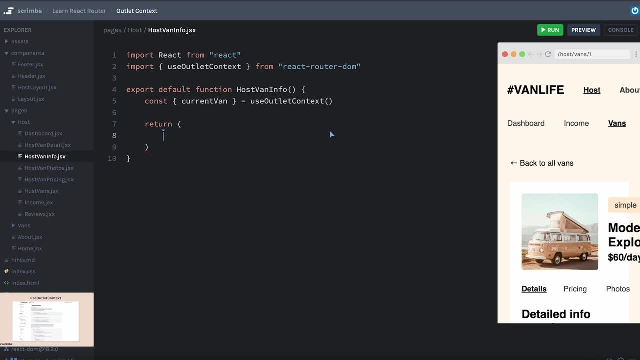 should have access to my current van So I can render- let's go ahead and create a section And let's- I don't know- maybe render this as an h4, since we're pretty far down this nested route that we have going here And we're going to display the name And I can access that with current van dot. 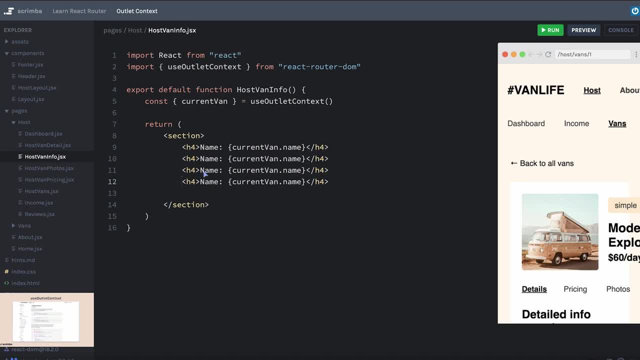 name And actually these are all kind of the same. If you look at the design they're the same level of typography. So we'll just use h4s for everything. say the category is current van dot. I guess type is probably should say type instead of category. That's all right. We'll say the. 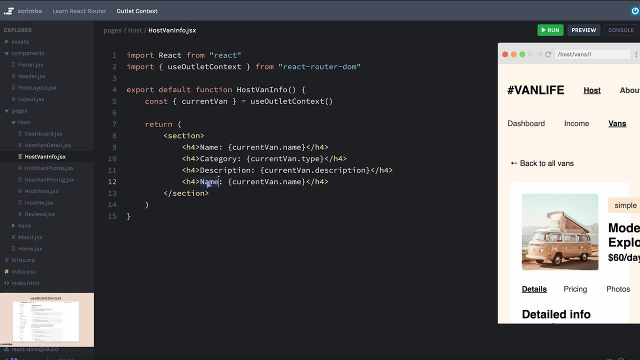 description is current van dot description And well the design has go back here. visibility public: that's not actually part of our current van, So we'll just kind of hard code that one visibility public. hopefully that didn't throw anybody off too much. looking for the visibility. 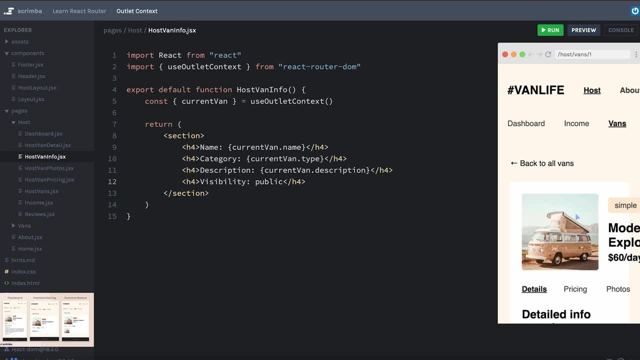 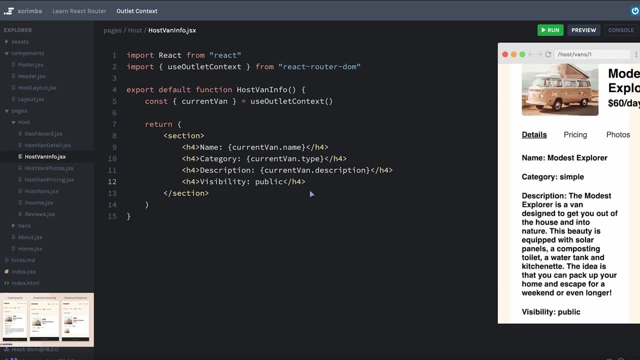 information inside the current van. I'm really sorry if it did, Okay. well, the route we're in is the detailed info, So let's hit save, scroll down And awesome. Okay, if we have some styling work to do, I'm just going to handle that for you. Okay, easy enough. 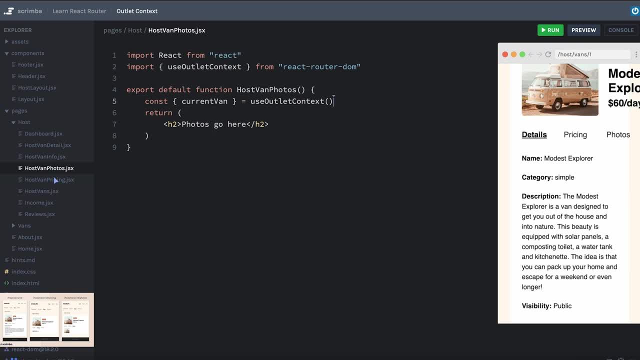 Now I should be able to just go to the photos and the pricing and do exactly the same thing, So I won't make you sit and watch me do all that. Okay, and just like that, we're rendering an image where we're pulling in the current van dot image URL. we'll hit save. 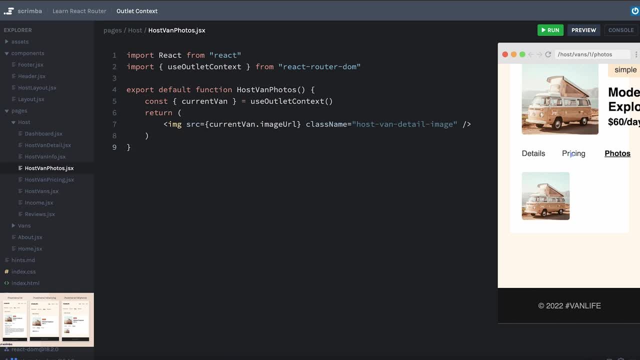 and go over to photos. Perfect, Of course, if this were a real site, we'd probably have multiple photos, But we're not going to worry about that because it doesn't pertain strictly to react router. Okay, and I will just do the same thing for the pricing. Okay, let's hit save. 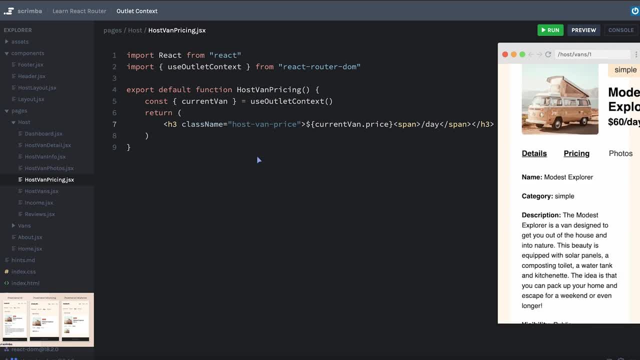 we'll go over to pricing And perfect. We have covered a ton of ground here. I mean, look at the app that we've been building. we have three different levels of navigation. we've learned about relative routes, relative navigation links, And well, there's just too. 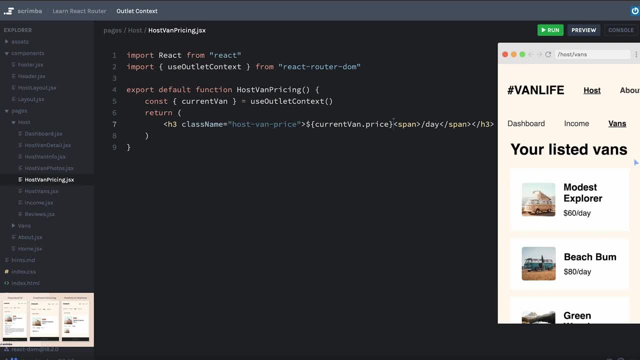 much to list. Assuming you've been able to follow along and do all of these challenges, you really should be super proud of yourself. Now we still have a couple features that I think would really be beneficial for us to add, And it's going to teach us a couple more aspects about. 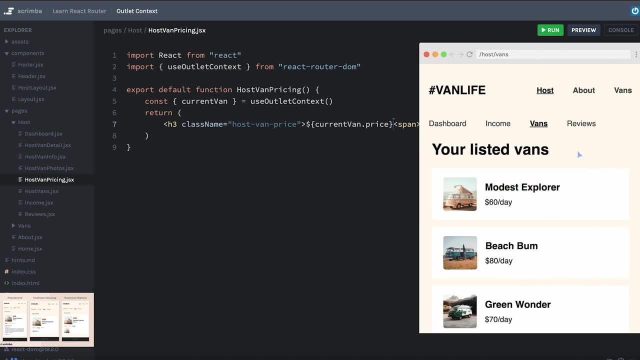 react router along the way, But this would be a great time to take a break, congratulate yourself, maybe show off all that you've been learning to a friend, And when you're ready, we'll move on to learning just a few more pieces about react router. This would be a great point in your 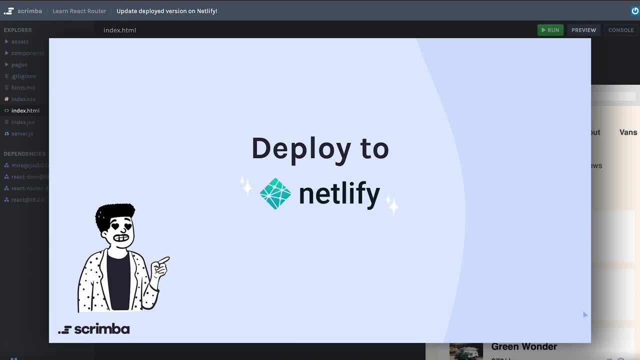 progress to update the deployment that you did to Netlify earlier in the course. we've got some great new features to show off And maybe you want to put it out on Twitter or share to some family or friends. So if you already feel comfortable deploying the updated version, 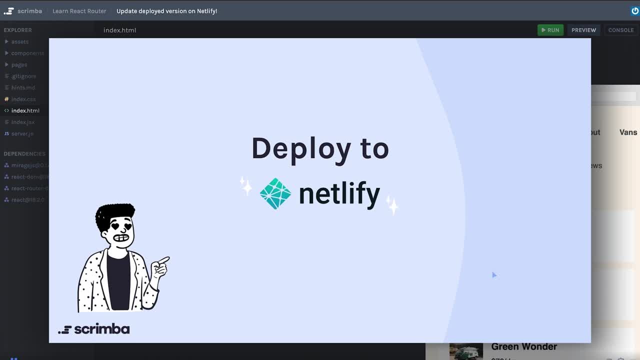 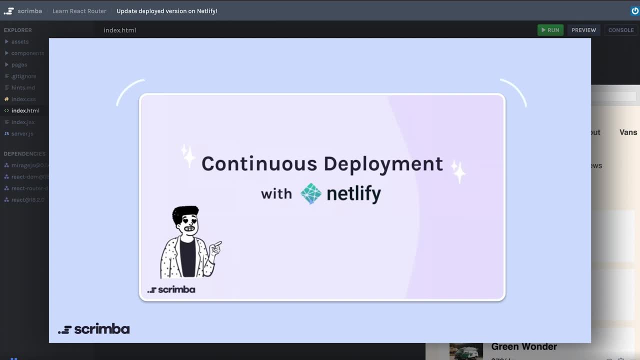 of your site to Netlify, then you can just skip this entire lesson. If, on the other hand, you have not yet deployed anything to Netlify, I have a link here to the original scrim back from the beginning of this course that talks about how to set up your Netlify account, how to push. 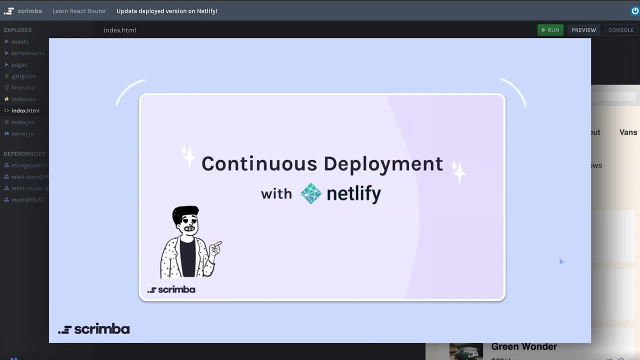 everything using Git and GitHub, with GitHub desktop and everything you need in order to get your site live. you can click the screenshot here, which will take you back to that other scrim showing you exactly how to do that process, And what we're going to do is going to be very similar to that. First, we're going to commit. 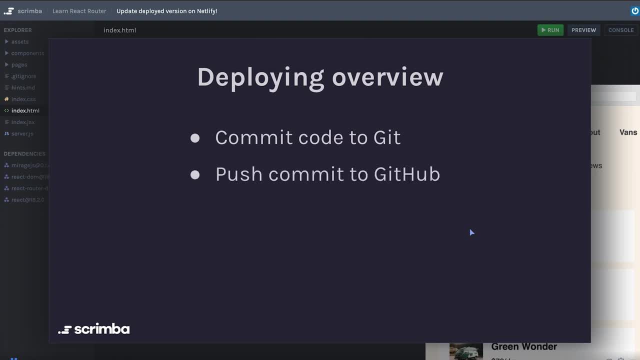 our local code to get, then we're going to push our code up to GitHub and Netlify will just automatically handle the rest. And, assuming that you already have an existing Netlify project that's connected to the same GitHub repository and you haven't deleted that folder or the GitHub- 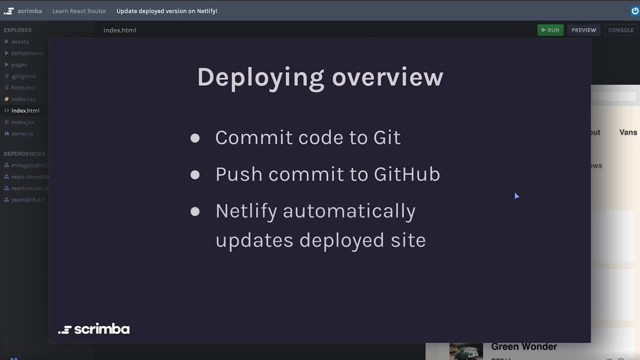 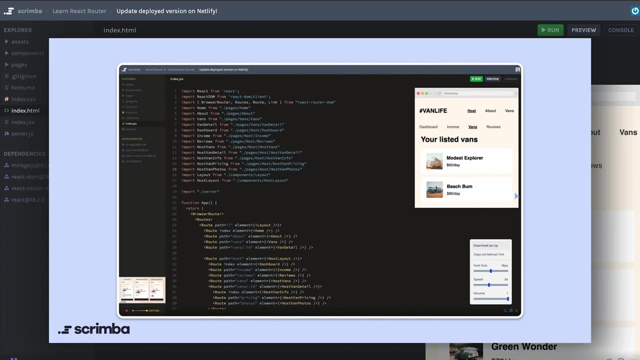 repository from before. then Netlify will just automatically update everything for you Now because we're here on scrim but when you first downloaded the code in the earlier part of the course. we have diverged since then with our code by writing a bunch of new code just here on. 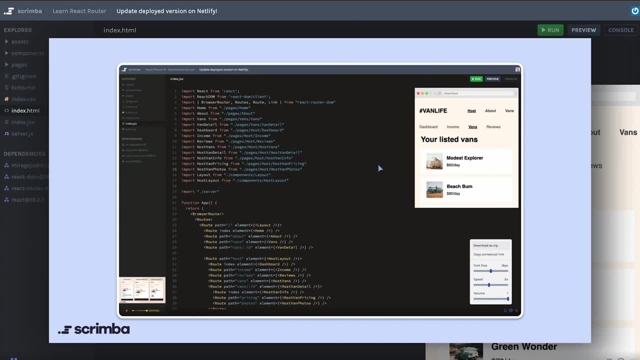 scrim, But so the first thing we need to do is download this entire project Again in the current design of scrim, but you can find that with the gear icon in the lower right a menu will pop up and you can click download as zip. Once you download that zip file and unzip it, 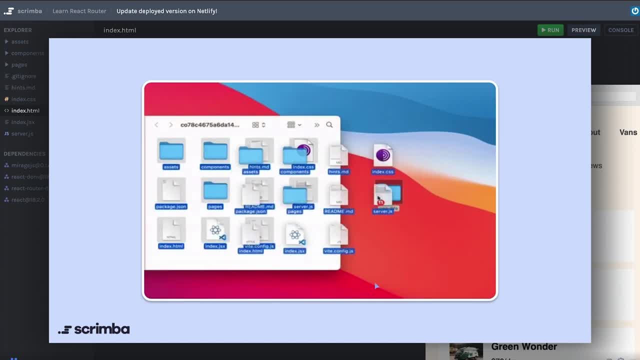 you will have all of your files from the project that we have, And what I'm doing here in this GIF is just dragging everything over to my existing van life folder, replacing all of the files from before. Now- something that's important to note: that doesn't. 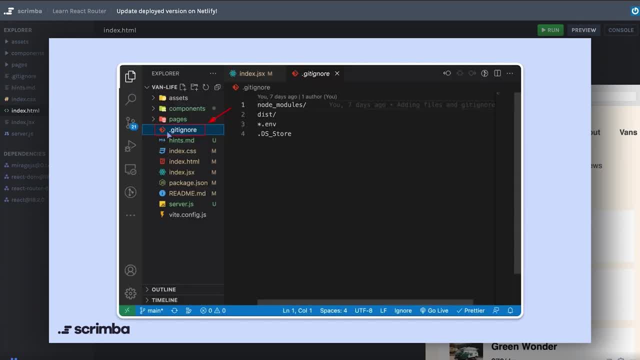 happen in this process is we are not deleting a hidden file called dot git ignore. So if you open the van life app with all of the new files that just replaced the old files, you should still see a file called dot git ignore with the contents that you see here. I've made sure that it's. 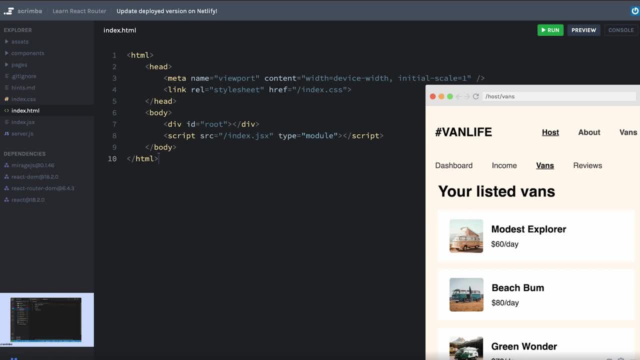 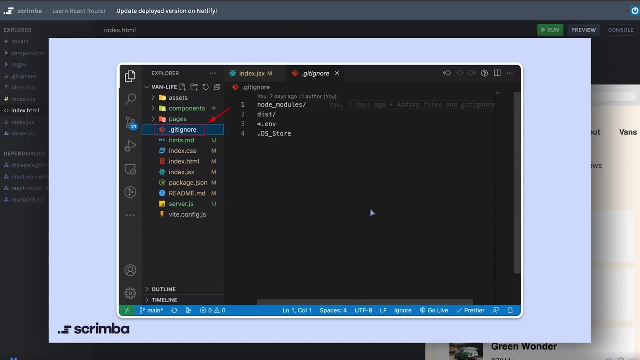 included here in the project, in case you downloaded the zip directly from this project, So hopefully that is still there for you and doesn't cause any issues. You can manually add this and that will work just as well. Then, if we open up GitHub desktop and we 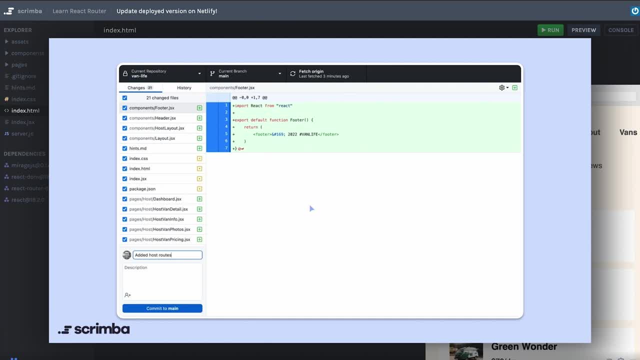 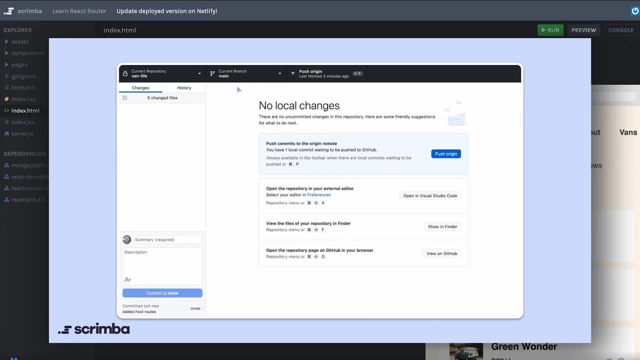 make sure that we're looking at our van life repository, we'll see the list of changes that happened. We can commit those changes by adding a message down here and clicking commit to main, which will then send us back to this state where we have no local changes And we can push our. 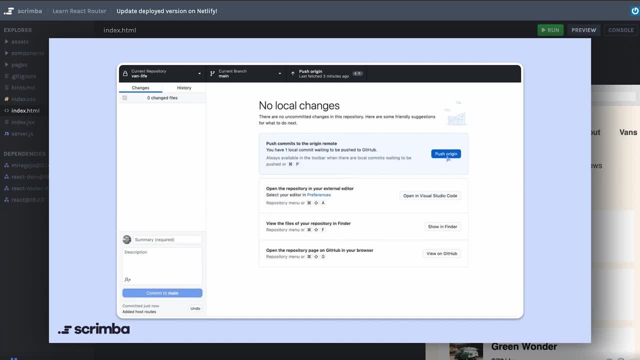 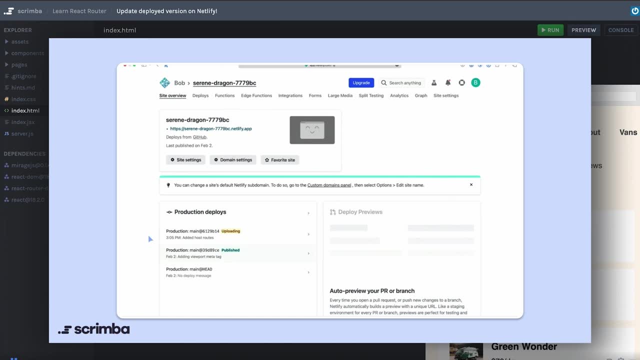 changes up to our GitHub repository by clicking this push origin button. As soon as you do that, Netlify is going to see that there has been a change on your repository and it's going to upload the new version, build it and deploy your site so that it's live for anyone to see. 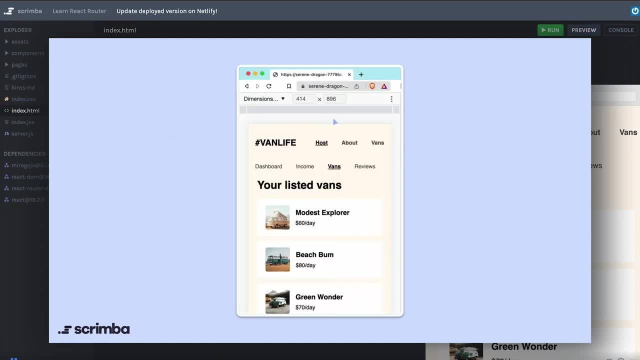 You can click on the link up here, which will then take you to your site, and voila, everything is ready to share, Just like before, if you'd like to share it out to Twitter. I think it's a great idea to build in public and to share your wins with the world. 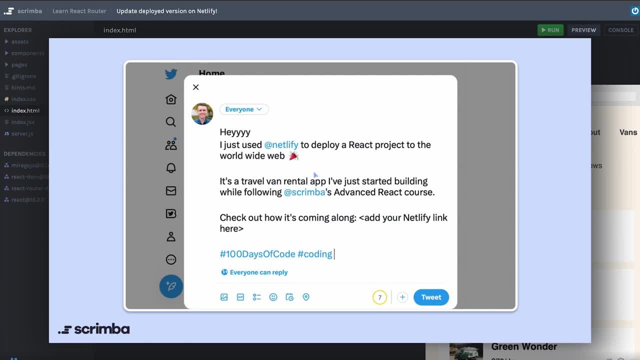 So if you're active on Twitter, you can click this screenshot, which will pre-populate a tweet for you. Of course, you can change it however you want. especially make sure that you add your custom Netlify link right here at the bottom of that. 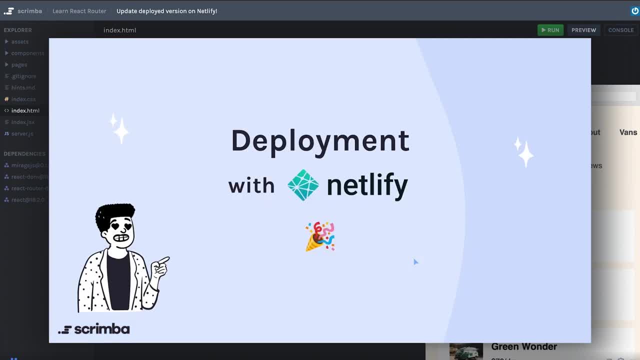 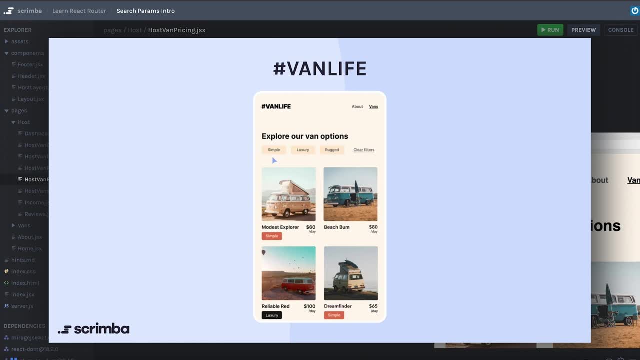 link, And that's it. Now we're ready to continue working on our van life app. You may have noticed that we completely skipped adding this filtering section on our vans page. This is the list of all vans, not just the host vans. In fact, you can even see: 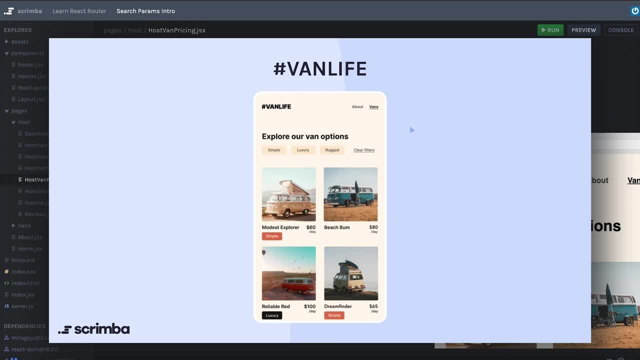 this screenshot doesn't yet include the little host link up at the top. In fact, you can even see that this screenshot doesn't include the host link that we added to our navigation bar. But don't worry, we didn't forget to do it, And now it's our time to tackle this feature. 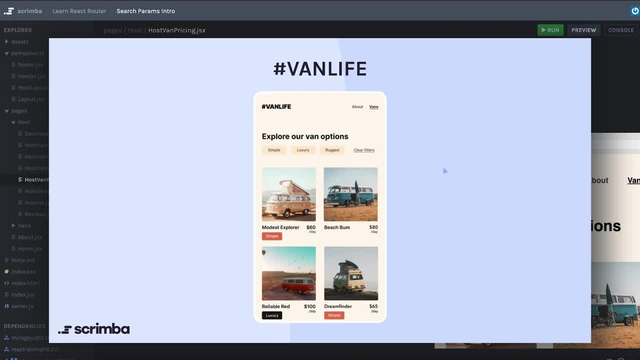 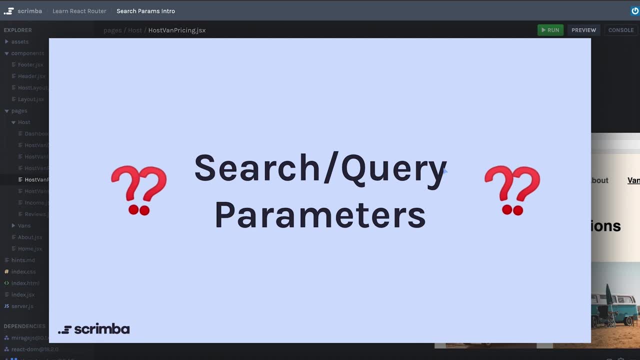 The reason we put it off till now is because it will require us to learn about something called search parameters or query parameters. I pretty commonly hear it called both of these things, so I just put search slash query parameters, because you'll hear spoken both ways. Let's talk for just a minute about what query parameters are. 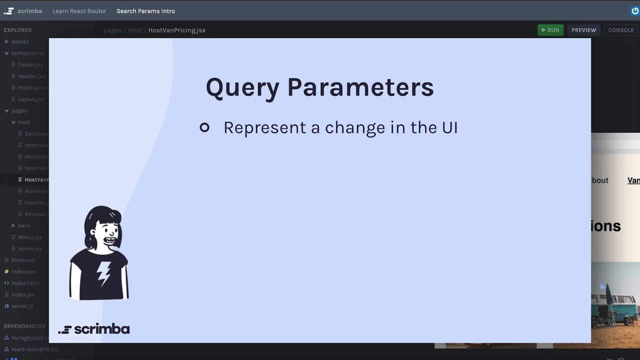 The idea of a query parameter is that it can represent some kind of change in your user interface- what you actually see on the page in your app. Probably the most common tasks for query parameters are something we call query parameters. The average process in your app is just width and 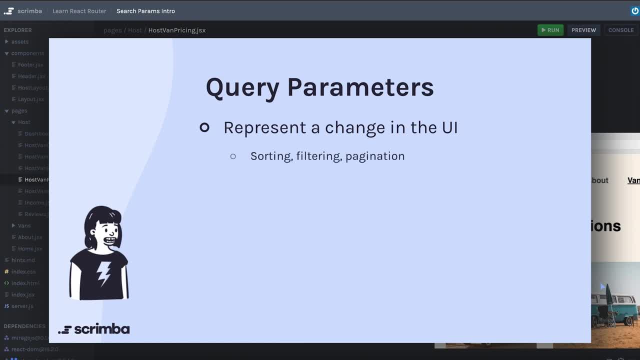 action, The VNs, the values, fields, tags and settings are ultimately based onares And the parameters are whenever you need to do any kind of sorting of your list or filtering of something on the page, or if you have a ton of results and you need to do pagination. We have a pretty limited 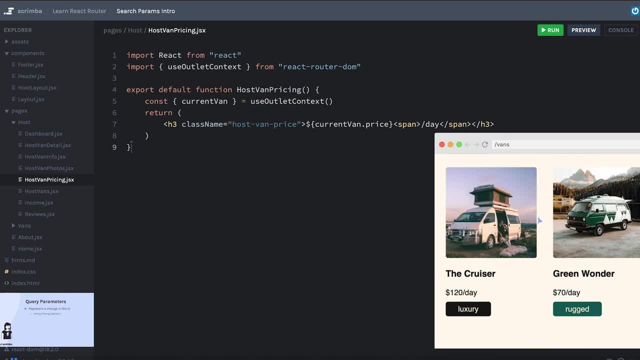 selection of vans on our site. but if we had, say, 2,000 vans that were listed, we might want some kind of pagination that said we only show 10 results at a time and the user can click through the pages to see more. Pagination like that and the kind of filtering that we're going to be. 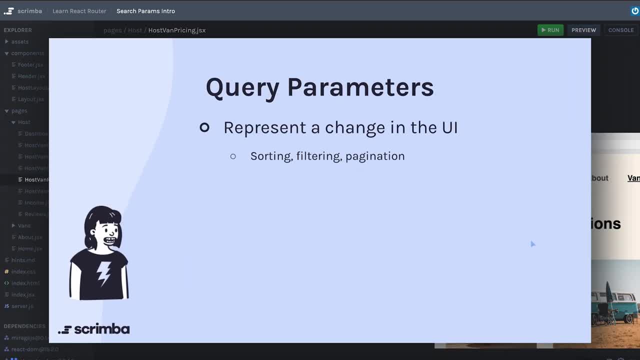 working on in this app usually happens within a query parameter. We're going to see in just a second what that actually looks like and how you implement it, but for now we're just talking about the theory. A really helpful way that I have found to think about query parameters is to think of 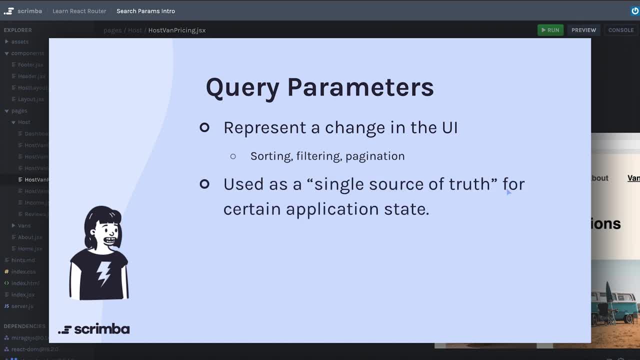 them as a single source of truth for some of our application state. I've talked about this before in another React course that I've created, and the idea is that it can be really important to ensure that the state you're maintaining in your app. 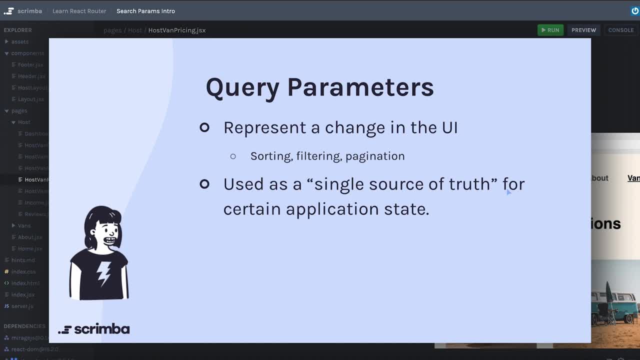 no matter how much you're working on, it is the same as the state you're maintaining in your app, No matter where that actually is happening, has a sort of central hub that we call the source of truth, so that everything else just derives the way that it looks, based on that single source of. 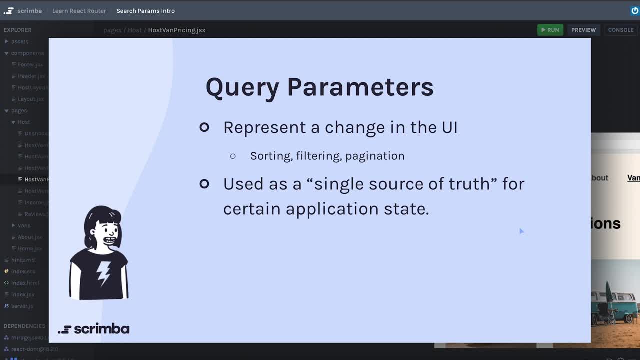 truth. Some examples of this might be something like React state or local storage or, as we're seeing here, the query parameters that are in your URL. Or you might be using a third-party library like Redux, where that single source of truth is maintained in memory, in a Redux store, for example. 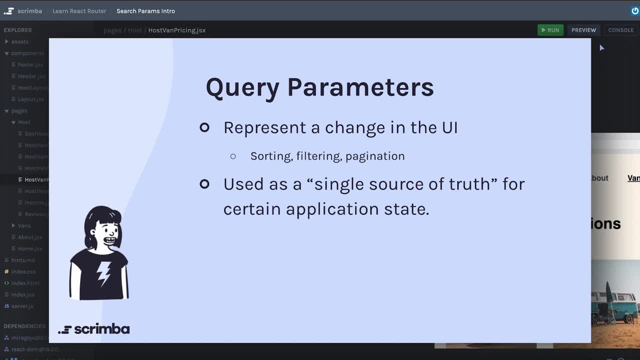 So, like I mentioned, sometimes query parameters, which will exist in the URL, can be used as a single source of truth for parts of your application state. A really helpful metric that I have used is to ask myself should a user be able to revisit or share this page exactly like it is and have 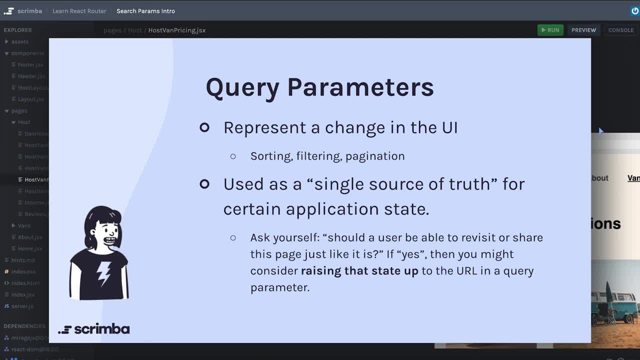 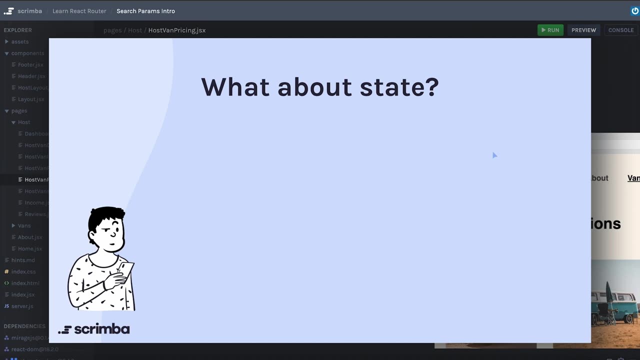 the experience be the same, or rather, have the results be the same? If the answer is yes, then it might be worth considering raising the state of our filtering or sorting, or pagination, or whatever it might be, up to the URL in a query parameter. So you might be thinking: well, what about React? 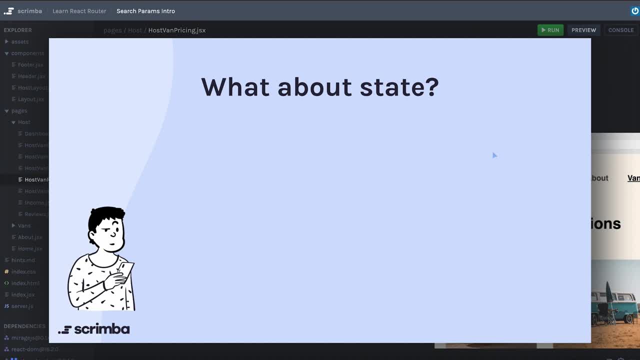 state. Maybe you've even done some filtering or sorting, or maybe even pagination, using React state as the single source of truth. Something you've probably noticed about React state is what happens when you refresh your page. In fact, I want you to think for a second. what does happen? 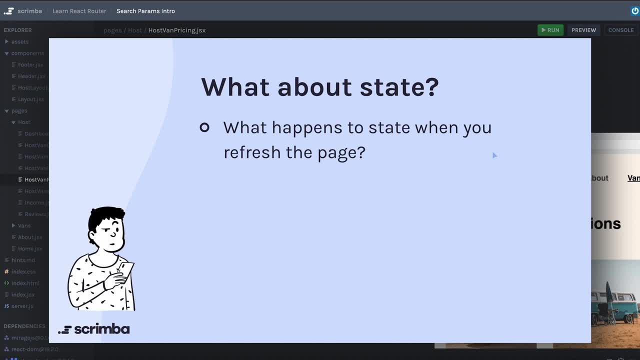 when you refresh your page. Say you're maintaining a counter and you've clicked the button seven times, so the count is currently seven, and then you hit refresh, What happens? The counter resets to whatever you initialized your state as Hitting refresh on your. 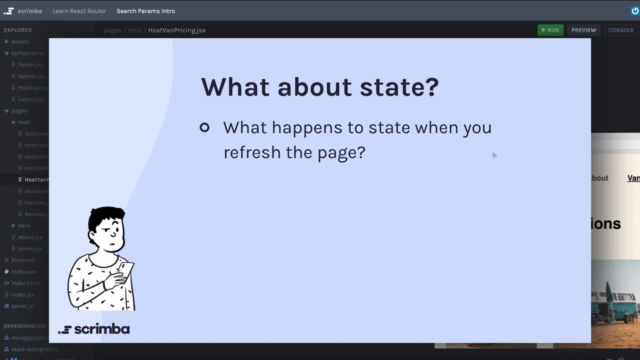 browser is akin to loading the app up for the first time. So, assuming you initialized your counter at maybe zero, when you hit refresh your counter is gone, your state is wiped away and everything starts fresh. As such, can you share the current state using React state of your app with a friend? 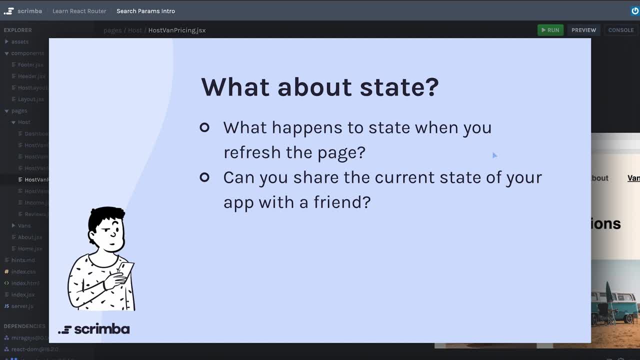 Well, no, If I had a counter app and, for some reason, I wanted to share the current count with a friend, and I wanted to share the current count with a friend, and I wanted to share the current count with a friend and I. 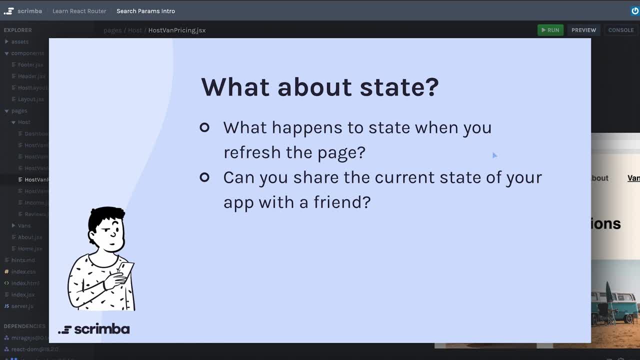 copied the URL and sent it to them. when they load it up it's going to be fresh state for them in their browser, So it won't include my count that I saw on my end Maybe a more realistic example using our van life app, if we maybe had four different filters and some. 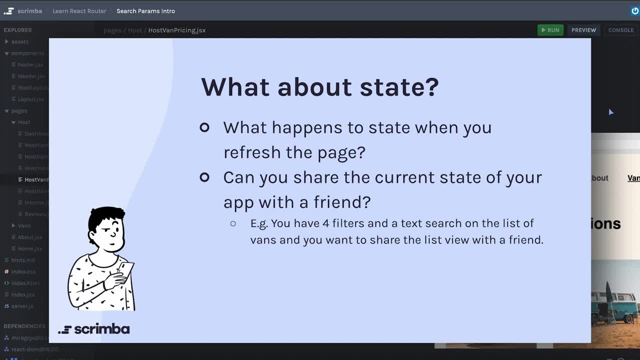 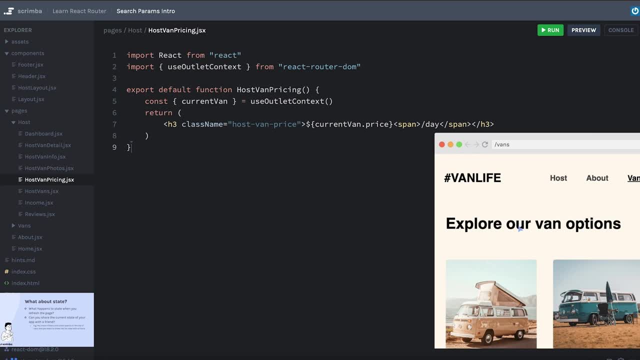 kind of text search or maybe even a location search, like if we wanted to only see the vans that were in our vicinity so that we could easily go pick them up. that might be part of the filtering that we're doing on our list of vans. So then let's say I want to. 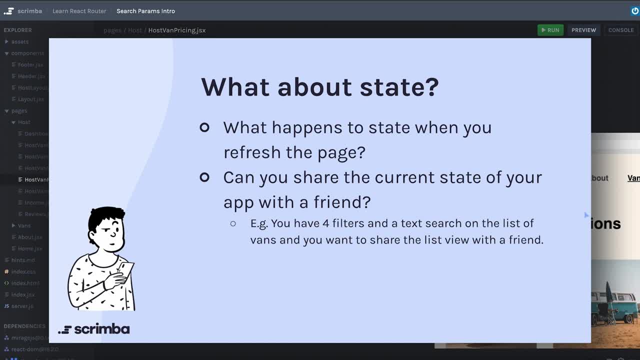 take that list that I've curated through my filters- text search, location search, whatever it might be- and share it with a friend. Well, if I'm holding all of that state in React state, I really can't do that in a meaningful way, at least not without some kind of crazy work. 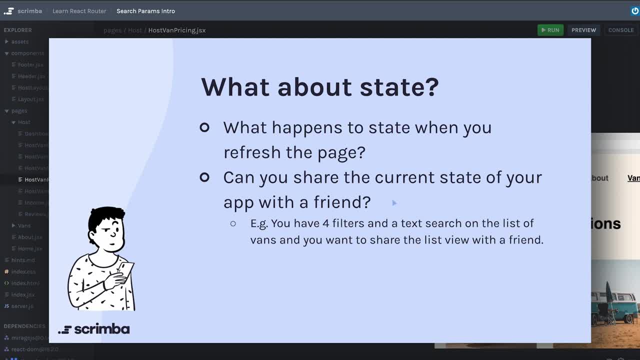 around. So this would be a great example where the state of my filters and text search and whatever else it might be, might be better to raise out of React and up into the URL. In reality, React Router is handling our URL, but it's not going to do that, So I'm just going to 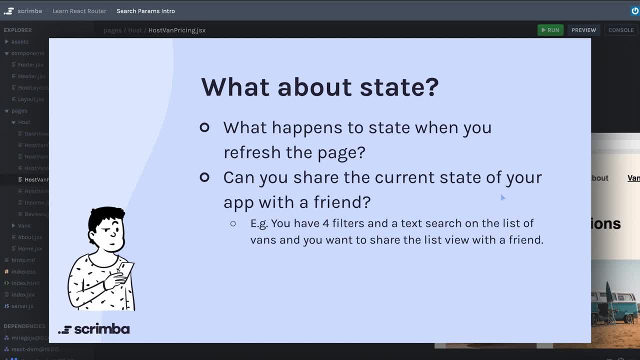 take the state of my filters and text search and up into the URL. and I'm going to take the state of my filters and text search and up into the URL, but under the hood, it's using the native browser APIs that are dealing with the URL. 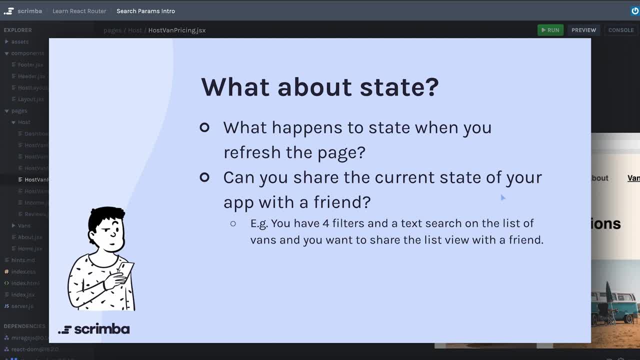 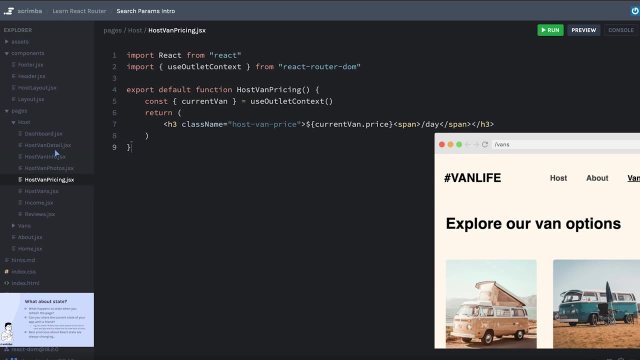 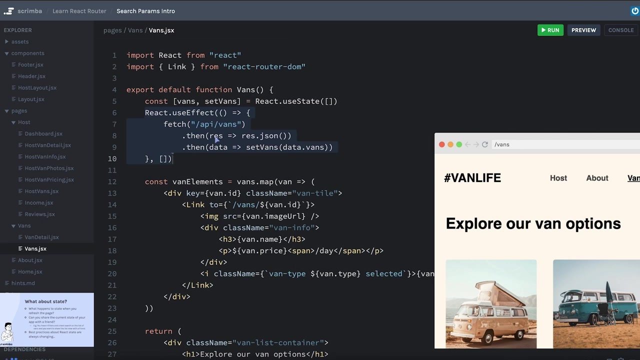 Now one thing that I've noticed over the last year- maybe two years- is that the best practices about using React state and actually about using other parts of React, like use effect. they're always changing. In fact, later in this course we are going to see an example of how we're not even going to be doing our fetching of our- let's see where do we have our vans here. we're not even going to be doing our fetching inside of a use effect and saving the 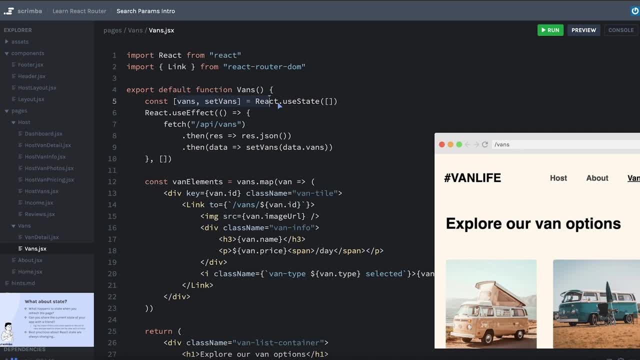 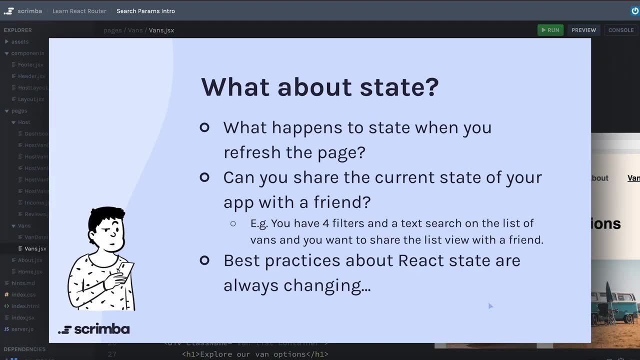 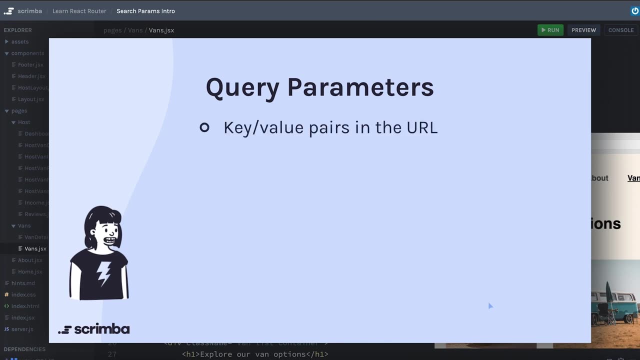 results in state, which might seem crazy. That might be the only way you've ever done fetching, but there's some serious drawbacks to the way that this is happening. Anyway, we're getting down a rabbit hole, So let me bring us back. We'll see really quickly how query parameters are actually structured. As I mentioned, it's part of your URL and it represents key value pairs of information that can live directly in your URL. 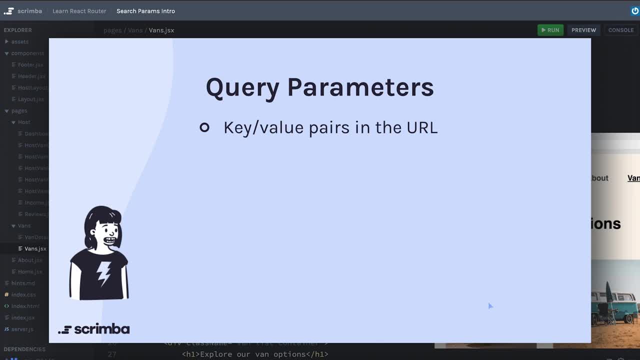 I'm almost certain you will recognize this pattern. You create query parameters by first starting with the question mark. So in our app, if we have slash vans, we would include in the URL a question mark and then we would associate some information, like the key of type. we would set it equal to a value of, in this example, rugged. 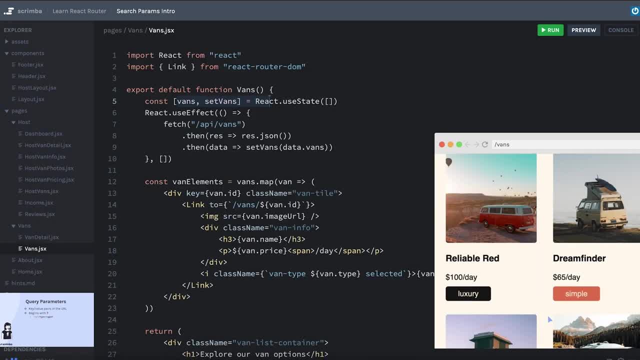 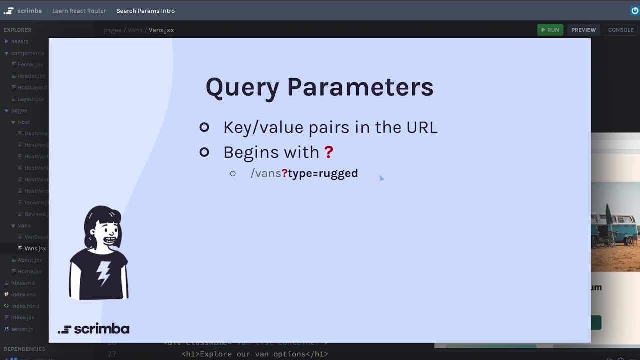 Remember, all our vans have this kind of type here. that's simple: rugged and luxury. Well, if we only wanted to see all of the rugged vans that were available, then we might include a query parameter where the type is equal to rugged. 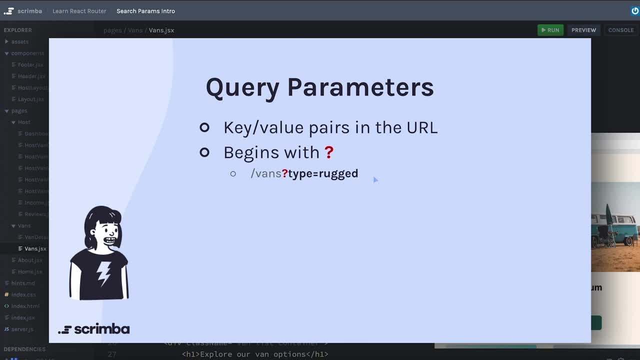 And there's nothing that stops us from having multiple query parameters. And there's nothing that stops us from having multiple query parameters. And there's nothing that stops us from having multiple query parameters. You may have seen URLs that were extremely long, I think. if you go to Amazon, any product page that you find will have a really long URL And if you look at it, it will have a number of different query parameters. 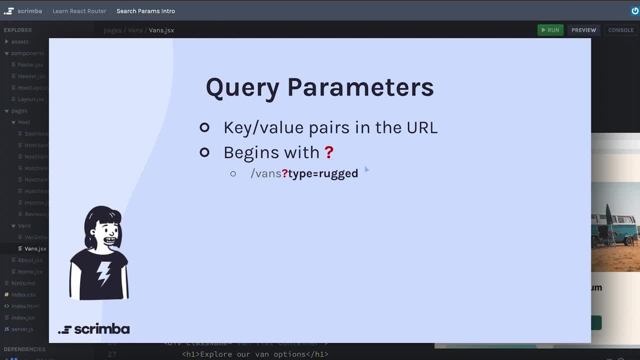 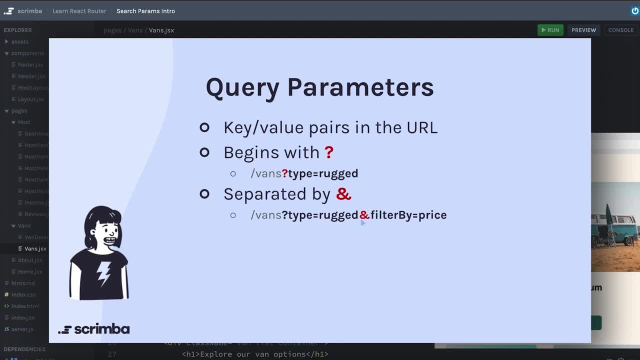 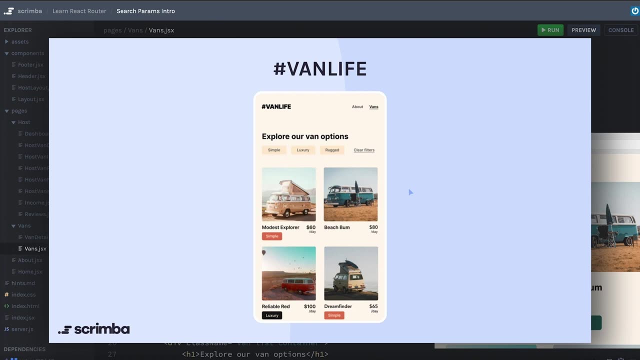 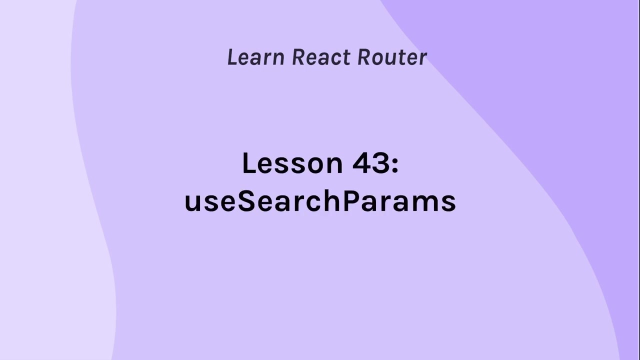 So, for example, if we wanted to filter by the type of rugged but also filter by price. So, for example, if we wanted to filter by the type of rugged but also filter by price, In order to handle search parameters in a React Router app, we're going to use a hook. 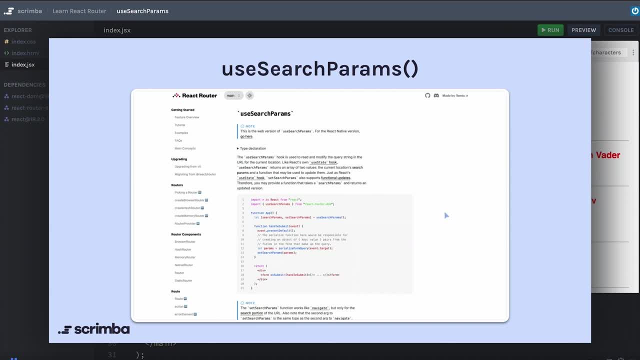 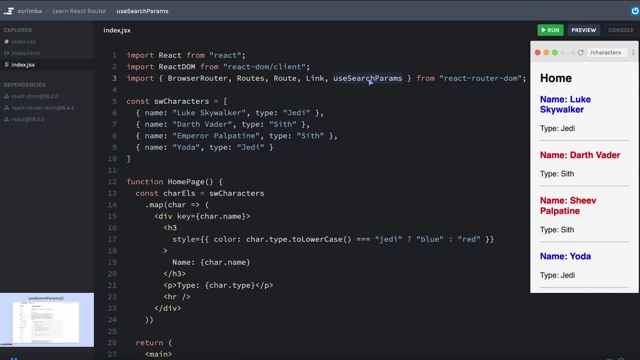 called useSearchParams. You can click on the screenshot here to go directly to the documentation. One thing that's really nice about useSearchParams is that it is very similar to the signature of useState. Let me show you what I mean. So here we have a very simple app that has a list of Star Wars characters. 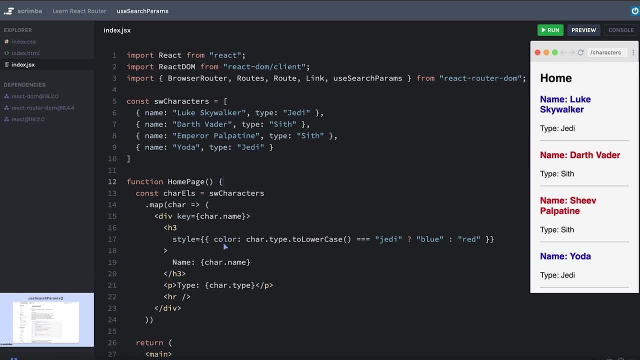 They're either Jedi type or Sith type. We have some conditional styling happening where they're either blue or red, depending on their type, And our goal is to make a couple buttons, So one will say Jedi, one will say Sith. Clicking them will add a search parameter to the URL, which will then make it so that 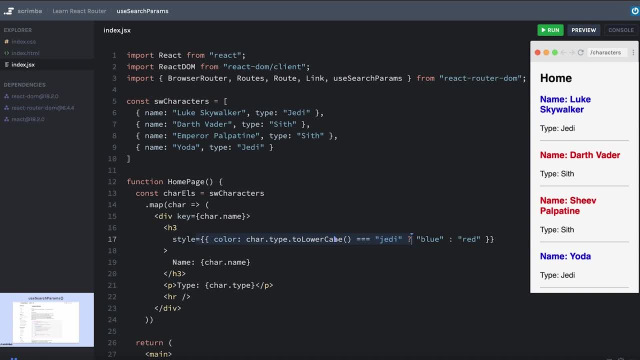 it filters this list and only shows either the Jedi or the Sith. To start out, we can use the hook for useSearchParams. We'll just do it here. at the top of our component We can say const, and then we will destructure an array that comes back by calling. 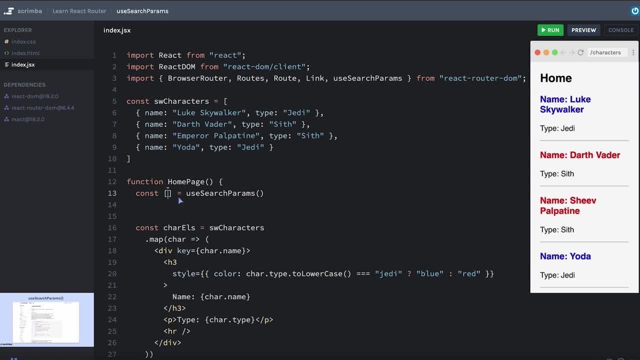 useSearchParams. Just like in useState, we will get back the value of the params we're creating. So we'll call it searchParams, And that's in the first index of the array that we're destructuring. And the second thing we'll get back is a setter function, just like in useState. 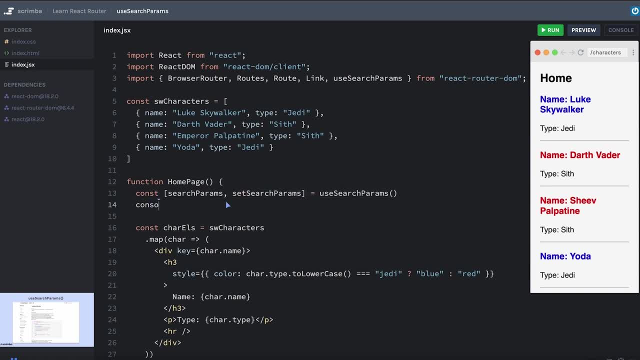 So we'll call it setSearchParams. Let's go ahead and consolelog searchParams And let's see what we get. Okay, so this is not just a regular object or a string or anything like that. It's actually an instance of the browser name. 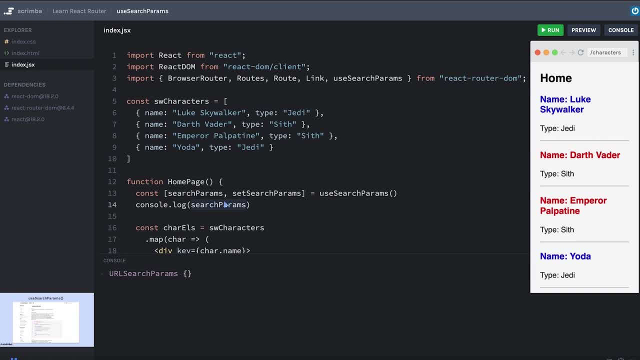 It's a native URL search params object. Because of this, the search params object that we have here actually has a whole set of methods that we can make use of when we need to, And if you're interested, you can go look at all of the methods in the URL search params. 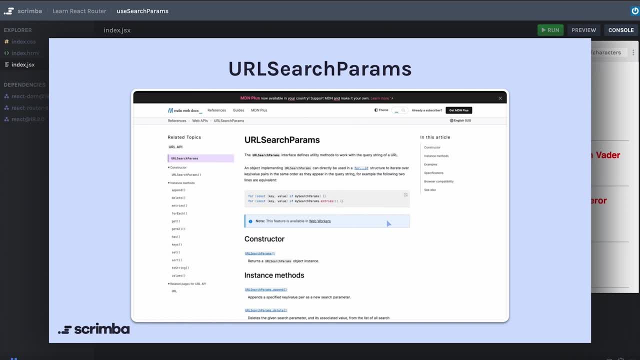 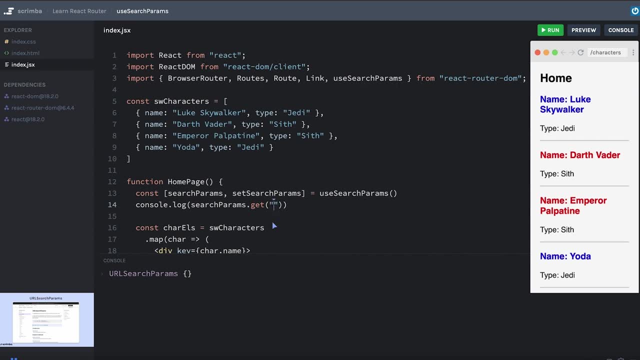 documentation on MDN. You can click the screenshot here to go there. One of the methods that is very useful is one called get, And we can provide the name of a key in a key value pair for our search parameters and it will return the value of that parameter. 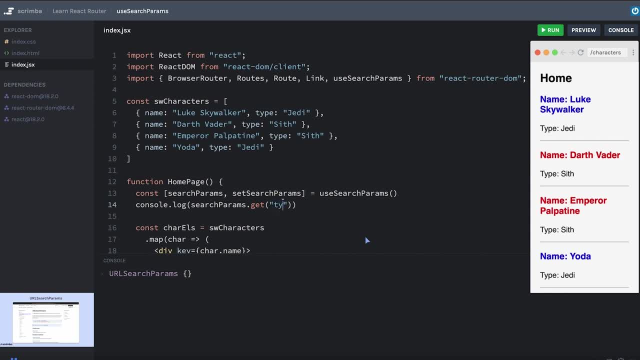 So, for example, we are going to be using a parameter called type And so if we say search params that get type, it will return that, and then we are going to console log whatever gets returned, or rather it will return the value of that. 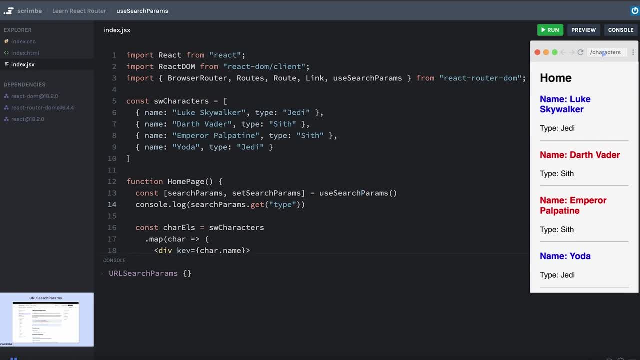 So I'm going to hit save, But I want you to take a look at what is currently in our URL and determine what you think the console log is going to return. Well, we currently don't have a query string in here, So let's go ahead and hit save. 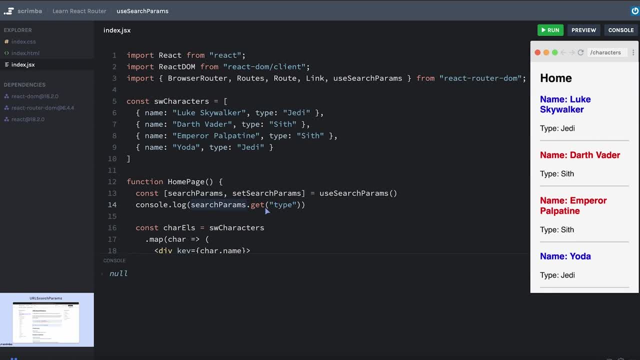 And it looks like from the search params object: When we try to get the parameter Of type, the value is null. So let's go ahead and actually put a question mark and we'll say: type equals sith. We'll hit enter. 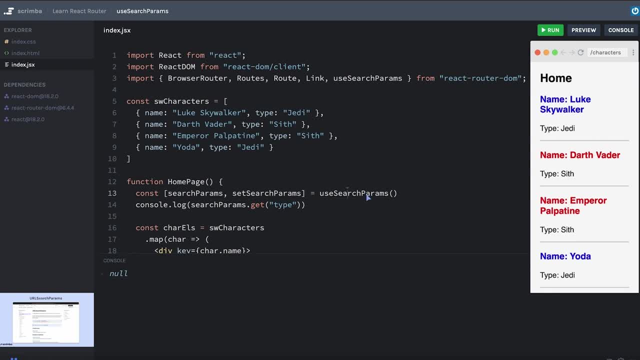 It should rerender our component and we'll see if our search parameters are working. Okay, look at that. When we console log the search params that get type, we get the value of sith. If we want a more full picture of what our search params are actually containing, at any 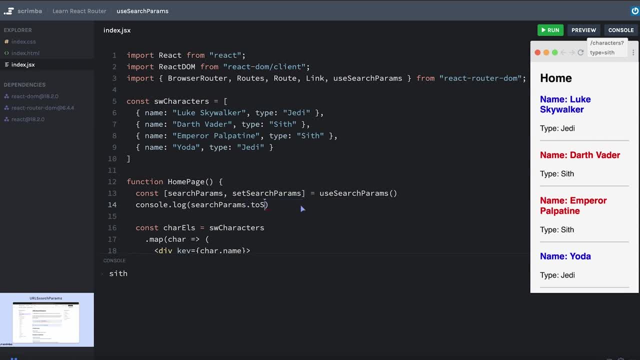 given time. we can use a method on the search params called toString And I'll hit save. Let's see what that does. And we get type equals sith. Remember we can separate the parameters with an ampersand, So if I had another one like and scrimba equals awesome, and that needs to be equals, okay. 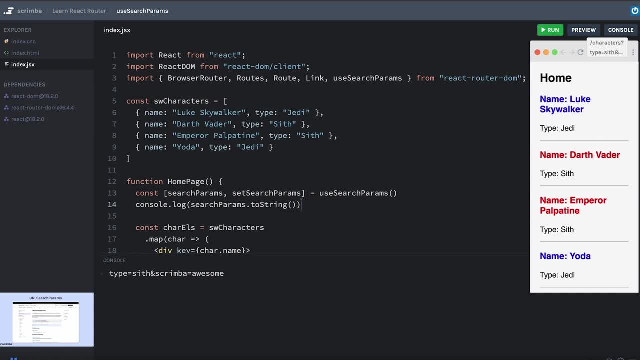 we can see that the search paramstoString will return the entire query string. It doesn't include the question mark in the beginning, though, So that's something to keep in mind. Okay, so we have a way to get me changes back. we'll say we want to get the type. 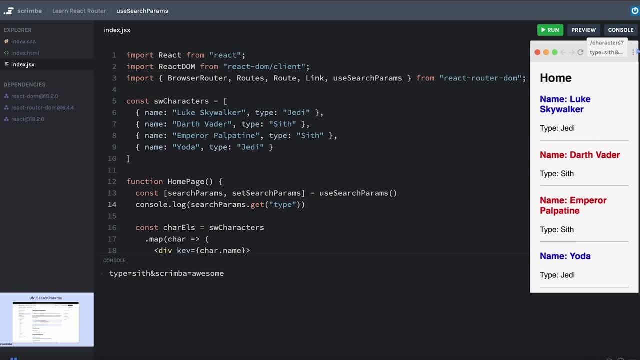 And I'll go ahead and get rid of. even though scrimba is awesome, I'm going to get rid of this other parameter here. Okay, we have a way to get the value of type, which currently is sith Soon, we're going to learn how we can actually set our search parameters so that we can change. 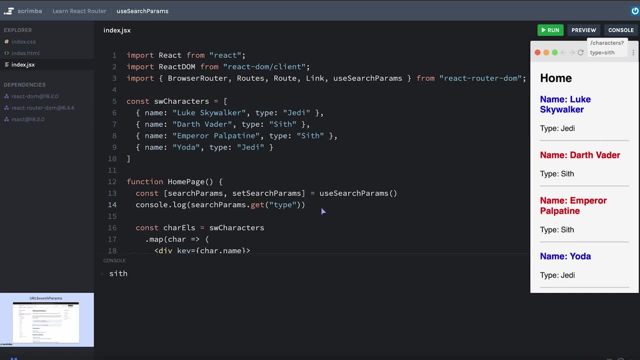 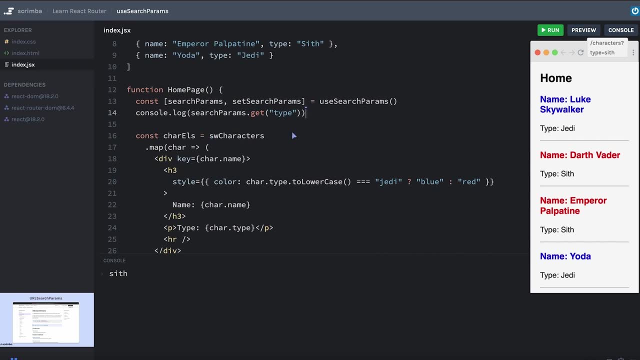 it on the click of a button. But before we even do that, I think it would be useful for us to use the value in the search parameter to filter down our list of Star Wars characters, so that it only displays the type that is in the search parameters at any given time. 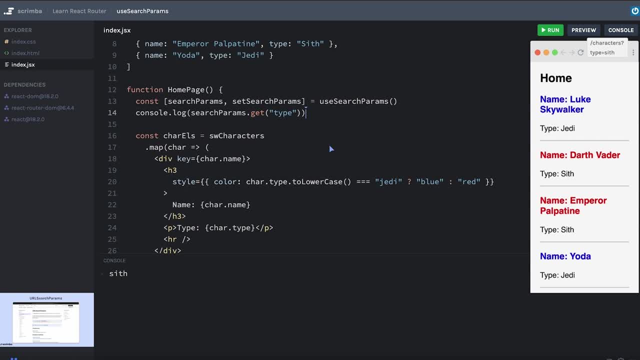 So that's going to be the next thing that we learn, But actually, at this point, let's get rid of this other parameter. Okay, we have a way to get the value of type, which currently is sith Soon, we're going to get rid of this other parameter. 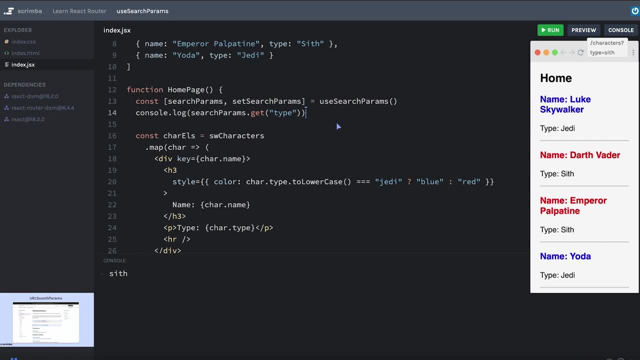 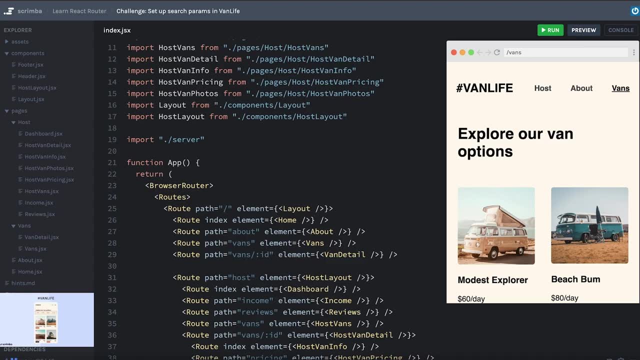 But obviously we have a way to get rid of this other parameter. So let's get rid of this other parameter. So we'll take the small portion that we've learned so far, we'll apply it to the VanLife app and then we'll come back to this and learn how to do the filtering. 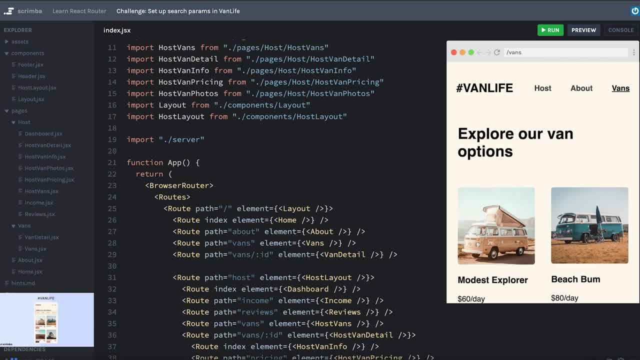 You know, sometimes when I'm watching a tutorial with somebody else doing all the work, I find myself getting lost a little bit in their code base. So this is a silly kind of intro challenge, But the first thing I want you to do is to try and figure out where it is we're going. 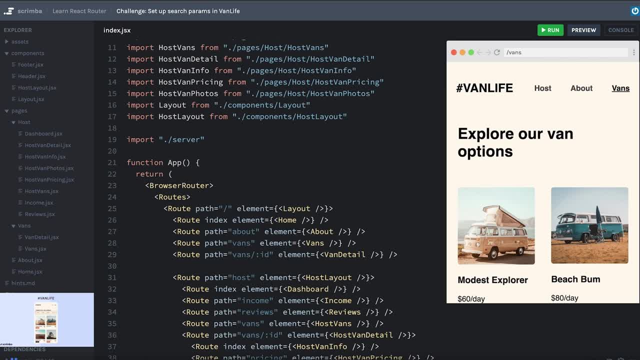 to be implementing this search params challenge. Remember, the idea is eventually we're going to get rid of this level in the search, going to add buttons here to our vans page so that when we click them it will alter the search params and filter our list so that it only shows vans of a specific type, Like we have the vans for. 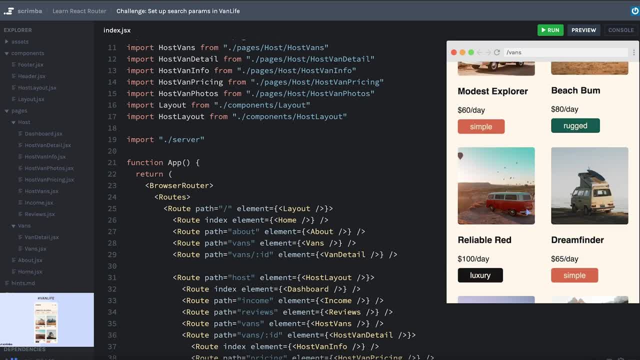 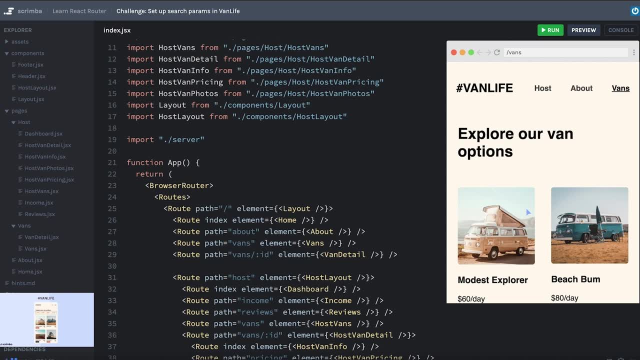 the simple, the rugged and the luxury types. So if you need to pause and find the correct file, you can do that, or you can just maybe say it out loud or something to show that you know where it is. we're going to be implementing this, So go ahead and do that now. 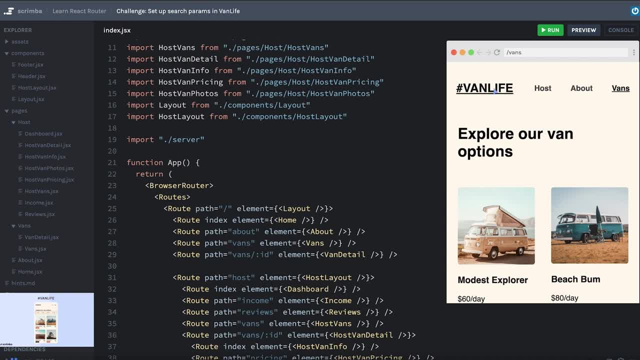 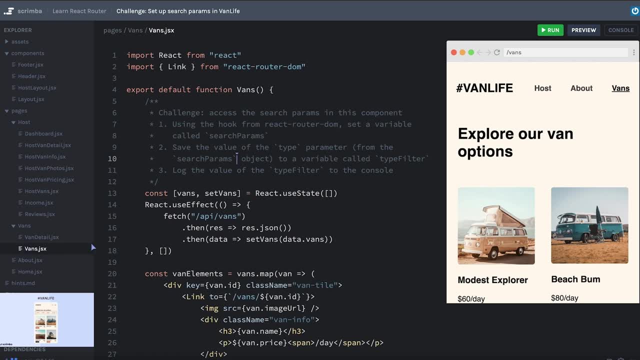 Because we are doing this work on the vans page. we are going over to the vans component here And hopefully you were able to find that or at least understand that that's where we would be doing the work. Again, the only reason I had you do that is because I know that for me personally, 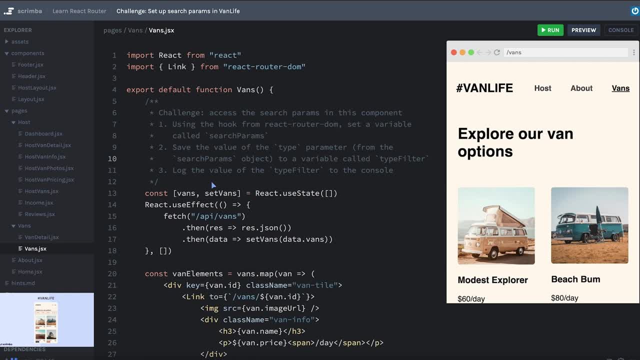 sometimes I realize I've gotten this far in a code base while watching a tutorial and then kind of realize I actually get lost in it pretty easily because I wasn't the one doing all the work. I guess that's a little different in this course because hopefully you've been typing along. 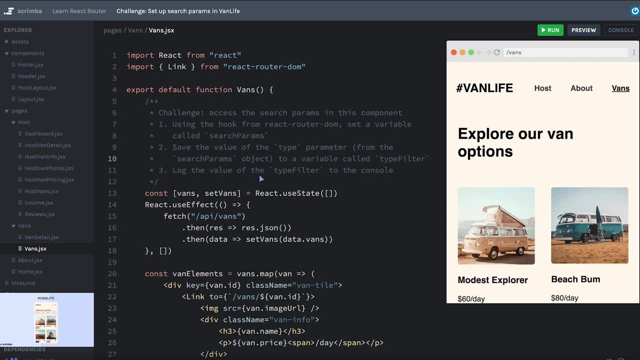 Okay. so we have our real challenge here, And that is to access the search params inside of this component. I guess an important distinction to make between what we're doing here with search params and what we have done in the past with state is to understand that state just lives inside of this component, whereas the search 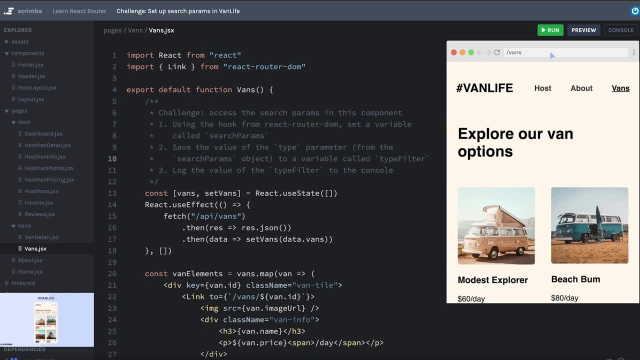 parameters. they're something that lives up in the URL. So even though we are going to be accessing the search params here in this component, we're not actually instantiating or initializing search params here. Instead, the search params variable is going to be the search params variable. 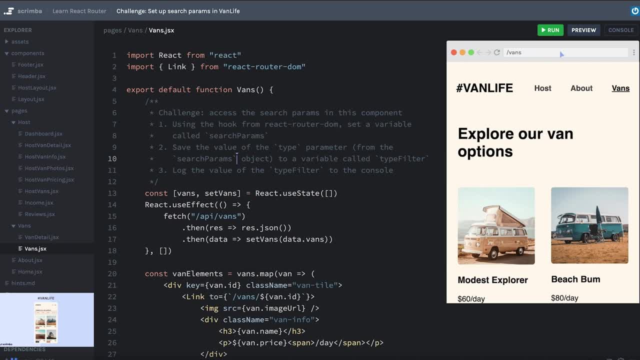 This is simply going to read the parameters that are up in the URL. we can modify the URL and we will be modifying the URL from this component, But it's a little bit different than states, and state is just living in memory for this component only. Anyway, I don't know if that clears anything up, or. 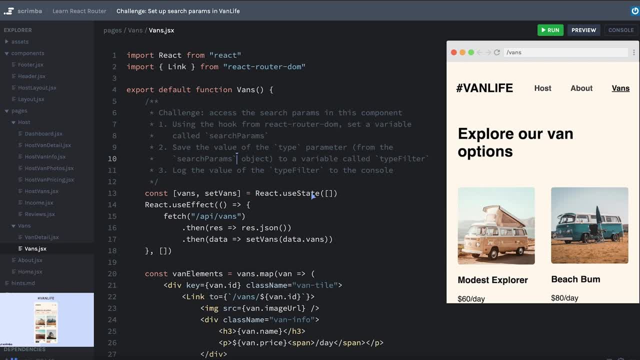 makes it worse, But hopefully that helps. So I've laid out some steps for the challenge. you need to use the hook that we just learned about from react router DOM, set a variable and use it to set a variable called search params. That search params object will have a variable called search params. 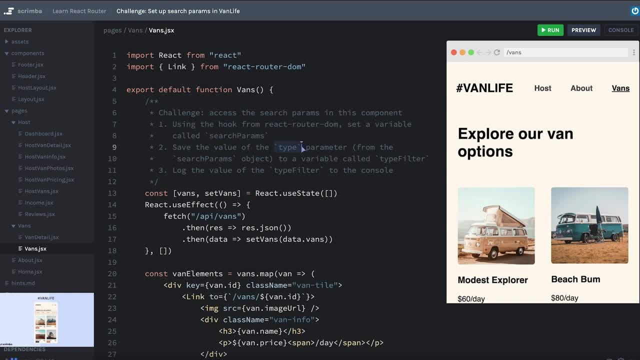 That search params object will have a property you can use to grab the value of the type parameter, And I want you to save that to a variable that we call type filter and then simply log the value of type filter to the console. Now remember, currently, as it stands right now in this recording, we don't 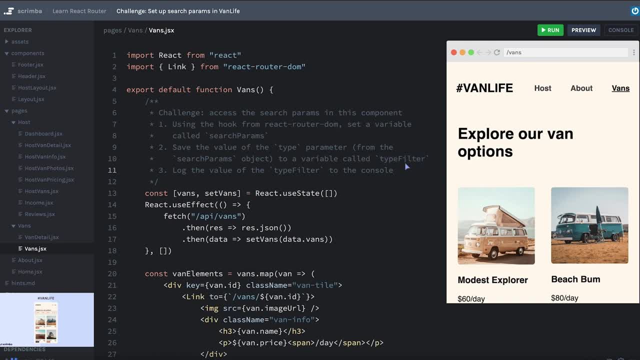 have a query up here. So don't be surprised if you get to the third step and you log the value of type filter and it isn't what you might think it would be. To test it out, you can simply type up into the: 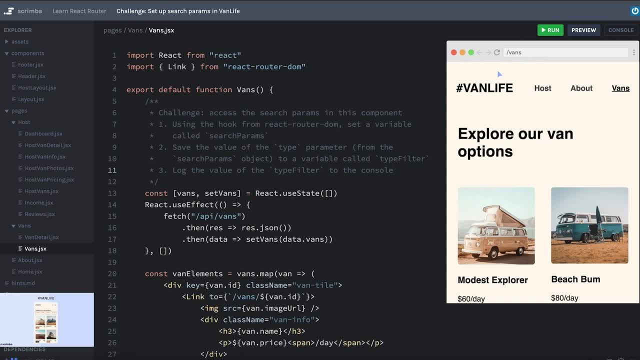 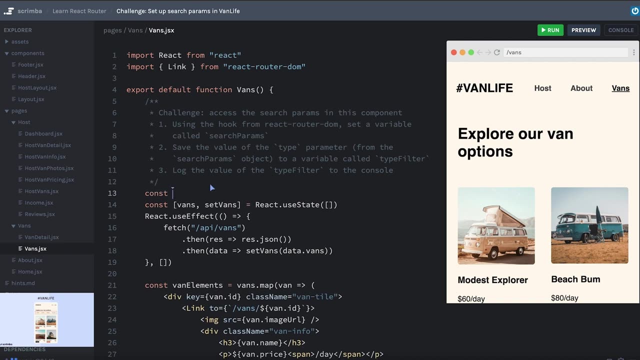 URL, question mark, type equals, and then whatever you want. All right, you should have everything you need. Pause now and work on the challenge. All right, let's get started. We will just do this right above our state declaration and we'll create a new. 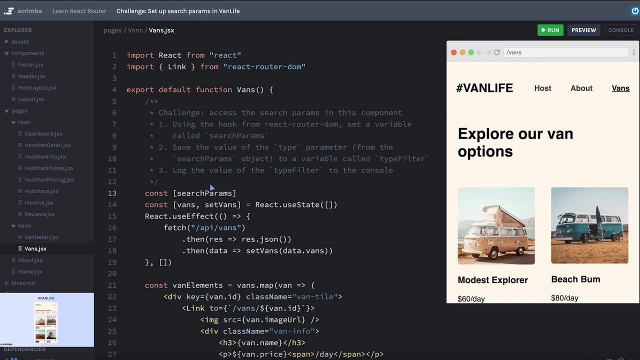 search params. object here, So search params, and we're not yet at the point of using set search params. but we might as well do it now because we know we are going to use it in the future. So we will call use search params And I need to import that from react router DOM. then maybe, right below our state, let's buy some. 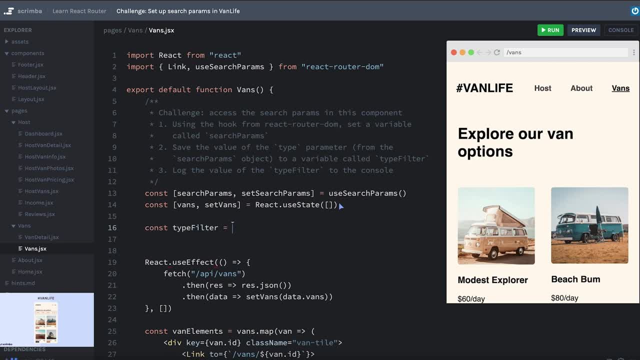 space here And we'll say: type filter is equal to search params, And remember, this is an instance of the native constructor URL search params. that comes with a number of methods that we just get for free, like dot get, and dot get is where we specify as a string the name of the key in the key value pairs of our search params, and it should. 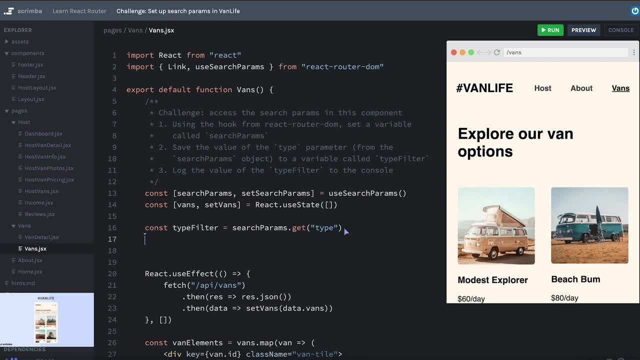 return the value At that key of type. So I'll go ahead and console log type filter. And again, because we don't have a query string in our URL, this I think will be null. is what we discovered. Yeah, so it's null. Now I can test it out by putting in the URL. 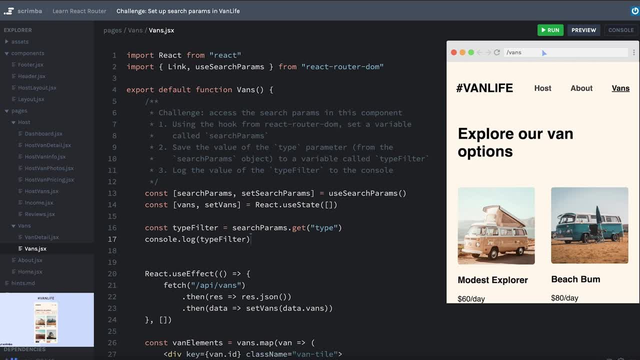 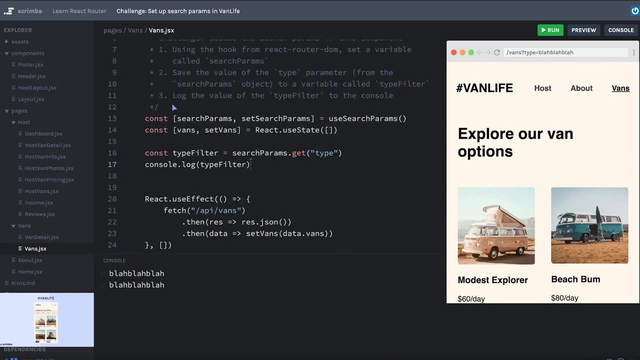 question mark type equals, and it really doesn't matter. I'll just say blah, blah, blah, hit enter And there it is. In our case, notice that we're getting it twice, And that's because we are rendering the component, we're grabbing the search. 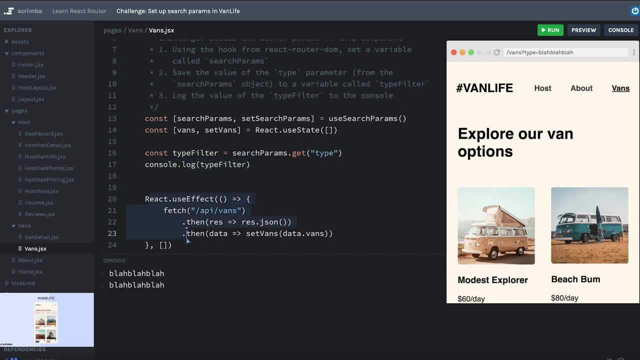 params Of type. we're console logging it and then our use effect is running. it's going and getting the data and then it's setting state, So it's re rendering this component, which is then running our code again. that's nothing to be concerned about, right. 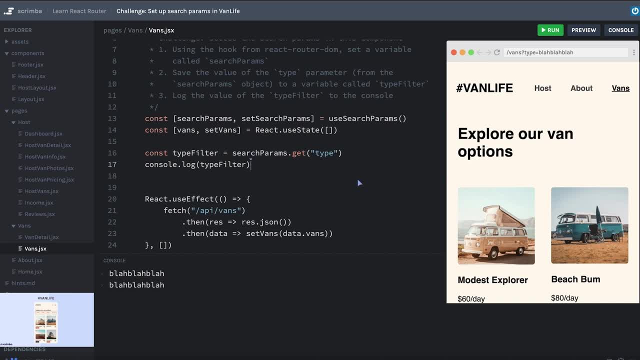 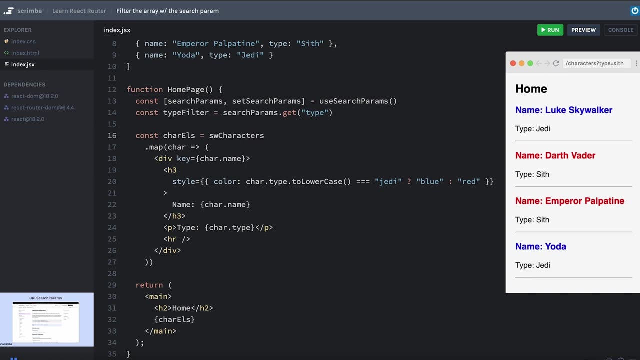 now. Okay, great work. The next thing we'll be doing is going back to our silly little Star Wars characters app And we will apply the search parameter to filtering the array. A notable thing that we are doing here is we are not using state in order. 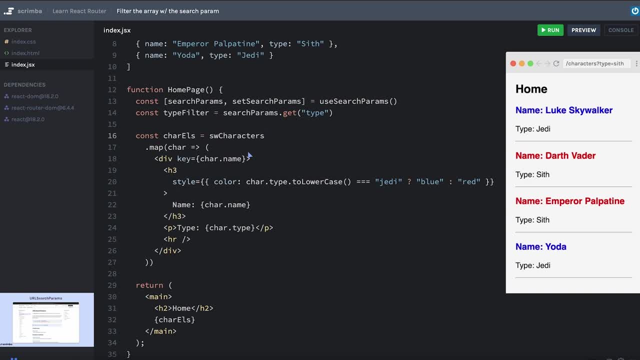 to maintain the information about the filter or the filter down list of characters or eventually the vans, but instead the filtering and the getting of the parameter and everything. this is all happening right here at the top of our component. Notice it's also not happening inside of a use effect or anything like that. the process of getting a search prim is really fast And the 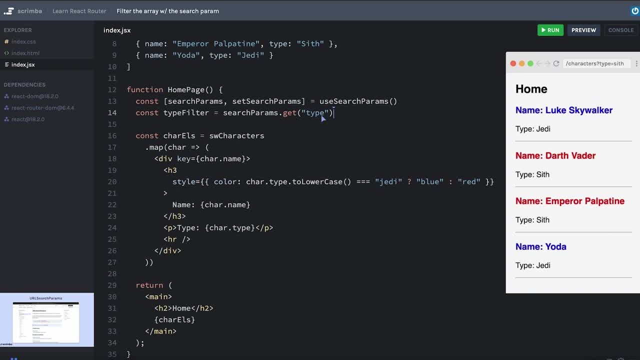 process of filtering down. in this example, the list of characters is also really fast, And so this isn't something that necessarily needs to happen as a search parameter side effect inside of a use effect in React. Instead, if we just put it here at the top level, 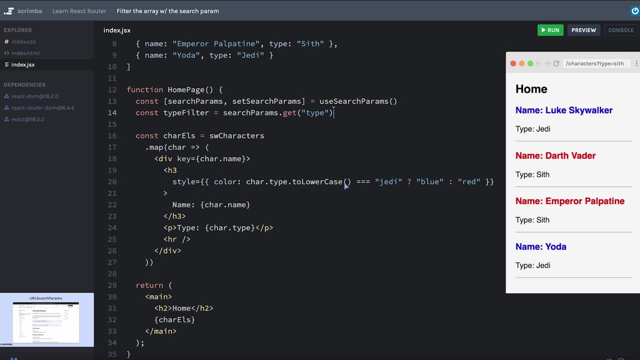 then every time this component re-renders, it will redo this work, and that's not that big of a deal. We don't need to worry at this point in over-optimizing this, because it's not showing us any performance problems. So here we're, creating our character elements, which is what 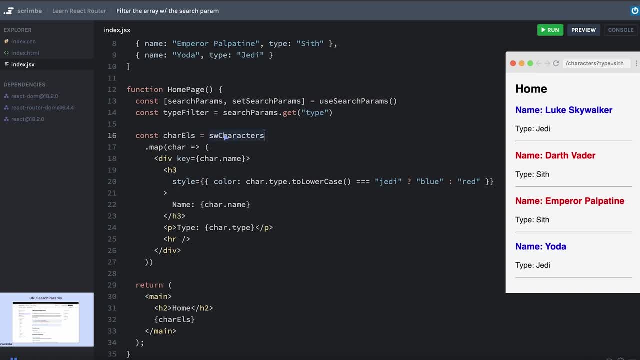 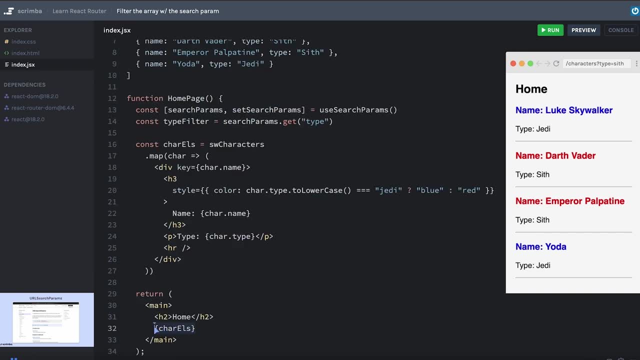 char-els is short for, and it's simply taking the full list of Star Wars characters up here and mapping over it to create the JSX elements that we want to display right here. So actually I want to type out just a quick challenge for you. I want you to think how we might approach. 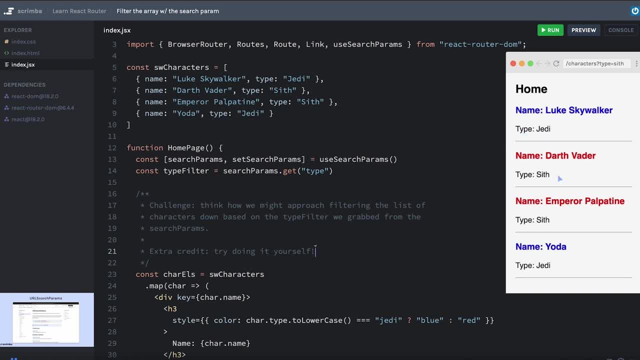 solving this problem of filtering our list of Star Wars characters down based on the type filter that we just grabbed from the search params. If you want a little extra credit- there's not really extra credit, but if you want to, I guess, feel extra good about yourself, then you could actually. 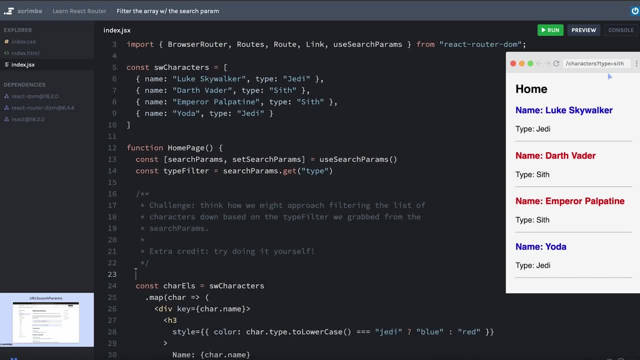 try to do this for yourself. Right now, we can see that there is a query in our URL. It says: type equals Sith. So if you're able to successfully do this, then it should grab Sith from the URL or from the search parameters and it should only show the two Sith characters that we have One. 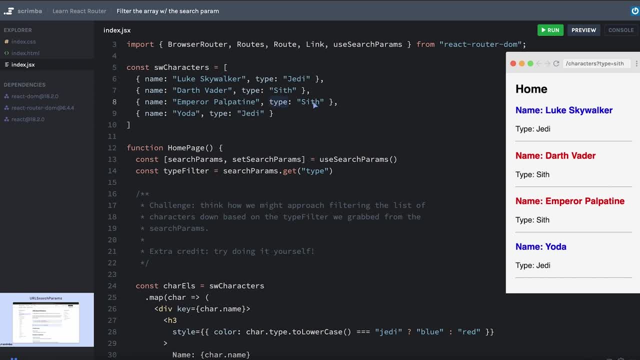 kind of gotcha here is: notice that the type in the object has a capital S in it, whereas the parameter has a lowercase s. That's something that you will need to take into account when you're working on this. Okay, pause now and either just think through how you might approach solving this. 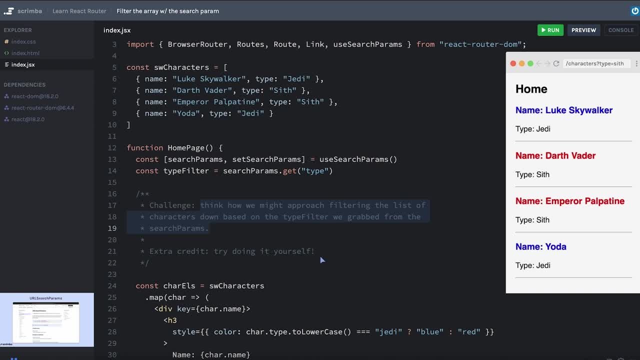 problem or, if you're feeling extra confident, try doing it yourself. I'm sure that there are a number of different ways to solve this problem. The first way that comes to mind for me is to simply chain a dot filter on our Star Wars characters before we then map over the array. Dot filter returns an array, but it will be a more limited. 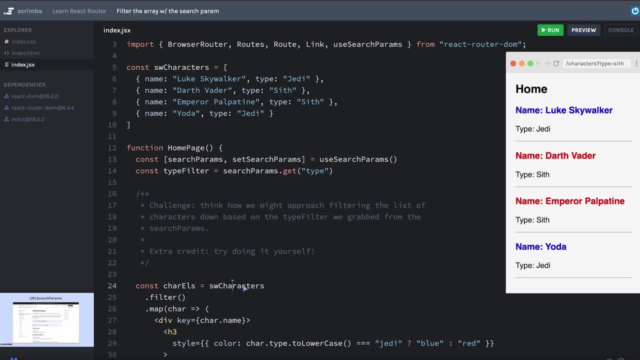 array than what the full array of Star Wars characters has. Dot filter returns an array and then we can just chain the dot map on top of the array that gets returned from dot filter. If it's easier to understand, you also could just set up a. 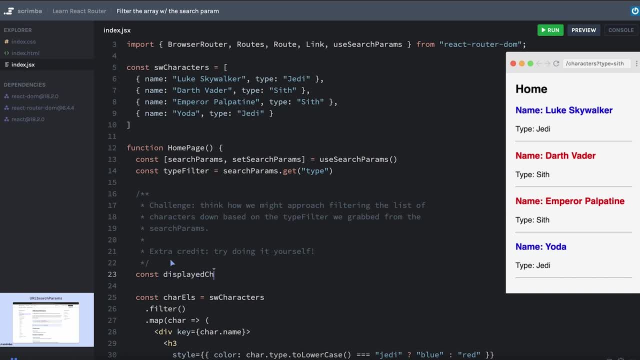 completely separate array variable, like maybe you call this displayed characters. that would be equal to Star Wars characters dot filter, And then you could just change this to say we'd get rid of this filter and we would say displayed characters. So that would also be a. 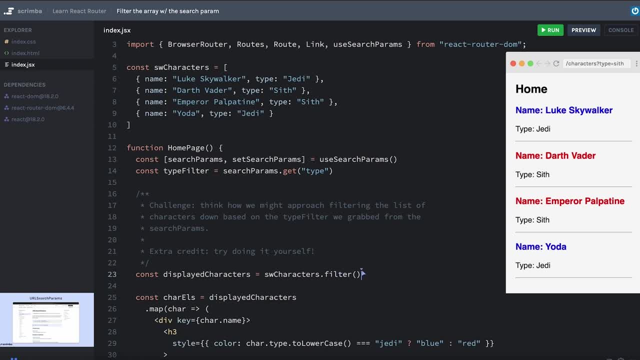 legitimate way to do that. Actually, in fact, you know what I think. I am going to do it this way just because there is a chance that we have no filter. In fact, we know that there will be cases where we don't have a filter, and so I may want displayed characters to sometimes equal the. 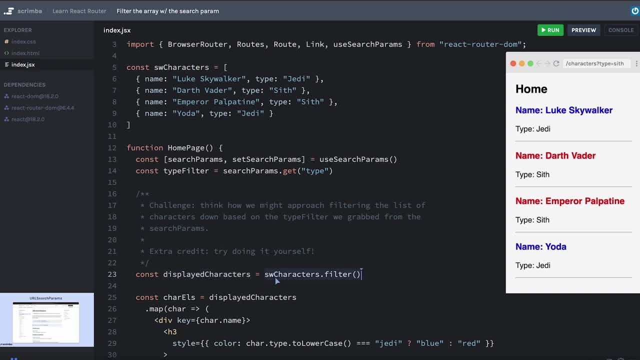 full list of Star Wars characters. So that might look something like this. If I say, do we have a type filter first of all? So I'll put a question mark- Let's actually move it down to this line. If type filter is a value, in other words it's in our case either Sith or Jedi, then displayed. 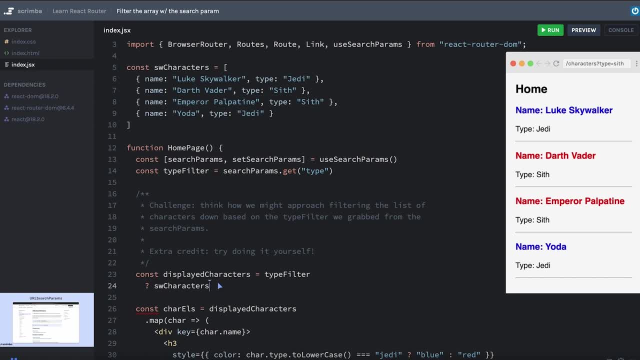 characters will be equal to the full list of Star Wars characters dot filter And we'll figure this part out in just a second. But otherwise it will just equal Star Wars characters. Okay, let's figure out our filter. Dot filter takes a function. We're going to have access to each one of the characters in this function. We need to return true or false. If we return true, 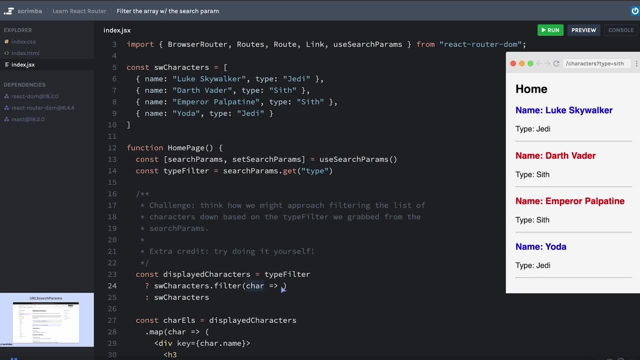 then it will keep this current character in the new array, and if we return false it won't. And so we can say: if the charactertype- and remember these- have capital letters- so I'm actually going to say charactertype- Dot to lower case, If that is equal to our type filter, then this will evaluate to true and therefore this character will get saved into the new array of displayed characters. 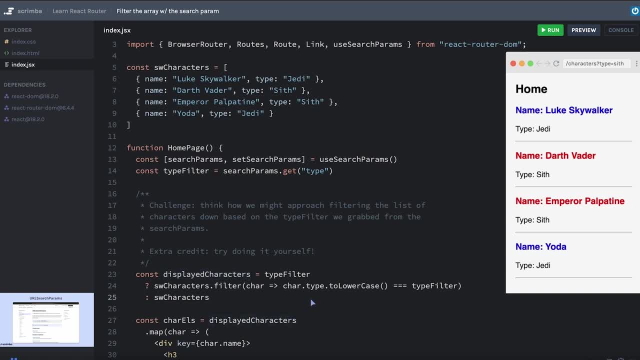 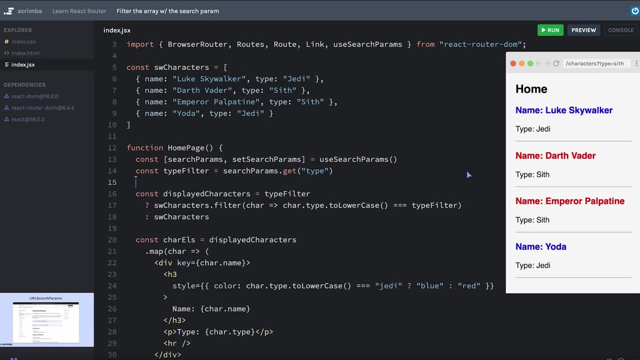 We already switched this to say displayed characters, So let me clear up this challenge text at a little space here. and we already have type equal Sith. Let's see if this works. I'll hit refresh. Cool, Look at that. Okay, we have just the two Sith Star Wars characters in our list. 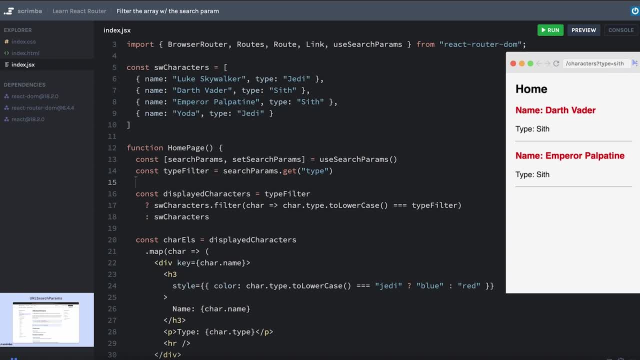 I should be able to change Sith or type equal Sith to type equals Jedi and hit enter and awesome. Okay, everything is filtering down, just like we'd think. Let's test it out without a search parameter, So I'll delete the search parameter up there and we have everybody. Awesome work. I really hope that went okay. 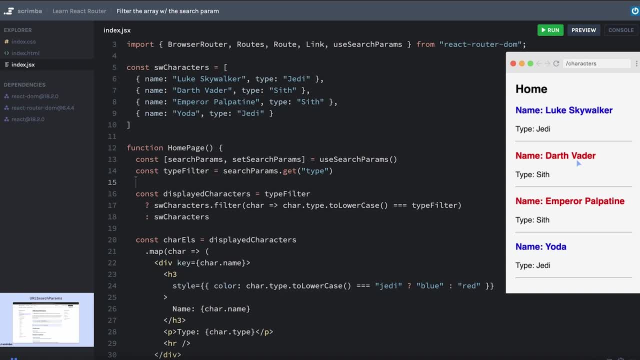 Of course, as always, if it didn't, just go back and try it again. And actually, even if you were able to do it, try scrubbing back to the beginning, before we had any of this code, and try doing it again anyway. 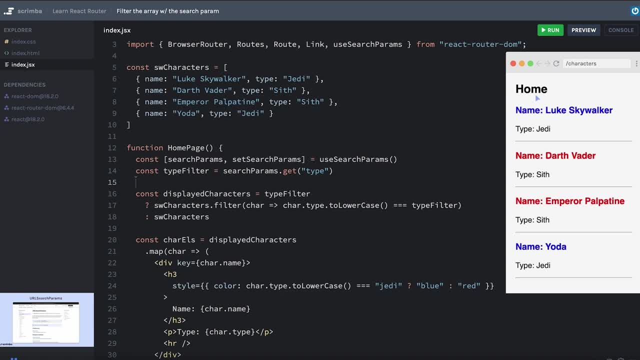 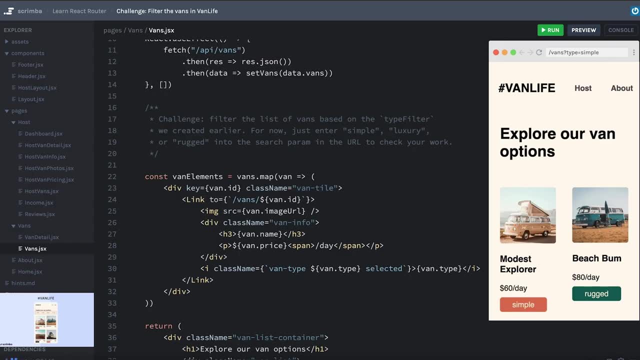 Next up is for us to apply our filtertype. We're going to apply this concept of filtering based on the search parameters to our van life app. Okay, your challenge for this one is to well, basically do exactly what we just did, but here in our van life app. 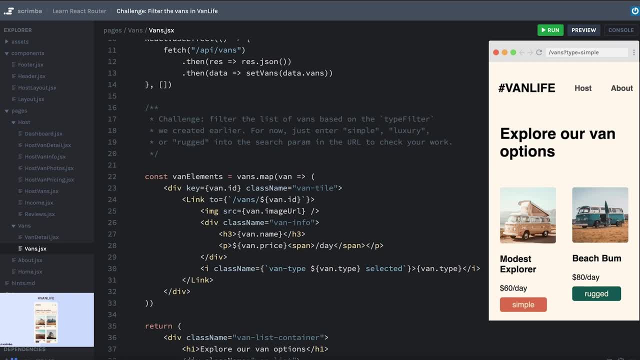 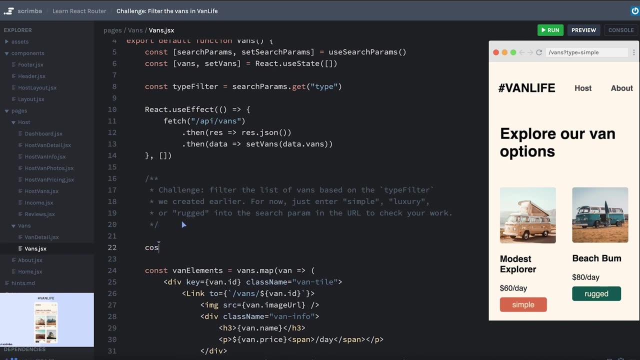 In fact, it's very, very similar. So hopefully you grasped what we just worked on, because now it's your turn to get your hands on the keyboard. Pause now and work on this challenge. Well, let's just do exactly what we just did. We'll create a const displayed vans. 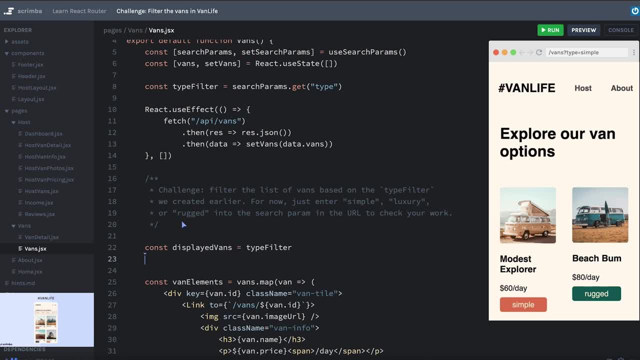 And that's going to check if typeFilter is a thing. If it is, Then we will use vans. This is the full array of vans dot filter. We'll look at each van and if the van dot type is equal to the typeFilter then it will return true and that will become part of the array in displayed vans. 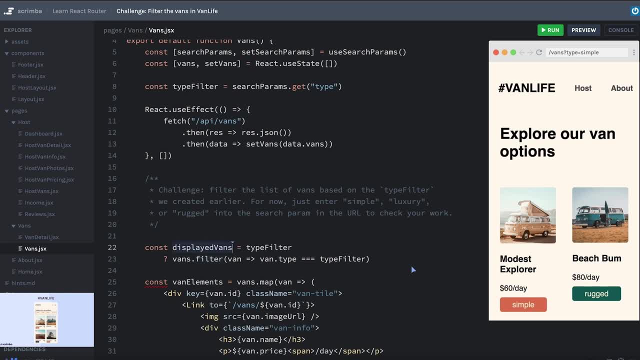 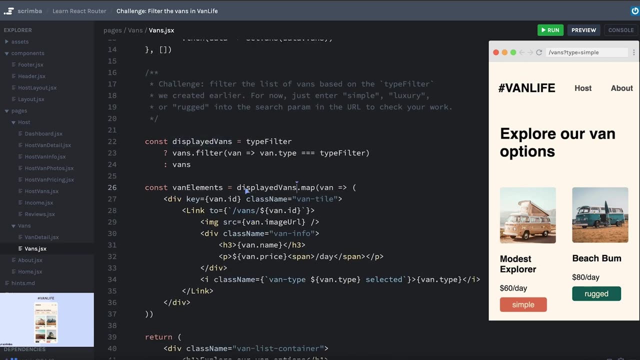 Otherwise, if typeFilter is an array, we only need a filter with a type Finished. if type filter is null- in other words there is no type equals whatever up there- then we just want to have the full list of vans and then, when we're mapping over it, we will just put our displayed 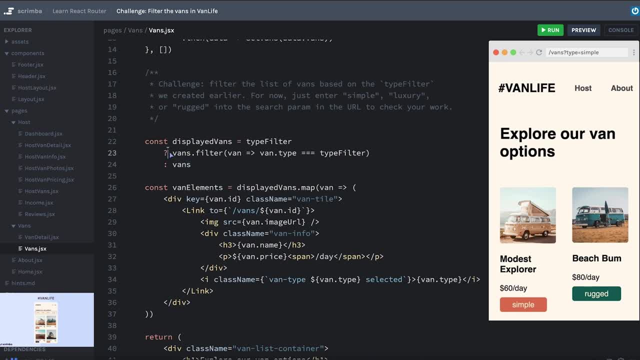 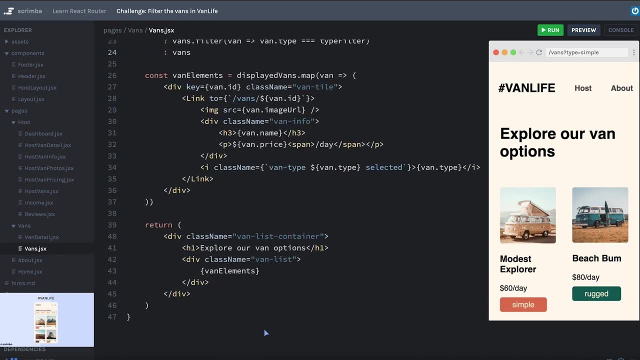 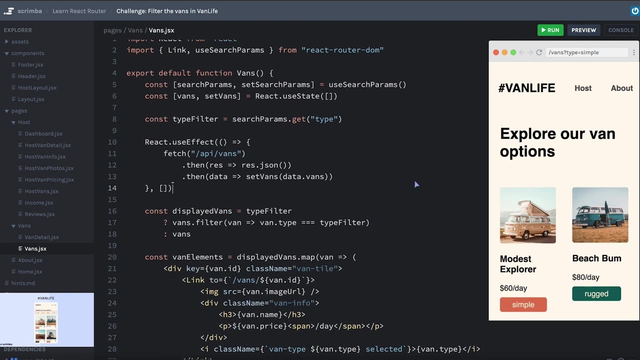 vans again. sometimes this will be the full array of vans and sometimes it will be a filtered down array. we'll just use displayed bands to map over that and create our van elements. i don't think anything else needs to change. let's clear this up and i already have type equals simple, so let's hit. 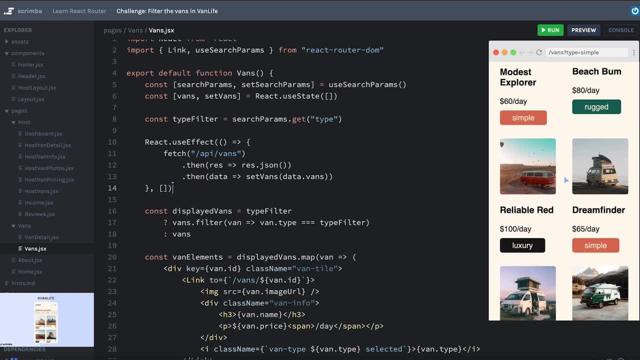 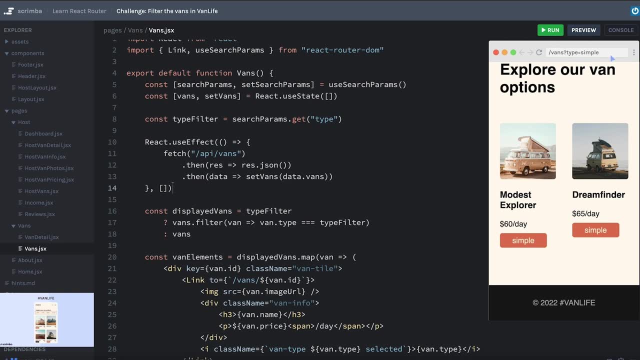 save. i'll scroll down a little so we can see that there's more than just the simple ones. cool, so i think the next logical thing for us to do is not have to actually type it up into the url, but have a way that we can click some buttons and have that change the query that's in the url. 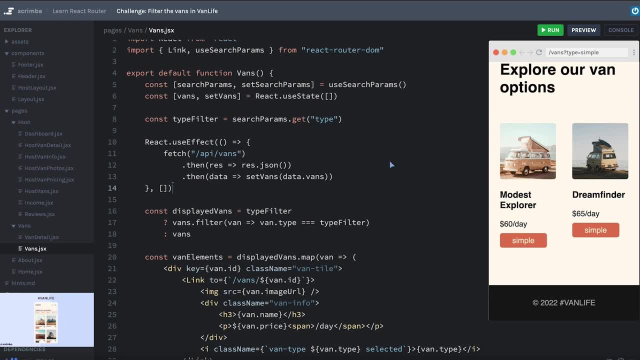 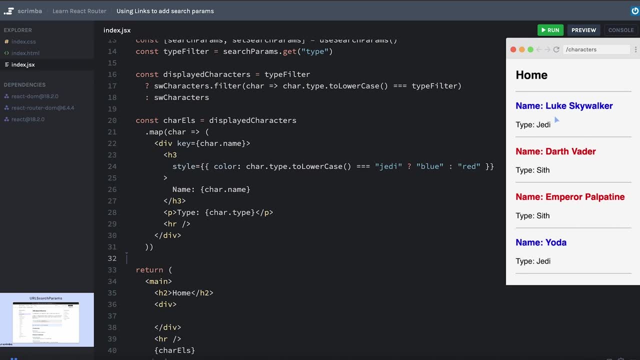 there's actually a couple different ways we can handle this, so that's what we'll be learning about next. the simplest way that i can think of to add search parameters is to simply use a link element. at this point, we're pretty familiar with using link to send us to a specific path, like if we were going. 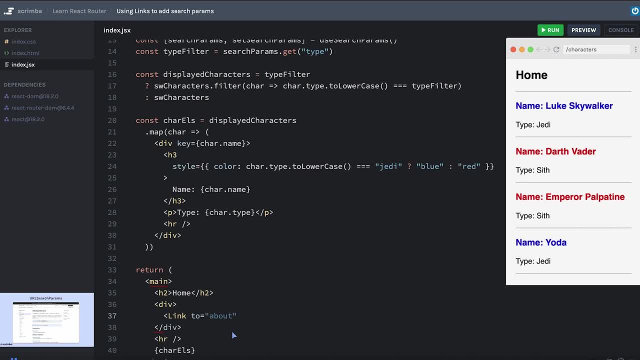 to the about page or something like that. but we also can use a link to not specify a new path that we're going to, but instead to specify a query. so i can simply say question mark, type equals jedi and have this link be, when it gets clicked, the way that we add the query to the top. i'll just create a duplicate of 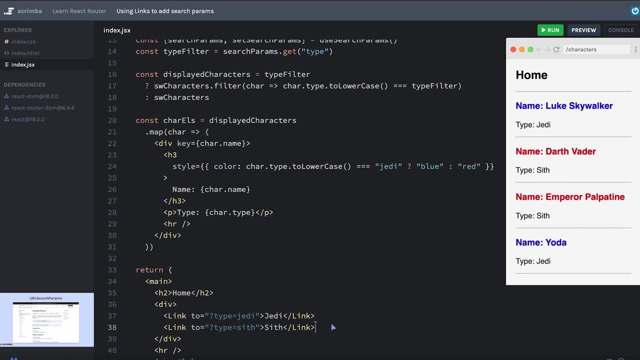 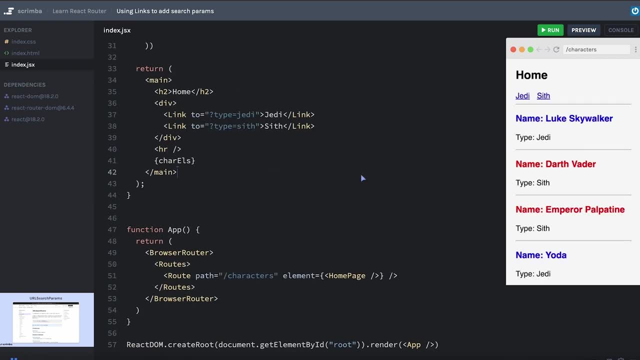 this. we'll say sith and sith, let's hit save, ah, and we do need to import link. so we will import link right here. let's try that again. okay, it's not much to look at, but we do have these links here, and when i click jedi, well, everything's just kind of working. we can see that it put the. 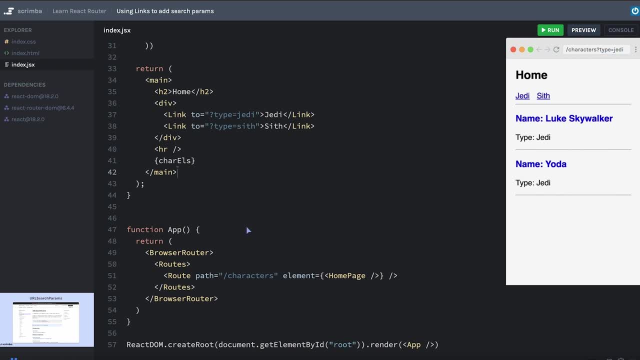 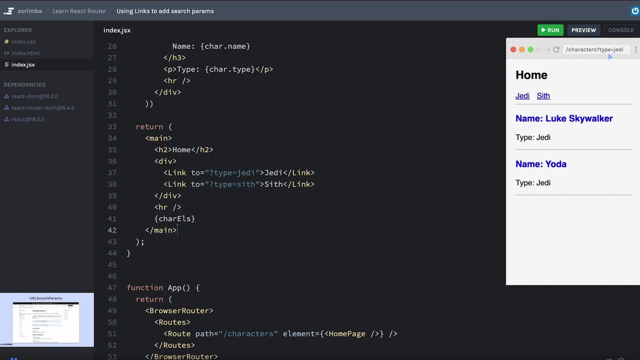 question mark type equals jedi in the url and because it started with a question mark react or knew that it wasn't changing routes per se- it's still the slash characters route, but it is adding some search params and because the search parameters changed, the component re-rendered. 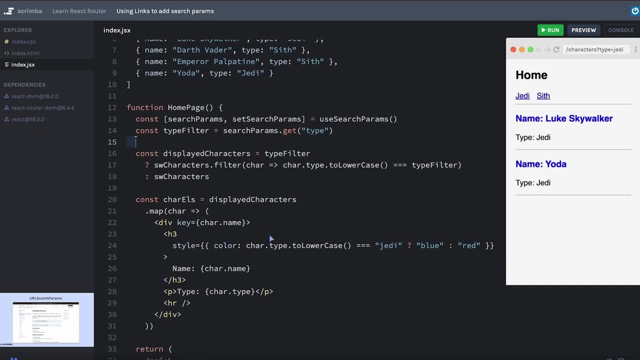 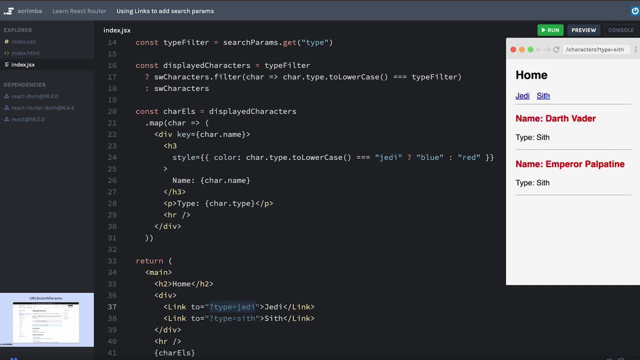 it re-ran our code that got the type and it did the filtering and everything like that. so again it's just kind of working out of the box. by adding question mark: type equals jedi or type equals sith, let's hit sith and we can see that's working as well. now let me throw in: 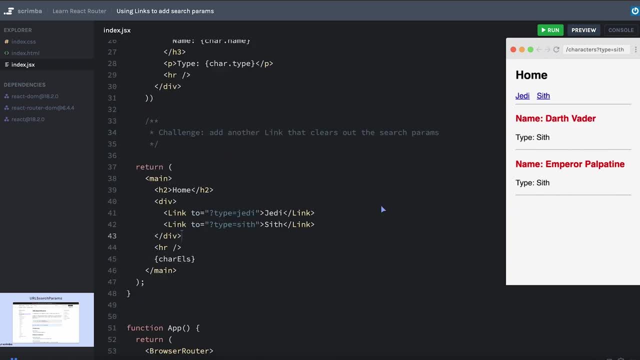 a quick challenge here. okay, your challenge is to see if you can add another link just right here next to the other ones, that clears out the search params. so, in other words, right now i'm filtered down by type, equals sith. i should be able to press a button or a link that says clear and 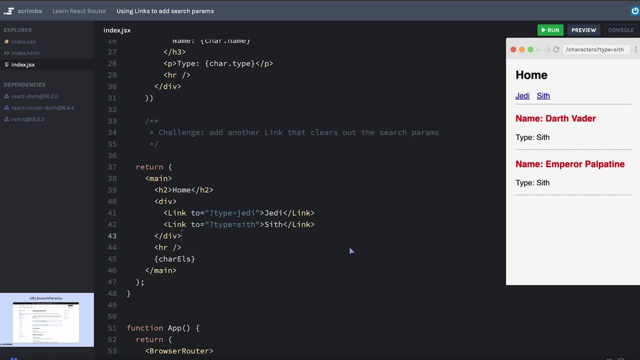 have it. show me everything in the list again. i haven't specifically taught how to do this, but i'm hoping that your intuition will kick in and you'll be able to figure it out. so pause now and give this a shot. i've found actually two different ways to do this, and i'm sure there's plenty more. 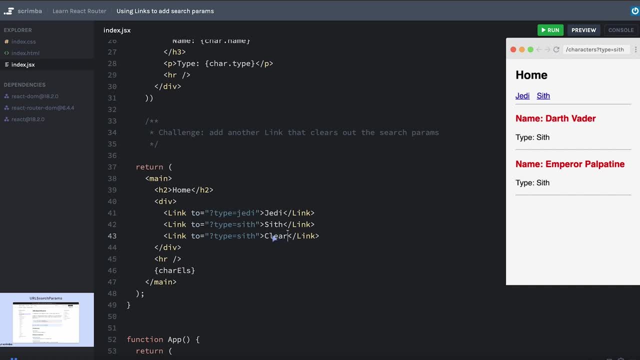 but i'm just going to duplicate the link. we'll change this to say clear and one way i found that works is just to say that the 2 is equal to an empty string. we'll hit save, i click clear and that clears out the search parameters and shows everything again. 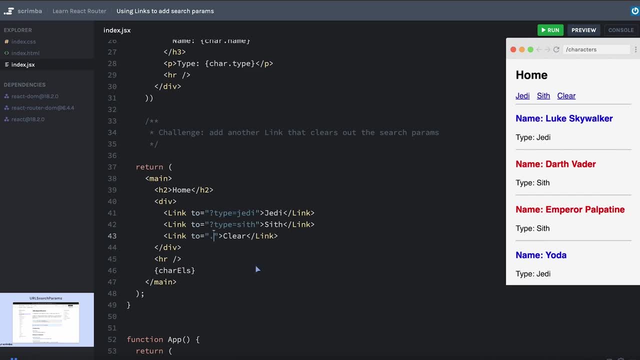 the other way that i thought about doing this is to say that i want this to go to dot and, if you remember, dot represents the current path or the current route. so let's hit save, i'll hit sith to filter it down and then we'll hit clear again, and sure enough. 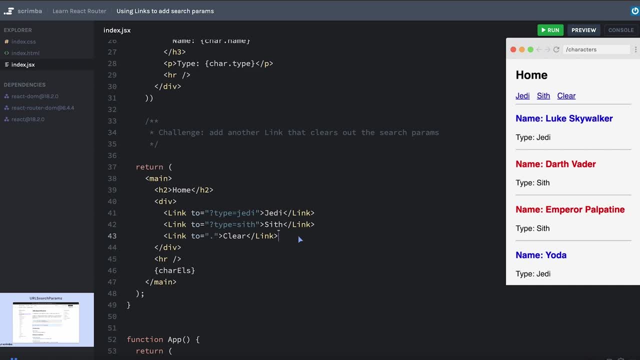 as well. i'm honestly not sure which one i prefer, so i think either way is going to be fine. i'll probably just leave it here as a dot, because i suppose you could argue that it's a little more explicit as to what we're doing. we're saying: just go to the current path, without anything else. 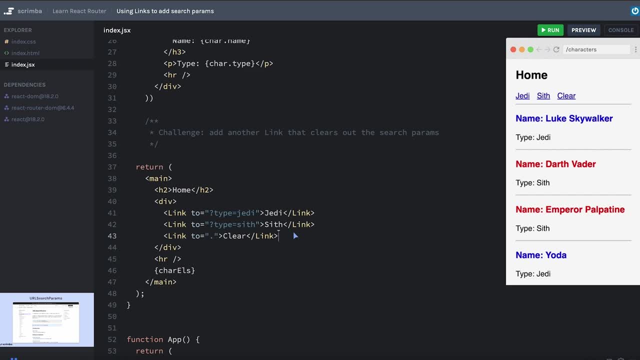 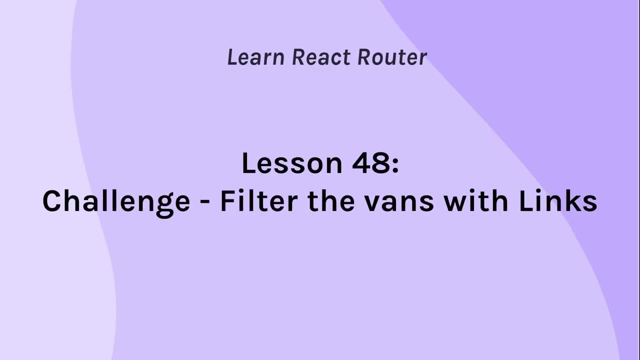 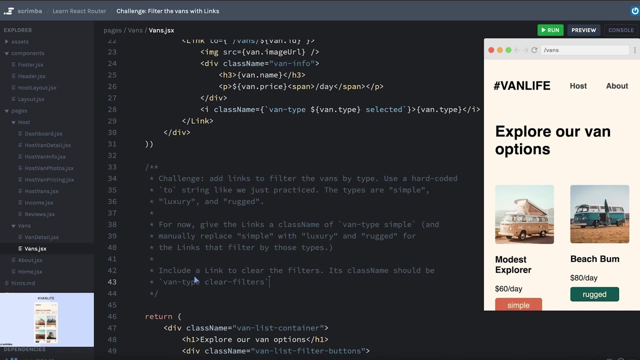 attached to it. okay, that was fairly straightforward, but there are a couple caveats that i want to talk about with this method of using the link. so that's what we'll be doing in the next scrim. okay, let's learn what we just applied by adding some links to our van life app, so that we can 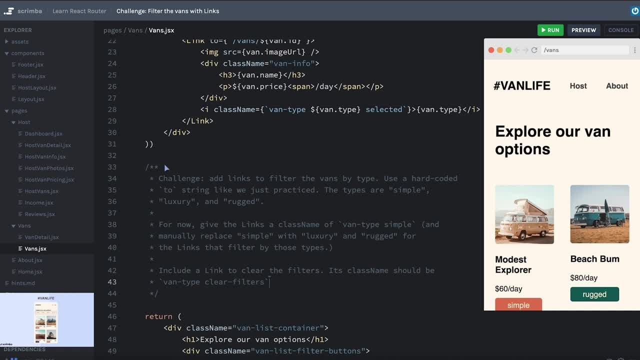 filter the vans by their type. for now, the links are just going to have a hard-coded two string, like we just practiced, and the different types are going to be simple: luxury and rugged. i've given you some class names to use, because we're not focusing on the css here, so i've already. 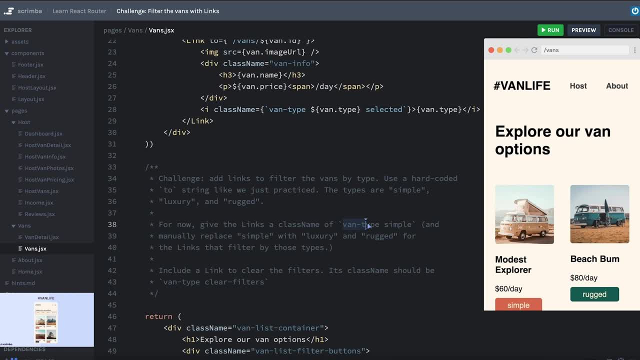 written some css, so for each of those links add a class name of van-type and then the type of that link. So if it's the simple link, it'll say simple. If it's the luxury link, it'll say luxury, and so forth. For the link that will clear all the filters, its class name should be van type. 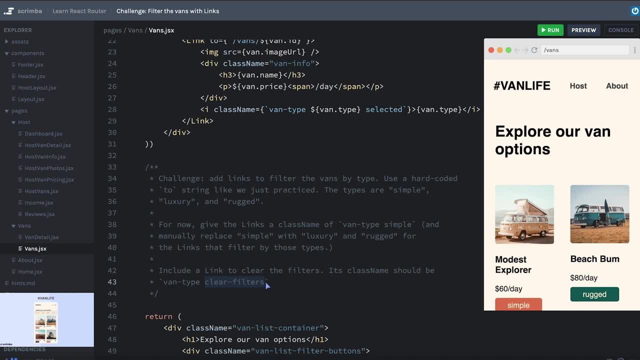 space clear dash filters. Give this your best shot. I'm sure you can do it. If you do get stuck, we're going to walk through it in just a minute, But of course, as always, you can reach out to the community for help too. Oh, and one last thing is, you'll add your links right here between this. 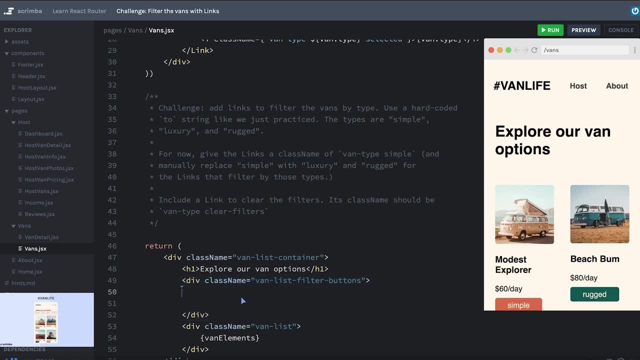 div that I created, So right where I'm putting my cursor. Okay, pause now and add those filtering links to our van life app. Okay, I can see that we already have link imported, So we should just be able to create some links. And while I'm at it, I'll just add the class names now. So our class. 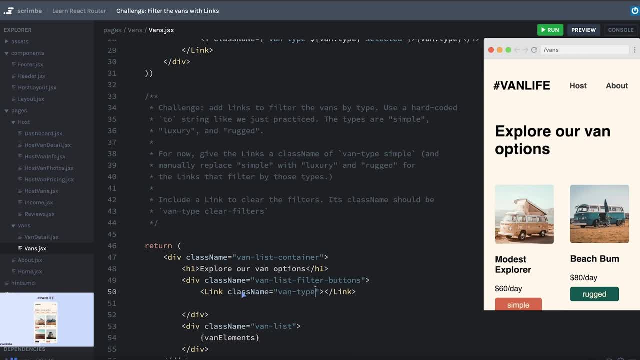 name is going to be equal to van dash type space, And then this is the one we'll change. here we're saying simple, Let's move this on to its own lines And we'll just leave it like that, And we'll give it a to property of question mark. type equals simple. And let's just start out there. 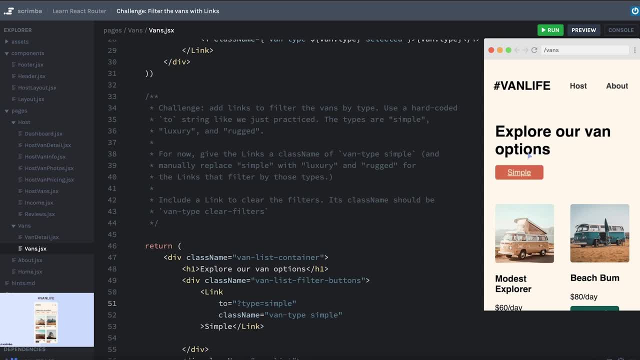 and see what it looks like. Okay, and let's see if it works, So I click: looks like some styling needs to be fixed. We'll click that. Okay, we get type equals simple And we only show the simple vans. Awesome, Let's go ahead and copy this link: create one for luxury and one for rugged, And I 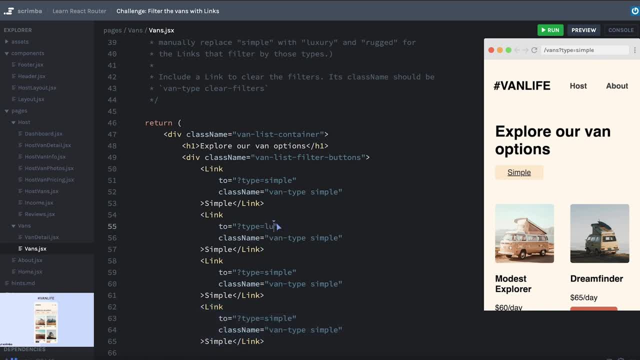 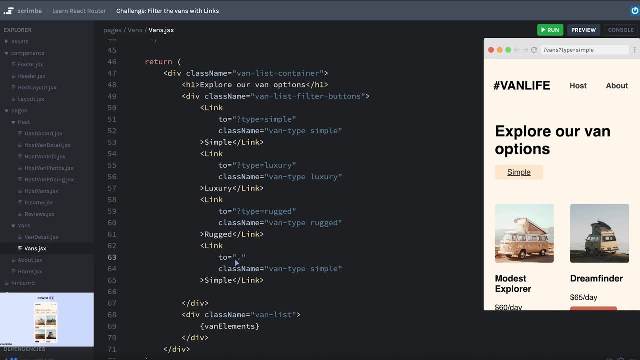 guess one for clearing the filters, And we'll just make some of these little changes like this For clearing out the search parameters. we will just hit that. the two is the current route And this will be clear filters And this will say clear filters or filter. Okay, let's hit save. 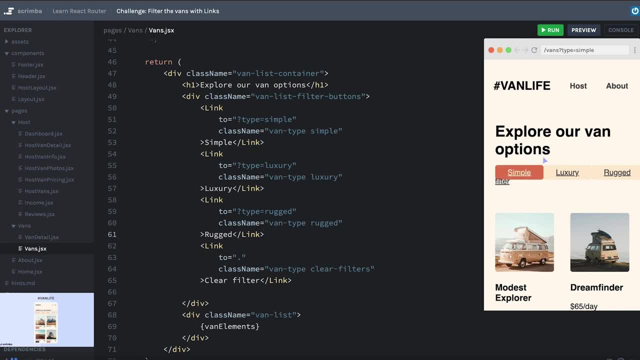 Okay. yeah, the styling is still needing some work, But we can see that everything is working Okay. Sometimes, when you're developing, it feels a little bit like a gamble. you think you've done everything right And then you find some major bugs. 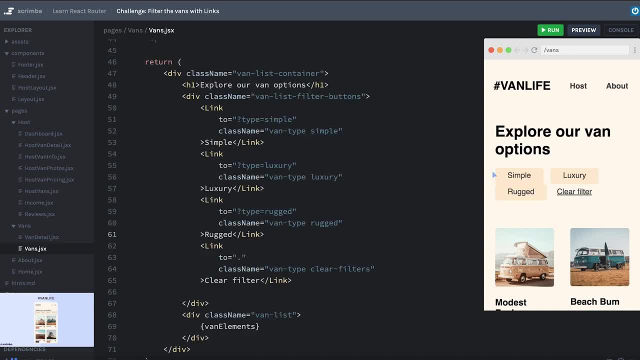 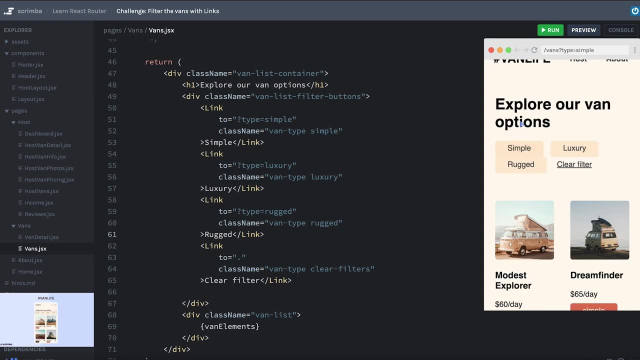 Let me take a look at it. Okay, there was a couple of styles I forgot to copy over. Hopefully that didn't throw anybody off too much. But the styles are one thing, the functionality is another. and the functionality is on point. It's working great. Okay, so now we've learned how to set a query. 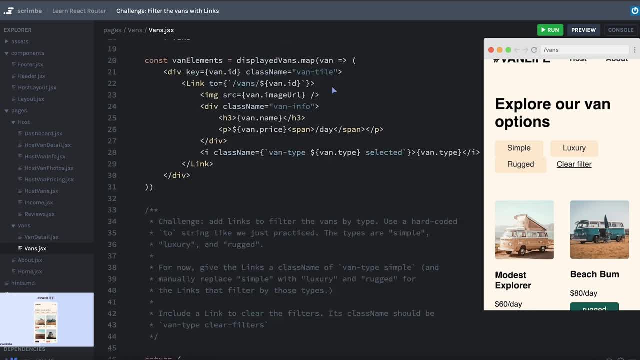 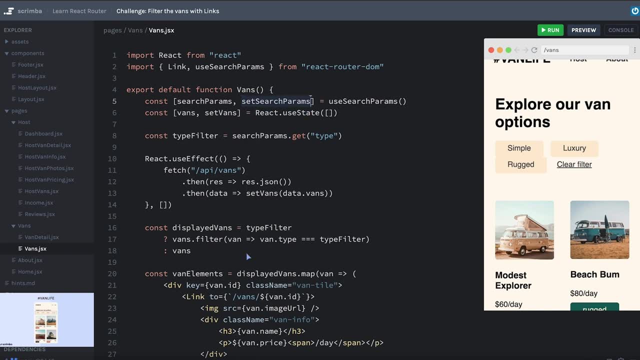 string using a link element in react router. But you might have noticed that we created this setter function When we're initializing our search params. we have this set search params function, but we're not actually using it anywhere. If we're going to link directly to a hard coded version of our search params, then we don't. 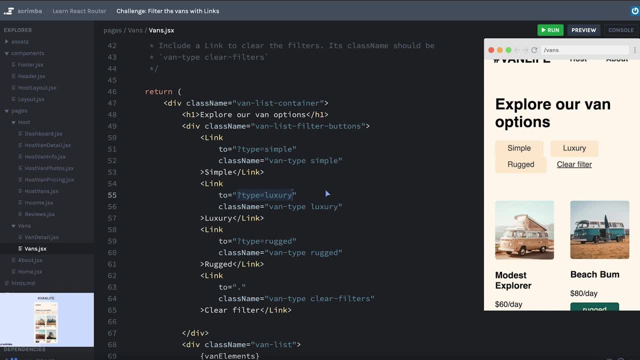 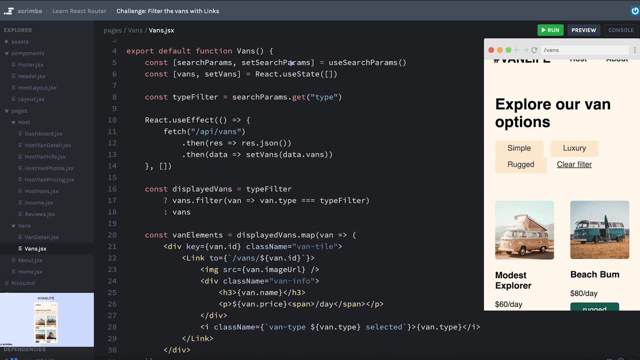 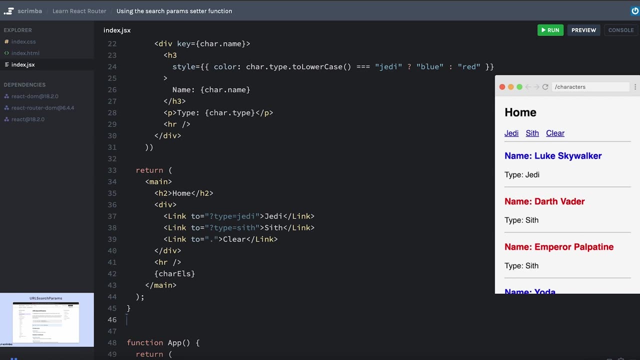 necessarily need that search params setter function. However, there are instances where you may need to use it, So we are going to refactor what we have and learn about using the set search params function that we have here. Let's take a look at another way that we can set the search. 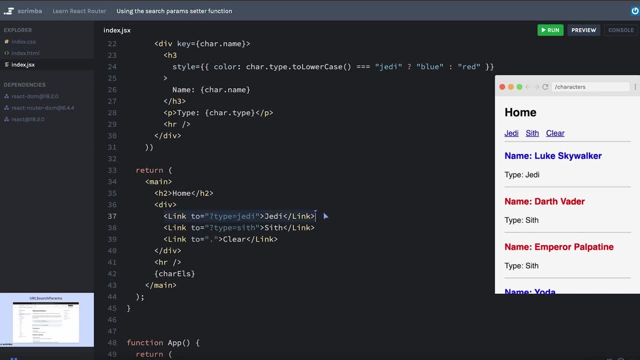 parameters in our app. The way we have our link set up is a really, really simple way to do this. There's some caveats with it- we're going to talk about soon, But first I want to comment these out. Actually, I'll move them. 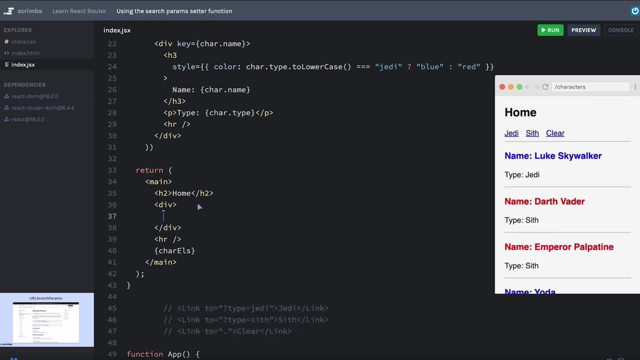 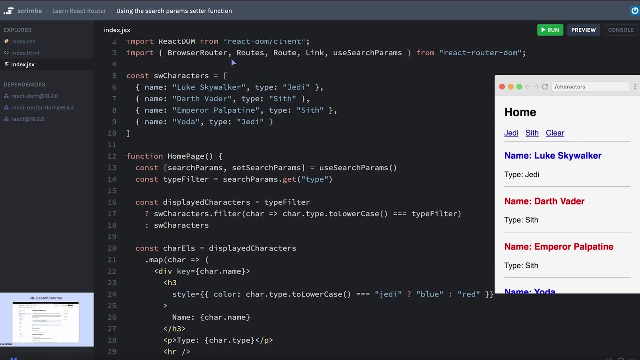 outside of my components so I can comment them out, And I'm going to show you another way. Instead of linking to the query parameter that we want, we can use the state setter function that we received when we initialized our search params. So this function here set search params just like in. 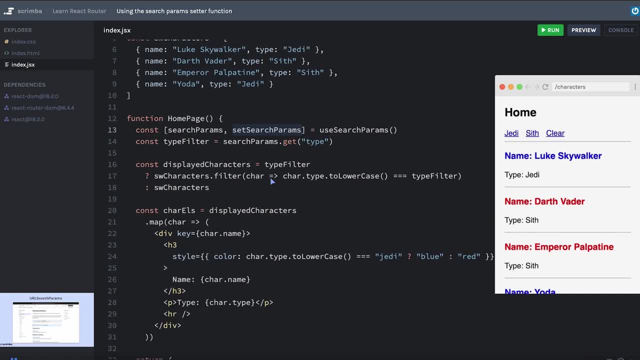 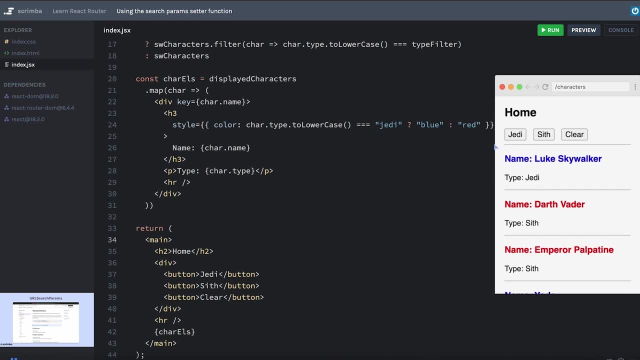 use state is a setter where we can tell it what the new search params are going to be. So let me create a couple buttons here. Okay, let's go ahead and type a little bit of this function here And again, this function will. 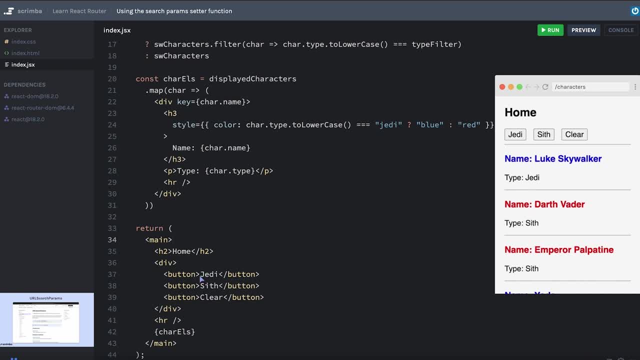 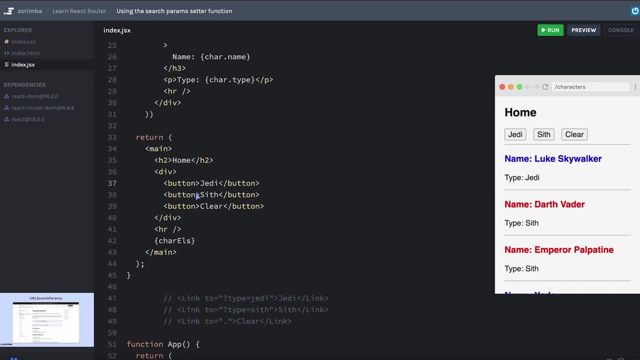 be a little bit different. So I'll hit Save And we have buttons instead of links. Of course, we could style these however we want. So this time around, because buttons are not part of the React router ecosystem, like link is, we are simply going to use an onclick event handler in order. 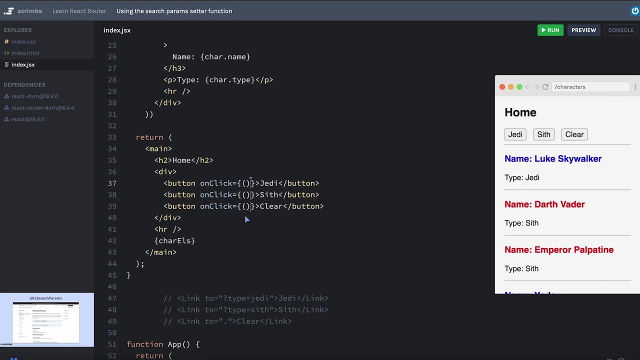 to call our set search params function. So I'll create an on click for each of these And these will have a callback function And that function is going to run: set search params. the setter function can either take a new value for the search params, which will completely. 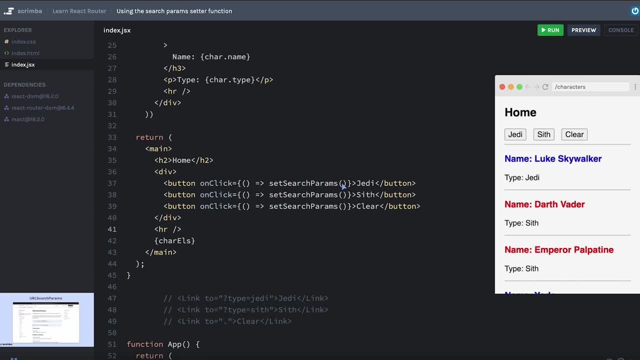 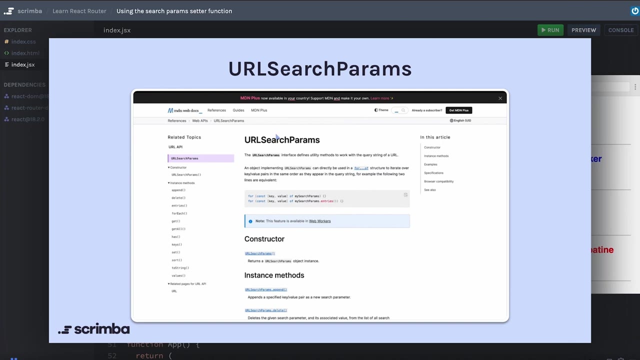 replace the old value or it can take a callback function. First we'll look at just passing in a new value. One thing I've learned with set search params is that it's very flexible. We can pass any value into here that the URL search params- this object here- can take. And if you look at the 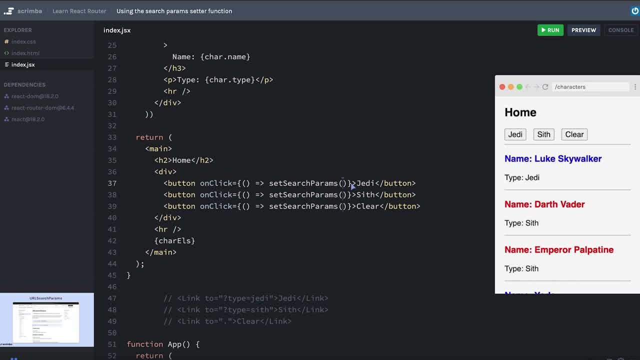 documentation here. I think there's four different types of parameters that you could pass in for it to generate search params. One of the ways that you can initialize new search params is by passing in a string that represents the new search params you want, So this is actually almost identical to 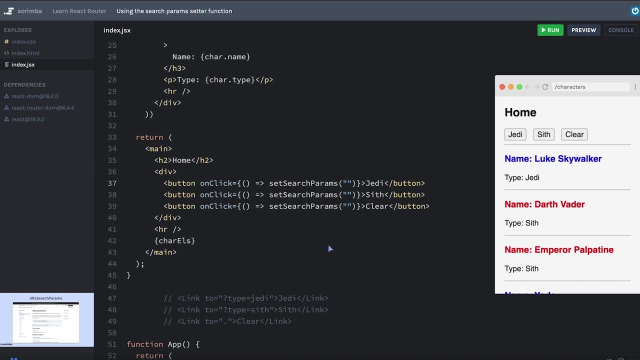 what we had with our links And the URL search params object is smart enough to figure out if there's a question mark at the beginning, so it actually doesn't matter. You can either say type equals, and then we'll say Jedi, this one will say Sith and then this one will actually. 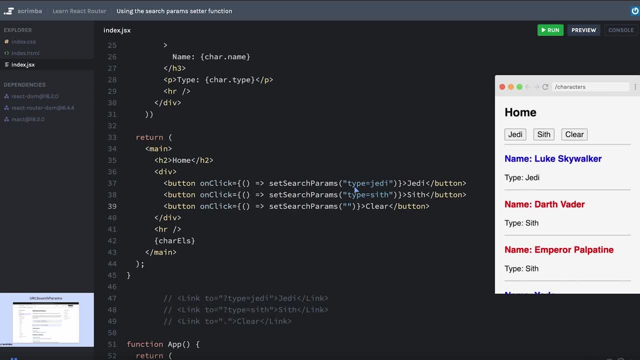 just say we want to set the search params to an empty string, Or I could put question marks here and it's smart enough to figure it out. So let's see with the question marks: Jedi shows Jedi. we see in the URL type equals Jedi, Sith is the same. clear, clears them out. 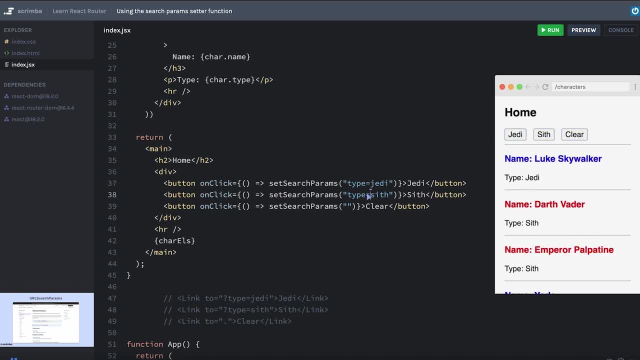 and without the question marks, it does the same. Okay, so yes, this works to pass in a string like this. However, I don't oftentimes see this string initialization used very often. More commonly, I will see a record initialization, or what you could just think of it as being an object. 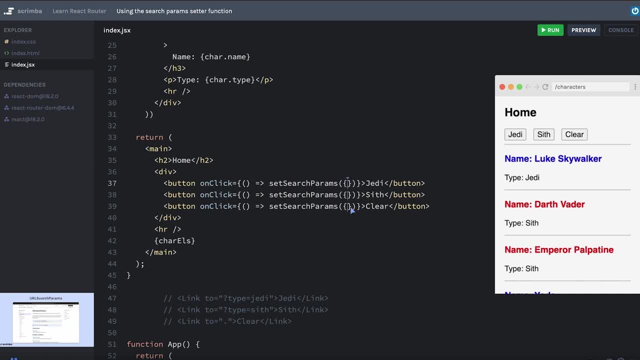 initialization. And this is very similar where the object has keys and values, just like our search parameters have keys and values. And so I can say that the type is going to be, and then I can pass in my Jedi Sith. and then here we're just going to pass in an empty object which says: 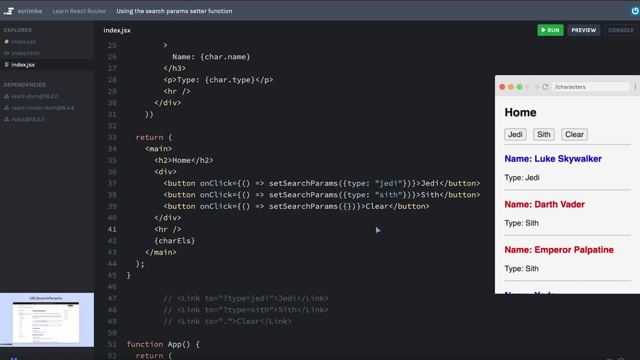 I don't want any search parameters. Okay, we'll hit save Jedi. we see that that translated into the query string, just like we would have expected, And that's happening by the URL search parameters. So we're going to pass in an empty object which says I don't want any search parameters. 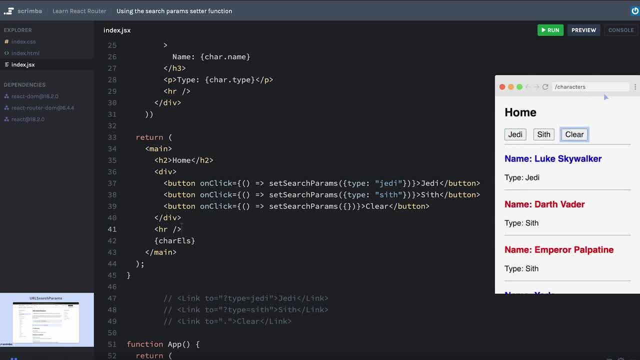 object under the hood Sith does the same thing and clear clears them out. Now, truth be told, there's actually other ways that we can initialize this exact same thing. Each one has their own use case, But more often than not, if you're typing it in, you're probably going to see people using 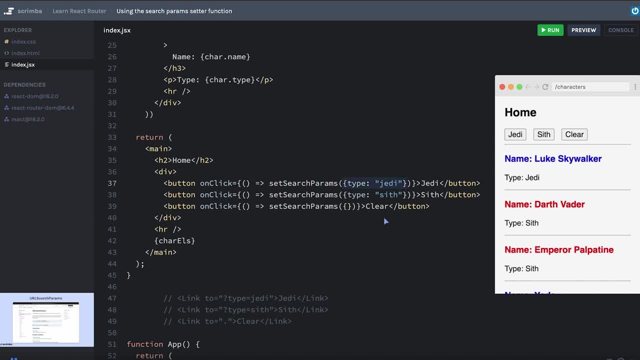 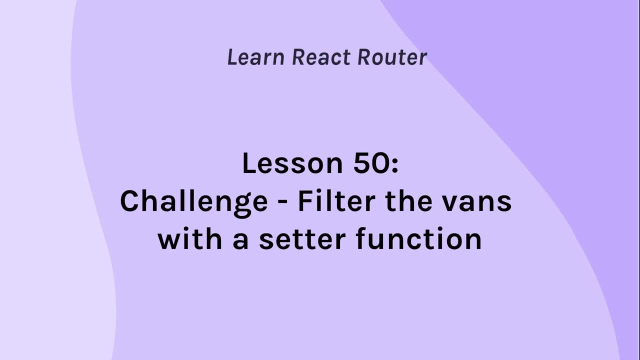 an object like this. So that's what we're going to stick with. Okay, time to practice this. Let's go over to the van life app and you'll get your chance to practice. Okay, challenge time again. your task is to change the links that we have. 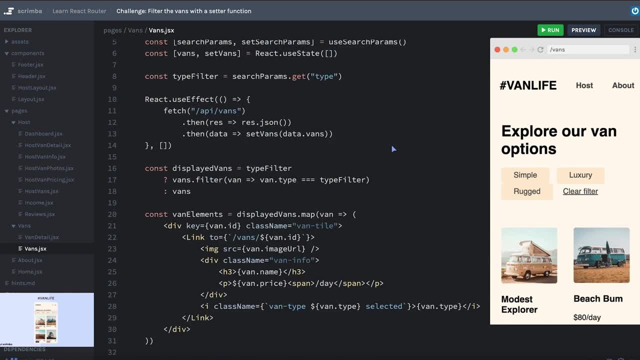 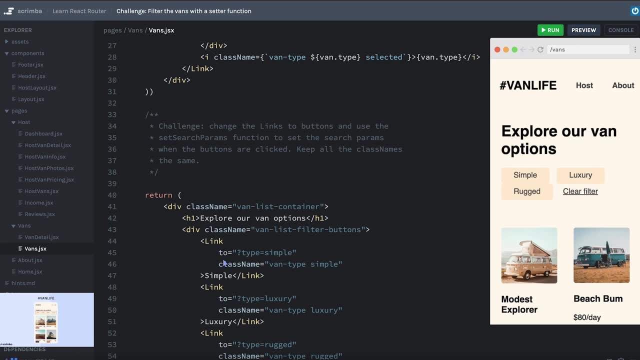 into buttons and to use the set search params function- which remember we instantiate it up here- to set the search params for the filtering of our vans. Make sure you keep all the class names exactly the way they are. Pause now and work on the challenge. Okay, this should be pretty. 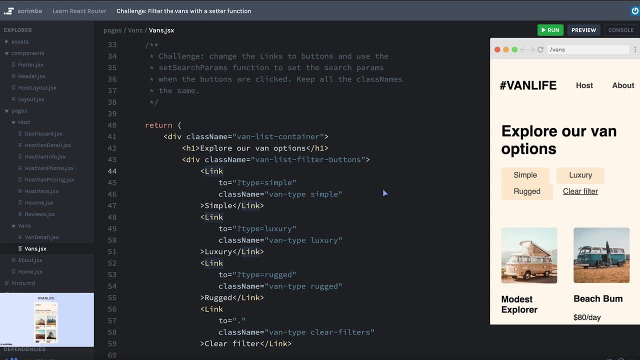 straightforward: Let's go ahead and select all of our links. We'll select the link to the clear filter option as well, And we will change these to the clear filter option, And we'll change these to buttons, And then, instead of having a to property, we'll select all those we're going to. 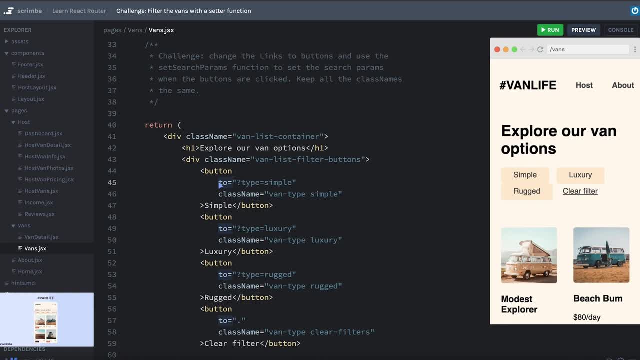 actually let's leave the string there for now. we'll say that when this button is clicked, so on, click is going to be equal to a function. we'll need to run that inside of curly braces And I can't just say set search params right here, because I would need to call it And that means 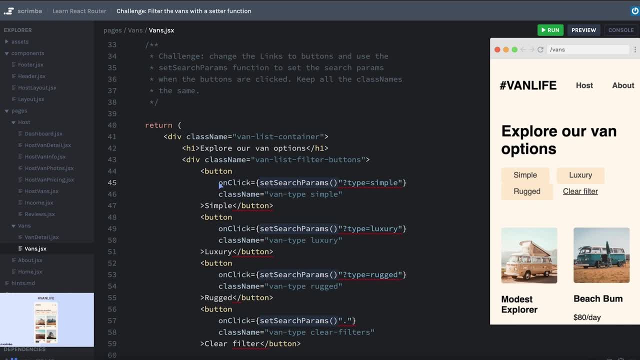 it will get called as well. So I'm going to call it curly braces And then I'm going to call it as soon as the page loads, not as soon as the button is clicked. we need to pass a function And let's go ahead and move. looks like my strings are a little off. That's okay, we'll make it so. 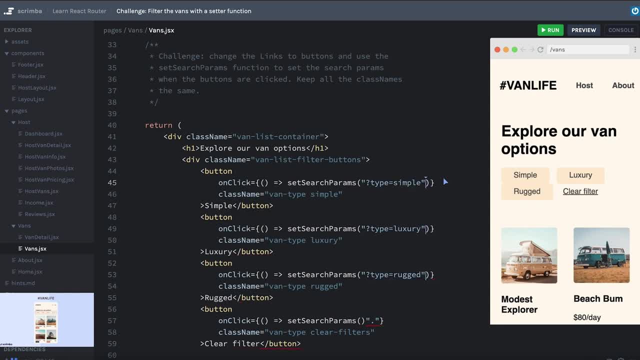 that this string goes inside here And then we'll move this string inside. Actually, this is just going to be an empty string. Remember the dot string like this, like we had with the link before. that's something specific to react router that it's doing under the hood, So set. 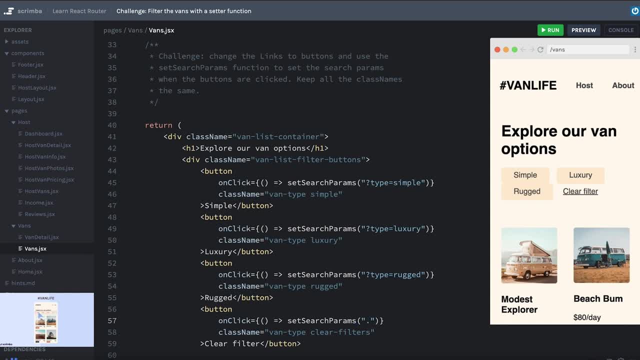 web search params is actually using the URL search params constructor And that won't, I don't think, know what to do with having a string of a dot in there, So we'll just have a be an empty string. Again. when we're passing in a string, we can include or not include the question mark. 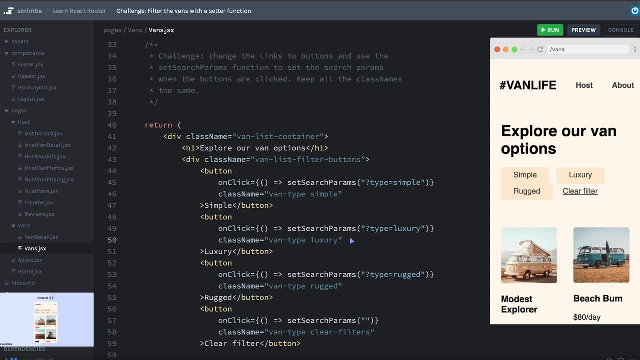 let's just leave it there, because we're actually going to change this in just a second anyway. So let's hit Save and type: simple, type Luxury, type rugged and gone, perfect. Now, like we learned, the string is not probably the most common way to do this, But it's not necessary. It's not necessary. 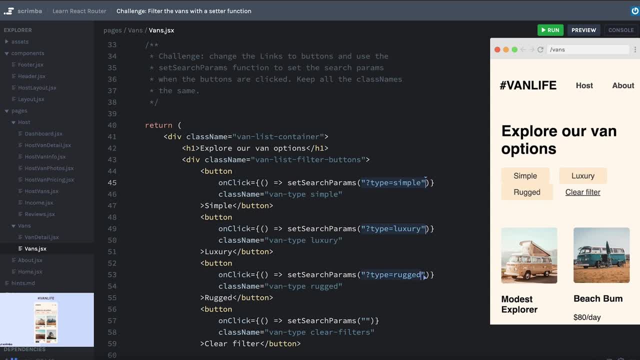 to use string, And again, if it doesn't make sense, you can use another string, or you can use the을l search parameter, But for theug search parameter is actually using the url search parameter, the most common way to do this, although it works just great. Instead, a little more commonly, 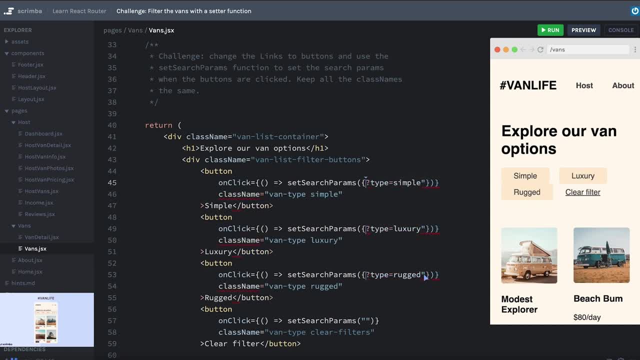 you'll see an object passed in. here We'll actually just manipulate the string that we had and turn this into an object like this, And then for here we'll pass in an empty object, which means that we have no search parameters when we set the search parameters. All right. 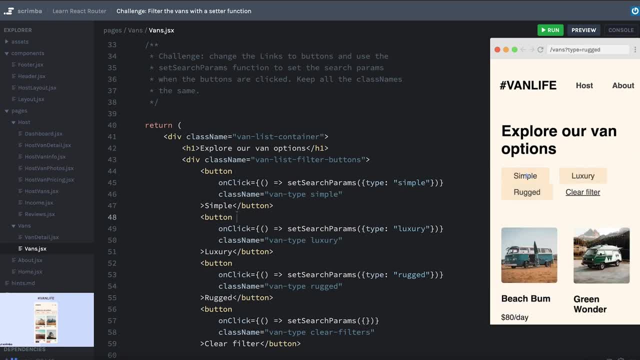 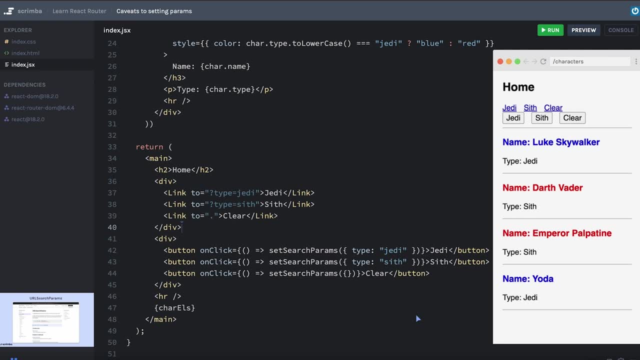 let's hit save And yet again it's working like we would expect- Great work. Now there's actually a major caveat to the way that we've been doing our query parameters so far, And let me show you what I mean. So up here I'm going to create a new query parameter that 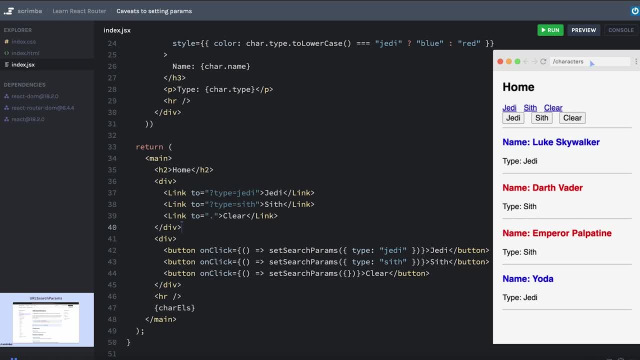 has nothing to do with what we've been doing so far. I'll say name equals Jill. We'll hit enter question mark: name equals Jill. That has no impact on the filtering of this part of the app. Well, and we know that it has no impact on any part of the app at this point, But it's so common. 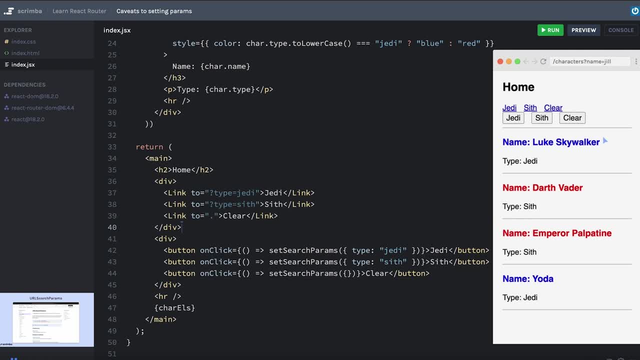 to have more than one query parameter, each one possibly having to do with the other one, With a different part of your app or a different page in your app. However, the way that we've structured this right now- because we're hard coding- a question mark type equals Jedi or Sith. 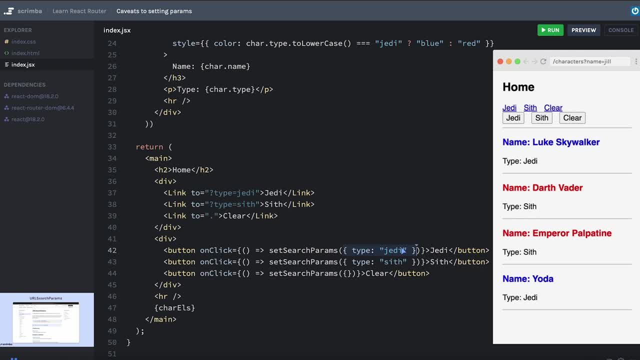 And over here we're hard coding this object that just has one key and value in it. As soon as I click one of these buttons or these links, I will lose the context of the query parameter. name equals Jill. So if I hit Sith, now it's changed the query parameter to type equals Sith, because 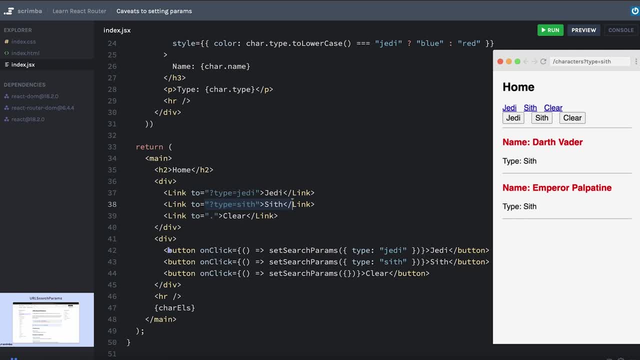 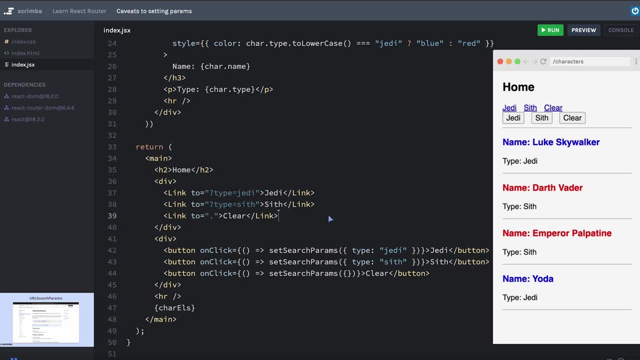 And the clear buttons would do the exact same thing. It clears out any search parameters that you might have, not just the ones that you care about in this specific component. So if, for some reason, you know for a certainty that you will not have any other query parameters in your 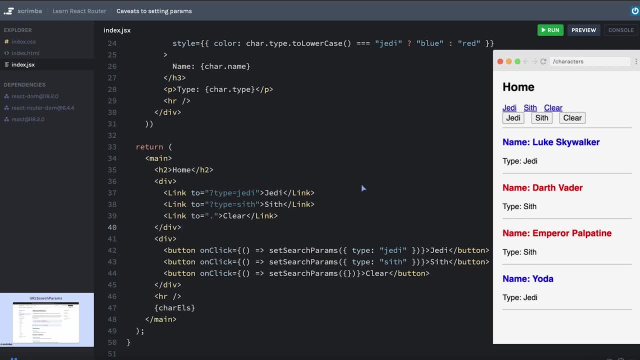 project, then the way that I've shown you here so far will work perfectly. However, for the purposes of education and an exercise in completeness, I'm going to show you some methods that you might use in order to merge your query parameters with existing query parameters, instead of completely. 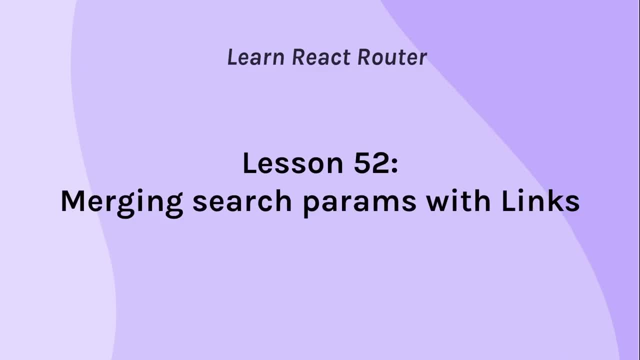 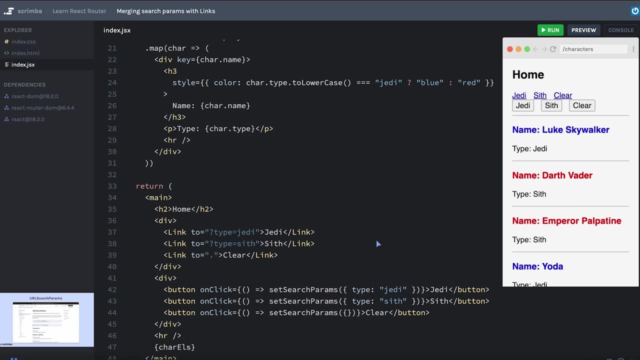 replacing them. So we'll do that in the next scrim. The main reason I think I want to show you how I figured out to do this is because I actually struggled with this for a long time, And I don't even mean when I first started coding. I mean 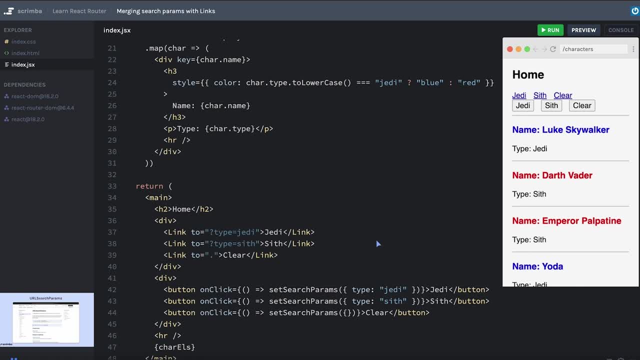 just as I was preparing these lessons, I was really trying to figure out the best way to do this, And I think I've come up with a good way, But a caveat to that is that it's not the only way. There are certainly 1000 different ways that someone could solve this problem, So I'm going to split this. 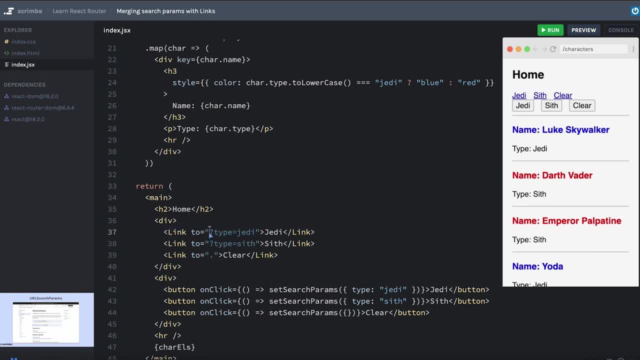 into two parts. The first part is how to solve this problem, And the second part is how to solve this problem, And the second part is how we can generate a query string, like we see here in our links, so that it will merge any existing query parameters with the one that we're trying to add. 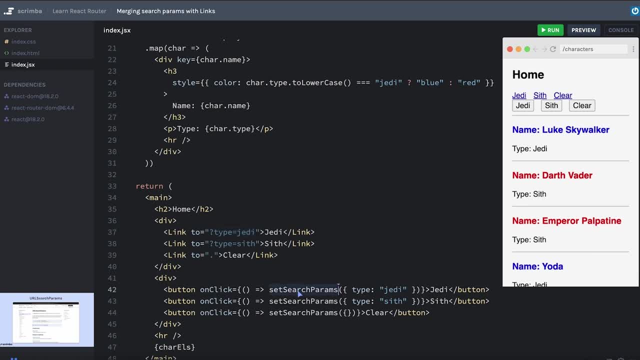 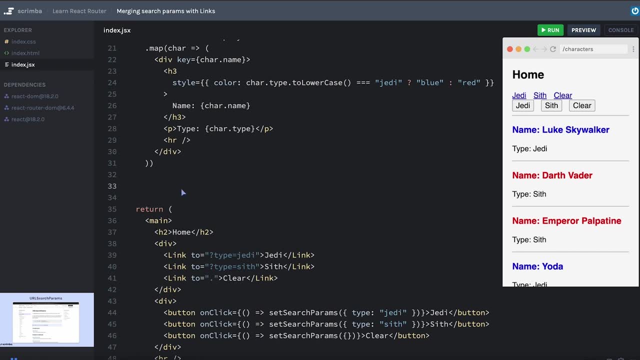 And an important thing to know about that is, we won't even be using the set search params, for that will truly just be using vanilla JavaScript in a sort of helper utility function that we'll create right here. And the second part is how we can do that using the set search params, because there's 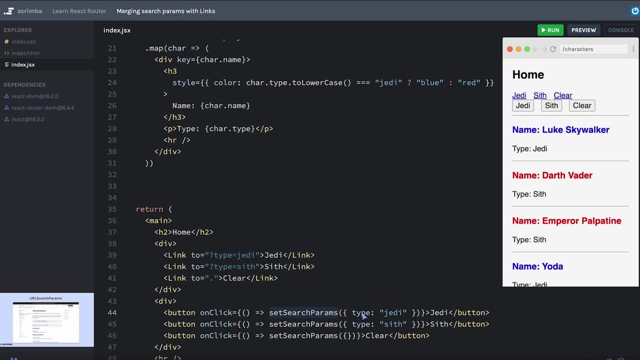 some gotchas with using the set search params method. that tripped me up for quite a bit of time. So let's start with how to generate a query string like this. This does require us to understand the URL search parameters constructor a little bit, but it's not too bad, It's just vanilla JavaScript. 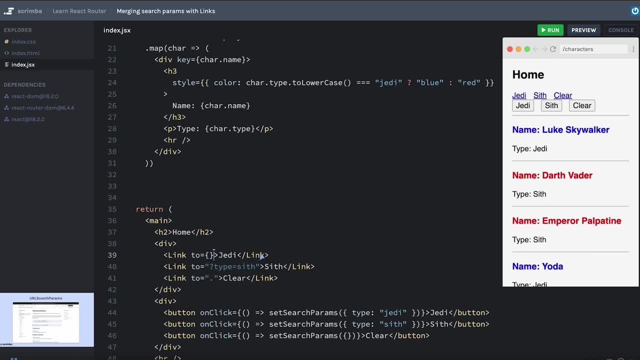 The idea is that instead of hard coding a string, here we're going to call a function, But this time because the to prop is not an event handler, like on click is. we can't pass it a function like this because it will just never get called. Instead, we are going to run a function as soon. 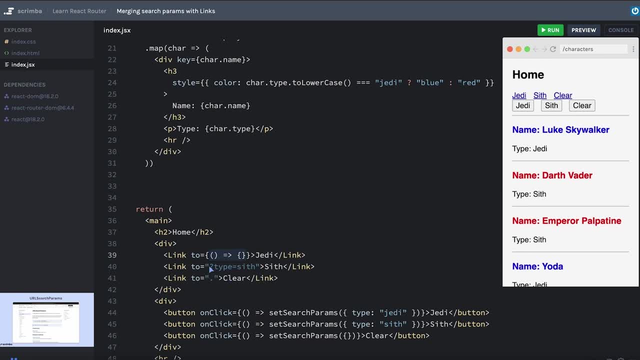 as this component loads And that's going to be called a function, And that's going to be called a function, And that function is going to generate a string which will get put in its place inside of the to prop. So let's get rid of this callback function And maybe we call this generate or gen. 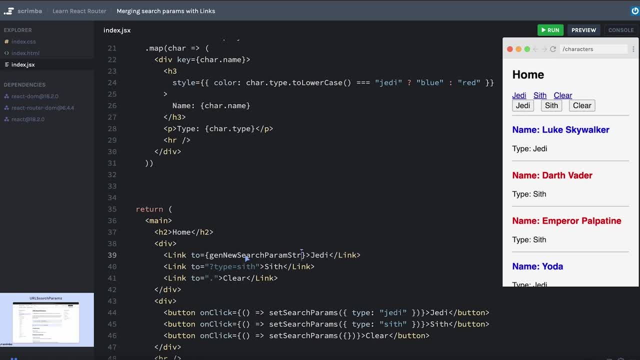 new search param string. It's kind of a mouthful And I'm going to make it so that this function will take a new key and a new value And in the case of the Jedi link, we're going to say that the key is type and the value is Jedi. 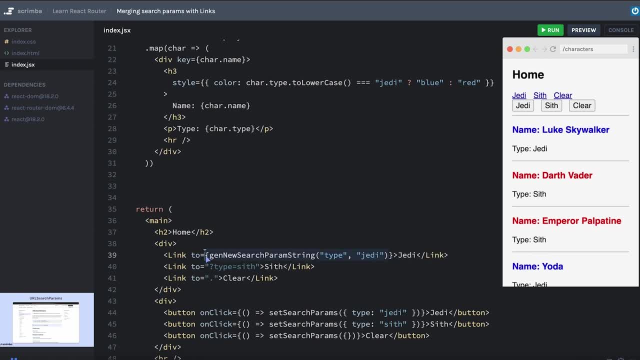 Keep in mind, I haven't written this function yet, So nothing's going to work quite yet. But let's go ahead and copy this to this one, And here we will say: what we really want to do is change the type to null, Or in other words, we'll just remove the type property from the search. 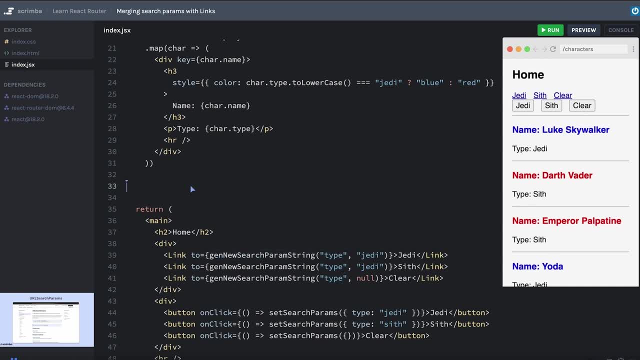 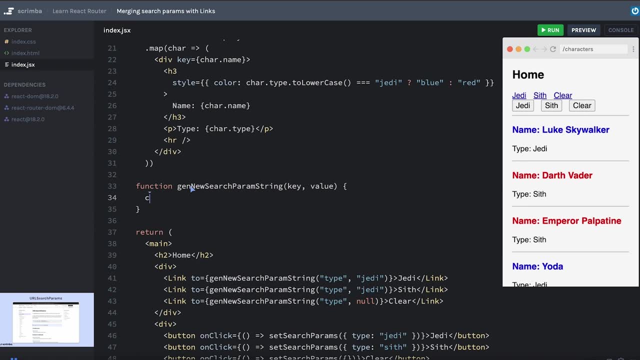 params entirely. Okay, let's actually create this function. So I'll say function gen search params. this is going to take a key and a value, like we mentioned, And what we're going to do is create a new set of search params, And I'm going to do that by using the new URL search params. 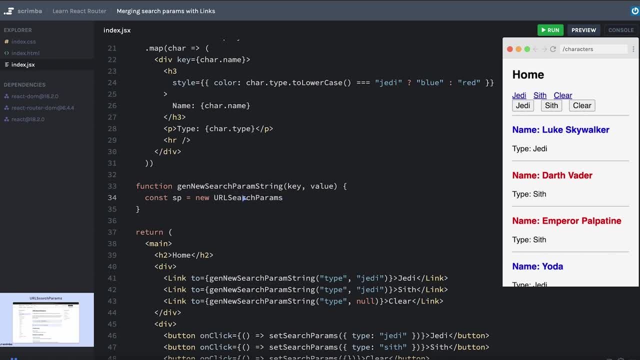 constructor. Keep in mind this has nothing to do with react router. this is completely outside of the purview of react router. at this point, the only thing we will use is we're going to initialize our new URL search params with the value of the old search params. We didn't talk about this before. 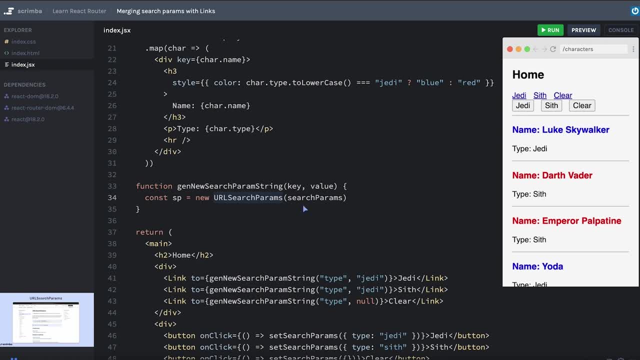 But you might remember I mentioned that URL search params is very flexible in how you can initialize it And you can take another URL search params object and use that to create a new set of that to initialize your new URL search params. So that's what we're doing here And then all we're 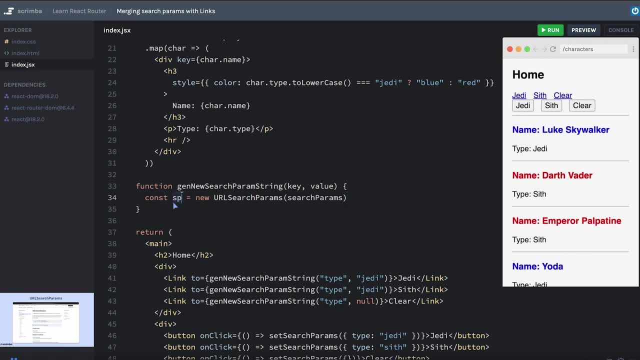 going to do is use those methods that we briefly mentioned, like dot set and dot delete, in order to alter the search params object that we just created. Now, we do have a couple different options for value. it could either be a string, or it could be the value of null, And so we're going to check. 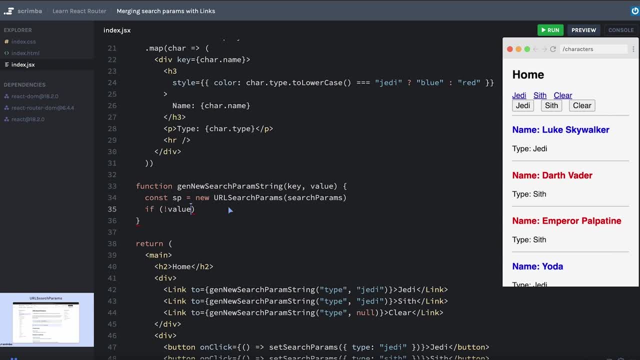 for that we'll say: if there's no value, or maybe more specifically, if the value is equal to null, then we're going to use the method dot delete. on the search params object. Again, this isn't something that I've taught per se. I'm just showing you one possible way to do this. Maybe I'm teaching this more to solidify. 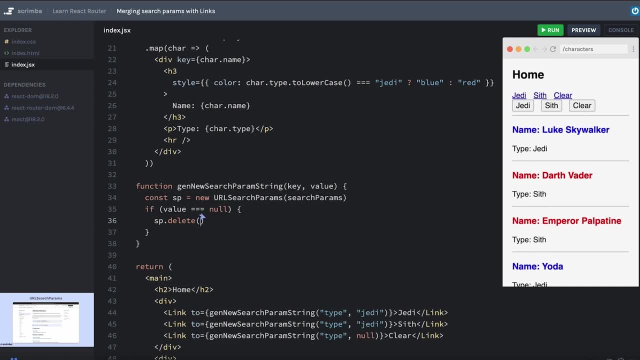 it for my own understanding, since this was such a struggle for me to grasp. Okay, and for the delete method, we're supposed to pass a string of the key that we're trying to delete. we know that it's going to be typed down here, But since we're passing that in as the value of key or the, 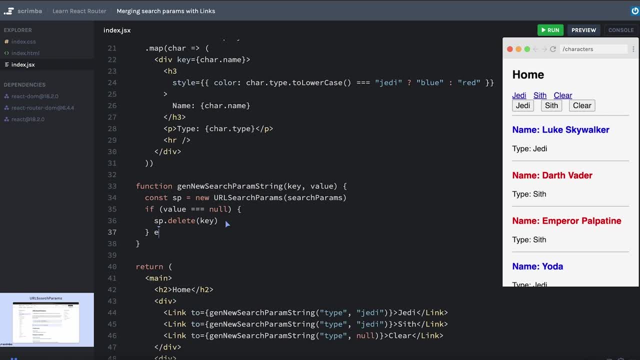 parameter of key. so we'll just say SP dot, delete key. If the value is not null, we'll say else. then we want to use a method called set, And set is going to take two parameters: it takes the key and the value. In our case this will say set the search. 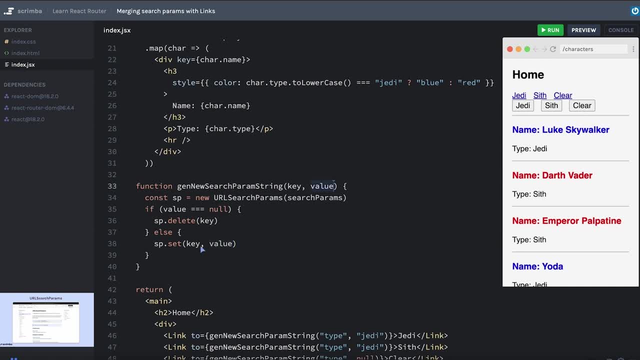 parameter of key equal to whatever the value is that we passed in. So the key that we passed in will be the key. the value that we passed in will be the value. Now we need to return something from this function because it's running as soon as the component loads And we know that we want it to. 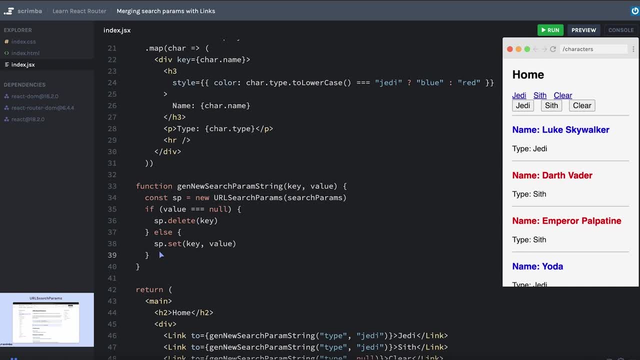 return a string that has a value of null. So let's say that we want to pass a string that has a value, a question mark at the beginning. Let's go ahead and consolelog sptoString. This is another method that we mentioned, And we will see what that generates for us. Again, it should run as: 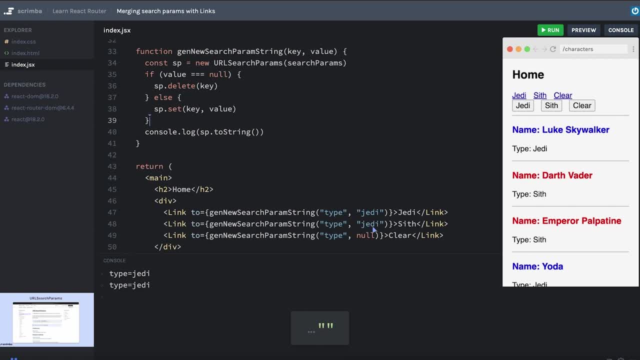 soon as we refresh the page. Okay, we get type equals Jedi. Oh, I forgot to change this one to Sith. Let's do that. Okay, we get type equals Jedi or type equals Sith now, And so we want to return that. Let's go ahead and return sptoString, But we also want it to start with a question mark. So 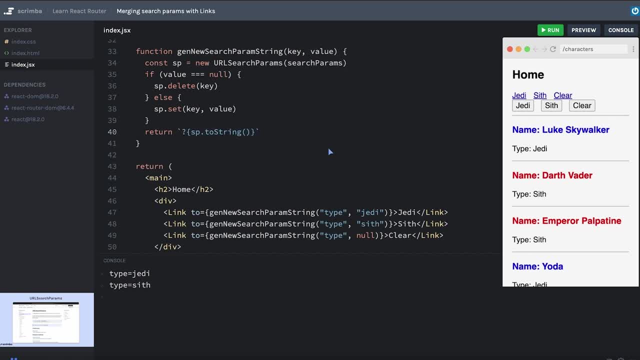 let's just go ahead and put that into a template. literal, we'll say question mark and then we'll interpret the value of sptoString there. Okay, let's hit save, Let's click on. the buttons are not quite ready, But let's hit. well, they should still work like they were before. Okay, so the 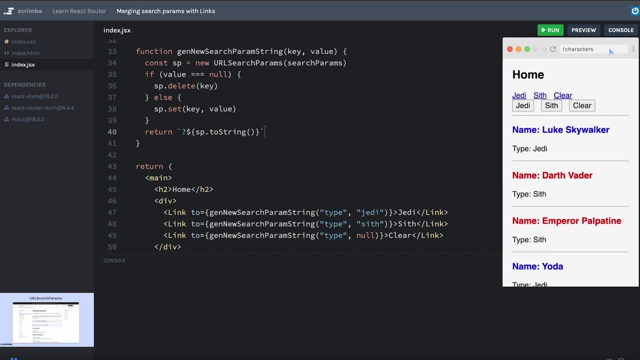 links are working just like they were before, But now let's go ahead and add name equals Bob And I'll click the link For Jedi And look at that. it actually concatenated. the ampersand type equals Jedi on top of the name equals Bob. Now let's go ahead and hit Sith, just to make sure that that's working. 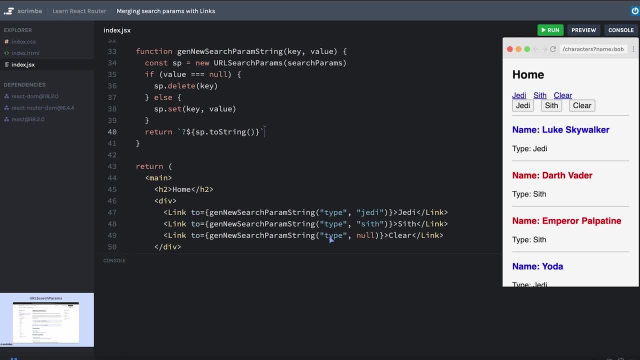 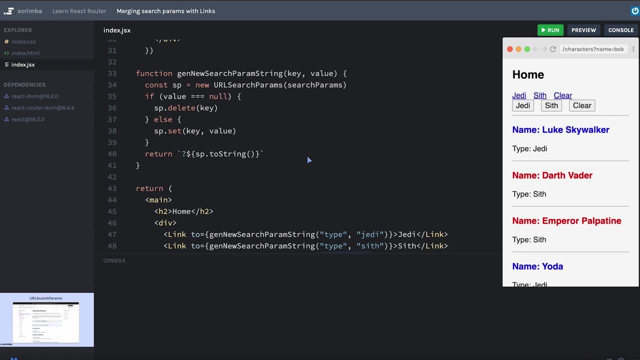 And then we'll hit clear And, sure enough, it only got rid of the type property on our search params. Okay, again, this is not something specific to react router, But because it was such a struggle for me, I really want to at least have some reference to how you could do this in. 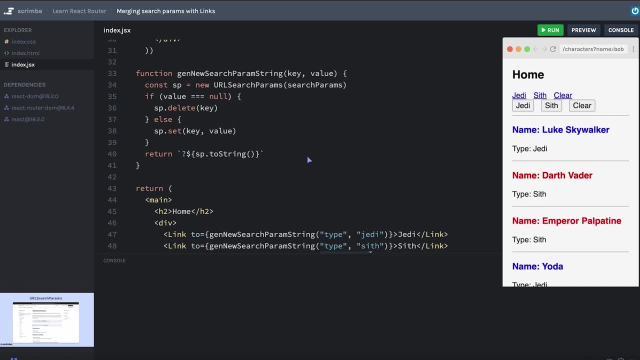 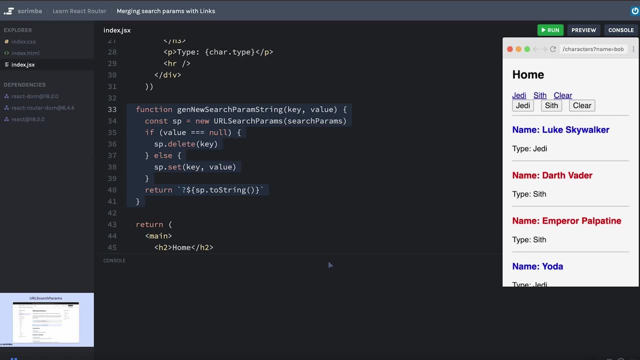 case you run into this problem so that you don't have to spend three or four days down a crazy rabbit hole trying to figure out how to do this In the end. I guess that's a little disappointing because this isn't a whole lot of code to solve this problem, But that's okay. 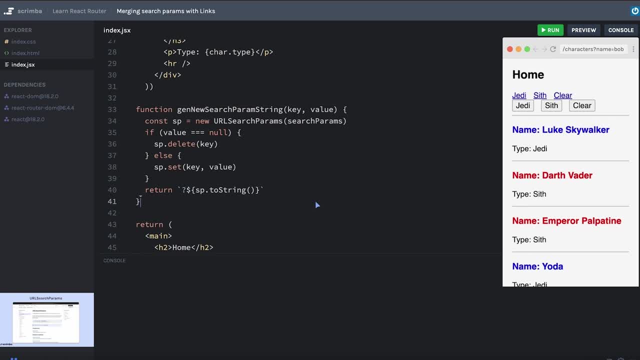 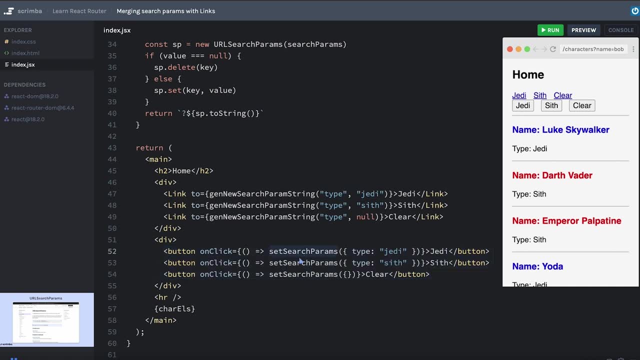 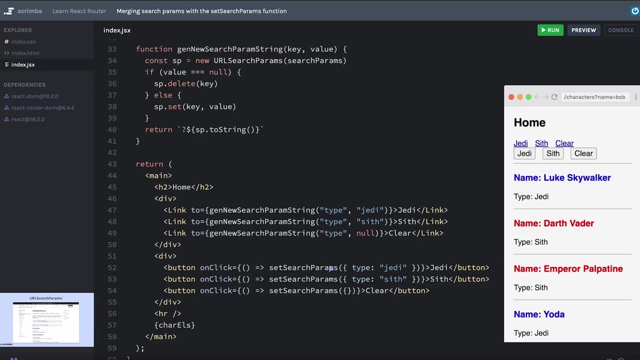 Sometimes in the pursuit of education, that's just what happens. Okay, in the next section, let's actually tackle how we might do this using the buttons and the set search params setter function. Okay, let's tackle doing this in our buttons as well. I mentioned a few times how the use search params. hook is going to work. So let's go ahead and do that. And let's go ahead and do this in our buttons as well. So let's go ahead and do this in our buttons as well. So let's go ahead and do this. 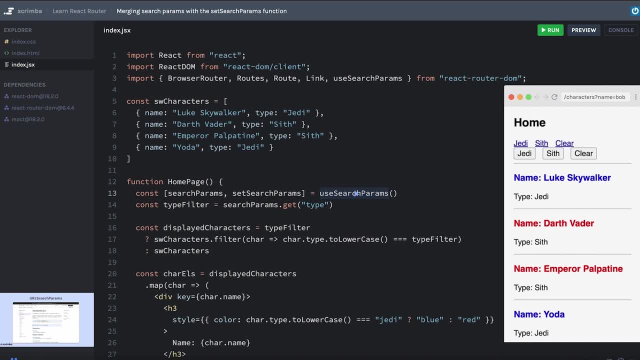 is very similar to the use state hook from react, And it's not just in that it returns an array with two items that include the value and a function for setting the value, But, more deeply, the function for setting the value can take two different kinds of parameters, just like in use state. it can either: 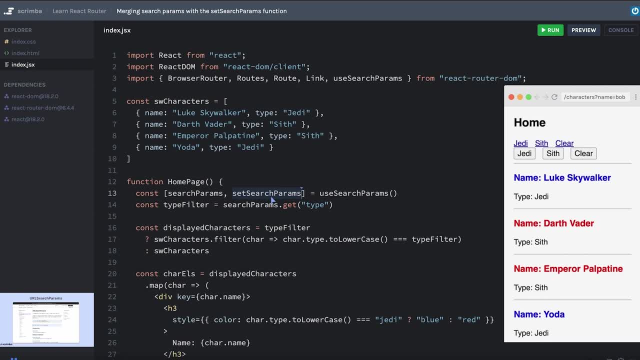 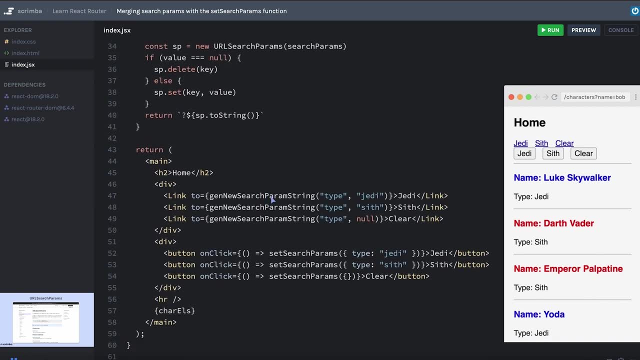 take a replacement value for the state, or it can take a callback function And that callback function will receive the previous state so that you can use it to make changes to it. Let's see what that looks like. We're going to need a little bit more room than just doing this in line. 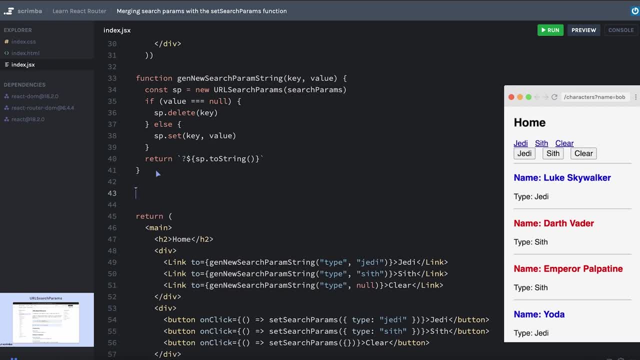 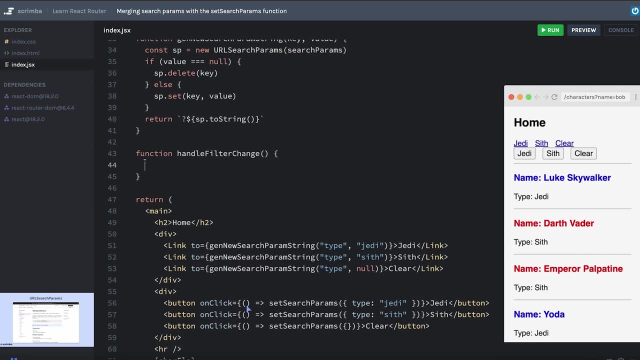 So below our gen new search param string function, we're going to create a function that's called maybe handle filter change. we'll just get rid of everything here And actually we are going to need to take a parameter. we'll probably call this the new filter or the maybe new type, And we will 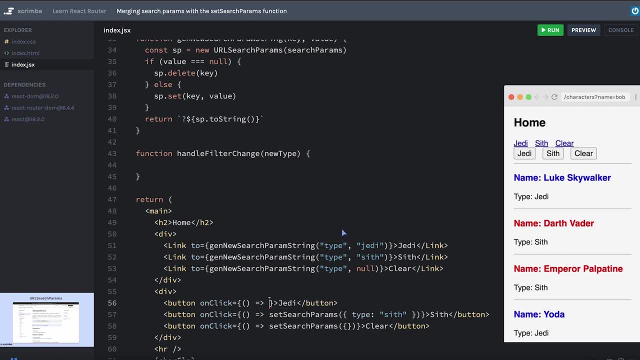 change everything here. Yeah, I think that's right. And we'll say: handle, filter, change parentheses. and then we're going to pass in the new type. we'll say: is this one is Jedi? And then we'll just do the same for these other ones. 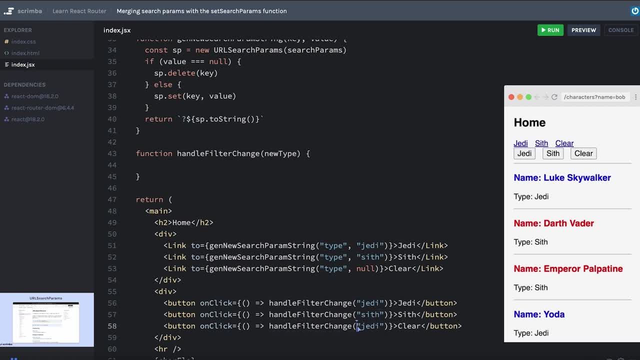 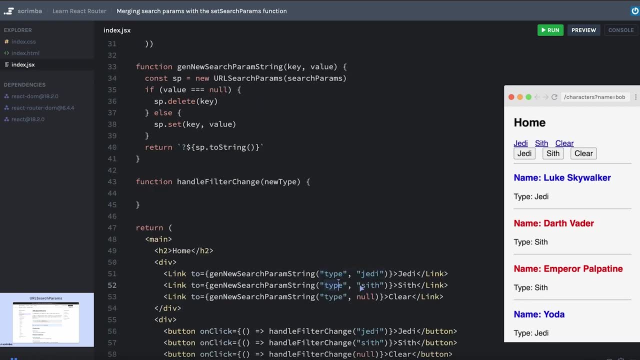 This time I'll remember to change this one to sith, And here we will pass in null. it might have been overkill to pass in both the type parameter and the actual value parameter or the key and value up here, Since this function is currently living in the place where the only 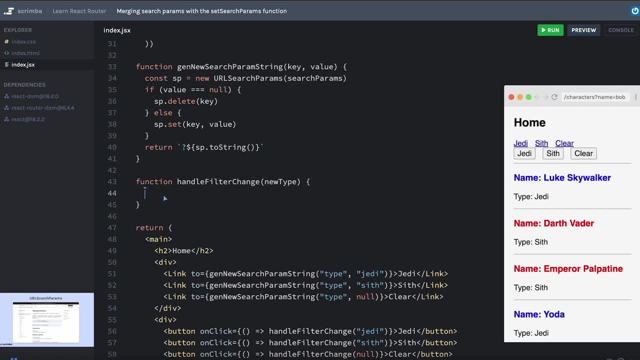 thing we're changing is type. I guess I wrote it so that we could eventually move this function out to some kind of utility folder and theoretically use it across the entire application in other circumstances other than type, Maybe just for the sake of being similar. I'll do the same thing here. 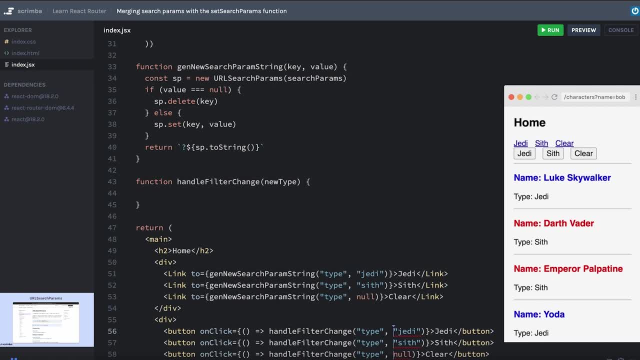 So we'll say we're going to pass in the actual key of the key value pair, and then we will not just take the new type, but we'll take the key as well. And what the heck? let's make this more generic too. We'll just call it value. Okay, back to what I was saying, The setter function. so we 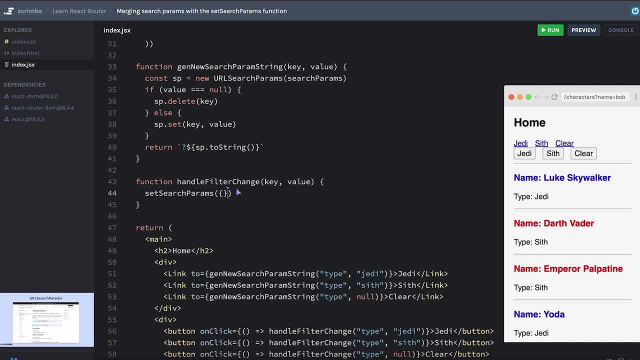 called it setSearchParams. We were just using it where we just passed in a new object that represented the replacement for the params, but we found that that completely overwrote any other parameters that we might have. Just like the state setter function with useState, we can pass. 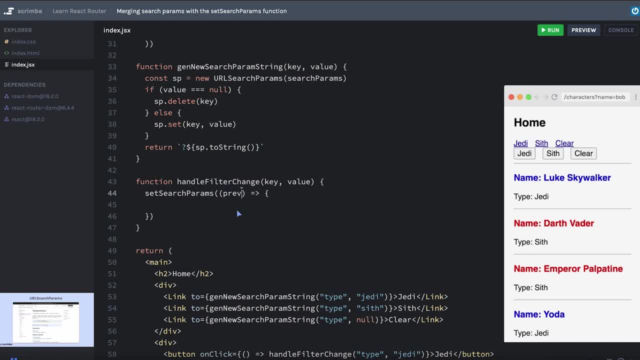 in a function and this function will receive a previous version of the params. Because it's an arrow function and we just have one parameter, I can get rid of those surrounding parentheses and we will do something very similar up here. We'll check if. 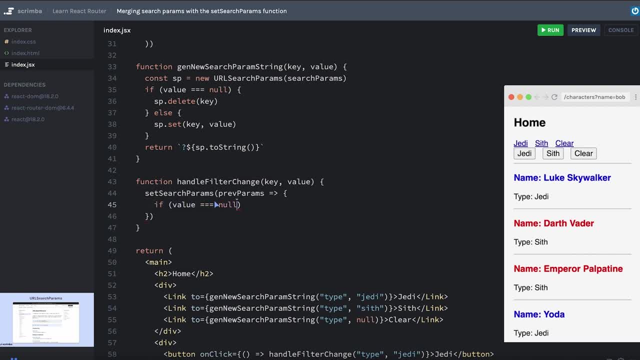 the incoming value is equal to null. Now this is where the setSearchParams setter function diverges pretty dramatically from the state setter function. In the state setter function, we would never take the state that we received here and make any direct modifications to it. Instead, we would. 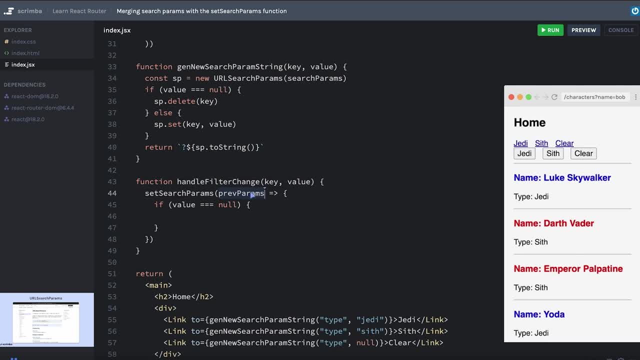 always create a copy of it somehow and only use its old values in order to determine the new values, and we would return a completely new state. As far as I can tell- and I've confirmed this, with the way that React Router has some of their internal tests set up, it's completely okay for us to modify the 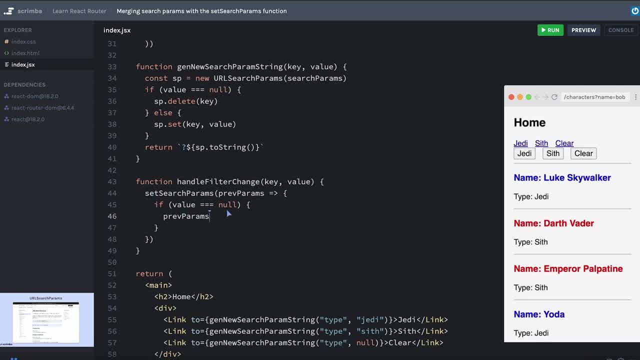 previous params object. So in this case I'm going to say if the value is null, then we'll run previousParamsdelete and it'll be the key, whatever key we pass in. If the value is not null, then we'll say prevParamsset- whatever key and then whatever value. And at the end- because in 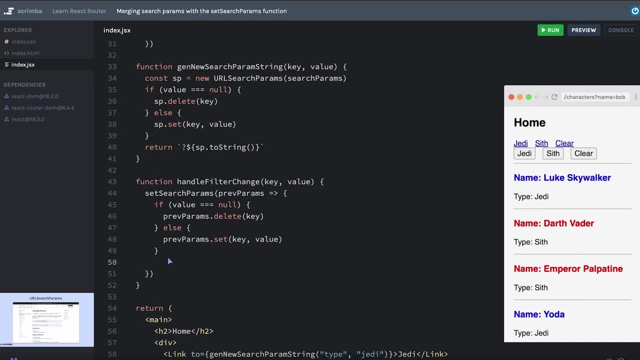 this case. we're not trying to turn it into a stress episode. we're going to give it a value of 6,5, string. we're trying to set it as a URL search params object. we're just going to return the. 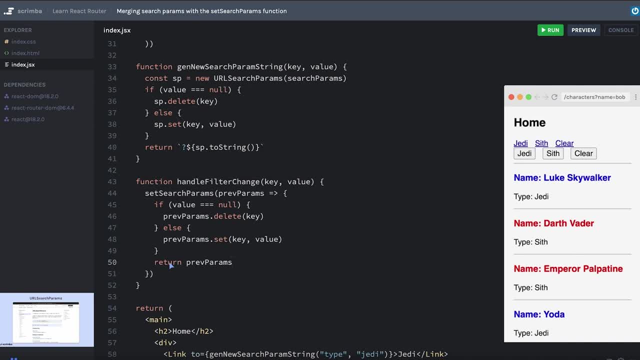 previous params. Again, this feels a little icky to me because I'm used to having the state setter be where you never modify the original object. But as far as I can tell, this is okay And I think that's all the code we need. Let's hit save Again. our links were working before. we still have the. 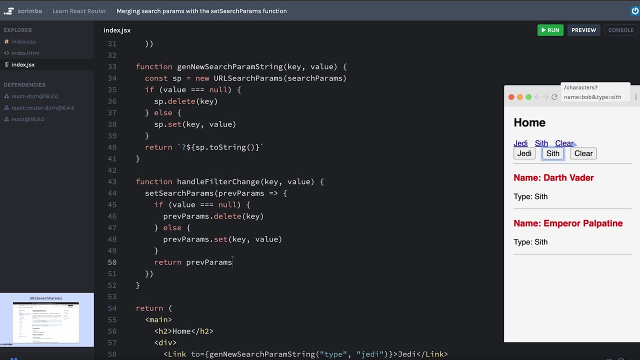 question mark. name equals Bob up there. Let's go ahead and hit Sith. Okay, it appended it to the string. That's great. Same with Jedi and clear clears out the type, but it does not clear out the name. Now you could go even further down this rabbit hole. The truth is, search params can have. 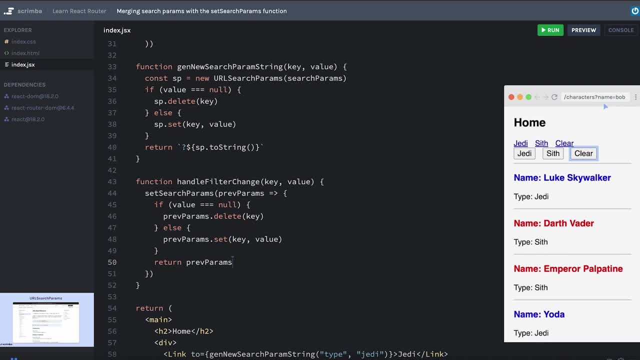 the same key multiple times. So, for whatever reason, if I wanted to, I could say: name equals Bob and name equals Joe, or type equals Jedi and type equals Sith, And the way that we've written this, it would clear out. Okay, I just had to confirm it. Yeah, it would actually clear out. 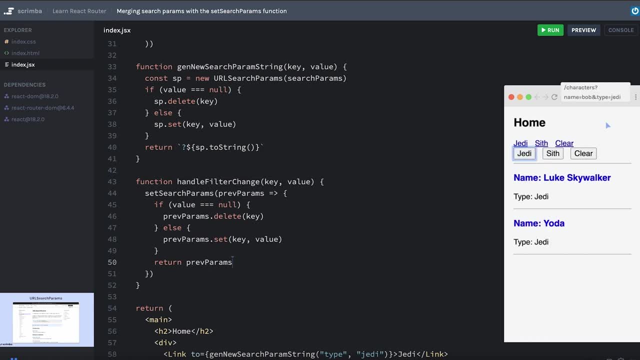 both types In fact. let's just see it in action. Well, let me start out. type equals Jedi. we'll get rid of name equals Bob, just to buy some space. Okay, question mark type equals Jedi and percent type equals Sith. So you can see that, okay, it's got both the clear function. 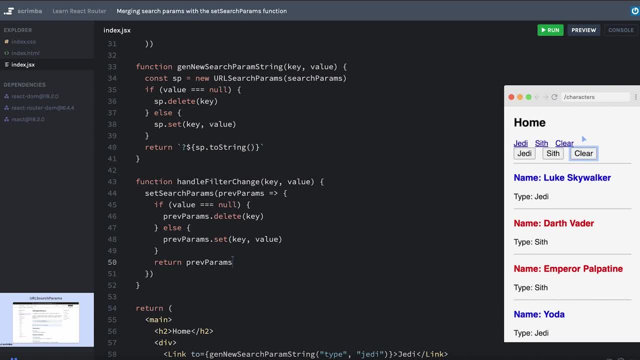 we'll just clear both of them out. So that might not be ideal. you would have to get much more complicated to actually search through the params object and only delete the type that you're trying to delete. But now we're venturing into a realm that's much past the scope of this course, In fact. 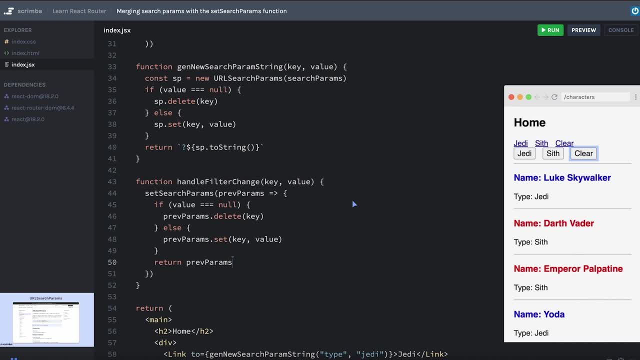 we might have already done that a little bit here, But that's okay, it's all great learning And hopefully I can save someone out there at least a few hours trying to struggle with understanding this. With that behind us, let's go back to the 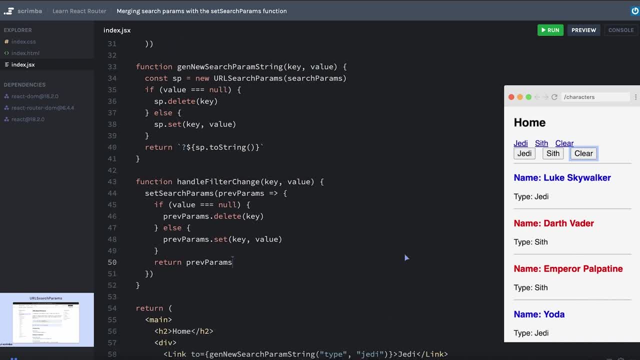 van life app. I'm going to implement some of these changes for you, since it is, like I mentioned, a little bit outside the scope of this course, And you know what? let's lighten it up a little bit. we'll have a pretty simple conditional rendering challenge. So that's what we'll do in the next. 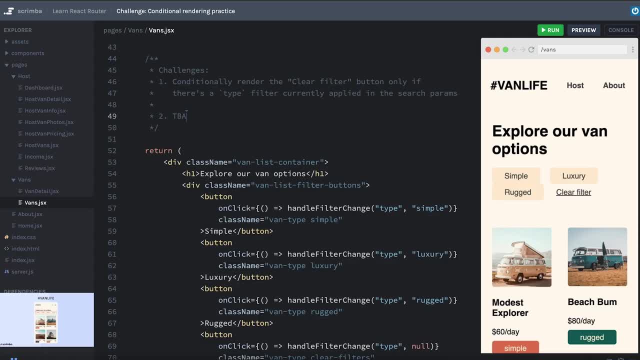 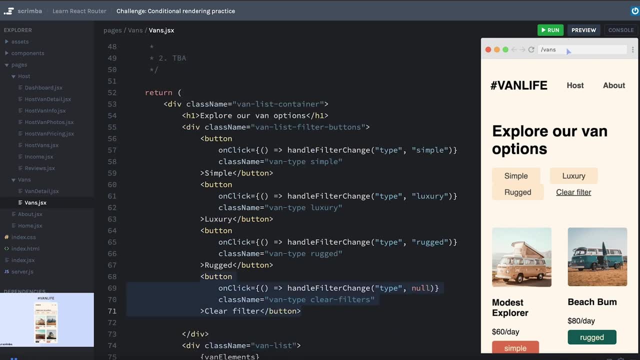 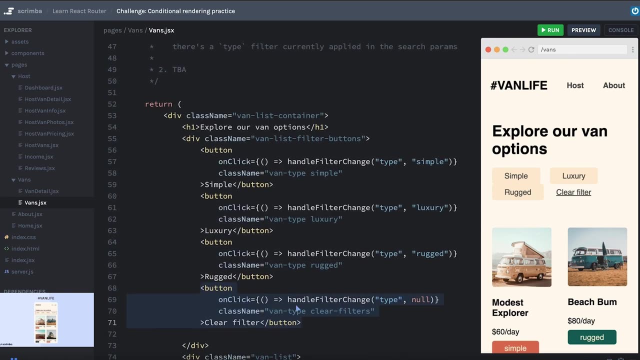 scrim. Okay, we'll actually be doing two challenges. The first one is to conditionally render this clear filter button Only if there is a type parameter currently being applied in the search parameters. We've been working a lot down here at the bottom of the file and changing the search parameters down here, But 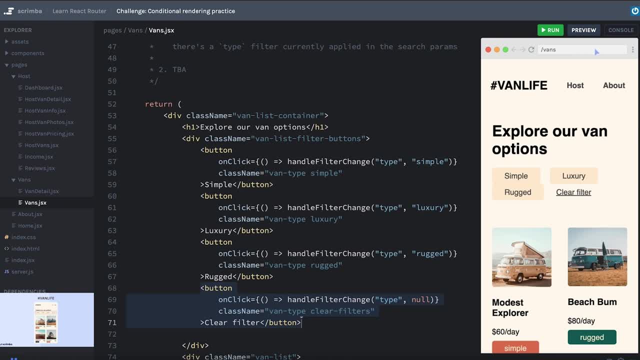 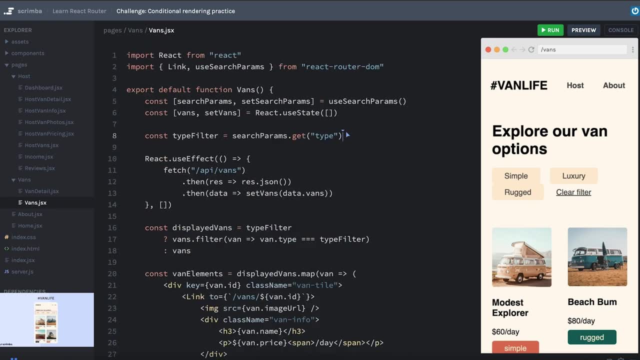 remember, every time we navigate to a new URL, even if it's the same base URL with a different search parameter, this entire component is getting re rendered, which means we have this value up here called type filter, which will always be up to date with the newest filter that we've applied. So 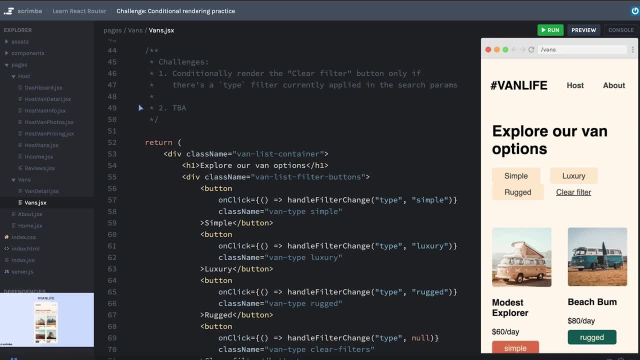 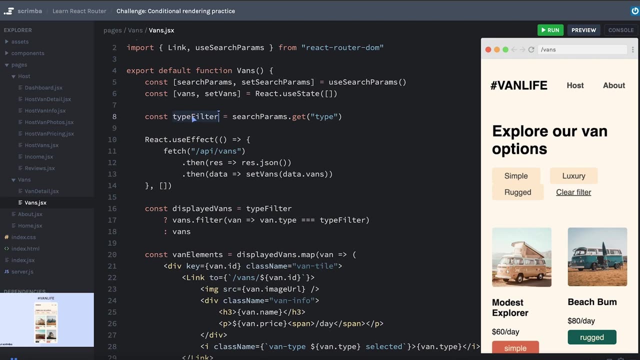 understanding that conditionally, render just this button and then we will be able to render this filter And we will jump into the next challenge right after that. So pause now and work on challenge number one, Because this whole component is getting re rendered. we have this type filter variable which will tell. 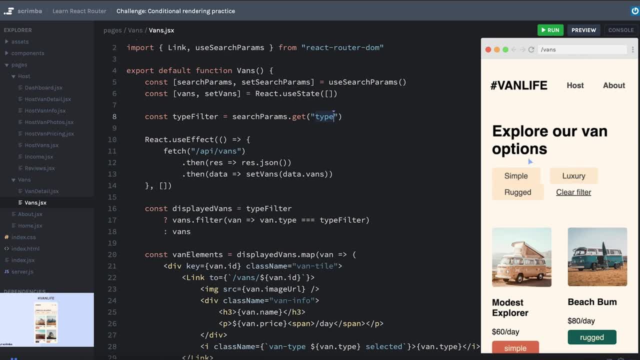 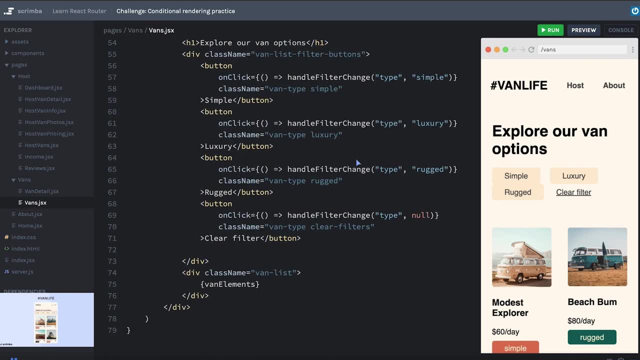 us if the type is existing. So it'll either be simple luxury rugged or it will be null if there is no type parameter in our search parameters. So I can conditionally render this clear button by first wrapping it in a set of curly braces And we'll just use some shorthand here. we'll say if type. 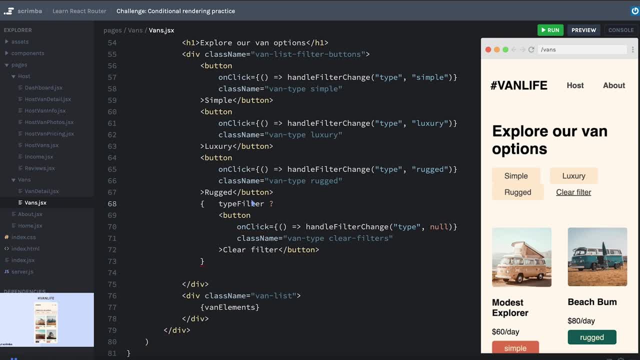 filter exists, it's got a value, then render this button Commonly. we will put something like a set of parentheses around the component, like that, And then we'll say: otherwise render no. so just don't render anything there. Okay, let's clean up the formatting a little bit. I'll put a little space. 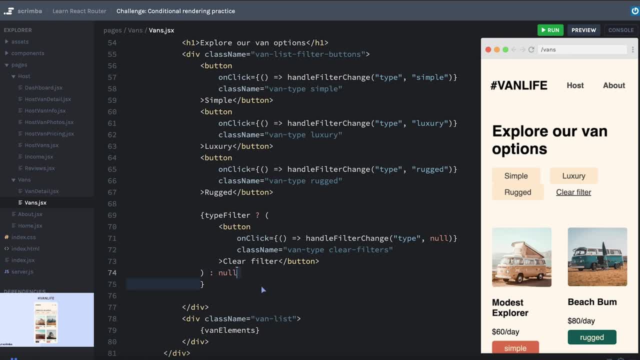 here too, in case that's easier to read, And for some reason I want to put this on the same line. I don't know if that's better Or worse, but it should be clear either way. Okay, let's go ahead and hit Save the clear filter should. 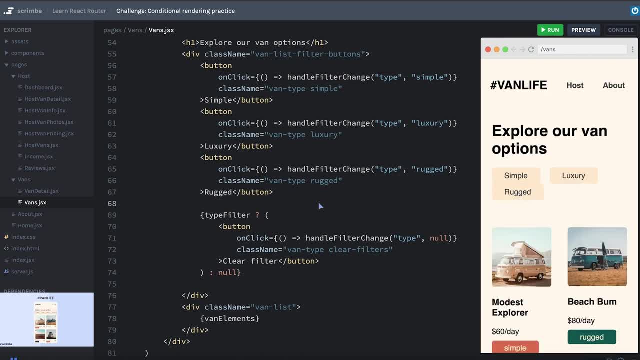 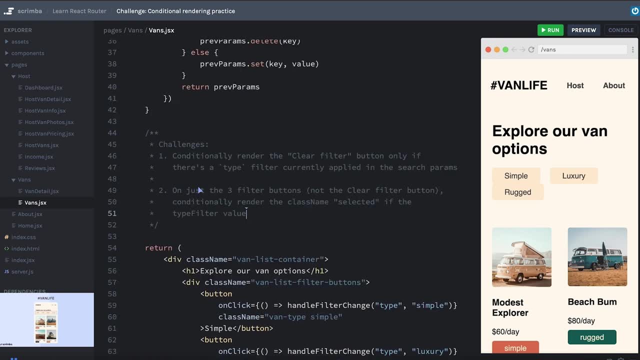 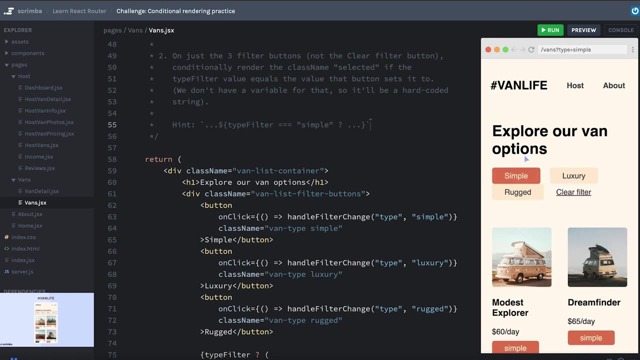 disappear. Perfect, because we don't have any parameters right now, And then when I click on these, it appears Awesome. Okay, let me type out the challenge number two for you. Okay, one of the things that's added in our CSS is, if there is a filter applied, then that color that you see when 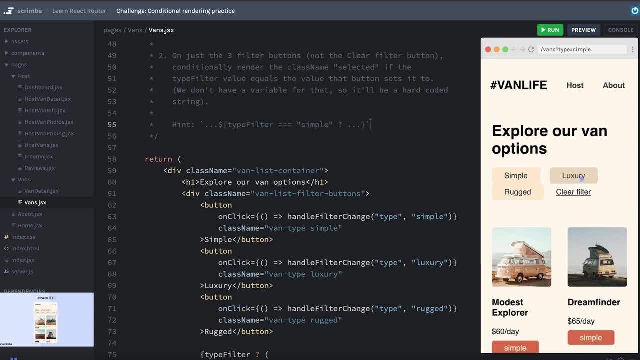 we hover will actually stay on the button as long as that filter is applied. Currently it's not doing that because it's only showing that on higher. However, there's a class called selected that I created in the CSS. that should make it so. 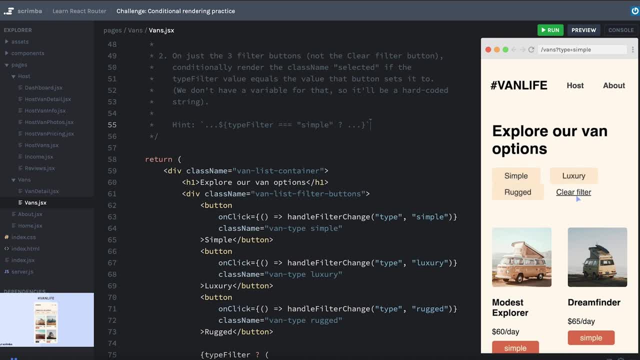 that it will stay that color if that filter is applied. Well, more specifically, if that class exists on the button. So your task is to conditionally render the selected class name if the type filter is equal to the value that the button wants that filter to be. I hope that. 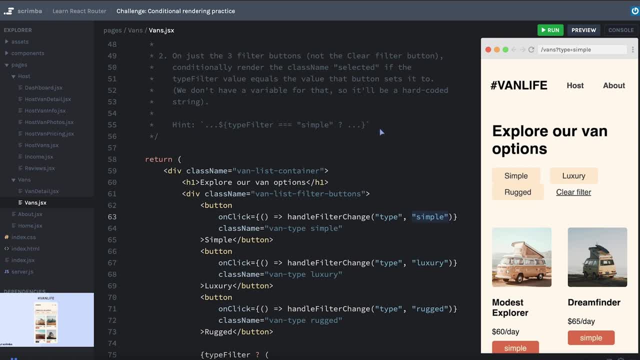 makes sense. I give you a little bit of a hint here, since it's a little bit difficult to explain, But notice here that I'm using template strings, But down here we are not. we're just using regular quotation marks. That's something that you will need to change. Oops, not there here. 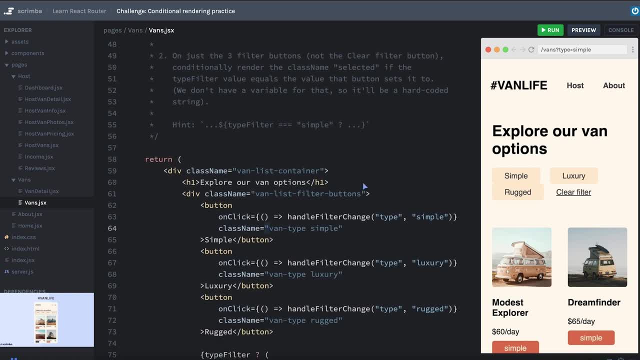 Okay, pause now and work on challenge number two. Okay, this line is going to get a little bit long. In case you're working on a small screen, I'm just going to squish this which clearly I haven't optimized my styles to handle a really 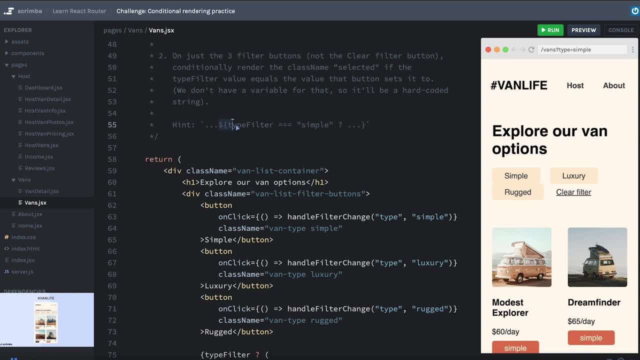 really small screen like that. So, because we're going to be interpreting some JavaScript inside of this string, we're going to use string interpolation, So I'm going to select these class names And we'll change this to a template string And oh. 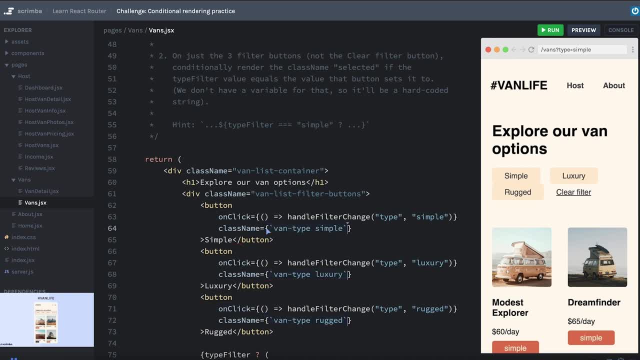 I need to surround this with curly braces- Awesome, Okay, and now I'm going to stick in my dollar sign curly braces. So I can say: if type filter is equal to- and then we will just grab these values here- Simple, luxury or rugged- then we will apply the selected class. 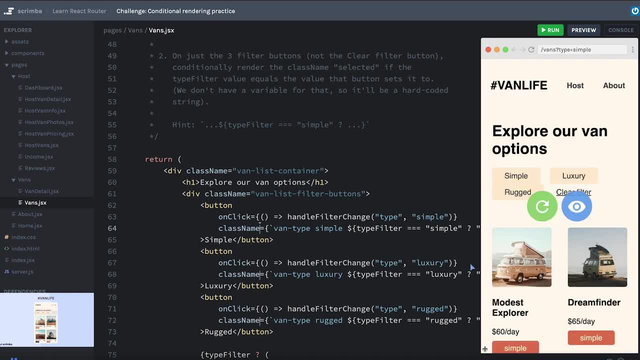 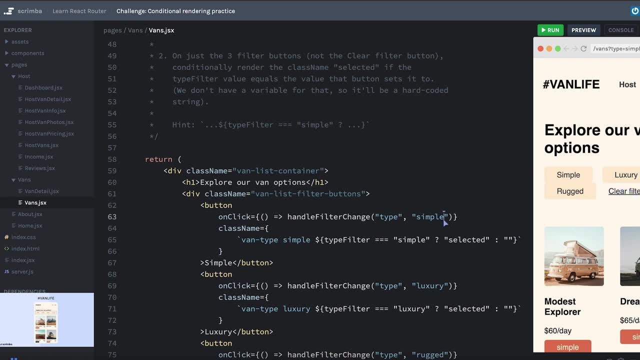 but otherwise we'll leave it as an empty string. You know what? just in case that is a little too wide, let's go ahead and just put this on the next line, like that. okay, first let's hit save. and well, this is good news. the simple is already highlighted, because when i 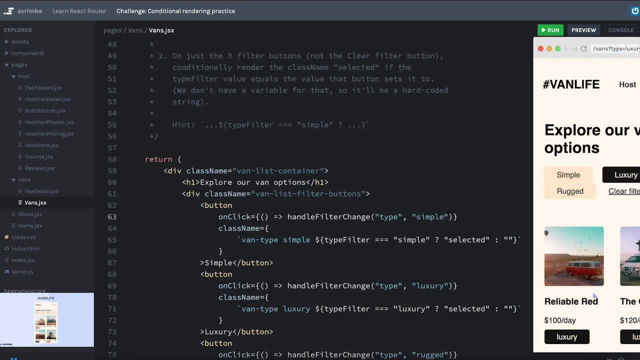 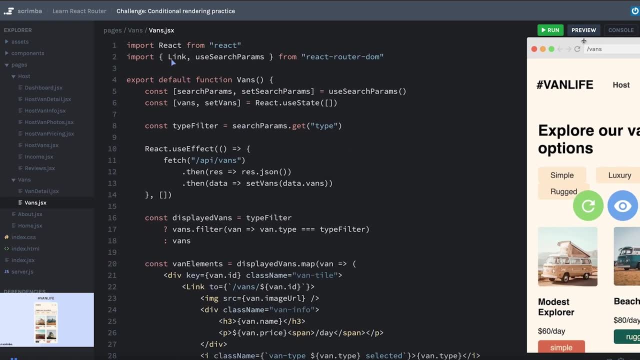 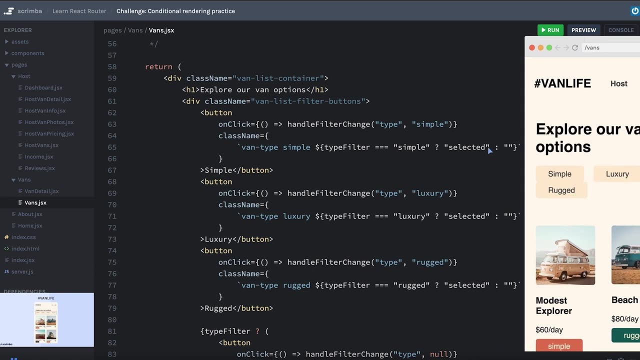 hit save, we had clicked the type equals: simple before, okay, luxury, rugged and clear now. just by way of information, one thing that i tried to do was use a nav link to accomplish the same thing, but it turns out the nav link does not care about your search parameter. so when i used a nav link, 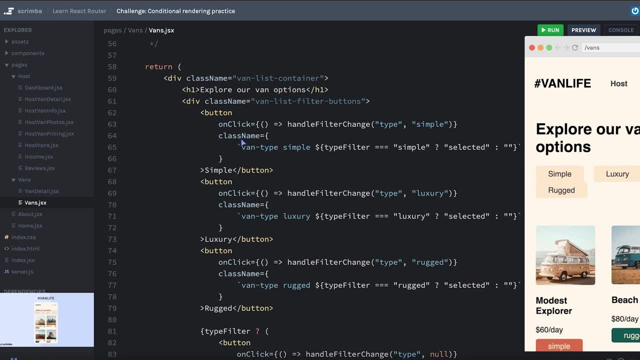 and i accessed the is active property on the render prop class name and tried to use that instead of the type filter equals the simple. it just didn't work well. what happened is all of them were highlighted because this route slash vans is active and the two prop was sending them to. 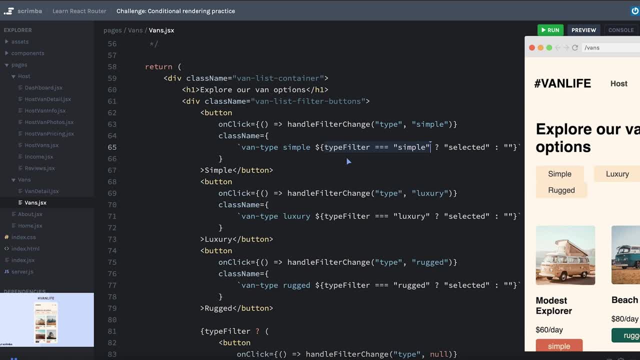 the same path. it just was changing the query string. so just a little extra information for you, as if there wasn't already enough to try and digest in this course. all right, at this point we have just a few more little odds and ends that we need to add to our app, so we're going to start working on those. 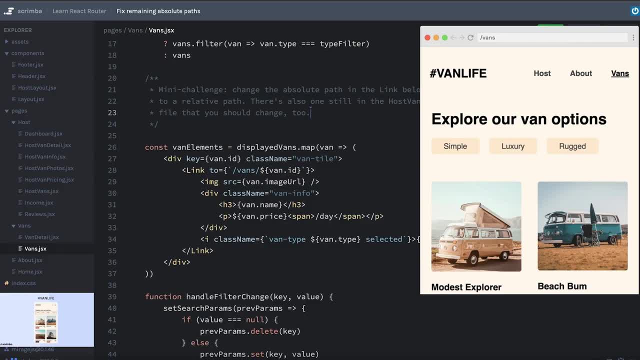 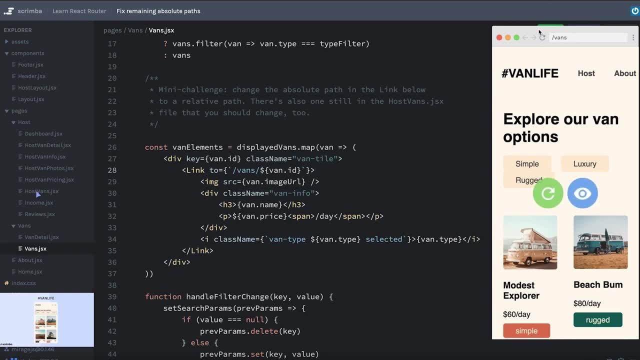 check it out, i found a loose end that i just forgot to fix when we were learning about relative paths, because here we have a link that still has an absolute path. i actually also found one over in the host vans page, which you'll go check out next, so i'm going to make 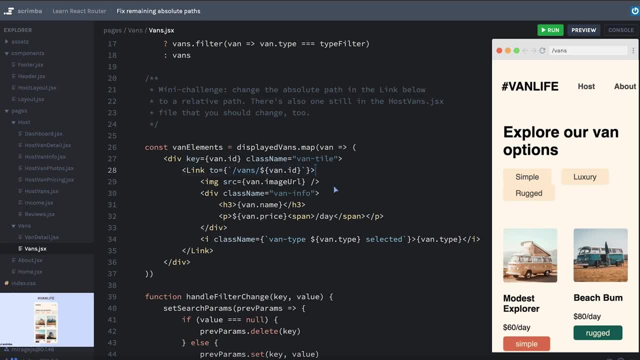 you make these changes, change the absolute path in this link and the one over in host van dot jsx to be relative paths. pause now and work on these many challenges. we know it's an absolute path because it starts with a slash, and so we had to give the 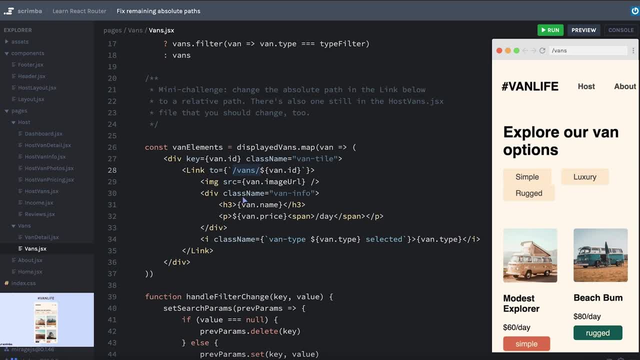 entire route all the way up to the id here. but we don't need to do that because we're already living within the context of slash vans and so we can just get rid of slash fans and then the slash and we can just have the van id. however, i can actually take this even one step further. 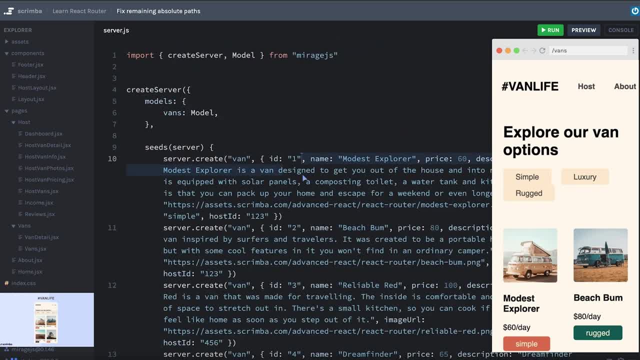 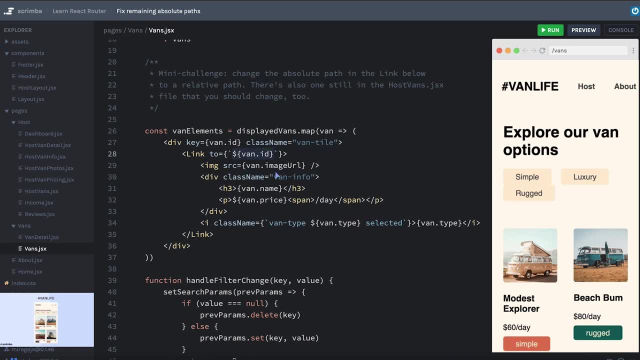 if we look closely at the server, the ids are strings already, and so rather than create a template string and then just the only thing i'm rendering is the value of the id, we can just get rid of our template strings entirely. let's say van dot id. like this: we can hit save and 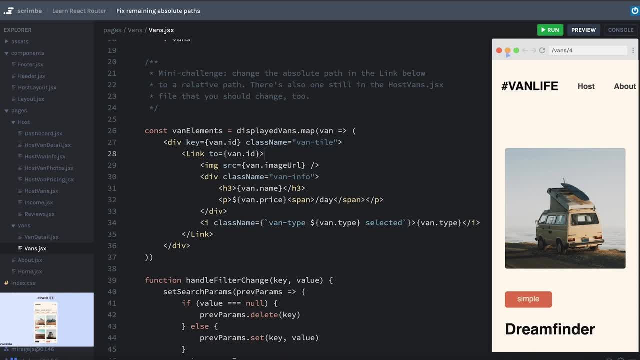 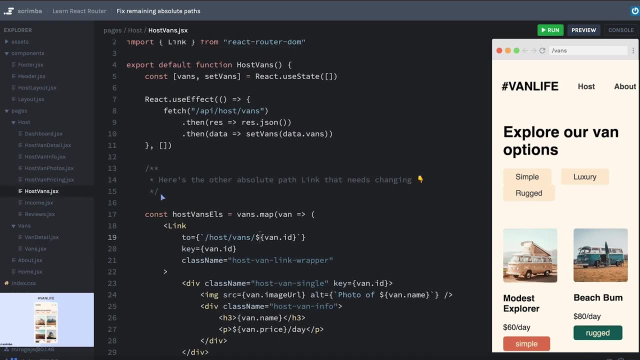 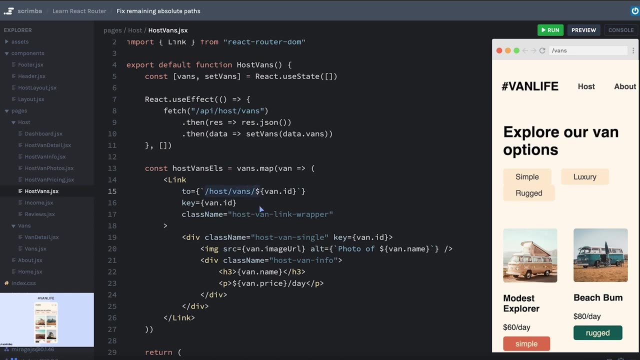 we can see that these are working just like they were before. okay, let's clean this up and let's head over to the host vans page. we're just doing the same thing, so we're going to hit, I'm going to clean this up too, and here we have slash host, slash vans, slash id, and we can just do. 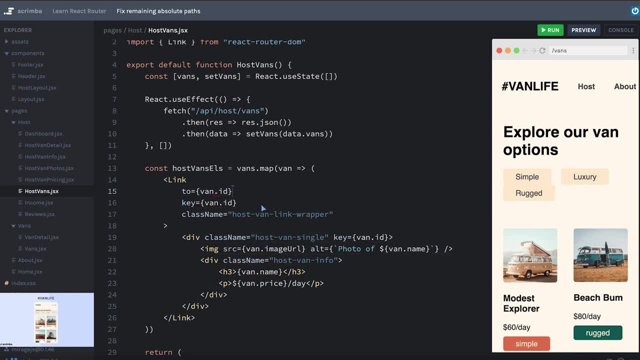 exactly what we did before and just display the id, because again, this component is living within the context of slash, host, slash vans already, and so the link is relative. to say, just append the id on the end of the url, we'll hit save, go over to host vans and clicking on any of these, okay, works. 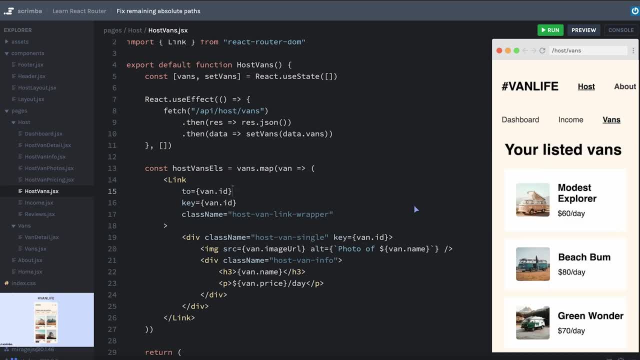 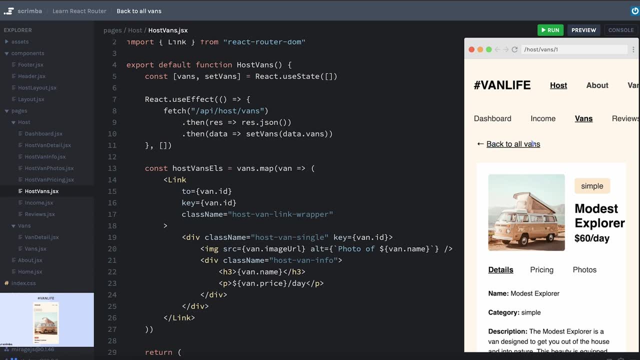 great. okay, there's at least one more loose end we need to clean up, so we'll do that next. the design did show this back to all vans link inside the host vans detail page and we already implemented that. however, the design also shows that there's supposed to be one on the regular. 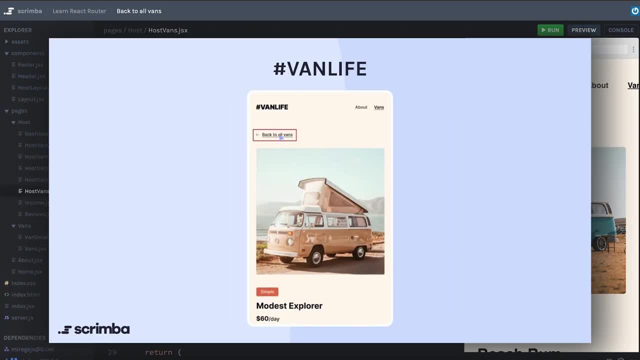 full list of vans detail page. you can see it here. we're supposed to have back to all vans. now. there's actually a bunch of different ways to implement navigation with reactivation and navigation, so we're going to go ahead and do that here and we're going to 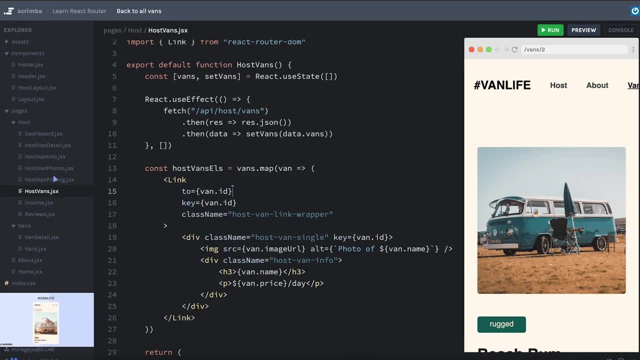 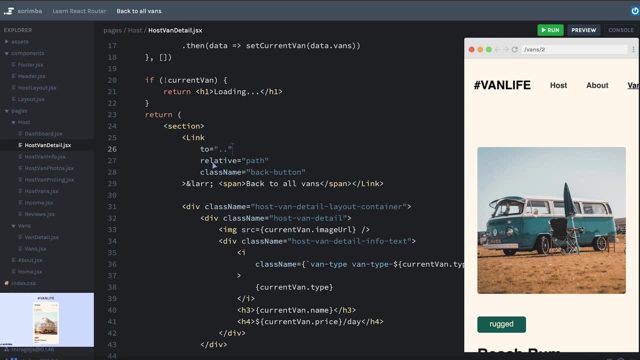 and we've already seen using the relative. let's see where is it, host van detail, this relative dot dot path which takes us up one level, and we talked about the relative equals path, which makes it so that it's a back button relative to the path, or rather it takes us up one level on the path. 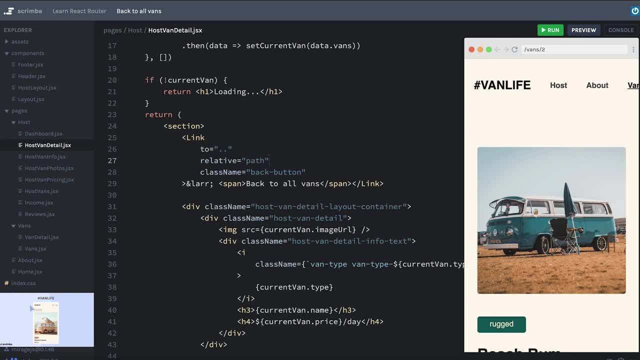 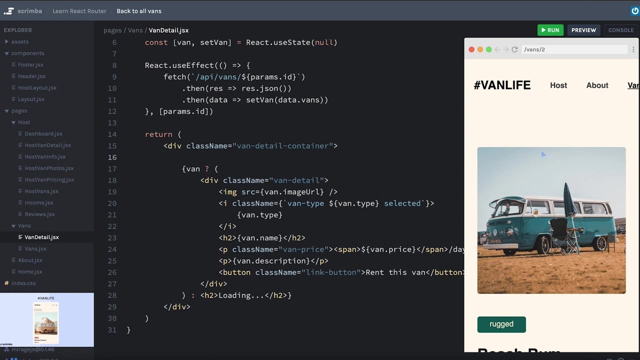 but not one level in the route hierarchy as we have here. so one thing we could maybe think to do is go here, just grab this link. we'll come to our host vans- no, our vans- detail page and then just right here above, where the van is supposed to go, we'll 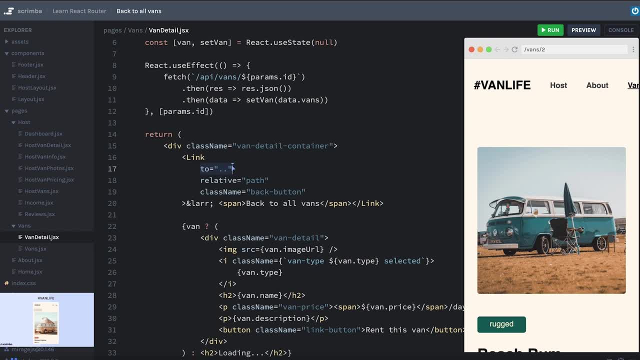 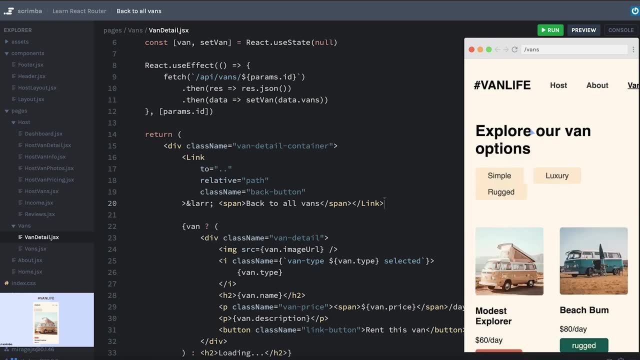 just stick our link. one thing that's, i guess, kind of nice about this is we have relative paths, and so i think this should just work. now we have back to all vans, we click it and, sure enough, it takes us back to slash vans. okay, we could just stop there, but let's try to think of the user's workflow. 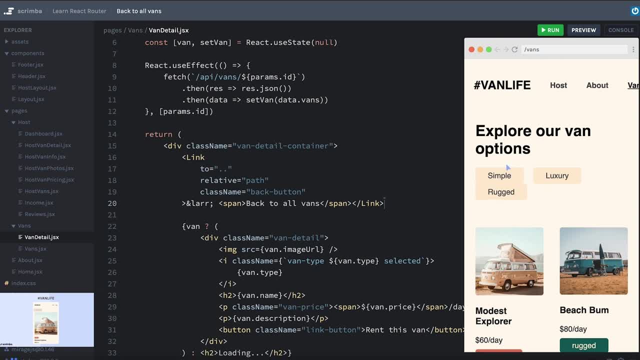 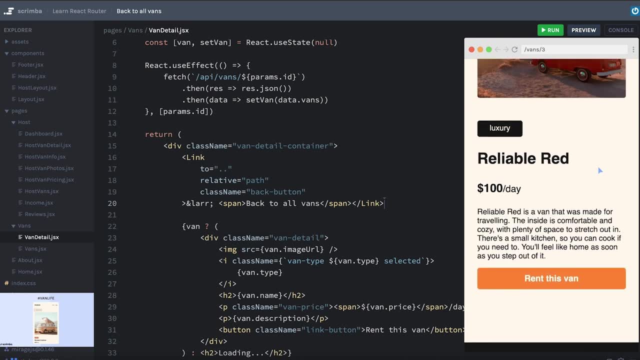 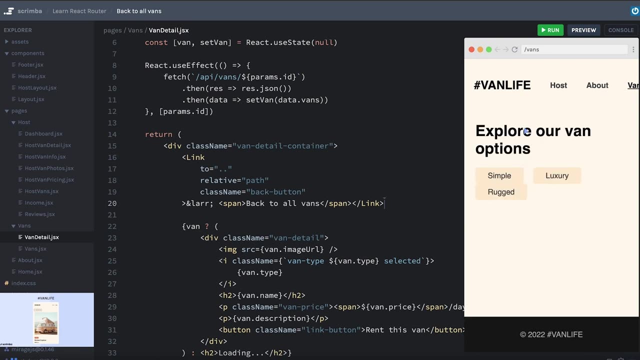 here. maybe they're on the list of vans page and they filter by, let's say, luxury. they click on good, reliable red, and they maybe look at this and say, oh, that's not for me, i'm gonna go back now. when they click back, what is it going to take them back to? well, let's see, we click back to all vans. and now 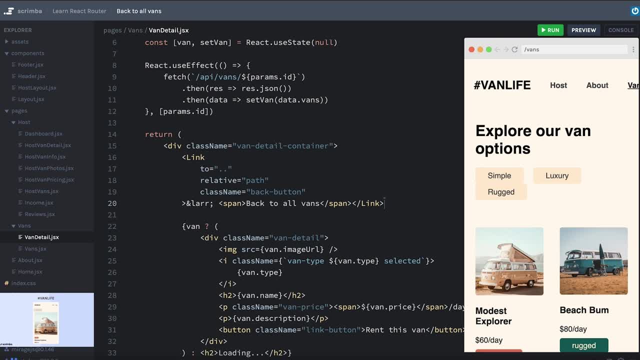 we're back at the slash vans page and they have lost their filtering. of course, with only one simple filter, it's not that big of a deal. but if you imagine something like airbnb, where you set up maybe four or five or six different filters for what you're looking for, if you were to go into 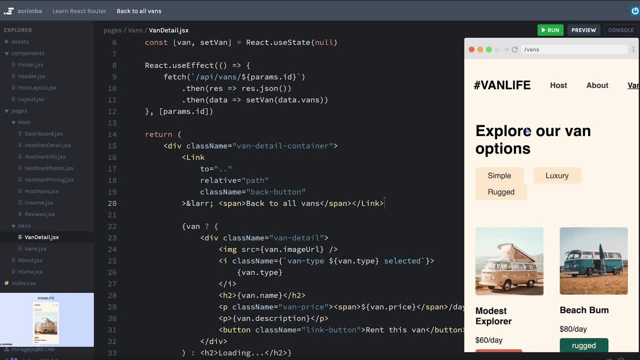 one and then click a link that said back, and it just took you back and removed all of your filters. that's not a great user experience. well, it turns out there's a number of different ways that we can implement: how to make it so that this takes us back to just the vans that we had filtered already by luxury. so that's the next. 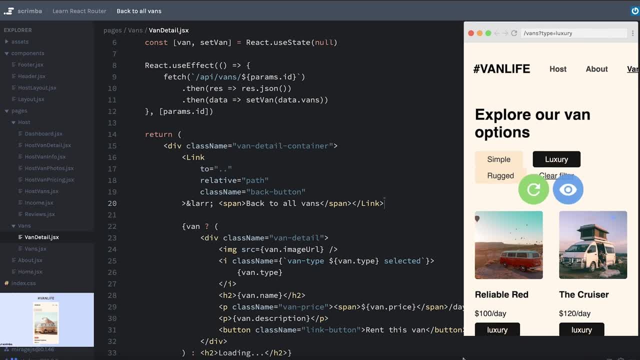 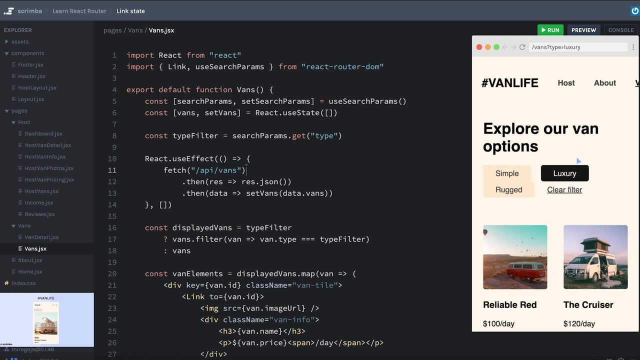 challenge we're going to be working on, but don't worry, it won't be too difficult. that's what we're going to start working on next. okay, so we know that we want to be able to filter the list, click on one of the vans and then have. 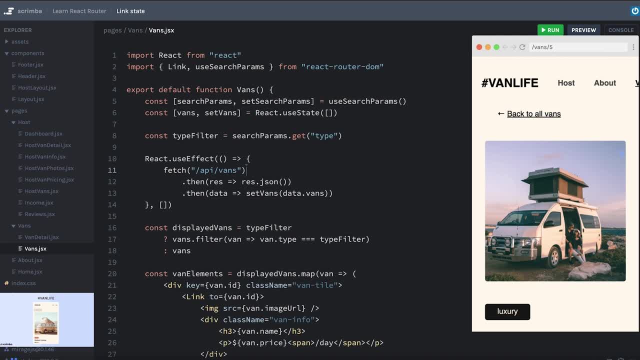 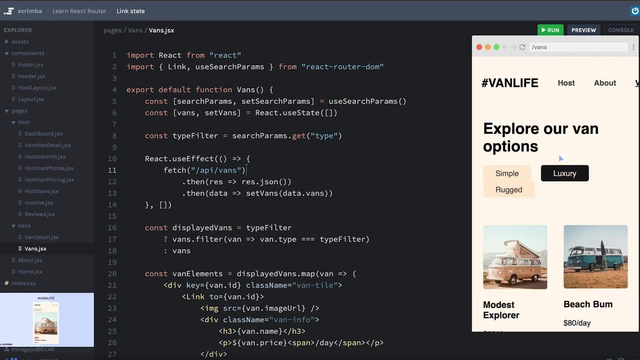 a search parameter, which is vans slash five, and then, when we're on this page, we can create a search parameter and then we can see that we're on the last page. so that's a way to get a lot of information that shows us what the filter used to be. on the last page, like i mentioned, there's 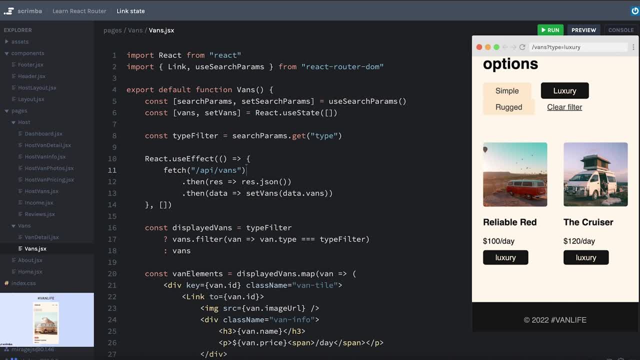 usually a lot of different ways to do things. for example, one way that we could accomplish this is take the search parameter directly from the current url and, instead of linking to slash vans- slash 5 in this example, we could just tack on that query string that represents the search parameters. 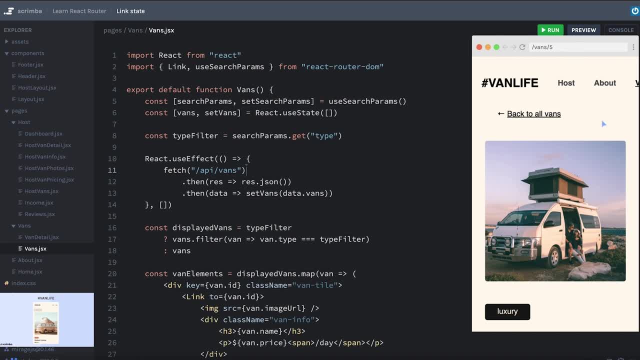 we would have that directly in the search parameters and we could pull it from the search parameters and go back to all vans. That said, I personally don't love the semantics of that solution, and the reason is because if I'm looking here at slash van, slash five, I can already 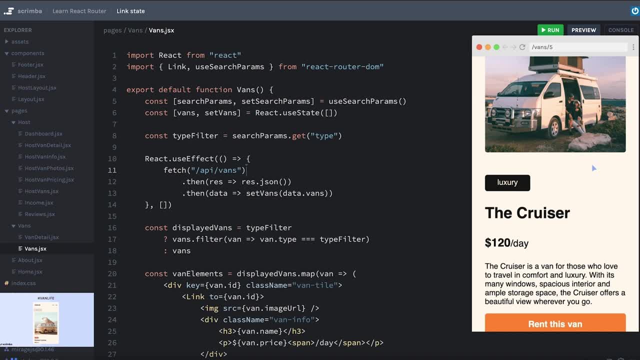 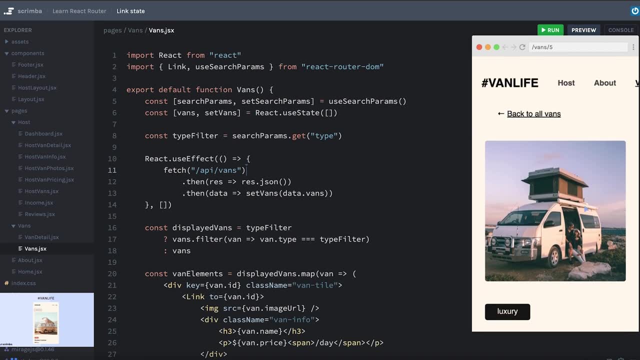 tell that this is a luxury van. The query string at the top that would say type equals luxury would feel redundant to me because this represents a single van, it doesn't represent a list that I can filter down, and at this point we could branch into two different user experiences. Let's say you: 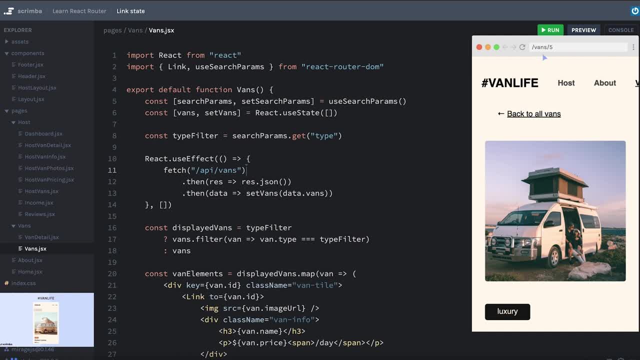 found this awesome van, you're really excited about it. you grab the url and you want to send it to your friend. If it has that query string in there, then theoretically they could come to this page and they could click go back to all vans and it would take them back to just the luxury vans. 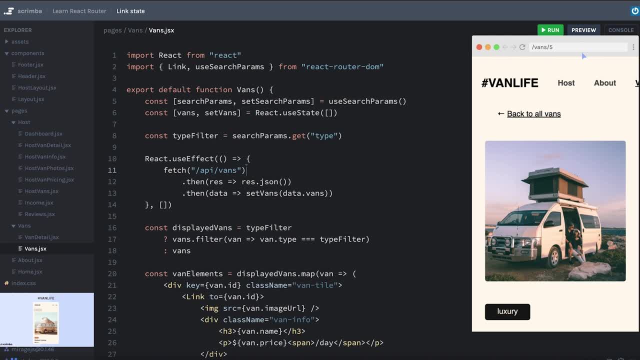 because it's been filtered, and if that's your desired use case, then that's the best way to go. The url is the only thing that will persist from one user to the next. However, my argument would be that that's probably not as common, So for this instance, let's assume that we really don't. 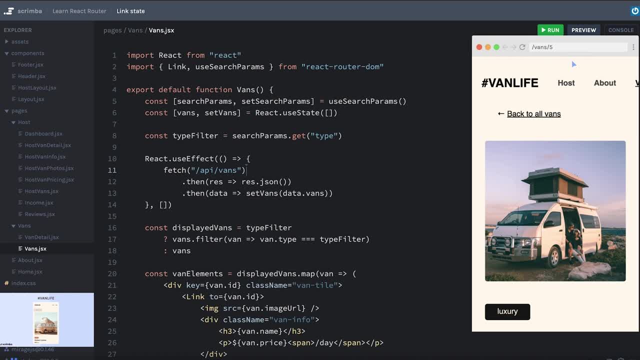 care about the url and we want to send it to our friend. If it has that query string in there, then we don't care about keeping the filtering when we're sharing the url to another friend. and by that I mean on the detail page, When we go back to all vans. if we filter it by luxury, we probably do want. 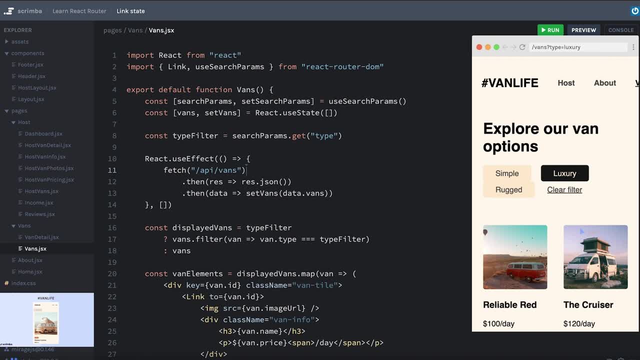 to share only the list of luxury vans when we're trying to decide what van we're choosing with the friend, but maybe I'm making too many assumptions. We talked about earlier how the search parameters are great for something that's going to persist, especially, like I just said, from one user to the 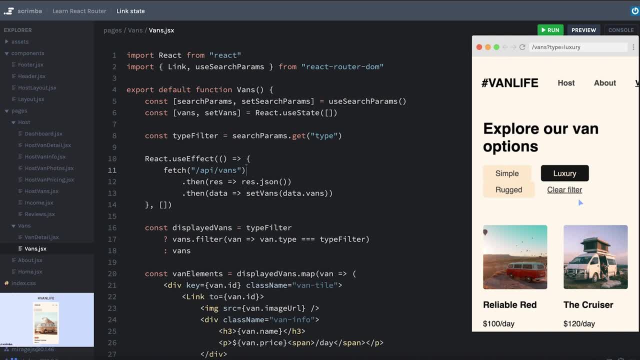 next, but I want you to pause for a second and see if you can remember what is the structure or maybe what is the tool that we can use if we want to save some information while we're still here on our page. but we don't necessarily care if it's going to survive. transferring the url to another. 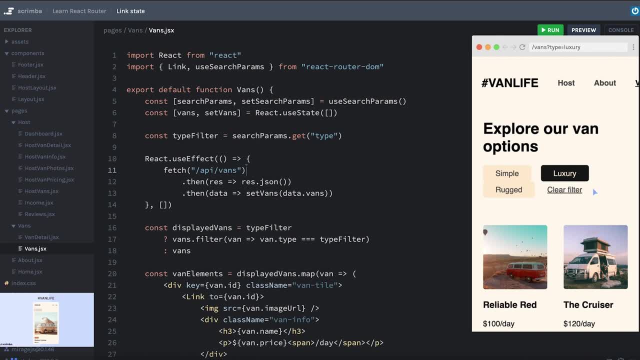 person. That's where state comes in, and in this case I'm not talking about react state, I'm talking about something called history state, and don't let that be scary. The truth is, the browser has the ability to save some kind of state between one link or one url and the next, and react router has made 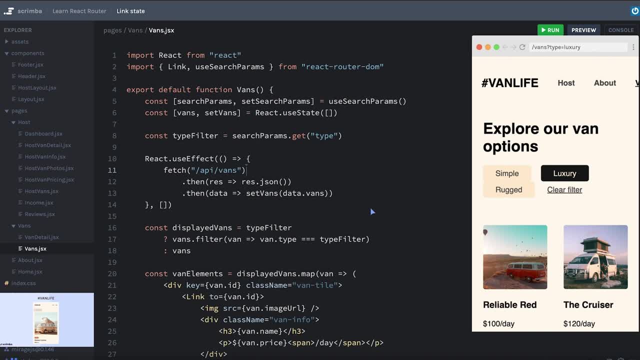 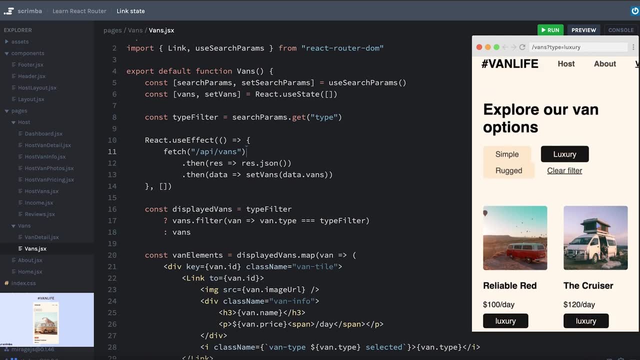 it very easy for us to save the url to another person. So if we want to save the url to another person, we're going to need to add some information to that link state. So first what we're going to do is add some state to our link. We're here in our vans page. this is the vans list page and the idea. 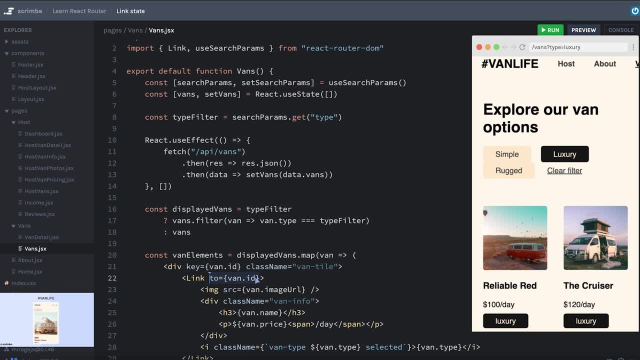 is to say, we want to link to the individual van, but we want to pass some additional information to that page. So the first thing we'll do is see how to pass that state to the next page and in the next scrim we'll learn how to, you could say, catch that state and make use of it. And this here is: 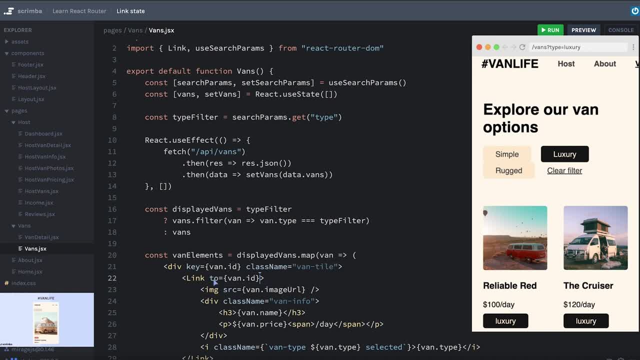 actually so simple. it's not even challenge worthy. When I'm linking to the link state to a resource, I can simply add another prop to my link, called state, and I could set the state to whatever I want. It could be a string, I could just say whatever and when I get to my next route, the 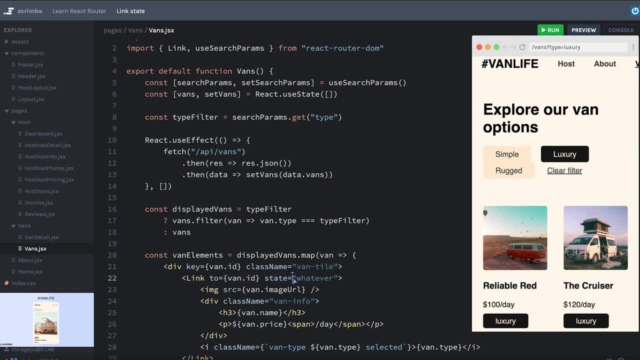 van slash id page. I can grab that state and it will be the string whatever. I don't prefer to pass raw values like this. in my state I think it reads a little better to pass an object, and so I'm going to use my curly braces to get into javascript and then I'm going to pass in an object and the 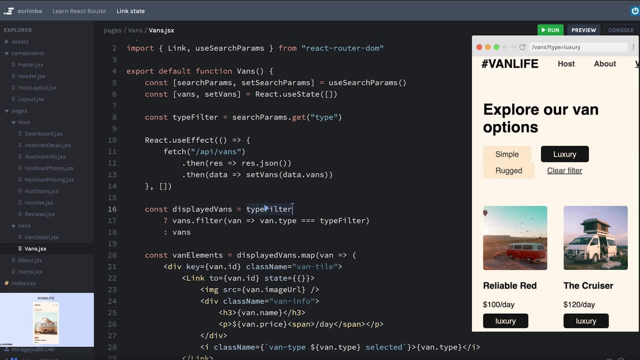 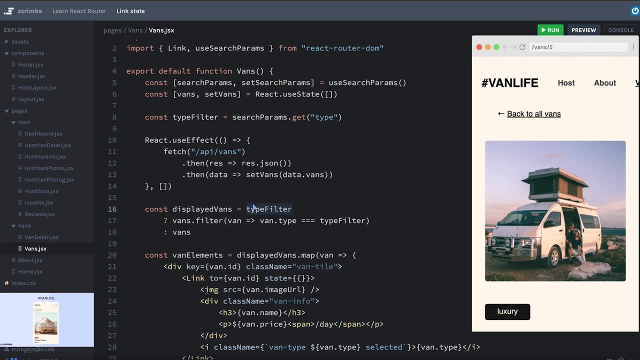 idea here is we want to pass an object to the next route and then I'm going to pass in an object and then I'm going to pass the information regarding the current type filter over to the next route so that that route, when we get to say one of these vans, can grab that information about the type. 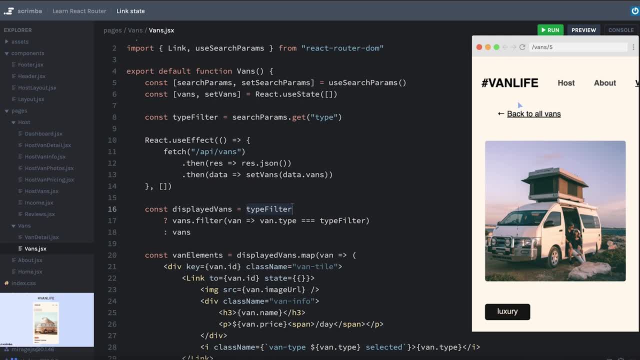 filter, knowing which type it was just filtering from, and can change the link here so that it goes back to just the, for example, luxury vans. Now I could just pass a property, maybe called type, and say that it's going to be equal to whatever the current type filter is. Remember, type filter is. 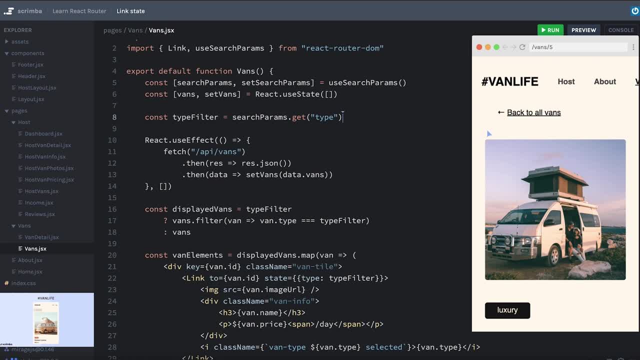 coming from the search params and so it's either going to be just the plain string, simple, luxury, rugged, or I guess it was null if there are no filters. but let's think one step ahead. If the idea is that I don't lose all of my query strings when I go into the van and then click back to all, 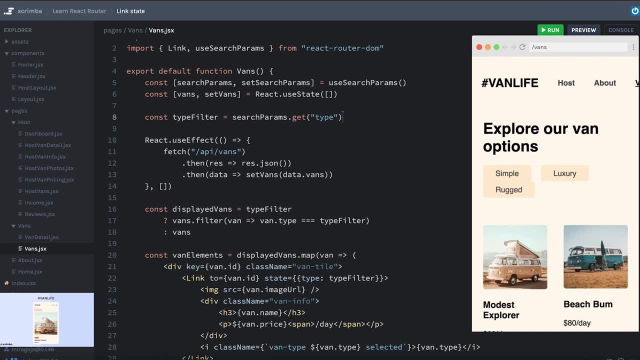 vans. I'm going to try and future proof this a little bit. so if I do have other query strings, like we had, name equals joe and I go also to rugged. so now I have two parameters: I have name equals joe and I go into an individual van when I click back to all vans I don't just want to have 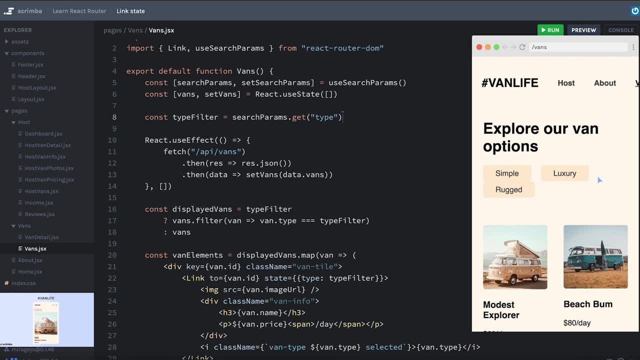 the type filter there, because maybe eventually we have this sorted by price or filtered by price within a certain range, or whatever other filters or sorts we might have. So yeah, let's try and future proof this instead of just passing the type by itself. I'm going to take the entire query. 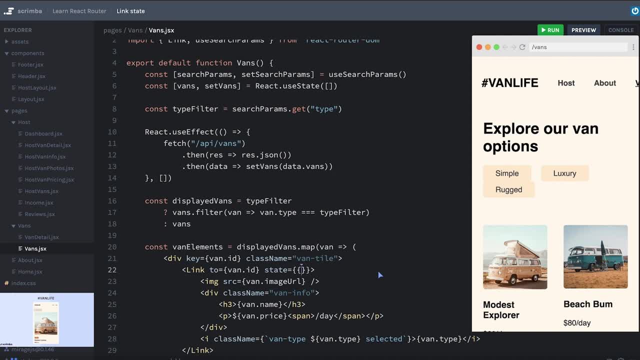 string and pass that down. so let's get our object back and maybe what I'll do is let's just call it search params. Actually, I could just leave it like this. I could just say: search params is the search params value that we have. this is the url search params object, but honestly I don't think the van detail page. 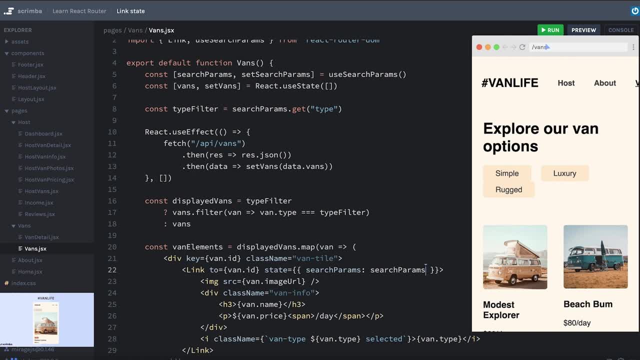 needs the entire object. I think really what it needs is just the query string. this one's just a judgment call, it doesn't really matter too much. maybe I will just call this search and then we'll say the value is search params dot to string. again, it probably just depends on the needs in your 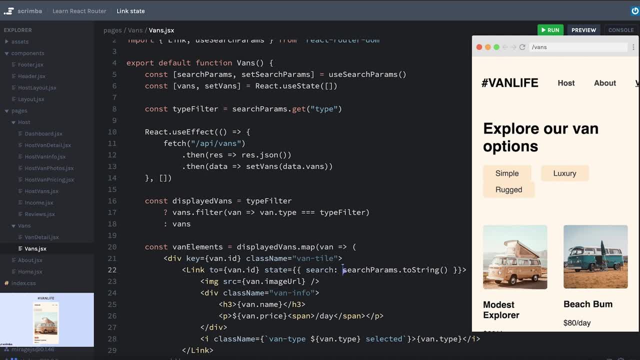 scenario. but the point is this should take the entire query string and pass that down to the entire search params in its stringified version and pass it along to the next route that we're linking to. this is beneficial again if we have multiple search parameters, not just one filtering. 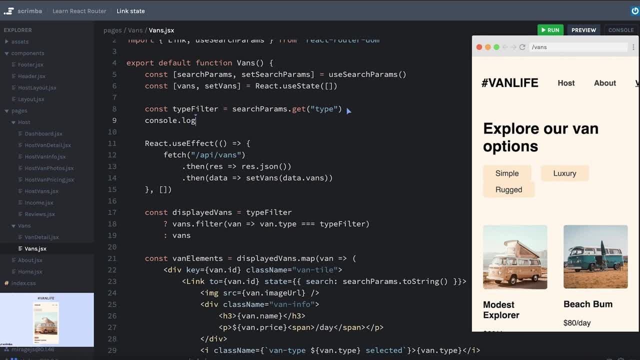 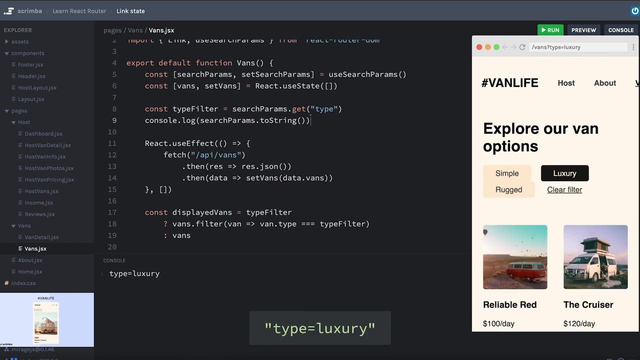 by type. and just in case you forgot, let's console log search: params: dot to string, so you have an idea of the value that I'm actually passing in the state here. let's save, open up the console and of course right now there is nothing. we'll hit luxury. okay, so it's: type equals luxury. 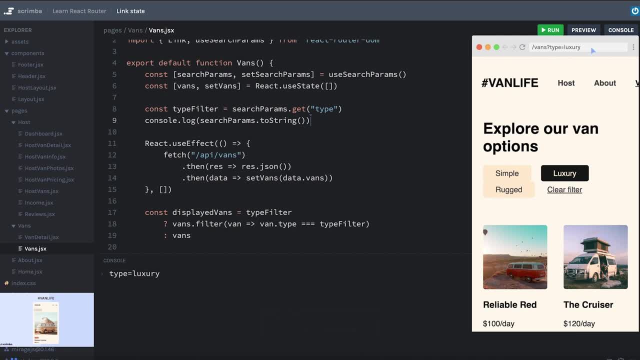 if I add other ones like: and name equals joe. now we have type equals luxury and name equals joe. just note that it doesn't have the question mark at the beginning, so we will need to add that manually. we could either do it here or I'm just going to do it on the other side of the equation. 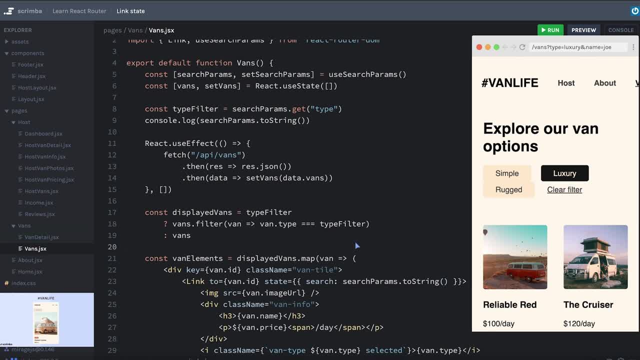 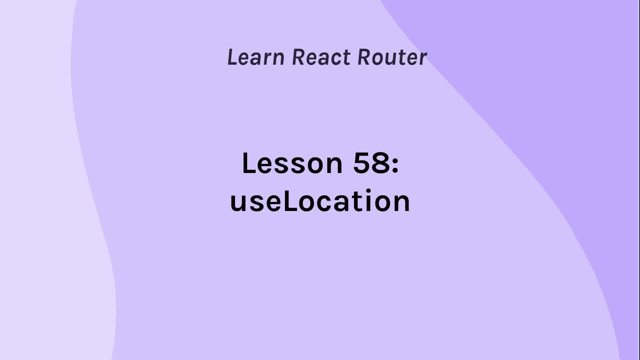 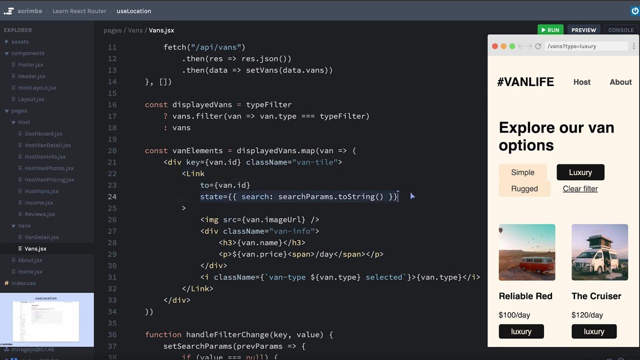 in the next scrim we'll talk about the van detail page and how we can grab the state that we're bringing in by adding it to the link to that page. okay, so we are linking to the van detail page by its id and we're passing the state along with the link. so let's go over to van detail and learn. 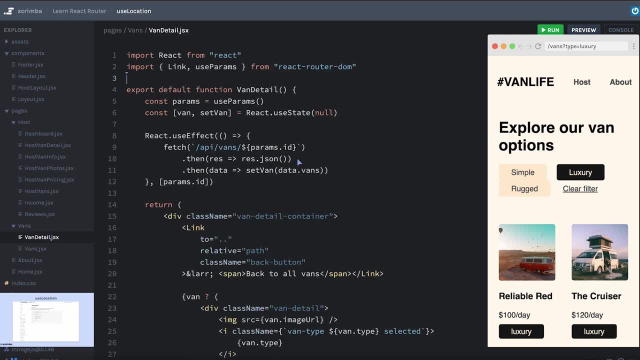 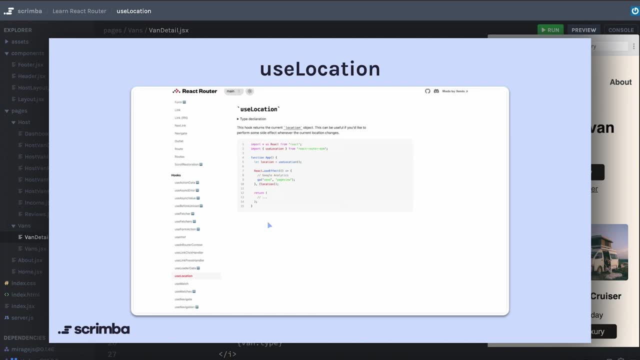 how we can receive the state from the incoming link that sent us to this page. doing so will require us to learn a new hook called use location, and I'm going to be perfectly honest. you can probably tell from the screenshot here. the documentation on use location, I think, has a. 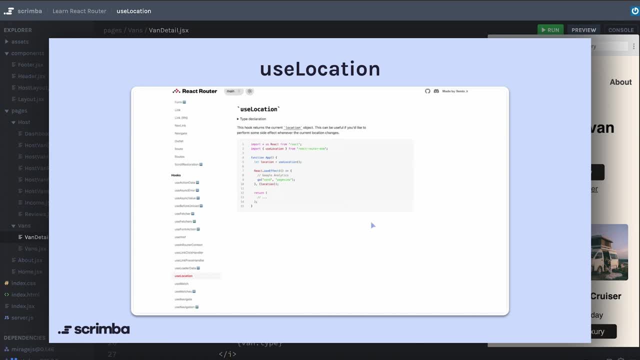 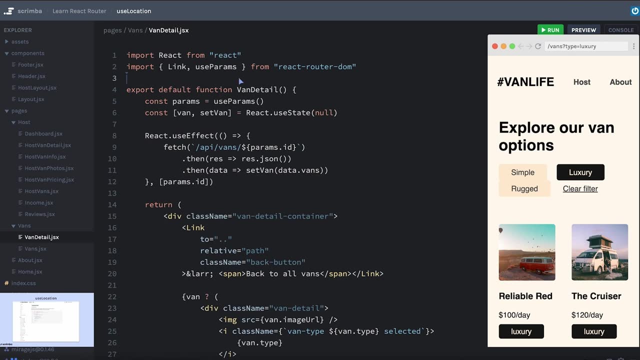 little bit of work to be done but nonetheless I link to it here just in case it gets updated or maybe I'll submit a PR and actually update their documentation to have more useful examples. so I'm going to import use location. use location is more like the use params, where it doesn't bring in an array like we have with use state or with use search. 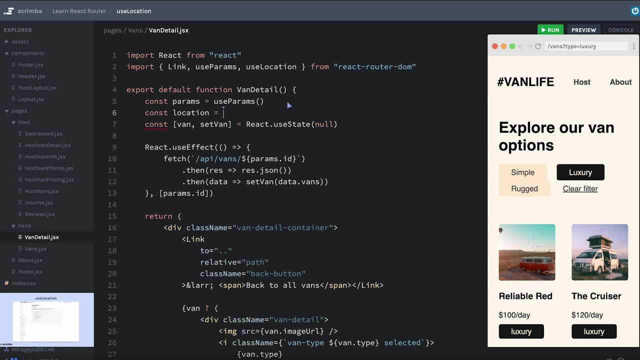 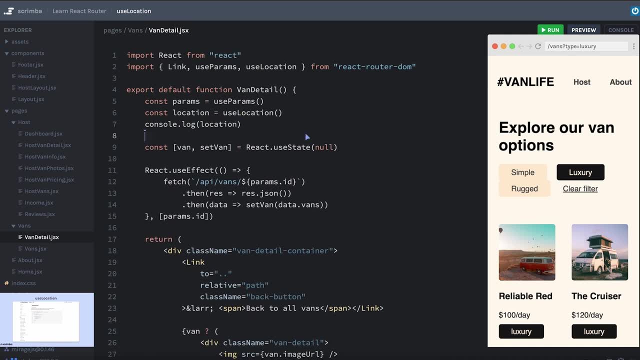 params. so I'm going to say const location equals use location and this location object is: well, it's just that. it's an object, so let's go ahead and console log it and we need to go over to the detail page to run that code. okay, and you can see it's an object with an. 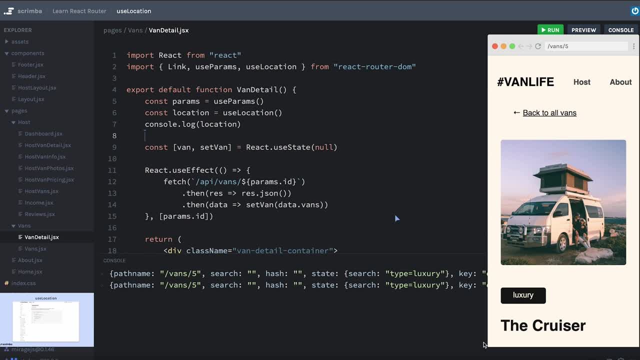 number of pretty helpful properties. path name gives us the absolute path to where we currently are in our routes search would have a query string there if this page had a query string. in fact, I can see that by saying question mark name equals bob, hit enter. okay, so now we can see. 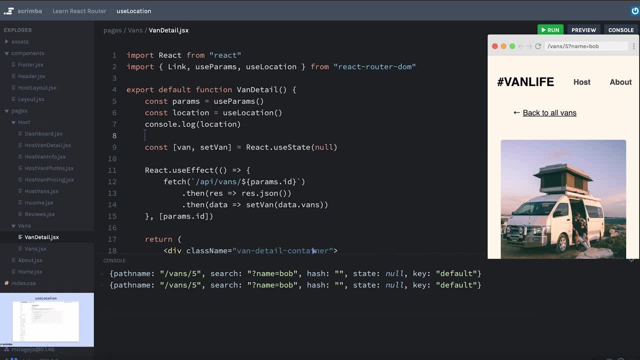 the path name is slash van slash five. the search is question mark. name equals bob and that came from the query up there. of course, you can also see that the state says it's null and that's because I navigated to a new page by adding this query string. so 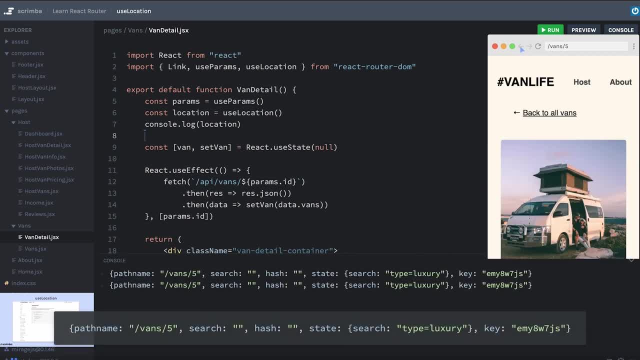 let me actually go back in the browser and I guess this brings up a really good point. you can see that just by hitting back I was able to bring back the search state. if you look in the console, there's a property called state and it has an object with a search property as a reminder. 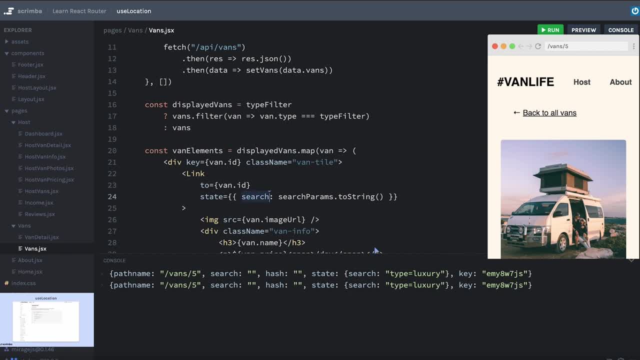 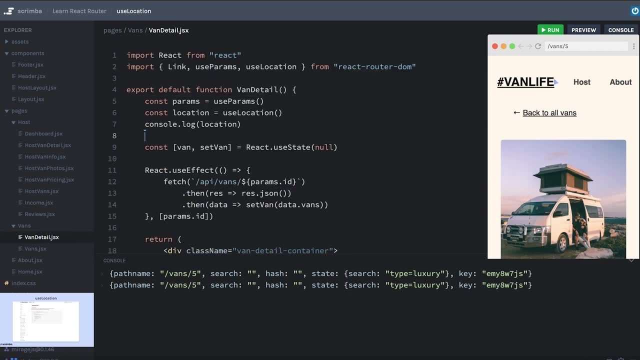 that's what we created. we chose to call it search. this isn't something browser specific. the property state, however, is something specific from react router. but the cool thing is, I was able to hit the back button and bring that state back, even though it did a refresh of my app. 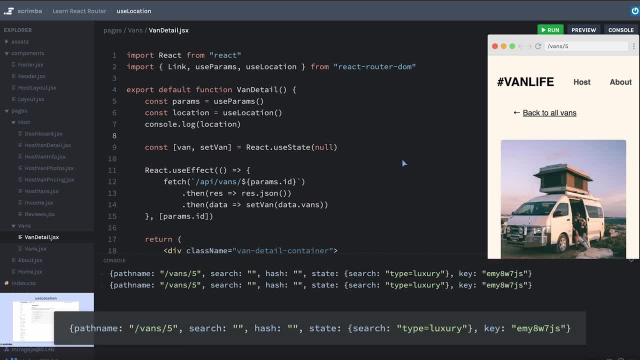 and, in fact, even if I do refresh the app, you can see the state is maintained. this is what I meant by saying that the browser has its own internal ability to maintain some kind of state based on where you are in the app and that's all. react router is using under the hood. now there is a 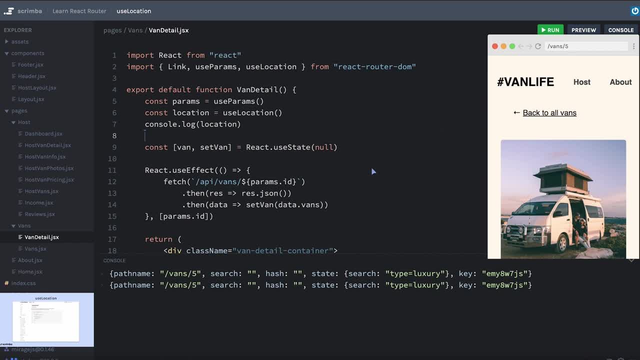 limitation to this. if I copy this URL and I send it to a friend, their browser does not have that same state. there's nothing in the URL that's hidden or secret about the state that I'm trying to maintain. it's something specific in our browser. in fact, even if I were to open a different browser. 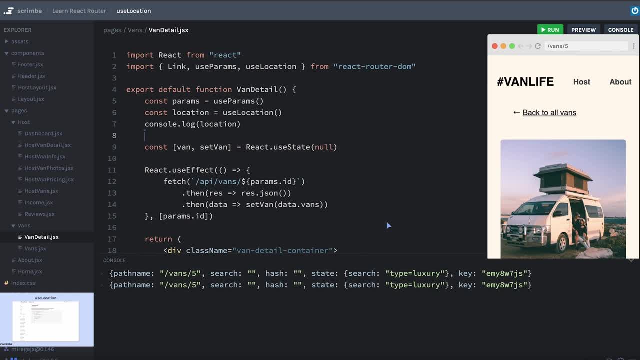 and use the same URL, that state would just disappear. in this case, though, that's probably okay, because if I'm in a new browser or I send the link to my friend, they may not necessarily care to go back to all the luxury vans like what I'm trying to handle here. okay, so by using the use location. 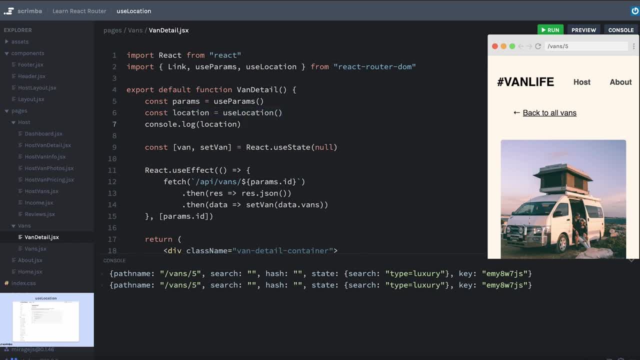 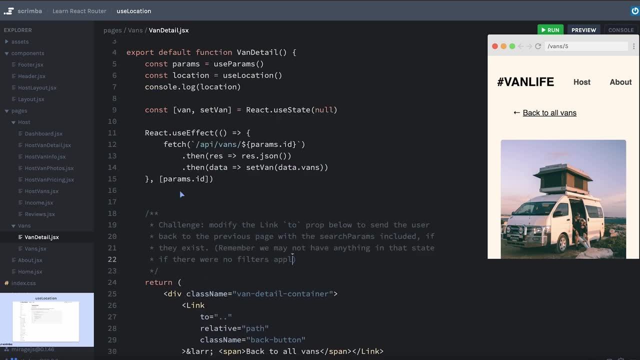 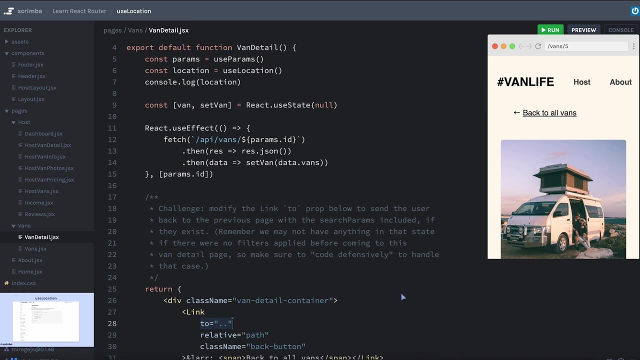 hook, we have access to the state which is an object that has a search property, because that's how we set it up in the vans list page. so that sounds like a pretty good time for a challenge now. okay, so we're going to modify the link to prop so that it can send the user back to the previous page. 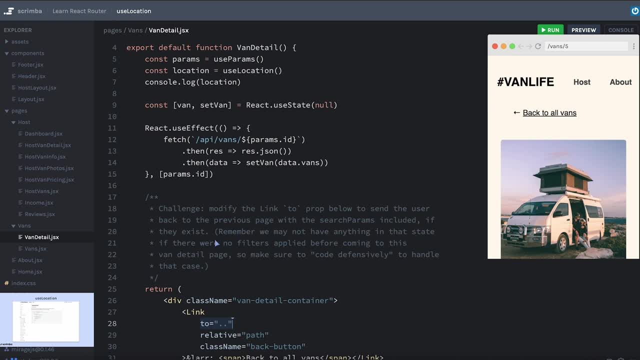 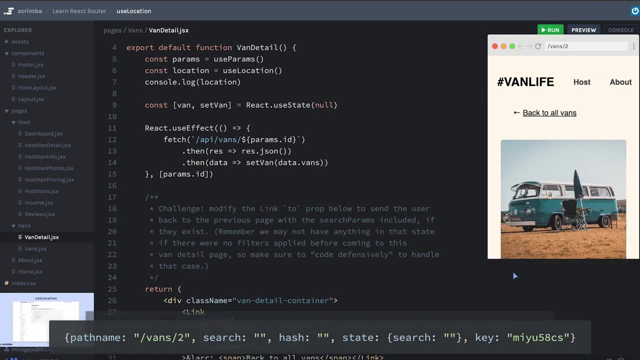 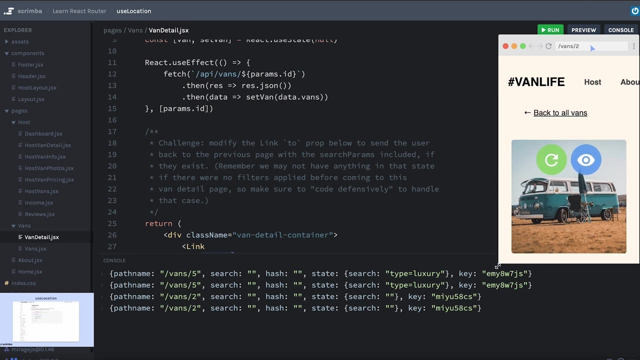 with the search parameters included. if- and this is important- if they exist, like the little note says here, we may not have anything in the state. if there were no filters applied, maybe I came to that page and you can see. in this case it says the state search is an empty string. or, as we discovered, 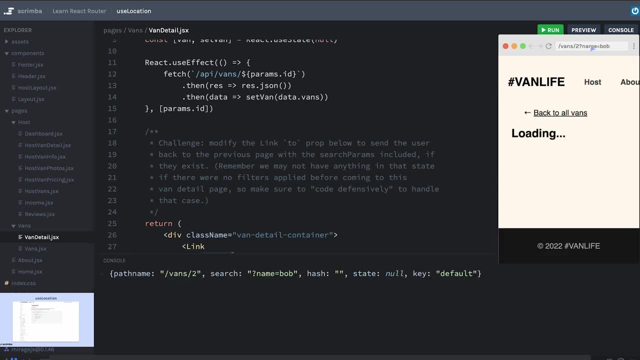 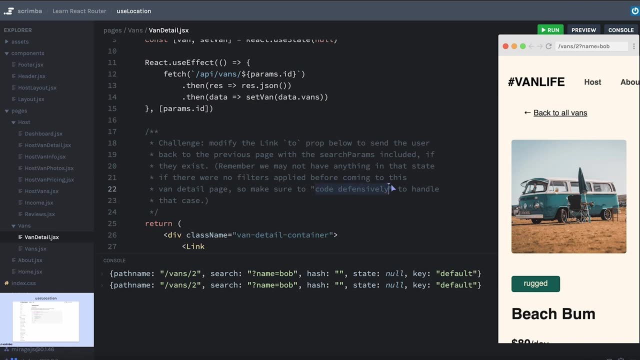 we may not be sending state at all. if I were to add a random parameter up here, say name equals Bob, then state is null, so we can have a state dot search. keeping that in mind, you'll want to make sure that you code defensively so that you don't run into a bug, in case that happens. okay, pause now and work on this. 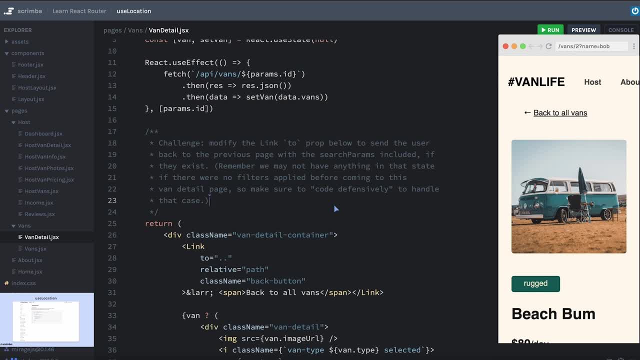 challenge. okay, now I did leave you in the dark a little bit and I'm hoping that you just had a chance to play with the code to figure this out yourself. but when we have a relative path like this, with just dot dot, I still can say question mark, maybe type. 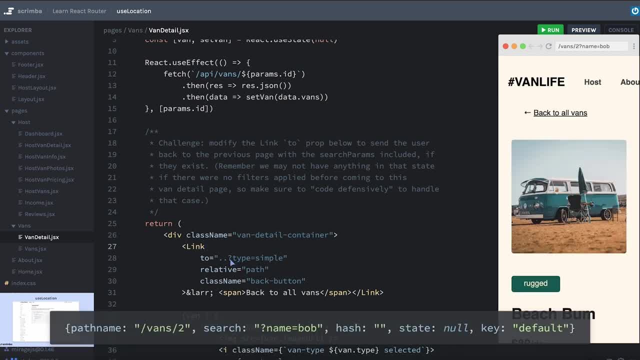 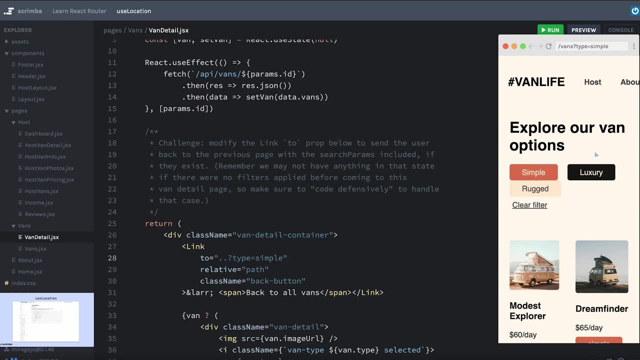 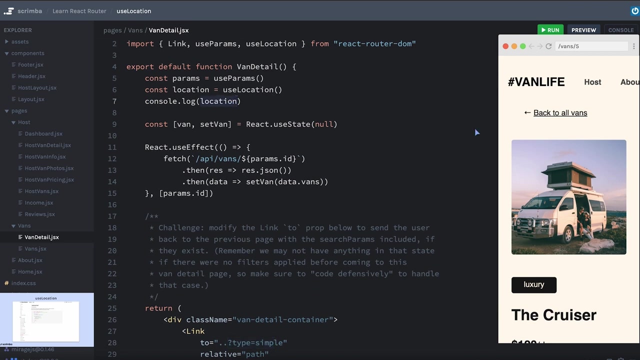 buttons. button type: everyone gets a check mark. right now, how do you hide your videos from YouTube? how do you hide your videos? something like this- how to hide your videos- will work if you can do it with Photoshop. but let's get straight to the lesat. we have a name, equals simple and have that work. so if I hit save, I'm just hard-coding. 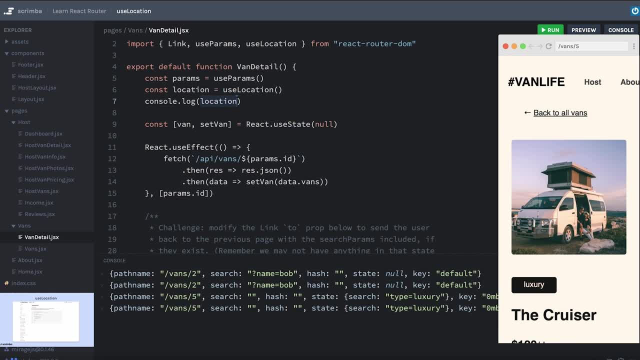 this, of course. for now, I'll click back to all vans and you'll see that our simple filter is applied. so let's change this bag to luxury. of course, what this did is it lost. the name equals Bob, but dot search and that's going to be the query that we want to include. Don't let this be confused. 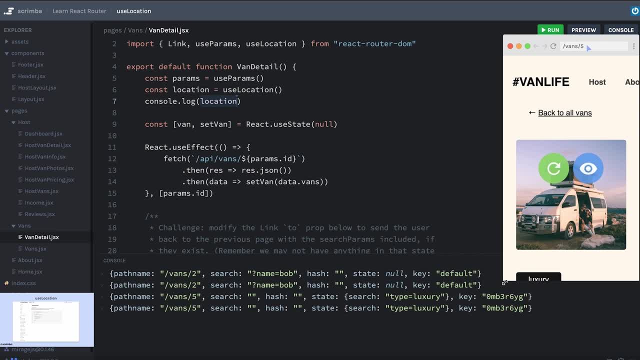 with the location dot search. Again, that's just whatever search is in the URL at the current time when this loads- And actually you know what I'm seeing something now: The way that React Router handles search is including a question mark at the beginning. So for the sake of consistency, 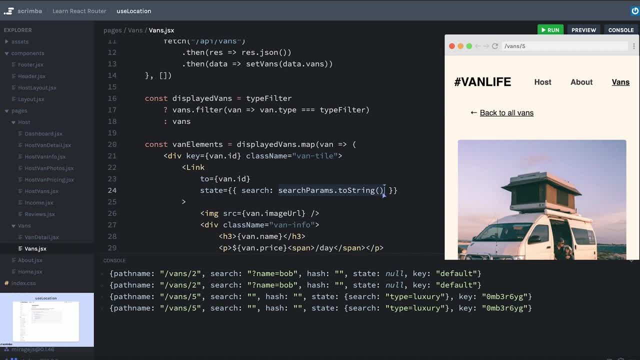 I'm going to make a quick change over here. Instead of the value just being the search paramstoString, I'm going to have it include a question mark, So we'll just do this. I didn't expect you to figure that one out. That's just a choice that I'm making. Okay, so let's try this. 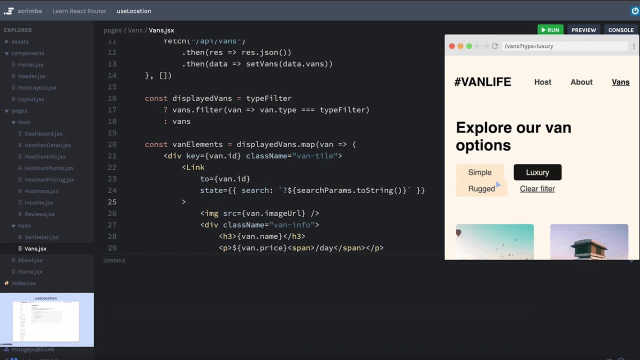 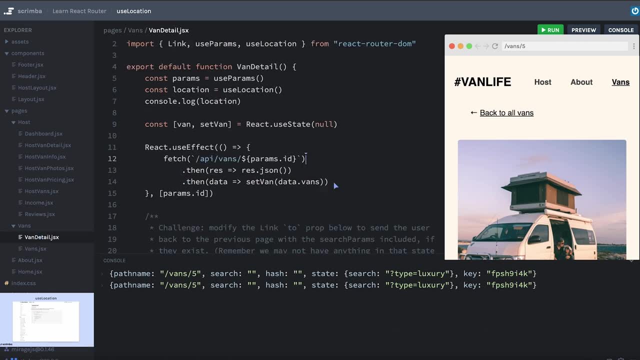 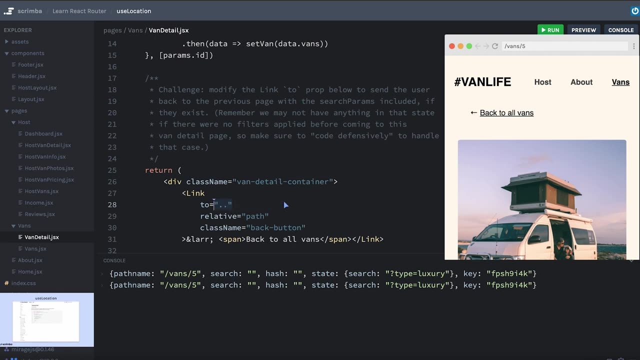 again. We'll go back to all vans. Let's maybe hit refresh, Change the type to luxury, Go over here. Okay, so now our search has the question mark in it Again. not necessary, but it seems a little more consistent to me. So because of that I can just change my to prop and we could just 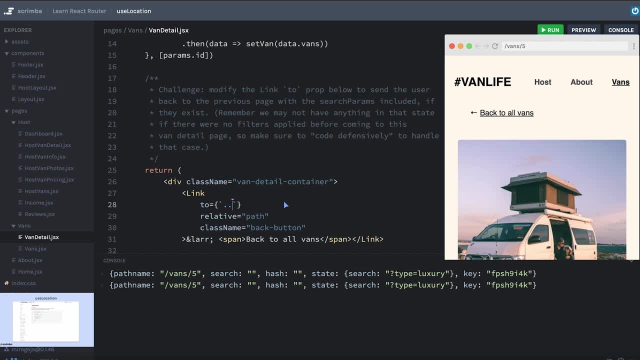 say: this is going to be a template string and it's going to start with a dot dot and then include locationstatesearch. right? Well, not quite, because again, there's a possibility that the value of state is going to be null If the value of statesearch is an empty string. this works. 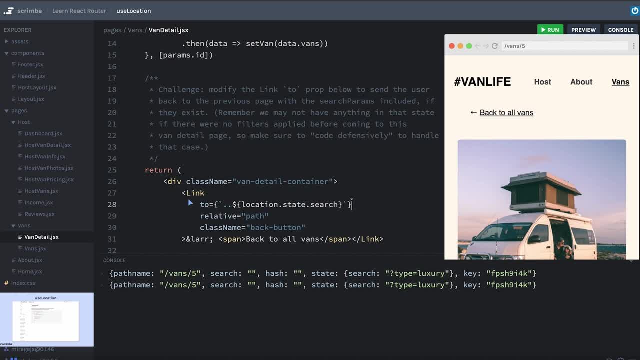 fine, But if state is null, this is going to throw an error. So what I'm going to do is create a sort of backup for the locationstatesearch. just in case it doesn't exist, Let's go ahead and save it. 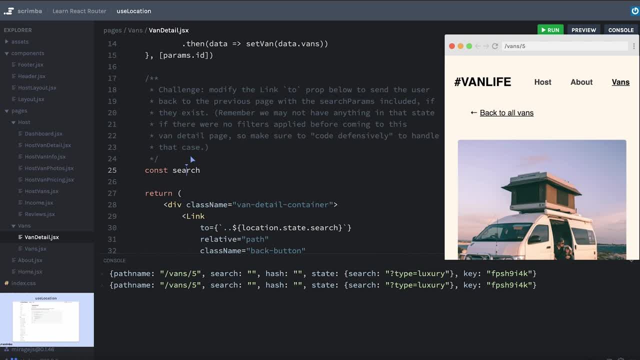 We'll call it. maybe, I don't know, we'll say const search is equal to locationstatesearch, and there's a relatively new feature in JavaScript that's called optional chaining. In fact, it's new enough that Scrimba is going to complain about the syntax, but I promise you it still works. 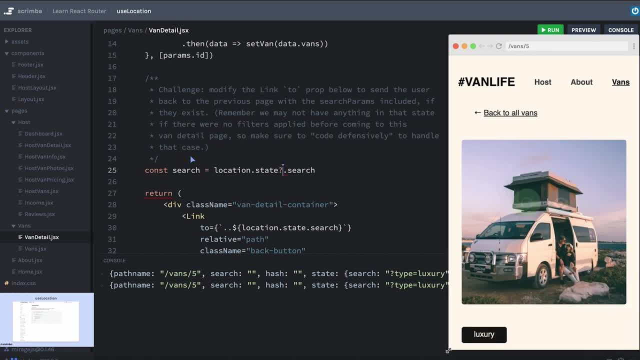 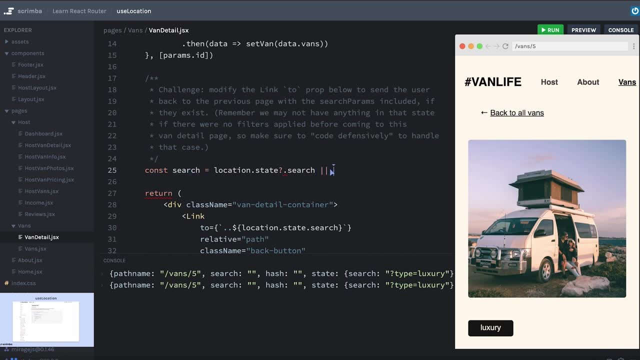 And so I can say: if locationstate is a thing, then check for a search property and that value is going to be the value of my new variable that I'm setting up. But if that doesn't exist, let's just say it's an empty string. 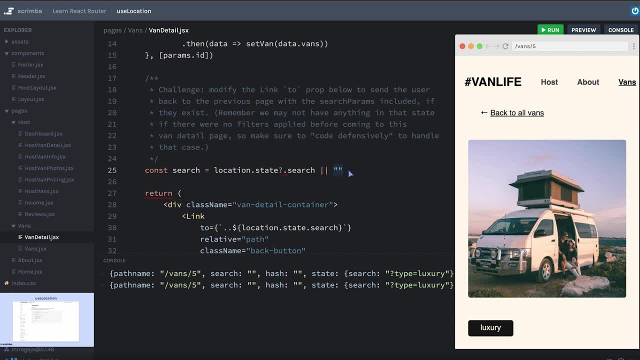 That gives me a fallback, just in case locationstate does not exist, my value will be an empty string. So I'm going to take my search and replace. well, I guess we can just delete that part and say the search will go here. Let's hit save. I'll close my console to buy some space. Let's go back to all. 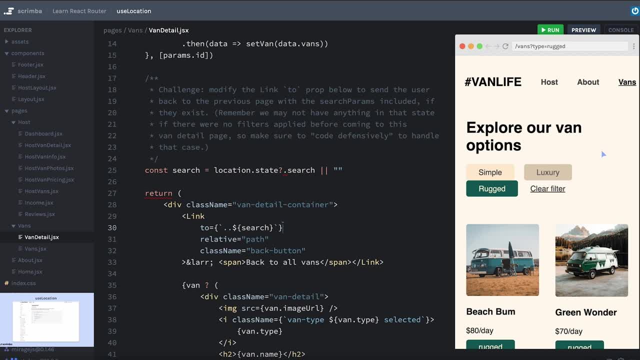 vans. And awesome that took us to type: equals luxury, Perfect, Rugged. go into one of them. back to all vans: type equals, rugged. If you didn't know about optional chaining or you didn't want to use optional chaining, you could also simply say something like locationstate: 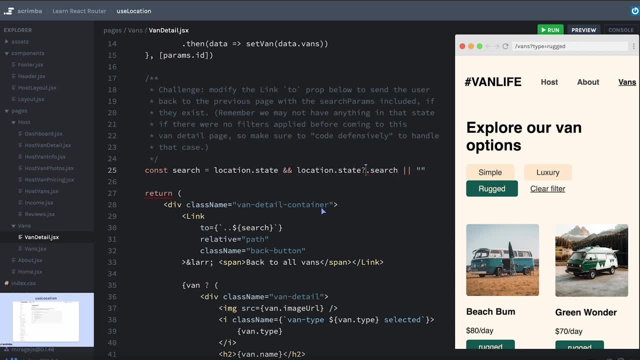 and locationstatesearch. This was usually how it was done before optional chaining existed in JavaScript. But because optional chaining does exist, even though Scrimba is going to complain about the syntax, I'm going to leave it in here. What's nice about this is it should work with any. 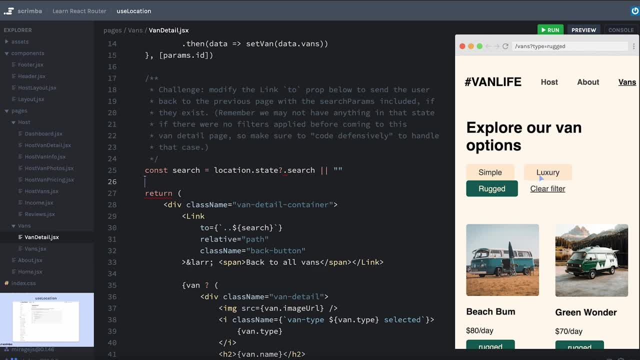 other filters or queries that we have included in our URL. So if I add back my name- and name equals Joe, I click on one of the rugged vans- Now we have type and name in our queries, We go here and then I say back to all vans: It's going to maintain both the type query. 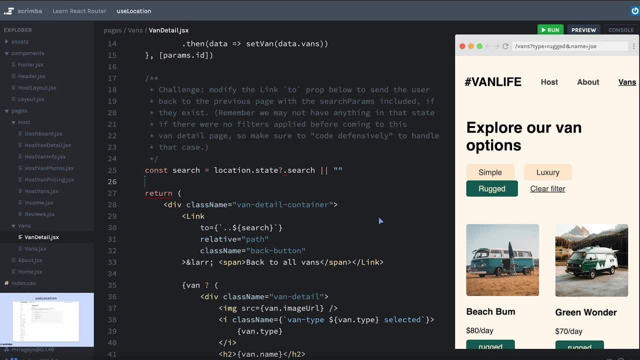 and the name query. All right, that was a lot to take in, As always. if you did struggle through this challenge, now that you've seen me do it, I recommend you scrub back to before the challenge and just try it again on your own. Practice really does make perfect, Since that one was pretty heavy. 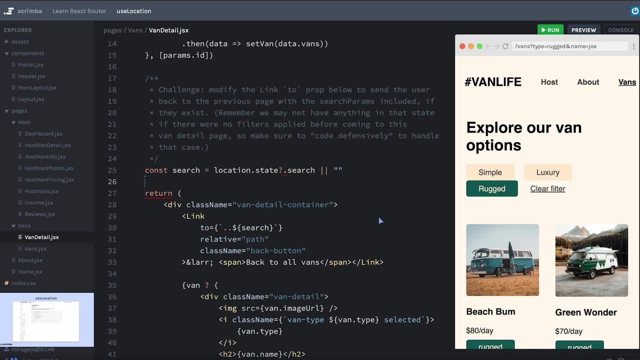 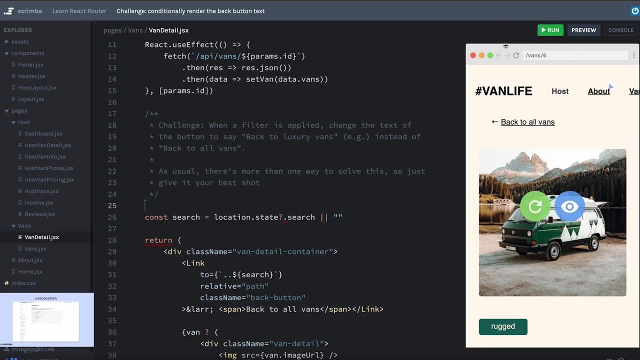 let's do a quick challenge. That's going to be a little bit lighter, And then we'll be ready to move on. Let's say a product manager comes to you and says: Well, when a filter is applied, we don't want it to say back to all vans, we want it to say back to and then the filter and so back. 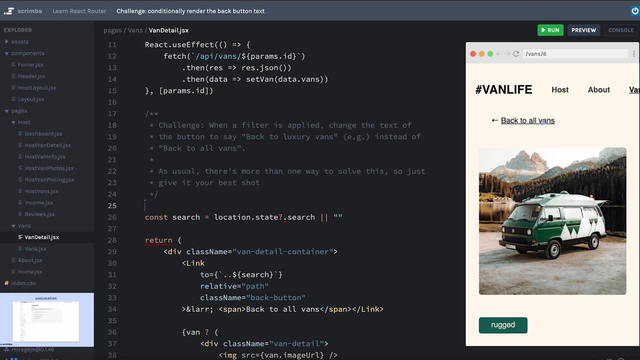 to luxury vans or back to simple vans. So that's what your challenge is, And I'm not going to give you too much more information. There's certainly more than one way to do this, But I want you to put on your thinking cap and try to figure it out. So pause now and work on the challenge. 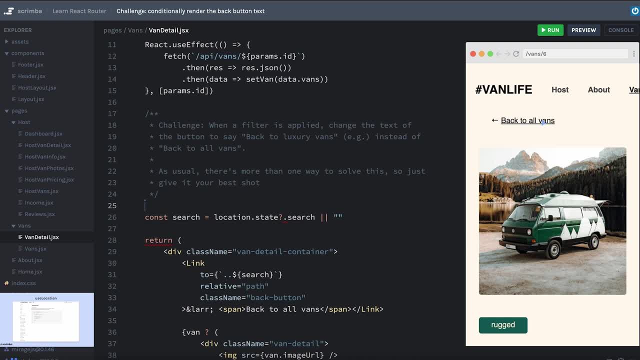 So one way I could do this is to take the string. let me open my console. I could take the location, dot, state, dot, search string and try to just do some regular string manipulation like split it on the ampersands and then split it on the equal signs and grab the one that's after the type or something. 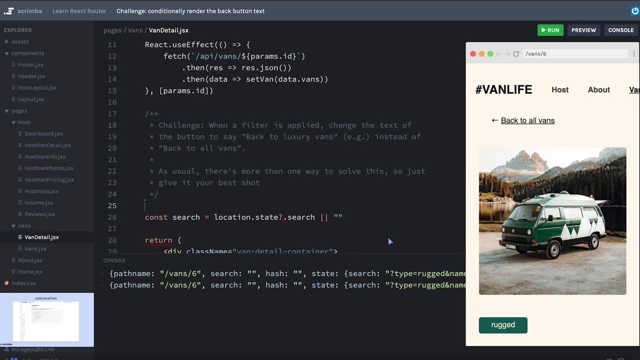 like that. However, because the string is a query string, one way to solve this is I could create a new instance of URL search params And then I have access to the methods like dot get, get the value of the type param. So that's one way I could. 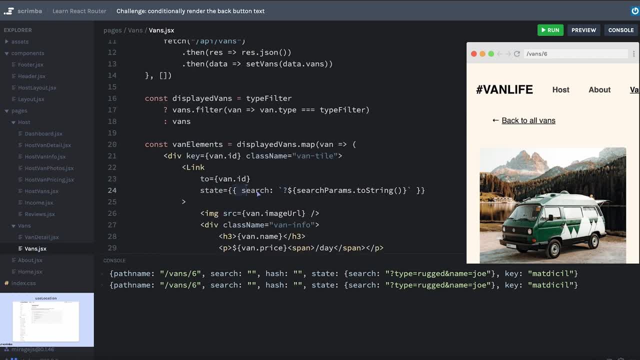 solve it. Another way I could solve it is in vans I could just pass more state through. So right now we have the search. I could also say I want to pass the type in, say the type is going to be equal to, and in this case we already have access to that with type filter. we put these on their own. 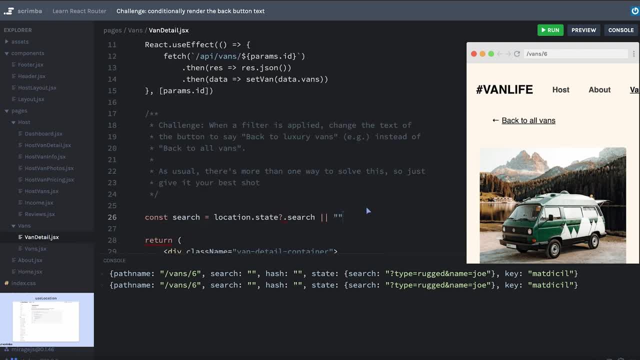 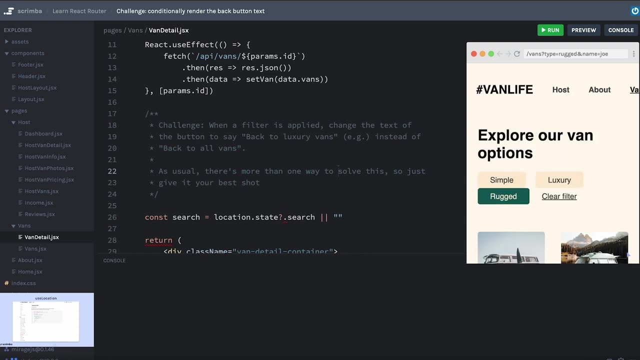 lines, And then, if I do that over in van detail, I can grab that string by location, dot, state, dot type. Since I've already got that typed out, I might as well just keep going down this path. So we'll hit save. Let's go back to all vans and just do a refresh, say rugged, Okay, so now you can see the. 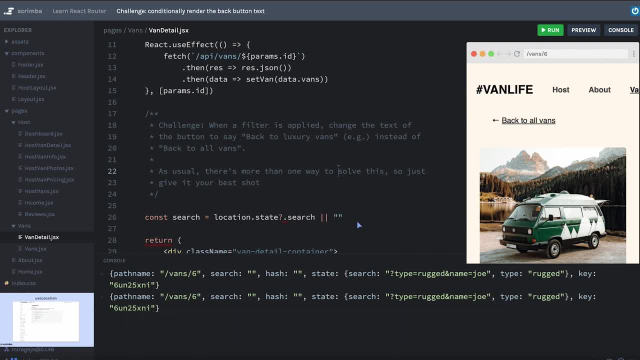 location dot state is an object that has search and type. So I'll just do something similar here. we'll say: const type is equal to location dot state, question mark dot type. And if that doesn't exist, like for example if location dot state is null, 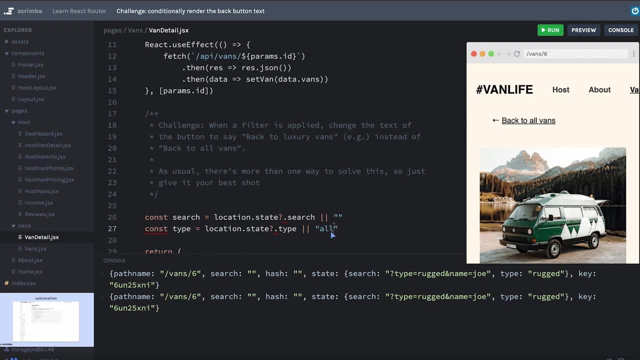 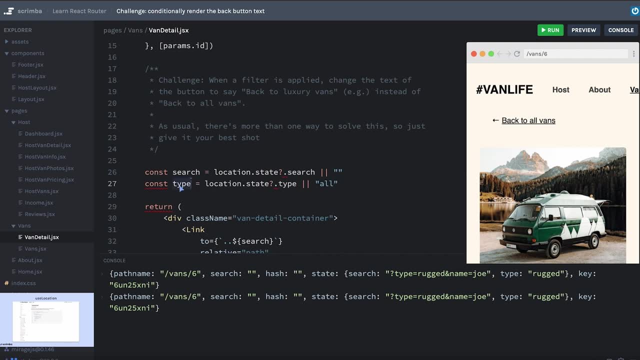 then we'll just set the type too. Well, actually, let's set it equal to all, because we do want it to say back to all vans if there is no filter applied- And now I can take this type and just conditionally render this word here- we'll just say back to and then put type. 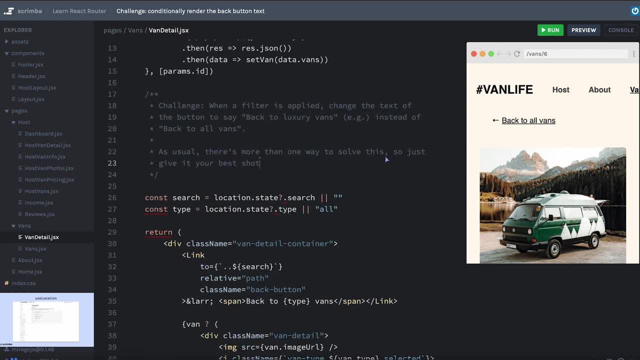 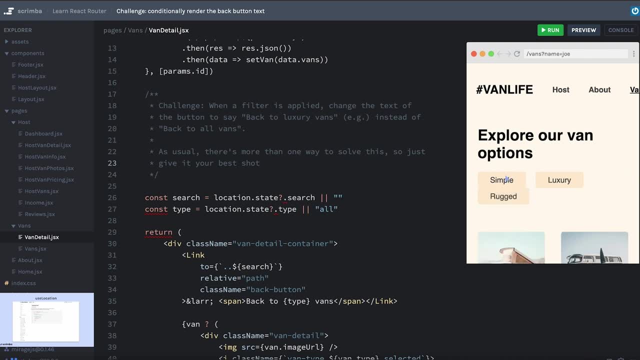 vans. Okay, let's see if this works. Let me close the console, Hit Save. Okay, it's back to rugged van. So I think it's working. Let's go back. we'll clear the filter. we'll go back to one of them. back to all vans. that's great. let's try luxury. back to luxury vans. simple. 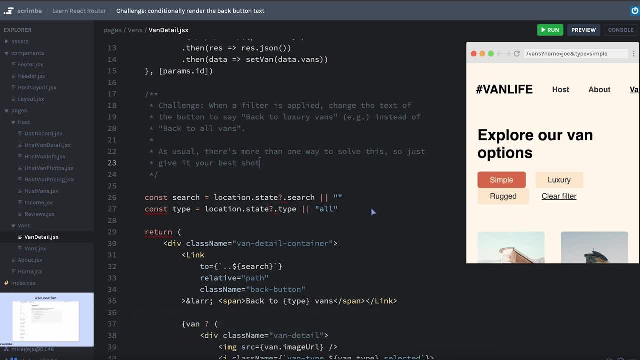 awesome again. we even talked about multiple different ways that you could solve this. at that point. it's just sort of a javascript challenge as a quick recap, passing state through the links can be a really useful thing. okay, hopefully that challenge went. okay again, review it if you need to, and then, when you're ready, we'll move on. 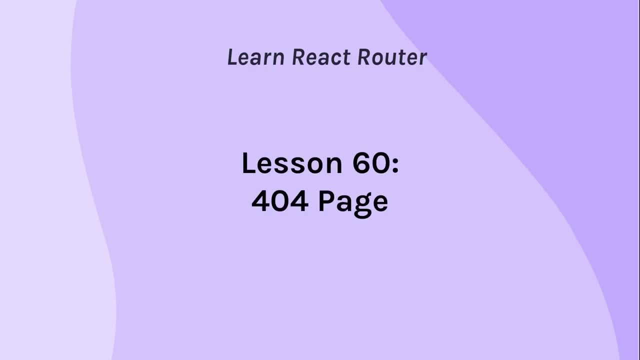 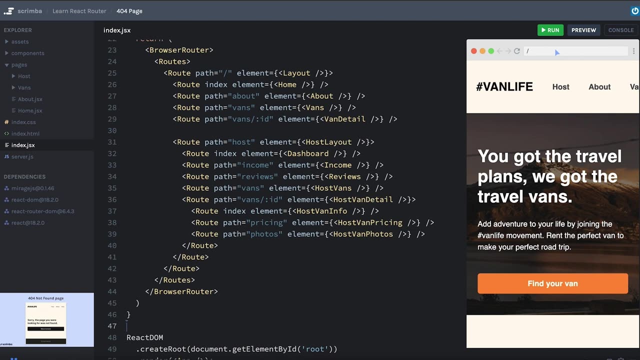 a really important part of any application is being able to give useful information to people when they come to a path that doesn't actually exist on your site. sometimes this happens if you have outdated links within your own site and they lead to pages that no longer exist, or it might. 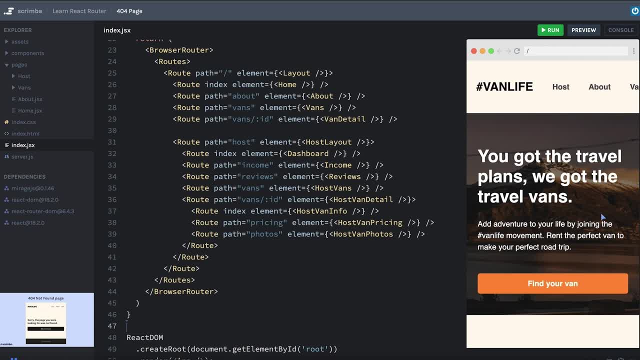 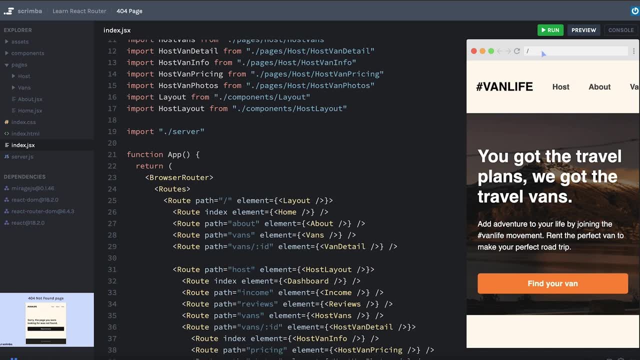 happen if somebody else links to your site and they either got the link wrong or again they're using an outdated link that no longer exists. for example, if i'm here and i'm using a link that no longer exists and i type in slash: blah, blah, blah and hit enter, you can see there's really no. 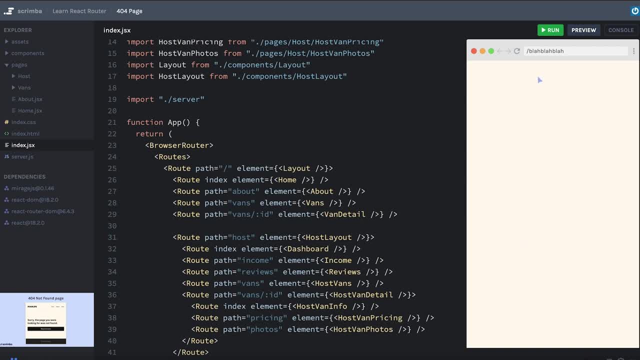 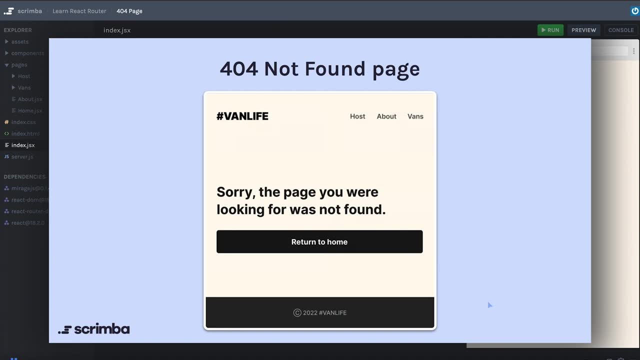 useful information on our site, because react router is not handling a blah blah blah route. this is where a good 404 page comes in, and i've seen some really creative, interesting 404 pages, but we're just going to keep it pretty simple for now. so how can we handle this in react router? 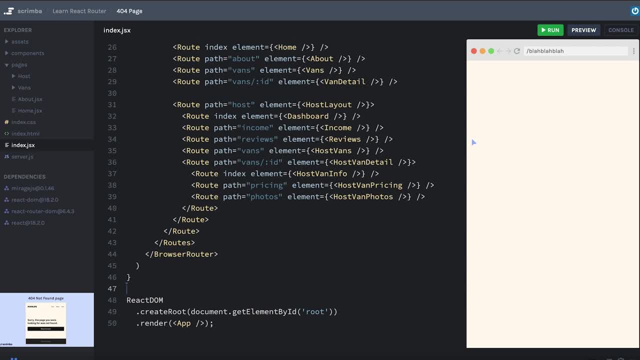 fortunately, it's really easy. there's something called a splat route or a catch-all route, and that has everything to do with what you put for your path here in react router. you can see that there's a lot of things that you can do in react router. 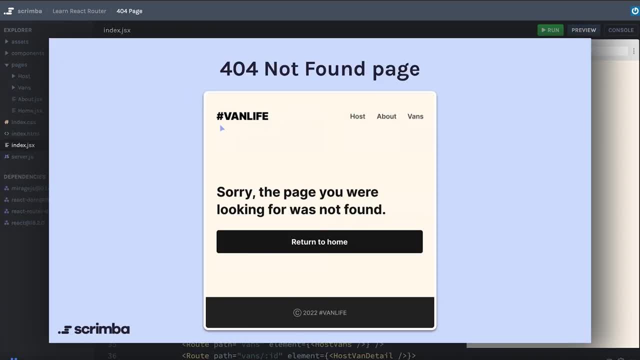 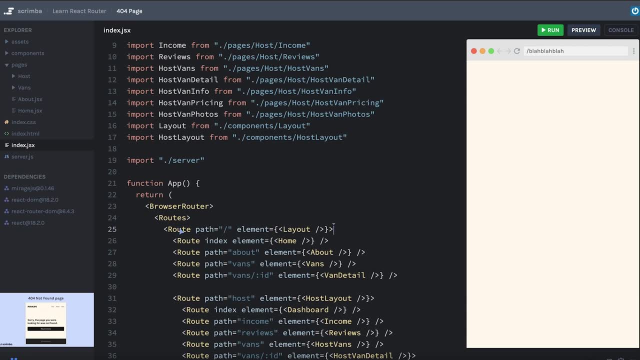 inside of my layout route, because you can see in our example here, we still have the navigation bar and we still have the footer. so that's the reason i'm choosing to do this as a nested route inside of my layout. i could, if i didn't want to have the navigation or footer, i could have a completely 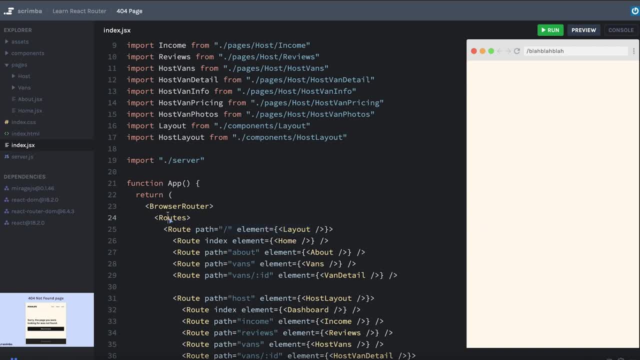 dedicated 404 page that didn't have those elements, in which case it would go as a child of routes right here, but let's keep it as a child of our slash route. so i'll create a new route and a catch-all route is going to be very similar to- if you've ever 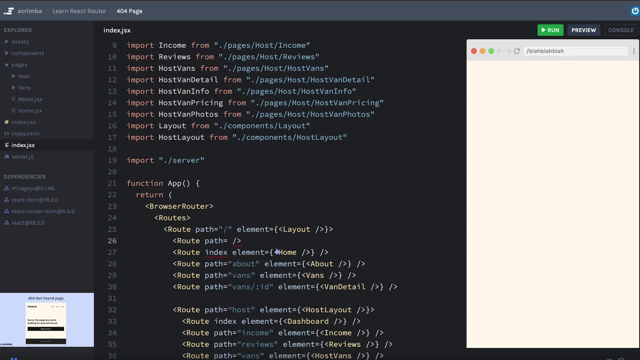 used a universal selector or a catch-all selector in css, we're going to use the asterisk. this essentially means, if there are no other routes listed, then use this route, which is why it's called a catch-all. it'll catch anything that doesn't match elsewhere. let's go ahead and put. 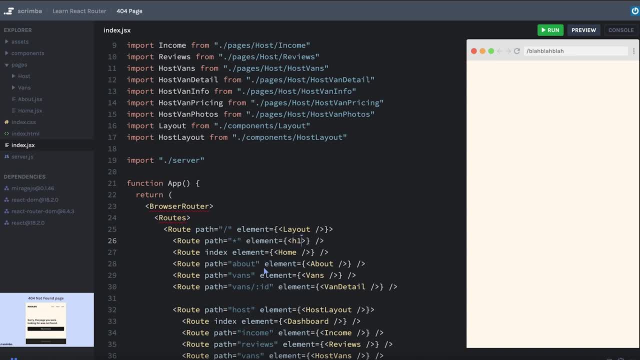 an element that just says maybe an h1 that says page not found. we're still on the slash, blah, blah, blah route. let's hit save and here we go we have. this is a very basic version of it, but we have a page not found- sort of catch-all here. one thing that's really cool about react router 6. 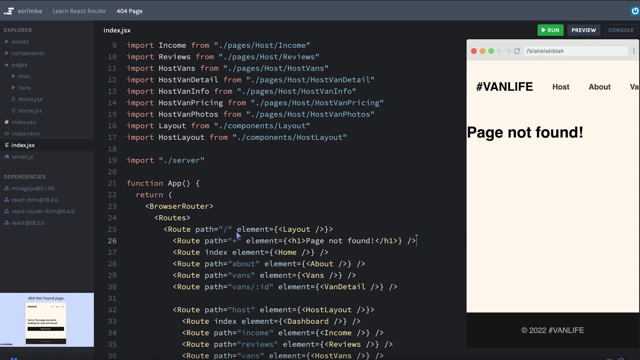 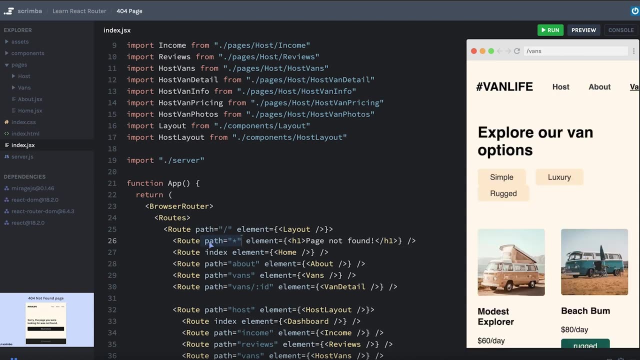 is that it's a lot more intelligent under the hood about scoring the paths that we have based on what the actual text of our url is. what i mean is that, even though our catch-all path is at the top of our list of paths, i can still navigate around my site, and it's not going to prefer the first one. 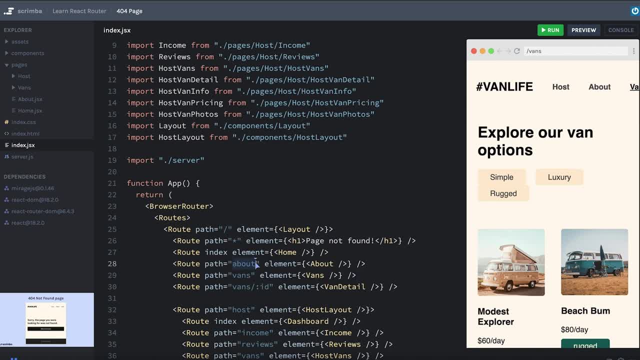 in the list. instead, it's going to give a score under the hood about which of these paths best works for me, so i'm going to go ahead and click on that, and i'm going to go ahead and click on the page not found, and i'm going to go ahead and click on the page that i currently am in my site. 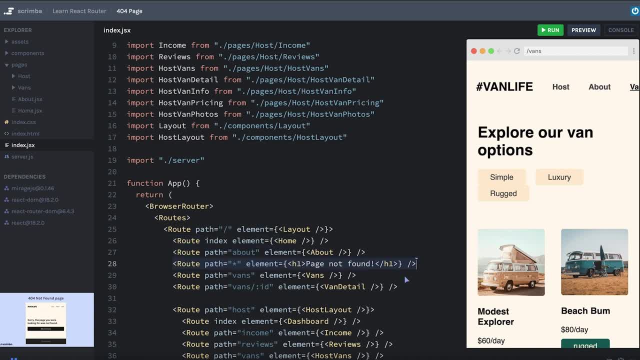 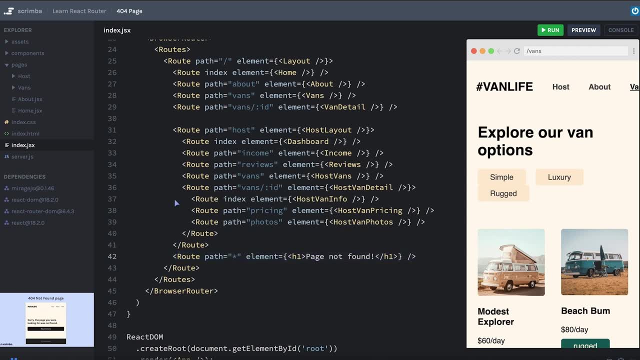 in the past we did have to worry about what order we put things in, but we no longer have to do that now. it feels a little bit out of order for me to put the page not found first, so i'm actually going to bump this down to the very bottom. that'll go right there. and because react router is really 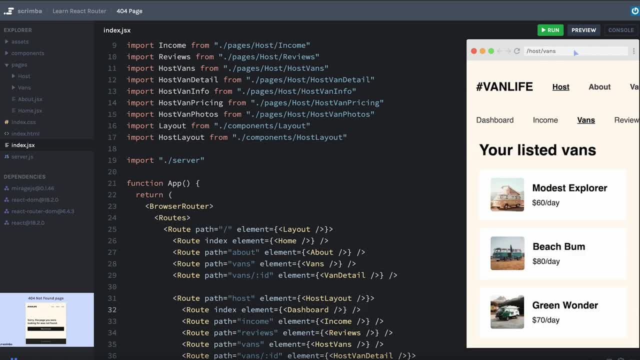 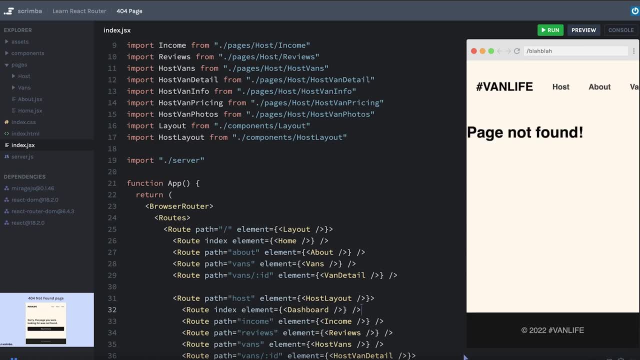 smart about how it prefers the different paths that we have available. it doesn't really matter, so i can just go ahead and click on the page not found. and i'm going to go ahead and click on the page not found. and i'm going to go ahead and click on the page that sent me to the wrong place, like. 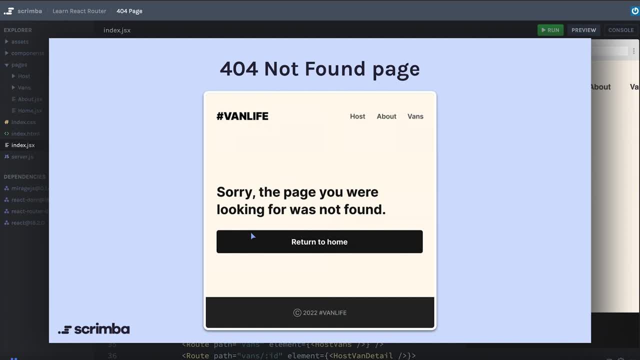 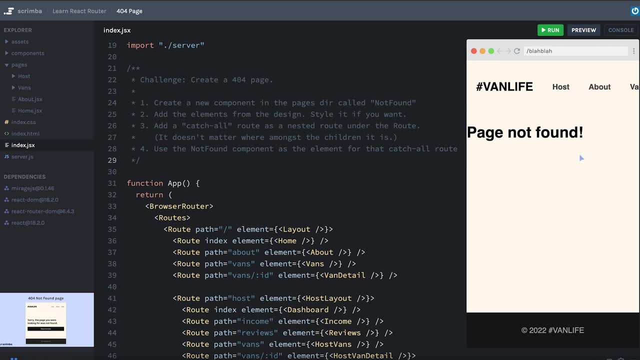 slash blah blah, we'll get our page not found the way that we would expect. now, this isn't very exciting. let's go ahead and, as part of a challenge, have you create a bit more of a polished 404, not found page? let me type that challenge out now. okay, i deleted the not found that we had before. 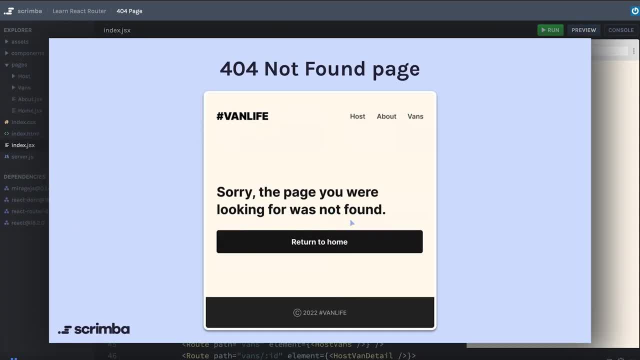 so if i hit refresh, we'll be back to a completely blank page and your challenge is to create an apigma. but the key components are just an h1 and a button that will take you back to the slash route. so if you just want to put those and you don't want to spend time with css, that's okay, so you'll. 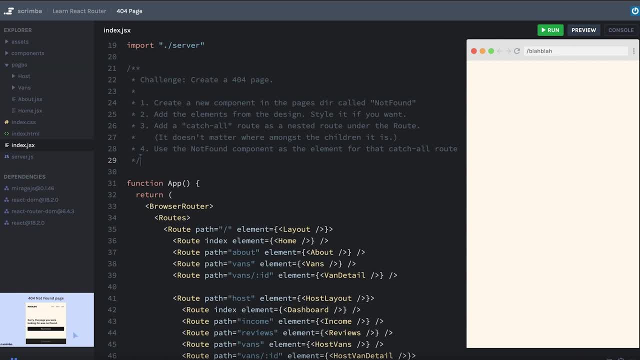 create a new component in the pages directory. you'll add that h1 and that button from the design and again you can style it if you want. then you'll need to recreate the catch-all path that we just created and you will import and use that not found component that you just created as. 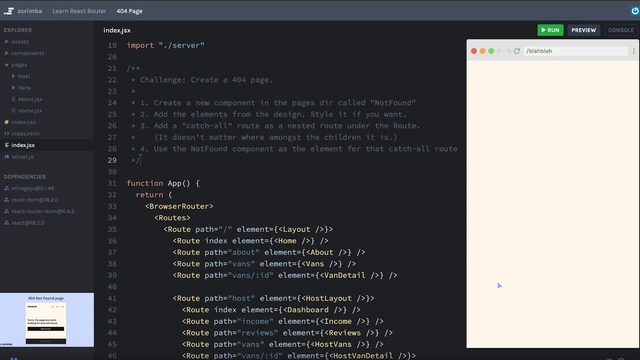 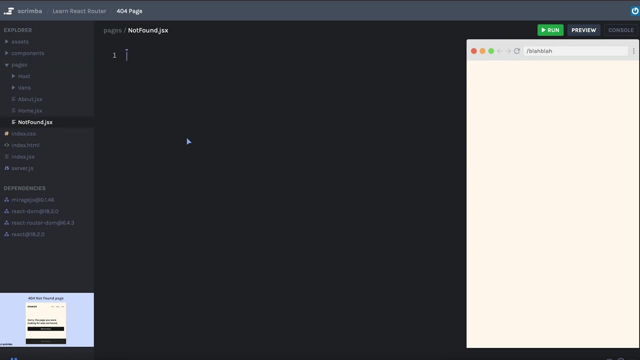 the element for that catch-all route. pause now and create our 404 page. okay, well, let's just go through one at a time. we'll create this new page called not foundjsx. i guess you could call it 404 as well. we'll get it set up like normal. 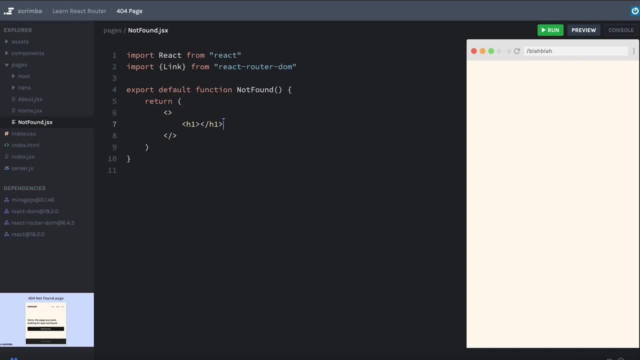 okay, and i'll go ahead and add the message that we see in the design. sorry, the page you were looking for was not found. okay, there's no styles quite yet, but you'll notice that i also already imported the link from react router dom because i wanted to send people back to the home page, so i set up the link. 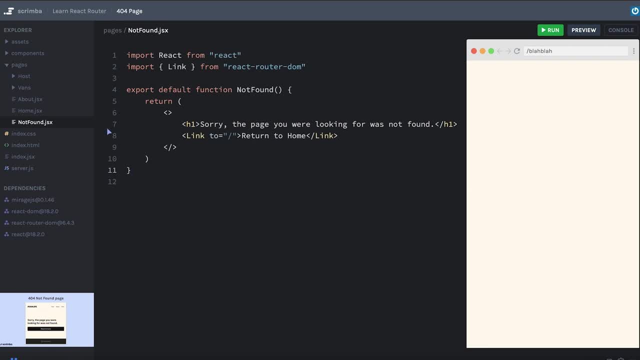 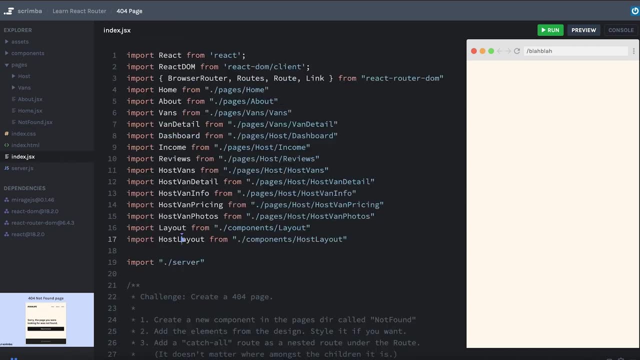 there. i'll have to make it look like a button instead of an anchor later now. let's make it so we can actually see this not found page. let's go over to our index. we will import the not found page and this one is under pages, and so i'll actually move this to be up with the pages. 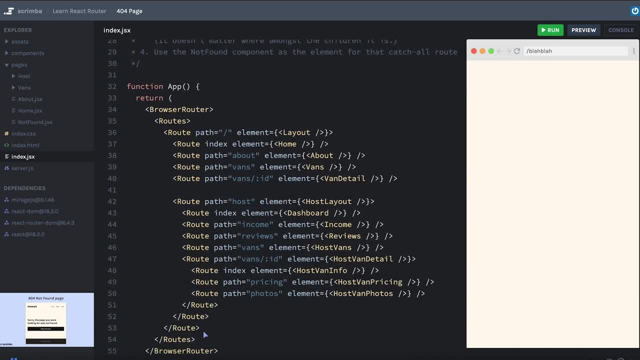 okay, let's add our catch-all all route. again, i prefer this one- just a personal preference- to be at the end, because that makes a little more sense to me. we'll say that the path is the asterisk and the element is an instantiation of not found. okay, we're still on the blah blah route. so when we hit, 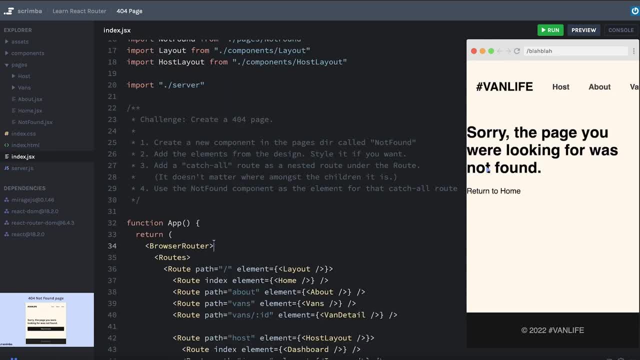 save. we should see our new, not found page. awesome, yeah, again. this, uh, return to home- is not styled at all like we would expect, but that's something that a magic snap of the finger is can handle for us just fine. so we have our 404 page. we're at the blah, blah blah route. return to 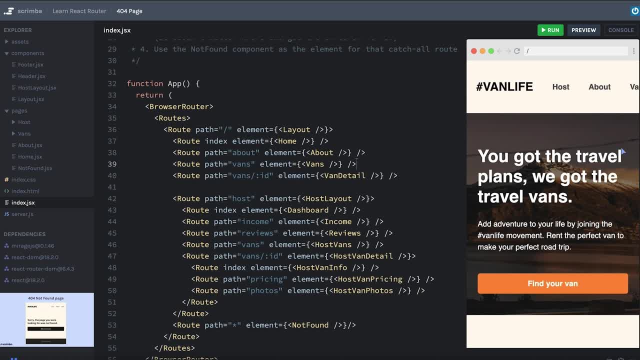 home takes us back to the home page. hopefully, this one felt like a quick win. it's fairly easy to understand. there's also some other things that you can do with these, what they call splat routes or catch-all routes, but for now we're just going to use it as our 404 page. great work, and i'll see. 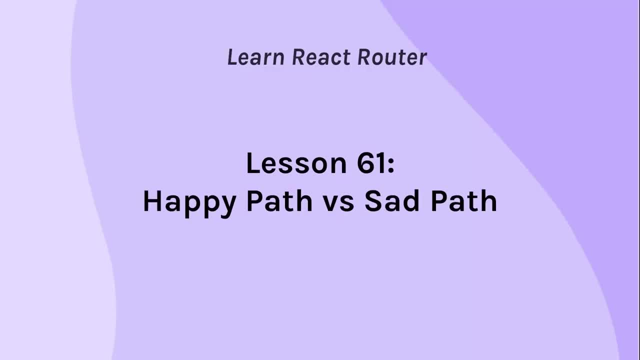 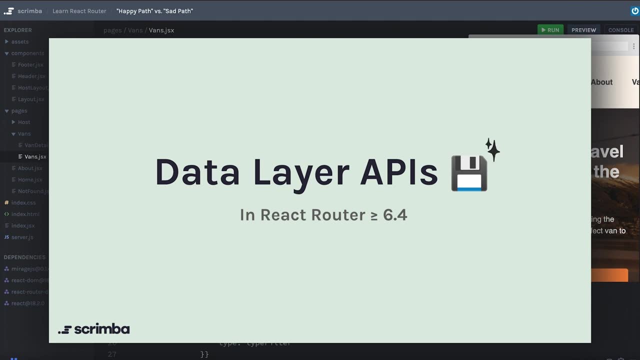 you in the next lesson. we are now basically done with the majority of the features that we plan to the van life app, but at the time of this recording there's a relatively new addition to react router that i want to make sure we cover, and that's something called the data layer apis that were 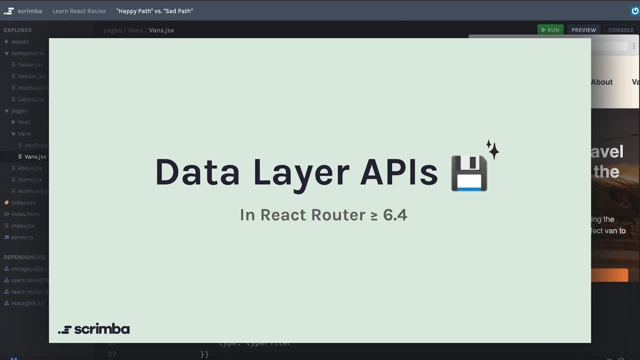 introduced in react router version 6.4. in order for us to really understand the purpose behind the data layer apis, we need to realize that so far, at least in this app, we've basically been coding what you could call the happy path. the happy path is when you, as a developer, just assume that the 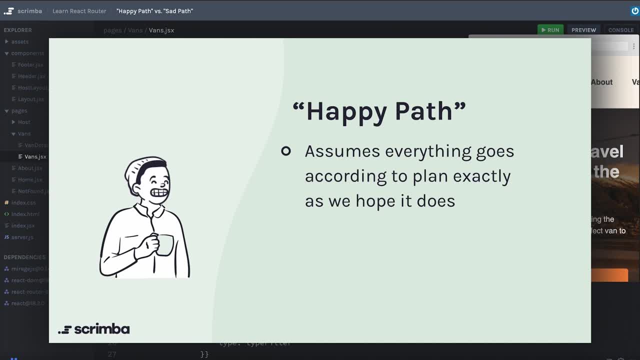 user is going to do everything exactly the way that you expect and everything just goes perfectly according to plan. coding this way can be great for getting something up very quickly if you need to show it off to somebody, but it doesn't account for any errors or other problems that do occur in the real world. so, although it's maybe a little more fun to 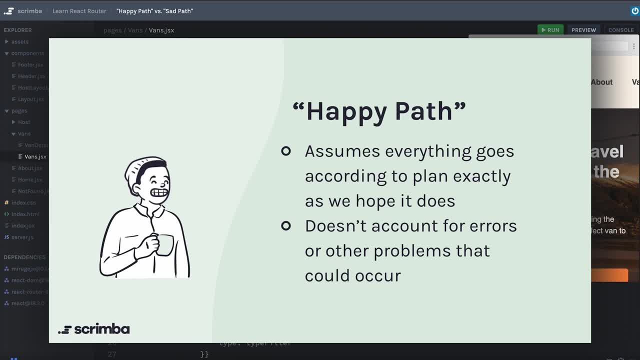 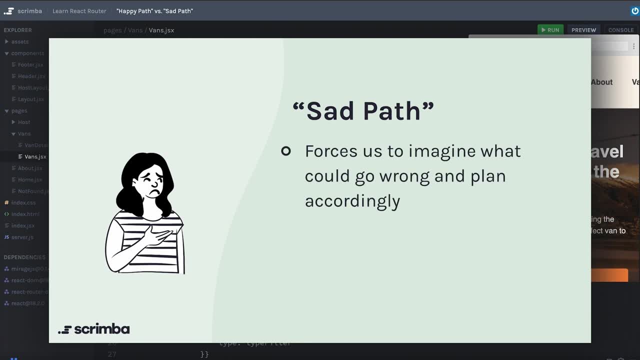 code the happy path, it's important that we, as seasoned developers, will code the sad path as well, and that's where it forces us to imagine what could possibly go wrong and makes us plan accordingly. so let's take a look at some of the other things that we've done in the van life app. 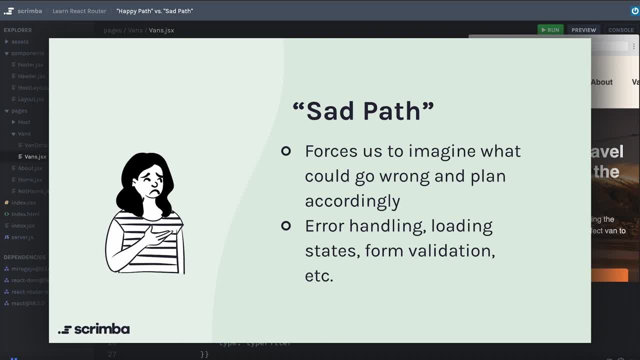 so we've used a lot of applications like error handling, loading states, form validation and all of those other really useful user experience things that you have experienced when you've used real applications. of course, you've also probably used applications that didn't code the sad path and hopefully understand. that can be a pretty frustrating experience that we don't want. 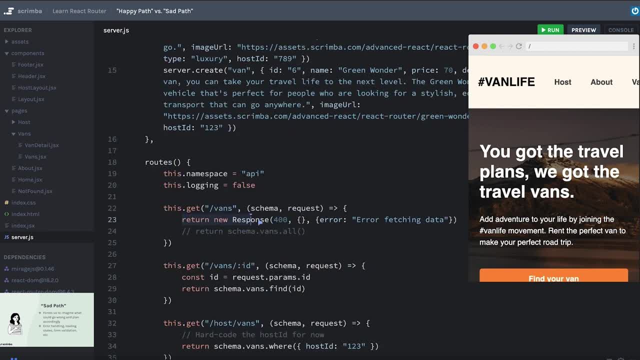 to give to our users of the van life app. let me show you an example of that. i've actually altered the server here to return a 400 level response. that's just a server response. that means that things are broken. it's not sending back what we'd expect. the syntax of this doesn't matter because it's specific to 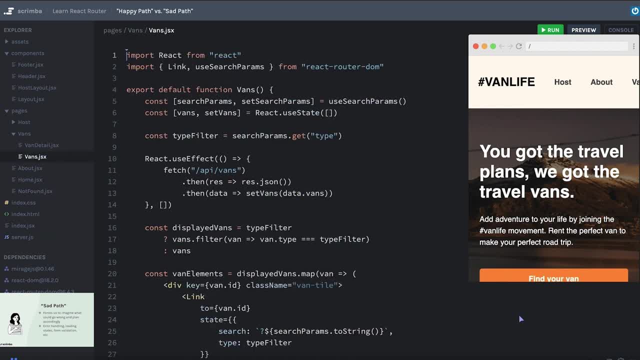 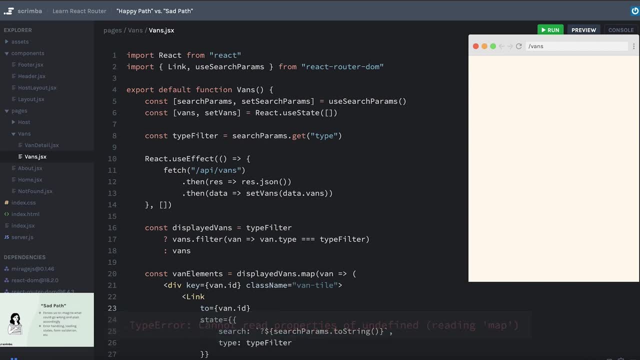 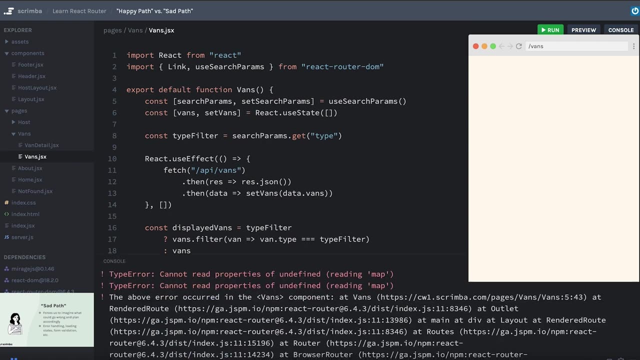 miragejs, but the point is over in vansjs. when we get to our vans page, we'll click on vans and you can see we don't have any kind of useful information about how the vans struggled to load. and maybe try again later, or try refreshing the page or anything like that. instead the app just completely crashed. 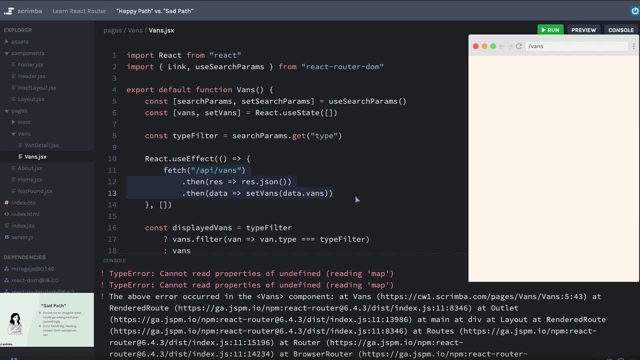 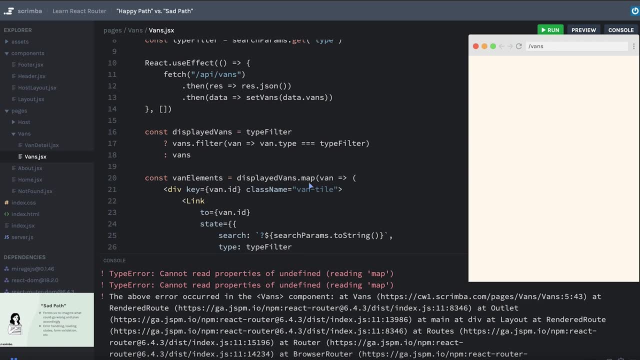 because it is expecting that this fetch request will work perfectly. it's setting the vans state and then we just assume that vans exist and we're mapping over them as if everything were just fine and of course that throws a type error, as you can see in the console, which is causing 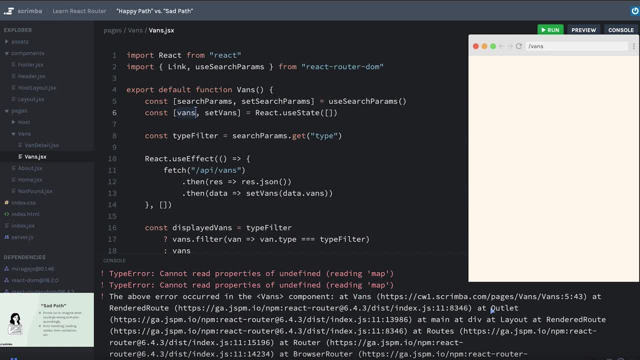 our app to crash. so in the next screencast we're going to see a little bit of the pain that is required for us to handle the error state and the loading state, which will then bring us back to these new data layer apis with react router, and we'll get to see that there's a big improvement. 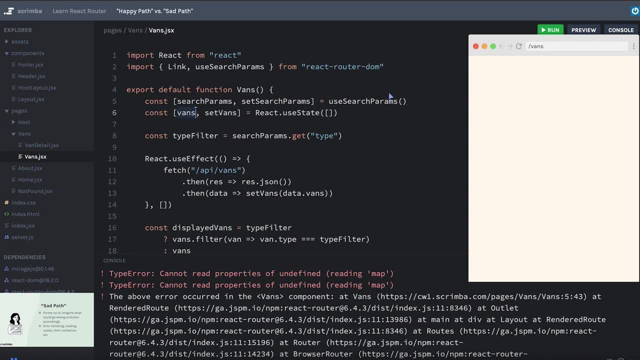 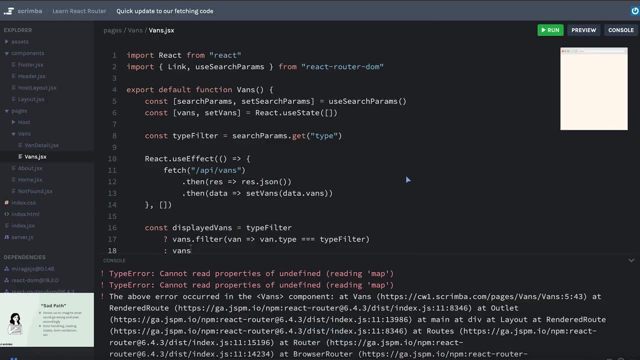 in the way that this can be handled. so let's go through and see how we might fix our code to better handle the errors that we're seeing. the first thing i'm going to do, just for the sake of best practice, is to take my fetch completely out of this component, considering i may want to fetch. 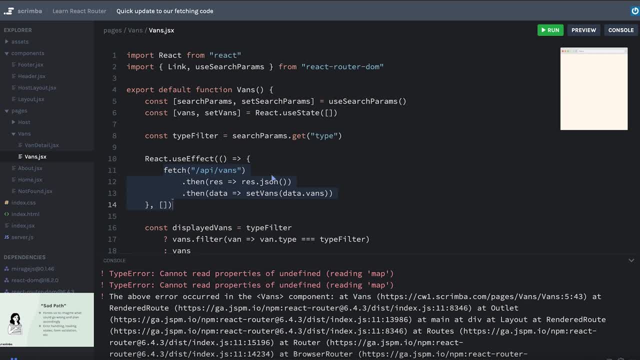 these vans somewhere else. instead of repeating this code over and over, it's a better practice for me to create some kind of library or utility where i can get the vans that i need from a function and then inside of my component i would just call that function. so let me create a new. 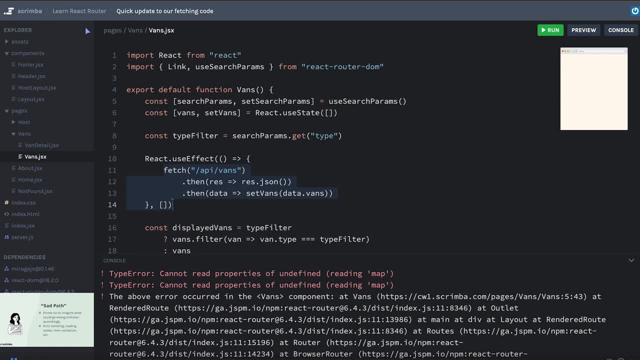 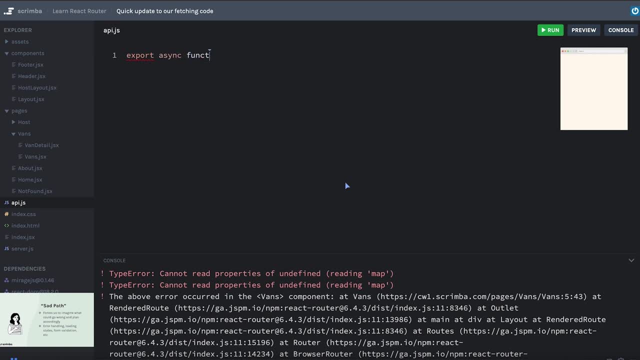 file- we'll just call it apijs- which is supposed to indicate that we are going to be interfacing with the api and i'm going to export. we'll use an async function that we call get vans, since i'm transitioning from what wasn't an async function before to an async function. 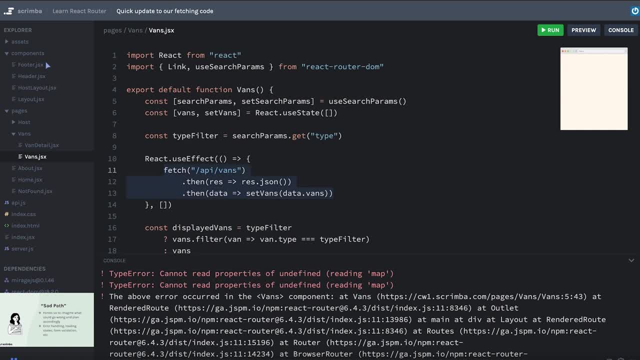 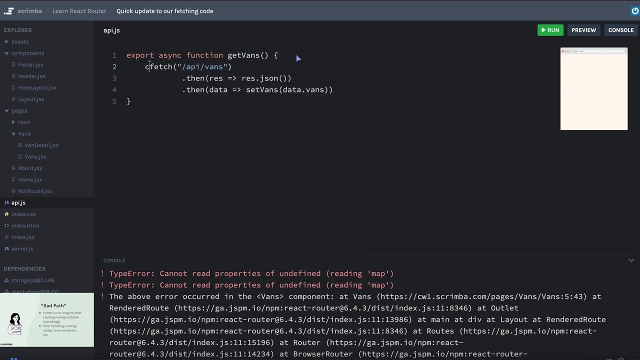 i'm going to be essentially using this code but rewriting it using async await, so let's paste this in as a reference, but we will change up what this looks like. we'll say the response is await fetch. then we will get the data. we'll say const data equals await resjson. 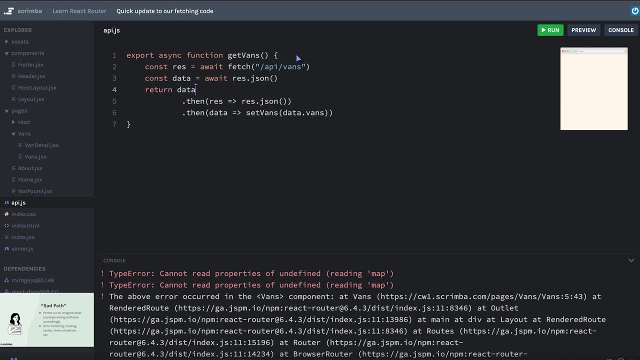 and then this function's job is basically done. it just needs to return the data, and i think it was the vans property on that data that we cared about. so we'll get rid of these lines of code. we're going to come back and actually work on the sad path for this, because right now it's 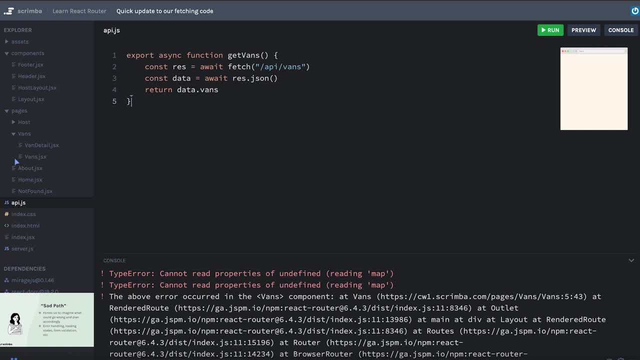 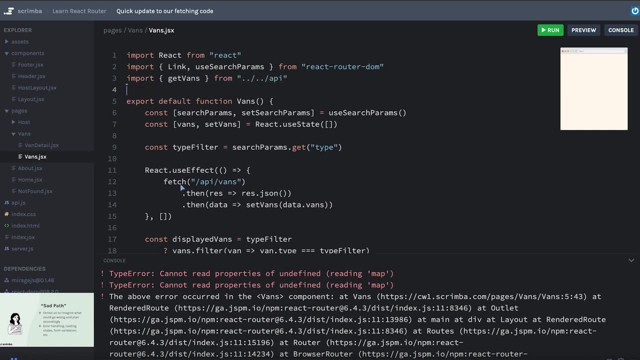 assuming that this fetch request is going to work, just fine. but let's refactor back here. we will import our get vans function and then, instead of manually calling our fetch request here, i could keep using my dot, then promise resolution syntax by saying get vans dot then. but while we're at it, i might 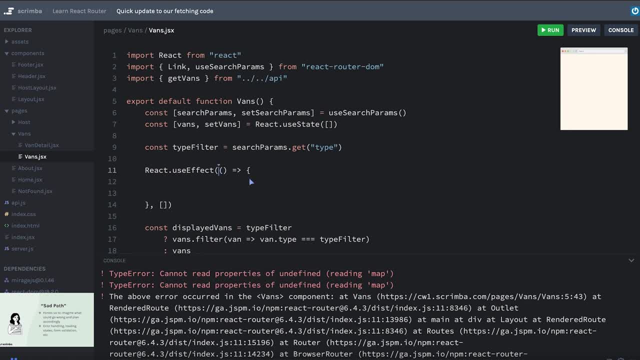 as well, update this and use an async function. now it's important, if you remember from the introduction to react course that i taught- if you took that, that you can't just change your function here from use effect into an async function. so the easiest thing is just to create a brand new async function inside here. so we'll say: 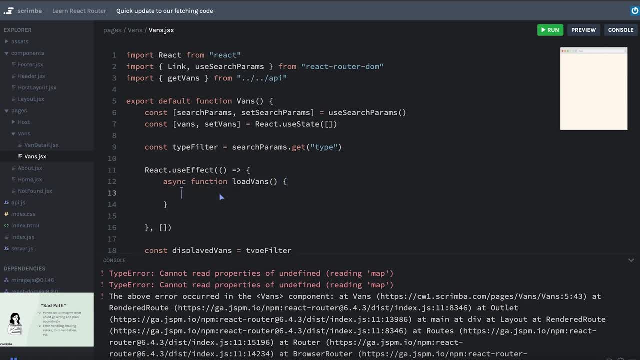 async function. maybe we'll call it load vans, just to get a different name. that's going to call get vans and we will save that data. we will just say const data equals and then we get to await get fans, because we now are inside of an async function. and before i forget, because i do, 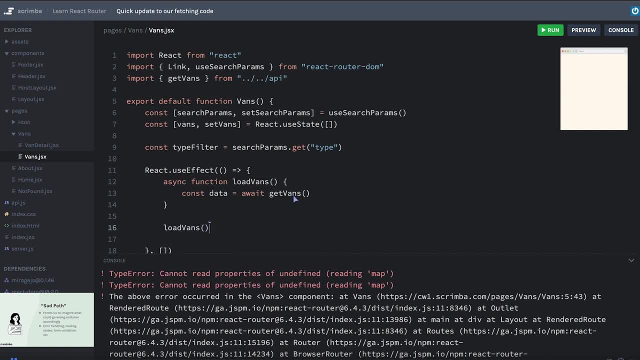 this all the time. i'm going to call my load vans function even though it's not quite done yet. otherwise, sometimes i end up pulling my hair out wondering why it's not working, when it's just because i forgot to call it async function. the function okay. so now i get to call my set vans function and pass in the data that we got from. 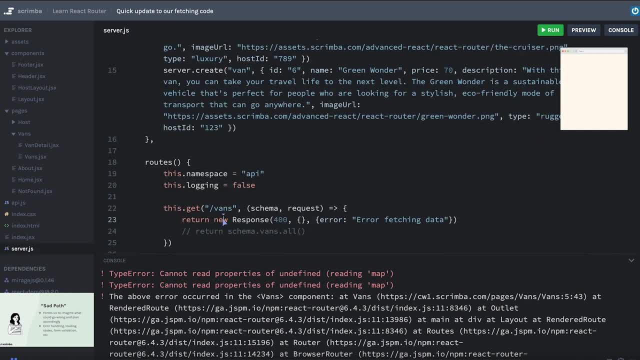 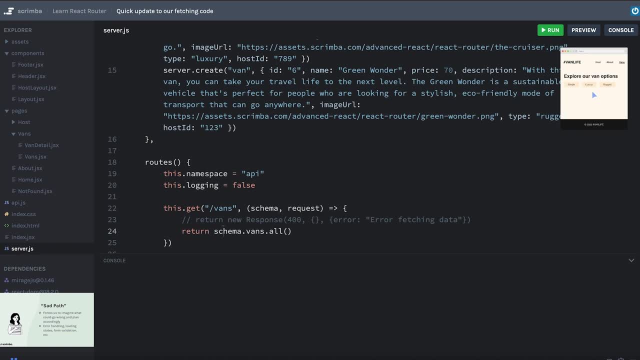 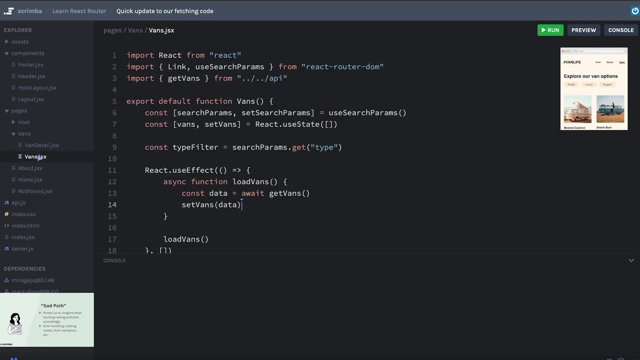 calling get vans. and just to make sure that this is working, i'm going to get rid of this 400 response and make it so that it's working again, so let's hit refresh, okay, good, our vans are showing up. we've made a little bit of refactoring using this apijs file and cool. now let's. 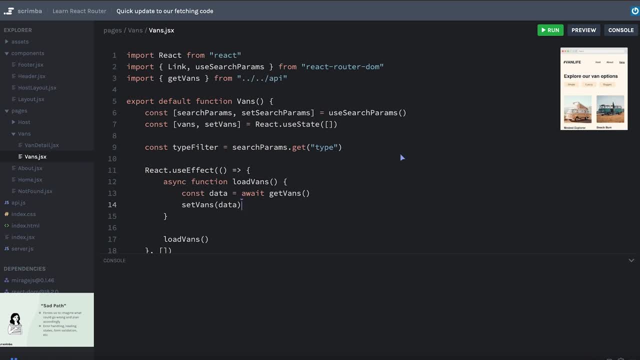 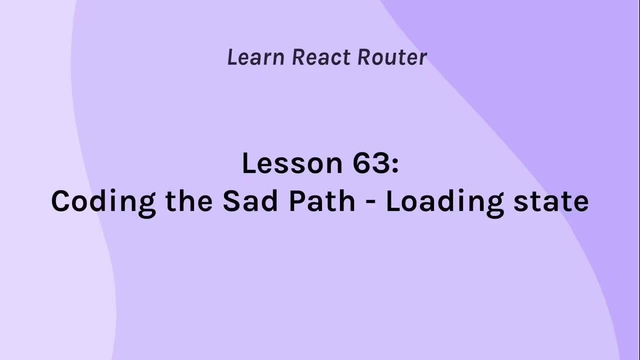 start working on actually coding up the sad path, just for the sake of compartmentalizing the top topics that we've been learning. we're going to do that in the next lesson. One thing about the way that the code is currently running is that we are only initializing the fetch. 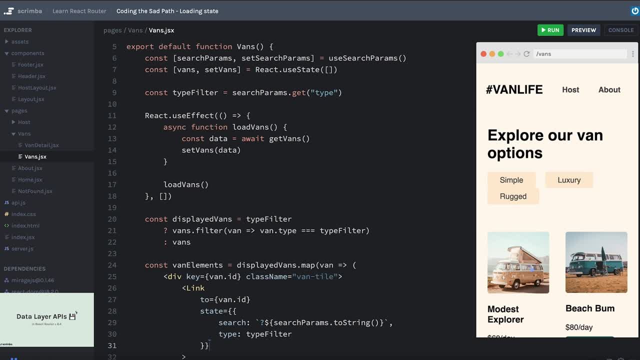 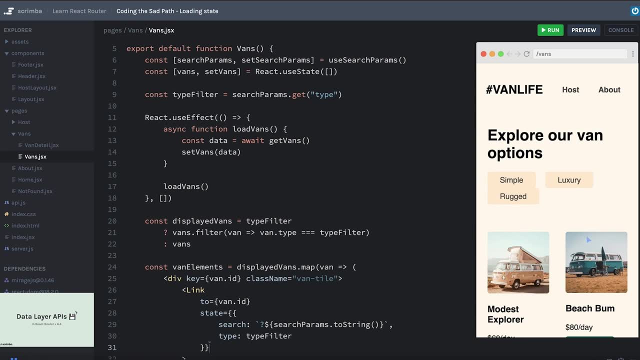 request to get our vans after this component has already been rendered to the page. The experience is a little bit jarring. If I hit refresh, you'll see we get parts of our page and then it starts to load as the data comes in. We do handle this a little bit differently, I think, under host vans. 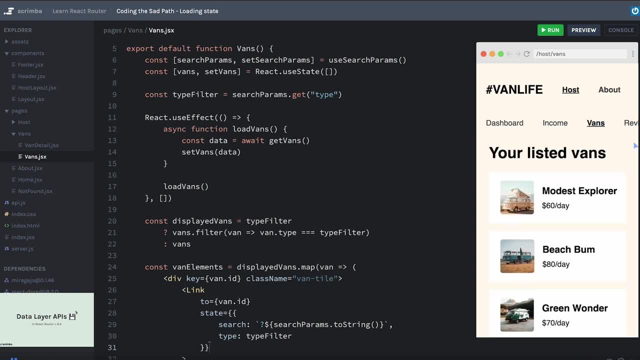 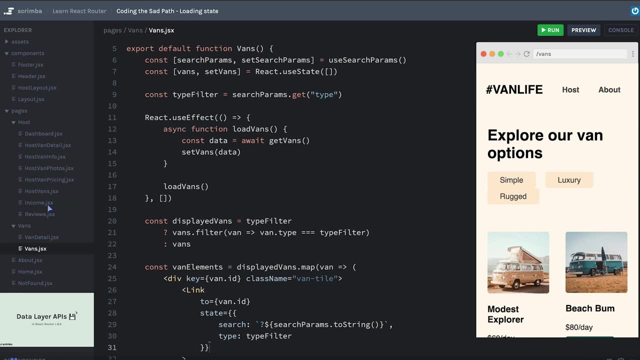 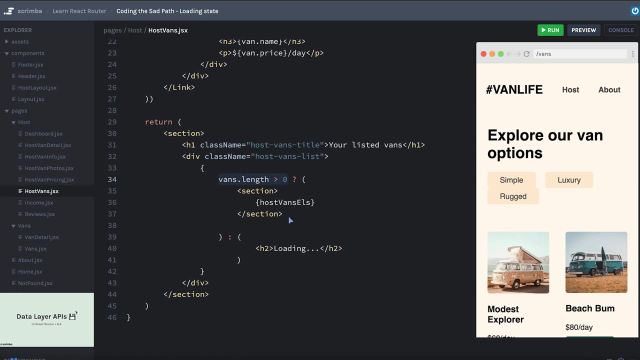 We have a tiny little loading state right there which in my opinion is a better user experience than what we have going on here. Unfortunately, the way that we are handling that in the host vans page, I think right here, is by assuming if the vans length is not greater than zero, then we are. 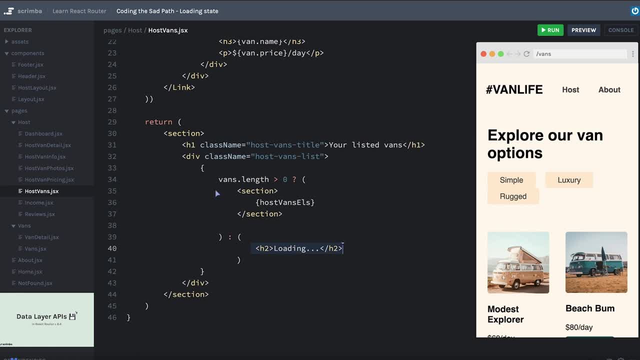 loading something. However, if we have an error, the vans length is not going to be greater than zero. it's going to be stuck on loading forever. Or maybe this is a new host on our platform? they don't have any vans listed. 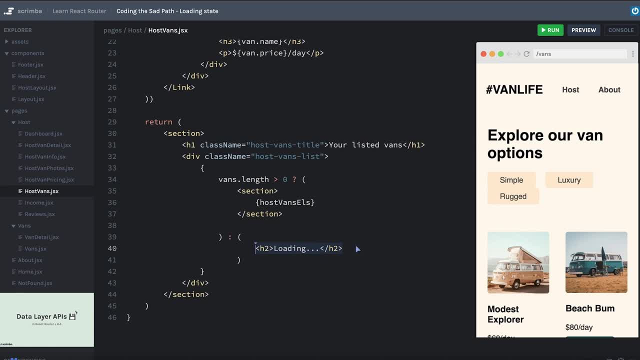 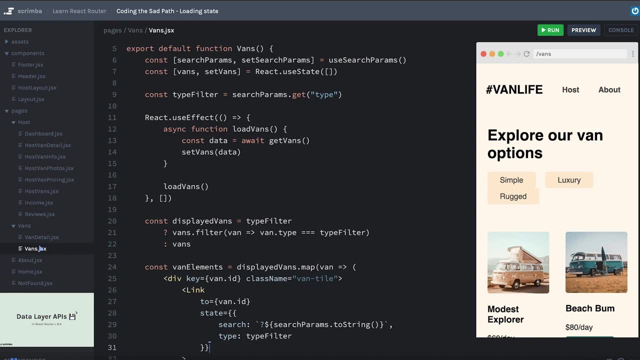 And so when they come to this page, it's going to say loading forever, even though there are no vans for it to load. So this approach was pretty naive and we're going to find a better way to do that. So let's go over to our vans page, And a relatively common way to do this is to set some 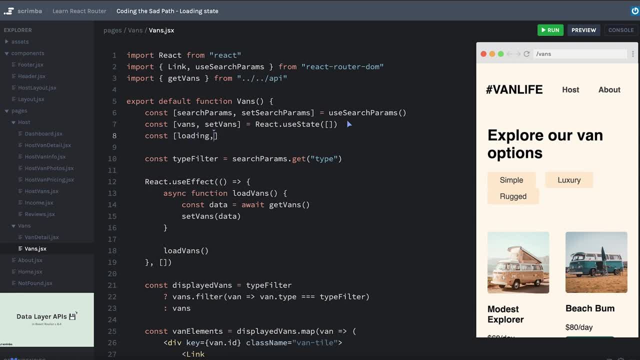 loading state. So I'll go ahead and create a loading and set loading Boolean which we will save in reactuseState. We'll initialize the loading state as false, But then as soon as we call our load vans false, we're going to see that we have a loading state. So we're going to. 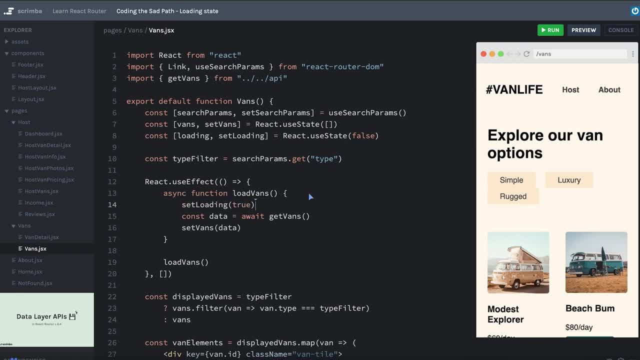 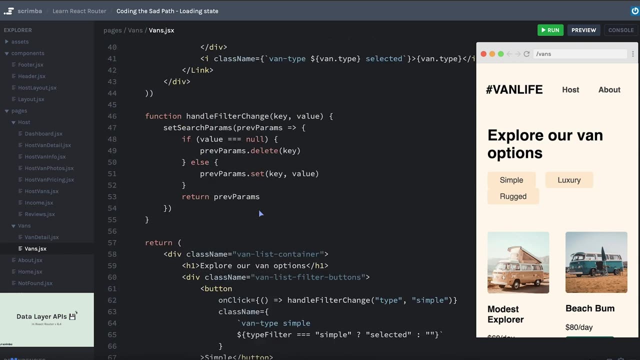 set the loading state to true And as soon as we're done setting the vans in our state, we will set the loading state as false again. So it will only be true for a short amount of time while it's getting the vans. But this allows us to use this Boolean of loading to either conditionally render: 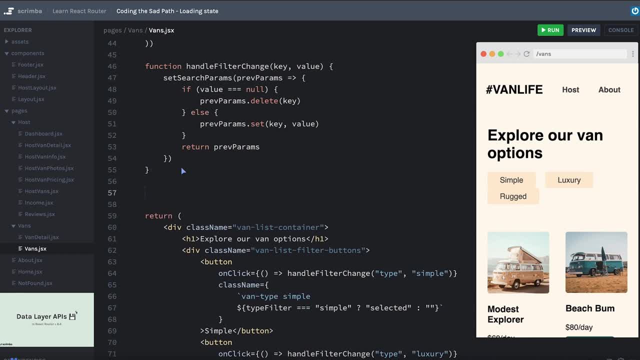 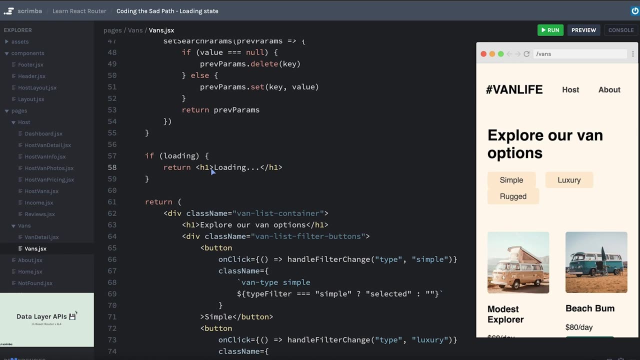 something on the page, or what I think I'm going to do, just for the sake of simplicity, is use an early return. So I'll say, if loading is true, then instead of returning the whole JSX we'll just do something simple like an H1 that says we are loading. It's not going to be. 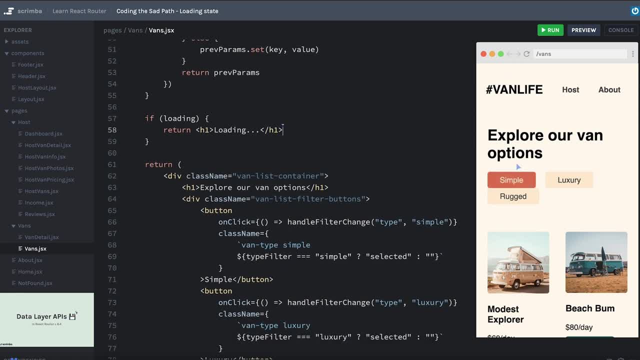 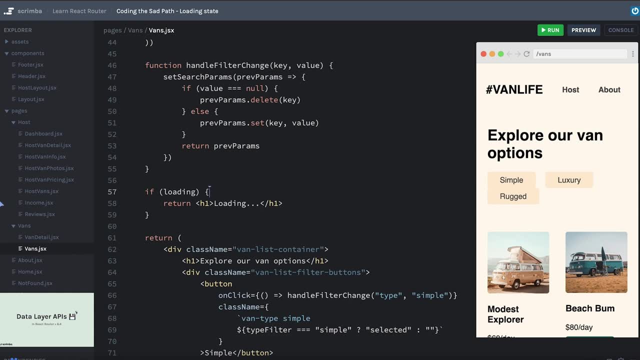 beautiful. We could conditionally render something, maybe underneath our buttons, But for now this will get the job done. Let's hit save And we see our loading for just a second, And then our vans pop in. In fact, while we're doing this, just to make it a little bit more apparent, if I go to 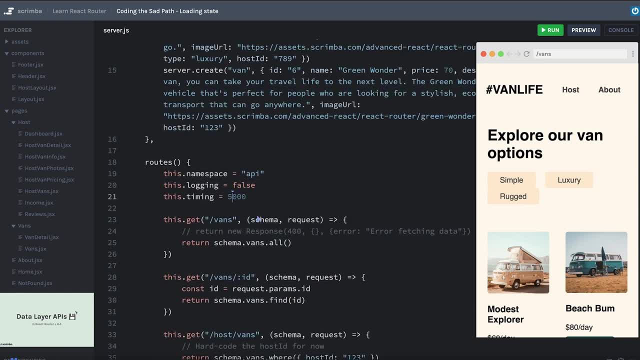 serverjs. I can add this little feature that says maybe, like it will take, let's say, two seconds for things to load. This isn't a syntax, It's just a little bit more apparent. So I'm going to hit save, And then after that I'm going to hit save, And then after that I'm going to hit save. 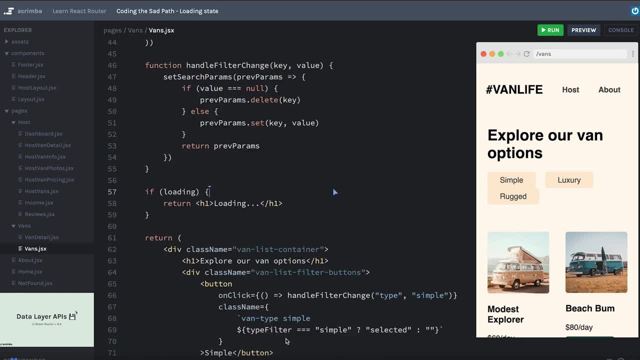 So you need to know again because it's specific to Miragejs. But now if I hit save, it will very clearly show loading for a lot longer than it did before, before things actually get loaded. Okay, that wasn't so bad. We created a loading state. we set the loading to true before we did. 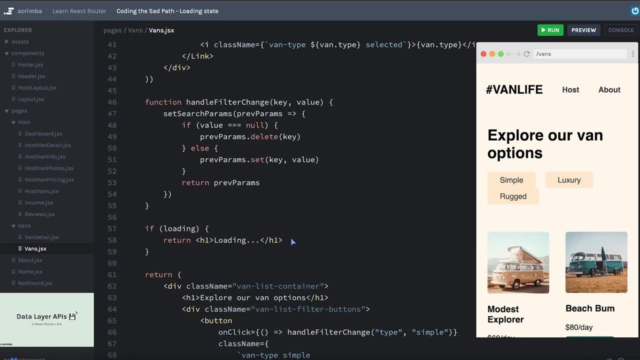 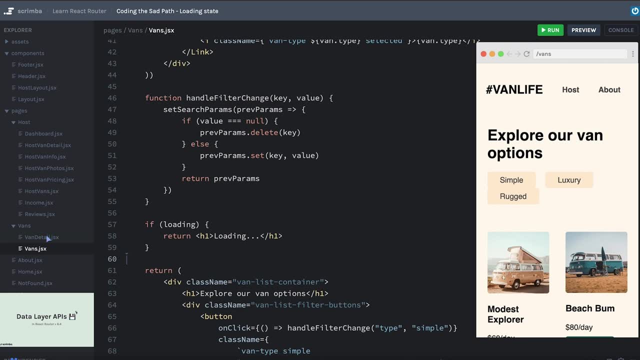 our fetch request And then, after the fetch request, we set it back to false And we handle the user interface case when things are currently loading. Remember, we would need to then do this for every component that is loading data, like the VanDT. 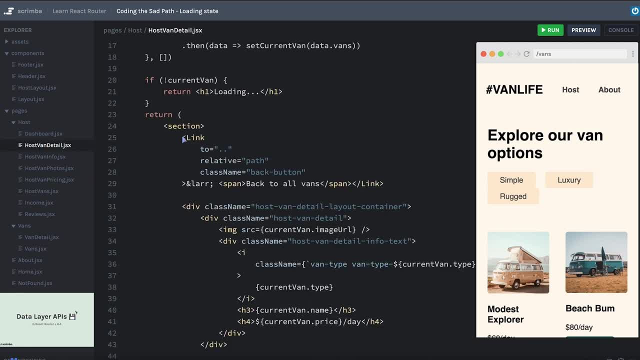 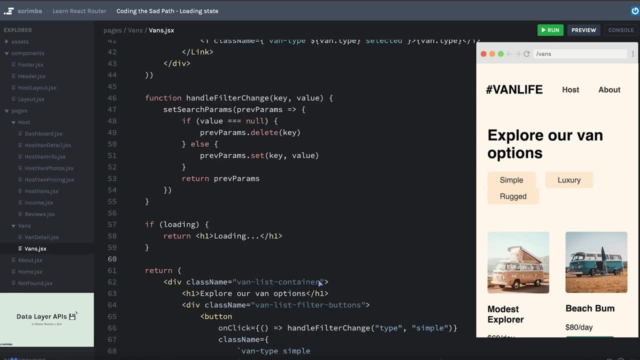 page, the host Vans page, and I think even the host Vans detail page has a fetch request. Yep, For now we're just going to worry about the Vans page, And it's again not so much the sad path per. 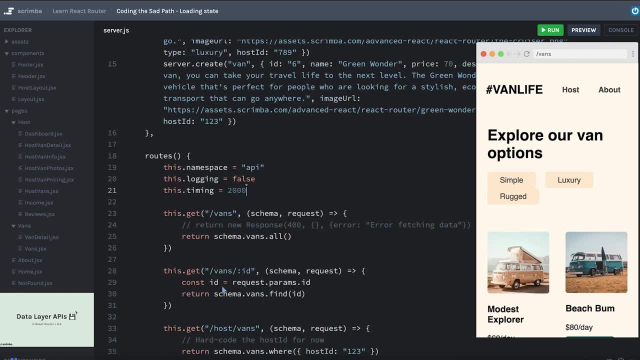 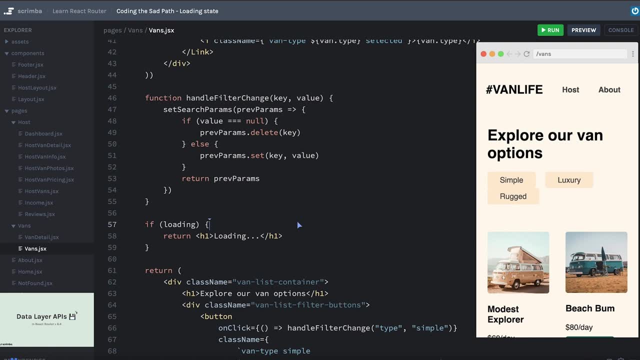 se, because we're not throwing errors right now. But of course, if we were to throw errors like we were doing before, where we're just hard coding a error response from the server, we are not yet fixing that problem, So we're going to have the app crash And that's not good. So in the next, 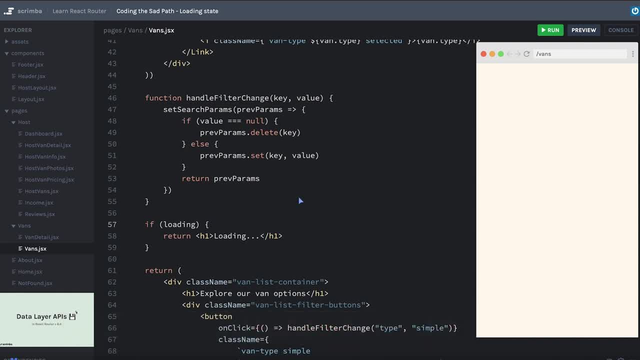 screencast. we're going to talk about how we can handle these errors, And then, after that, we're going to talk about how we can handle these errors. But remember, all of this is leading back to these new data layer APIs that we're going to be talking about. I think this buildup is important. 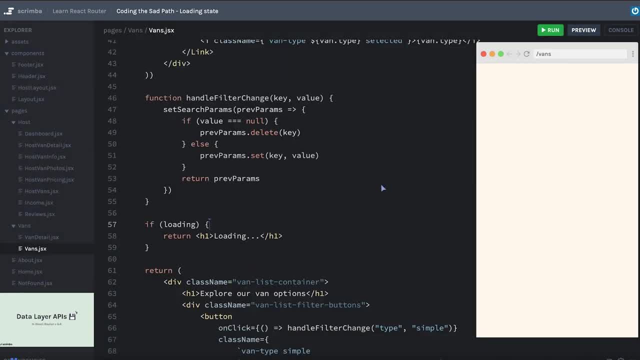 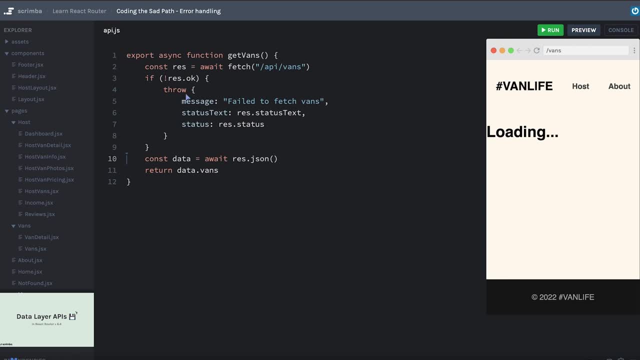 which is why I'm taking time doing it, But this is also just good to learn anyway. Okay, I'll see you in the next lesson. Okay, I mentioned before that we had written our little API: get Vans function in a happy path sort of way. that didn't account for any errors that might be happening. 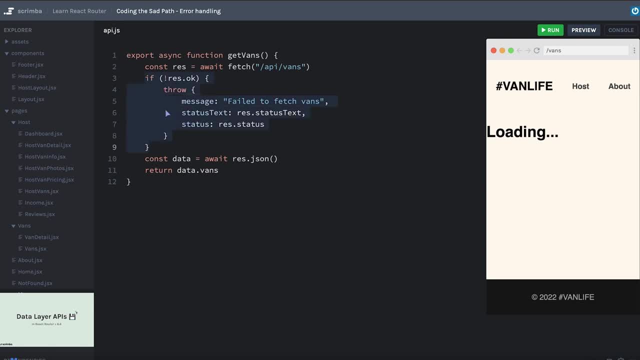 And so behind the scenes, I went through and I added this little check to make sure that the response has come back. okay, this is something that's built into fetch. it will have a res dot okay property And if it's a 400 level or 500 level response code then it will not be. 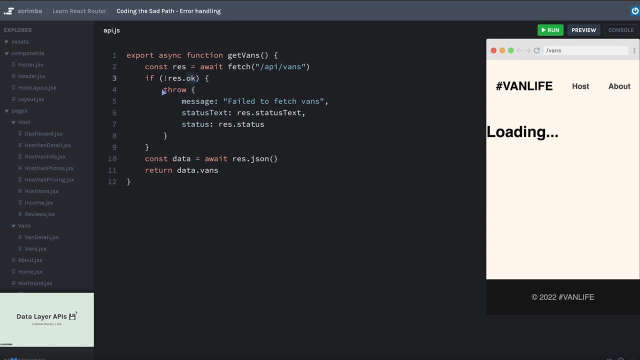 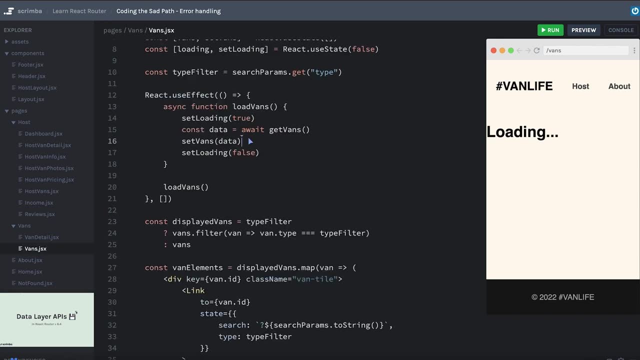 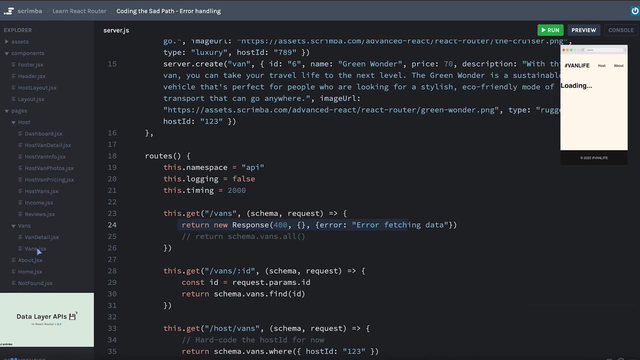 okay, that will be a false value. So if that happens, then we're throwing an error And currently we're not handling that error in our Vans JS page. this is still assuming a happy path, And I've changed the server again, like we saw, to only respond with a 400 response. So let's go to. 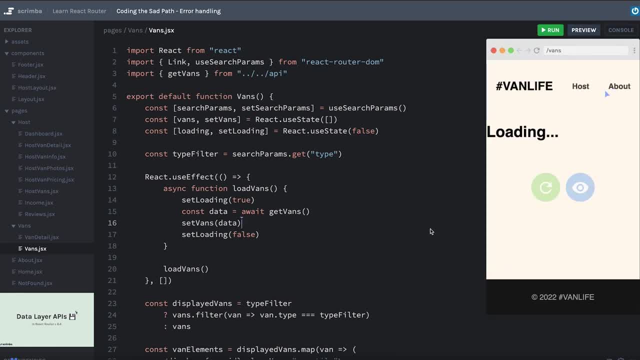 SX And let's handle our sad path here. Now. you'll notice that this says loading here, And that's because, if I refresh this, we'll see that our Vans never come back, but our error is successfully throwing. So let's go ahead and fix this Now. when I'm making this request, because I 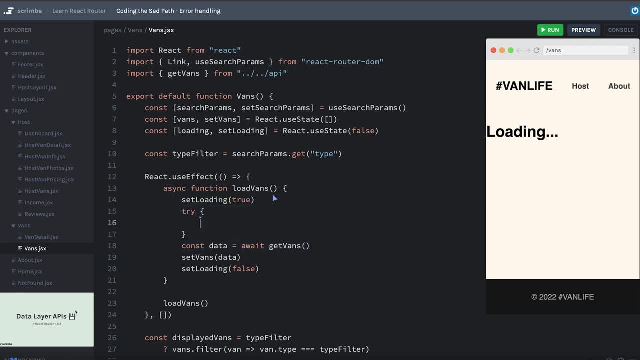 don't know for certain that it's going to work correctly, I'm going to wrap it in a try catch block. This is the common way to do this inside of an async function. So I'll move my set Vans up here, the try will assume the answer, And then I'll go ahead and fix this. And I'll go ahead and. 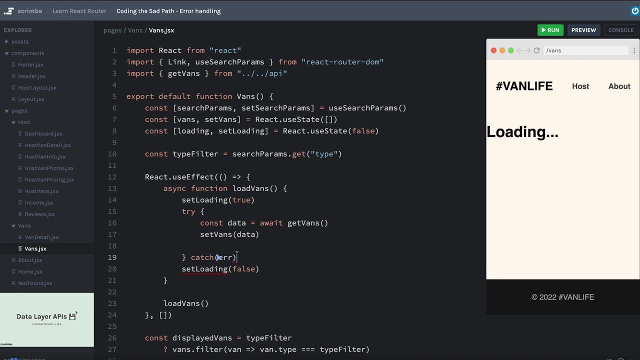 fix this, And then I'll go ahead and fix this, And then I'll go ahead and fix this, And then I'll happy path. But now I have the ability to catch any errors that might happen, And the catch block will be the sad path. Now, what should happen when I get an error? Well, first let's just console. 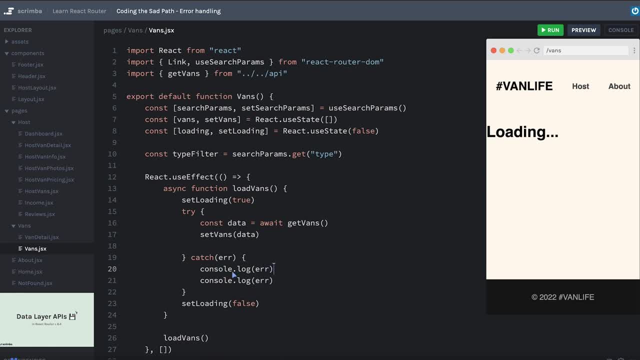 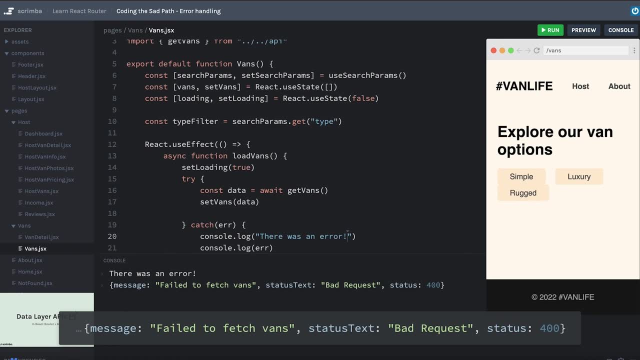 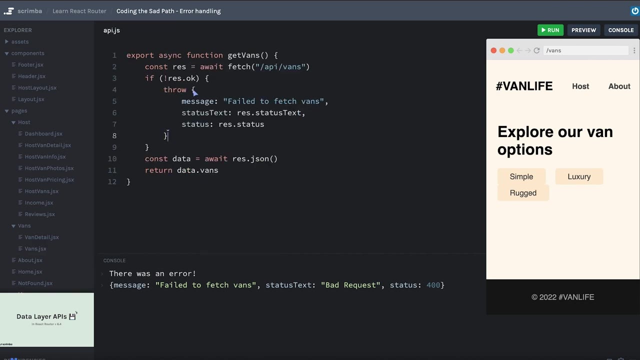 log the error to see what shows up. And actually let's go ahead and console log something like there was an error in the console. Okay, we get there was an error And look at that, we get our error that we threw from the server. No, from the API file this object. 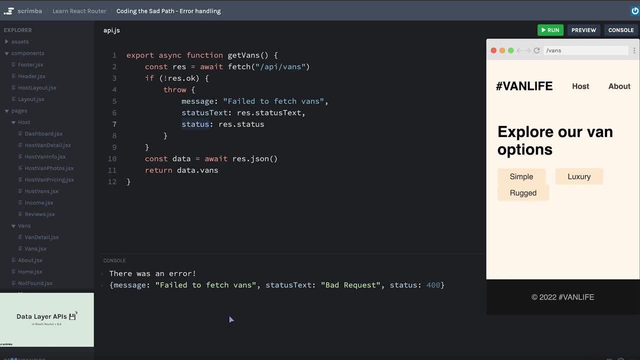 here that has a message, status text and status. we can see that that is coming through in our console just fine. So now we are handling that error. we're not displaying anything, but we no longer show loading. we just don't have any Vans to display. That's not super useful for the user. 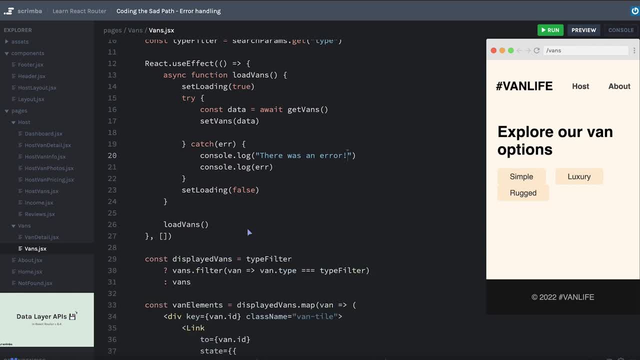 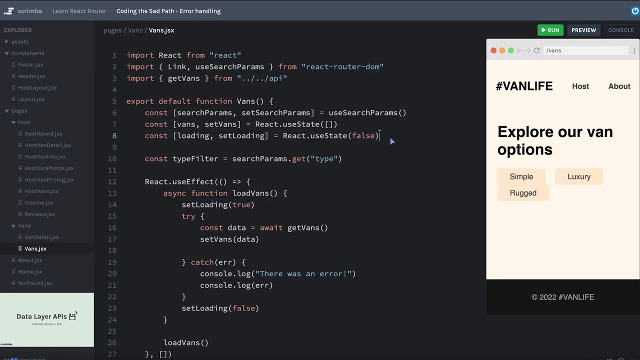 So let's go back to Vans jsx. we'll buy ourselves some room by closing the console And, similar to what we did in the loading state, we're going to create another state that is for errors. So we'll say: if there is an error, we will. So I have set error. we'll probably start this out as a null. 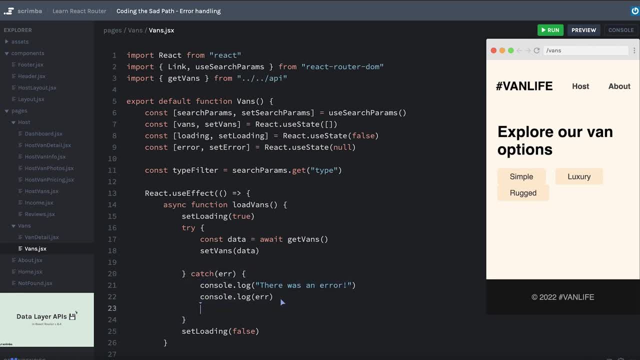 error. And if there is an error that happens here in my catch block we will set the error And we'll just pass in that object that we got from the error that got thrown earlier. Let's go ahead and get rid of our console logs And just because it exists, I'm going to use a finally block. I. 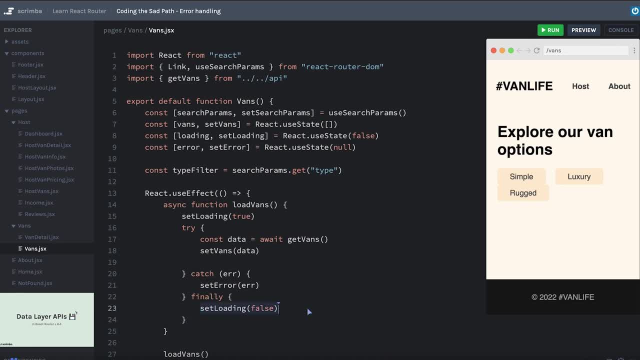 don't get to use this super often, So go ahead and put our loading to false, Because whether we get the Vans or we get an error, we want to set the loading back to false. Okay, now we can handle the case when there is an error. we have this early return for loading. 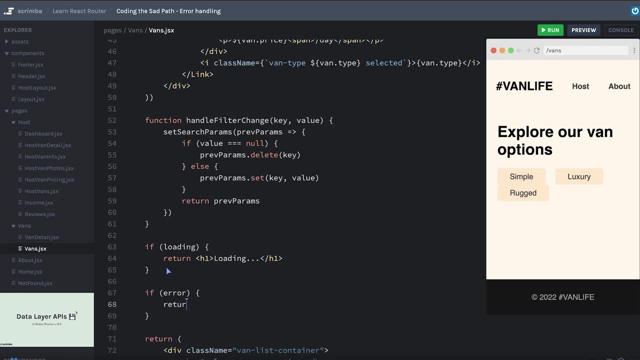 we'll do the same thing if there's an error. So we'll say: if there's an error, we'll return. let's just do another h1 for now, And we'll say there was an error, And then we'll go ahead and just stick. 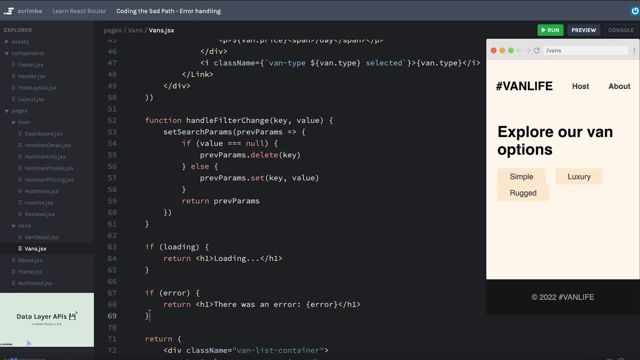 the error in there. Let's see what that looks like. Again, I'm hard coding an error in my serverjs, So we know that it will error And it's taking a lot longer than before. Okay, so I can't do this whole error object here. Let's. 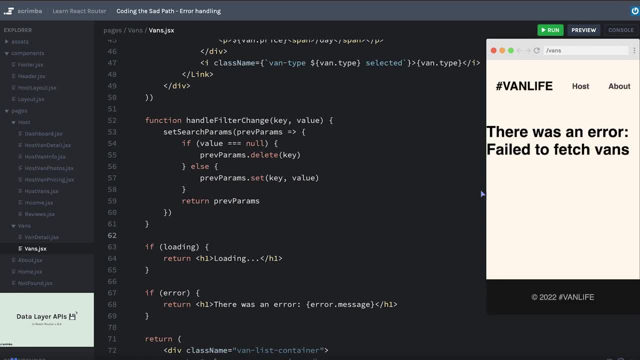 maybe do. error dot message, I think, is what it was. Okay, there was an error failed to fetch Vans. It's not beautiful, just like our loading isn't beautiful, But it is some feedback to the user that tells them that something happened. Now again, we would want to do this for our van detail. 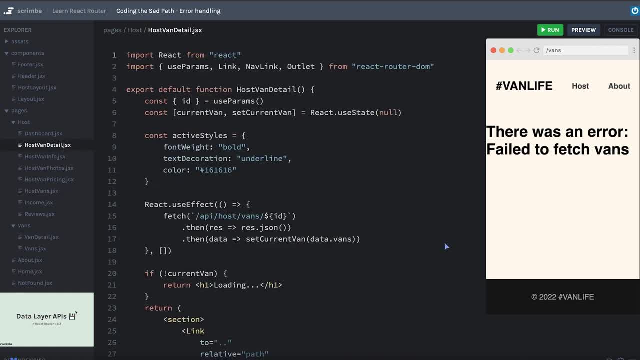 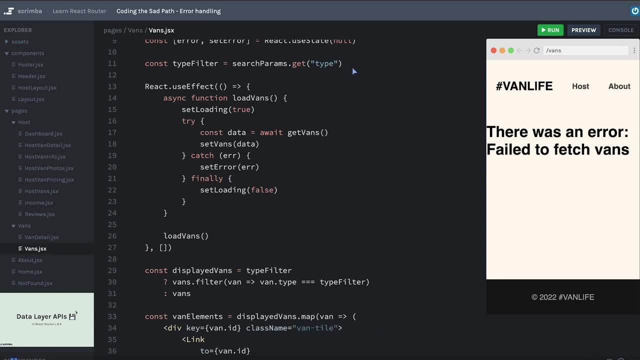 page, our host Vans page, our host Vans detail page, And hopefully you're starting to see that there's a bunch of repetition. there's a lot happening just to handle this sad path And, if you think really hard about it, a major reason that all of this is happening is because we are only starting our fetch request. 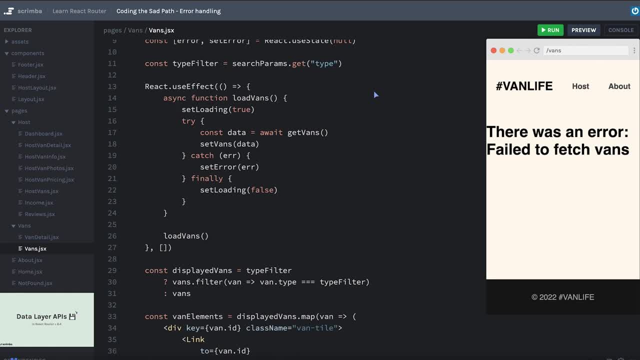 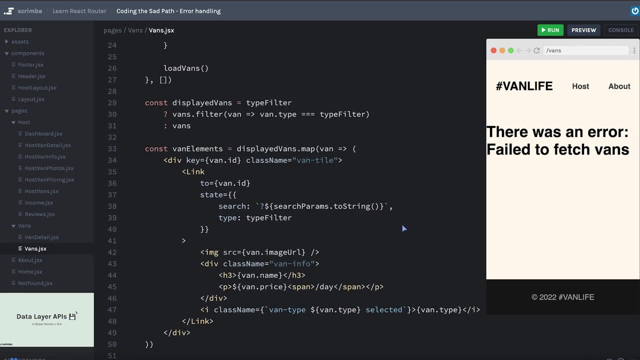 after this component loads. Remember when we weren't considering the possibility that Vans would not come back as an actual array of Vans? That's back when we saw that when there was an error in the server, it actually crashed our app because we were trying to map over something that was not an 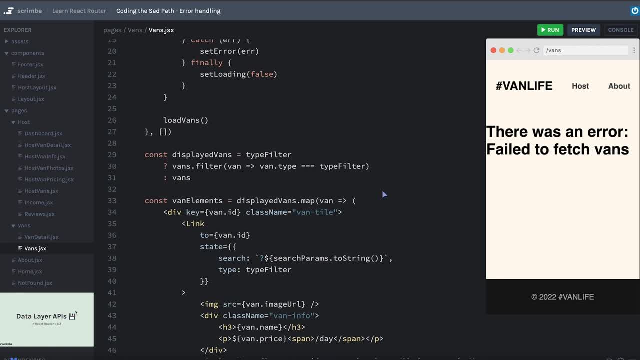 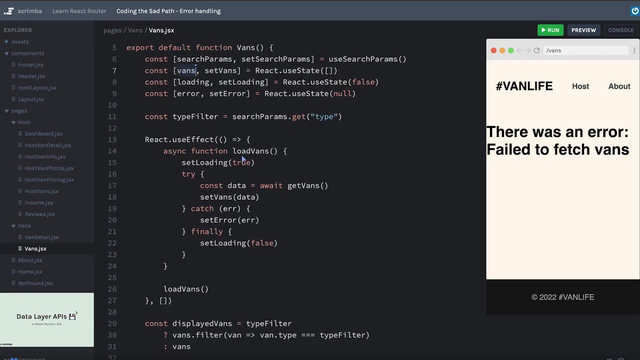 array. Well, if we didn't load this component before we had access to the data, then we wouldn't have to worry about that, And theoretically, the same would be true of the loading state and the error state, Because we're sort of prematurely jumping to this route and then starting a fetch request for the data. 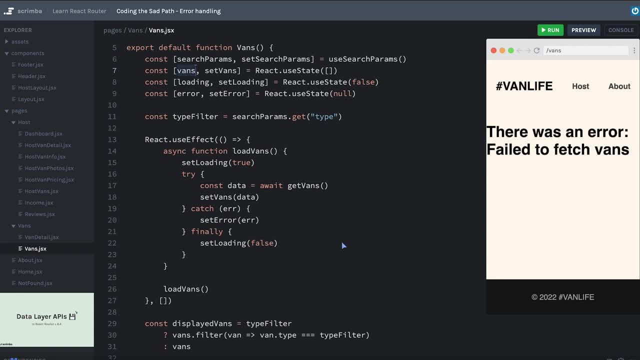 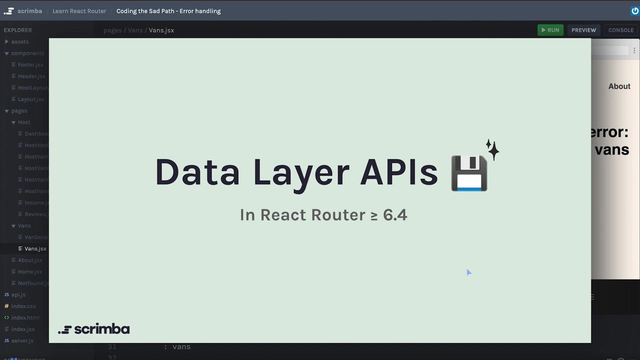 there's a bunch of little edge cases that we need to handle. Now all of this leads us back to the data layer API's. react router has introduced to us a way that we can load our data before it ever transitions us to the route, which will allow us to get rid of quite a bit of our boilerplate code that we have here. So let's finally dive into these data layer API's, and we have a bit of setup to do before we can use them, So let's get started with that. 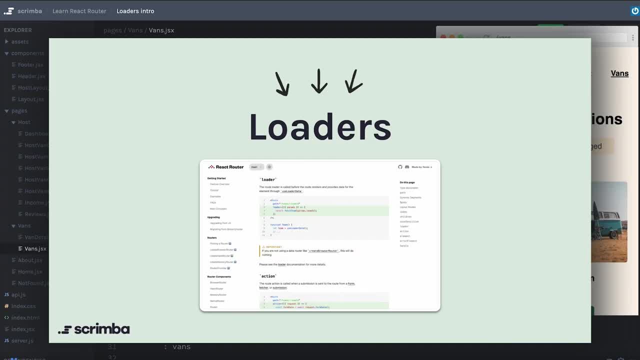 The first aspect that we are going to learn about in the new data layer API's and react router is loaders. you can click on the screenshot here, which will take you to the loader prop in the route component, which we're going to get to in a little bit. but I think it's helpful to know that the data layer API's are not going to be the same as the other APIs, So let's get started with that. 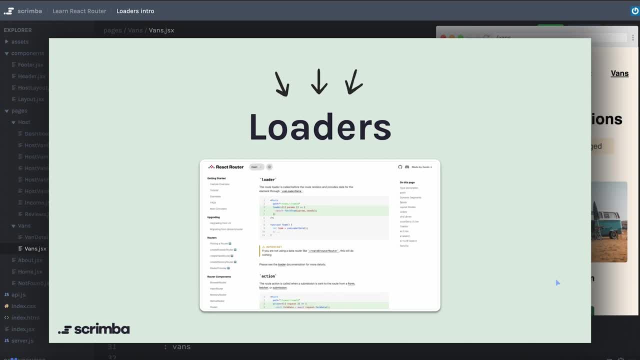 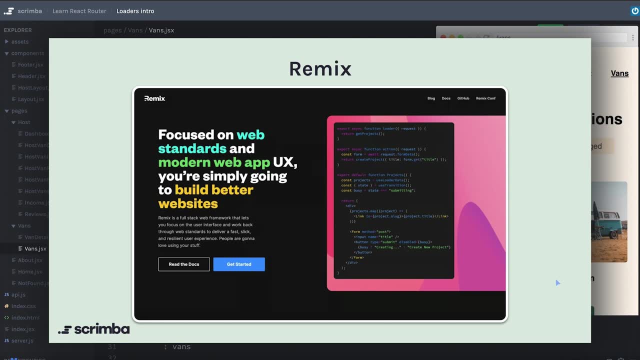 So let's get started with that. Take a look at the loader information here and we're going to look at how Much опасness there can be faced with a loader and being людям to have a Client thinnest layout algorithm and then father-원�始까지. 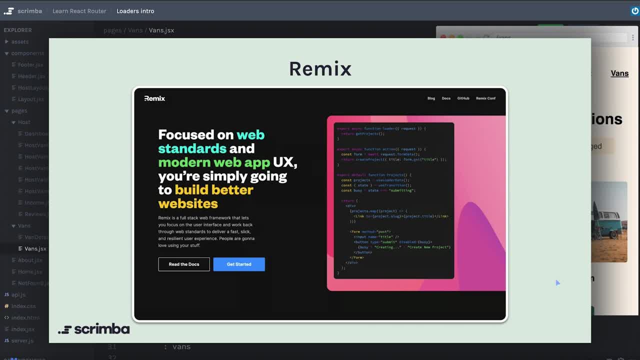 allow if you want to show the loader needs. That's no need to be put an example of how far we can go. Even on the Glowty play. uploading an API is going to be really hard to over. like go to all the space. 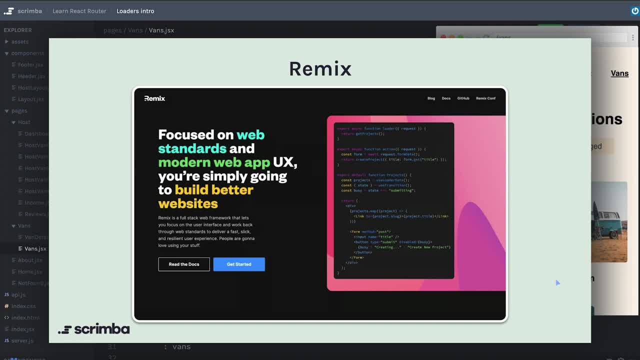 and it can take a lot of work After that. we're especially familiar with Grub holding. I also know that the creators of react router are also the creators of a framework called remix, else called actions, directly into react router. in fact, you can even see if you look closely. 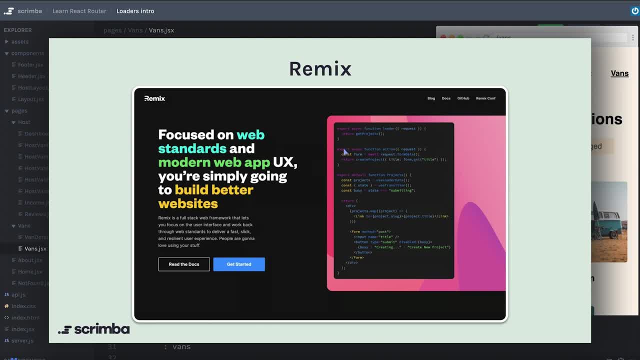 in the screenshot, we'll see this export async function loader and there's this export async function action. that's the aspect that i'm talking about: loaders and actions. so how does this affect react router? well, as you saw, we are currently using a use effect in order to fetch our data. 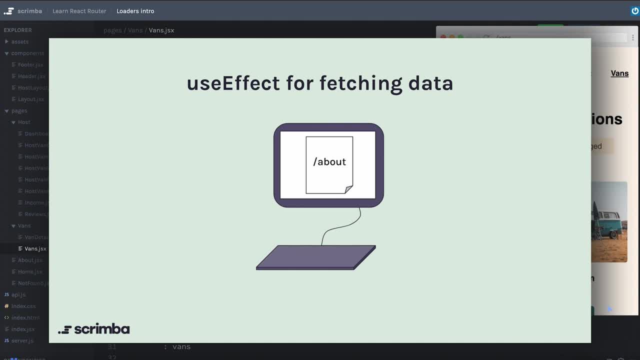 and for a really long time in react. this was kind of taught as the de facto way to fetch data for your components. let's say that i'm currently on the about route and i want to transfer over to the vans route, so i click the link in my navbar which will take me to vans, and what happens is: 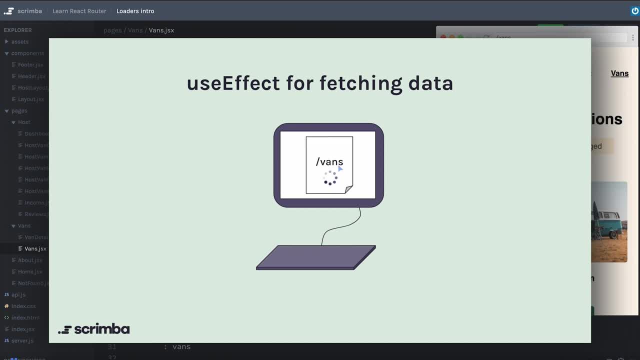 the about page goes away, it gets swapped for the vans page and because we're fetching our data inside of a use effect, it immediately starts loading the data, or rather fetching the data from some external source. oftentimes this request is pretty fast and once the request comes back with 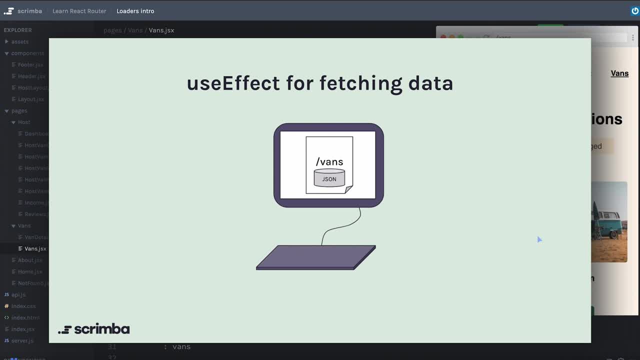 a response. then we get some json from the API that we were fetching data from, And then React does its thing, where it re-renders, It, takes that JSON and displays it the way that we told it to in the code. And we can certainly make this. 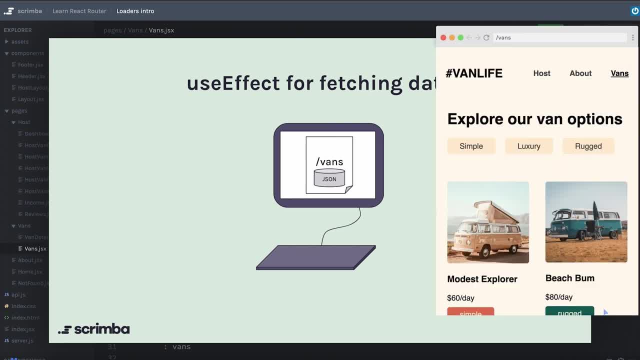 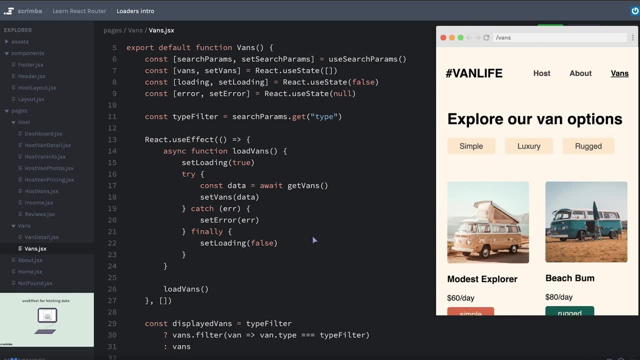 work. Like I said, this is how things were done for quite a while. But, like I mentioned, because we're only loading the data after we have already loaded the page, or rather mounted the component that represents our page, we have a lot of extra stuff that we need to add. We're saving state for 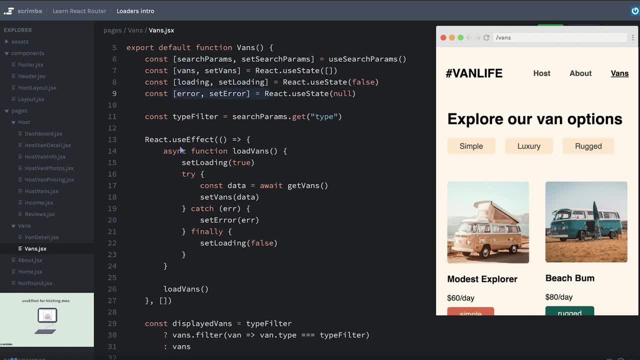 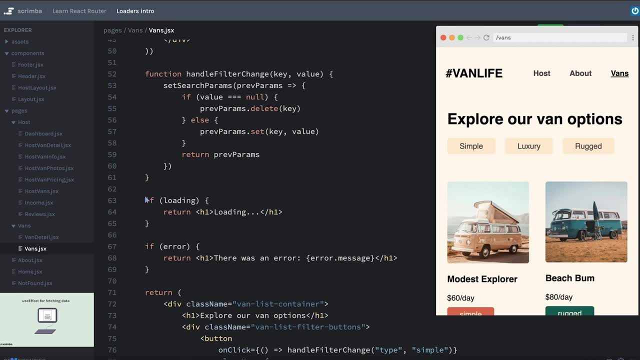 the vans themselves, the loading state, the error state. We have this use effect which is calling the data, and it's got some error handling built in. We're also handling if it's currently loading and if there's currently an error. And it's certainly not the end of the world, But let's. 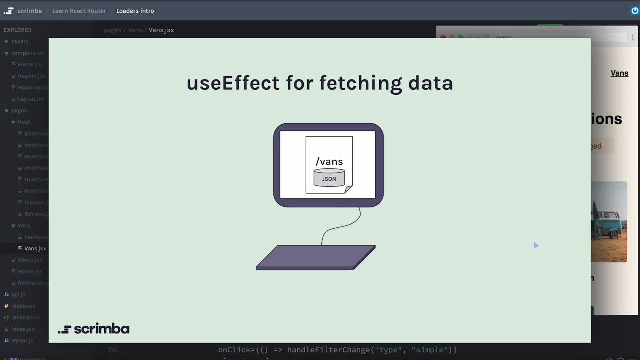 take a look at the paradigm shift that we're about to learn when we use a loader for fetching our data instead. This might seem like a small tweak, but we're going to see how it can dramatically change our code. So we're here on the about route, We click over on the bottom of the page and we 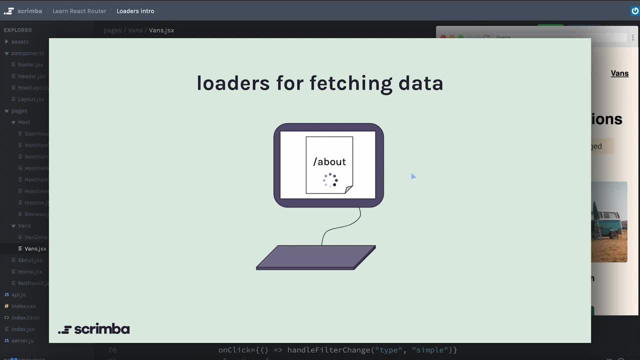 click on the vans route And the first thing that happens is it delays for just a moment or two. During that delay it's starting the fetch request to get the data for the vans page And that way, when the data is finished, coming back from the request, it is already a part of the vans page. 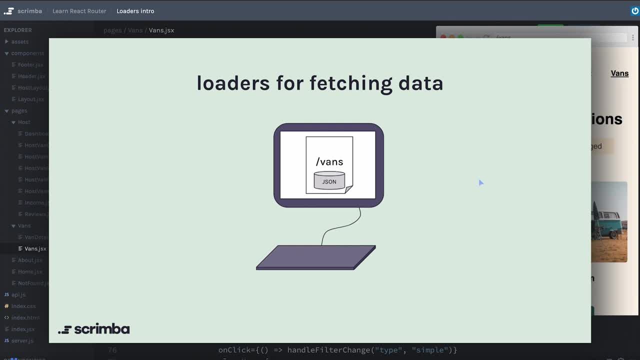 when it gets loaded up. Again. this might seem like a small difference, but we're going to see how it's going to allow us to simplify quite a bit of the code that we have Now for a high level overview of how we will end up using loaders. the first thing we're going to do is we're going to 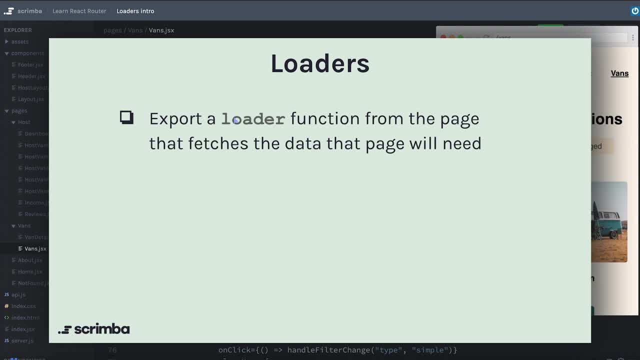 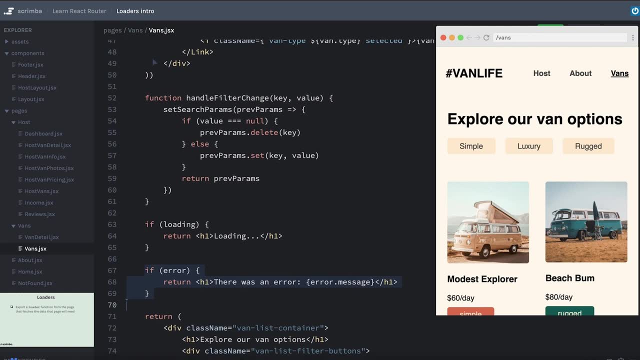 export a function, we will call it loader. it doesn't technically matter what it's called from the page that will fetch the data that it needs. In our case, we're going to be working on the vans JSX page because this page needs data, So we're going to be creating another function that isn't 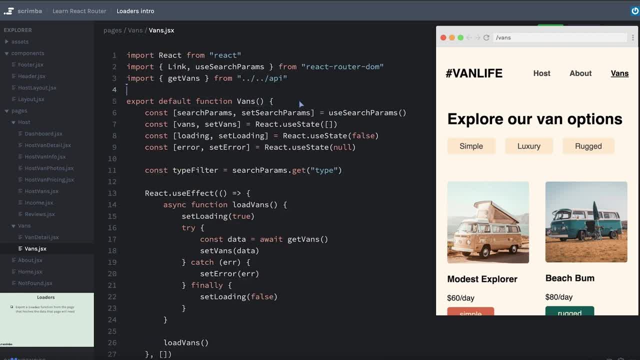 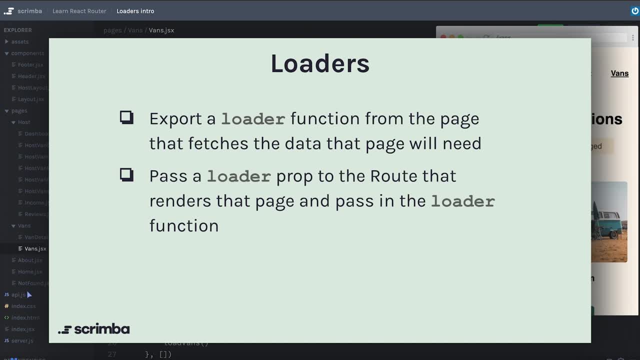 our component. it'll just be right here above it probably, that we'll call loader And that will be the function that gets the data, Since we're exporting it from here over in our index JSX where we have our route definitions. we're going to export a function that gets the data And that's. 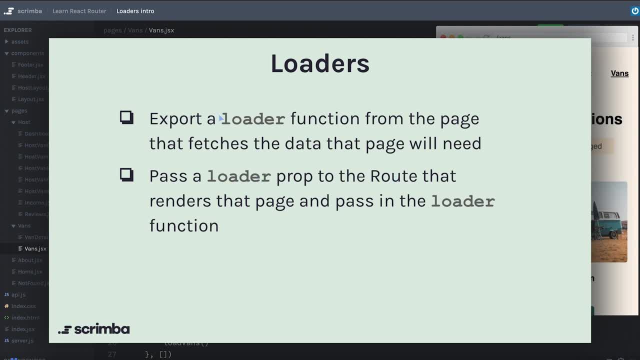 going to pass a loader prop to the route And we'll pass in the loader function that we exported from our vans page And then back in our vans component. we'll use a new hook from react router called use loader data, which allows us to get whatever data was returned from the function that 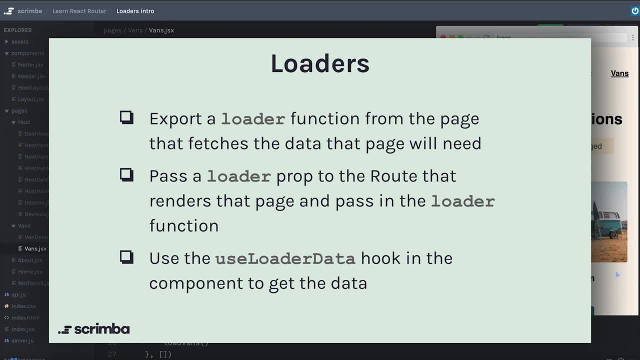 is doing the fetch request Again. this is a high level overview. we're going to obviously go through each one of these steps, So don't worry if this seems a little overwhelming. There is one tiny little problem before we can start working on this, And that is we need to opt out of the 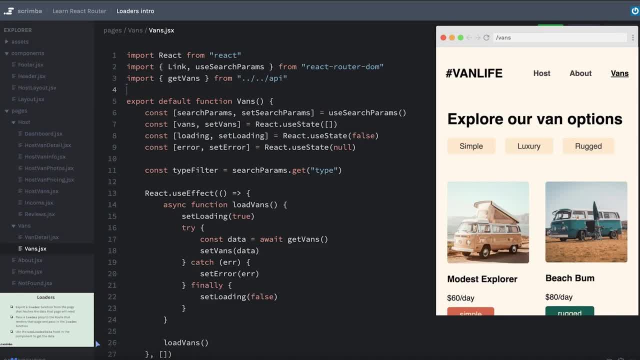 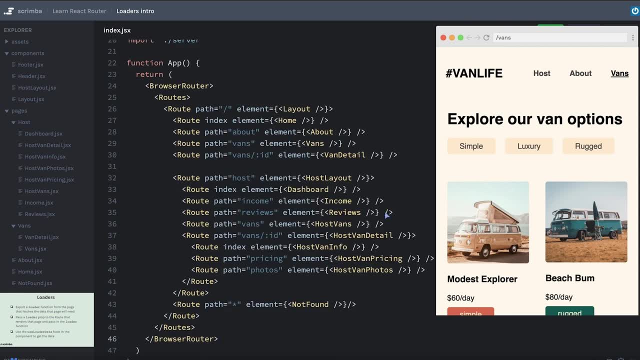 vans page. we need to opt in to the new data layer API's, And the way that we do that will require us to make some changes to our browser router setup that we have here. So first we're going to tackle that And then we'll be coming back and actually creating our loaders and changing how the data 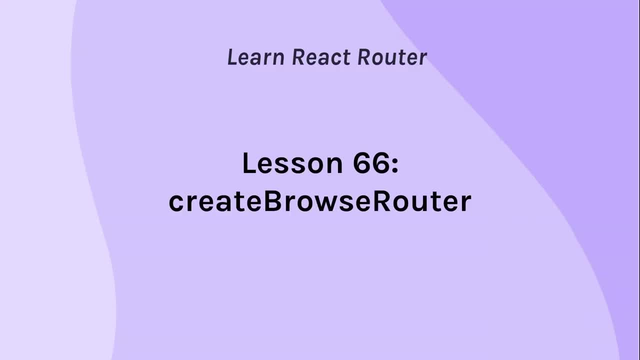 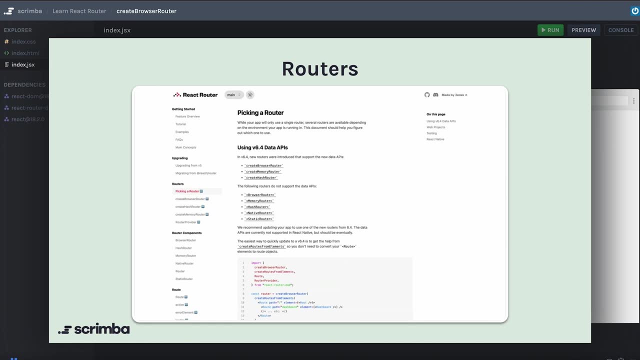 loading happens on our vans page Before we can take advantage of any of the data API's in React router 6.4.. And later we need to change the way that we're instantiating or creating our router. you can click on the. 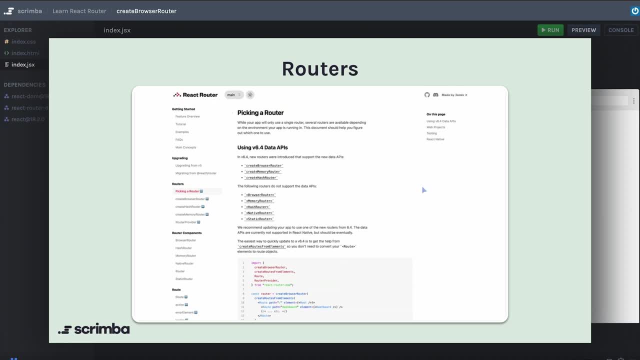 screenshot here to go to this, picking a router page in the React router docs. But you can see from the screenshot that there are a couple different ways to create routers that do allow us to use the data API's And then there are some other ways that won't include the capabilities of the data API's. So you can see the top of that list that does. 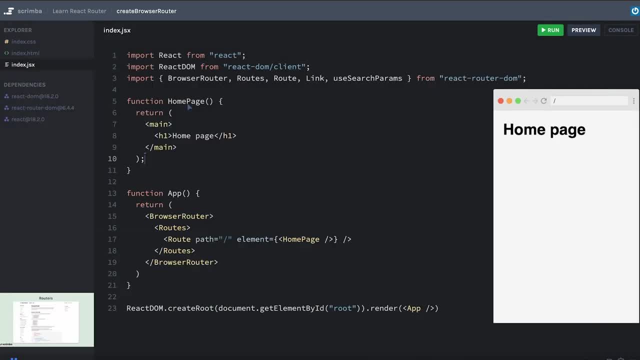 not allow for the use of data API's is the browser router, And that's the one that we've been using. This is actually that silly Star Wars app that we used when we were learning some search params. I've cleared out anything that wasn't really relevant. Actually, there's a couple other things up here. let's get rid of those And you can. 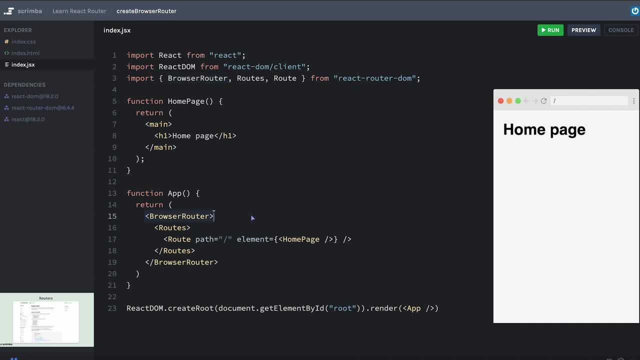 see that what we were doing is importing browser router and then just creating an instance of the browser router component here. Well, in order to use these new data API's, we need to create our browser router in a little bit of a different way. So the first thing I need to do is import something called create browser router, And maybe the astute 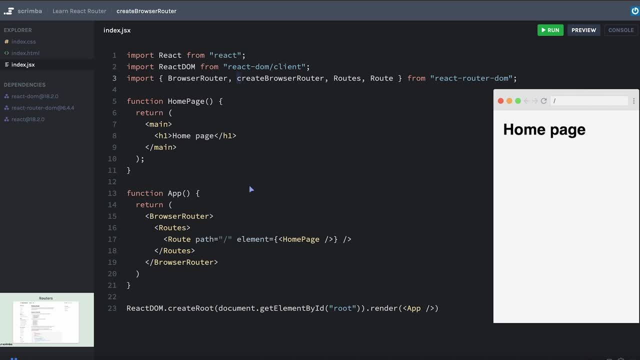 amongst you would notice that with the lowercase c, that means that this is not a component. Instead, it's a function that we're going to run. So I'm going to save the router that this function returns. So I'll call create browser router and then save it. 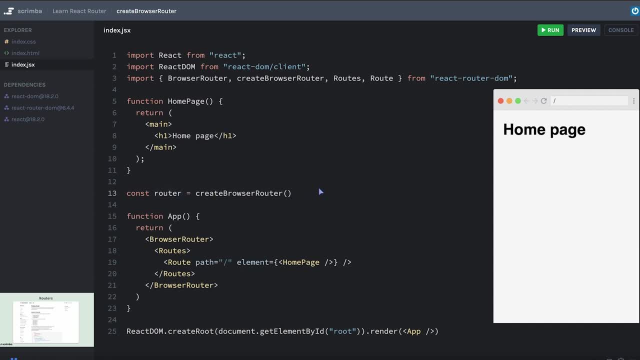 as a variable called router. Now, what we have always learned, what we've always done, is defining our routes based on a series of nested components, But one thing that maybe we didn't know was happening under the hood is that this routes component, it's actually taking every route that we have in here and it's just turning it into a plain JavaScript object, or 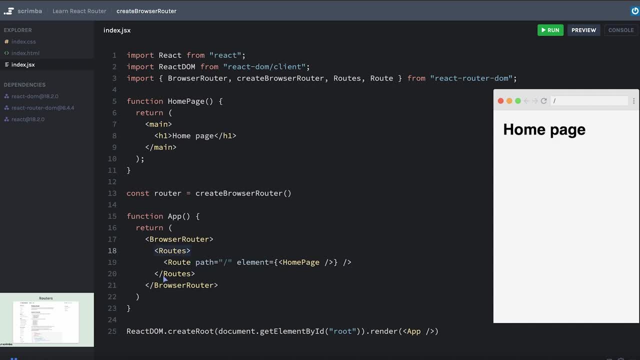 maybe more accurately, it's recursing through Because we have all of the children of this routes component in its turning every route and every child of those routes into an array of route objects and those might look something like this: Let's say we have an array, In this case we only have one route. So this: 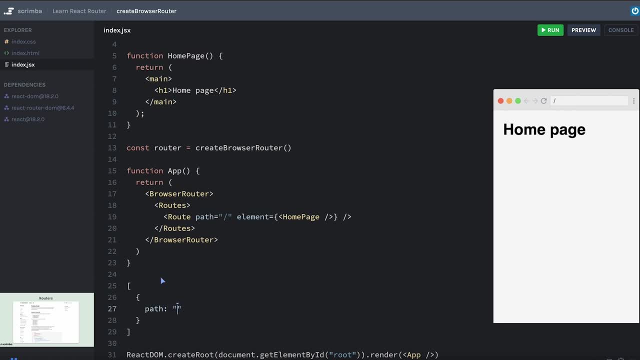 will be our route object and it's going to have a path which is just slash. that's going to have an element which is the homepage component that we have there And if this were to have any child routes, which we already did, your home page component will. 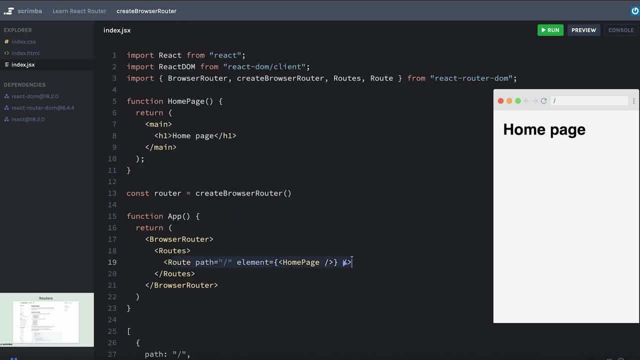 be the same travels that we've taken out of our ROOT component And it's going to be an array that we've thought about and that we'll any child routes, which it doesn't currently because it's just self-closing, But if it did, 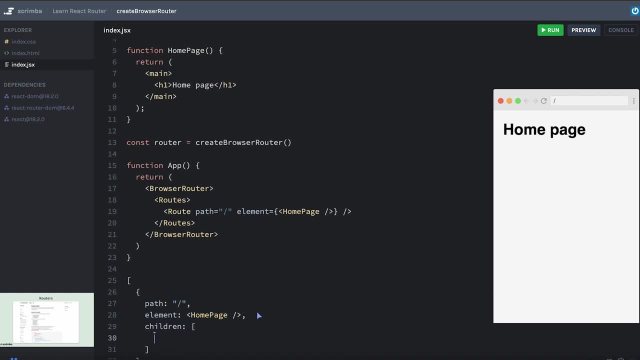 then there might be a property called children and that would be another array of nested objects and so forth. So this routes component behind the scenes in the source code of React Router. that's all it's doing with our routes here is it's turning them into an array of objects with. 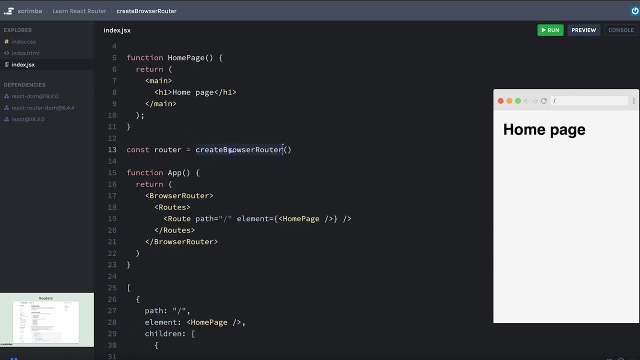 nested arrays of objects and so forth. So with Create Browser Router we could go down the path of basically rewriting all of our routes. In this case there's only one, but obviously in the van life app there's a lot more. We could go through the process of converting all of those. 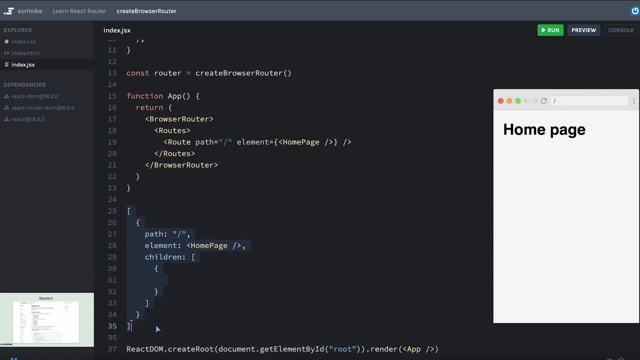 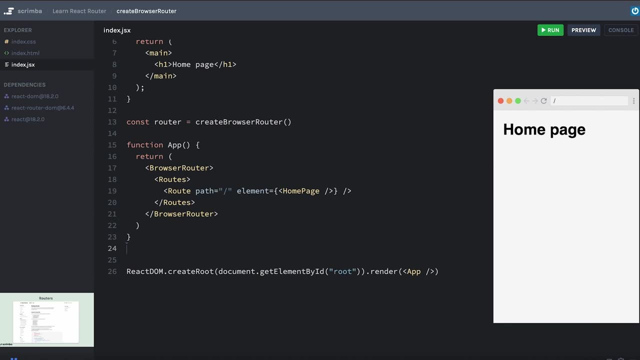 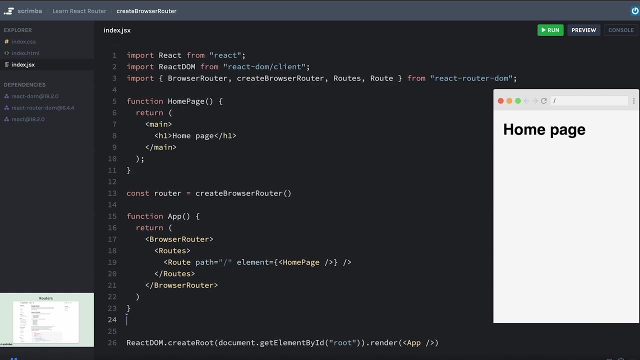 manually into an array of objects like this. However, in order to make things a little bit simpler for updating our code from a version prior to 6.4 up to version 6.4 and making use of the data layer APIs, they also included a utility function called create routes from elements. 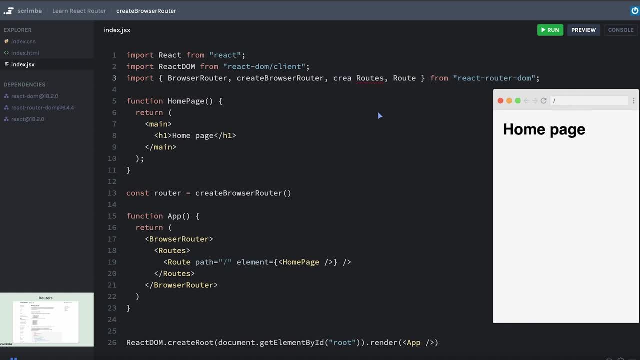 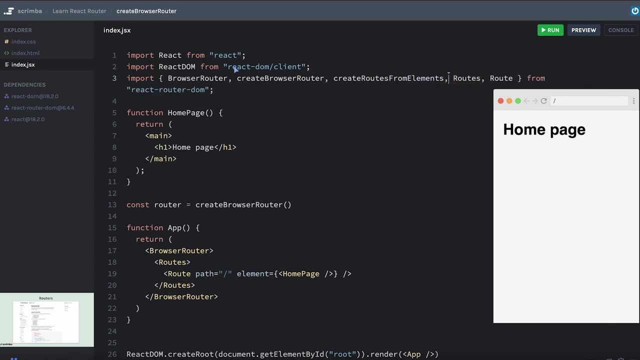 So I'm also going to import that, just to make my life a little bit easier, since I already have my routes defined. So we'll say: create routes from elements. And this is getting a little crazy. I'm going to put each of these on their own. 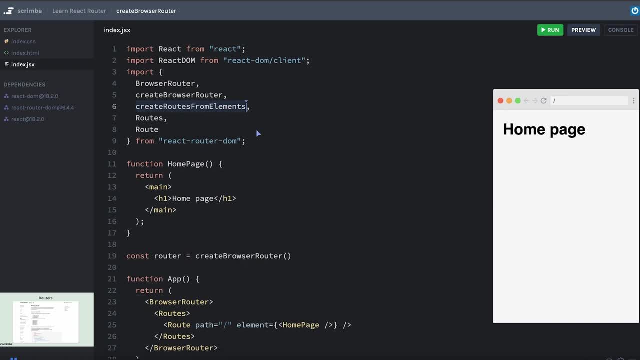 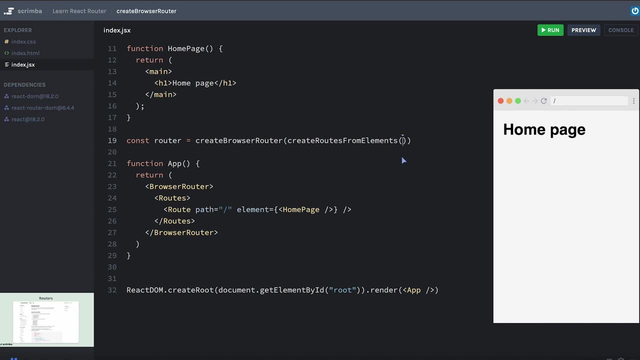 lines. Okay, so what we can do is, when we call create browser router, we will inside of there also call create routes from elements, And this way I can put my route elements directly inside of the create routes from elements. Basically, this function will turn my route component into. 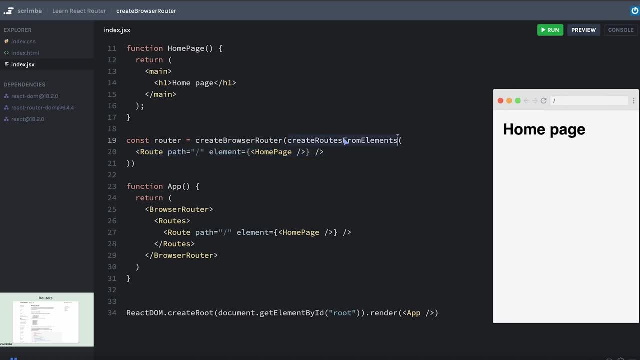 an array of objects and it will pass that object to create browser router. So basically, it does all of that manual work for me. To be totally honest, if I were creating this from scratch without some existing routes already defined, I'm not 100% sure which way I would use. I'm so used to using components. 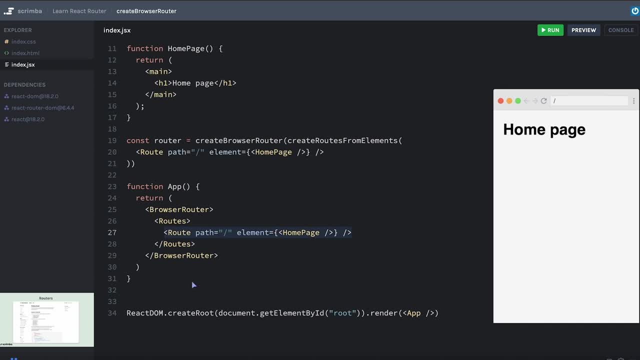 like this, that I might just turn to that, naturally, instead of typing out an object or an array of objects and whatnot. But I don't know, maybe the standard way will be just writing out objects. Either way, this should do the trick for us. there's one last piece that we need to do, And that: 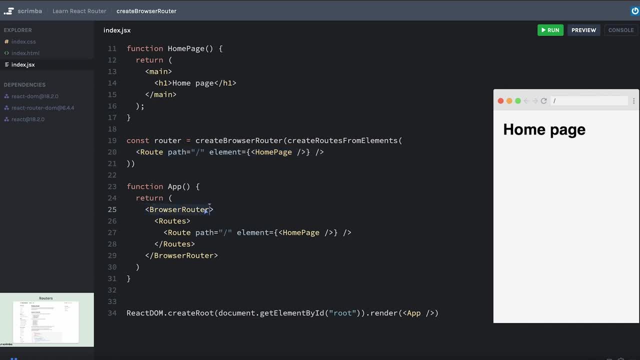 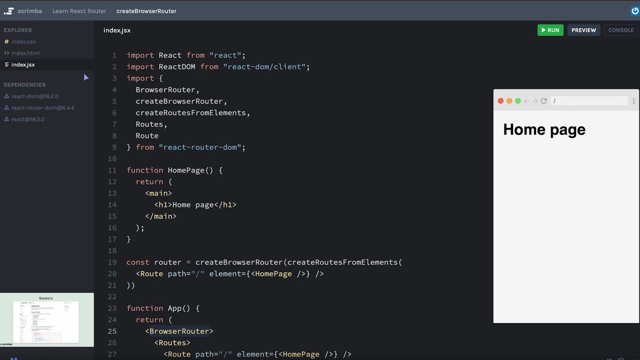 is to get rid of our browser router, Because browser router was specific to the non data layer API routers that we could choose from. we need to use something different. So there's yet another thing we're going to import. Actually, maybe I'll just replace browser router here And what I need. 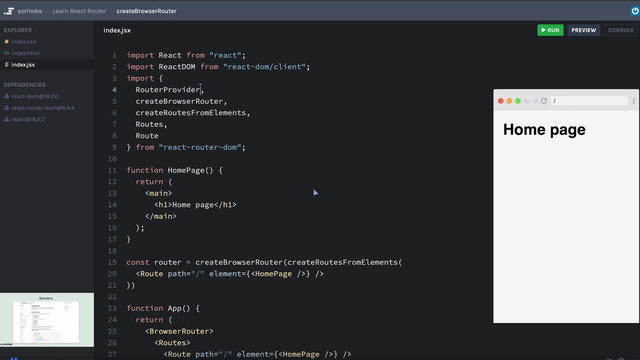 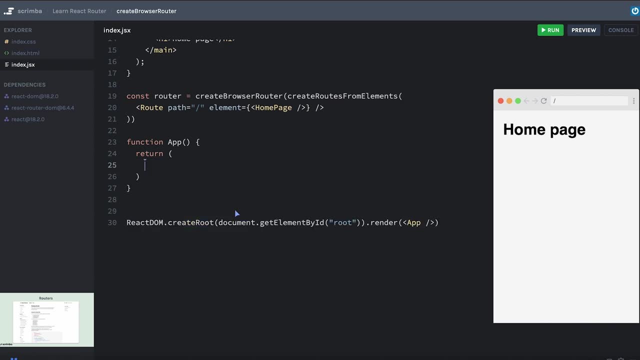 to bring in is something called router provider, And this is a component, so I can get rid of my browser router And I can actually get rid of- Well, actually, I can get rid of everything here. So we're going to create our new router And that's going to. 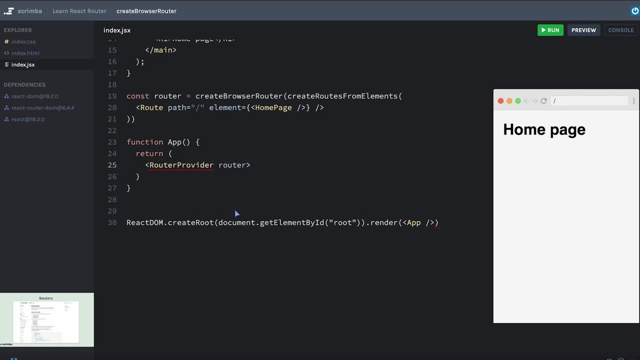 be by using the router provider, And then we're going to pass a prop called router and its value needs to be the browser router that gets created from create browser router. So I've said the word router too many times for it to make sense anymore. But router equals router. 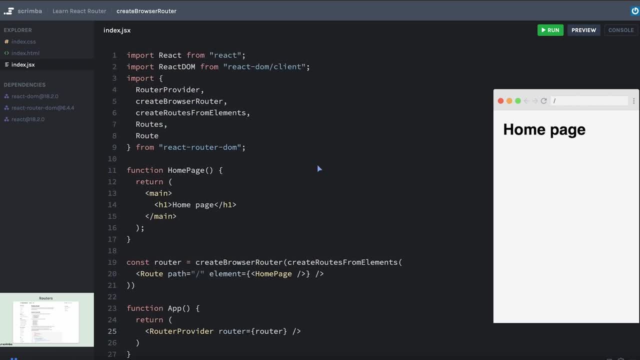 And then this can just be a self closing element And I guess let's cross our fingers, we'll hit save And okay, homepage is still working, And well, that's all we have to test. So I'm going to recap what we did, Because in the next lesson it will be a challenge to 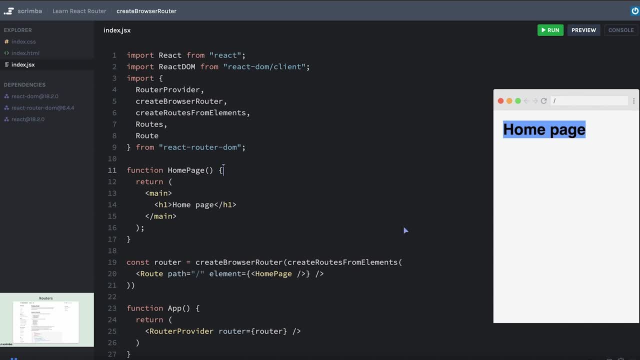 create the browser router, just like we did here, but for our van life app. So I have three new imports: router provider, create browser router and create routes from elements. actually don't need this routes import anymore because I'm not using routes. And then outside of the function. 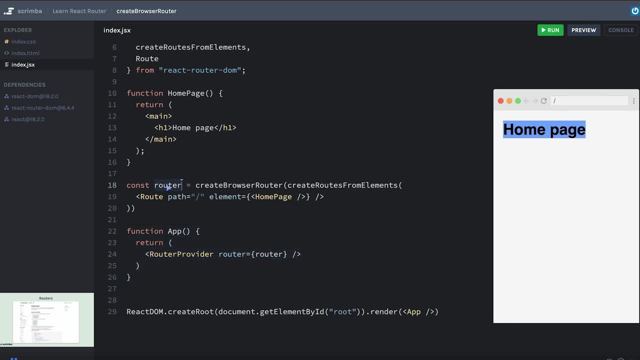 where I'm going to be using this router provider. I created a new variable called router. the name of this variable doesn't matter And I'm calling create browser router And because I already had a route defined as a component like this, I'm also using the router provider. I'm also 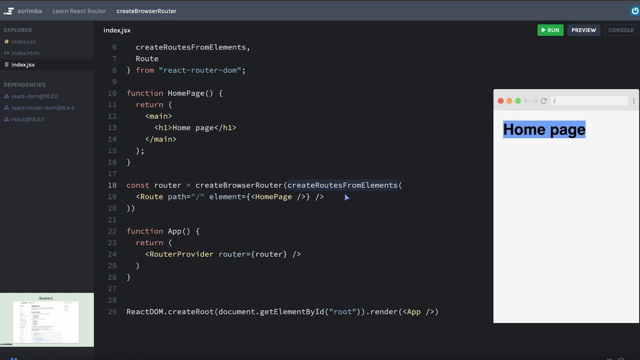 using create routes from elements. that allows me to just copy and paste my entire route definitions right here into the new create browser router function that I'm calling. Then, with this router variable defined, I'm going to use the router provider and pass that variable to the router prop in my router provider component. Okay, 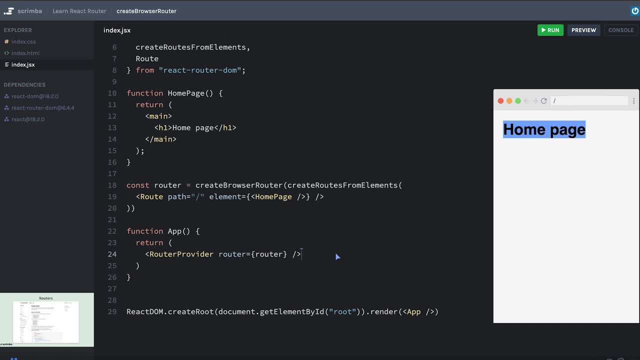 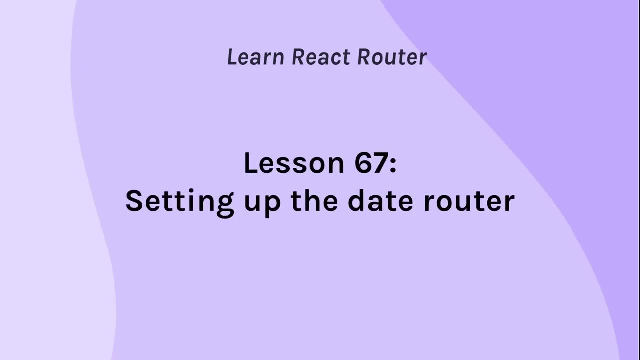 that's a lot to take in, especially not having typed anything in this lesson. So look through the code if you need to, And in the next lesson I'll have you work on it yourself. Okay, here we are, back in the comfort of our van life app. 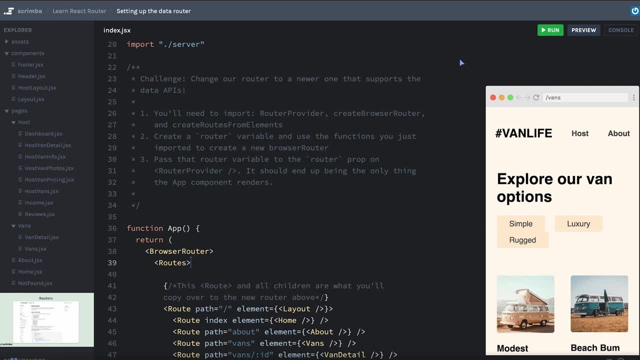 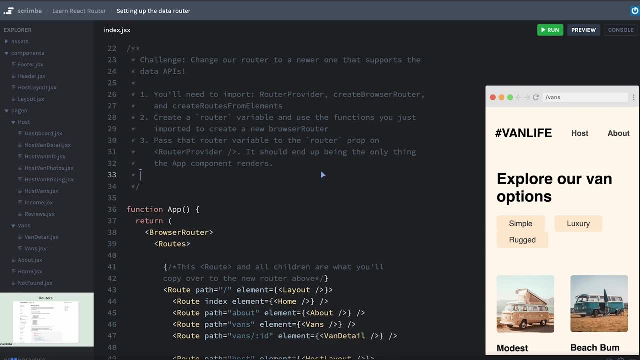 your challenge is to change our router so that we can use the newer one that supports the data API's. then we'll finally be prepared to start actually learning about the data API's and loaders. So you'll need to import these three things that we learned about in the last lesson. 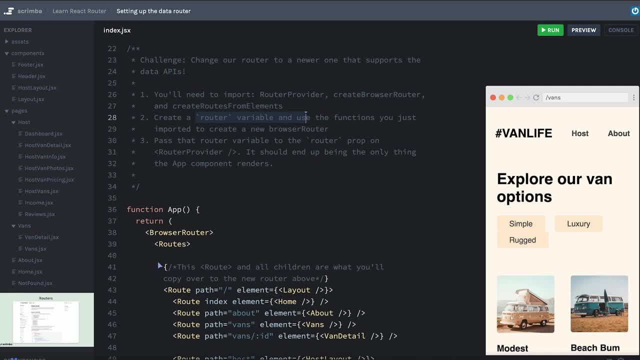 you'll need to create a router variable, And I put a little note here just because in our example, we only had a single route that didn't have any children. But in this case, you're just going to be copying and pasting all of the data that we learned about in the last lesson, So you'll need 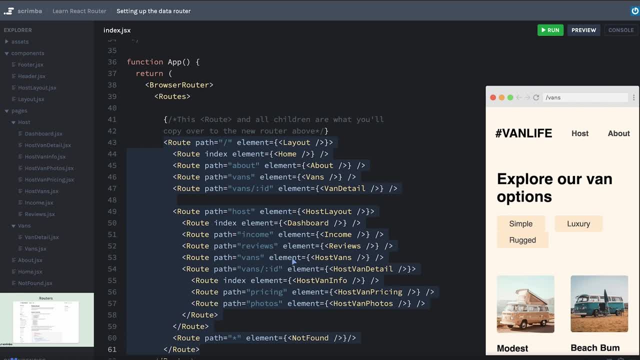 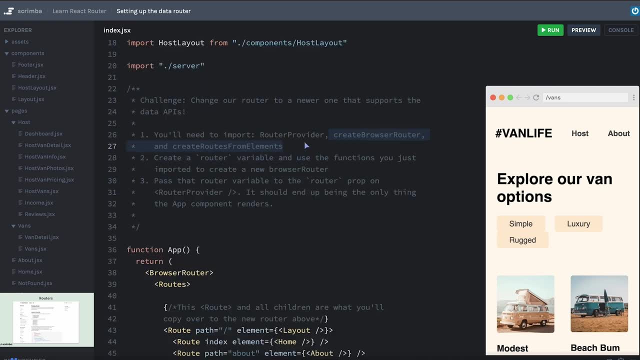 to import these three things that we learned about in the last lesson, you'll need to create a router variable over everything inside of our main route here and all of its children. So that will go in your router variable which makes use of these different functions that we are importing. 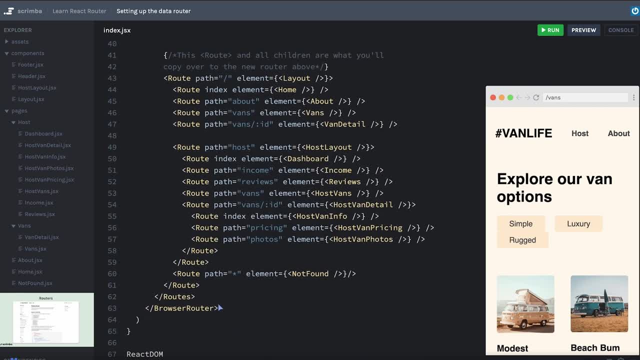 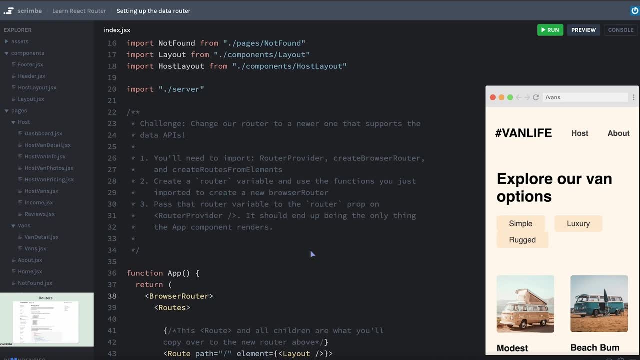 And then you will replace basically everything in our app all the way through- Yeah, everything- with the new router provider that we imported. I think you have plenty of hints here, So I'm not going to make it too easy on you. I want you to get your hands on the keyboard, of course. 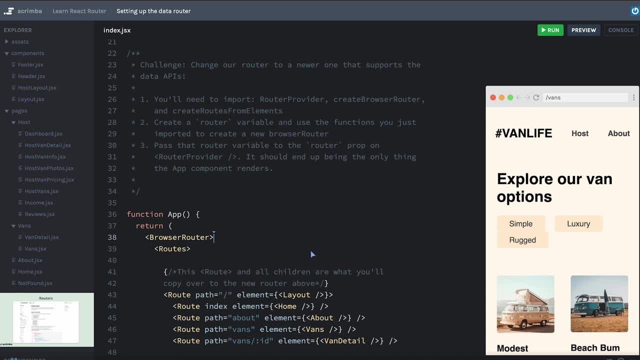 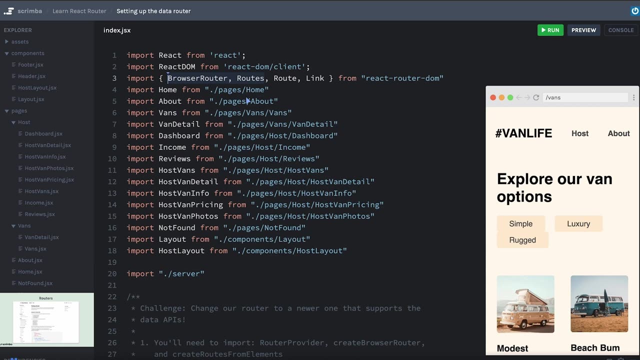 and practice everything you can practice. So pause now and work on this challenge. Okay, I am going to cheat and just copy these things. we'll import those. let's see there's a couple things we can get rid of. let's get rid of our browser router and routes: it will import. 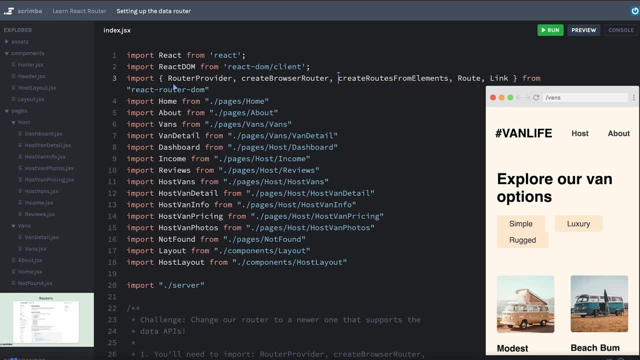 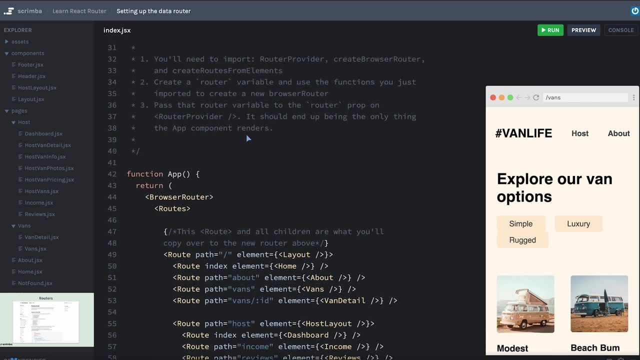 those and then kind of clean up my language here. And while we're at it, I'll go ahead and put these on their own lines, since we are running out of space. Okay, that looks better. Now let's create a variable here. 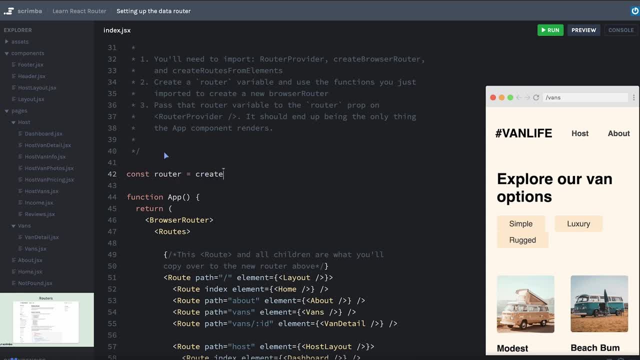 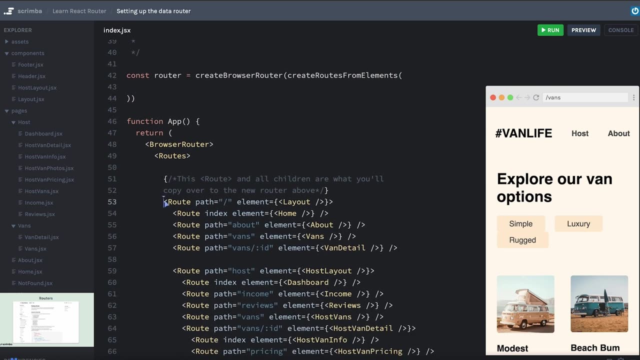 We'll call it router And we will call create browser router, And then- so we don't have to manually go through and change all of these routes into an array of objects- we're going to call create routes from elements, And then I can just take my main route here, And I'm actually 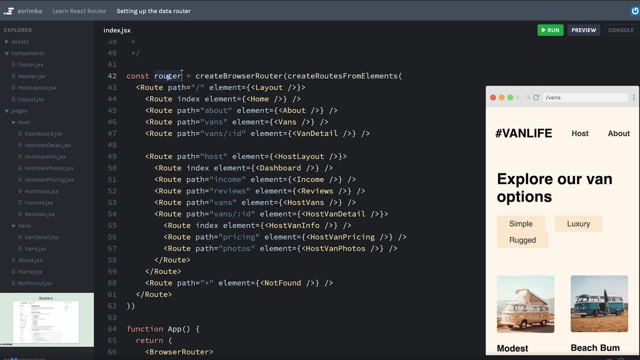 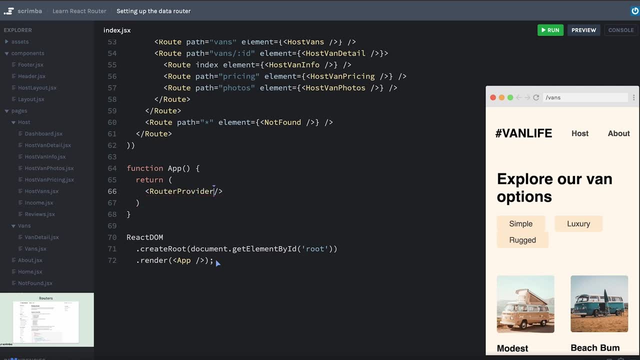 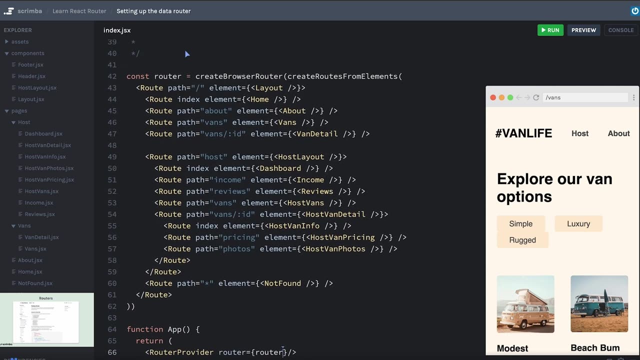 just going to slide it up. that creates our router, And then I can replace our browser router with the router Provider. that will take a router prop and its value will be the router that we created above. Let's double check. I'll clean up the challenge text And let's give it a shot. I'll hit save. 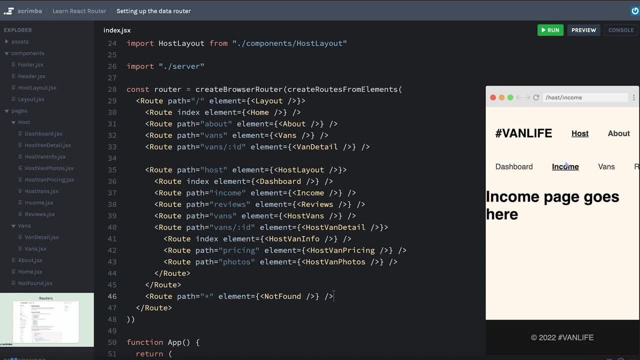 And, sure enough, everything seems like it's working. Let's kind of navigate around our app a little bit And perfect. So again, we didn't change anything. that will be visibly different on our page, But fortunately we now can find a router that we created, So let's go ahead and create a. 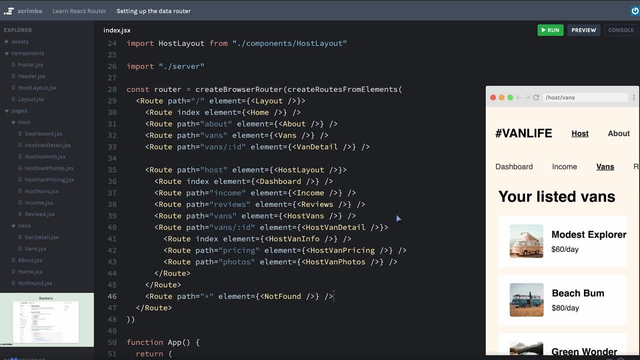 router And finally jump into learning about loaders, which is what all of this has been a build up toward, As always. if you want to practice doing this again, just to see the two different methods of creating routers, you can scroll back to the beginning of the lesson and try it out. 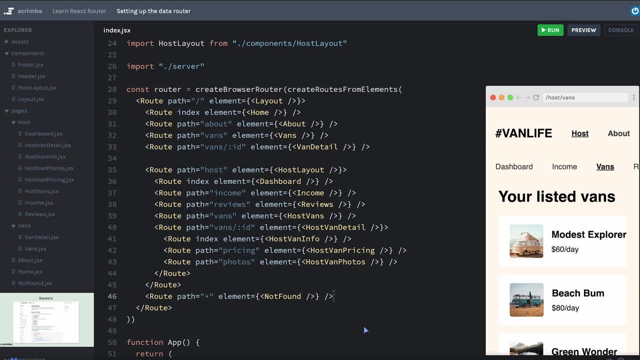 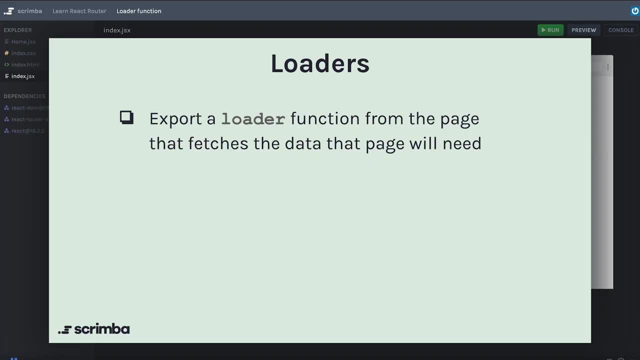 again from scratch. Then, as always, when you're ready, we will keep moving forward. Okay, we're going to approach loaders just one step at a time. The first thing we need to do is go to the page that normally would use a use effect to get data as soon as that page is loaded. 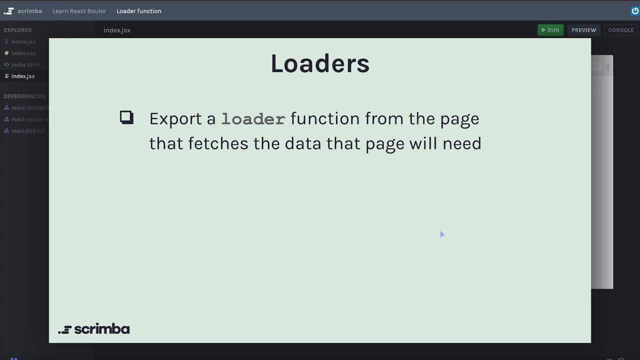 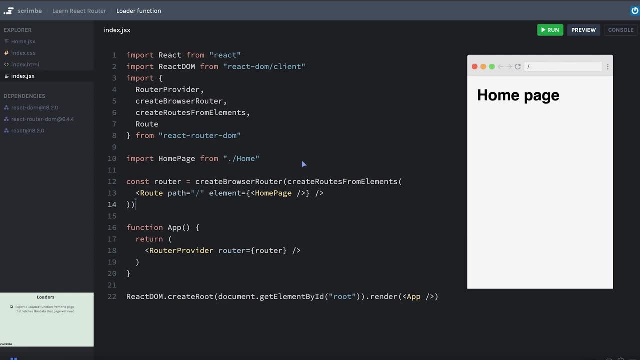 And what we'll do instead is export a separate loader function instead from that page that will fetch the data that we need for that page. So I tried to make this as simple as I could. I did move the home page from our previous example to a separate component just so we could get this even. 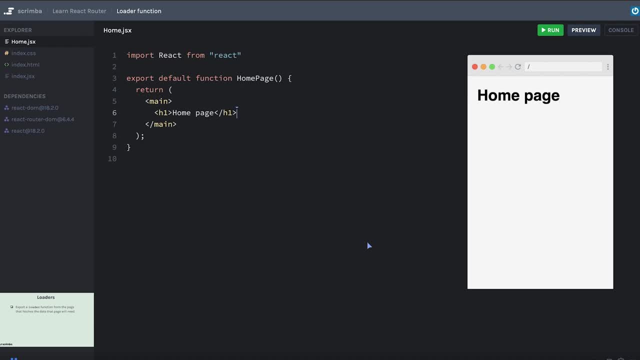 a little bit closer to what we have in the van life app. So here I have my homepage And, let's say, I'm going to be getting some really basic data outside of the component that I have defined. I'm going to create a function called loader And I'm going to create a function called loader, And 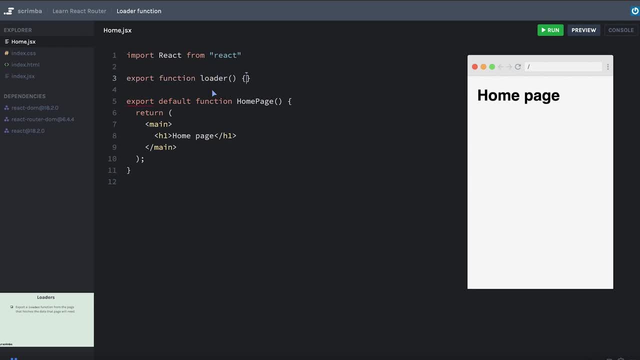 I'm going to create a function that I export, called loader. Now, with react router, the name of the function actually doesn't matter- A fun fact in remix it does matter. it has to be called loader. But since we're not using remix, we're using react router, we can really call it whatever. 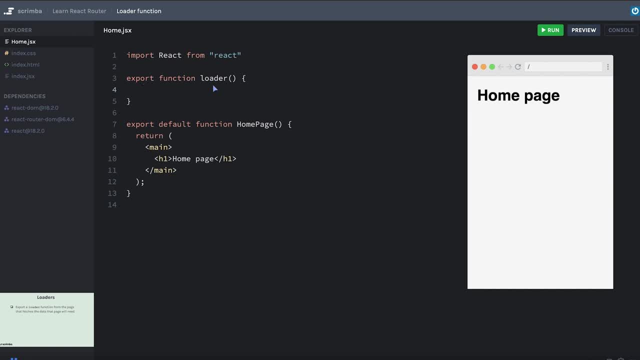 we want, And the job of this function is to get the data that we want to get. Now, to make things even simpler to understand, the truth is, it doesn't really have to be a fetch request per se. I think it almost always would be, But to keep it as simple as possible, I'm just going to return. 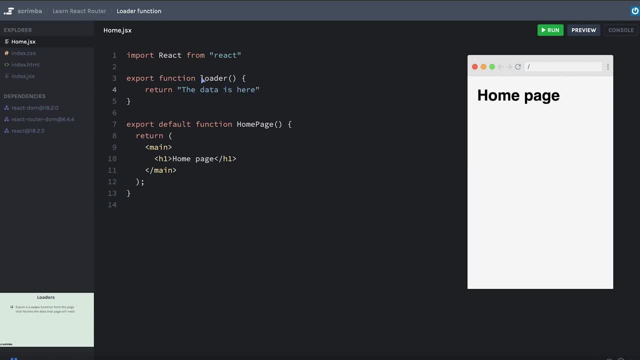 a string that says the data is here. we'll see when this comes full circle and how we actually get the data from our loader into our component in a couple lessons from now. Okay, so it's really as simple as that. we export a function whose job is to get the data that we want to have access to in. 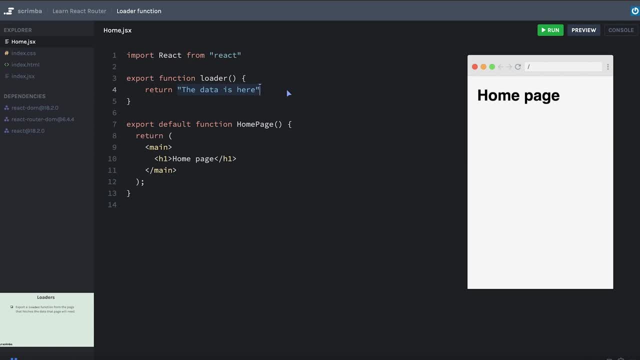 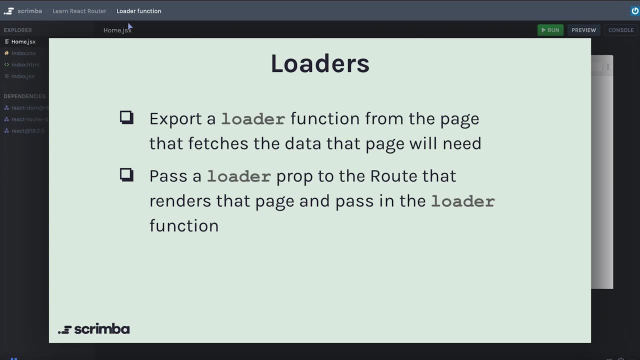 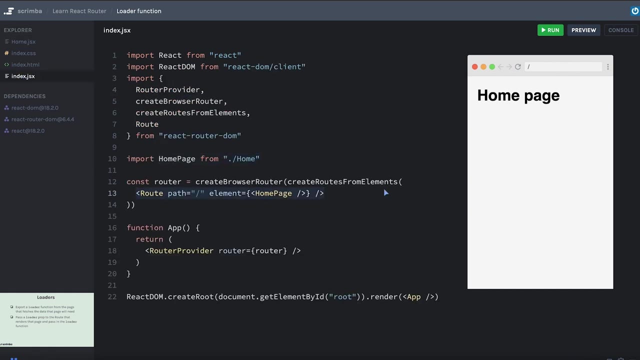 our component. For now we're pretending that the string is the data that we have fetched from some API. Next, we're going to pass a loader prop to the route that renders this page, the homepage, our loader function. So let's go over to index. In our case, we only have one route, that we're. 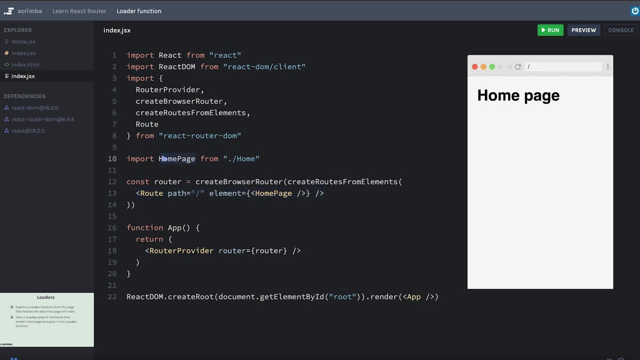 defining And notice that I'm importing homepage as a default import from my home component. I can also bring in my loader function that I exported as a named import or a named export over there, And all I need to do now is to add a new prop to my route that's called loader. 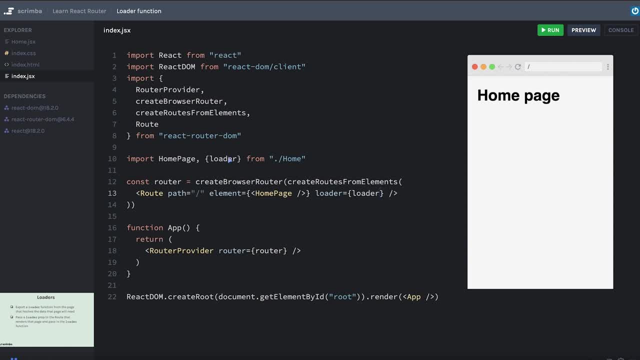 and I will pass in the loader that I imported with my homepage. Now think in the van life app how we have multiple page imports, many of which will have their own loaders. So I'm not going to be able to just import a named function called loader for every single. 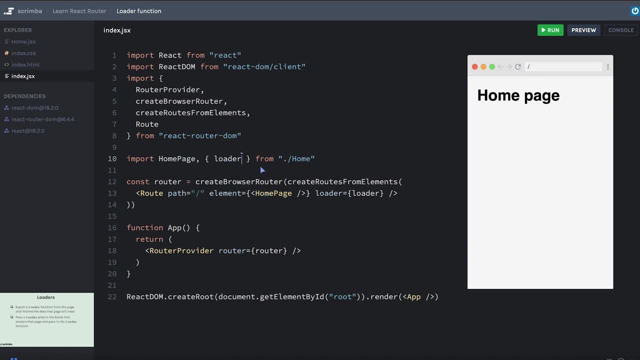 one of them. In our case it's fine because it's our only one. But a really common practice is to rename it as you're importing it. So I might say import loader as and then maybe say like, homepage loader, and this should probably be lowercase, And then I would change. 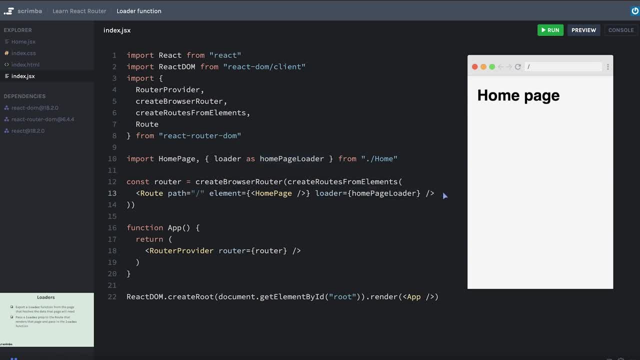 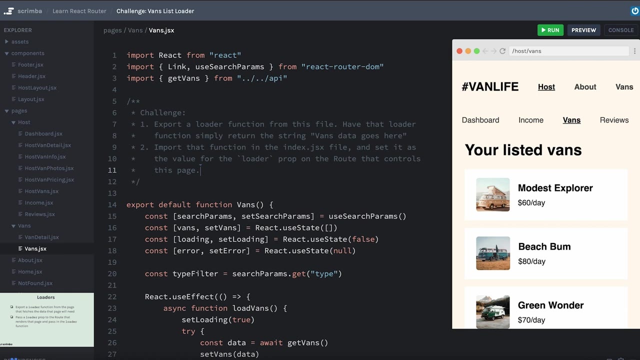 loader equals loader to loader equals homepage loader. That's a great start. It's not quite done yet, But let's go back to the van life app and give you a challenge so that you can accomplish those steps for the vans page. Okay, you're basically going to do the same thing that we just did, But here on our van life app. 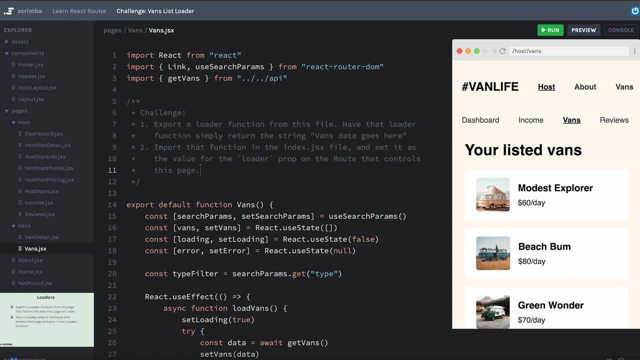 it's not going to be exactly what we ultimately want, But we're going to iteratively get there. So your challenge is first to export a loader function from the file that we're currently looking at. For now, we'll just have that loader function return. the string vans data goes here, or 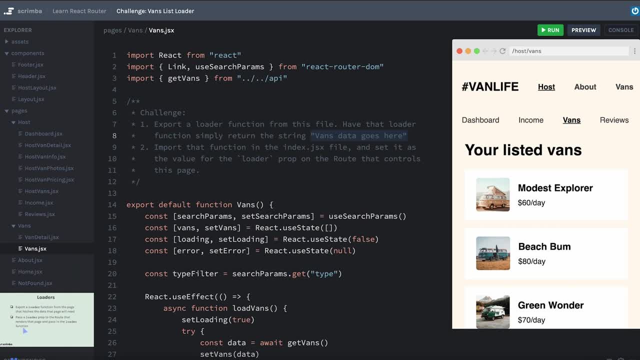 something along those lines. then, over in our index JSX file, we need to import that function and we will set it as the value for the loader prop on the route that controls this vans page. pause now and work on the challenge. Okay, let's export a function that we'll call loader. 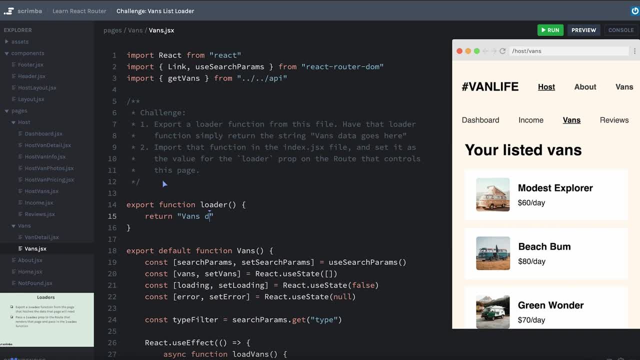 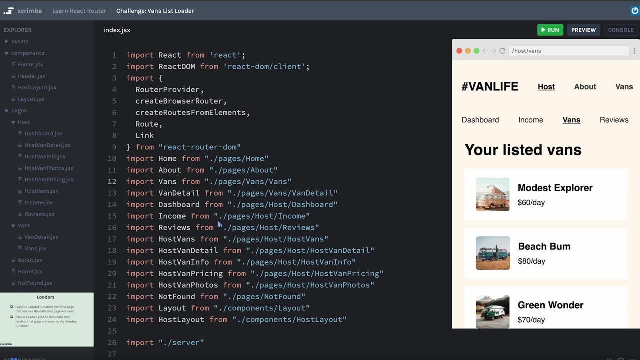 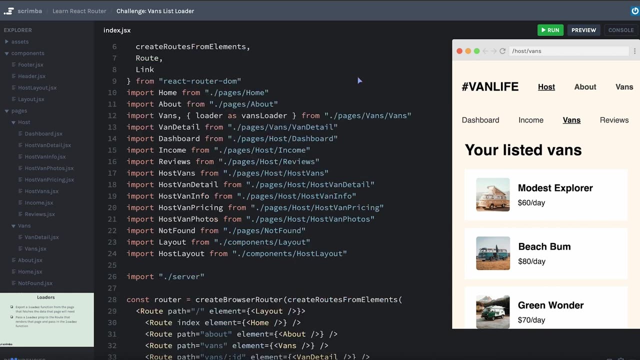 And it's just going to return the string vans data goes here And then over on index JSX. we will import it. Now that file was right here with the van, So we will bring in the named import loader. Let's call it vans loader. Okay, and down on our vans page. 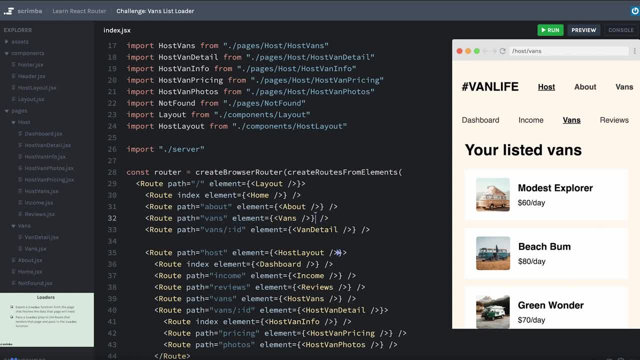 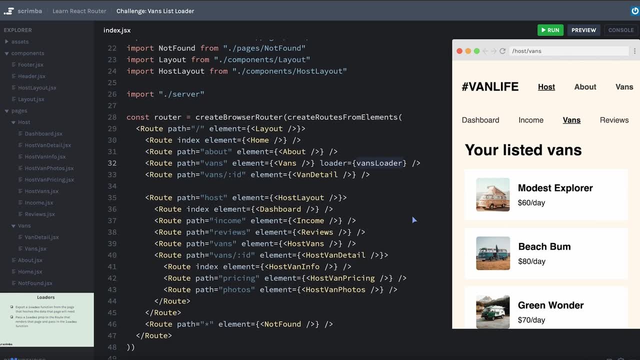 which is, let's see, slash vans. we are going to add our prop called loader and set the value equal to vans loader. Okay, that's everything we are equipped to do right now. Let's go back and complete the circle so that we can actually 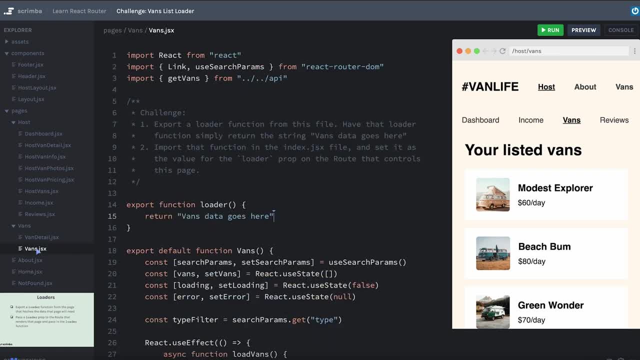 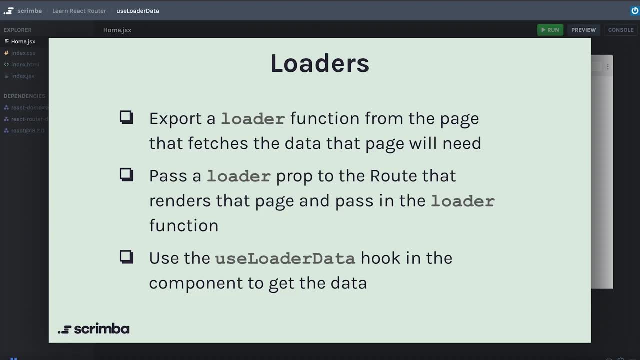 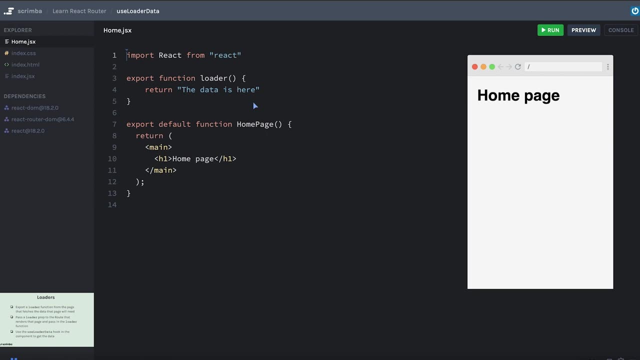 pull in the data from our loader into the component where we're trying to get it. The last thing we need to do in order to get this loader actually working is to use the use loader data hook inside of our component, And up until now it may not have been totally clear what 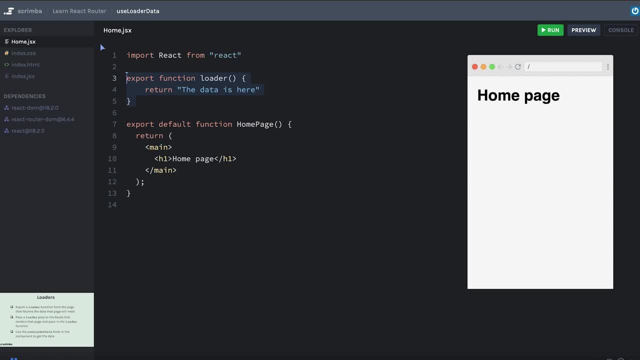 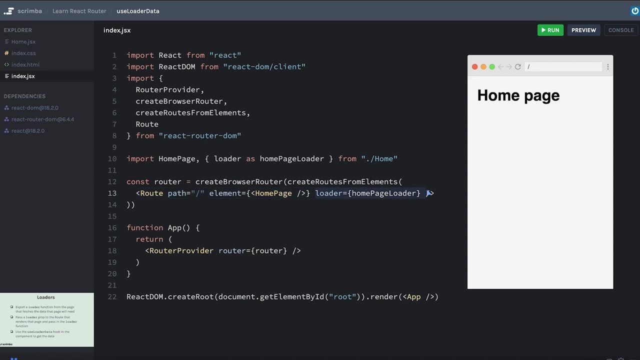 direction we're heading in, because we have this random function that's inside of our component file And then over here we're importing it, setting it up as the loader. this seems a little bit out of place, But because we've done that little extra work, what's really nice about this is inside of our 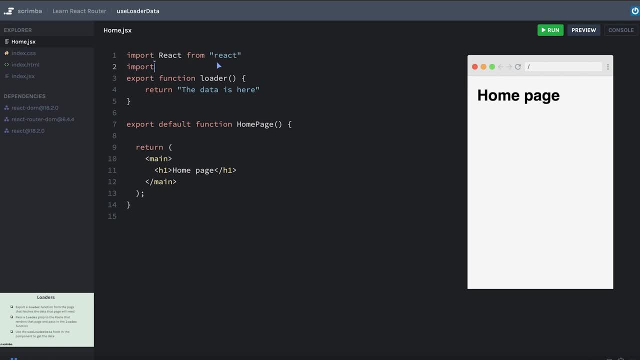 component. we can use a hook called Use loader data. So I need to import that from React router Dom, loader data from React router dumb And I can use that hook to grab the data that is being returned for my loader. So I can say use loader data. 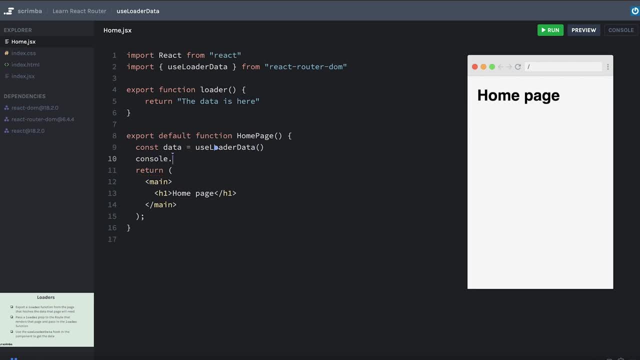 And I want you to pause and just think for a second. what do you think console logging data is going to show you? Okay, so here we've hit the Add button, we're gonna say appropriate, but then like show first, think about it and then actually try to run it and see if what you thought is what. 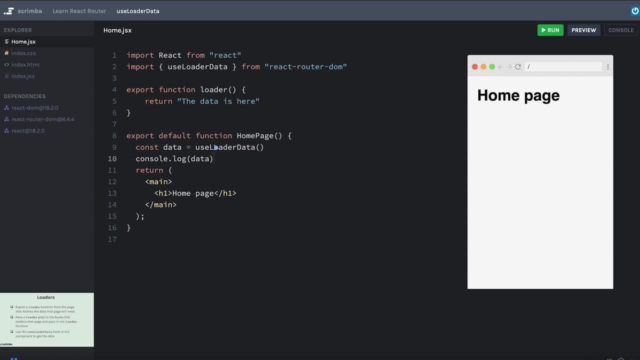 actually happens. well, let's hit save and we get the string. the data is here. so hopefully that makes sense, because whatever we are returning from our loader is exactly what will come back when we call use loader data. so how is this different from using a regular use effect? 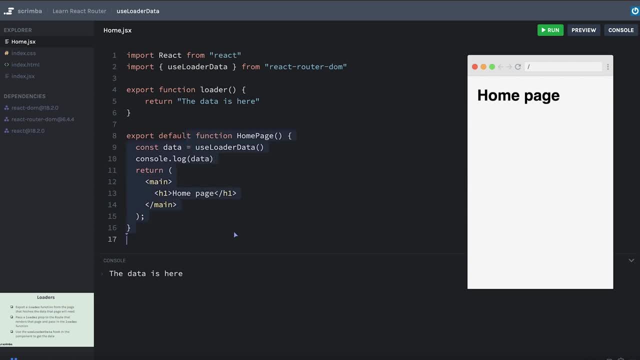 well, because we are not doing our data fetching inside of the code of our component, react router can delay the rendering of our home page component until the loader has finished its task. so it's a slight change in the paradigm of how things get loaded. in fact, if you look at the documentation, 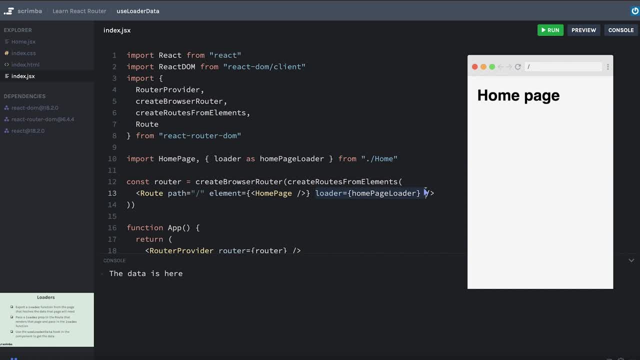 react router specifically says: we don't care how you fetch the data. the only thing we are doing with our data apis is changing when the data gets fetched. so how is that useful? well, we're going to apply what we've learned to the van life app, and then we're going to start. 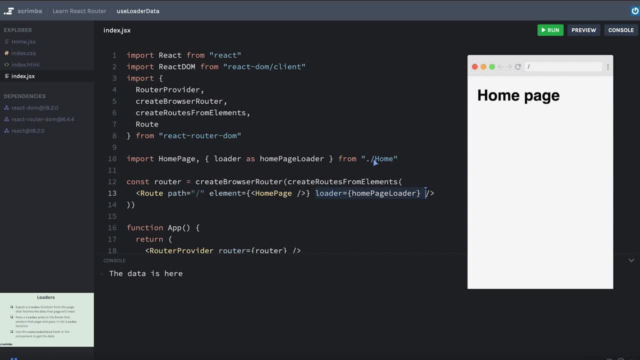 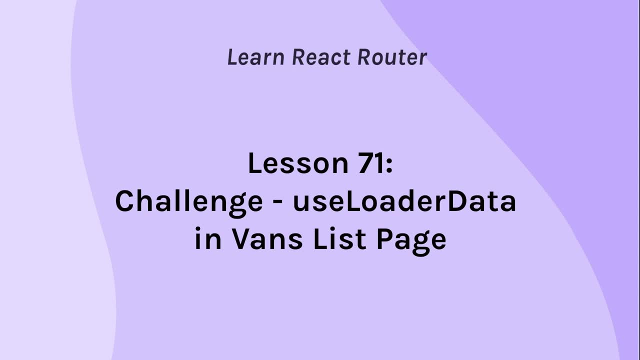 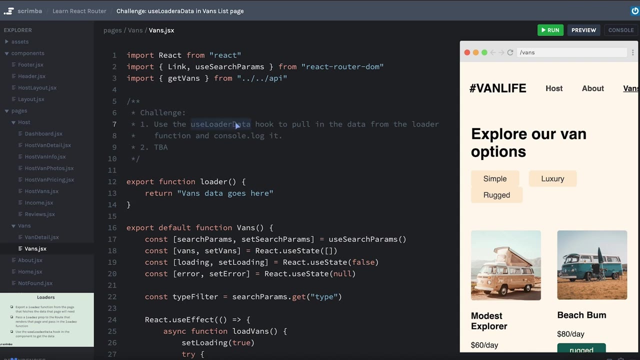 making some major changes to our code, which hopefully will highlight how beneficial it can be to use these data apis. so let's do that next. all right, so let's do exactly what we just did. your challenge is to use the use loader data hook to pull in the data from our loader function. 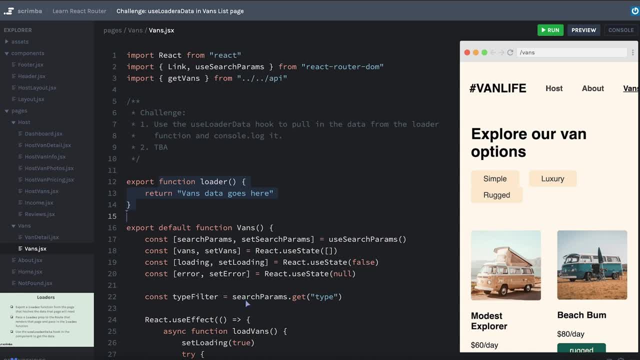 and then i'll just have you console log it inside of your component. here, of course, it's not actually data yet we are eventually going to use the get vans function, which really gets data, and use that inside of our loader. for now we'll stick with what's here. so pause now and work on this challenge. 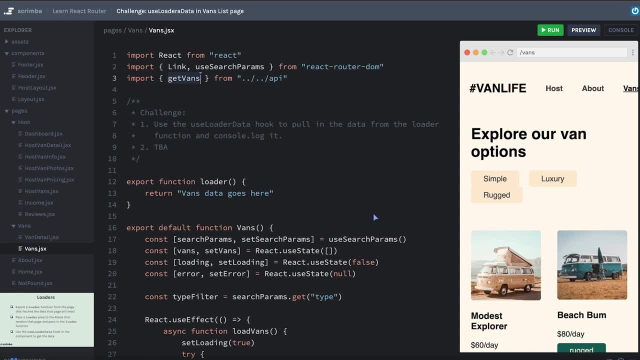 okay, let's pull in the use loader data hook and we will. now let's do it down here. we'll say const data equals use loader data, and then we will console log the data and if everything is connected upright, then it should give us the vans. data goes here. 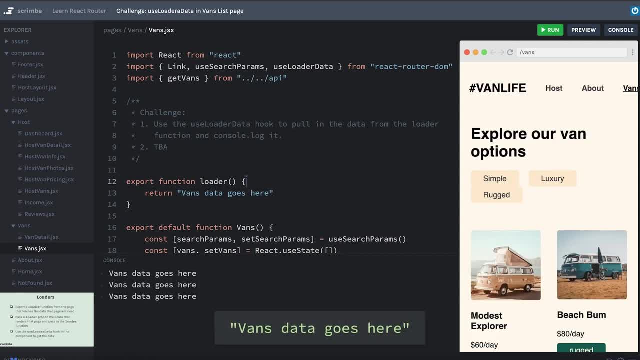 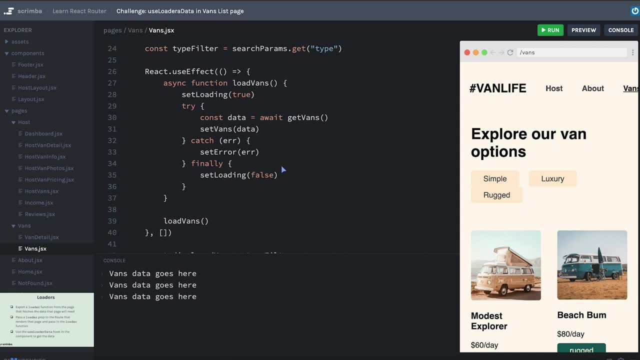 string. let's open the console. hit save. okay, vans data goes here. now notice that it logged it three times. that's actually because we have this use effect. it ran when the code first loaded and then it set the van state, and so it had to reload the page again, and i'm not exactly sure why. the third: 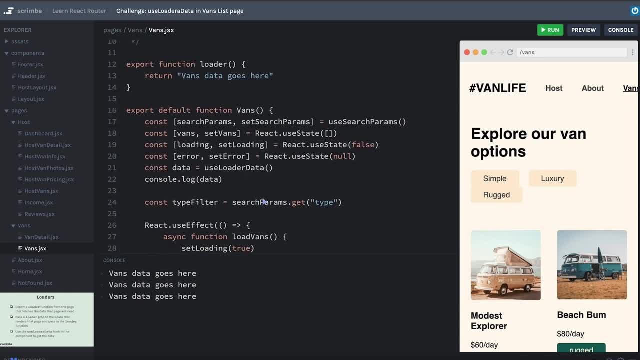 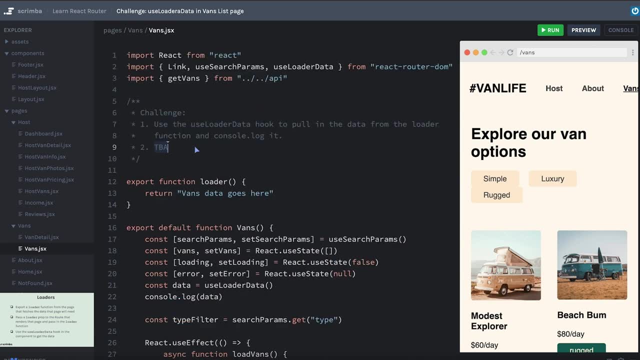 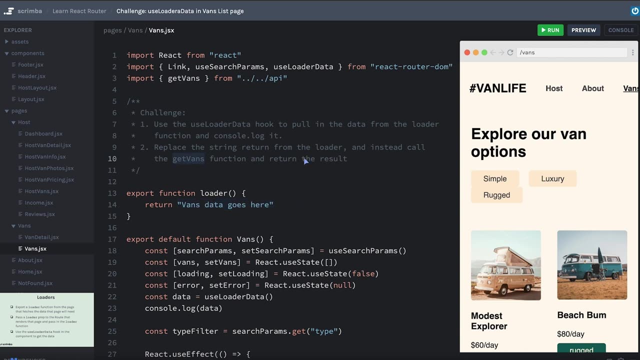 one is happening. oh, because of set loading, probably. so we're actually going to address what's going on here, but for now let's do part two, which i'll type out right now. so, here in our loader, instead of returning a string, i want you to place a call to the get vans function and return what gets returned from get vans. 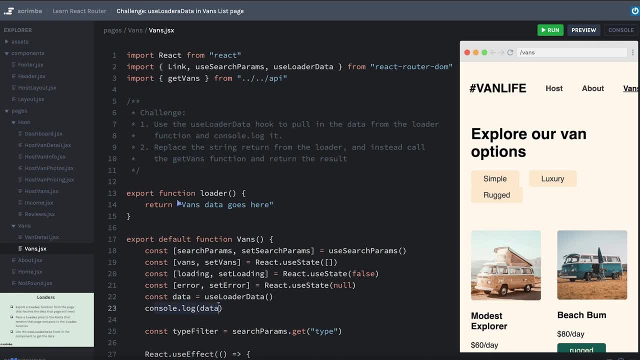 we're still pulling in the data and console logging it. so really, the only change should be what happens right here. pause now and work on part two of the challenge. okay, simply enough, instead of returning this string, we're going to place our loader and we're going to return the data and console logging it. so really, the only change. 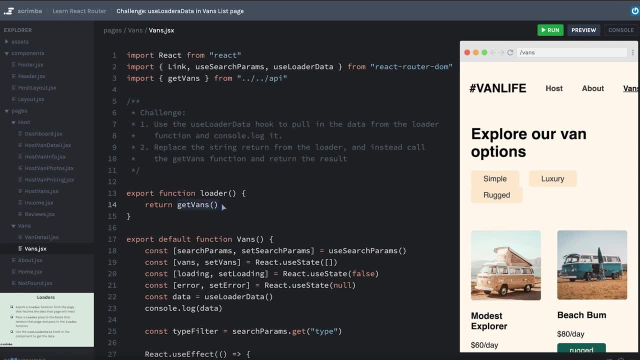 should be what happens right here. pause now and work on part two of the challenge. so really the only change: call to get vans, which should return our list of vans, and then from our loader we're going to return that list of vans that came back from this function call. everything else is still hooked up. 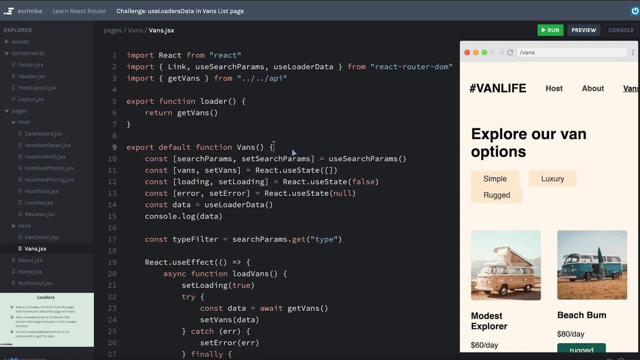 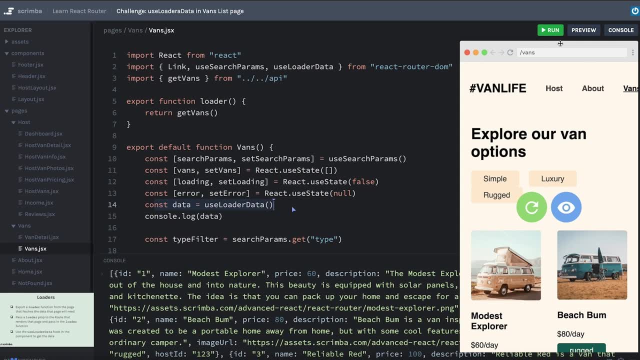 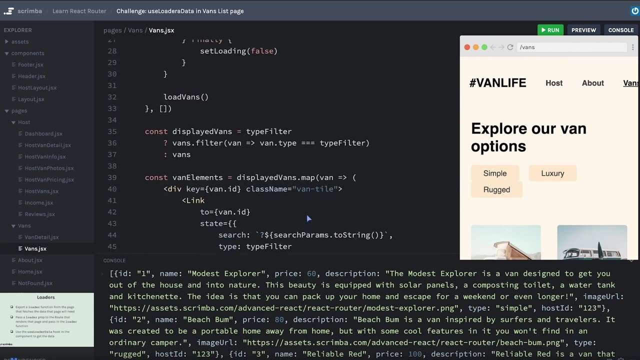 here. so let me buy us some space here. we'll get rid of that. we'll hit save. check the console. awesome, look at this. we have all of our vans which came through in the use loader data. now, currently we are only pulling it in and then logging it. we're not actually rendering that anywhere on. 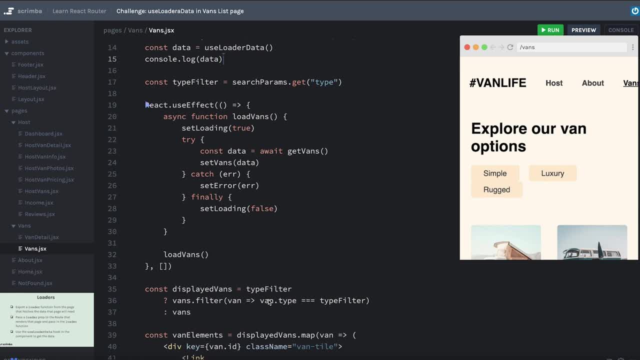 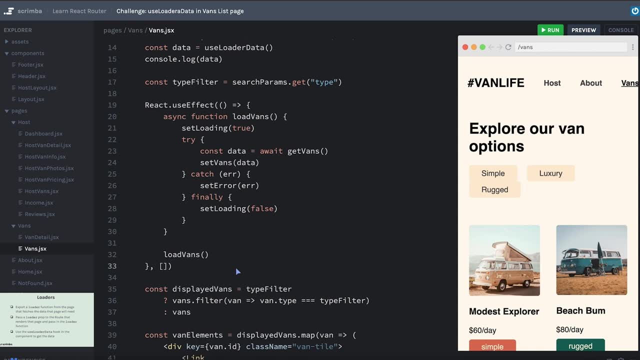 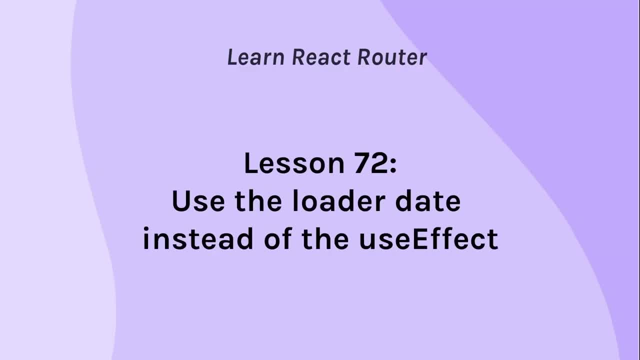 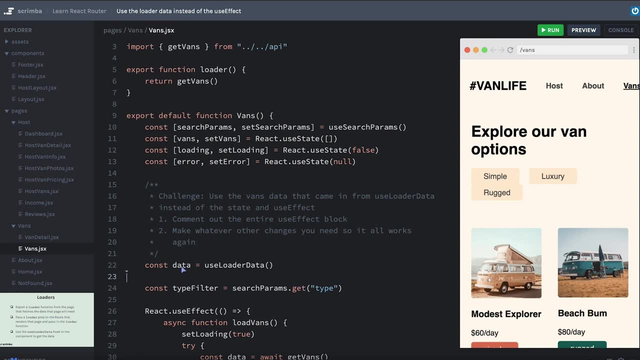 deletions in the next scrim. okay, so instead of just console logging the data, i actually removed that console log. we want to use this data in the component, so your challenge is to make use of the data here throughout the component, instead of using our state and our use effect. 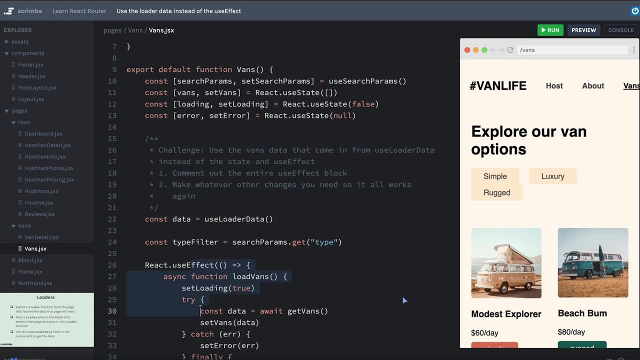 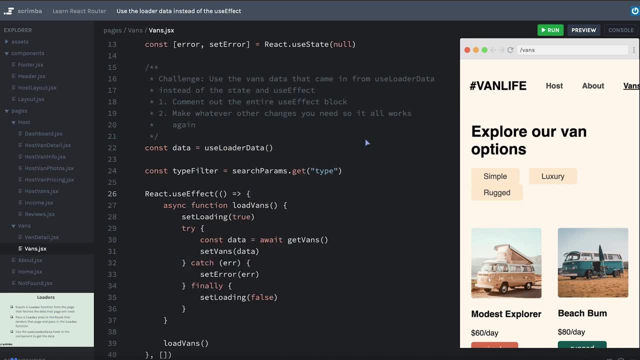 to fetch and to hold the array of vans. the first thing you'll need to make sure that you do is just to comment out this entire use effect block, and then you'll need to figure out what other changes you need to make so that things start working again. as a hint, i personally would make a change. 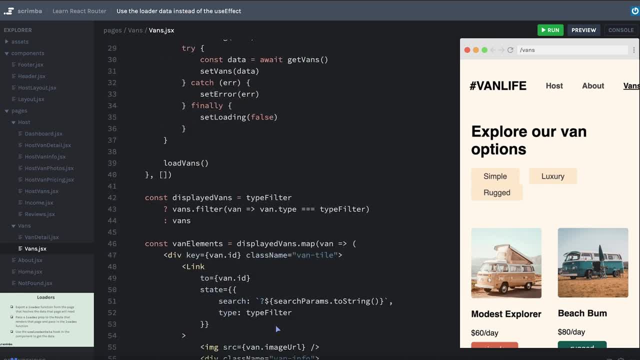 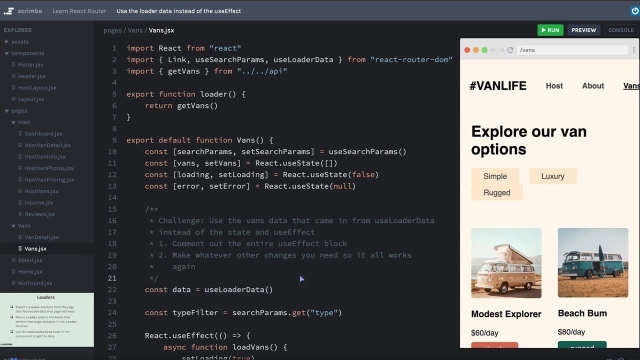 up here near the top instead of going through and changing a bunch of different things down here below. hopefully that's not too cryptic. i'm sure you'll be able to figure it out. i'm trying to be vague so that you have to really think about it. pause now and work on the challenge. 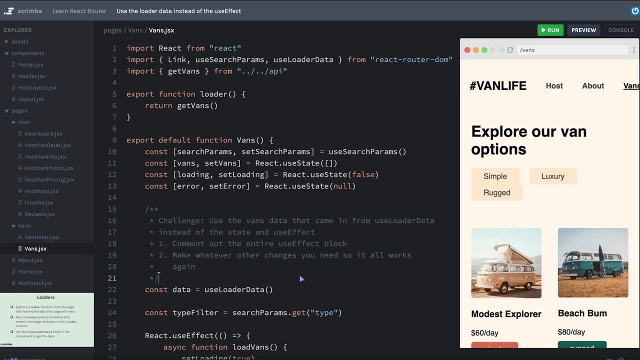 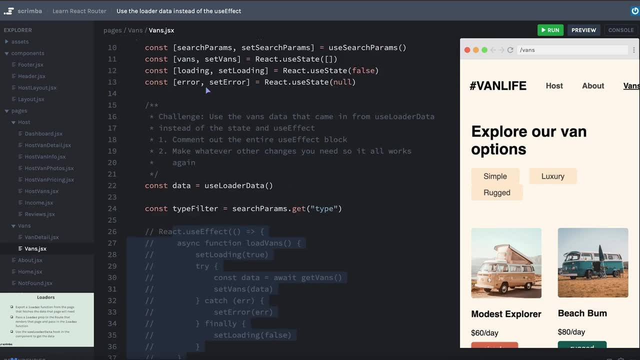 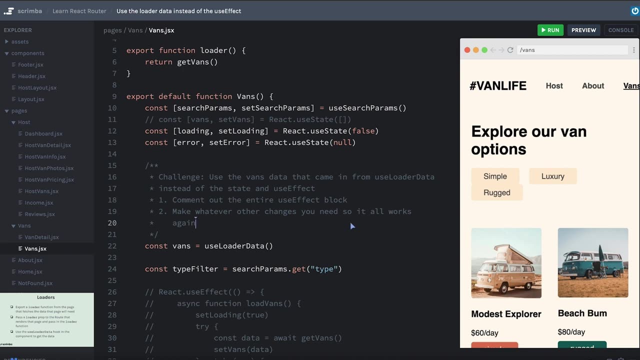 okay, let's comment out this use effect to start, and then, instead of going down and changing wherever it says vans to data, i'm actually just going to change here to vans and then comment out my use state. so let's hit save and, sure enough, everything is working, we can go into the vans. 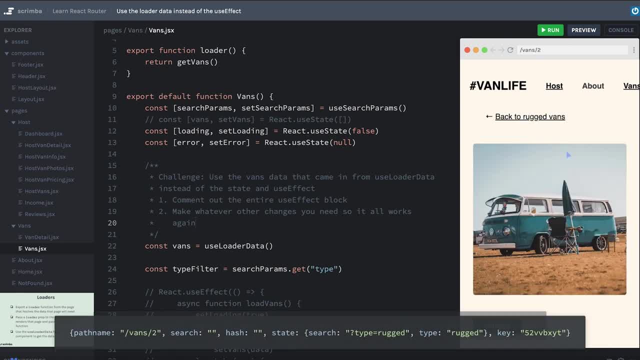 we can set filters and go there. this is still working awesome. now, if you did have a chance to play around with the vans, you can go into the vans and you can set filters and go there. this is still working awesome now, if you did have a chance to play around with. 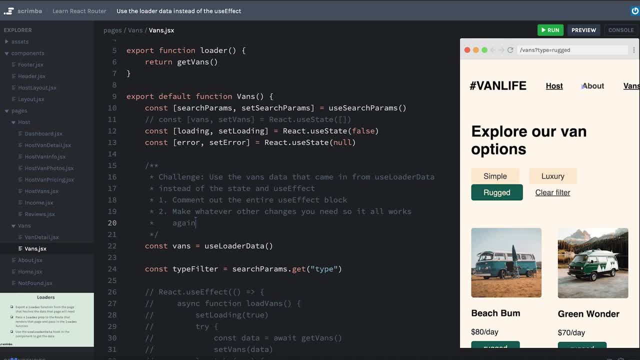 this a little bit. you might have noticed something, and that's if i go back, say, to the host page or the home page, then i come back to vans. i'm going to click it right now. you'll see that there was a slight delay before our vans actually got loaded. remember react router? here is 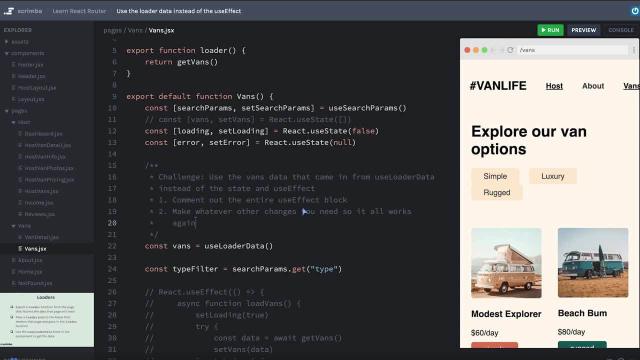 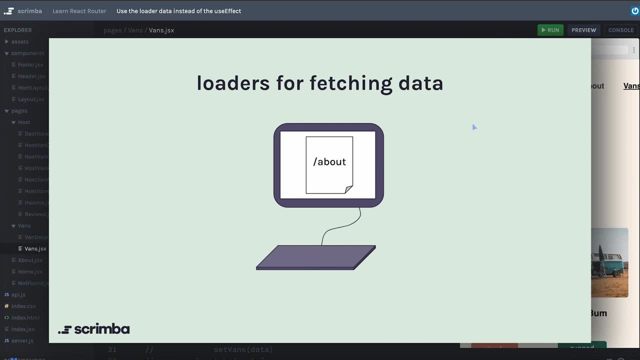 making changes not to how the fetch occurs but to when the fetch occurs, like we saw in the slides. say, we're at the about page or some other page. as soon as we click to the vans page it's going to start the fetch request then and all of a sudden it's going. 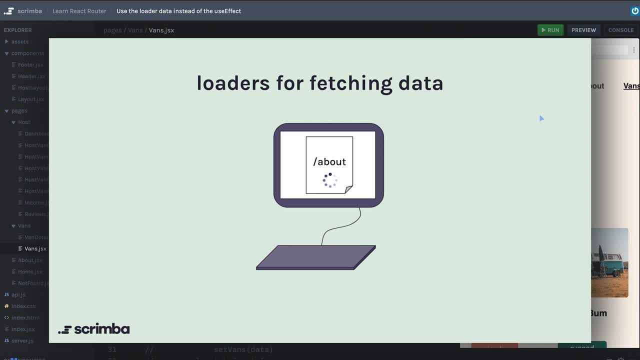 and only after the fetch request has completed and the loader has gotten the data, then it will transfer us to the vans page and it will include, as part of the use loader data hook, the json or whatever data it is that we pulled in from our loader function. so what does this mean for us? 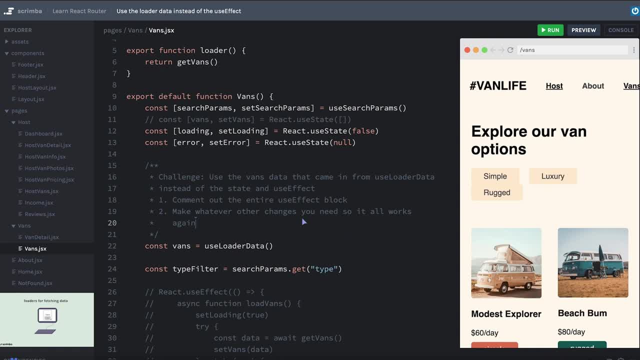 well, that means that we get to do one of the most cathartic things that i think you'll ever do as a programmer, and that is to delete a bunch of code. for example, we no longer need our loading state because we are already here in the vans page and we don't need our loading state because we are. 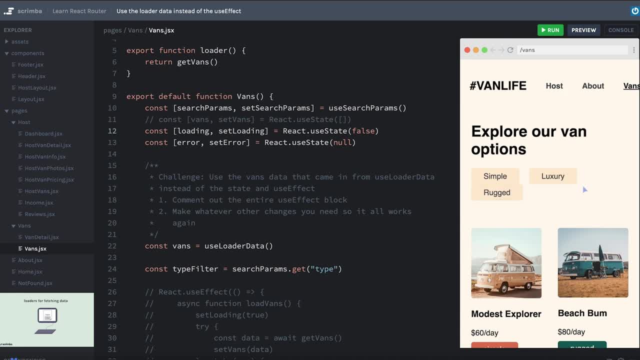 already here in the vans page and we don't need our loading state because we are already here in the vans page. and we don't need our loading state because we are already here at the page and the data has already come into that page. so i can just get rid of my loading state, which means i can. 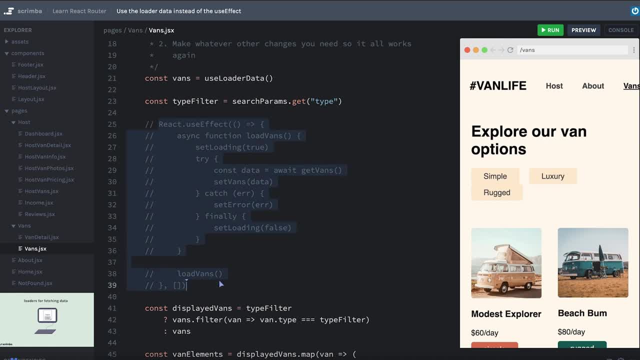 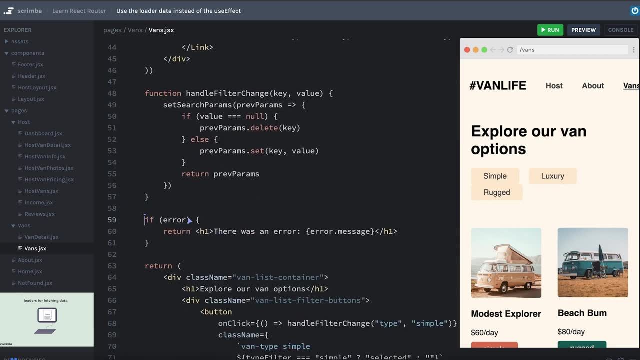 also. i mean, we saw first of all that this whole use effect we didn't need anymore. we can get rid of that, and we have this loading state down here that i don't need to handle anymore, so we can get rid of that. so let me clean this up too. while we're in the habit of deleting things, i also can. 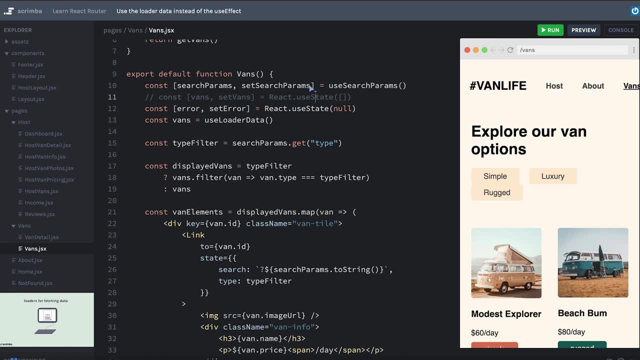 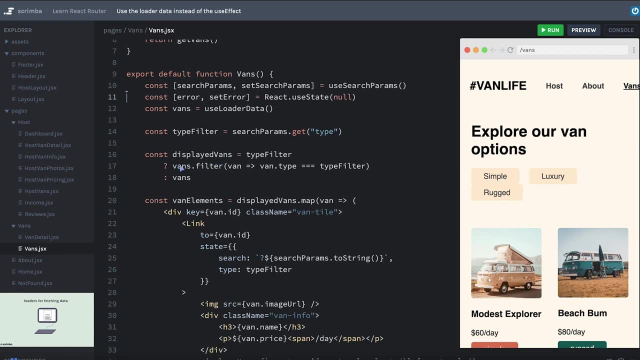 delete my state instead of re-rendering my component, because i am setting the state with the data that has come in. after the component has come in, i can delete my state, and i can delete my state after the component was loaded. i know that the data is going to be there when i pull it in with. 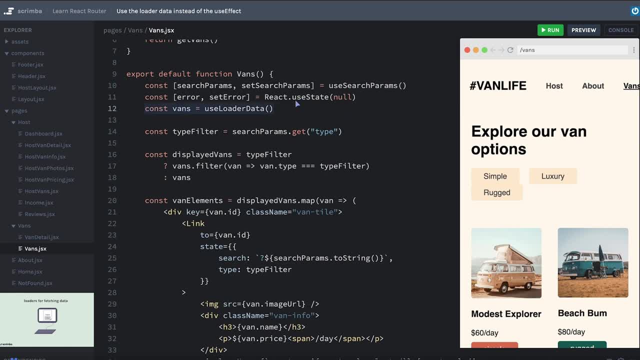 the use loader data hook, in the sense i get to treat this much more synchronously. instead of having to think about how the component needs to mount and then do a fetch request and then update the state and then to re-render because the state has changed, i don't have to worry about any of 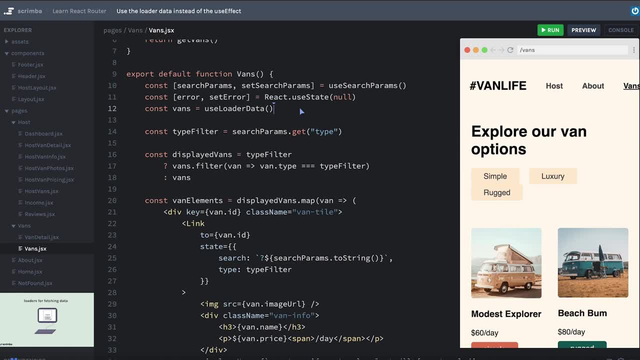 that the mental model for this is significantly simpler. not only that, but i can still do my loader loader code right here in the same loader code in the same file and start looking for some models and start looking for some models for that. and start looking for some models and start looking for some. 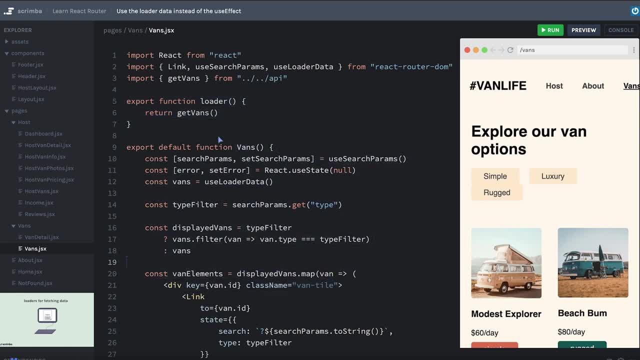 file where I'm concerned about the display of that data that gets loaded from my loader. I don't know, maybe you're not quite as excited about this as I am, but this is a really nice paradigm shift. Now there is something that we lost when we deleted our use effect, and that is that we are 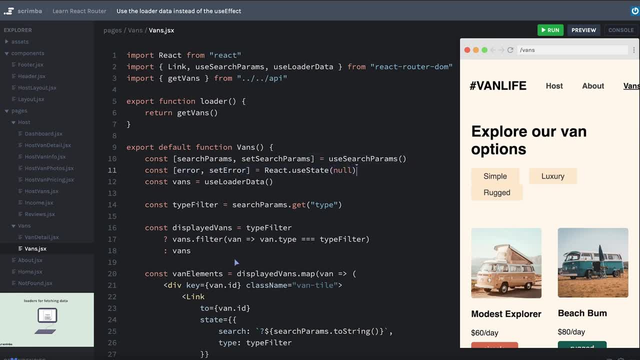 no longer really handling any errors. Remember, we had that catch block in our try catch that would set the error. Well, because we deleted our use effect, we're not doing that anymore, But that wasn't a mistake, because React Router has a way for us to handle errors and it's very simple. 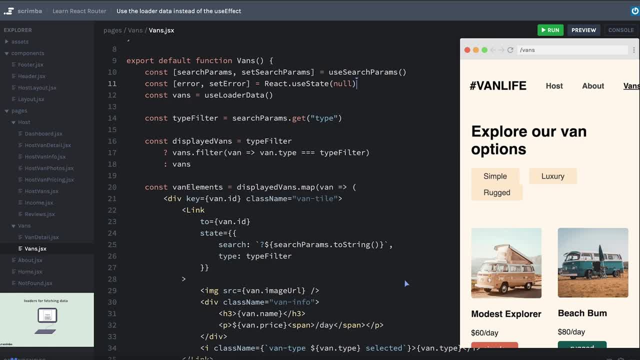 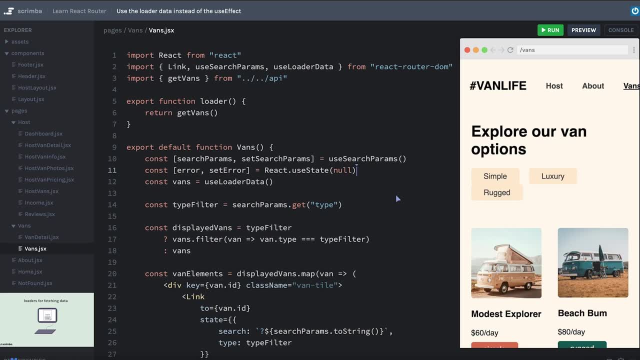 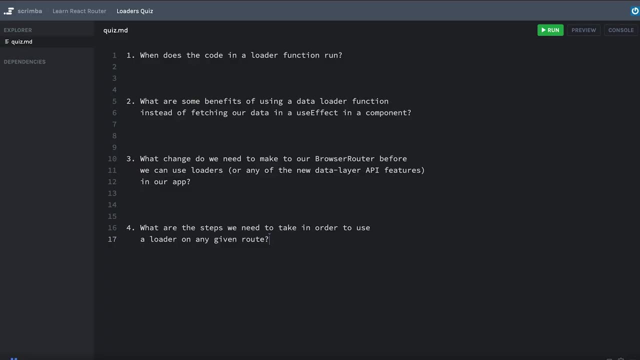 Once you've had a chance to bask in the glory of having deleted all of that useless code, let's spend a minute to learn about error handling when we are doing our fetch request before the page loads instead of after. Surprise, we're actually going to do a quick quiz before we. 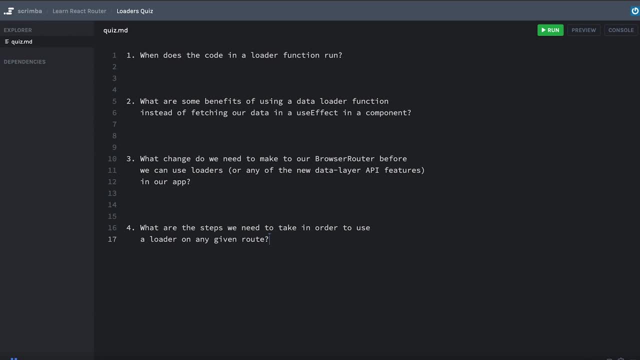 move on to handling errors. So you know the drill, pause the screencast, click into each of these and actually type your answer, And then we will go through all of these together. Okay, number one: when does the code in a loader function actually run? 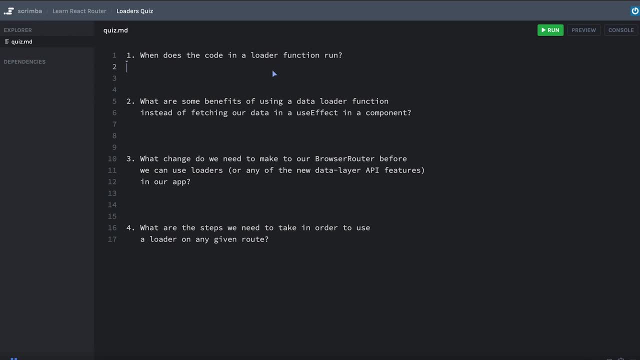 Unlike how code inside of a use effect runs, which happens immediately after a component mounts to the page, a loader function runs before React Router allows the route to change and that new component to load. So, in short, a loader function runs before the component loads. 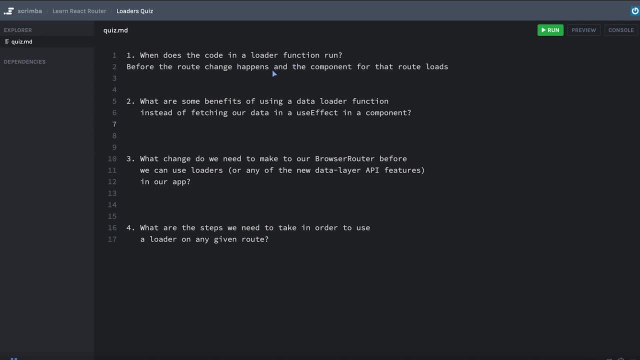 And the route change happens, Okay. number two: what are some benefits of using a data loader function instead of fetching our data in the use effect in a component? Well, one of the main benefits is we don't have to handle error state, which, again, we're going to be talking about next. 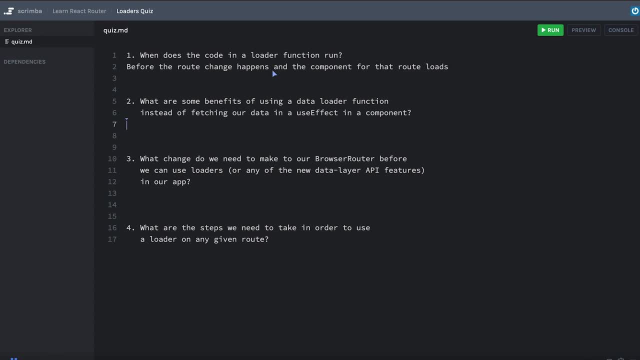 We don't have to write a lengthy use effect. that's part of our component code. We also don't have to worry about loading state, because we know this component won't mount to the page until the loader has already completed its task. Or in other words, we don't have to worry about loading state. 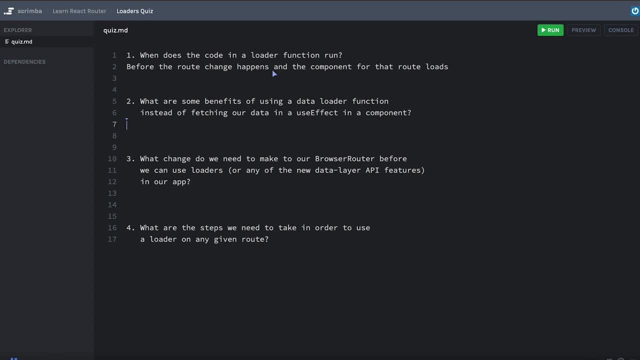 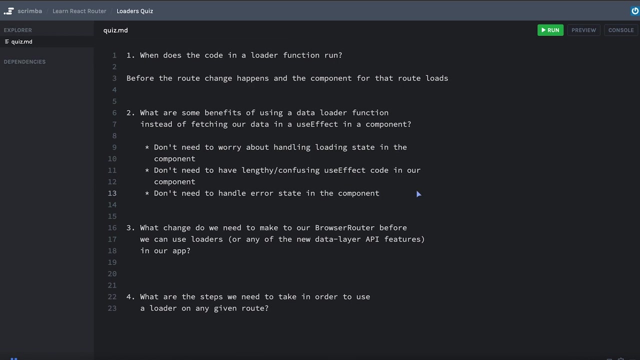 until the loader has finished its task. We know that when we access the data with use loader data, we will have access to the data as if it were happening synchronously. So we'll type something like that down: Okay, number three. what change do we need to make to our browser router before? 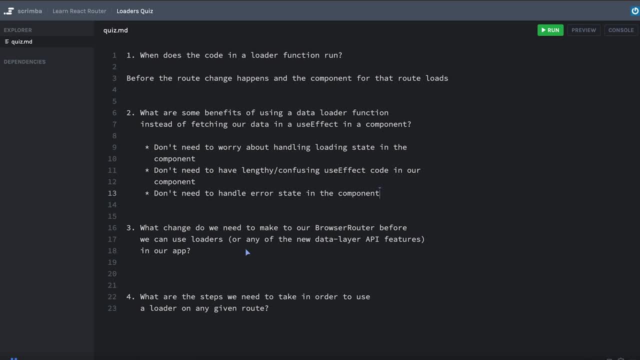 we can use loaders or really any of the new data layer API features in our app. I guess the wording of this could be a little bit like a trick question, because we just need to get rid of our browser router and we need to use one of the accepted data routers instead. 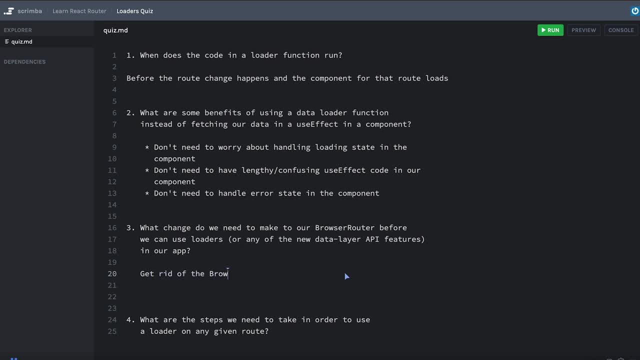 So we need to get rid of the browser router altogether And we need to use the create browser router function instead. If you're really wanting to jump both feet in to the new system, you can choose to use create browser router with the array of objects, As we discussed in the 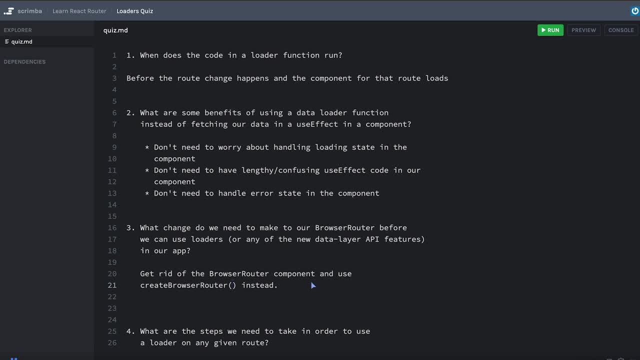 lesson. you can find more examples of that on the React Router docs. Or if you already have a browser router, you can use the create browser router function instead And we need to have some pre written code that you're trying to transition to this new router using create browser. 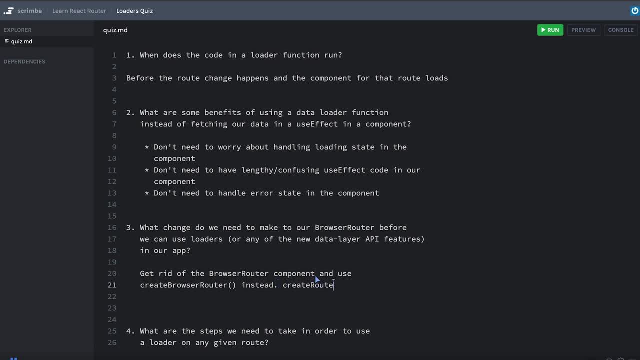 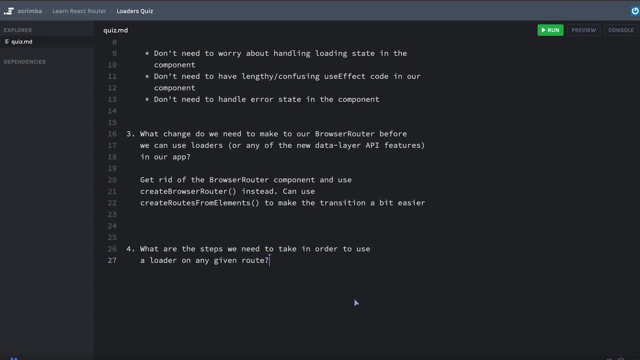 router. you can use that function, create routes from elements to help you make use of the code that you've already written. Okay, and then, lastly, what are the steps we need to take in order to use a loader on any given route? First, we need to define a new loader function and export it. Usually, 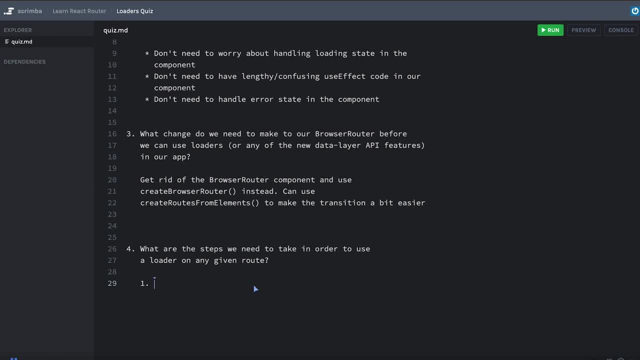 it's defined in the same file that our component is being defined in, And so we can write that down, say: define and export a loader function. Secondly, we need to import the function that we just exported into our route definitions and set it up as a loader on the route that we are trying to gather data for. 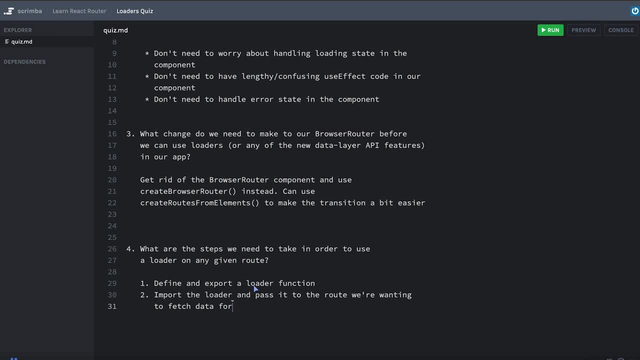 Okay, and lastly, we need to use the use loader data hook inside of the body of our components so that we can get the data that was fetched or produced or evaluated or whatever it is inside of our loader function. Okay, that was a lot of information, but hopefully it sunk in. Okay when. 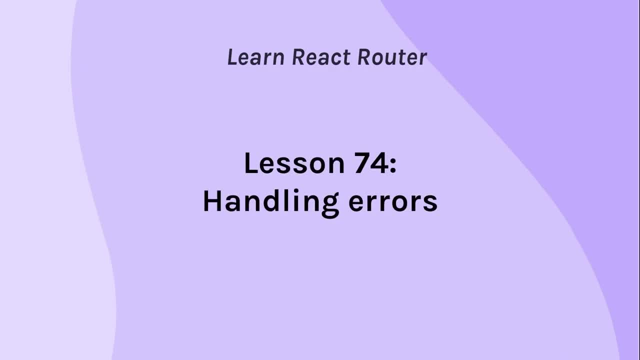 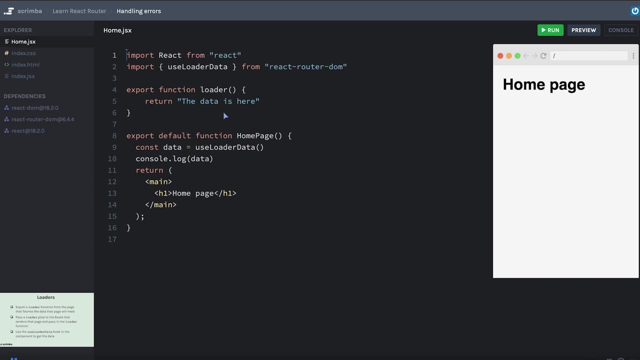 you're ready, let's talk about error handling. Okay, let's see how we can actually handle any errors that might happen Now. this example might be a little simplistic, because we're not getting any data that will ever fail, because JavaScript is. 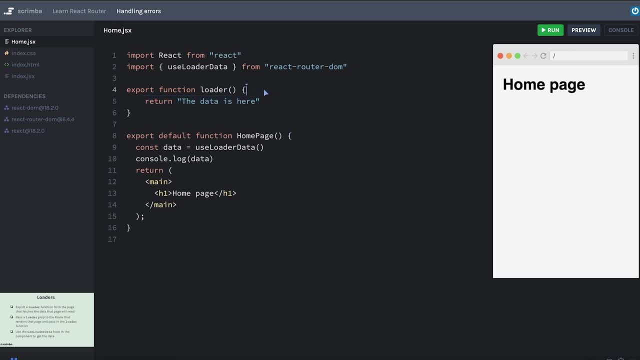 probably not going to fail just returning a string like this. So let's see what happens if I were to just manually throw an error. We'll say the throw new error. we'll give it a little message that says this is an error error. I'll comment out my return, even though it'll never get run because I'm throwing an error. 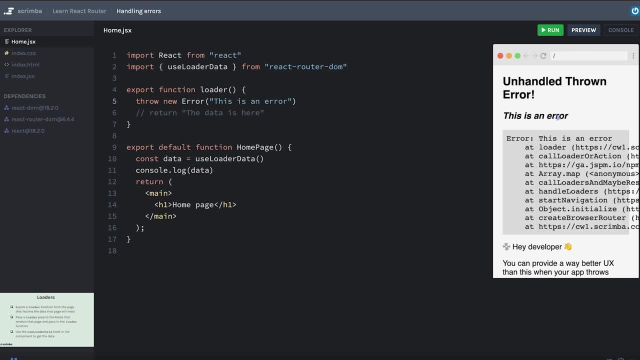 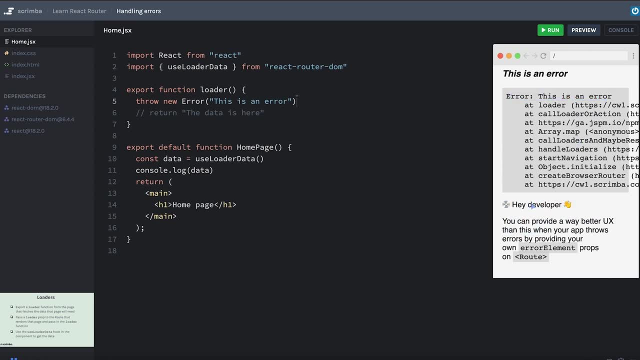 manually. Let's see what happens. I'll hit save. Okay, we have an unhandled thrown error. This is an error. It tells you some of that information about the error and then it even has a little message here that says: hey, developer, you can provide a way better user experience than this. 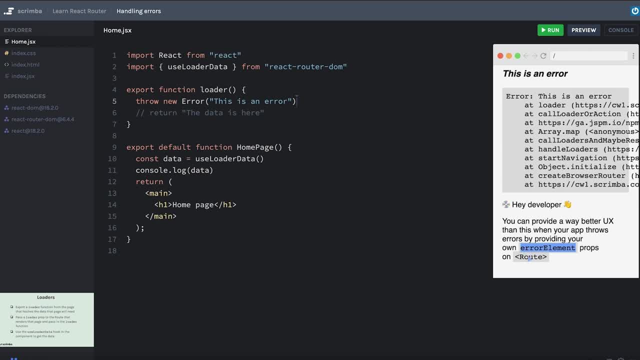 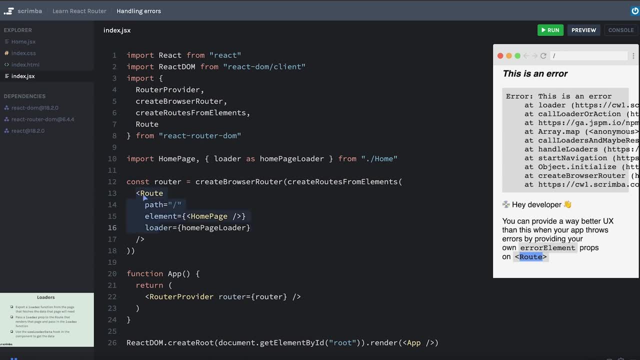 when your app throws errors by providing an error element prop on your route. Okay, so what does that mean? Well, if we go over to indexjsx here on my route, you can see I've put things on their own lines to buy myself a little bit of room- We have this element prop, which is basically what. 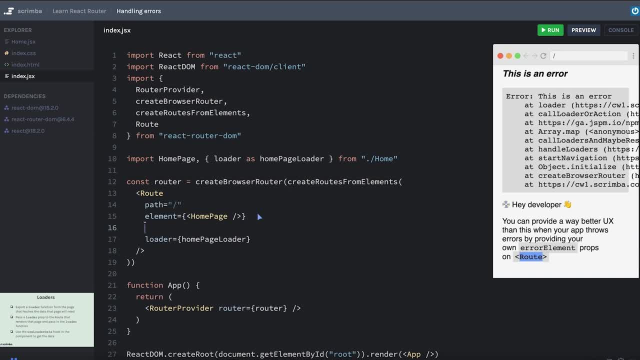 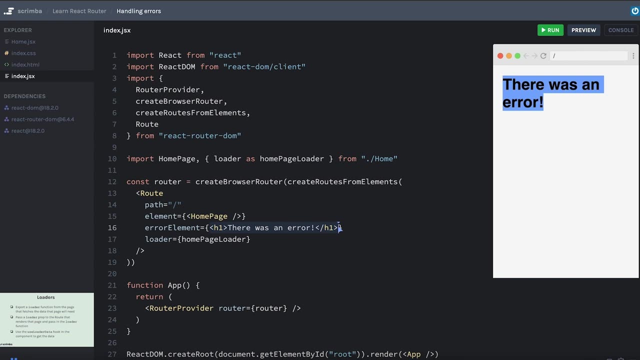 element should I render, assuming everything is going well? Well, we can also add a prop called error element. Let me just hard code something for now, maybe just an h1.. It says there was an error and let's hit save. Okay, we get, there was an error. This is our h1. that is being rendered instead of. 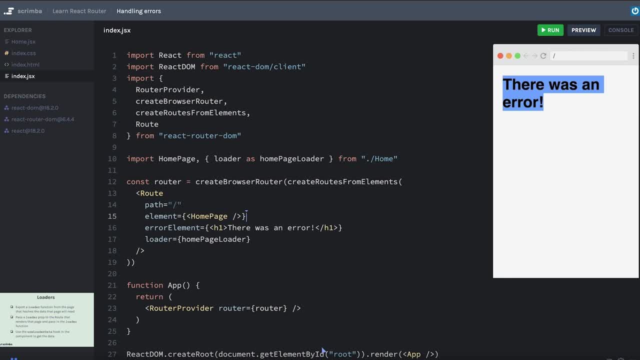 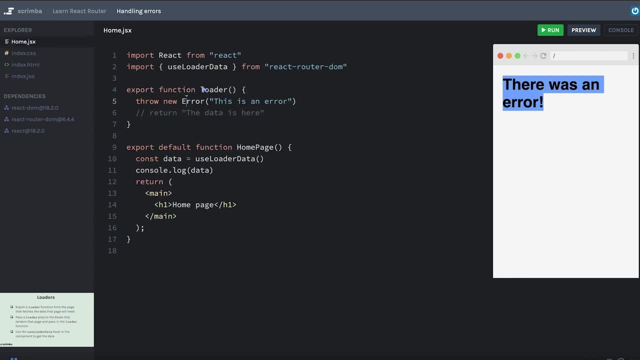 the element that was supposed to be rendered, because our app is experiencing This is our h1 that is being rendered instead of the element that was supposed to be rendered. One thing that's neat about this is it will handle more than just an error that's happening inside of. 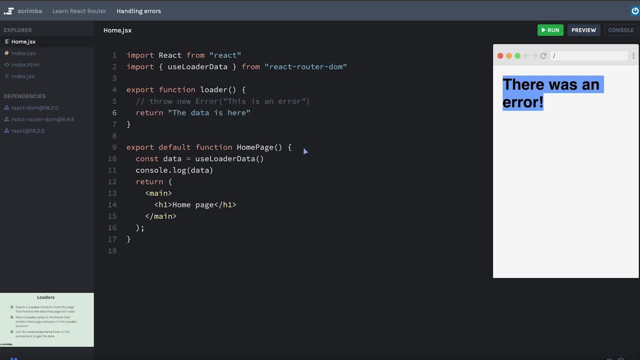 our loader, For example. let's say our loader is working just fine, but for some reason we maybe try to access a property of an object that doesn't exist, or a function that doesn't exist, or something like that, and that throws an error here. So let's say we're throwing a new error. This is a common 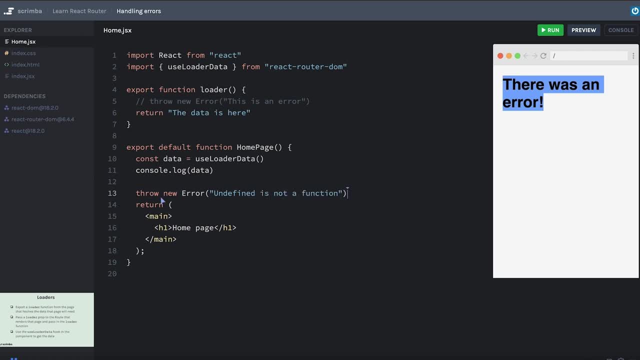 one. We'll say undefined is not a function. This is just pretending that we're trying to call a function that we think exists, but it's actually a value of function. So let's say we're trying to call a function called undefined. Now we're not actually using this message anywhere, but let's hit save. 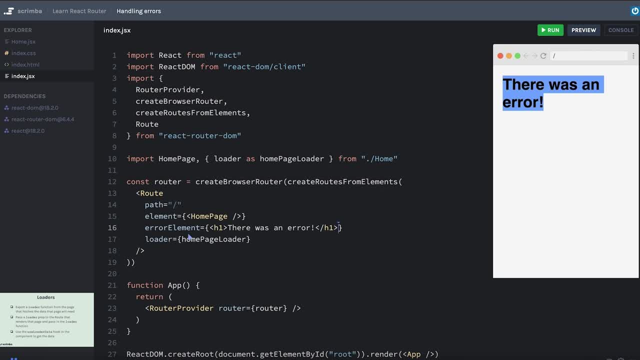 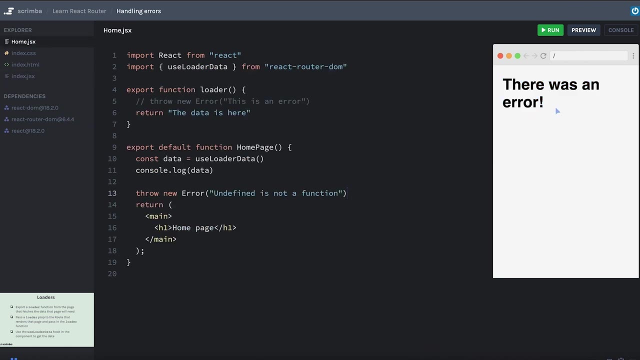 and we get our error element that we set up here. So I guess the point of this is the error element will happen anytime your component that you're trying to run has any kind of error. It could be an error that occurs in the loader, or it could be an error that's just happening inside your component, Just spitting out an h1. 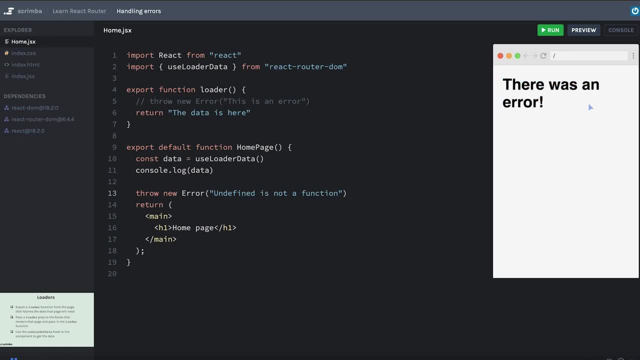 that says there was an error isn't the best user experience either, but hopefully you can see that you could tailor a well-designed and hopefully this is just a very useful error component that will display some really useful information in a nice way that isn't quite so jarring as what we have here. Okay, so let's go back to the van life app and we will bring back the 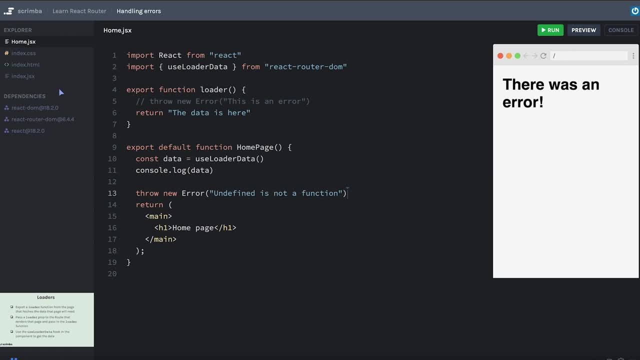 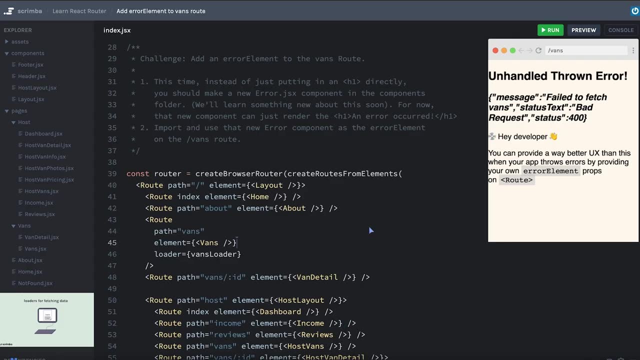 ability to do some ever handling by using an error element in our route. Okay, let's apply what we just learned about the error element prop, and we'll forento to the van's Herrert patch item on the trash calender app. However, you're going to do a little bit more than what we just learned about, Instead of just going to put the error measurement. 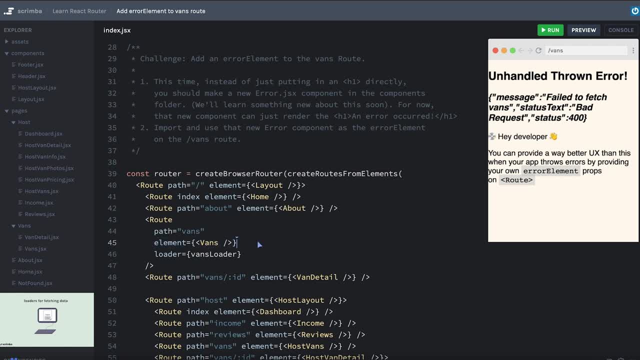 in small error button or something as Ching a little bit, even if that doesn't help, withuinely push h1 directly inside of our error element. I want you to create a completely separate component up here in the components folder that you can just call errorjsx. At this point we're not 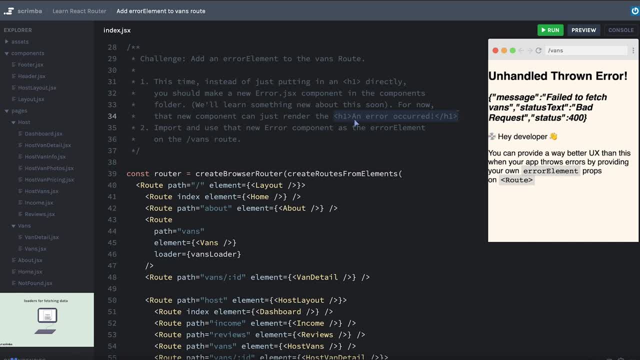 going to get much more complex than just rendering an h1 that says something like an error occurred, and then you'll want to import and use that error component as the error element on the vans route. Remember, right now our error is coming from the fact that we have just hard-coded an error. 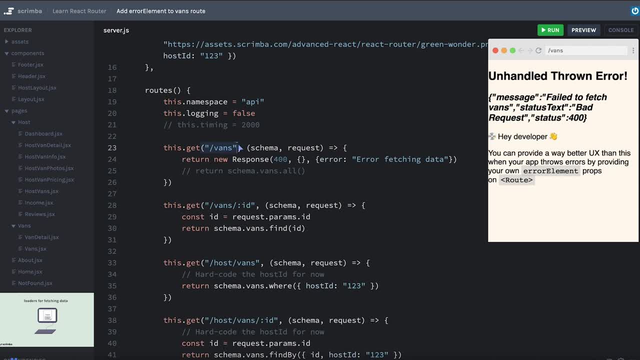 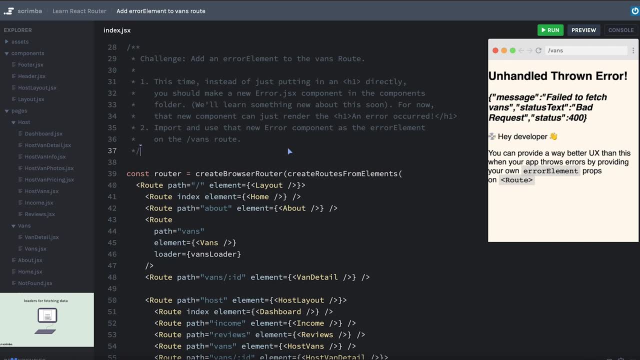 response when we try to get the vans from the slash vans route. So let's go back here, to where you can see the challenge. pause now and add an error component to our vans route, All right up in our components. I'm going to create a new file called errorjsx. We will set. 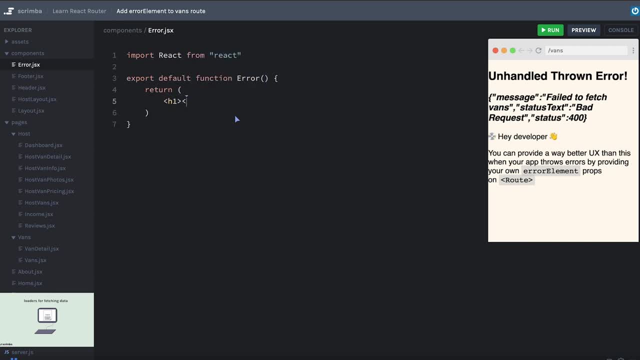 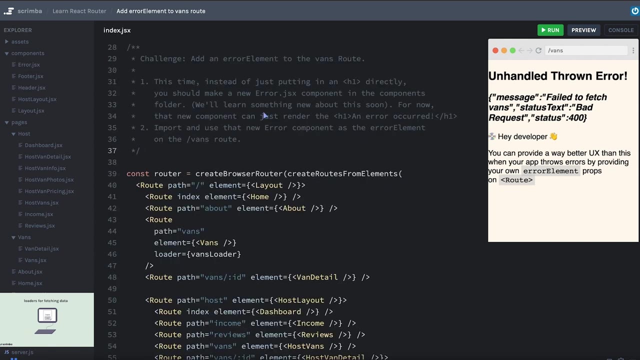 that up and, like I mentioned, we're just going to return an h1 that says an error occurred, and we're going to revisit this later and beef this up. We're going to see how we can make this a little bit more useful, but for now this will do the trick Over in indexjsx. we have done step. 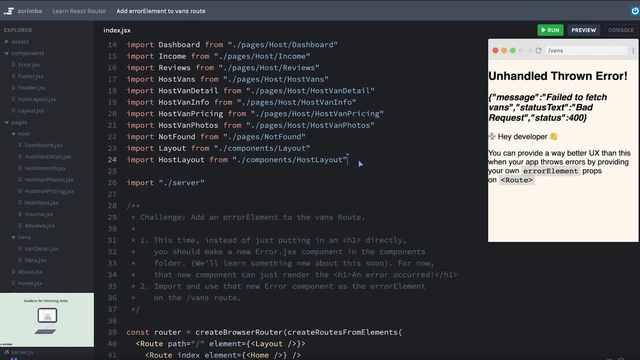 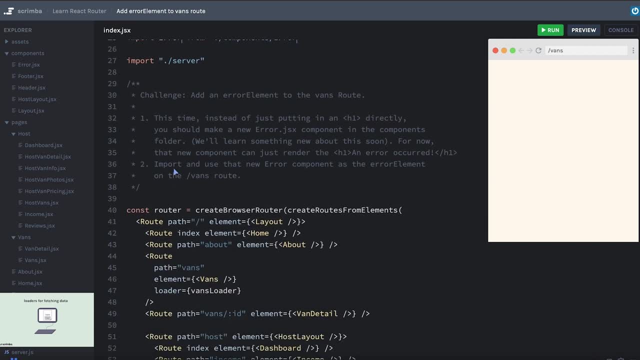 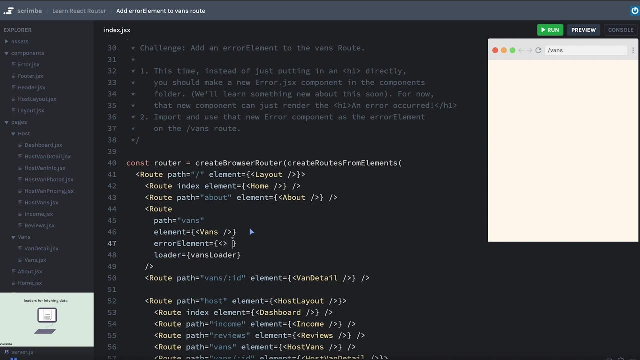 one, so let's do step two. We're going to import the error component. Oh, and I refreshed it. so now we have an error, but let's call this error and down here, maybe just right below the element, we'll create an error element and we'll create an. 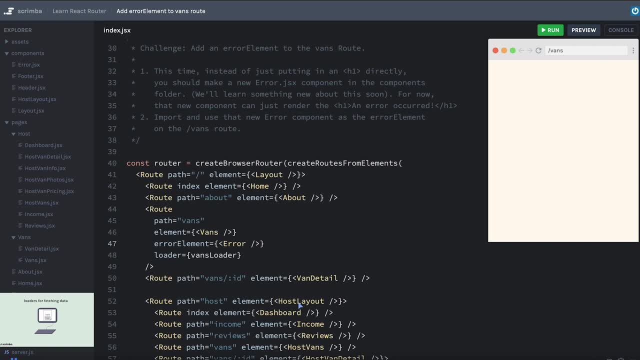 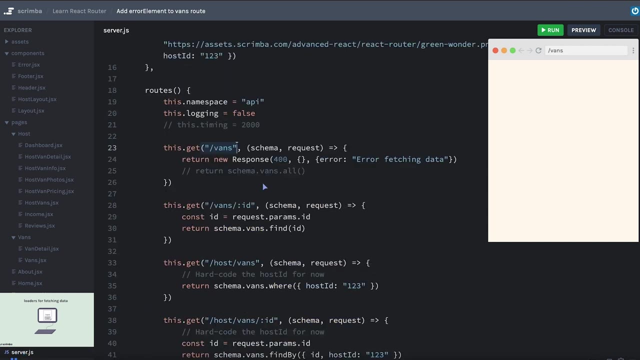 input instance of our error. Okay, so when I hit refresh, React Router will see we're at the slash vans route. That has a loader attached to it, so it's going to run the vans loader. The vans loader makes a fetch request to the slash api slash vans endpoint that we have. 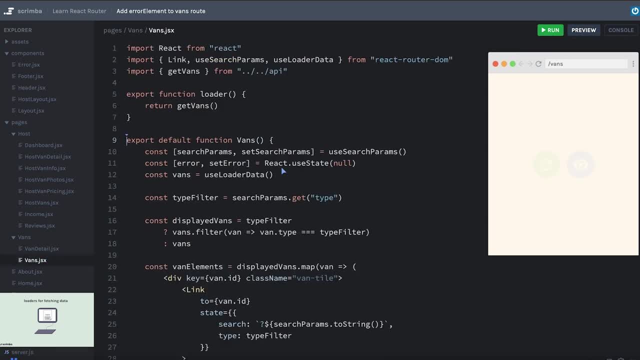 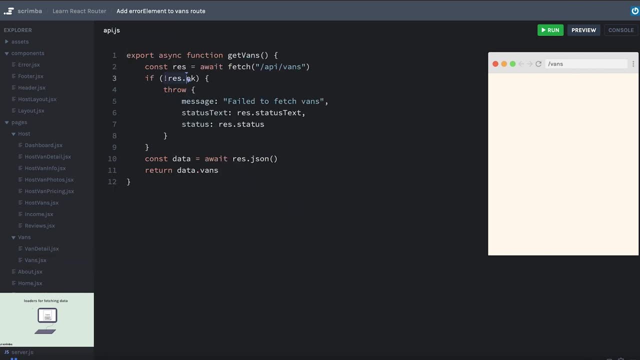 on our mock server and the loader will interpret the 400 response as a problem. Let's see that's in the api: get vans, so in api. yep, it'll be not okay because 400 response with fetch is not okay and so it will throw an error and because the loader threw an. 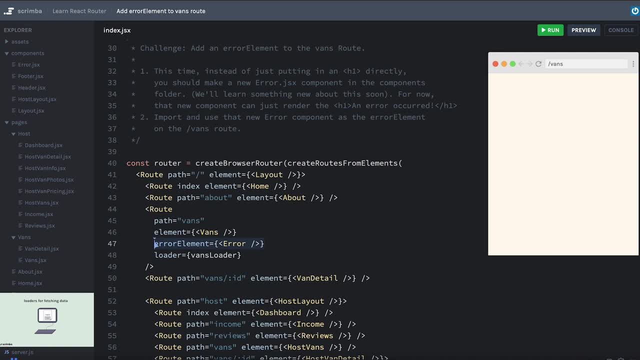 error. it's going to search for an error element and that's the element that will get rendered, so let's give it a shot. We'll hit save. An error occurred. Awesome, so it worked as we would expect, but right now just having an h1 that says an error occurred is not all that useful. 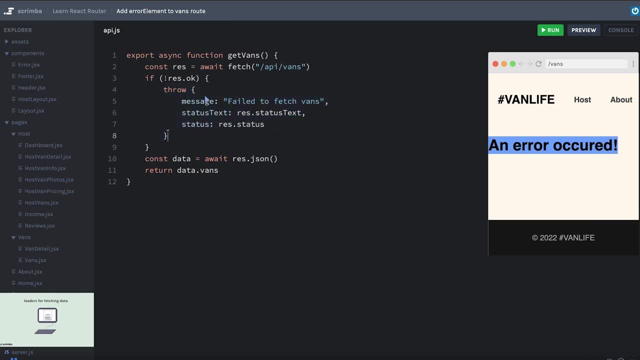 and we did take the time to provide some additional information in the error that we're throwing, like having a message that at least says failed to fetch van. so that's a bit more descriptive than just an error occurred. so how can we get the information? 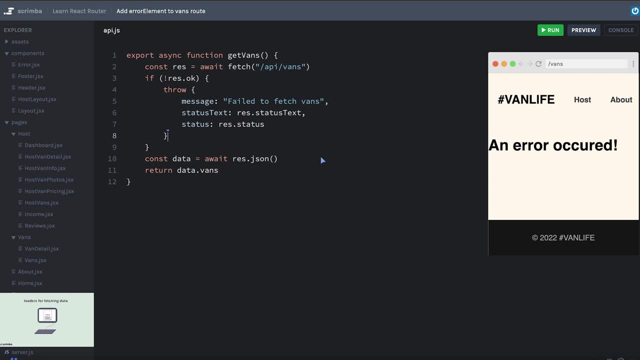 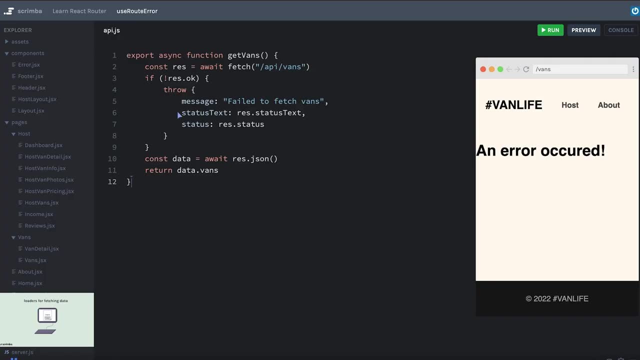 from the actual thrown error to display on our page. Well, that's what we're going to learn next. All right, let's learn how we can actually take the information from the error that got thrown and display that on the error element that we have set up. At least that way we would have. 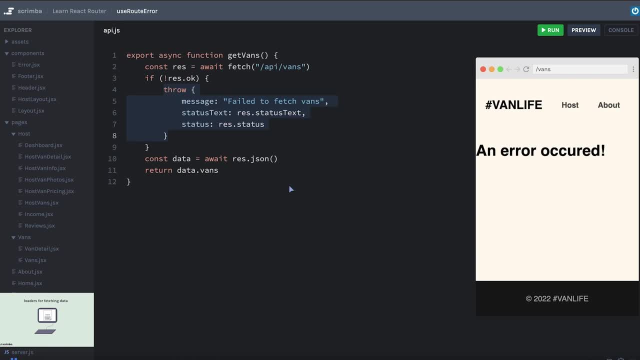 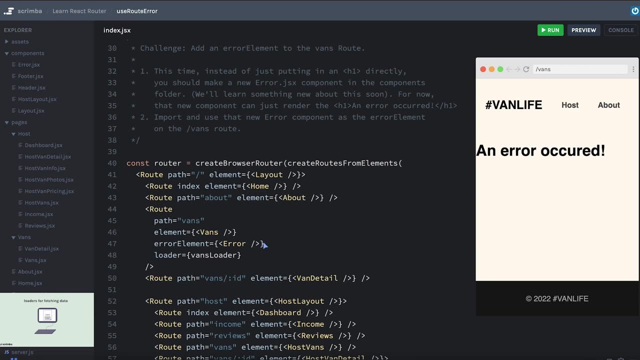 some additional information to display that ultimately would lead to a better user experience, even though they're suffering through an error. When we have an error element that is catching an error, there's a special hook in React Router we can use to display information about that error. so let's go to the error component that we just 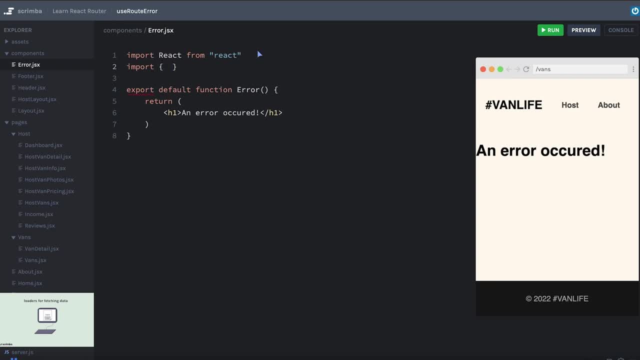 created and I'm going to import a utility hook called useRouteError. that comes from React Router, DOM and, just like some of the other hooks, we can just grab the error. We'll say that's equal to whatever comes back by calling useRouteError and we're going to import a utility hook called 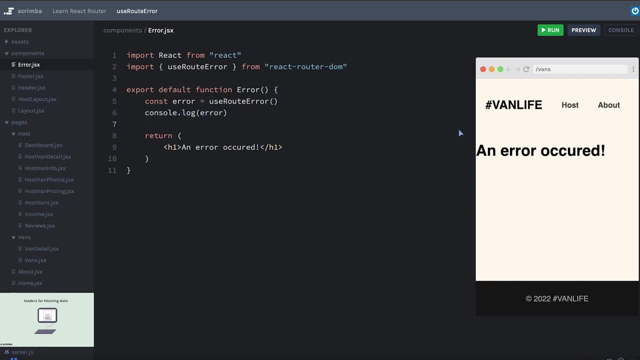 useRouteError and let's go ahead. consolelog the error to see what we get. Hit refresh, open the console. Okay, look at what's in the console. We have an object with a message, a status text and a status properties, and I want you to think: where did that object come from? 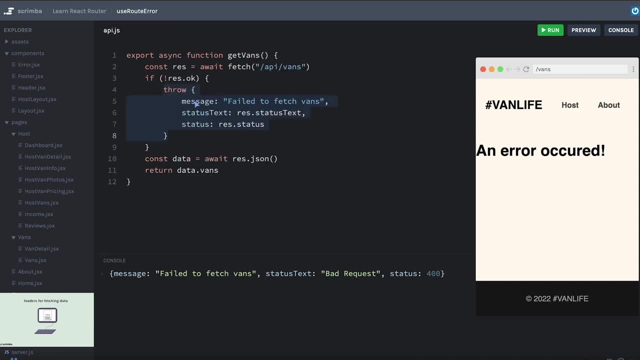 Well, that's the error that we threw from our apijs file. We said: try to get the vans in this get vans function by fetching the data from slash api, slash vans, and if the response is not okay, in other words if it's not a two or three hundred level response, then throw this. 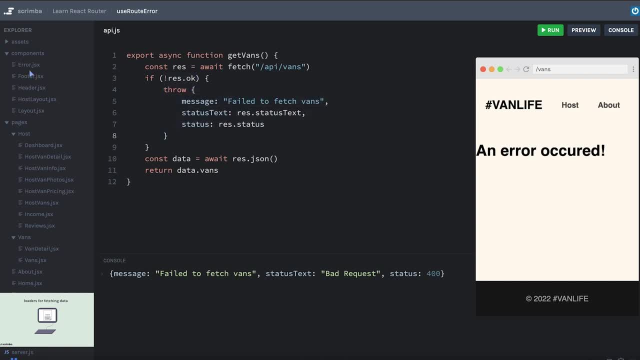 object as an error and so that object is what we're catching inside of errorjsx. If we use errorjsx in multiple places, then it's possible that this error will come back different. so we would want to make sure that, as we're throwing errors inside of our api, that we're doing it. 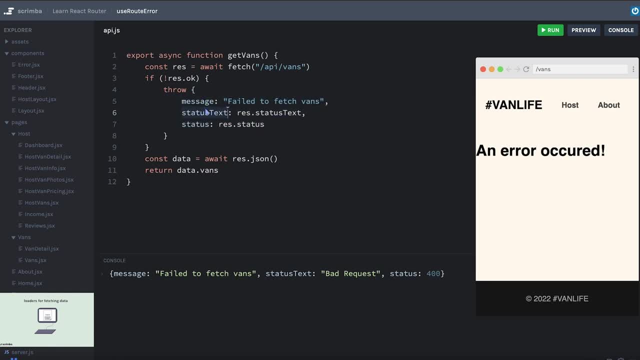 pretty consistently, preferably with a message, status text and status properties. That said, we're just going to be doing this in one place For now, so I'm going to give you just a really quick challenge where you can use the information. 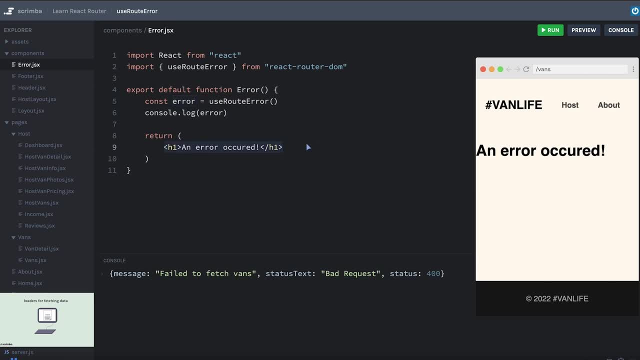 from our error object to have a little bit more of a descriptive error message. Let me type that up now. Okay, so simply put: use the error object that we just got from use route error to display something a little bit more helpful in our h1. here, In fact, you don't have to stick to just an. 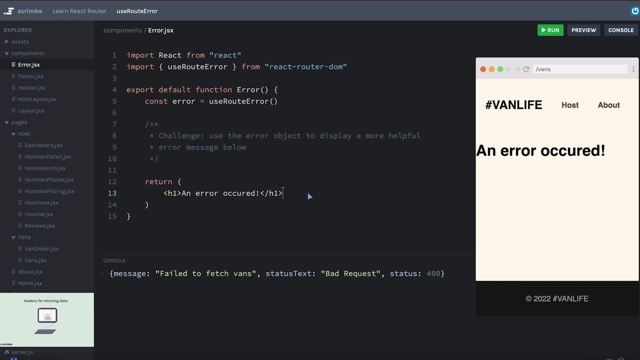 h1.. You can go a little beyond that and design it. however. you want Pause now and work on this challenge? Well, the error has a message property, so why don't we just go ahead and we will include the errormessage as part of our h1.. Let's see what that would look like. Okay, failed to fetch vans. 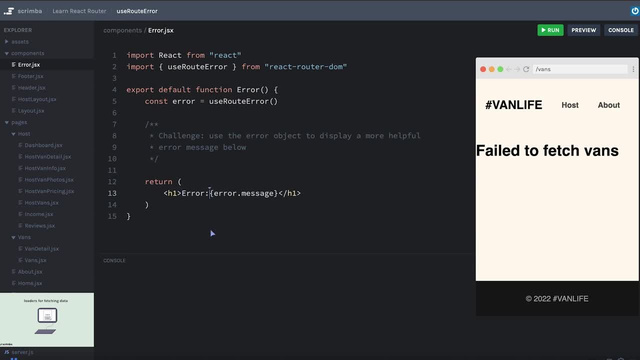 is already better. Maybe I'll say error colon just to make it clear that that's an error. And you know what? I'm going to bring back my console log of the error. here We also have a status text property and a status text property, So we're going to go ahead and do that And we're going to 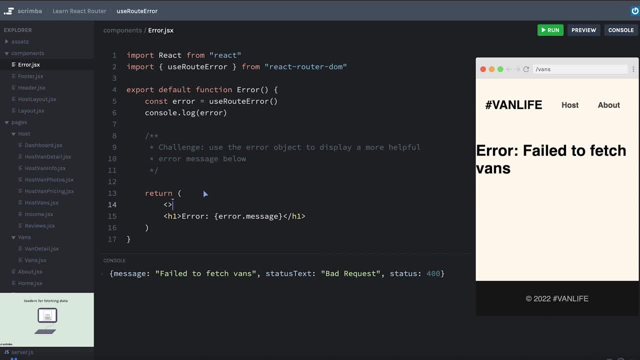 create a status property. This might be more interesting to a developer instead of the actual end consumer. But I might want to put something like: I don't know, I'm curious what it would look like if I put it inside of a pre tag. So we'll say, maybe we'll put the status, So this is error. 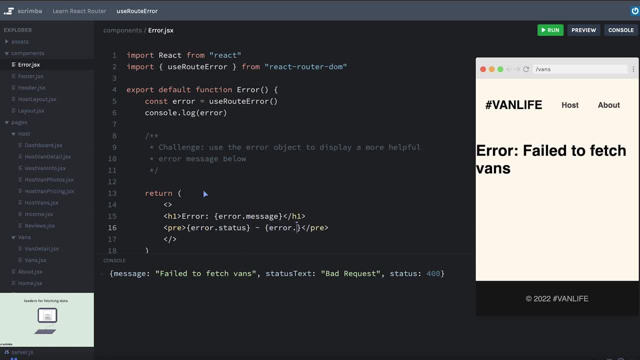 dot status and then a dash and we'll say error dot status text. See what that looks like? Well, the pre tag definitely makes it look like it's an error. It's obviously not very beautiful, But the point is we have an error and it accurately looks like it's an error. So we're going to put 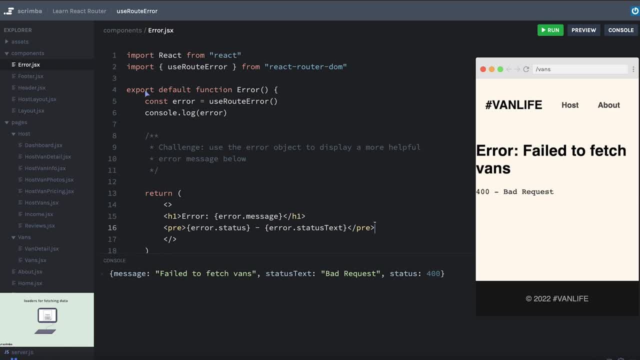 an error dot status text And that accurately conveys that message to the user and to the developer. Okay, let's get rid of some of our extraneous things here And awesome. Now. we could make this a little more robust if we wanted to maybe check for the fact that there's a message. 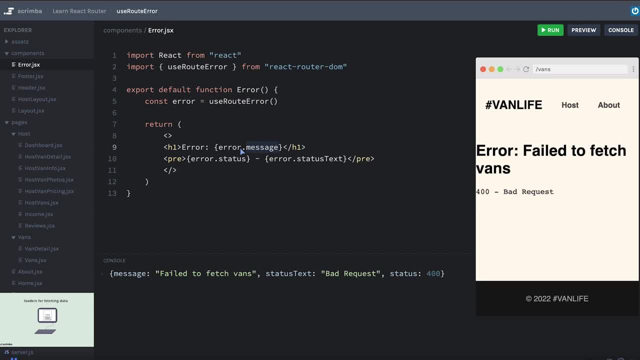 property on here, And if not, then we could have some kind of generic error message. And same goes for the status and the status text. Maybe, if those don't exist on our error that we pulled from use route error, we can either just omit this pre tag completely or have some other kind of message. 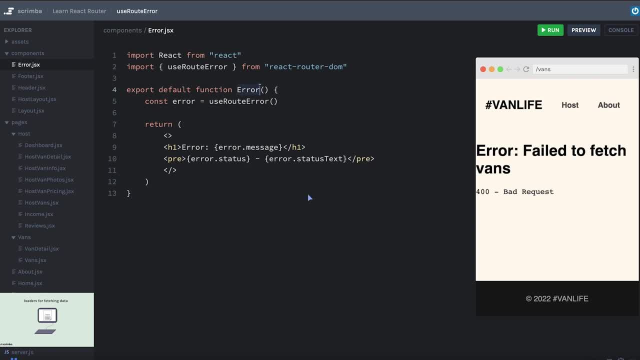 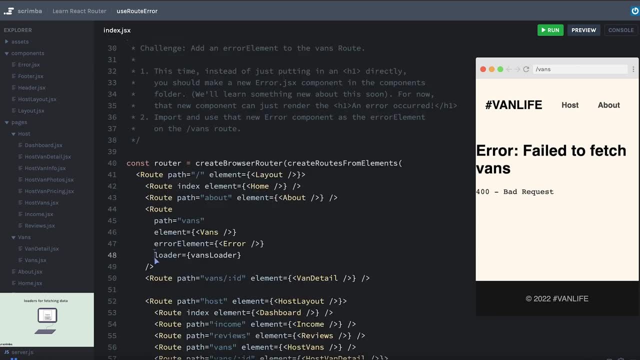 there. At this point I'm not going to worry about that too much. Along those lines, if we did want to make our error a little bit more generic, an important thing to know is that, even though we are throwing the error inside of our 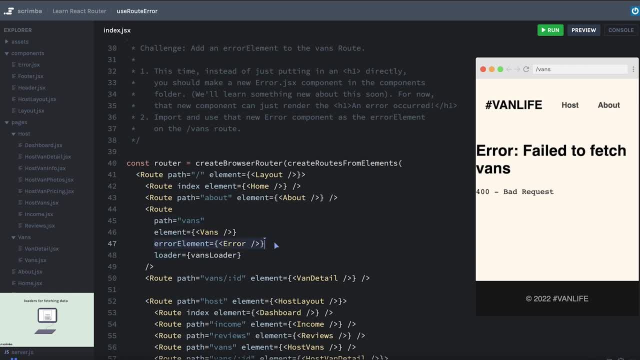 loader for the vans path and that is the same place that we have our error element. we can actually set up the error element to live on a different level in the hierarchy of our routes. What I mean is we could say: let's get rid of the error element here on the vans path. we could put 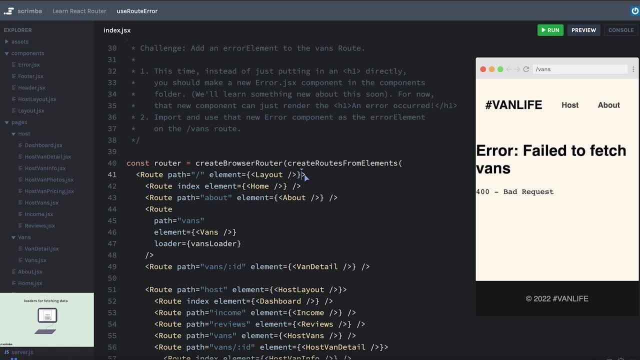 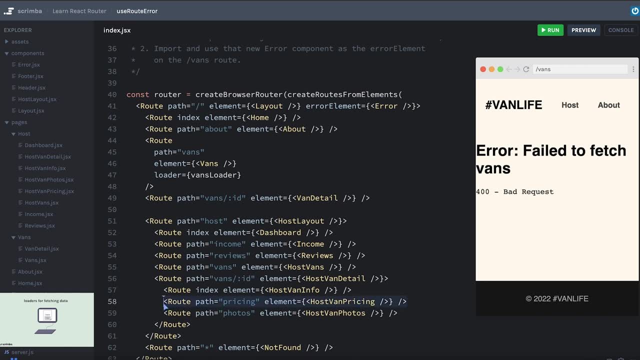 it up on the main path And let's say this needs to go right there. And by doing this, any error inside of any child route- let's say it's even the most nested child route way down here- any error that gets thrown will bubble up to the 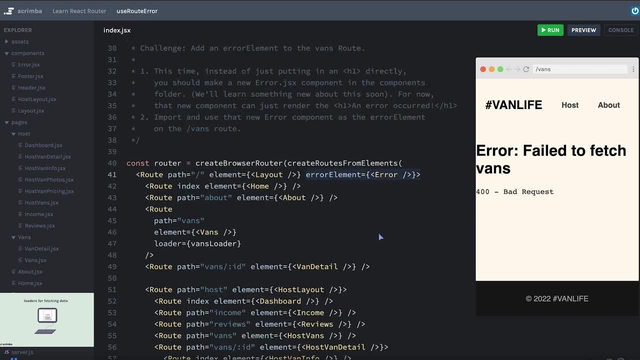 nearest error element in the route configuration here. So, even though my error element does not live on the same route that has the error being thrown, I can hit save And the error element will still correctly catch the information where the error was being thrown. Now in this case, because we put 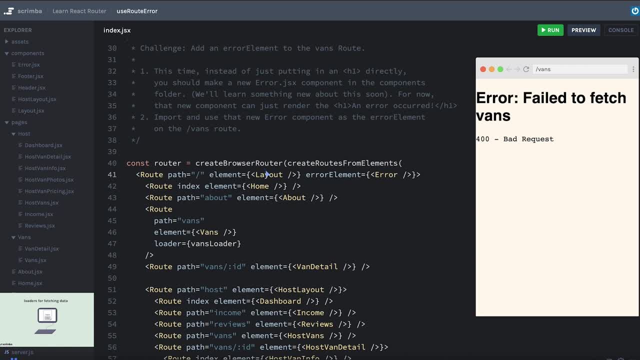 it on the same level as the layout. our layout is not getting rendered, And so we no longer see our navigation bar or our footer. So you'll want to be strategic about where you place your error elements, But the important thing to know is that at this point, this error element would now catch any error anywhere, in my app even. 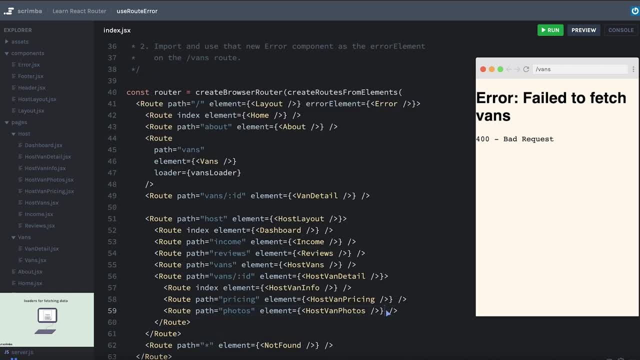 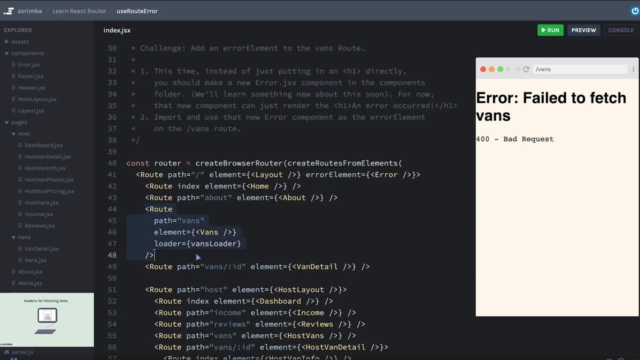 if it happened way down here, If, instead, I put the error element down here on my what is a slash host, slash van slash photos route? any error that's thrown from this vans route is not going to get caught by an error. In this case, I'm going to be creating a new one which is going to show up as an error element here. 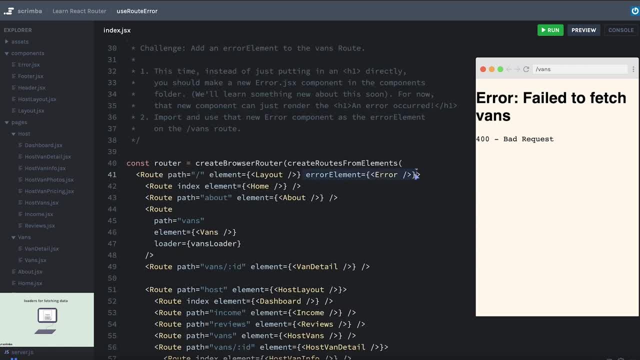 And then this error element is going to show up in the hierarchy, And I'm going to make sure that this error is not showing up in the hierarchy, And so, in this case, I'm going to create an error element that's way down here in the hierarchy. This way, you could have multiple different error elements. 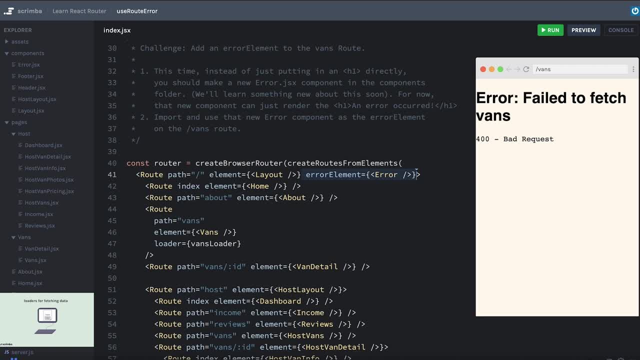 each of which can be sort of a fallback, depending on where you want that error element to show up. Maybe you want most of your page to show up and just one little nested portion that had the problem could show that there was some kind of error. The options are basically endless and you have as much. 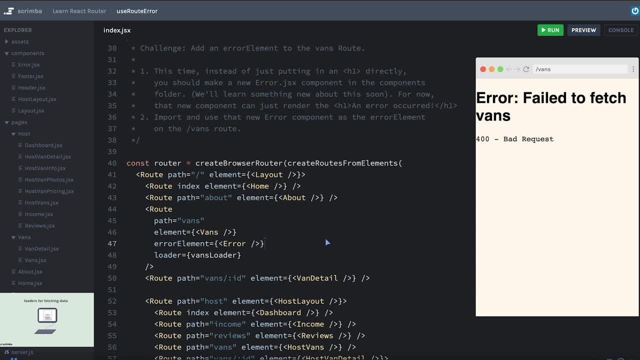 flexibility, as you need to make those error elements and error boundaries work the way you want them to work. In the meantime, I'm going to move this back down here And, as always at this point, play around with this, the code. make sure you understand what's actually going on. you can come over here to apijs and mess. 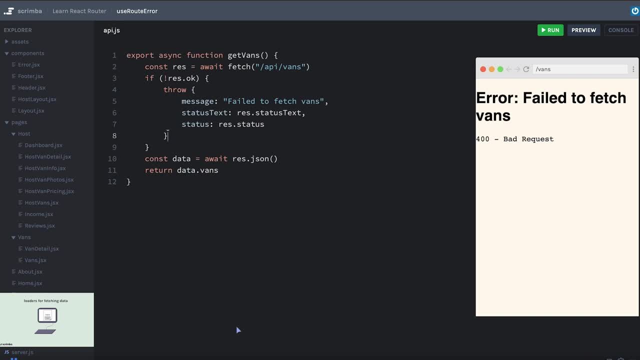 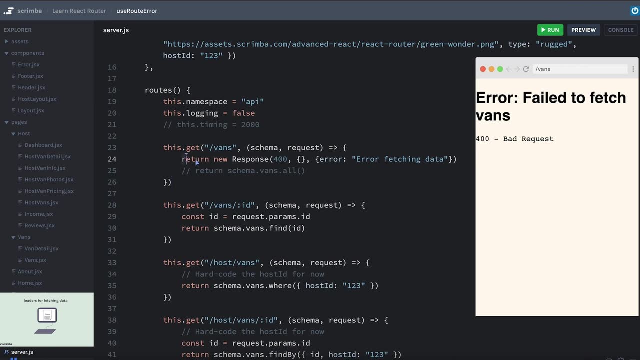 with the error that we're actually throwing and see how that affects the rest of the app. you can come to serverjs. one thing i did at one point was to choose a random number and to half of the time have it return an error and half of the time have it returned correctly. 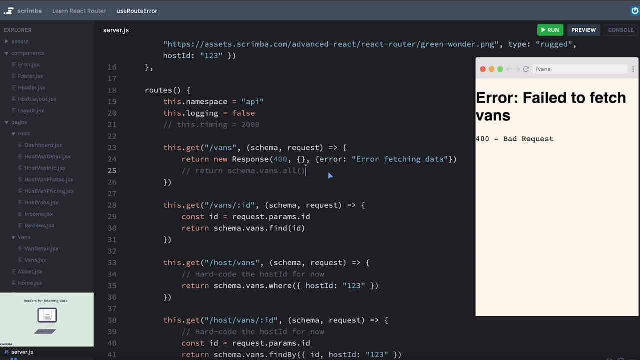 just play with the code. the more that you get your hands on it and mess with it and see what breaks and then go ahead and fix it, the more you're actually going to deeply understand what we're learning about. since we moved our error elements, i'm going to hit refresh to see the updated view. 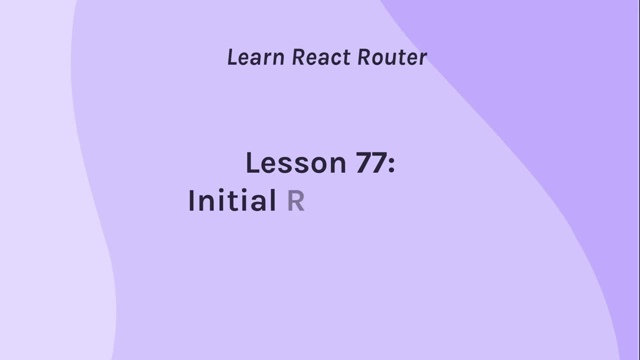 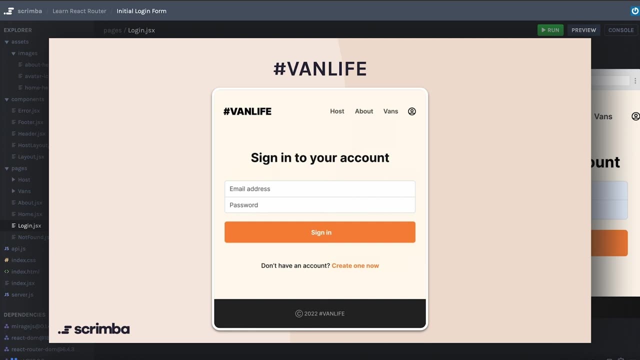 and when you're ready, we will move on to the next topic. in order for us to talk about some of the last remaining topics we have yet to learn in react router 6, we need to include some sort of authentication, and there's a bit of gray. 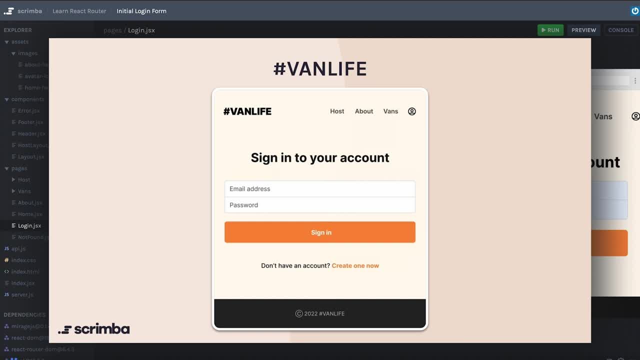 area here, because this isn't a course about authentication, but we need to have authentication implemented, at least in a very basic way, in order for us to talk about those topics in react router 6.. so this is a design for the login page that we're. 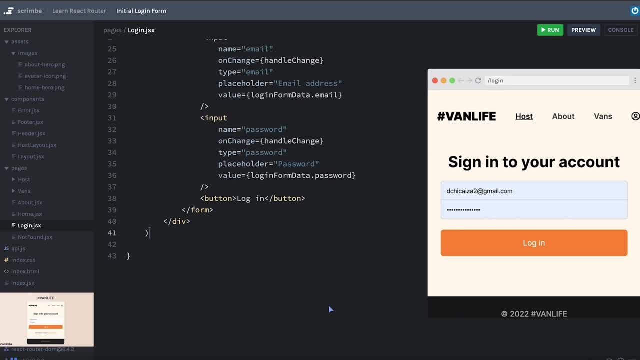 going to create- and in fact, i've already created it for you, hallelujah. and so, instead of throwing you into a bunch of code that i just wrote for you, i'm going to walk us through it step by step, so you know what steps i had to take to create this form and get it all set up. it doesn't do. 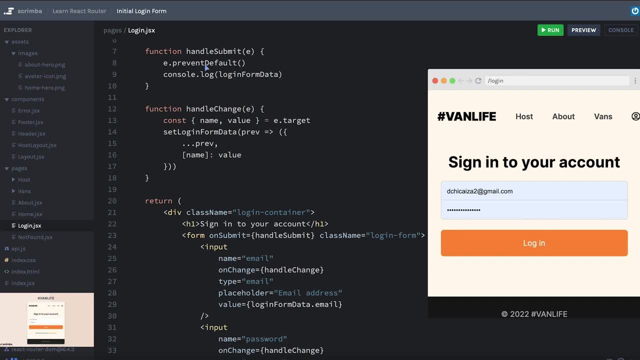 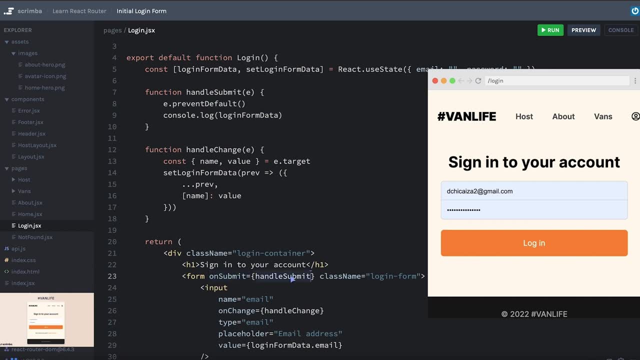 anything yet we're going to be adding to the form, but it's just a basic form right now, the handle submit which happens when the button is pressed. you can see right here the form on submit runs. handle submit: it's just console logging this form data. this form data is just. 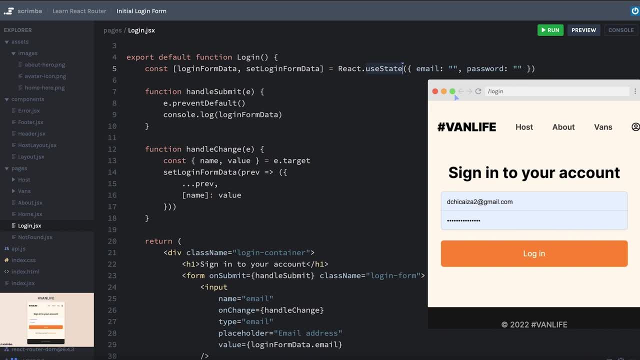 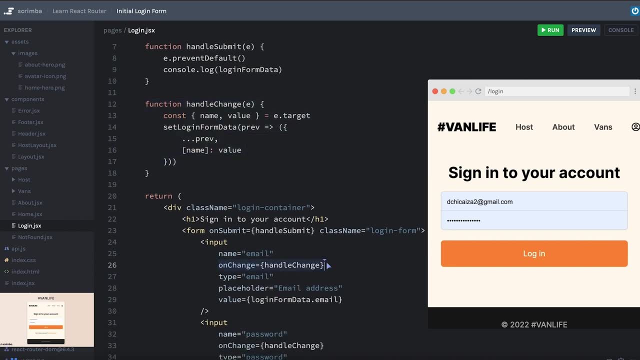 some state that we created right now. it doesn't have anything in it, it's just an empty email and password. we have a handle change function which is going to run every time there's a change on either of the inputs. this is just so that react is maintaining state for the login form data on every. 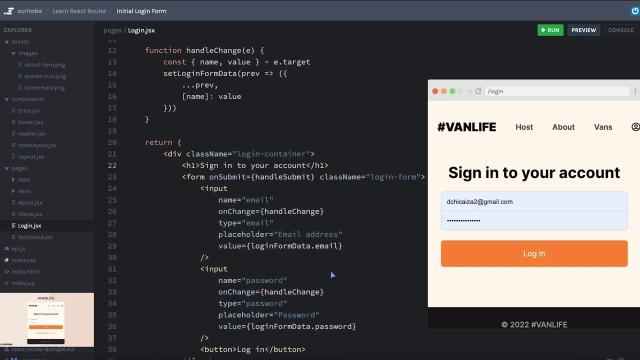 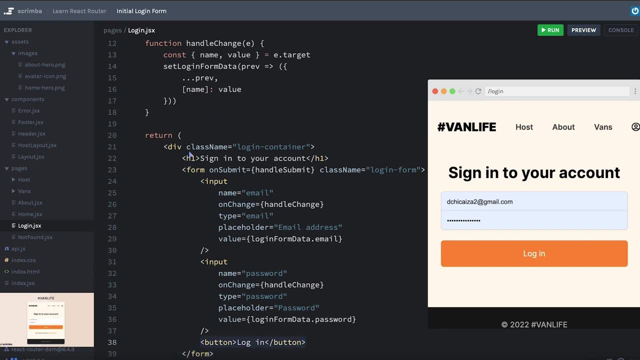 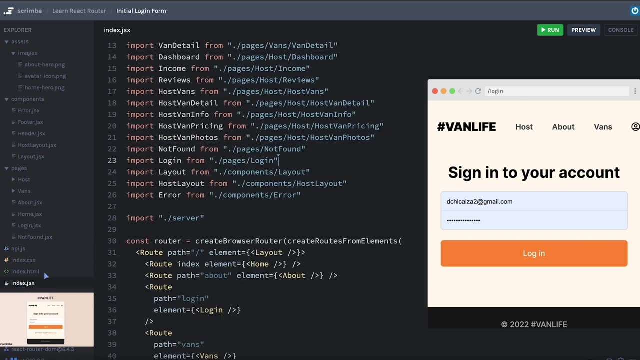 change and that's basically it for now with the form. because the button is here inside of a form, it will trigger a submit event. on the form, i of course added a bunch of css that you can feel free to go to indexcss to look up, but the other piece is in our indexjsx. i imported the login form and 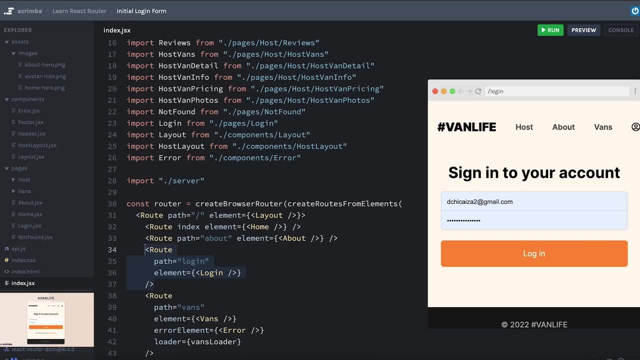 i set up a login route on the top level and then in the header, i just put this little icon which is living up here as avatar icon in our image assets. now why do we need some form of authentication to talk about react router 6? well, the main reason is this host route. 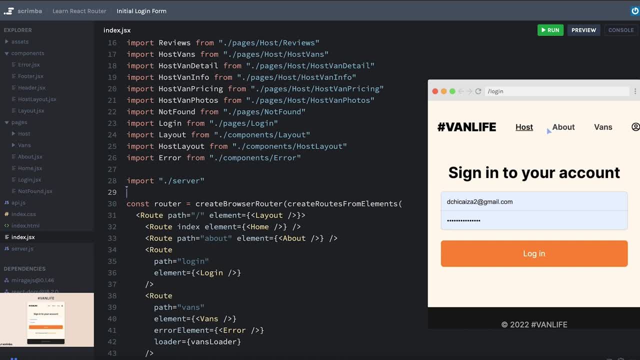 we want to make it so that this host route is a protected route, which means you have to be logged in before you can go to this host route. right now, we sort of naively have this host route up here and you're able to see all the vans whether you're logged in or not. and, in fact, if you remember this, 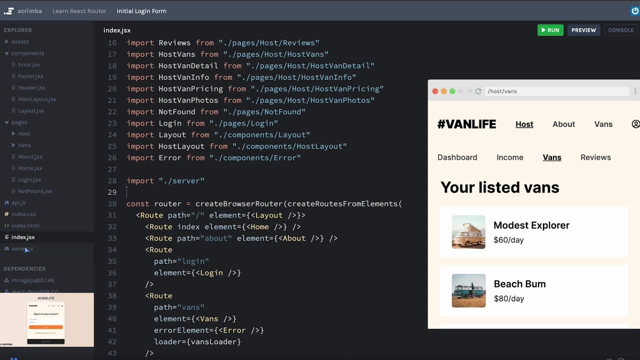 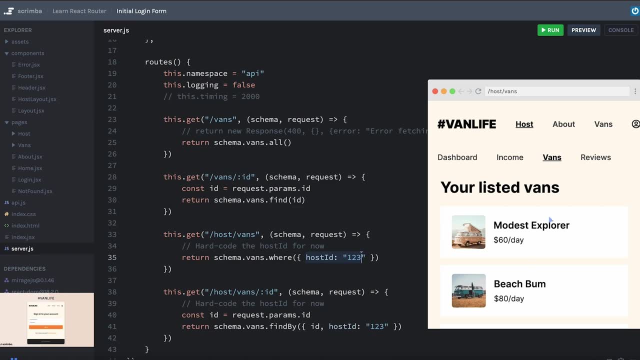 is hard coded the vans to be the user with the id of one, two, three, i think, in our user host vans where the host id is one, two, three. so it's all pretty naive, just for the sake of what we learned already. but let's look at the host vans first and then we'll talk about how to use it in our host. 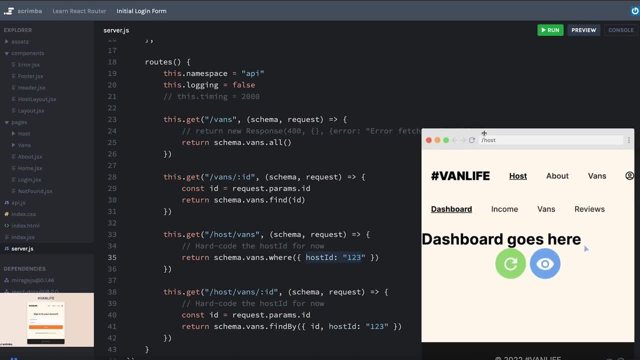 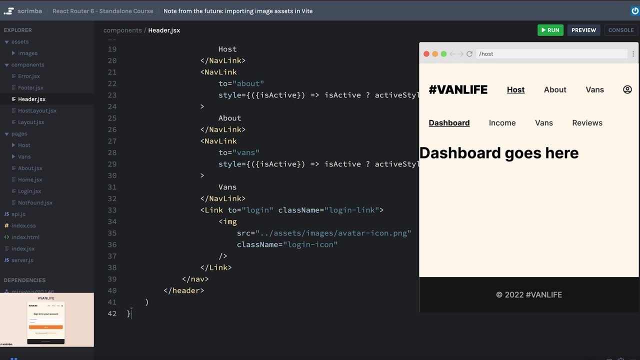 route. we want to make it so that this host route is a protected route, which means you have to be logged in before you can go to this host route. let's learn about protected routes, so that's what we're going to be doing next. i am coming to you from the future. i've actually already finished recording. 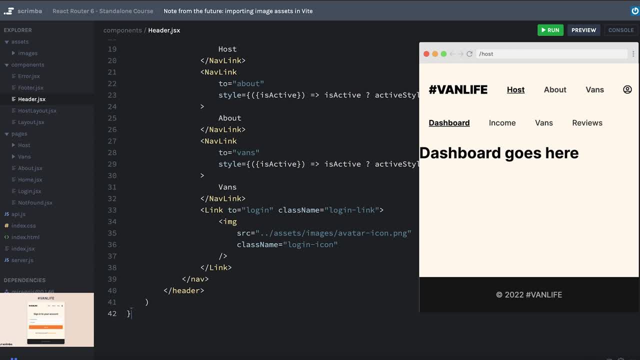 and editing the end of this course, but i did become aware of an issue that you'll likely come across time and again throughout the remainder of this course. it's relatively minor, it's not that big of a deal, but i did figure out what was going on and thought it would be good to 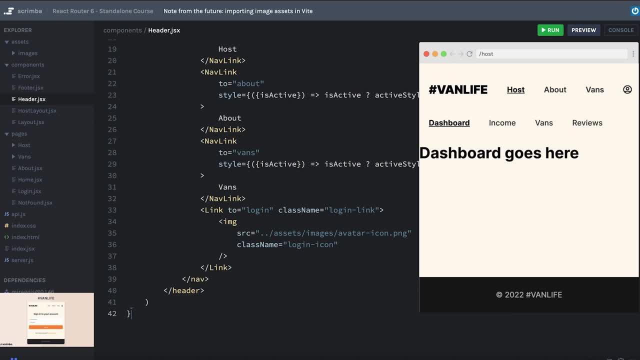 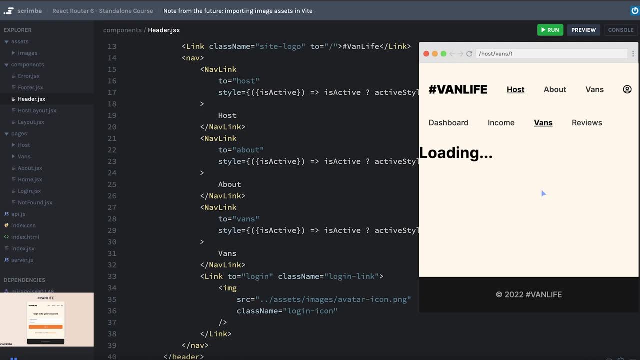 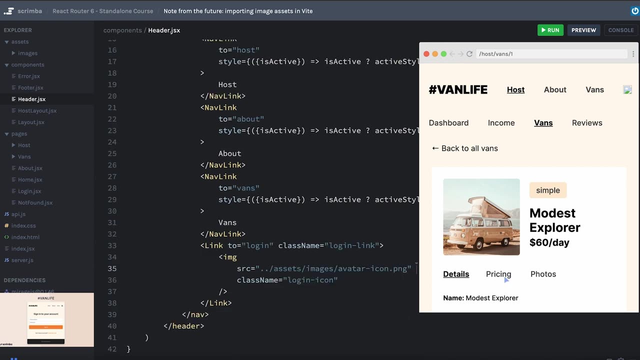 give you a quick update on that. so you'll notice that right now. i just imported this avatar image and everything seems to be working fine. but if i go a couple levels nested deeper into my url and then hit refresh, you'll see that the image breaks now. in the past, scrimba has done okay to. 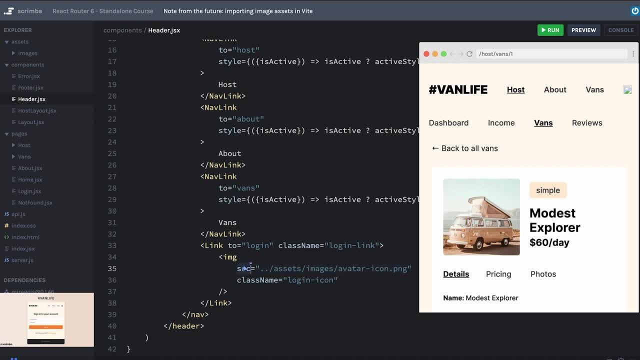 just put the relative path to the assets right here inside of the source of an image element, and in the past i've had to do that because the bundler that was bundling this code under the hood inside of scrimba was webpack, and i guess it was just kind of able to make this work. however, this 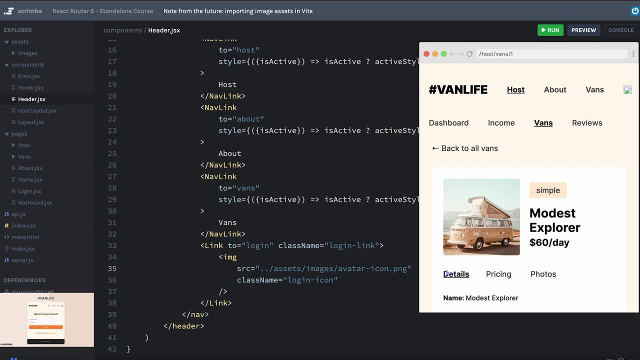 was a conflict of interest for me, so i'm going to go ahead and do that. and i'm going to go ahead and constant source of questions from students, because when you're following along on your local machine, you'll find that this just really doesn't work very well. now a quick fix here on 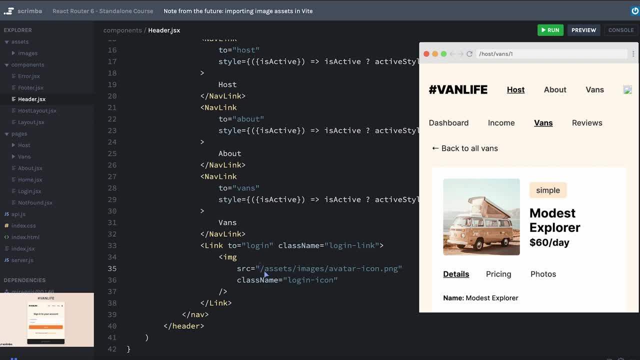 scrimba. that i guess i could have done is just get rid of the relative path and have it be absolute to the root of the project. so if i hit save, you'll see that now my avatar image comes back. that said, now we are bundling all of our projects with veet. it is much faster and it's just overall better. 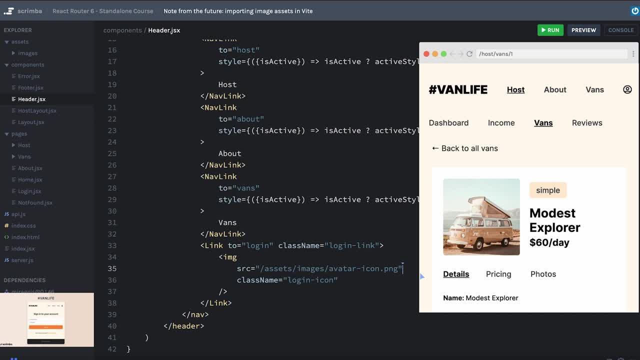 than webpack, and now that means that i can, inside of scrimba, actually do things in a bit more of a realistic or correct way, because when my project gets bundled up, my assets might end up moving or getting renamed, and having this hard-coded string here really won't handle the shifting around of 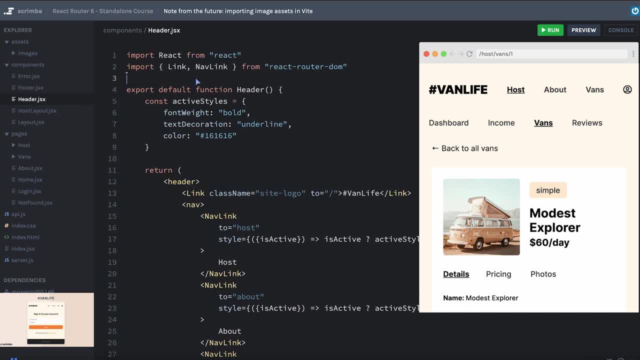 our files very well, and so the real way to do this is to import any assets that you need to use inside of your markup, and i can do that by just saying i want to import- let's call it image url from, and then we will just grab the absolute path to the image and put it in there, and of. 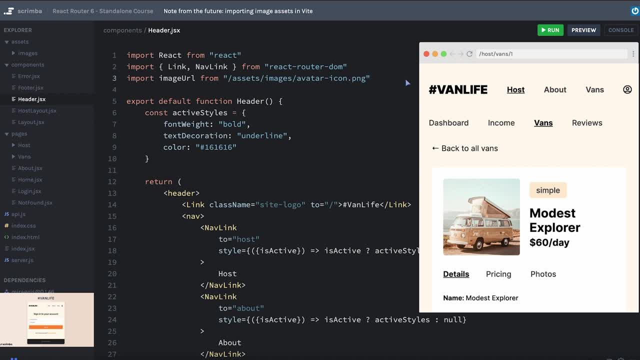 course, this is different than what you might be used to seeing, because we're used to importing javascript functions and components and everything like that. here we're importing from an npm package and elsewhere we're importing from our own javascript or jsx files. but just know, under the hood, veet is able to handle this and apparently i didn't know this until recently. 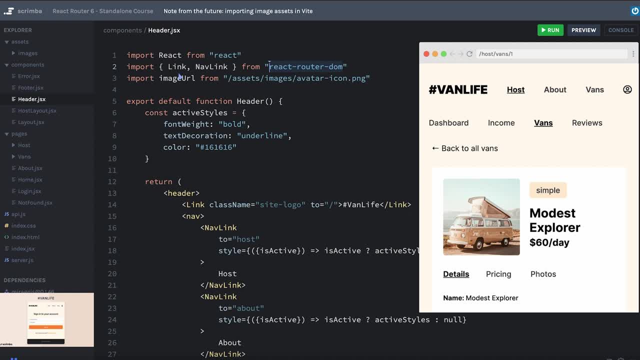 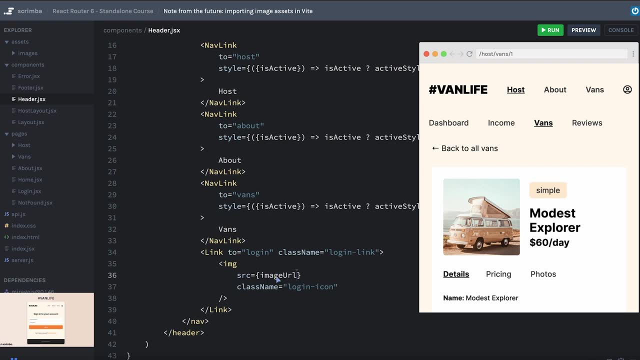 but apparently scrimba is also able to handle this internally. so if i just take this image url, i can now use this as my source and that way, when it gets bundled, it will just have the correct path, file name and everything, so that it works just fine. so, even though we're still in this nested 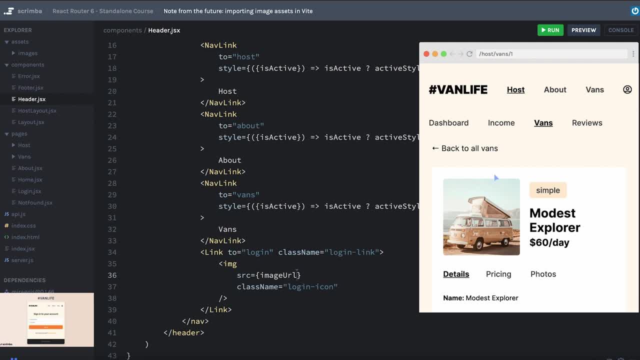 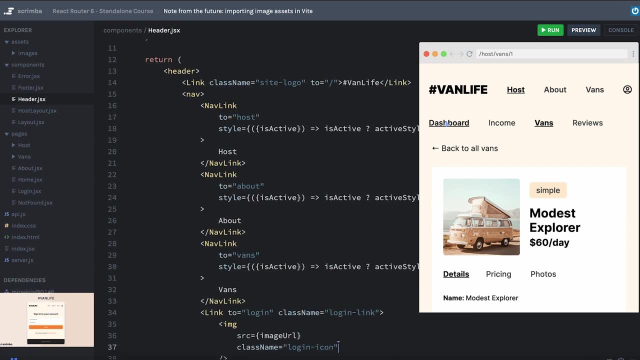 path, i can hit refresh and my avatar is still showing up. so if you are following along locally, then please just do it this way. ignore the silly way that i had it before and excuse any times in the remainder of this course that you see the little broken image icon up there. doesn't happen. 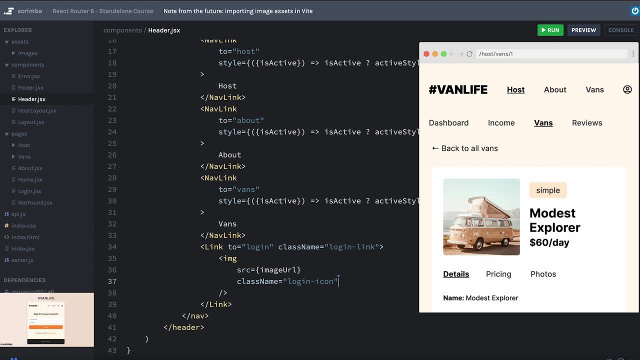 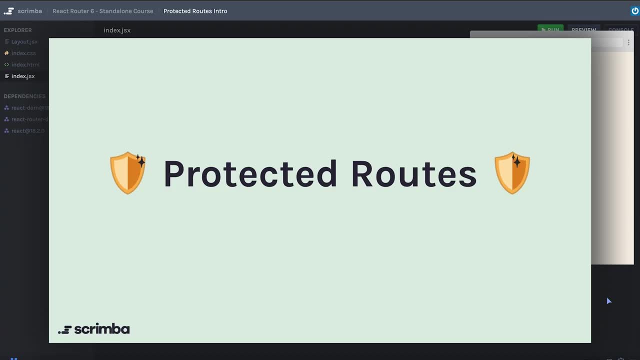 terribly often, but it does happen sometimes. okay, let's keep forging ahead. it's time for us to venture into a topic that is often called protected routes. as a pretty important caveat to this section, it's important to know that protected routes is not really a specifically created api that exists. 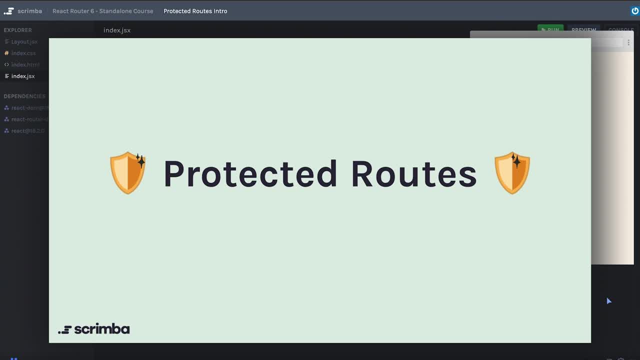 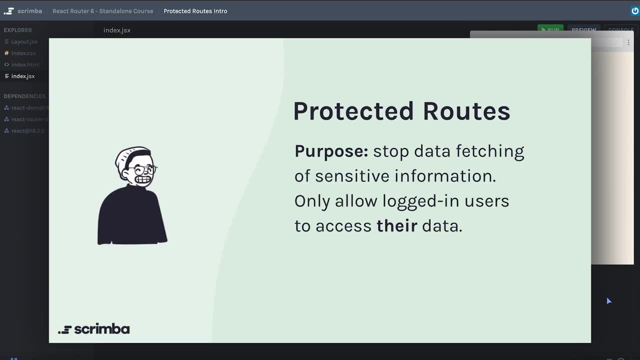 in react router, but rather it's a paradigm or a pattern that you can use in order to protect certain routes. so what do i mean by protected routes? well, the purpose of protected routes is to stop data fetching of sensitive information, so that only logged in users can access their data. 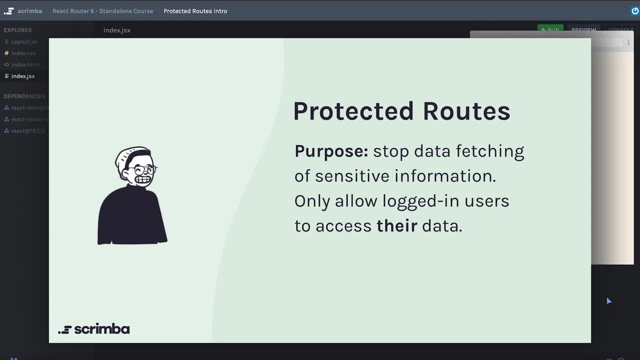 and maybe on top of that, they'll be able to access the data that they're using and maybe, on top of that, that users can't access other people's data In any given website. there's going to be information that you want publicly available, And then there's going to be user specific data, which oftentimes 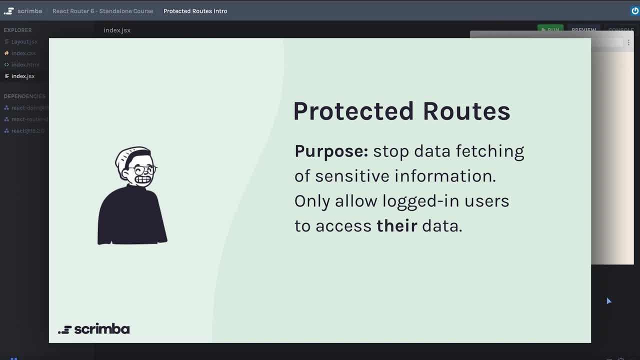 needs to be protected through some kind of authentication. the user needs to be logged in to see that data. Now, at this point we're at kind of an interesting fork in this course, because we have transitioned to using a data router And we've already started implementing loaders in our 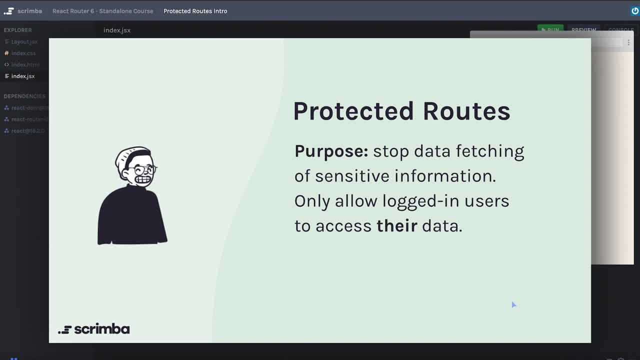 vanlife app. However, I think it's going to be useful to see how this issue of creating protected routes is solved, both with a data router, like we're using, but also, in a more traditional sense, when using the older routers that existed before. React router introduced the data routers in version 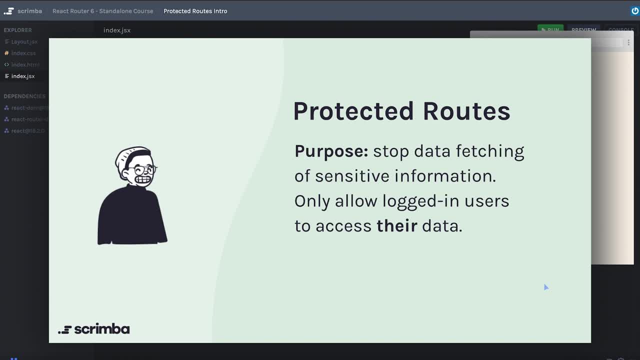 6.4.. Unfortunately, the approach to creating protected routes is very different between the two, And so I think it's going to be helpful for us to see how we can do it not using a data router first and then, and then we're going to see how we can use it with data routers. We won't dive very deep into the non. 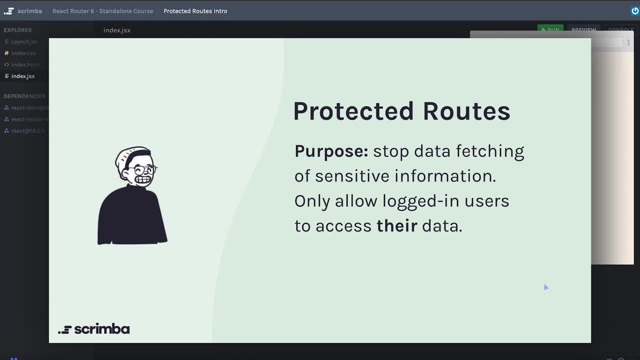 data router version only, because it won't apply to us throughout the rest of this course with our van life app. And then, naturally, we will dive a bit deeper in how we can create protected routes using the data routers, In order to help us understand why the approaches are so different. 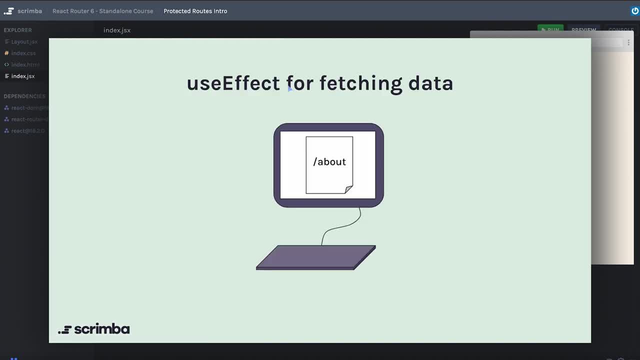 we need to remember what is happening when we're fetching our data. If we're using a use effect in order to fetch our data, then first what happens is we transition to a new page and then the fetch request is kicked off. This means that the vans page has to take into account the fact that there's 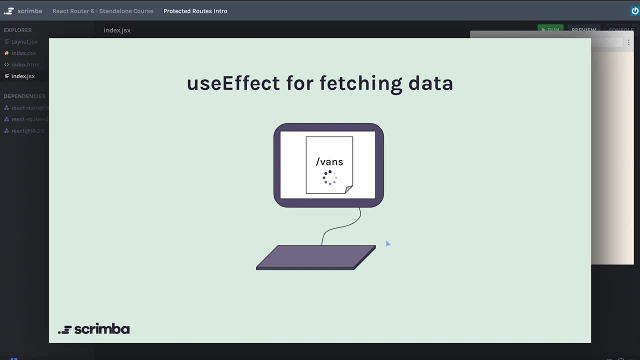 a loading state and maybe an error state in case the data doesn't come back correctly, And then, after that fetch request is completed, the JSON will get sent to this component, it will re render and then that re render will maybe set the loading state to false and it'll set the list of vans into 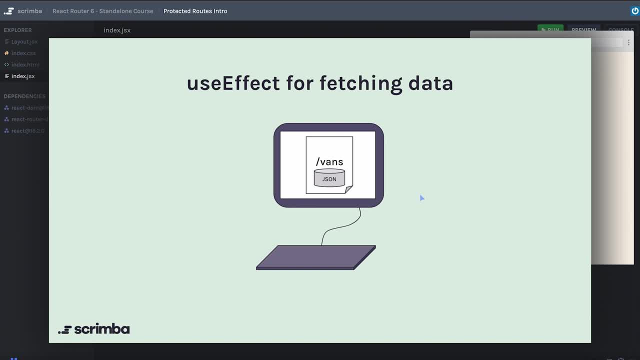 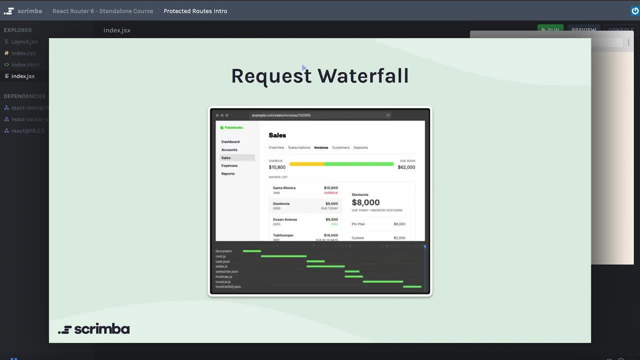 state and therefore render the list of vans In react router. when you have nested routes that are all displaying on the page at the same time, sometimes it's possible that you end up with something called a request waterfall. This screenshot comes from the remix homepage And if you click it you can go to a link there. 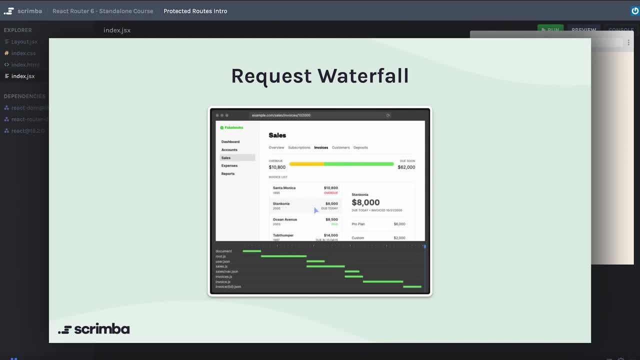 and see a much more interactive version of it that will show you side by side what a request waterfall looks like versus how remix and, by association, react router handles data fetching. But here what you can see is we have a side navigation which might have some kind of loading state And, in order for the rest of the nested route to load, 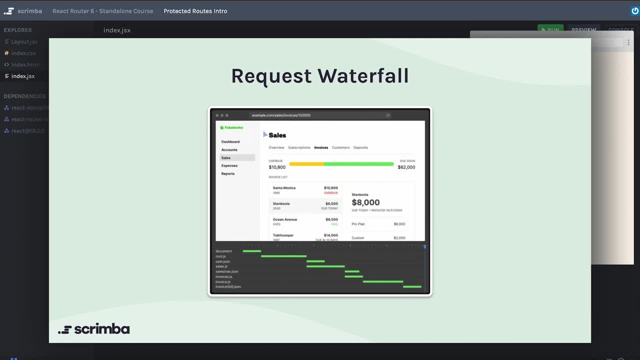 this first needs to load. then, when this part loads, or rather the sales nested route loads, then, and only then, can we start kicking off a request to get the list of invoices. Once the list of invoices loads, then, and sometimes only then, can we kick off another request in order to 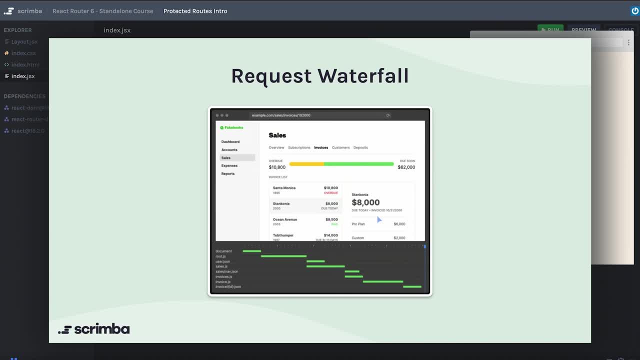 get the specific invoice that we're trying to see. So this is where the name request waterfall happens, because everything has to wait for the previous one to finish in order for the next one to start. So I'm not necessarily saying our van life app is set up exactly this way. 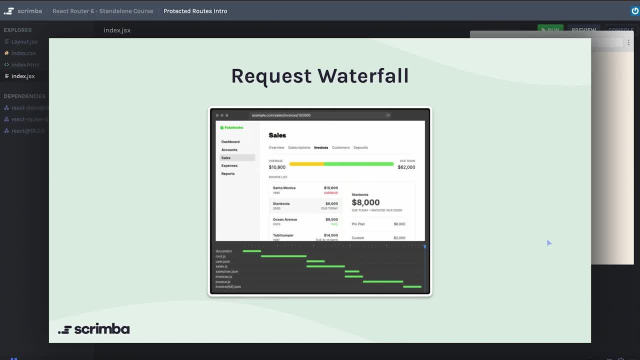 we're using some workarounds to kicking off this many requests, But it's just important to know that this is not an uncommon thing in react apps. So when we have a series of protected routes or routes that we only want a logged in user to, 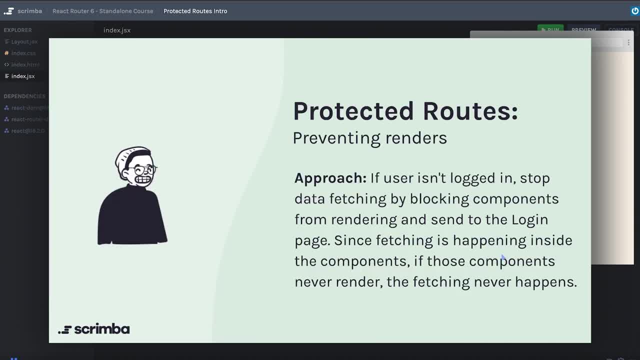 access. in the more traditional setup for react router, a very common approach to creating protected routes is to prevent renders from happening of those protected routes or those components that have sensitive information. So if the user isn't logged in, then we stop the data fetching by just blocking those components from rendering in the first place. 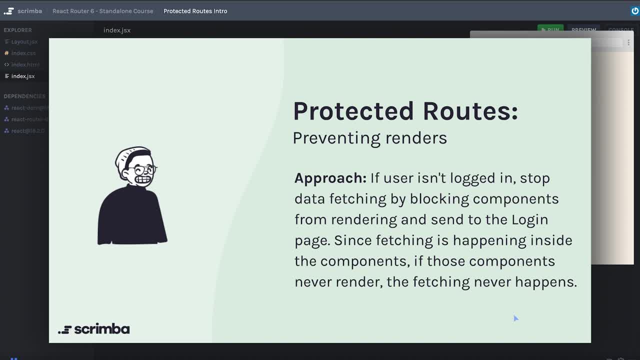 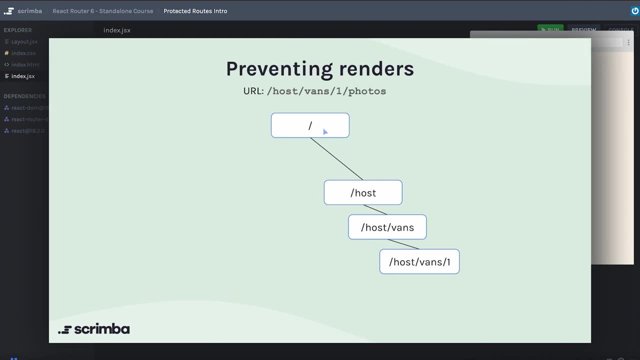 and instead send the user or navigate the user to the login page. And since that fetching is happening after the components are rendered to the page inside of a use effect, for example, if those components are prevented from rendering in the first place, then the fetching will never happen. This might look something like this: 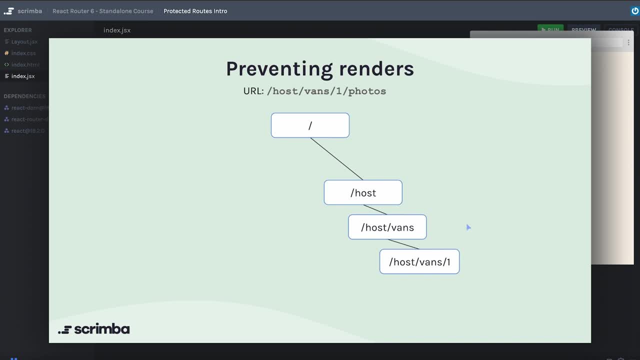 you have your homepage and then you have a series of protected routes. we only want users to get to the host page or any of the nested routes under the host page if they're logged in. So what this looks like is we can introduce an auth required layout route, maybe to be clear. 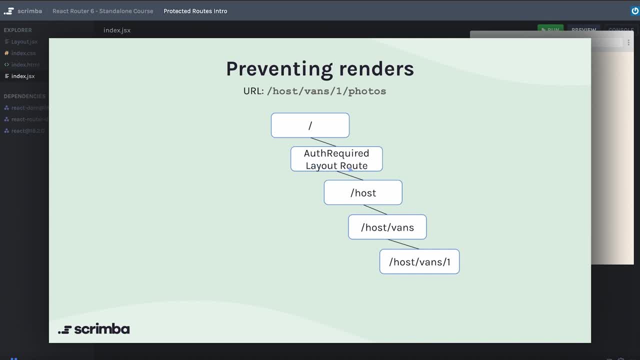 auth required is just an arbitrary name that I came up with, But it is a layout route that wraps all of the protected routes And the job of that auth required layout route is to check if the user is currently logged in. If the user is logged in, then it will allow the nested route. 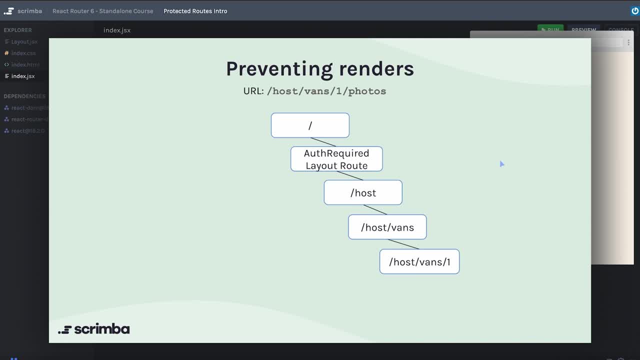 components to render to the page And therefore they are then allowed to trigger any kind of fetch requests that they might be doing. However, if the user is not logged in, then it's just not going to render those and instead it's going to navigate them to the login route. So, for the sake, 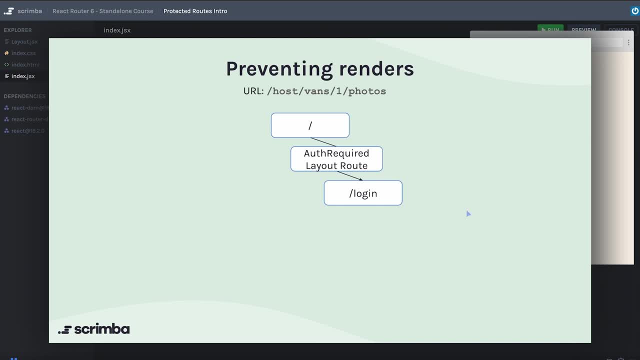 of completeness, we are going to take a look at what this approach might look like in the code, But then we're going to talk about why this doesn't work for us when we're using loaders inside of a data router with react router. So in the next scrim. 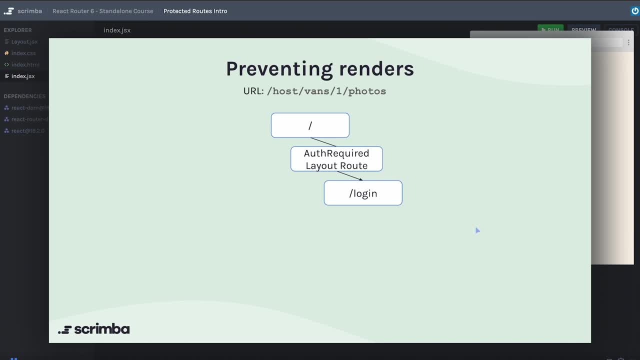 we'll take a quick look at how we might implement this auth required layout route. Let's see one way that we could implement this auth required layout route in order to protect any nested routes that we don't want an unauthenticated user to access. At this point, you should be familiar with the concept of a layout route. Here we can see that. 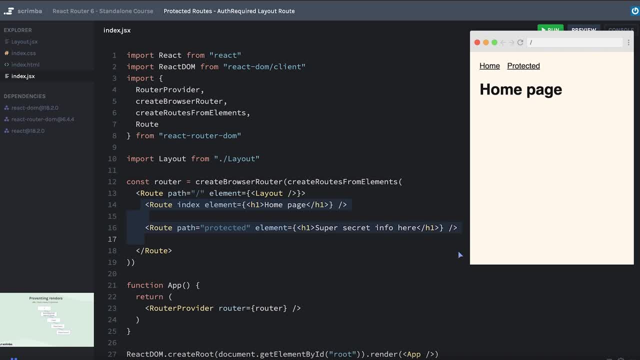 we have one route that is wrapping all of the other routes in our really simple app here that only has two routes, a home and a protected route, And, as you know, the job of this layout route, for example, is just to create some shared user interface that will be consistent throughout. 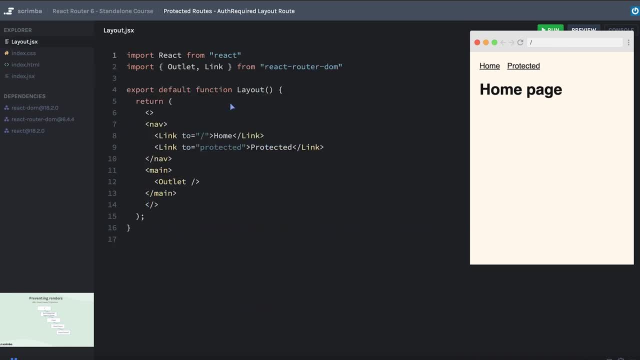 any of its children routes. If we go to that layout, we can see that it just has a navigation and then it's got this main tag and it wraps an outlet, And the job of the outlet, of course, is to render any children routes that match the current URL. And while this is how we have been, using layout routes. so far, there isn't anything stopping us from doing that, So we're going to take a quick look at how we might implement this auth required layout route in order to protect any nested routes that we don't want an unauthenticated user to access And, as you know, the job of this layout. 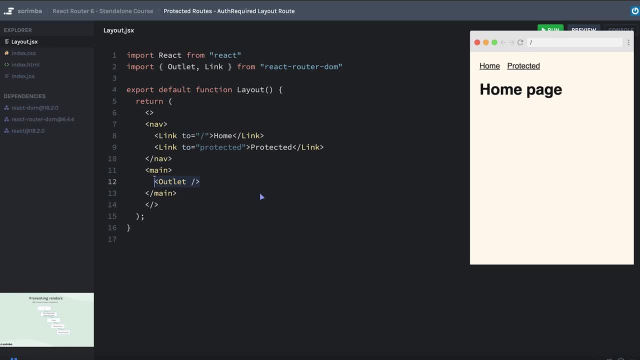 route is just to create some shared user interface that will be consistent throughout any of its children routes, And while this is how we have been using layout routes, there isn't anything stopping us from creating a layout route that can do some logic and, conditionally, either render the outlet, 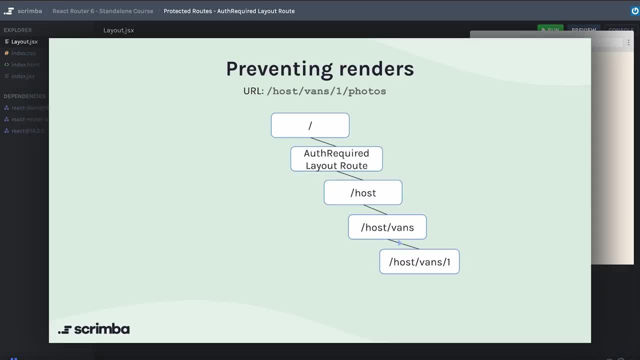 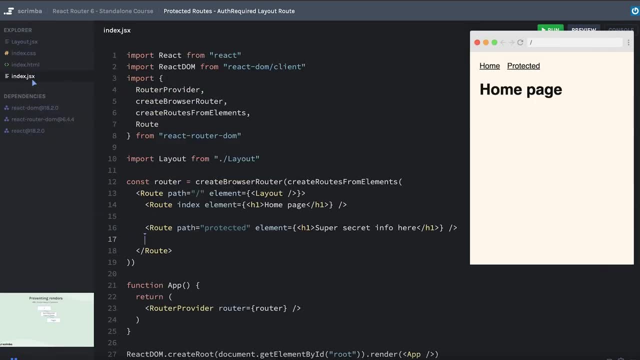 or alternatively, in the case of what we're doing here with protected routes, instead send the person or navigate the person to a different route entirely. So let me go in here and create a new component. I'm going to call it: auth required dot JSX. 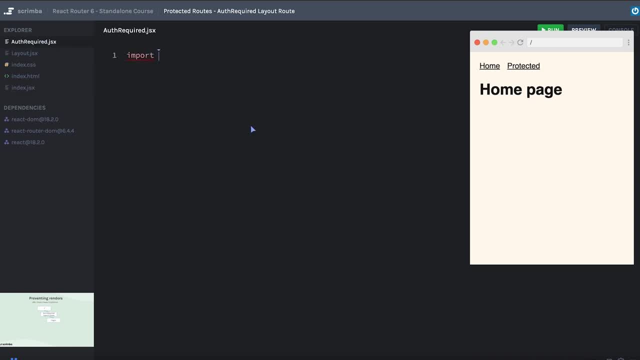 And we'll go ahead and get this initial layout component set up. Then, before we actually start working on the code inside of here, I'm going to go and actually wrap my protected route inside of this auth required layout route. So I'll need to import auth required And then we'll set that up. 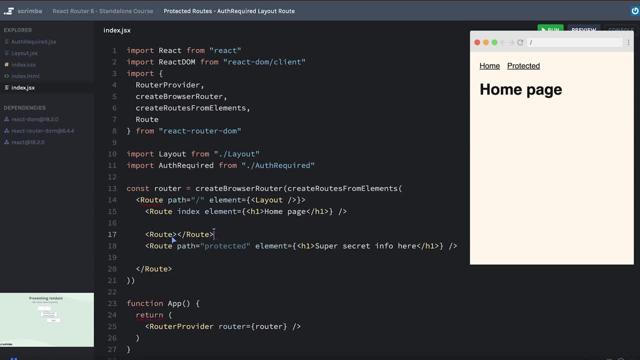 as its own route, which will be a parent of our protected route. In this case, we don't need to worry about anything dealing with a path, because all we really want is for the elements to get rendered, which will then, as we'll see, conditionally render, I think. 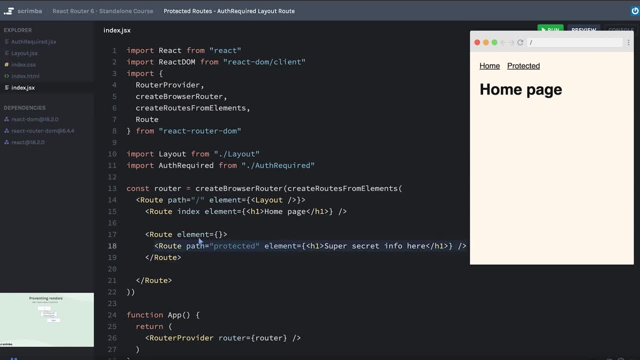 either this child route or we'll navigate the person to the login route, which we don't have a login route here, but we'll get there soon. Okay, so my elements will be the auth required component that we just created. we'll hit save. we'll see that nothing is going to show up. if I go to 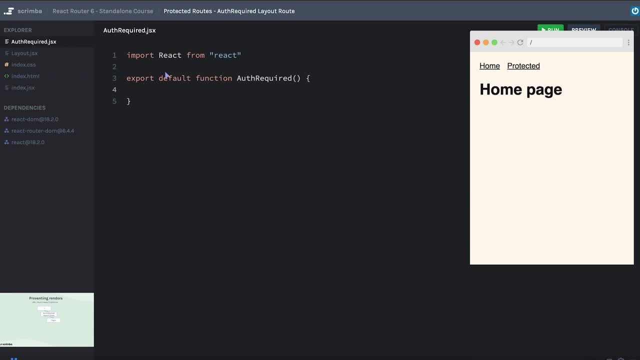 protected because I'm not rendering an outlet over there. So let's go do some more work over here. We'll import the outlet component from react router DOM And then, just for the sake of taking things one step at a time, we'll just go ahead and immediately return this outlet, Of course. 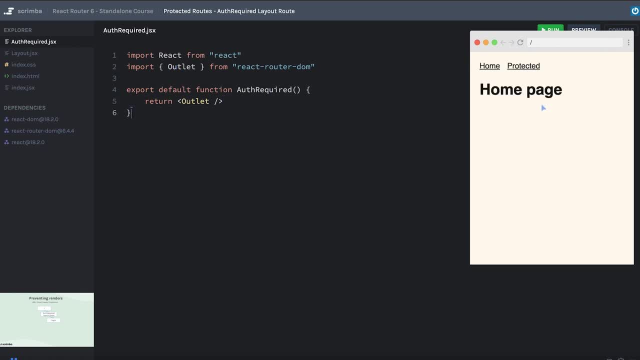 this means that this auth required is not performing any kind of work or creating any kind of benefit. But now I can go to protected and I can see my protected route component here again. One thing I think could be helpful at this point is to just start making a few comments. 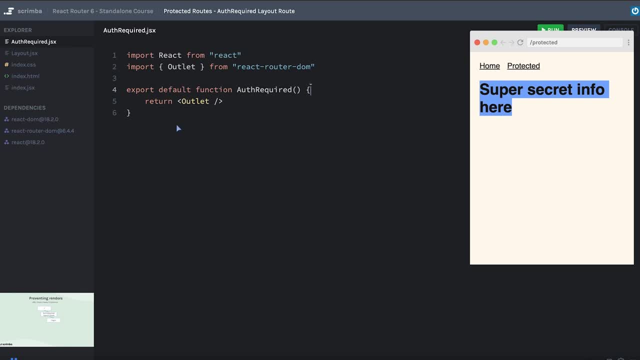 as to how we're going to implement this auth required protected routes component, Because at this point we don't have any real authentication setup. we're going to sort of fake our authentication. So we'll say: first we're going to fake our authentication, that'll make more. 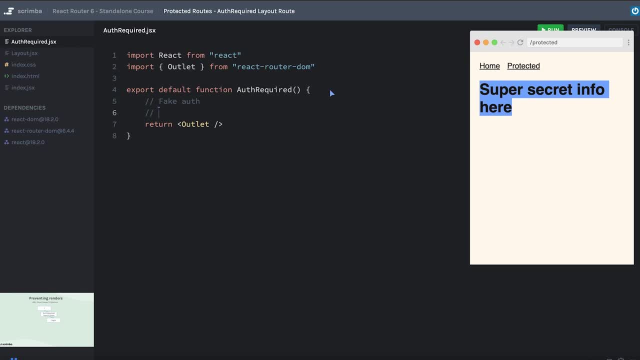 sense in just a minute. And then we're just going to have some simple logic. we're going to say if the user is not logged in, then redirect them to the login route And otherwise we will return the outlet. So here we are doing a check to see if the users logged in And if they 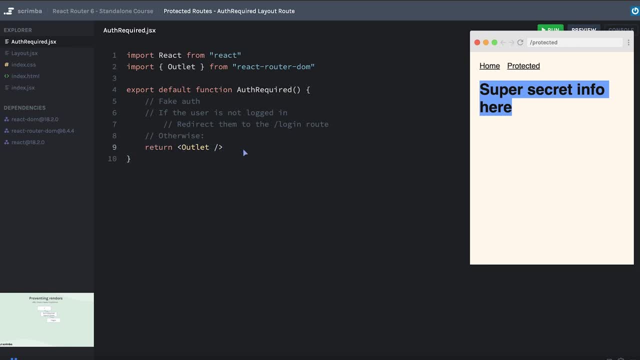 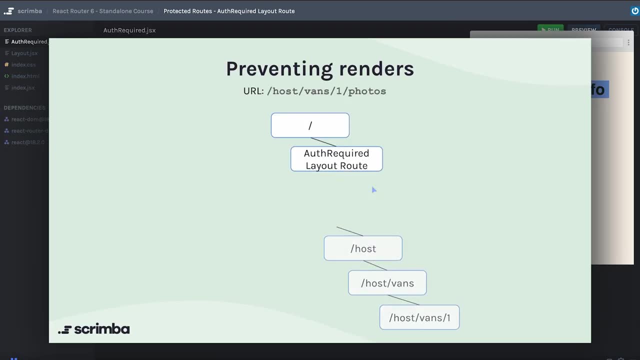 are already logged in, then we just return the outlet, as we normally would have expected, like we were doing right here And as we just saw in the comments. if they're not, then we'll simply redirect them to the login page, like we show here. Now we've already covered quite a bit. 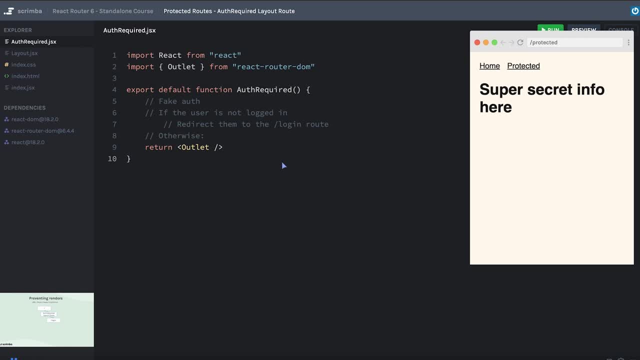 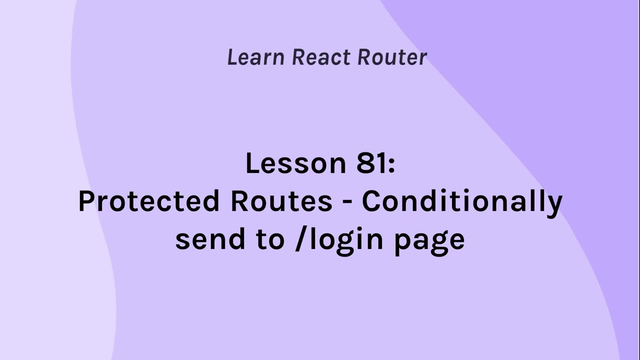 of ground in this scrim. So if you feel like playing around in the code, you're more than welcome to, and when you feel ready, we'll move on to the next lesson, where we will actually implement some of this logic. You might be asking yourself. 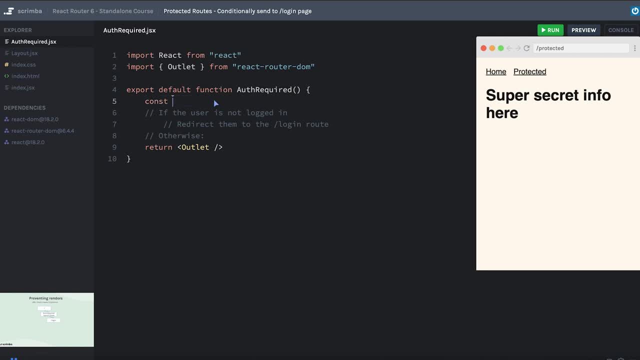 how are we going to fake authentication? Well, I'm going to take the shortest shortcut we can and say: is logged in is true, Because this isn't a course about authentication specifically in one form or another. we're going to be faking our authentication, kind of similar to this, So I hope that's not too. 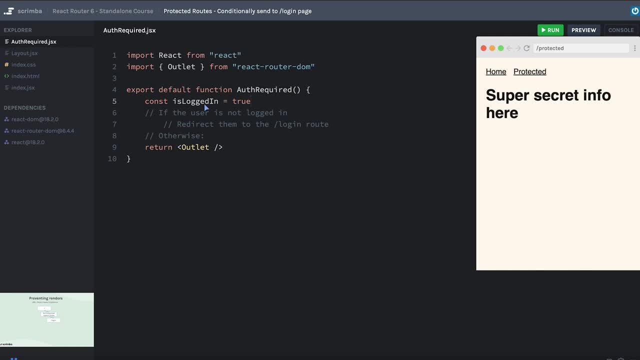 terribly disappointing, But it should help keep our focus on react router and how to build something in react router, like when we're creating protected routes. Okay, and then, simply enough, with the rest of this logic, we can just use a conditional and say if the user is not logged in. 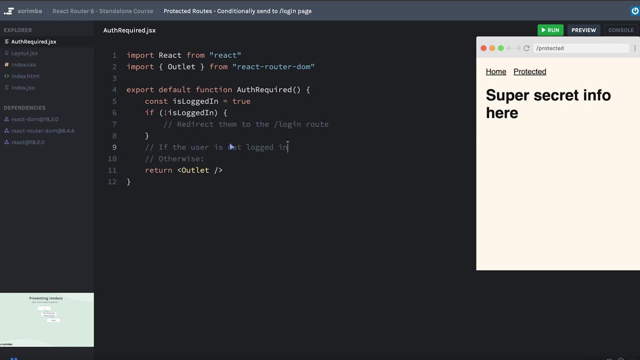 then I'll go ahead and move this up here And we can just get rid of this. I could have an else and say return outlet, But because we are going to return something from within our if I can just consider that an early return and then I don't actually need my else, because if I'm returning in 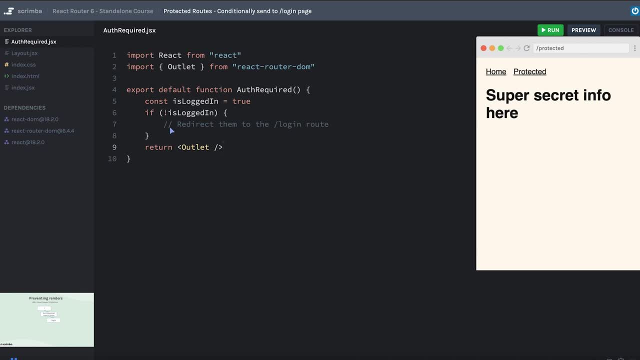 here, then this return will never get run. Okay, so how are we going to redirect the user somewhere without any kind of interaction on their part? Well, you should already be familiar with the link component, the idea of a link component. So, for instance, if we want to log in, we want to log in. 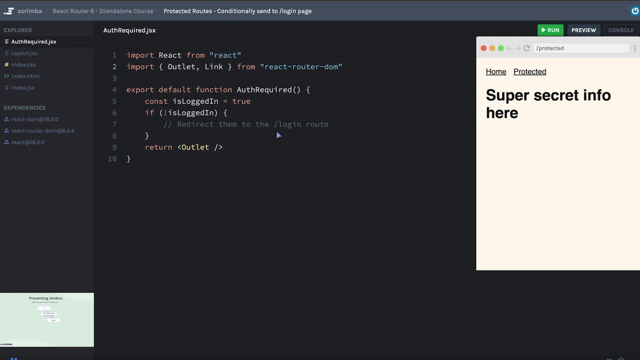 The idea of the link component is that when you render a link and the user clicks it, then it sends them to another route in React Router. Well, React Router also has a bit more of a forceful version of that which is called Navigate. 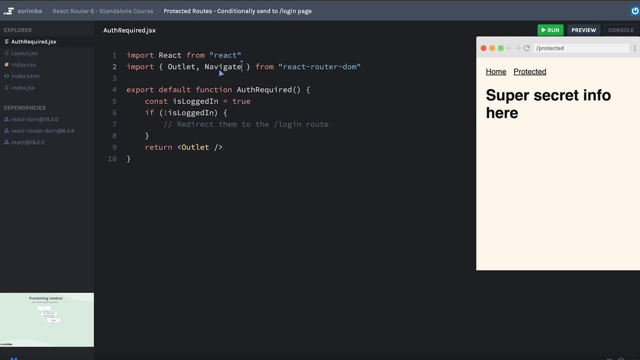 And it is a component, And if the Navigate component ever gets rendered by React, then it will immediately and automatically send the person to a new route that you specify in the Navigate component. Simply enough, I can just say I'm going to return an instance of the Navigate component. 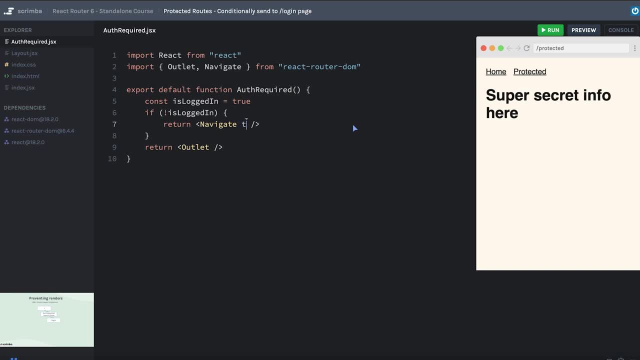 And, just like with link, there's a prop called to. there's also a prop called to in Navigate, So I can say: Navigate to slash login. Now, remember, we don't have a login route registered in our router quite yet, but we can still test this. 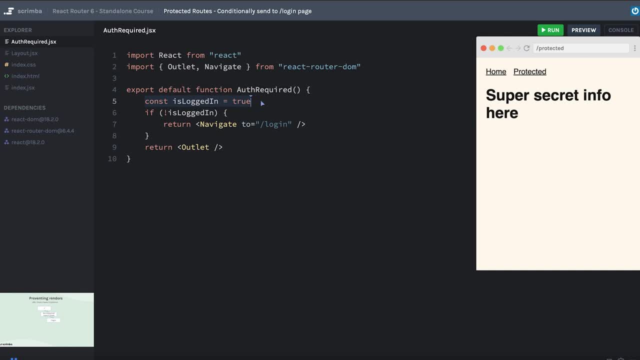 So I'll hit save. Remember I've hardcoded that my authentication is currently set to true or my is logged in. variable is set to true, And so I'm able to get to my protected route. Just fine, Let's go home. We'll change this to false. 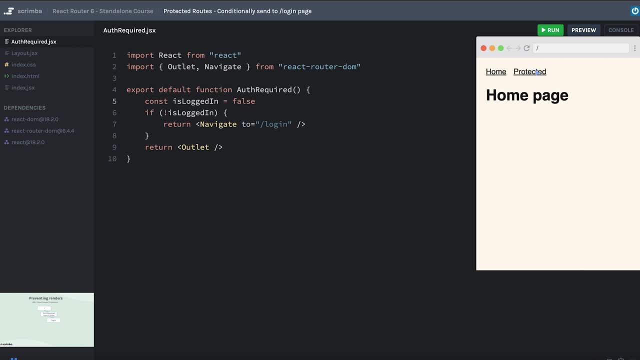 I'll hit refresh and try to go to protected and we'll see what happens. And okay, this is great, Although we don't have a login page And so we get this 404 not found. But the point is it sent us to the login page. 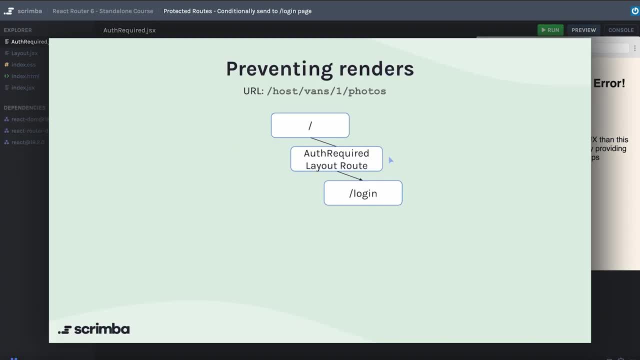 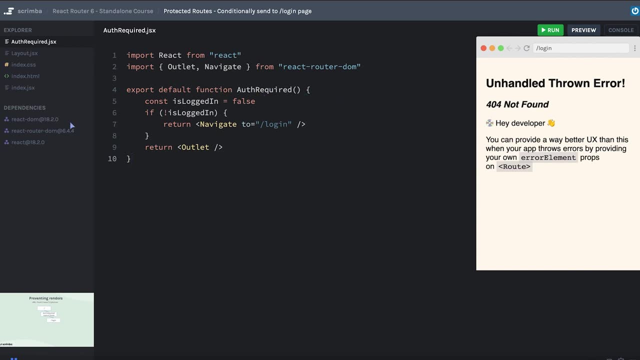 Remember, the approach we're taking is to prevent renders entirely of the protected routes And that's exactly what our auth required component has done here, Because it's wrapped as a parent component, or rather a parent route to our or children routes that are protected. 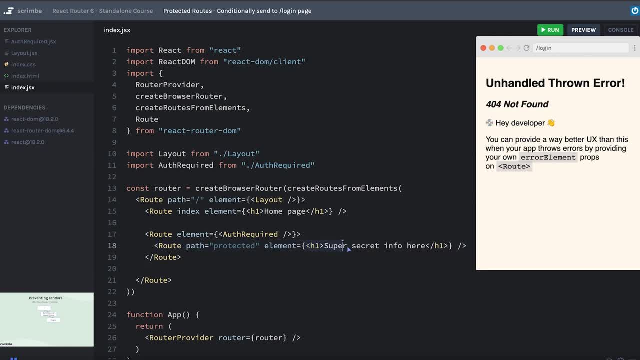 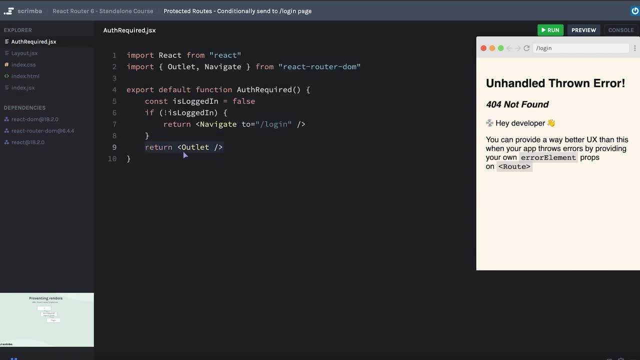 it intercepted the rendering of this route, or rather this h1 here. it's not really even its own component, And before it ever allowed that to be rendered by returning this outlet, it instead sent us to the login page By doing this. 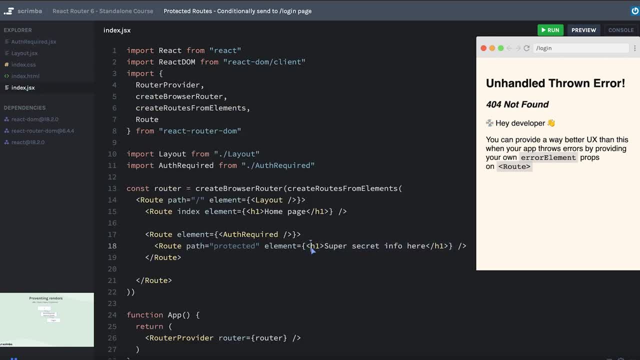 if we did have some sensitive information that was living inside of this component against just an h1, but imagine that this is a component that's doing some kind of fetch request to some sensitive information. by stopping this from ever getting rendered, it's not going to kick off that fetch request. 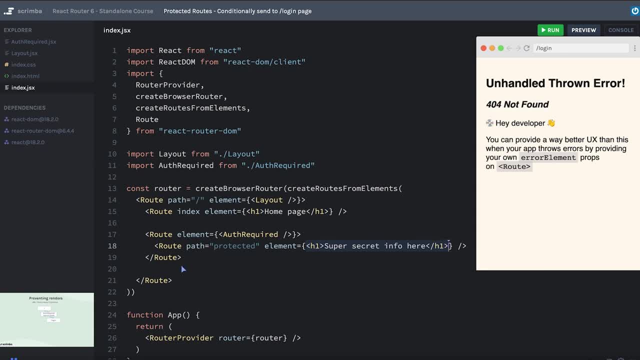 Now, before we move on, it's, I think, important to remember that this is the approach that you would use if you were not using the features that come with the data layer API's and the data routers. Technically, we're using a data router because we're using this, create browser router function. 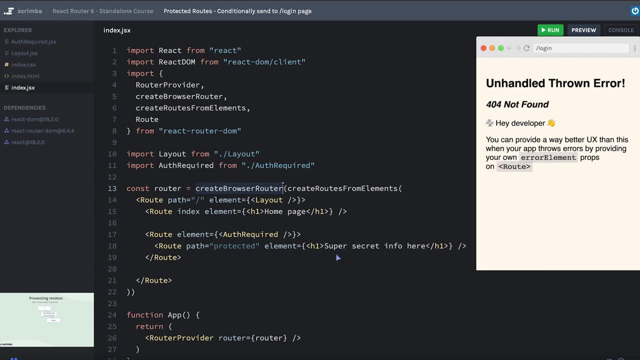 but we're not using any loaders here, And the fact that we're not using any loaders means that it's okay for us to do it this way. However, once you introduce using loaders inside of any protected routes, then then everything kind of changes. 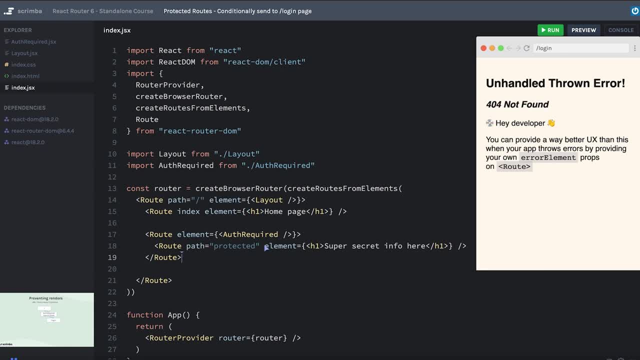 So, as I mentioned, this is about as far down this path as we're going to go. I think it's really important to see this because, at least at the time of recording, this is the most common way that you will see people accomplishing protected routes. 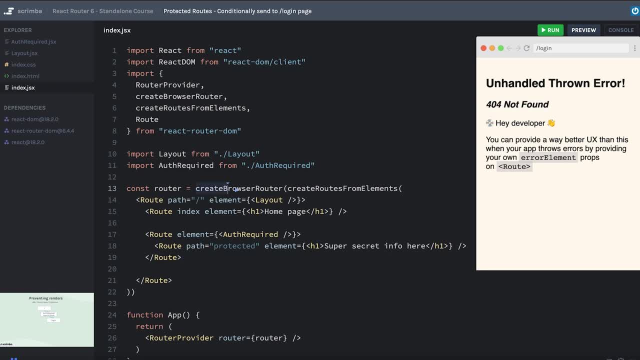 And that's only because most of them are not using these data routers quite yet. However, for us, we are going to jump into the future and actually use loaders and see how we can accomplish protected routes when we're using loaders. It's that time again. 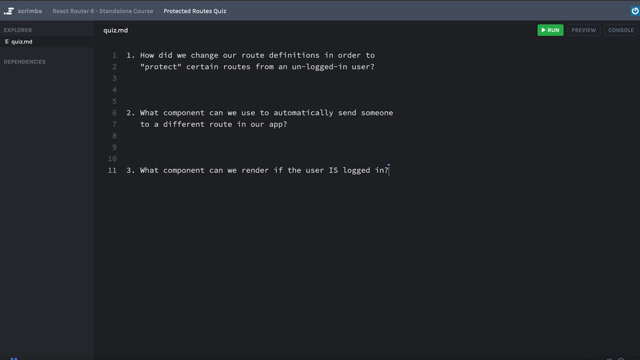 let's run through a quick quiz that deals with protected routes. Like before, I want you to actually click into the lesson here and type down your answers, And when you're done you can hit play and we'll go through the answers together. 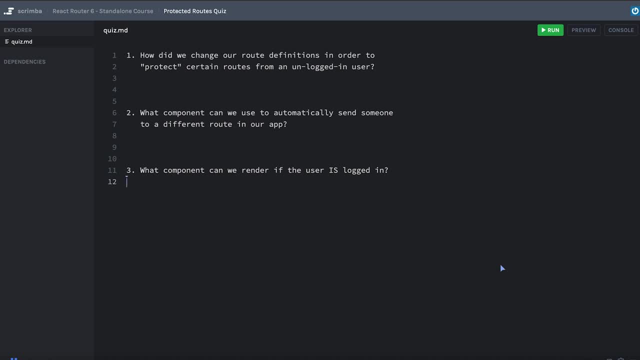 So pause now and work on the quiz. Okay. so how did we change our route definitions in order to protect certain routes from an unlogged in user? Well, the first thing we did was to to wrap all of our protected routes in a layout route that has some logic inside of it that will protect those routes. 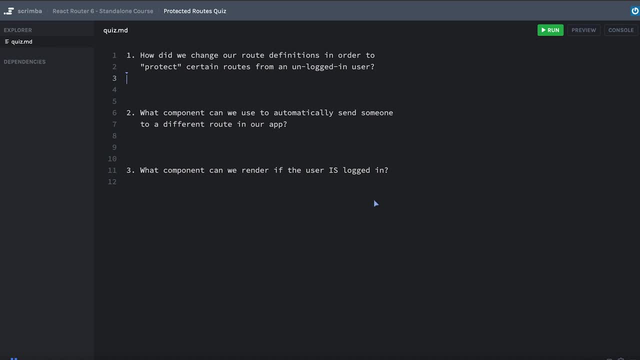 If the user is not logged in. with the next two questions we'll talk about how it actually protects those routes. But for now, for answer number one, that's good enough. I guess one thing we can be a little bit more specific about is that the way in which it protects the routes is by redirecting the user, if they are not logged in, to the login page. 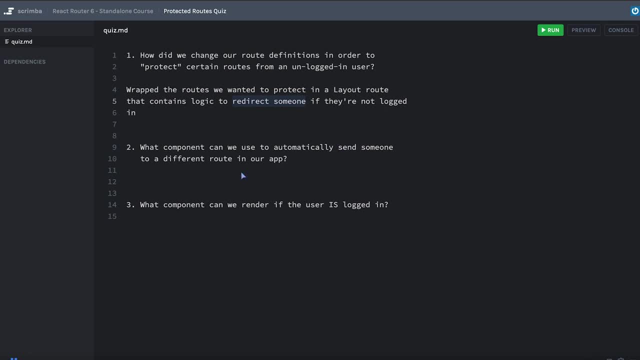 Okay, number two: what component can we use to automatically send someone to a different route In our app? Well, that would be the navigate component. If the navigate component renders at any time, it will automatically forward them to the location or the path that we specify in the two prop. 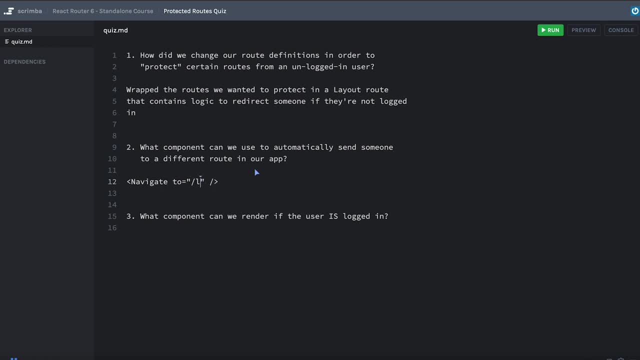 So I can say: navigate to slash login, for example. Okay, and lastly, what component can we render if the user is logged in? Well, if they're not logged in, we will render the navigate component, But if they are logged in, 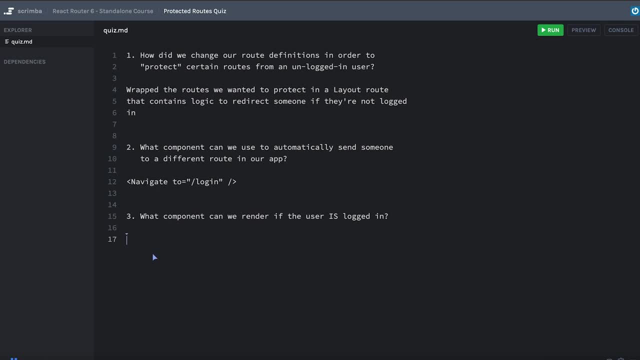 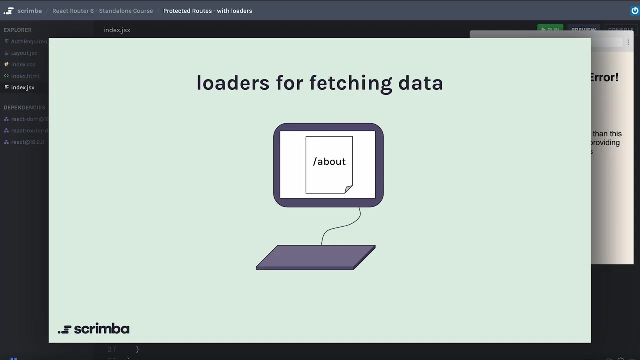 then, because we have wrapped a layout route around our protected route, we want to use an outlet in order to render the contents of the route that they're trying to reach. Okay, short and sweet, Let's keep moving forward. Okay, so let's start seeing how we can include protected routes when we're using these new features with the data layer, API's, loaders and actions and so forth. 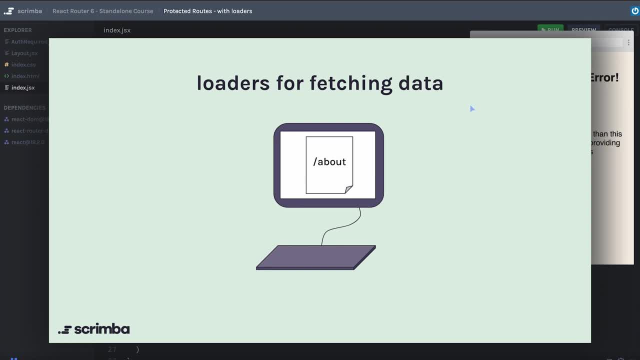 As a reminder, if you're using a loader for fetching data, the fetching actually happens before the route transition And before the target Component. the next component that you're trying to route to actually renders to the page. This means if you were on the about page and you wanted to go to the vans page, 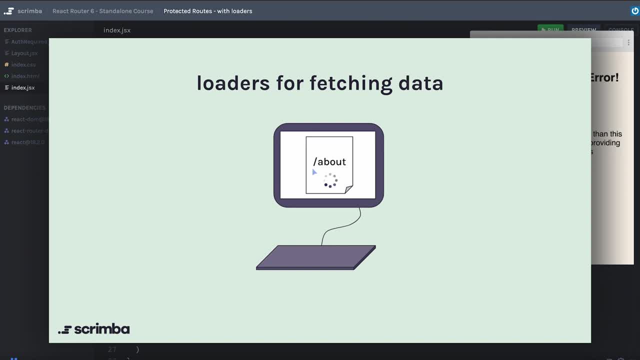 when you click the link to the vans page, it's going to kick off the fetch request from the loader of the vans page first, before it ever transitions or renders the vans page. It gets the data and it includes it immediately inside of the vans page. 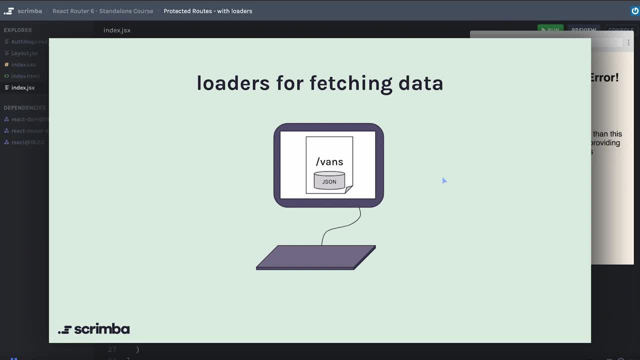 A major benefit of this is that we don't need to check for the loading state, because this component will, Okay, only ever be rendered to the page if the loading is complete and there are no errors, which also means that we don't have to necessarily check for the error state. 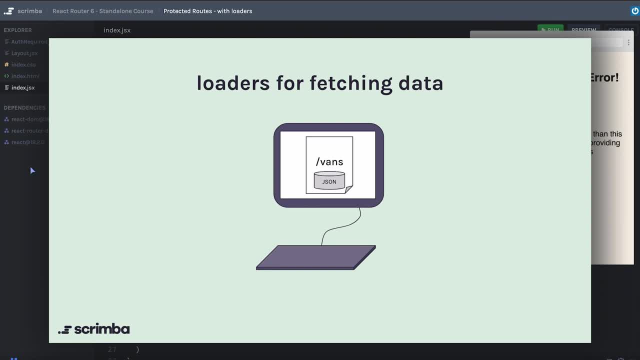 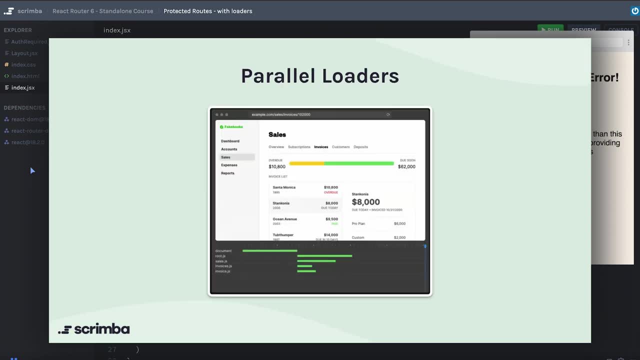 We can handle that in a more declarative way inside of our route definitions. We saw the diagram from the remix website of a request waterfall And if you went to the website to look at that diagram, you would have also seen what it looks like to load things in parallel. 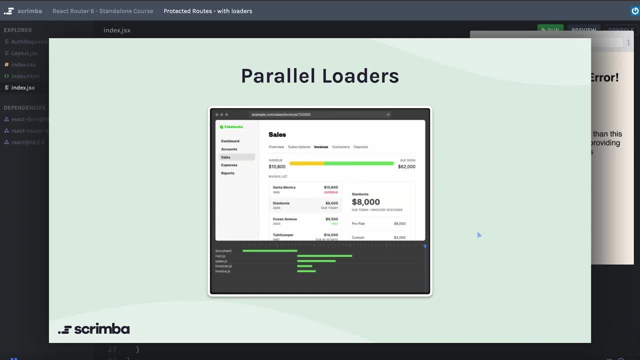 Another benefit of having these requests available to the data router before the routes even load is they Know how to run your fetch requests before ever transitioning to that route. So in remix, which is what this diagram on the website is actually referring to, 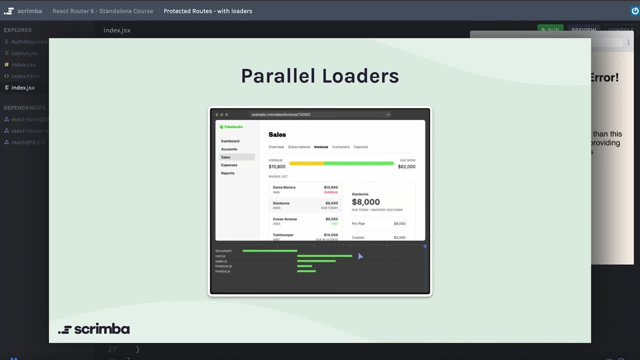 but also in react router when you're using loaders. if you have some nested route that you're trying to reach, all of those fetch requests can happen simultaneously. In other words, all of the loaders that are required for your current route to display correctly are run in parallel. 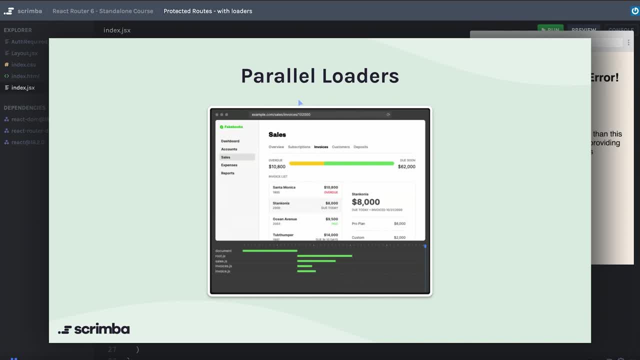 They don't run one after the other, but instead they all can run at the same time, And then, whenever the final one of the loaders finishes, the entire completed page can render to your screen. So I want to preface this by saying this is something that oftentimes leads to faster loading and arguably will also improve the user experience in the end. 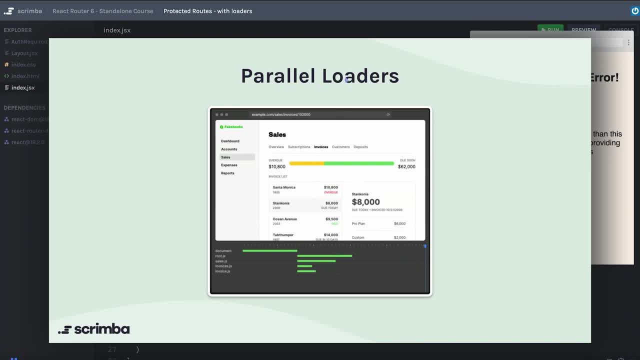 So the reason I preface all of this is to make it known that because all of the loaders for all of your routes will run as soon as you start the transition to that route, it means that we can't put a layout route to wrap our routes and stop the fetch requests from running, because they all just 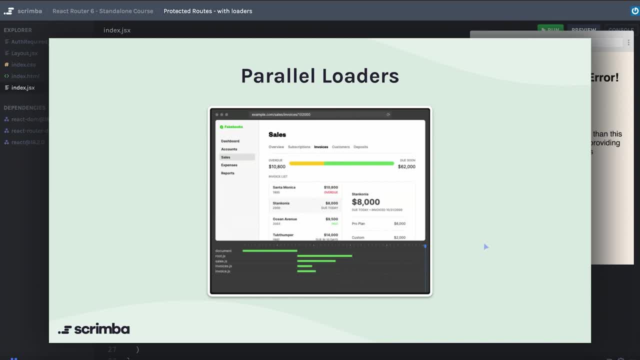 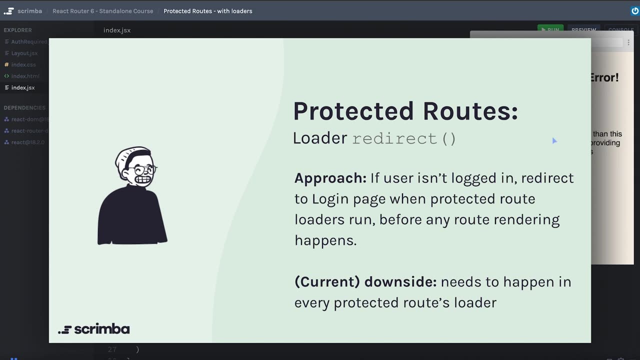 start running, even before it transitions to that component. we no longer can try to prevent the components from rendering, because the fetch requests are happening before the opponent is rendering anyway. So that means we need a slightly different approach to create protected routes when we're using loaders going to use a function that we are about to learn about called redirect, and it's going to happen inside of our loader function. 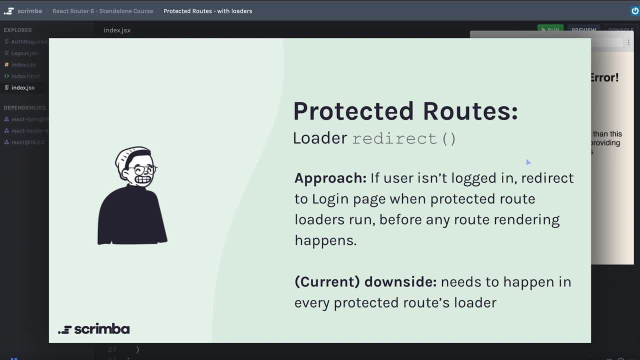 So the high level overview is: if the user is not currently logged in, then we will run this redirect function And we'll send them to the login page inside of our loaders before any route rendering happens. Now, at the time of recording this, there is a downside to this approach and that is that the check for the currently logged in user and the redirect has to happen in every single protected routes loader. 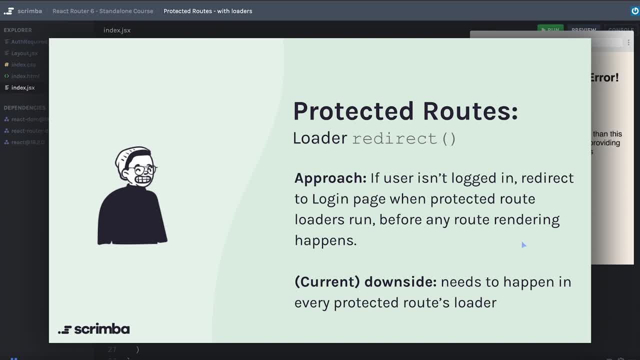 That said, there is currently a proposal out there to include something called middleware inside of react router that would allow someone to run a function before any of the loaders happen. Again, when I'm currently recording this, that is, it is not yet implemented into react router. 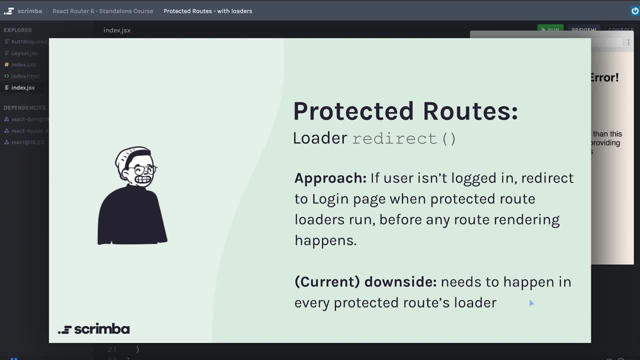 So I'm hoping in the future I can record an update that basically amends this and says: now we can use this middleware to run this check instead. But for now, we'll just have to do a little bit of extra work in order to run all of our checks inside of every loader, of every protected route. 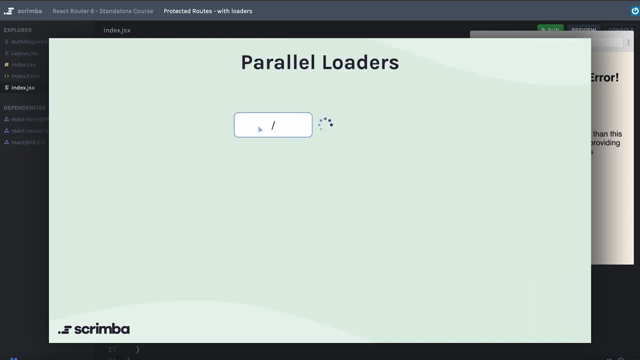 Okay, let's see a diagram of how this works. So, with parallel loaders, we might be loading something on our homepage, at which point we might go to a nested host page, and all of these are going to load at the same time, like we saw. 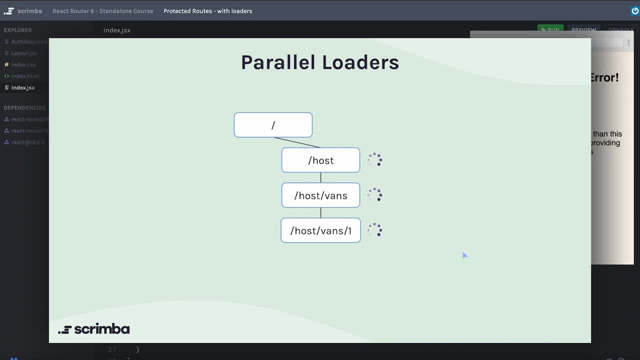 in the previous diagram, And all of these loaders are going to check if the user is currently logged in. Now one of these loaders is going to recognize that the user is not currently logged in, And so they will call this redirect function, which will cancel any loading. that's happening and it will never kick off a fetch request. 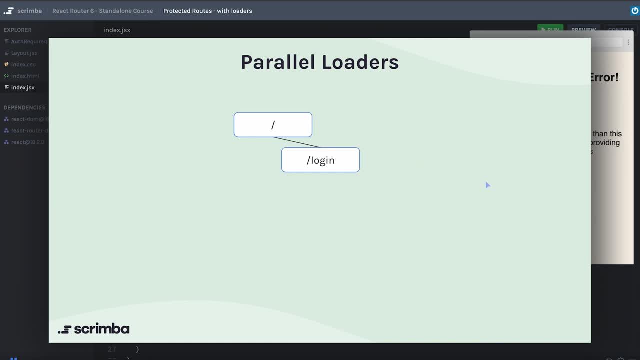 And instead it will redirect the person to the login page. This way, we still accomplish the goal of never kicking off a fetch request to protected data if the user is not logged in. By the way, the reason it's important not to even kick off this fetch request. 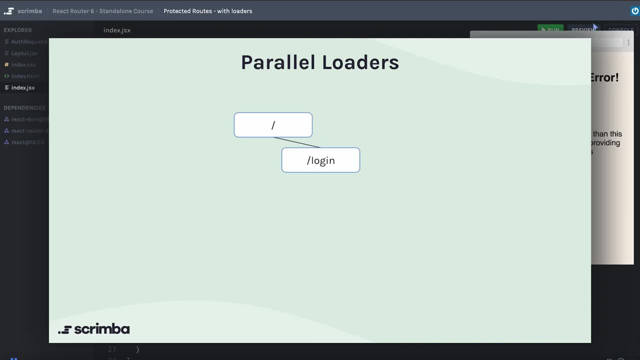 Is if we did and the data came back. if I were to go into my developer tools inside of my browser and look at the network tab, I could potentially get access to sensitive information that I'm not supposed to have access to. Okay, that's enough theory. 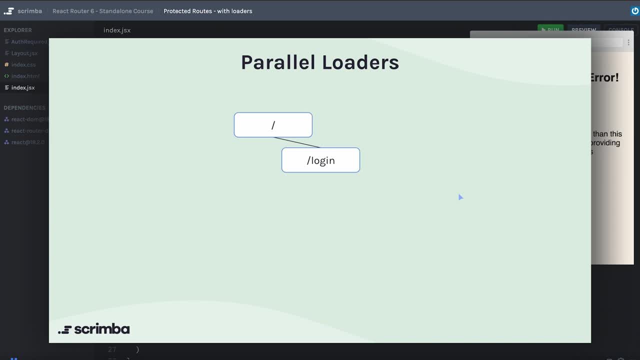 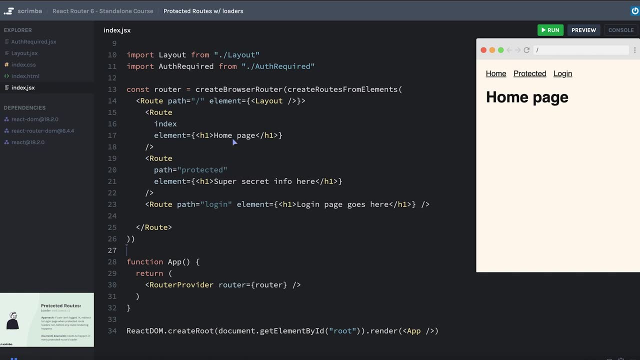 Let's actually jump into some code and see how we can implement this. You should be familiar at this point with the concept of adding a loader to our routes. Typically, we have a separate component and in that same file- Okay, That component- we can export a function called loader, and then we set a parameter or a prop on our route that's called loader and we just say this is the home loader. for example, for the sake of brevity and being able to see everything in one place, instead of having a separately defined component and a separately defined loader function, I'm just going to inline my loaders. 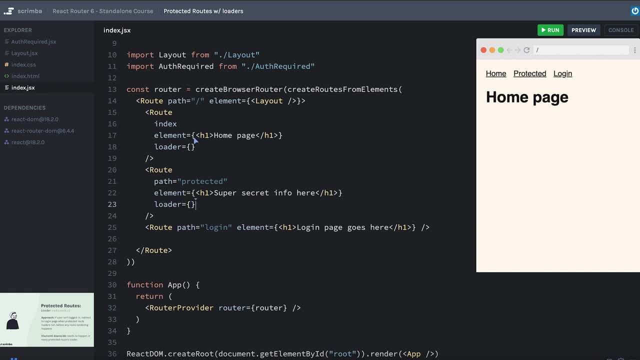 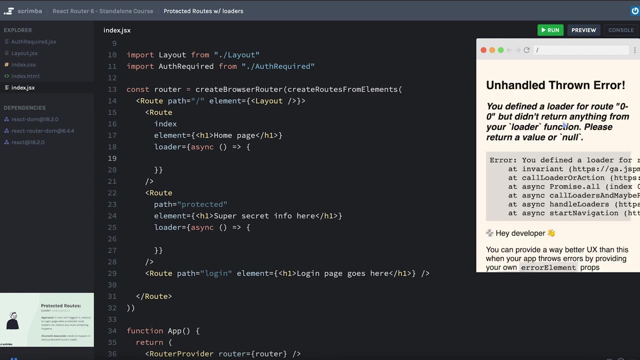 So let me create a loader here as well, And I'm just going to make these some asynchronous functions for now, And we'll just use an arrow function And open up the bodies. Now it's pretty important that you return something, or even if you return null from your loaders, because otherwise react router is going to complain. we can see here: you defined a loader, but you didn't return anything from your loader. please return a value or null. 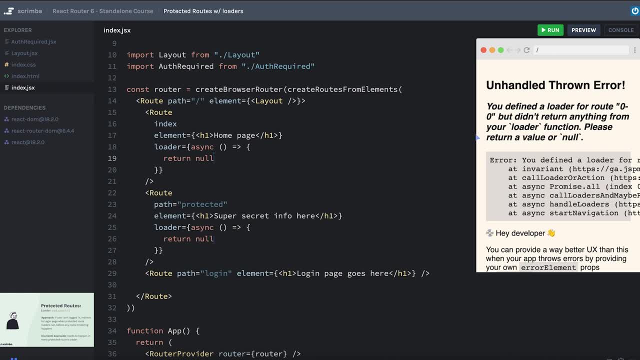 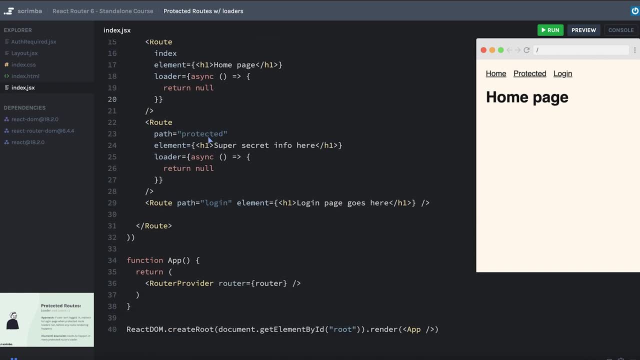 So the first thing I'm going to do here is just return null so we can get rid of that error. Suppose the homepage one isn't quite as important to us at this point, So we are going to focus on our protected route loader, similar to what we were doing in our auth required. 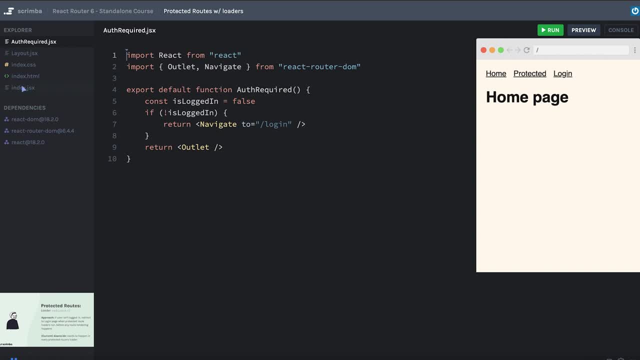 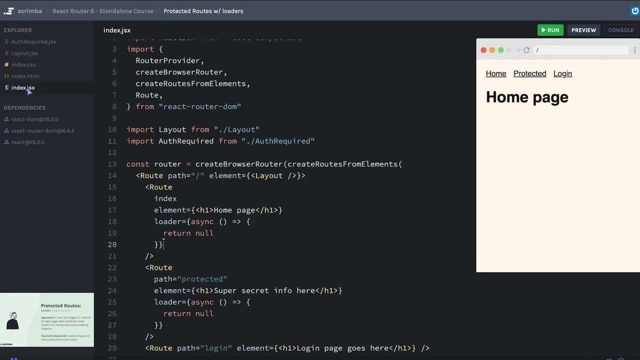 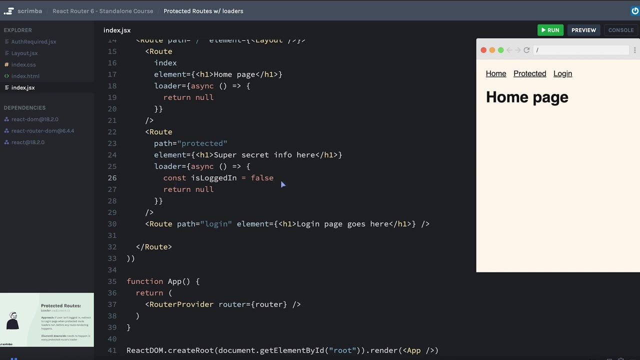 layout route which I left here just to be able to see, but you'll notice that I've removed it from our route definitions. similar to what we were doing over there: we are just going to fake our authentication And so over here I'm going to say on the top line of my loader for my protected route that const logged in equals false for now. 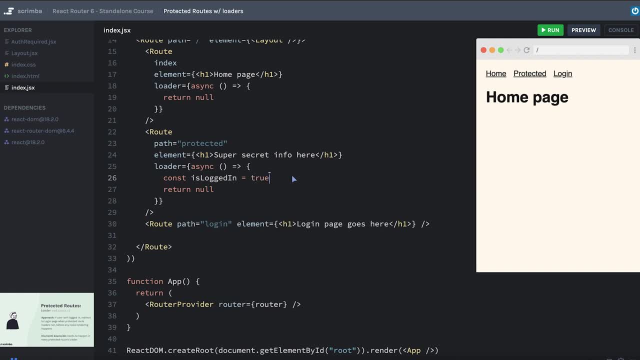 Actually, let's go ahead and start this with true, Okay, and then, similar to what we had before, I can say: if we are not logged in. if not is logged in, then what we want to do is to return that mêmes. 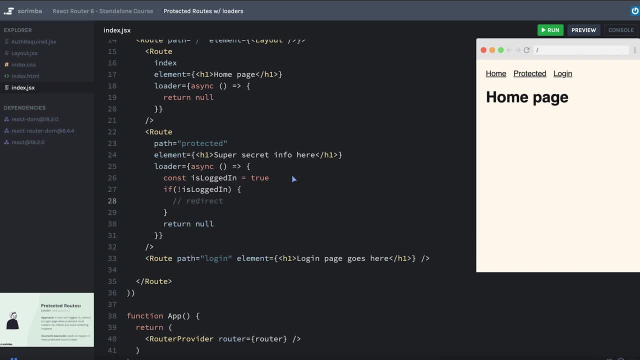 As well, And that's going to do something. So if I say, if not, I'm going to go ahead and do that, Okay, redirect to the user. So I'll just put that as a comment here Now, because this is happening. 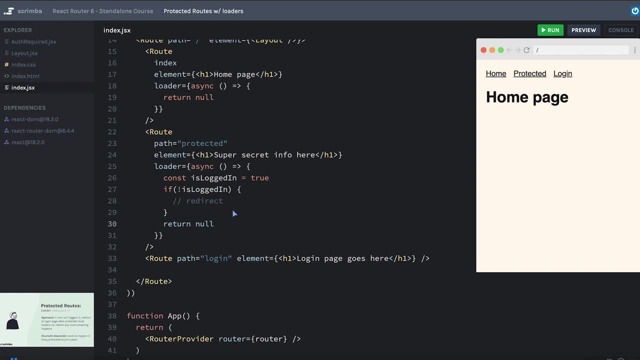 inside of a loader. I don't need to then do any kind of other redirect or anything. the loader is already the precursor to this route: loading, or rather this element being rendered to the page. Now, how do I do this redirect? Remember, right now I'm not inside of a component, I'm just 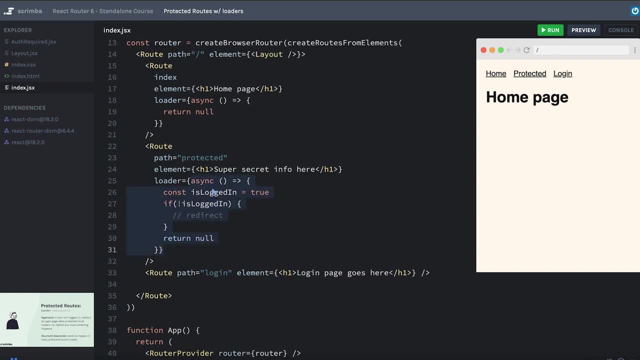 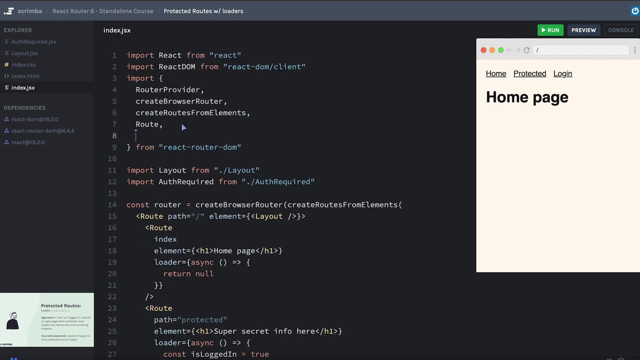 inside of a regular async function, which means I can't use the navigate component. I can't return navigate because I'm not inside of a component that is ready to render anything to the page. Because of that, React Router gives us another utility function that is called redirect, And so 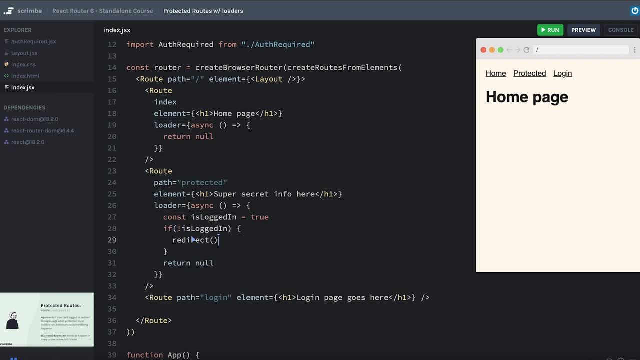 I can come down here and I can simply say we're going to redirect the user to slash login. Now, a common paradigm that I have found in my discussions with some of the core team at React Router is that many people will actually throw this redirect instead of just doing a return. 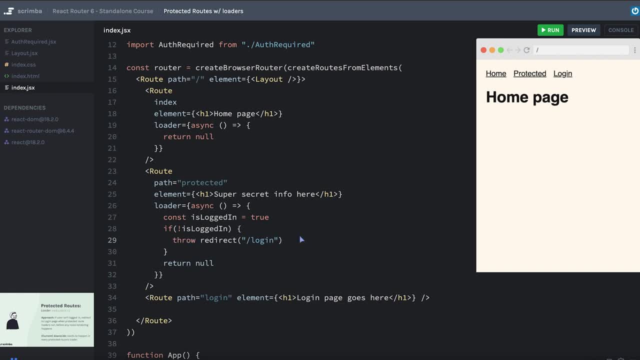 I assume Because it's kind of conceptually similar to a server that would be returning a 400 level error that says that the current user is not authenticated to access that endpoint. Either way, we're not going to see that. throwing our redirect is going to make that big of a. 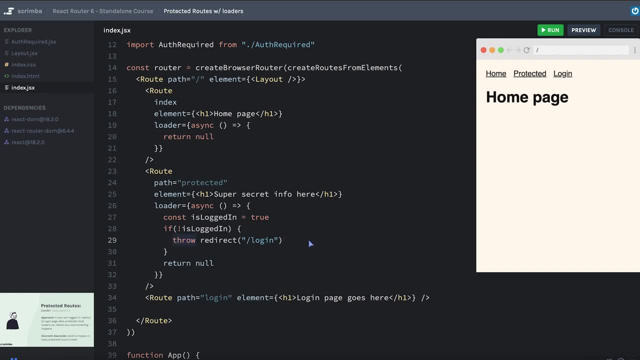 difference. So, because it appears to be convention, I'm just going to leave it there. Okay, let's see what happens. I'm going to hit save, I'm going to try to go to protected, And oh well, of course. 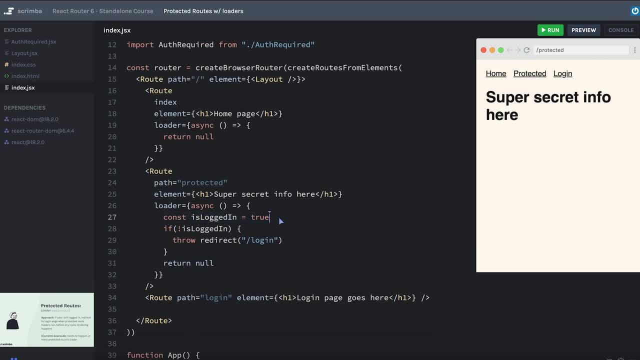 that worked because we hard coded that the user is currently logged in, So it's good to know that our protected route works. Let's go ahead and change this to false And hopefully actually let's go home first, hit refresh and I'll click protected And perfect. 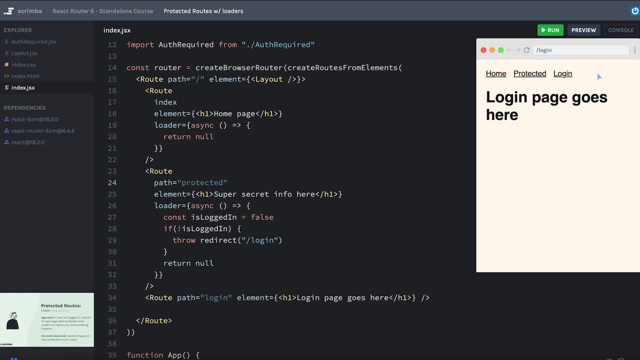 that takes us immediately to the login page. Now, I think this is pretty neat, But I want you to pause for a second and think about this. If I hit the back button, where is it going to take me? Because the loader intercepted the direction to the protected route And before that. 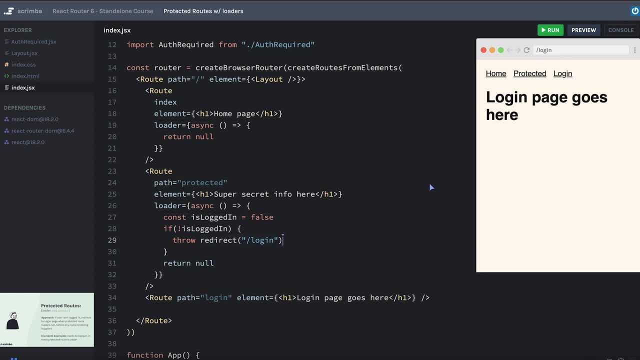 it could even render. it sent me to the login page. if I hit back, it's going to take me back to the homepage where I was before I attempted to get to the protected page. I think the benefit of this is going to be a bit more obvious when we finally get back to our van life app and start 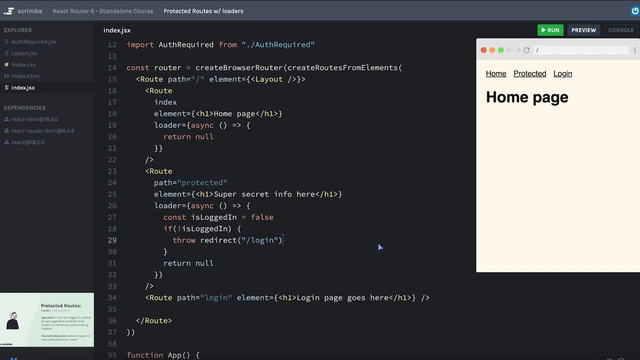 applying what we've been learning. But conceptually, I think this is pretty neat because the loader is running before the route transition ever happens. Okay, we're almost ready to jump back into van life and start implementing this. I'm excited to get your hands back on the keyboard. 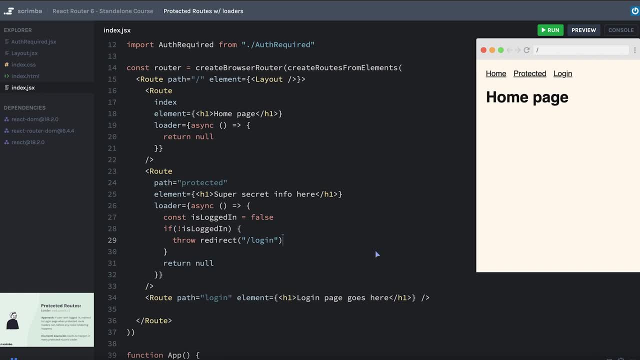 I know I've been talking for a while, but I'm going to jump back into the app and start implementing this. I'm excited to get your hands back on the keyboard. I know I've been talking for a long time. While we have this setup here, I think it would be pretty interesting to see for just a 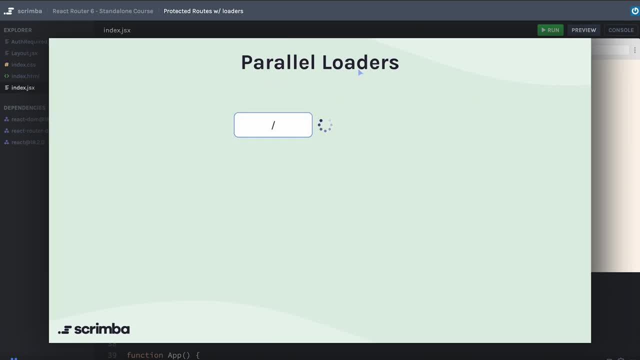 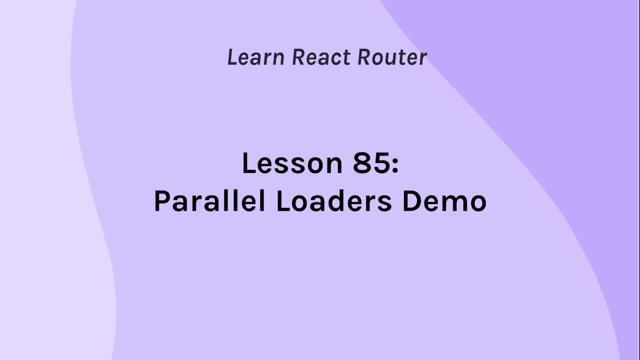 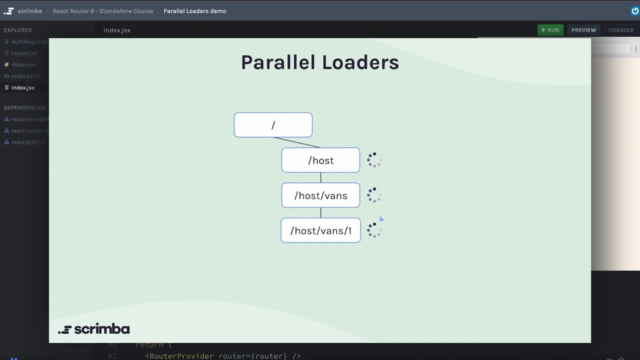 second what we're talking about when we talk about parallel loaders, And so I found a way that I can demonstrate this, And we're going to do that in the next scrim. Okay, do you remember when I was talking about how, when you have nested routes, how the loaders for each of those nested routes will? 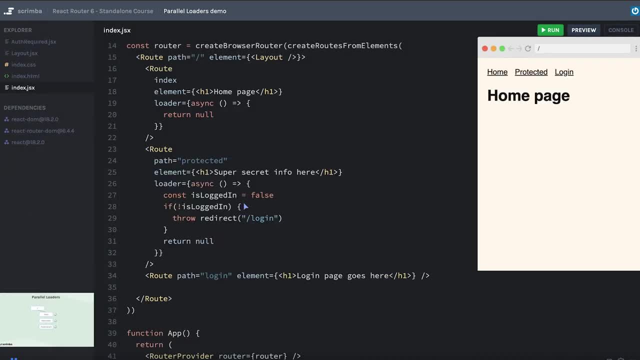 run in parallel. Well, we can see this in action by kind of faking the concept of fetch request. But first we need a nested route And we don't have that per se. we have this index route And then we have 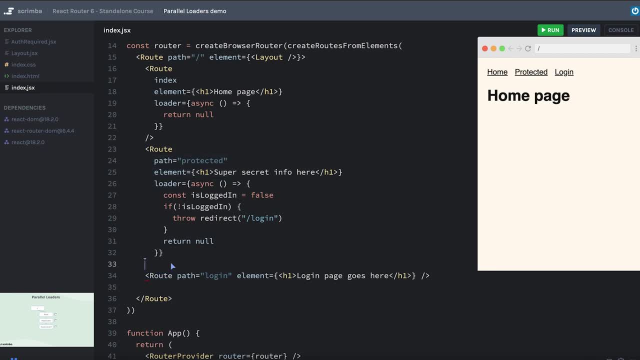 a protected route. Let's go ahead and turn our protected route into a parent, So we'll close this as a separate component And then I'll create a new route And this one will say the path is- I guess it really doesn't matter, We'll just call it nested, And it'll just say nested protected. 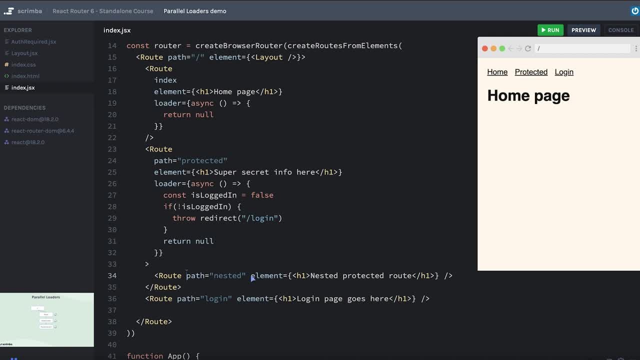 route. Okay, I'm going to create a loader for this one as well, So let me put these on their own lines. create a loader that looks just like the other ones. it'll be an async function. Okay, let me get rid of the authentication stuff that we're doing up here for now. 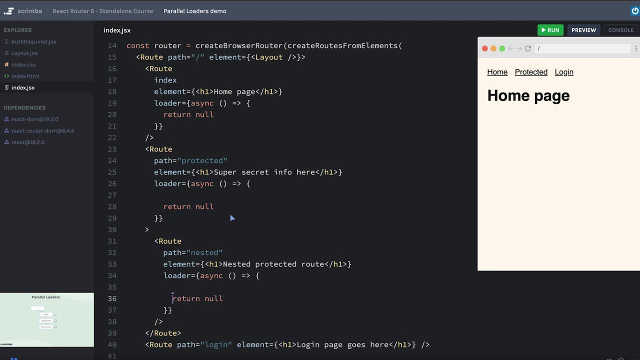 And instead- well, let me move this- return null, because that's going to be important to be done there, And we're going to do something fun. in each one of these, we're going to create a random number And then we're going to use that random number as part of 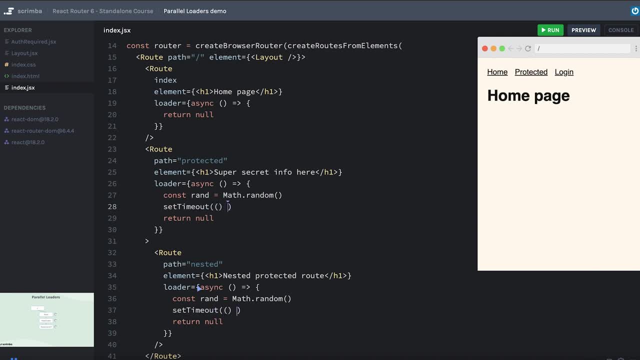 a set timeout. set timeout takes a function to run, So we'll do this. And then the second part parameter is the amount of time it's going to wait before it runs, So we'll put that random number in there. The idea here is that we will run this function at a random amount. 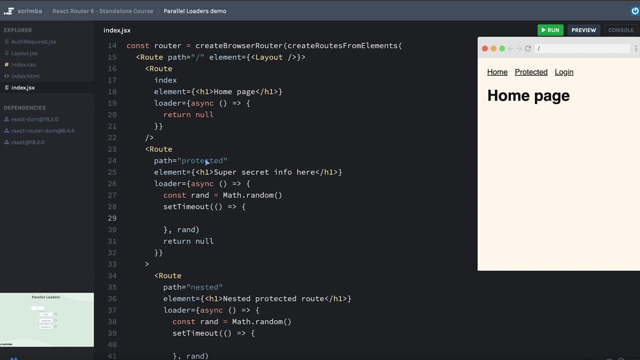 of time between zero and one seconds, so that sometimes this protected route up here will have a let's do. we'll just say console log protected route And down here we'll say nested protected route. So sometimes this set timeout will finish first and sometimes 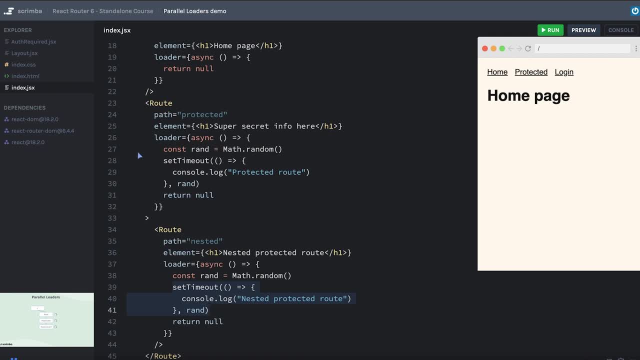 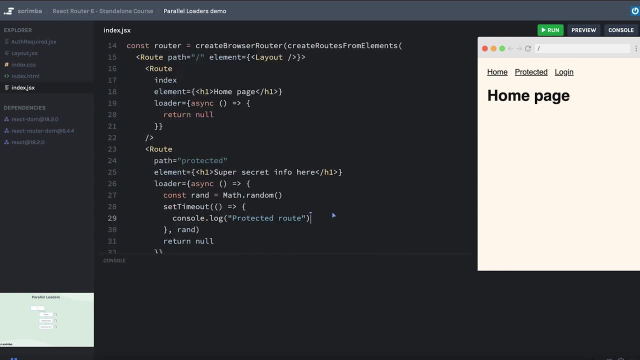 this one will finish first, And if our loaders are truly running in parallel instead of in sequence, then we should sometimes see this console log first and sometimes see this console log first. So I'll open up my console and we'll hit refresh, But first we have. 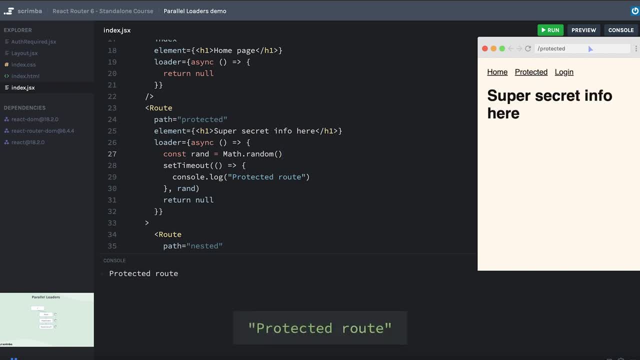 to go to our protected route. Actually, that's only going to run the protected one, So let me type in slash nested at the end And I'll hit enter And okay. so this time we got protected route first and then nested protected route. This helps us see that multiple loaders are. 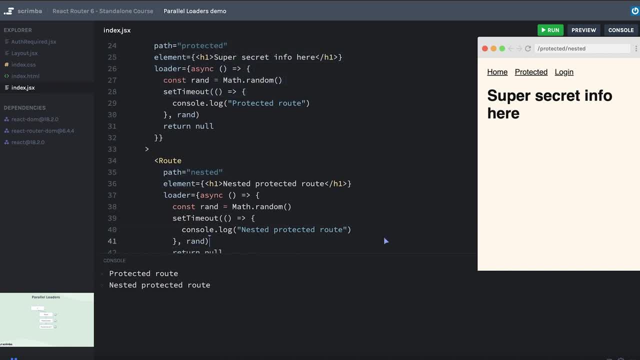 running one for this parent route and another for this child route. But now let me just keep hitting refresh until we see something different. Well, one thing I can do is make the spread a little bit greater. we'll say maybe times two here. let me hit refresh again. 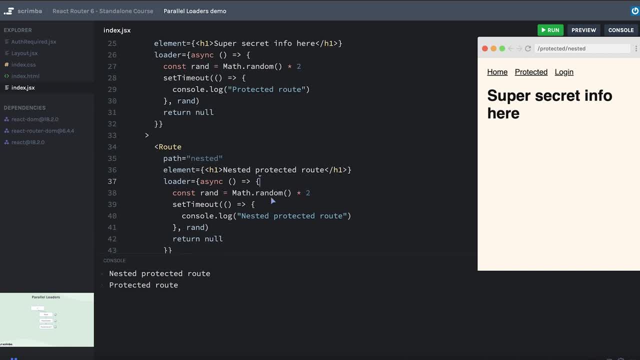 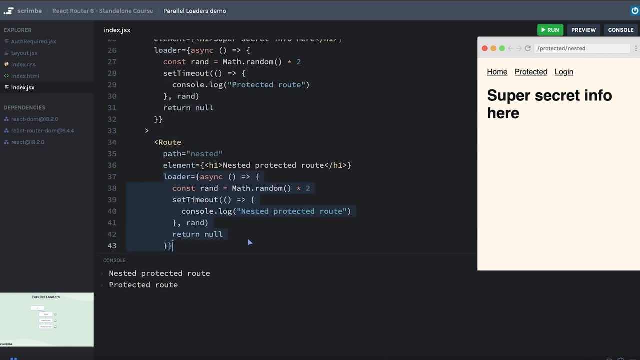 Okay, here's an instance where the nested protected route finished first, before the protected route. This really does show us that react router is not waiting for this loader to finish before running this loader, But instead both loaders are running at the same time. Okay, that was a lot of work to get to. maybe a bit of an underwhelming result. 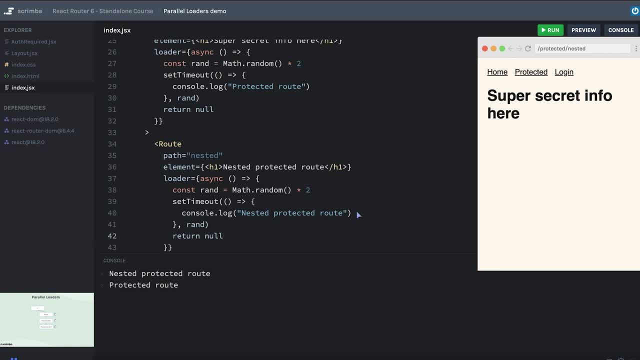 But if you're a nerd like me, it's kind of cool to see that these are running truly in parallel, And it also helps us better understand why we're having to take this different approach, as opposed to just putting a parent route around the other ones. Because if we imagine, 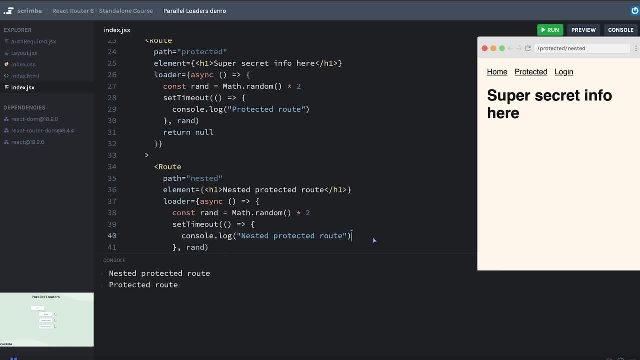 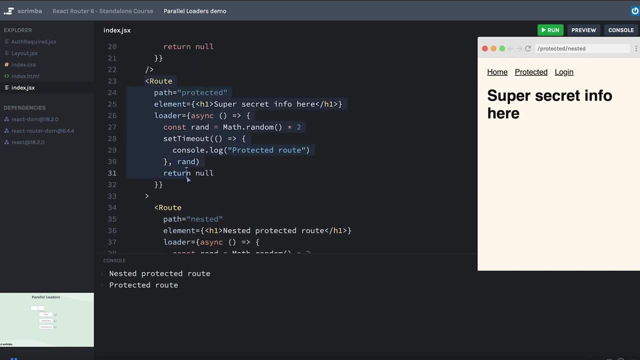 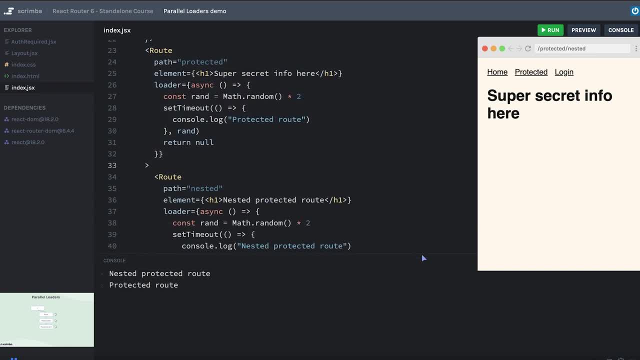 route that is trying to stop the rendering of my child route, because the loader is happening before the renderings happening. Okay, we're done with that. aside, let's go back to our van life app, finally, and get your hands on the keyboard with a challenge and have you implement protected. 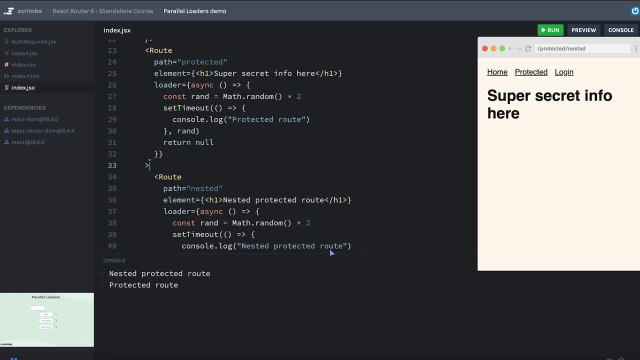 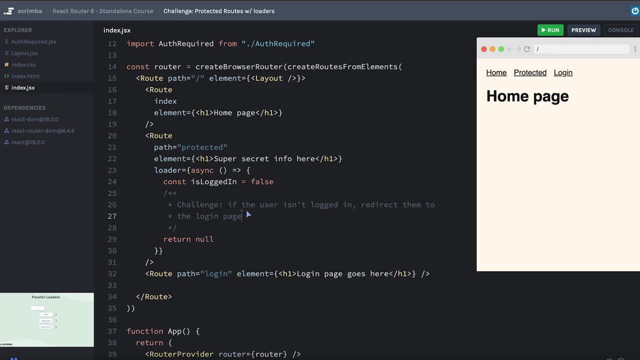 routes, as we've learned in the last few scrims in our van life app. Actually, you know what I lied. I'm feeling a bit guilty for how much talking I've done without getting your hands on the keyboard. So before we go into something with slightly higher stakes by going into the van life app, 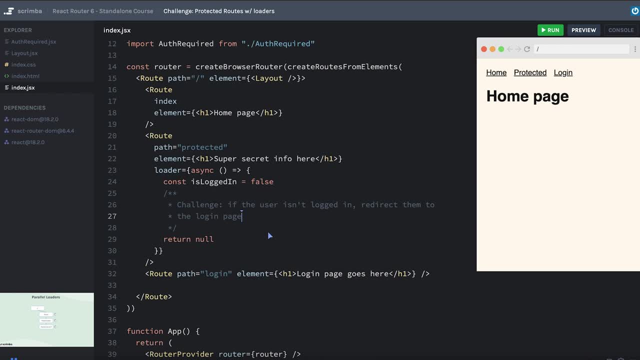 and having you implement what we've learned. I want you to get your hands on the keyboard now, while we're still here, and simply rewrite some of the code that we just wrote. So your challenge is to, if the user isn't logged in, redirect them to the login page, If you need. 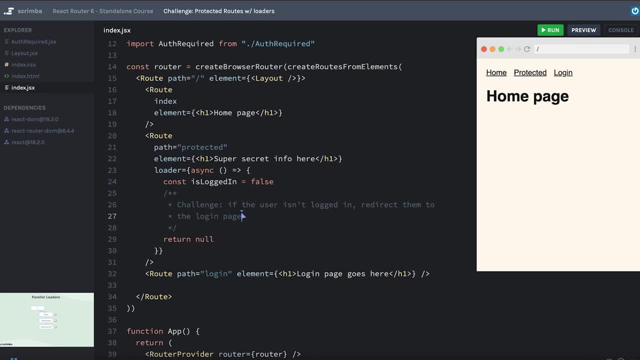 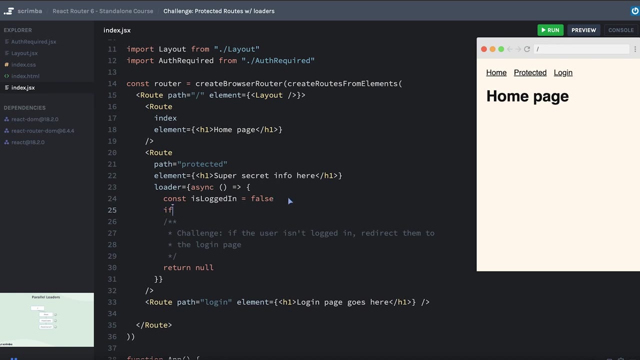 to go back and see how we did that. that's completely okay. pause now and work on this challenge. Okay, well, you might have noticed that we are already importing redirect. that's from when we did this before, And all we need to do is check if the current user is not logged in. 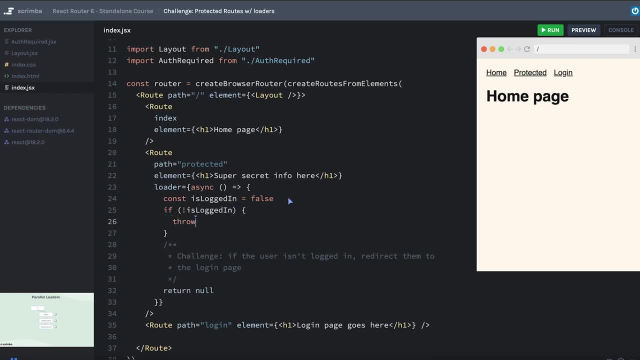 so not is logged in, then we are going to- and in this case we're going to throw like we're throwing an error. we're going to throw a call to the redirect function And it'll take us to slash login. we have to keep our return null there, just in case, And so we're just going to keep. 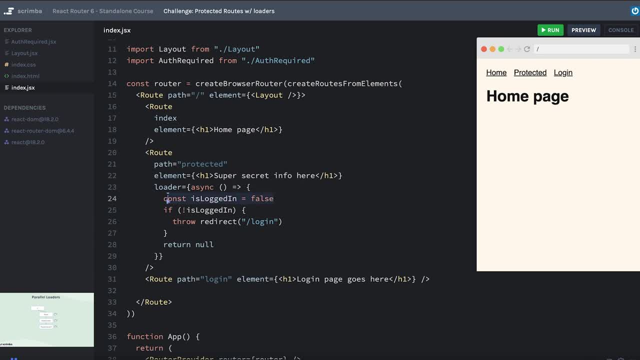 the return null there, just in case. And so we're just going to keep the return null there, just in case. And so we're just going to keep the return null there, just in case. Let's go ahead, hit save. we're currently not logged in because of this variable. we'll hit protected, And sure enough. 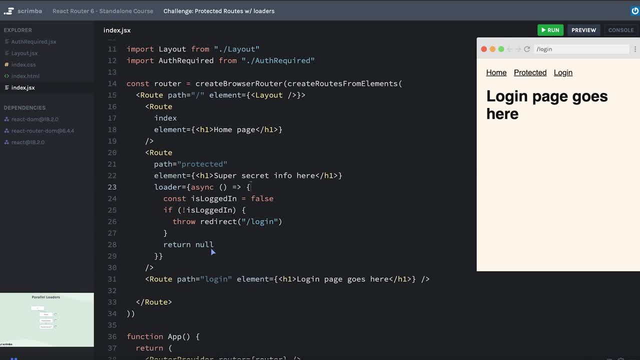 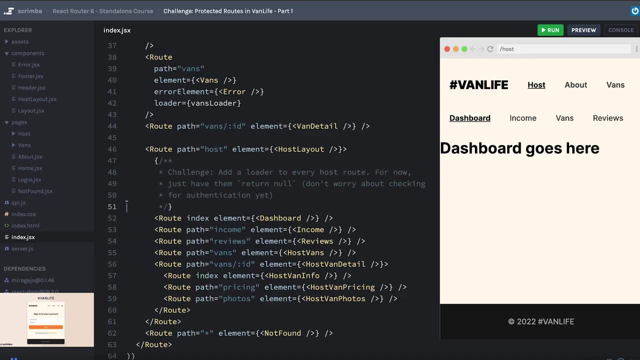 it takes us to the login page. Okay, let's make our way back to van life, And it'll be your task to do the same thing over there. Okay, we're going to try and take this one step at a time And unfortunately, in this challenge, you're going to get firsthand knowledge of that downside that. 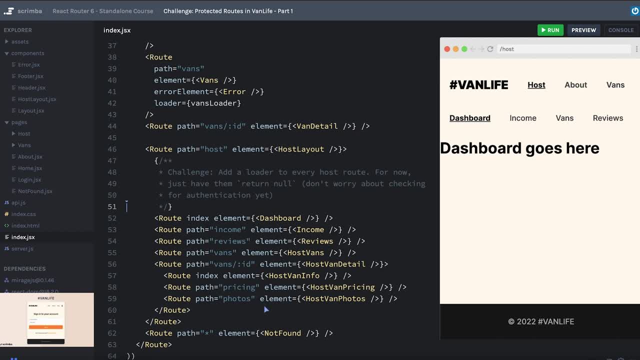 I was talking about, where you have to include a loader on every one of your protected routes in order to protect all of the routes, And that's again just because they will always run in parallel. As a reminder, at the time of recording this, there is a proposal for a middleware that 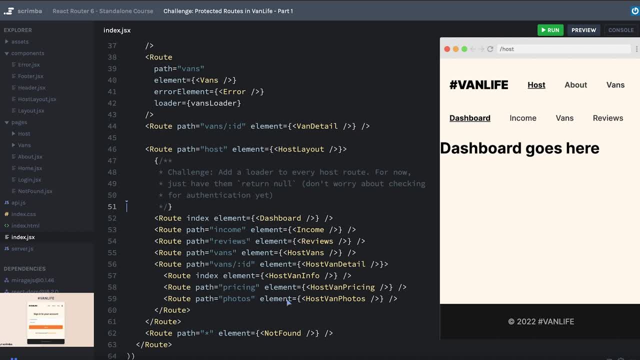 would run before any loaders, where you could instead write this authentication check before any of the loaders, in which case you wouldn't have to write them in every single loader. But as I'm recording this, it's not quite yet a part of the react router API. Hopefully, 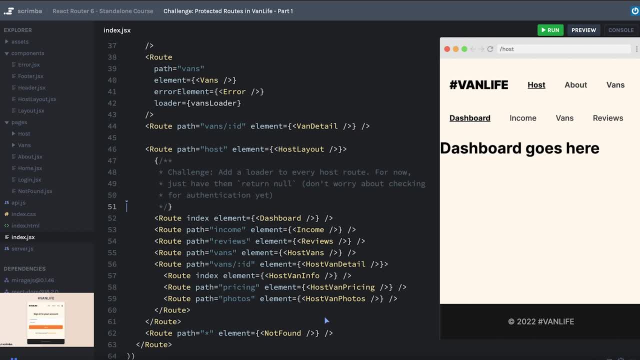 I'll be able to re record this in the future and update with some good news. Okay, so I'm sorry this will be a little bit tedious of a challenge, but it's going to set us up to make these protected routes. For now, don't worry about checking for anything dealing with authentication. 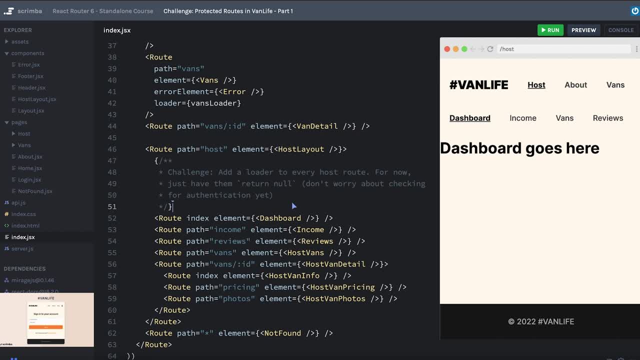 so that we can just take it one step at a time. Pause now and work on this challenge. Okay, I am going to make use of multiple cursors here. So first, just because it will be a little bit long, I'm going to put everything on its own lines And this is going to go. 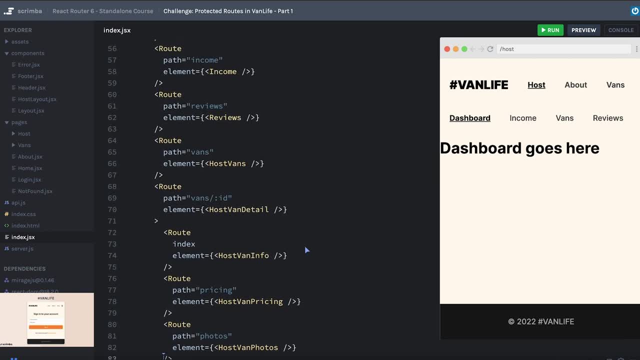 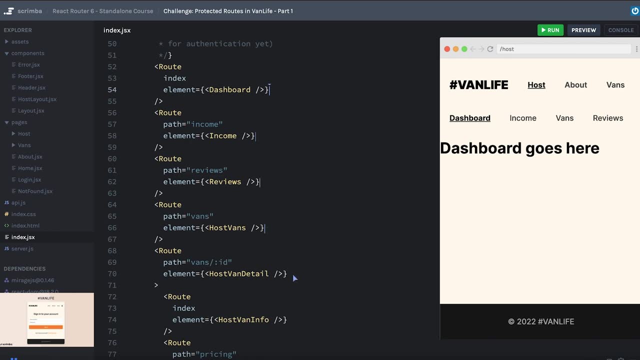 in a little bit lighthouse and you'll see it will get significantly longer, but that's okay. Okay, the only reason I did this on its own lines is so that it would be really easy for me to include a loader on every one of these. Okay, so we'll include a loader. 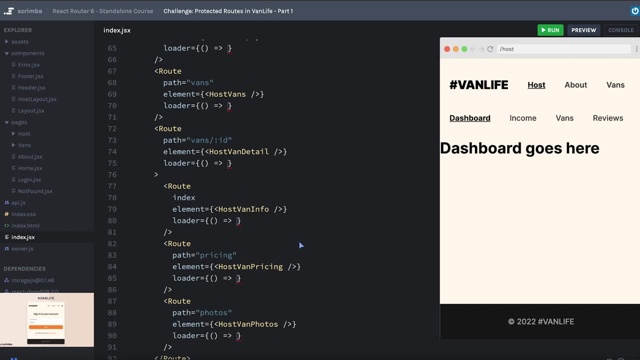 And for now we're just going to do an inline function here. One thing to note about loaders is that they could either be an asynchronous function or not an asynchronous function. I happen to know that it's going to be useful for us to make these asynchronous functions, So I'm 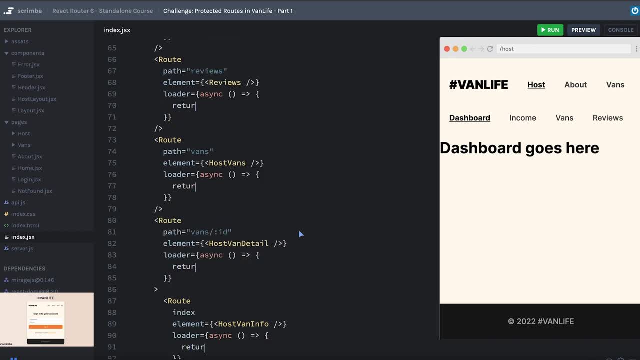 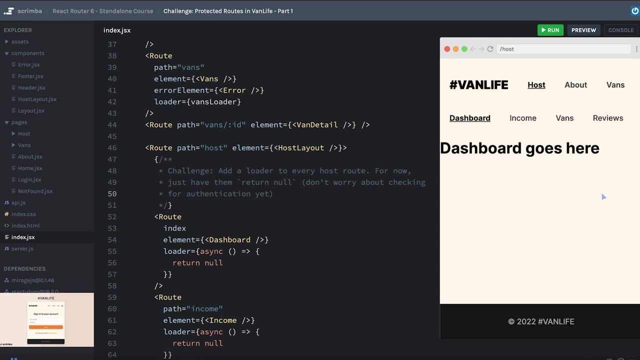 going to do that And I'll open up the bodies here and just return null. Okay, I guess the main way we'll know if this worked for now is that we don't get any errors when we load. Okay, perfect, This was a bit procedural, So in the next lesson, hopefully, it'll be just a little more exciting. 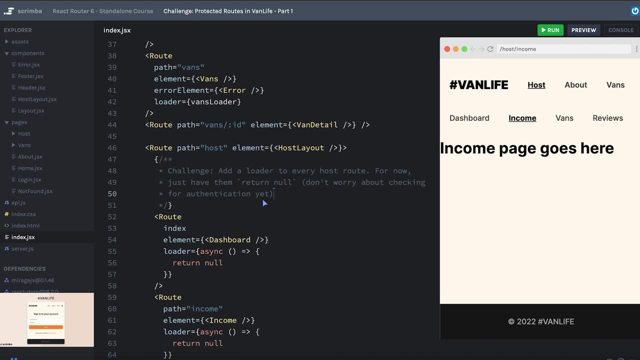 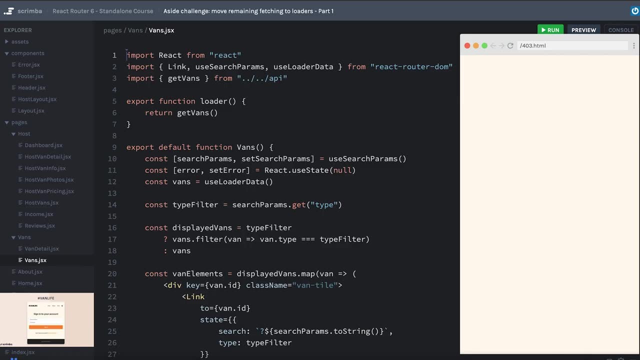 And we'll actually start including some checks for authentication and protecting these routes. Before we continue on with protected routes using loaders, we do need to make a few changes to our host routes Because, although we have implemented the loader for our vans dot JSX file, we have not done that for our 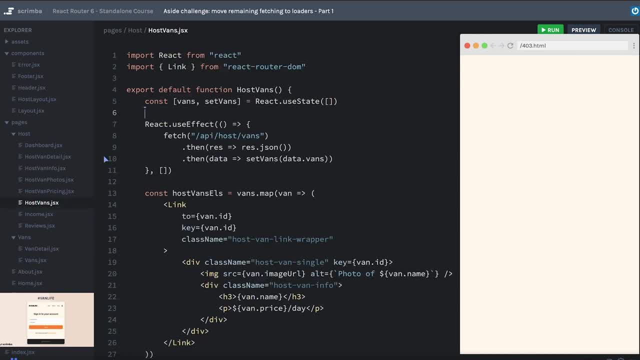 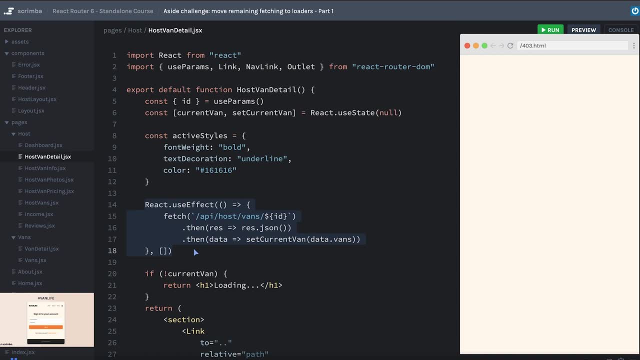 van detail page, our host events page or our host van detail page. These are all still using a use effect in order to fetch data. I think technically we could still get things to work, But it would be a little bit more complicated. But I think technically we could still get things to work, But it would be. 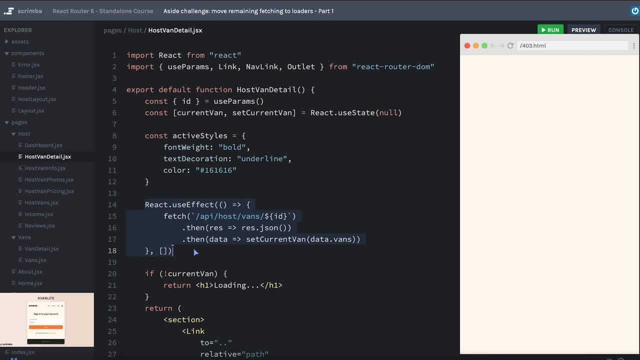 a strange mashup of these two different paradigms, where loaders really should be what's used in order to get data for the component that needs it, especially since we've already started creating some loaders over here inside of our route definitions. So I'm going to walk us through. 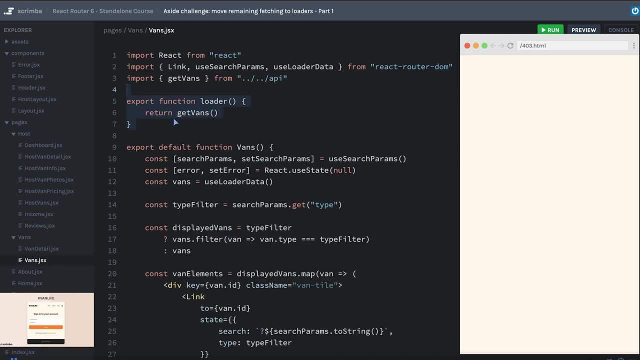 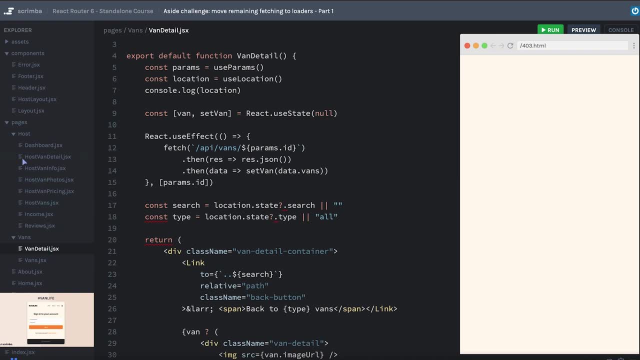 a quick refresher on how we did loaders with our vans page, And then I'm going to implement it in van detail And then your challenge is going to be to also implement it in host fans and host fans detail. So you might remember when we 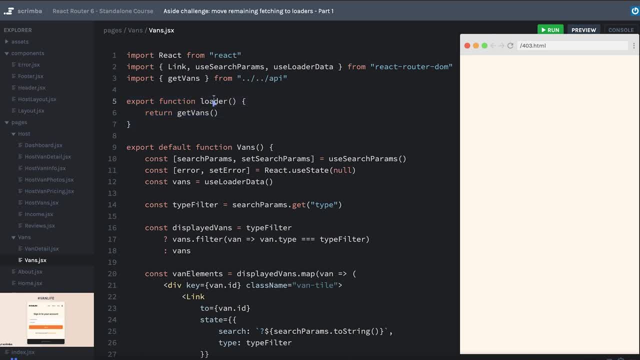 were doing this. what we did is we exported a function called loader And all it does is return the promise that comes back from get vans. then we're using use loader data in order to get access to our vans so that we can then map over them, filter them and do whatever else we need to do. 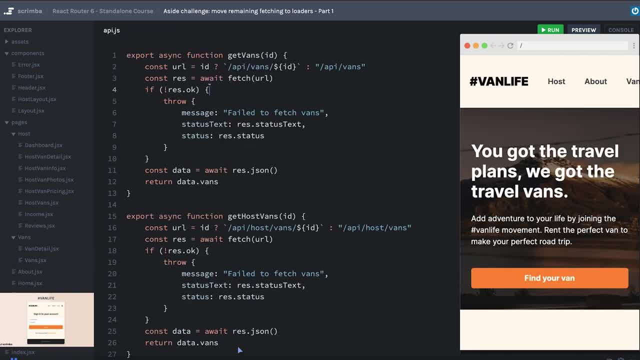 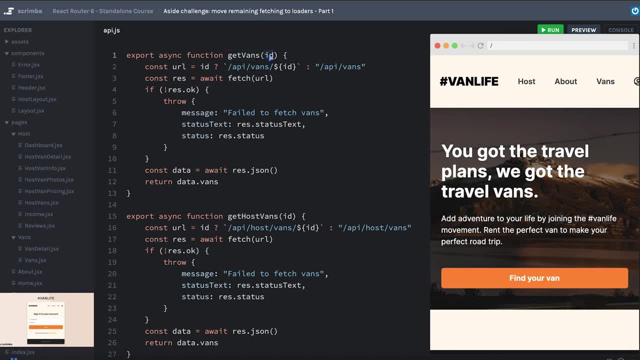 with them in our file. If we go to API JS, you can see that I have beefed up our API functions here just a little bit. our get vans function is now able to take an ID if necessary, And so we're sort of overloaded. And so we're able to take an ID if necessary, And so we're sort of overloaded. 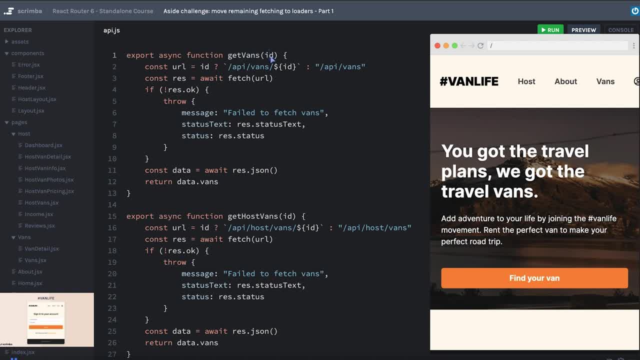 this function, where we can either not provide an ID and get a list of all the vans, or we can provide an ID and get the single van with the ID that we specify, And then we have a separate get host vans function which is almost identical to this, except it reaches out to slash API, slash host, slash vans. 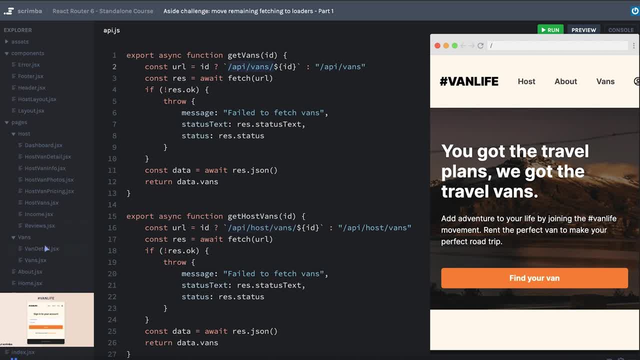 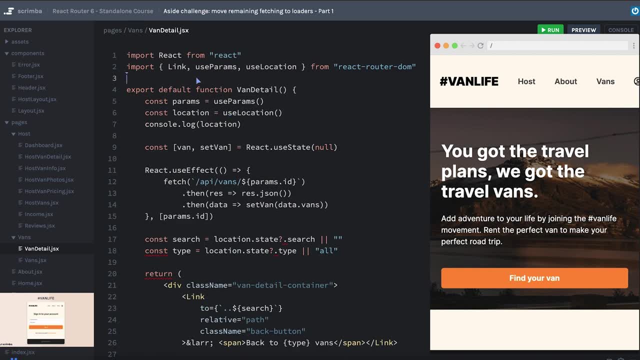 instead of just slash API, slash fans. Okay, so let's go to van detail and refactor this so that we essentially do the same thing as we did over in vans. we're going to come up to the top, going to export a function called loader. Eventually we'll see that these functions 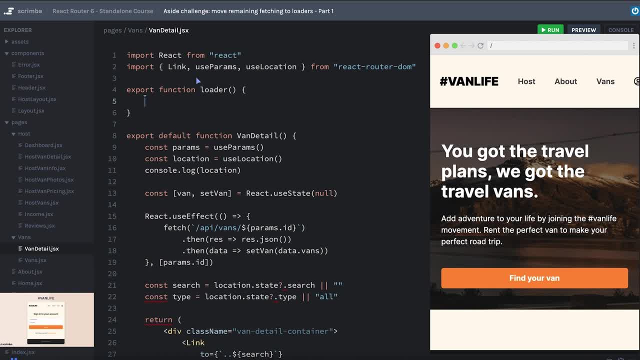 can be async if we want them to be. I'll come back later and implement that if we need to, And all it's going to do is return a call to get vans. Let's see, let's go to vans. Okay, this is basically exactly what actually. it's literally exactly what we had there. Now we 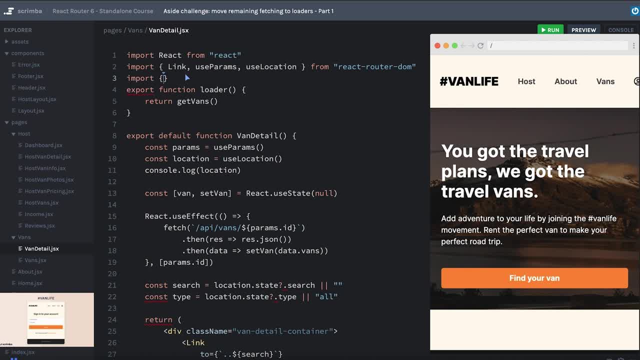 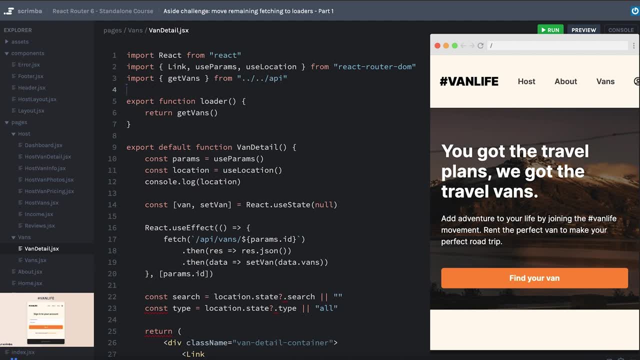 need to import get vans for that to work, So we will import get vans from the API file. However, this time, because this is the van detail page, we need access to the ID of the van that we're trying to get. Before, what we did is we used the use params hook, which allowed us to access params. 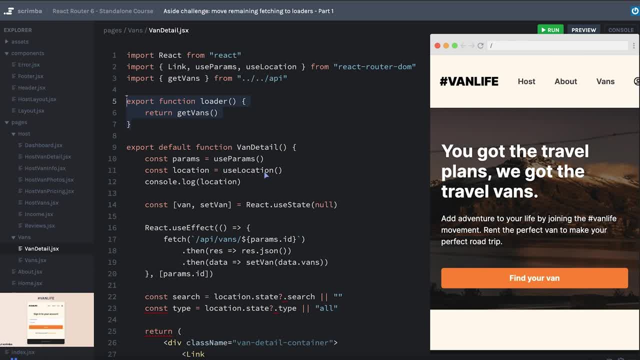 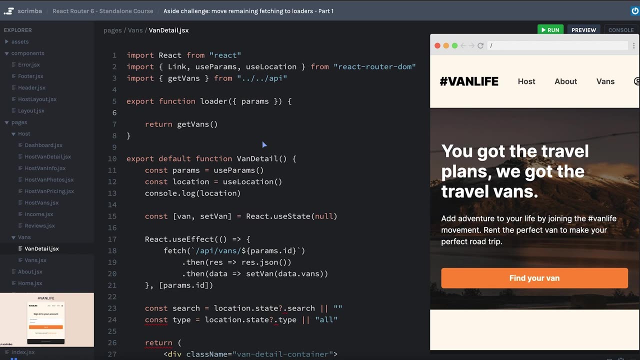 dot ID. But since the loader function is not a component, we can't use hooks inside of it. hooks can only be used in components that get rendered. Fortunately, we have immediate access, as one of the parameters to this function, to an object called params, And so this is exactly what you. 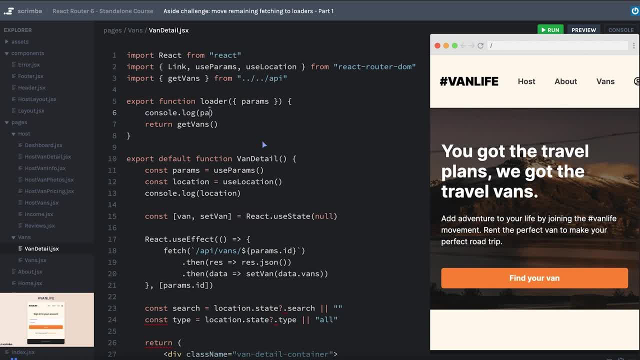 would think We will now have paramsid, So I'll go ahead and just console log params, Let's refresh. Oh, actually, before that will work we need to go to our file here and set up the van detail to have a. 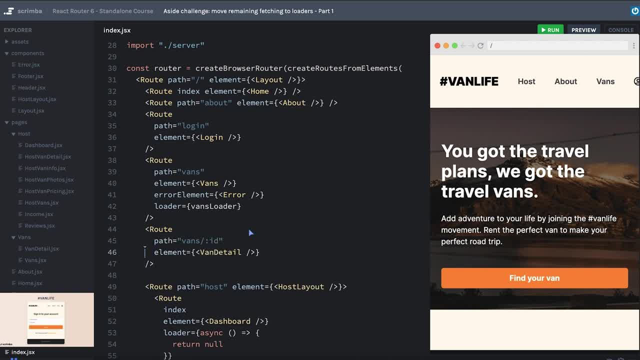 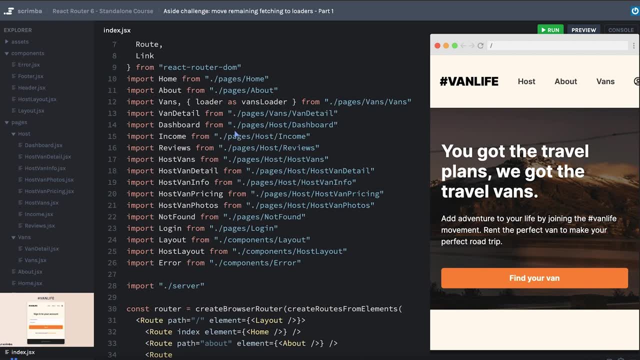 loader. So we'll move these on their own lines. say, the loader is equal to, we'll call it the van detail loader, And then we need to import that. So here we're importing van detail, we will also bring in the loader. 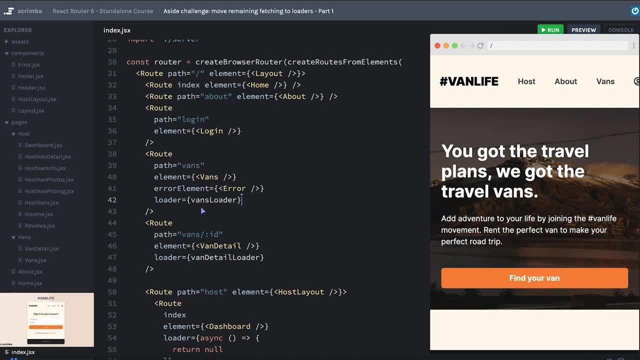 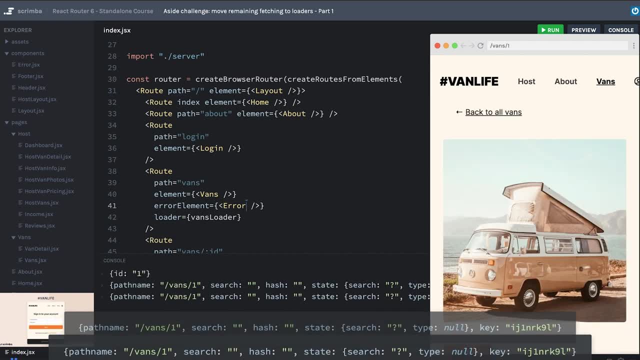 As then detail loader. Okay, let's give this a shot. Now I will hit refresh, we'll open the console, I'll go to vans and then go to the van detail page And, sure enough, we get the object with the ID of one. 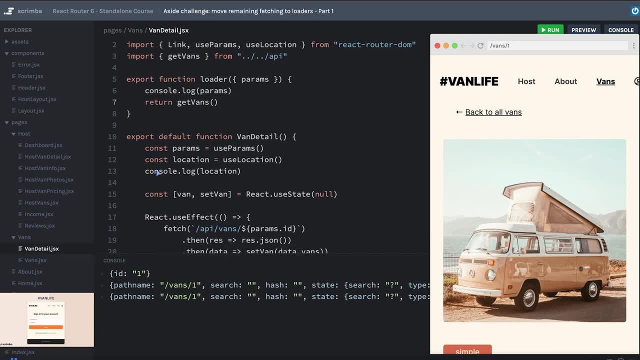 it looks like we have another errant console log hanging out somewhere And that's right here with console logging our location. we'll go ahead and get rid of that. Okay, so I have access to the params object. it has a property called ID And so I need to make. 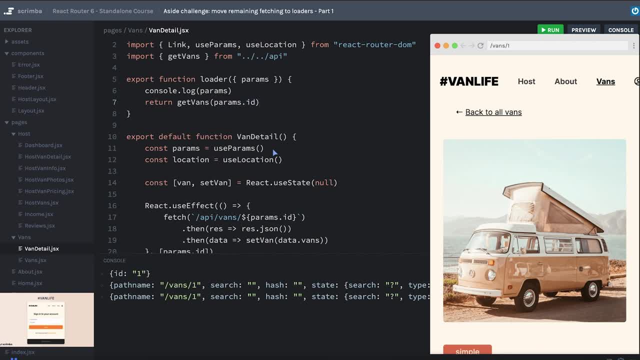 sure that I pass. that is with the prompt. But once we get there it's not going to get loaded. We'll need to؟ in to my get vans function And then I'll need to use my use loader data hook And that should get. 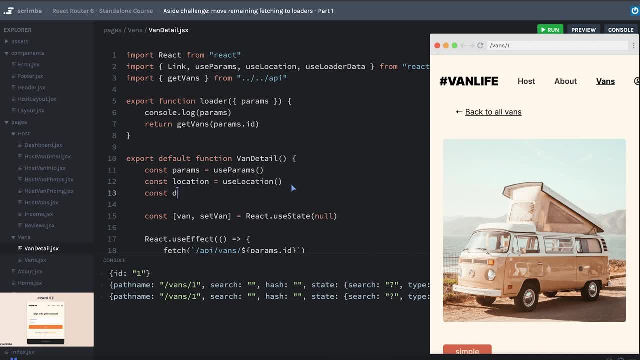 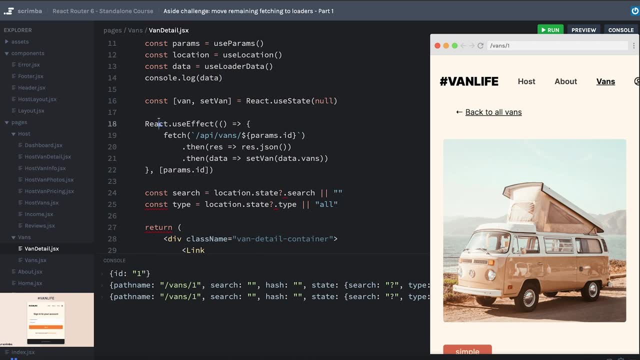 me access to a van object. I think let's call it data. We'll say use loader data And then we'll console log the data. I'm going to comment out my use effect here And actually I'm going to put a. 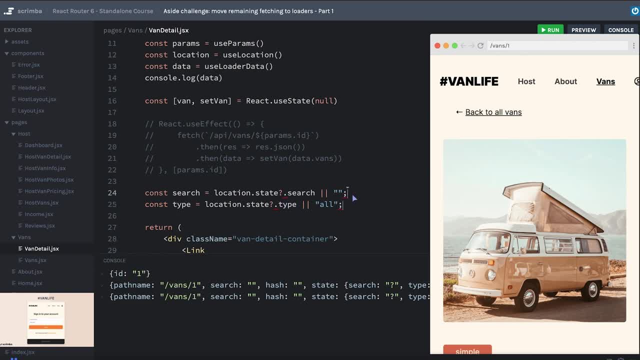 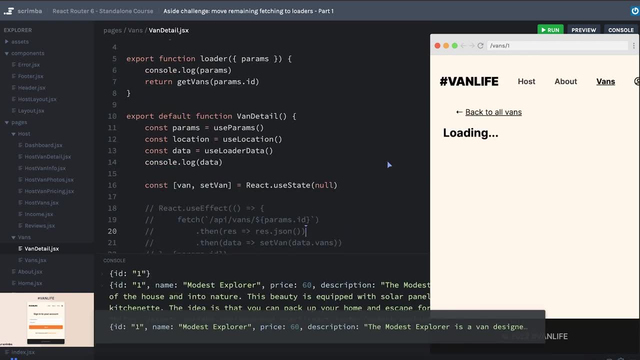 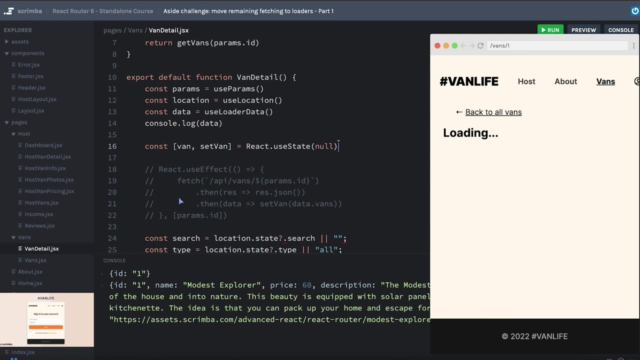 set of semicolons here, just so that it relegates these squiggly lines to the semicolon instead of making it look like our return is broken. Okay, let's hit save. Awesome. Now our loading is freaking out a little bit because our van is not coming from state anymore, because we are no longer. 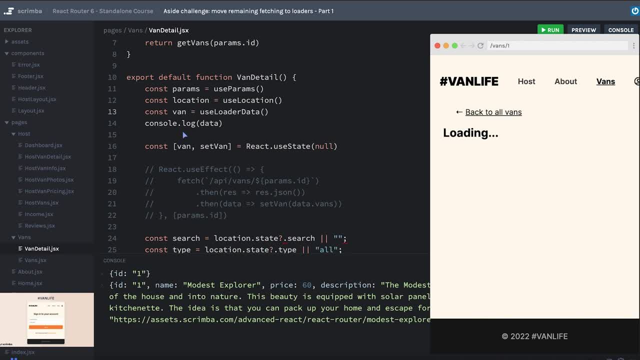 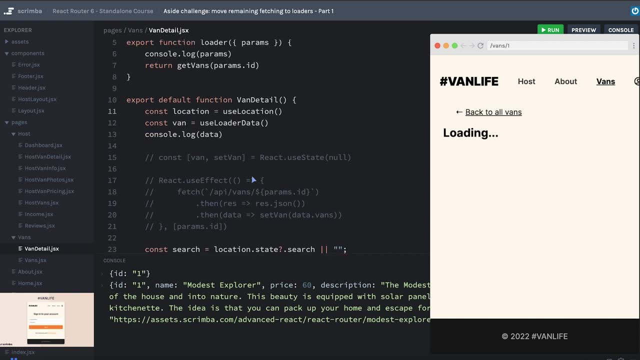 fetching it. So let's go ahead and call this van, so that we can just reuse that name. We'll comment out our state- we shouldn't need params anymore, because we're doing that in the loader- And let's hit save. Oh, of course I'm still trying to console log data. we can get rid of our console log now. 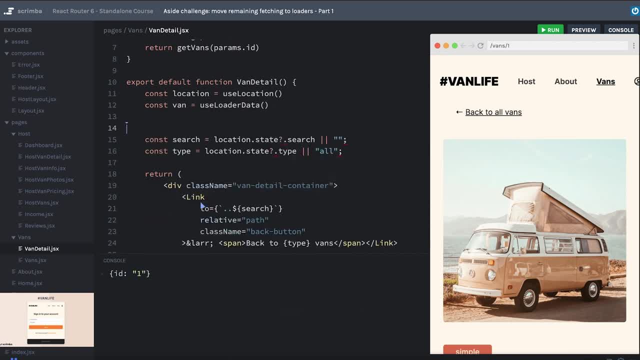 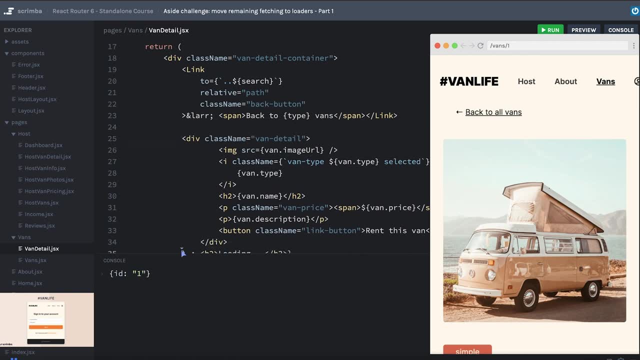 Okay, our van is showing up, So let's get rid of this code here, And then we no longer need to check if van exists, because we can be pretty confident that it is going to exist, since we are loading it before the route ever loads or before this component ever mounts. So we will get that in. 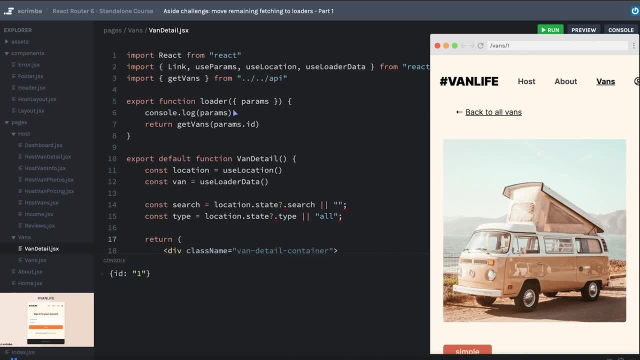 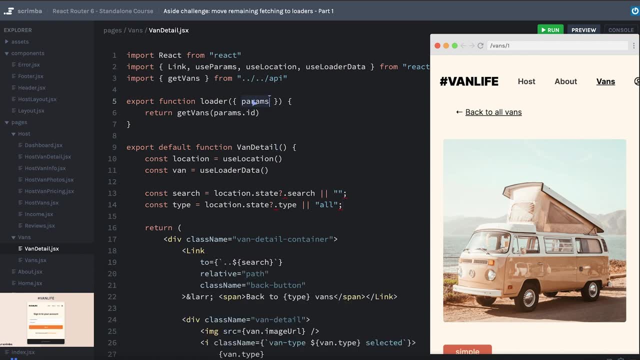 there, fix up some of these formatting issues And let's get rid of our console log up here. while we're at it, hit save And cool. Okay, now that you've seen how we can do this and how we can add parameters directly inside of our loader, it's going to be your turn to do this for the host vans. 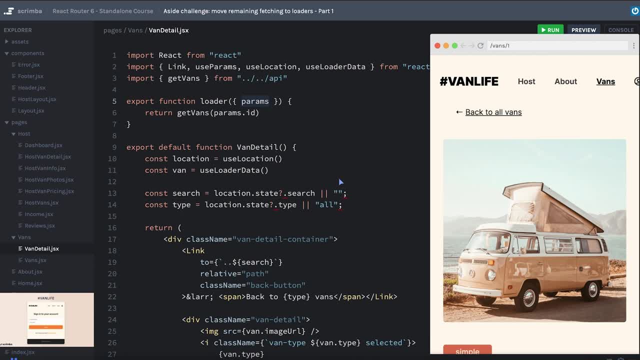 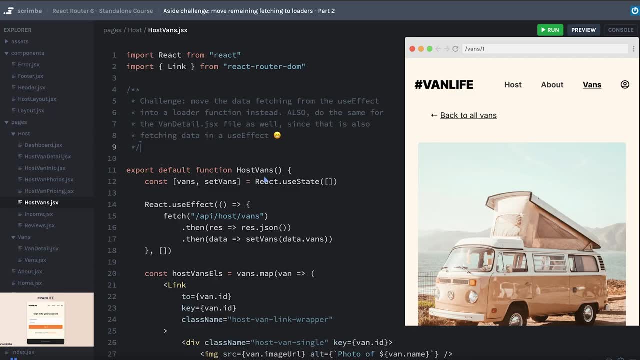 page and the host vans detail page. So that's what's coming up next. Okay, just like I did in the van detail page, you are going to do for the host vans page and the host vans detail page. Currently, both of those are fetching data from a use effect And we want to move that to a loader. 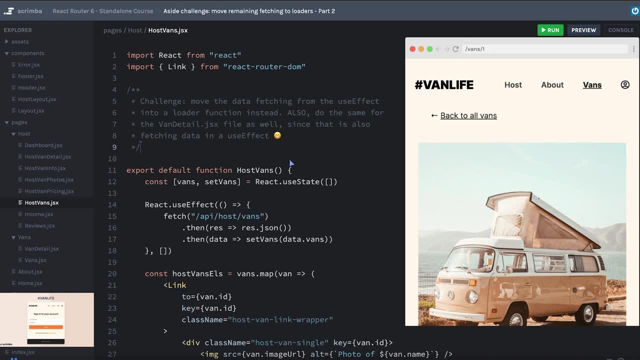 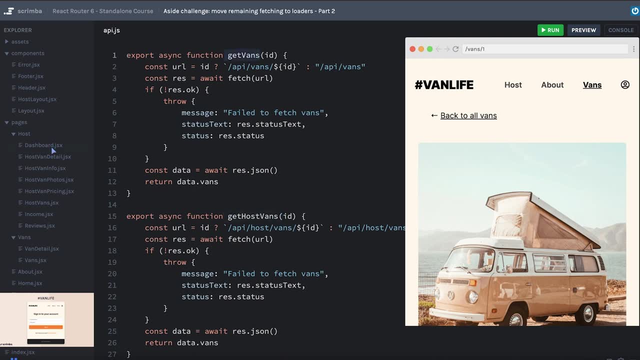 instead. So that's exactly what your challenge is. you can read it here. One thing to note is that we're going to be using the get host vans function instead of the get vans function, since we're dealing with the host routes now And also the inline loaders that we put. let's see where are. 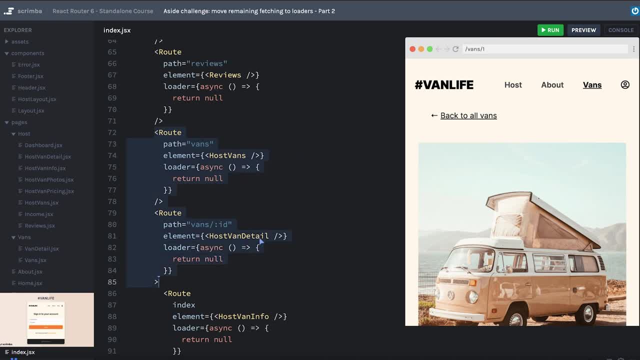 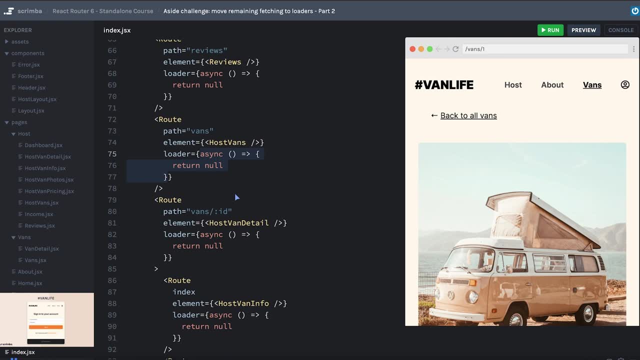 they right here and here for our vans page, our host vans page in our host fan detail page. these inline loaders you'll just replace with the ones that you will import up above, that you are exporting from those component files here. Give this your best shot. If you need to look at the 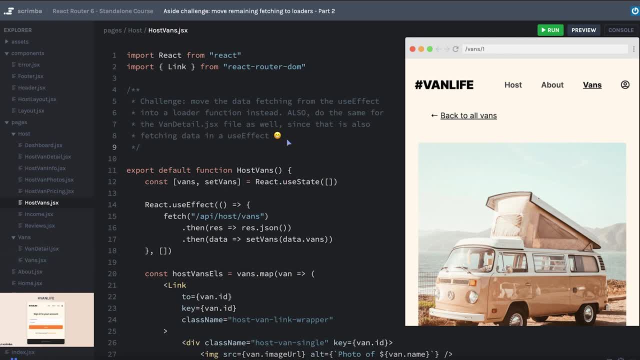 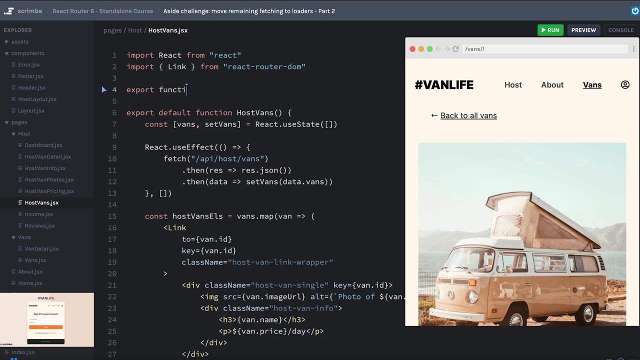 vans or the van detail page. that should help you quite a bit, And then we're going to go ahead and edit it And then we'll go through it together. Pause now and work on this challenge. Okay, we'll just clean this up because we know what we need to do. we are going to export a 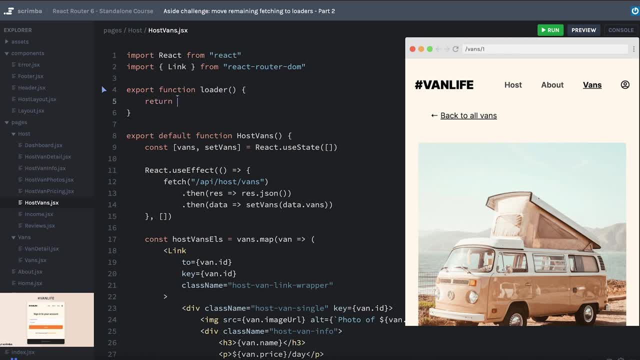 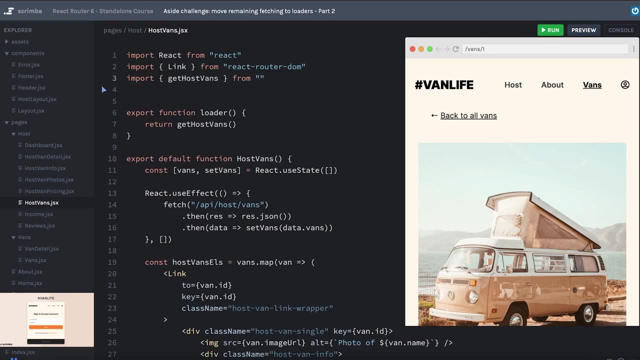 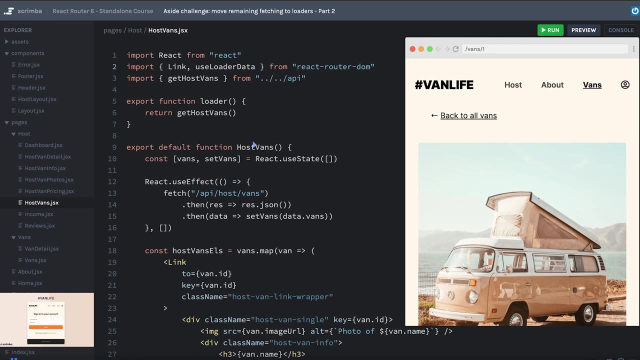 function called loader. we're going to return get host vans and then we need to make sure we import that, And this is coming from the API file. Okay, and then here we're going to export the val adder And then we want to add the variable name. 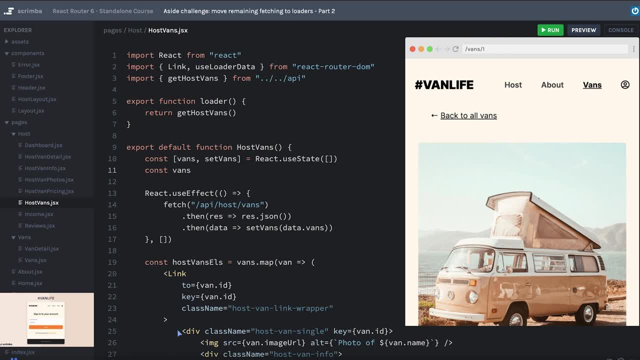 so that we can call that, and we need to add the variable name so that we can call this vans. We also need use loader data while we're in the same file and we'll go ahead and grab the list of vans. we'll call it vans, just like our state. So we don't have to make other changes, down below at least. 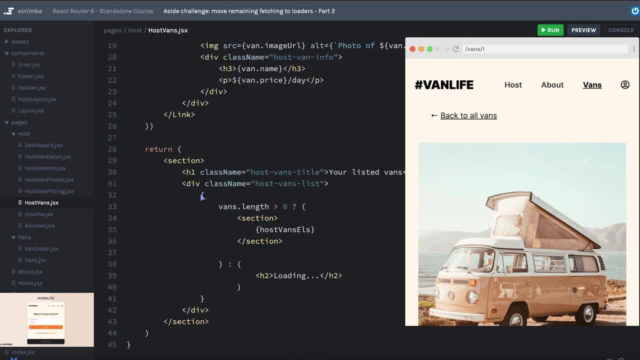 not too many, And that's going to be equal to use loader data. you can get rid of our state. we can length check to see if it was loading or not. This, of course, just assumes that the host has fans in their array. So we can get rid of that completely now and get rid of this completely. We'll do a. 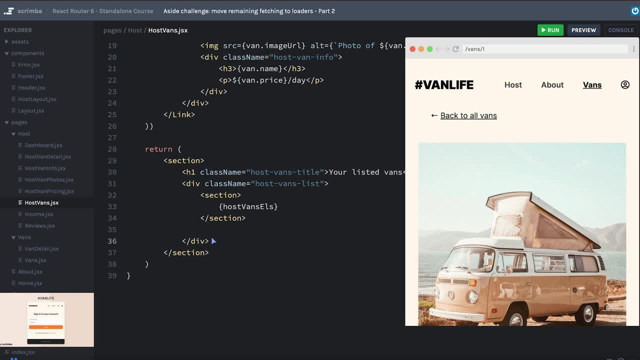 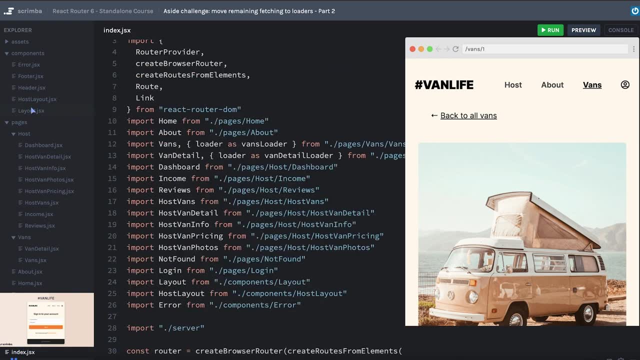 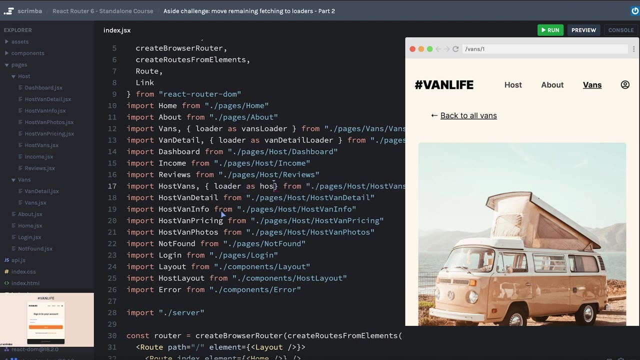 little reformat, so much simpler, And I don't need that curly brace either. That feels really good to clean up that code. Okay, we're not quite done, Of course. let's go over to our index file And we will come up to the top And right here, host vans, we're going to import the loader as host. 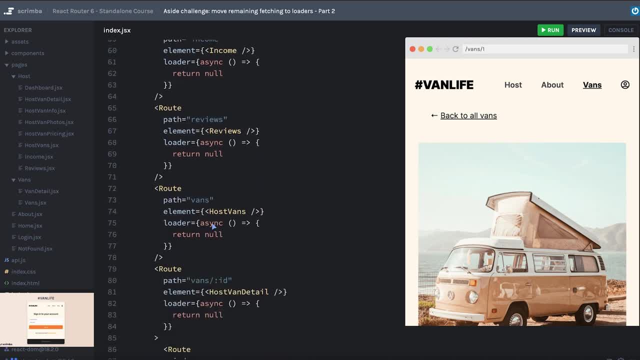 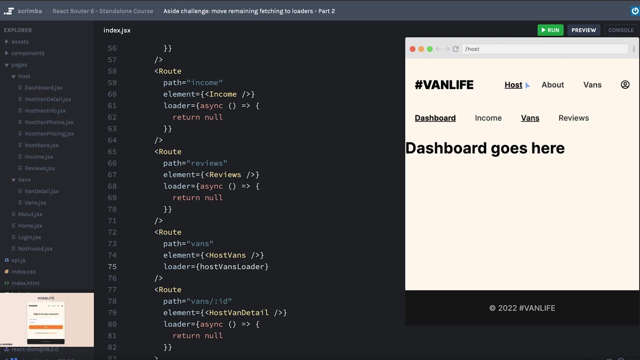 vans loader and then come down to our route, which was this one, And again, like I mentioned, we'll just replace the inline one with a named function. Okay, that was a lot of work without checking how we were doing, So let's go ahead and refresh, And we can test this by going to the host. 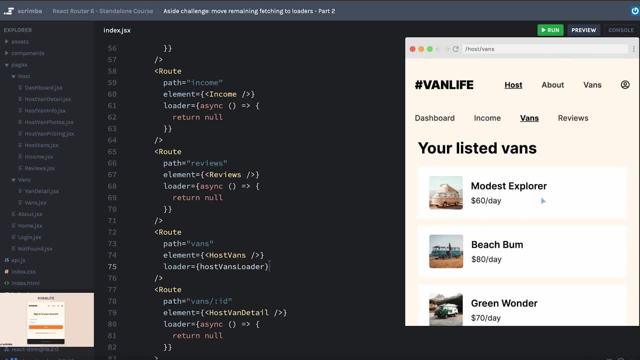 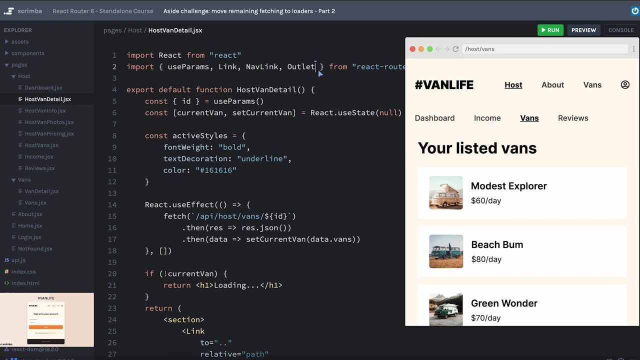 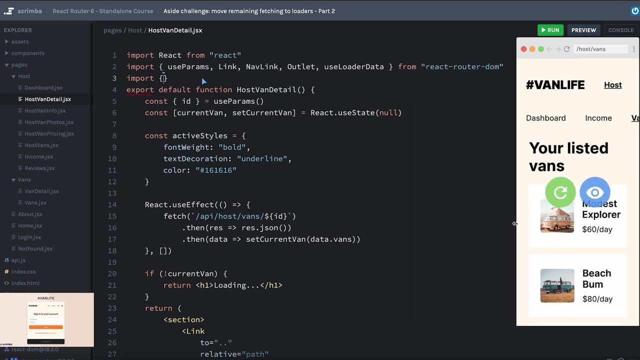 page and vans. Okay, our vans are coming in, Perfect. So now we will just do the exact same thing for our host van detail, And I'm going to fly through this pretty quickly. We know we need use loader data from react router DOM. we need our get host. 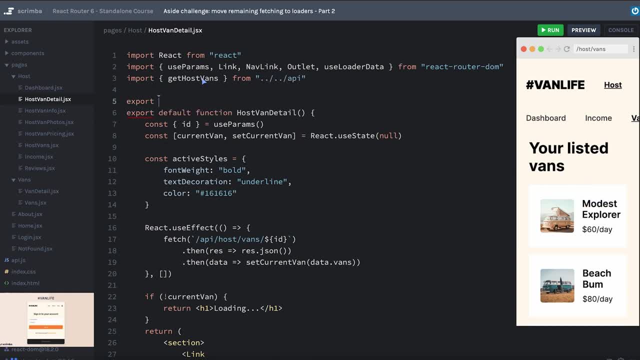 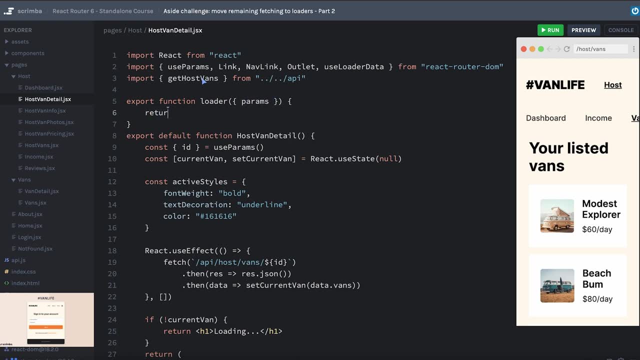 vans function from the API file. we're going to export a loader function. we will need access to the params this time, And so we are going to return get host vans by passing in params dot ID. we don't need use params, but we do need. we'll just keep calling it current van And that will be from. 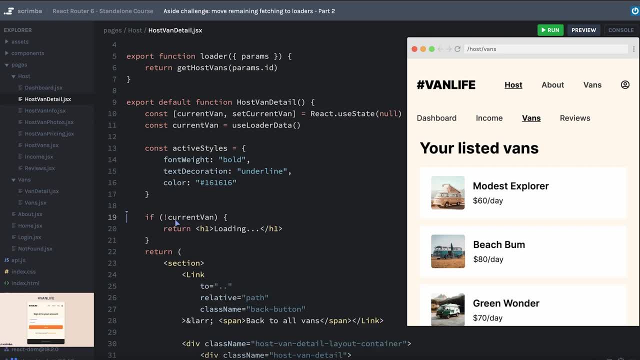 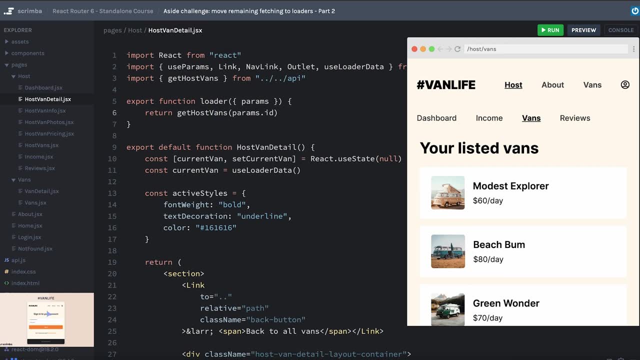 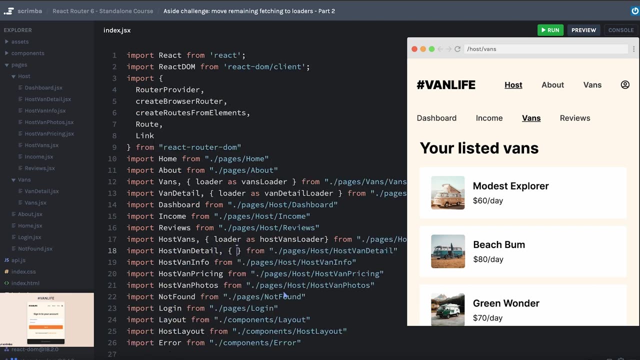 use loader data. we don't need our use effect, don't need to worry if there isn't a current van And everything else. I think should be the same. So let's go back to our index file. we will import- see where is our right here. host, fan detail. we'll import our loader as host and detail loader And 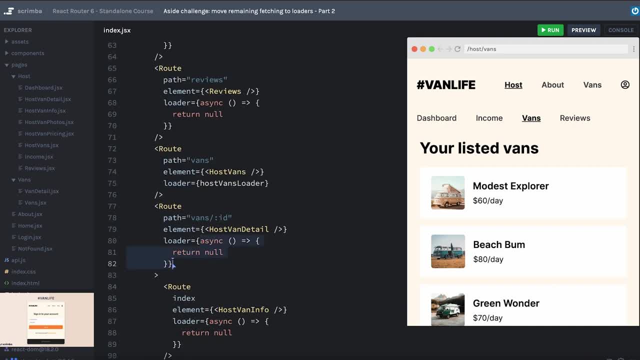 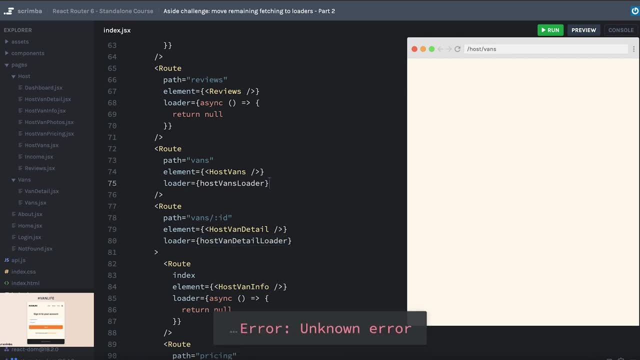 once again, we will replace. we can find it right here we have our inline. we will replace it with the host van detail loader function. we'll hit Save And oh, it looks like I got close, but not quite there. 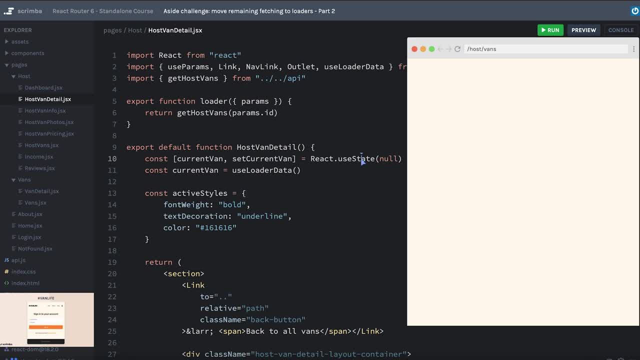 We'll see if we can figure this out. Oh, you know what? we are still using the current van state. I forgot to get rid of my state. we need to get rid of that because there is a duplicate declaration for it. Okay, let's try again. Most fans click on one of them, Perfect, Okay, hopefully that was. 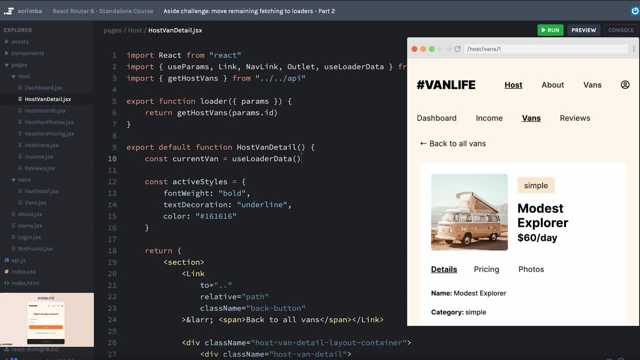 good practice. It's a good example of spaced learning and repetition. That's been a minute since we've dealt with the loader, So this is kind of good to get the practice back in, And now we're perfectly set up to finally go back to implementing the protected routes, now that we're doing things a little bit. 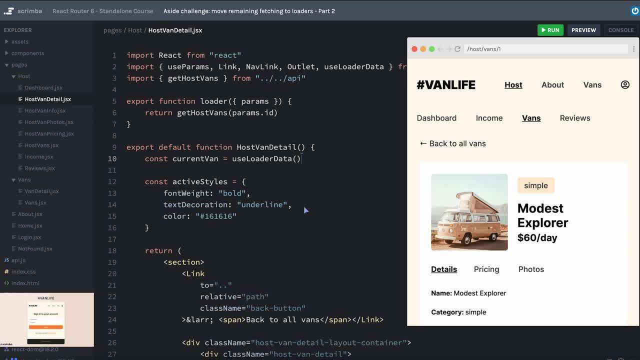 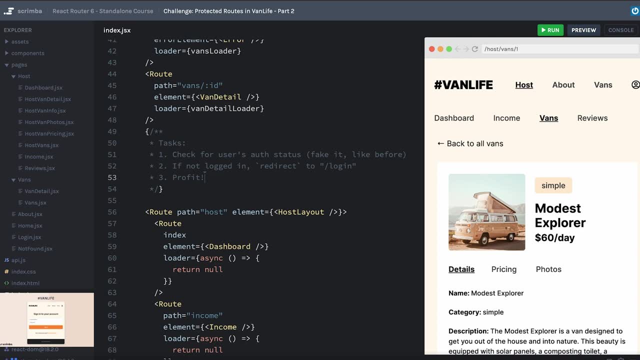 more in line with how it should be done with using loaders. Okay, so we have a task now that we're finally back to including protected routes in our loaders, And those tasks include checking for the users authenticated status, which we're just going to fake it like we did before, And if they're not logged in, we want to call that. 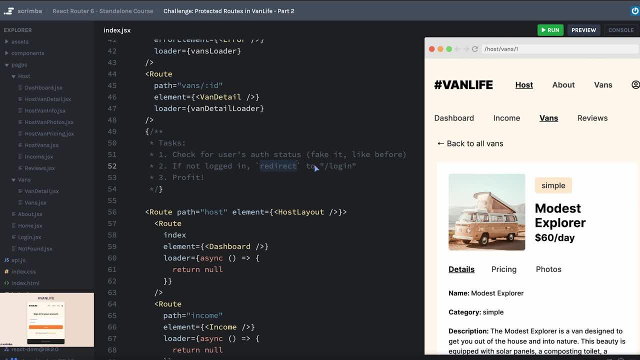 redirect function that comes from react router DOM to the slash login page. And I was about to write step three and realize that that's it. I know that it seems like we're doing a lot of work here because of the way that our loaders are, but we are going to see how we can simplify it a bit Now, rather than inside of every. 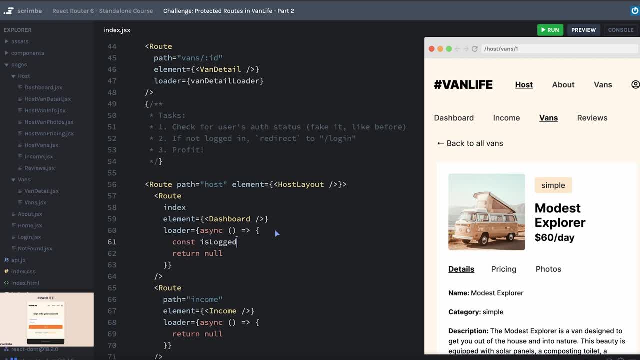 loader doing some kind of cons is logged in equals, false or true, and then trying to duplicate that for every loader. I'm going to create a new file that I call utils dot j s. that's just down here at the bottom, And we're going to create a. 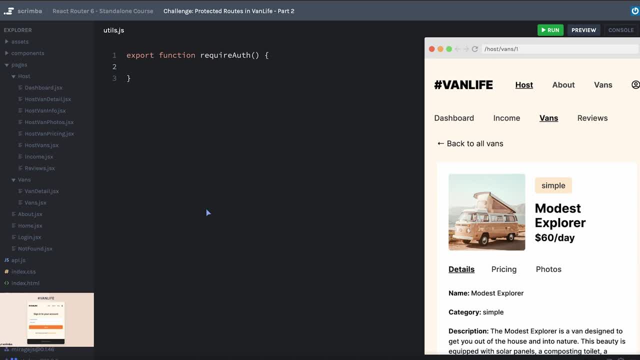 function that's just called require auth, Because this is a custom function, you could call it whatever you want, And inside this function I'm going to use my fake login status. So I'll say: is logged in equals false, And then I'll do my. 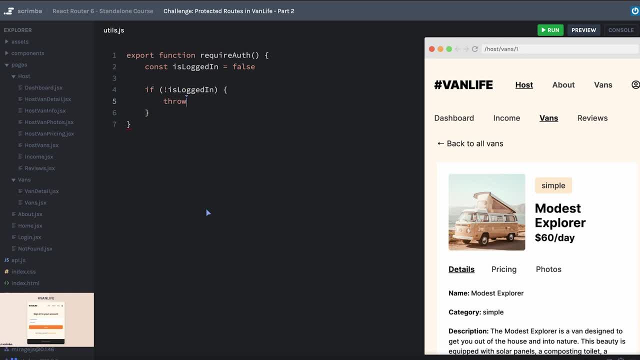 check that says if not, is logged in, then we're going to throw that call to redirect to the slash login page. And redirect is not a global function, we need to import it. So I will import redirect from react router DOM And eventually we're going to do a bit. 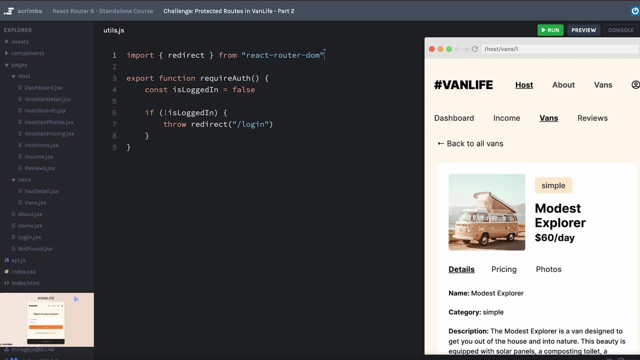 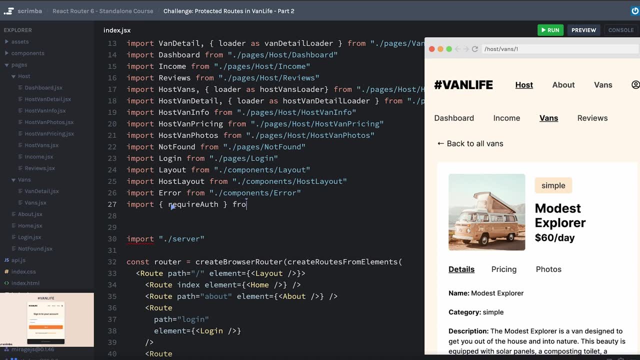 more work in here, But for now I think this should be good. So let's come back to our index. we're going to import our function that we just created that's require auth from the API- know, from the API- and then we'll do the other version of it. 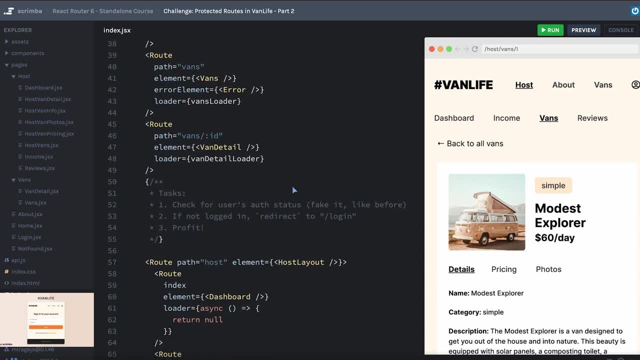 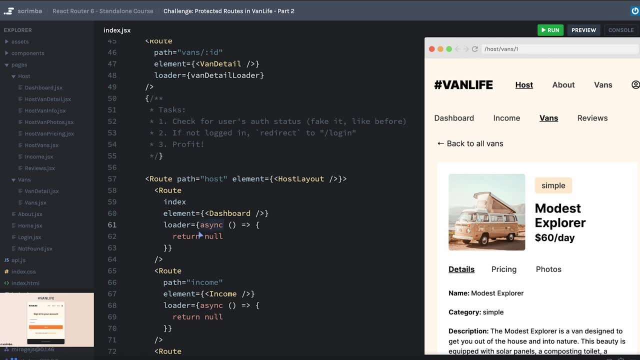 utils file, And then we do have the tedious task of including it in each one of our loaders. Now this brings me back to a point I made earlier about how our loader can be an async function. what we currently have in our utils, as this hard coded is logged in value and this conditional. 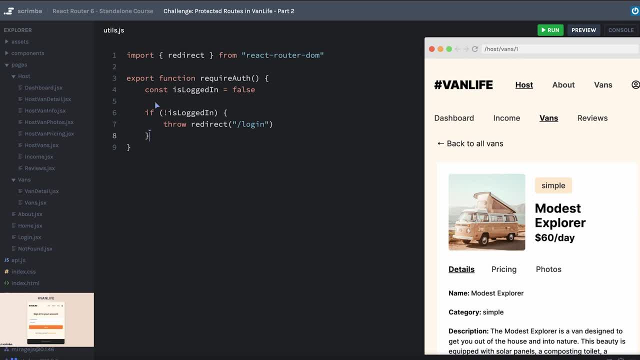 check. none of this is an asynchronous operation in JavaScript. this will just run line by line, and it will run very, very quickly. However, much more commonly, in require auth. we might be reaching out to a database of some sort, or a server rather, in order to ensure that. 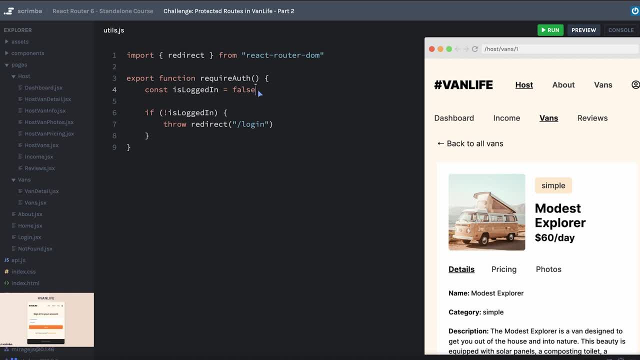 the user is currently logged in, And doing that may be an asynchronous operation, And so we don't want require auth to kick off a request and then continue doing fetches in the loaders if the person is not allowed to access that information. So, although what 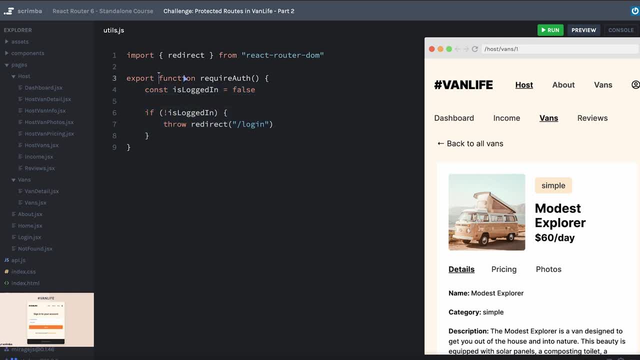 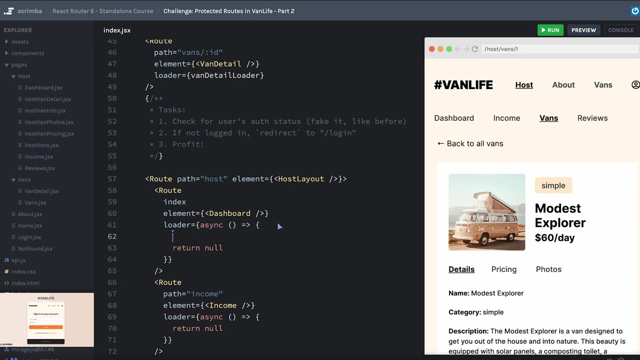 we currently have is all synchronous. we are going to pretend like it could potentially be asynchronous and turn require auth into a to an async function, which means that it's going to by default return a promise. And then we'll go over here and we will make use of all of our async functions by using 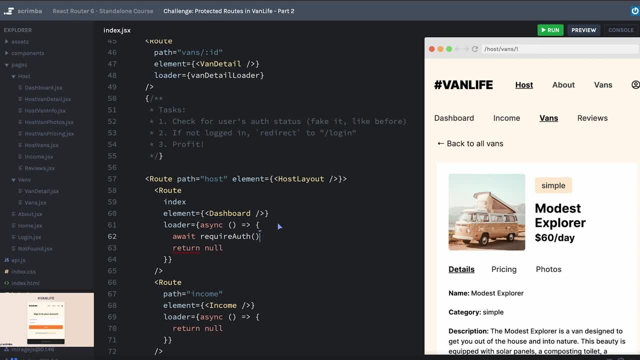 a weight. we're going to await require auth Again, even though we currently are doing synchronous operations with require auth. at some point in the future we may not anymore, And so it will be important that we wait for require auth to kind of authenticate the user. 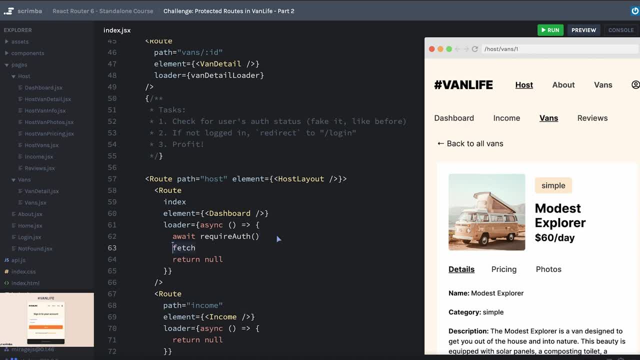 before we do any kind of fetching requests inside of our loaders. Most of these loaders are not doing any fetches, And if they were doing fetches, and if they are doing fetches, we are importing them as functions that come from the components, like this one right here. So that leaves us with 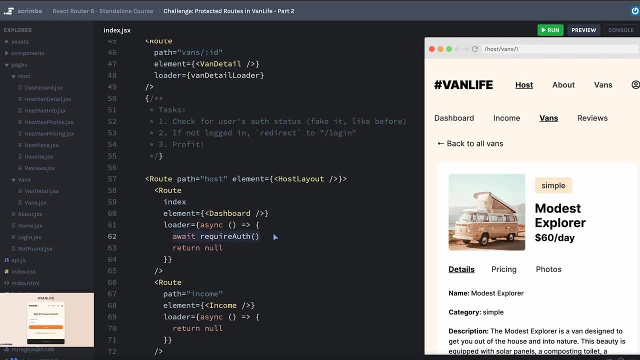 two different ways that we can make sure that we include this await, require auth everywhere that needs it as a protected route, And I actually think I want this to be a challenge because it is going to take just a little bit of critical thinking, So let me type out. 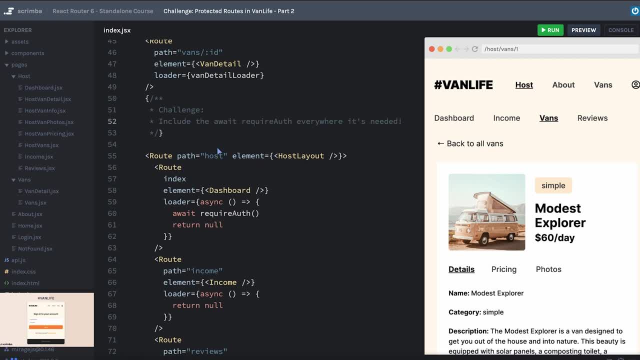 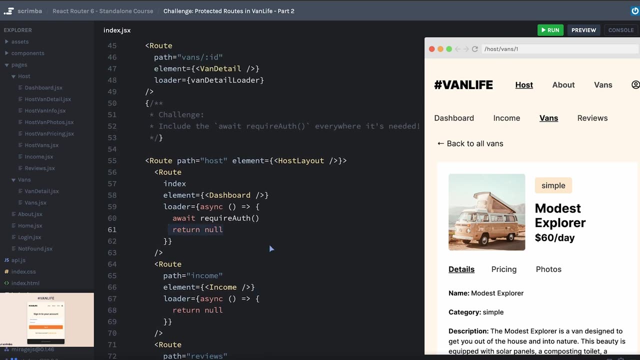 this challenge. Your challenge is to include this await, require auth everywhere that it is needed in order to protect all of our host routes and the nested routes therein. Now, one thing we can do just to simplify our code a little bit: this return null is a little bit extraneous. I can just say: return await require auth, and that should get the job done as well, So I won't need two extra lines, in which case, because I'm using an arrow function, I could simplify this by just having it do the implicit return. 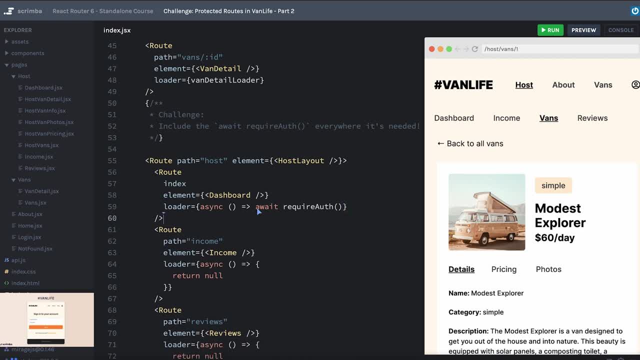 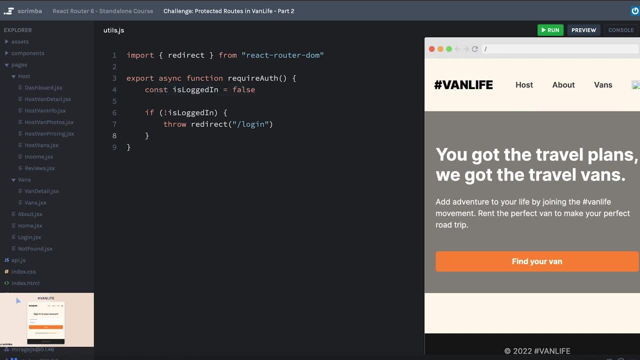 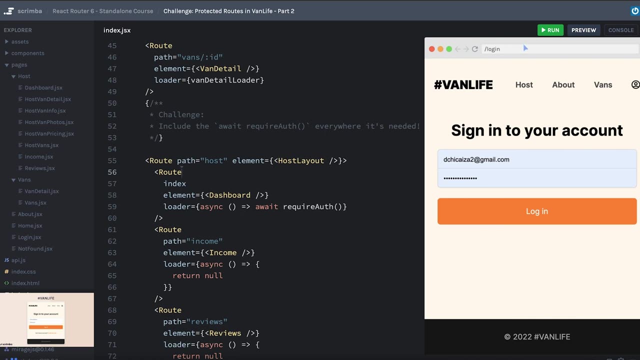 Okay. So let me go to the homepage. in our utils we are hard coding that we are not logged in, And so I'll hit refresh and try to get to the dashboard And, sure enough, it's taking us to the login page. Let's see if I go to slash host, slash vans, Okay, and we can see. 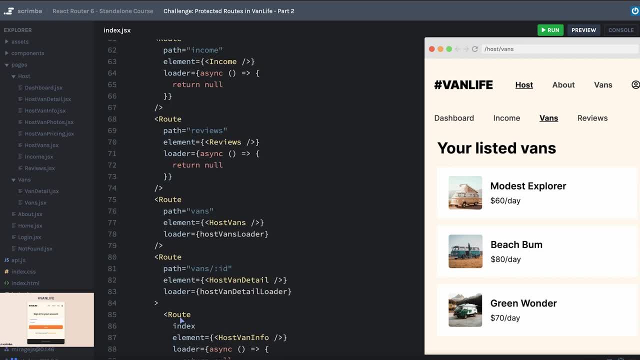 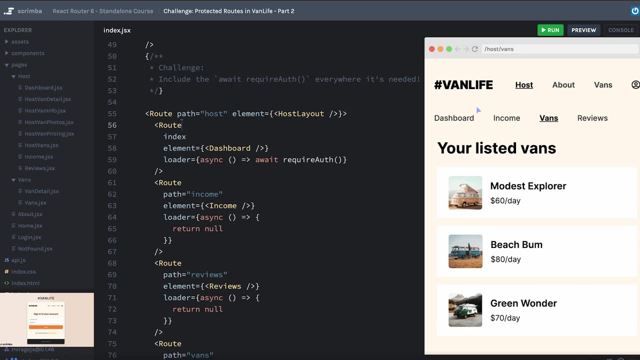 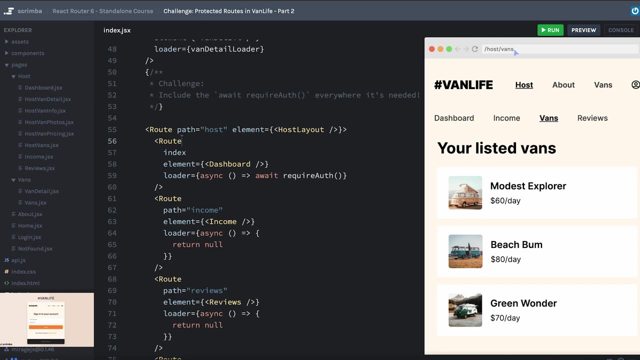 that I'm able to get to host vans because we haven't yet completed those protected routes. So that is your challenge: include, await, require, auth Everywhere it's needed, and it should make it, because we're hard coded as being logged out- it should make it so that you can't get to any of these host routes And you're probably. 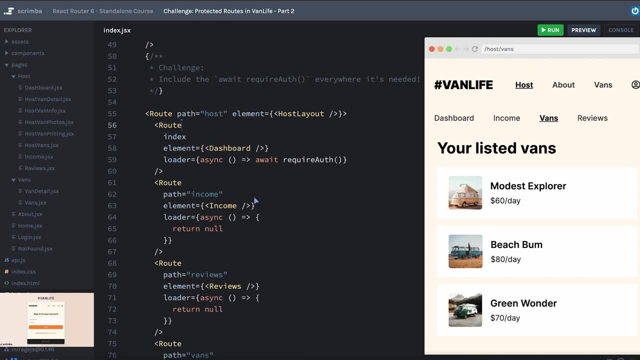 going to have to type a bunch of them out just to test. So one last thing: when it does come to the loaders that we're importing, things will have to change a little bit, as opposed to just tacking it on to the inline loader like we've done here. But I think you 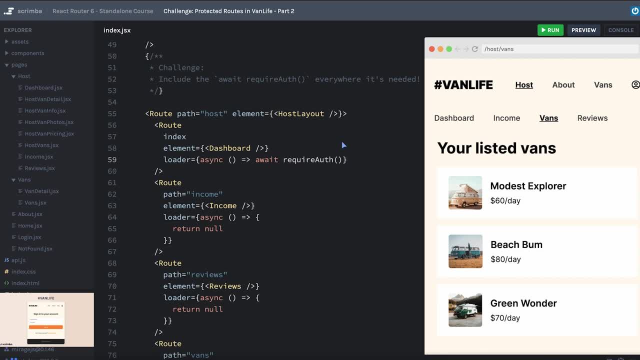 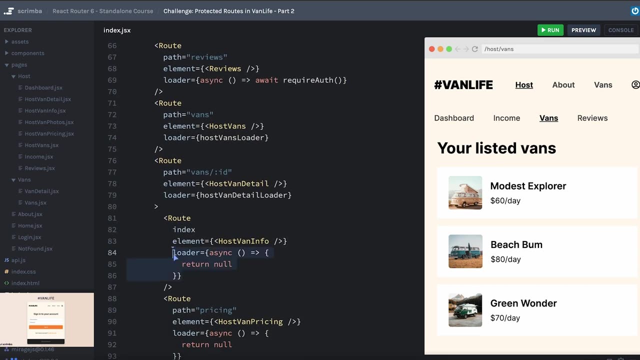 probably figured that out. Okay, pause, now work on this challenge. Okay, well, I should be able to just copy this loader and put it on every line that is still using an inline loader, So fortunately that covers a majority of our loaders here. 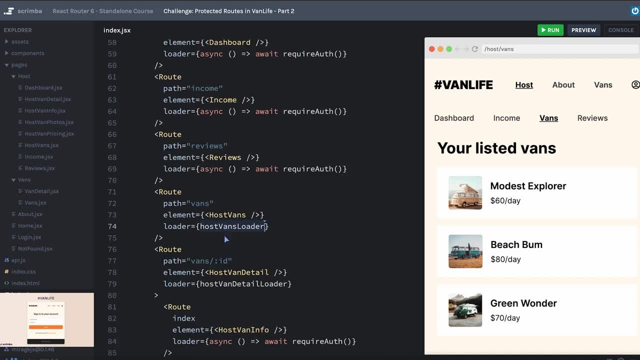 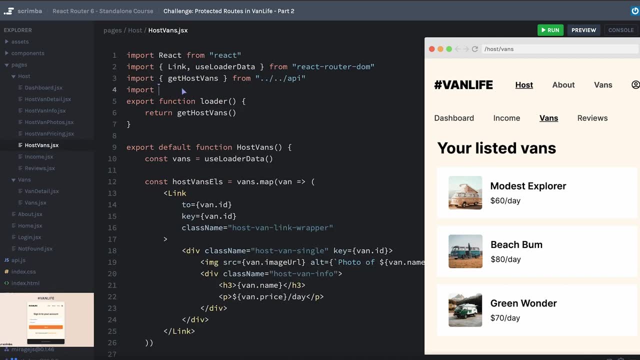 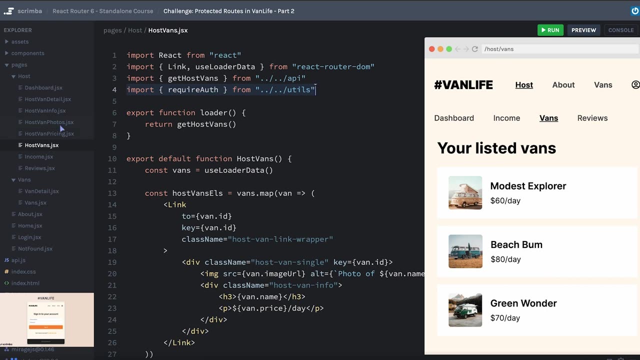 Okay, and then for the remaining two, with our host vans loader and our host van detail loader, we can go over to host vans and we need to import our require auth from the utils file. I'm going to copy this and just put it right over in host fan detail while I'm doing this. Okay, and then I'm going. 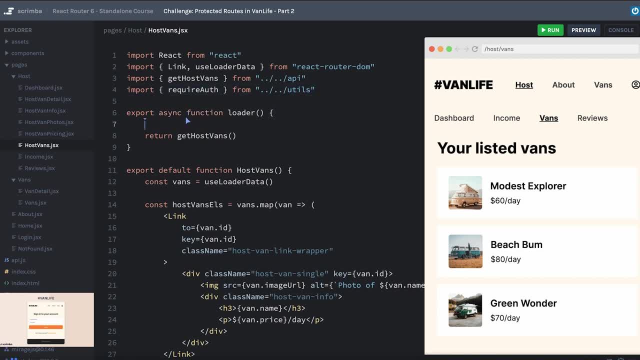 to make this an async function. This might have been one of the trickier things, But we did not make this async originally. But now we want to make it async so that we can await, require auth. Alternatively, we could just say: require auth, dot then and do promise. 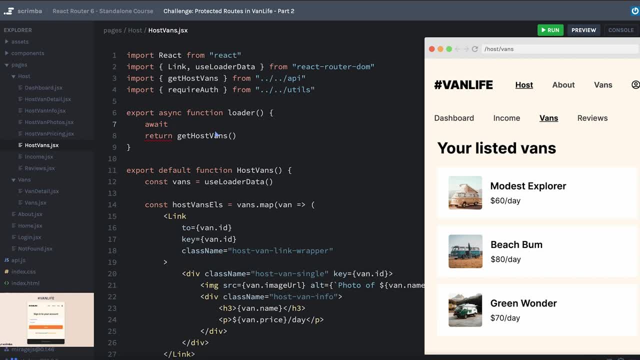 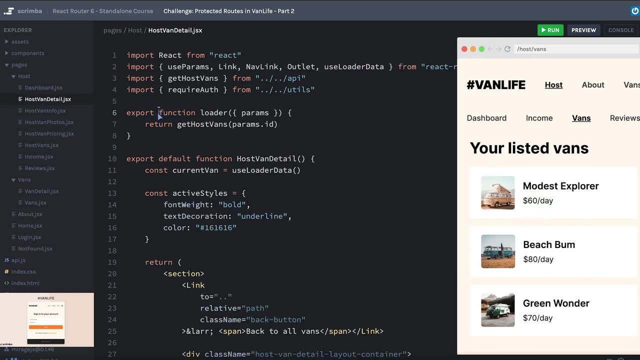 resolution that way, But I like the await keyword, So we'll say await require auth. that ensures that this function can run completely before it ever tries to get a list of the host fans. Okay, and then I should be able to go to my host fan detail, make this an async function and do the exact same thing. Okay, moment of truth. 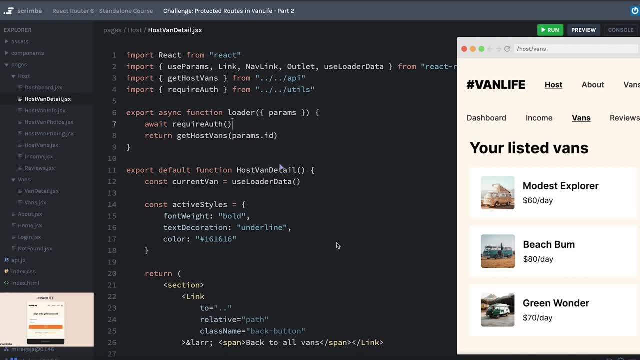 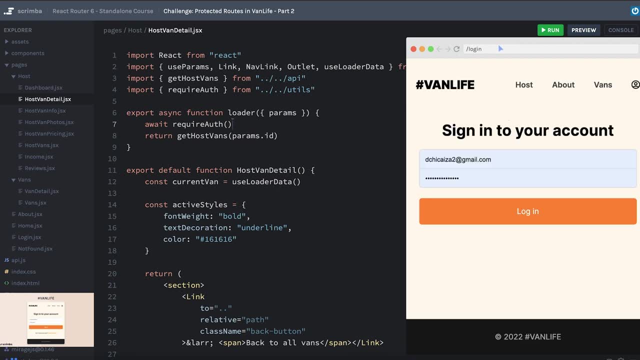 we were able to get to slash host slash fans before because we did not have a protected route there. We'll go ahead and refresh And sure enough, that took us to the login page. So if I try to go to slash host login page, slash host, slash vans, let's say, slash one slash photos. 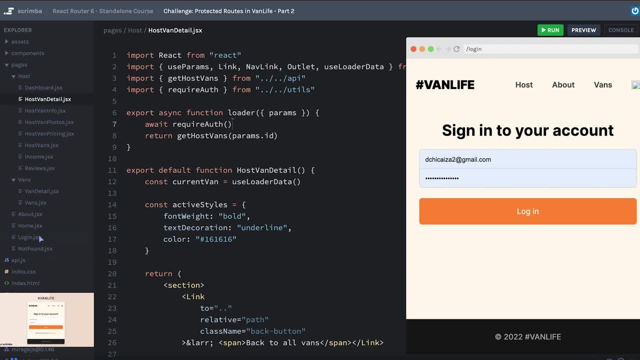 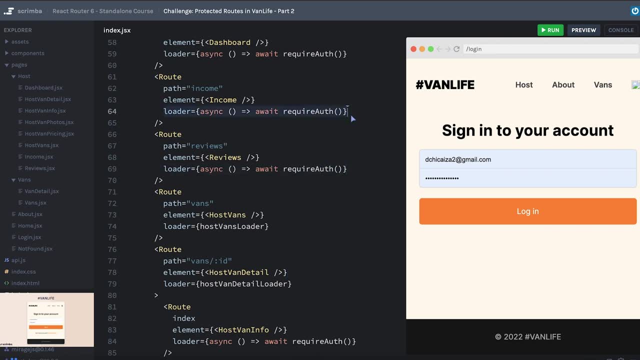 Awesome login page Also. I feel like once again, it's important that I point out that there currently is talks on better ways to handle this, where we can include middleware to the loaders that will run before any of the loaders, so that we will only have to do this in one place. But 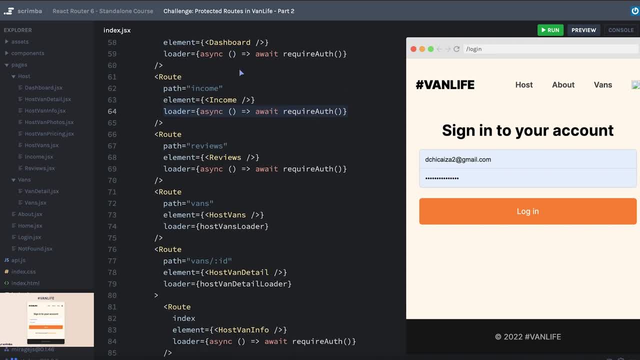 for now, this is what we have to work with, And even though there is quite a bit of representation, we're still going to be able to do this in one place. And even though there is repetition here, I still really like the way that loaders will run before the route transitions, and 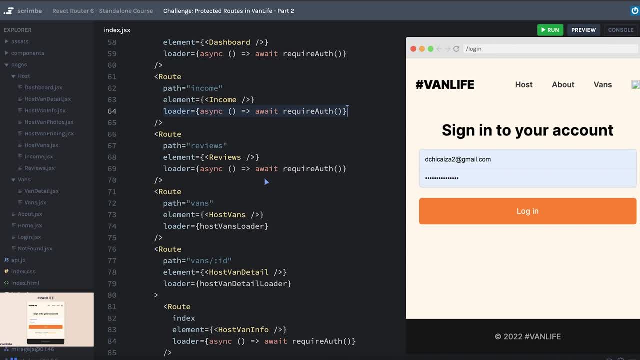 gives us a more synchronous feel to our components. No longer do we need to remember about render cycles and what will cause and what won't cause a re render in our components, then having to set up error states and loading states and all these other things that were really just about managing. 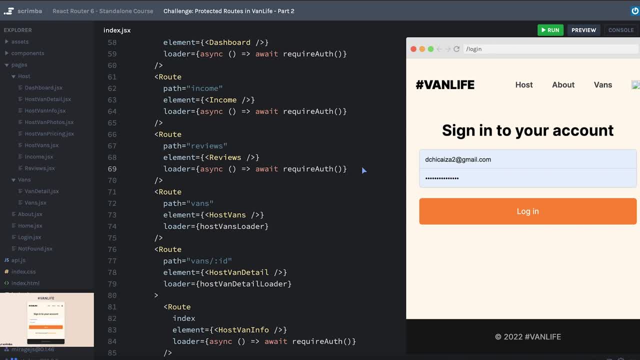 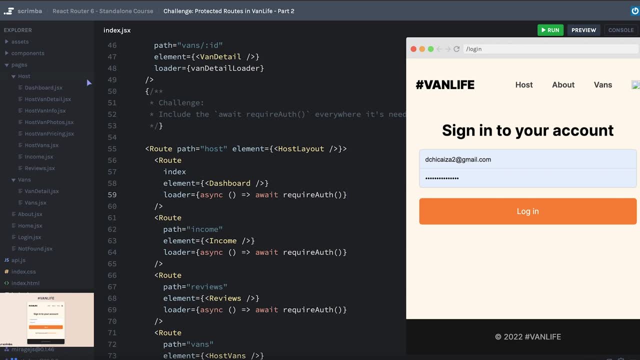 the react render cycle and not about managing our actual data that we care to use. So yes, you might be thinking to yourself: this is so much harder than just including an auth required component that wraps everything else. But for one, the benefits of using loaders in the correct way, I think, outweigh any of 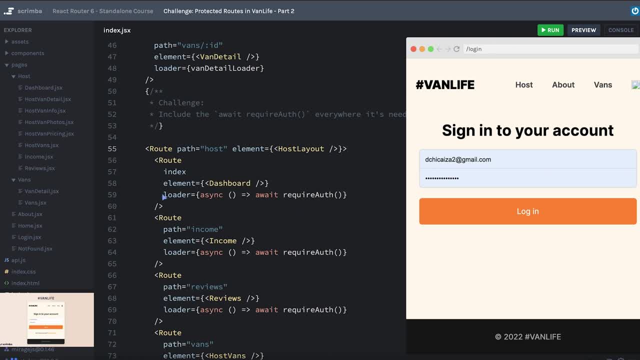 the costs that we have here And, secondly, we very likely might be getting a middleware solution to this problem. Okay, we've been staring at this login form for a while now and we haven't been able to make any use of it. Now that we are set up correctly, it's time for 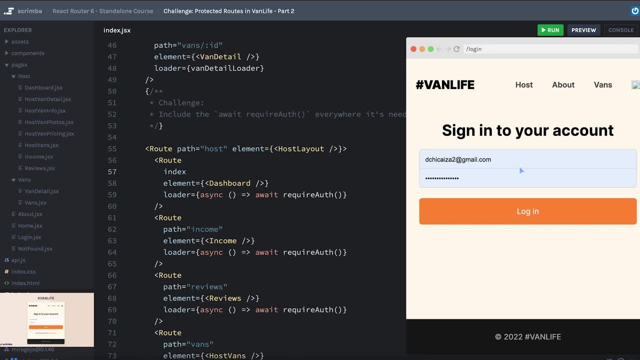 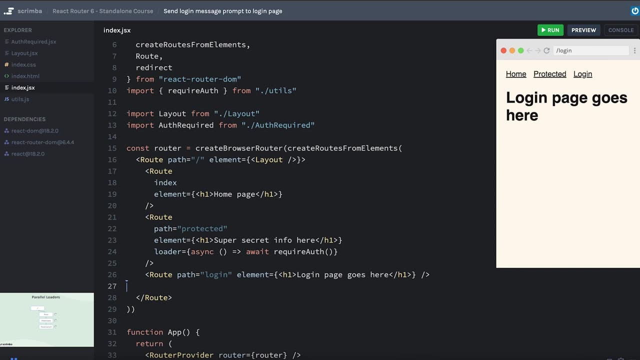 us to go in and actually make use of our form, And I can promise you you are going to fall in love with the way that forms can be handled with react router, using the data routers that we're learning about. So that's what we get to look forward to next. Here we are, back in our simplified app, And 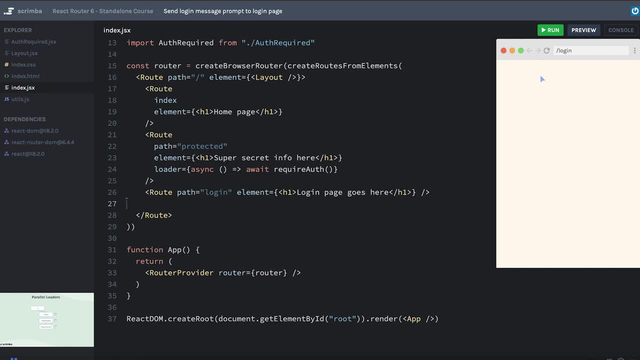 what we want to work on next is have it so that when someone tries to go to a protected route, that there's some kind of feedback that says: here's why I sent you to the login page. for example, they tried to get to protected. it sent them to login. we should probably display. 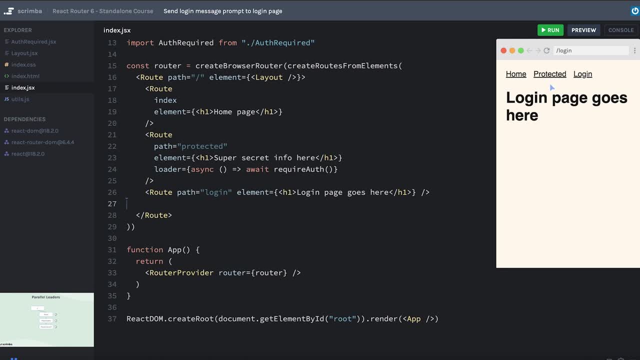 a message that says you must log in first. we don't want that message to show up when they just go directly to the login page. But if they try to go through a protected route and they are not logged in, we do want to display that message Now over in our auth required. this is the layout. 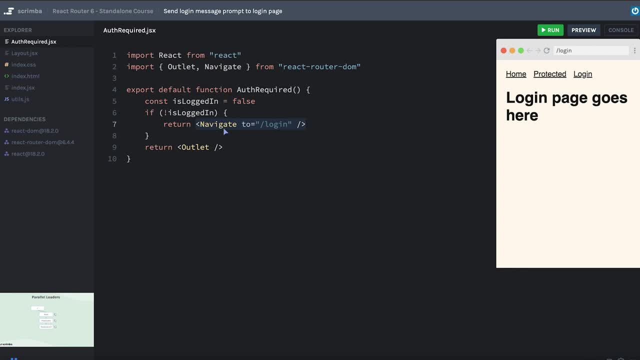 component When we were doing that before we were using loaders. you might remember that we have this navigate component. When you're not using loaders, you can just pass state, similar to how we did with links earlier in the course. you can pass state and that state could. 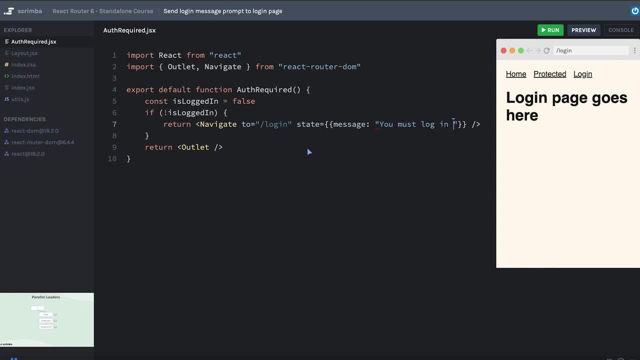 have a message that says you must log in first. This works because when you get to the login page you can check the location to see if there's a state dot message variable, And you do that with the use location hook. But now that we're not using the auth required layout route but instead, 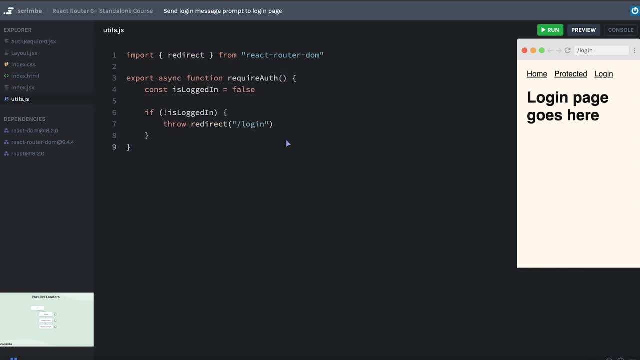 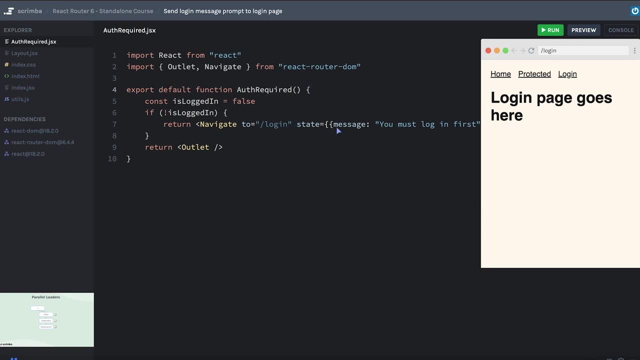 we're using this utilsjs In order to navigate or redirect people to the login page. we don't have the option to pass a state message through this navigate component, like we did Before. So how can we accomplish this when we are redirecting to the new location instead of using 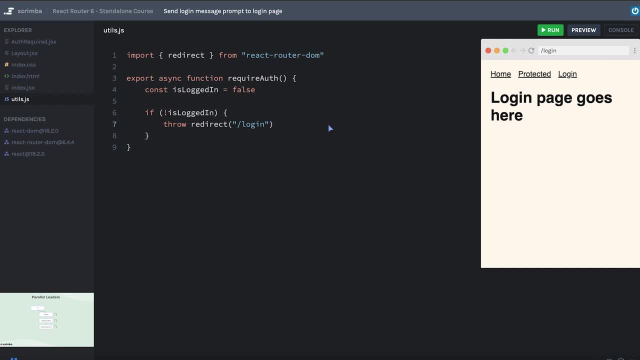 this navigate component. Well, the most common thing that I have seen is to include a search param that includes the message that you want to send along to the page that you're about to load. So in the require auth function here that's as simple as saying question mark, maybe something. 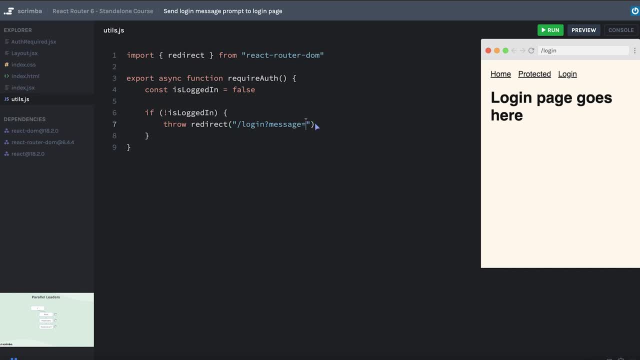 like message equals, and then we can include the message that we want to send. So you must log in first. Okay, let's see what this looks like. we should be able to see that in our browser, So I'll click protected. And now, if you look in the URL, it says not just slash login, but slash login question. 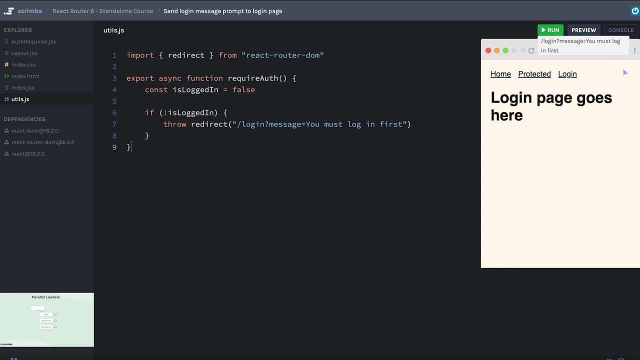 mark message equals you must log in first. you might notice that it's not URL encoded. If I hit refresh, it automatically gets URL encoded where we have the percent 20.. That's representing the spaces between the words. But even if we didn't have that it would work just fine. So let's go. 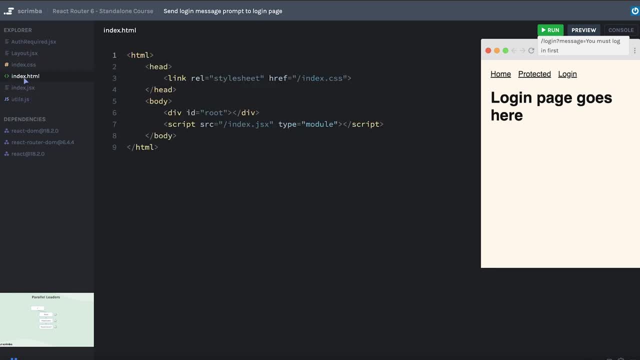 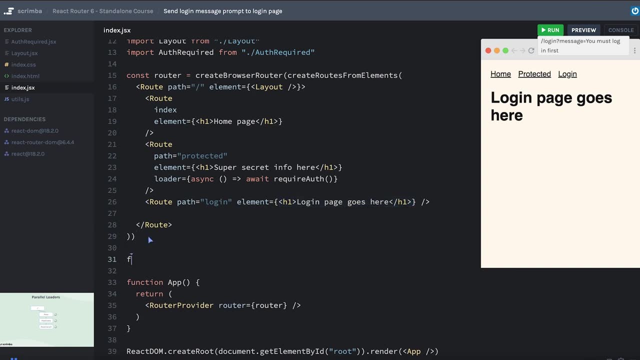 over to the login page, And that is not a dedicated login page here, It's just this h1,, which means at this point it might be worth just throwing together a quick login component. So I'll do that really quick, Okay. so now I have this. 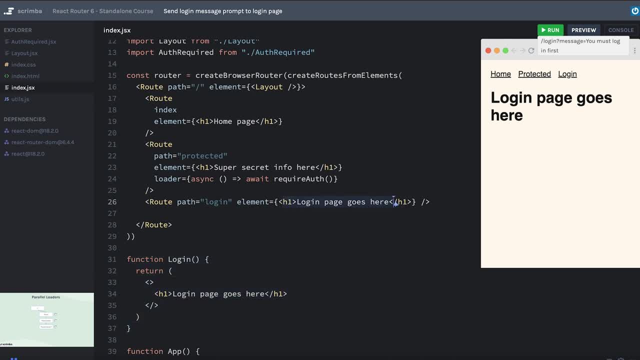 login component. And then, instead of rendering an h1, I'm just going to render my login component. And now I should essentially have the same thing, So I'll hit refresh. login page goes here: Awesome, Okay, now that we have a dedicated login component, in the next scrim we're going to see how we can. 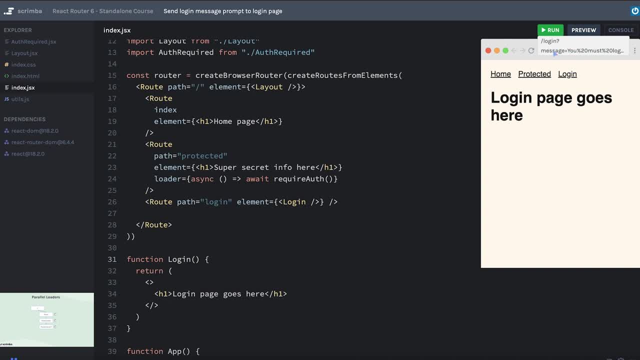 actually pull in the login component. So let's go ahead and do that. So I'm going to go ahead and use the query string that's saved in the search param of message so that we can display it on our login page. Then, once we've done that, we'll go back to van life And you'll have a challenge. 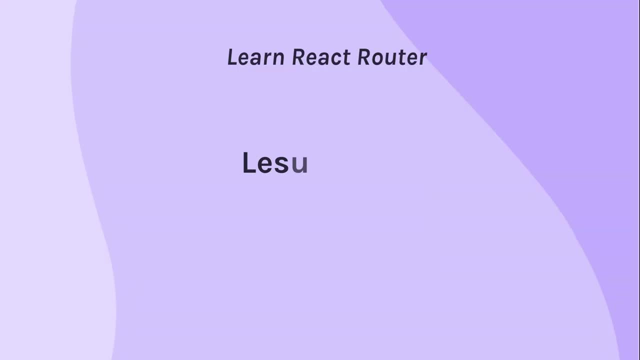 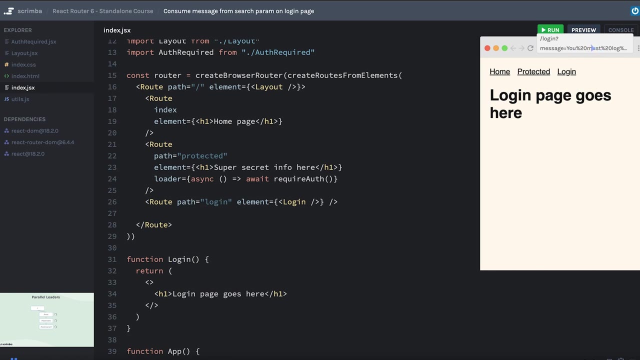 where you get to implement this in the van life app. Let's see how our login component can consume the query string that exists up in the URL, if it exists, when it gets to the login page. And actually, what I want to do is have just a quick thought experiment for you. I want you to think. 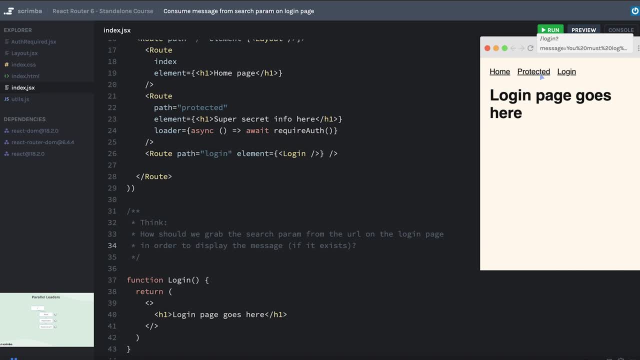 about this in our login component. how should we grab the search param from the URL on the login page in the login component in order to display that message, if it exists? I'm not asking how we should display the message. I'm asking how should we get the value from the search param of message. 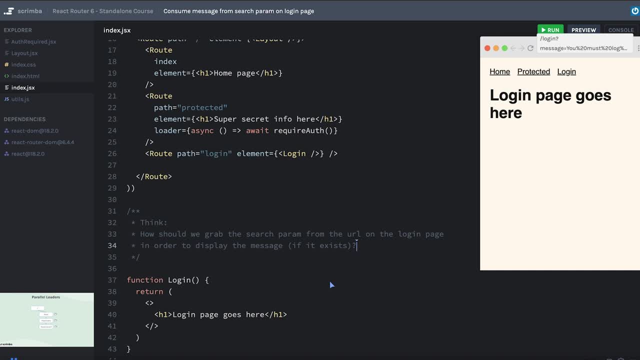 So I'd actually like you to pause and think through this, try to come up with an answer. if you want, you can even click into here and type down your answer. So pause now and see if you can come up with an answer to this question. 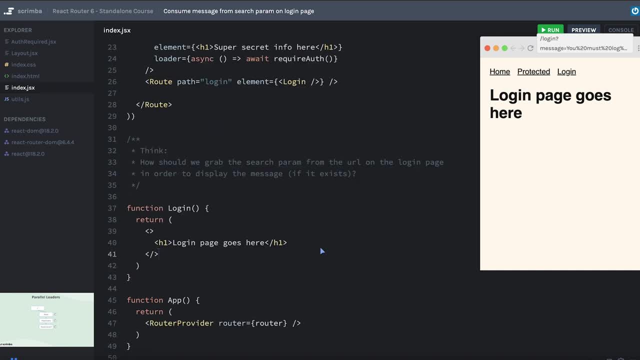 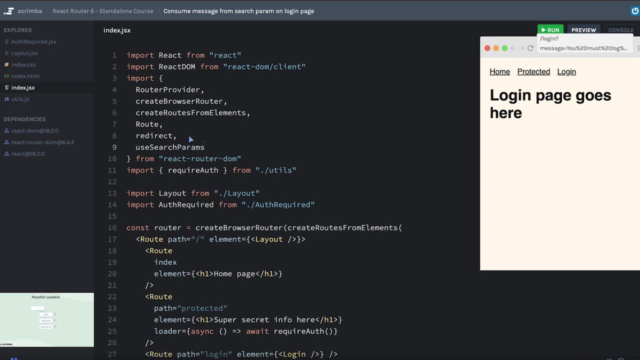 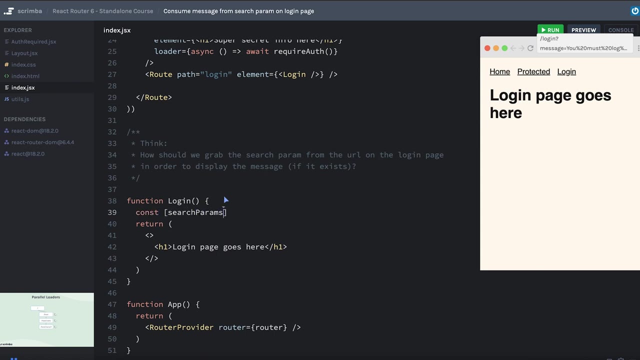 Well, the first thought that you may have had. if you remembered, way back at the beginning of this course, we learned about the use search params hook which we can use inside of our component, And then that gives us access to the search params and a function to set the search params. 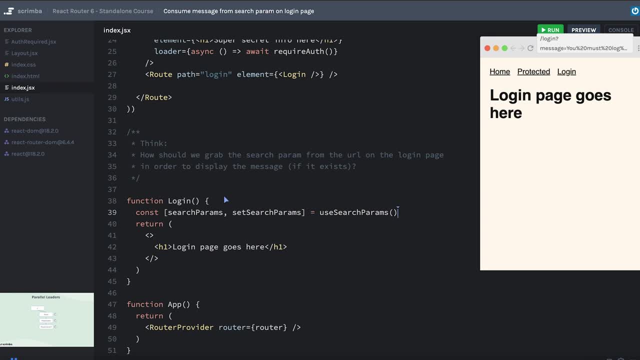 And that's equal to use search params. I'm mostly going down this path to show you that it should work just fine. I can console log and remember this search params is actually the native web search params- constructor or object, And so it has a parameter called dot get and I can ask it to get the message And we'll go ahead. 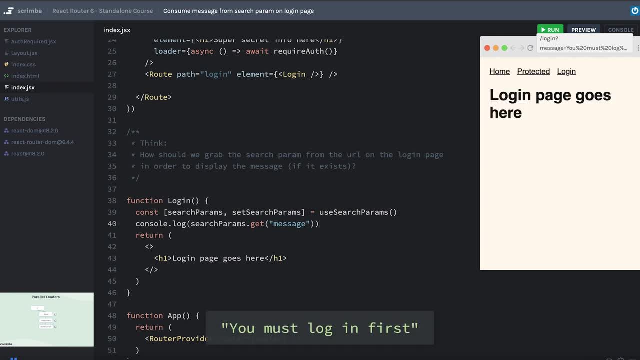 and console log that. So let's just give it a shot. I'll hit refresh, open the console And, sure enough, we get access to our search params that are in the URL. However, now that we're using the data router, it can be really beneficial for us to just go all in both feet into really working. 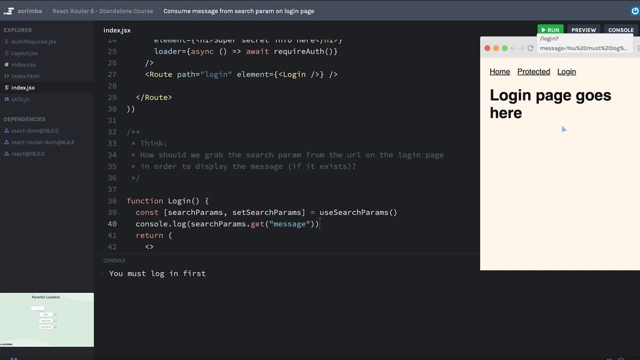 with those API I that we get with the data router, including using a loader. So another way that we could get the search params- let me comment this out- is to include a loader. So I will have a loader function And in this case I don't need to export it because I'm just kind of stuffing everything into 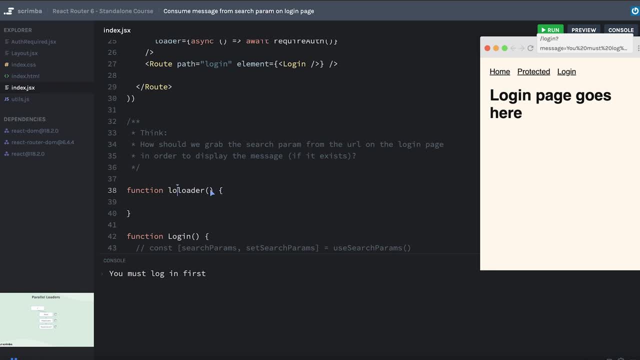 one file here. Maybe, just for the sake of keeping our names similar, we'll call this the login loader, And the login loader, just like we saw before, where it can have access to a params object, it also will have access to a loader. So we'll call this a loader, And then we'll go ahead and 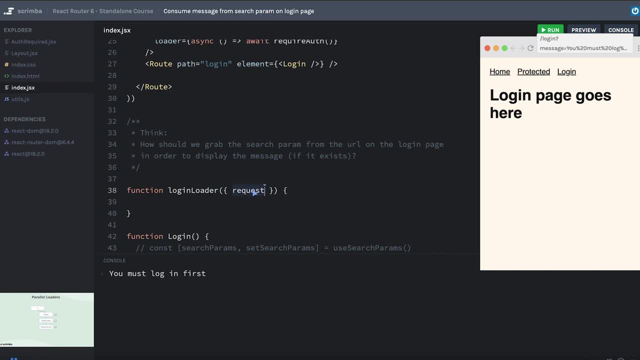 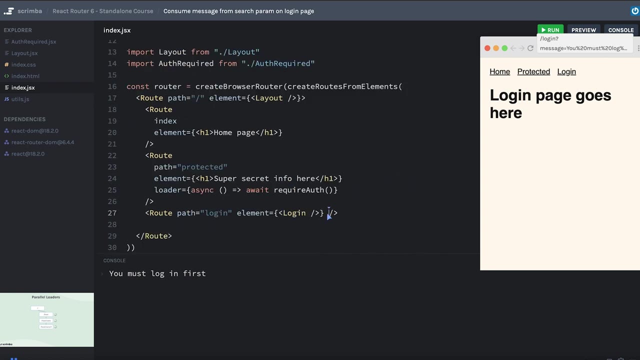 just log in to this loader. Okay, so we'll go ahead and we'll click on the loader And we'll see that we have access to the full request object. this request object is a native web request object that you could just go to MDN and learn more about. So let's go ahead and console log this request. 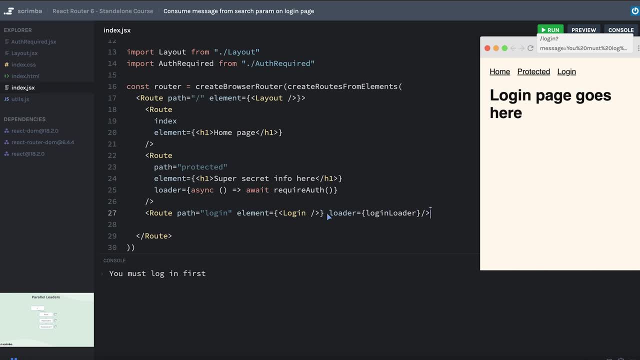 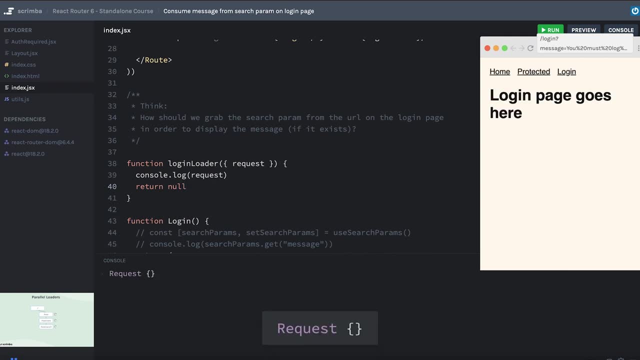 And I need to set my login loader up on my login page. So we'll say that this has a loader that's equal to the login loader, And just so we don't get that error, we will just return null for now. go object: capital R, request object which represents an object that has a request constructor And in. 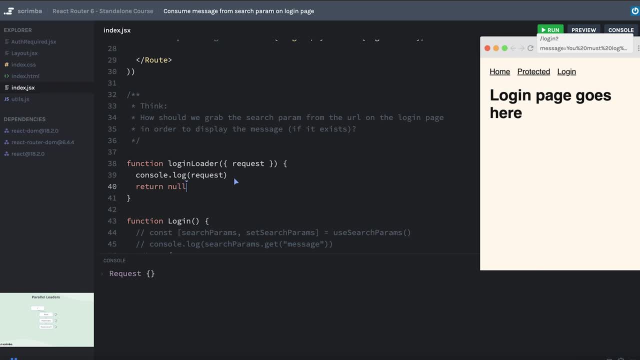 this case, like I mentioned, it's coming from the web. this is not something specific to react router. this request object has a URL property, So I can console log that and we can see the full URL. that does include the search params at the end. If you look in the console, there's the 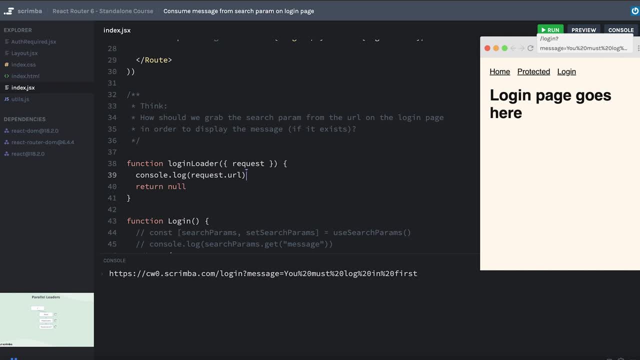 question mark message equals and then the HTML encoded. you must log in first. So what we can do with that request URL is create again another native constructor called URL, And so I can use the capitals URL instructor, which will give us a URL object And, as I mentioned, this again is just. 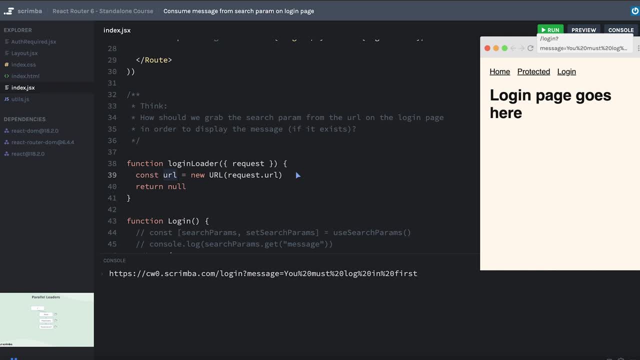 a native web interface. That's one of the things: that if you get involved with the new react router and the remix team, they will constantly be telling you that they're just using the platform. there's no need to reinvent the wheel when these tools are really amazing And they've been at our 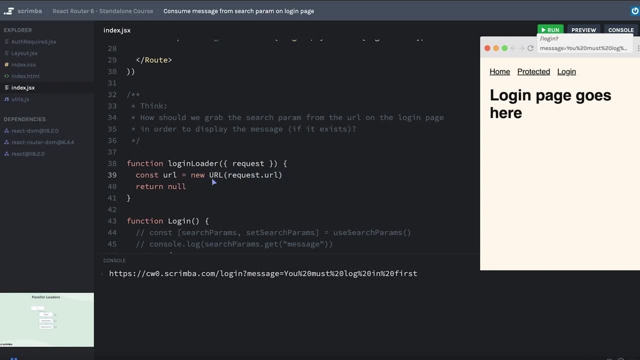 fingertips in JavaScript For many, many years. if you were to go to MDN and learn about URL, you would also learn that you can access the search params object on top of that, And that object is an instance of the search params constructor, also from the native web. So if I were to, let's go ahead and console. 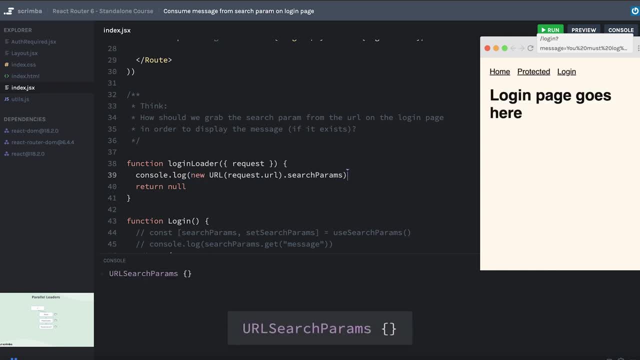 log this whole thing And we can see that I get an instance of URL search params. This is exactly what we had down here where we can run this dot get message on top of it, And so let's go ahead and add that on dot get message And we'll just console log that whole. 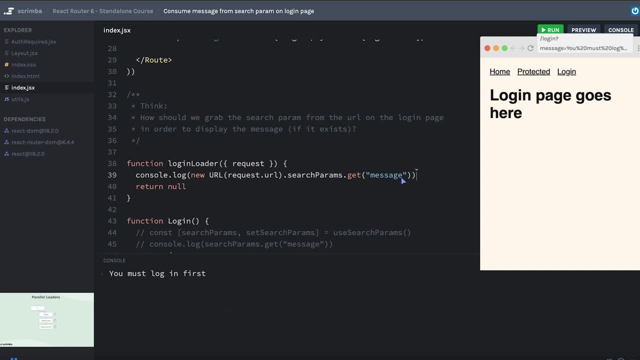 thing And, sure enough, we are back to a place where we have our message, And I know that this looks a bit more verbose than what we had before, But I would argue that what you're writing here is much more akin to native JavaScript for the web, as opposed to something that has been created by 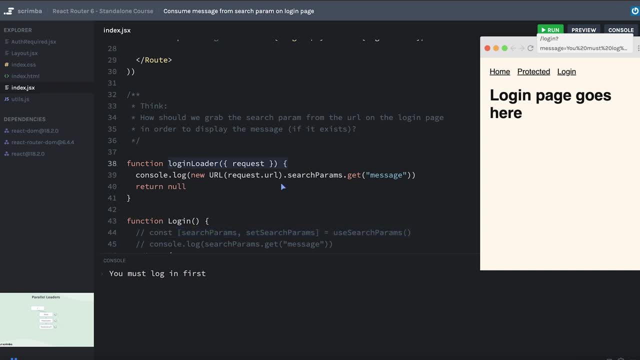 a third party library, Obviously loaders and the whole concept here, this request object is being passed in by that third party library, But in the meantime you have just become more knowledgeable on the native web, So I think that's pretty cool. Again, I'm probably just nerding out about this, So I'm going to go ahead. 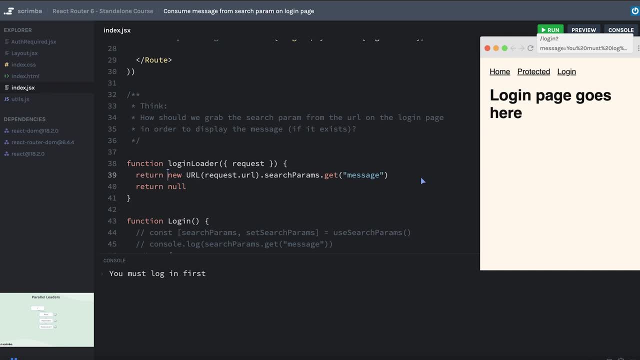 and well, this is all chained together. So I'm just going to return the message that comes back from this search params. we can get rid of this, return null. And now I want you to think how can I grab the information from my loader inside of my login component? In fact, I'll just go ahead and 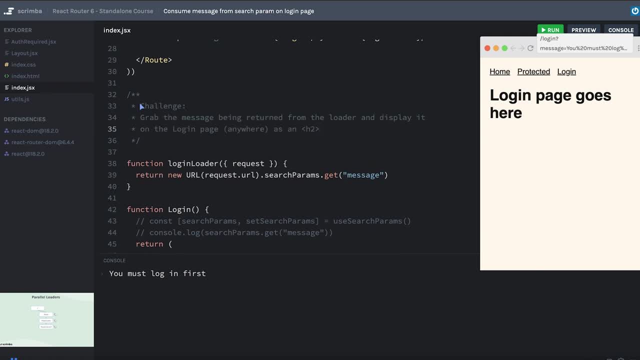 make that a challenge. Okay, so the challenge is to grab the message that's being returned from the loader right here and display it on the login page. I'll go ahead and just erase these two lines And you can display it either. I guess you only have two options: It's either above the h1 or below the h1.. And just go. 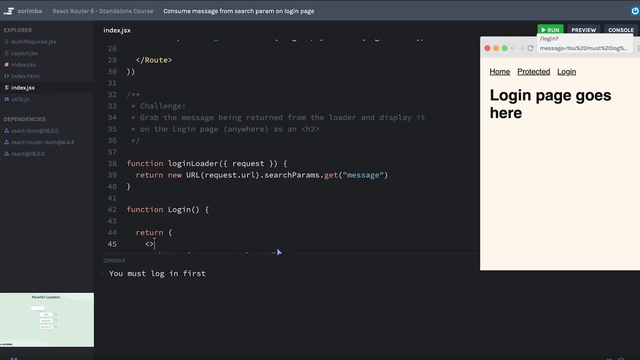 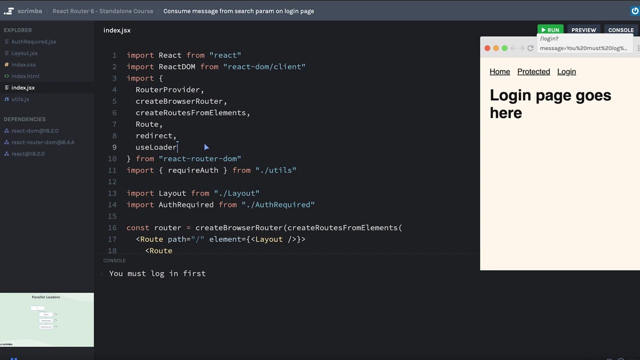 ahead and make it an h2 on the page. Pause now and work on this challenge. In order to get information from the loader, we need to use the loader And we're going to use the loader And we're going to use use loader data. I don't need this use search params anymore, So I will grab use loader data. 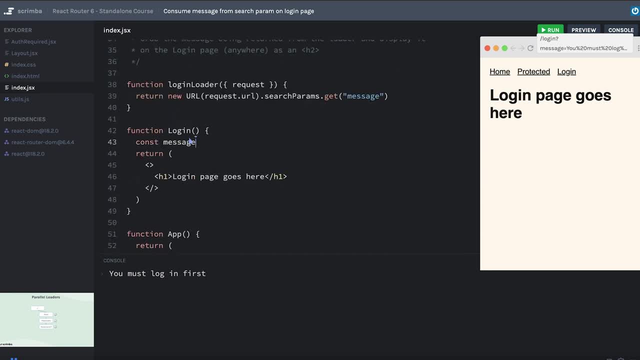 instead, And down here I can grab the message from: use loader data And let's go ahead and console log that message, just to make sure that it came through. Okay, Okay, we successfully got. you must log in first. But I am curious, before we finish this up, what happens if I just go to slash login. 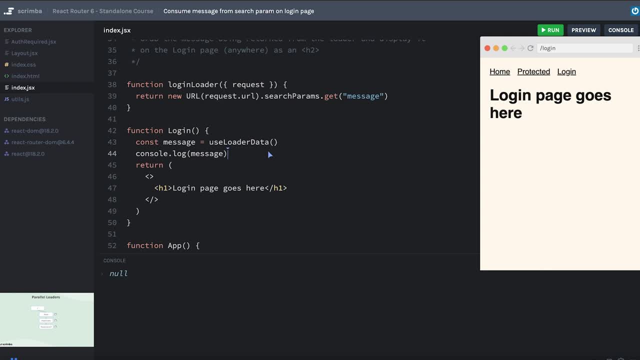 instead. Okay, we do get null. Okay, so, getting a value from the loader, I'm going to go ahead and go ahead and add a value of null- is not too big of a deal If I try to render an h2 that has the. 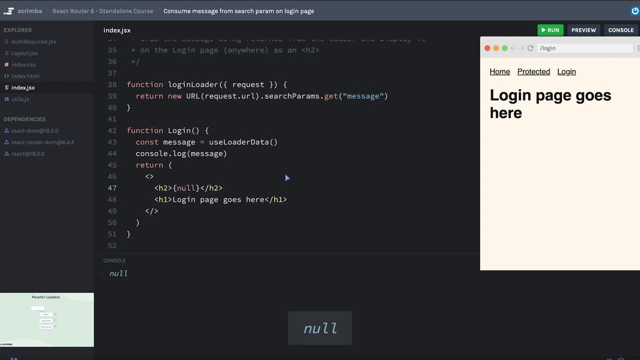 JavaScript value of null in it, then it simply doesn't display anything. But if you go into the developer tools, it will show a completely empty h2, which feels a little bit extraneous to me. Plus, I think it's informative to do a conditional render here so that other developers might see. 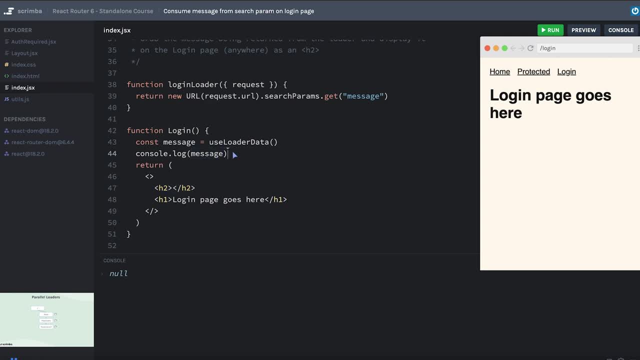 this and know that it's possible that this message will be null, And so I am going to do that. I'm going to, instead of having just an h2, I'll go ahead and do a conditional rendering that says: if there's a message, then I. 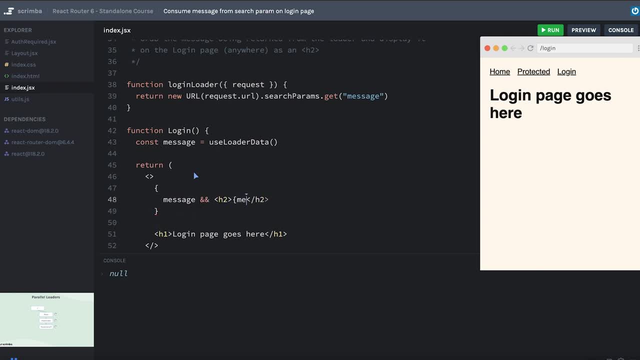 will display an h2 that has the value of that message in it, And this isn't long enough to be on its own line. Let's go ahead and just put this all in one place. Okay, we're on the login page. we'll hit refresh. there's no message there because we didn't come from a protected route. 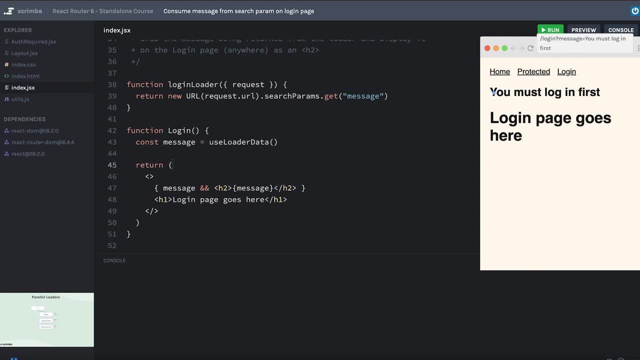 And then I'll click protected And awesome, we get our message. you must log in first. Now. I know we spent a lot of time talking about this message, But in the end we did was we added this message inside of our require auth function. we added a loader to our 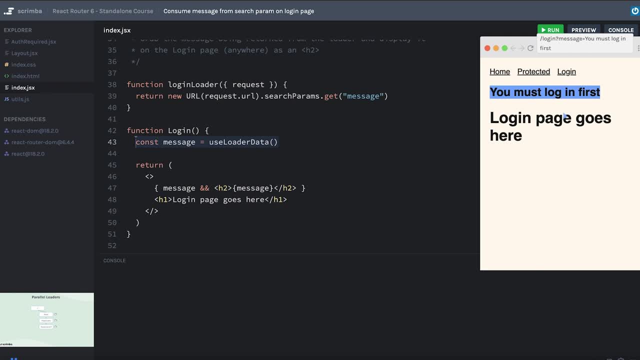 login page in order to load whatever data might be necessary to correctly display this page, And then we did a conditional render. if that message exists, then display it in an h2.. Obviously, we'd probably want to make it red or something that will stand out a little more. Okay, let's go take. 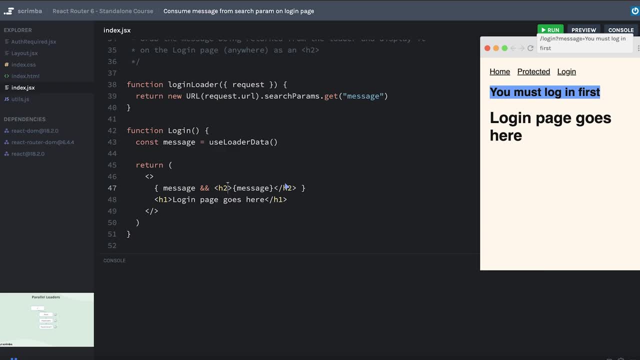 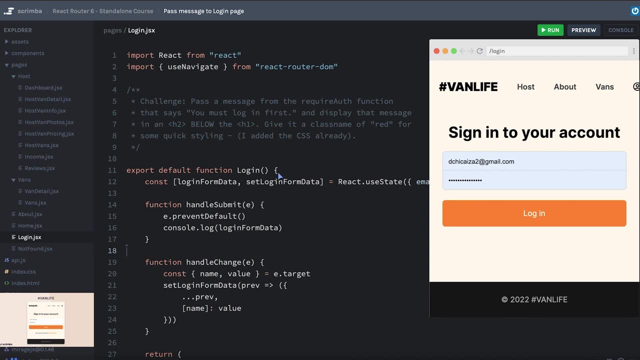 all of this new information and apply it to the van life app. Okay, let's put together what we just learned by passing a message from the require auth function, which is down here in the utils js file, that says you must log in first and display that message in. 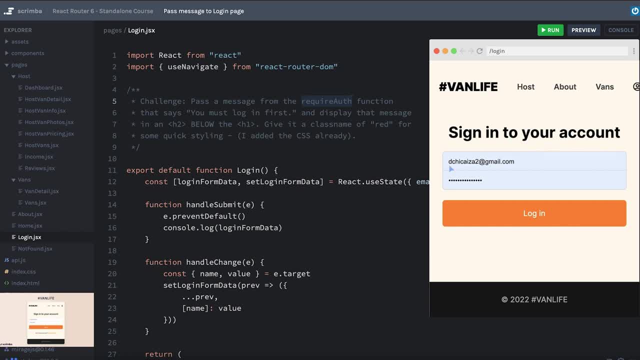 an h2 below the h1 that says sign into your account. I wrote some CSS that just has a simple red class And so you can just add a class name of red to get some quick styling. And yeah, that's it. I'm not going to go too much more into detail. to give you a chance to think critically and 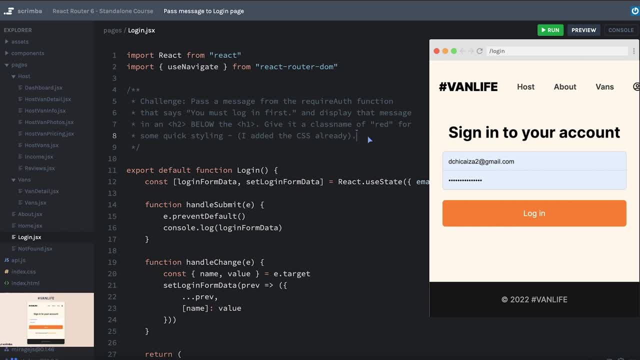 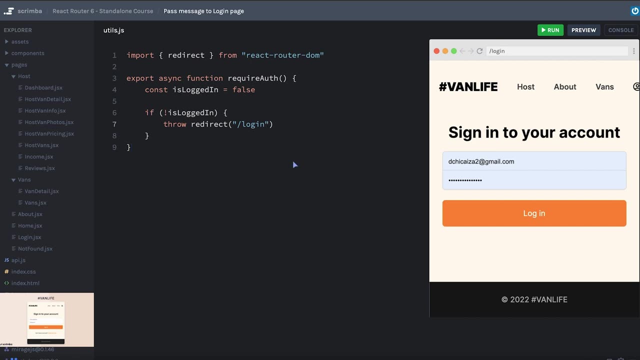 actually write all the code you need. So pause now and work on the challenge. Well, we could start from pretty much anywhere, But let's go to utils js And I'll just say: we'll throw the redirect to slash login. question mark message equals: you must log in first. Okay, easy. 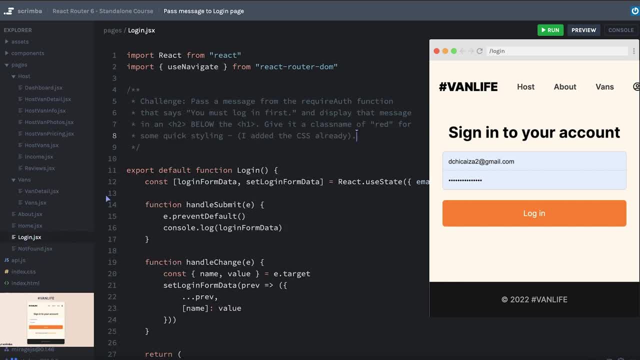 enough, Then I could make a decision. if I wanted to use the use search params hook, I could do that and it would probably work just fine. But again, in an effort to really keep with the theme of loading any data that we need for our login component inside of a loader, that's. 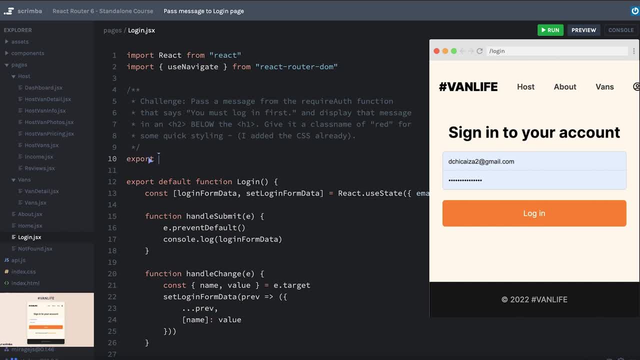 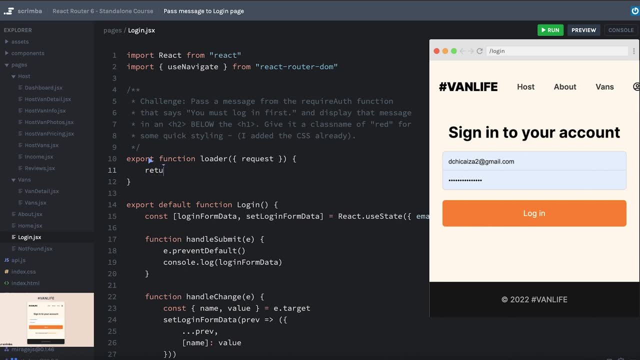 associated with this component. I'm going to go ahead and export a function called loader- And I already know that I'm going to need access to the request- And we'll just go ahead and chain everything kind of like we did before, if it makes more sense to you to split it out where you get. 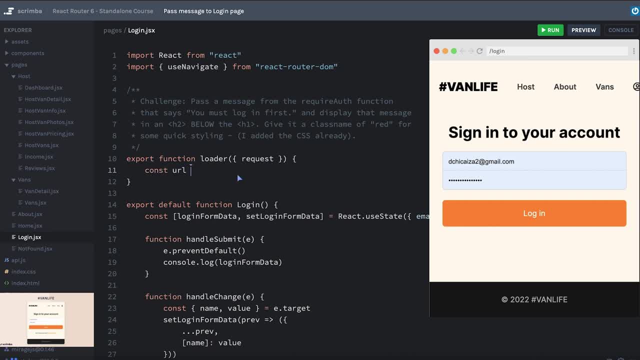 the URL and that's equal to the new URL of request that URL. and then you get the search params and then you return the value of message. that's totally fine. I'm just going to do it all in one, So we'll say: new URL of request that URL. that will give me an. 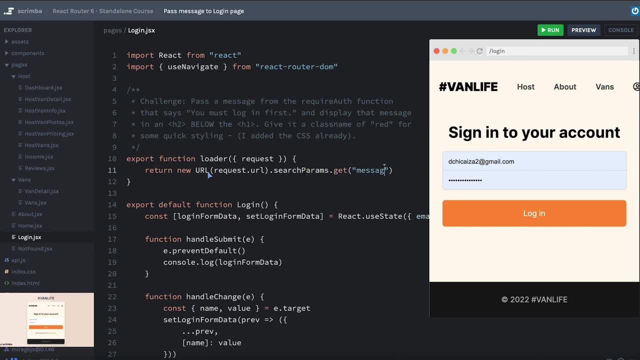 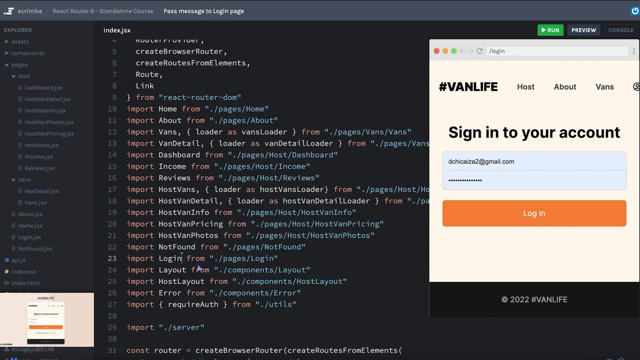 object of search params which I can use the method of get on and get the message. Okay, I'm exporting this loader And before I can do any kind of use loader data I need to make sure that I go over to my route definitions And let's import it. Let's see, here's our login, So we'll import the. 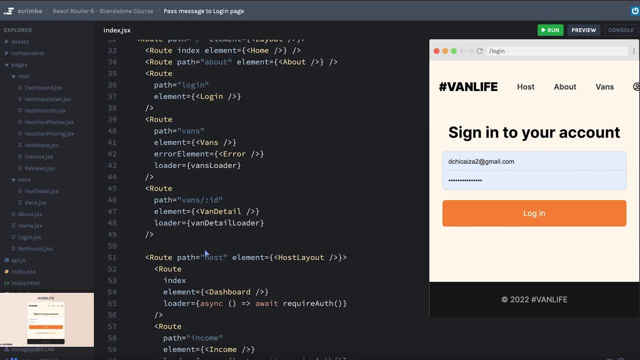 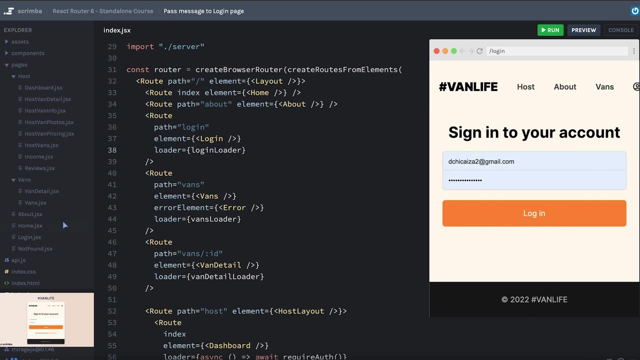 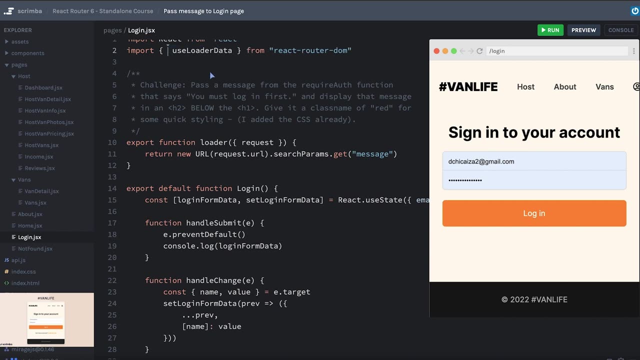 loader as login loader and then add it to my login page, which is right here near the top. So my loader is equal to the login loader. Okay, that means here I can grab, use loader data, And actually you know what I think this is a remnant. 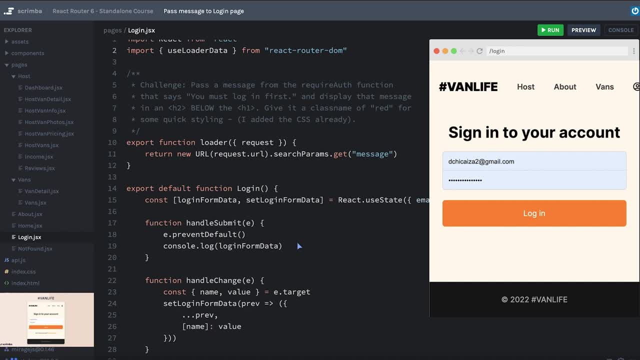 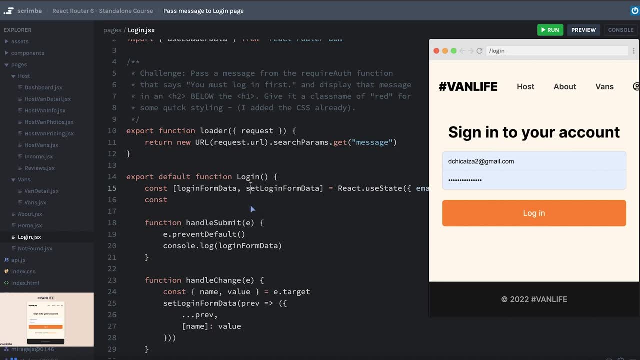 from when I was testing something before. we don't need the use navigate hook right now, So I'm going to get my use loader data. we will do it right here after state, which, as a sneak peek, I'm really excited to get rid of. we're going to clean up this form quite a bit with the abilities that come. 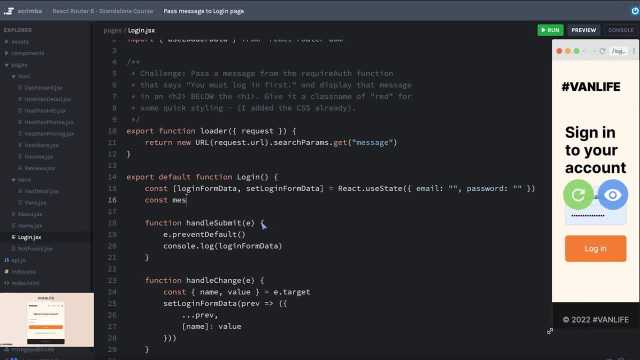 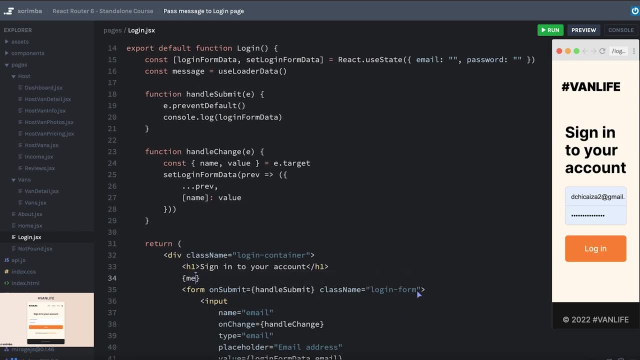 from the new data routers, So get excited about that. Now I can get the message by accessing use loader data And then, just like I did before, I will conditionally render it and we'll say: if there's a message, then we want. 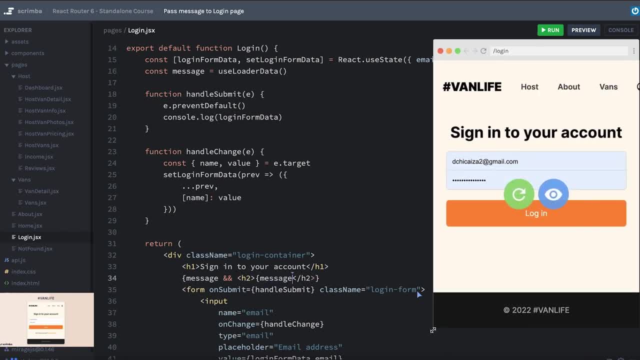 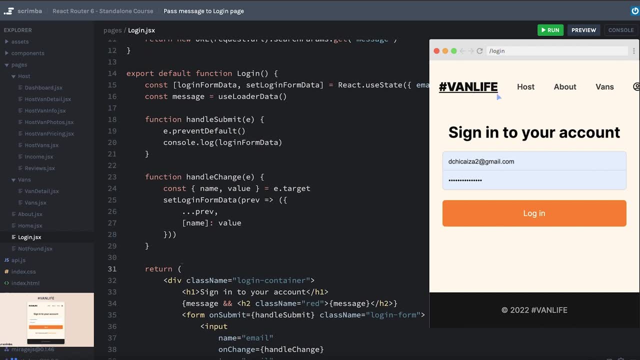 to display an h2 that contains the text of that message and has a class name of red. Okay, let's see how we did. We're at the login page, So we shouldn't have any kind of message when we refresh. But now, 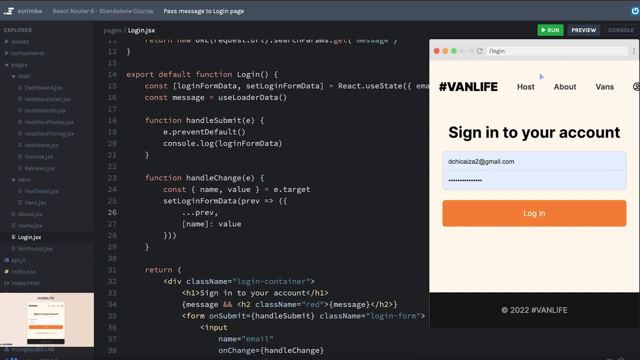 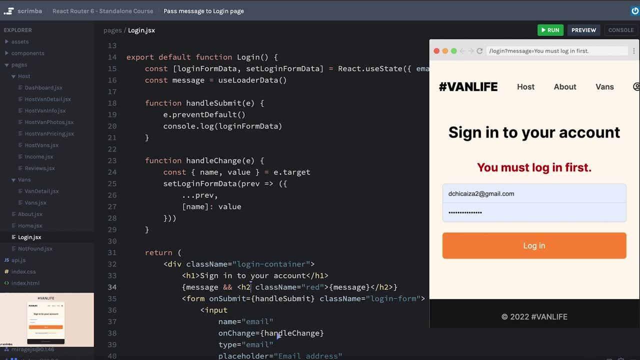 if I go to the host page, which is protected by our require auth function, I get that message in my URL And, sure enough, it shows up on my page. I'm gonna make a quick judgment call. the h2 looks a little imposing. Maybe I'll bump this down. 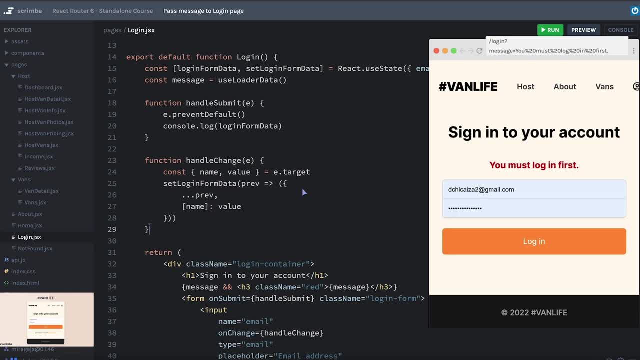 just a tiny bit to an h3.. Okay, that's a little less intense. Hopefully all that went okay. I know that was quite a number of scrims just to pass this message here, But we are going to be coming back and passing additional things as we are doing our redirect, which will make the user 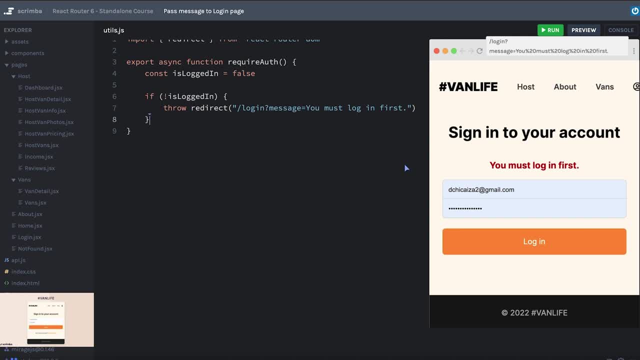 experience even better, But that's going to happen a little bit in the future. But we're going to be coming back and passing additional things as we are doing our redirect, which will make the user experience even better, But that's going to happen a little bit in the future. For now, it's finally. 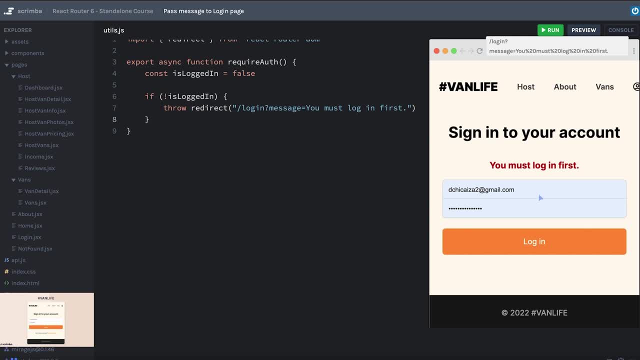 time for us to come back to our form and actually start learning about how forms are made so much simpler in react router if we use something called an action, which is kind of a sibling to loaders. So get excited, That's what's coming up next. 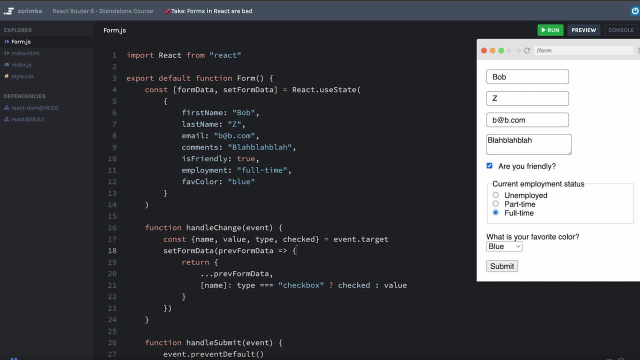 I've got a bit of a hot take to add to this course, And that is the fact that forms in react are just bad. There's a number of libraries out there that attempt to make forms in react a little more bearable, But the truth is they're just a really difficult thing to work with in react. you can get used to it. 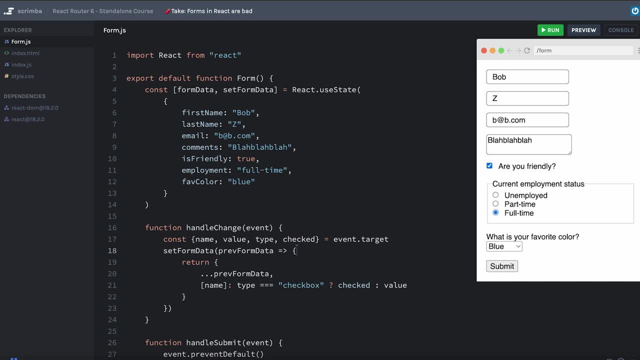 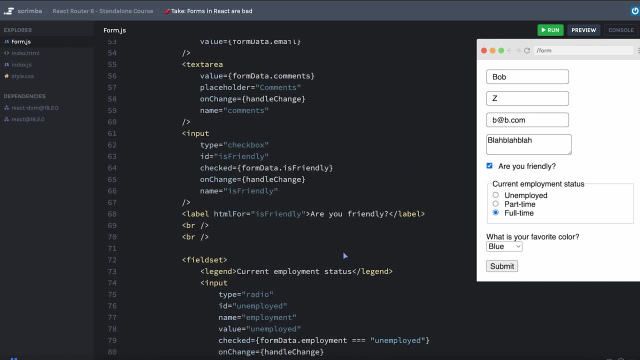 and you can get good at them, But they're still pretty difficult And the reason is we try to build a system over the top of the native input form elements that attempts to bypass the state management that already happens natively, internally by forms and brings that out into react and forces react to. 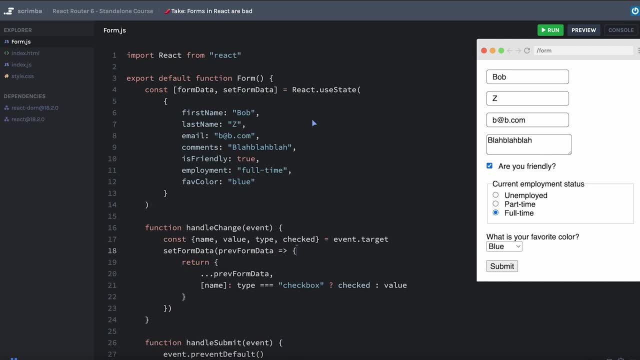 maintain all of that information. You can see in this form, which I copy and pasted for my learn- react for free course- that we have to create our own state that manages every piece of data that we're trying to maintain. We also have this handle. 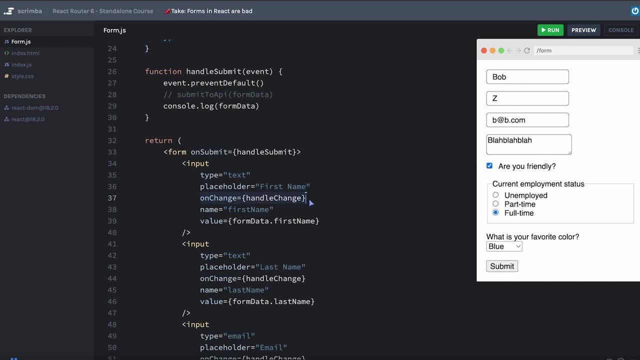 change event, which is put on every single input and manually tracks any keystroke or change that happens to the input in order to update state. And then we have to control the value, So we have to tell the input that its value is what is being held in state. And all of this is sort of extra on top of what is already. 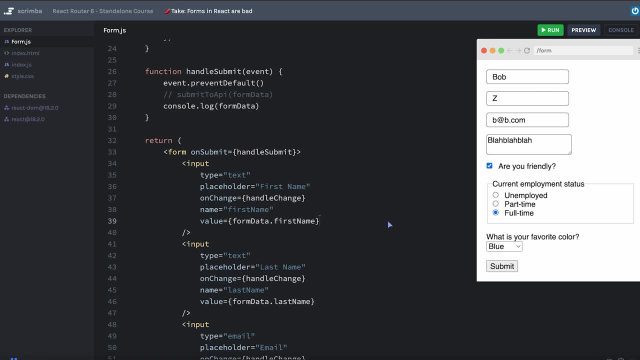 happening internally from a form. You see, originally with forms you would have your form element. you would give it a method. So submitting the form would usually do a post request or a put request out to a server somewhere. you would add an action attribute which told it which endpoint to send that form data to, And then that 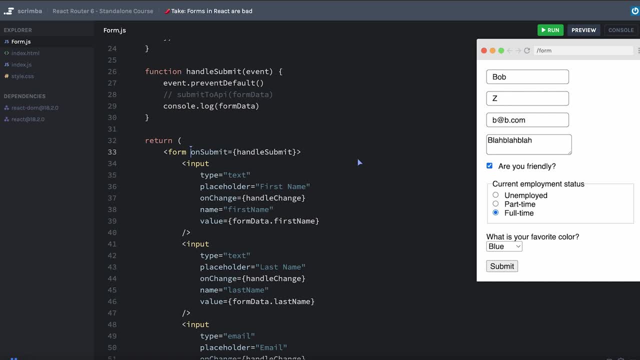 endpoint on the server would take that data, it would process it and it would do something with it, like log the user in or validate that the inputs were valid or create some new resource or anything that normally would be handled by a form. So you've heard me talk about the full stack framework remix. 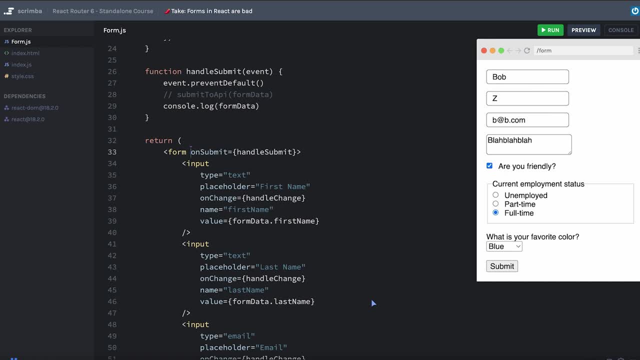 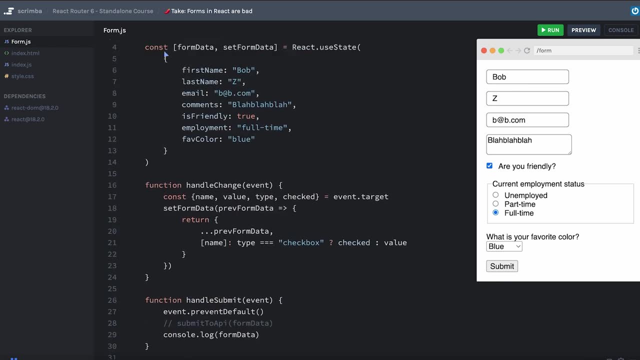 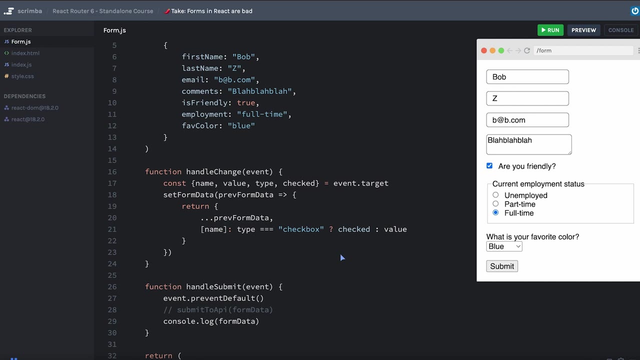 which was created by the same people who created react router, And what they decided to do is to, instead of completely subverting the entire purpose of a native form and overriding it with our own logic, they decided to use the native capabilities of an HTML form and remix in some more abilities with modern JavaScript. Anyway, all of this is to say that 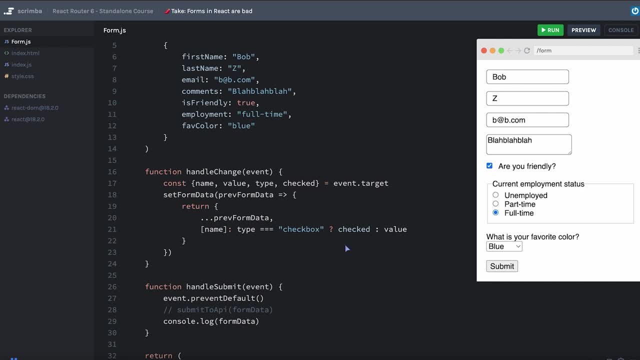 there's a perfectly good native ability for forms in HTML to maintain their own state and to submit their information. So when the concept of action actions was introduced in react router 6.4, we gained the ability to sort of go back to those earlier times when we could make. 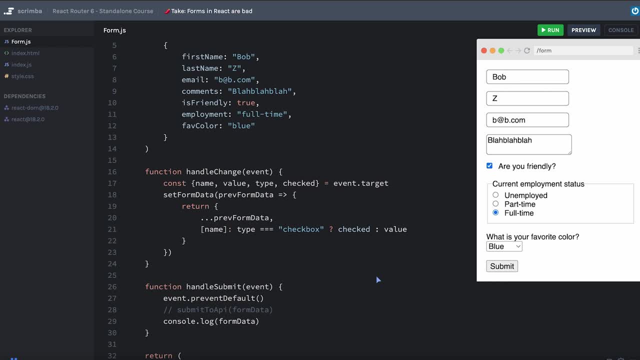 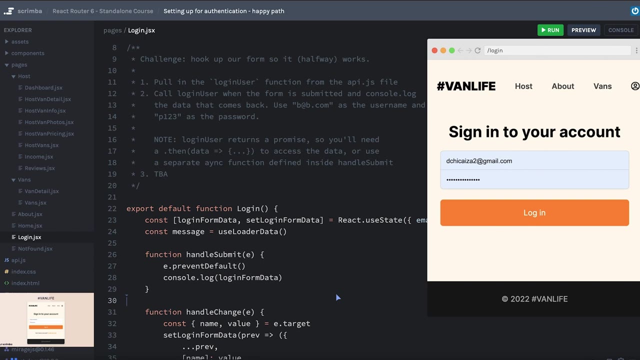 forms in react a little bit easier to work with. So in the next few lessons we are going to be refactoring the login form so that it can use this new actions feature from react router. We're going to see an example of what I was talking about, where forms in 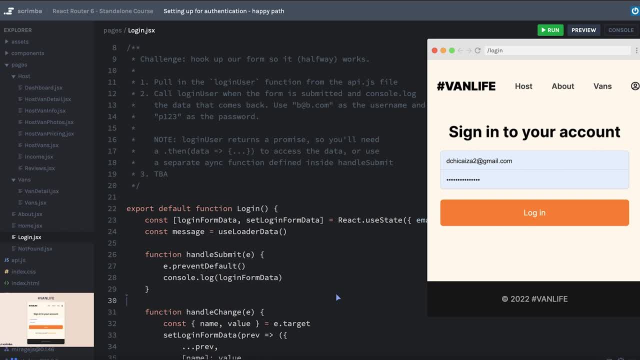 reactor just pretty difficult to work with compared to native forms which have their own state management system and submission abilities in HTML. To do that, we are going to complete a couple of challenges. First of all, I want us to hook up our form so that it at least kind of halfway works. I've done a little bit of work for you. 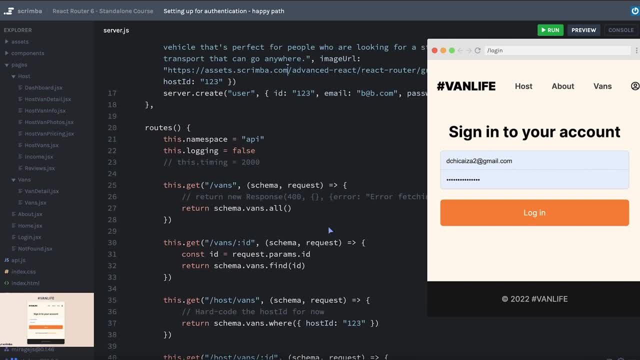 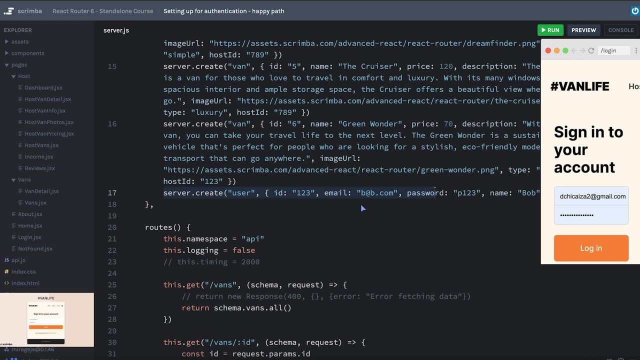 behind the scenes over in our serverjs file, I've created a model for users and I've entered one user in the server, the fake database that we have. Once again, this miragejs server file is not important for you to understand the syntax of, So I'm going to. 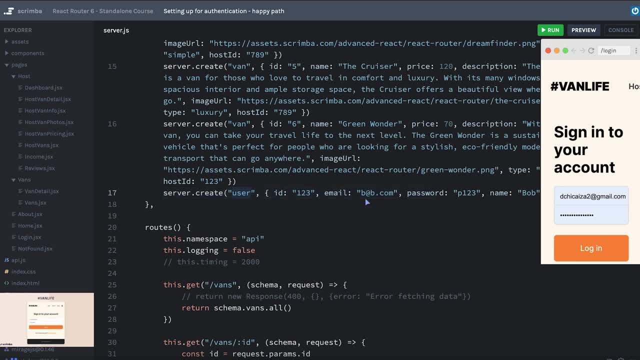 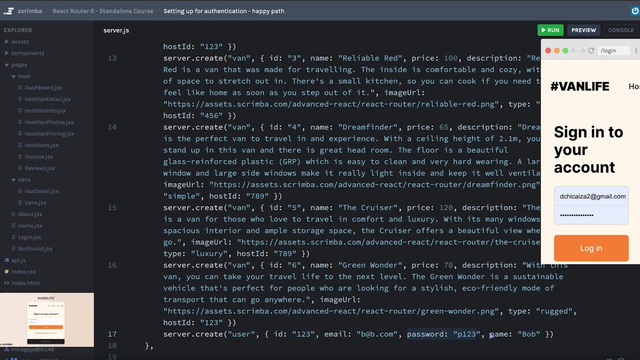 go ahead and create our fake database and field it with an default user And then we're going to launch this. So we're going to go ahead and load it and we're going to say add user user but just know that I've created a user in our fake database. It has the email of b at bcom. 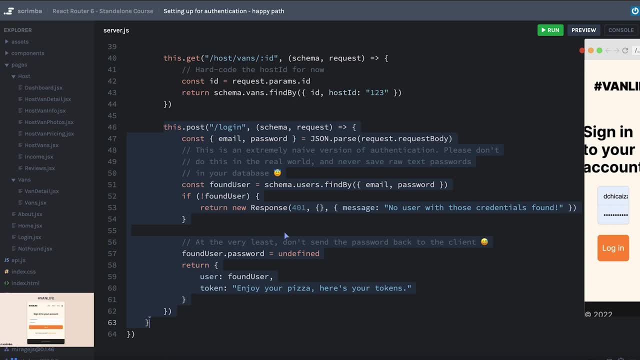 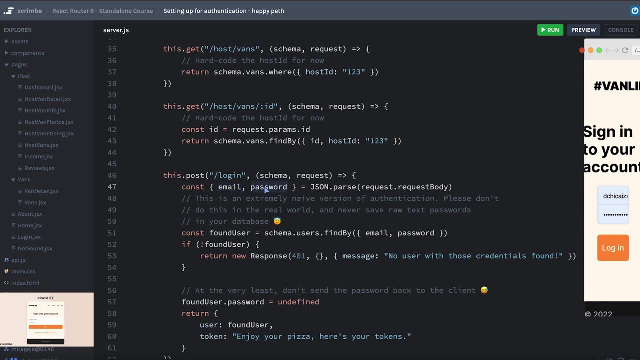 and a password of p 123.. You can see, of course we're just saving this raw password here, which is never a good idea, but that's beside the point. I've also created this endpoint here for slash login, which is simply finding the user in our fake database and if the provided credentials 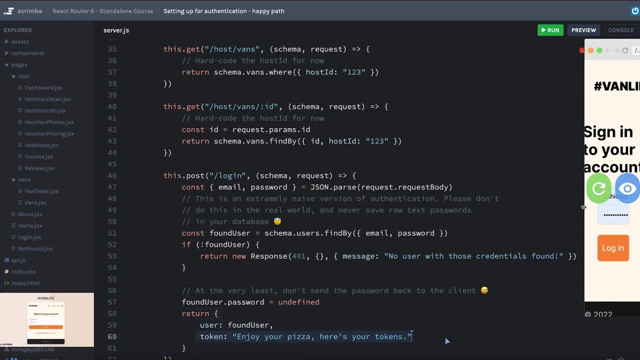 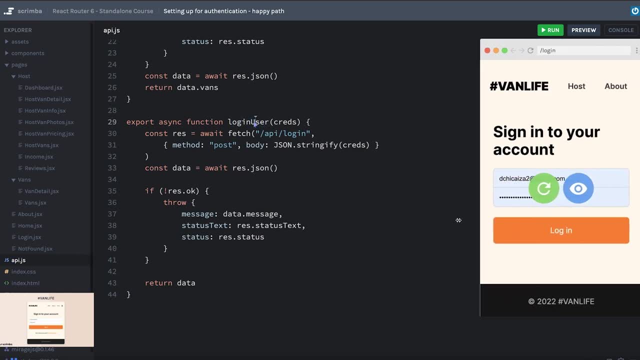 will return the user object and a fake token that we have here. I've also created a new function inside of our APIjs file called login user. So this is the interface that you'll be using. It makes the fetch request for you. It handles any errors that might come back. 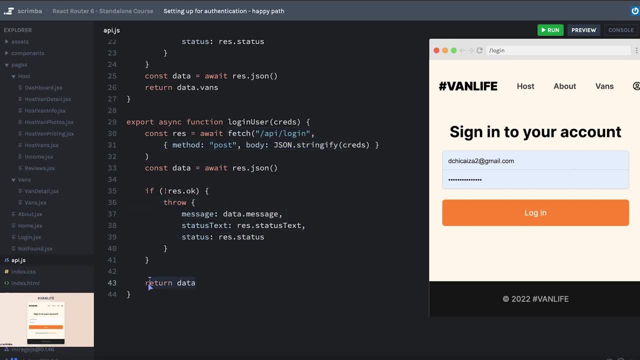 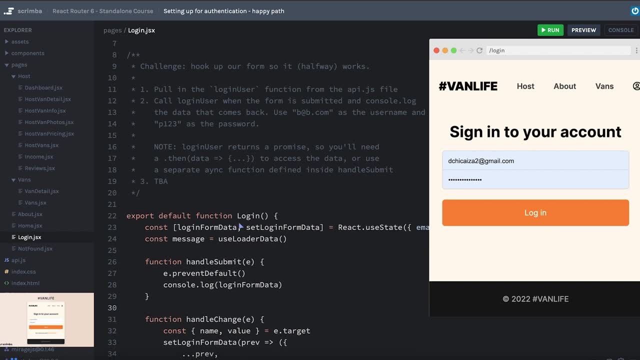 It will send those errors forward if there are errors, but otherwise it will send that object that has a user and a token that came from the server. So that brings us to what your challenge actually is. Your challenge is to pull in that login user function. 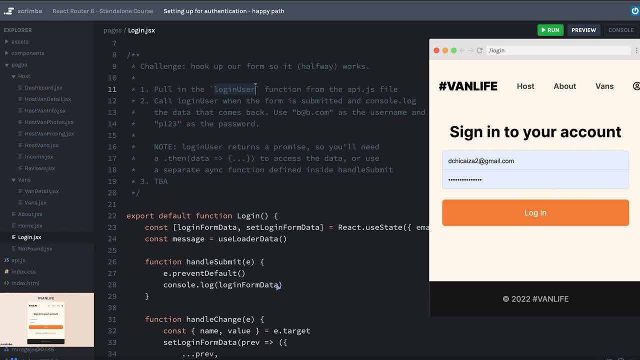 from the APIjs file and then call login user as soon as the form is submitted, passing the login form data that we just currently are console logging. And one thing to remember is because login user from APIjs is an async function, that means it's going to automatically return a promise. 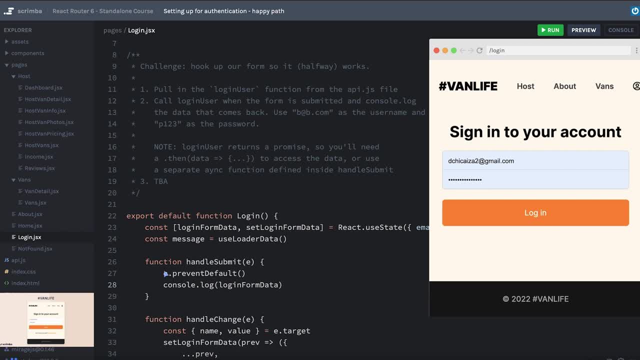 In which case you'll either need to create a separate asynchronous function inside of your handle submit or you can just use the dot, then syntax and chaining to log that data to the console. And in case that wasn't there and it wasn't clear from the first part in step two: 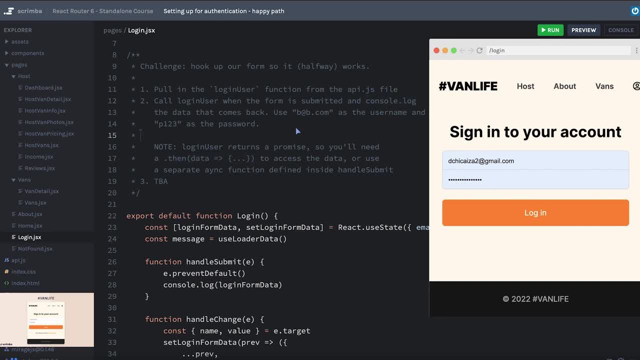 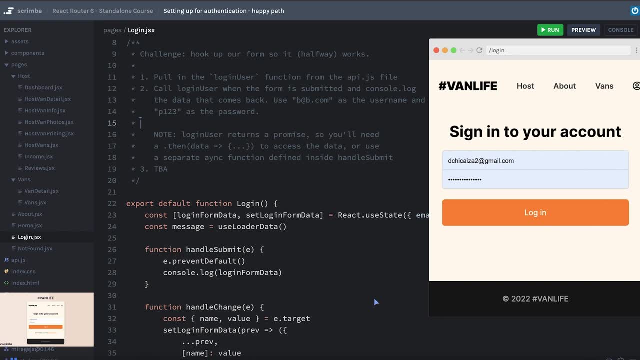 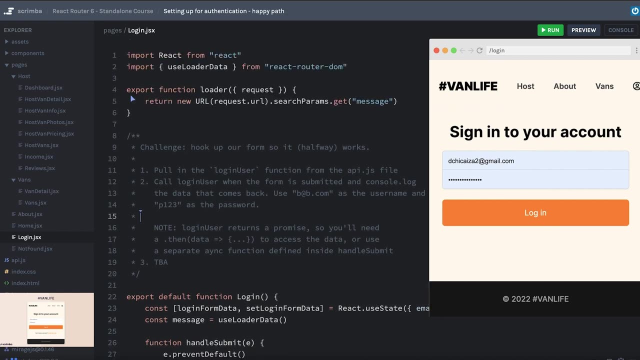 you just need to console log the data that comes back. You don't need to worry about setting anything else up at this point. Okay, I think that's enough information for you to get started. So pause now and work on this challenge. Okay, let's import our login user function. 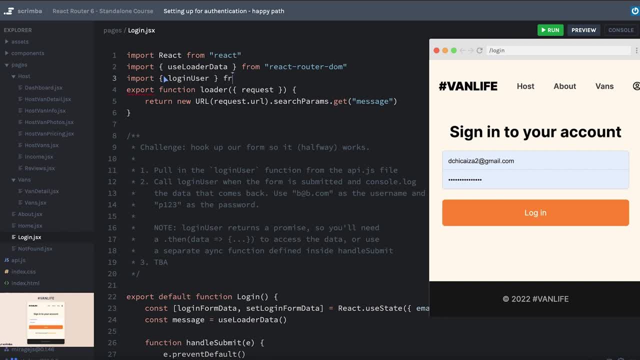 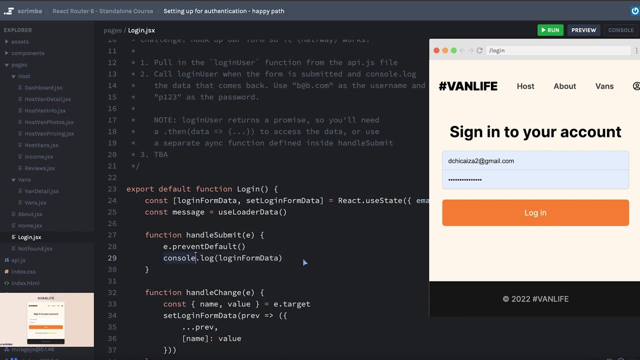 So we will import login user from see how far back do we need to go. This is inside of the pages directory, So we'll go back one directory and get API, If I can spell it right. API there we go, Okay, and then, instead of console logging, our login form data. 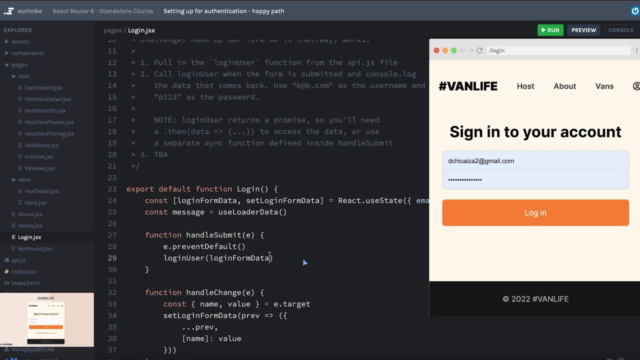 I can just call login user and I'll pass that login form data And I'm not going to bother at this point in creating a completely separate async function here like sign in or something. I'm not going to worry about that, I'm just going to use the dot, then syntax. 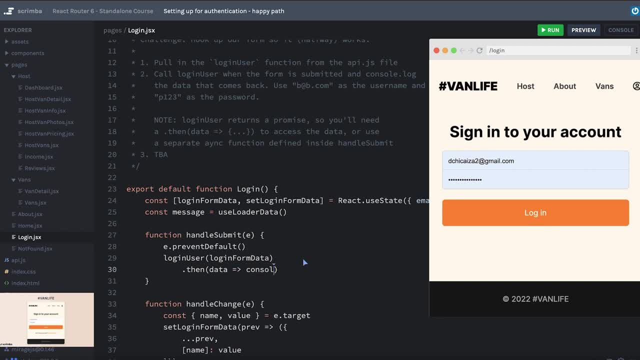 And let's see. we will get some data back And we'll we'll console log the data. There might be a mistake or two here. Let's see how we're doing. We'll hit save And we will enter b at bcom and p123.. 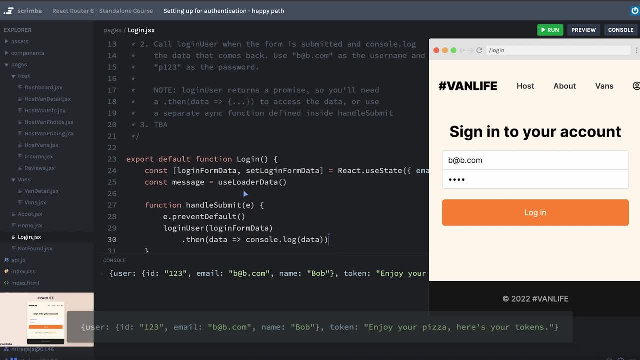 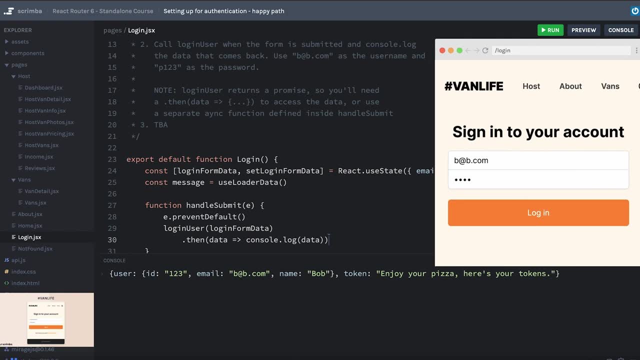 Hit login, open the console and perfect. There's our user object and the token that we were expecting. This is the point at which you might typically take this user object and save it somewhere so that you can have access to it elsewhere in your application. 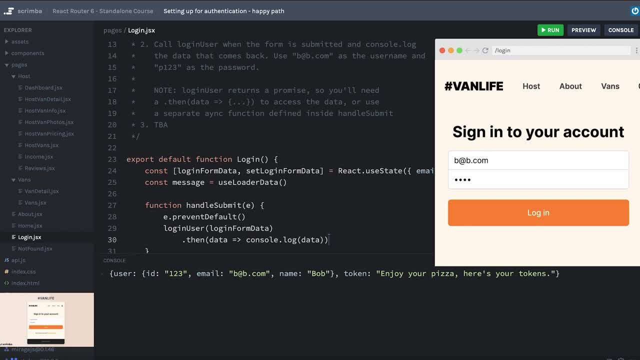 For example, you might put it in context so that you can- I don't know- display the user's name or their email address in multiple places. You also would likely want this token to live, preferably in some kind of cookie, although sometimes people might put it inside. 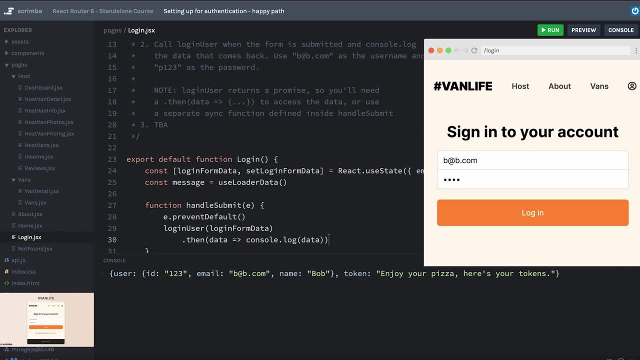 of local storage or session storage. However, we are going to be bypassing all of that for now because that's not terribly important for us when we're learning react router and client side routing in general. We're going to continue opting for kind of a fake. 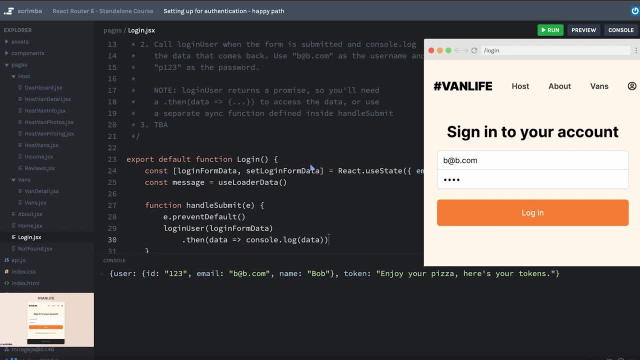 version of authentication so we can see the routing aspects of authentication, And then it will be up to you to actually implement your real authentication In the way that you want. Our next step is to not just code up the happy path, which is all we've done here. 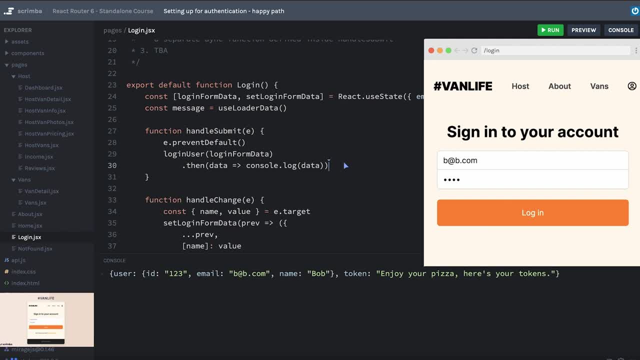 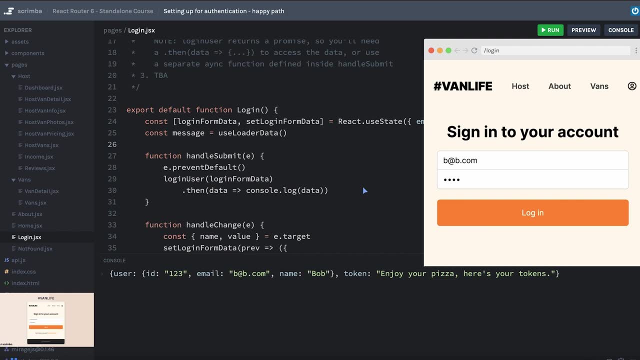 We're assuming that login user is going to work flawlessly. So for the next part of this challenge, we are going to code up the sad path, all with the goal of embracing actions, which I mentioned earlier, is like a sibling to loaders. 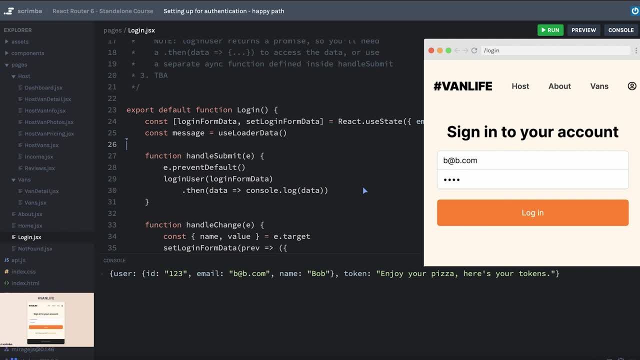 which will allow us to really simplify our code and think about it in an entirely different way, which I would argue is a much simpler way to understand. So that doesn't mean that you can skip the next steps, All of these challenges that we're doing here. 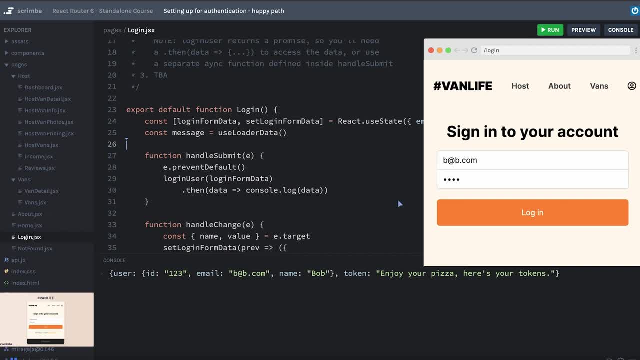 are still going to help make you a better react developer. So I really implore you: keep doing these challenges, and then you will feel even more cathartic when we get to erase a bunch of the code in favor of something simpler. So at this point, 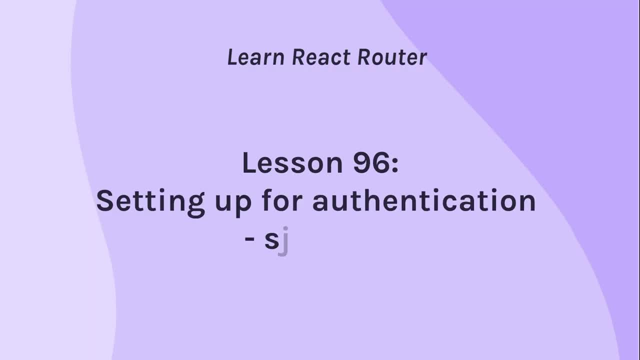 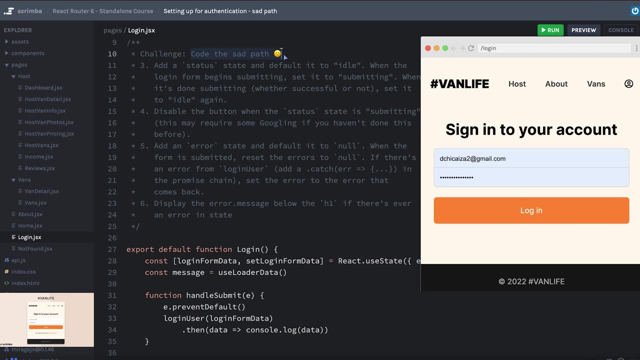 let's move on to the next part of this challenge. Our job is never done as a developer until we have also taken into account the possibility of the sad path. So that's what our challenge is going to be here. You can see, I even started this on number three. 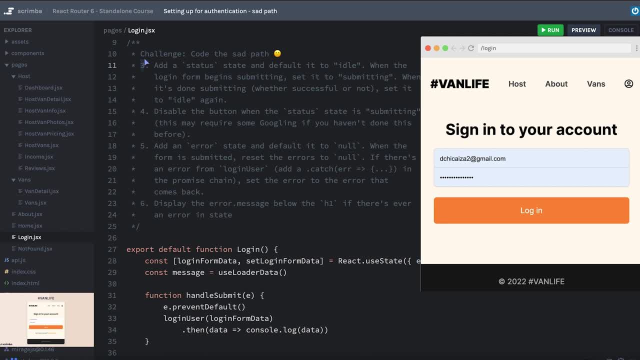 because that's where we left off. The job wasn't quite finished. I won't necessarily read through all of these steps. You should be able to accomplish everything, And I've tried to specify where you might need to go to Google in case there is something in this challenge. 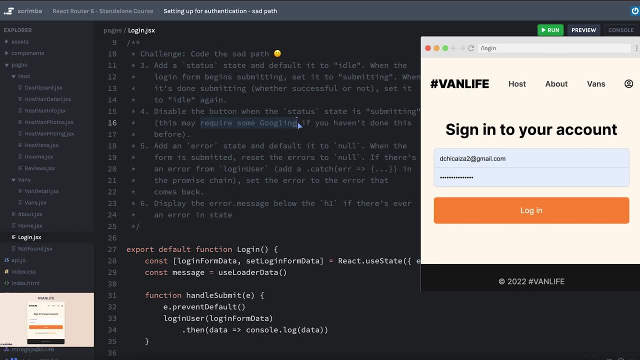 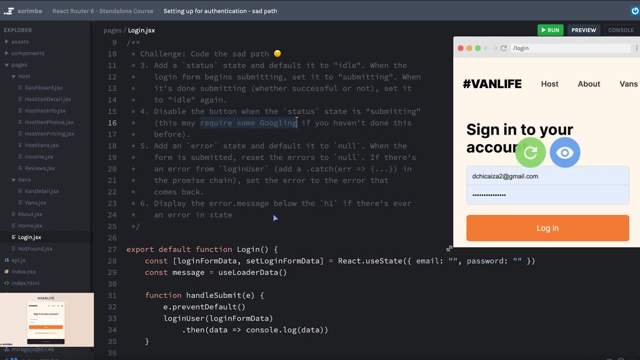 that you haven't quite tried to do before, but that's okay, That's the regular job of a software developer. So read through these challenges one by one, very carefully, start working on them, And when you're done with the challenge, we'll come back together and work on it. 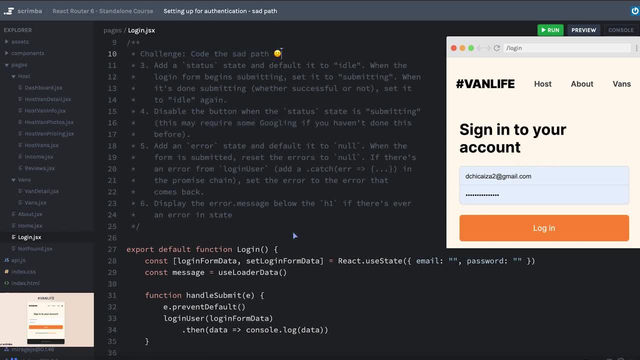 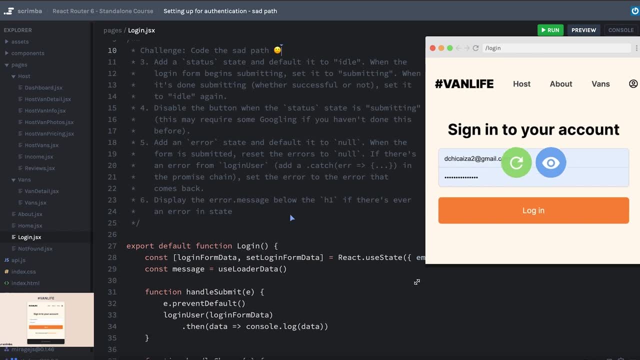 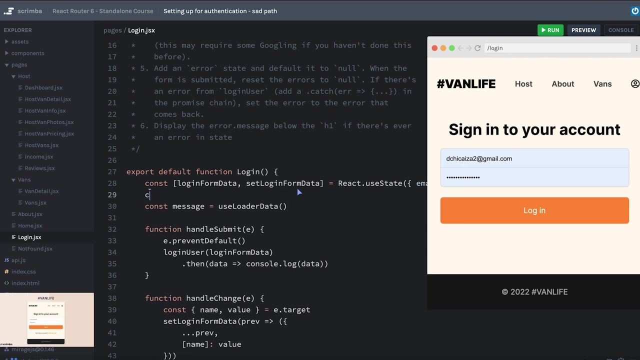 So pause now and code up the sad path for us. Okay, let's go ahead and add a status state. We'll default it to the string idle And let's see. we'll just do that, maybe right below our other use state. 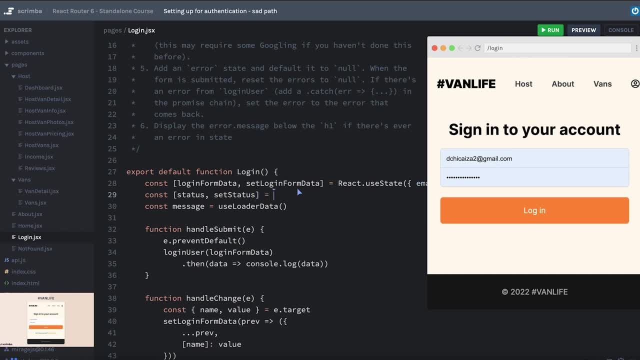 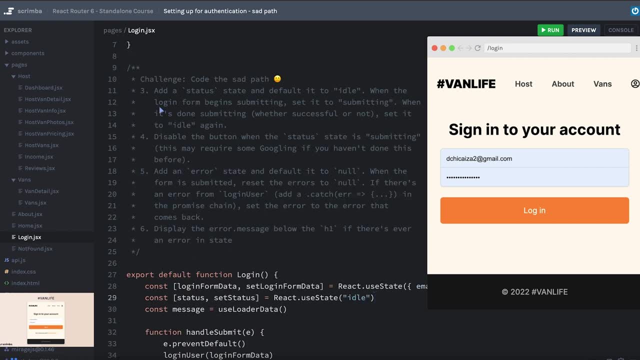 So we'll have a status, set status And that's reactuseState, with a default of idle. There we go, Okay, and then when the login form begins submitting, set it to the string submitting And when it's done, submitting, whether successful or not. 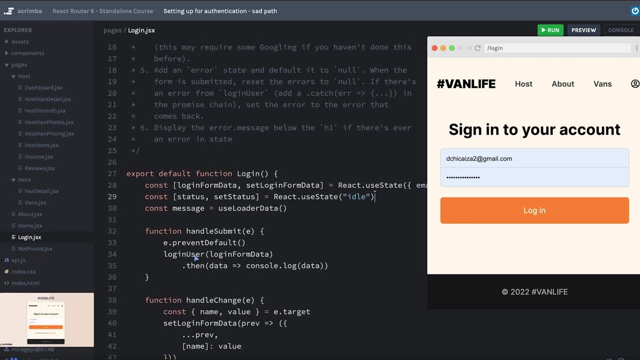 set it to idle again. Okay, so set it to submitting as soon as the form starts submitting. So right here we will call set status, We'll say submitting, And it might be tempting to inside of my dot then to open up that function and set the status back to idle. 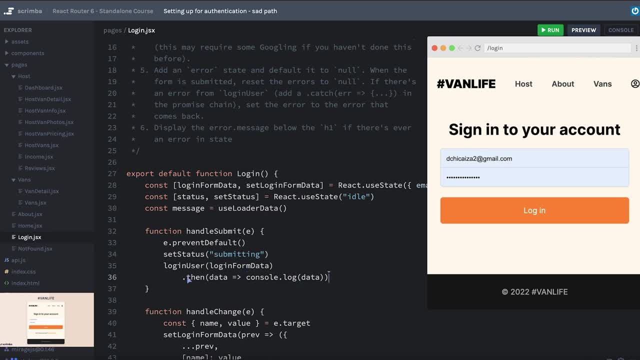 However, because we are working on the sad path and there's a possibility of a dot catch that will eventually run, I'm going to use a promise chain that you might not be quite as familiar with, And that is dot. finally, This is code that will run whether 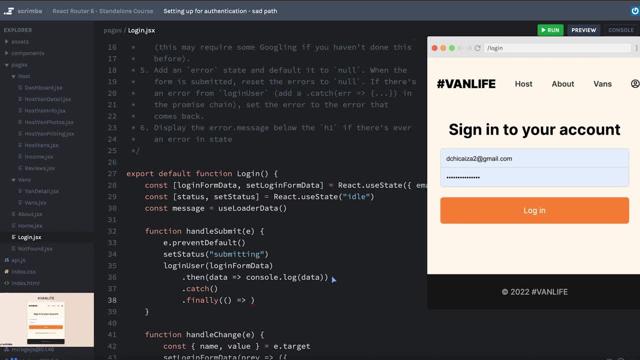 this is code that will run, whether the promise resolved or was rejected, And so in here I can set my status back to idle, And that way it will go back to idle whether or not the login user was successful. Okay, let's see. 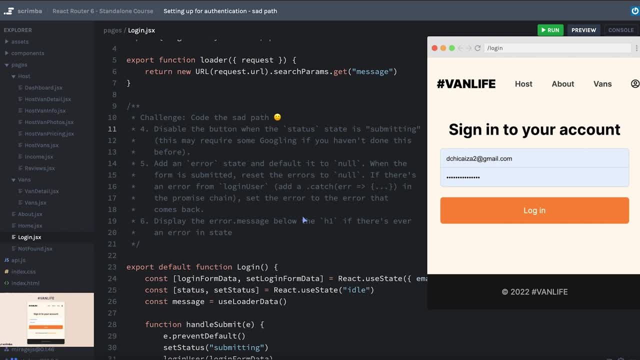 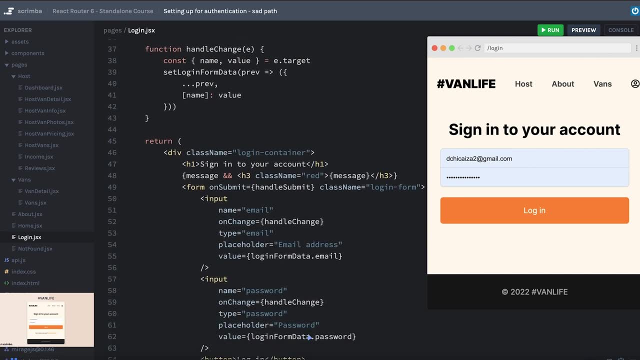 That should do it for number three. I'm just going to erase these as we finish them. Disable the button when the status state is submitting. So this might have been one where you needed to go out to Google for some answers, but on button elements in JSX. 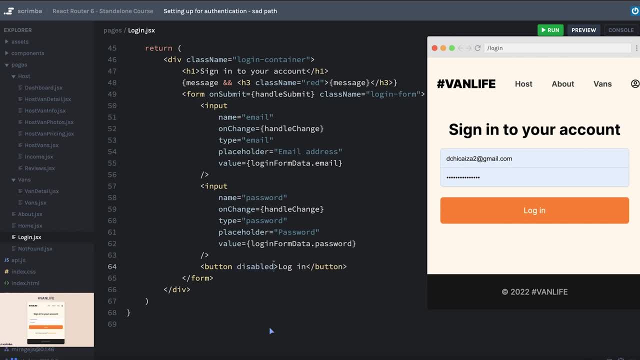 and well, actually in HTML there's a property called disabled and in JSX I can set that equal to an expression, And if it evaluates to true, then the button will be disabled, And if it evaluates to false, then the button will not be disabled. 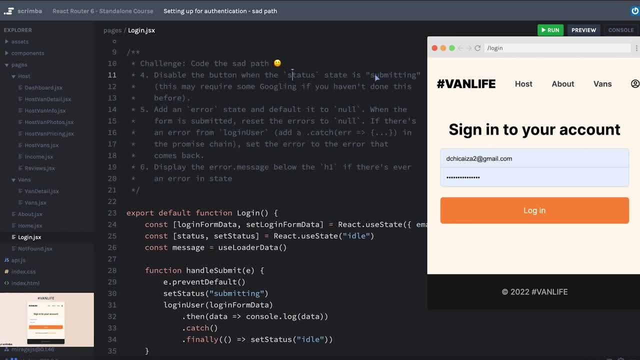 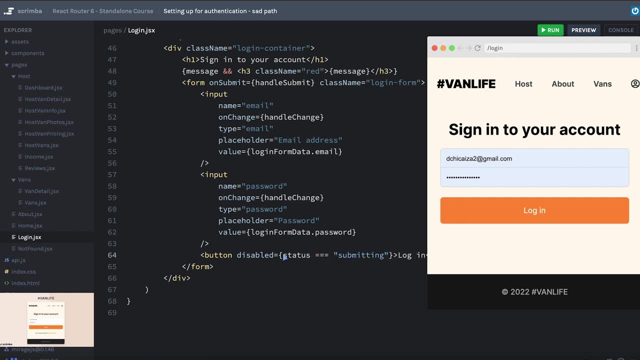 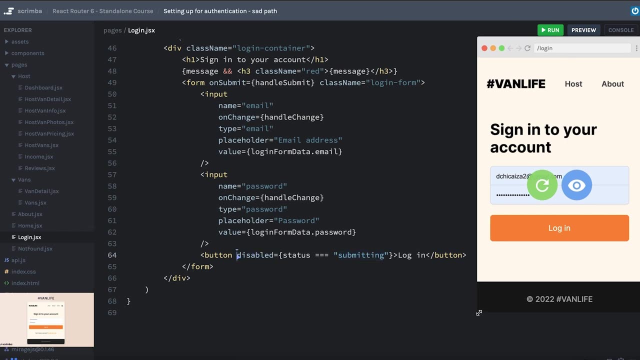 And so it says to disable the button when the status is submitting. So we can say here: if status is equal to submitting, this will evaluate to a Boolean. if the status is submitting, In other words, if submitting equals submitting, then that will be true and the button will be disabled. 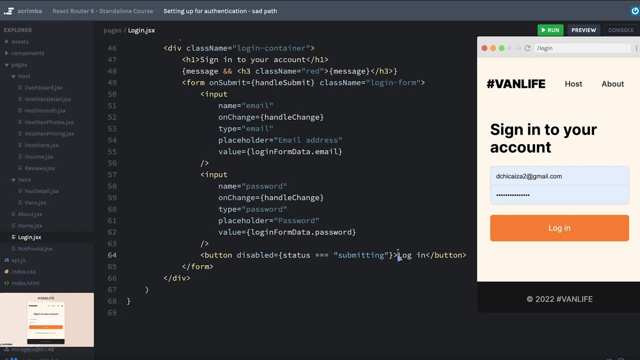 And actually you know what? this wasn't part of the challenge, but I think I want to change the text to say logging in if it's currently in the process of submitting, And so I can do that with just some basic conditional rendering. I'll go ahead and separate these things out just a little bit to 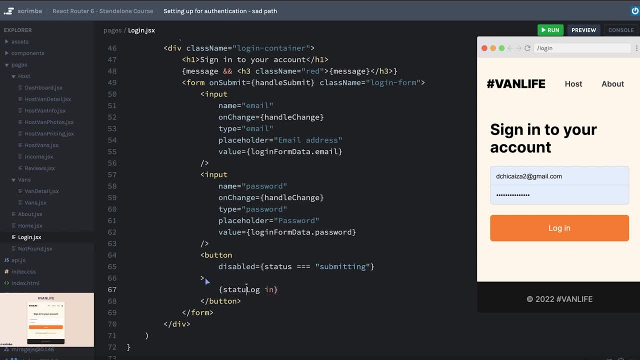 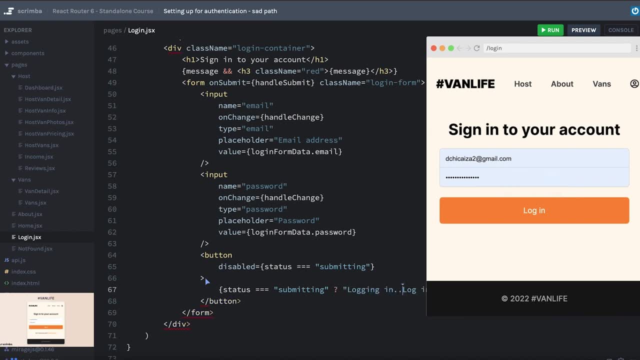 buy myself some room, And then I'll open up an expression. I'll say: if the status is equal to submitting, I'll use a ternary here. then we'll say logging in And we'll do dot, dot, dot, But otherwise we'll say log in. Let's put these on their own lines like this: Okay, and I think we. 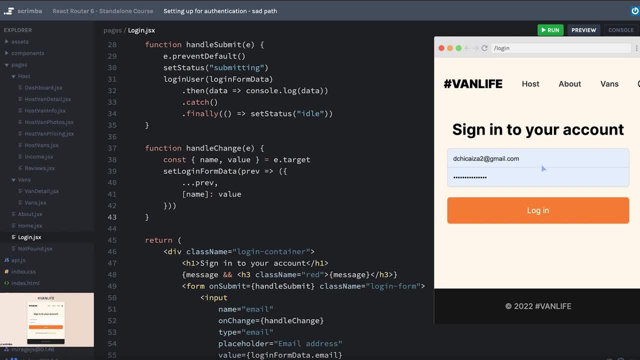 should be able to test this Now. I'll hit save And I guess we can try b at bcom p 123.. We'll hit login. Okay, it said logging in for just a brief second. it was a little bit hard to see And we. 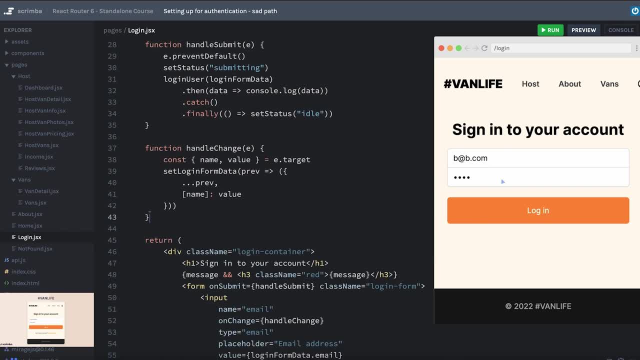 still got our console log of the data back. That's good. If I were to maybe not enter any values in here, that should be an error. And okay, we get our object here. that is, console logging with the no user with those credentials found. I think we're getting a little bit ahead of. 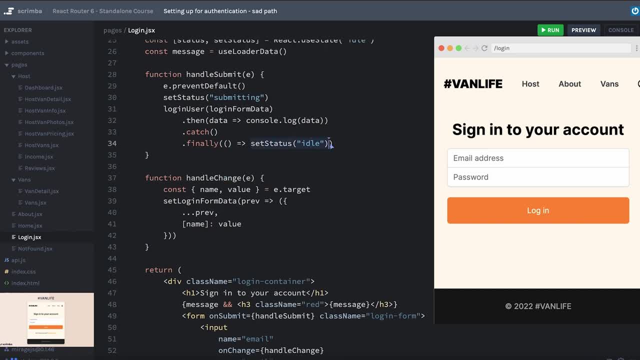 ourselves. But one thing that's nice is because our dot finally is setting the status back to idle. our button now says log in again. if we had only set the status to idle inside of our dot then then it would probably be stuck in the submitting state because we'd never set it back. 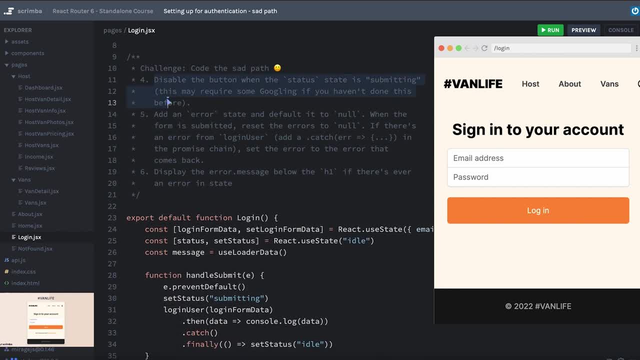 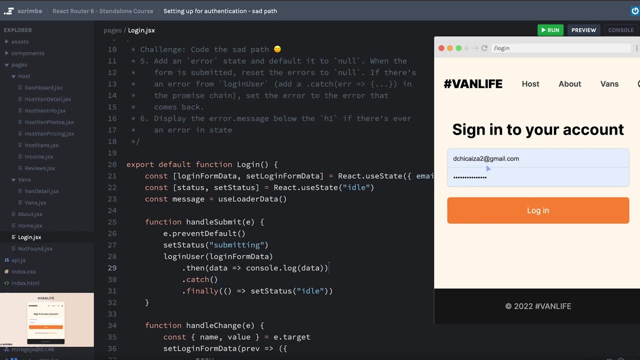 to idle. Okay, let's go back up. we have done number four, let's go ahead and erase that. Okay, let's actually catch the error that comes back when we are maybe not submitting something or we have incorrect username and password combination. So, number five: we need to. 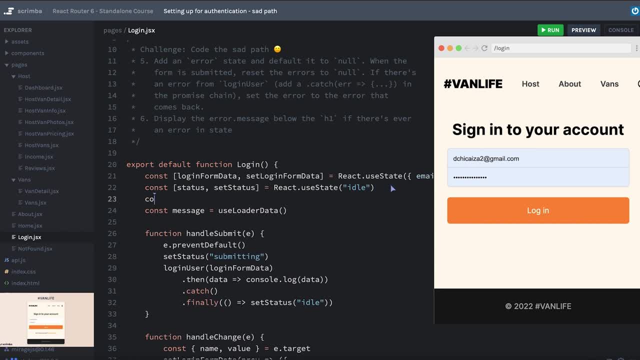 add an error state and default it to null. Again, we'll just do that with states. So we'll have const error, set error, And that is react dot use state and default to null. When the form is submitted, reset the errors to null. Okay, so that's something we can probably just do here. 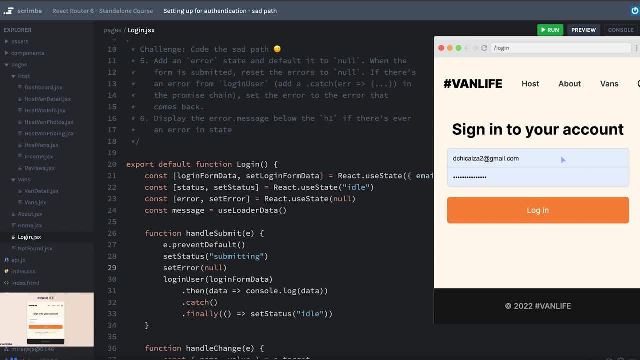 we'll set the error to null, just in case there is an error and then the user fixes it and hit submit Again. we don't necessarily want that Error to stick around. that might not make a huge difference. We're just trying to cover all of our 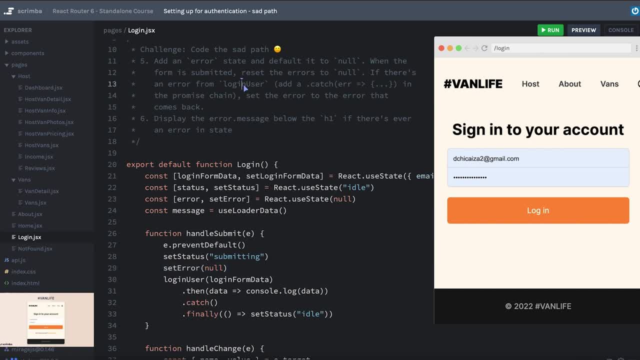 bases, So we'll leave it there for now. If there's an error from login user, add a dot catch in the promise chain- then we need to set the error to the error that comes back. Okay, so we have a dot catch ready, we'll catch the error and we will simply set the error to that error object: That: 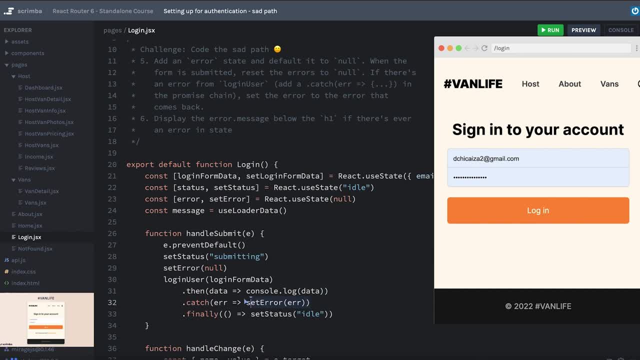 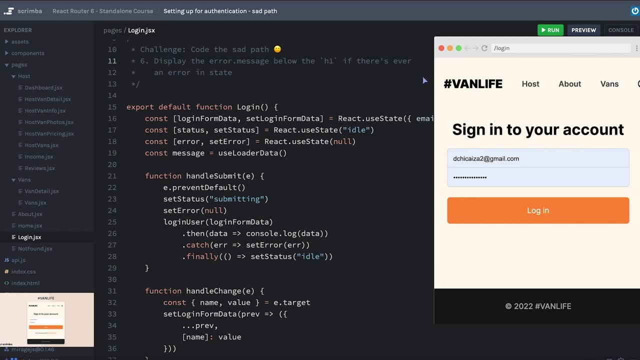 way we can save it in state. we can start rendering things on the page when that state changes. And actually that's part number six, So I'll delete five, we'll just add the error to that one and we'll select the Bliss script and say: 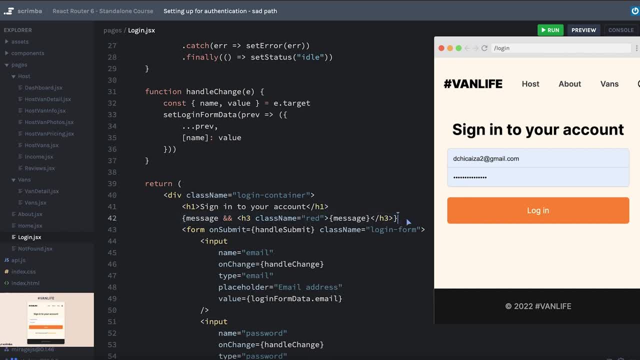 display the error dot message below the H one. if there's ever an error in state. okay, so that would be right here, kind of akin to our previous message that would say you must log in. So I guess we can. actually, you know, I'm just going to copy this line down and we'll say instead: if there's 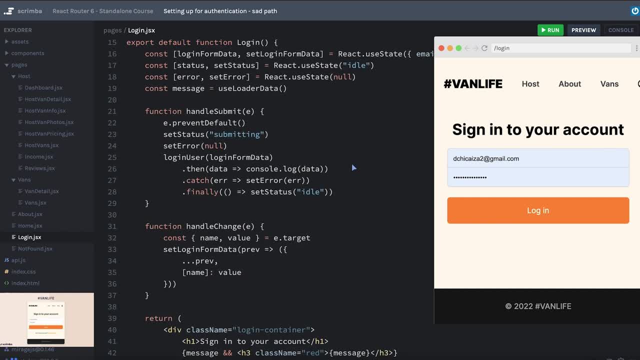 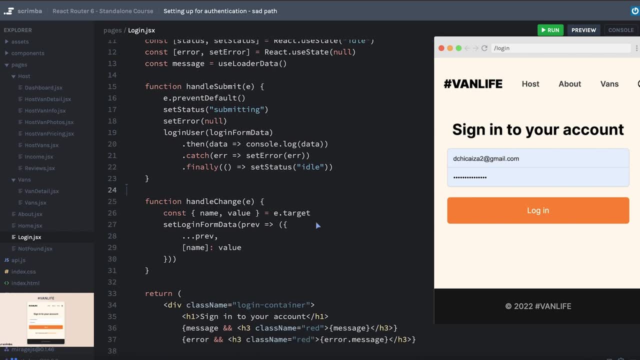 an error in state. then we will display: Oh look, we're even using the same terms. I can say error dot message. yeah, let's clean this up, Kind of anticipating that we did everything perfectly, but we never know. Let's go ahead and hit save. I'll just click login without providing anything, And sure. 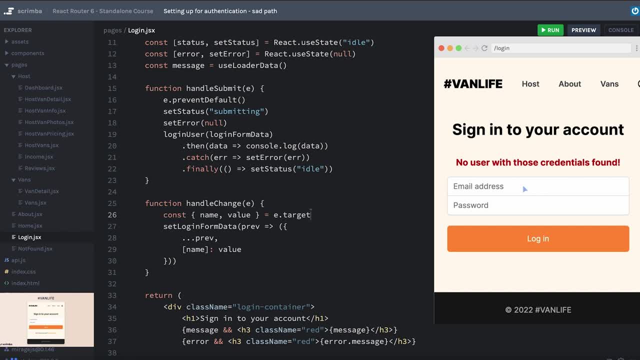 enough, no user with those credentials found. Perfect. If I were to say something like c- at ccom we don't have a user with those credentials- and put anything in for the password, we should get the same thing. And I guess one thing that's nice about clearing the error to null is that when 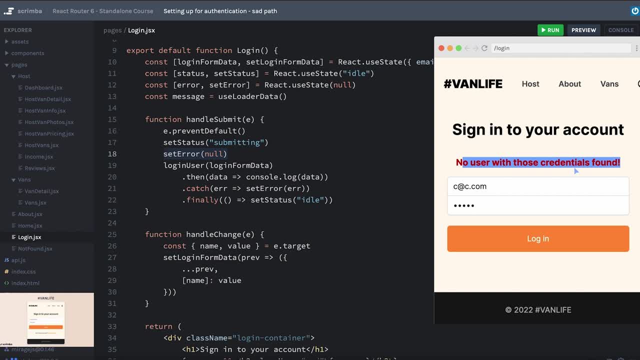 we logged in, it made that error message disappear, which made it much more obvious that we are having yet another problem with no user with those credentials found, And it's not just the same one that's from before, By the way, if you're wondering where this message is coming from, 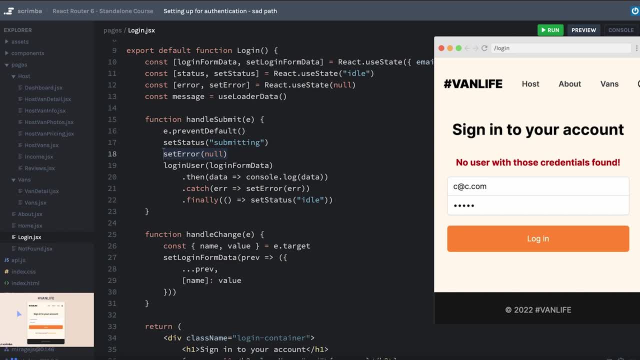 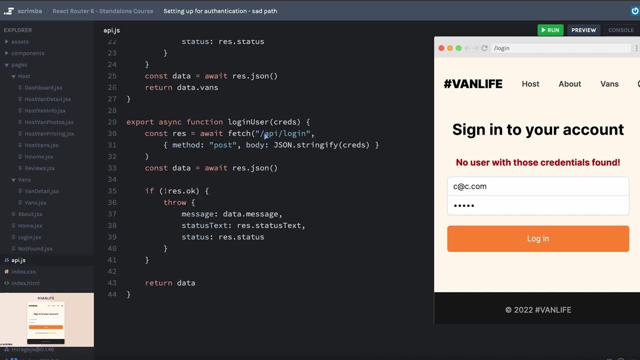 in the first place, since you didn't code up the API JS or the server JS additions that I made. that's where they're coming from. Login user is making a request to fetch the data from API slash login. it's passing those credentials And if there is an error on the server. 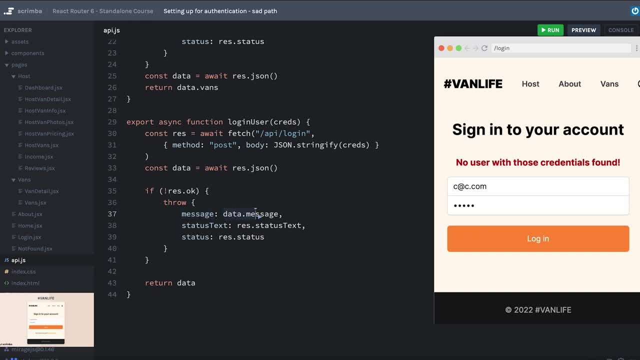 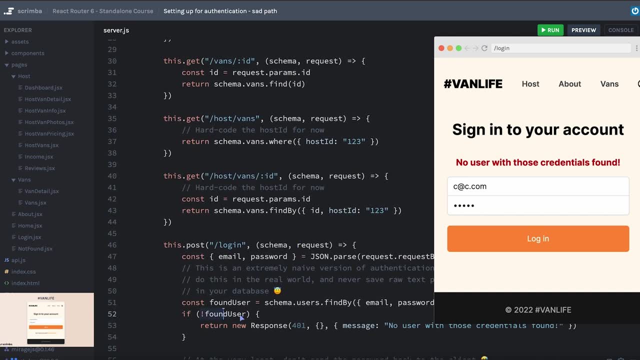 then it's going to throw this error which has a message property with data dot message And that is coming from the server. So we go to server JS And we can see that if there is no found user, then we just return a 401 response and have a message that says no user with those credentials. 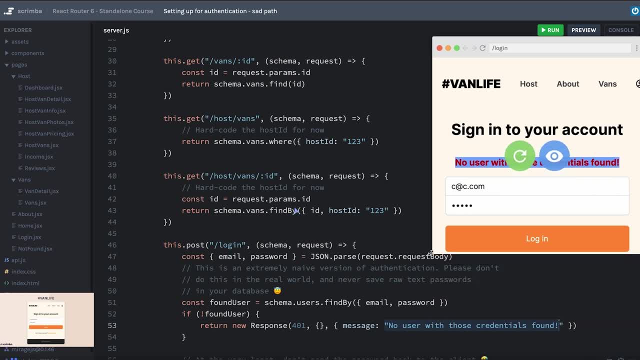 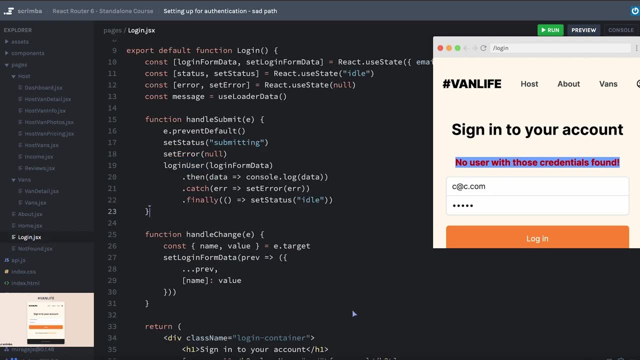 found which makes its way back to our front end and displays to the user: Okay whoo, that was a lot of work. Let's go check out the login page and admire what we've done- And maybe admire isn't the right word. 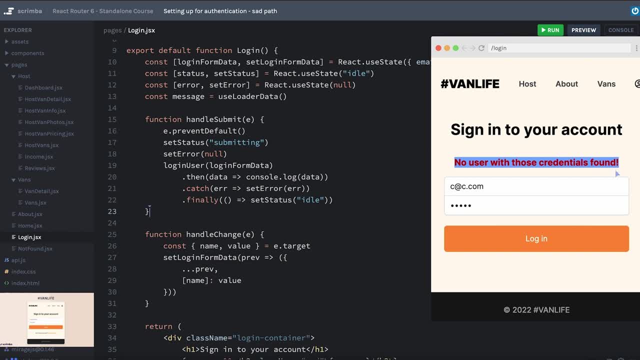 So, as a reminder, if you're using a third party form library in React, then you might be able to avoid a bunch of this. Also, if you're using a fetching library like 10 stack query- formerly known as React query, or SWR, or one of those other similar libraries, you might be able to. 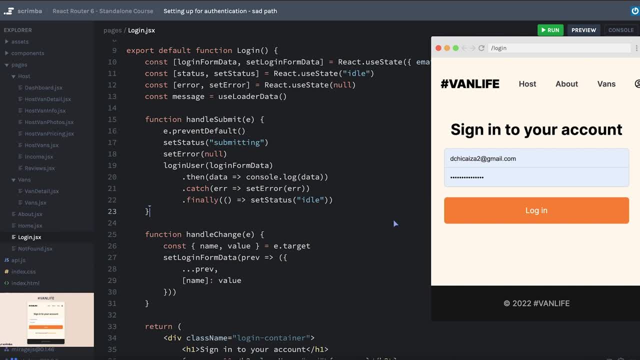 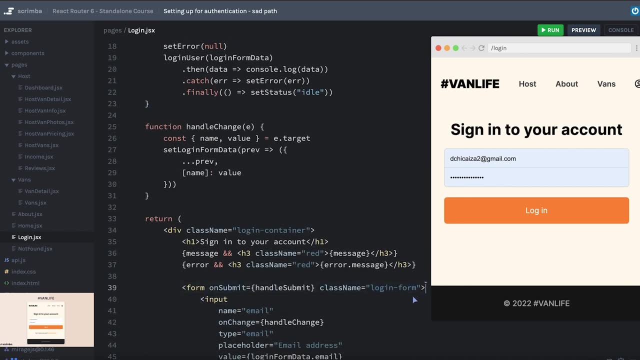 avoid some of this boilerplate code. However, we are going to see how React router has brought back our ability to use the native form element. its internal state that it's already able to maintain its ability to submit that form, And then we're going to process the data from that form And we'll see. just 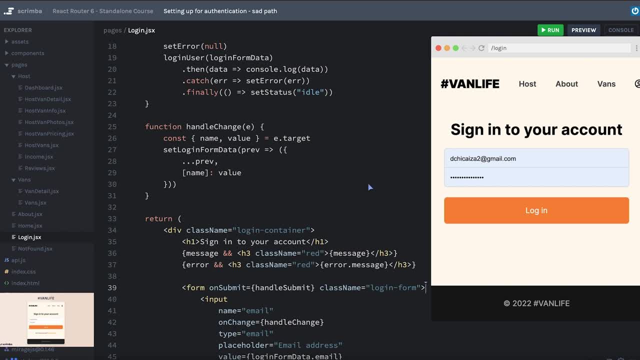 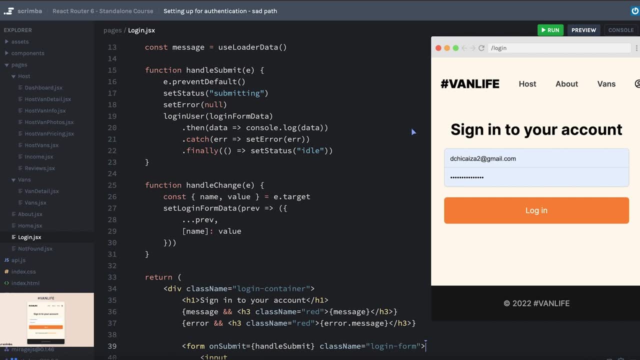 how much simpler our form can get. However, before we jump into that, I promise only one more thing. we're going to learn, And it's going to be very quick. we're going to see that there is a programmatic way in which we can send somebody to a new route, mostly. 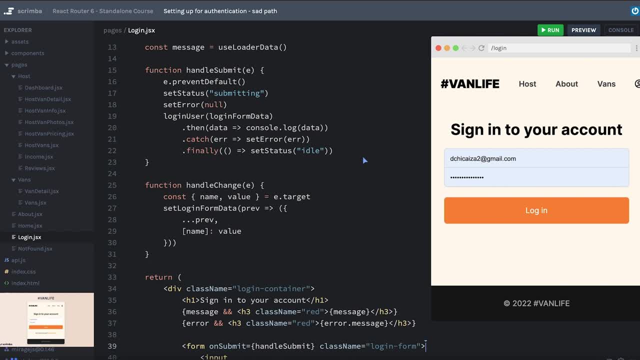 so that I can check that off my list as something that I've taught you. The way that we'll do this when we start using actions will be slightly different, So, like I said, I just want to get it out there and consider it taught so that we can finally move on to actions. This 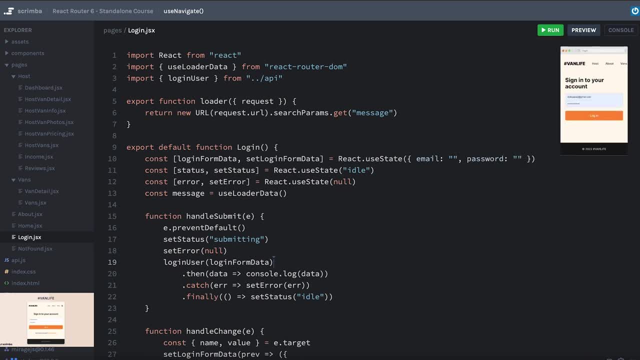 last topic is so simple to grasp that I'm actually not even going to bother including this as part of a challenge or an aside or anything like that. I'm just going to show it to you, because then we're going to jump into refactoring everything. Anyway, we've. 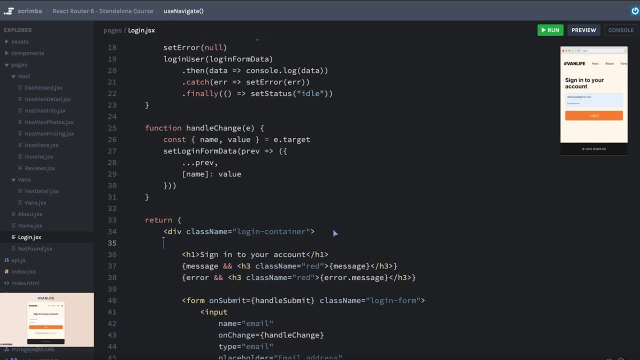 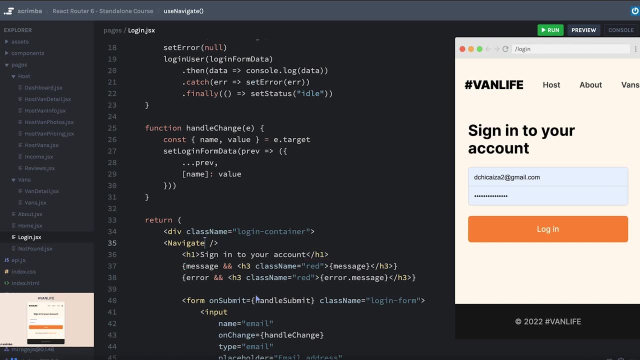 learned about the navigate component from react router. if we ever were to render a navigate component like this- and of course I would have to import it from react router- then it would immediately redirect us to a different route that we specify here. So, for example, if I went to the slash about page, if I hit refresh, 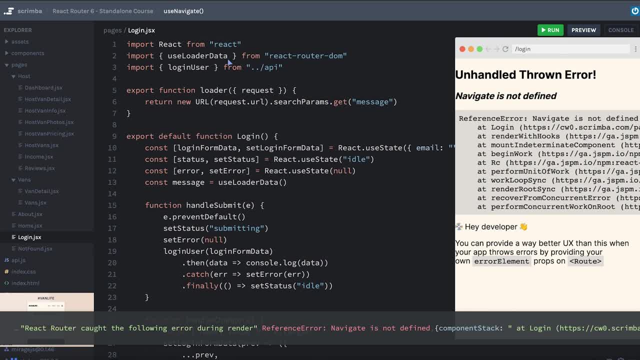 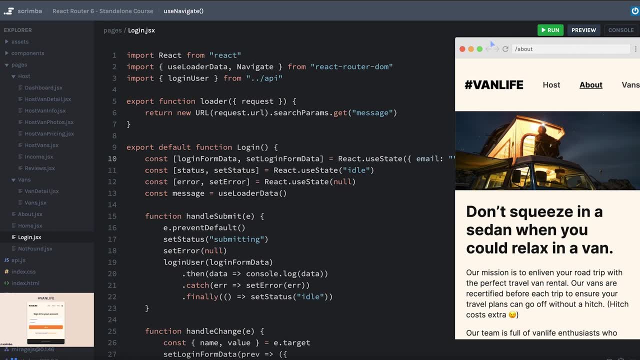 here on the login. well, I need to import, of course. I just talked about this. So import, navigate. okay, let's try again. Okay, so you can see. it tried to load me to the login page and it immediately navigated me to the about page. So that's just a refresher of. 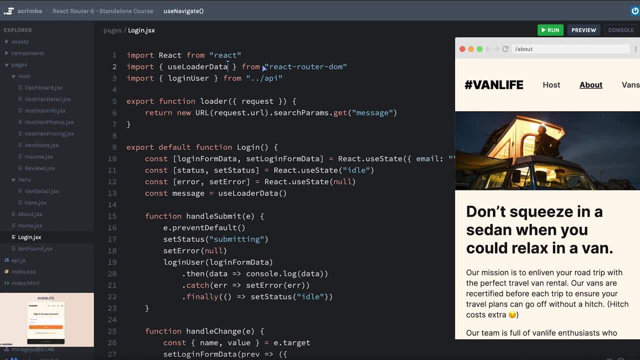 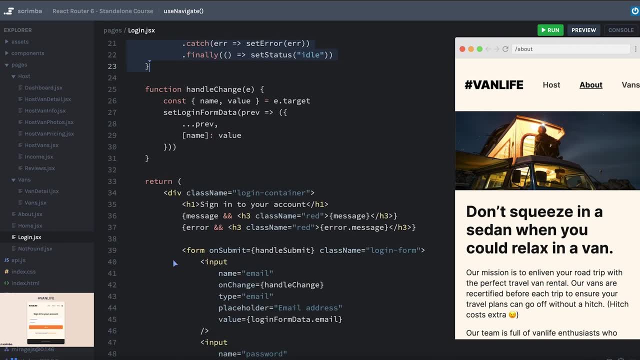 that which we've already learned. that is a component version of what we're going to learn, Which is a hook called use, navigate if inside of your more programmatic code, not the UI code that we have with JSX, but rather the code that's actually handling the logic, If 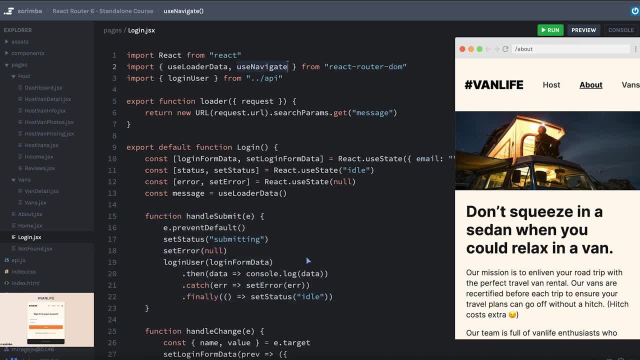 in that code. you want to navigate somewhere, you can use the use navigate hook to get access to a function that I'll call. navigate equals use navigate And this function, when you call it, will navigate you to a new route. In fact, under the hood, the navigate component, I believe. 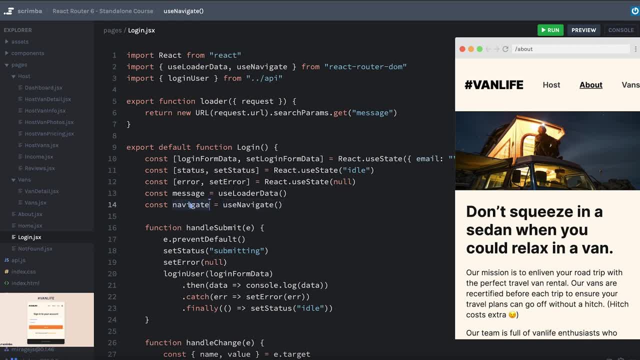 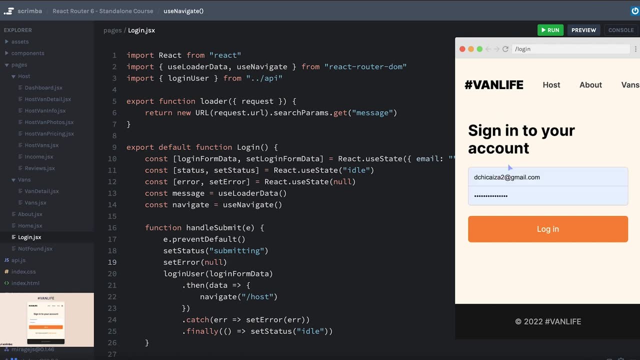 is just using use navigate. So instead of console logging our data here, we might decide that we just want to navigate someone to the slash, not about, let's say maybe slash host page. Okay, so I'll refresh, I'll go to login, And one thing that I did have to change is over here in utilsjs I made 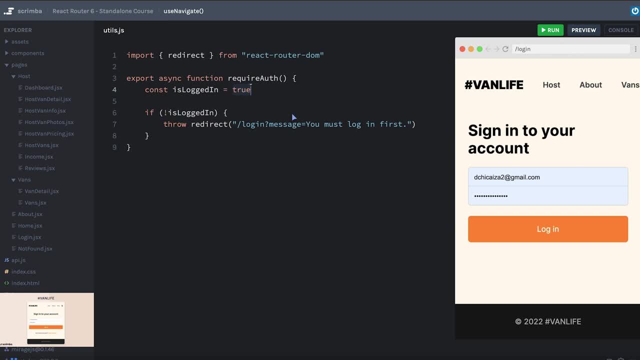 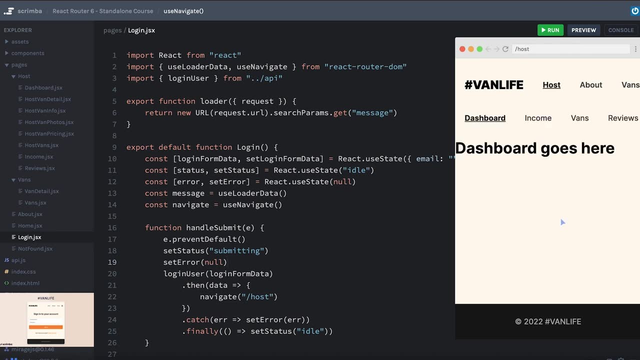 sure that this It is logged in is true. That way it wouldn't forever redirect me back to the login page. And let's see So be at lett arecom. P one, two, three, log in, log out the login. logging in and it redirects me to the host page. There are options to navigate, For example: 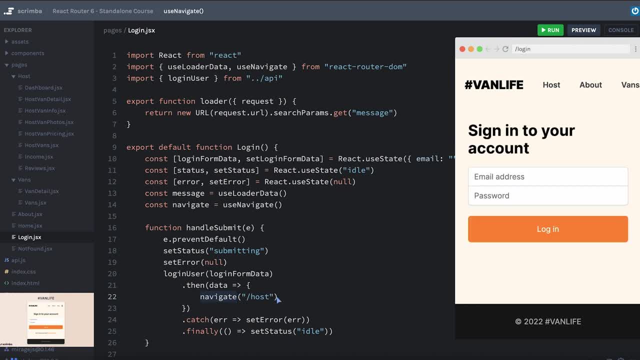 right now. if I hit back, I go back to the login page. There's an option I can include that just says replace true, And this means it will replace my location in the history stack with what used to be there. That might not make a ton of sense. Let me hit refresh. I'll log in again, If you want. 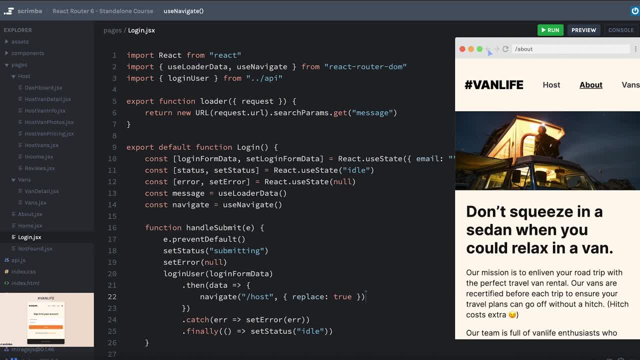 to three, I'll hit login, But then, if I hit back, it takes me to the page I was on before. I went to the login page. Instead of creating a new entry in my browser history for the login page, it just replaces it with the new one for slash host. Now one thing you might be asking yourself is what is? 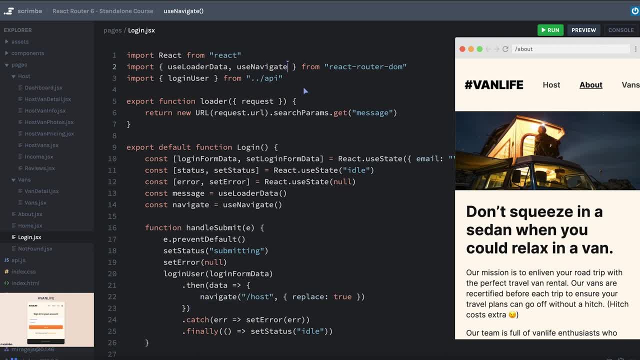 the difference, then, between using this navigate function and using the redirect function, which we learned earlier. an important thing to keep in mind about react is that any hooks that you have like use navigate, they must be run at the top level of your component code. However, when we're 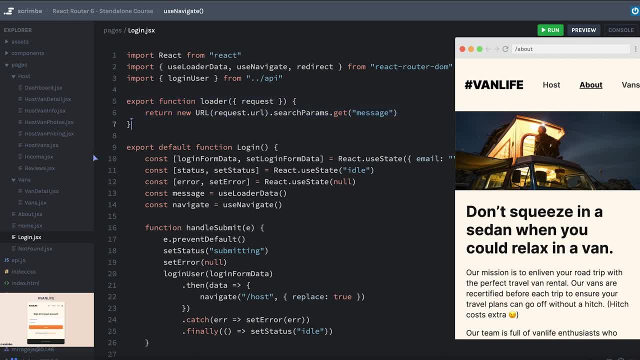 working with a host. we're not going to be able to do that, So we're going to have to do that with other functions, like we have with our loader And like we're about to see with our action function. we're not able to use hooks like this because this function is not a component. It's not. 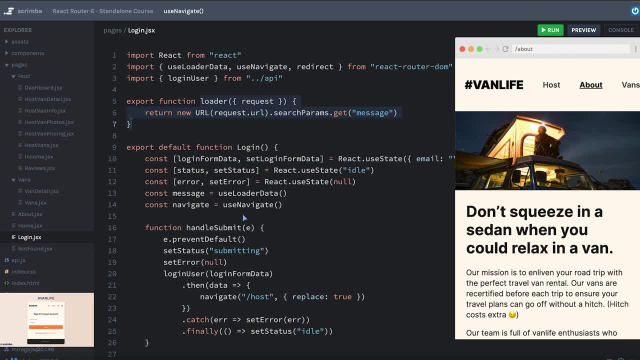 rendering any UI. it's simply helping the component do its job. So, while use navigate works, if we're going to be running it inside of a component like this, it's not going to help us when we're working with loaders or actions. Now I do want you to keep this little nugget of information that we covered. 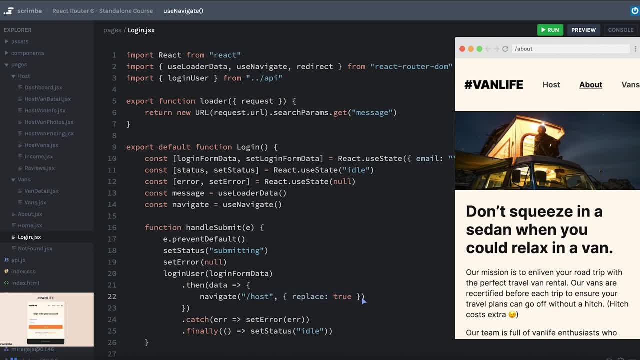 about replacing the entry in the history stack, And if you want to keep that information, you can also do that in the stack, because we're going to come back to that. And it's also important to note that if you're using navigate like this inside of a component, you're oftentimes going to need a use. 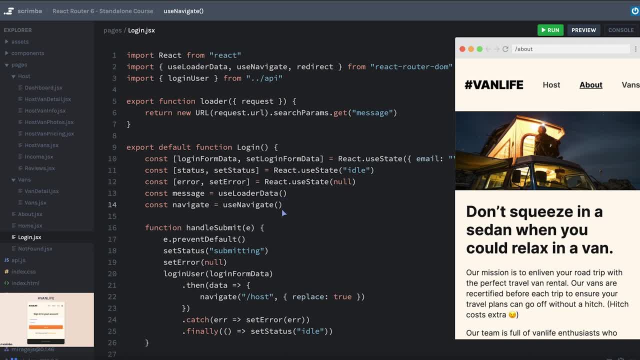 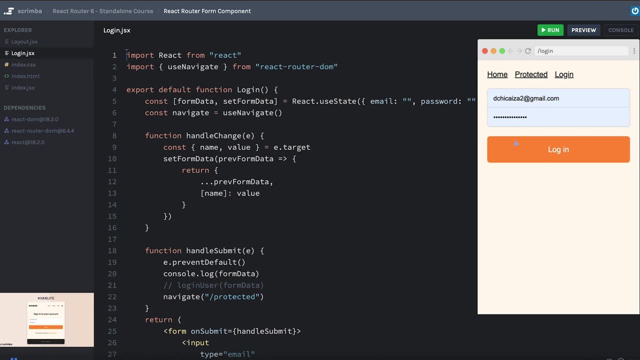 effect in order to avoid some kind of difficult bugs that can happen when you're using navigate. Okay, that's enough delaying, I promise let's move on and finally start learning about how we can simplify and improve our forms using react router. We're back here at the super basic version of our 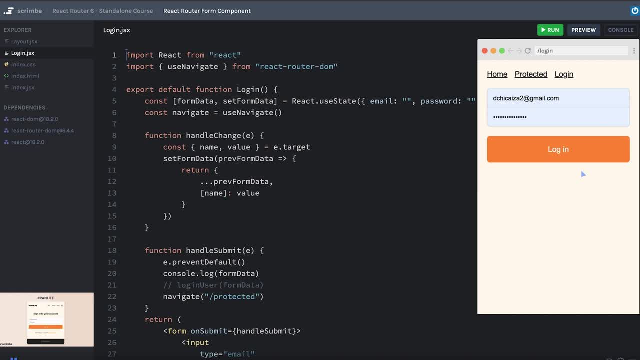 web org web app that we have, And I've spruced up this login form just a little bit And our goal is to set ourselves up so that we can use the new actions feature with the React Router data layer APIs. You see, natively forms know how to handle their own state and they know how to submit to. 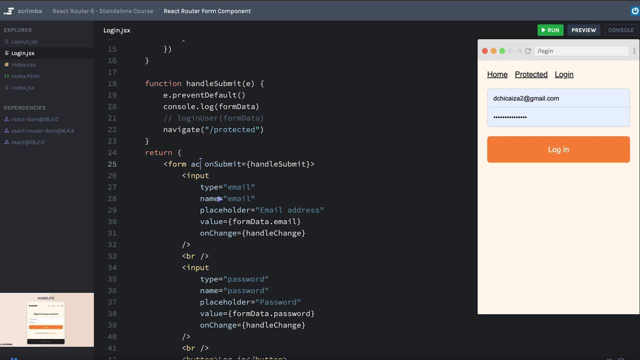 some kind of backend. So traditionally I might have a property or an attribute on my form that would say action And I would provide to it maybe a PHP file- let's call it loginphp- So that when I submit this form, or rather when the submit event happens, the PHP file would get called. 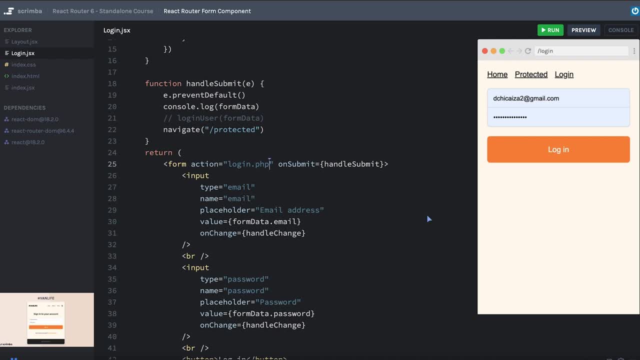 it would serialize the information from the form, either in a query string in the URL, or it would collect it together as form data and send it to the loginphp file, which would then process the data and do something in response. Well, we don't have a. 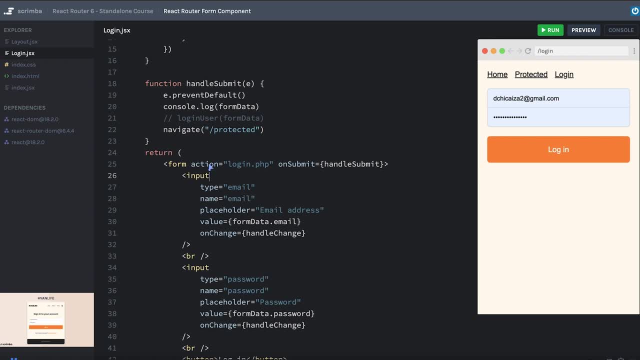 backend to submit to, But maybe you can see where the name for the action function which we're about to learn about comes from. Instead of submitting to a backend, React Router gives us a back end to submit to, So we can see where the name for the action function which we're about. 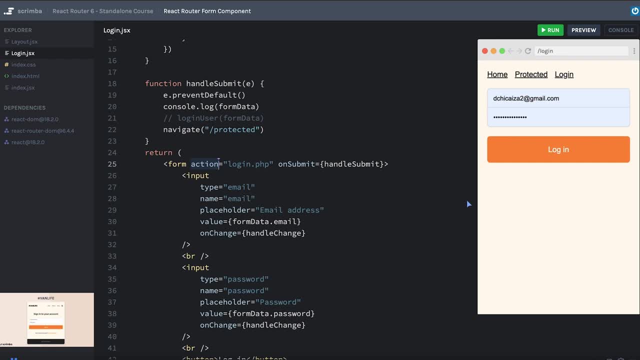 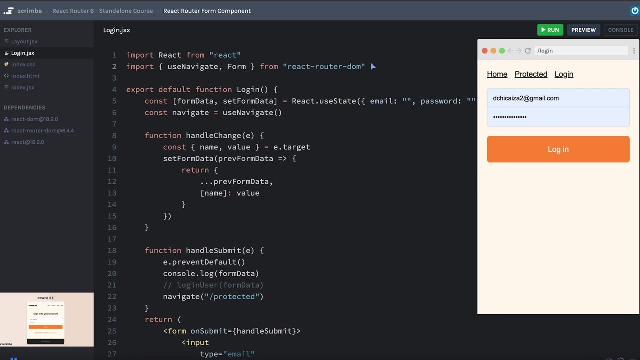 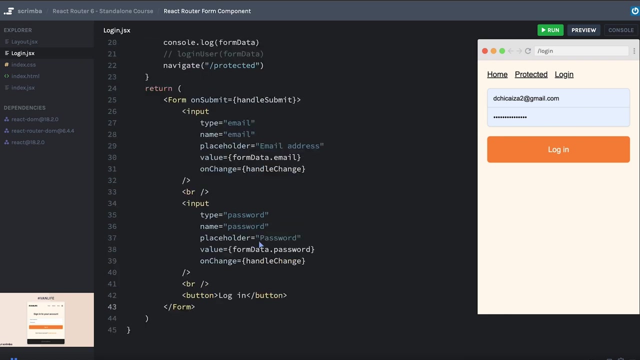 to learn about also comes from. Instead of submitting to a back end, React Router gives us a back end to submit to, So let's get rid of this action. And in order to use the action自 own state and has its own way of relying on the native HTML form, we can set it up to use the 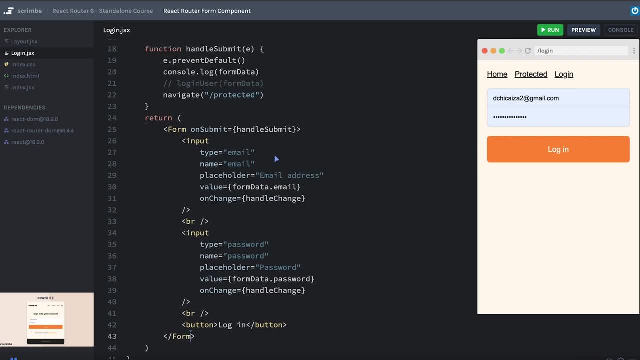 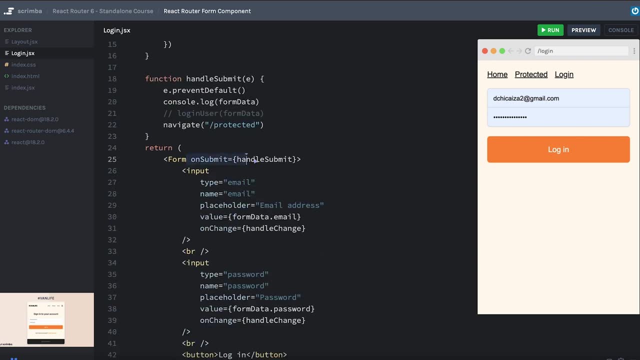 way to submit the data that's in the form. we no longer need to do this imperative handle change or handle submit functions that we had before, which means I can start the really exciting act of deleting some code. I can get rid of my handle submit, which means I 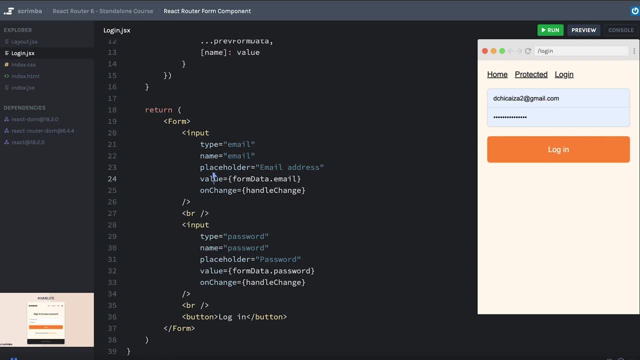 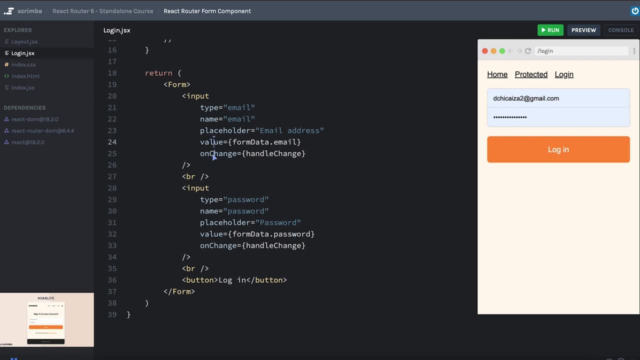 can get rid of this whole function here. that feels really good. We're no longer going to be controlling the state of the form with our internal state, which means I don't need to control the value And I don't need to watch for the on change event, which means 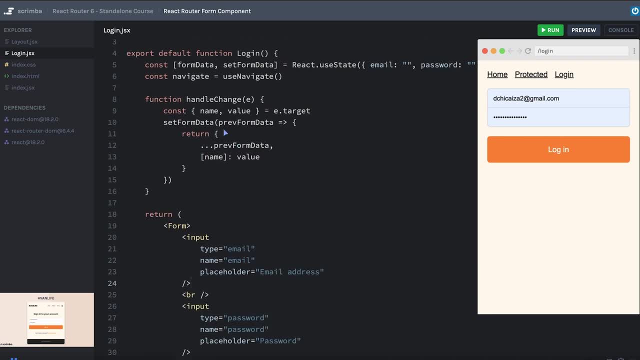 I can get rid of those four lines of code as well, Because we're not using handle change anymore. I can get rid of this whole function. Our on submit is where our navigate was being used. we don't need that anymore And we're going to let the form maintain its own state. 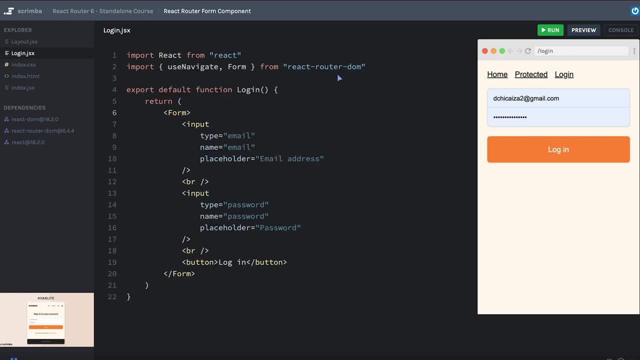 so I can get rid of my react state And just look at that. Obviously, we're not working in quite the same way that we were before, But the form is so much simpler to understand and reason about And, on top of that, as we're going to see if we need to learn information about, 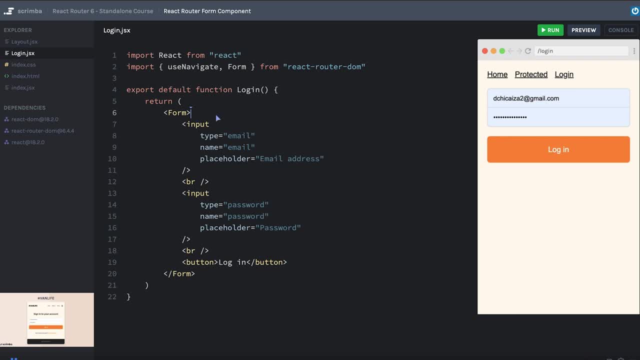 the form. we don't need to go to the react documentation on how to handle forms in the react way. we can simply go to the MDN docs and learn about the form object and form data. I'm getting a little bit ahead of myself, probably because I'm excited to delete code, So in 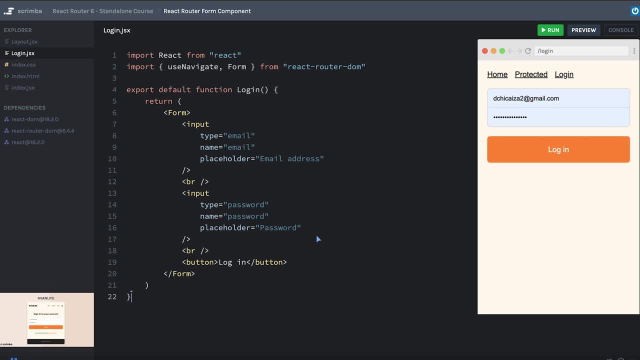 the next scrim, let's jump in. we're going to learn about how to set up the action function in react router Where a form would submit typically to some kind of back end. in react router, our capital F form is going to run a function that we tell it to run. The syntax for setting this: 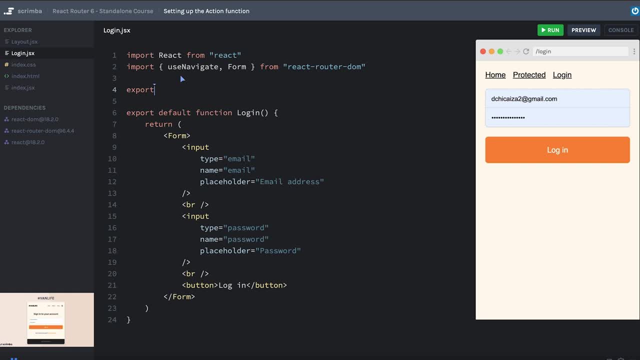 up is going to look very similar to loaders, where we had a function that we exported, that we were calling loader. Instead, we're going to create a function called action. Once again, the actual name for this function doesn't matter, But there's pretty much no reason. 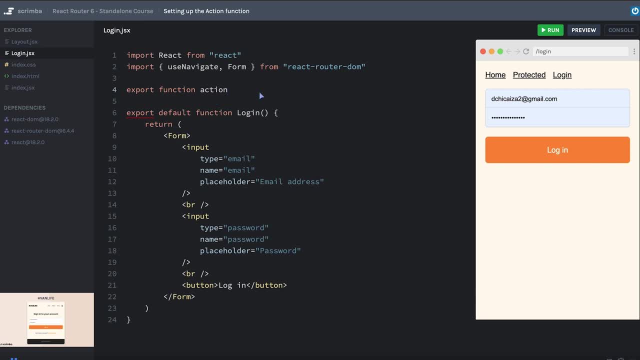 not to stick to the convention of using loader and action And then, in remix, if you're actually building a remix app, I think it does matter that this is called loader and action. Now it's up to you if you want this to be an async function or not. I'm going to choose for it. 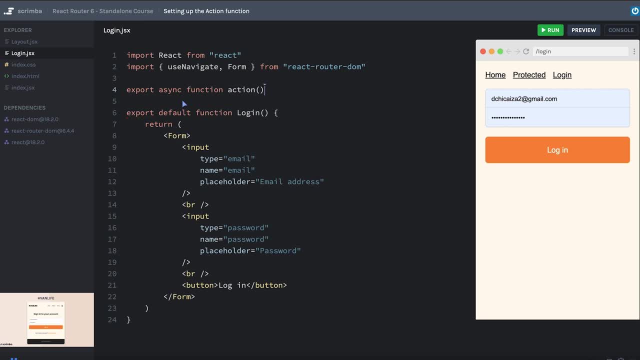 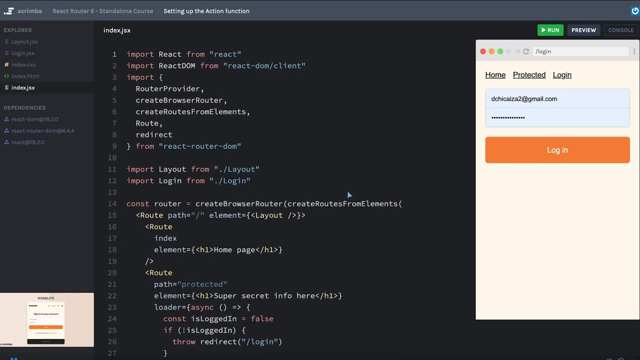 to be an async function, just to make the syntax a little bit nicer to deal with. And just like we did with loaders, I'm going to go over to my index where my route definitions are, where I'm importing my login. I'm going to grab my action. That's a named export. 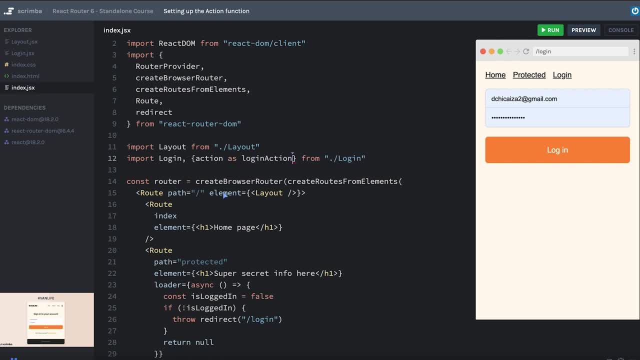 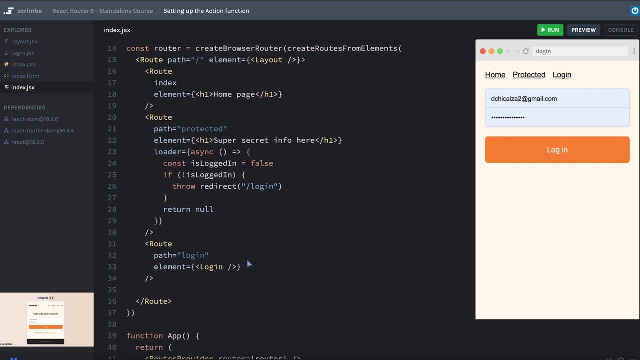 So I need to say action and then we'll just rename it as login action, just for the sake of it, Just in case we have other actions that we were to need at some point And where before we had a prop called loader, this time we're going to have a prop called action And I'll 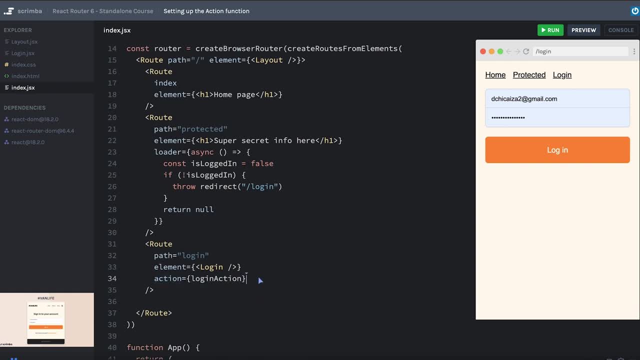 just set up that imported function as the action on this route. So what exactly does this mean? Well, if I have anything that submits a form from my login component on this login route, it's automatically going to call the function that I pass into the action prop. 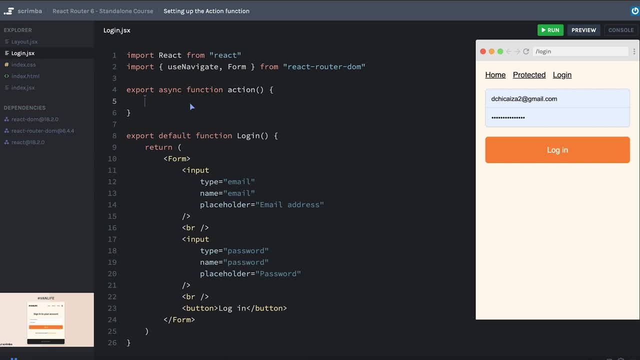 on that route. So let's go back to login And maybe for now I'll just console log. I'm the action function And we're going to submit this form And we're going to see something pretty interesting. So I'll hit Login And 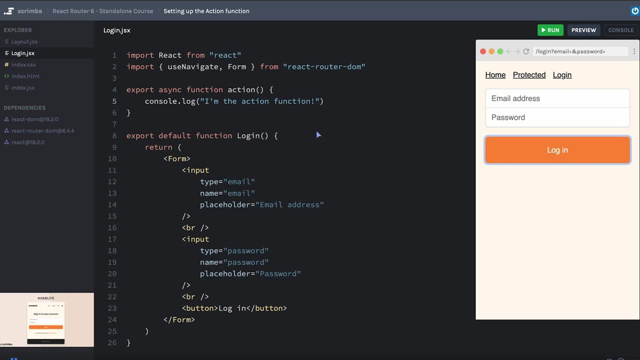 it looks like nothing happened. If you have quite the eagle eye, you might have noticed that in our URL it did serialize the information based on the names of the form, email and password, and put them up inside of the URL: login Question mark. email equals nothing and password equals. 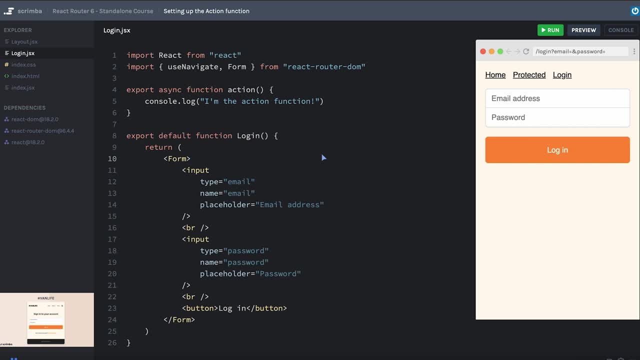 nothing. That might seem confusing first, but you would quickly learn that that's the default way that forms work. If you don't tell it that you are performing a post request as part of your form, then it assumes that you're doing a get request And in a get request it's serializes the inputs and it puts them up in the 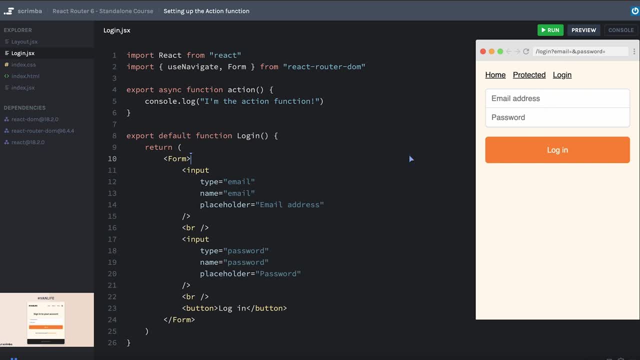 URL. However, we are going to be handling our login form as a post request, which means on my form I'm going to include the- by the way native attribute called method and set it equal to post. Now one last thing: before we actually submit this, I'm going to get react router complaining. 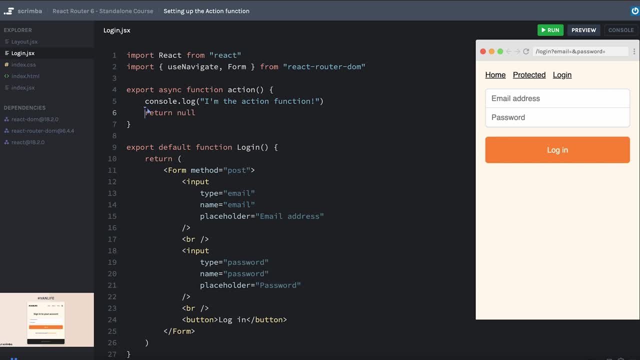 that I'm not returning anything from my action function, So I'm just going to add this: return null here. Okay, now that I've told my form that its method is post- and again, this is something native to HTML forms, this is not something specific to react router- I'll go ahead and hit. 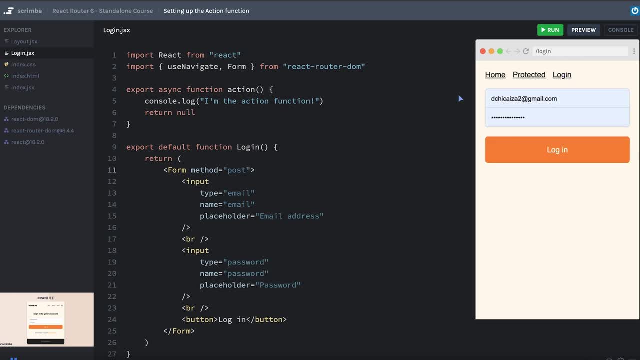 Save And let me click on login to get rid of those query strings. Again, we'll hit login And sure enough, I get my. I'm the action function console log running Now. you probably remember that I'm the action function console log running Now. you probably remember that I'm the action. 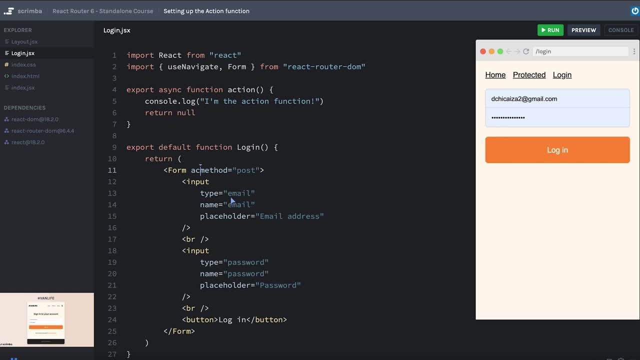 function console log running. Now you probably remember I was talking about how native forms would take an attribute called action, where you could tell it where to submit that information to, like some kind of PHP file And technically, in the react router, capital F form you can also. 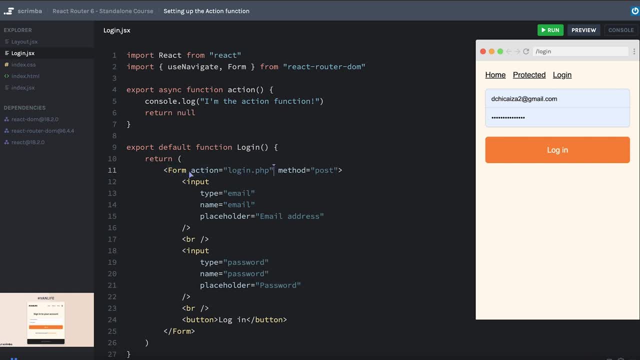 include an action prop here. However, the react router form does a pretty good job of having sensible defaults where I usually don't find myself having to include an action prop at all. Generally speaking, the default is going to be wherever you set that action up in your route. 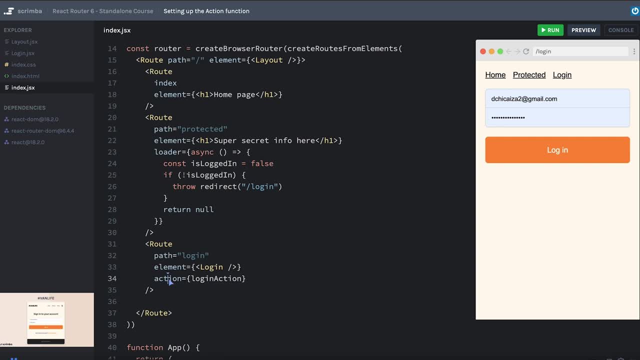 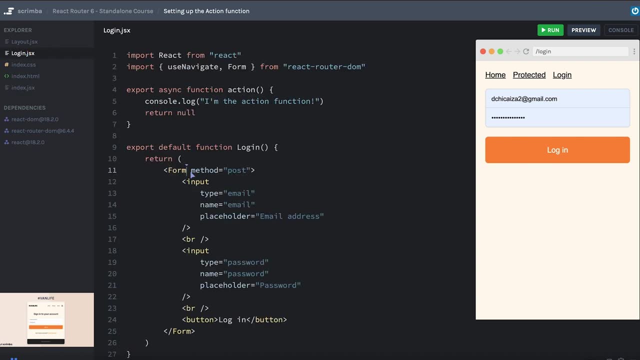 definition. So here I told it that the login action is going to be the action that should occur on the login path, And so that default will just automatically be included or understood by this form. So instead of saying action equals slash login, since that's the route where the 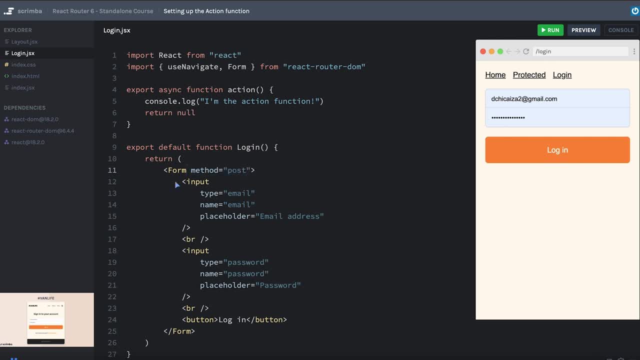 action function will be handled. I can just omit that, and it'll usually have the correct default there. Okay, the last thing I want to do is see that there's actually an object coming in from the action function here. So I'm going to go ahead and hit submit, And I'm going to go ahead and hit submit. 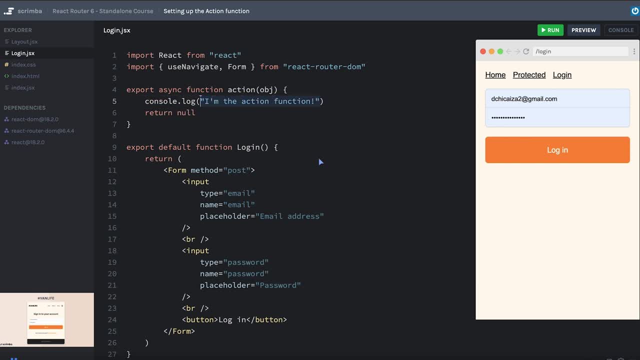 So we'll go ahead and console log the objects just to see what that looks like. I'll hit save and submit And we can see that object has a request property and a params property. that should look pretty familiar, because that's exactly what gets passed into our loaders as well. 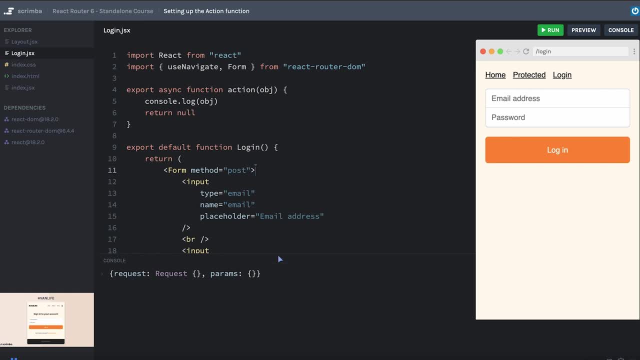 And that's where we're going to get access to the information that gets submitted in this form. That's what we're going to be working on very soon, But since we've covered a bit of ground already, we are going to come back to the van life app and apply what we've 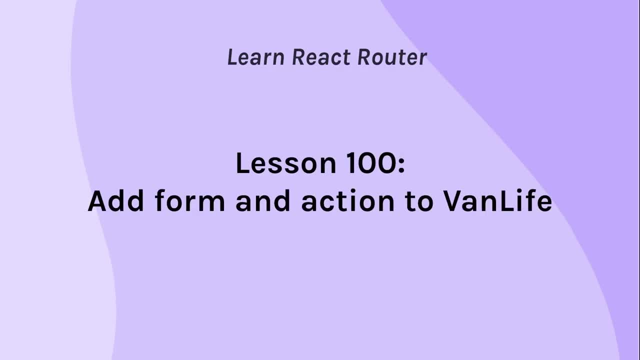 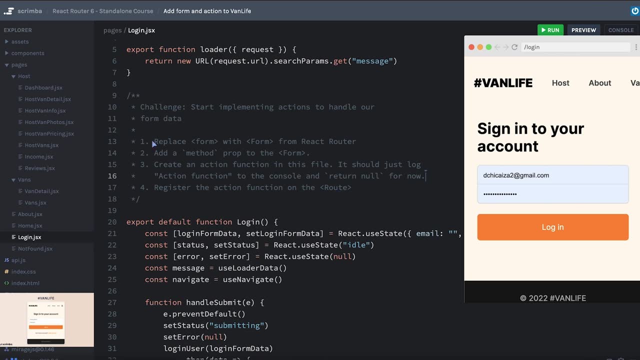 learned over there. All right, let's apply what we've learned about action functions and start building it into our sign and form. In this case, I was pretty explicit about the steps you'll need to take in this challenge, So just make sure to read these steps carefully, And you should. 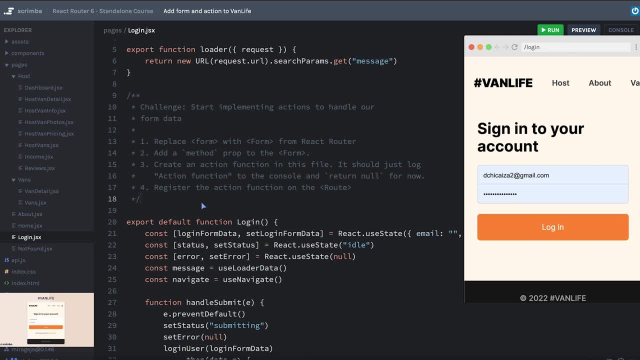 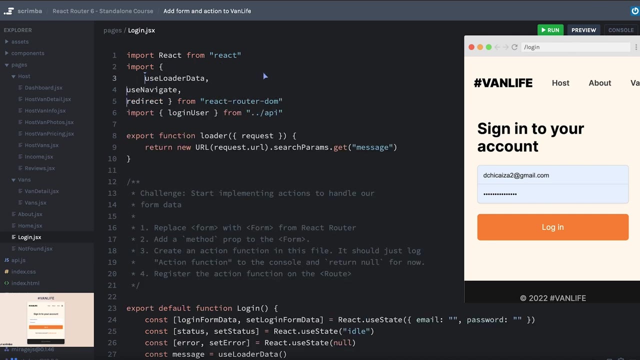 have a pretty easy time of this. pause now and work on this challenge. Okay, in order to replace this form with the capital F form, we will need to make sure that we import that. just because this is getting a bit long, I'm going to go ahead and 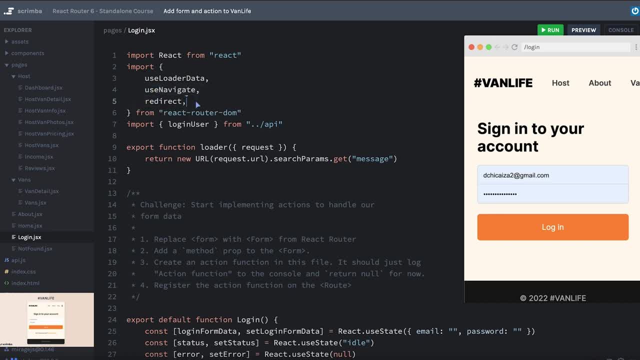 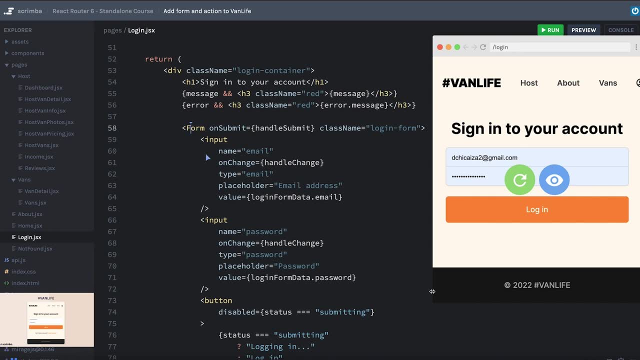 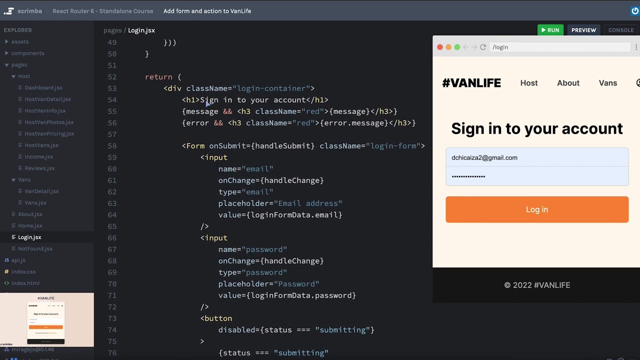 put things on their own lines And then we'll import our capital F form and go down and replace our form. Let's see where is it right here with the capital F form that comes from react router. Okay, we need to add a method prop to the form. So right here, we'll say the method is going to be. 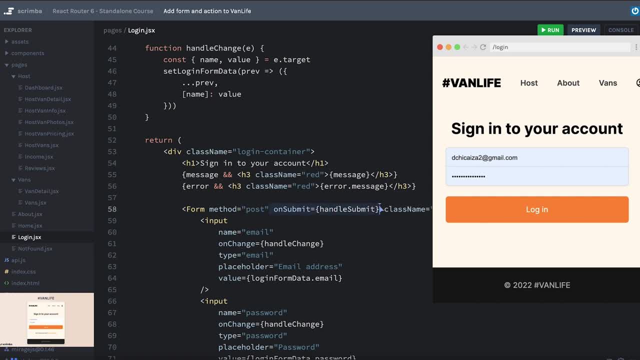 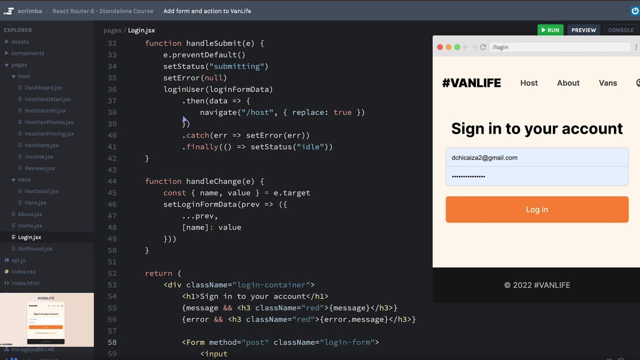 post, And this is getting a bit long. I already know I'm not going to need my on submit, So I will go ahead and get rid of that And I'll leave this here just so I can reference it if I need to. we're just going to worry about the form for now. Okay, so let's see. 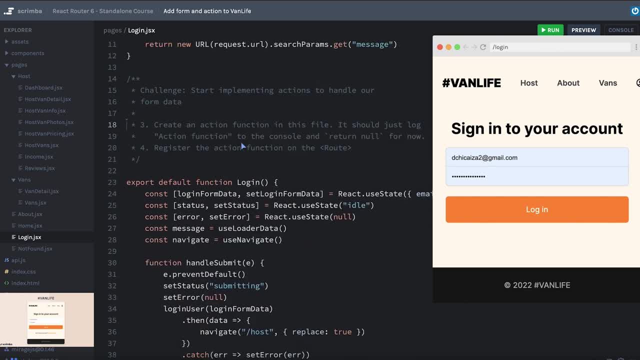 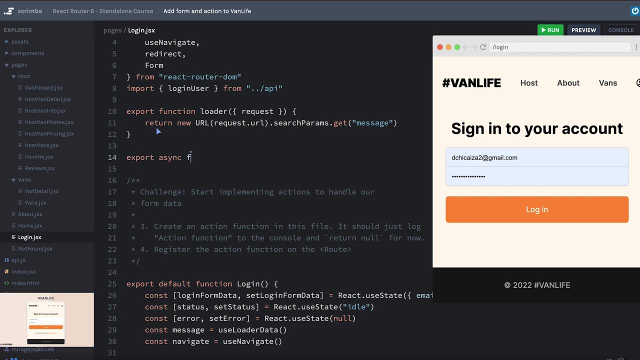 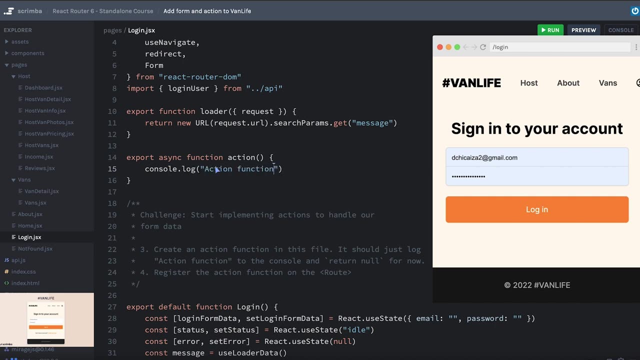 that was number one And that was number two. Okay, so we need to create an action function in this file, maybe just right here below our loader. I'll go ahead and create an async function called action And I'll just have it console log action function, And we'll make sure to do the 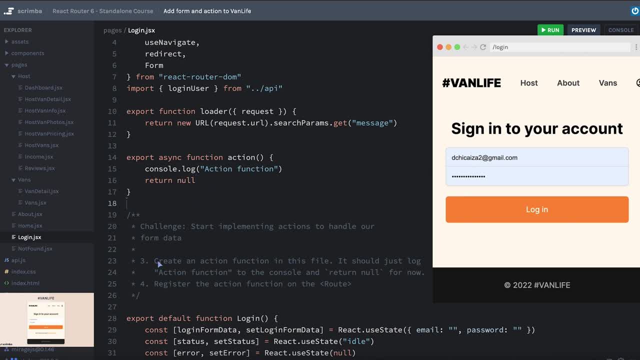 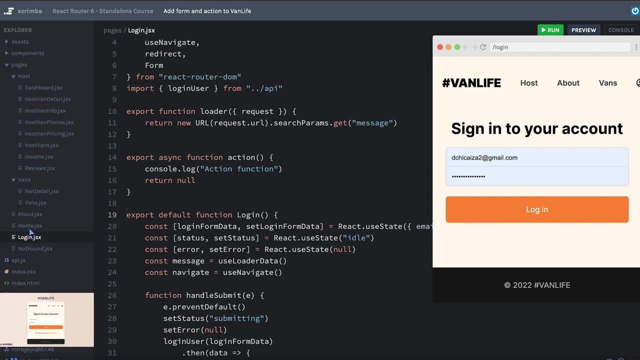 same thing in the file, just so react router doesn't complain to us too much. Okay, that's number three. And then for number four, to register the action function on the route. okay, we can do that. Get rid of this. we'll go over to. let's see, we're already exporting. it will come to our index. 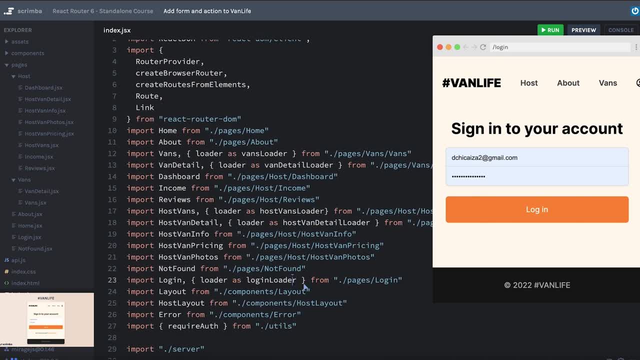 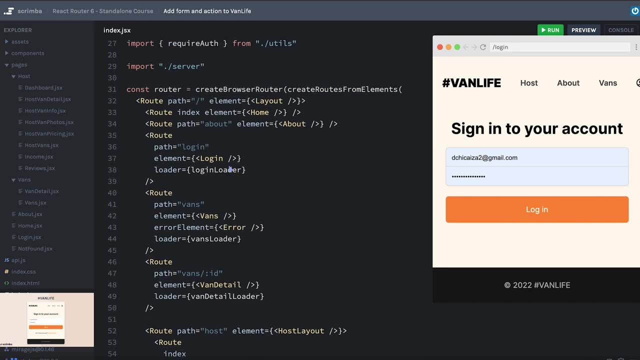 file come up to where login is. we have our loader as login loader And we'll go ahead and bring in our action as login action And, just like we did see where it's here, we go loader, we'll say action, action. Okay, let's hit refresh And let's come to login, Just so we can take a look at our code. 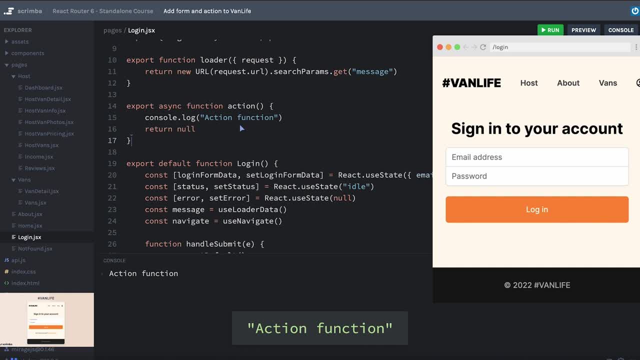 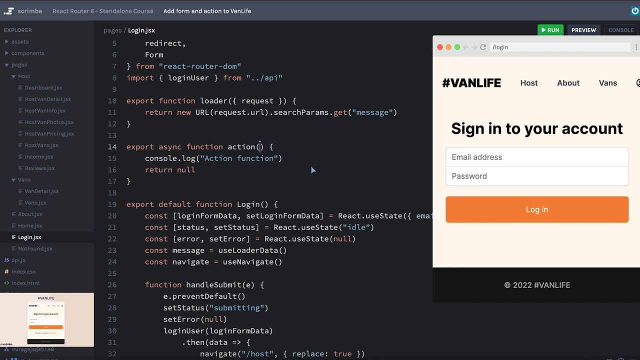 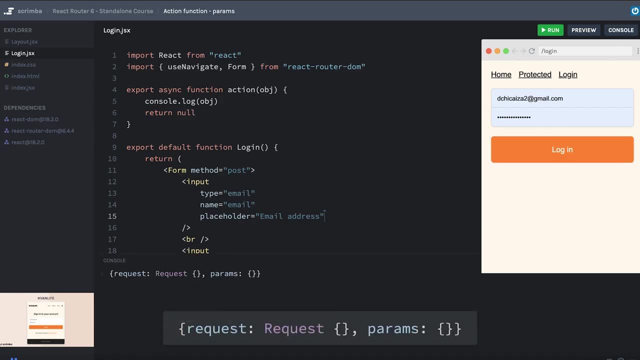 We'll hit the login button And, sure enough, the console log for action function ran. Okay, let's go back to our practice app And we'll learn how we can pull in data from the form so that we can actually do something with it. Okay, let's submit our form again So we can see what gets. 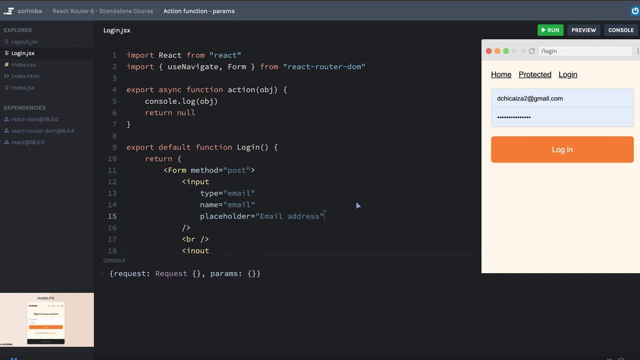 logged to the console. Again, we have an object that has two properties: request and print. So we're going to call it params. We'll take just a few seconds to talk about the params and then we're going to focus mostly on the request. when you see params inside of our loader or our action, 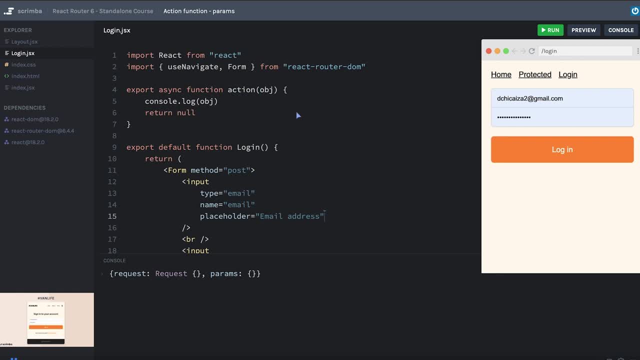 objects that gets sent as the parameter to the function params is referring to route parameters. So if our path were something like slash login, slash colon ID or colon whatever, that would mean that this path or this route has parameters attached to it that we could. 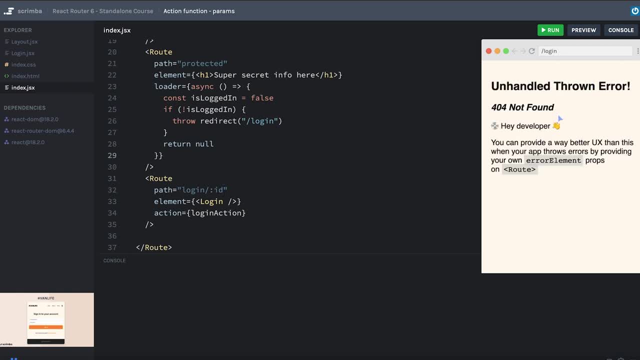 grab from our action function. In fact, let me hit save our logins going to be gone because that route doesn't exist and we'll say login slash, whatever in the url. we get our login page back. we can go here, we'll submit the form and now we can see that the params object. 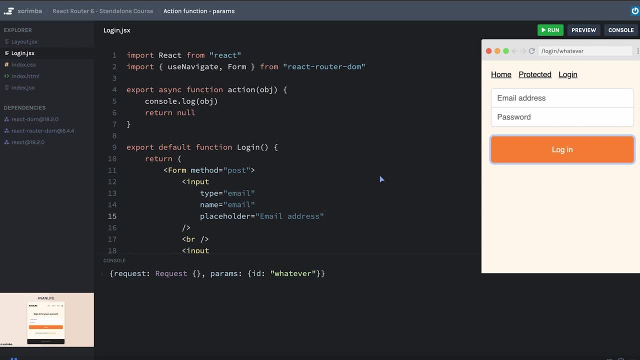 is not empty. it has a property called id and the value is whatever, because that's the parameter for this path. so it's really just good to know that in our action function, if we needed access to our params- for example if we were trying to update one of our existing vans- we'd be at maybe slash. 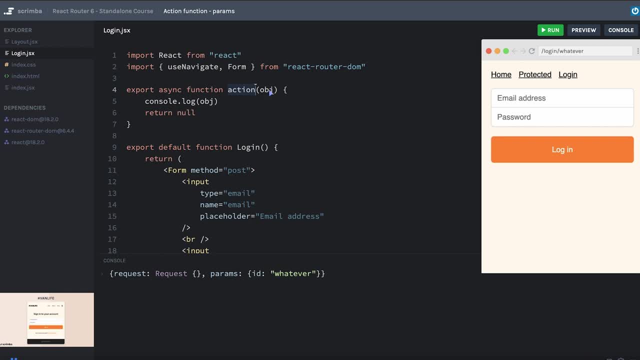 host slash van slash one, we can grab the parameter of the url and say, hey, we need to make a request out to slash api, slash fans, slash one, which we grabbed from this object, and make whatever change was necessary. let me go ahead and undo this, because that's not our use case here for the login page. 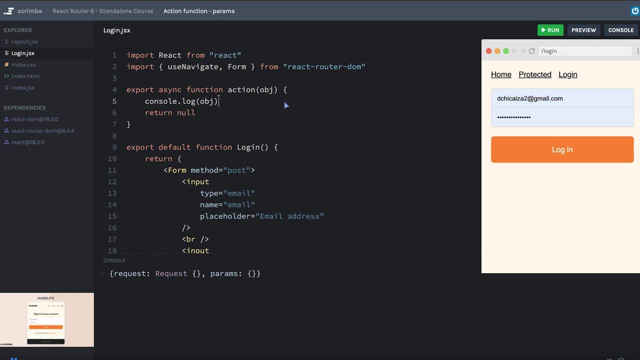 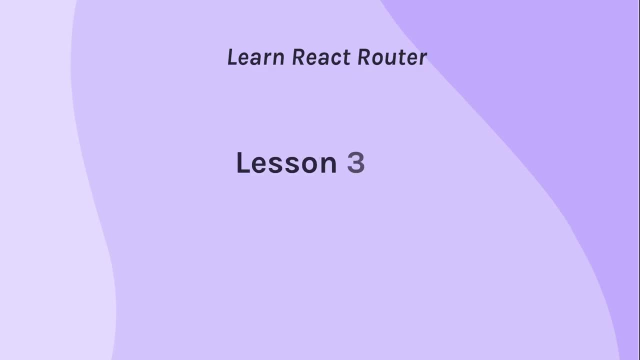 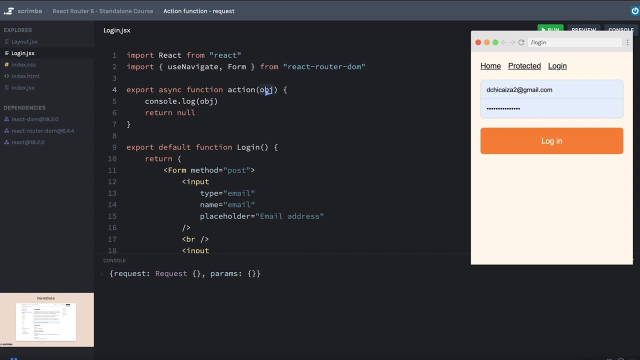 okay, now let's talk about the request object. and i think, just for the sake of compartmentalizing the different topics into their own scrims, we're actually going to do that in the next lesson. okay, let's look now at the request portion of this object. so instead of pulling in the whole 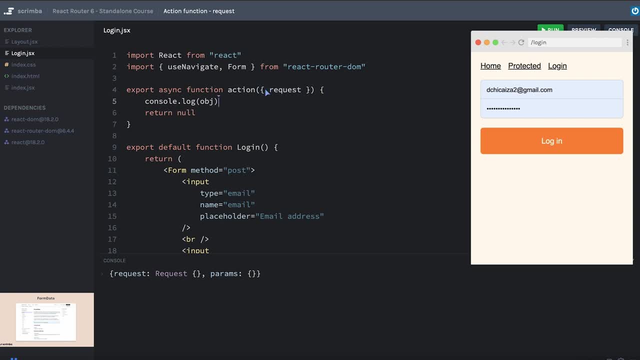 object. i'm actually going to destructure it and just grab the request part. in our case, we don't need the params part, so we'll just leave it this way. now, the reason this is called request is because in a native form, when you submit it, it normally would send a request out to that back-end. 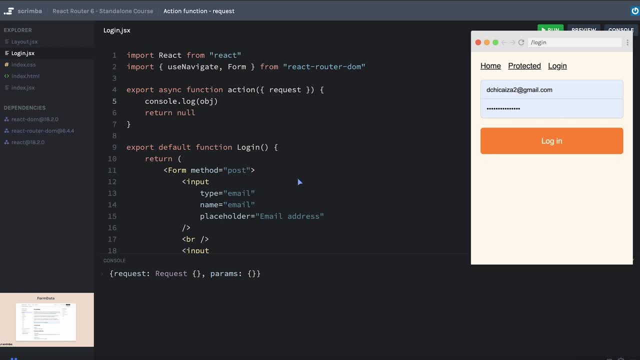 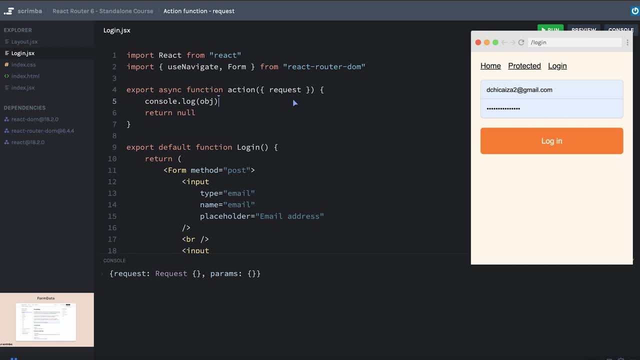 end would process that request and do something with it. in our case, because we're just working entirely on the front end react router with this action function- is basically intercepting that request and giving you access to it here in your action function, which gives you the chance to. 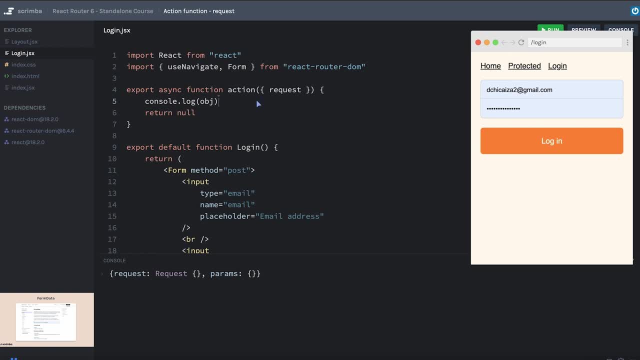 process the information from the form in whatever way makes the most sense for you. essentially, this action function is replacing the handle submit function that we had before inside of our component. so what can we do with this request object? well, one of the pieces of that request object is the form data that's coming from our form. i can get access to that form data by: 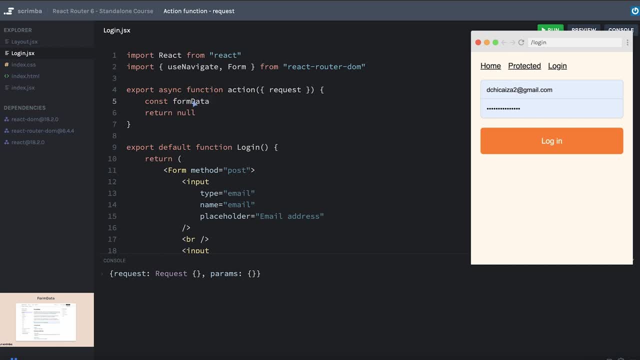 saying const form data or really whatever you want to call it, is equal to request dot form data. now, calling this form data function is actually an asynchronous function. so i can say i'm going to await the value that comes back when the promise is resolved and that will give me the correct access to my form data object. and this form data object is: 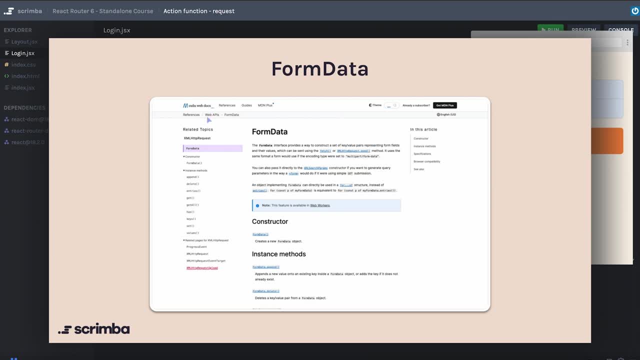 the native javascript form data object that you could go to the mozilla developer network docs and read about. in fact, if you'd like, you can click the screenshot here to take you to the mdn docs about form data. instances of form data have a property called get, and so now i can gather. 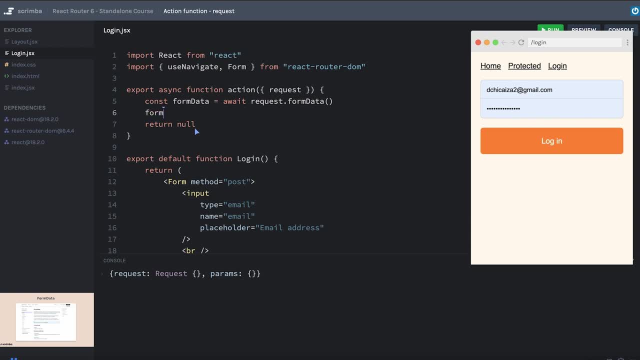 information from the inputs of my form by saying form data dot get, and then i would pass the name property of the input that i'm trying to get information about, or rather trying to get the value from. so because this was named email, i need to make sure that i say formdata dot get email and for password, i'm going to do the same thing for the. 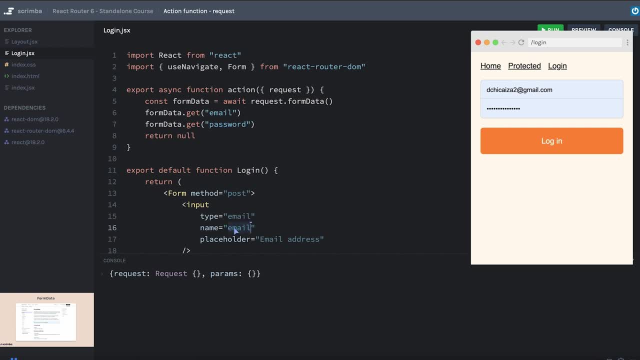 password. so i'll say password. if this email were named the name property or something like blah blah, then i would have to say dot get blah blah. let's keep it as email for now. just getting it from the form data is kind of useless to me unless i save it. so we will save it in a variable called. 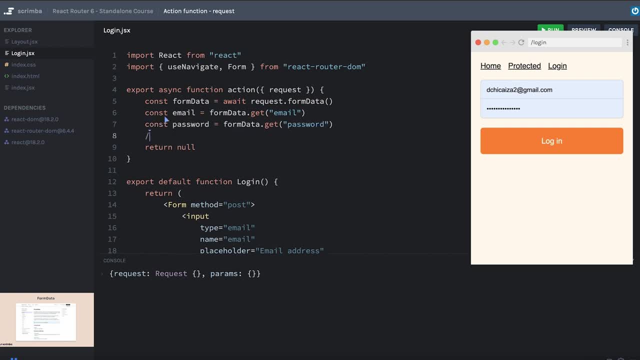 email and and password, And at this point, I could then just process this info however I wanted. In the case of our van life app, this is where we would pass the email and password to the login user function, So let's go ahead and make sure that this is working correctly. 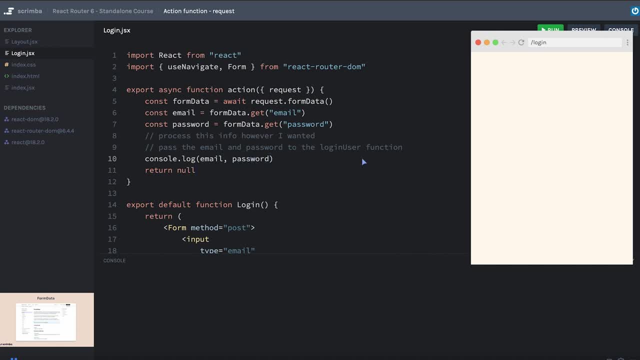 We'll just console log both of these. we'll go ahead and hit save, we will fill in bfbcom And then I'll just do SDF and hit login And cool. inside of our action function we now have access to the values of our inputs. Since we're here mentioning the login user function, 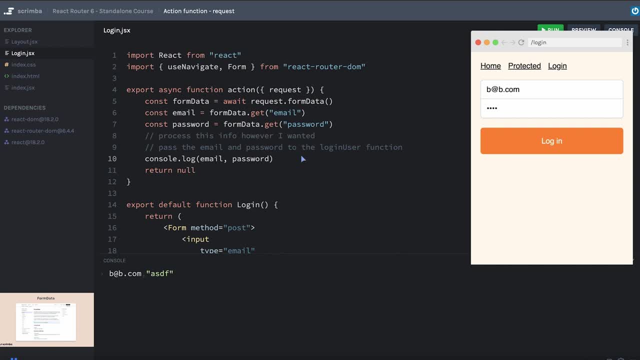 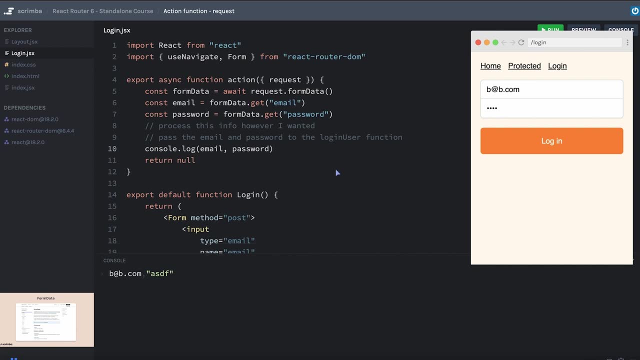 from our van life app. that's a great segue for us to take what we've learned here and apply it to our van life app. However, before just jumping ahead, feel free to take some time to play around with this code. If you want, you could add an input or two and try. 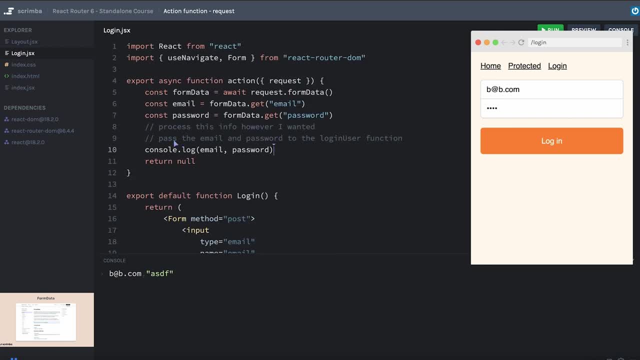 to get the values from your action function and try to commit the process that we've done here to memory, Because your challenge is going to be to apply these exact same principles to the van life app. So that's what we'll be doing next. 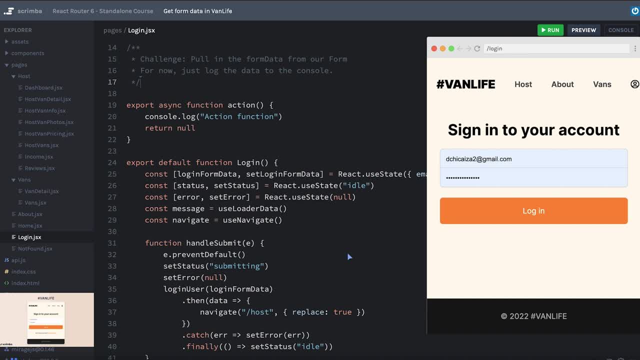 Okay, now it's your turn to get your hands on the keyboard. you'll essentially be doing exactly what we did before. your challenge is to pull in the form data from our form when it gets submitted, And for now, you can just log the data to the console. you'll probably 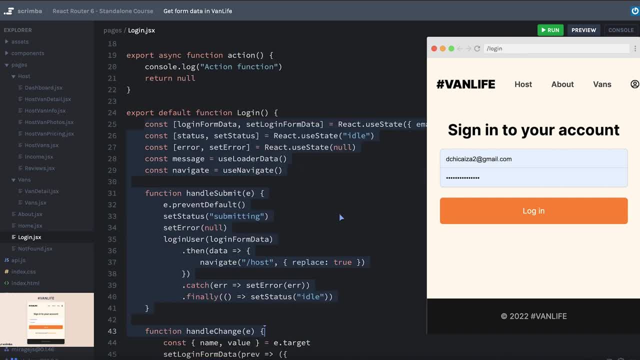 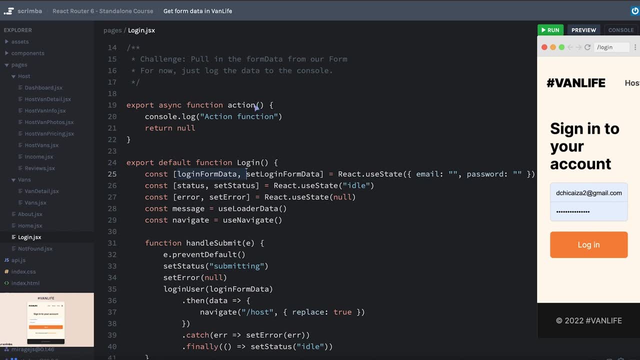 notice that we're still doing all of the more imperative form handling stuff that we were doing in react, including, say, saving the form data as part of react state. But for now it should still work. if you pull in the email and password to the action function and just log, it will be getting rid of a lot. 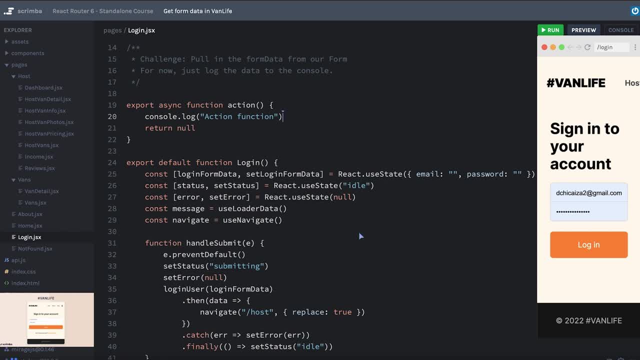 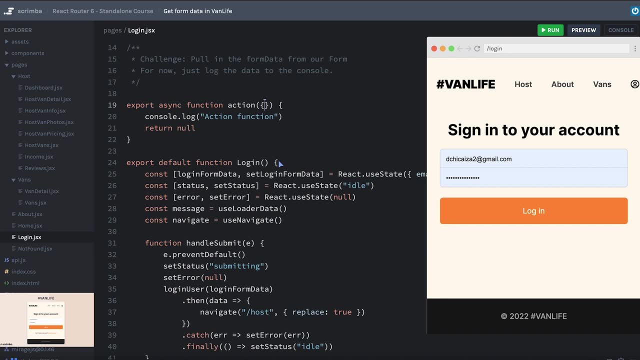 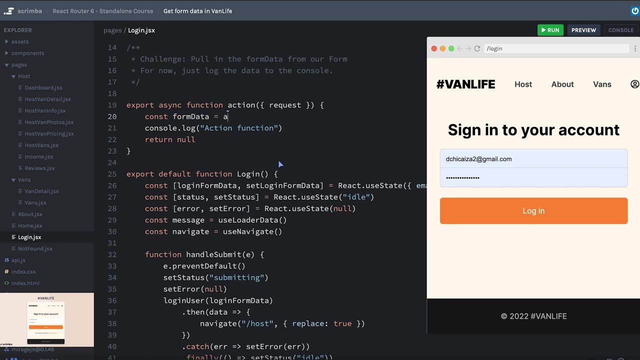 of stuff here soon. So pause now and work on this challenge. Okay, our action needs to get access to the request And with the request we can get access to a form data object by saying: await- request dot form data. This await can be tricky to remember. hopefully that didn't trip anybody up too much. And then 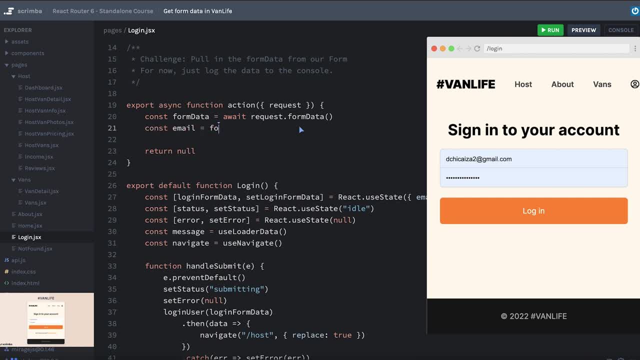 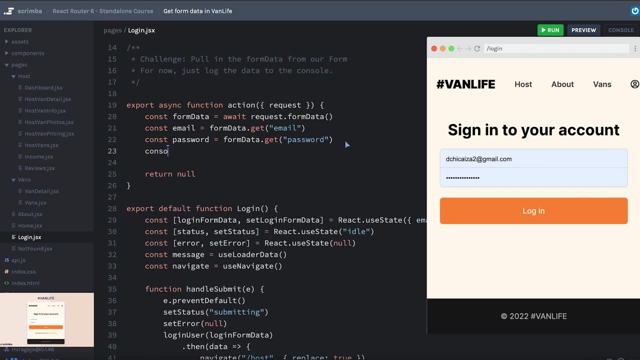 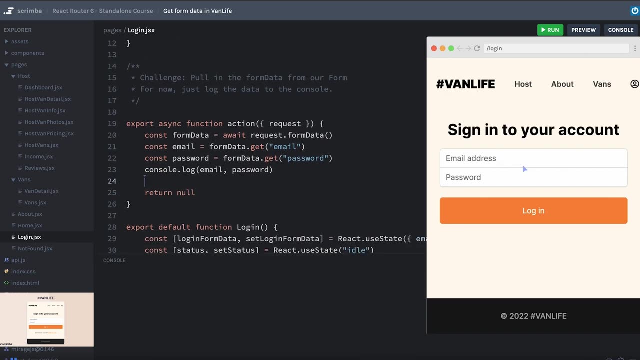 once we have access to our form data, we can get the email with form data dot get email And we'll just do the exact same thing with the password. Let's go ahead and console log our email and password. We'll hit Save. open up our console. Then be at bcom p 123.. Login. 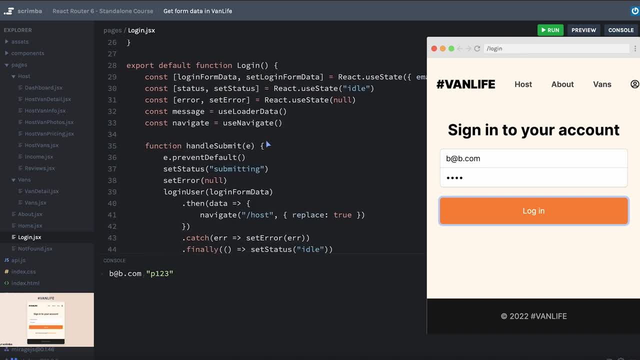 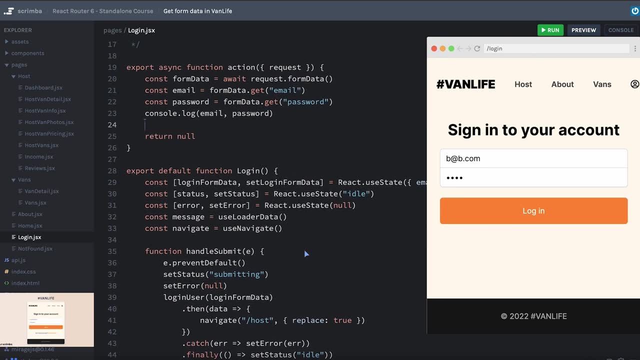 Awesome Again. our action function is slowly starting to take shape as a replacement for our handle submit, but with a number of really nice additional benefits that we haven't yet talked too much about Before we start. a major refactor of the login component code: we are going to take the email and password and actually log our user. 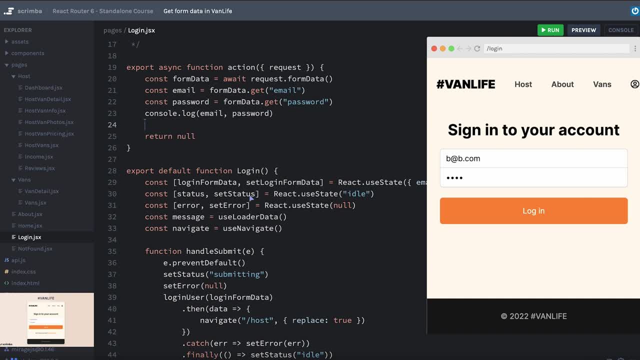 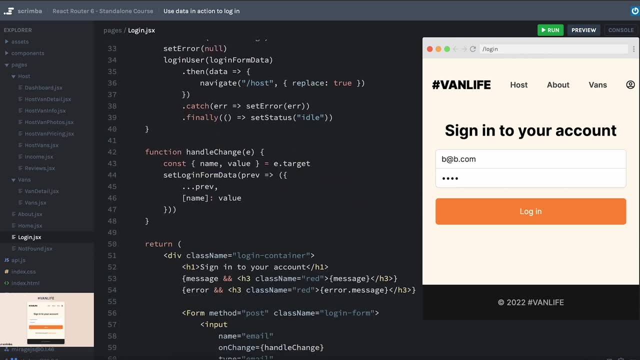 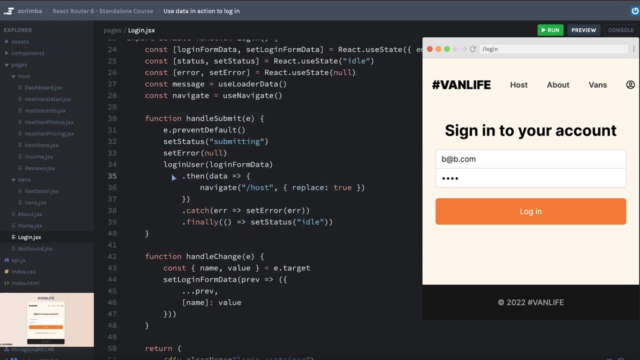 in and kind of complete that workflow, And then we'll come back and we'll start cleaning up our login component. You might remember, in our form we had an on submit event handler that was calling our handles submit function here. This is the function that was logging in our user. But now 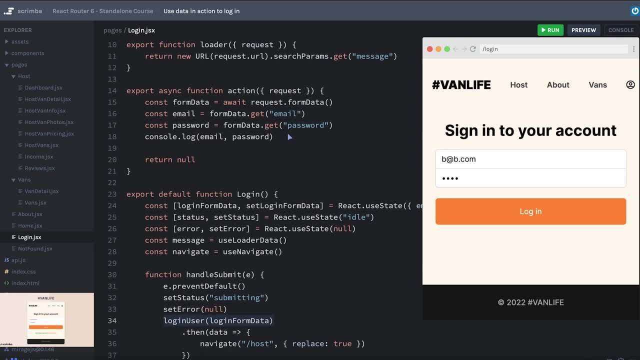 that we're using these actions or this action function, we're no longer logging in our user. hopefully it's not too big of a leap. to see that really all we need to do is to take our login user function and call it up here in our action. So we'll go ahead and call login user this. 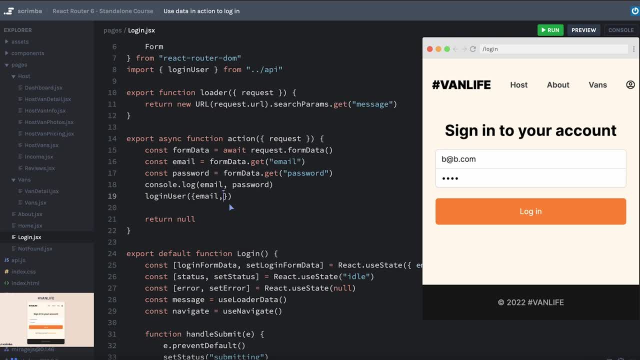 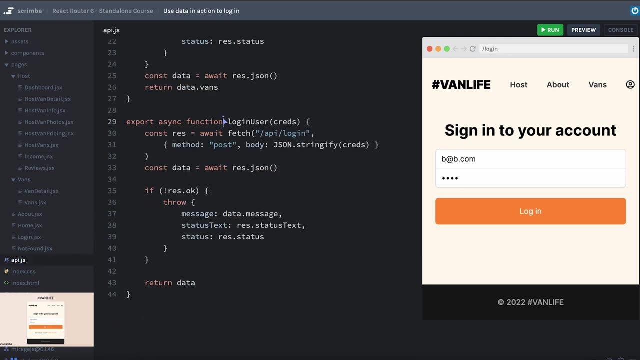 function expects an object that has an email property and a password property And since we chose to name our variables email and password password, we can use this shorthand to pass in an object with these properties. the login user function is an async function. we can look here in the API js file and see that. 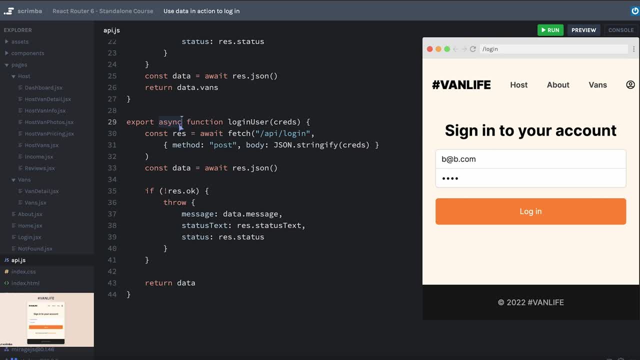 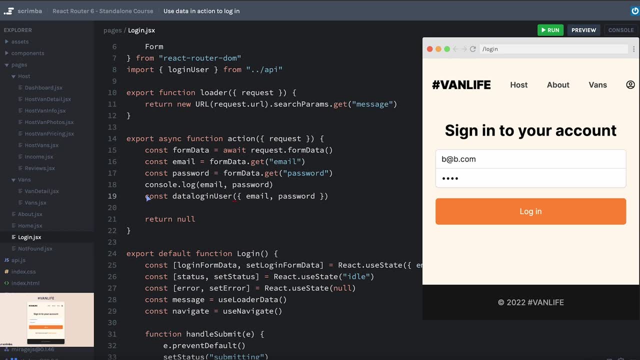 it's an async function And it's going to return data. But since it's an async function, it's automatically going to wrap that data in a promise And I can unwrap that by using the await keyword. So I'll say: const data equals await the call to login user. let's. 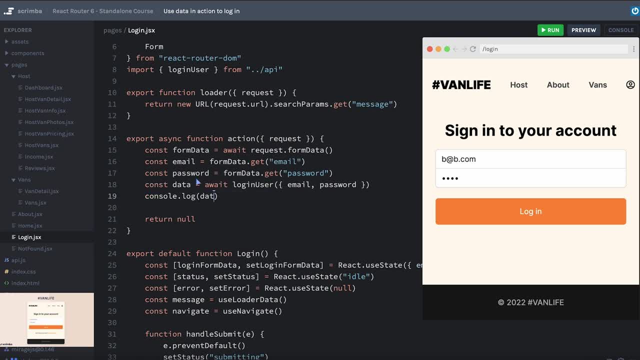 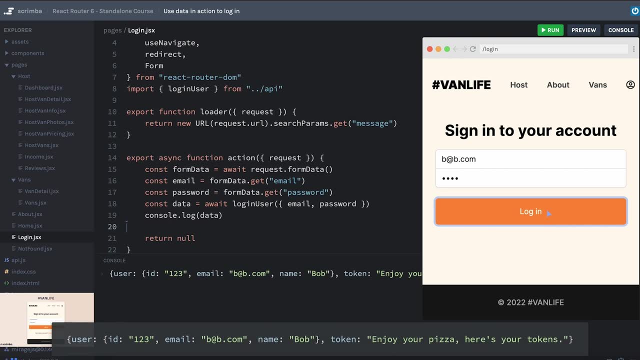 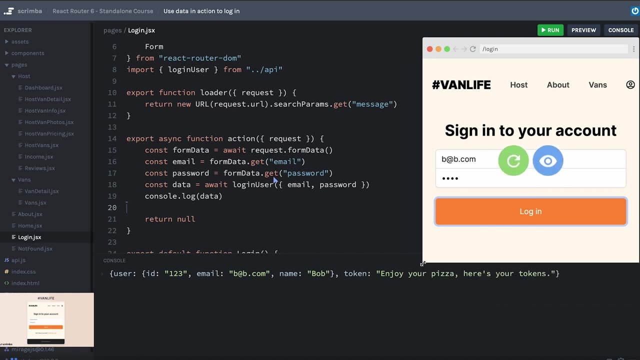 move our console log down here and change it to log our data. we'll hit save, put in B at bcom P 123.. And sure enough, there we go. we get our user object, which you might then decide to put into some kind of authentication context or into local storage or wherever. 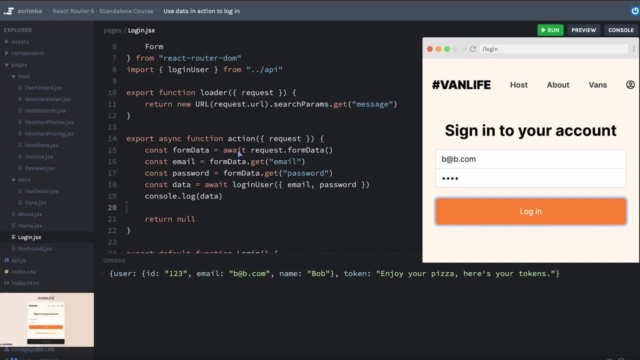 makes the most sense to have information about your currently logged in user, And then we also get our token, which we could save in a number of different ways. Oftentimes it's best to put it inside of a cookie, which might be something that's actually handled by your server, Because we 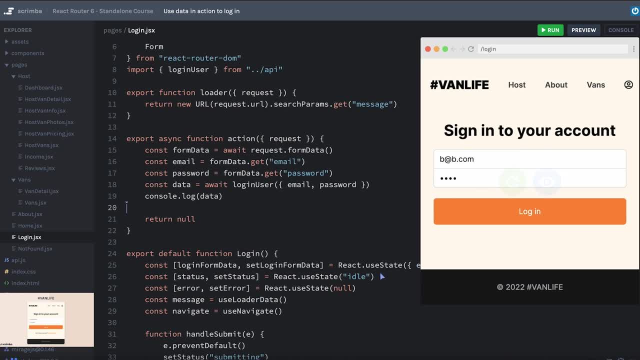 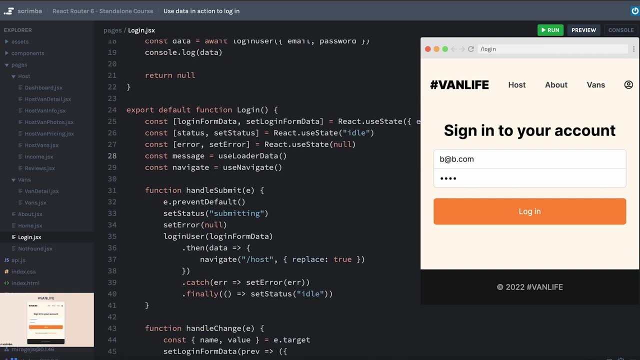 did go out of our way to code our sad path where we have the different status and the error states that we're maintaining in our component. we're not quite ready to just delete everything, But we can start on that path. For example, right now we are no longer needing. 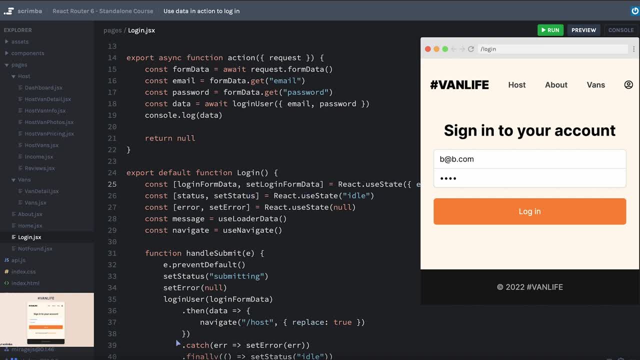 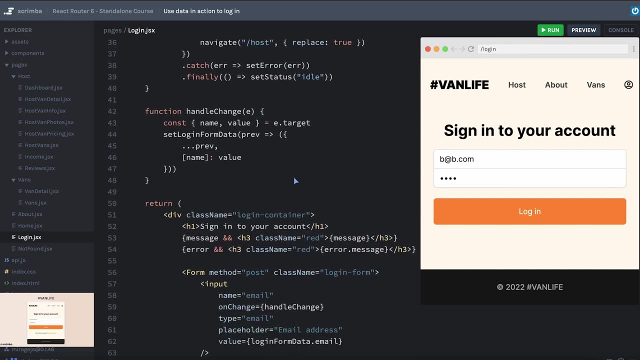 the state where we're maintaining the values of the inputs. Instead, we're using the internal state of forms to handle that. So I can go ahead and get rid of that local form state. I can come down to my forms and I can get rid of my own change And my value props right here. we don't need 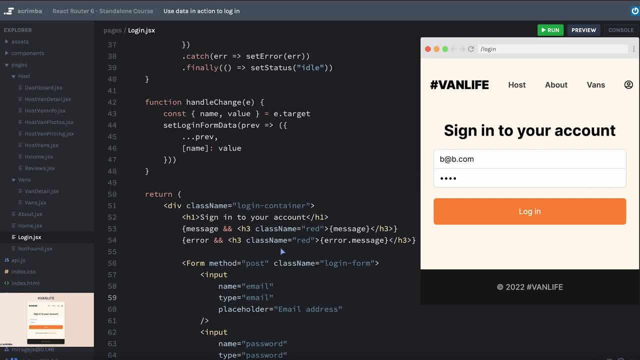 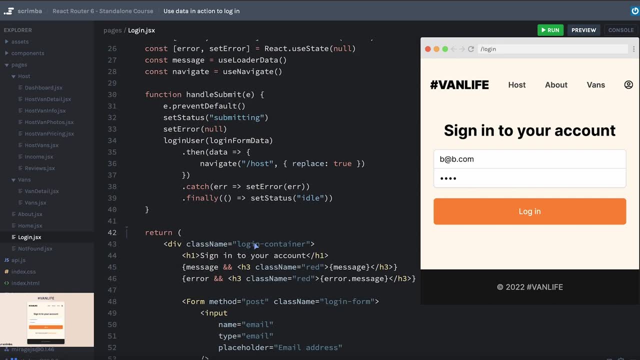 those anymore. That simplifies our form quite a bit And because we're not watching for changes in the form manually anymore, I don't need my entire handle change function. This is a great start. we're gonna see that we can clear up even more of this later, But 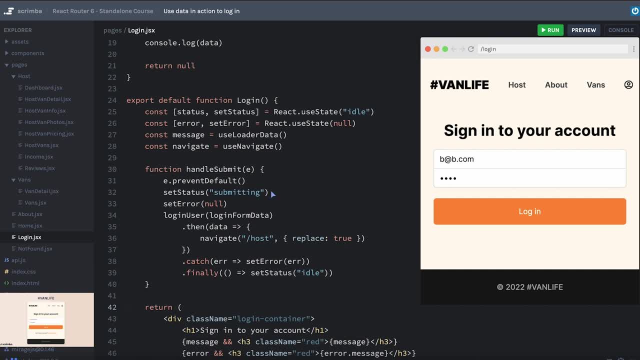 for now, we've made some good headway, And there's one really small change that I want to make, just to make our app seem a little bit more realistic, even though we're still doing fake authentication. So we'll touch it up and we'll be right back. 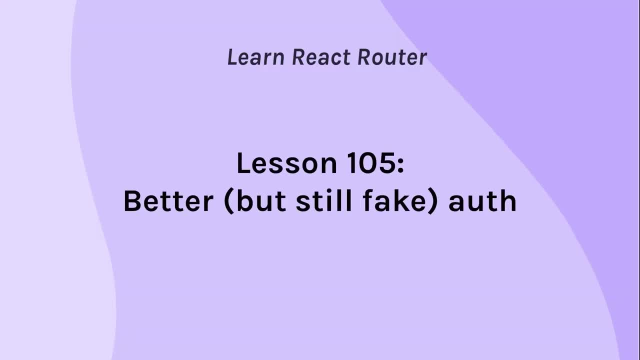 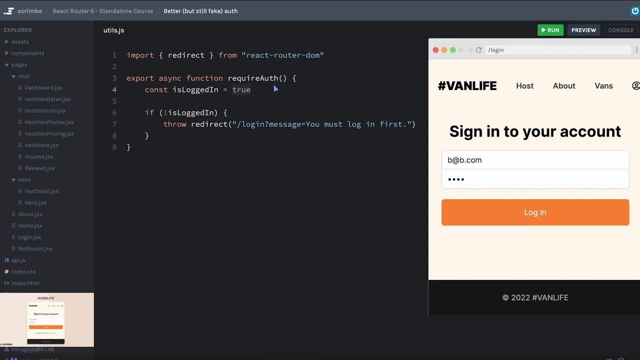 on that. next, In our require off utility function, we are still hard coding the fact that the user is logged in And although I'm not going to suddenly insert real authentication and dealing with authentication context, saving the user across the entire app or anything, 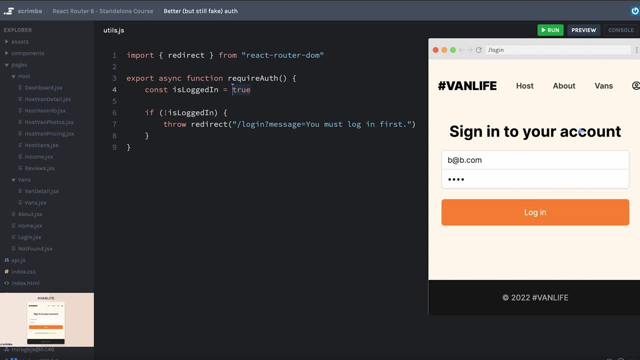 like that. I do want to make it so that, in some form or fashion, when we log in from our form, it remembers that we're logged in And then we can also log out and see how our app would react to that scenario. So I'm actually going to type this up as a challenge for you. 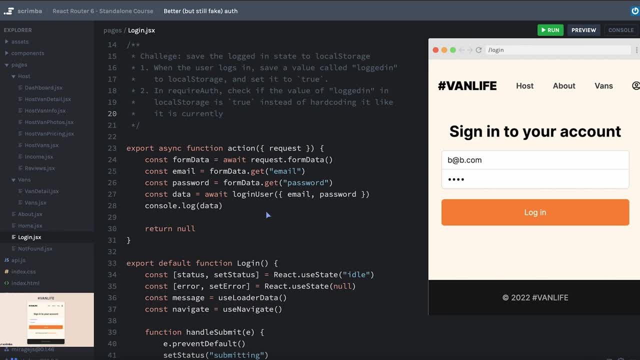 Okay, so we're going to be saving the logged in state to local storage, just again as a temporary way to fake our authentication. I could have just typed this for you, But I figured this might be a good way for you to navigate yourself around the app and to 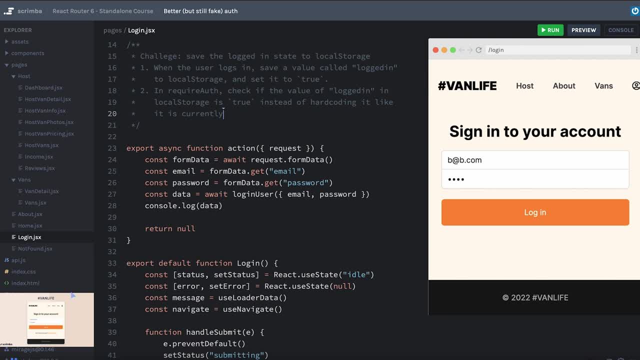 think critically about how this might work and play with some of the different files that we've created. So when the user logs in, I want you to save a value that we'll just call log in. So I'm going to type log in to local storage and set the value of logged in to true, maybe. 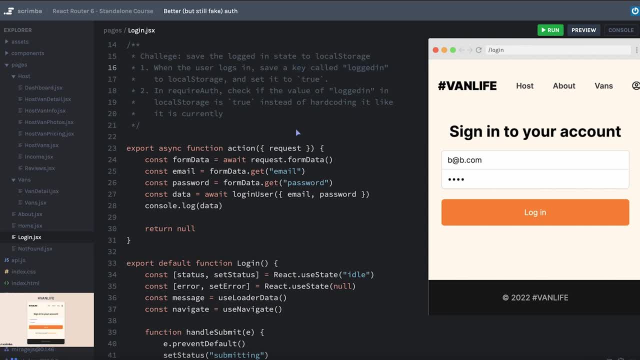 instead of saying save a value, we'll say save a key called logged in and set the value of that key to true. Then, over in the require auth function, you need to check if the value of logged in and local storage is true, instead of hard coding it like it currently is. It's. 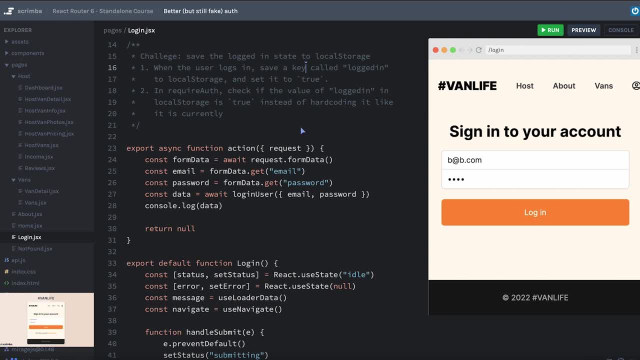 a fairly straightforward challenge. it shouldn't be too difficult. If you need a reminder on how to deal with local storage, you can always do a quick Google search. it's a pretty common thing, So you should be able to find good answers out there. And hey, you dispel challenge. 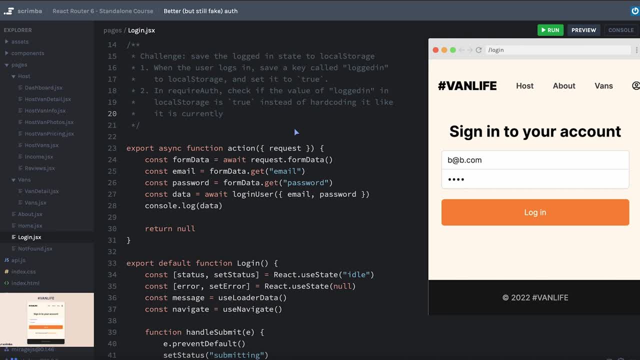 right. Okay, pause now and work on this challenge. The user is logging in here in our action function, or rather, we're calling the login user in our action function. Right now we're still only coding the happy path, But we're going to get to the sad path later. For now, 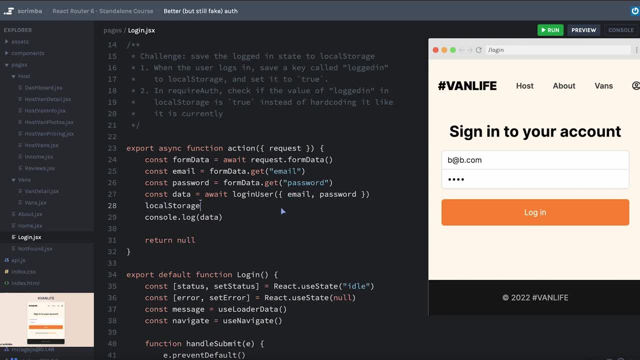 we'll just assume that everything will work well, And so I'm going to say: local storageset item with the key of logged in to the value of true. In reality, I think this might get stringified, But that's okay, it'll work, because we're just going to completely remove the. 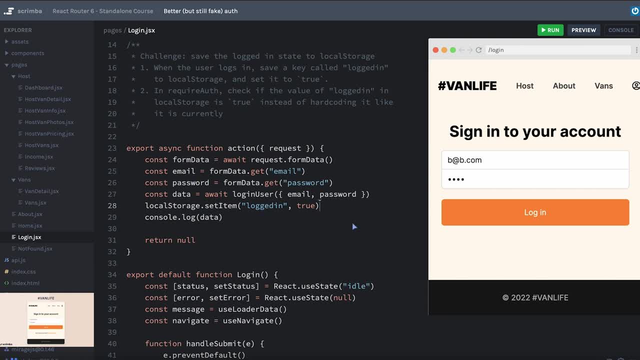 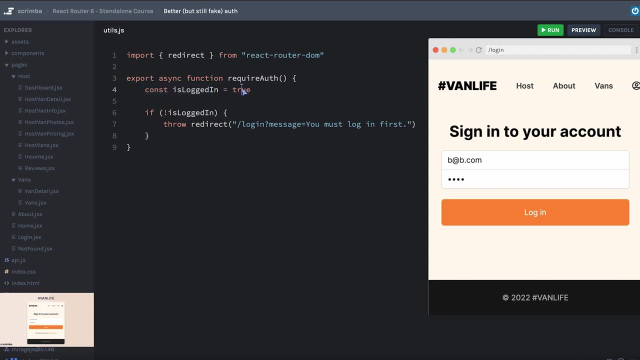 logged in value from local storage when they log out. So that's okay for now. we'll get rid of this console log And then over in our utilsjs, instead of hard coding is logged in. we're going to set it equal to local storage. dot get item of logged in And that should. 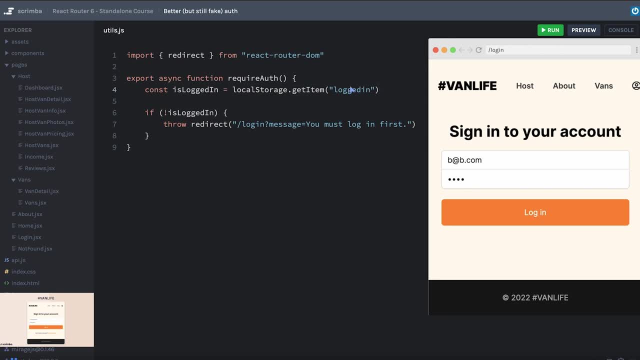 be it, And now we'll make sure that we don't set it to false, because I'm not sure if that would work. I guess we can test it, But we'll just go ahead and remove the logged in item completely. Okay, let's hit refresh, And we should be able to test this now by trying to go to host. 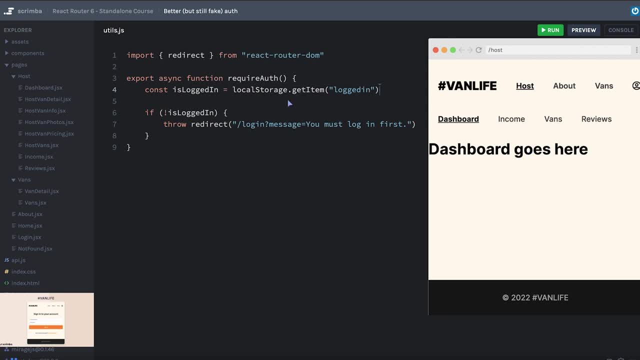 So since I'm in host, it appears that I am logged in. I have something in local storage- maybe from testing this previously- that says that I am logged in And now that I think about it, unless I open my developer tools, which is probably what I should just do- I 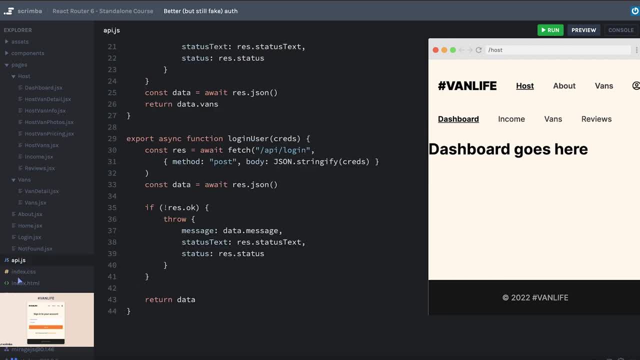 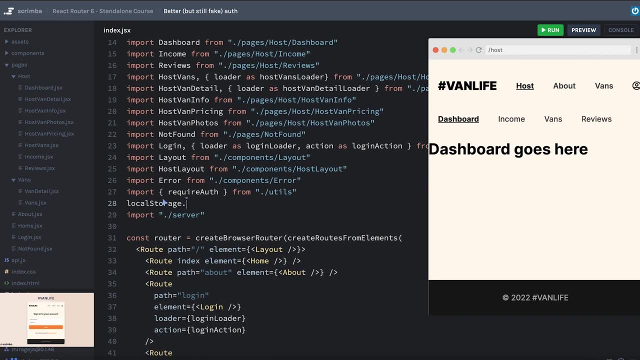 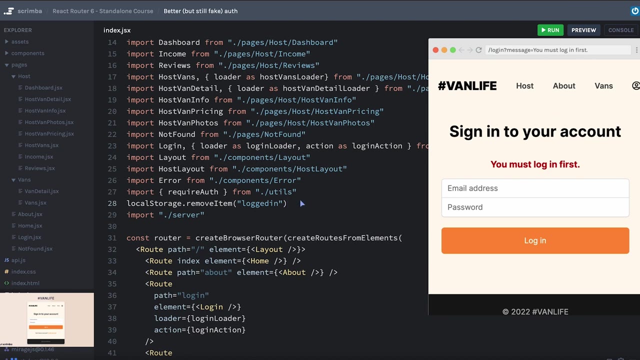 will be able to do that. So let's open up a local storage, And I think it's going to be a great way to clear out my local storage. So maybe what I'll do is just go to my file here in the index And I'll just type in: local storage, dot remove. item logged in: run this. 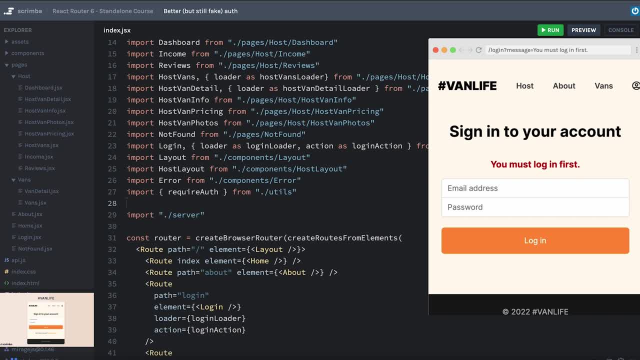 code. Okay, cool. Well, it looks like it sent us to the login page, So I think that worked. Then I'll clear that what we should probably do is put just a simple button- that will be temporary- that allows us to clear out that local storage. 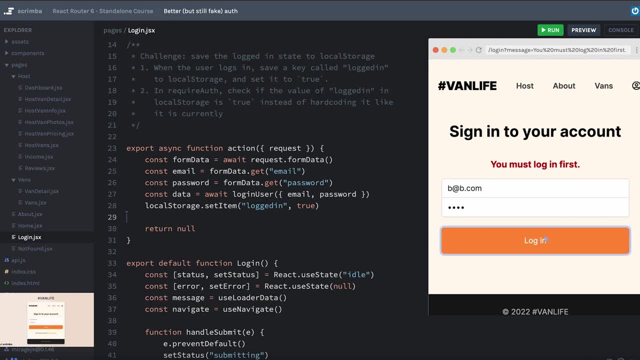 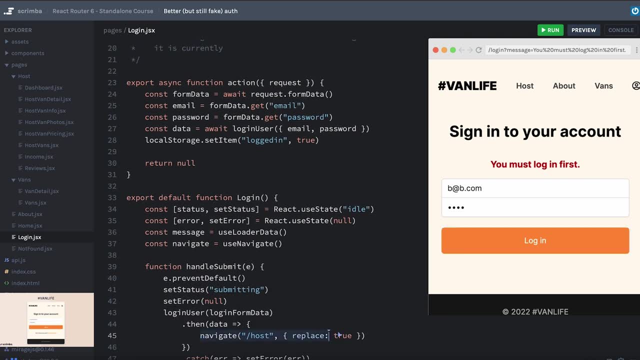 type in b at bcom and p 123, login and we are presented with what our next challenge needs to be, Because before we were redirected to the new page with this navigate function inside of our handle submit, but we are no longer using our handle submit, So that is. 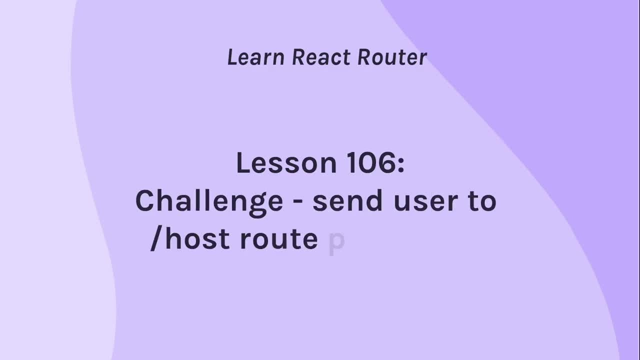 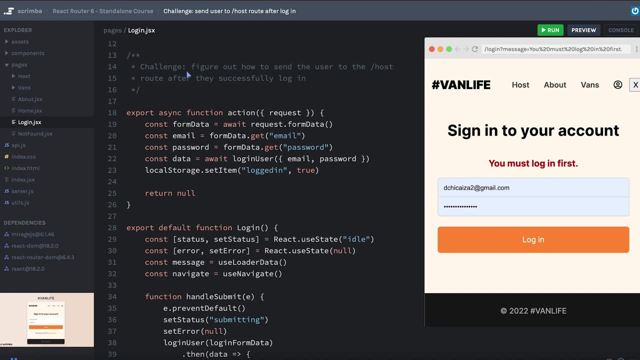 what we are going to be working on next. I was realizing that you should actually know everything you need to know in order to complete this challenge by yourself. As a reminder, the idea is, once somebody successfully logs in, they should be sent to the host route. Eventually, we're going to add to that to 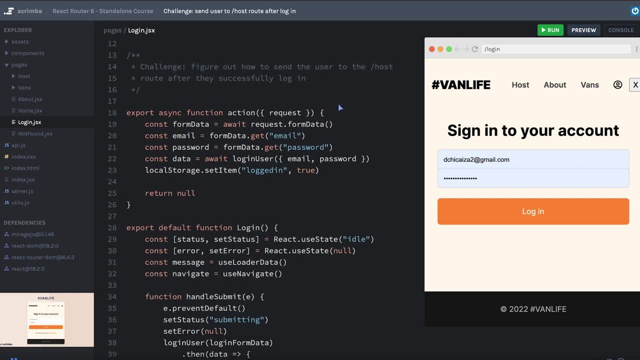 make it even even better user experience. But I wrote this a little bit vaguely so that you have to really critically think. you can go look at other parts of the app if that might be helpful. Just a quick hint: you're not going to be able to use the navigate function. 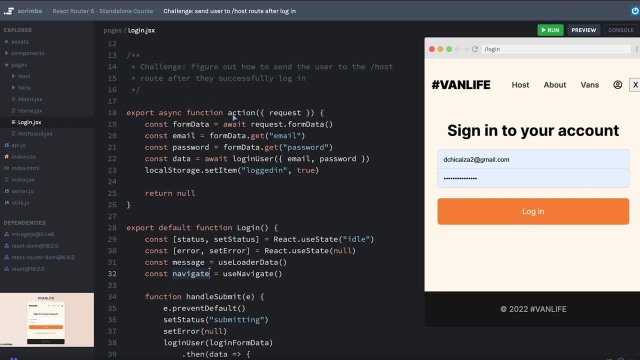 That's because we're going to be sending the user to this new route inside of our action function And the navigate only comes from calling the use navigate hook, which can only be called inside of a functional component, And our action function up here is not a component at all. 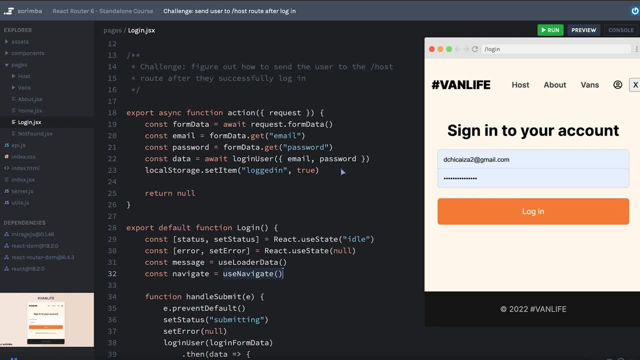 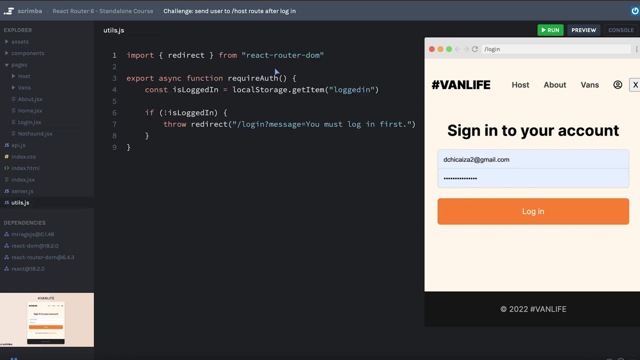 So that's enough of a hint. pause now and work on this challenge. The tool that we need is the redirect function, So I'm going to pull that in. you might remember that from our require auth function, where we are redirecting people to another route, And in this case we're including a 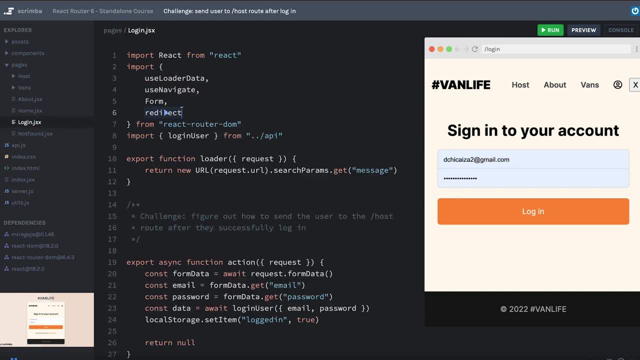 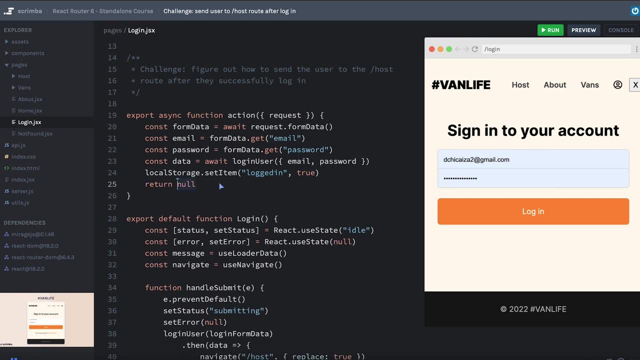 message on top of it. So back in loginjs, we will pull in our redirect And then right here we will call- and actually I'm just going to return a call to redirect. So we'll do redirect And for now we're going to hard code in the slash host route. we'll clean. 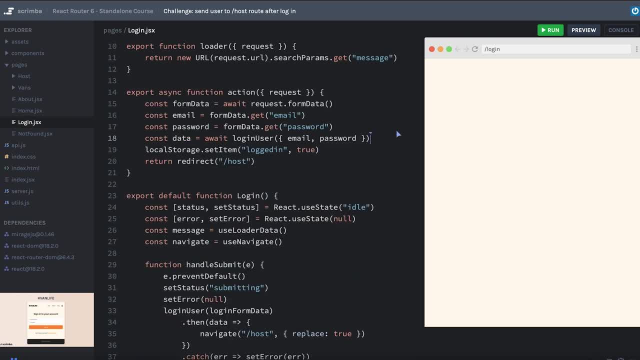 up this challenge text and cross our fingers, We'll hit save. log in bicom p 123, login and there we go Now, something I did just to make our lives a little bit easier is I included this little, admittedly very ugly button here in our header that we can click in order to clear out. 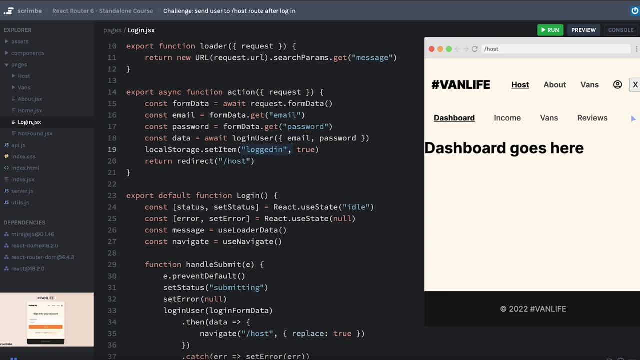 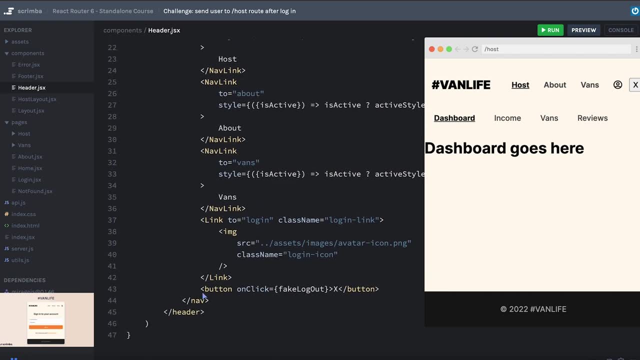 local storage, or at least to clear out this logged in value of local storage. You can see it over here on components header if you want. There's the fake logout function and just a simple button with absolutely no styling that, when it's clicked, calls fake logout. Now you'll notice that. 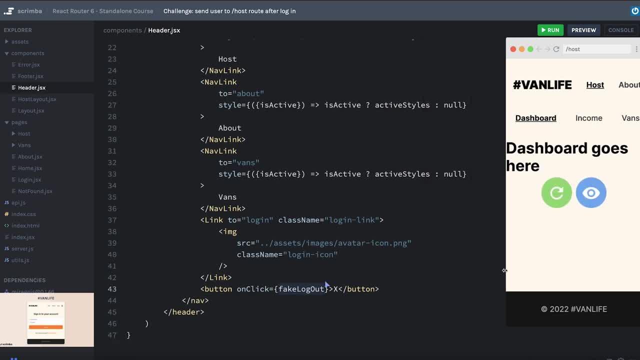 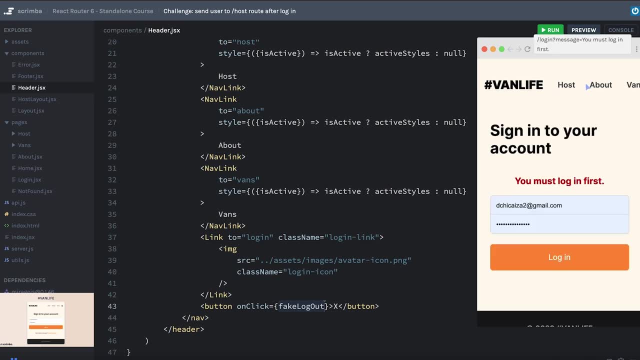 clicking logout doesn't actually change the user interface And that's because react is not observing local storage to make updates to the UI if that happens. But now, if I click host, it should redirect me to the login page because it knows that I'm no longer logged in. 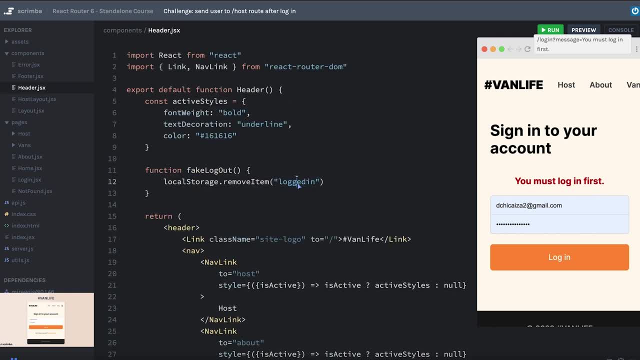 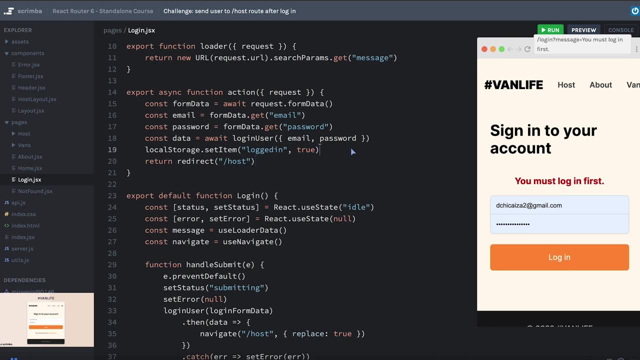 or rather that there's no more local storage entry for logged in. Okay, hopefully that went okay for you. Now, with this redirect included in our action, we have a little bit of a funky user experience. that happens, So let me show you. I go to the home. 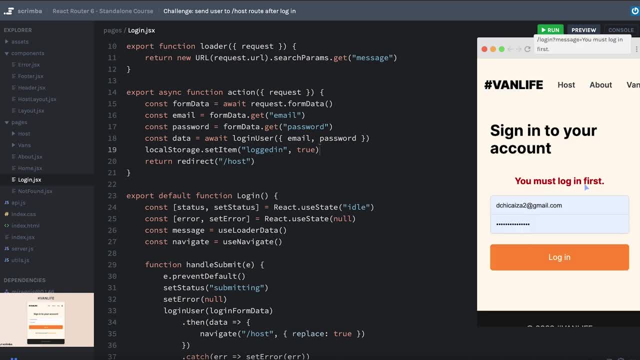 page. I'll try to go to the host page. it'll take me immediately to the login page. I'll go ahead and log in bbcom p 123 login And then if I, as the user, were to hit the back button, I'm sent to. 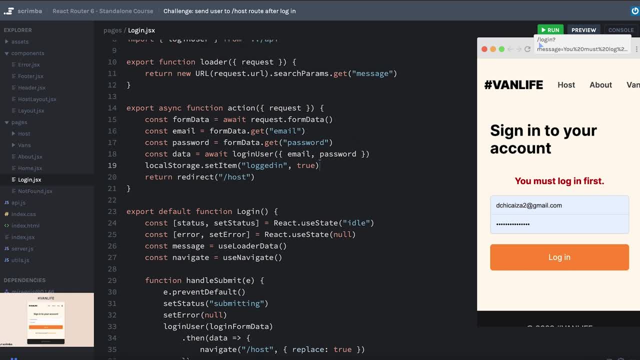 the login page And maybe, what's worse, because we have the query string that has the message that you must log in first in the URL. it means that this page that we're seeing makes it look like we're maybe no longer logged in, Although I can get to the host route because technically, 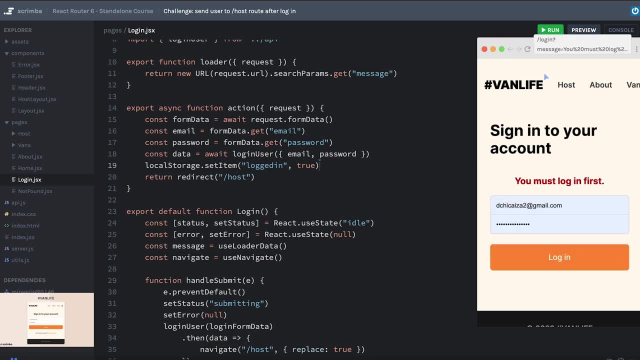 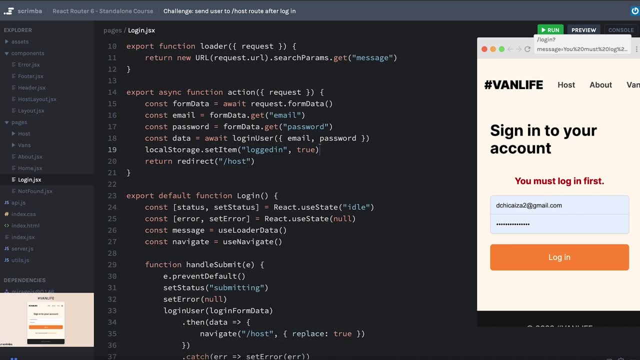 according to local storage. I'm logged in, So this is kind of a funky experience. Ideally, we wouldn't be able to see our little detour to the login page at all, And fortunately, in order to do that, it is very, very easy. We'll talk for just a second about the history stack in. 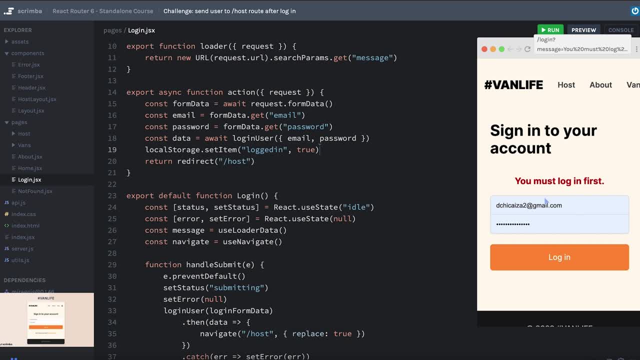 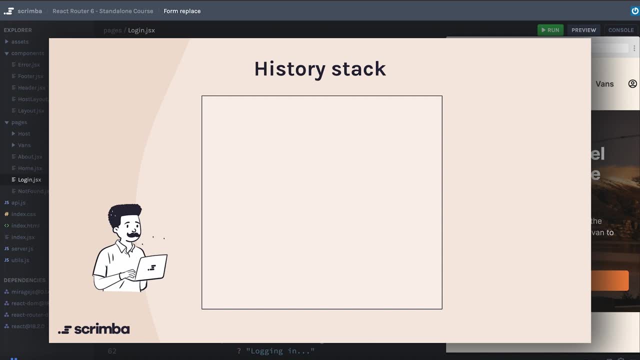 the next lesson and then see how we can essentially avoid having the back button take us back to this login page. As I mentioned, making this little user experience improvement is actually a really easy thing to do in the code in the way that we have our code set up, But I think it's. 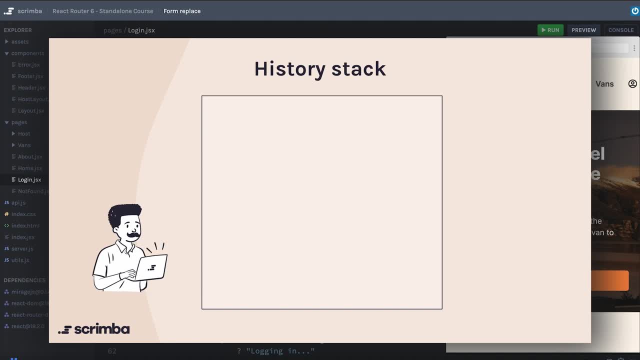 useful to understand the concept of the history stack, just in case you don't have any previous experience with it. The idea behind the history stack is that your browser maintains a. you could think of it as an array of locations that your browser has visited And, under the hood, when you 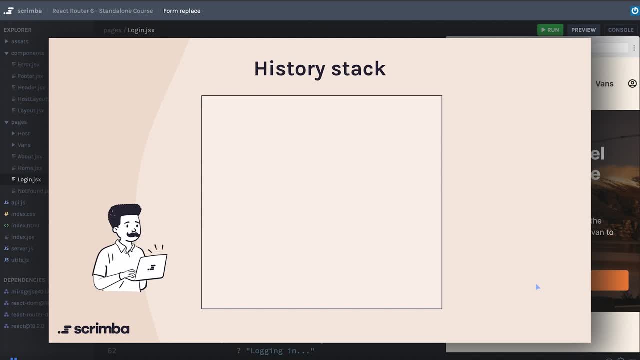 transition from one route to another. in react router, it is automatically pushing new entries to the history stack for you so that you are able to use your browsers back and forth. So if you're using the back and forward button, the way that you would expect a regular app to work- So for 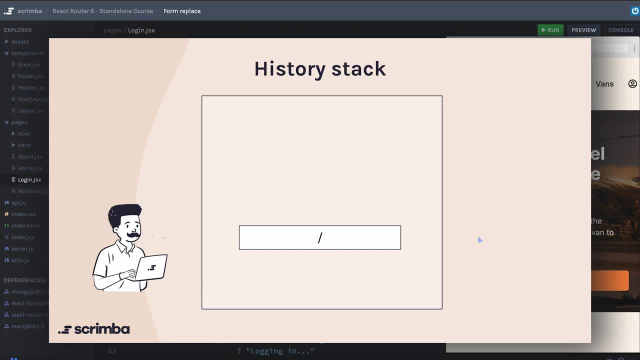 example, if you show up at the homepage you would enter in the slash route to your history stack. then maybe you visit the About page, So that would enter in the About page to your history stack. If you hit the back button it would pop that off the stack and you would be back at the homepage. 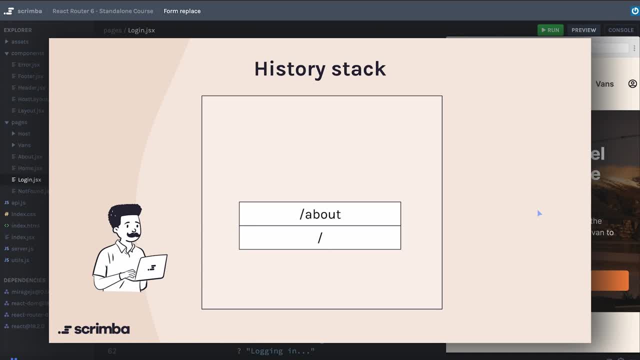 hitting forward again would take you to the slash About page. This is all exactly how you would expect. Now, let's say our user is not currently logged in and they try to get to the host page. What exactly happens Before the host page can load? the require off utility function that we set up stops the route. 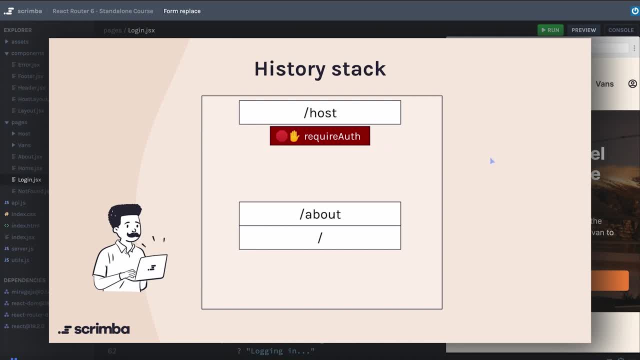 transition from happening, And that's because we set require off to run inside of the loader for this host route And the loader will always run before the transition to the host route happens. inside of require off. we redirect the user to the login page, and so the login page is what actually 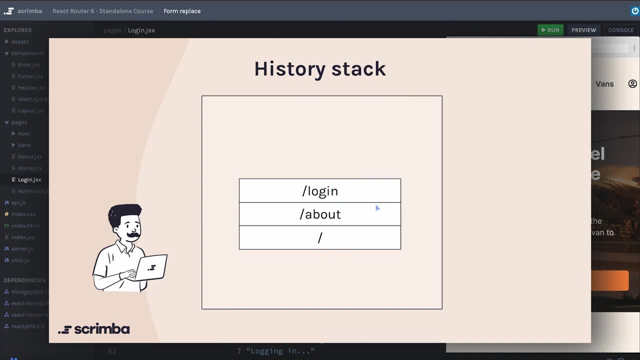 gets entered into the history stack, So that's a good thing for us. However, once the user logs in, we are routing them to the host page, and the host page and the login page are both in our history stack. This means that if the user hits the back button, they will end up on the login page. 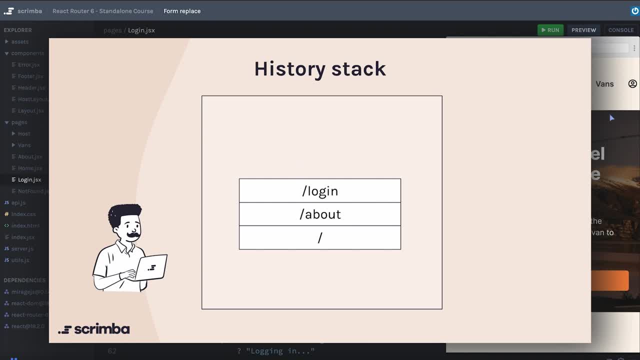 despite already being logged in. Now we could change our setup so that if the user ever gets to the login page, it will check their logged in status. To be totally honest, this is probably the best solution, because then it doesn't matter how you get to the login page. 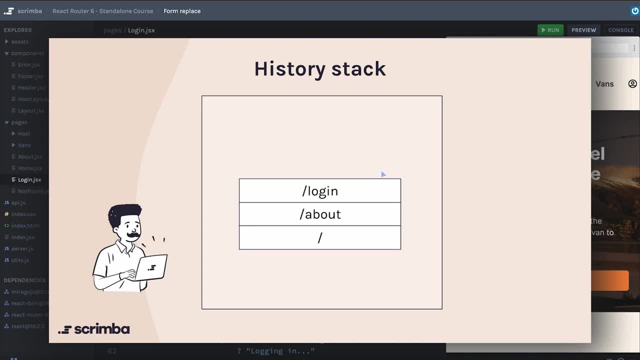 If the user were to type slash login, then it would automatically redirect them somewhere else, So that's definitely something you could play with For the sake of simplicity. we are going to take a little bit of a different approach And while we're at it, we'll learn a cool new tool that we can use. 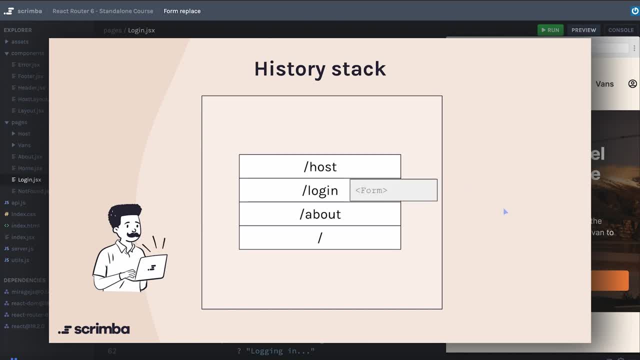 So on our login page we have our form, which is our login form. we can add a very simple prop to that form, called replace. One thing that takes a little bit of time to get used to is recognizing that the submission of a form is actually considered a navigation event. 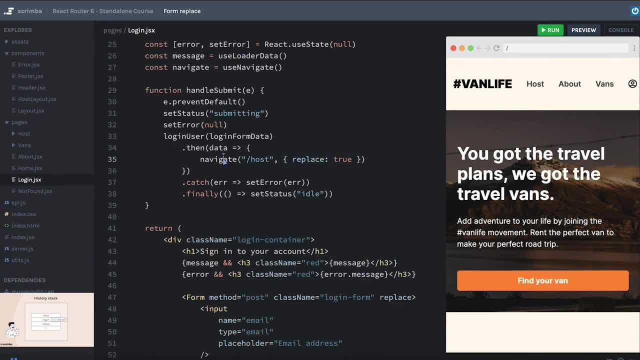 And so similar to how we had this little option that we have on our navigate function that says replace true. This replace true says: forget the current route that you're on. just replace the current route, which is the slash login route, since this is the login component. replace it with. 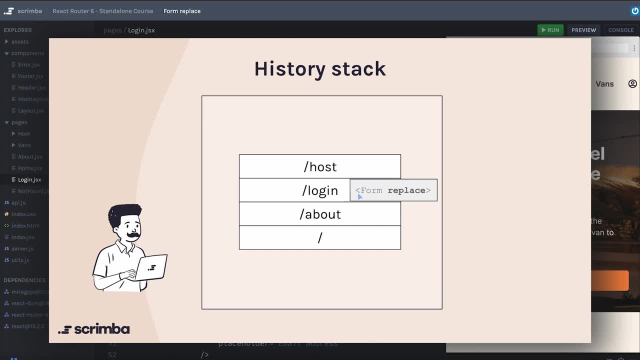 slash host. Well, the exact same thing is going to happen with our form. because the submission of the form is also considered a navigation event, we can instruct it to replace the current entry in the history stack with the upcoming entry in the history stack. 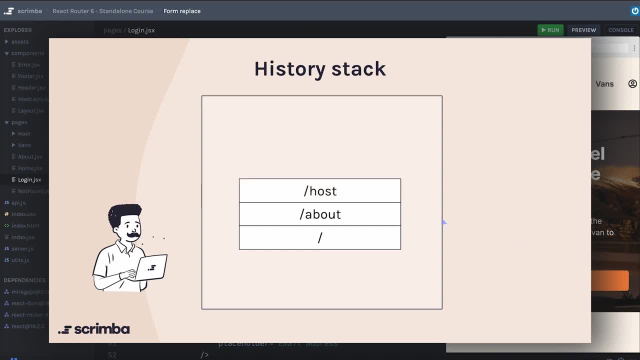 And so what happens is the login essentially gets removed from the history stack, and we have sort of an amended history here that allows the user who now is logged in and is at the host page to click the back button and go back to the about page. as if the little 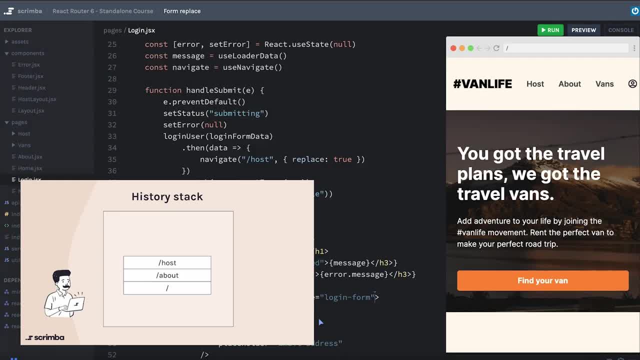 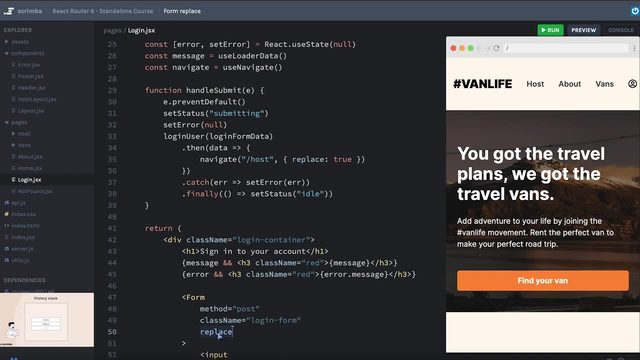 detour to the login page never happened, So this is as simple as adding the replace prop to our form. we put these on their own lines And by adding the replace prop here when we submit our login form, we will see that exactly what we saw in the diagram will happen. 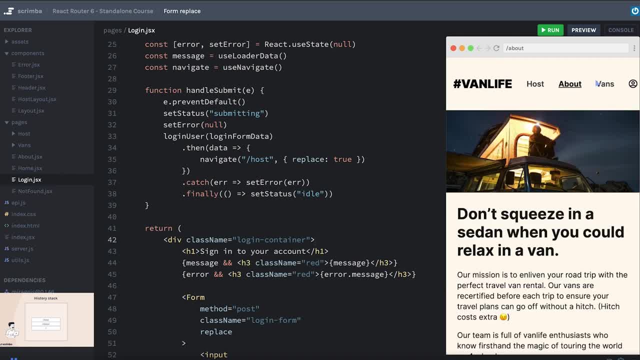 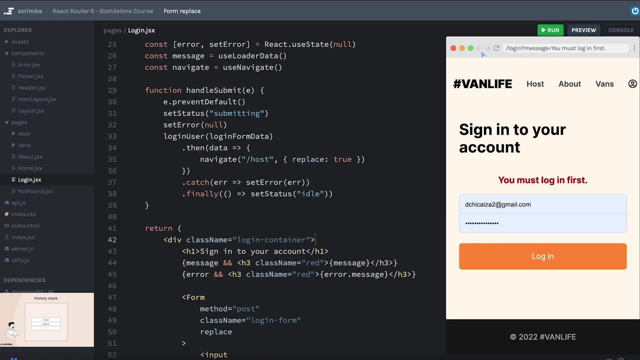 So I'll go ahead and hit refresh. I'm at the homepage. maybe I'll go to the about page. I'll make sure I'm logged out here and then I'll go to the host route. This redirects me to the login page. 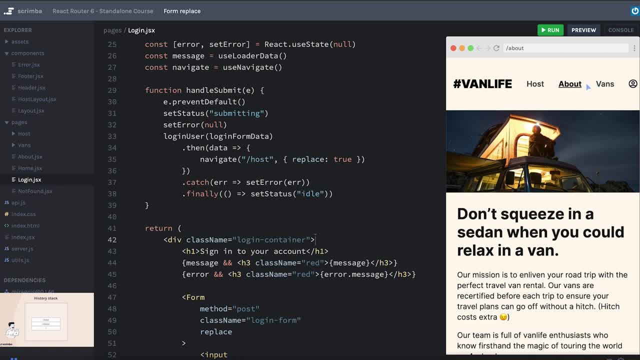 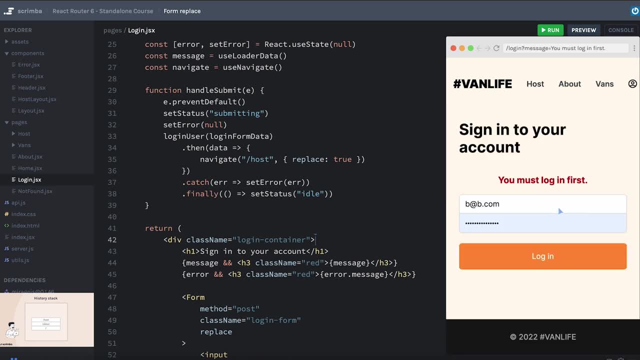 Notice that if I hit back here, I go to the about page. I don't go to host. it didn't complete the transition to host So that never got entered in my history stack, And then I will go ahead and successfully log in. 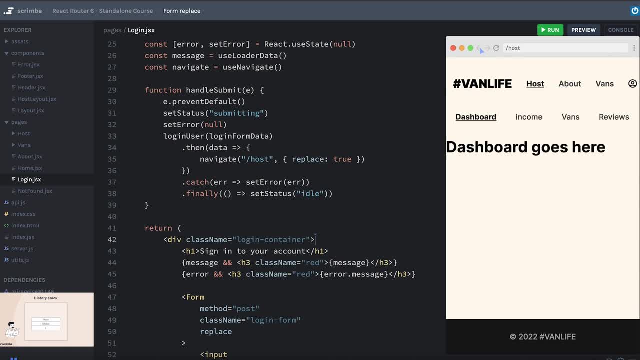 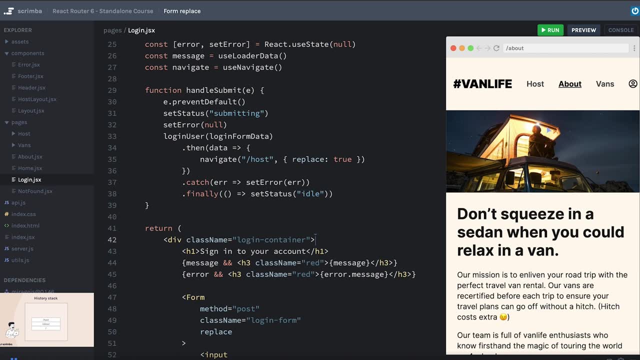 Okay, we're at the host route. And now, if I hit the back button, it takes me directly to the about page, which is just what we saw in this diagram. It's where I was before I ever made that detour to the login page. 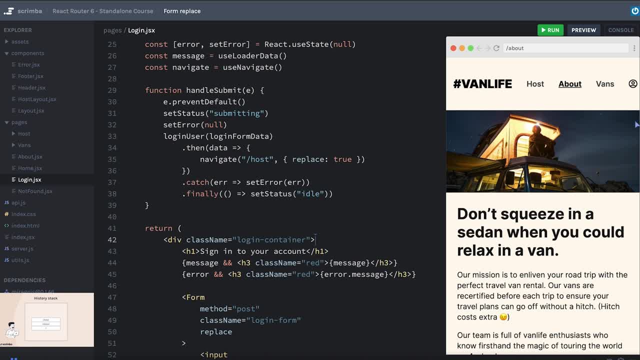 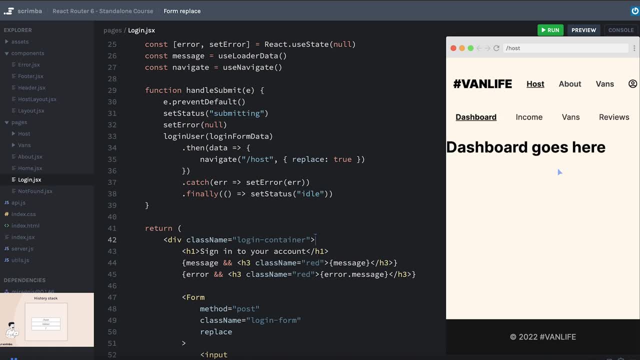 The same thing should happen if I were to clear out my logged in. entry will go directly to the login page, not via the host route. I'll enter my credentials again. login takes me to the host page. if I hit back, we're back at the about page, just like before again. 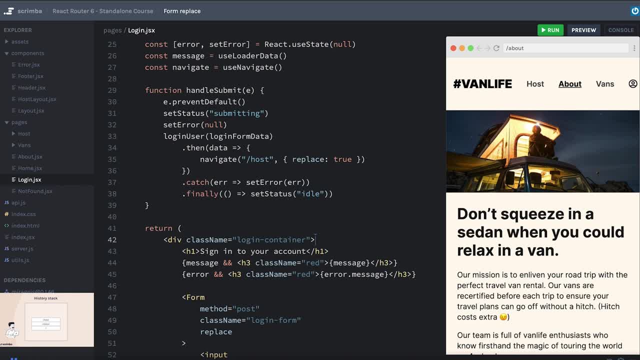 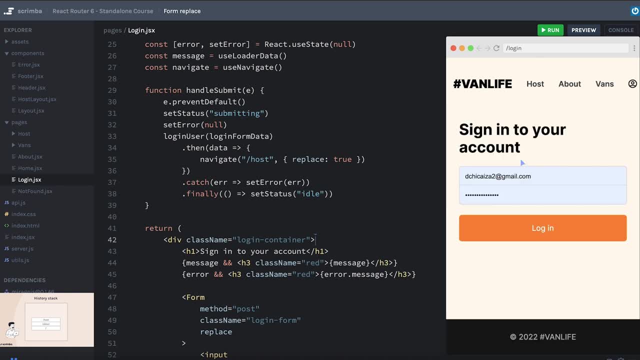 a more robust solution would be to first of all not render a login link at all if the user is currently logged in, or another solution could be to just make it so that the loader is currently logged in and redirect them somewhere meaningful if they already are. 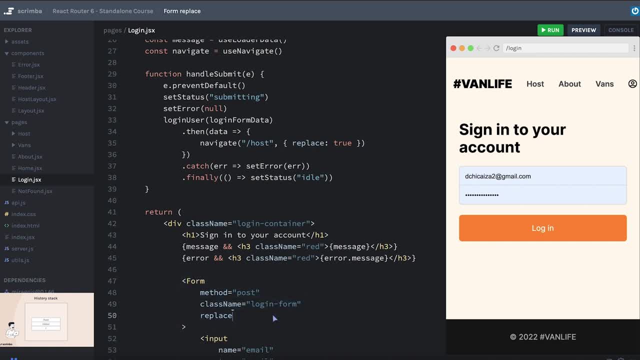 But at least now we've learned the concept of a form submission being considered a navigation event And this cool new prop that we can add to our forms if we ever want to ensure that the history stack doesn't include the route where we're currently rendering this form. 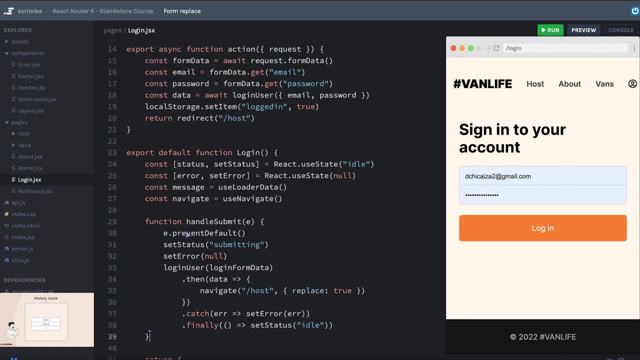 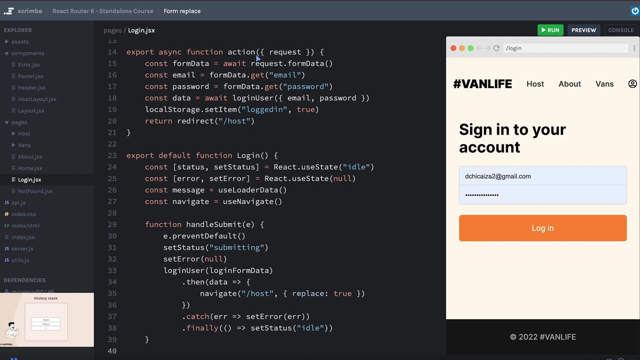 Okay, we have been working on our happy path, transitioning it from using our more imperative form submission methods like our handle submit function. Here we've got an action function that's working fairly well. let's go ahead and start coding up the sad path, using our action function and moving a few things out of our component. 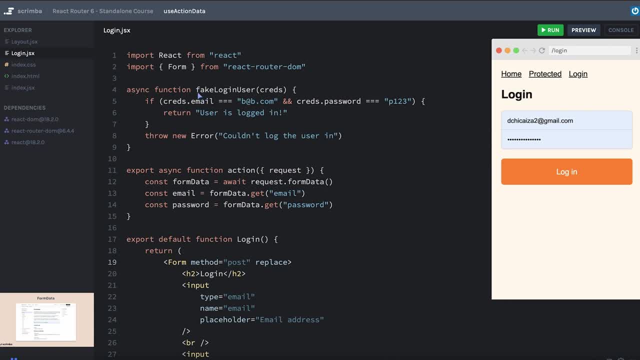 We're back here at our simplified app And I've created this fake login user function. All it really does is it takes an object with an email and a password property. It's just hard coding to check if those are equal to b at bcom. 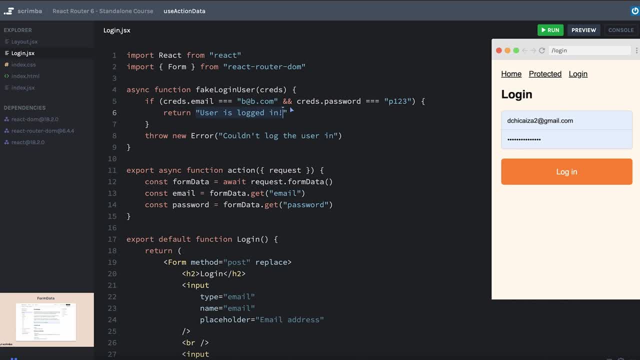 And P 123. And if that matches, then it returns something. we're not actually going to be making use of this right now. I just wanted to have something there. If, on the other hand, it is unable to log the user in, then it's going to throw an error. 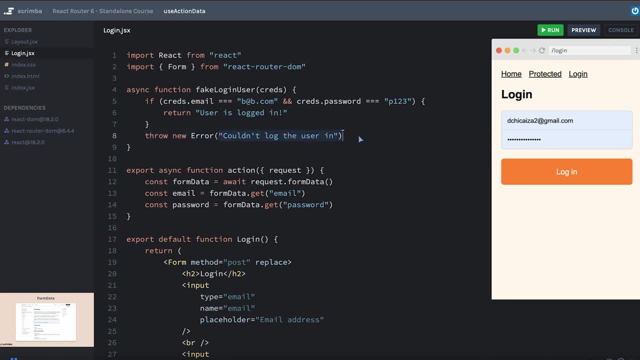 with a message of couldn't log the user in. we want to start handling some errors where, if the information that's passed in the email and password is incorrect, we want to be able to display to the user that something is wrong. Before we started working with the action function, we had to maintain all of our errors. 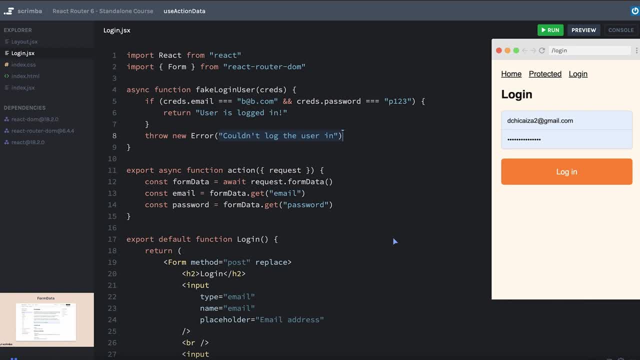 in the state as react state inside of our login component. However, now we're going to have access to a little bit of a better way Now. first of all, it's important to know that if I'm in my action function and I throw, 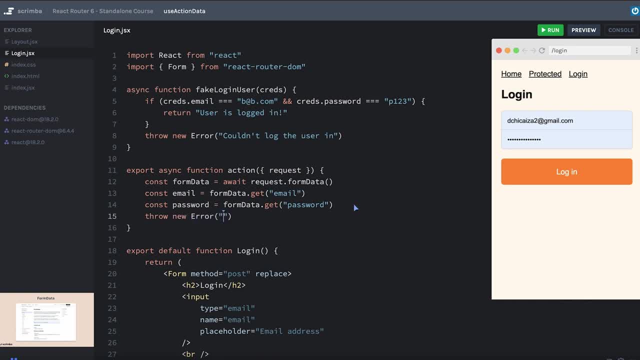 some kind of error. let's go ahead and say we're throwing a new error. There was an error, Gabe. that's just hard coded into the action which will happen when I hit login. Let's see what happens. I'm going to hit login and we get an unhandled thrown error. this screen that you might remember. 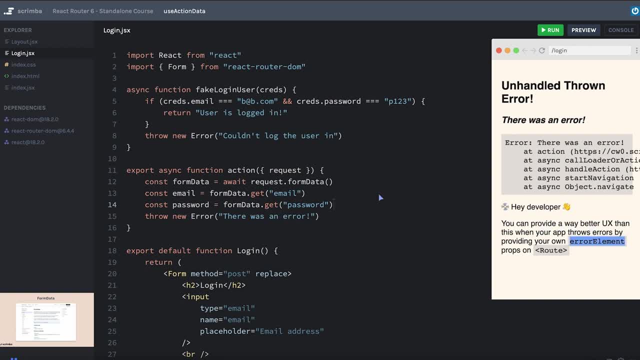 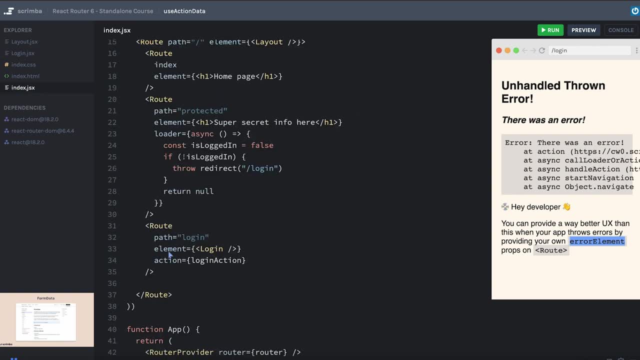 seeing before word instructs us to use This is an error element. When an error is thrown inside of our action or our component or our loader. it's going to then exit out of the regular element flow of our route definitions And it's going to look for the nearest error element. 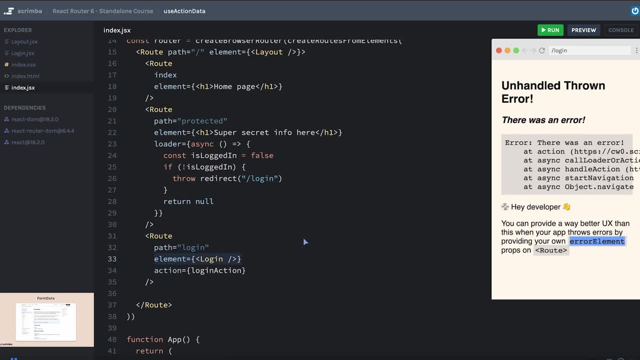 Now. we don't have an error element anywhere on here And we've already learned about that. So if you need a refresher, you can go back to the previous part in the course where we talk about the error elements. But that's not actually what we're concerned with right now. what we're concerned with 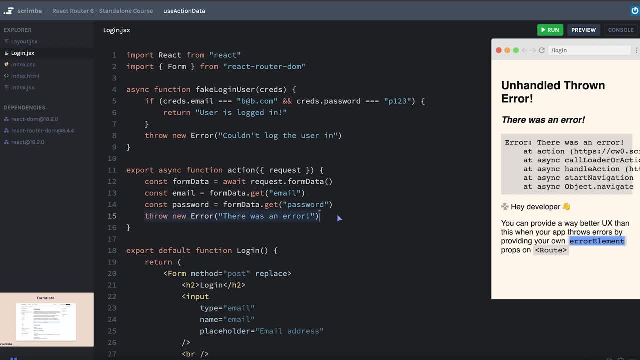 is not throwing an error, Because we don't want to take the user away from the login form just because they got the information wrong. Instead, we want to keep them here on the login page and simply display some information that might help them understand that their attempt to login was not successful. 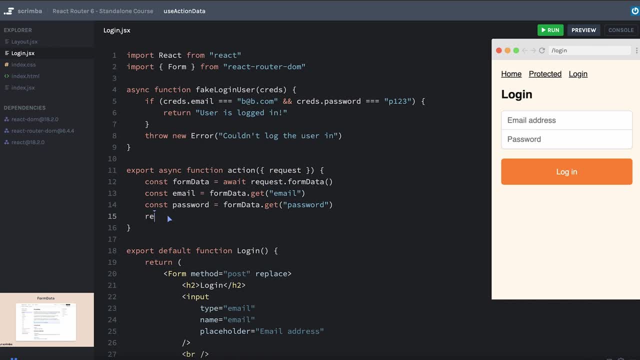 So in our action, if, instead of throwing an error, we return something, let me go ahead and just hard code a string that says I don't know, couldn't log in. this gives us a chance in our component, So we're going to do that. 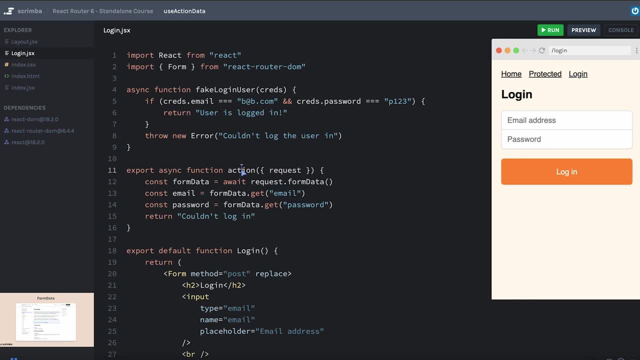 And we're going to use the action function And we're going to use the action function to receive the data that we're returning from our action function and display a helpful message here in the actual component, In order to grab data that has been returned from an action function very similar to how. 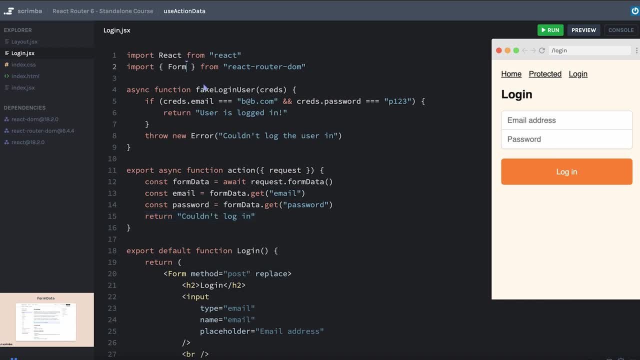 we did in a loader function, we can use a hook called use action data. Remember, when we return something from a loader, we can use use loader data. the naming convention is very similar for an action, So we will use this use action data hook inside of our component. 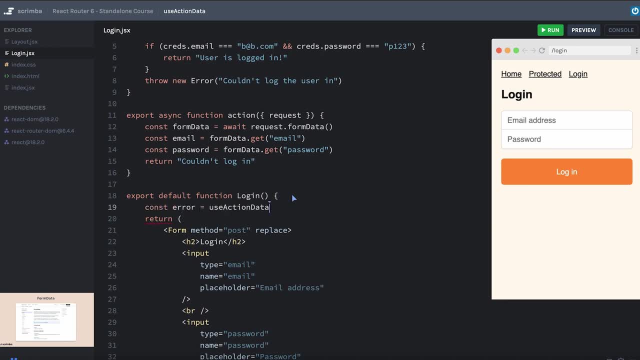 And let's go ahead and just call it error, because we know that's exactly what it is And we'll get it by calling use action data. Now think for a second when I refresh this page, what is going to be the value of this? 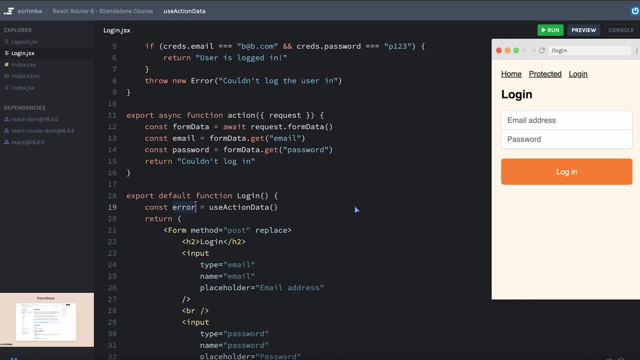 error variable. Remember, the action function will only run after the form has been submitted, And so when we first render this component, we're not automatically submitting the form, And so we can see when we console log this error. Okay, We're going to get an undefined value. 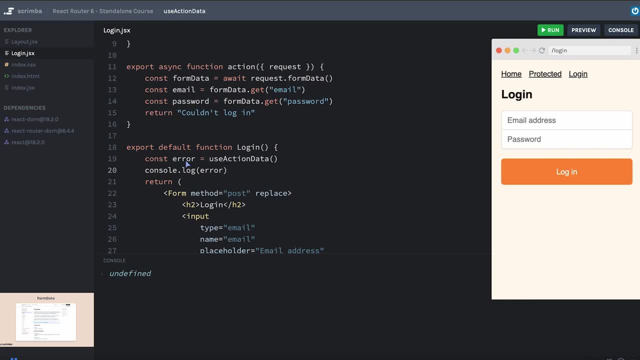 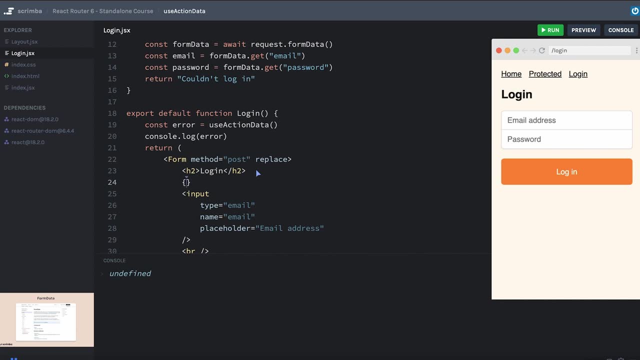 So that just means that when we are trying to display this error, we need to make sure that we are coding a little bit defensively, which means using our good, trusty friend of conditional rendering. I'll go ahead and say: if there is an error, then we'll display. maybe. 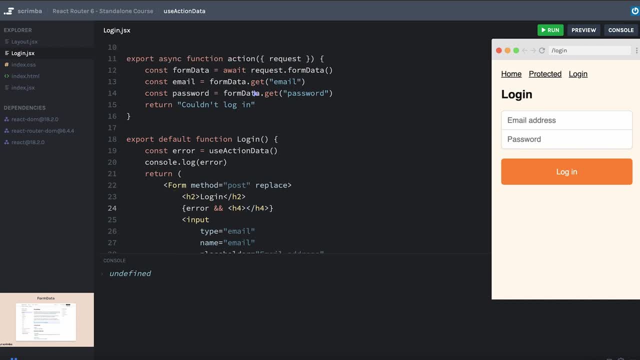 just a little h4.. And because the error, so to speak, that we're returning from our action is just a string, I'm just going to go ahead and display that error right here. We do have a little class, Yes, that we created earlier, called red. that will make this stand out a little bit more. 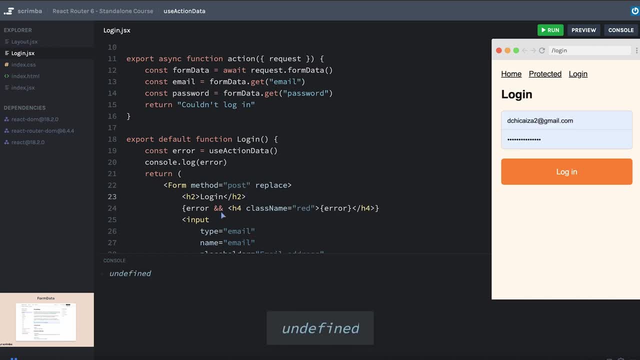 So let's go ahead and hit save. we still have undefined, But because we're now checking if error exists first, before displaying our h4, we don't have any problems And then I'll click login and perfect. we get the string that we returned from our action. 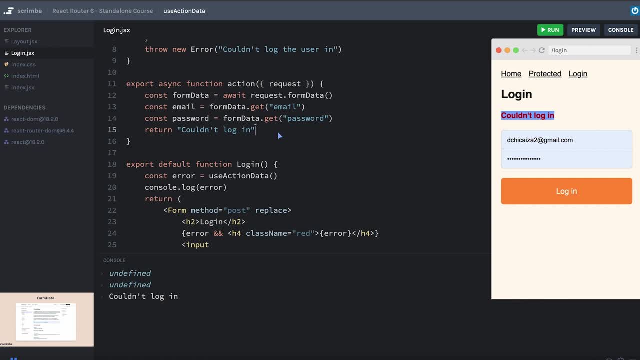 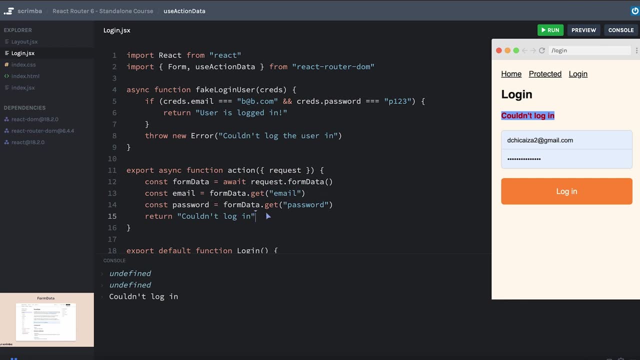 function Great. Now that brings us to the next step, which will be to check for any errors inside of our action function, so that we can redirect, like we were doing before If things go well, or return some helpful information back to the form so that the user 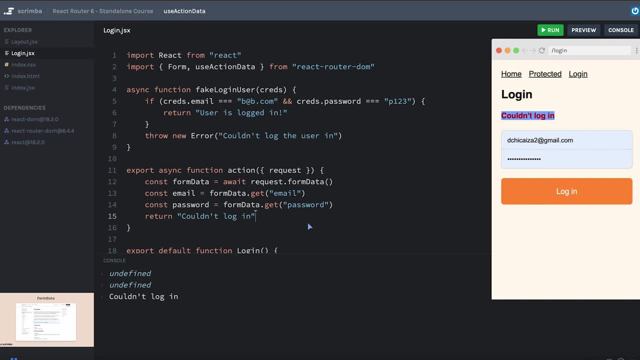 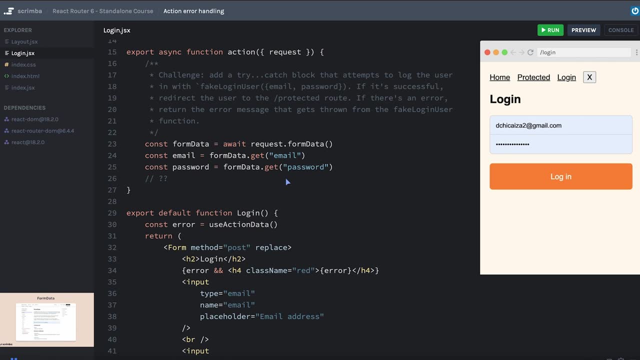 can take action accordingly. So that's what we'll be doing next. Okay, let's apply what we just learned about returning values from our action function in this challenge, where I need you to add a try catch block that tries to log the user in with our fake login user and we pass the email and password to it. 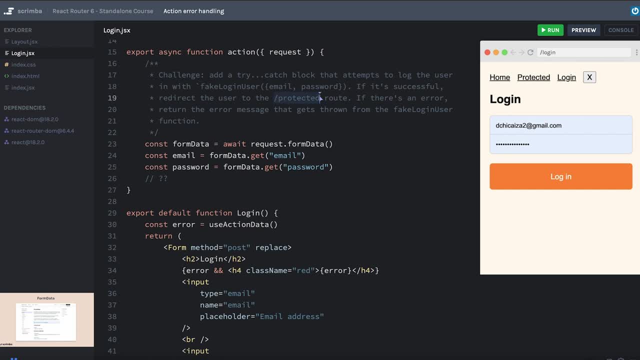 If it's successful, then you can redirect the user to the slash potential, And that's what we'll be doing next. Okay, let's apply what we just learned about returning values from our action function in this challenge, where we can redirect the user to the slash protected route. 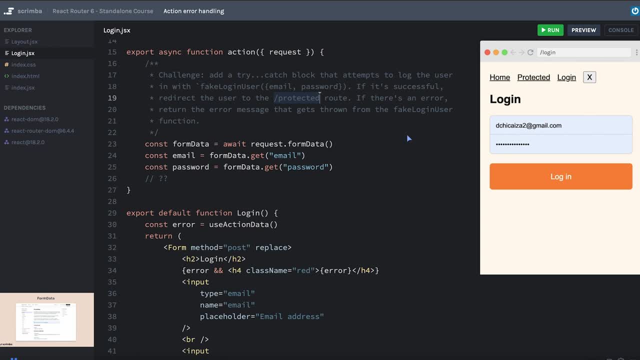 But if there's an error, you can return the error message that gets thrown from the fake login user function. I put this down here because this is where you can start your coding. you can just put this above the try catch and start your try catch right here. 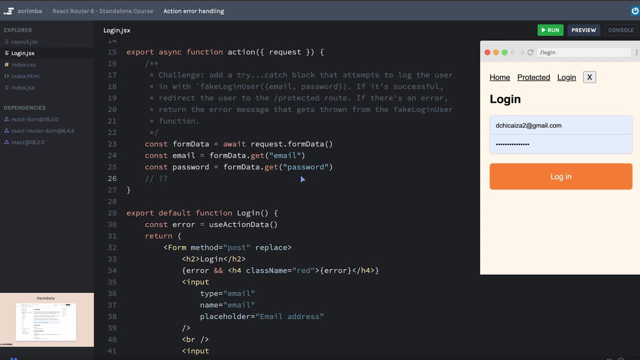 Okay, pause now and work on this challenge. Alright, so let's open up a try catch. One thing that I kind of like about try catch is that I can put all of the code for about 15 minutes- my happy path inside of my try and then just catch any errors that might occur along the way. 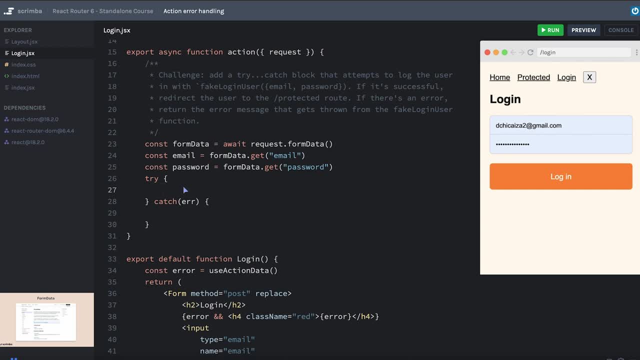 this works for a simple task like this. if it becomes more complex, you may need to either nest a try catch or do multiple try catches, but we're not going to worry about that here. so, first thing, we need to try to log the user in. so we're going to call fake login user and we will 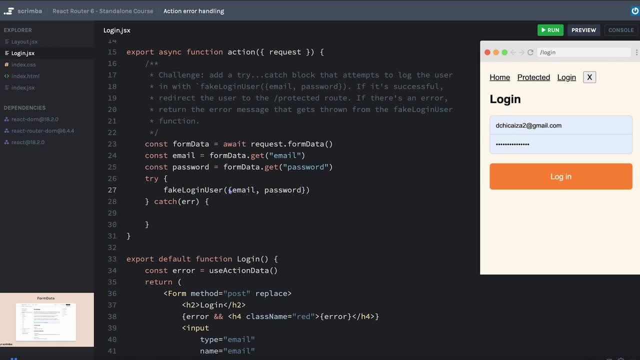 pass the email and the password and i'm wrapping those together in an object because the fake login user expects an object to come in with an email property and a password property and i believe this is an asynchronous function, so we will need to await that. i mean, we can just come. 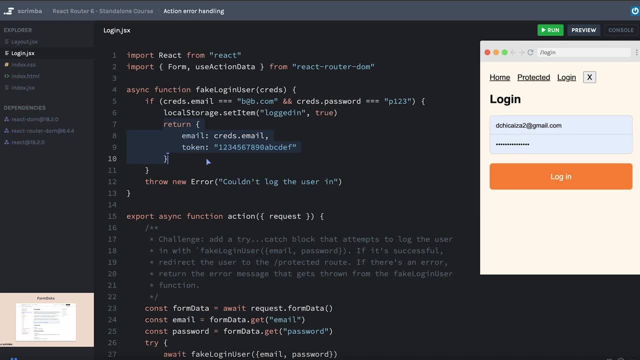 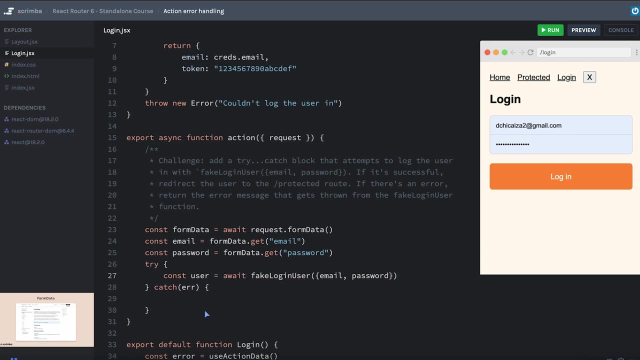 up here and look: so yeah, it's an async function and it's returning an object that has an email and a token. we're not really using that, but just for the sake of it, i'll go ahead and grab it in a variable, okay, and then, assuming that is successful, which we can do because we're here inside of our 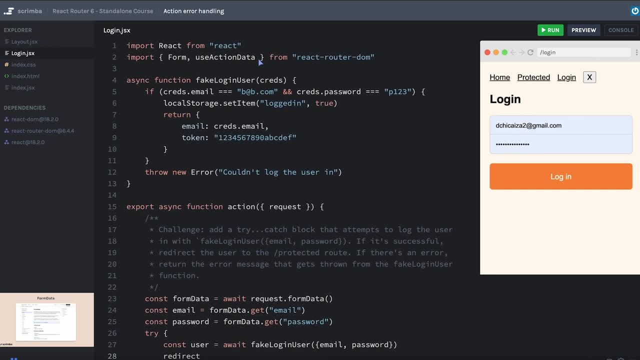 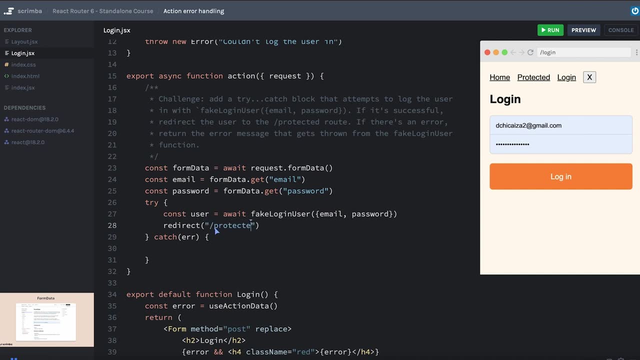 try. we can redirect the user which we need to import from react router, so we'll pull in redirect. we want to redirect them to the slash protected route and i don't think it's strictly necessary, but for some reason it feels better to me to return the redirect, so we'll go ahead and add that there. okay, now, inside of our sad path, if we do have, 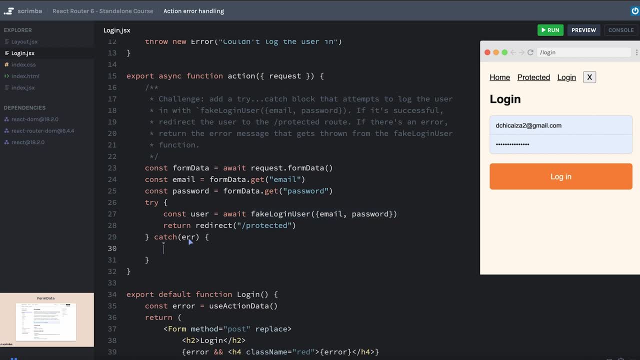 any errors in the process of trying to log the user in, then we're going to receive that error and we will just go ahead and return the message portion of that error. there's more than one way to do this. you could send the whole error object down in case you needed other properties from that error. but in our case 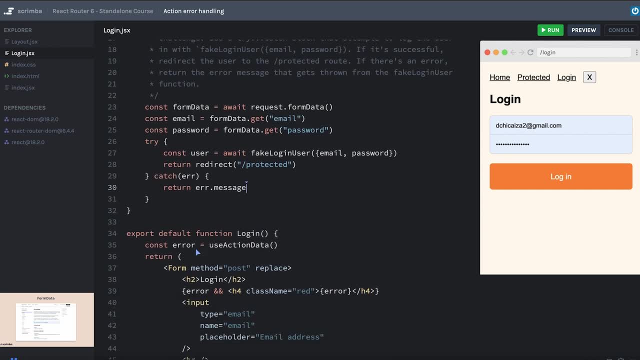 let's just go ahead and send the message down. maybe to make that absolutely clear inside of our component, instead of calling this error, let's go ahead and just call it error message. that way it's pretty clear that we are talking about the string message that comes from our action function. 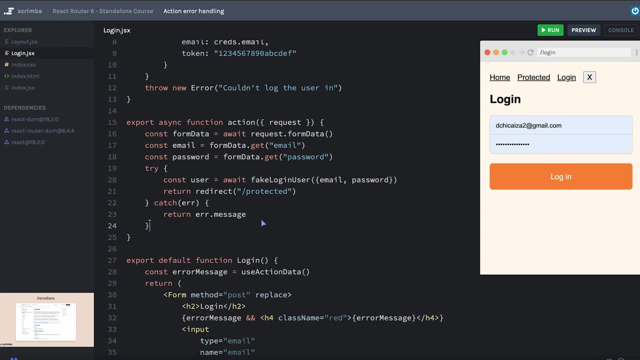 okay, let's clean up our challenge text and give this a shot. first, let's try to log in for real. we'll do b at bcom and p123. log in. here we are at our super secret information. okay, we'll click this to log out. try to go to. 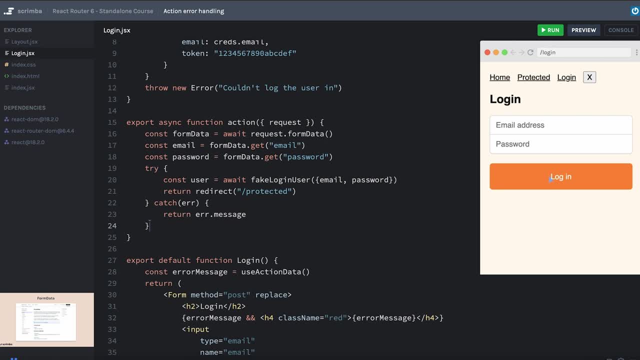 protected. that takes us to the login page, and then let's just try to log in without any credentials. couldn't log the user in? perfect. okay, with that little bit of practice under our belts, let's go back to the van life app and we will implement the same thing. 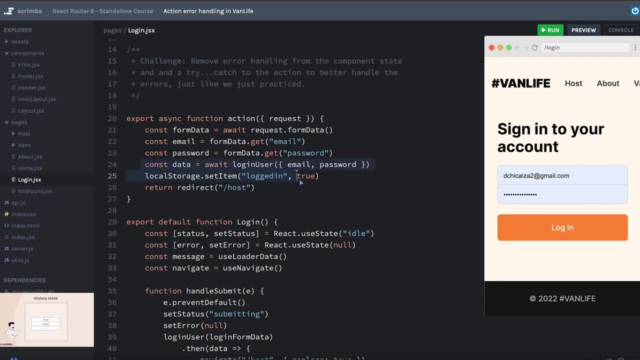 currently our action still only has the happy path here, and so we need to, as part of your challenge of the error handling that's currently happening inside of our component and the error component state, and create a try catch inside of our action so that our action can handle errors in a better 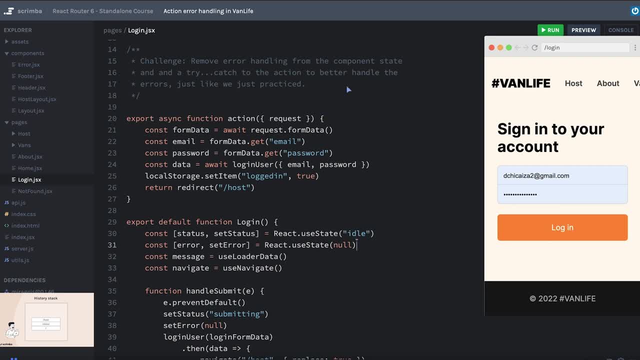 way, like we just practiced. now, if any of this seems like it might be a bit complicated for you, that's probably another good indication that it's time to go back, maybe re-watch a couple of the last lessons, as we have been practicing doing error handling inside of. 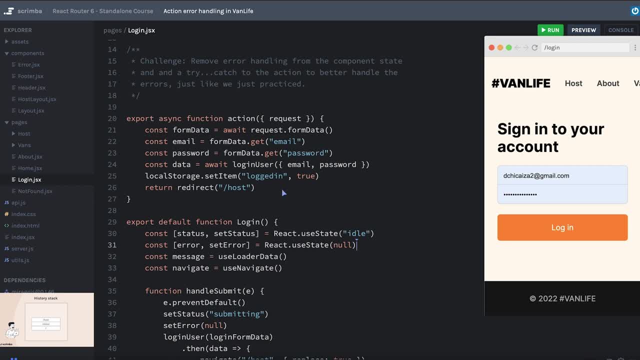 our action function because, as it stands, if you've been able to follow up until this point, then you should be able to complete this challenge without too much difficulty. so now is your time to prove to yourself that you can do it. pause now and work on the challenge, okay. so right here is where our 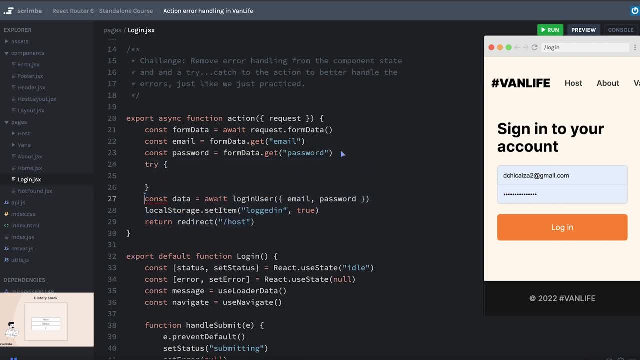 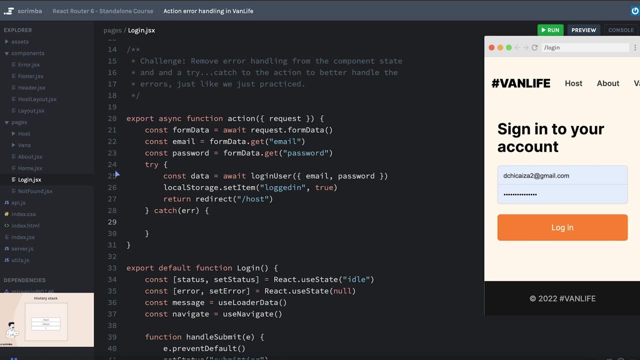 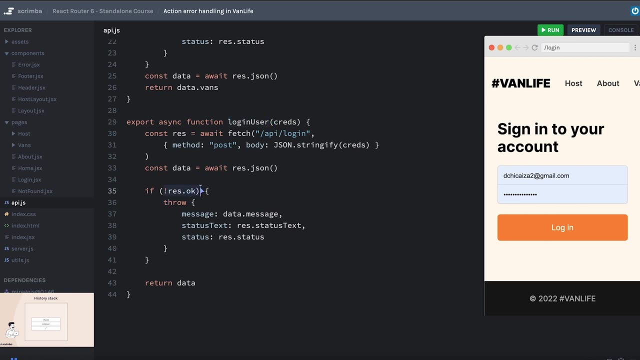 happy path exists. so i'm just going to wrap that code inside of my try catch, and right here we will include our catch of the error. we can actually see what this error object is going to look like if we ijs login user function. we can see that if something doesn't go okay, then it's going to just 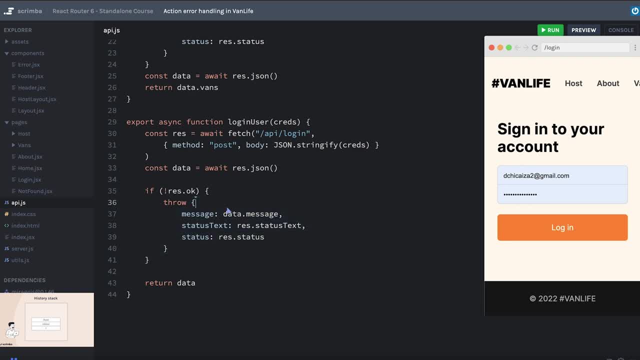 throw an object that has a message property. in case you weren't familiar, in javascript you can throw anything. you can throw a string or a boolean or, in this case, an object. you don't always have to throw an actual error object that's made by the error constructor. so i'm, in this case, throwing 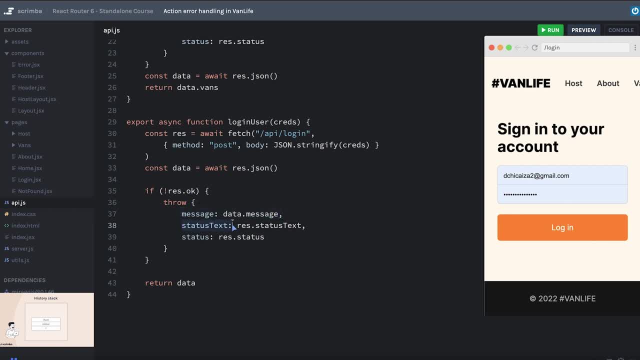 an object so that i can include a message property but also include the status text and the status, just in case that's useful. it's not terribly important at this point this time, but mostly it's important to know that we have this message that is going to come from. 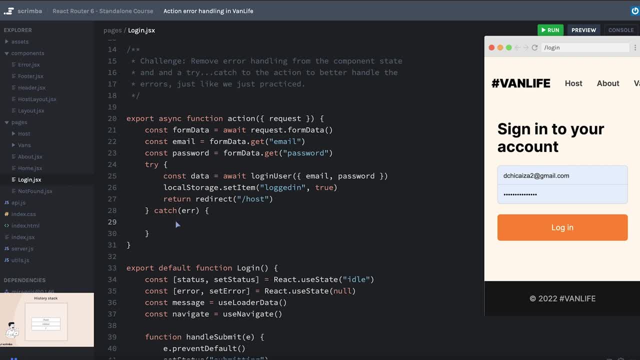 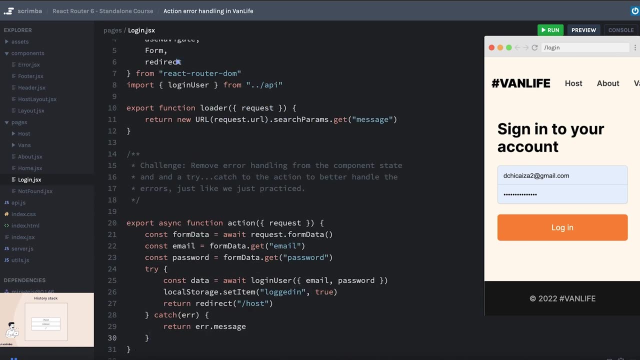 our server file. okay, so in loginjs we will just return and i think we can just stick to the message. i don't know that we necessarily need the status or the status text to display inside of our component, so we will just return the errormessage and then we need to use use action data, so i'll 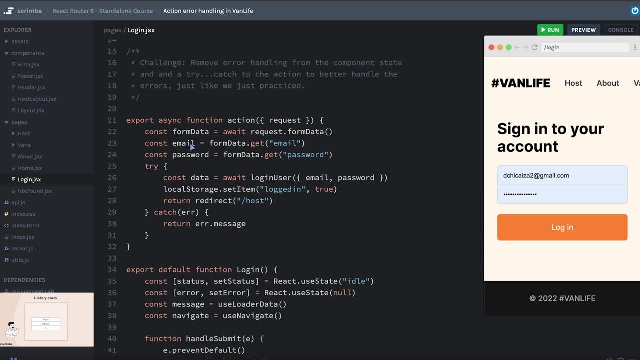 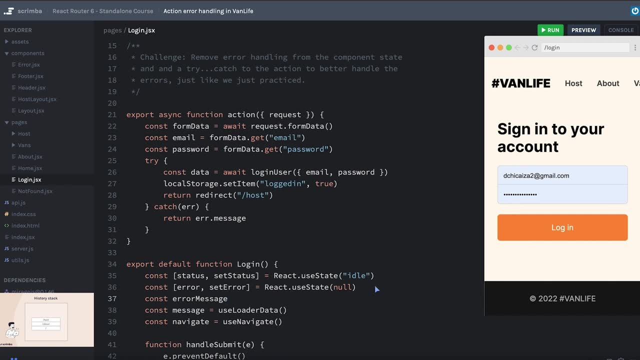 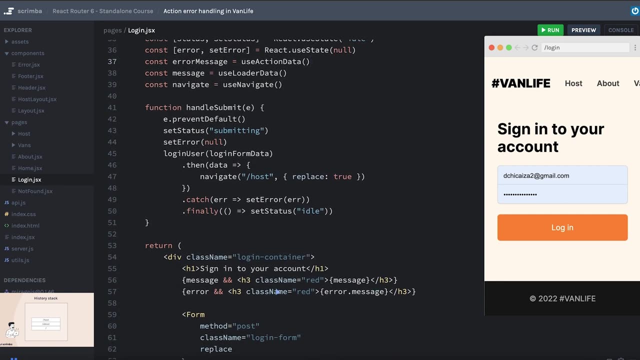 go ahead and pull that in use action data and inside of our component we can grab the error. maybe this time we'll also say error message, like we did in our practice, just to make it really clear that we're just pulling in a string message and we can get rid of or update this. so it's not 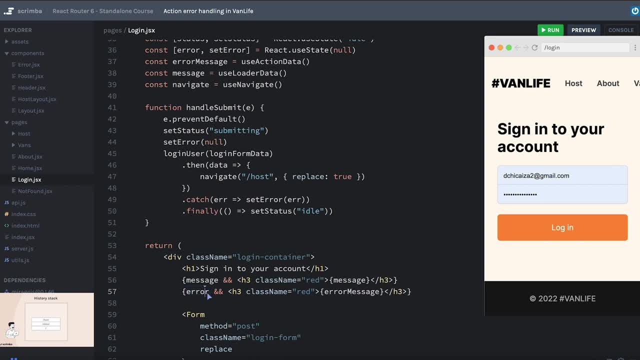 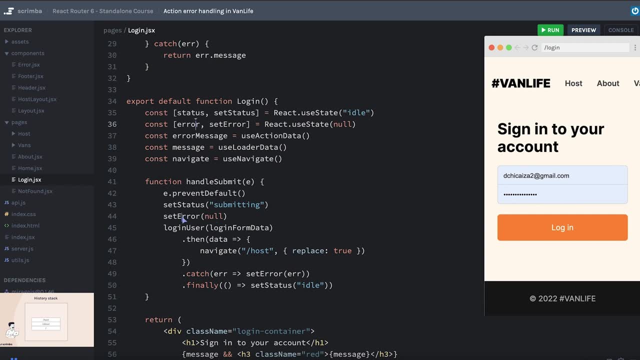 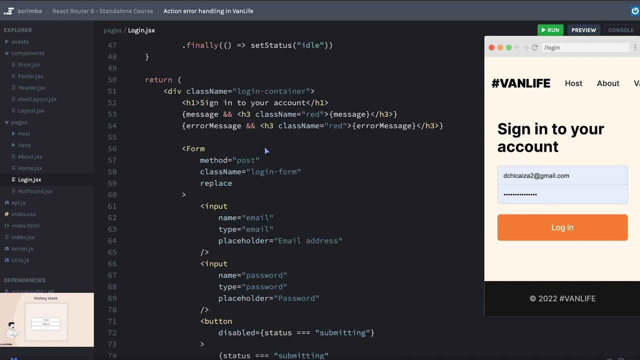 errormessage or error anymore. we'll say: if there is an error message, then we will display this h3 and we can start getting rid of any of the error handling that we had before. so we had some error stuff here inside of our catch. here we were dealing with errors. let's get rid of all that. 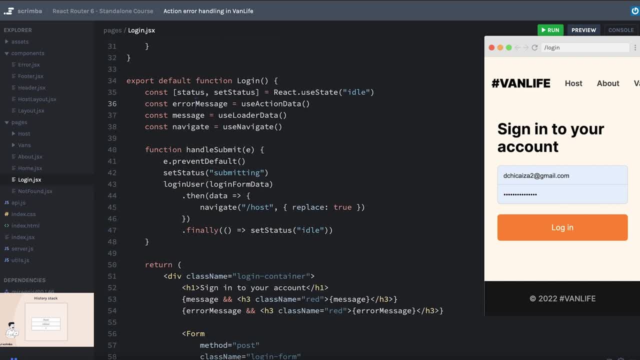 and i think that should be everything. we are right on the cusp of finally getting rid of our handle submit, but we have one last thing that we're not yet accounting for, and that is these statuses on the state of our app: if it's in the process of submitting or if it's idle. fortunately, we have 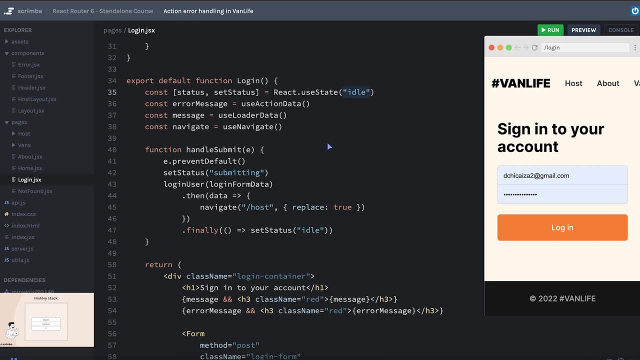 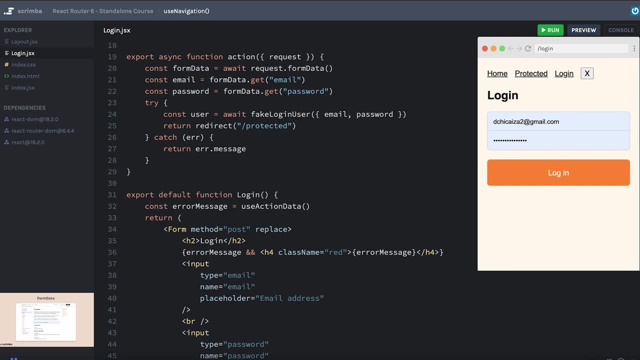 a pretty easy way to update this, and so that is what we're going to be learning and adding next here in our practice app. we don't yet have any code that gives us a good indication of the status of our app when we're in the middle of submitting our form. in our van life, what we're 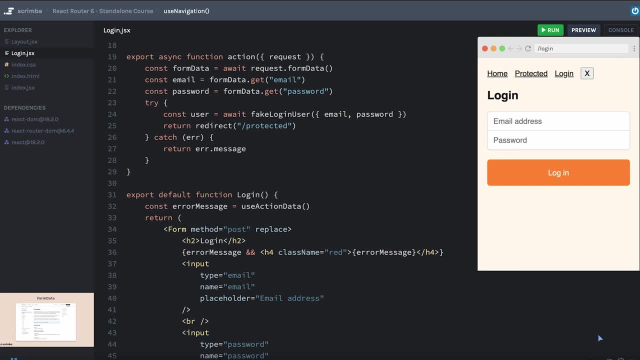 currently doing is setting up some local react state that has a status property and we're setting that status manually while we're in the process of submitting our form. however, because the form submission is now happening inside of our action, we can't update our local component state because the action is not part of our component. it doesn't have access to our state. 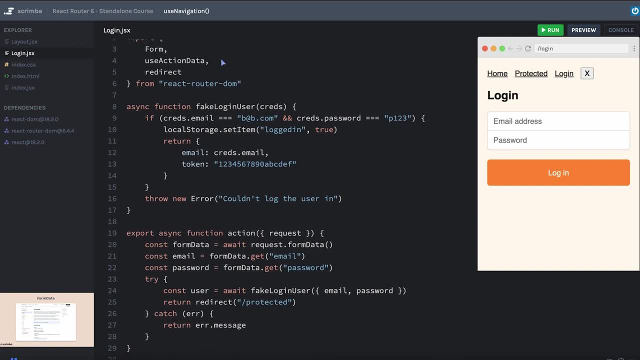 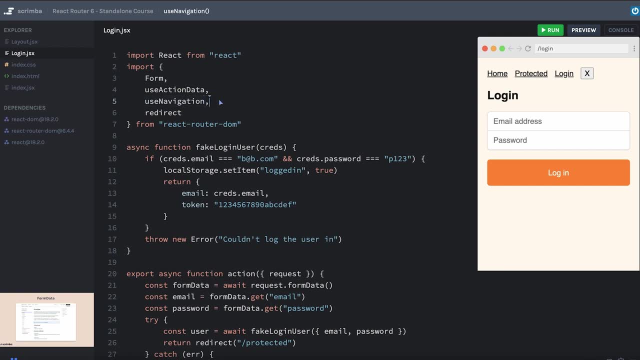 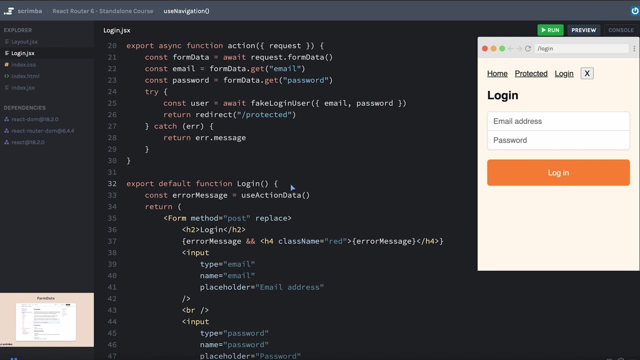 fortunately, react router gives us a utility that we can pull in, called use navigation. this is not to be confused with use navigate, and use navigation will give us an object that gives us information about the current status of navigation in our app. in other words, if react router is in the process of, for example, loading in a loader, that navigation object can. 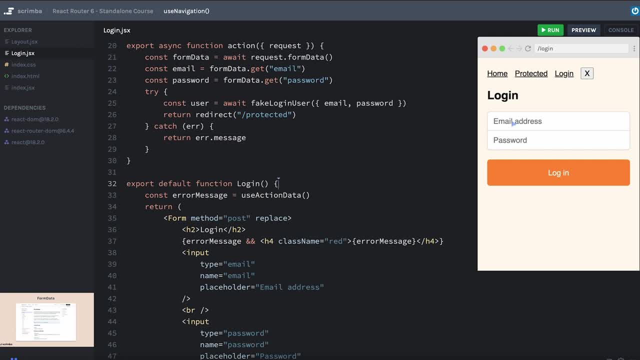 give us information about that. or if we're in the process of submitting a form, like we're doing here, it also will give us information about that. so that's actually pretty easy. we can just grab the navigation object we're going to use navigation and there's a property on this navigation object. 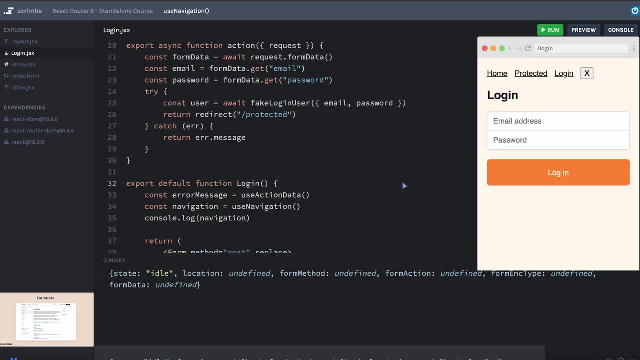 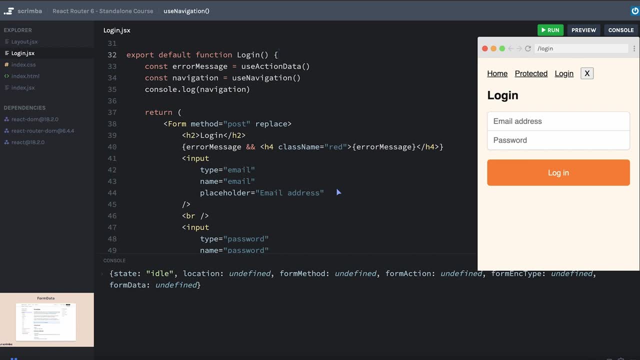 well, let's go ahead and just log the entire navigation object, open up the console, i'll hit save okay, and even just rendering our component for the first time we can see that it's an object. it has a bunch of different properties, but currently the only one that is not undefined. 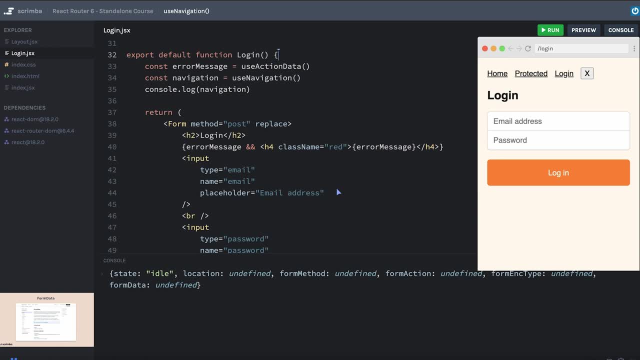 is a property called state and we can see that that state is set to the string idle. maybe you can see where i'm going with this. that navigation state is going to be our replacement for the local state that we had set up in our van life app. so now that i have access to navigationstate in 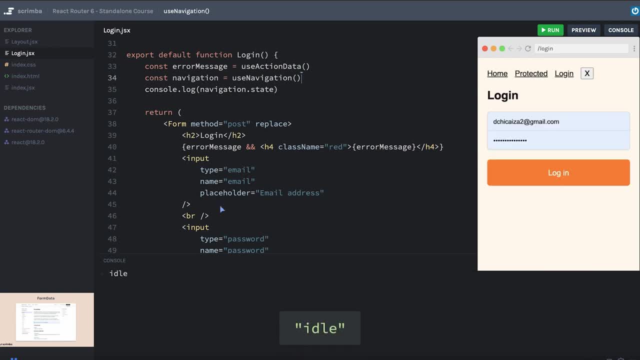 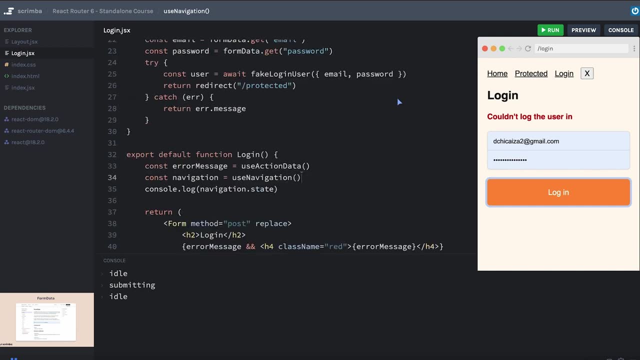 fact, let's keep the console log here. i'll hit refresh. we can see it's idle. i'll go ahead and click login. we can see that it changed to submitting and then it changed back to idle. in our case this is happening very fast because our login user function is just checking against. 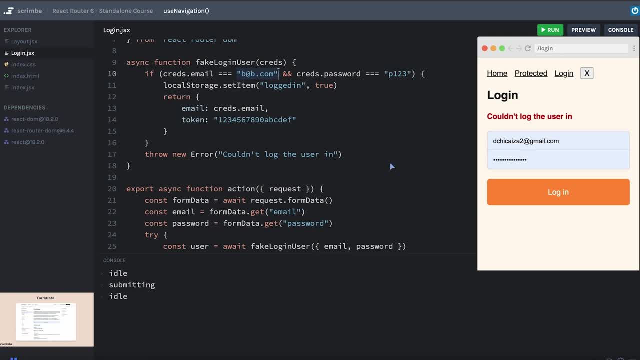 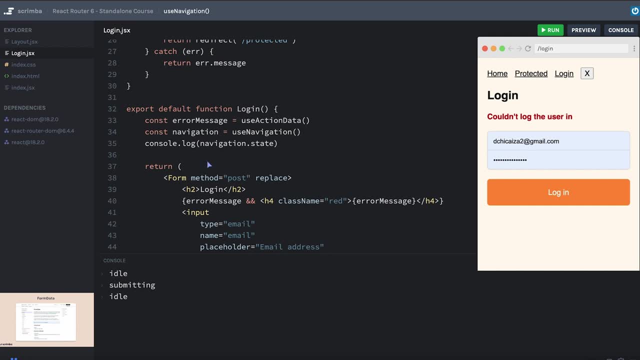 a hard-coded b at bcom and p123. it's not actually reaching out to any kind of database and so we don't even see a delay really, but it's cool to see that we have a lot of different options here. we can see that we have a lot of different options here. we can see that we now have access to some. 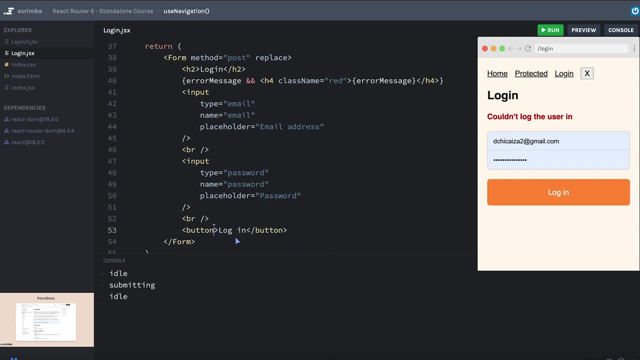 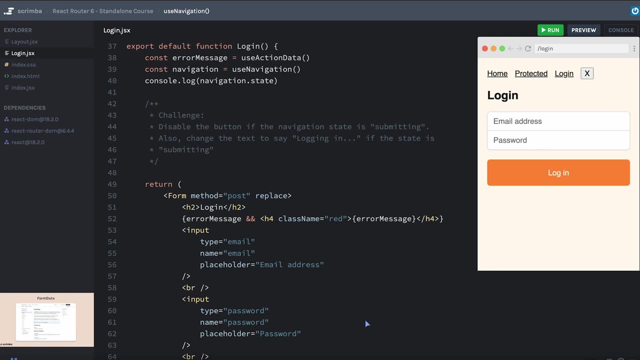 navigation state that we can use when we want to do things like disable the button. in fact, i wasn't planning on doing this, but let's make that a challenge, because you should be able to do this by now. okay, your challenge is to disable the button if the navigation state is set to the string. 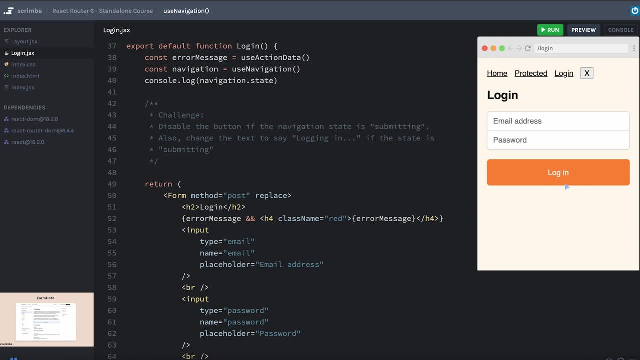 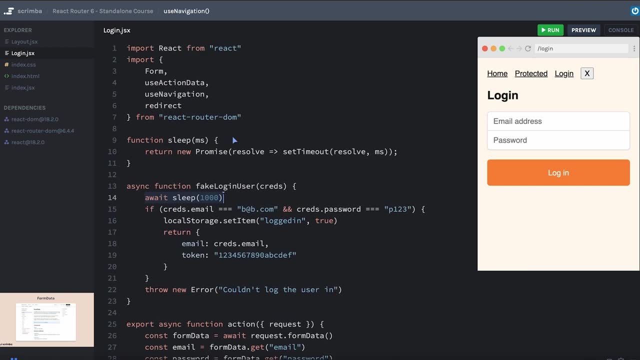 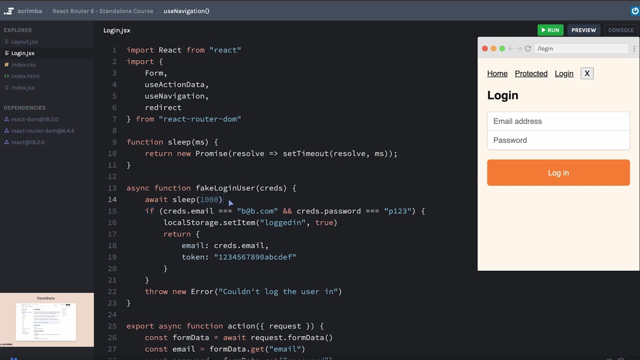 submitting, and also to change the text to say logging in instead of just login again, if the state is submitting now. because we don't have any kind of delay in this function. i added this little sleep function, which is just right here. it all it does is pause execution of this function for 1000 milliseconds, or one second, so that you 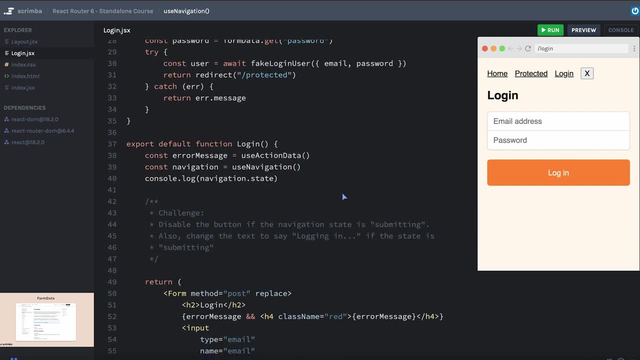 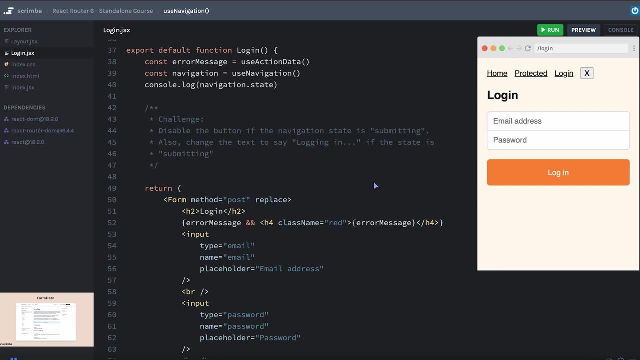 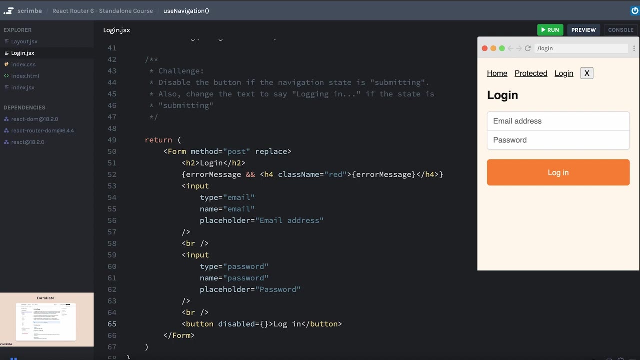 actually have a chance to visually see the change that's happening when you're logging in. okay, pause now and work on this challenge. all right, so on our button we can add the disabled prop and set it equal to. if navigationstate is equal to submitting, and that should handle the 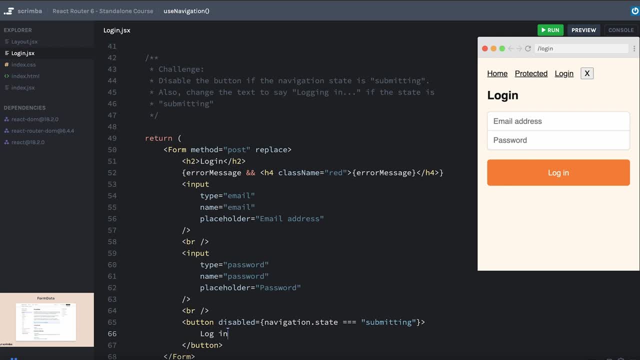 file. we've got to check that here and we're gonna do so. in the box we have the disable of the button and the text. we'll go ahead and wrap this in a javascript expression so that we can say navigationstate- i'm gonna spell this: right- is equal to submitting. we'll go ahead and use a. 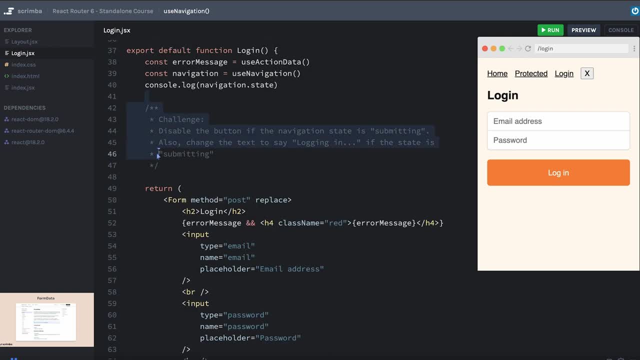 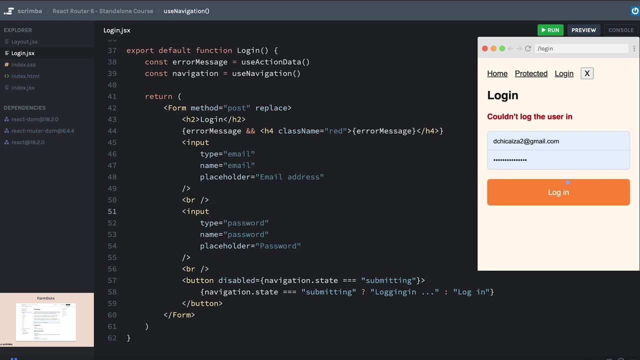 turner, here it's question mark. then it's going to say logging in, but otherwise it will say login. let's clean up our challenge text and we'll get rid of this console log while we're at it and don't have a space there. Sorry about that. So we can see that's working. the button is. 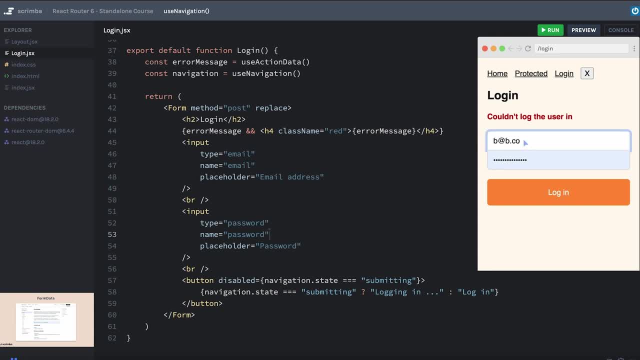 disabled And then, if we actually log in, we get the same thing, and then it redirects us to the protected route. Perfect, Okay, that's how we can set up navigation states, or, as we were calling them in van life, the status. So now we'll go back to van life and implement this method for. 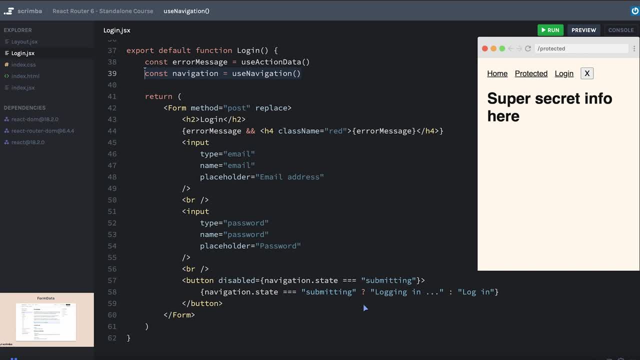 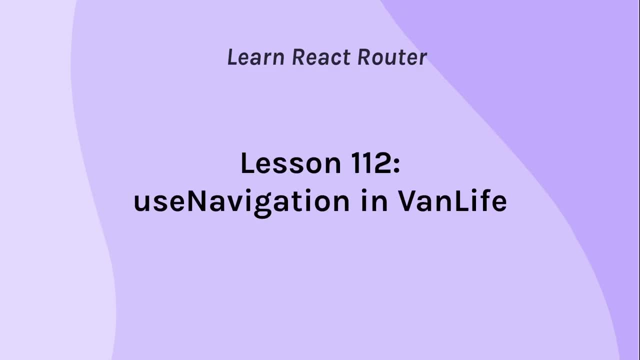 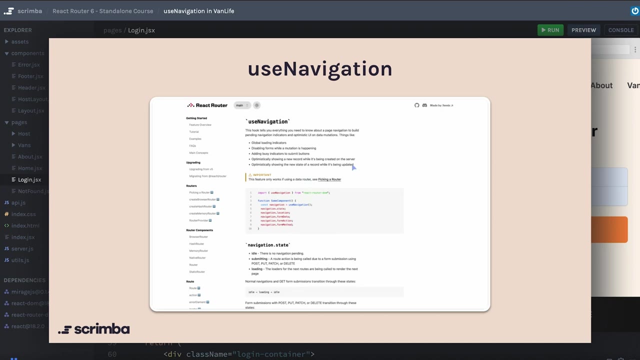 tracking our current navigation state, And that should allow us to finally get rid of our handle submit and the status state that we had. One thing I did forget to mention is that I have a link to the documentation for use navigation right here, So you can click the screenshot if you'd like to. 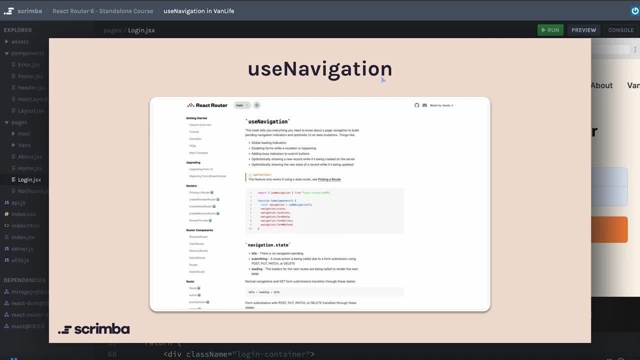 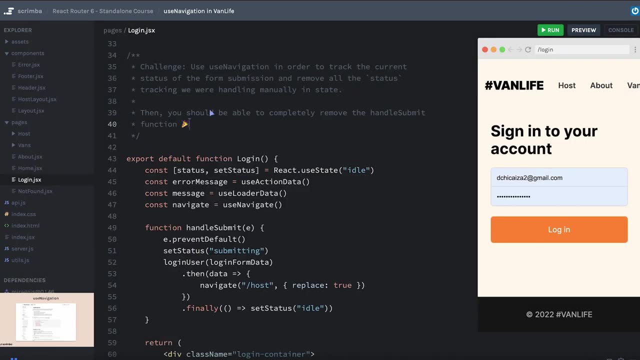 go read more about it. There is quite a bit more to the use navigation hook and that navigation object that we aren't currently using in our app, So it could be fun to go read up on it, But once you're ready, we have the challenge of including use navigation to track the current status of the. 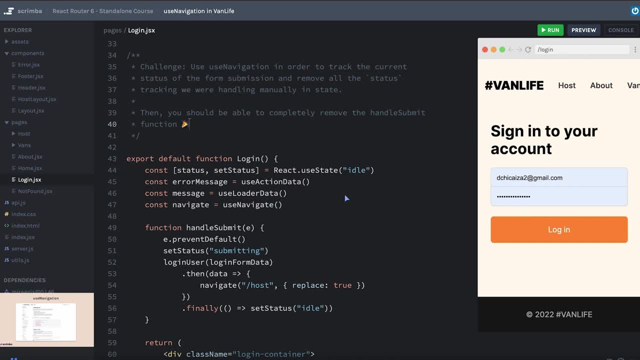 form submission and remove all of the status. So we're going to go ahead and do that, And then we're going to go ahead and remove all of the status tracking that we're currently handling manually in our state. Once you've done that and it's working, then you should just be able to. 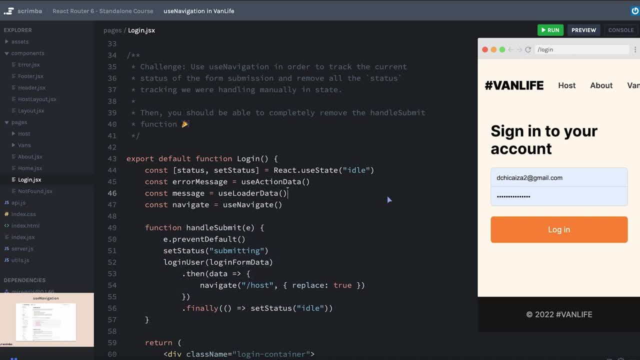 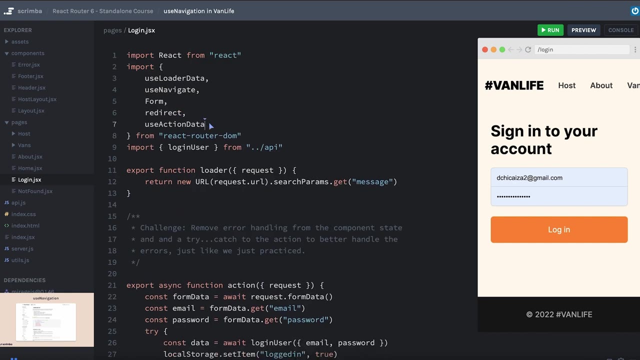 completely. finally remove our handle submit function. So let's get to it. Pause now and work on the challenge. Okay, let us pull in use navigate. Actually, you know what? we don't need to use navigate anymore. So I'm just going to tack on to the end of that and pull in use navigation. 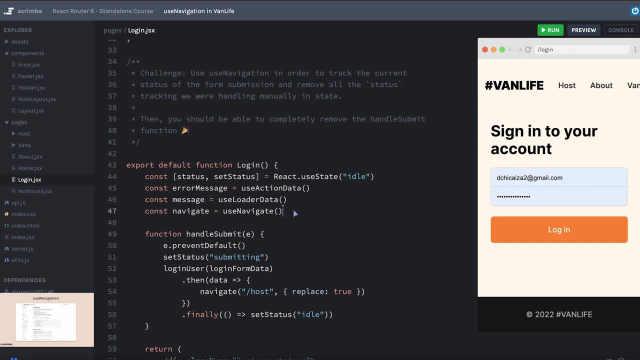 instead. Let me just double check. we're not using navigate so we can get rid of this. this is going to go away when we get rid of our handle submit function. Actually, you know what I'm impatient. I can't wait. I'm just going to remove that completely. Wow, that looks so much cleaner. Okay, we're. 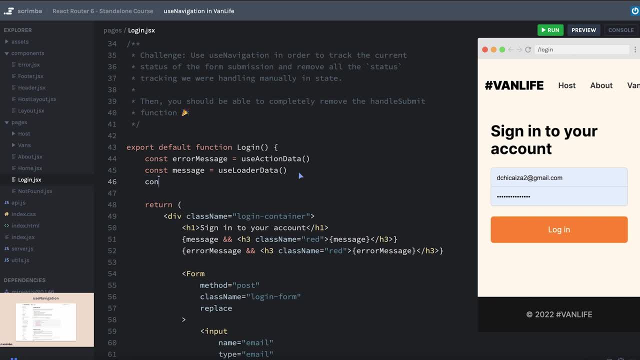 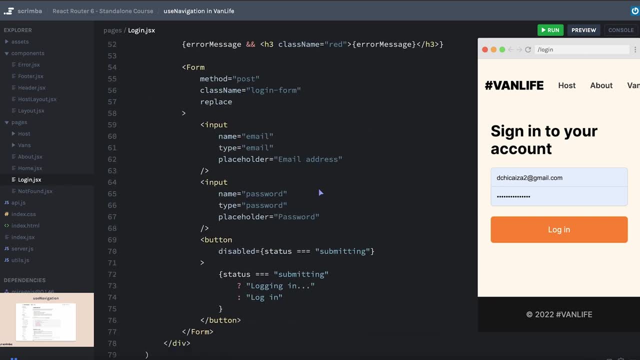 broken. Let's go ahead and fix what we have broken, So I'm going to pull in. navigation is equal to use navigation, And you can probably see that I was already using the conventions for use navigation just because I knew that's what it was going to look like, So I'm going to go ahead and pull in use. 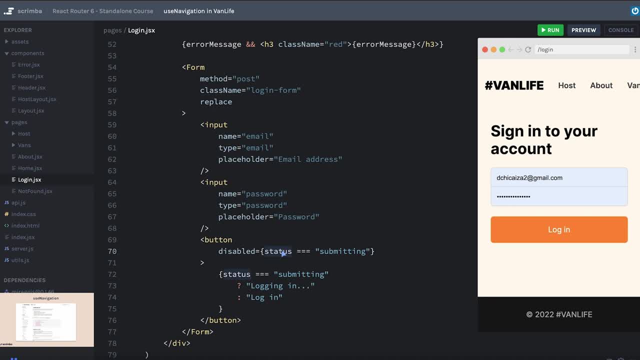 navigation is equal to use. navigation is equal to use navigation, And that's what it was, Which means I can just change status to say navigation dot state instead. the idol value and the submitting value was one that I chose because I knew that it mirrored this navigation states. so everything else. 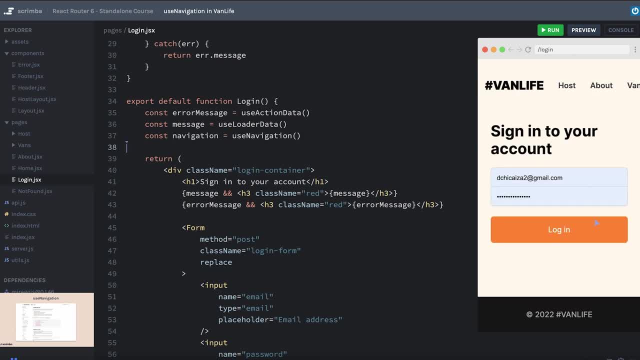 should be able to stay the same. Let's clean up our challenge text. we'll hit Save And let's give it a shot, So I'll try logging in without anything. Okay, we did see, it's a logging in, although I did. 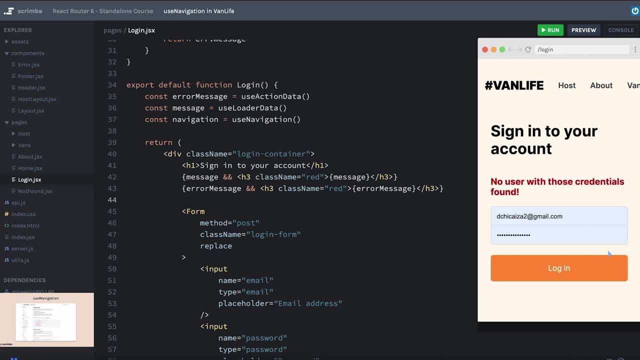 Okay, so let's go ahead and try it again. I'll hit refresh logging in. Okay, perfect. No user with those credentials found will log in via bcom p123.. Login and it takes us to the host dashboard. So now we can see that our form. 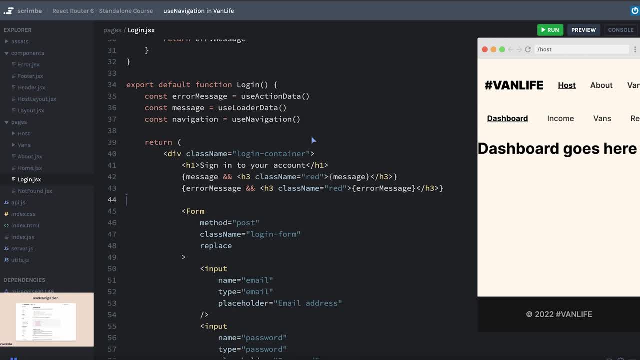 is doing everything that it was doing before, But we've been able to offload a lot of that boilerplate, imperative stuff that we were doing before with all of our local state And we've offloaded it to react router so that it can handle. 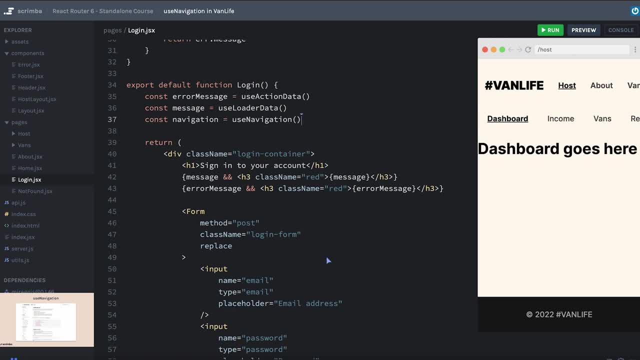 some of those very common tasks for us. If you've been able to follow up until this point, congratulations. I know that we've covered a ton of ground. we've really refactored a lot of things, including a complete paradigm shift. that. 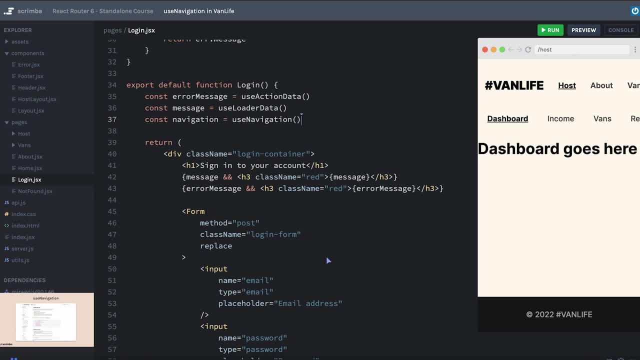 you might not be used to if you've been working in react for a little while. I've heard someone called these new data layer API's with react router, kind of like remix light, And the truth is, if you can grasp what we've been doing here, 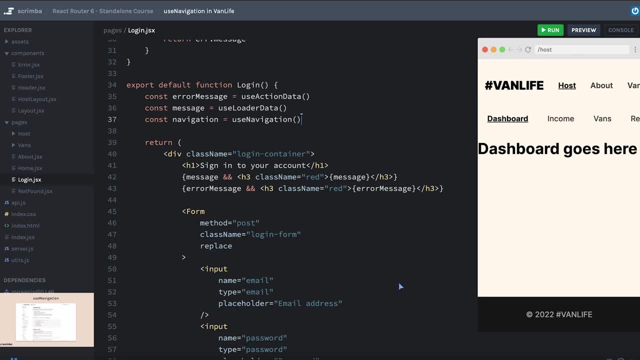 then you would be really primed to jump into remix and be able to start creating full stack applications. There's quite a bit more to learn with remix as well, But you'll be pretty surprised to see just how familiar remix feels once you've become accustomed to the patterns of 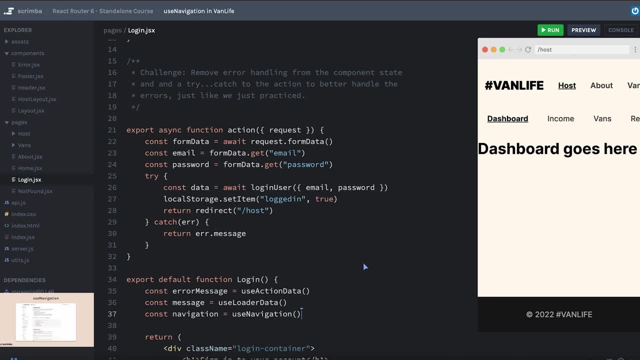 using actions and loaders, changing when data fetching happens with our components and all of the benefits that come there, And in the next few lessons we're going to be touching on a little bug that we have, or maybe it's just a inconvenience with the user experience when it comes to redirecting to the 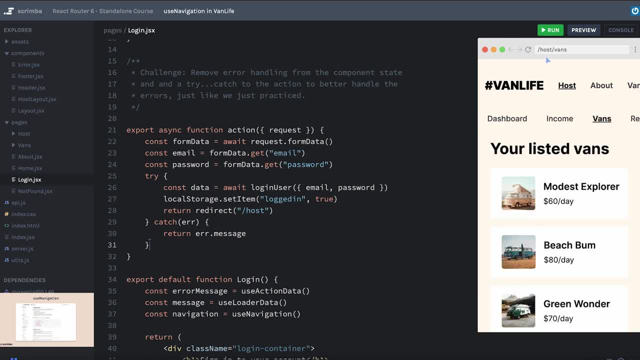 login page. For example, if I go to a nested protected route like slash host, slash vans, slash one here, and I'm not actually logged in, so I'll log out with my silly button here And then I'll try to refresh the page now that I'm logged. 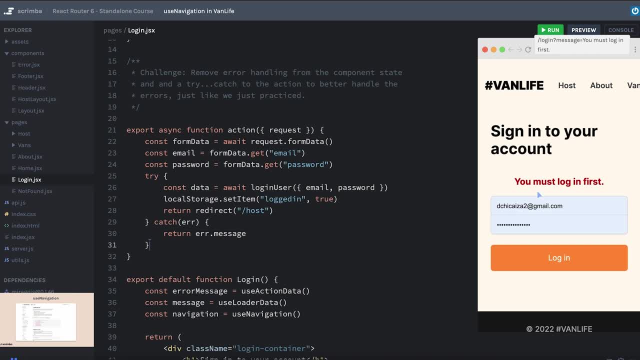 out. we'll see that it takes me to the login page And so I can go ahead and log in, But then what will happen is it will automatically send me to the host route. It's not a bug per se, it's just kind of a bad user experience Because 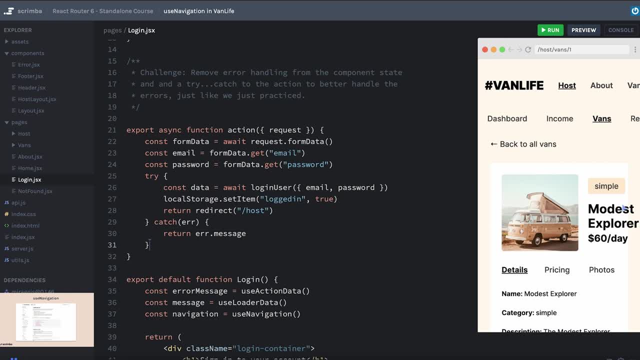 what I'm expecting is to go back to slash host, slash fans, slash one. one way to fix this involves two different parts, So we'll be jumping in and out of the host route, So we'll be jumping into fixing that. for moving on to some of the last, 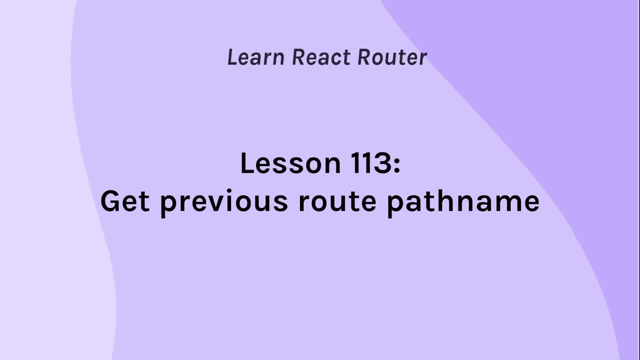 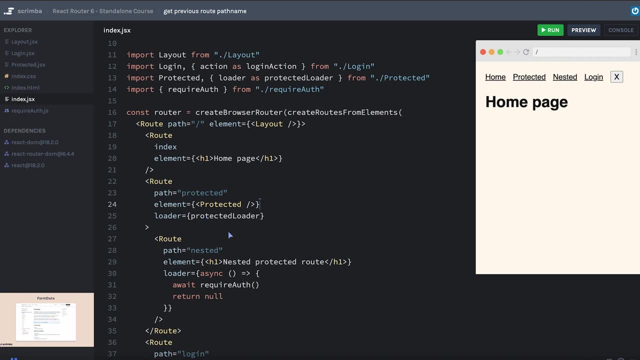 features that we have to learn. I've made a few small updates to our practice app here. First of all, I've moved the inline protected component that we had- it's really just an h1- and the inline loader function that it had over to its own. 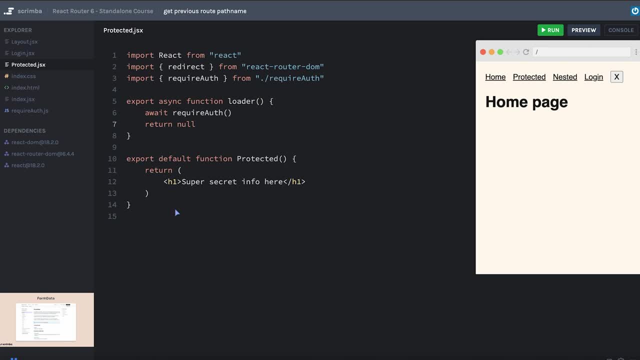 separate component file here, So we have the actual component right here. Again, it's just an h1. But this way we have a separate loader that lives in the host route. So what we can do is we can put in the inline protected component. 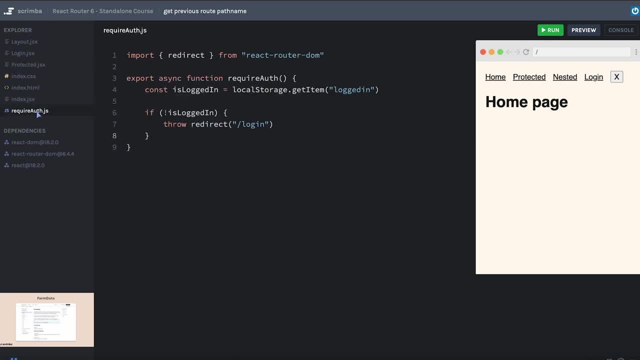 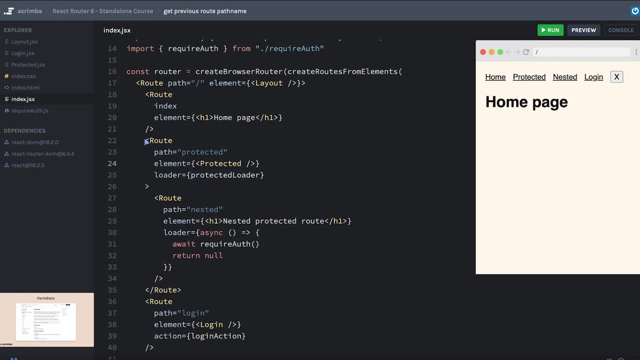 here And then we can also do some other things over here. So I've moved the inline protected component to the host route And then we can do some other things over here, And then I'm importing the pieces that I need, like redirect from React. 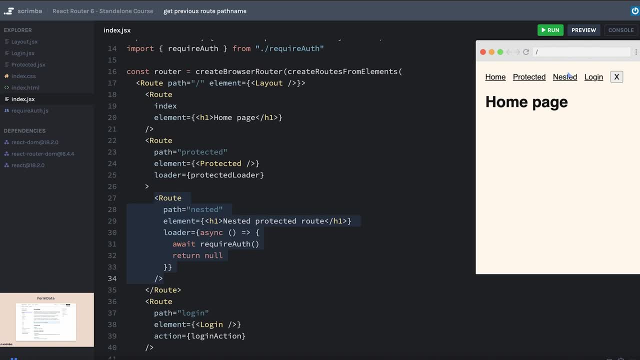 router and a new require auth function which I just put over here in its own utility file, here called require auth. Also, for the sake of demonstration, I slash protected And if I go to nested it takes me to slash nested in the URL. Actually, you know. 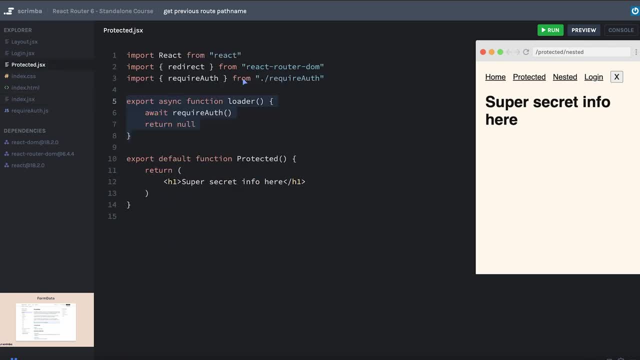 what the nested has, this h1. And the reason it's not showing is because I need my outlet. So go ahead and put that in here And we'll just wrap this in a fragment and put in our outlet. Okay, so now with the nested route, we have this nested protected route h1 showing up, And again, that is. 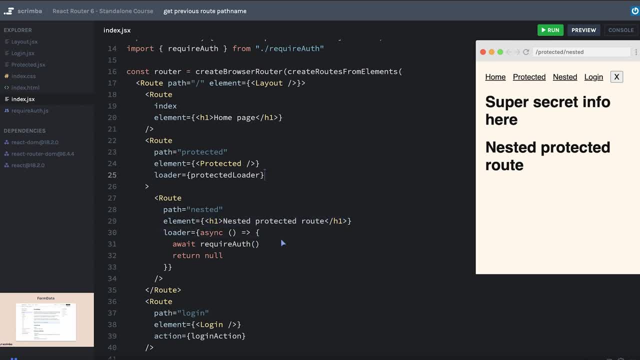 just here in line, just for simplicity sake. Okay, so those are just some simple updates I've made, And the reason that I did that is because let me go ahead and log out. Let's say we want to get to this slash, protected, slash nested route, which I can get to by clicking this nested link here. So 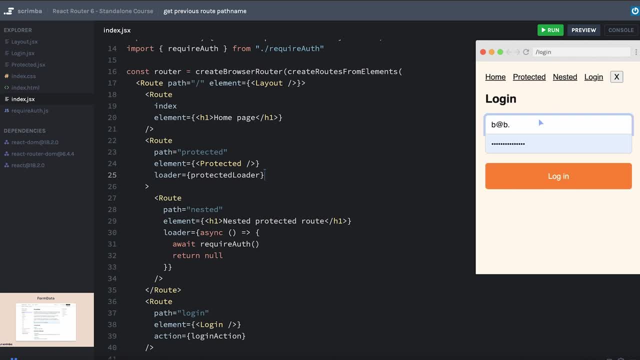 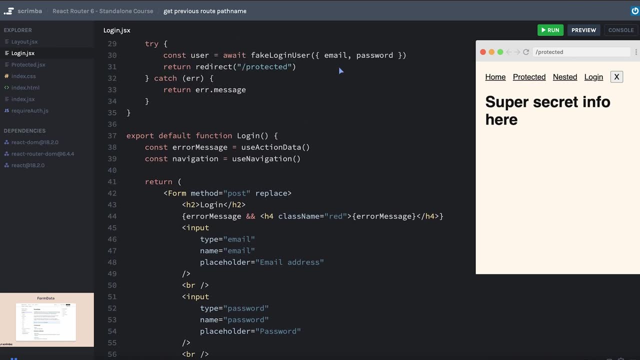 I can go ahead and do that. It takes me to the login page. I log in with b at bcom p 123.. And because of the way that we've written our login component up here in our loader, we have hard coded that it should send us to slash protected. In our case that's not terribly difficult to then. 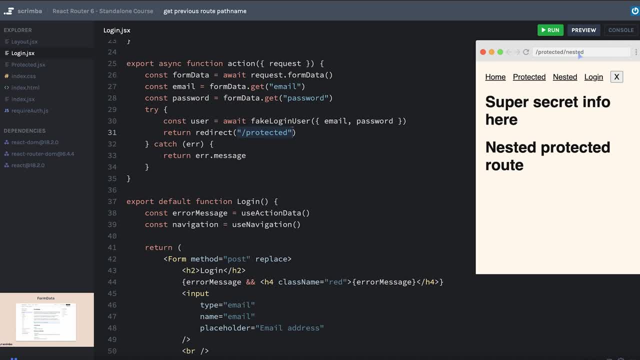 just get to the nested route by clicking the link. But the point is, if we did have some kind of complex nested route that the user was trying to get to and they were redirected to the login page, if we just hard code that we want to send. 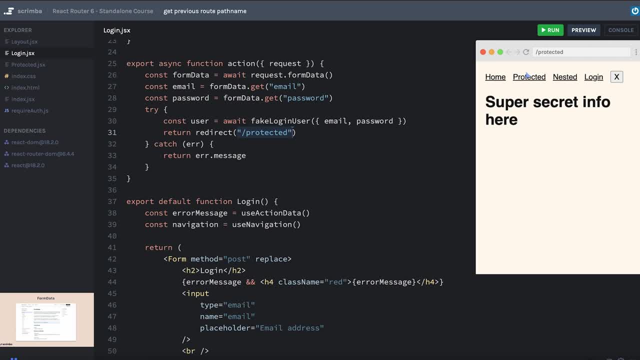 them to slash protected. it's kind of a weird user experience. Let's say, for example, they tried to get to this nested route by clicking a link from their email And maybe it has some kind of user ID in it that isn't accessible by navigating somewhere on the site, But instead you have to. 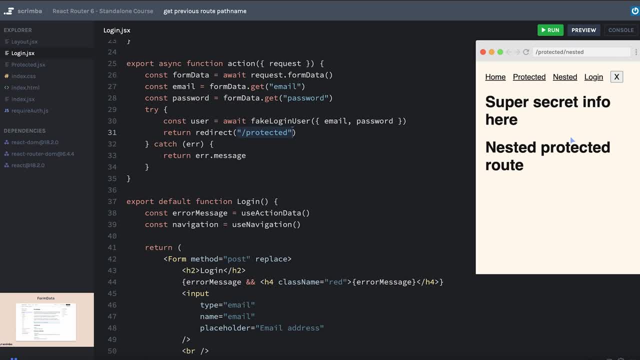 get there- or at least it's much easier to get there- by clicking the link in the email. If we were sending them to the slash protected route, then they're going to have to open up their email clients again and click on the link again. Now that they're logged in, hopefully it opens in the 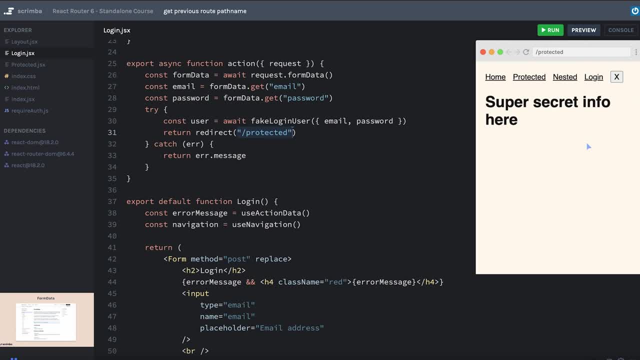 same browser and still has the same session, they don't have to log in again. So I'm hoping that you're seeing a limitation by hard coding the slash protected route here when we redirect the user after logging in. So what we are going to focus on is making it so that, if the user- let me- 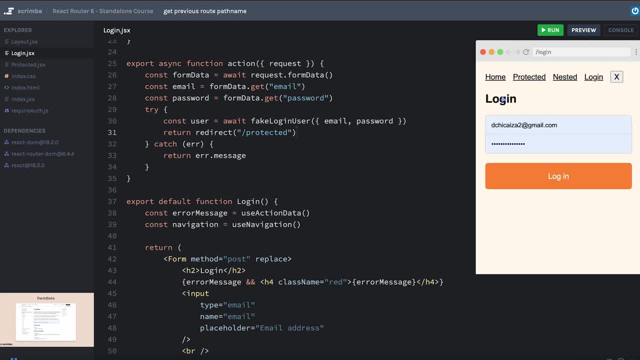 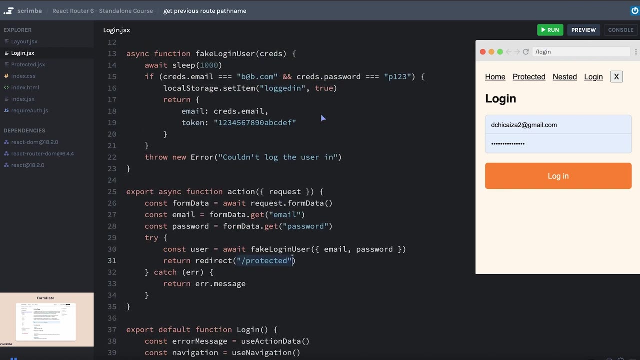 log out again and try going to the nested route. if the user is redirected to the login page, that they're connected to that nested page instead of the hard coded slash protected route. Now, in the past we have been able to get the path name by using the use location hook that comes with react. 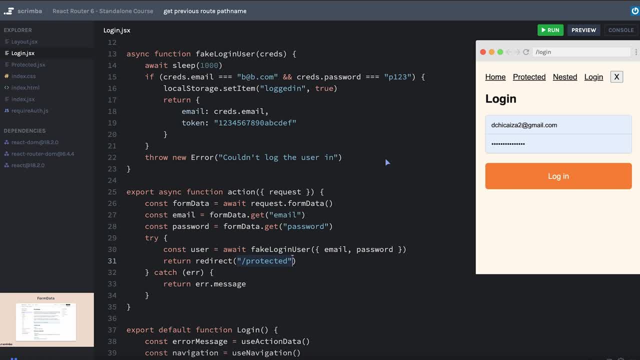 router And we could make that work. However, because we're now using the data layer API's with react router 6.4, we have another way that is a little more congruent with the new paradigm that we're using. you see, our loaders and our actions will both receive access to this request. object: 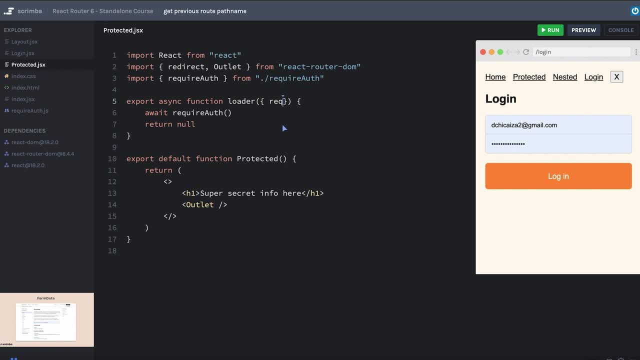 let me go over to my protected route And I'm going to go ahead and click on the nested route loader and pull in that request object And we will go ahead and console log the request. Actually, let's do request URL. Well, actually, no, let me. let me do request first. we'll hit save. I'll make. 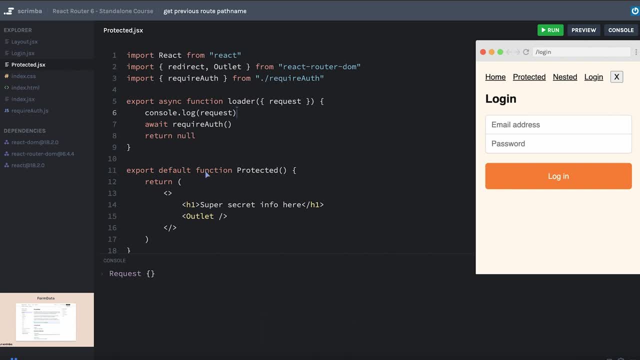 sure I'm logged out. I'll go to protected and we'll open the console. Okay, so we see that we have a request object And this request object is the actual native web request object. it comes from the request constructor. you can go to the Mozilla Developer Network docs in order to learn. 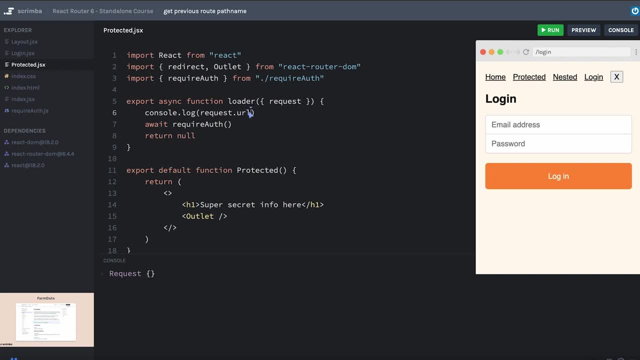 more about request objects And we're going to go ahead and click on the request object And we'll go ahead and click on the request, And request objects have a property called URL, which gives us access to the URL. Now we'll be able to see that when I refresh and click protected, we get 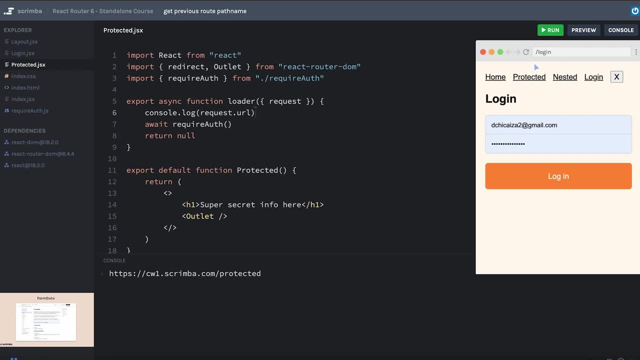 the entire URL and it's just a string In our case, because our mini browser is running on the scrim platform. it shows our full protocol. we have HTTPS and then the cw1.scrimacom as our base URL, And then at the very end we see slash protected. Now I could go out of my way to try and 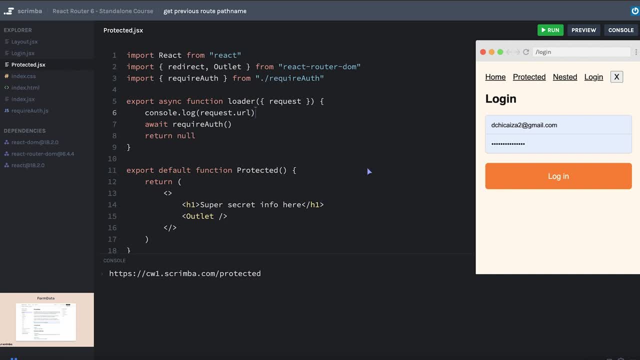 grab the slash protected portion of the URL using some kind of string manipulation. But another thing we can learn is that we can construct a URL again using the native URL constructor. So let me actually set this as a variable. I'm going to say const URL equals new URL, And this capital URL that comes from just 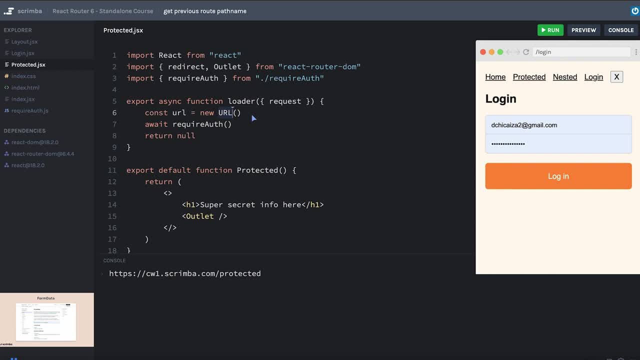 web API's, So this constructor is just universally available. as a constructor I can use as long as I'm writing my JavaScript code or the front end, And when I pass the actual URL, the string URL, by that request, that URL, I've now created a URL object. Let's go ahead and console log URL. 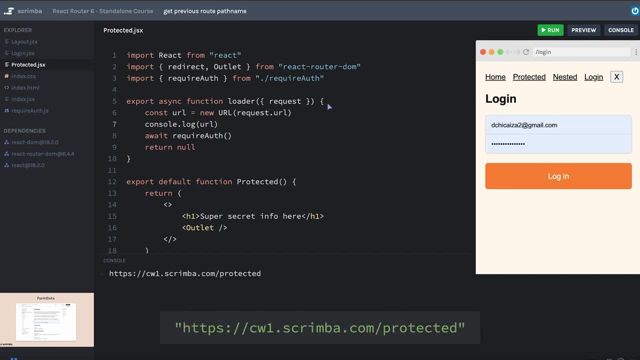 And I'll try to get to protect it again. Okay, so it's string representation is showing up exactly the same, But what's nice about this URL object is I can actually access properties like path name, for example. you might remember when we were using the use location hook, the location had 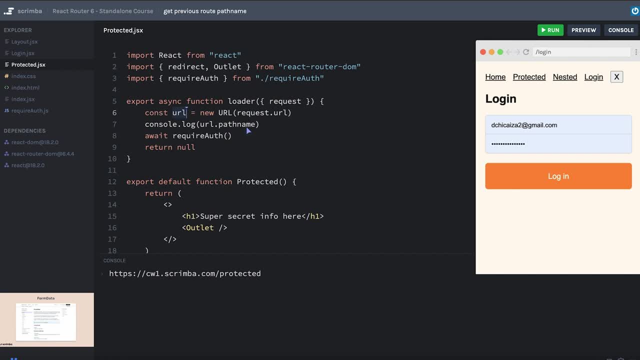 something called path name And that is just coming from this URL object, And so if I were to console log URL dot path name, go to protected, I now have immediate access to the path name that I was trying to get to, And if I go to the nested route, I can see that it gives me the full path. 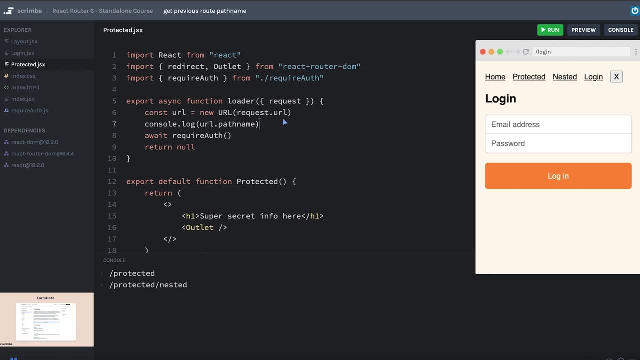 name of the nested route: slash protected, slash nested. Now I do want to address something here. I think, for maybe the untrained eye, this might seem like a lot of additional work to get to just the path name, having to pull in the request object and create a new instance of a URL object. and then access the path name property. But the other thing I want to add here is I want to have a path named property where I can say if I'm going to go back and create a new instance of a URL object and then access the path name property, but then add to that path name property and then access the path name property. 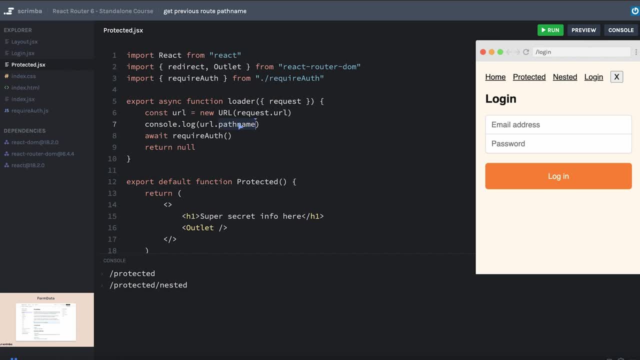 property. but to be honest, having been in the game for a while now, I didn't really take the time to learn some of these platform APIs, like the URL constructor, until this became pretty much the right way to do this in Remix and by association, React Router. 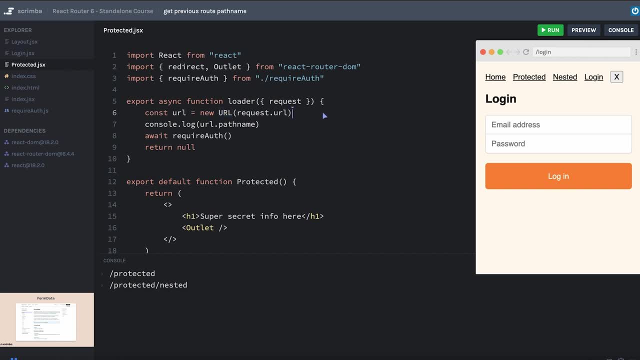 So, honestly, I actually really appreciate that I've spent a lot more time learning native web APIs and spending time on the Mozilla developer network docs than having to parse through a bunch of Google results and stack overflow questions, hoping that I get the most modern answer based on the newest version of React Router. 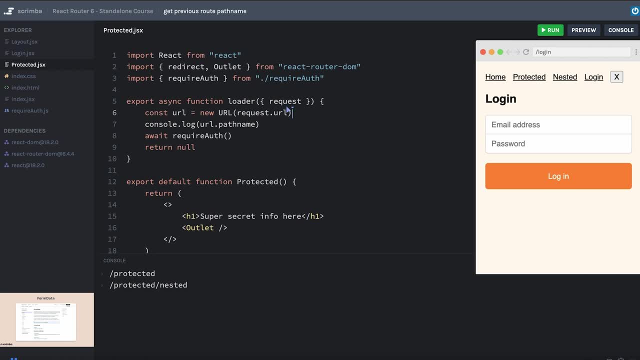 But instead I can just spend time on the Mozilla developer network docs and find the information I need, because it's using the platform, It's using the constructors and the tools that already exist in the web. Okay, we've spent quite a bit of time just to get to this URL, that path name, but hopefully 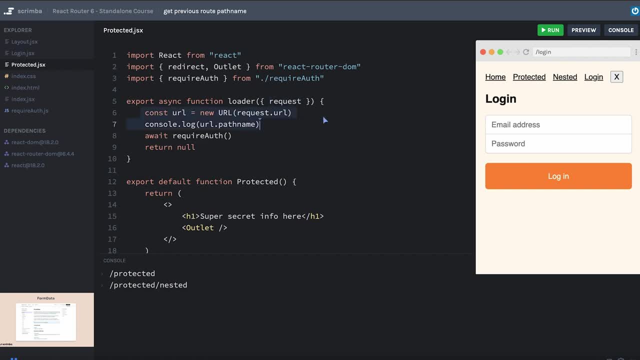 you can see, in the end all I did was pull in the request, create a new URL object and then access properties from that object. So, for the sake of time, we're going to end this scrim here, and in the next scrim we will. 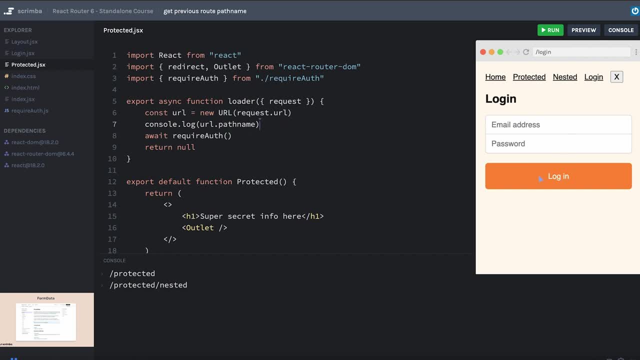 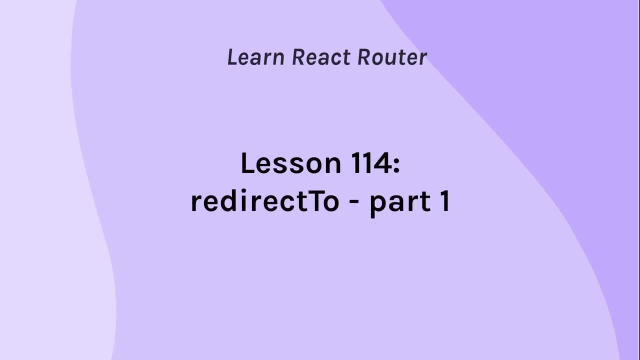 talk about how we can make Use of this so that, after the user logs in, they can be redirected back to this URL, dot path name. So that's what's coming up next. Okay, so we've started diving into the weeds on how we are going to solve this problem. 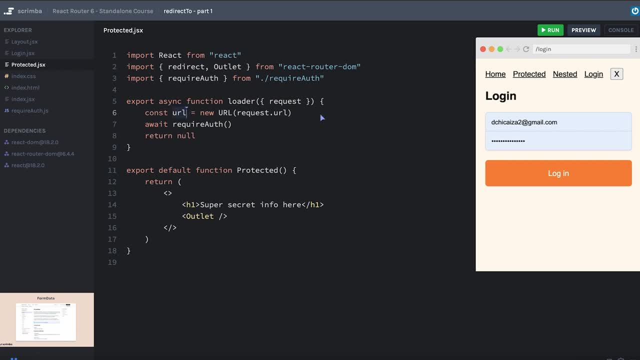 We now have access to a URL which has a path name property that we can use, But what exactly is the overall strategy? I think that might be helpful for us to look at. Remember, it's our require auth function that is in charge of redirecting. 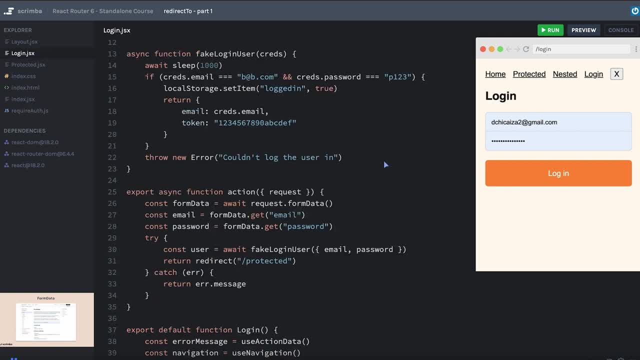 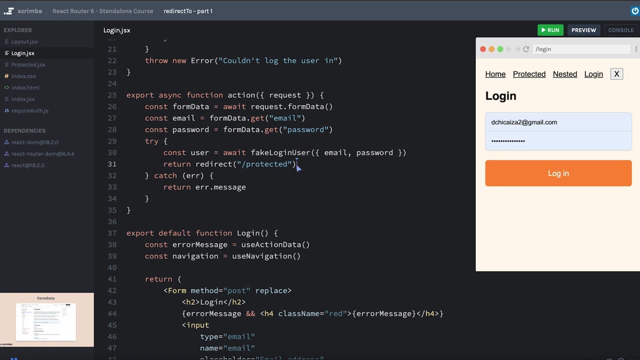 Users to the login page, and then the login page is in charge- let's see where is the action function right here- is in charge of redirecting users to the route that they're supposed to go to, And this is what we're trying to fix. 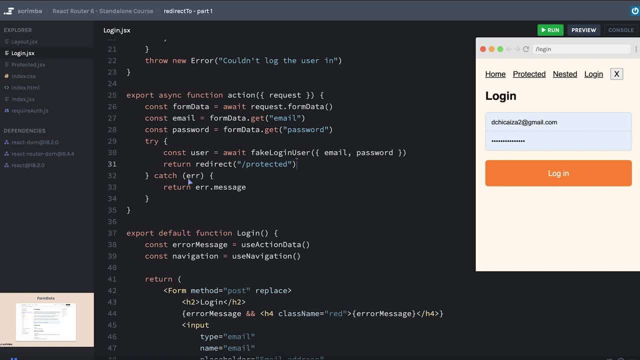 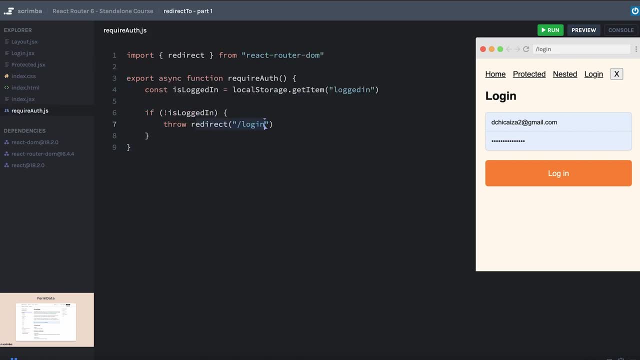 Remember we don't want this to be hard coded to slash protected. So that's kind of the workflow that we have. The protected loader runs that calls require auth. that redirects people to the login page and the login page, once they successfully login, redirects them to the route that they 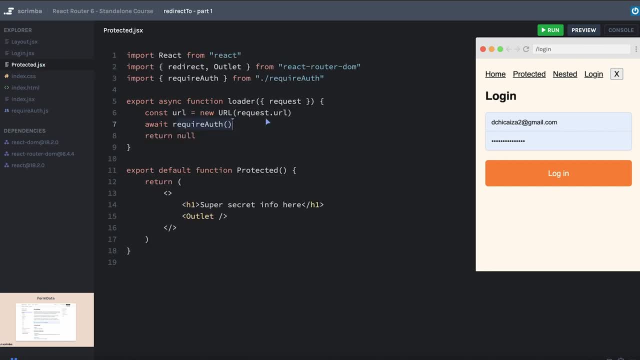 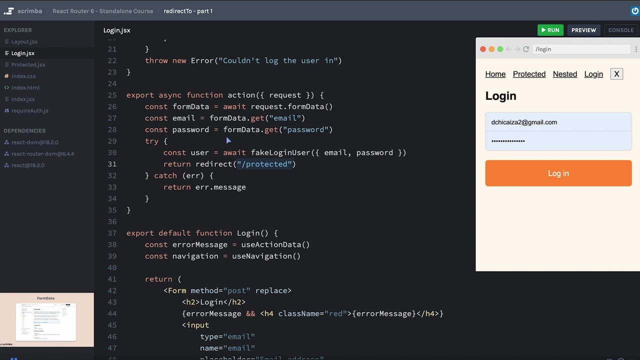 are trying to go to. So how do we get information from our protected route, which is where we have access to the request and easy access to that path name, to the require auth function and then from the require auth function to the login component? Well, we saw very briefly when we redirect a user using the navigate component or the 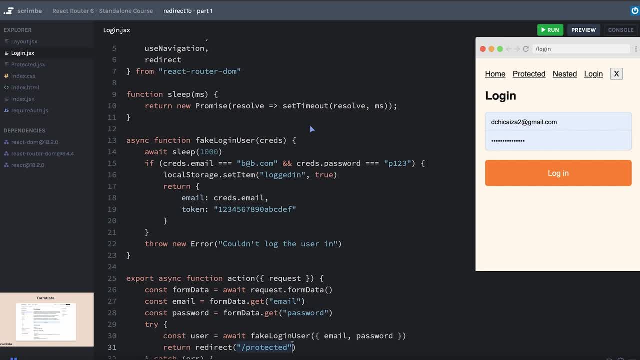 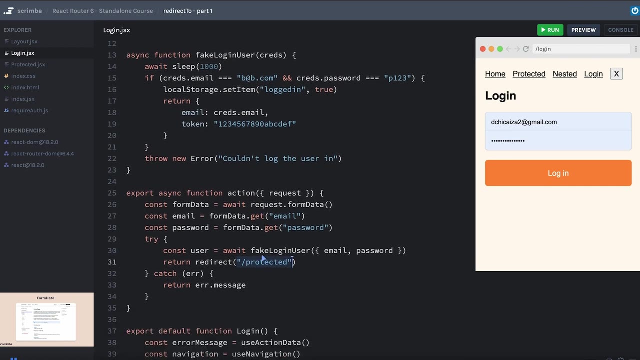 use navigate hook, we're able to pass some state through the navigation events to the next location and that location object can grab the state that was passed to it. However, those are hooks and those have to happen inside of components And mostly we are working inside of loaders and actions. 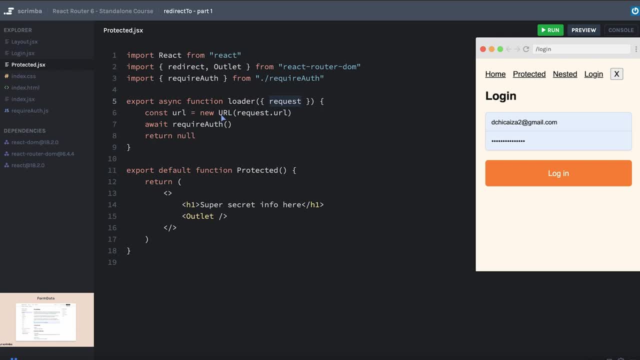 Because of that, the most common way is for us to pass information through the URL. So actually right here in require auth when we redirect someone to the login page. I want you to think for a second. how can we pass information using the URL? We can use search parameters or query strings just like we did in van life. We can use search parameters or query strings just like we did in van life when we created a query string. We can use search parameters or query strings just like we did in van life when we created. 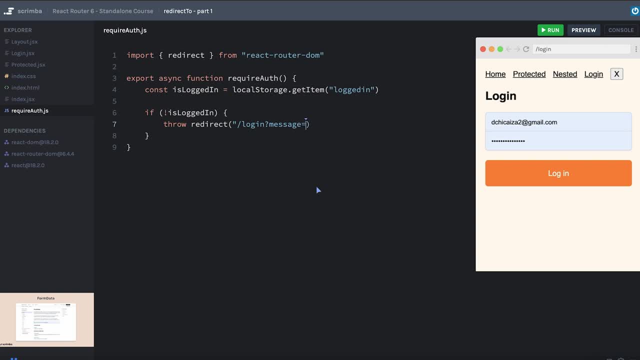 a query string. So in van life, where we said question mark message equals you must log in first, We can use this same strategy to pass information from our require off function to the login page and then have the login page make use of that information to redirect us back to. 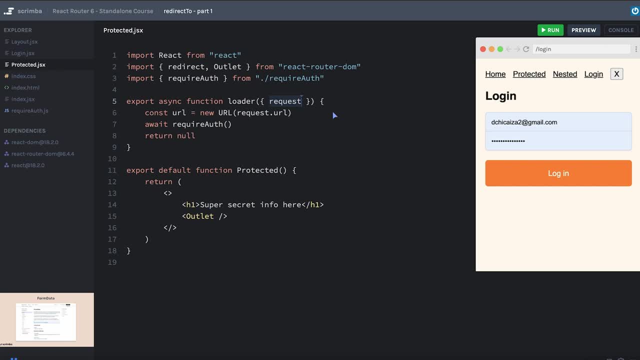 the correct spot. So the next question, then, is: how do we get this path name that we're able to access on our URL object to the require auth function, so that we can include it in a query string To get a path name that we're able to access on our URL? object to the require auth function. 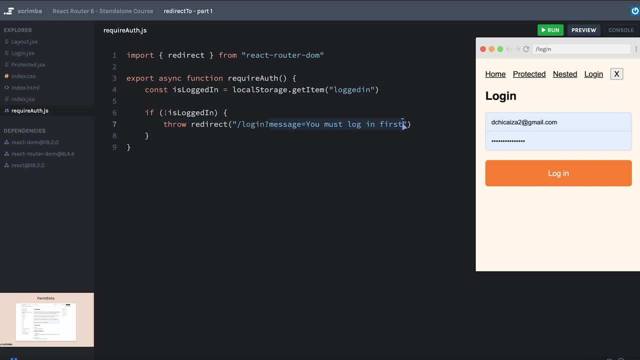 a query string. Maybe this would be a query string like redirect to. we'll set that equal to some question marks for now, And actually this seems like the perfect opportunity for a challenge. Okay, so your challenge is to figure out how you can get the path name from this URL. object. 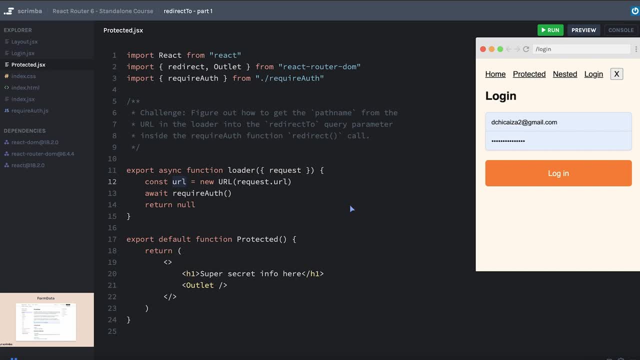 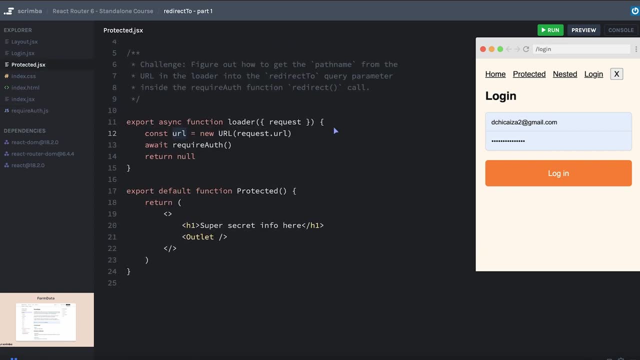 from this loader into the redirect to query parameter inside the require auth function, right here where the question marks are. So let's come back here to the challenge text. Okay, pause now and work on this challenge. One approach you may have taken was to just pass in the URL dot path name directly to the require. 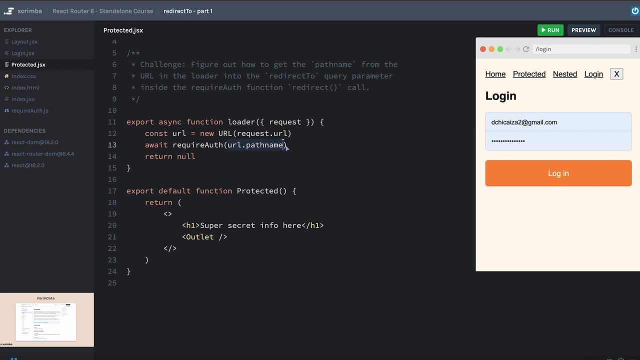 auth function And then over in require auth, we would receive the path name and just stick it into the query string right here. However, I happen to know that I'm likely going to be calling require auth, And then I'm going to be calling require auth, And then I'm going to be calling. 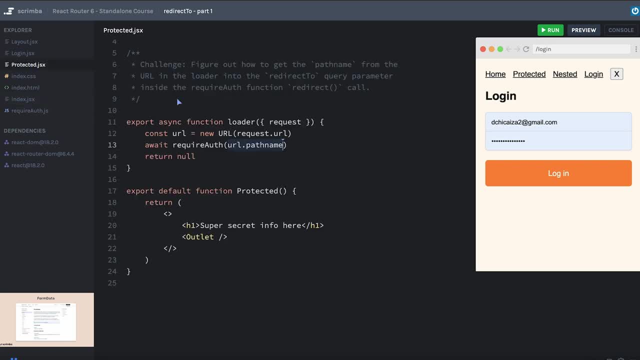 require auth in more than one place, which means if I did it this way, I would need to run this code and this code every time I wanted to use require auth. So instead of that, I'm going to copy this line and get rid of it and then just pass the entire request object down And, that way, require. 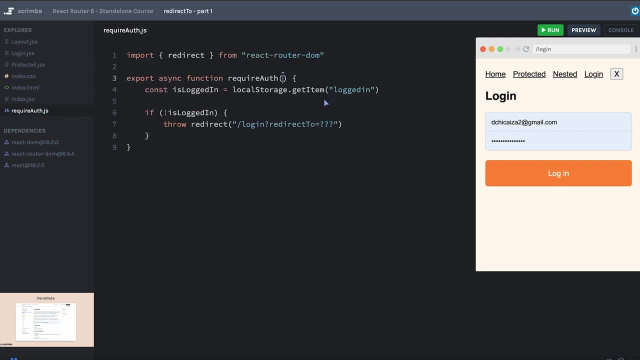 auth can do that logic and figure out exactly how to get the path name. So we'll say it's receiving a request object And I'll paste in that line. I'll even make a separate one that says dot path name. actually I'm just going to tack on dot path name, since that's all I really care about. 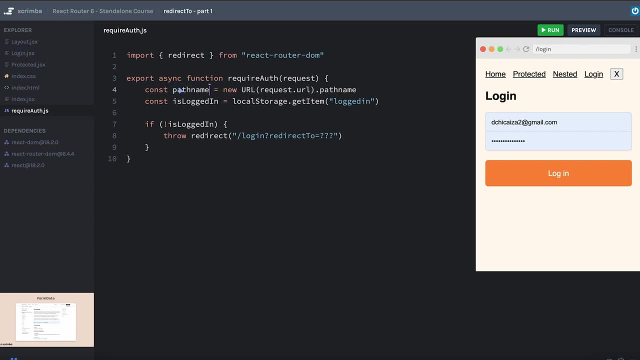 And then we'll change our URL to say path name And then, now that I have that value, I can stick it here inside my string. I'll make these into template strings So I can do my interpolation here and just say: we're going to pass the path name as the value to the redirect to query string. 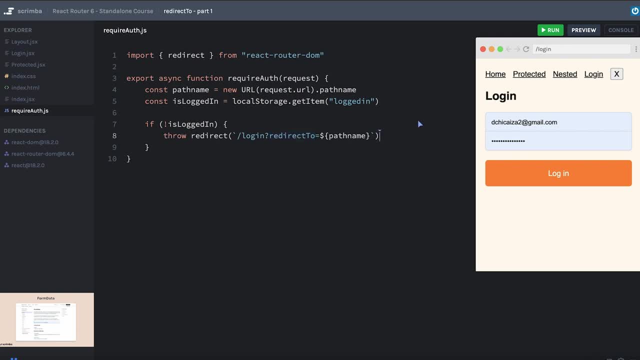 Okay, we've covered a fair amount of ground for one scrim. So in the next scrim we're going to see how we can from the login page. we're going to see how we can. from the login page, we'll see how we can directly redirect back to the right spot when the user logs in. 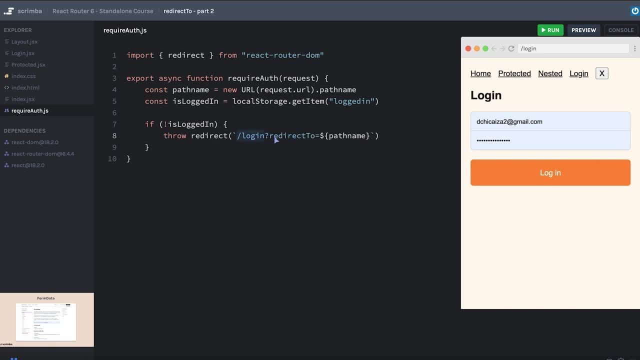 So we are sending users to the login page. we're passing the information about where we want them to redirect to after the login is successful. So I want you to pause here and think: where will I need to write code next? Okay, if you said that we need to save the results in the video editing, I'm going to save them in the video editing screen. 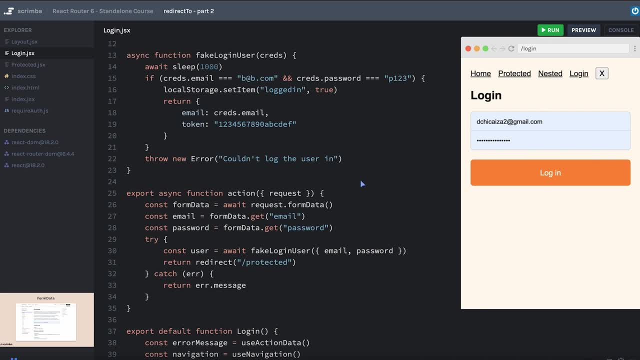 to go to our login page and our login component. you would be correct. But if that was all that you came up with, I want you to think even more specifically. I'm here inside of my login file that has the action and the login component: couple helper functions that are just helping. 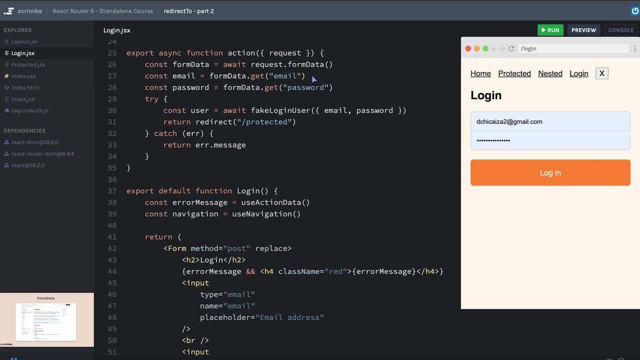 us kind of fake authentication for now. So, more specifically, where am I going to receive that query string that should be coming in through the URL? Remember, as long as I'm logged out and I tried to get to one of these protected routes, I now have redirect to equals slash. 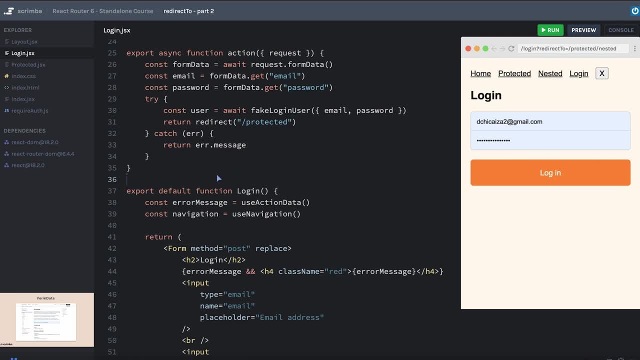 protected slash nested in my URL. So again, more specifically, where in this file, loginjsx, am I going to receive this redirect to value, so that I can well redirect to the correct spot? Well, technically, I would have access to it inside of a loader function. 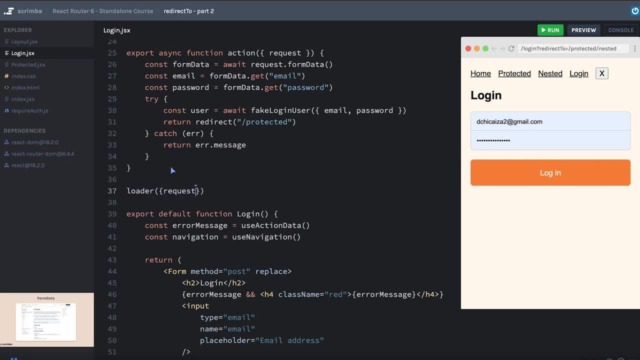 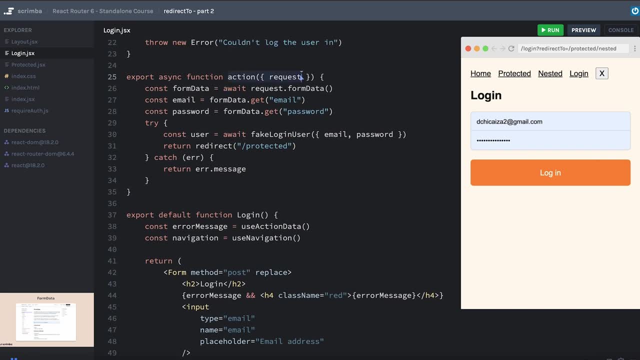 if I created a loader function, I would be able to access the request object. However, the loader is not when I want to redirect to that new location. it's right up here in the action. we already have access to our request And so I can use. 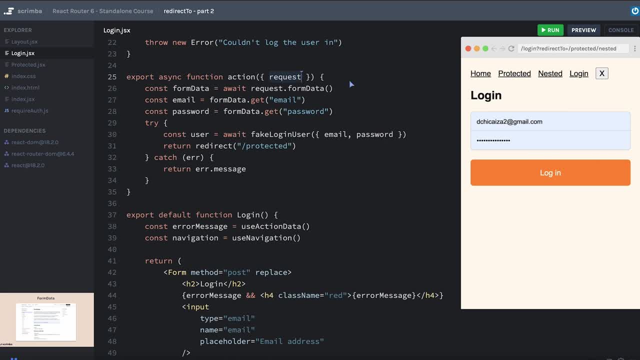 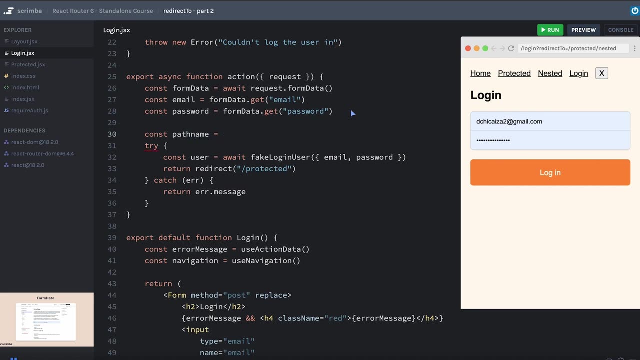 this request to grab the URL, grab the search params from that URL and use that as my redirect value right here on line 31.. So right here, above our try, we will maybe just get our. we'll say const path name is equal to, and then I can just grab the URL. I'm going to do this, all kind of. 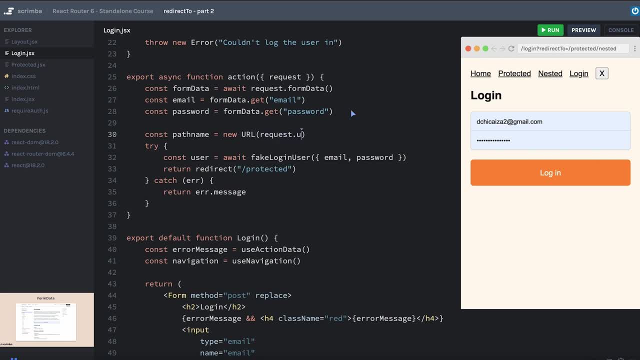 chain together. So I'll say I'm going to create a new URL from request dot URL. that's going to give me a URL object And then I can grab a property on it called search params And that is an object that has a get value And I can grab the search param with the redirect to key. 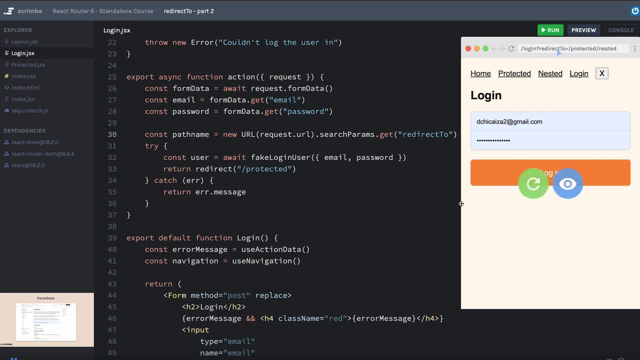 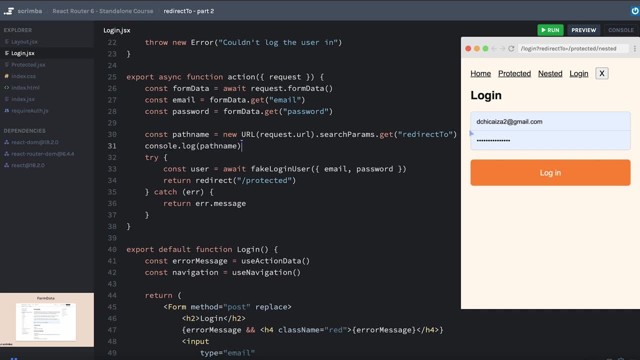 which should get me the value In this particular case, as we can see in the URL: slash protected- slash nested. let's go ahead and console log that console log, the path name. And because this is is inside of my action, i'm only going to see this console log if i try to submit my form. so i think. 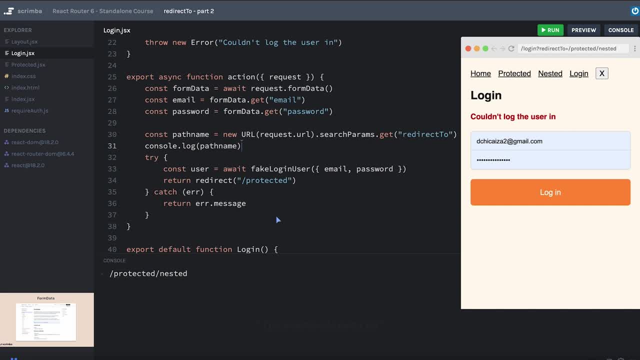 i can just hit login and, sure enough, there it is: slash protected, slash nested. so all i need to do now is to replace this protected with path name. okay, let us give it a shot. i'll refresh. make sure i'm logged out. i still have my redirect to in the url, so i don't need to change anything there. we'll. 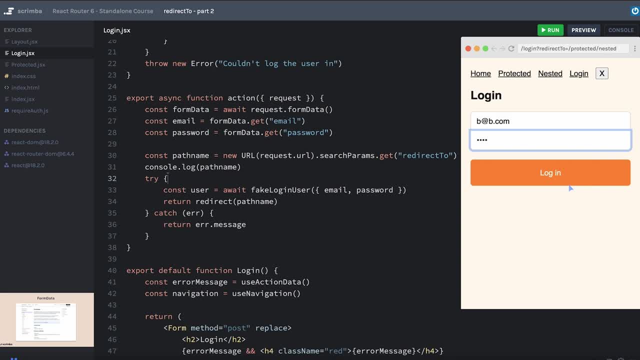 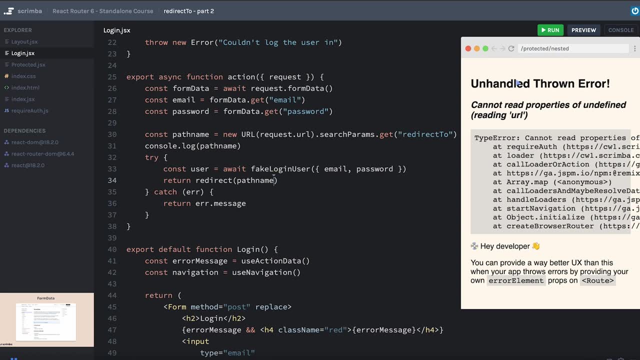 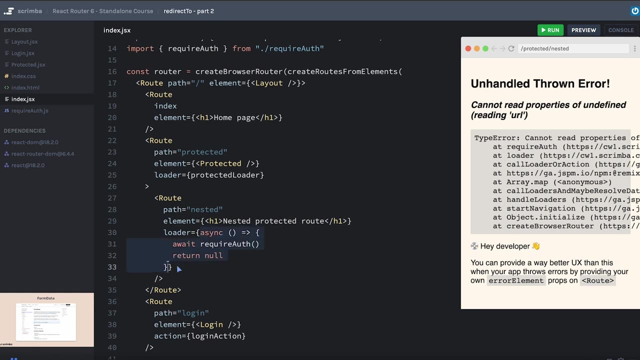 go ahead and log in. b at bcom p123 log in and oh, we were so close. what happened here is our slash protected, slash nested route is running a loader as soon as it loads and we did that in line right here, but we are missing something from this function. can you think of what it might be? 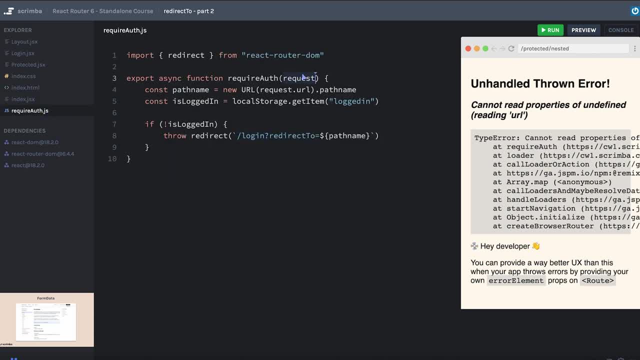 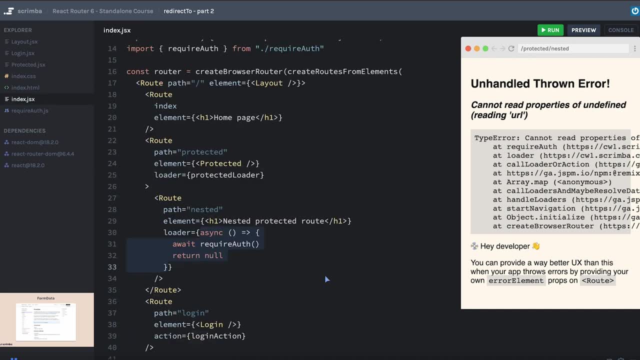 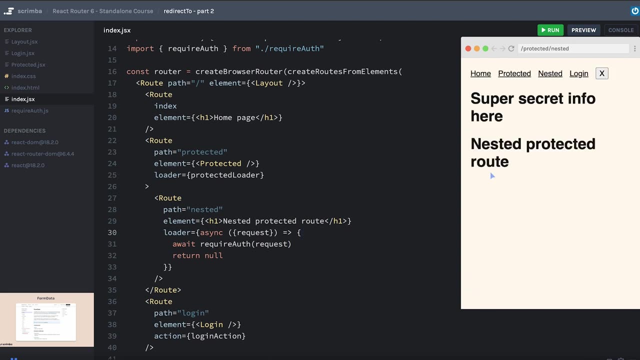 well, we taught our require auth that it will be receiving a request object and we did that inside of our protected loader here, but we did not do that inside of our nested loader. so one thing we could do is just grab the request and pass it along to require auth. that should fix this problem. okay, here we are on the 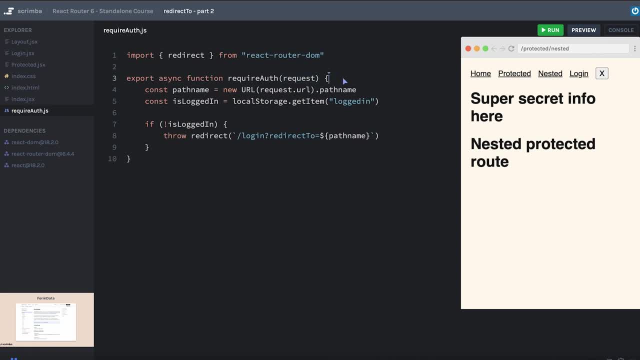 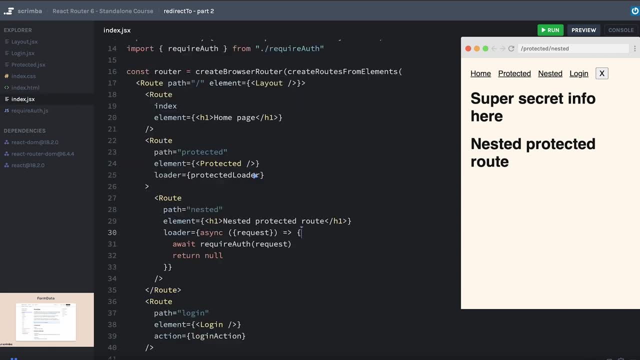 nested route. alternatively, we could go to require auth and make sure it only does this if request exists. i think, since we have it fixed right now just by passing in the request inside of this loader, that's probably going to be good enough for now. actually, now that i think about it, we might 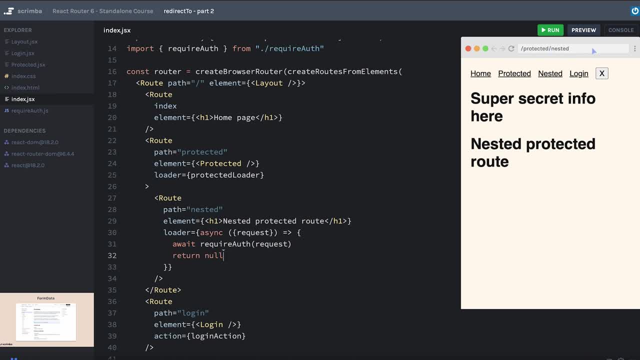 have to do it that way, since we want to be able to redirect back to the nested route. we need to make sure that if the require auth ever gets run here, then it will pass that request through successfully. so it's a good thing we tested that. let's just make sure again. i'll make sure we're logged out. go to the nested route that. 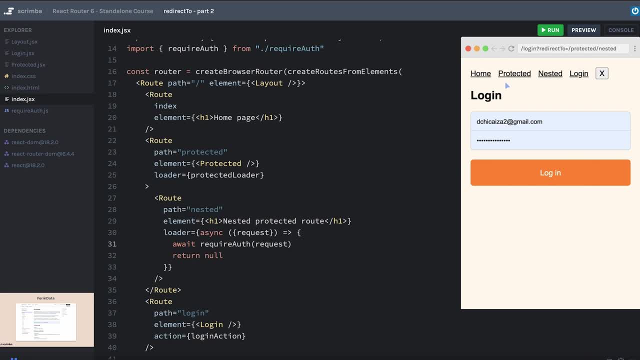 took us to the login page. i guess that was a little hard to see because we were already on the login page. i'll go home and then nested. that takes us to the login page b at bcom p123. and okay, here we are now. one last final thing i'm going to 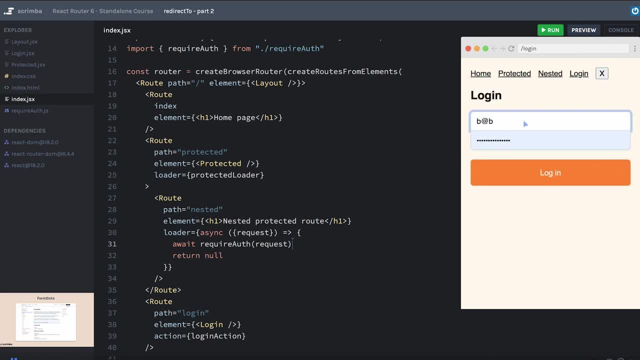 do is log out. go to my login page and log in like normal b at bcom p123. get logging in and we get a problem. it's taking us to slash login, slash null. so this is an interesting one. i think it could be a good exercise if you want to try and see if you. 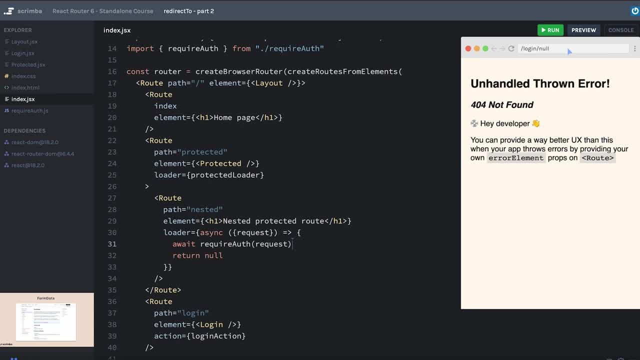 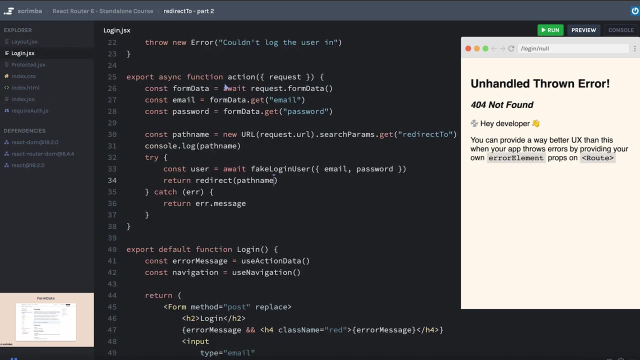 can debug that. you can pause now if you'd like to do that, and then we'll be going through it together, okay, so why is this happening? well, let's go through the regular workflow just to try and debug this in the login page. this action is going to run. 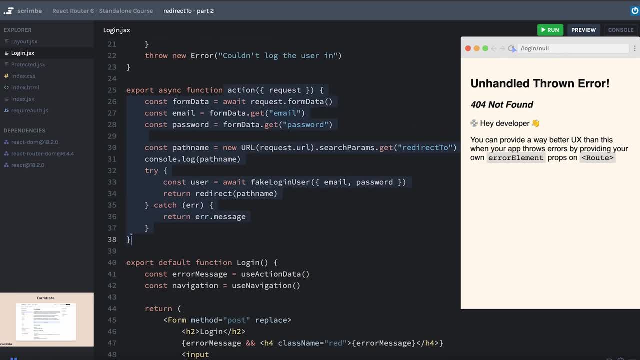 every single time we submit the form, whether we are coming to our login page via another route that we're trying to redirect back to, or if the user actually clicks the login page. when they click the login page, there is no query string for redirect to, which means when this line runs. 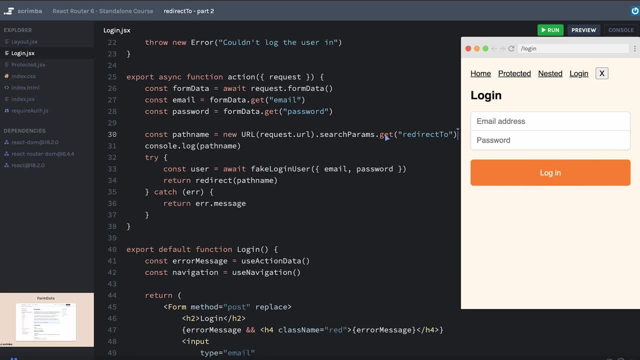 this path name is going to be null because the url does not have a search param, especially not of redirect to it, doesn't have any of that, so we're going to go ahead and do that and we're going to search parameters, and so callingget on something that doesn't exist will return null and then we're. 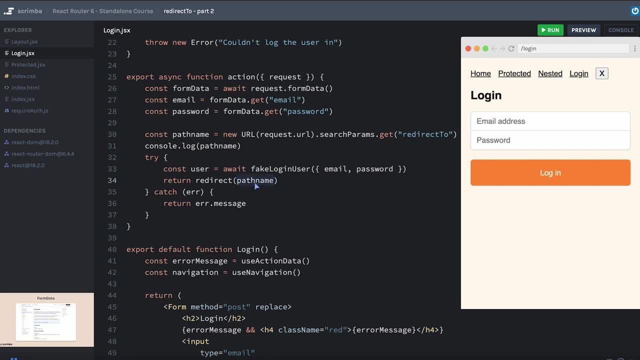 kind of stringifying that when we put it inside of our path name it's going to be null and because it's a relative path, it's not setting it up as slash null. for example, i mean, this would be like a string but it's not slash null, then it's using it as a relative path to the login page, which. 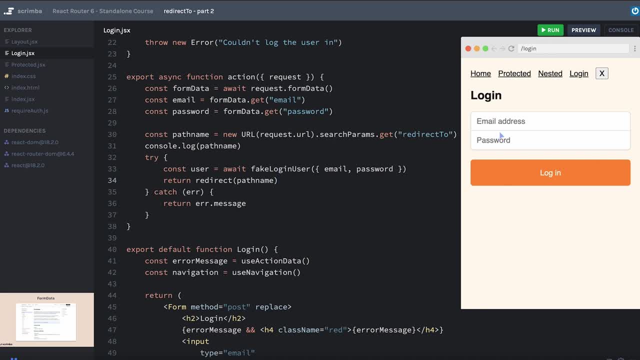 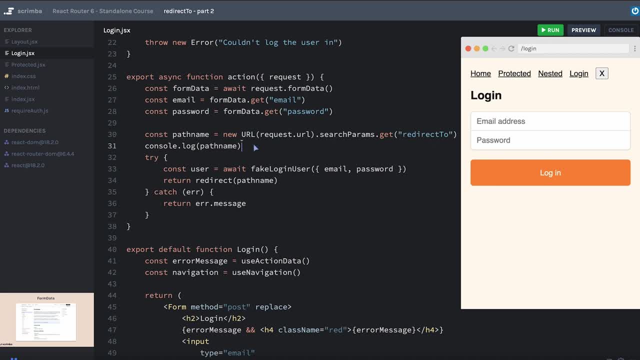 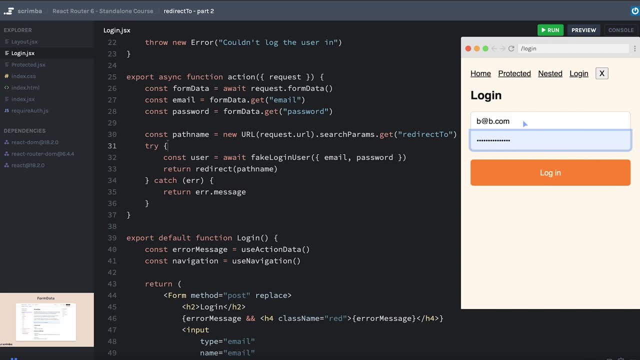 and we're going to go ahead and do that. and we're going to go ahead and do that and we're going to. let's just go to slash protected. so let's try this again. we'll get rid of that. console log. hit save, we're just on the login page. there's no query string there. we'll type in our username and. 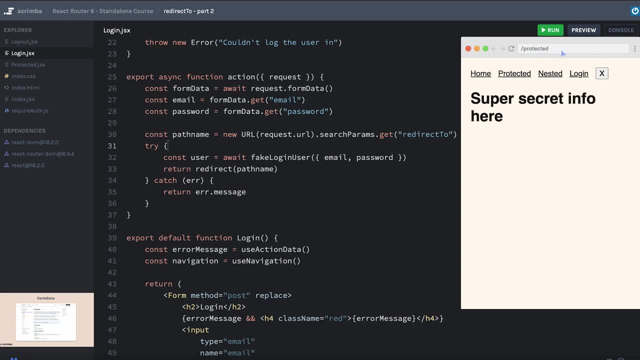 password and great. that took us to the default route of slash protected. and now, if i log out again and try to get to my nested page, log in: perfect. our redirect is working just like it was before. okay, we have covered a ton of ground. let's go back to the van life app and see if we can. 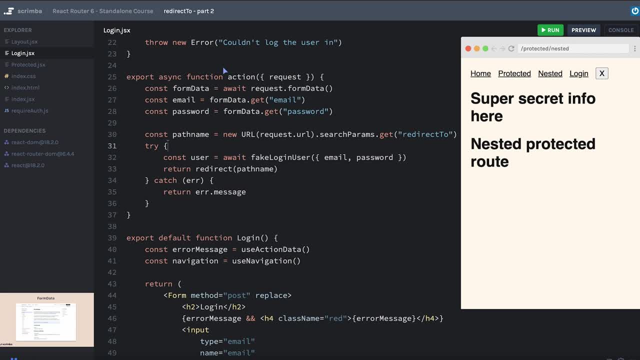 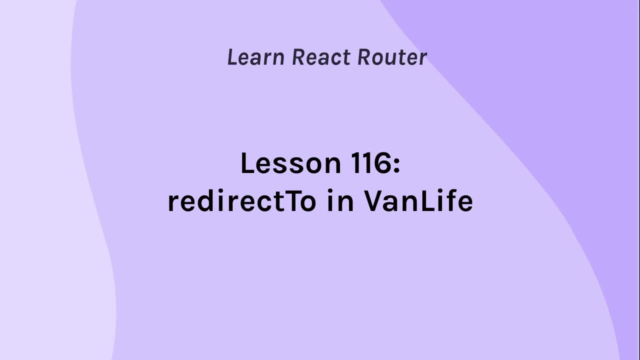 see if you are able to get your hands on the keyboard and complete the challenge of implementing this redirect to pattern that we just did over there in our van life app. okay, your time to shine. your challenge is to implement the redirect to feature, like we just did. 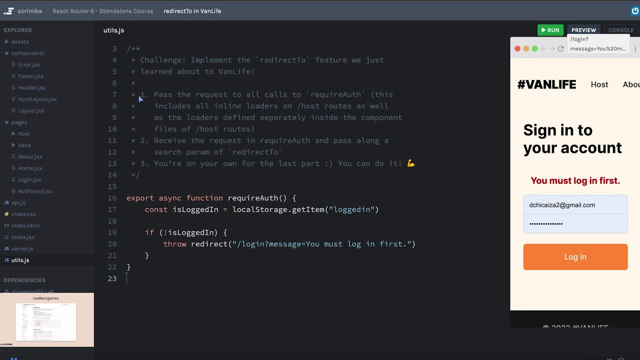 in our practice app, but here in van life i've given you some starter instructions, just since it took us a little while to get there in the last app. this way it can be a bit of a refresher. so make sure you read through numbers one and two really carefully and then for: 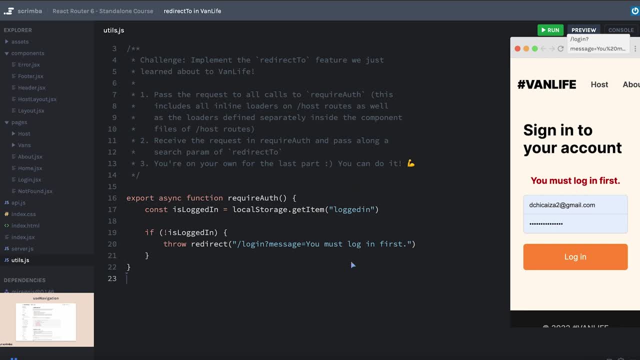 number three. you are on your own for the last part, but i know that you can do it. pause now and work on this challenge. okay, we are going to pass the request. object to every function call for require off. that happens inside of our protected routes, of course, so let's go to. maybe let's start here in our index and 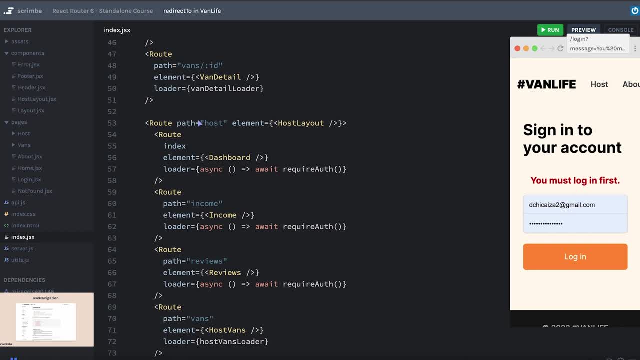 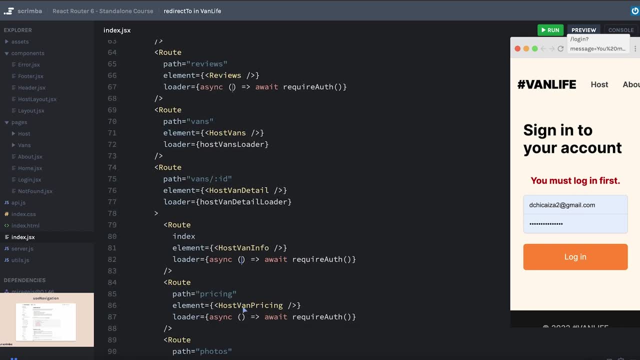 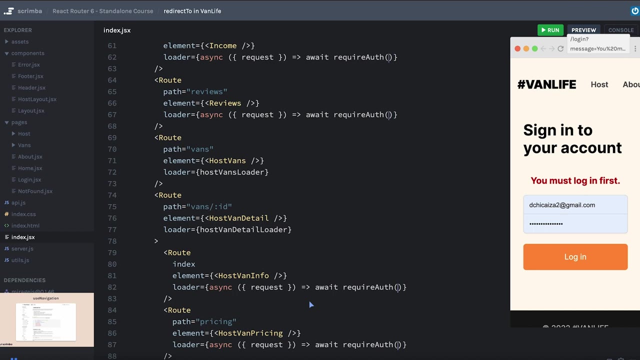 we'll just see all of our inline loaders that we have that are nested inside of this host path. we are going to add the request object here and i think there's more down here- host and info, pricing and photos. so we will go ahead and receive that request object and then we will pass it through to. 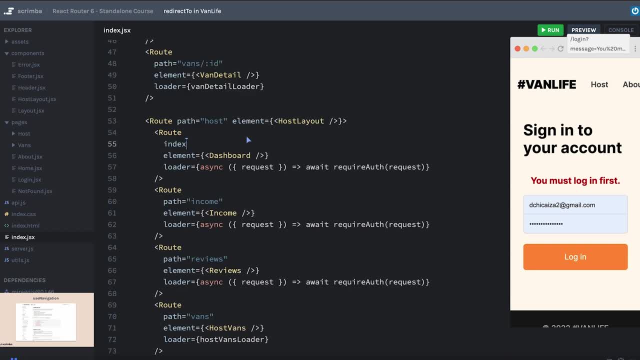 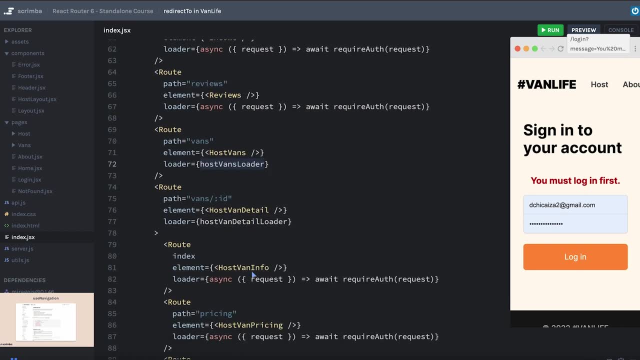 require auth, and then inside of the other loaders that are separately defined, but only the ones that need to be protected with require auth. so that is our host vans loader and our host van detail loader, and i think that's everything. so let's see where are we here? nope, not vans. 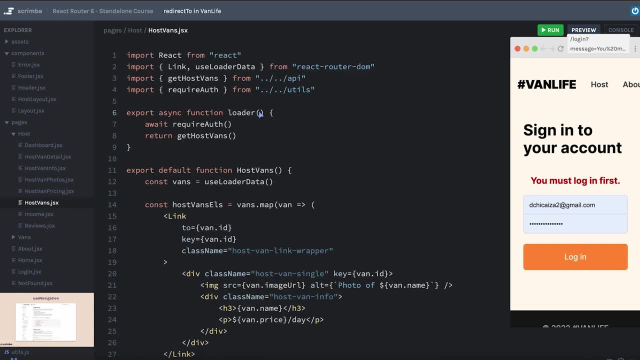 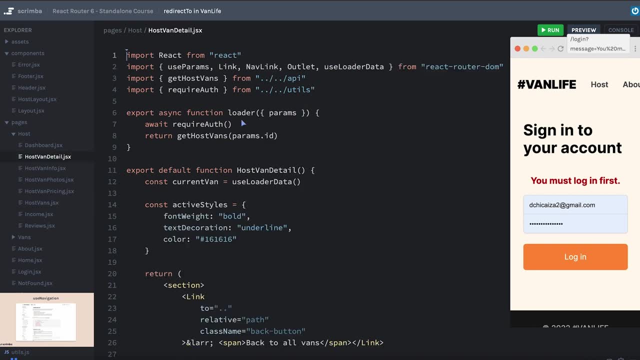 under host: host vans. okay, this loader right here. this needs to receive the request object and pass it to require auth. and then the same for our host van detail. we're already receiving params, so we will just also pull in request, pass it to require auth. okay, that is a good start, let's go to require. 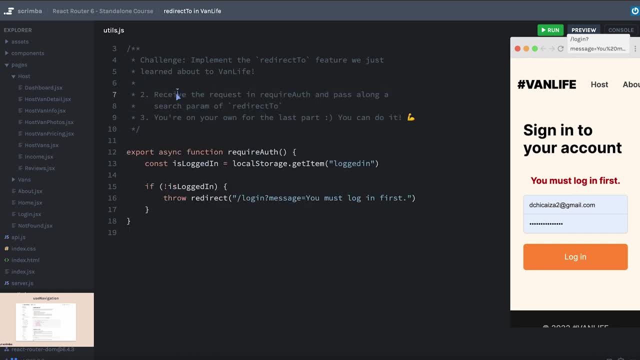 auth and that should be everything for one. we'll go ahead and clear that out. then require auth is going to receive the request. we'll. we'll remove thebstrc for this one. we're going to leave it as it is and we're going to let it. 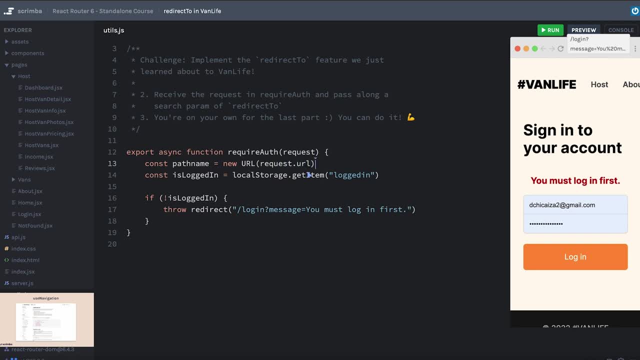 just be the datamask which should deliver the request object to the host. so we'll leave that out as well. all right, and we're going to run the path name and then here we'll say we want to construct a url. actually, we can just do it all in one. we'll say the const path name is equal to new. 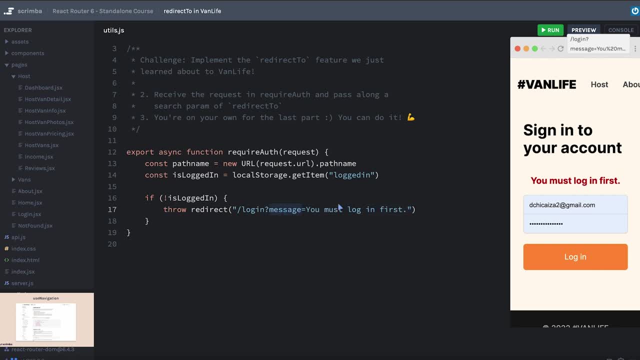 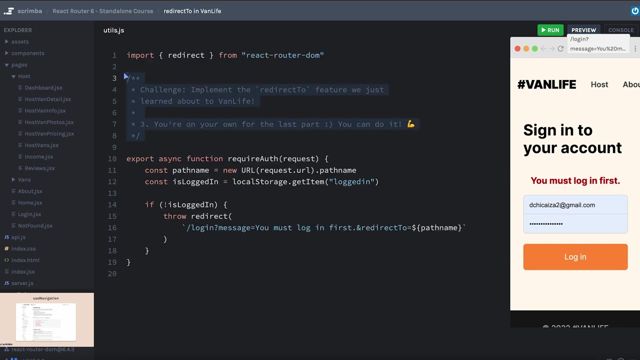 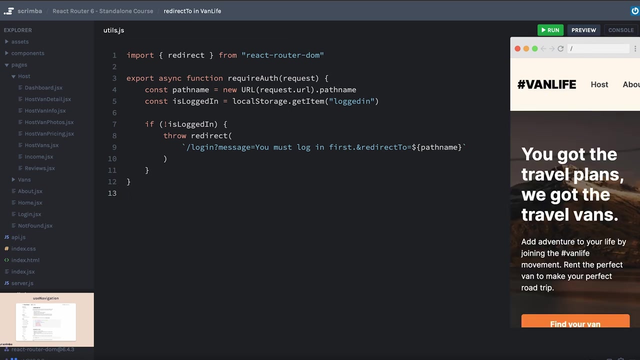 url request: dot url, and then we'll use dot path name to grab the path name that the app was trying to get to when we were first trying to get to the protected route without being logged in. okay, and in strings, And I'll just put this on this online so that it can be a little easier to use, And we will add in with an ampersand, we'll say: and redirect to equals, and then we'll pull in our path name. Okay, so this alone we should be able to test. Let's clear this out, And since we're on our own for the last part, we'll clear out the rest of this challenge. Let's hit save, Okay, and then I'll make sure I'm logged out. I'll go, maybe, to the homepage and then I'll go to host. 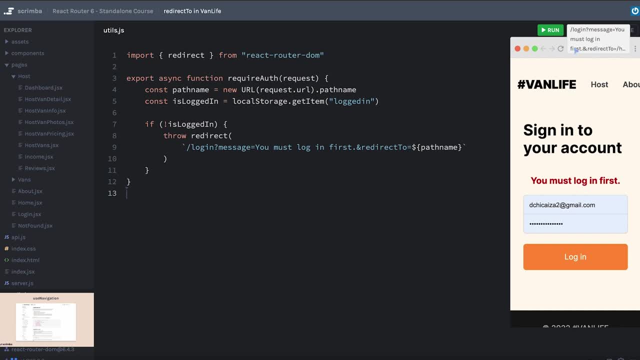 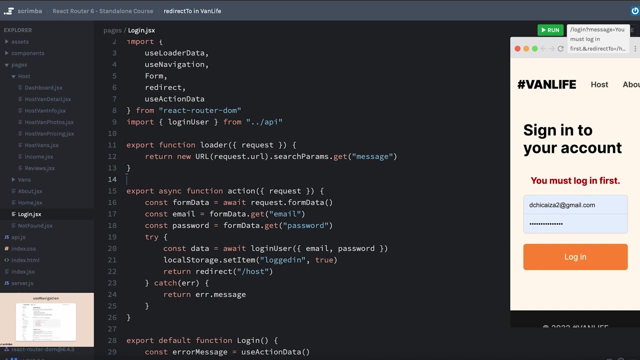 Okay, and if we look closely, we have the whole thing up there. we have slash login question mark message: equals. you must log in first and redirect to equals slash host- Perfect. Now for the last part. we need to go to our login page, receive the search params so that we have access to this redirect to in the URL and then use that as our value for slash host, or rather in place of the hard coded slash host that we have here. So actually we already have up here where we are grabbing the search param for message, So I'm just going to copy. 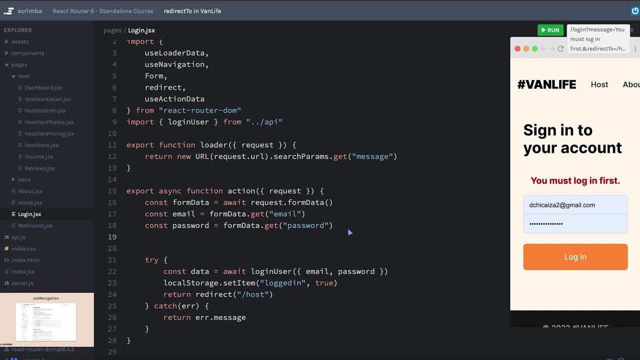 this, because I guess I'm a cheater- And right here we will say that our path name is equal to, and then I'll just paste that in but change this to redirect to, since that's the key that we're trying to get the value from, And maybe I will put this on its own line, just in case that's getting a little wide for anybody. And I'm going to have a default of slash host. That way, if someone is coming through the regular login workflow, where they actually manually go to slash login, we're not going to get null in its place. 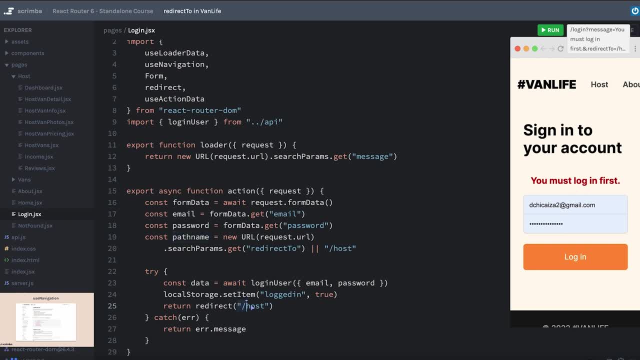 Okay, so we'll take this path name And that is where we are going to redirect to. Let's hit save. We will log in. b at pcom, p 123.. Okay, so that took us to slash host. That's where we had been trying to get to before I'm going to go somewhere more deeply nested. Let's go to vans, maybe one. we're going to log out and then try to get to pricing. Okay, great, We can see in the URL: redirect to equals, slash host, slash vans, slash one, slash pricing. 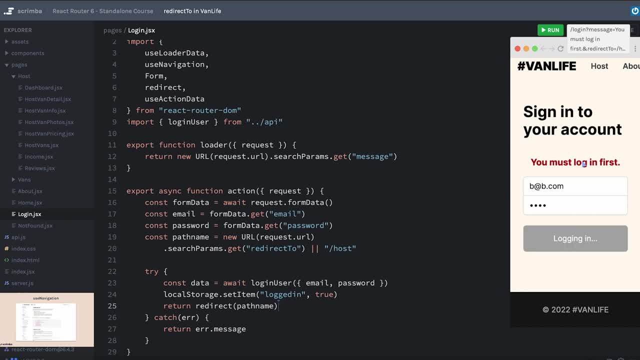 Let's go ahead and log in again. p 123. Enter, And here we are: Perfect, Great work. I know that may have been a challenge, especially that last part, since I kind of took the training wheels off and let you ride on your own. If you did struggle with it and you had to watch me do it, that's completely okay. But now is the perfect time to scrub back and to try the challenge again, maybe from the very beginning, all by yourself. Great work, and I'll see you in the next scrim. 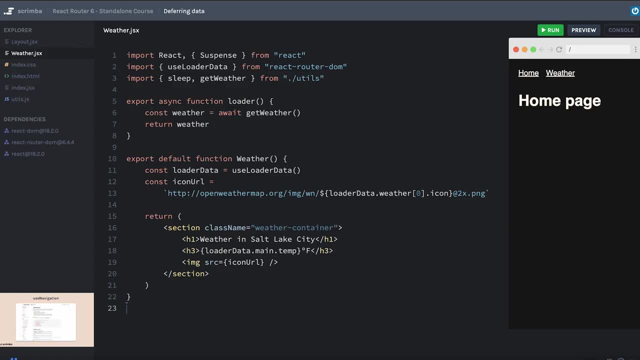 At this point in this course we are really going to be talking about how to get to the next scrim. We are really rounding the corner on the final topics that we're going to learn about react router, And at this point we are starting to venture into some more advanced territory. It's nothing to be worried about. we're going to go step by step so that we can understand everything we're learning. But it also will touch on a couple topics in react- not react router, but core parts of react that you may or may not be familiar with. I'll try to give a bit of an overview of them, But we won't be diving deep into those topics. specifically the topic of suspense, the motivation for what we are doing. But I'll try to give a bit of an overview of them. And I'll try to give a bit of an overview of them, But we won't be diving deep into those topics, specifically the topic of suspense, the motivation for what we are doing. But we won't be diving deep into those topics, specifically the topic of suspense, the motivation for what we are doing. 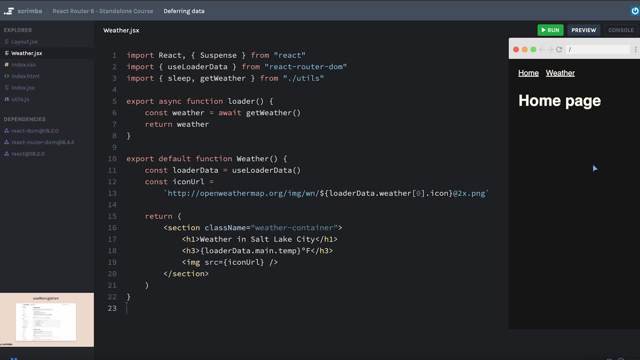 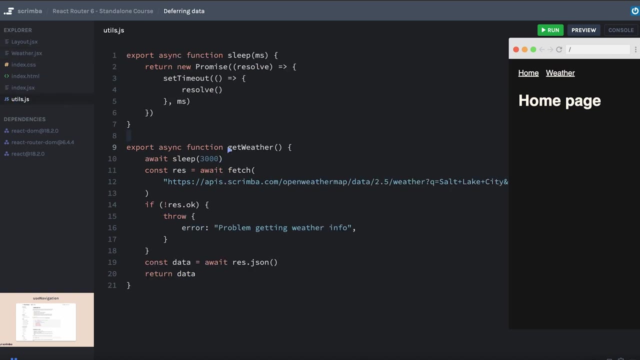 can be seen here in this little weather app that I created, clicking on the weather link, which I'll do in just a second- we'll get the weather for the current location where I'm recording this, And the API is actually not very slow. So what I've done in the utilities JS, where I'm creating this get weather function, I've added a three second pause just to make it so that it's as if getting the weather took a bit longer than it actually does, And this is really to highlight one of the things that you certainly noticed when we first entered the app. 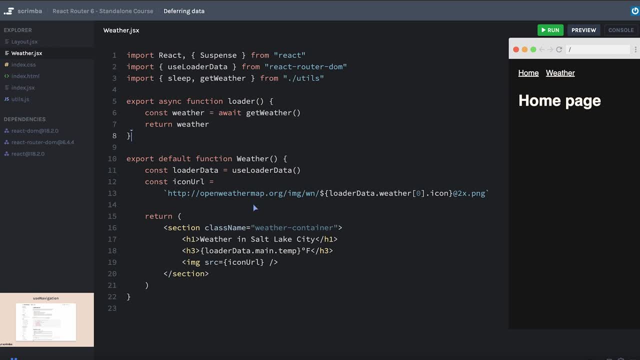 introduced the idea of a loader. See, the benefit of a loader is that we can write our code as if the data always exists at the time of rendering this component. For example, I can say that loader data is equal to use loader data And I don't have to do optional chaining or any kind of ternary check to make sure that loader data exists at the time this is being rendered. Otherwise, I could get some kinds of errors for trying to access the property main of undefined, for example. that is a nice benefit, But you might remember. 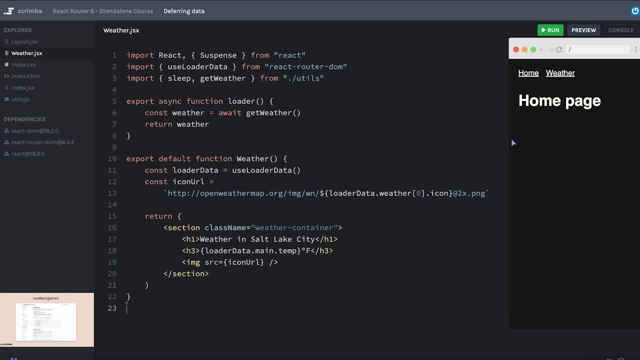 from van life. when we first implemented the ability to go to the vans page and load up the vans, we used react state to show that we were currently loading the vans and we had a nice little loading message so that the user, when they click the link, would immediately go to that page and be informed that the vans are loading. When we switched to using a loader- because it does the fetching before the component renders- there's quite a bit of a pause before you switch to the next route. So here if I click weather I will click it right. 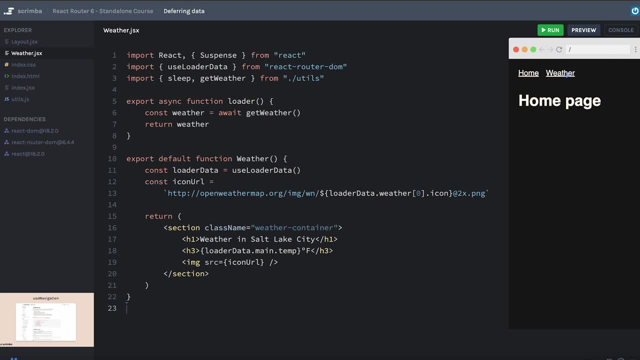 now, Three seconds feels like an eternity, especially when you're not navigated anywhere and it doesn't feel like anything really happened. So on the developer side, we get some nice benefits by knowing that our weather component will only load after the data has been fetched and is ready. 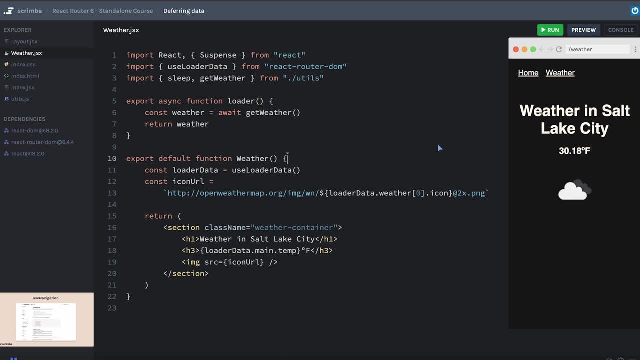 for display, But on the user side we have a bit of a worse experience. So over the next few lessons we're going to be learning about using deferred data. this is going to give us a chance to bring back that user experience where clicking the link on a route that needs to fetch data. 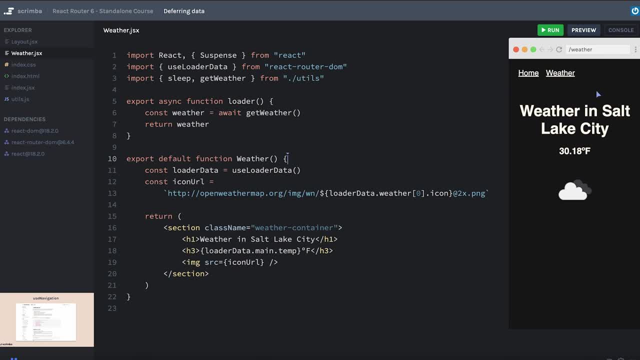 will transition us to that route immediately, And it will give us a nice API that allows us to render some kind of loading state in the meantime, all of which we will be able to do without creating any of our own manual react state. So buckle up and get ready to dive into world of 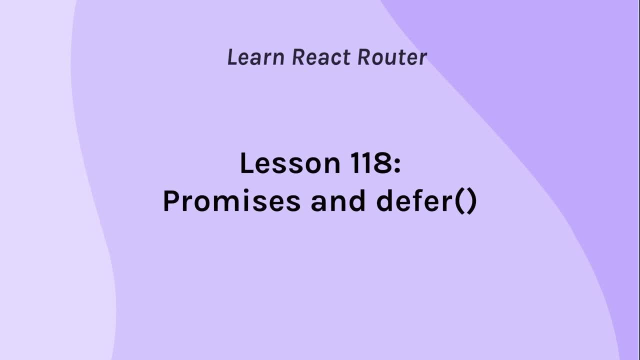 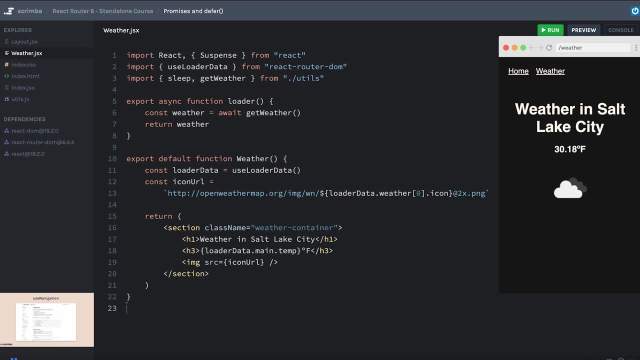 deferred data. It's probably safe to assume that some of you watching this might be a little bit hazy on your understanding of promises and how promises work. I won't have time to dive deep into promises, But one thing that I wanted us to remember is that when a 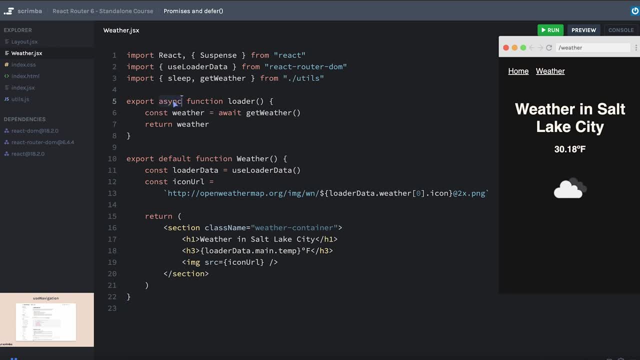 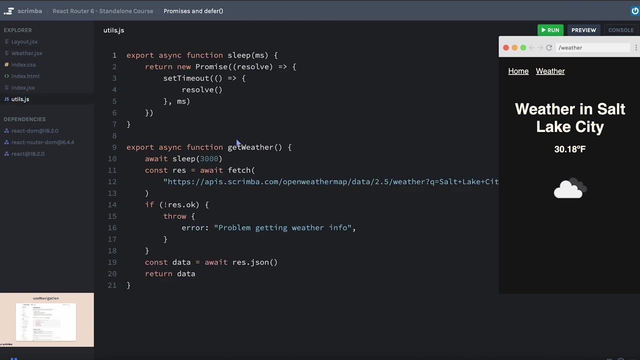 function is an async function, it will always return a promise. So when I say a weight get weather, that's an indication to me that get weather returns a promise, because a weight can only be used on a function that is returning a promise. If I go over to my utils js we can see. 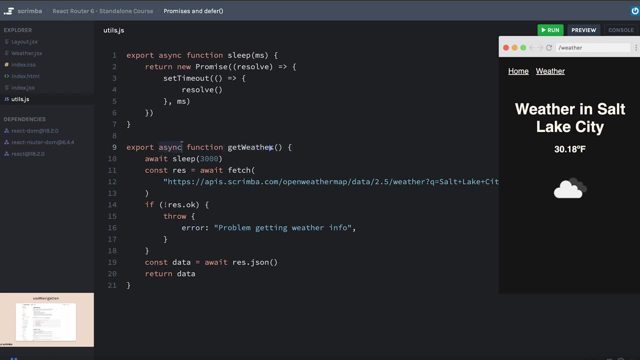 that get weather returns a promise. So when I say await, get weather returns a promise, get weather is an async function and therefore it is always returning a promise. When we say return data, what's really happening under the hood is we are returning a promise that, if it's, 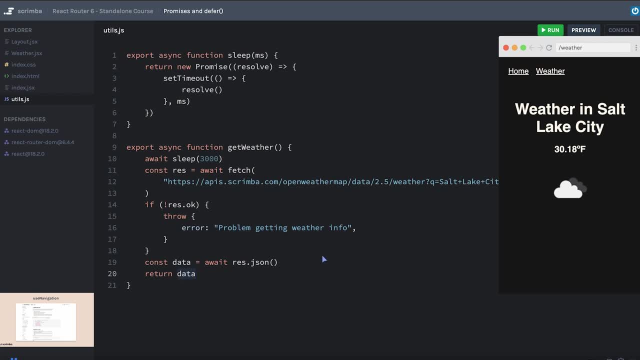 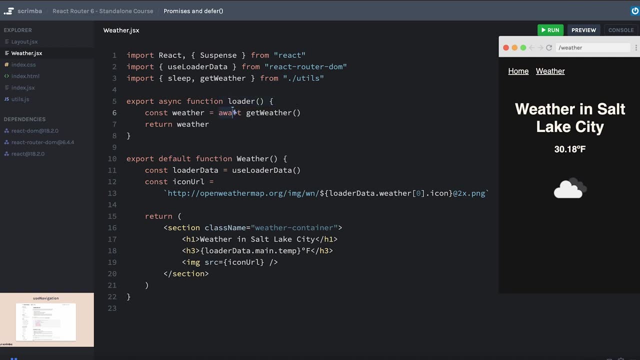 resolved, we'll return data. it's not important that you have that perfectly memorized or understood. The point that I'm trying to make is that when we have our loader function and we are calling a weight get weather, what's happening here is we are waiting for the get weather call. 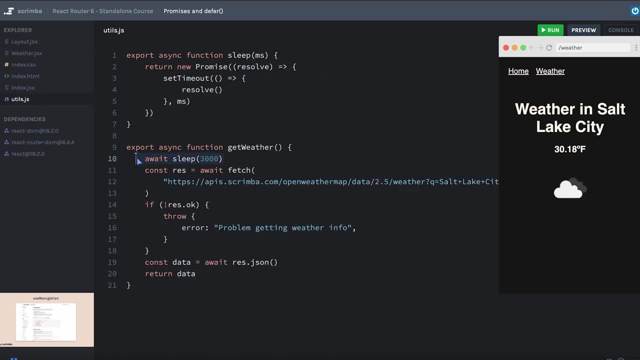 to finish, And remember: get weather is sleeping for three full seconds. So we're waiting for the get weather call to finish, And remember get weather is sleeping for three full seconds before it even executes the fetch request And then, naturally, the fetch request is going to take. 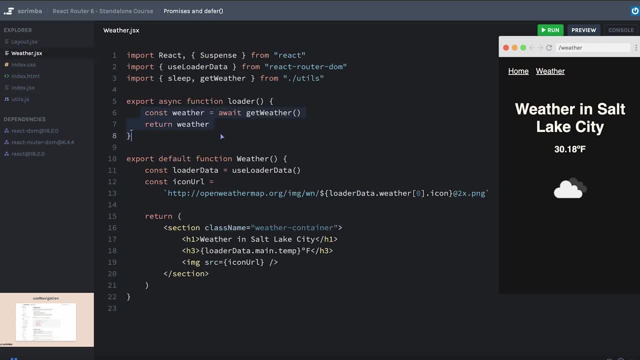 some time to complete as well. And with loaders, the code inside of my loader needs to complete before the component will ever get rendered by react. That's beneficial to us because we know here that loader data will be accessible to us no matter what, unless, of course, there's some kind 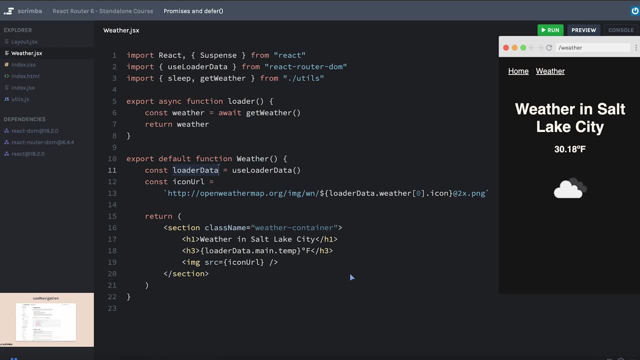 of error, in which case this component shouldn't get rendered anyway. it will have some kind of error element that gets rendered instead, But in order for us to be able to get the get weather to bring back the benefits of switching to the route immediately, before ever kicking off the. 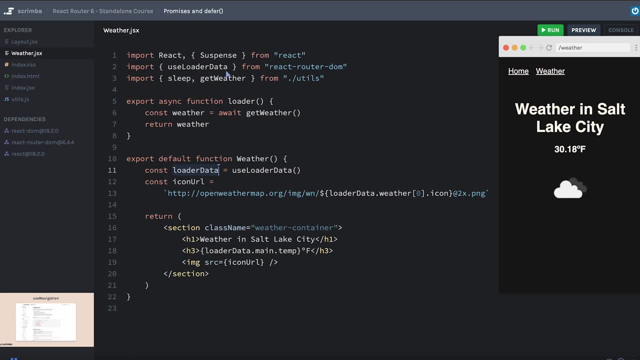 request in our loader function. we need to use a utility that comes from react router DOM called defer. the entire process that we're about to go through starts with react router, knowing that its loader function is allowed to wait or defer the loading of our weather data to a later point. 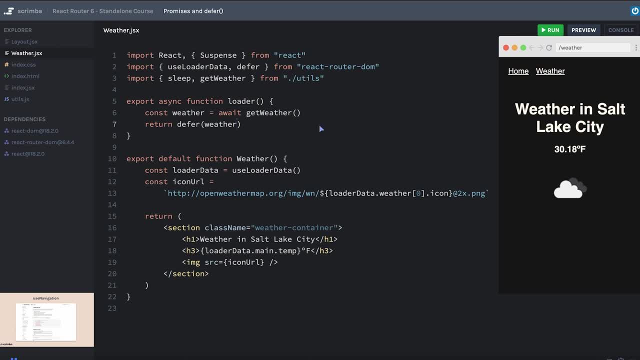 and therefore will not block the user interface from loading Or, more specifically, it will not stop the weather component from being rendered before the data is completely gathered from the get weather function. Now we're not quite done yet, because weather is still the actual. 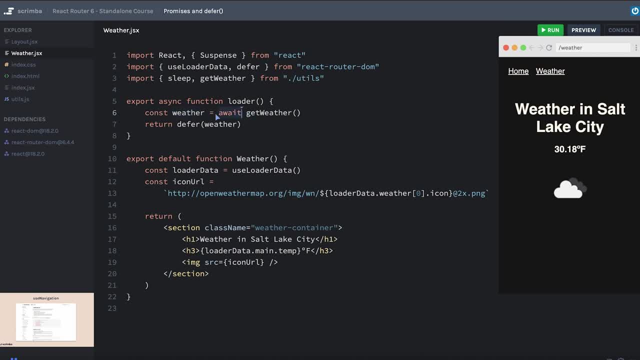 value because I'm using this await keyword which is pausing execution of my loader function. So I need to get rid of a weight which means that weather is no longer the actual resolved data from get weather. I want you to pause for a second and think. what kind of construct in JavaScript is this? 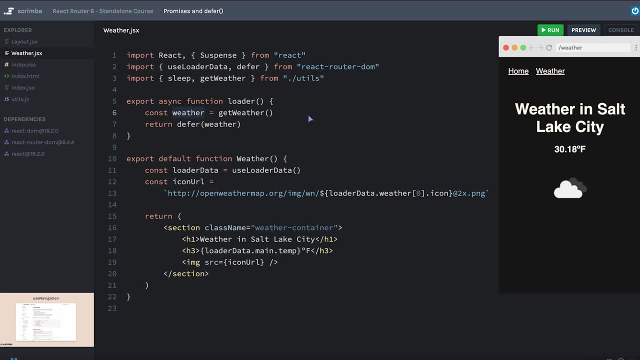 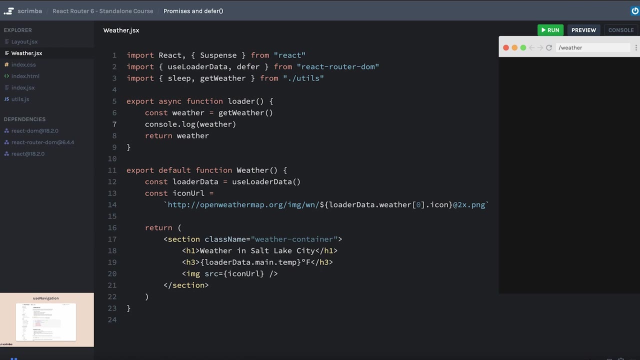 I'm going to remove my defer right here And we'll probably get some errors here, But let's give it a shot and see if at least- Okay good, We can see that weather is not the actual weather. Instead it's a. 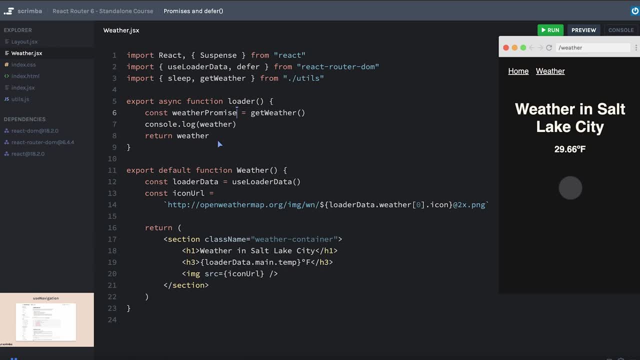 promise object. So just for clarity, I'm going to rename this weather promise. now that we've gotten rid of a weight there, we can get rid of our console log And let's bring back our defer call. Now, what defer expects is an object, And the key of that object is what I want to call the data that 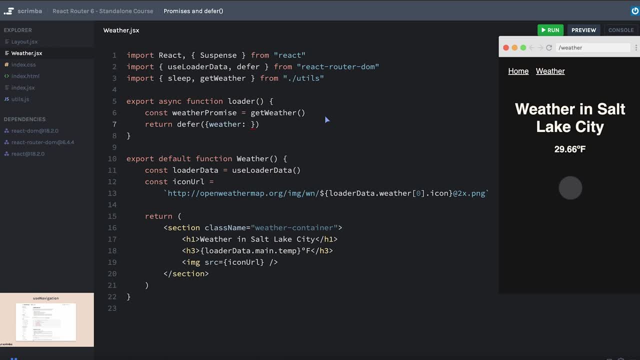 eventually will get resolved, whenever the promise gets resolved, And I'm going to pass to it the promise that eventually needs to get resolved and become the weather data that will get passed down to my use loader data. I understand that we jumped around a bit, So I'm going to 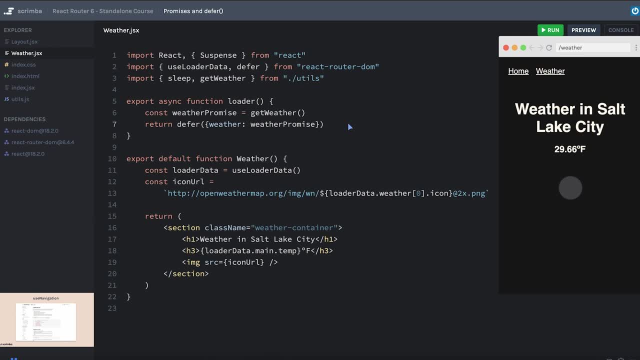 undo everything and just show you that we actually haven't changed all that much. Okay, this is where we were before. we needed to import defer. we're going to remove our await forget weather, which means that this is not really the weather. it's a promise to get the weather. then we're going to call defer. 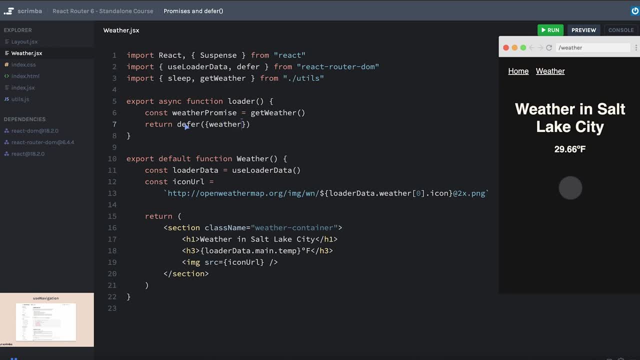 pass to it an object, give it a key of whatever we want to call the data that we are deferring till later, and then pass to it the promise that it should work on resolving for us and putting at this part in the object that's coming to. 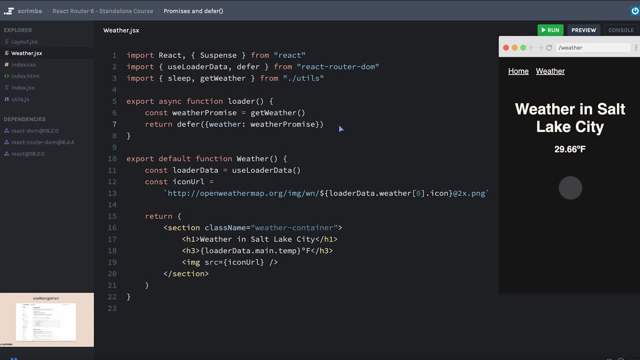 other data. The tricky thing about learning this- and partly why I call this an advanced topic- is because there's quite a bit to put together before any of it will work. So for the sake of practice, I'm going to once again undo everything and have you type this out again. So if you need to take a 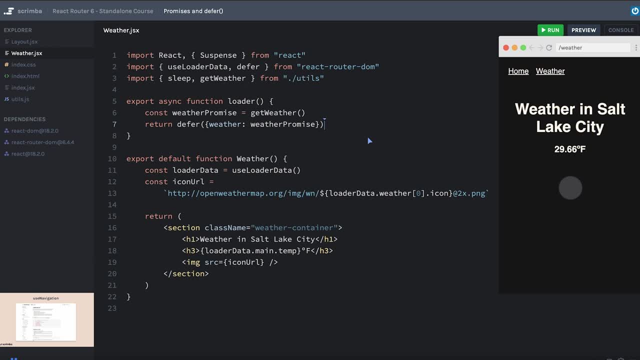 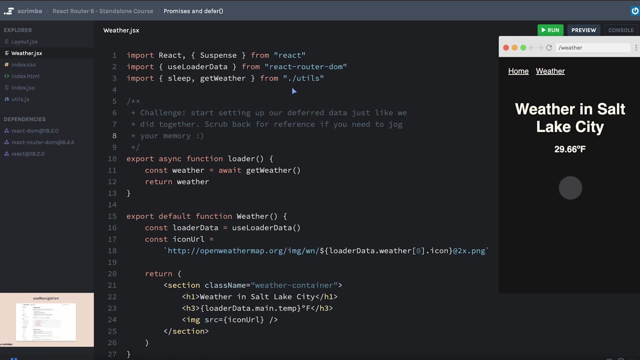 look at what we just typed in again. try to commit it to memory, because you're going to be typing it in just a second. Okay, let's do it one more time. Start setting up our deferred data, just like we did together, And, of course, you can scrub back for a 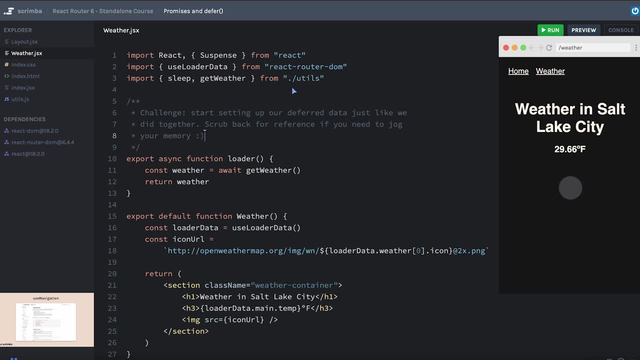 reference if you need to jog your memory Again. the tricky part is we're not quite ready to have this actually work for us, So you're just going to have to try and do it from memory. Pause now and work on the challenge. 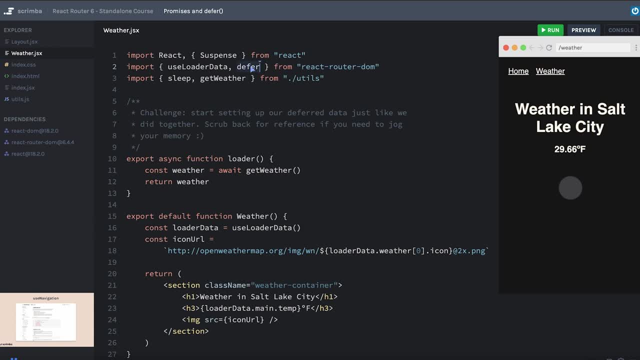 Okay, let's start up here again. we're going to pull in this defer utility, get rid of a weight you will call defer. we're going to pass an object where the key is what we want to call the data when it gets. 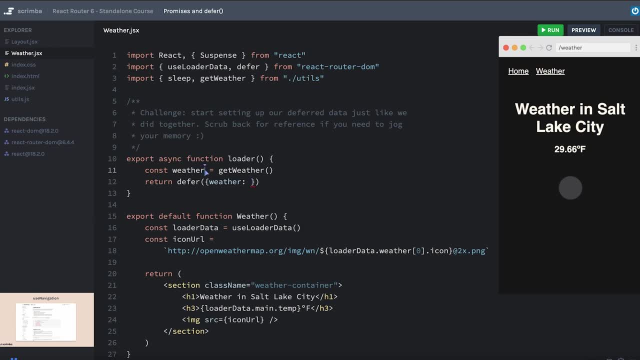 pulled into use loader data, And the value is the promise, So let's call this weather promise. This part is not strictly required. it just makes it a lot easier for another developer to understand what's going on here, And we'll pass this in Now. of course, we could gain some shorthand benefits. 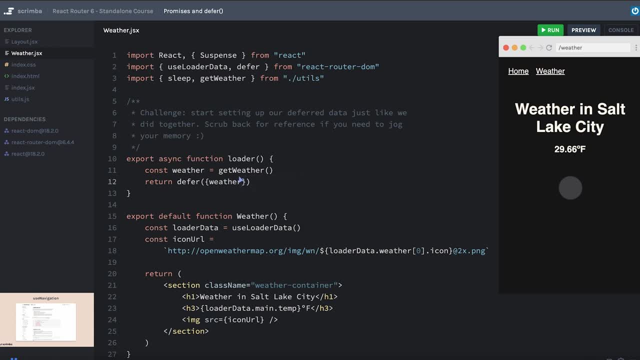 if we just kept this as weather, because I could then just say weather. But for the sake of learning, we'll do this Again. I don't have a great way to test this yet, because we have quite a bit more work to do down in our 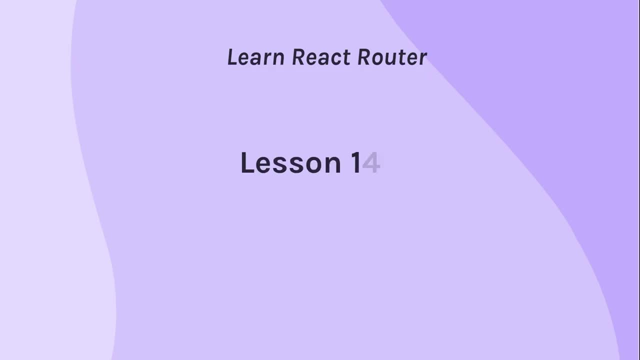 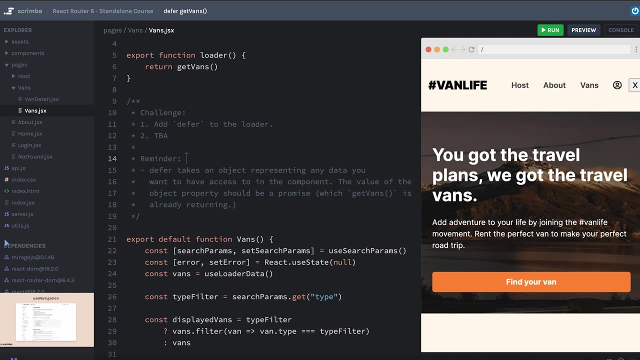 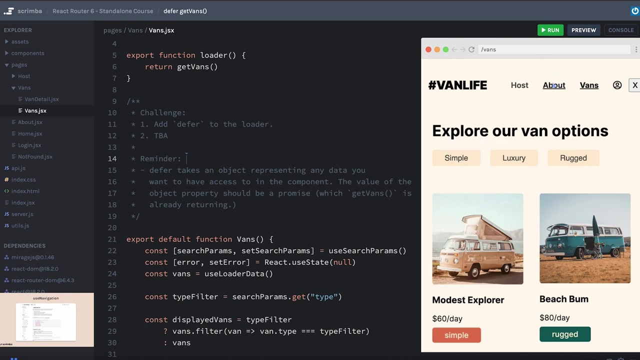 component. So that's what we'll be jumping into next. Okay, let's add defer to the loader of our vans route. I added another one second delay on our server, So when I click the vans we can see that it does take a little bit of time to get over there. In the end, I think it's. 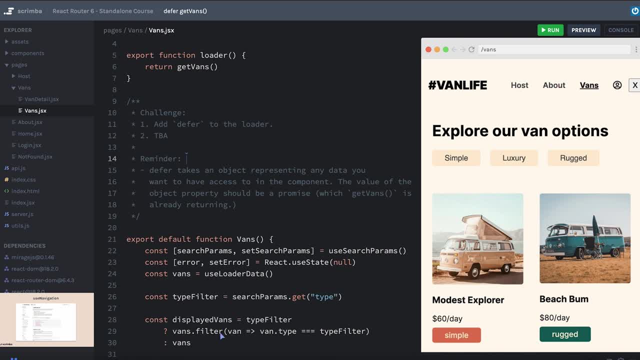 important to remember that. it's just a trade off that you have. you can simplify your developer experience and also parallelize the loader. And I also have a quick question for you, that is, is it going to be able to minimize all of the loaders, so any nested? 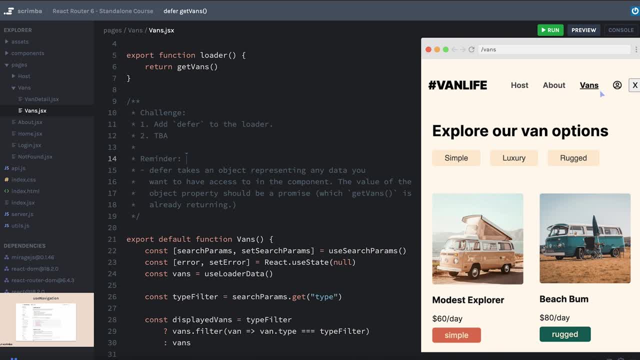 resources can be more easily retrieved And as we get closer to adding for a wait and suspense, we're going to see that we can bring back some of the snappiness that we got when we first started using React Router. That way, when we click the vans, 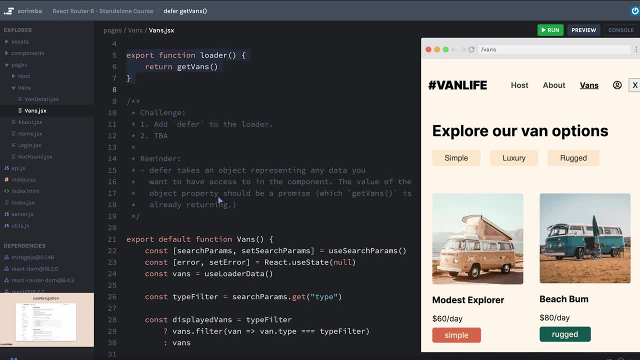 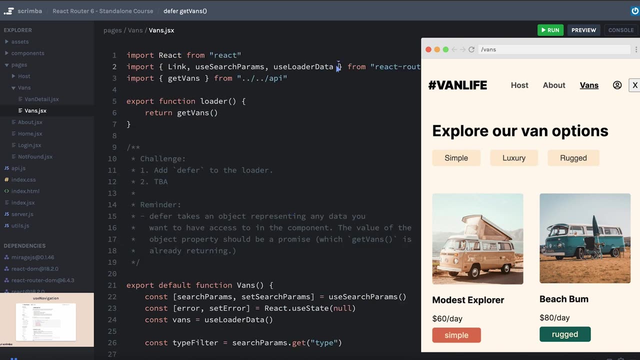 to add defer to our loader, which is up here, and then there will be more to the challenge later. i have a quick reminder here, in case that is helpful. so pause now and work on the challenge. okay, let's go ahead and import defer from react router. i'll put these on their own lines. 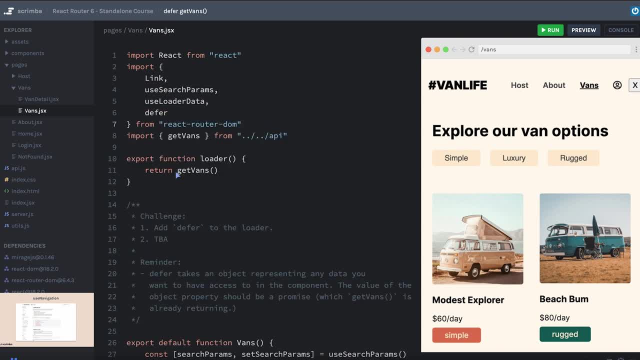 just to make it a little easier to read. okay, and now i can return a call to defer. we'll wrap our get vans. get vans is going to return a promise. notice that this is not set up as an async function and we're not using the await keyword. so get vans is going to return a promise, just because. 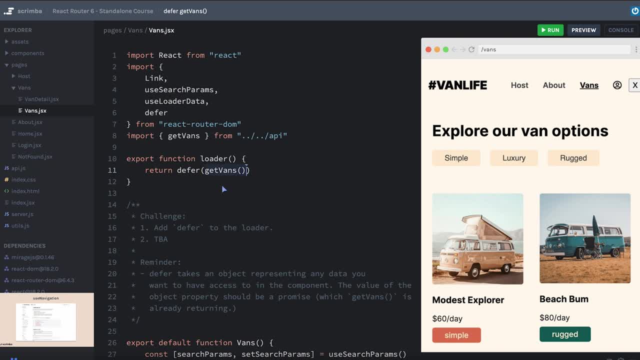 that's what it does in the api file and i need to wrap this in an object and we'll call the value that is going to be resolved. maybe vans like this. okay, short and sweet, as i mentioned, we still have some steps to take in order for this all to work together. so let's go back, learn a little bit more. 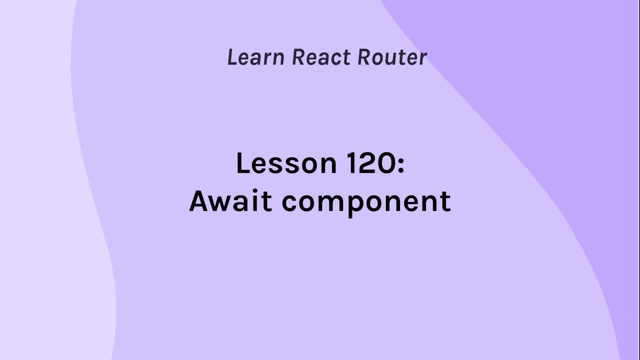 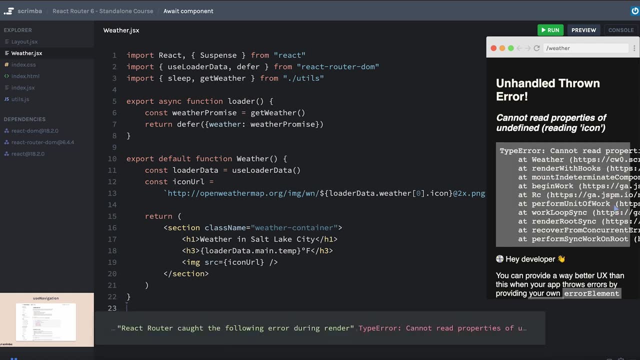 and then we'll come back to that in a minute. so let's go ahead, and go ahead, and go ahead, and here to van life, if we try to get to our weather page now, we'll see that, well, we are broken and that's because the protection that we had before, where we could be certain that our loader data would be defined and 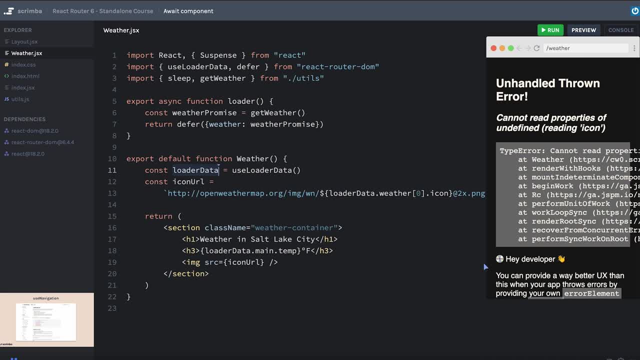 ready for us to use when our weather component was mounted is no longer the case, and that's because we are allowing the loader to defer for a later time and we're no longer awaiting our get weather call. so the next piece in the puzzle is to use a component from react router called await. await does a few different things. 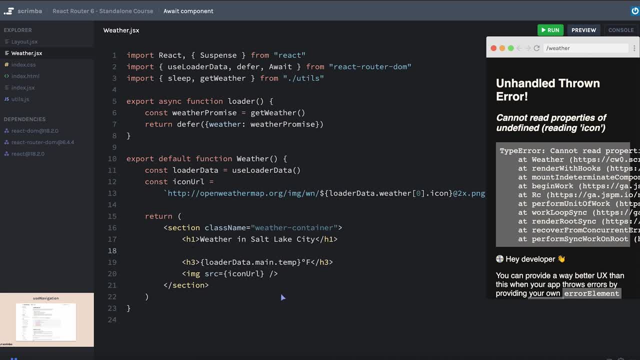 first of all, it allows us to surround the code that we will be waiting for when this component first renders, and it will conditionally render only after the data has finished loading. it'll make a little more sense if we just do it, so i will put in my await component and this will 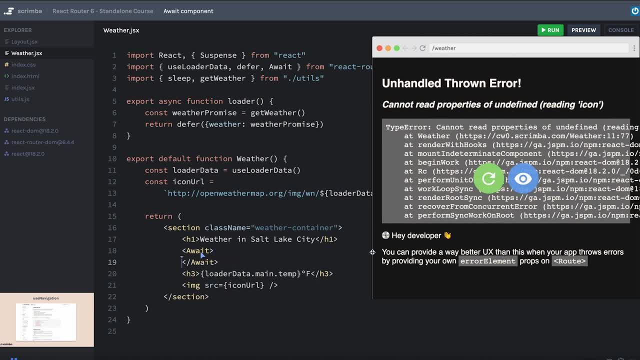 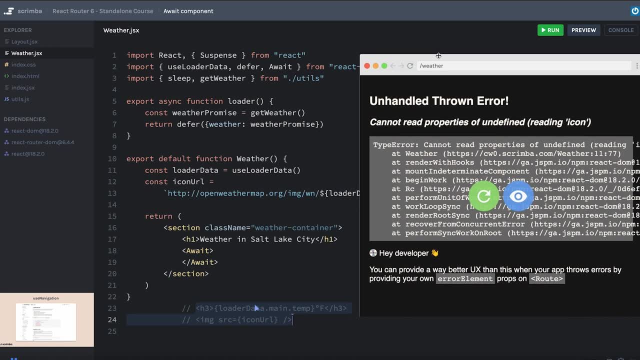 not be a self-closing but instead will take some children, and i'm going to move this h3 and this image out and just comment it out for now. we'll bring it back in just a minute and there's two major parts to the await keyword that we need to use. the first one is a prop called 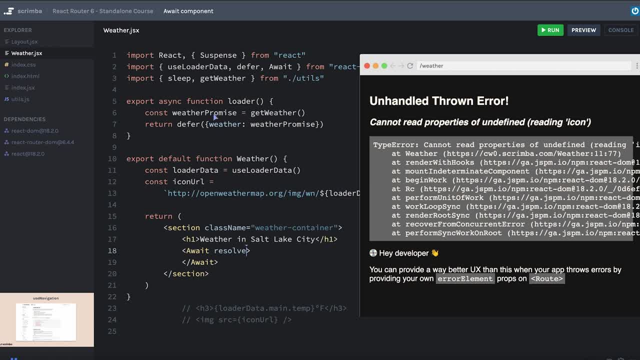 resolve. our job is to pass the promise for the data that we're trying to get to this resolve prop, and i want you to think for a second: where am i going to get this promise from? well, up above, we are returning this object that has a weather property. we're pulling in loader data, kind of. like we had before, except before the change, and we're just going to go ahead and recheck. thiscker is called expected weather property buy up to the object isper 1917. we're pulling in this express title, kind of like we had before, except before. it's not it'saha facing ovst and, as you can see, it'sa. 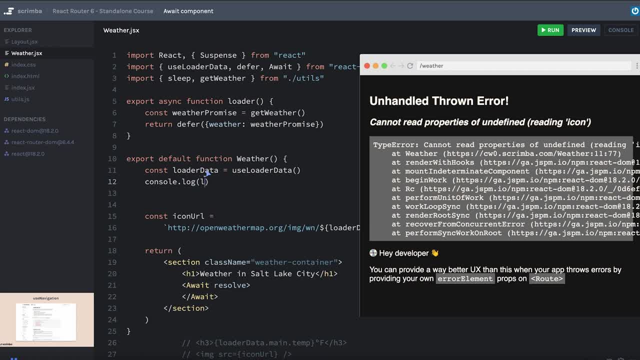 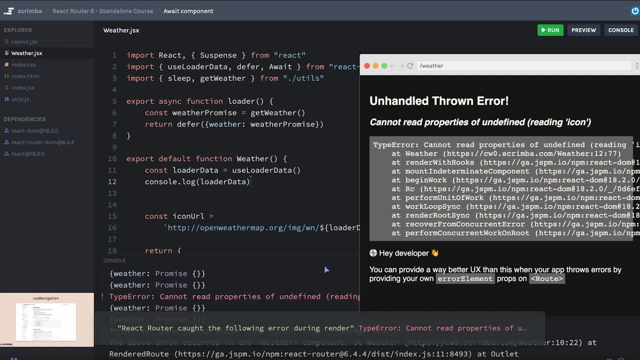 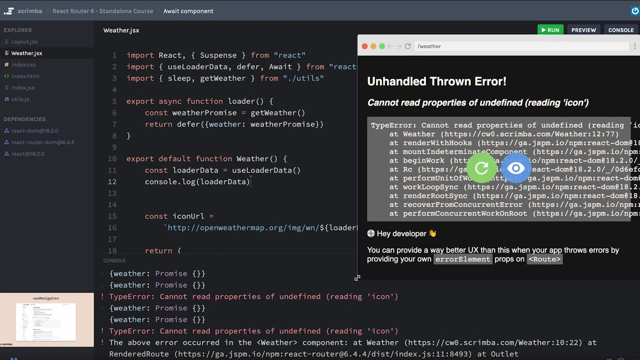 four, it was the actual data. Let's go ahead and console log loader data And we might still have this unhandled error thrown, But let's see if it logged that to the console. Okay, loader data is an object that has a weather property whose value is a promise, So that's the promise that we need. 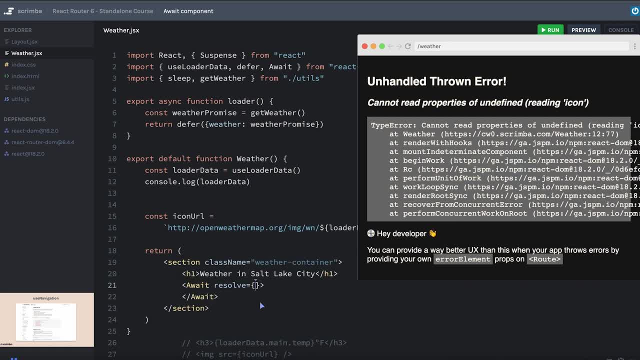 to pass to resolve. In other words, we give our promise to this await component. I'll call it loader data dot weather And under the hood, the await component will take that promise And, after it has been successfully resolved, it will call a render prop child function. 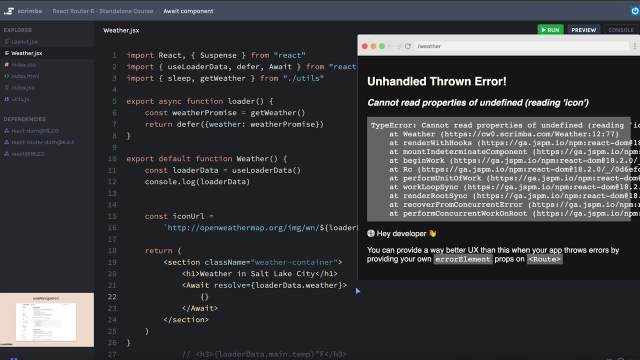 Earlier in the course, when we were talking about dynamic class names with the nav link component from react router, I mentioned that if you are taking this react router course as a part of my larger advanced react course, we will have already talked in detail about render prop. 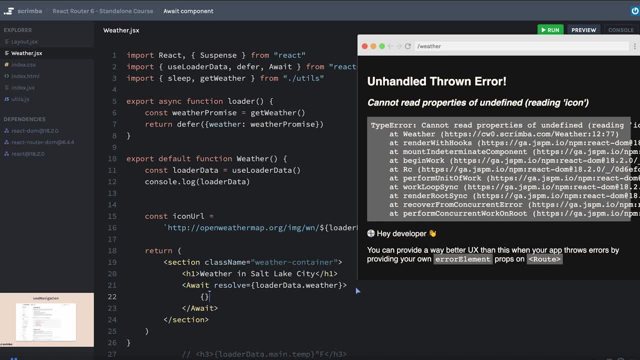 And how they work. If you're taking this as a standalone course, you may or may not be familiar with the concept of render props, But as a quick high level overview, I can pass a child to a component, And that child doesn't necessarily have to be another component. We're very used to having 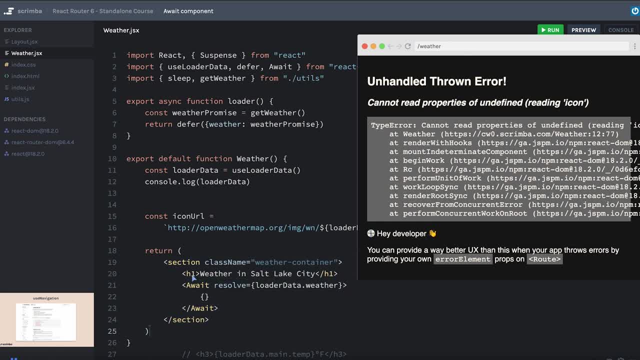 parent child relationships with our HTML or our JSX elements, like we have already here. But when I have a custom component, I don't necessarily have to pass another JSX elements as the child to my component. Instead I could pass a function, for example, and the code of that component could take that function. 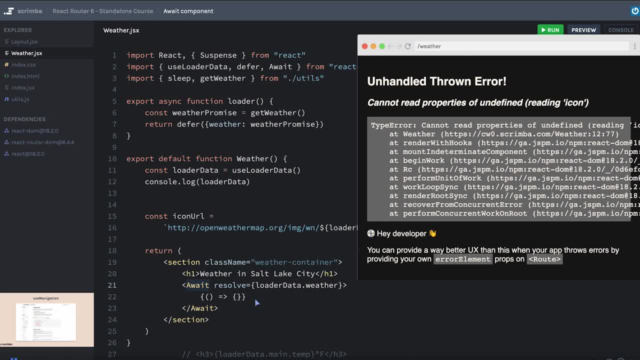 and run it, passing any arguments to it that it wants to. That was a really quick rundown of render props and probably didn't do it justice, So I'd recommend going and checking out my advanced react course to get a much more in depth look at render props. That said, the await component does use. 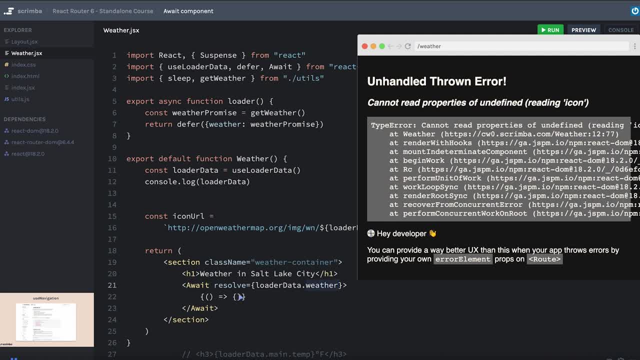 render props as a child. And when our promise finally gets resolved, it will pass to this function the loaded weather, And we can call this whatever we want, But in our case it makes sense to call it loaded weather, And loaded weather will be the data that we used to be calling loader data. So inside of this function, 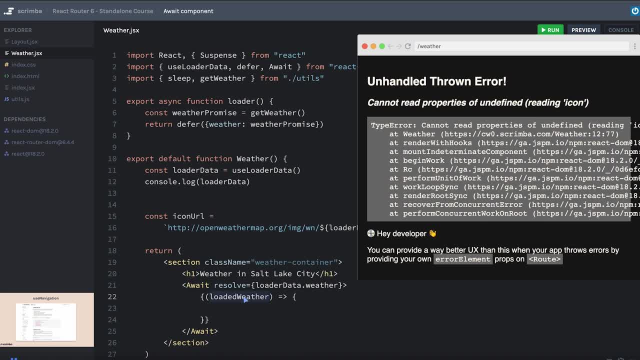 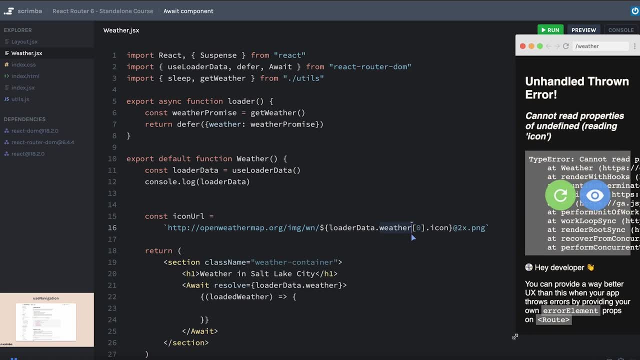 is where one we can have access to our loaded weather, for example. this icon is going to be broken because loader data is a promise and does not have a weather property. That's actually the error that we see over here. it's saying that we can't read the property icon of undefined, And so I'm going to bring in 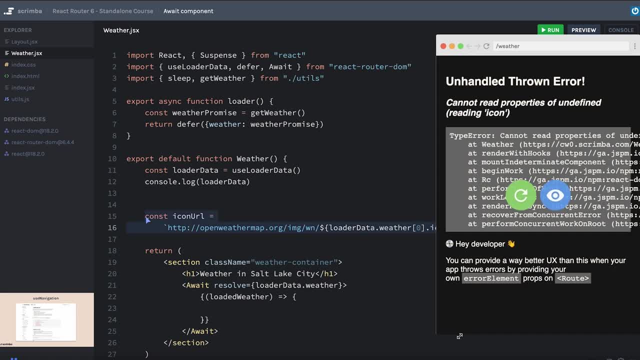 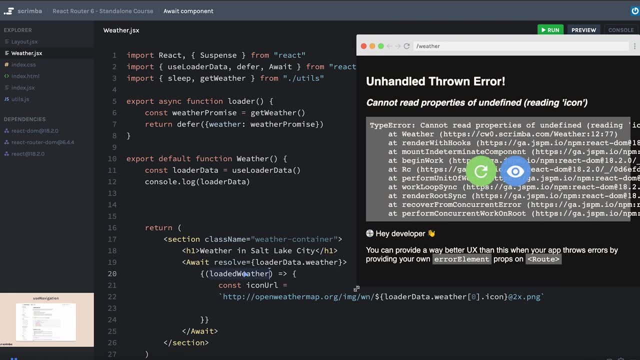 the property icon of undefined, And so I'm going to bring in the property icon of undefined, And so I'm going to bring in this URL assignment inside of my render prop over here And I can make the changes needed, like changing loader data to loaded weather. In fact, let me move this console log down And we will. 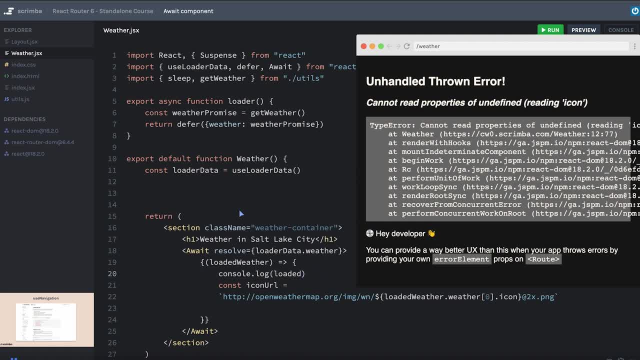 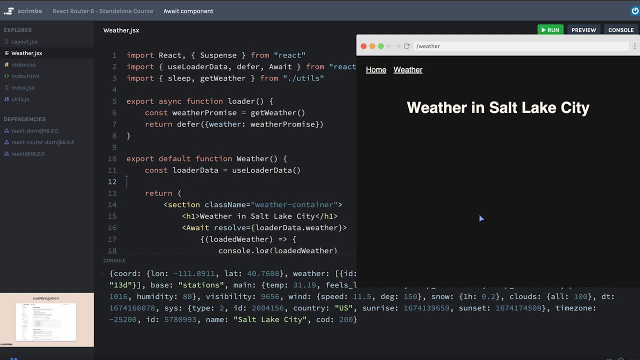 console log, our loaded weather, so we can see what we're working with And there's a chance we'll have an error. Let's take a look. Okay, and it did take a full three seconds plus a little bit to actually render anything on this page, But you can see that the loaded weather is the weather. 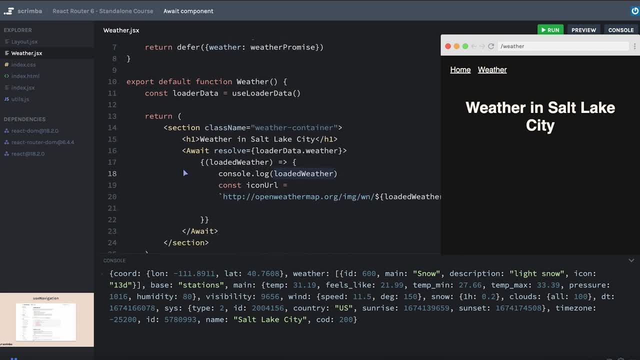 object that we were working with before, And because the await component will only render the children inside of the render prop, or rather it will only call this child function after it has finished resolving our data, we can again like we had in our original setup- be sure that loaded. 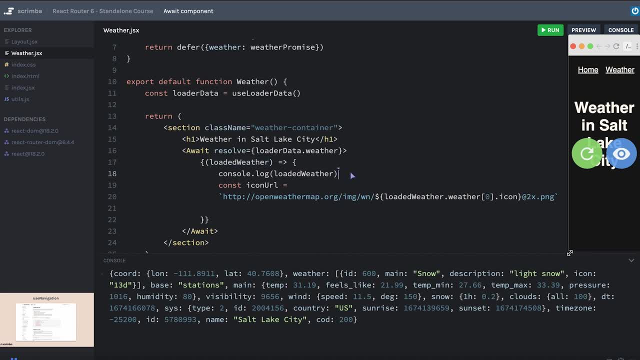 weather will exist when we're writing our code here. So let me get rid of my console log And I do want real children to exist here. So I'm going to return the markup that I want to display when the loaded weather has finished actually loading. So I'll open this up And I'm just going. 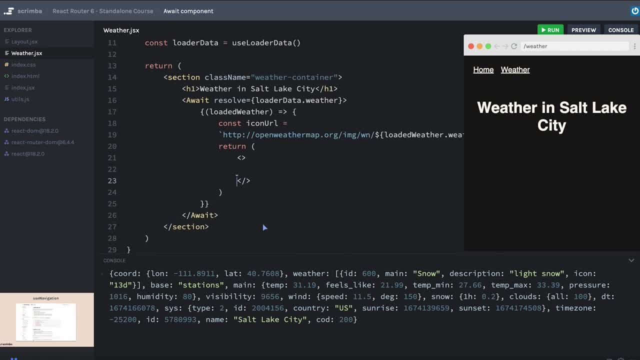 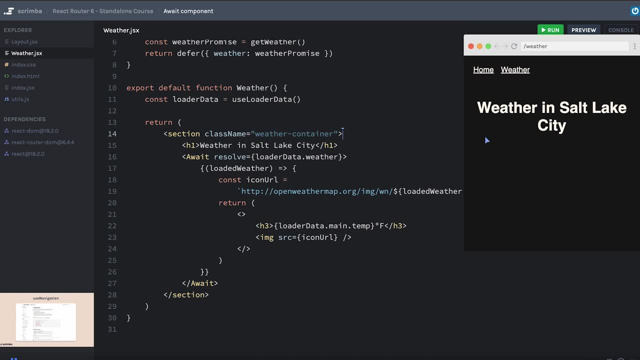 to put a fragment and then pull in these components that we had before. Now at least we're not broken. Let's hit save. we'll see that it will also take a bit of time for it to load, So I'll hit save right now, Okay, and then, lastly, we need to make sure that we have a loader, that we're 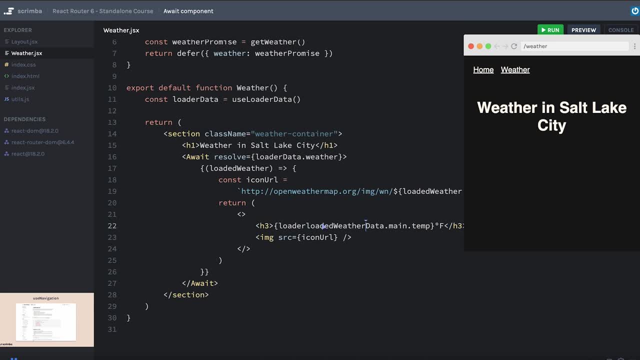 going to need to update loader data here to be loaded weather And let's go ahead and hit save again. I'll hit save right now. Okay, it's working. Obviously, we haven't quite fixed the user experience issue, But we were on the weather route. Of course we could see that even the navigation 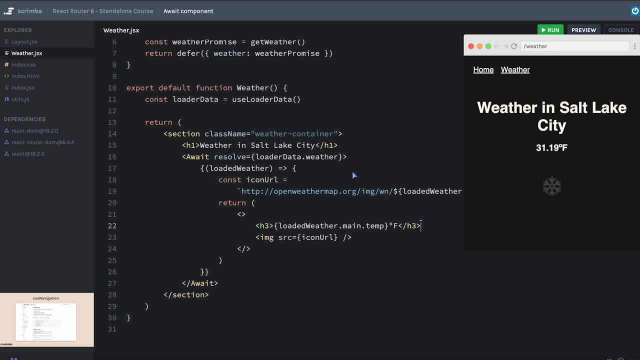 bar didn't render, which is a problem of its own that we're about to fix And cool. Well, it might seem like we're done, But once again, there's a lot of pieces to making this work in the way that we would expect, And we can actually get some. 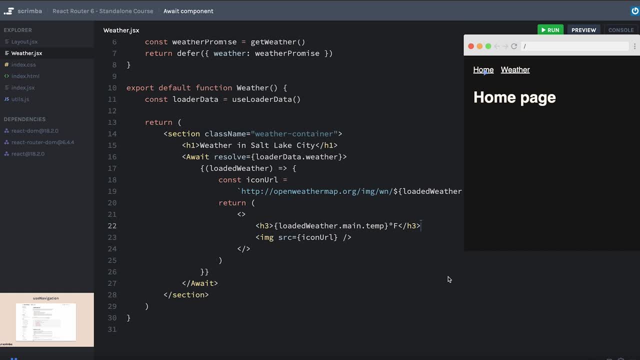 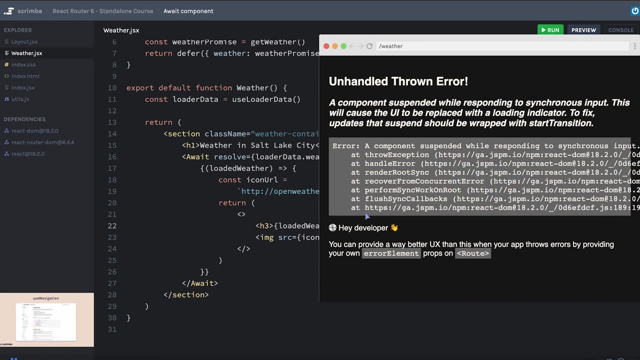 information out of it. So let's go ahead and hit save And we're going to hit save And we're going into the problem that we're still facing. if we go to home and then go back to weather, we'll see that it says a component suspended while responding to synchronous input. That doesn't necessarily 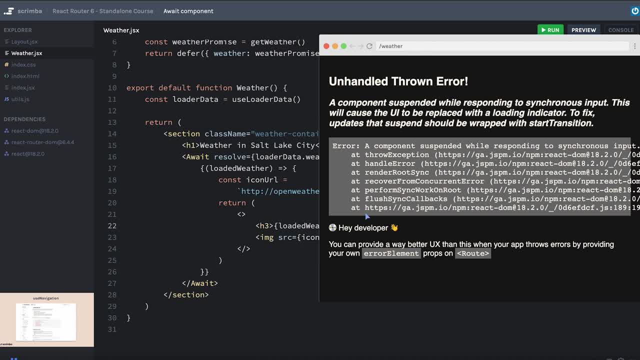 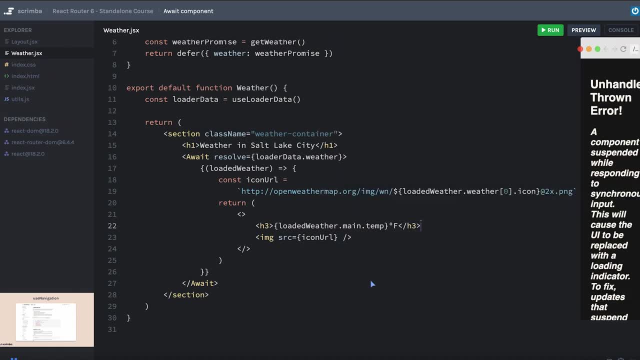 have to make sense, But it is something that we are going to fix by using a tool that comes directly from react- not even react router this time, but from react Before we plow ahead because we have covered so much ground. I want to get your hands on the keyboard practicing these. 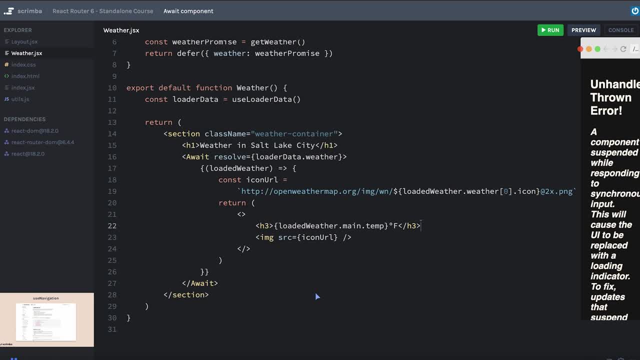 things. I know that we covered a lot of ground here And it may start to look a bit complicated, but the truth is, all we did was we added an await wrapper around the code that we wanted to display after the data had been loaded, And we put that markup inside of a child function that will receive. 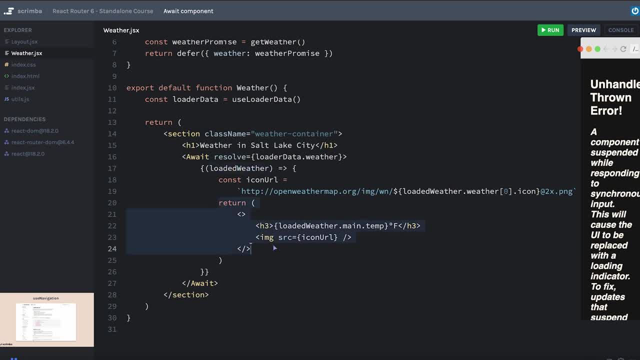 the successfully loaded weather and allow us to return whatever user interface that relies on having that successfully loaded weather. Let's bring this back over to van life So we can practice this and then we will come back. we'll learn about suspense and then come back again to van life and 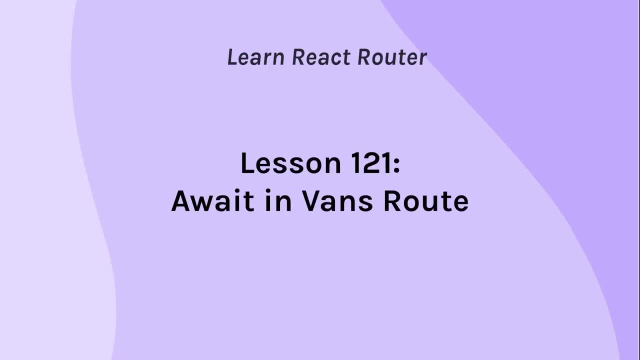 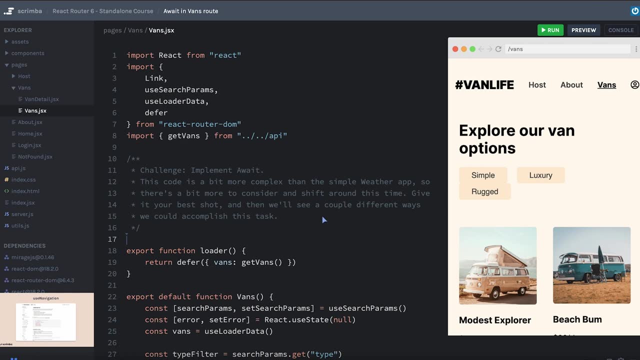 apply it. Admittedly, the code in our weather app is significantly more simple than the code here in our van life app, And so I've made a note of this. your challenge is to implement a weight. However, it's important to note that the code here is more complex, And so, rather than maybe spoon feed you. 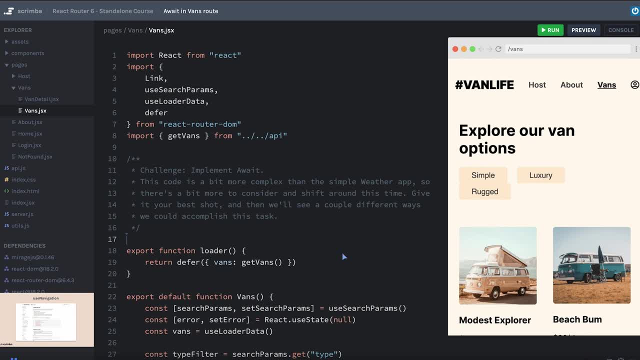 the answer or set you up perfectly for solving this. I think this might be a good opportunity for you to really put on your critical thinking hat and see if you can solve this on your own Really quick. I'll highlight what the issue that we're going to face is And then I'll 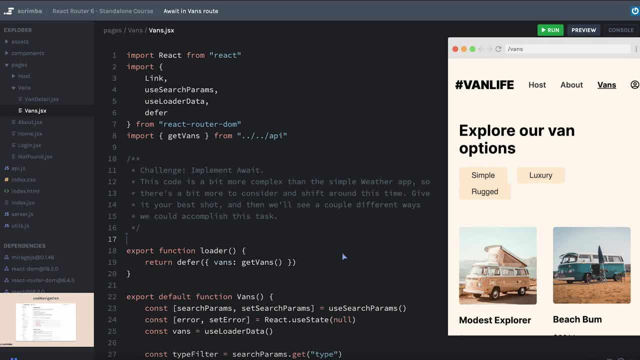 leave it up to you to figure out a solution. There's going to be more than one way to solve this. In fact, we're going to see two different ways. So the issue is: before, when we were pulling in vans from use loader data, we had the vans available to us. But now, because we're using, 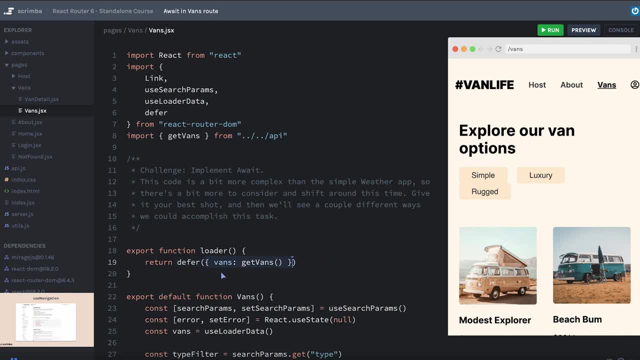 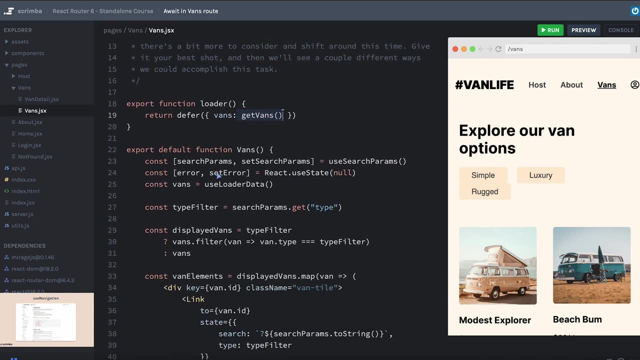 defer. we just have an object that has the ability to resolve fans Eventually. the benefit that we had before was we could just assume vans were available to us. But because we are deferring the loading of our vans to after the route transition happens, we have to make some other tweaks. 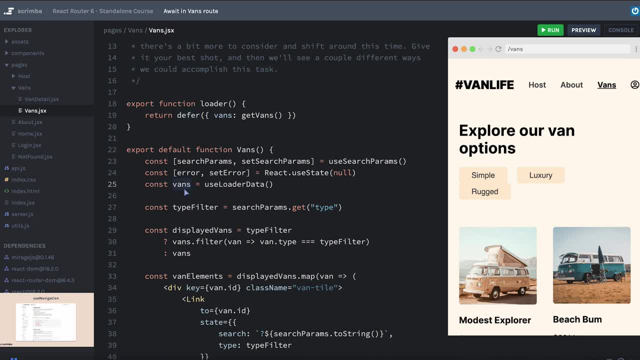 The reason this is a problem is because we are making use of this vans array, For example, when we filter the vans and create our displayed vans variable, and then we map over that in order to create the van elements, And then at the bottom we render our van elements way down here at the 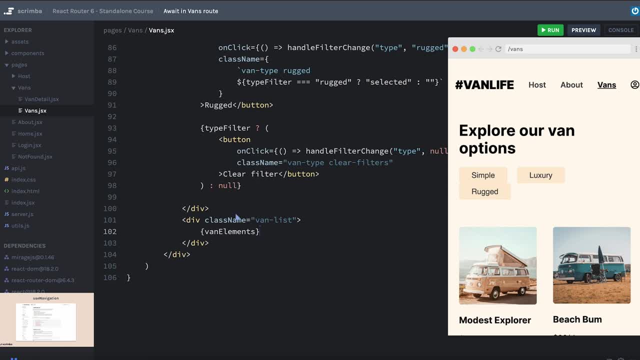 bottom. So you're going to have to think carefully about where we use our await component, because I can't just put it here inside of the rendered markup near the very end, because because at this point in the code it has already been rendered. So we're going to have to think carefully about. 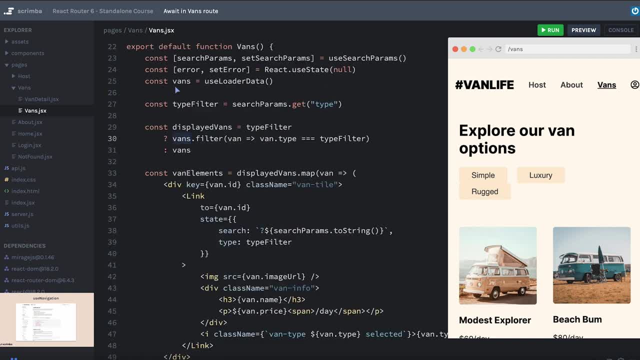 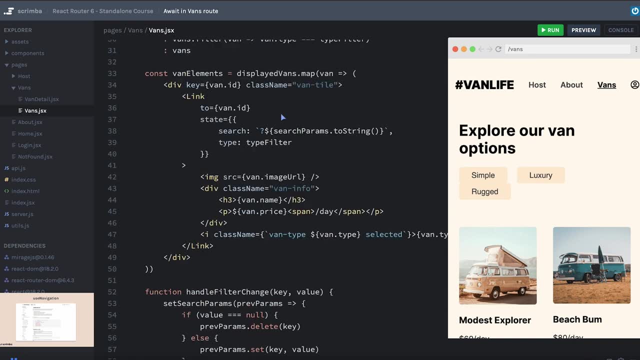 where we can put the vans anymore, And then we have to work between vans and we have the glue elements that are in the container andПoreVans array. For those of you who want to use the glue elements on the container, I myself have already attempted to make use of the Vans. 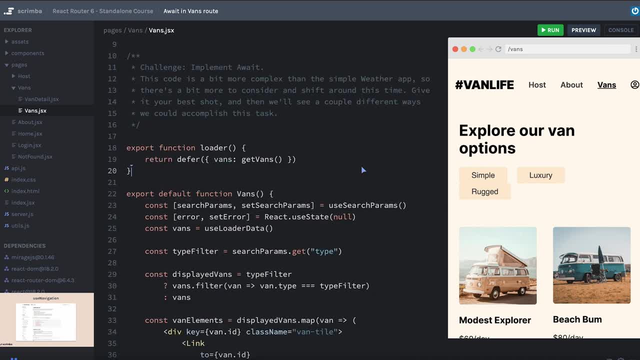 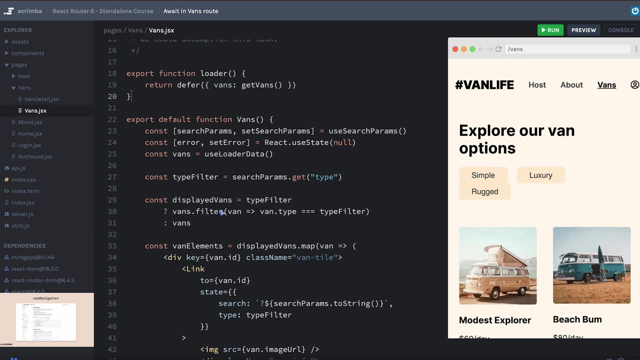 array, even though it's still an object with a promise inside. So give this your very best shot. I understand this might be a little more difficult, but I also think it's really good to stretch yourself and push yourself in order to grow. So pause now and work on this challenge. 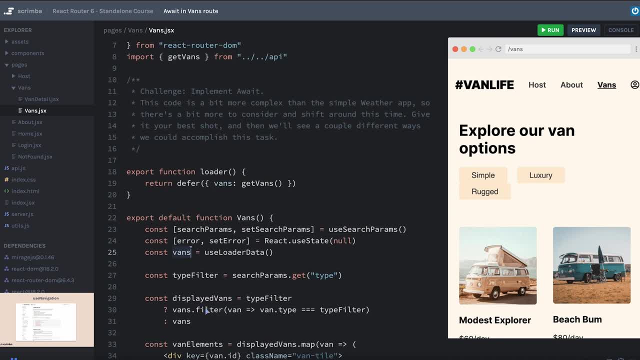 use loader data because the name vans implies that we have access to the vans. i'm instead going to change this to something like data promise. maybe this way i can immediately know that i'm going to have some problems when i try to, for example, filter over the vans ray, because i don't have 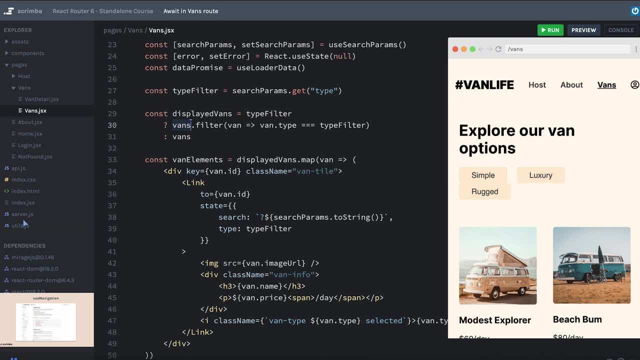 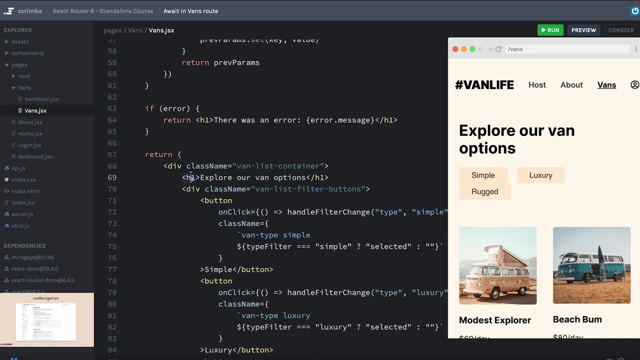 access to the vans array anymore. so let's go down to where we're starting to return the elements that we have, and i need to decide where i want my await to live. i think it might be okay for us to leave our h1 as soon as we get to this page, because it's not waiting on any data, but i don't. 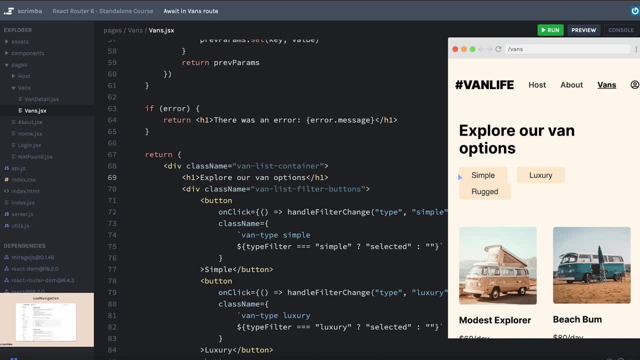 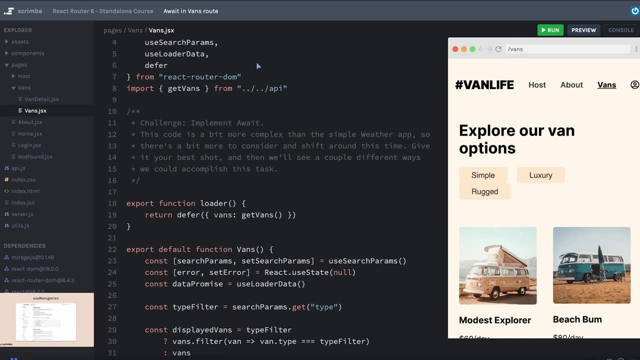 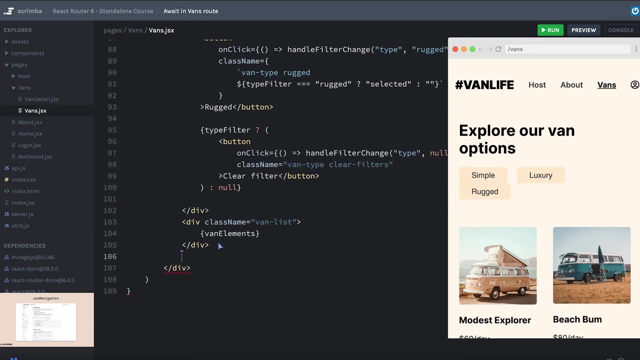 know that i want my filtering buttons to display if the data isn't there. so maybe right below my h1 i'm going to include my await component and i need to make sure to import that, and then let's just wrap everything that we have below it. that'll go down to here and we'll format. 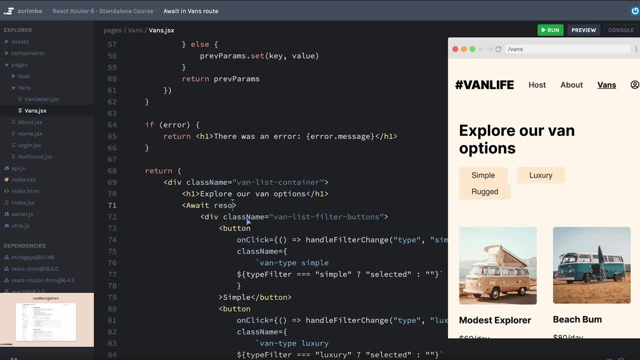 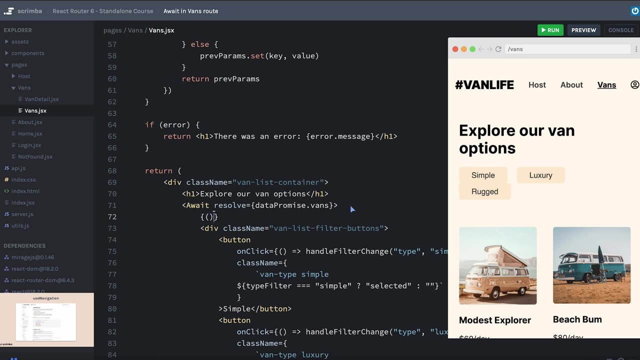 this, okay, and then the await component will take a resolve prop and we're going to pass data promise and in our case we just specifically want to wait for the vans array to resolve. then await expects a child function. so i need to enter into javascript and then put in my function here and we'll open that up and this function is going to receive. 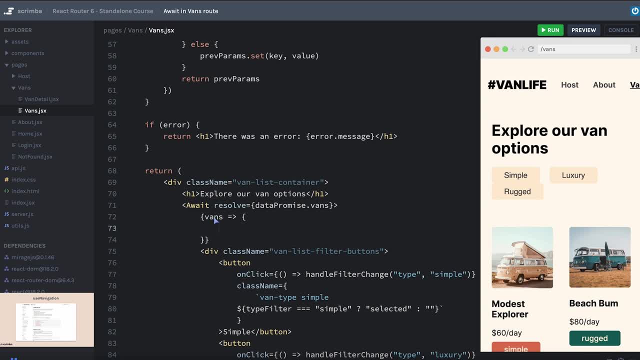 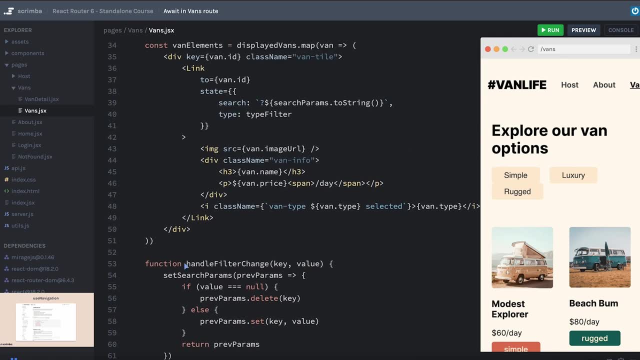 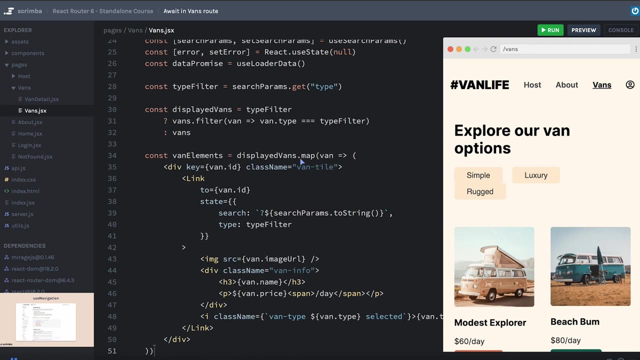 the array of vans as the data. now that i have access to this vans keyword, i can just take everything above it that was expecting to have access to vans and move it inside of that child function. so i want to have all of my van elements because that relies on displayed vans. 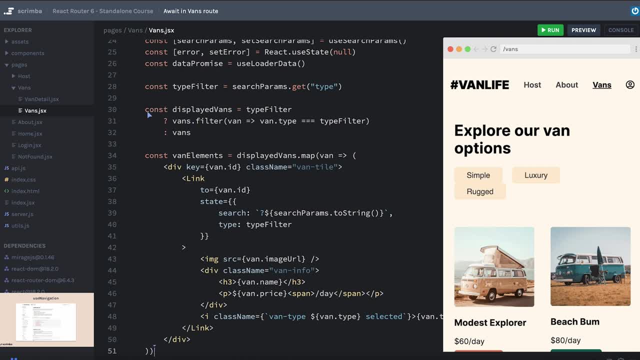 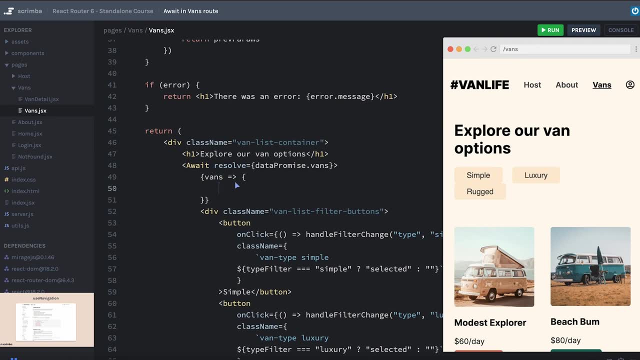 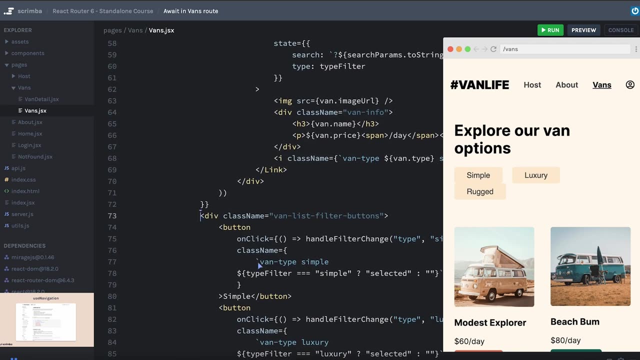 so i'll need to bring in displayed vans, which relies on the vans array. so i'll just go ahead and cut all of this and paste it down here, where to go inside of my await render props function here, so we'll paste it and format it, okay, and then i have all of this markup that i need to. 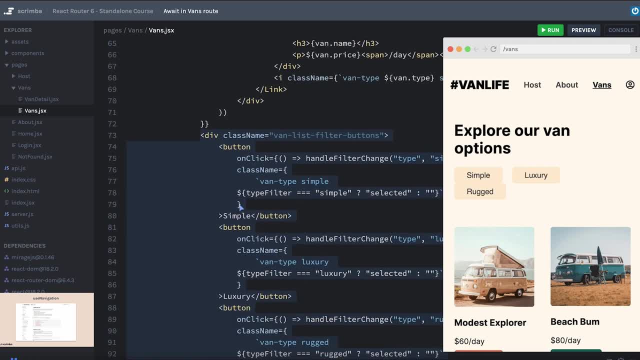 be returning as the children elements. so we'll go ahead and cut that out. and right here we're going to have all of the children elements. so we'll go ahead and cut that out. and right here we're going to have all of the children elements. so we'll go ahead and cut that out, and right here. 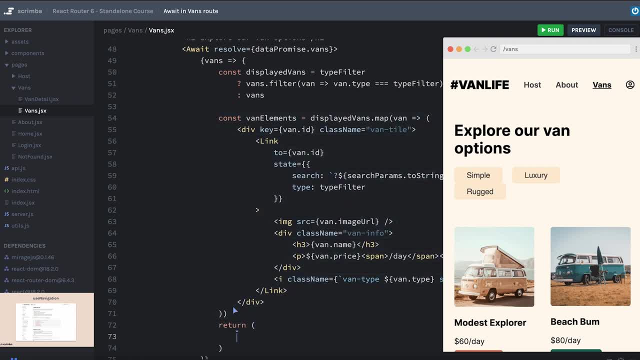 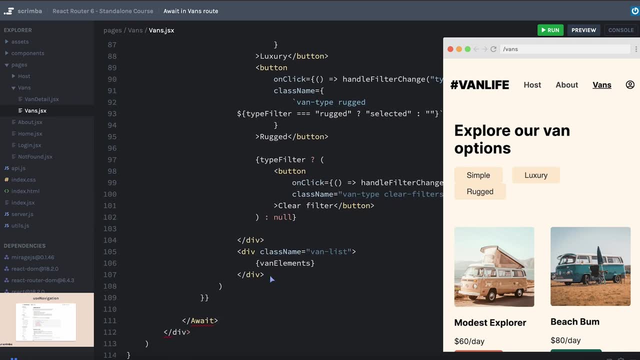 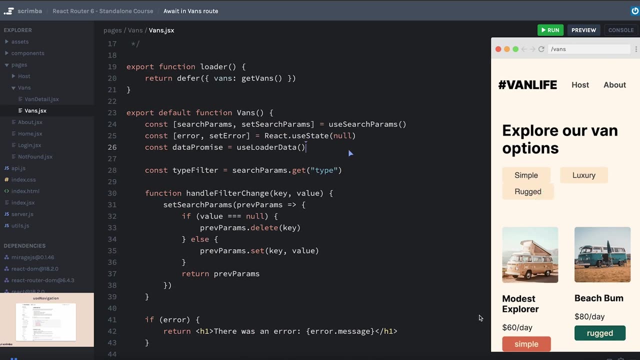 below our van elements. we will return and then we'll paste that back in, and i think we have an issue here because we're trying to return two divs, so let me just wrap these in a fragment and perfect. okay, that seems to fix that. let's cross our fingers and hope for the best. we'll hit save. 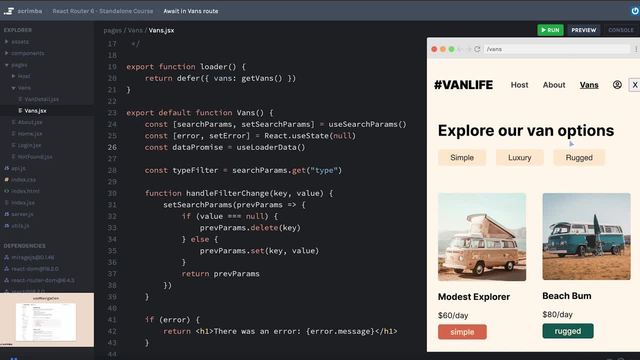 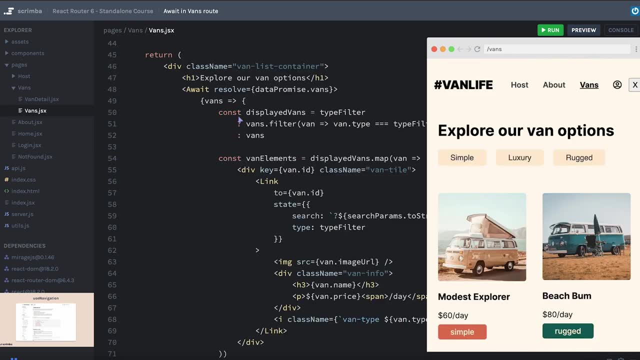 okay, and we have an issue right now where the entire screen shows up as blank. we're going to be fixing that very soon, but we have our vans data showing up, awesome, okay. as far as await is concerned, this is a great start. we could just leave it like this, but i did want to show, just for the sake of 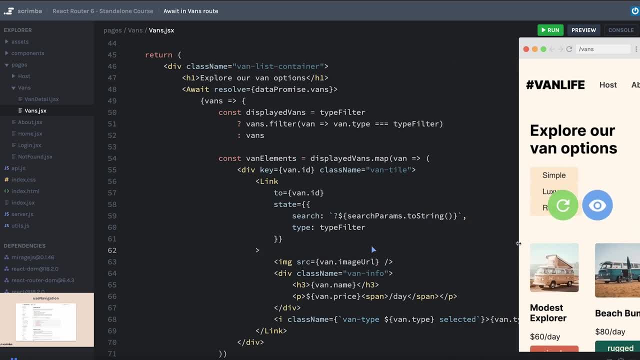 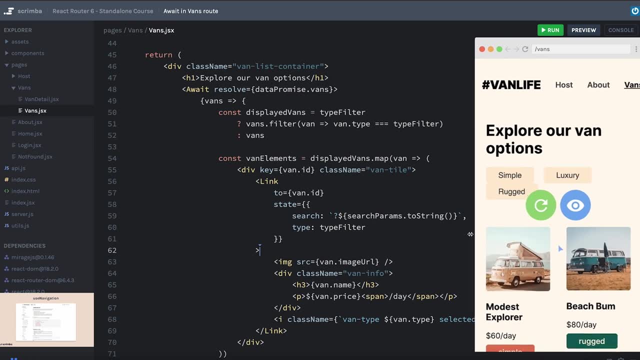 learning another way that we could solve this problem. it's actually only going to be one extra step beyond what we've already done, and then we'll be able to learn the final piece we need in order to get the user experience back that we're hoping for, which we'll be able to show a little loading. 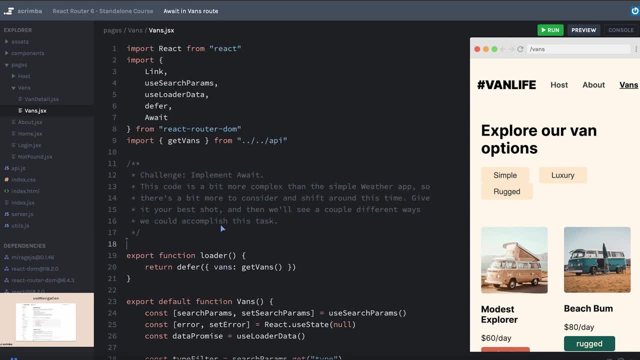 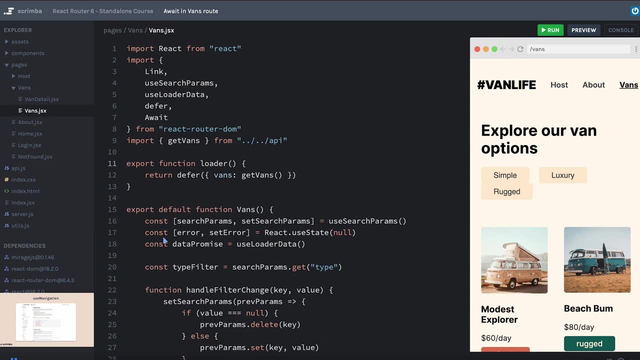 state here when we get to this component. so i know this challenge might have been a little bit difficult. if it was, that's completely okay. as i always say, it's important for us to get experience by trying these difficult things. so if you weren't able to get experience by trying these difficult, 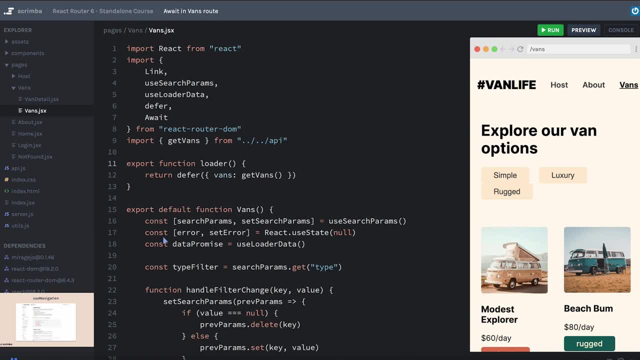 things. so if you weren't able to get experience by trying these difficult things, so if you weren't able to solve it on your own, that's okay. as always, just scrub back and try again. remember there's nobody that's giving you any kind of grade. by completing this course faster, it's more. 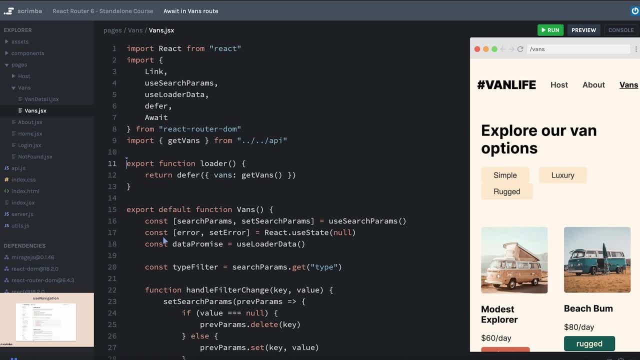 important that you grasp the concepts that we're learning and reach out to the community for any help you might need, for just kind of plowing ahead. so take all the time you need with this code, try rewriting it again if you'd like, and when you're ready we'll move on and see another. 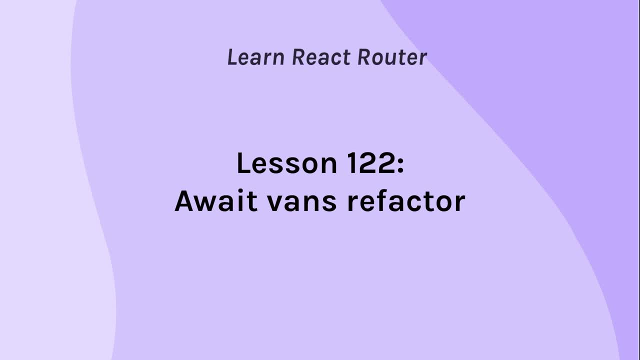 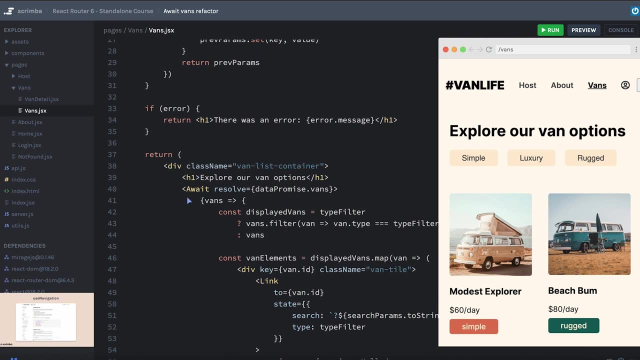 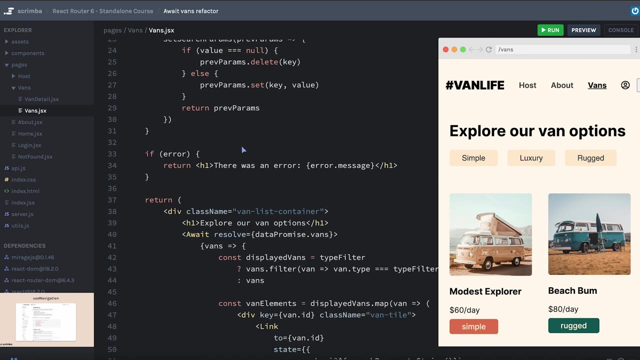 way we could solve this. we've seen one solution where our await keyword is up here pretty high inside of our return, and then we just grabbed everything that was above it, everything that was, i guess, preparing the elements to be displayed, and just shoved it down here inside of our return. so everything is just happening right here in line. this isn't. 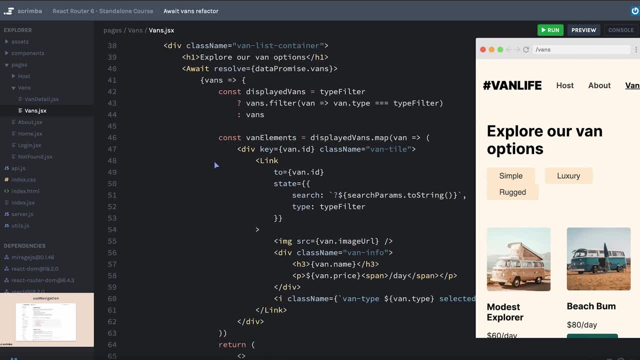 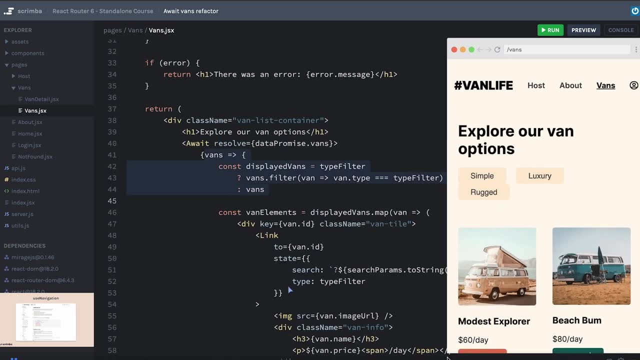 terrible by any means, but it is a little bit difficult to parse and to read because everything is so deeply nested. but if we think about it, what we have here is a function that is handling all of the preparation for what should be ultimately displayed. so one thing we 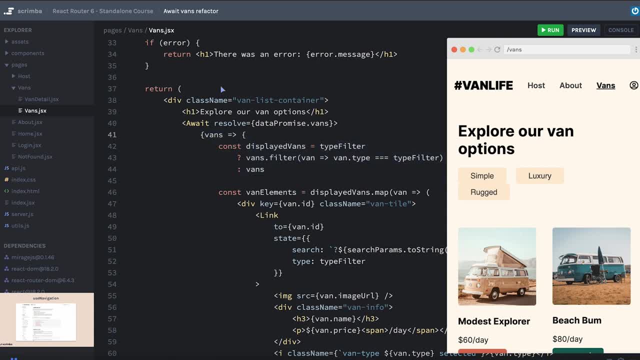 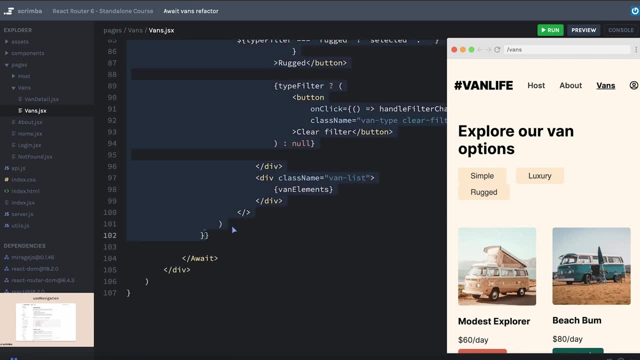 could do and again, like i mentioned, this is just a minor refactor but hopefully it will improve. the readability is we can take this whole function. i'm going to go all the way down here to right here where the function ends and we'll just cut this out and we can see. that was the 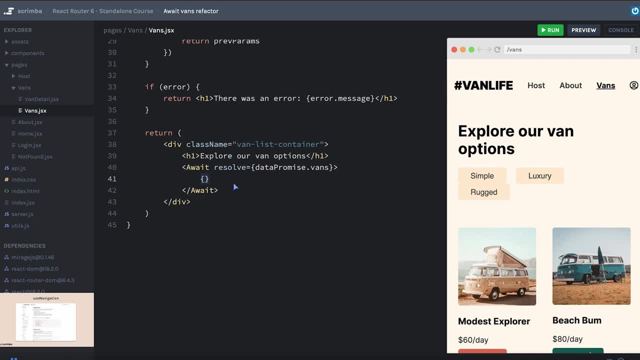 right level, because we just have an empty set of curly braces now, and then, before my return, i can just define a new function, and maybe we'll call it render and elements, and then let's paste the function that we just created, and it doesn't need to. 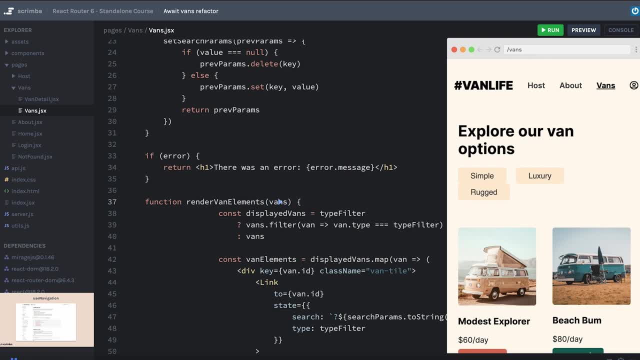 be an arrow function per se, so i'll just go ahead and tidy this up. i'll format this, and so now everything is multiple layers, less nested and i personally think is a little bit easier to read, and then we can simply pass the reference to this function inside of our await way down here. 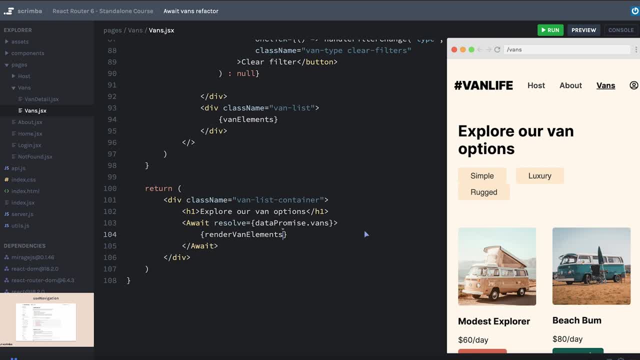 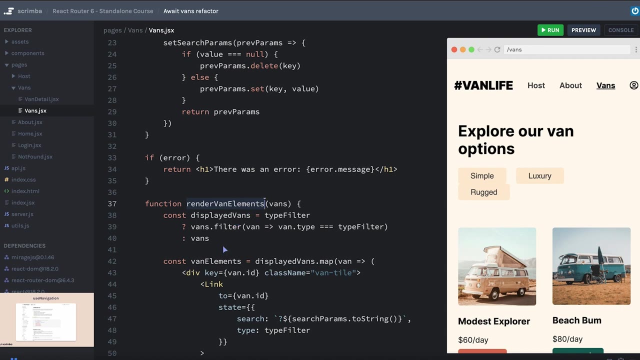 at the bottom. so i think at least this has simplified the level of nesting and it's also simplified our return and then, if we really wanted to clean this component up, we could make kind of a utility helper function where this function render van elements might sit inside of a different file and then just import it if we really wanted to. 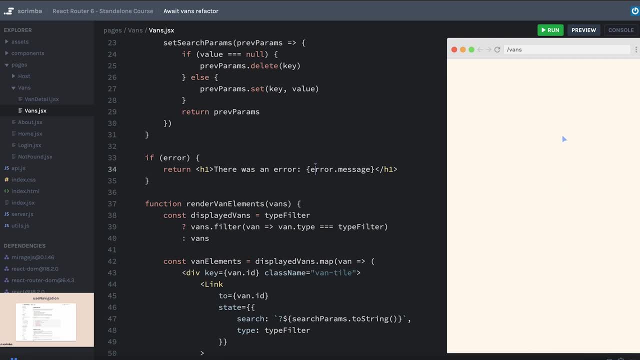 So let's hit save and see if this works in the first place. Okay, we did get the delay where the screen is blank Again, that's what we're going to be fixing next, But everything seems to be working and we can go into one of the nested vans- Perfect. Now it's time for us to 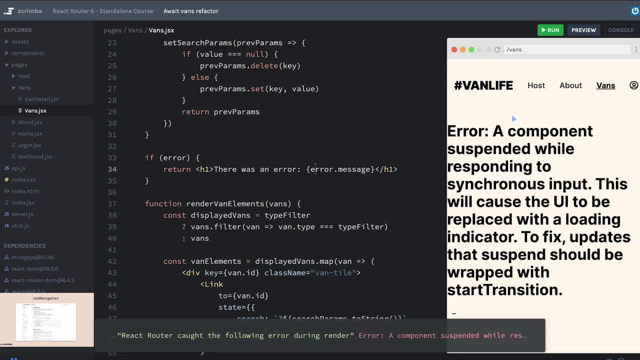 solve the last little problem. You can see if I click back to all vans, we actually get an error displaying saying that a component suspended while responding to synchronous input. The fix for this is not something specific to react router, but instead react itself. So next we're going to. 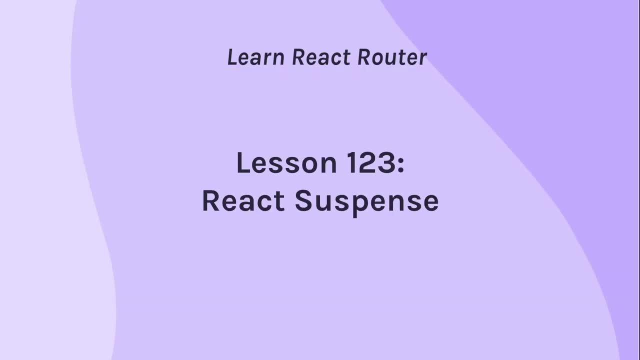 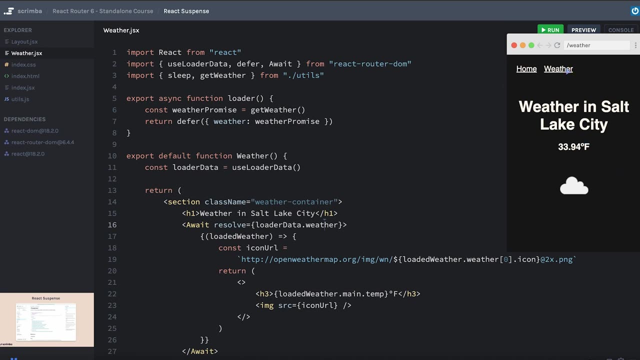 start learning about the suspense component in react. Here we are back at our trusty weather app, And you might remember that we had a little bit of an issue. I'm going to go ahead and refresh this and we'll see that it's blank for a couple seconds And then all of our data gets loaded in. 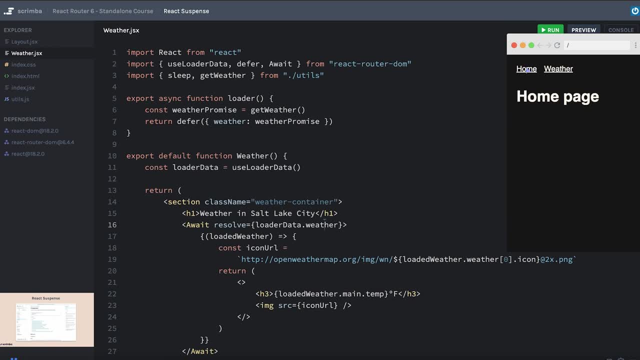 at once. Not only that, but if I go to another route and then try to come back to whether we actually get an error that gets thrown, we can see that we have a little bit of an error that gets thrown, And we can see that. 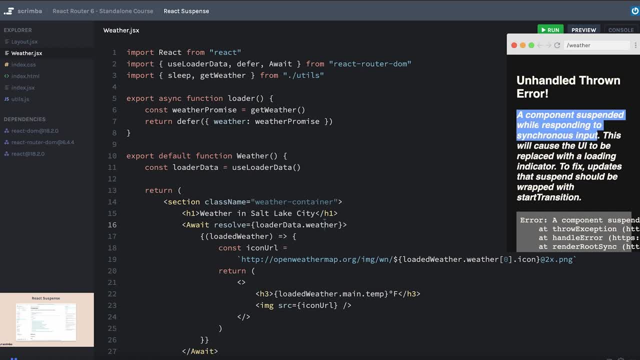 it says: a component suspended while responding to a synchronous input. This leads us to the final piece in our puzzle of actually creating the user experience that we originally set out to create, And that is by using something that comes from react, called suspense. you can click the screenshot. 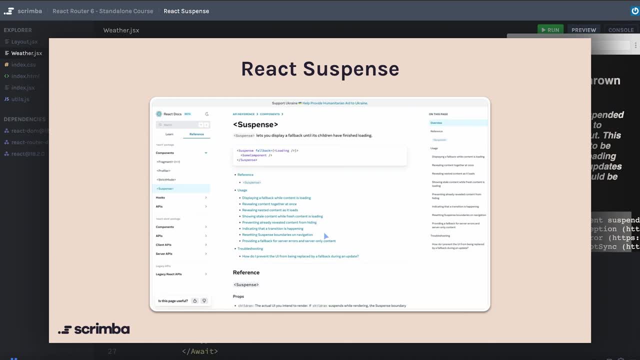 here to go directly to the react documentation on suspense. It's fairly thorough, So you're welcome to read through the entire thing if you want. I'm not going to be teaching all of the ins and outs of suspense as a part of this course. I'm simply going to be showing you. 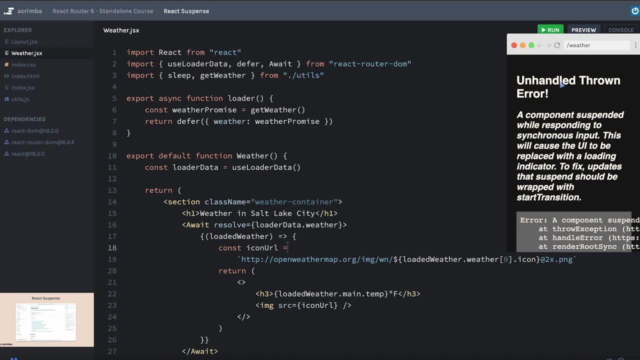 how we can use suspense to finally get to that finished point that we've been trying to get to this whole time. react has introduced the ability for mostly libraries- third party libraries- to suspend rendering of your react application until something has finished. The benefit of this is we. 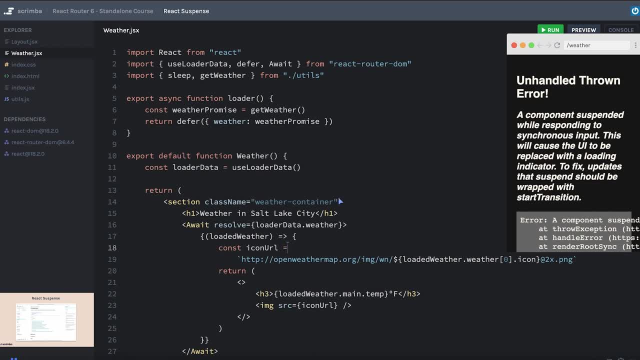 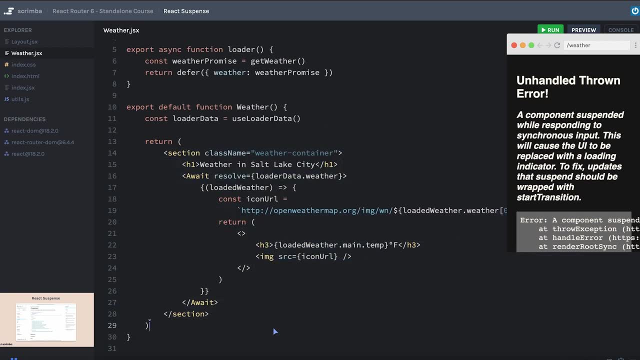 can treat our components as if they were synchronous, like we see here, where we're pulling in loader data and then we are just rendering what we need with that loader data instead of initializing our fetch request after the weather component is done. So we're going to have to maintain the loading state and the error state and all those other. 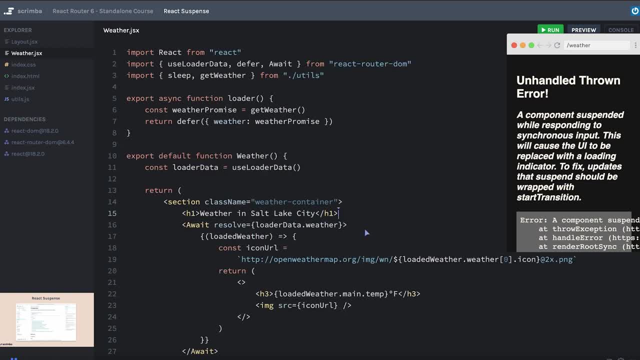 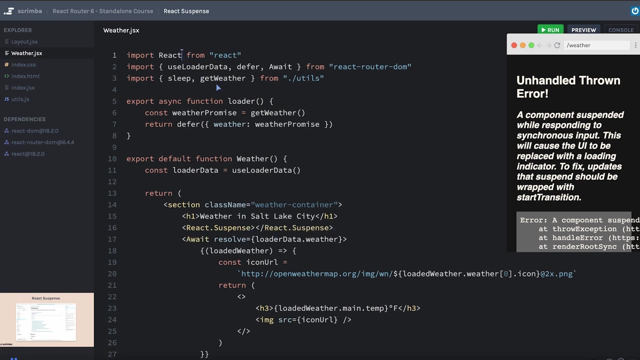 things that we used to be doing. Suspense allows us to wrap our suspended component, which is this await component, in another component called suspense. Now I can just say react dot, suspense here. Or, if you don't like the dot syntax, you could separately pull in suspense like this: 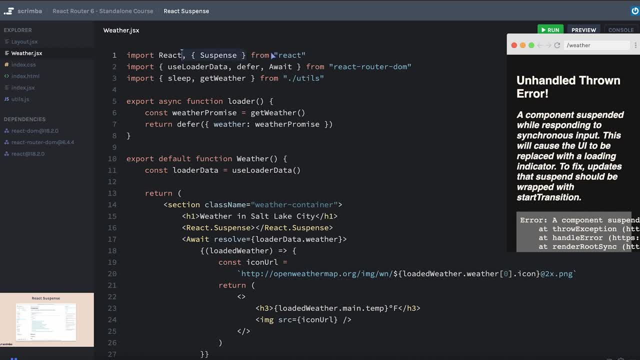 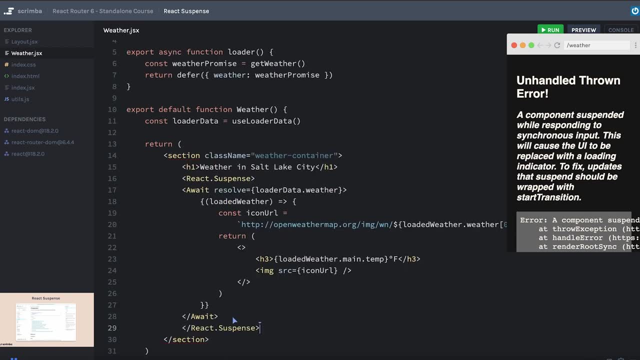 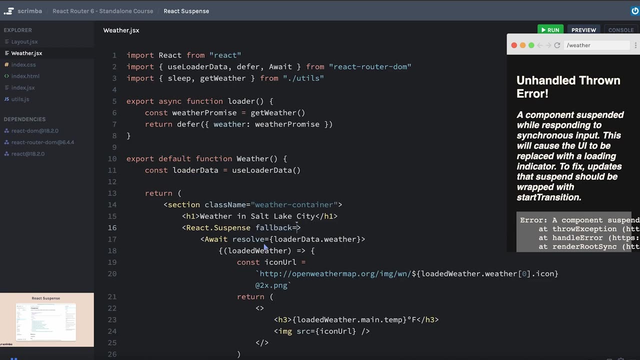 just to be totally clear that suspense is coming from react. I'm going to leave it as react dot suspense For now. I'm going to put my closing tag down here after a wait and we'll indent, And then the last thing that I need to do is provide a prop called fallback. The idea of fallback is that 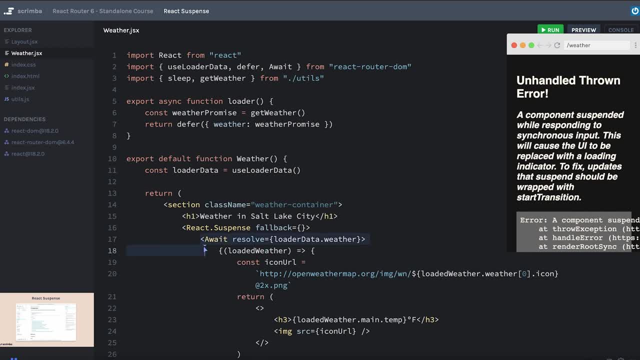 it gives react, an element to render, while it's waiting for the other component, that is suspending, to finish. In this case I can just put maybe an h2 that says loading, And maybe I'll be a little more clear and say loading weather, And with that we're going to be able to put a prop called fallback. 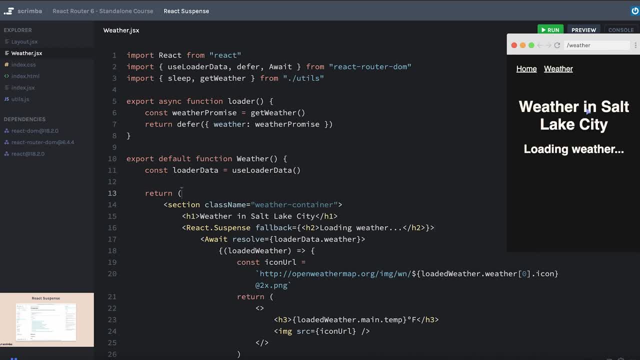 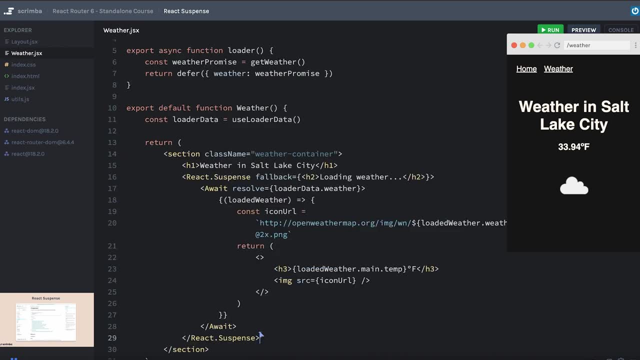 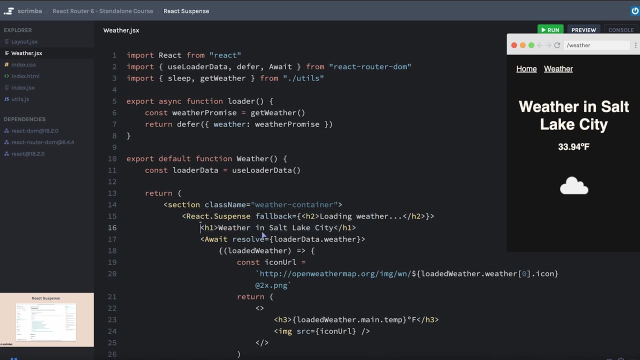 And with that simple addition I can hit refresh. we see loading weather and then we get our weather. Now notice that I put my suspense boundary- you could call it- underneath my weather in Salt Lake City h1.. If I were to move this up by one, let's go ahead and indent that I'll hit. 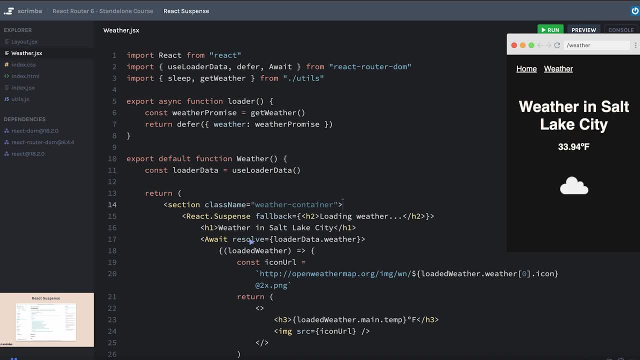 Save And we just get loading weather. it doesn't have that h1 displaying anywhere. And then it displays what is inside of the suspense boundary, Because I have this text hard coded. probably doesn't need to be inside of the suspense boundary, But of course, if I wanted to pull the 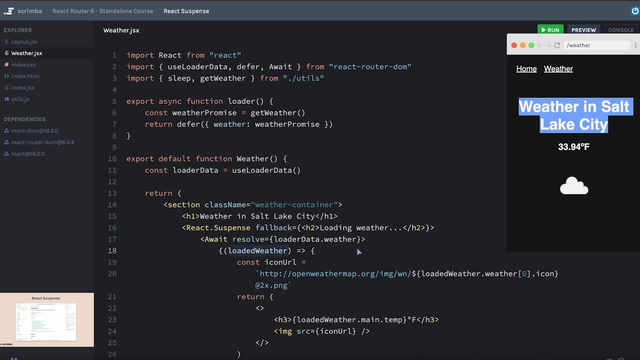 city from my loaded weather, which actually is part of the data that comes in, then I would just need to move this down inside of this callback function, So it would be down here where I'm returning the weather specific data. I think the way it currently is right now is probably fine. 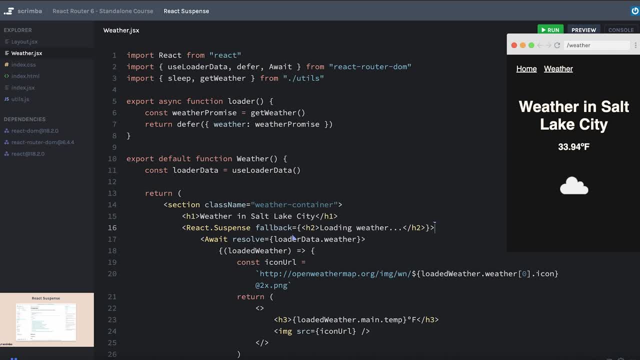 Now that we've added this suspense boundary, we also are handling that exception where this component was suspending, And so I can go back and see if it's still there, And I can go back and see if it's still there, And I can go back to my home And let's go ahead and refresh, just for. 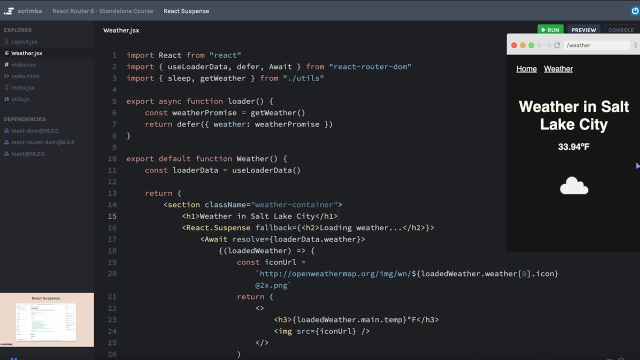 giggles, And then we'll go back to whether we get loading weather And then we get the weather loading in. Finally we're back to a point where the user experience is a lot smoother. And sure, we've had to learn a lot along the way and make quite a few changes to the code, But in the end 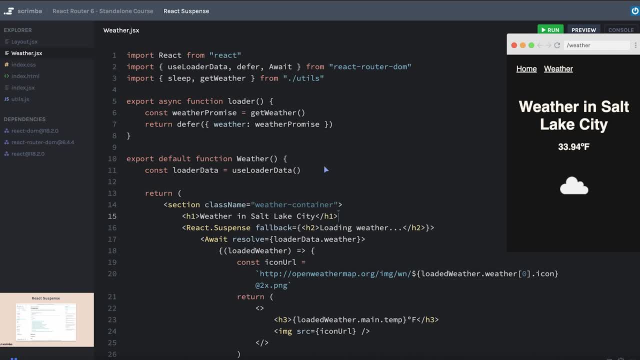 I don't have to maintain all of that error prone react state. In the meantime, it's all being handled in a very declarative way by other libraries. Okay, I've talked quite a bit. Let's practice this in two phases. I'm going to erase what I did and have you do it again, And 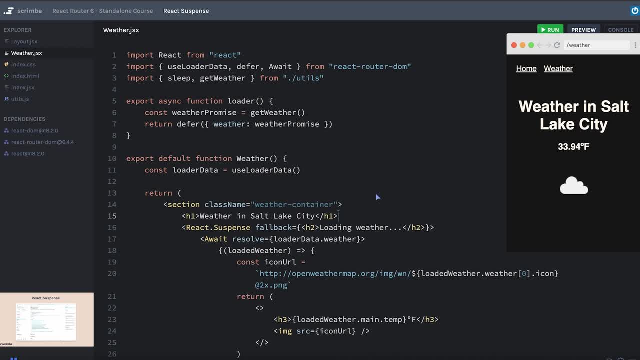 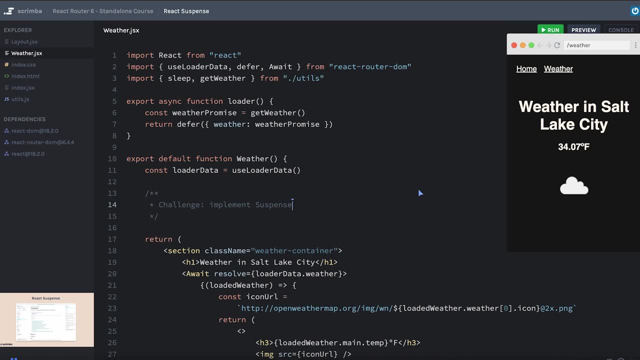 then we're going to move back to the van life app again and have you implement it there as well. Okay, simply put, your challenge is to implement suspense. pause now and work on the challenge. Maybe just to see it the other way: This time I am going to pull in suspense as a separate. 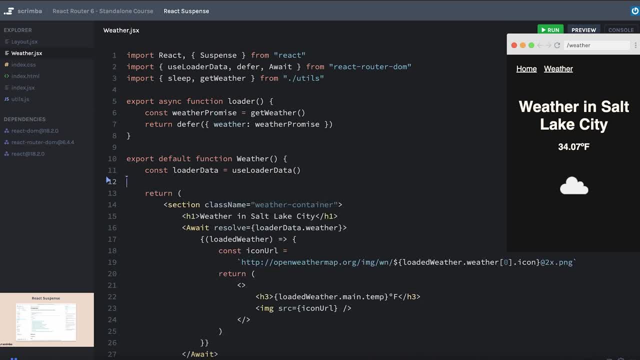 component up there. We'll just clear out this challenge, since that's an easy one To remember, and we will just wrap our await in the suspense component. Okay, and we can't forget, I need to give it a fallback property. This is the element that will display while it's waiting. 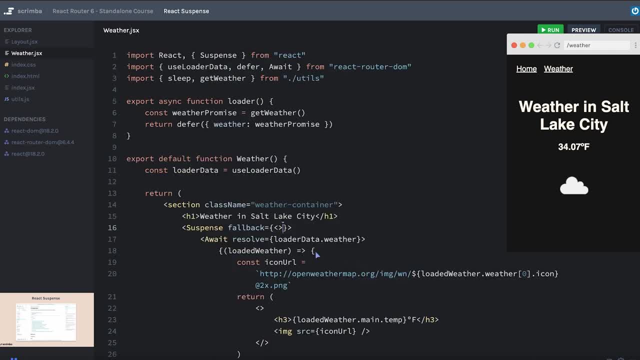 for the suspended component to finish, And so we'll just put back our h2, that says loading weather, it's saved. And then we're going to go back to the van life app And then we're going to save. we get loading weather, and then we get the weather. Okay, let's jump back into van life and 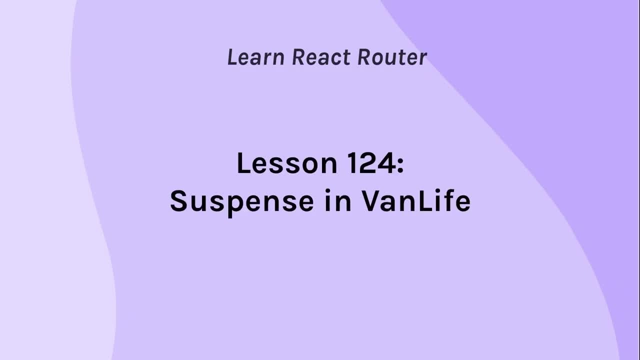 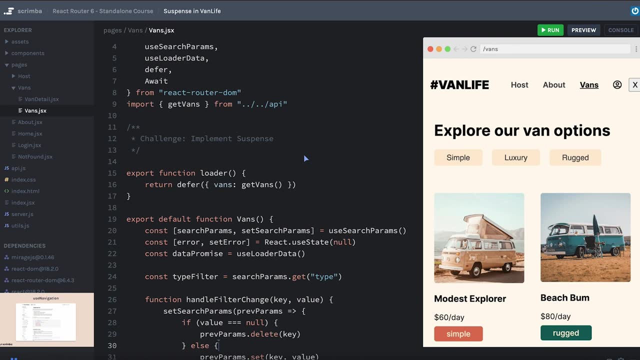 implement what we've learned. Short and sweet, your challenge is to implement suspense. pause now and work on the challenge. The error that we saw earlier was that the component suspended while responding to synchronous input, And that component that suspended is our van life app. So we're going. 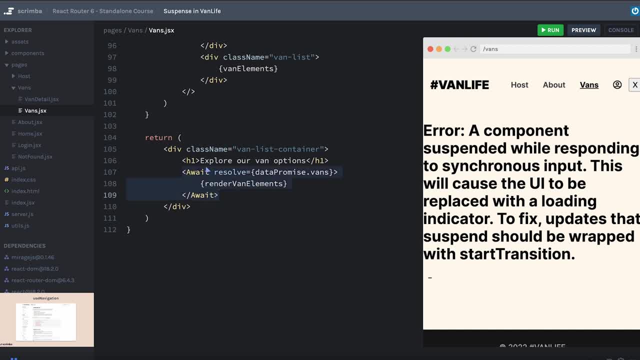 to do an update to the function. So we're going to call it react to reactdotsuspense And what we're going to do is we're going to call it react to react to that suspense is going to be something that we like to call it a way component way down here at the bottom. So any components that are 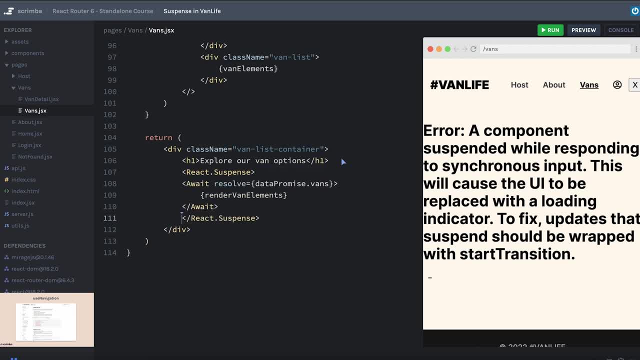 going to suspend. we need to wrap in a call to reactdotsuspense. I haven't imported it separately, So I'm just going to call it reactdotsuspense And we'll move this down here and indent And then 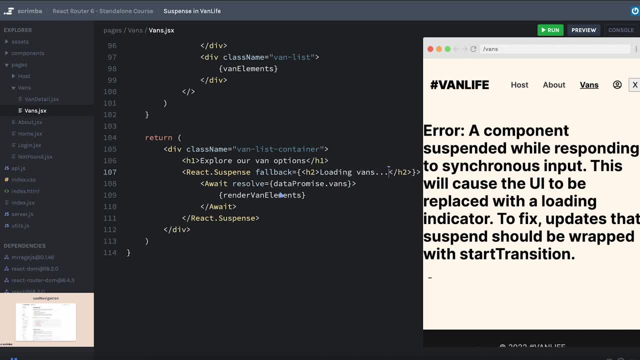 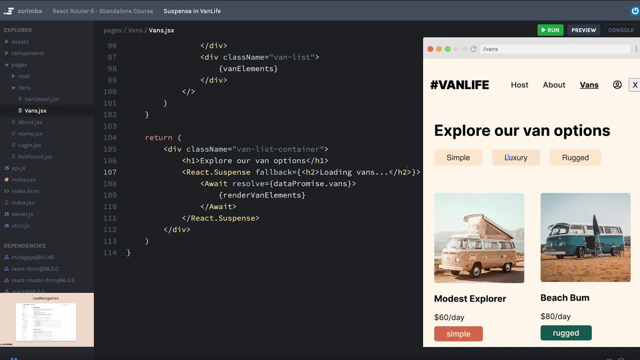 lastly, we just need to provide a fallback prop, And I'll just be a little bit boring Again. we'll just say: loading vans. Okay, let's refresh vans h2 there for us while things were loading in, and we're back to a really snappy user experience. 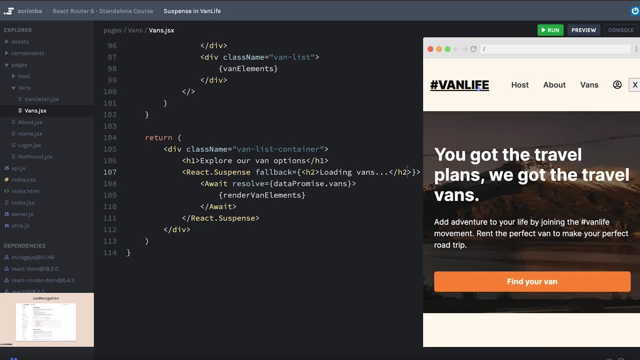 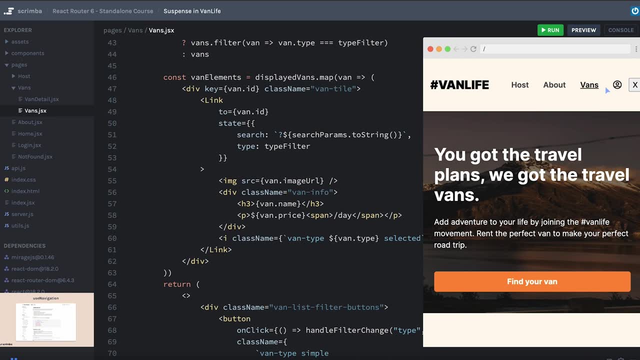 now i do want to be totally clear. it's not that big of a deal if you don't want to go out of your way to include await, suspense and defer because maybe the transition to the new route is not taking very long. we need to remember that i did include a delay right here inside of our server. so 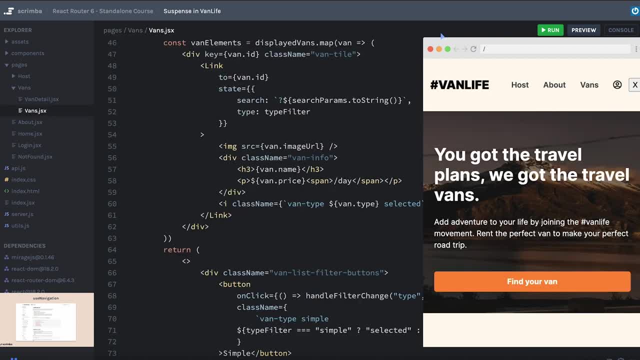 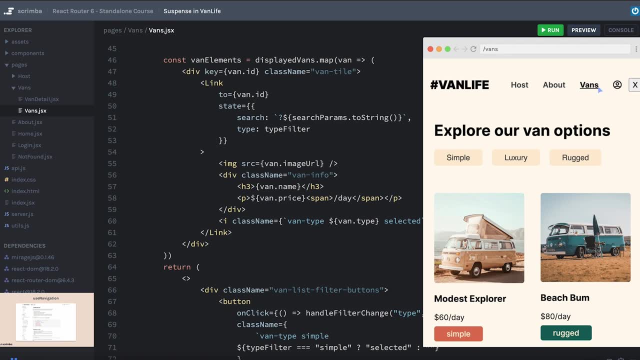 it's pretty much manufactured delay. i'll come back here to vans and then we'll click on the vans route and we can see that it's pretty snappy anyway, even if it were to delay for a half second or so before coming to the new route. in the end it really just depends on what user experience you 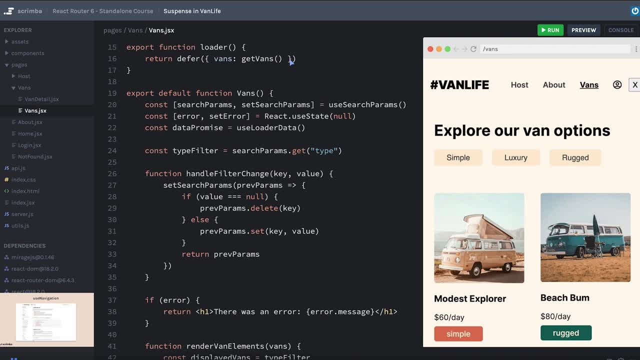 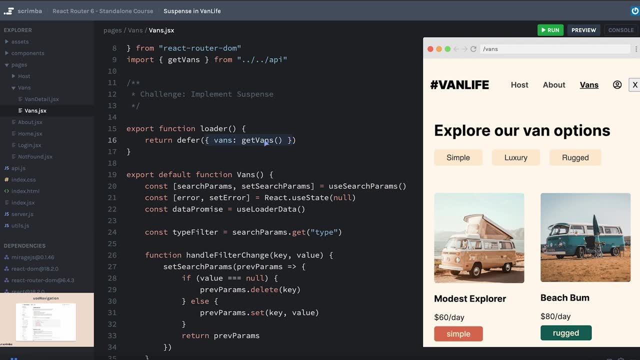 want. there's one last thing that i just want to touch on really quickly, and that has to do with this defer function. you can see we have changed this to be an object, and that's because, if we did want to include additional data, maybe there was something like the user that we needed to. 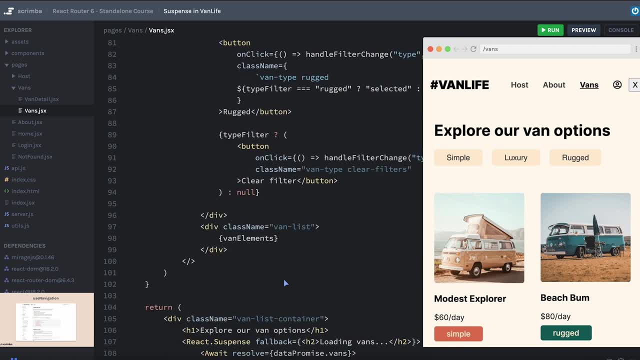 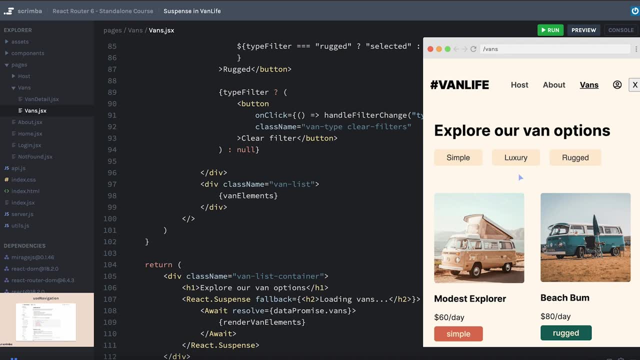 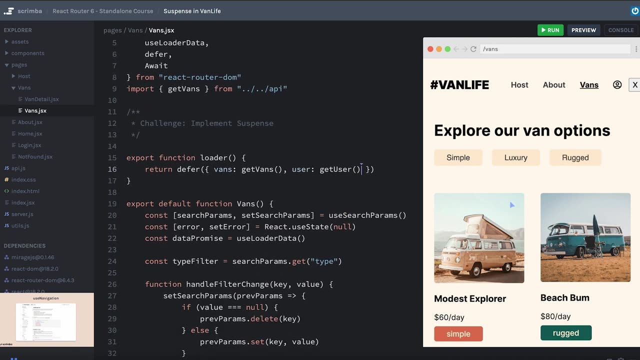 pull in and we say: get user, then we could have different await boundaries and suspense boundaries, depending on what data we want to display first or what data we do or do not want to defer on. if there was some data that was absolutely crucial for us to load before we even transition to this route, then we do have some flexibility because we can come to 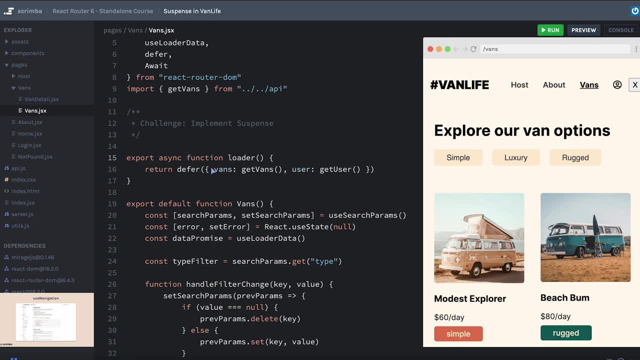 our function. we can turn it back into an async function and any pieces of data that we want to delay transitioning to the new route for we can just include a weight in front of the promise. by doing this, it means that we can put a new function in the new route and we can see that the new route transition will not. 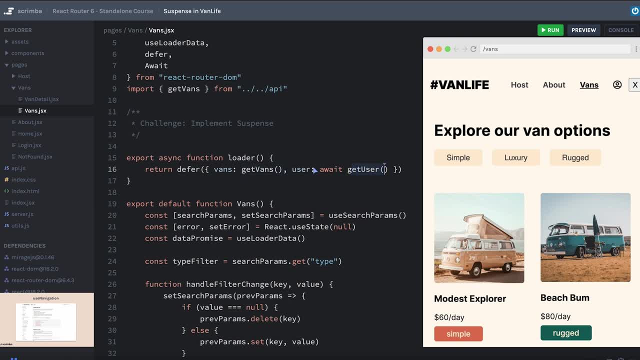 start until this get user function has completed. but if the get vans function takes longer than the get user function, then it will transition as soon as the user is ready and we'll get our suspense boundary while the get vans function is still resolving. in our case, we don't have any use for. 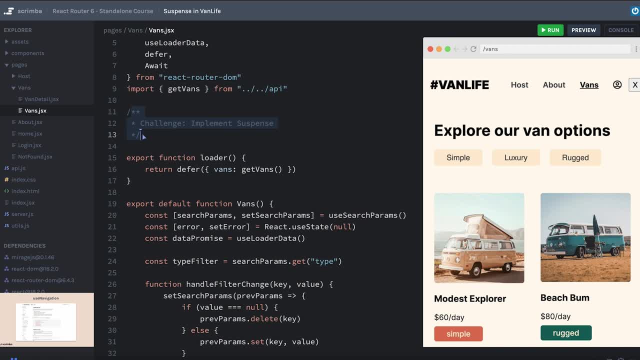 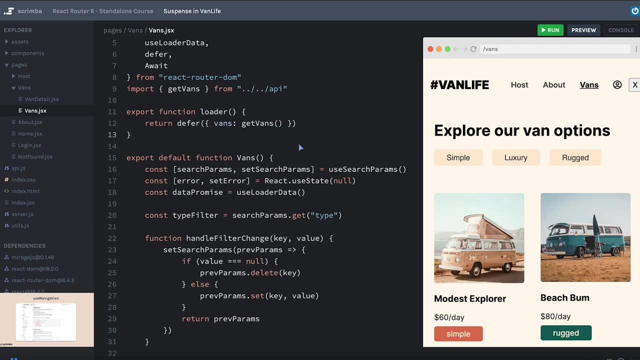 this per se, so i'll just go ahead and delete this, but i just wanted to round out our experience there by mentioning that, just in case that was useful to you at some point in the future. by the way, if you want to learn more about it, you can go there for more information. now we've been working. 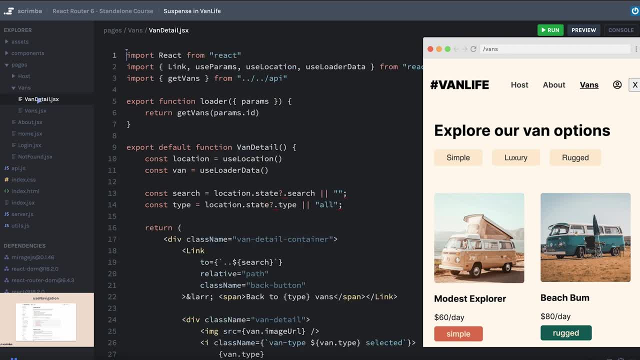 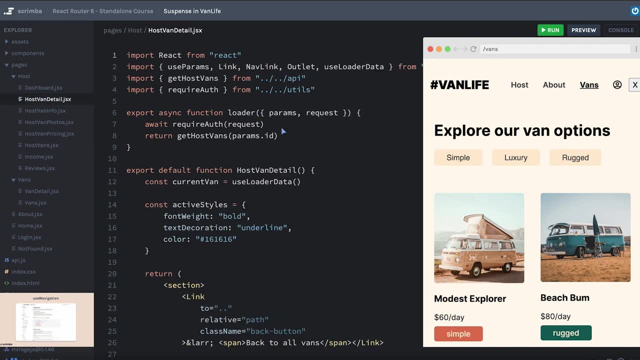 exclusively inside of our vans component here, but we still have changes to be made in the van detail page, the host vans page and the host van details page. all of these are using a loader and could potentially be using defer, like we just did in our vans page. so for the sake of some extra exercise, 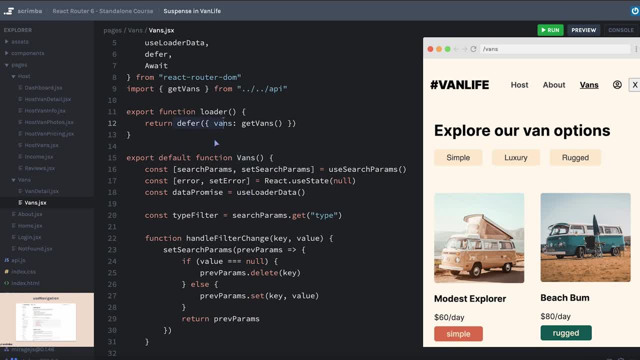 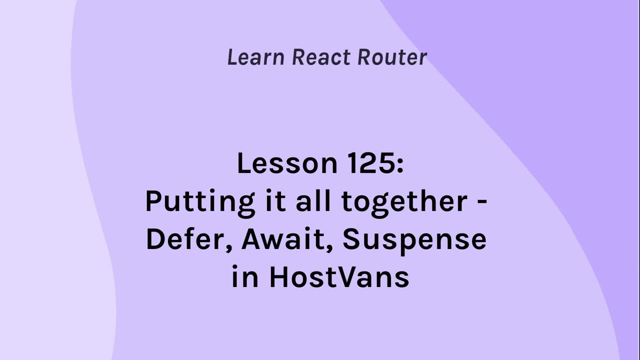 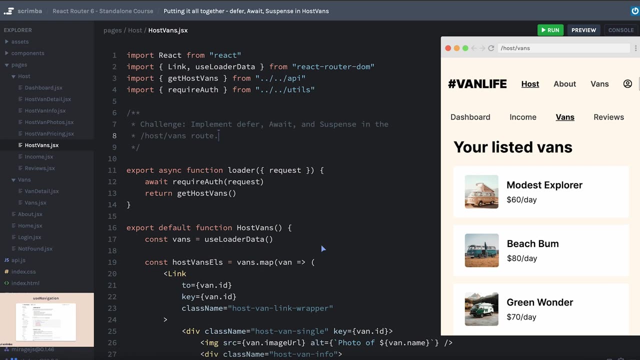 we are going to implement defer and await and suspense over in our host vans page. we're going to go ahead and do that in our host vans route. so that's the challenge that we'll be doing next. practicing one little piece at a time, i think can be really helpful for grasping the concept. 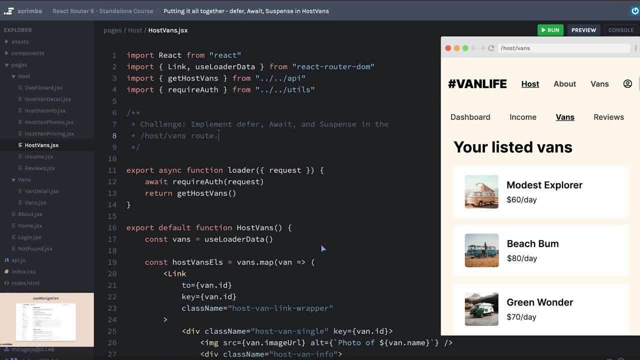 of something. but it's also super important to take the time to put all of those little pieces together and challenge yourself by doing them all at once. it's kind of like learning a new language. you could memorize little phrases here and there, but the real growth will happen as you practice. 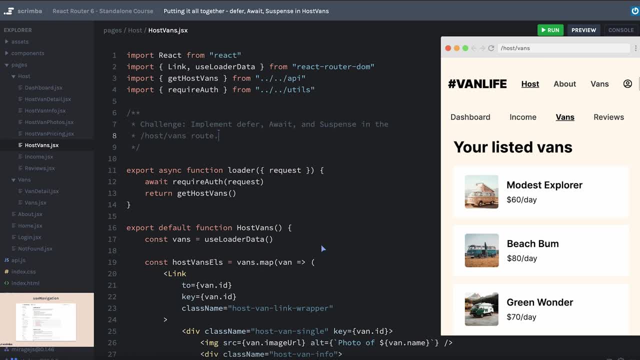 real conversations and put those phrases together: your own understanding when you're listening to someone else speak to you. maybe i'm extending the metaphor a little bit, but it's similar with music: you can practice small sections of a piece of music, but it's a whole different experience to put it all together and what people are expecting. 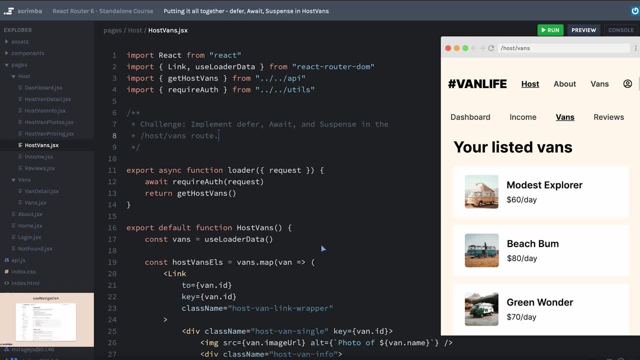 is not for you to just perform a small piece, but to put the whole thing together, and it's the same with our code here. so your challenge is to implement defer, await and suspense here in the host vans route. so pause now and work on this challenge. so let's helloым. 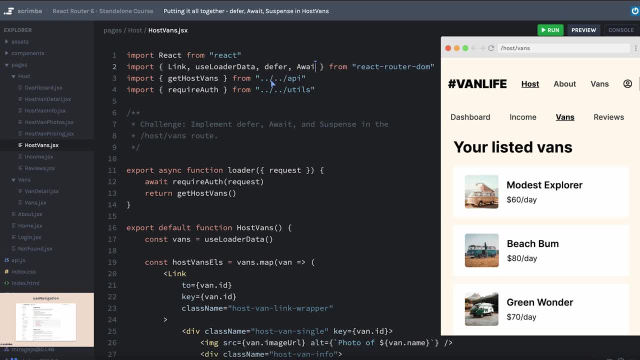 okay. well, we know already we will need to import, deferr and await, so i'll just do that now and inside of our loader we are going to return a call to defer. let's wrap that in that function and defer expects us to pass an object and we'll give it the key of vans. 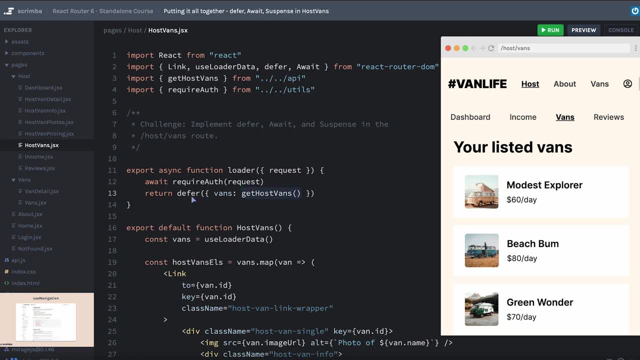 okay, so now this should be a promise that will get resolved eventually. but we will not wait for the route transition to happen, but instead we will defer this data for a while in our div and we'll end up waiting for theну. we're going to close out the disk. we'd probably do that just in the word. 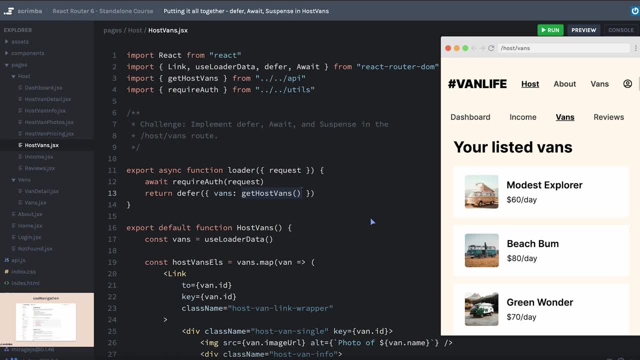 and we're going to do that just in the word. so you go letters together that you'll find. the link to our drena still doesn't always allow you to ever print, but i'm gonna show you how you write you as you go through that. for after the route transition happens. okay. so inside of our host vans- we were calling this vans- 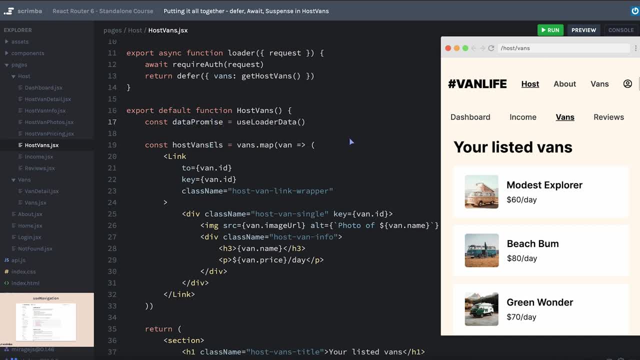 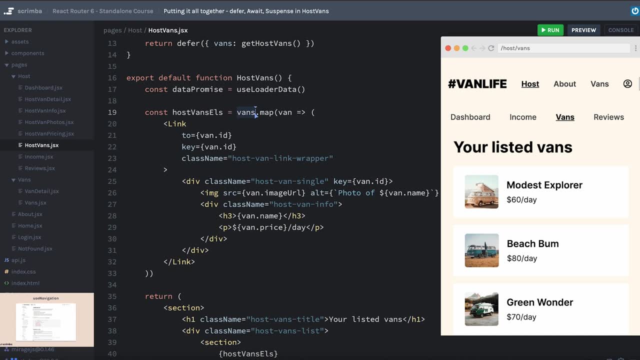 maybe let's call this. i think we chose data promise before. let's just stick with that. we'll say data promise is coming from use loader data and our host van elements needs access to vans in order to successfully complete the map. so let's do what we did before, where we create a function. 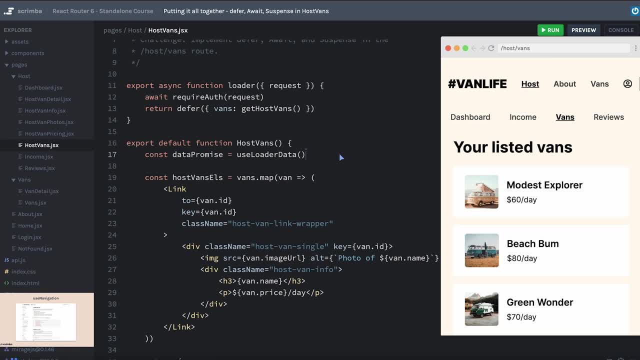 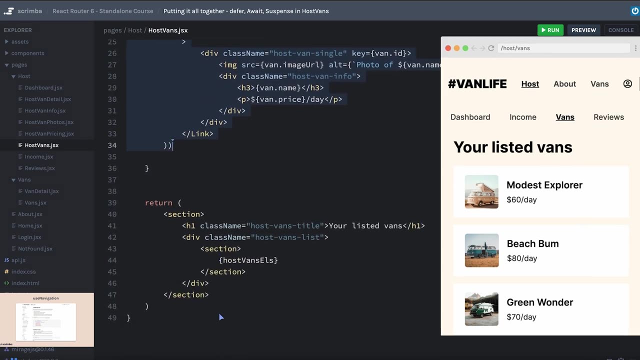 and that function will be in charge of all of the rendering tasks here. so we'll create a function that we'll just call render. let's see, render van elements. that's going to take the array of vans and we can move this host van elements inside of that function and i'm going to keep my h1. 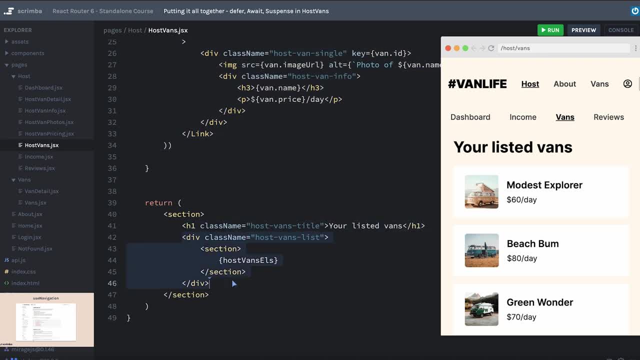 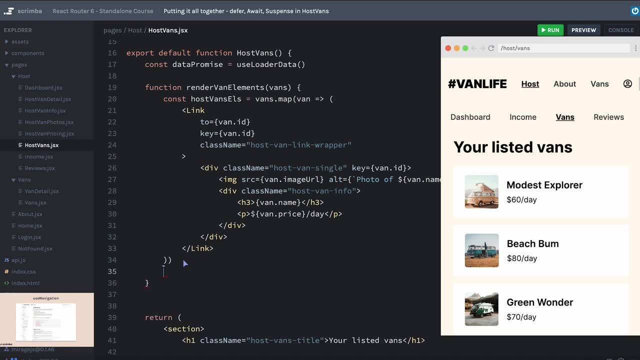 like we did before. but we will return this. so let's cut this out and inside of our render van elements. so i guess it will be right here. we'll paste that in. actually we need to return that, so i'll type in return and then paste it in, and now we have a function which. 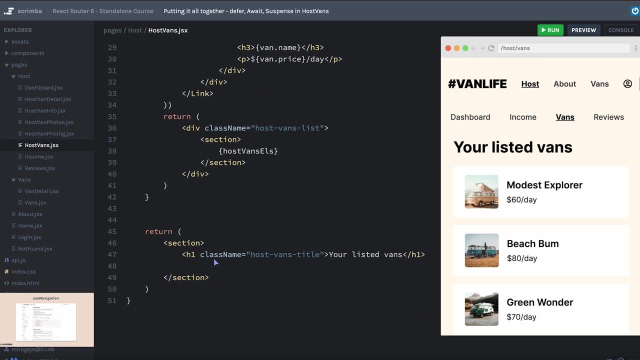 will be the render prop child function that we pass to the await component. so let's render weight and as the child of a weight, we will render the van elements and we need to tell it what it needs to resolve. that's going to be our data promise dot vans. okay, and since await. 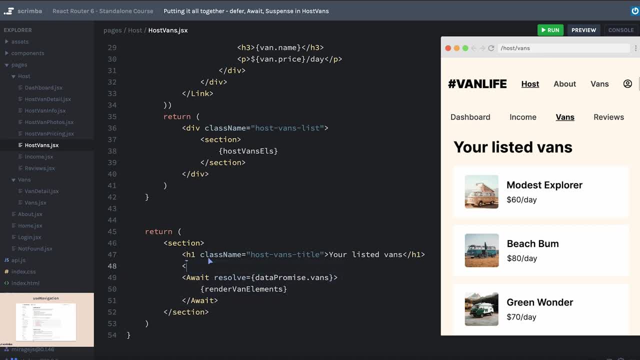 will suspend rendering. we need to provide the suspense boundary, so that's with react dot suspense, and lastly, we just need to provide the fallback, not finally back prop, so that it knows what to do. of course, this is where you'd probably be better off putting something a little fancier, like a fun spinner of some sort, or maybe something animated that makes 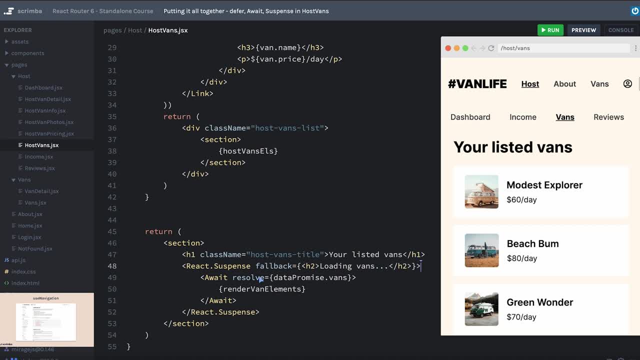 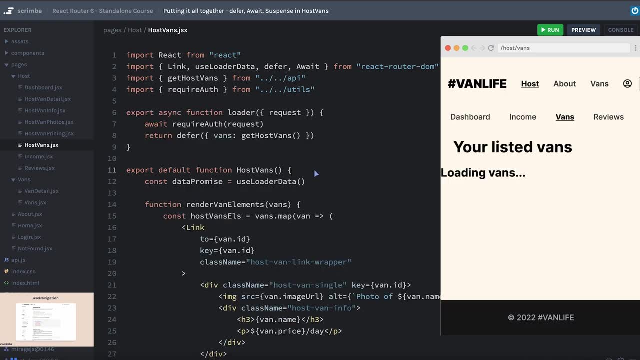 it a little more exciting than just saying loading vans, but for now this will get the job done. okay, let's see how we did. we'll clean up the challenge text and hit save. okay, and it was. it was pretty brief. it showed up as loading vans for just about a half a second while it was loading. 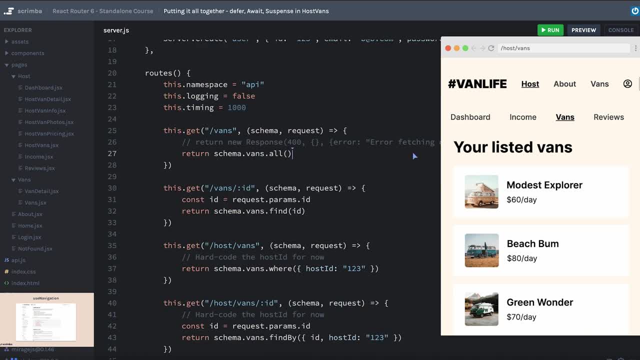 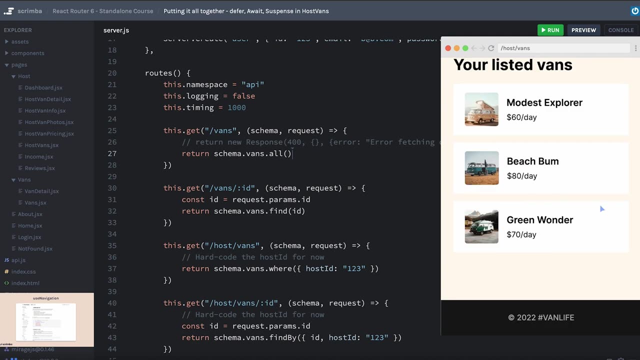 i guess it can come back to my server and putting this timing delay and hit save. we'll see if that makes a difference. let's hit refresh. okay, we get loading vans and then the fans come. in. this way, the transition to the vans page is really snappy and we at least get some kind of feedback that says that the rest of the ui 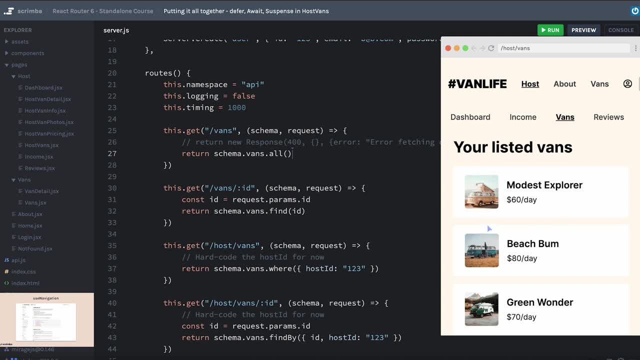 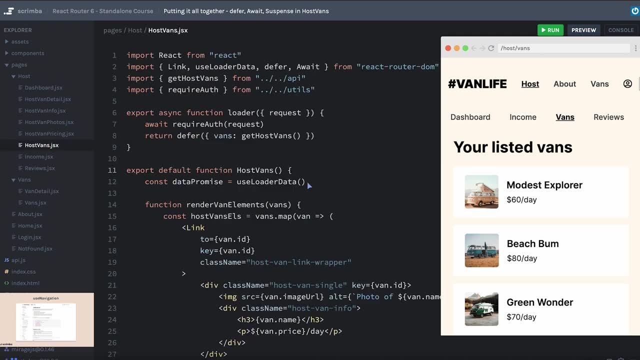 with the vans is still loading. awesome work. i hope that went okay. putting it all together can be a really good experience, especially when we see in the end it truly wasn't that much work to do and instead we got to simplify quite a bit of our code, or at the very least we got to give a little. 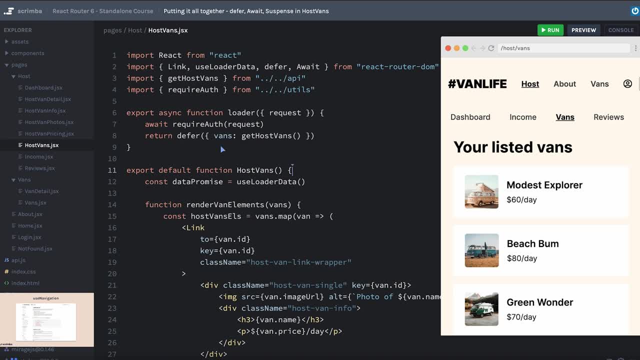 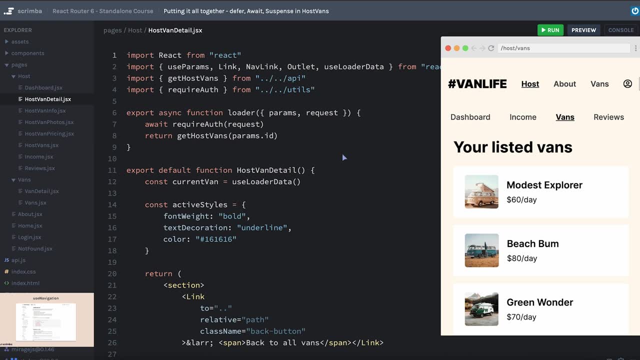 bit of a better user experience to our users. now, at this point we still have our van detail page and our host van detail page, which is not using defer, await and suspense. but for the sake of not beating a dead horse, i'm going to actually implement those myself for the next scrim that 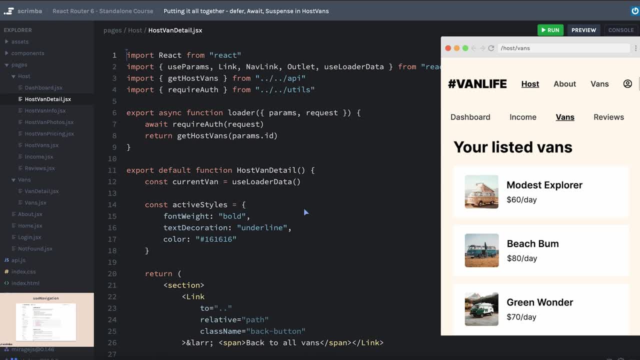 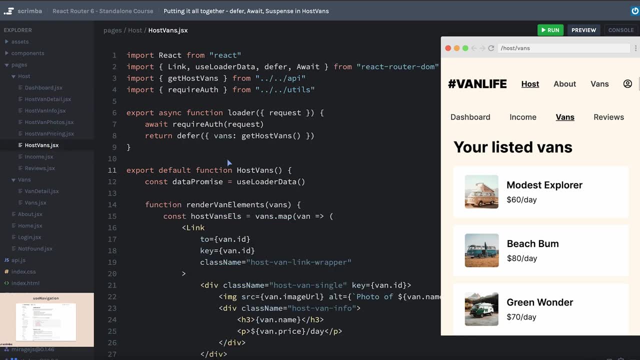 said, if you would like to practice this even more, you can go to the van detail page and the host van detail page and do exactly what we just did in the host vans page: implement, defer, await and suspense. just to get a little extra practice, i'm going to leave it up to you. i trust you to know that if you 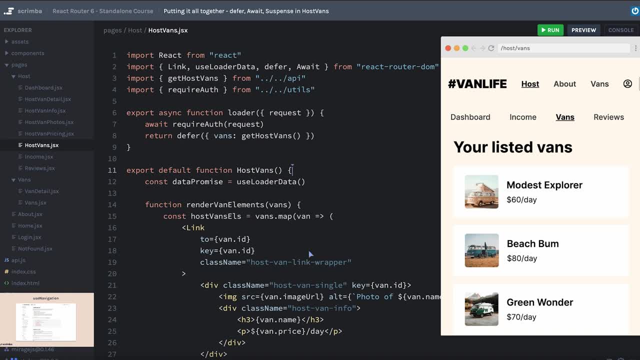 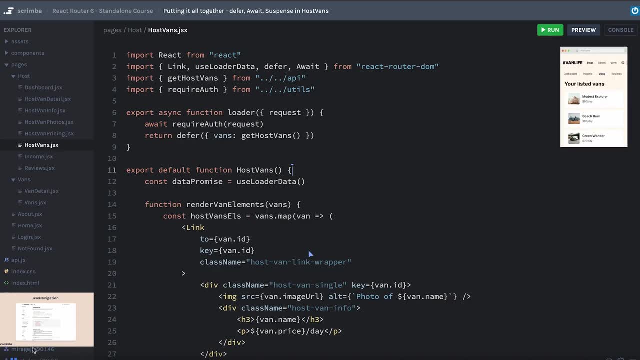 need more practice with this. you have some places where you can do that more practice and if not, you can move on. we have just a couple of little loose ends to clean up, so that's what we're going to do in the next lesson. look at us here at the end of this project, just dotting some i's and crossing. 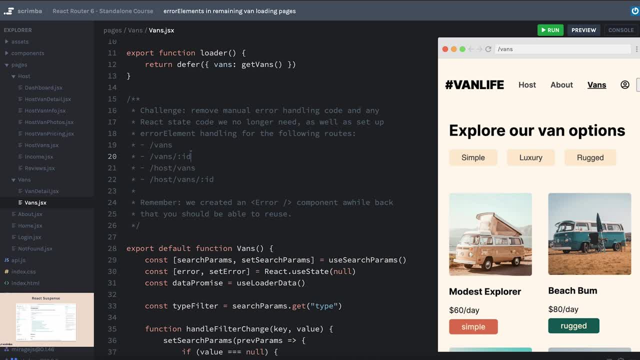 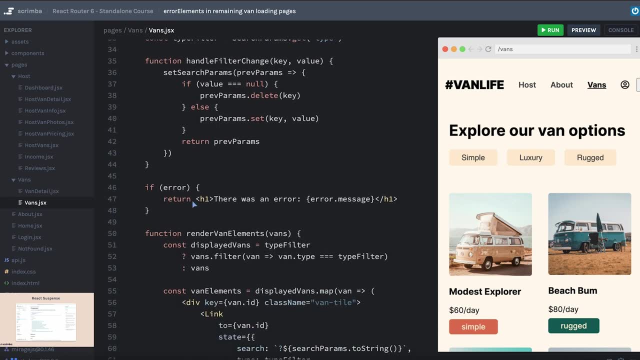 some t's before we can finally move on to the next lesson. call it done. one thing we can look closely and notice is that we are still doing a little bit of manual error handling. here we are maintaining our error in state and down. here we have an early 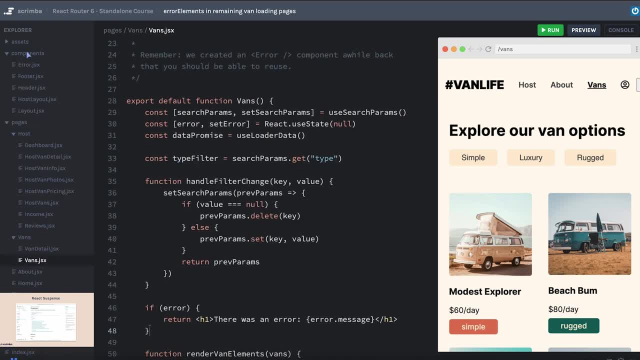 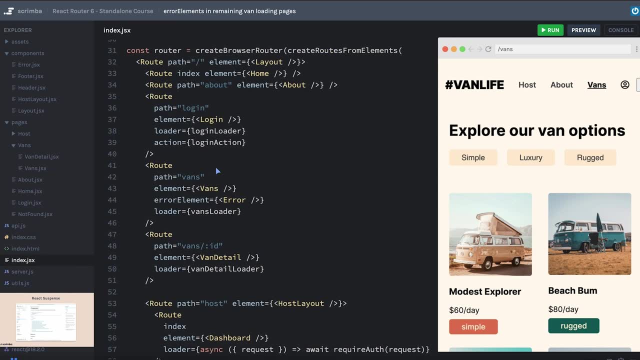 return for the error. but a while back we did learn about the error element, property or prop on routes. let's see, let's go back to our index here and if we go up here on our vans route, we have this error element that is handling this for us. but we haven't yet implemented that everywhere. 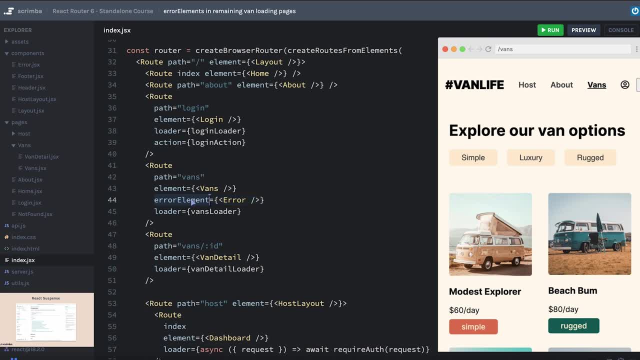 that we might need it as a reminder. the error element will render this error element to the error component anytime there is a thrown error, either inside of this route or inside of any of its children routes, if you've ever created an error. boundary component using class components. 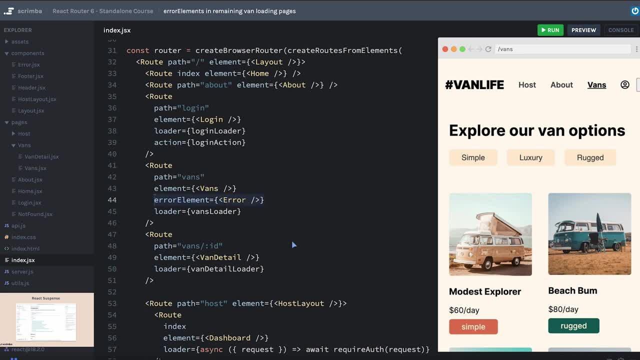 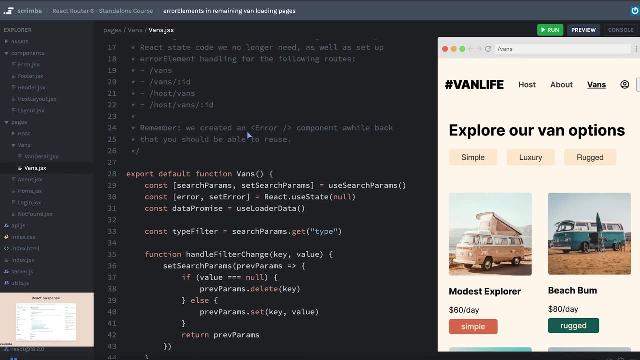 this essentially gives us a really declarative way to create those error boundaries on the route level. but we have only done it here on the vans path, so let's open up our vans page again, where our challenge text is: your job is to remove any manual error handling code, which i believe is. 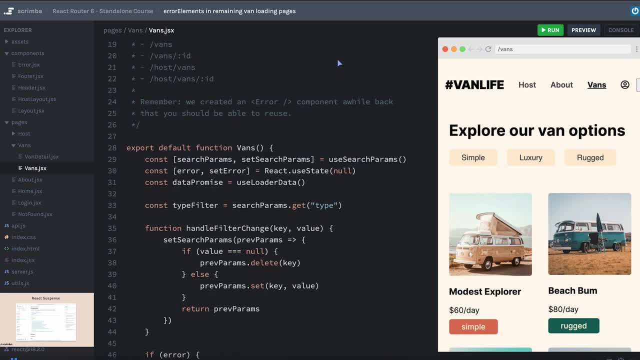 only in this component, this vans component right here, and all of the other components that we've already created. so we're going to go ahead and do that and we're going to go ahead and do that and also to set up an error element for error handling on the following routes that i have listed here. 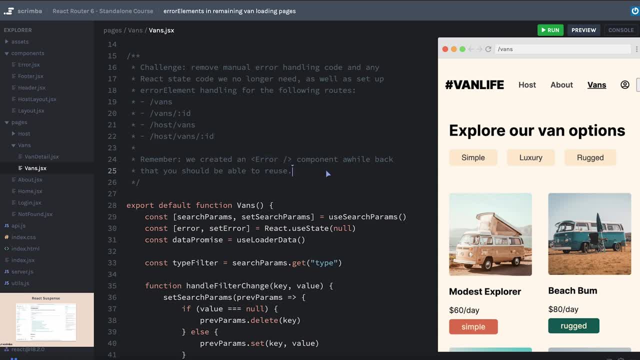 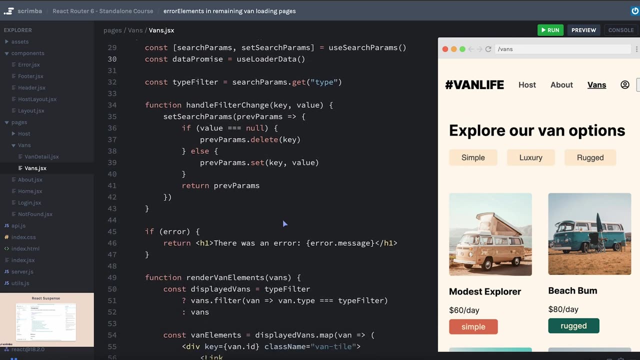 as i mentioned, we created an error component that you should be able to reuse for those error elements that you put on the routes. so pause now and work on this challenge. okay, well, let's get rid of our react state here and this early return. we don't need those. 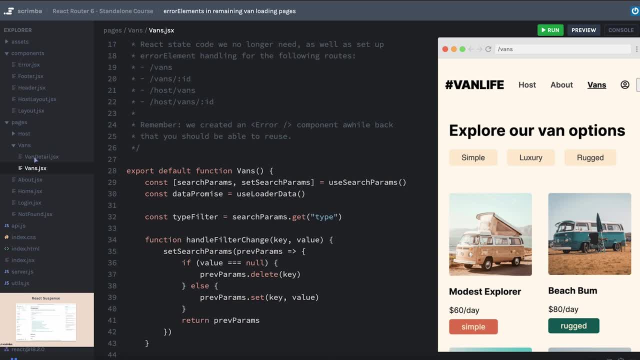 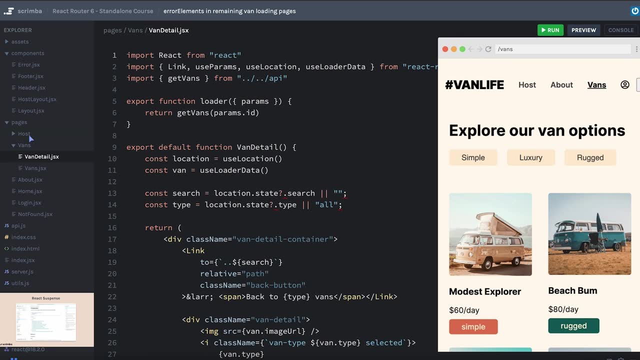 and actually this should be pretty simple. i'm just going to check just to make sure, but it looks like i don't have any react state that i'm maintaining here or any error handling over in my host pages. we've got host vans. yep, it looks like we already removed the error handling. 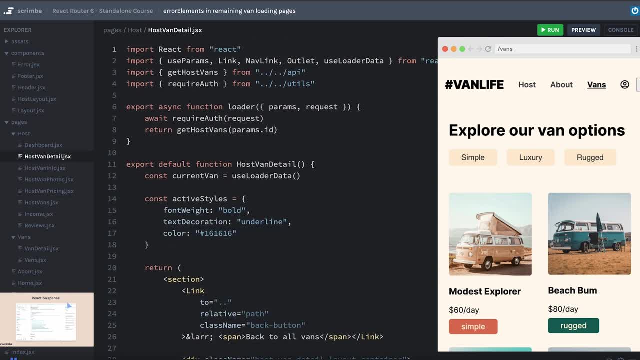 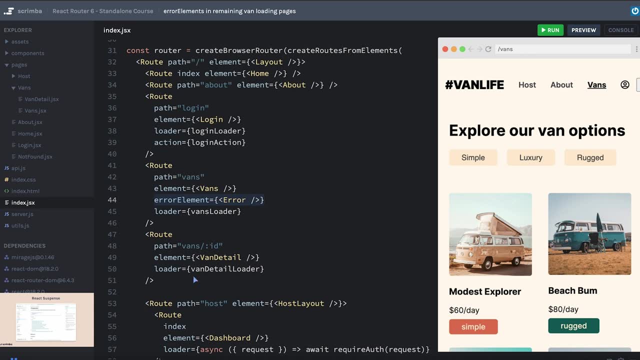 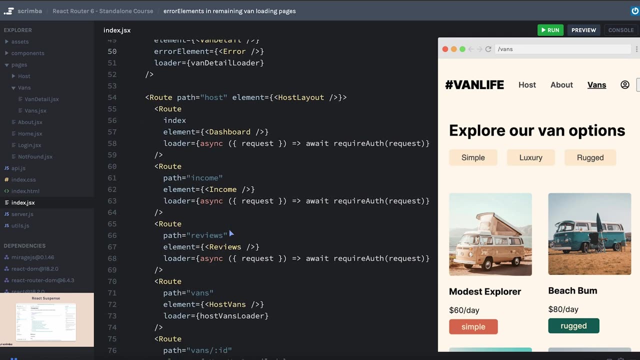 there and host van detail same thing there. okay, so we should just be able to go over to our index page and, honestly, i'm just going to take this error element of error and start pasting it everywhere that needs it. this is our van detail page. we want it there. we also want it. let's see here: 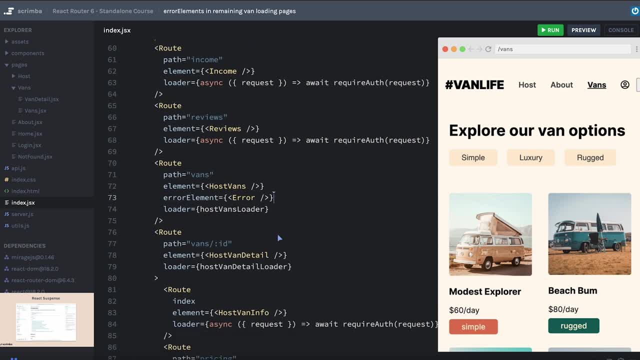 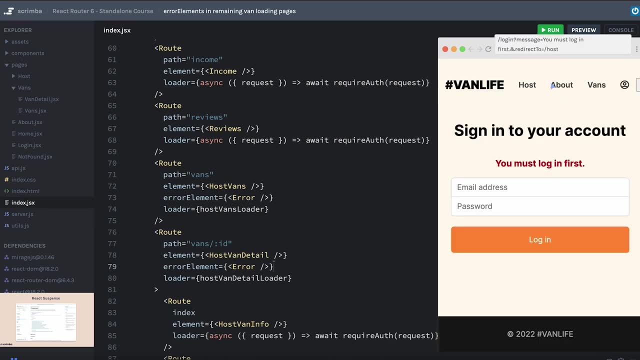 we have a loader that is grabbing some data. we'll put it there and with our host van detail page, okay, let's hit save. we're going to log out. just to make sure that we're logged out, we'll go to the host page. you must log in first. if i try to go to slash host, slash vans, okay, we get the same thing: log in. 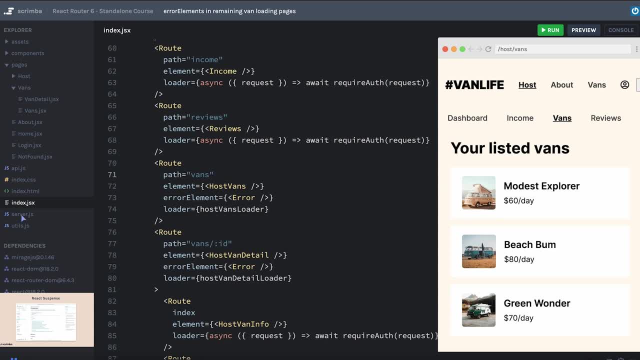 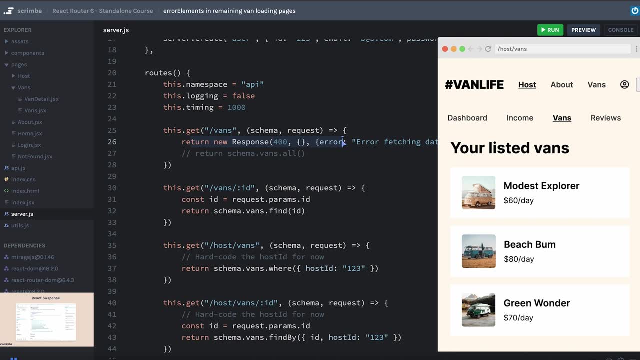 okay, that loads just fine, and then we can really test this by going to the server. and here on the vans page i have this commented out, just in case i needed it again: we're just going to hard code a 400 level response from the server and i'll go to vans and okay, it's not super. 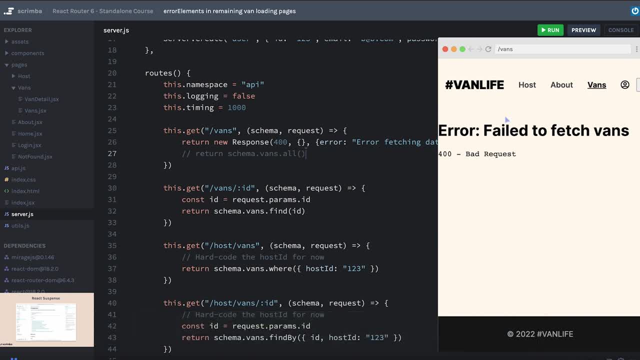 pretty. we could probably make some improvements here, but at least our app is not completely crashing because we have this error boundary. let's undo this so that we aren't hard coding an error and we'll refresh just to get our vans back. you have been doing an amazing job following so far. 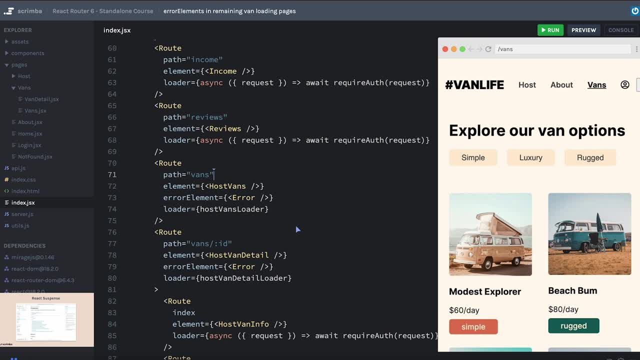 so you should definitely take the time to congratulate yourself, and if you've been sitting down for a while, maybe it would be a good time to go back to the server and see if there's anything that you've learned and accomplished in this course. while we're on the topic of dotting our 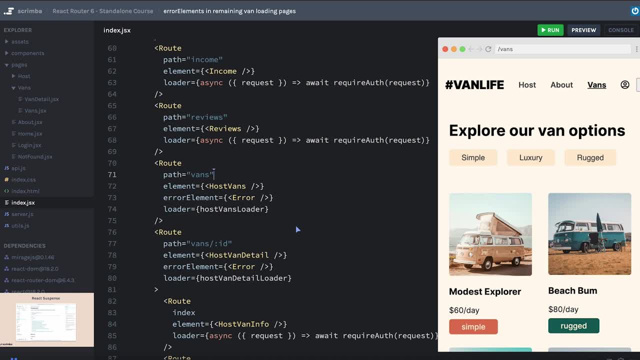 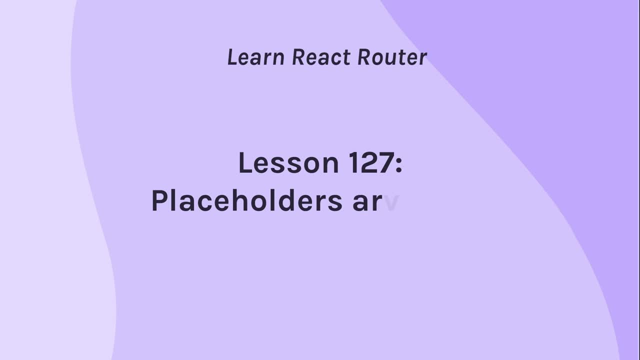 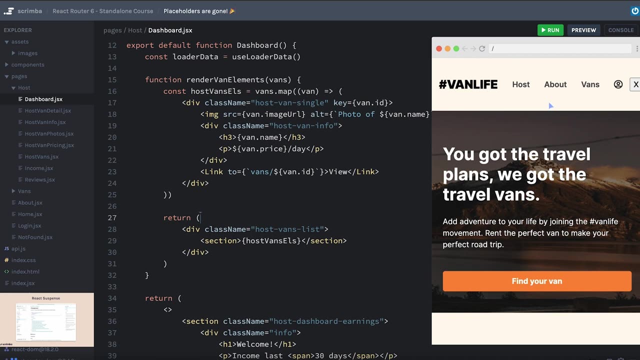 i's and crossing our t's. i do have a little present for you, so i'll reveal it to you in the next scrim now. we have been staring at these- default dashboard goes here, income page goes here pages for far too long, and so my surprise to you is that i have completed them for you. 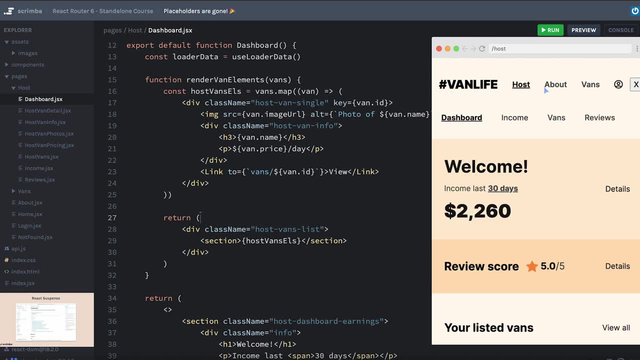 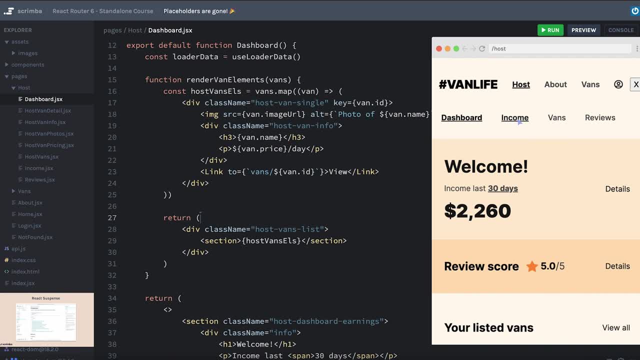 to be honest, i've taken some pretty serious shortcuts here just for the sake of getting the design up. if we come to the income page, we can see this graph. well, it turns out this graph is just an image, and the image is completely static. it's not pulling data from anywhere. 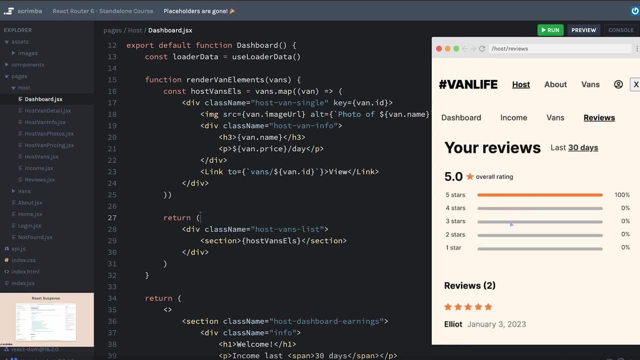 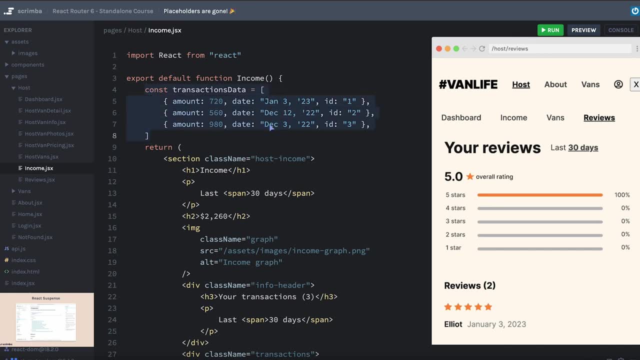 i've done the same thing over in the reviews page. we have this reviews bar chart and this is just an image that's being rendered here. if we go to those pages- the income. i just created a transactions data array that we're looping over and displaying same with reviews. we just have some reviews data. 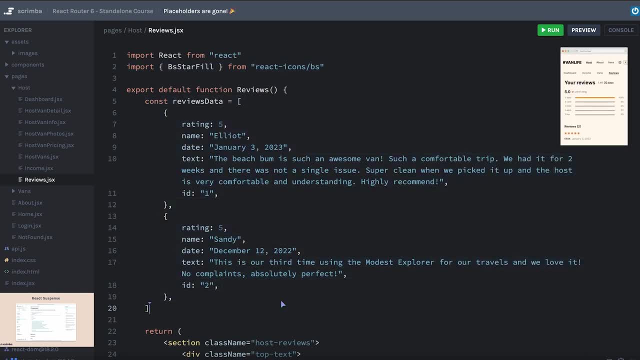 hard-coded right here inside of our component. of course, if we were doing this for real and we actually had a server where we could get this data from, we would be pulling this in inside of our loader instead of doing it in any kind of use effect here inside of our component at this point. 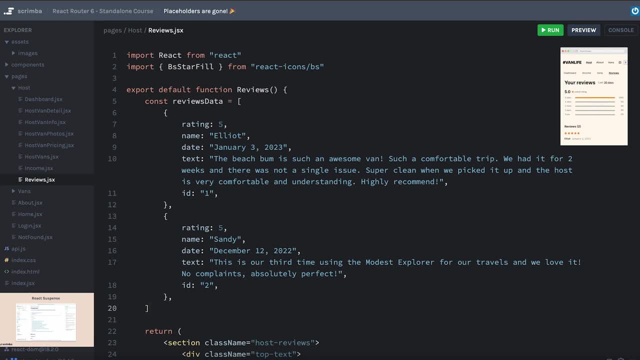 in the course we have covered all of the topics that pertain directly to react router that we planned to cover. i suspect you have spent a fair amount of time on the react router documentation, as i have sent you there a number of times throughout the course. so when you find yourself, 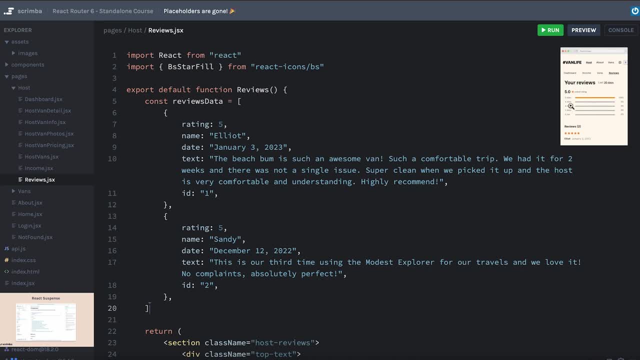 working in react router in your own browser. you can use react router to do all of the things that you need to do in your own projects. hopefully, you not only feel really comfortable with the topics that we have practiced and learned, but also feel comfortable going to the documentation and learning. 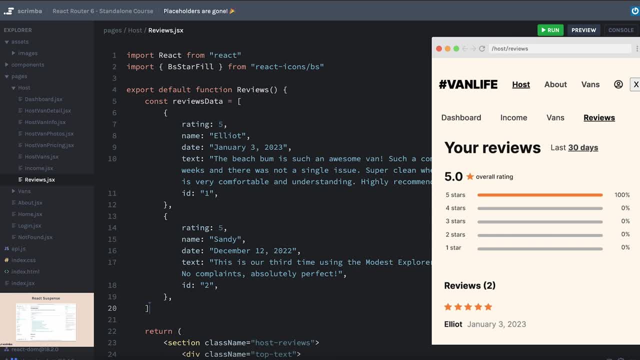 what you need to learn. i also can personally recommend that you check out the remix discord server, since react router is a part of remix. if you have any questions about react router, there's a really great help channel there that some of the core contributors to react router and remix will. 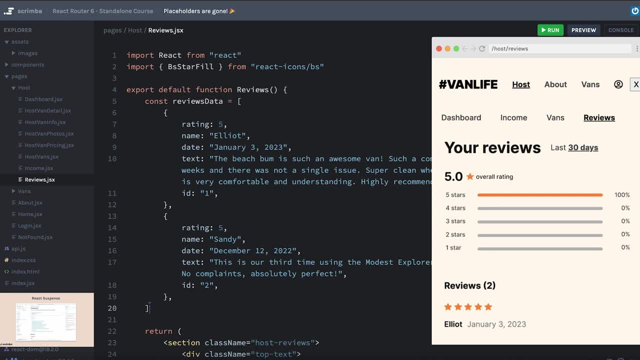 oftentimes be able to answer questions from. in the last part of this course we are going to be jumping into using firebase as our mode of use for our project. so if you're interested in using firebase as a tool, you can follow the link above here to download the actual database and then. 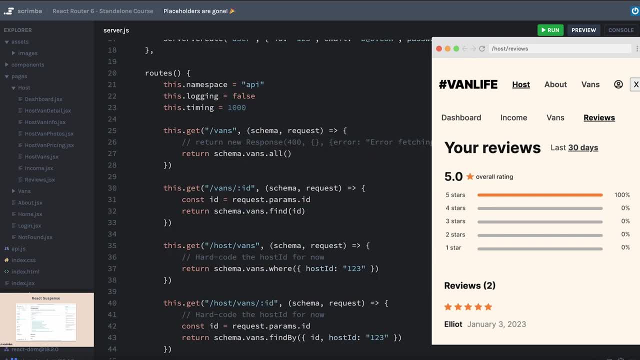 download it to your Mac and on the right side of the screen we have the first step of storing our data and grabbing data from a real database online. our mirage js server has served us really well throughout the beginning parts of this course and, as a final way to tie the bow on this app, we're 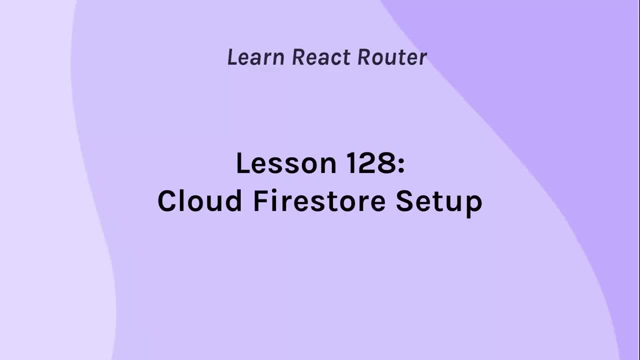 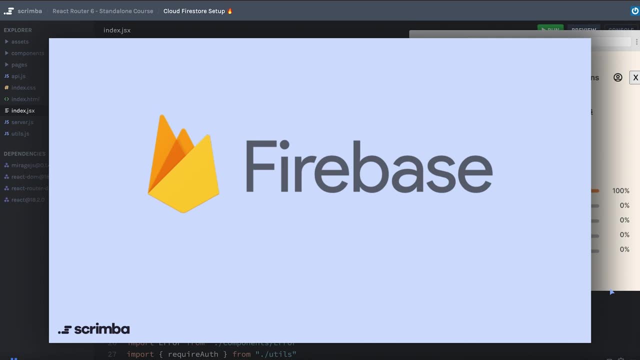 going to migrate our data to cloud firestore, which is a part of firebase, and refactor our app so that we are pulling data from a real database. as i mentioned, mirage js has been an awesome server for us thus far. however, it's time for us to move on to a real online database and we forward it to a new. 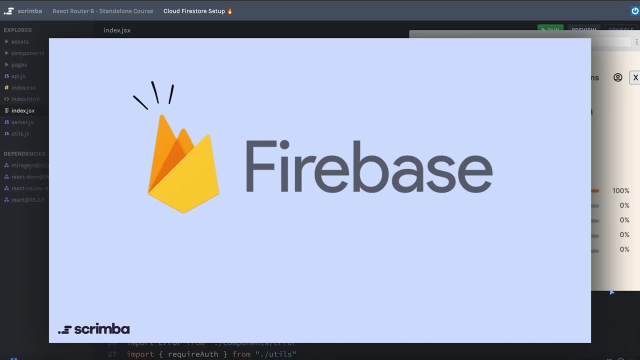 console, which will take us back to where we started our project. so here's how we take our data and read our data. through a different database, we quickly vinegar our data and take it into our directory. we'll keep a so that we can really round out this project piece and if you're someone who's searching for a job, 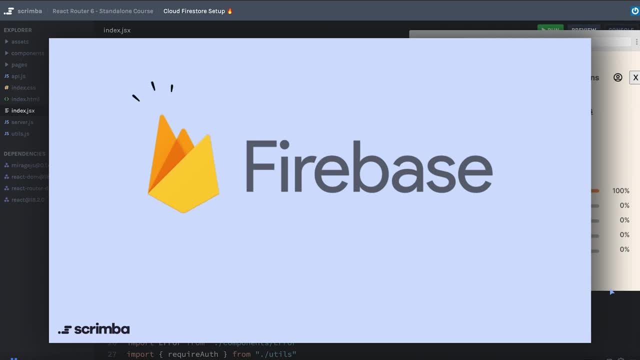 especially if you're just learning web development for the first time. using a service like firebase can be a great way to get real data, real api endpoints that you can reach out to without necessarily having to build and maintain your own server and database. so for this lesson we are: 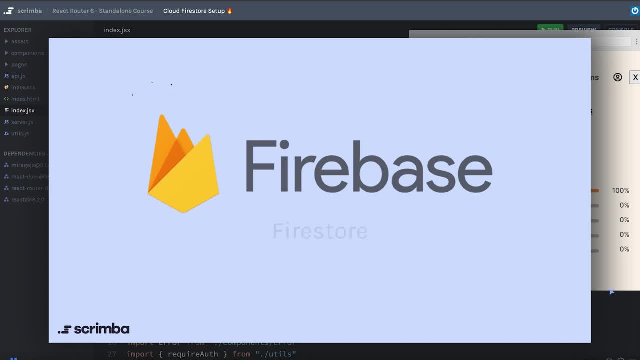 going to walk through how you can set up firebase and, specifically, we're going to be using firestore, which is one of firebase's databases, so that we can migrate our data over to firebase, and if you are following along here on scrimbacom, then this would actually be a great time to stop following. 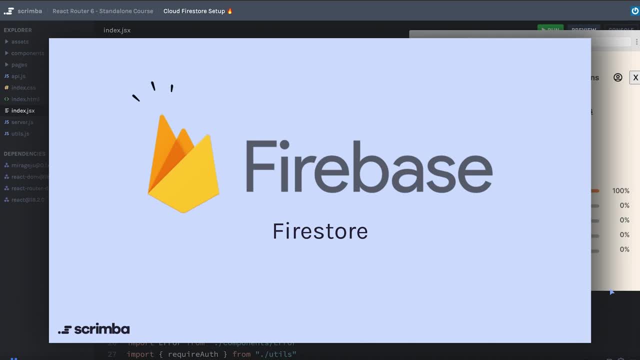 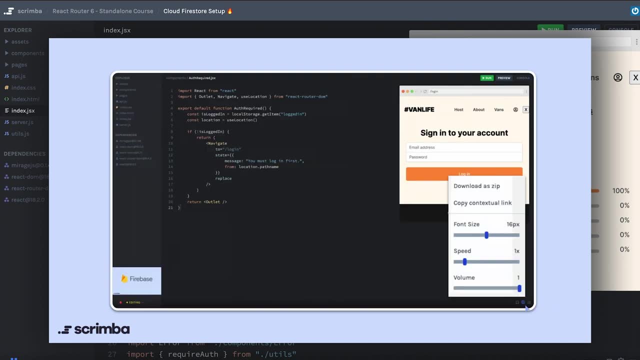 along here on scrimba and actually download this code to your local machine and follow along on your local machine instead. in order to do that, you can go down to the little gear icon in the lower right now. at some point in the future, scrimba's design is going to change, so it's. 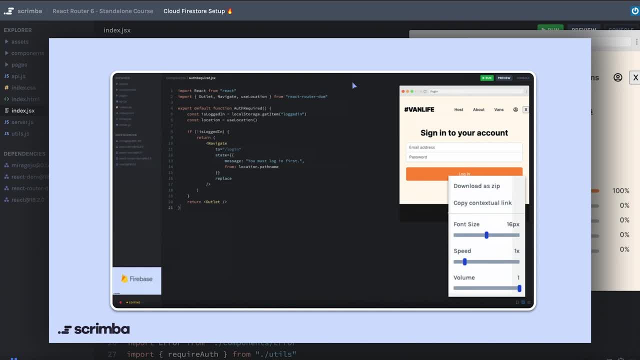 possible that this gear icon may not be exactly here. in fact, everything might look completely different. but either way, you can search the app for this option that says to download as zip, or at least worded something. you can search the app for this option that says to download as zip or at least worded something. 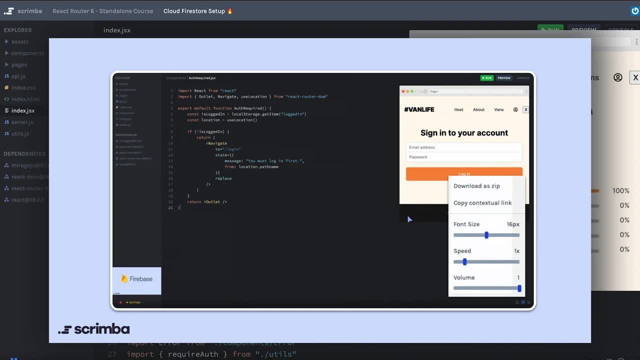 similar to that. once you download this project to your local machine and unzip it, you should have access to a folder. now i'm going to be using vs code for my editor. you can open that folder in whatever editor you prefer, and then you need to install the dependencies. now i've done that here. 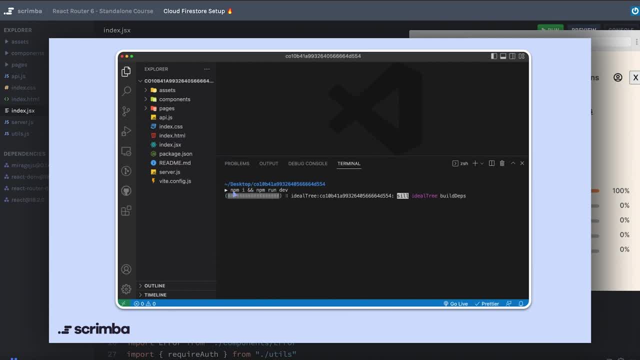 all in one line with this double ampersand. so what i did is i ran npm install, or npm i for short, and as soon as that finishes, i'm going to run the development server by using npm run dev. you can see that under the hood, we're using veet in order to package. 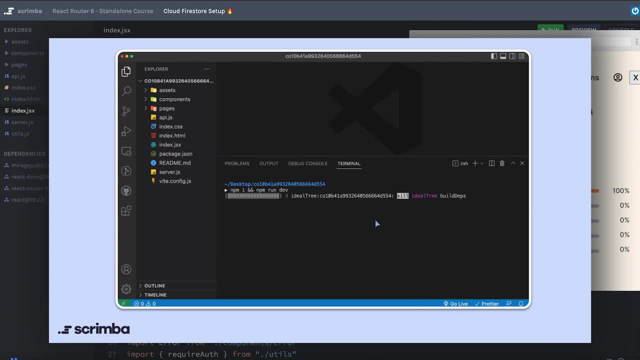 and bundle everything up, and it should be really quick when you do this. once that's all set up, you should have a new folder called node modules in your project and it should tell you that you have a local environment. the default, i think, is at port 5173, where you can open up this project locally. 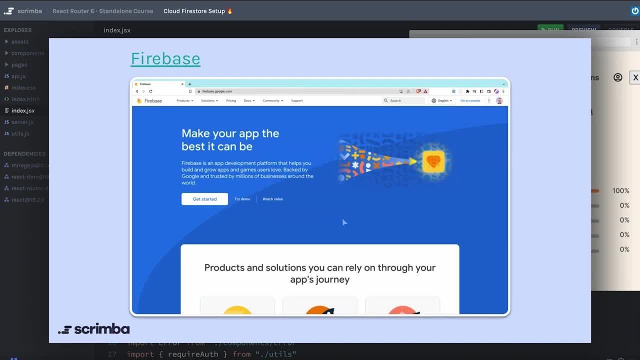 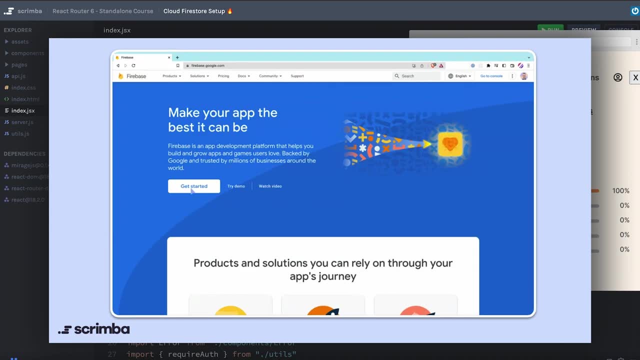 okay, at that point we can head over to the firebase home page. you can click the screenshot here to head directly there, and once you are there on that site, you can click the button to get started. that'll take us to a screen where we can create our first project. so we'll click. 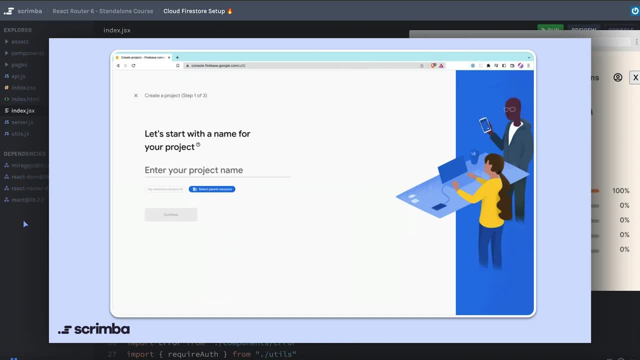 the button create a project, we'll enter a project name- i'm just going to call it van life- and we can hit continue. at that point we'll be given the option to include google analytics in our firebase project, if you would really want to. this will take a bit of extra setup, so for now i'm just 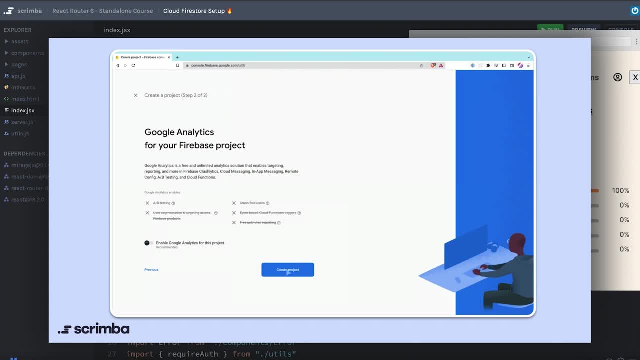 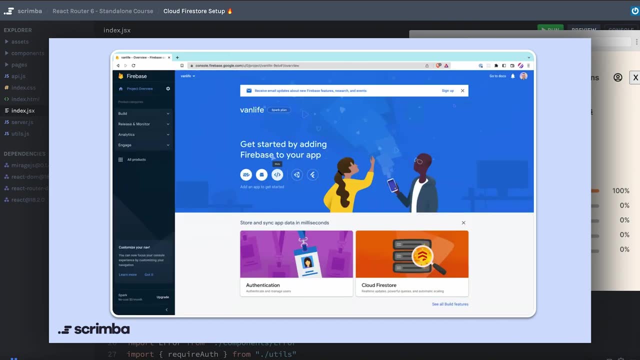 going to uncheck that and then click create project. we're then sent to a loading screen and when it's ready we can click continue and that will drop us into this project overview page, which is sort of a dashboard for this van life project. firebase projects can consist of multiple different applications, like, for example, if you had an. 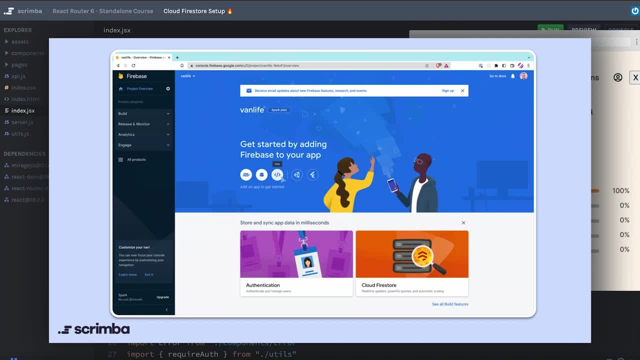 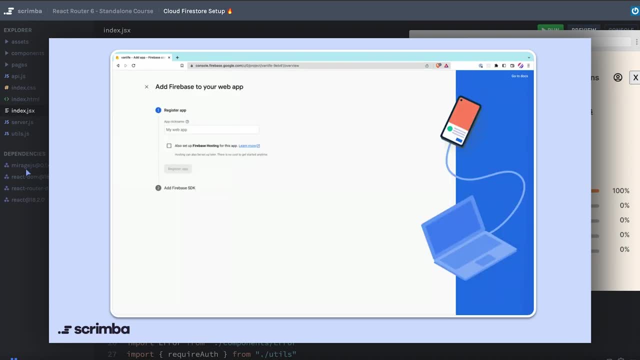 ios app. that was a dedicated ios app and a dedicated web app. for now, we are only concerned with the web, so i'm going to click this little angle brackets web icon here. in order for us to register our web app, we need to give it a name. so i'm going to just put in van life here, or if you. 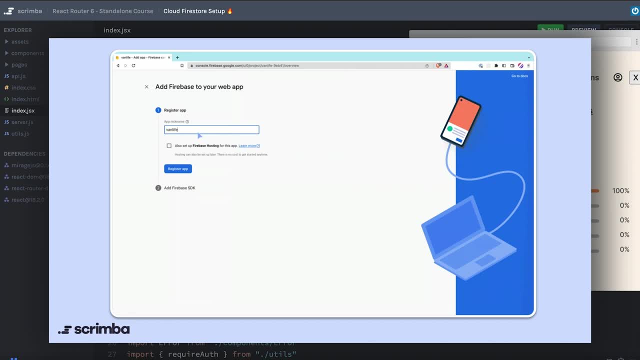 knew ahead of time that you were going to have other apps. you might call this something like van life web, and then i'll click the button for register app and this will give us some important installation information that we are going to need. so this would be a great. 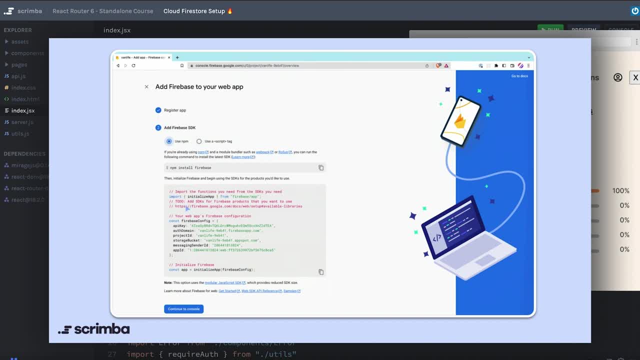 time to click the little copy button, or, of course, you can highlight it and copy it. if, for some reason, that gets lost after you copy it, that's okay. it's pretty easy to get back here and i'm going to show you how to do that. once you have that, you can click continue to console and this: 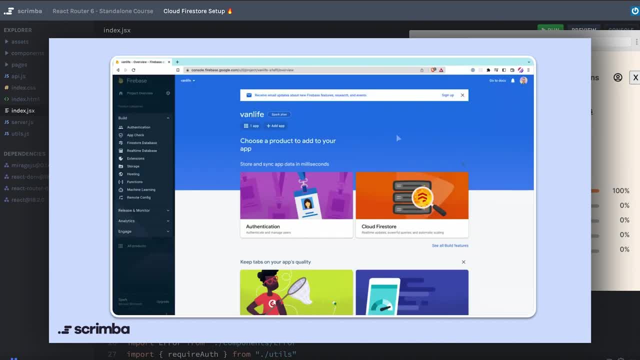 will drop us into the web app that we just created for van life, and the next step is to tell our van life project that we want to use firestore as our database. so probably the most accessible thing is going to be the build option. so you can see that there's a orange rectangle here that says cloud. 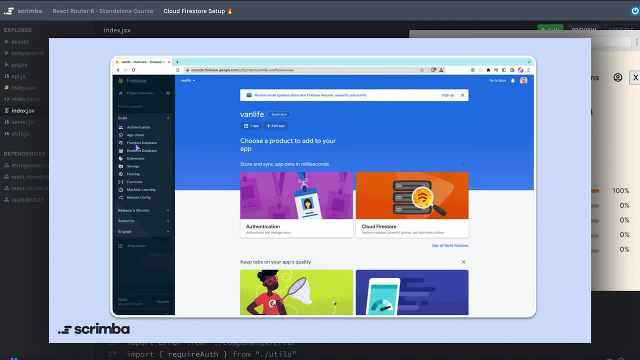 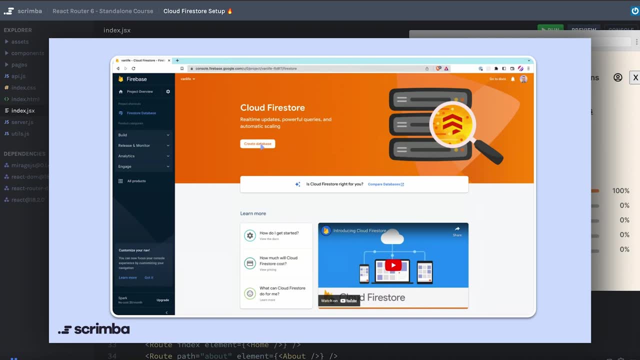 firestore or over on the left you can drop down the build option and click the firestore database there. clicking either one of those will take you over to the cloud firestore home page where we can click this create database button. it's going to ask us if we want to start in production mode or 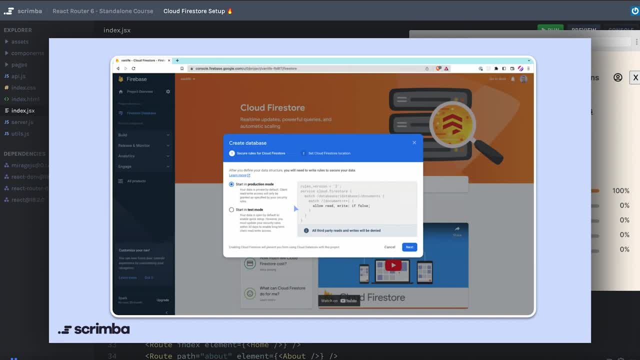 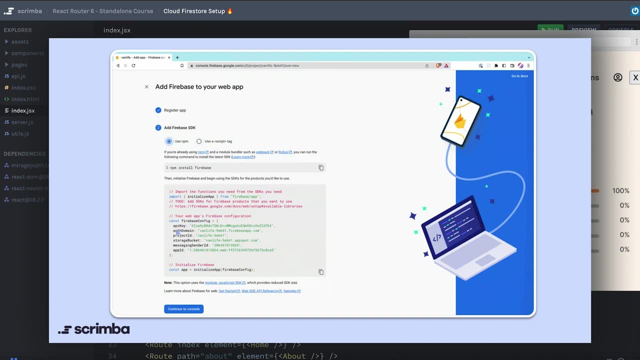 test mode and this is kind of an important thing to understand about firebase. you might have noticed that a couple slides back. i was completely okay exposing this api key and if you are familiar with it you can see that it's a little bit different than the other ones, but usually you want these to. 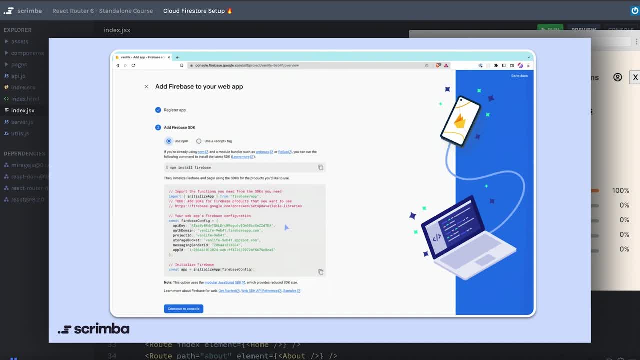 remain secret. for most api keys that i've used at least. they expect that you keep the api key hidden, you don't commit it to your github repository and you only make requests using that api key from a server of some sort. however, firebase is a little bit different, and that's because they use something. 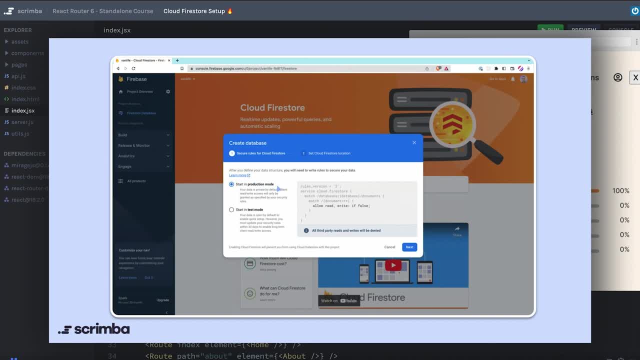 that they call security rules in order to secure your data. so you can see here in production mode if you look closely. it says allow, read, write if false, which means that nobody, not even yourself, is allowed to read and write. this is their way of forcing you to take the time to learn about. 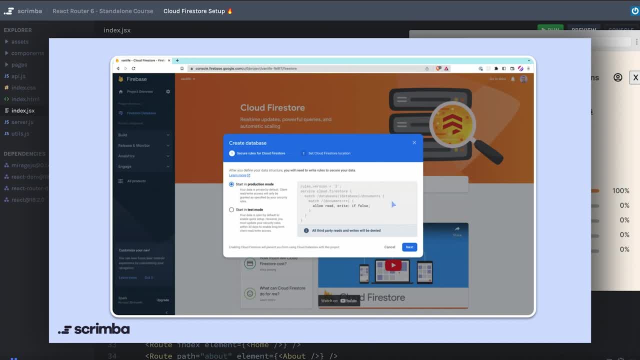 security rules and actually implement what makes the most sense for your needs. but for us we're going to be okay, just starting in test mode, which basically says you are allowed to read and write for about the next month from when you created this database. for now that's going to work okay. 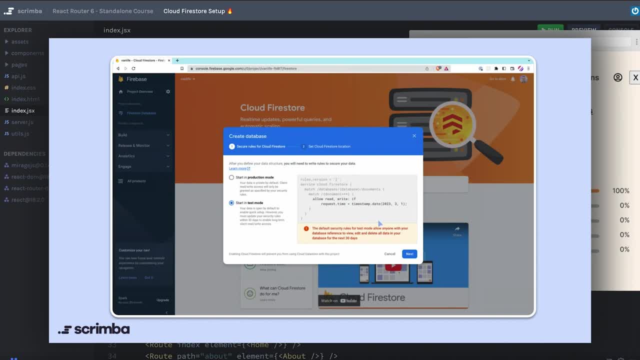 for us. you will need to make sure that you look up a little bit about how to create security rules with firebase, but for now this is going to work okay for us, so i'll go ahead and click next. it's going to ask us to set our location. 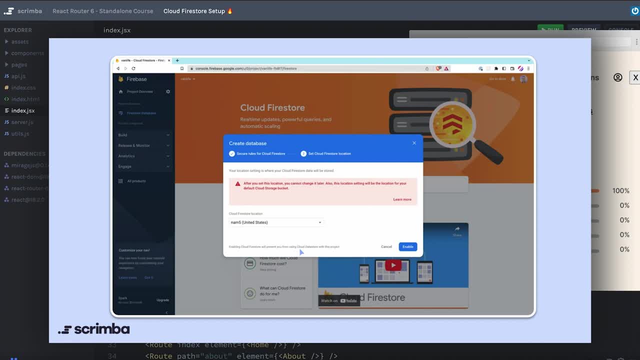 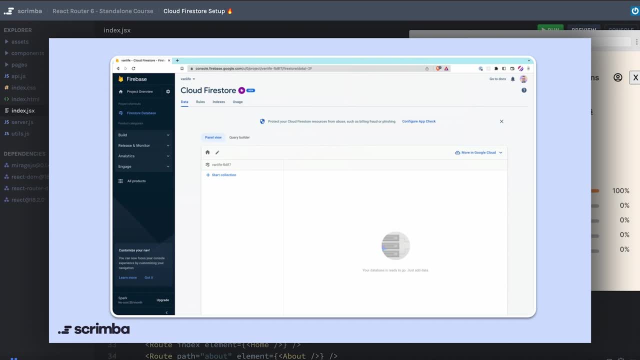 you can click the drop down and just choose the location that is closest to you geographically and then click enable. that will drop you into the cloud firestore database view where, once you have some data in here, you'll be able to actually peruse the data and see all of the data that you 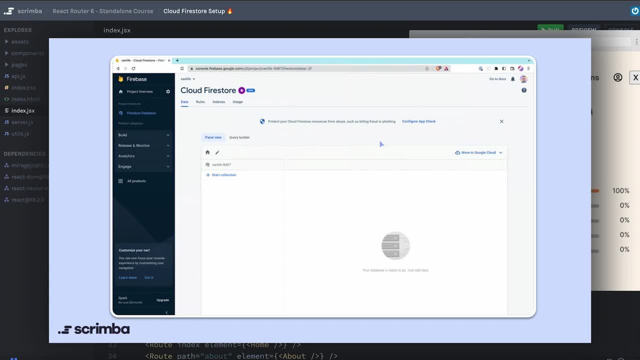 have in your database. what i did on my instance of this database is i actually just copy and pasted the data that we have from our six van objects and put it here in cloud firestore for us so that as we start doing our refactoring we are primed to grab that data from firestore. 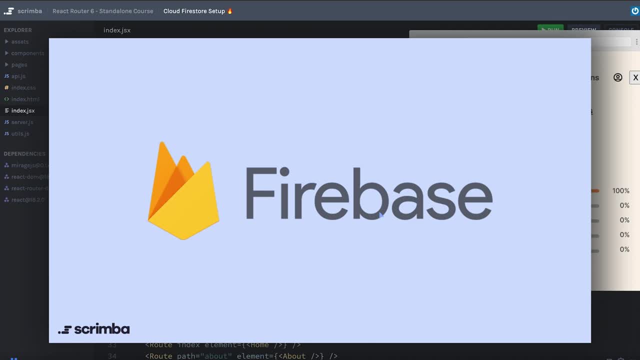 and that is it. we have set up our firebase firestore for us to start making changes to our code, and even though that may have seemed like a lot of different steps to take, if you think of the alternative, which would be to spin up your own server and connect a database and have database, 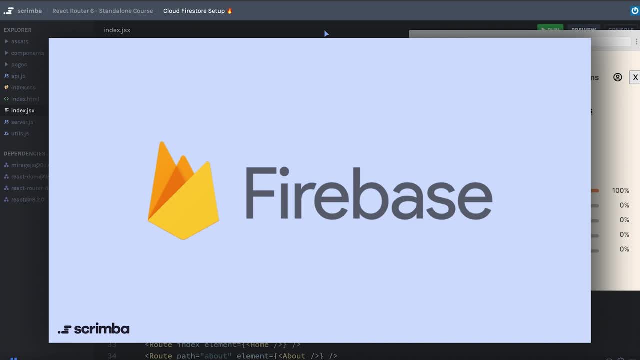 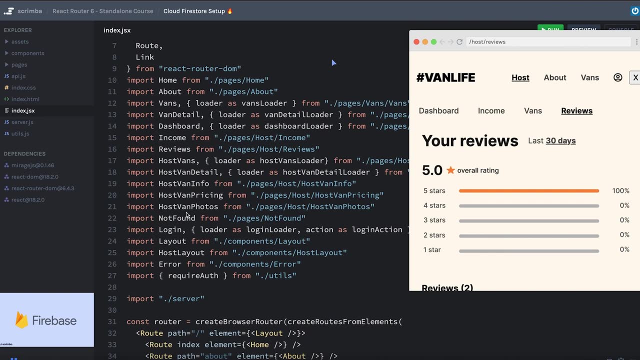 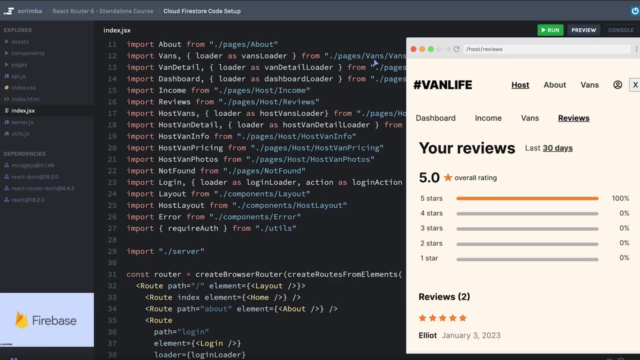 structures and everything set up. this truly was like a walk in the park. so let's jump into our code and we will start making refactors so that we can pull data from our firebase firestore instead of using our fake mirage js server- one really nice side effect of us having put all of our fetching code here inside of our api js file. 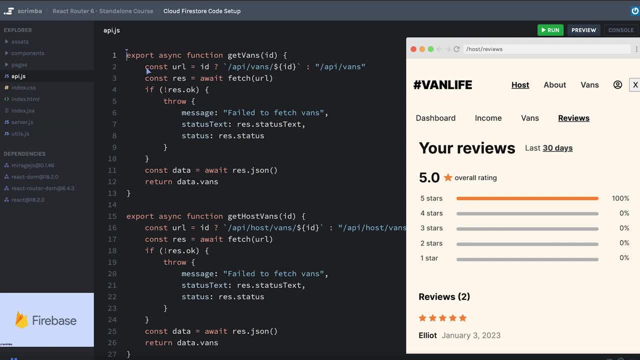 is, i won't have to go to all of my components in order to change where i'm getting this data from. right now, we're doing a fetch request to this local api, which is handled by mirage js, and all we need to do is change where that data is getting fetched from. so that's what we're primarily going. 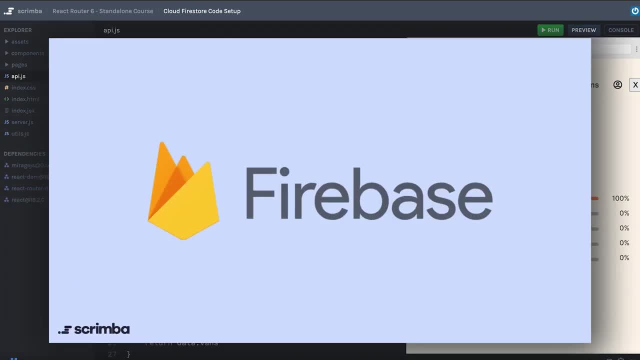 to be working on. but first we need to set firebase up in our code so that we have the ability to access our data from firestore. you might remember me asking you to copy down that configuration object. if you did, great, we are about to use it. if not, it's pretty easy to get back to from your 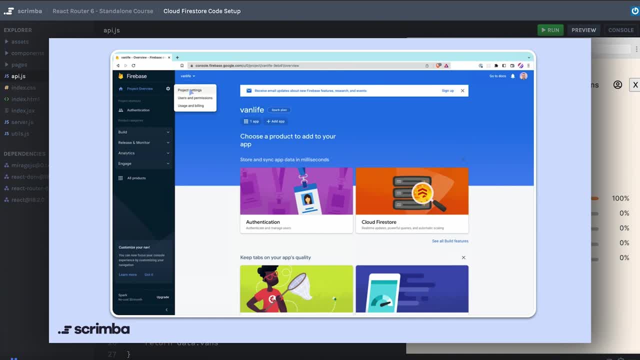 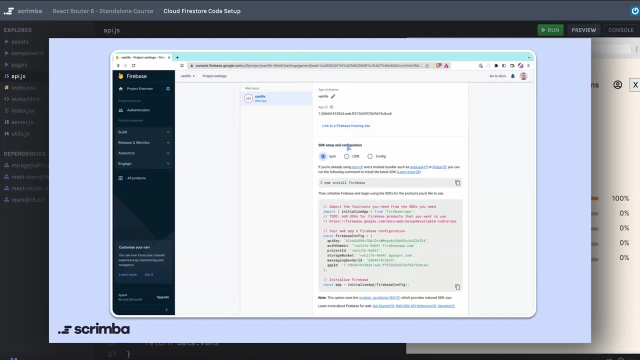 firebase console. you can click on the gear icon in the upper left and choose project settings. that will take you to the project settings page and on this general tab, if you scroll down to the bottom, you'll see that configuration object again and you can click the rectangle to copy. 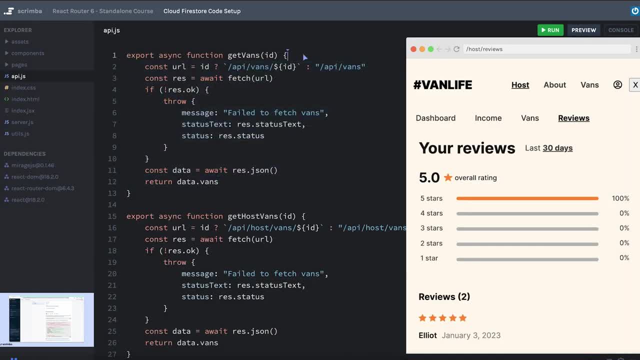 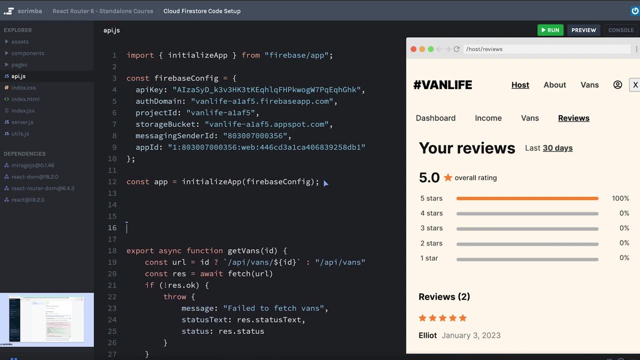 that so that we can use it then back in our api js file. i'm just going to paste the configuration object in here and paste that in and we can just clean up some of these comments for now, and i'll give a little bit of space before our actual api functions, just so we can clearly 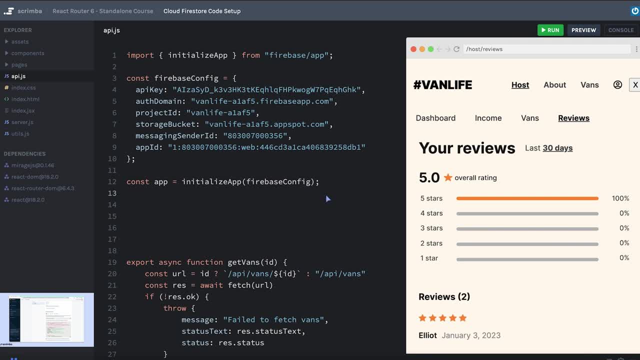 see what is firebase related now, firebase is a whole suite of different tools and firestore is just one of those tools. here we have initialized an application which will allow us to connect to our vanlife application in firebase. we also need to write code that is specific to firestore, so i'm 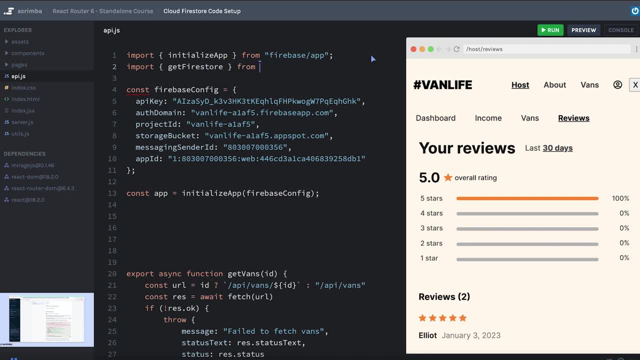 going to import a function called get firestore, which will come from firebase slash firestore. now, one of the major benefits of firestore that we actually aren't going to be using very much is its ability to have real-time data. in other words, i can create a connection between my application and the database and, if that data ever changes, 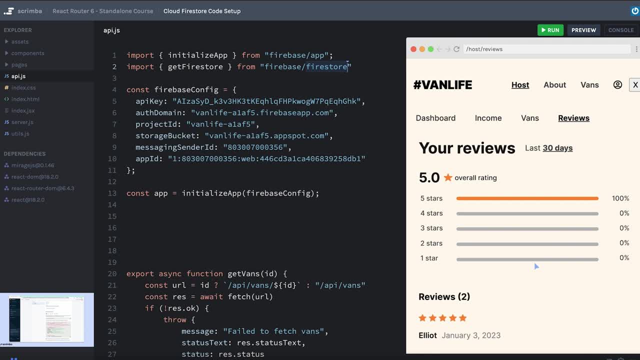 in the database. my application can listen for those changes and, without any prompting on my end, refresh my user's view so that the data can be real time. this is perfect for applications like a chat interface, where you want a new chat message that gets pushed to the database to also 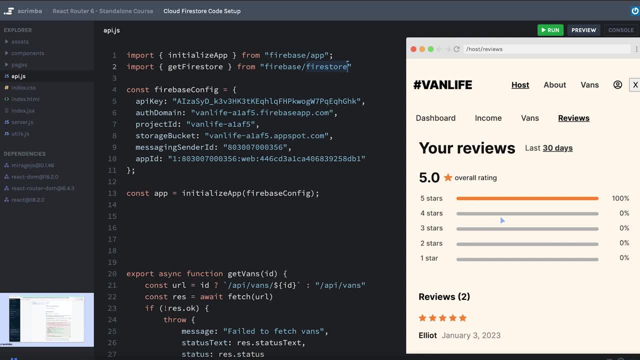 immediately display on your front end without the user having to do any kind of refreshing of the page. however, in our case, we are not going to be using any of those real-time features from firestore, and so i found there is actually a subset of this package: firebase firestore. 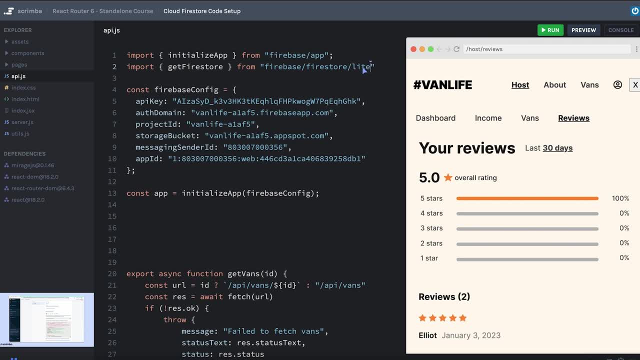 called slash lite, which is a lighter weight version, as the name would imply, of the full firestore library that allows you still to do reads, writes, updates and deletes, but with a a lot of opeloupes, which are actually very, very difficult to use, and this is why we're going to 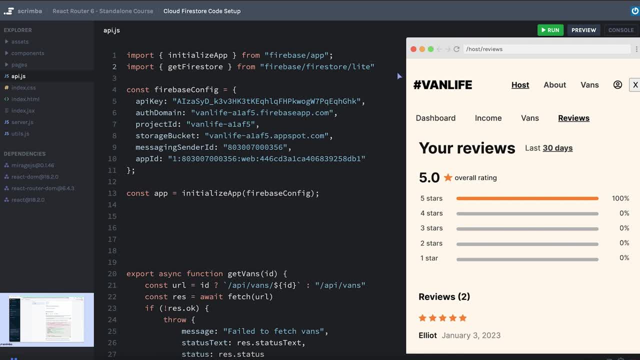 that allows you still to do reads, writes, updates and deletes, but without including any of those real-time features. So because I don't need the real-time features, I'm going to go ahead and use the slash light version of this library. 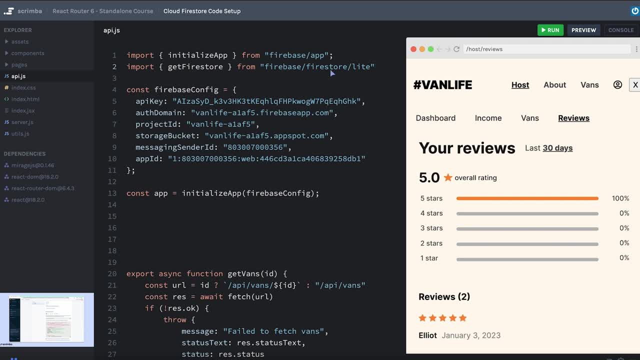 If you do feel like you want to play around with the awesomeness of Firestore's real-time data, then you can just delete this slash light at the end. Now that we have access to this function called getFirestore, I'm going to create a database object. 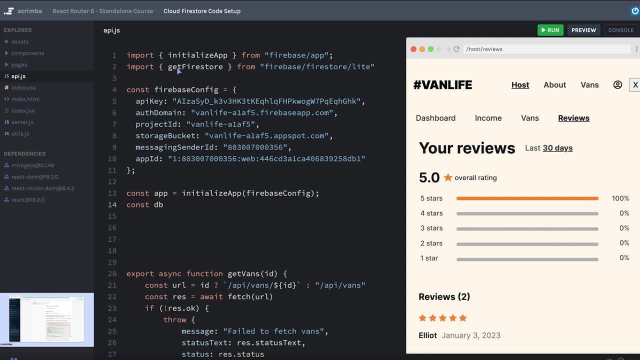 which I'll be using anytime. I need to interface with my app's Firestore, and so I will set that equal to getFirestore, and I need to pass in the app that we just created when I was initializing the app, and with that we should be set to start refactoring the fetching functions. 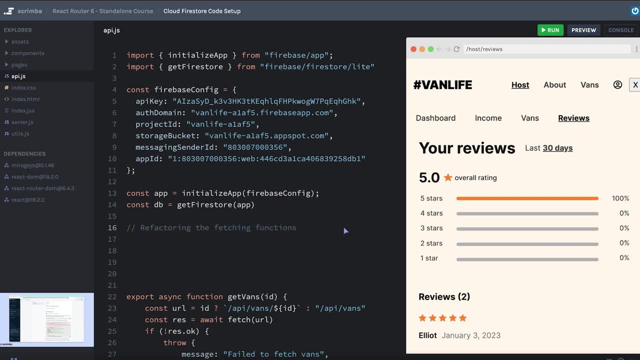 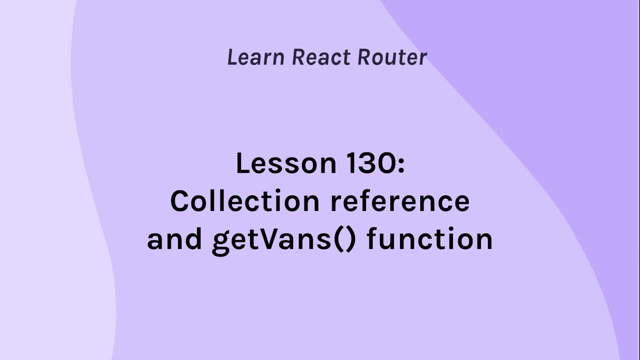 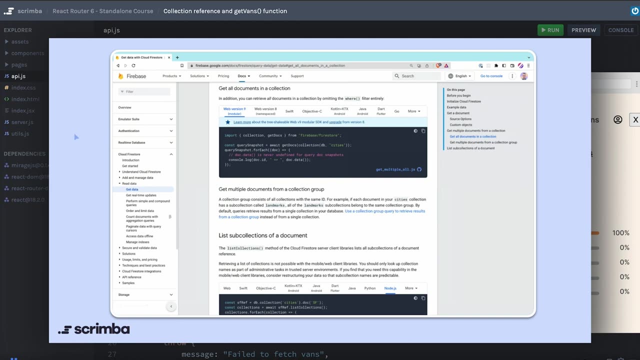 that are currently reaching out to Miragejs, so that it will instead be reaching out to Firebase. So that's what we'll be starting on next. Right from the start, I'm going to show you the documentation for Firestore. You can click the screenshot to go over to the documentation. 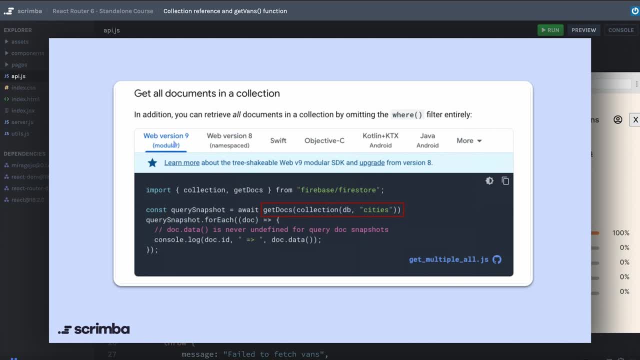 One thing that I noticed as we are using this web version 9,, which is more modular, is that it includes a lot of nested function calls. For example, when we want to get documents from a certain collection, most of the documentation shows calling this function called getDocs. 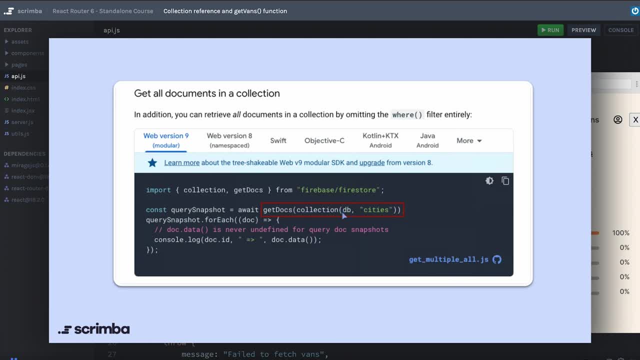 and inside of that you pass a call to the collection function and inside of that you pass your database, like the one that we created, and the name of the collection that you're trying to get. This might be completely fine to you. 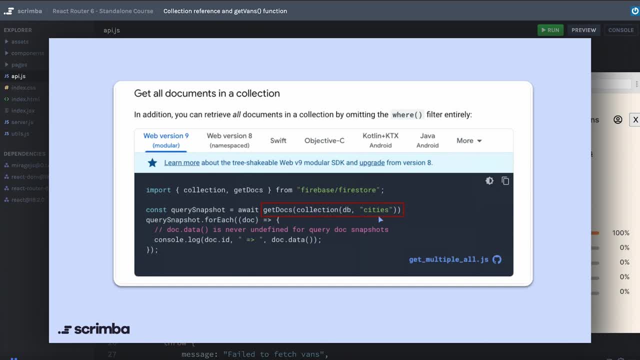 Maybe this might be a little bit more difficult for you, but it's fine, This makes perfect sense. It makes sense to me, but it's still a little bit confusing. It also requires a lot of duplicated code where I'm going to be writing collection db and, in our case, vans- multiple times. 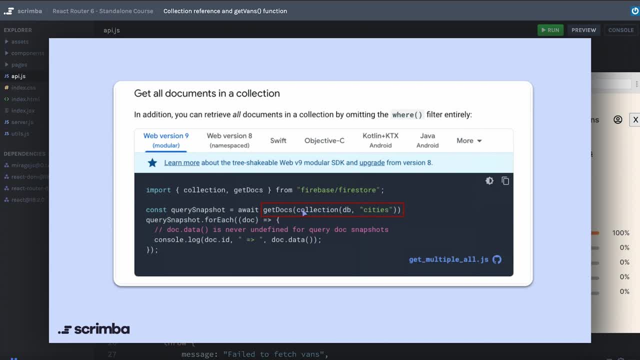 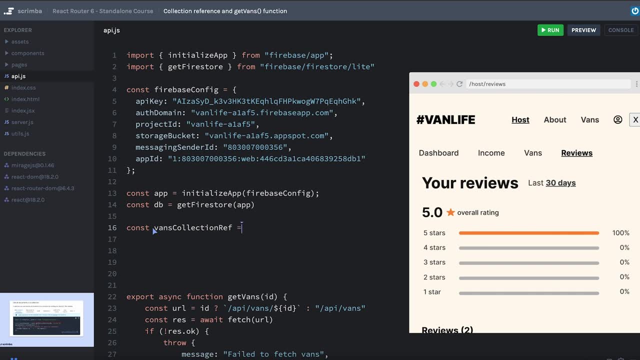 So I'm going to do it a slightly different way. I'm going to reference my collection in a separate variable, So I'll call it maybe vans collection ref and set that equal to a call to the collection function. I'll pass in my db that I created and pass in the string vans. 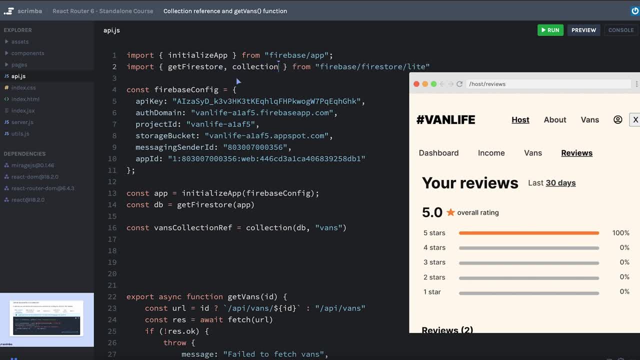 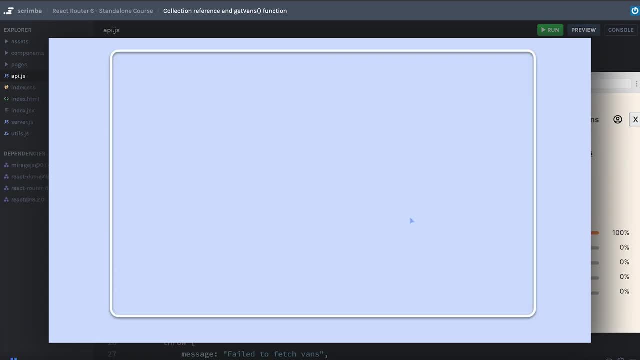 Before anything else, I need to make sure that I pull in the collection function, because this is something that comes from Firebase And if you're wondering why this string vans is here, if you remember back a little ways when I was creating the data, 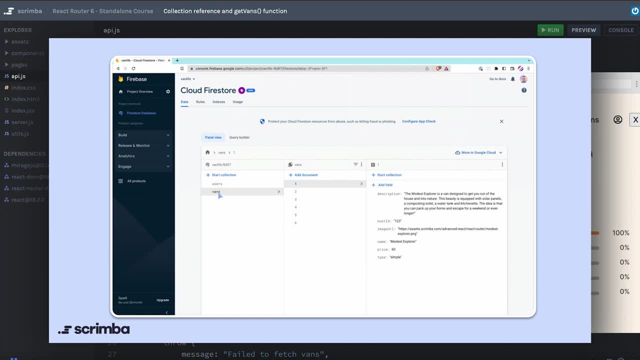 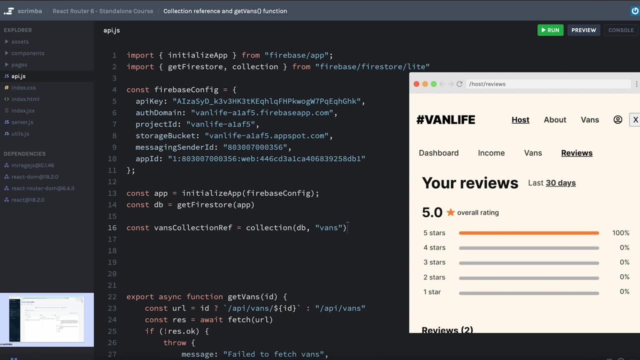 I had created a collection that I called vans. If I had named it something different, I would need to put that different name here. Now, first things first, before we move on. I lost a lot of hours trying to figure out when I was practicing this: 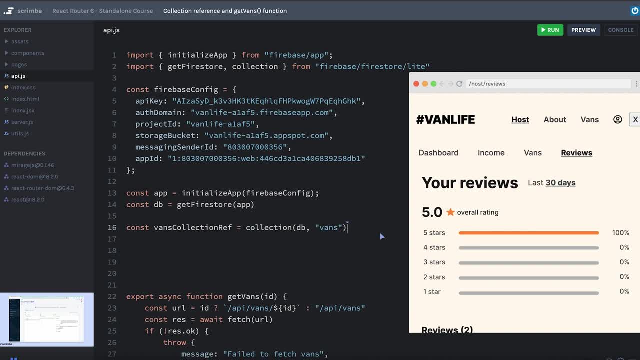 why my requests out to Firebase weren't making it all the way to Firebase. In fact, they weren't even making it to my network tab in my developer tools. And the reason, as it turns out, is because MirageJS was intercepting every request that goes out. 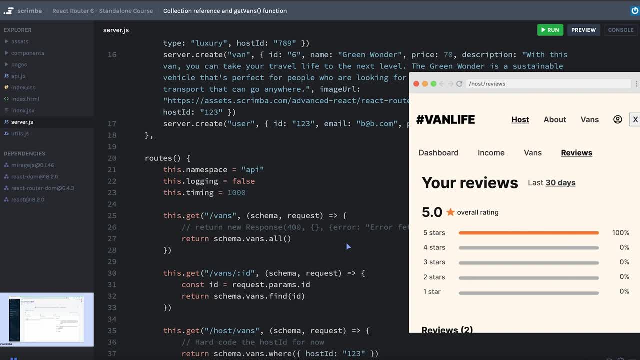 This makes a ton of sense when you're using Mirage, because you can make a regular fetch request in your code and not have to worry about it trying to reach out to a real resource or anything. However, it did cause me to pull my hair out quite a bit. 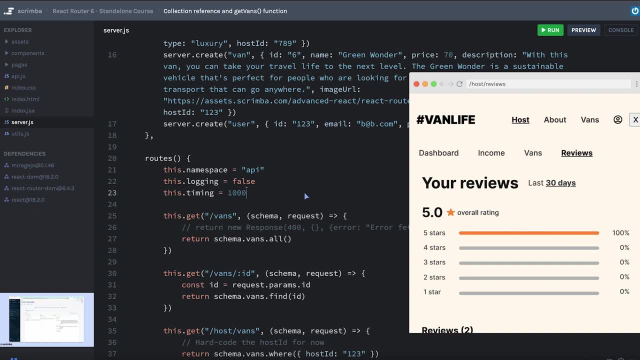 as I was trying to figure out why I couldn't get any data from Firebase. But fortunately, MirageJS has a really easy function that we can include, called thispassThrough, And we can put any of the requests that we want to make into the collection function. 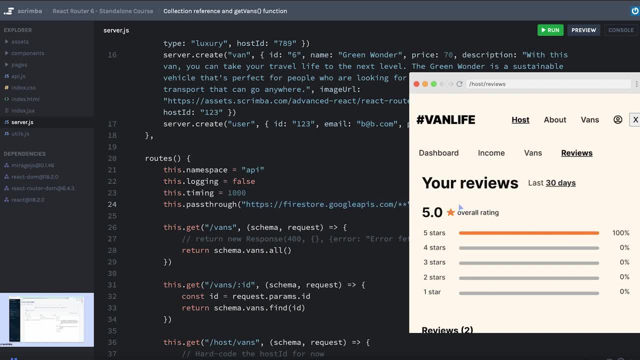 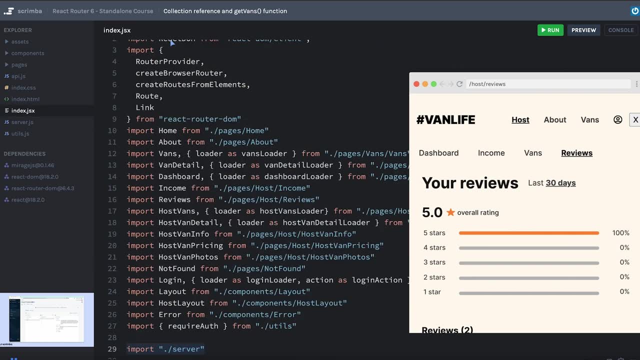 and we can put any URLs that we want MirageJS to allow outgoing requests to. So, if you're following along, I suppose one thing you could do is just delete this import server from your index file, Or I think maybe a better solution would be to use the thispassThrough function. 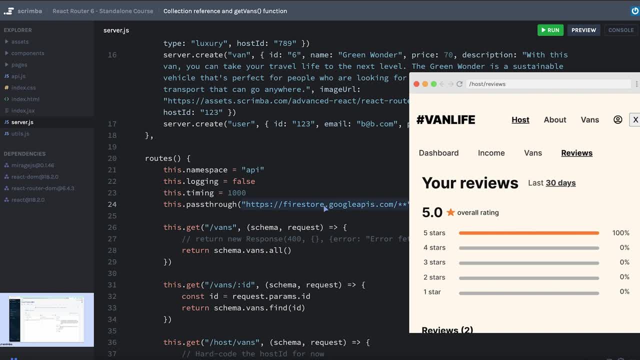 and just make sure that you include this URL so that any requests out to Firestore will make it past the sort of net or sieve that MirageJS puts up. Okay, let's go back to our APIjs file and start working on our get vans function. 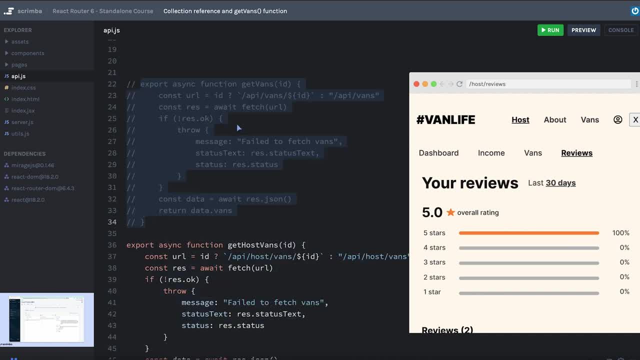 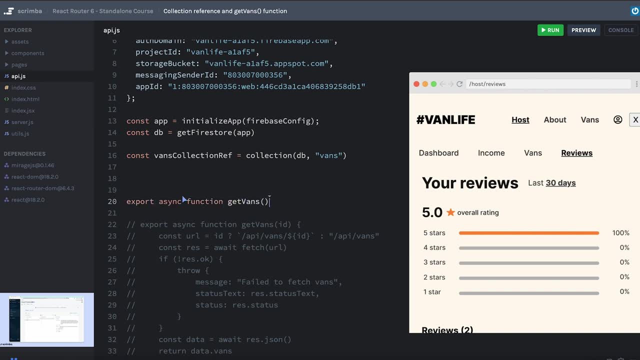 I think we're good. What I actually might do here is comment this out as I start working on them and create a new version of it. So I'll just export async function, get vans and maybe I'll worry about this ID thing later if I need to. 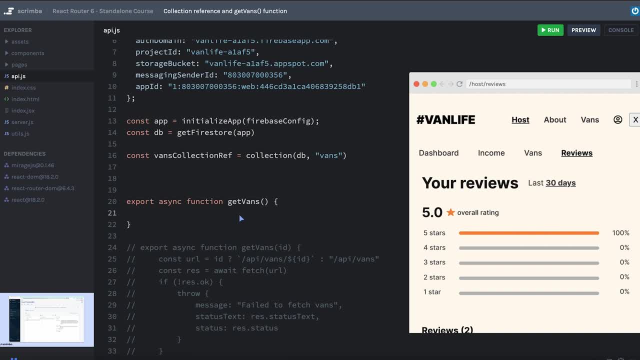 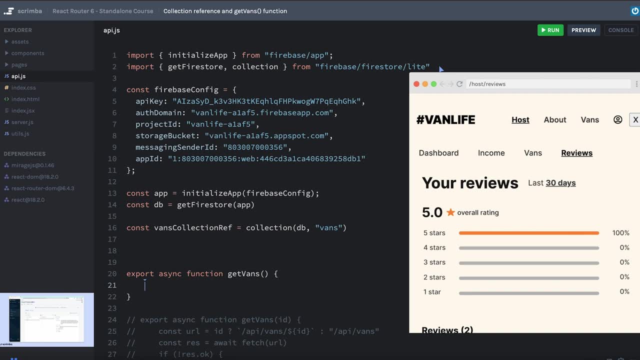 Something that can be really helpful to understand about Firebase because of those features where it can have a real time component to it. Anytime we go to get data from Firebase, it calls it a snapshot. The reason is, if we were to make a request to get the list of our vans. 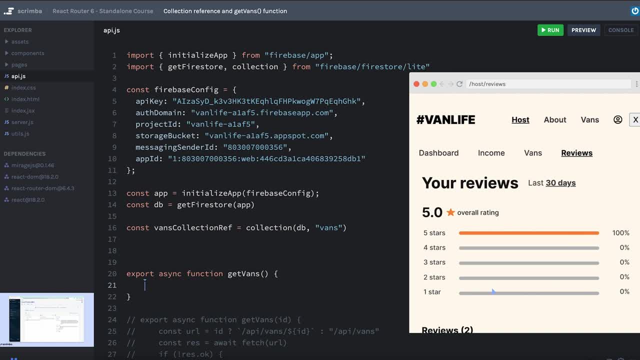 and then, after we got the data back, let's say a 10th of a second later, that data were to update somehow, the data that we just got from Firebase would technically be outdated. So the terminology of snapshot starts to make a lot of sense, because it's sort of like a snapshot of the data at that given point in time. 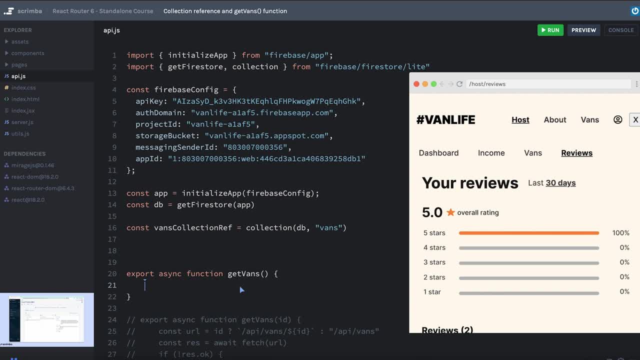 But with the understanding that it could have changed even perhaps immediately after we finished making our get request to the Firestore database. So that's just a preference as to why I'm about to name this variable a snapshot. So we'll call it query snapshot. 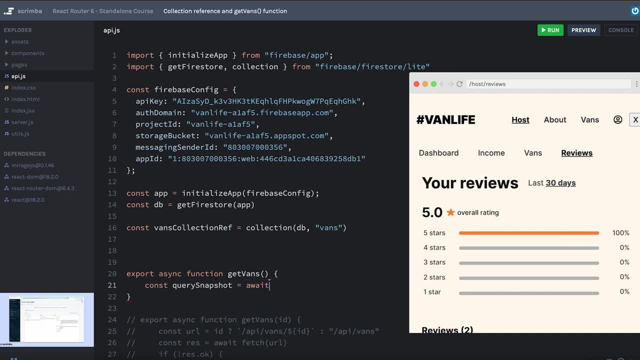 And that is going to come from a call. we'll use the await keyword. it's going to come from a call to the function called get docs need to pass the collection reference that I want to get the documents from and that's going to be our vans collection ref. 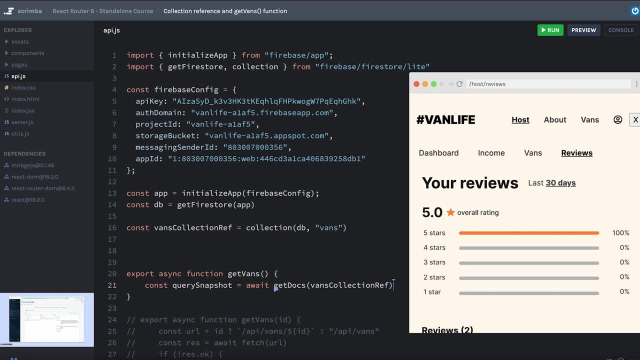 And what will come back will not just be an array of documents, but instead will be this snapshot of the query of the documents. Really, that just means that it's going to have a bunch of additional metadata about the docs that come back when we take the snapshot. 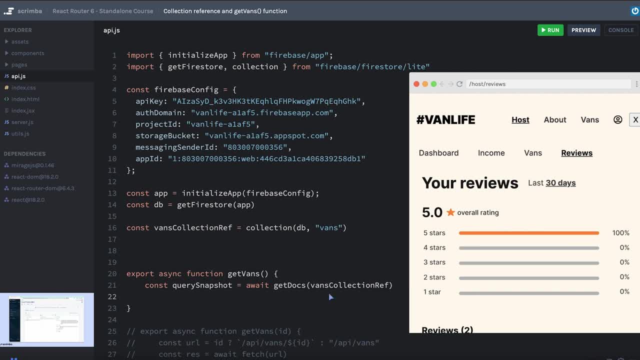 So what I'm going to do is take that query snapshot and turn it into a data array that hopefully we can make it so that it mirrors the same data structure that we're already expecting in our component files, so that we don't have to go make a bunch of changes to our components. 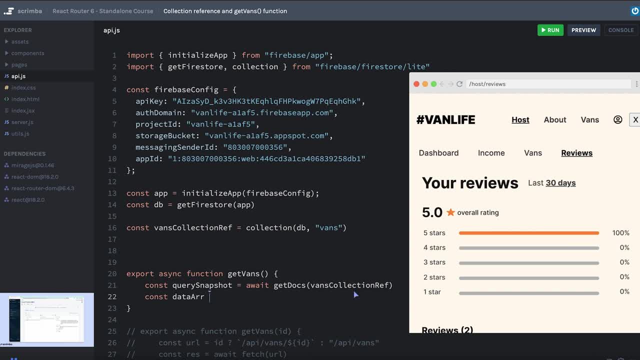 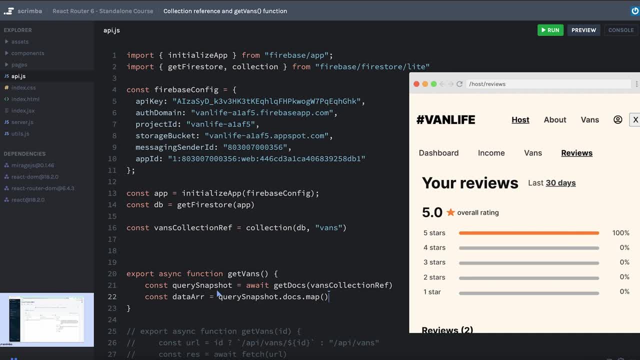 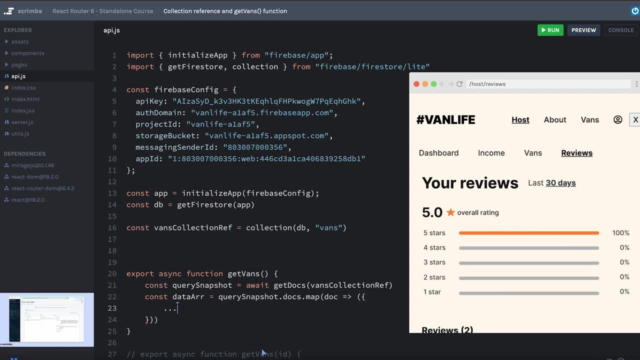 And I want to include all of the data from the document. So I can get that data by saying doc, dot data and then calling that as a function, And, as it turns out, this data does not include the ID of the doc, And so I also want. 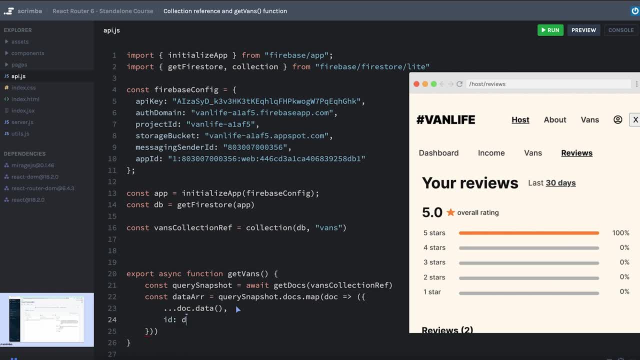 To include that as a property here that I specify with doc dot ID. this ID could be something that is generated by Firestore when you create your documents, or, in our case, I created this manually so that I could just have the simple IDs of 12345 and six. okay, we went through that blazingly fast. I guess as a side note, it's important to know that I'm going through this Firebase information more as a reference instead of actually teaching it, and that's because in the scrimba front end developer career path we introduce our students to Firebase pretty early on. 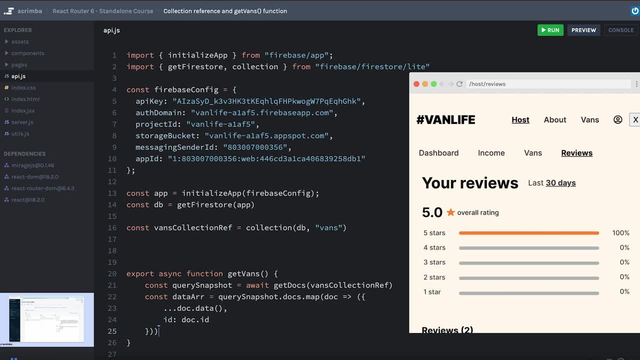 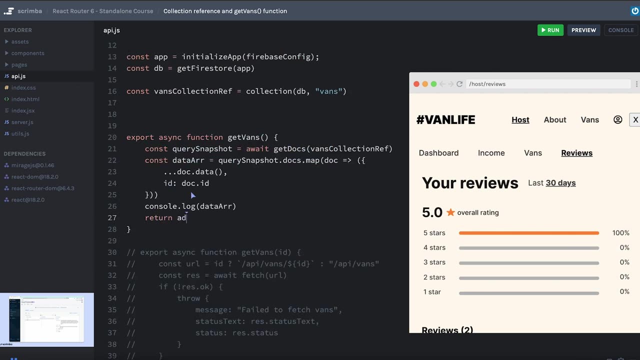 And that's because in the scrimba front end developer career path we introduce our students to Firebase pretty early on. And that's because in the scrimba front end developer career path we introduce our students to Firebase pretty early on In the career path and much of this has already been taught. So I just want to preface why it seems like suddenly Bob is going really fast through this information instead of making me sit and practice it. So let's go ahead and console log our data array, And then we need to make sure that we also return the data array so that it can be used by any loaders that are calling get vans. Now if I tried to load up one of my van detail pages, it will probably be broken because the old version of get vans was able to take an ID. 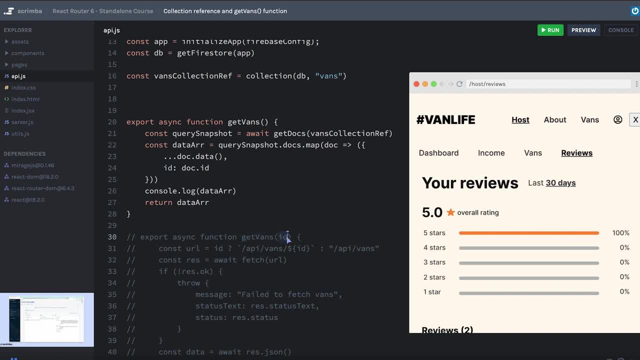 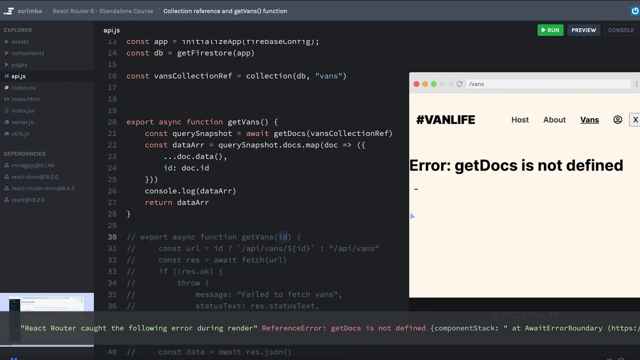 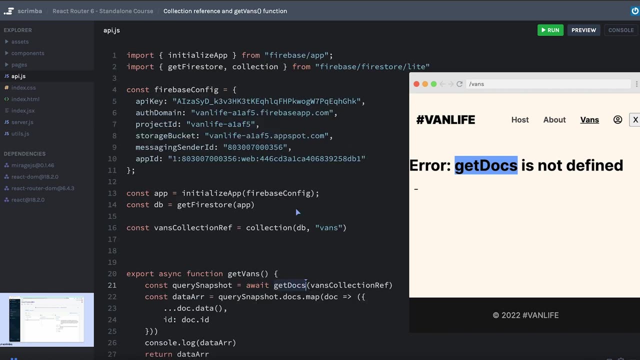 And those van detail pages need to pass in an ID. So let's just avoid doing that for now. I'm gonna go back to my homepage And then we'll click the vans page. Oh, okay. well, actually this error boundary has been really helpful. I called get docs And let's see where was that right here and I forgot to import it. So sorry for anybody that was screaming at me to remind me to import that. Okay, let's try saving. Okay, so our vans came in. we have our console, which is displaying all of the information that we have saved in Firebase, so it should now be able to read the data. And, yeah, I hope you enjoyed that And I'll see you guys in the next video. Bye, bye. 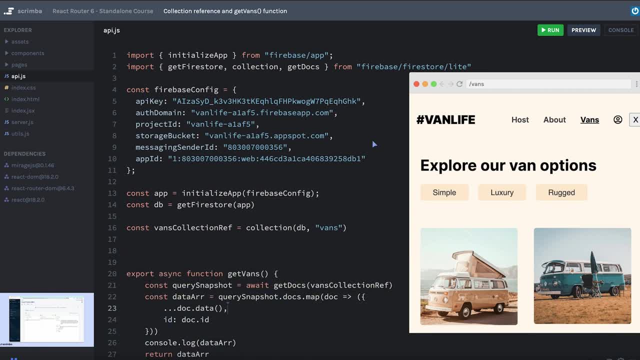 store. What's really nice about the way that we have the setup is I didn't have to make any changes to my components or my pages because we had a nice separation of concerns where we had these API functions that are in charge of getting the data that is needed. 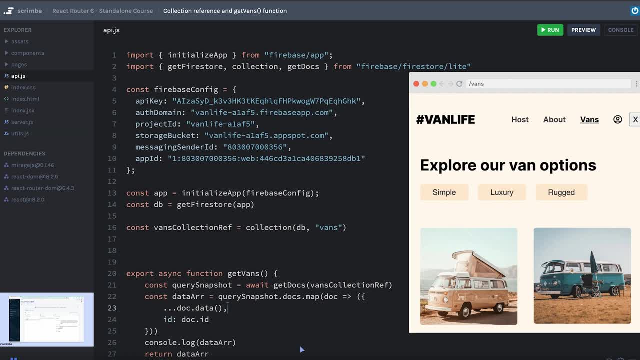 by the pages. we can just make changes to those functions and get the data from a different place. As long as that data is in the same shape, you could say, as what we had before, everything should just kind of work out. the component shouldn't really care how or where. 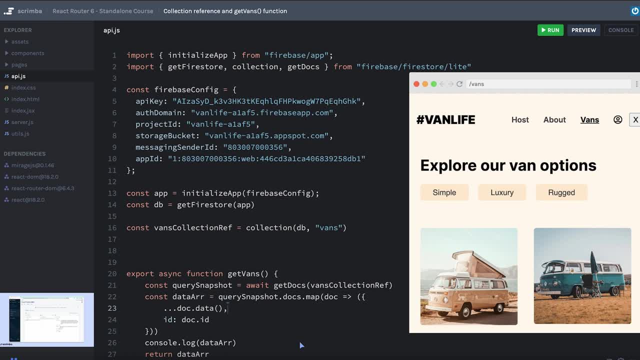 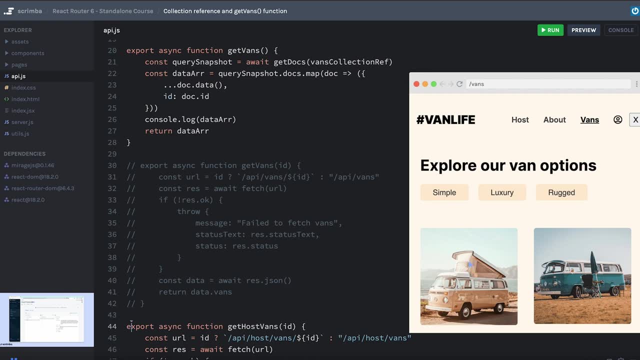 the data is getting fetched from, really should just be taking that data and displaying what it needs to display accordingly. Okay, we still have a bit of work to do, Because right now, if we click into one of these, we can see that a bunch of information is missing. 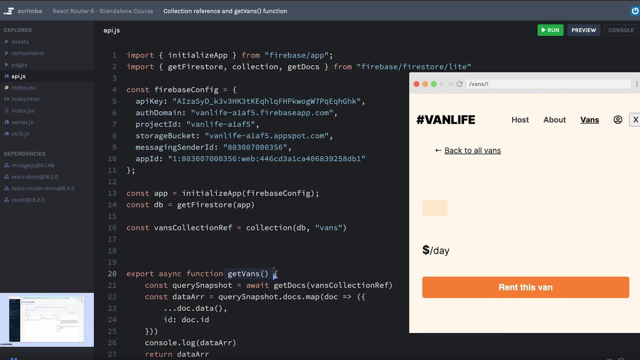 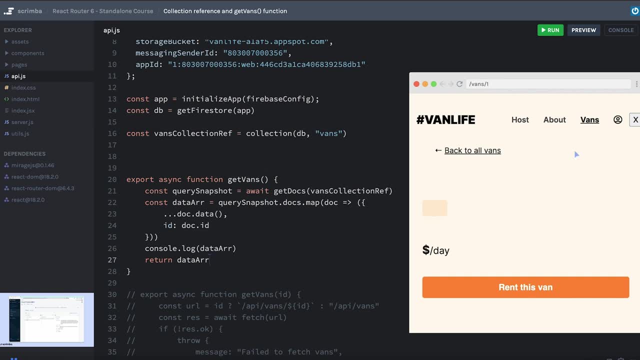 And that's because we have altered our get fans function. it no longer has the ability to take an ID. So next we will start working on being able to fetch data on a single document so that we can fix this page. In the earlier iteration of our get fans function we can. 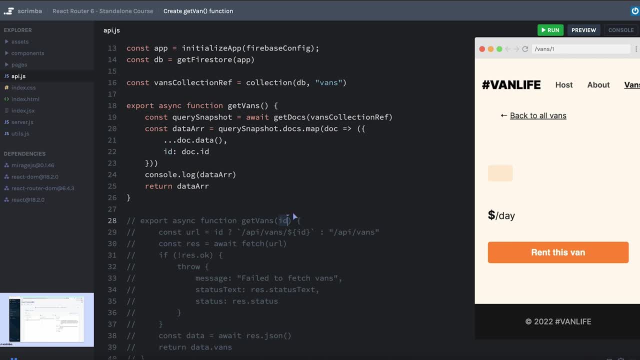 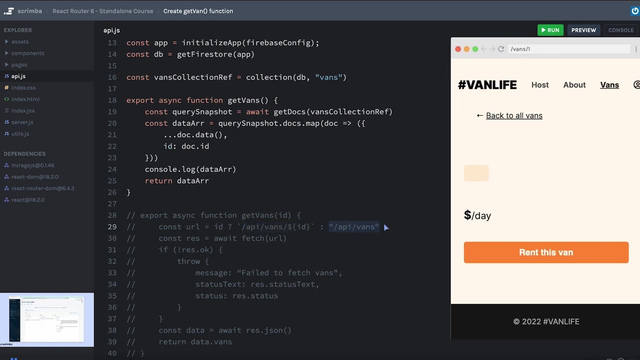 see that we had a function called get fans function. we had this one that was a bit overloaded. it was able to take an ID and if it had an ID then it would call out to this endpoint, And if it didn't have an ID it would call out to this endpoint. I'm going to just make 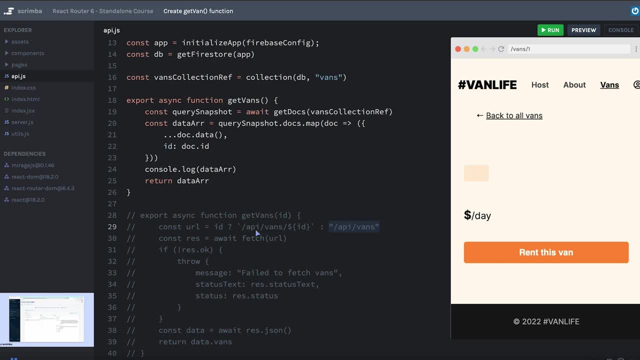 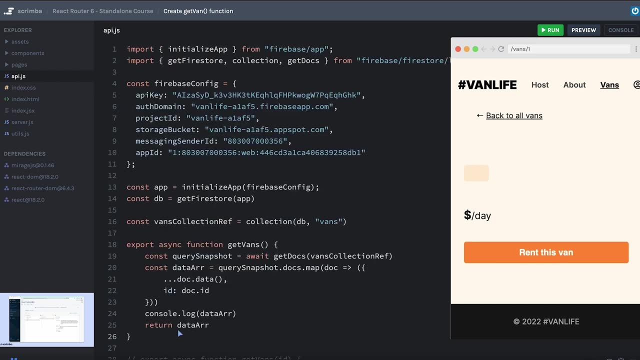 an executive decision to split these functions into two separate functions. One really good approach when you're creating these functions is to make sure that your function can do one thing and it does that thing really well. This will also help with unit testing, if we were ever to add unit testing to this project. So I'm going to create a new function will. 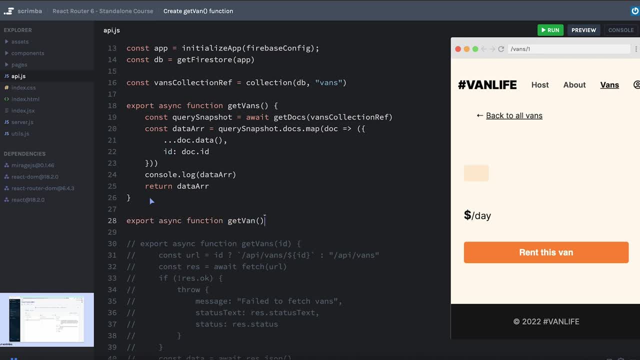 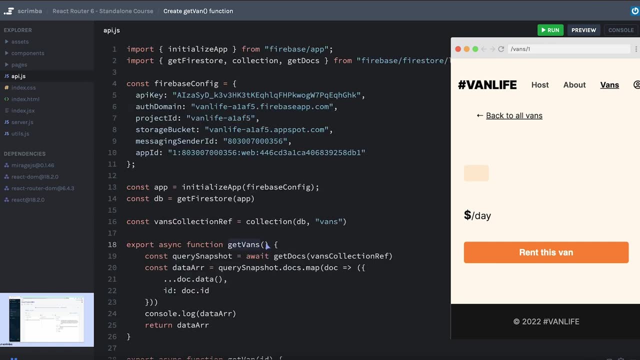 export the async function. we'll call it get van, just singular, and that will take an ID. This does mean that we'll have to go into any files that originally was calling get vans and passing an ID, and instead just update it to say get van, and we'll have to import it as well. And 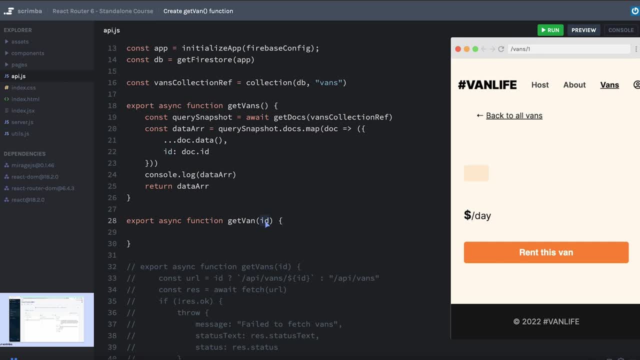 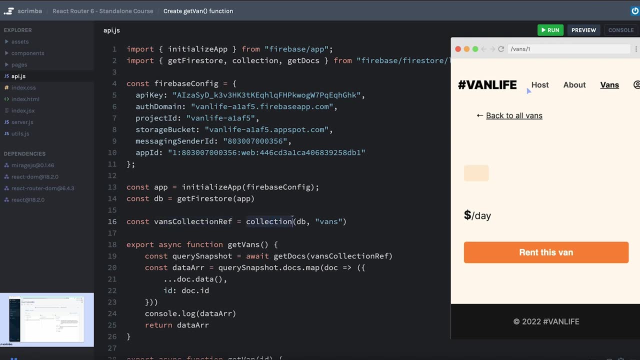 we have access to an ID and we're reaching out to Firestore. we really only want to get a single document. before we created this vans collection reference using a collection function that comes from Firestore, But this time we only need to get a single document reference. 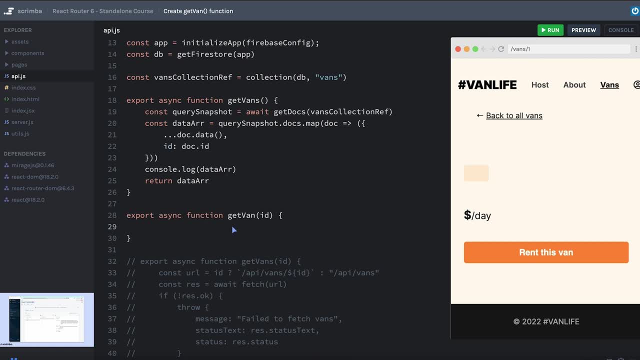 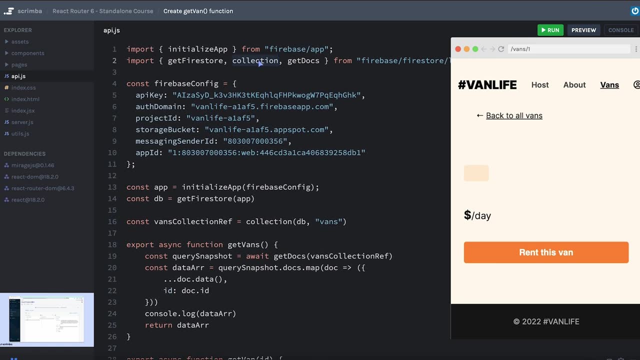 not a whole collection reference. So right inside of our get van function, I'm going to access that document by using a new function called doc. just like how collection was a way for us to get a reference to a collection, doc is a way for us to get reference to a. 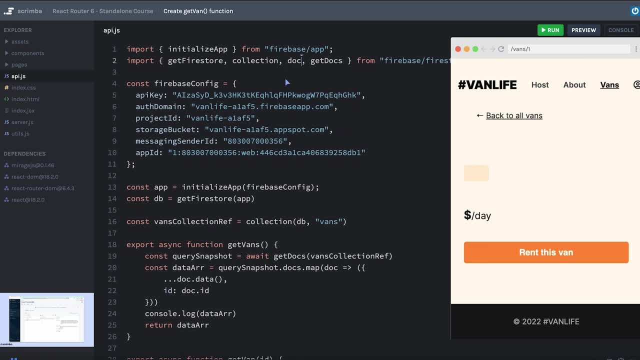 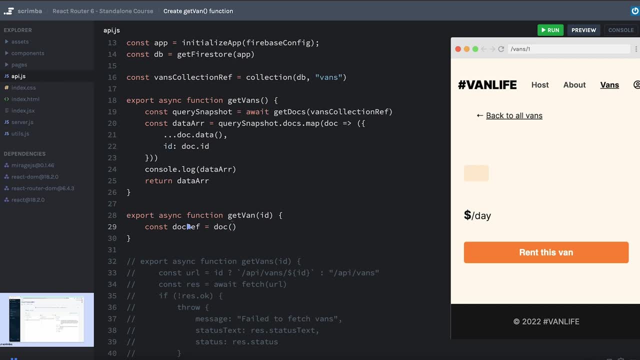 single document, So I'll need to import that. we'll bring that in right after collection And I will save this as we'll just call it maybe: doc ref. it's going to be doc And the doc is going to take three parameters. where the collection took two, it took the database. 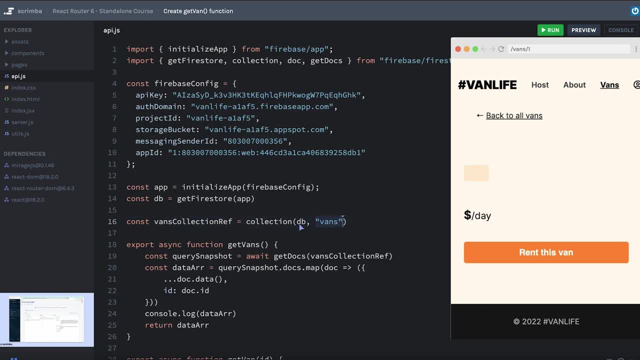 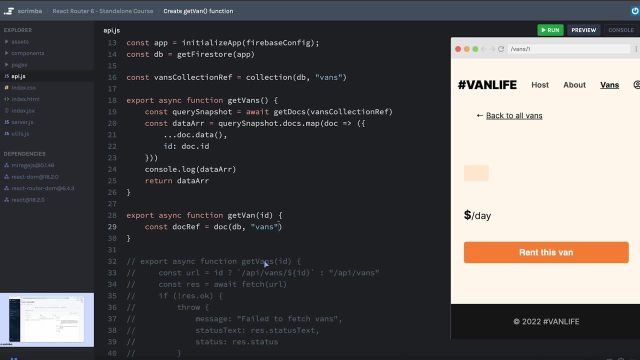 instance, We also need the string of the collection that we're trying to get from that database. we're still going to take the database. we also need the string name of the collection that we're reaching into, But then, even one level deeper, we need to pass the ID of the 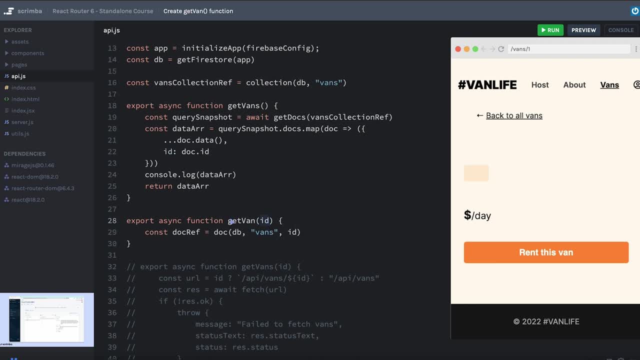 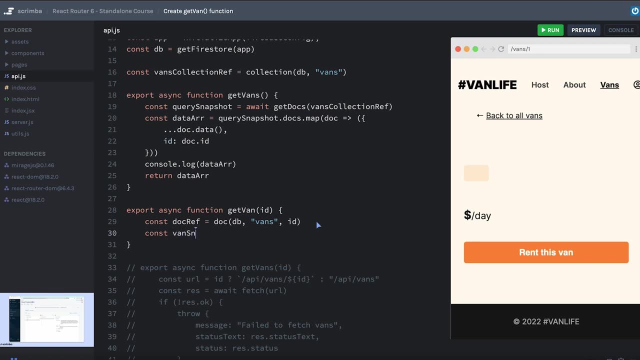 document that we are trying to get And that's the idea that's coming from our function right here. Now that we have a document reference, we can get a document snapshot- maybe I'll call it van snapshot- And that's going to come in by calling a function called get doc. 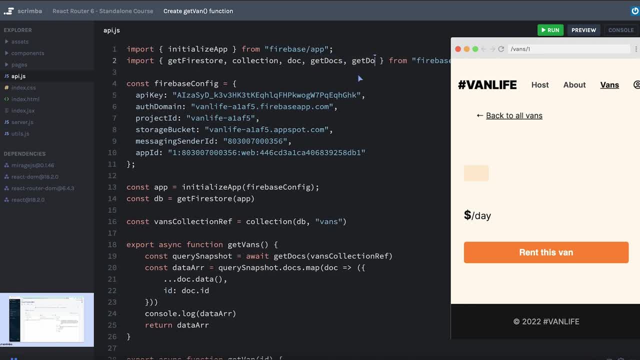 just like we had get docs, So I can get a single document. but I'm going to pass a new function to get doc reference And then, in order to get an array of docs, I can use get doc in order to get a single. 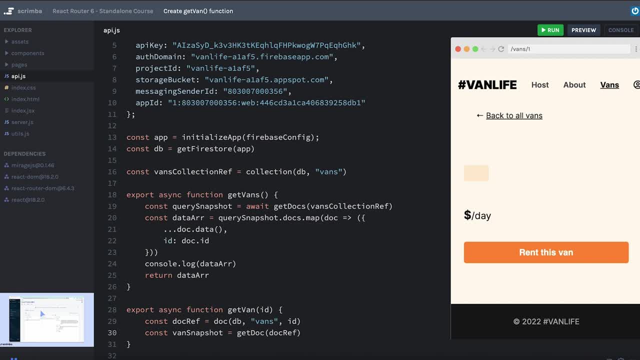 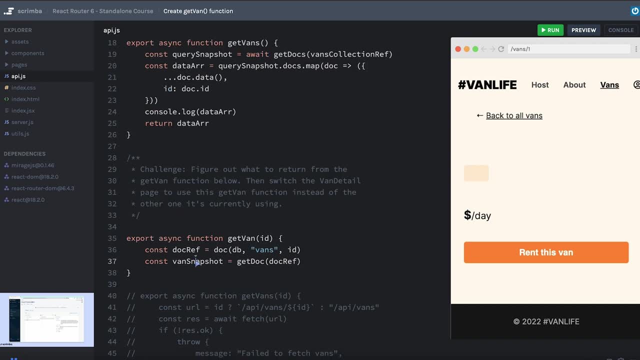 document. And just like we did before, where I passed the collection reference to get docs, I'm going to pass the document reference to get doc. And at this point I think it actually would be helpful for us to do just a little mini challenge. So I'll go ahead and type. 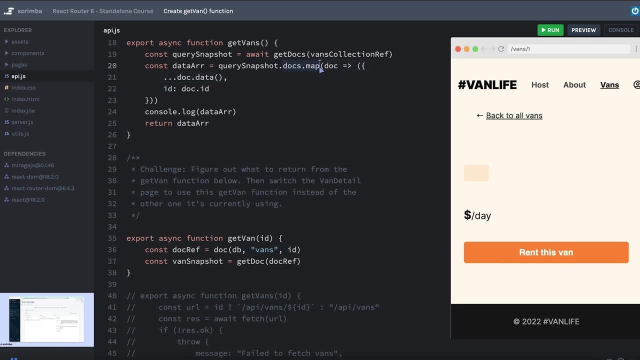 that out? Okay, we have access to our van snapshot And, in this case, unlike what we were doing, access to the one document that we're trying to get. So I haven't necessarily taught how to do this, but I'm hoping that, through some inference, looking at our function up here, 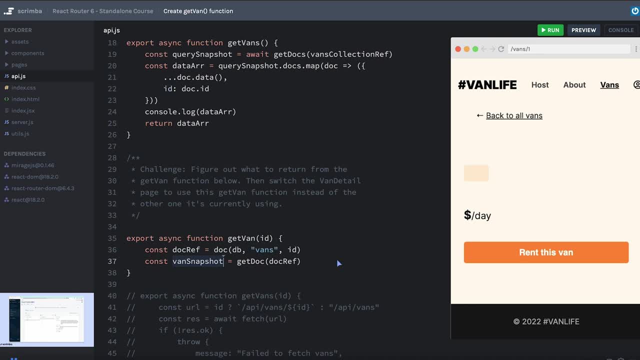 Or, if you would really like to, you can go to the Firebase documentation to solve this challenge and figure out what we need to return from the getVan function And as a part of that, you'll have to go over to the van detail page and 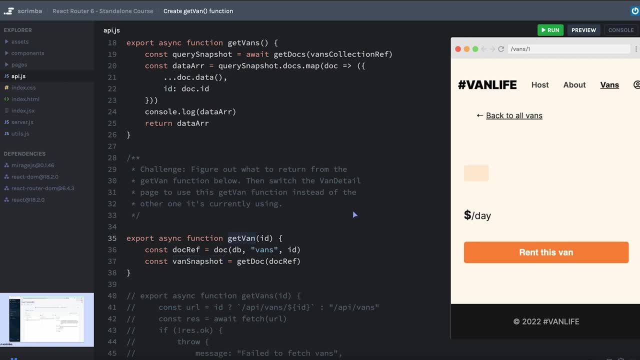 switch it so that it uses this getVan function instead of the other getVans that it's currently using. Okay, so pause now and work on this challenge. What we had to do before was iterate over the array of documents and take each one of them and return this object here. 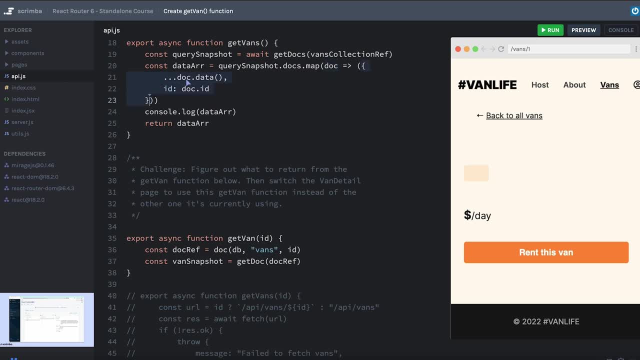 which has all of the data from the document, And then it separately gathered the ID from it as well, since, for some reason, the ID property of the document is not included in the data of the document. Well, in our case, we don't need to iterate over an array. 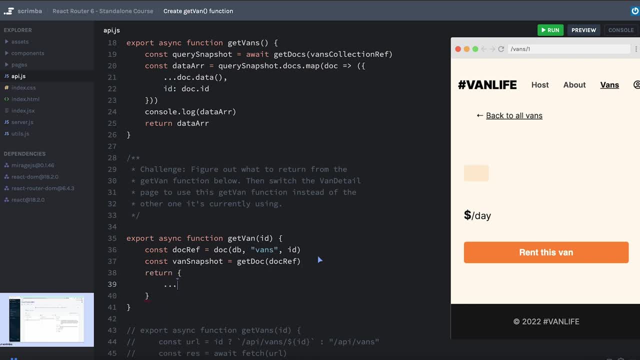 we can simply return the object that has all of the values that we use from the van snapshot, And rather I should say all of the values of the data portion of the van snapshot, And then we will also create an ID for it, which will be vanSnapshotid. 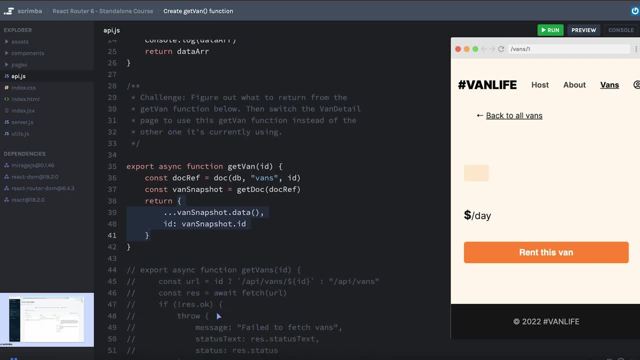 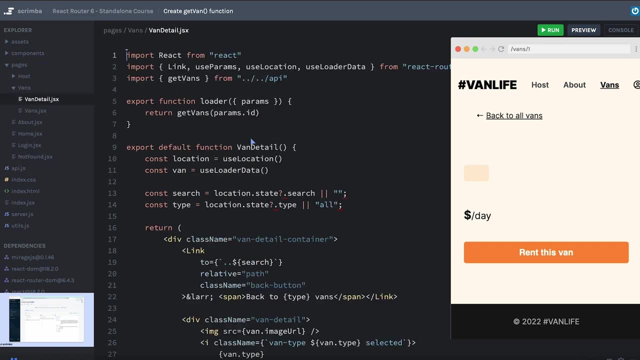 This should put it in, so to speak, the same shape as what the original getVans was doing before. at least we'll hope so. So let's go over to our. let's see where is it vanDetail We're going to pull in. in this case, we don't need the getVans anymore. 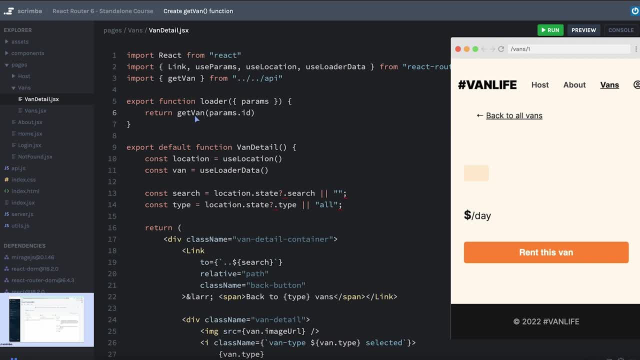 We're just going to do getVan and then we'll need to make sure to change it in our loader, and actually I think that might be it. Let's see, we're already on the vanDetail page. Let's cross our fingers and hit refresh. 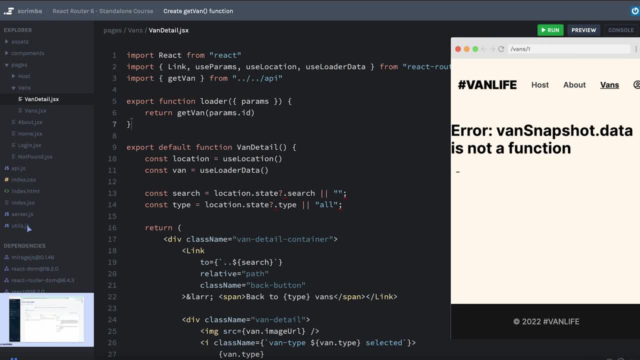 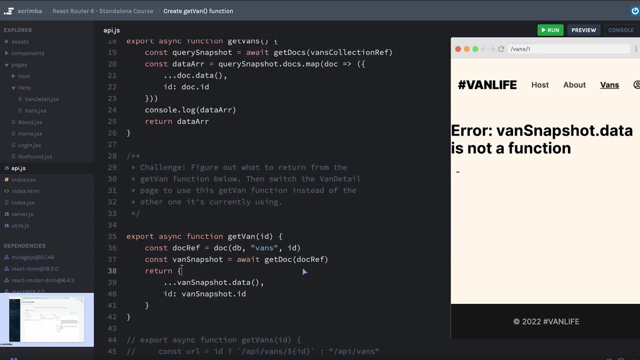 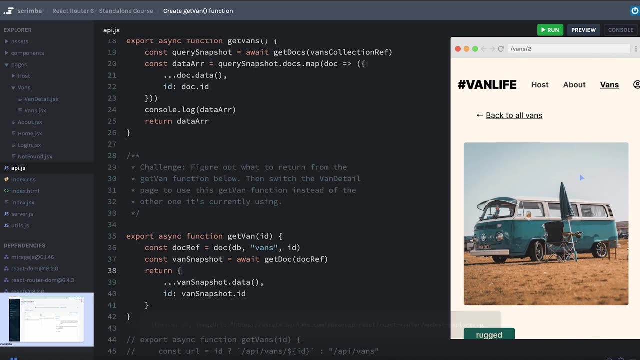 And hmm, vanSnapshotdata is not a function. I bet someone else has already seen what I did wrong here. We need to use await getDoc. Okay, let's try again. super close, Awesome, there we go. I should be able to go back to all vans and go into a different one. perfect. 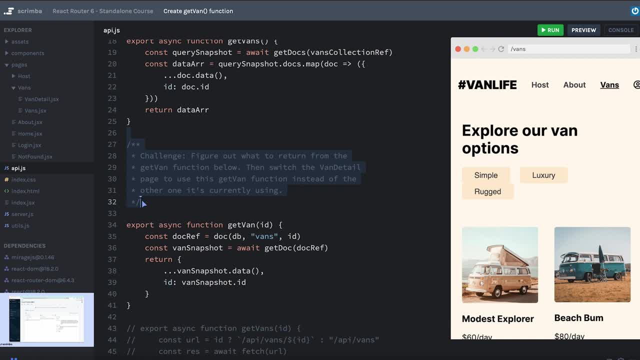 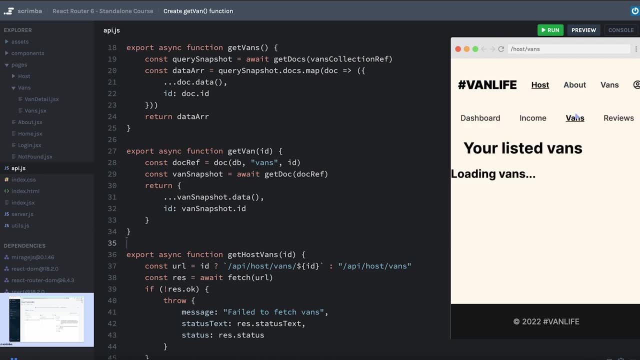 I guess, while we're at it, let's get rid of this console log up here, We'll clean up the challenge and we can actually get rid of our old function as well. Okay, now let's go back to our host pages and we will change our function so. 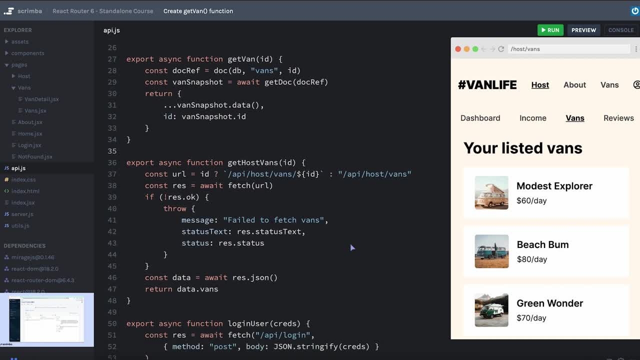 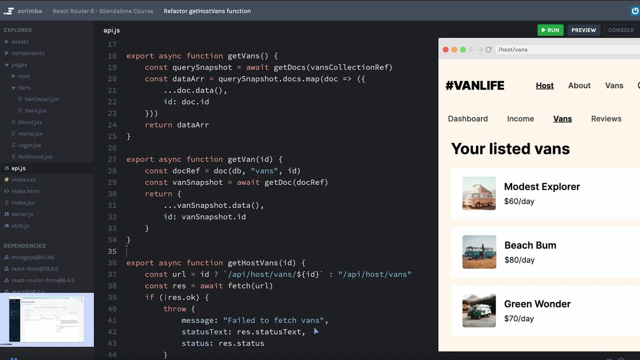 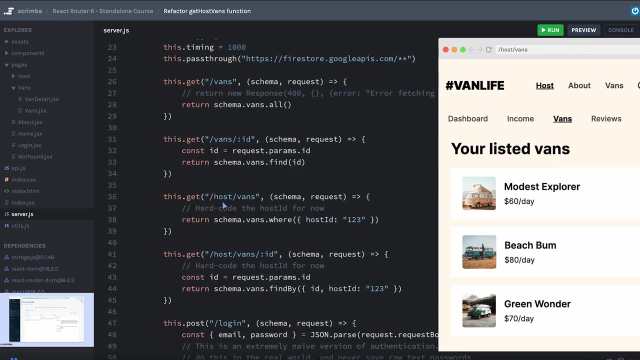 that we're getting vans from Firebase instead of from our fake server. Let's switch over our getHostVans to pull from Firebase instead of from our MirageJS server. Now, you might remember, over in ServerJS, our getVans or our host vans is just hard coding the host ID of. 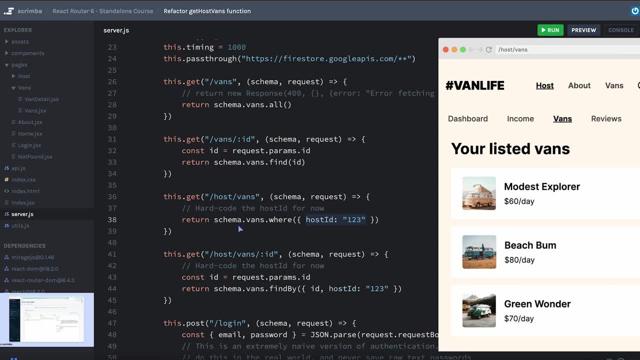 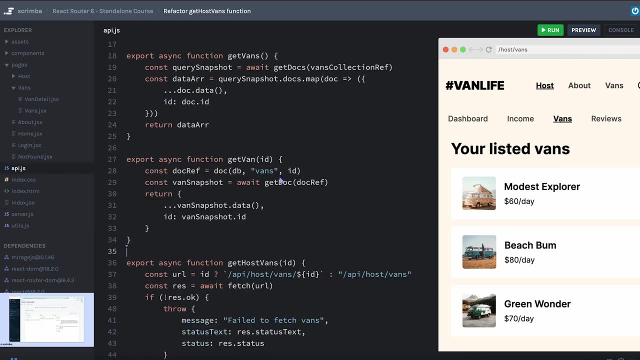 123.. Since we're not dealing with authentication right now, I'm going to do essentially the same thing, but this time we'll be pulling it from Firebase instead of from MirageJS. So in our APIjs file, what we are going to write will be very, very similar to what we 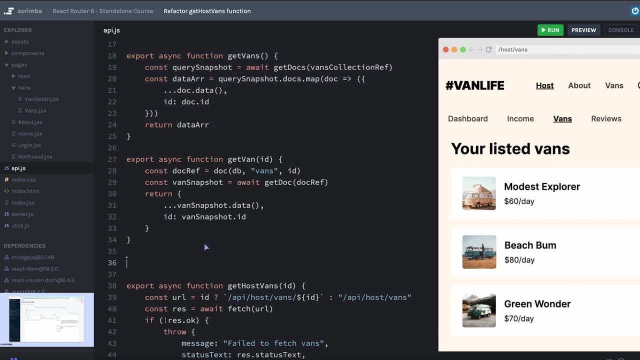 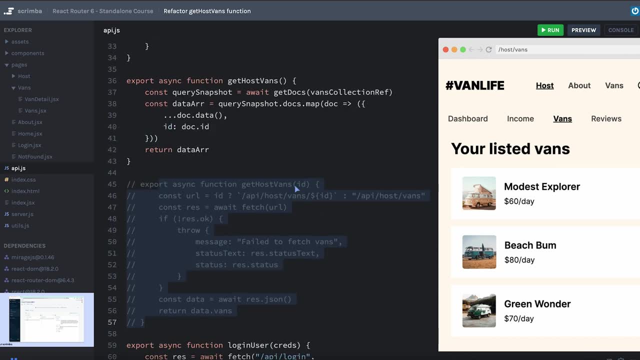 have in getVans. So I'm going to copy that function, bring it down here and then I'll rename it getHostVans and comment out the code we have in the existing getHostVans. And for now we also are not going to overload this the way we were before, where it was taking. 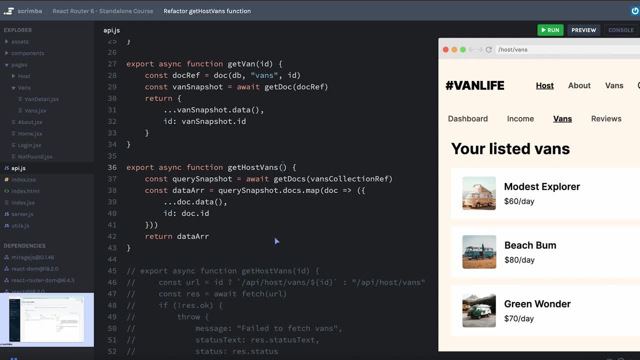 an ID, So we'll just forego putting an ID here in the parameter list. Now one thing to know about grabbing data from Firebase: if you are trying to get the entirety of a collection, then you can just pass the vans collection reference that we. 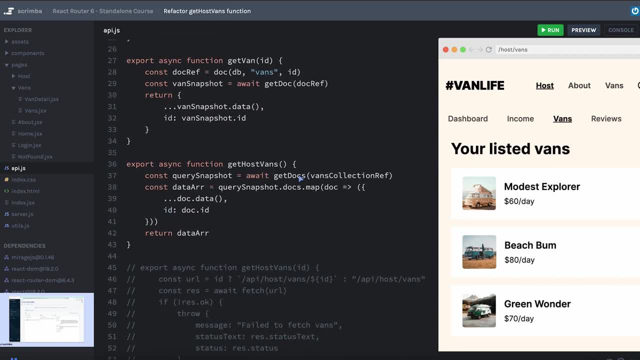 created up above right here. you can pass that to the get docs function and it will just get all of the documents from that collection. However, if I only want to grab certain of the documents from that collection, then I need to create something that's called a query. 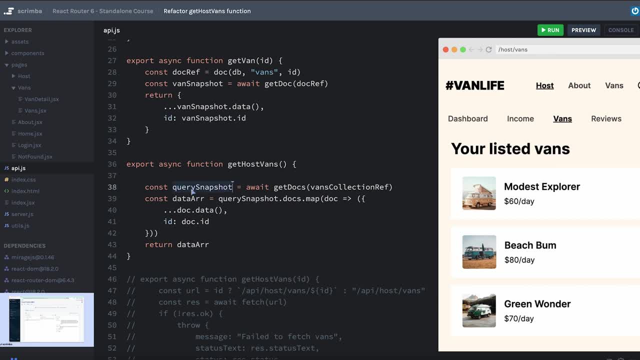 Don't let that be confused with the query snapshot that we had before, So let's do that. In fact, we might be better off calling this something like van collection snapshot, But just for legacy reasons I'm going to leave it as query snapshot. 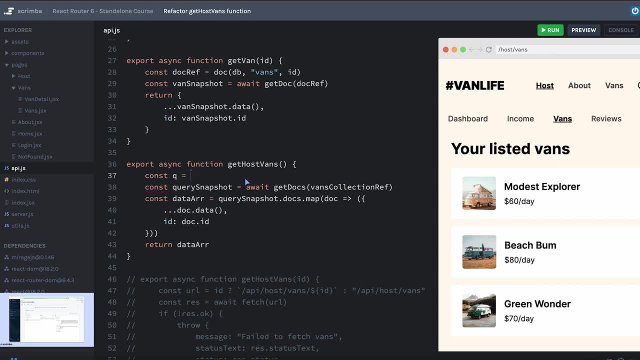 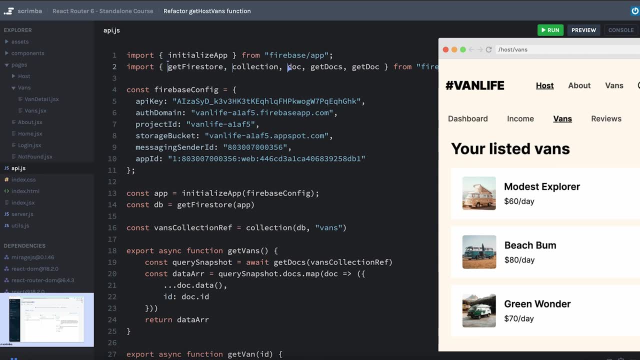 And maybe for now I'll just call it Q, to mean my query, and we can call a new function that's called query. So we'll go up to the top here. I'm going to put these on their own lines and bring. 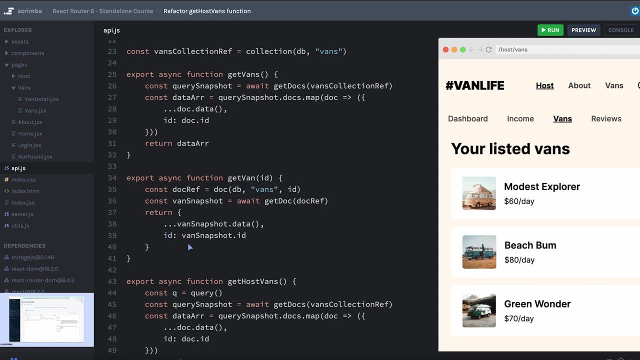 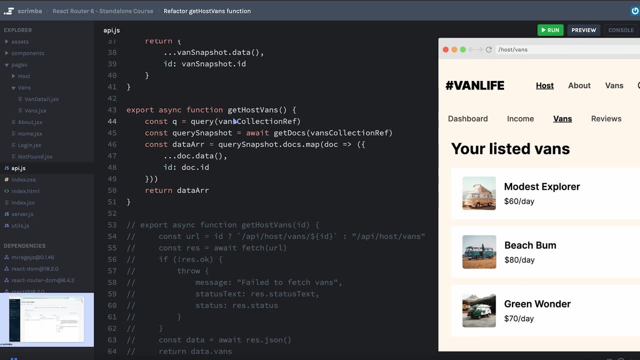 in query and query is going to take- see where are we down here. query: this function is going to take first, the collection reference that we want to fill Through And secondly, some kind of filtering operation. And this filtering operation is going to come from yet another function that we pull from. 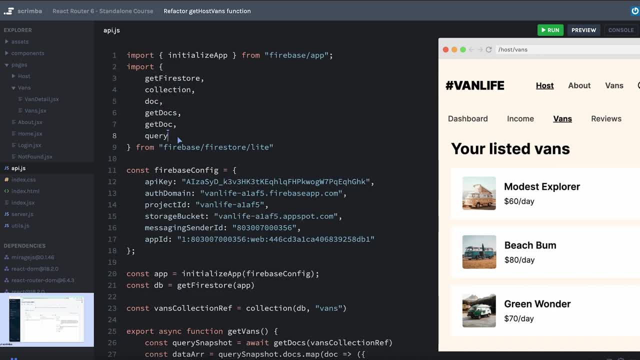 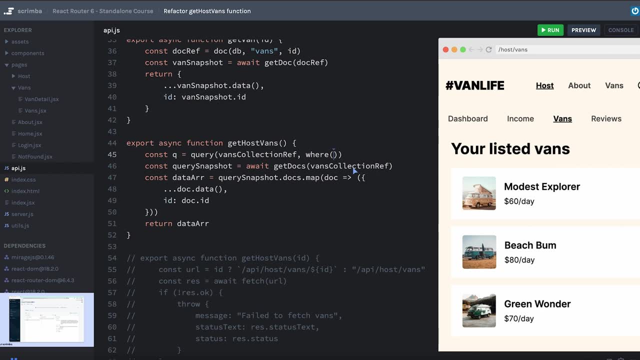 Firebase called where. So let's go ahead and pull in where and you'll see why it's called where in just a second. because when we're calling it, we are going to provide three different parameters. The first parameter will be one of the properties of our documents. 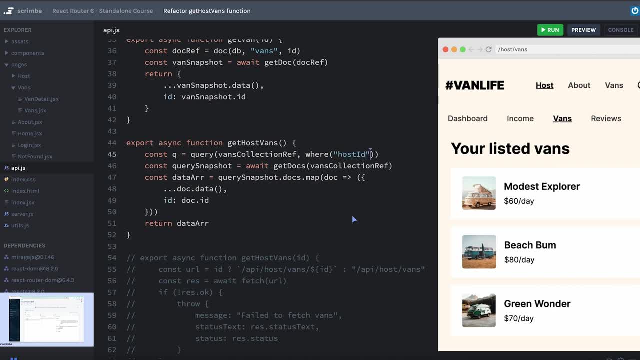 In our case, we have a property called host ID, And so it's saying where the host ID And then the second parameter Is going to be some kind of equality operation. In my case, I want to say that the host ID is equal to, and in Firebase we'll just use: 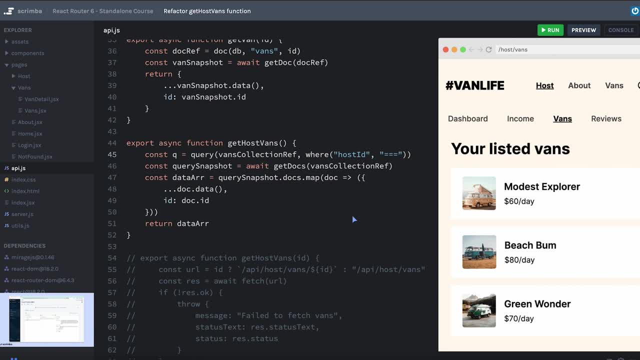 a double equals. I don't know that they have the same conventions that JavaScript has with the triple equals. So in the docs they talk about using a double equals, So where the host ID is equal to, and then we provide some kind of value. 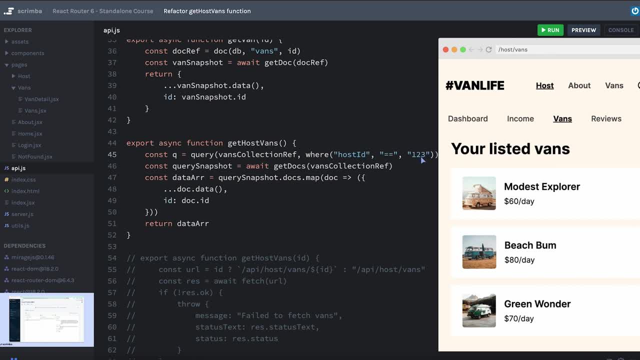 In our case, like I mentioned, we're going to hard code this to the host ID of 123.. So you can see why it's called, where it's kind of like an English sentence, where the host ID is equal to 123.. I know that. 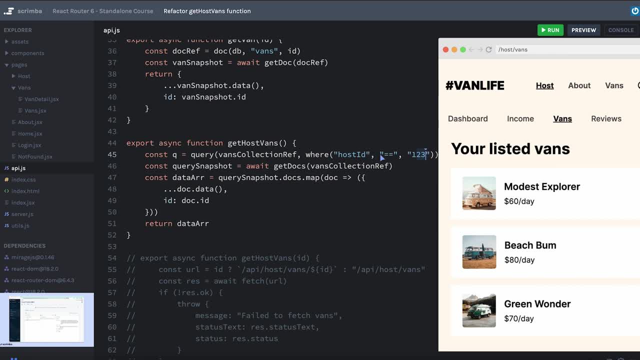 The syntax for this is, admittedly, a bit strange, but that's just how it is in Firebase, And what we've been constructing here is a query object that we called Q and that will allow us to filter documents out of the van collection. So, instead of getting the entire van collection, we're going to pass our new Q variable, or. 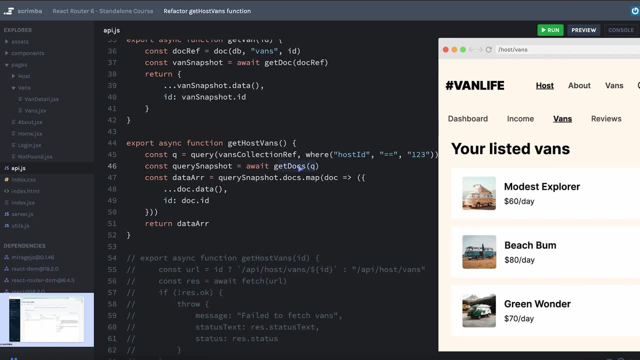 our query that we just constructed to get docs. At that point, everything else should essentially be the same. we're going to receive an array of data. we're going to loop over it. change the shape of that data so that it fits the. 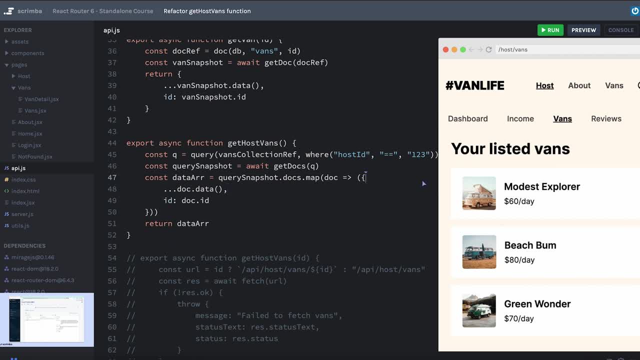 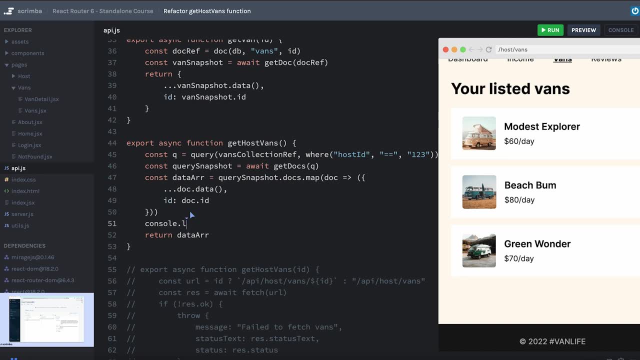 way that we need it to fit, And I think we should just be able to hit save and see everything kind of just work the way it was before. In fact, it's a little bit difficult to tell that it's working at all. let's just make. 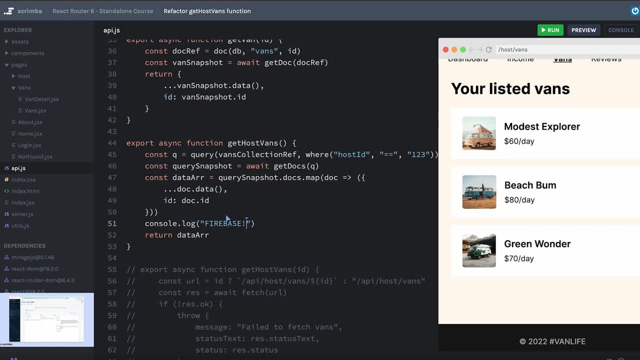 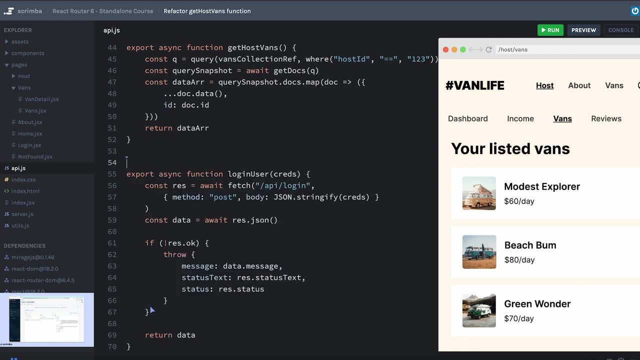 sure, this is the code that's running. we'll just yell Firebase at it in our console. Okay, well, that's running. So great we can go ahead and get rid of this old version of the function, And because we have the same name, it should just work. 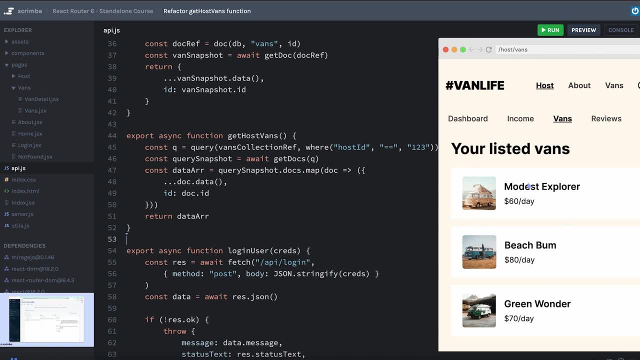 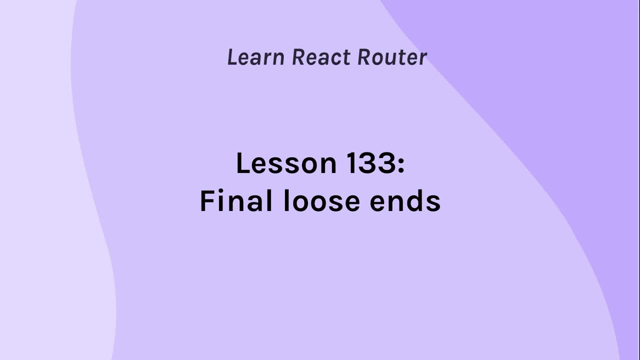 However, the function that we just deleted, that we had commented out, is what is controlling the detail page. So this is what we're going to fix next, Just for the sake of completion, we're just going to take a look at the instance where 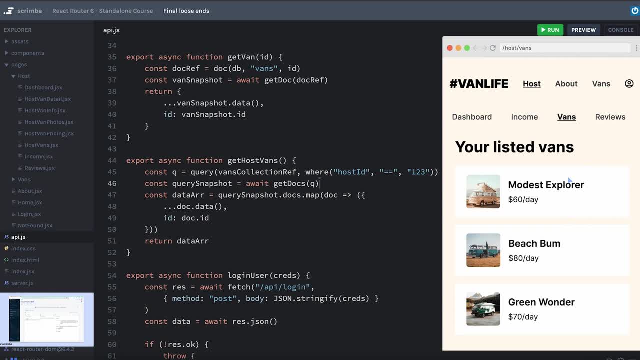 the host wants to get a single van. Now, because we're not using real authentication, we're not actually going to be able to make it so that only the logged in user can access their vans. Remember- we're currently hard coding- that the get host vans is coming from 123.. 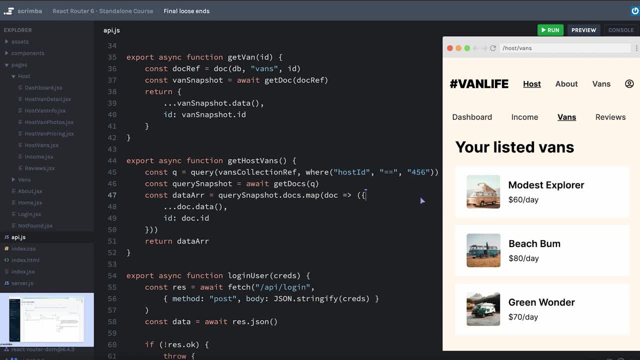 If I were to change this, for example, to 456, and hit refresh, We can see that our host vans will show reliable red because in the database reliable red has the host ID of 456.. And apparently no other vans do, because we're also pulling from get host vans on our dashboard. 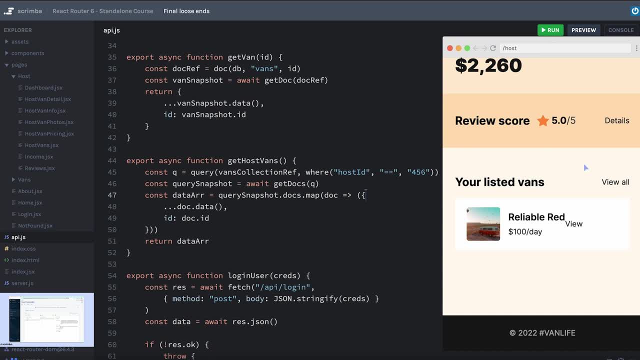 by changing it here in our API JS file. It also updates our dashboard at the bottom when we have your listed vans. But the problem is when we go to the detail page of these vans. so I think if I click view, we can see that the van information is not coming in currently. 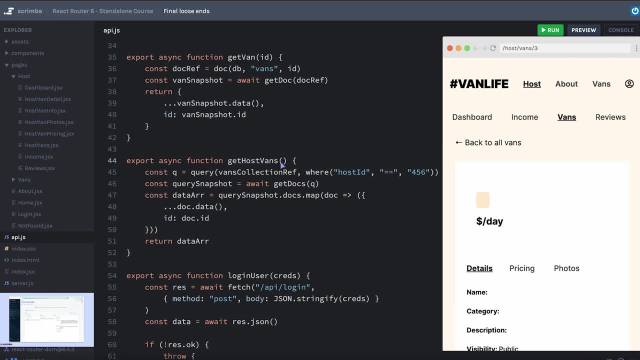 Originally get. host vans is not coming in currently. Okay, So we can see that the host vans had the ability to take an ID, But with Firebase, if we are trying to get a single document that also is ensuring that the currently logged in user is the only one that's able to see it, then we would have. 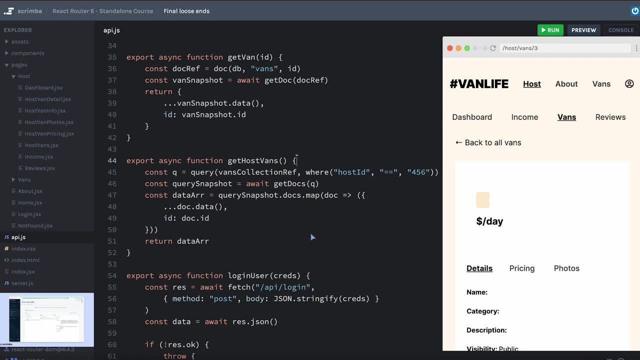 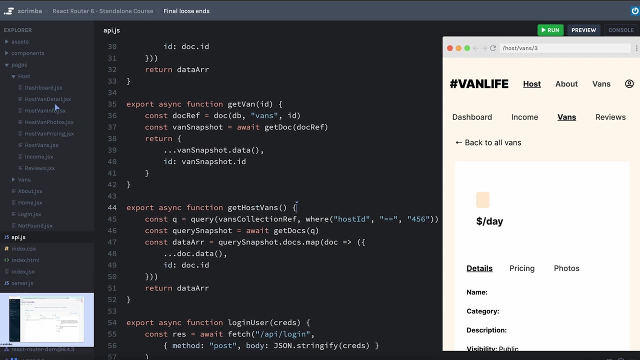 to set up some security rules inside of the Firebase console in order to ensure that we were only getting vans that the currently logged in user was allowed to see. Since we're not dealing with authentication and really not bothering with some really stringent security rules, what I'm going to do is simply go to my host van detail page. 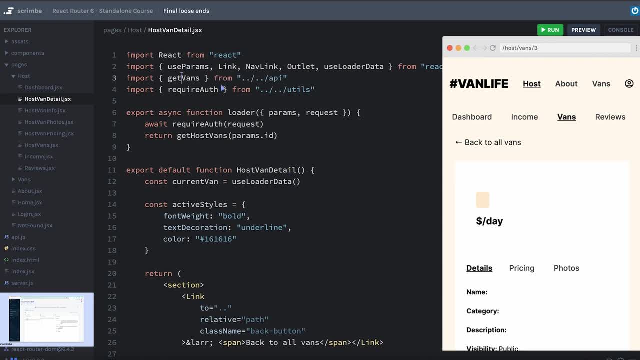 And instead of pulling in get host vans, I'm just going to pull in get van, as this will allow us to pass the ID, And I guess I'll need to change it down here as well. That way, this page will get fixed again. 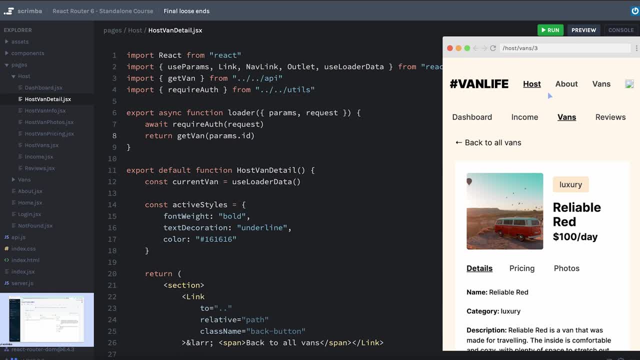 Of course, the problem is that anybody could go to this page and see this information, because we're using a more public version of this get van function. that doesn't really care what the currently logged in user is. For us right now, this isn't a big deal because we don't actually have any edit functionality. 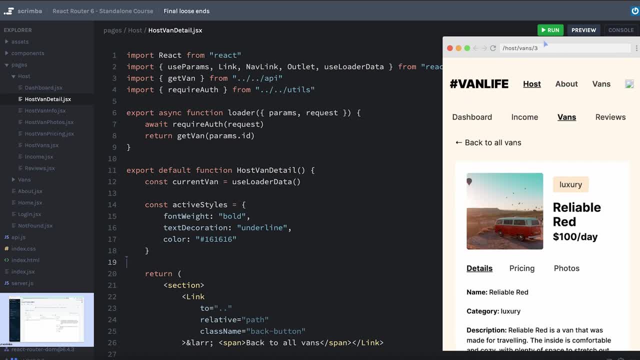 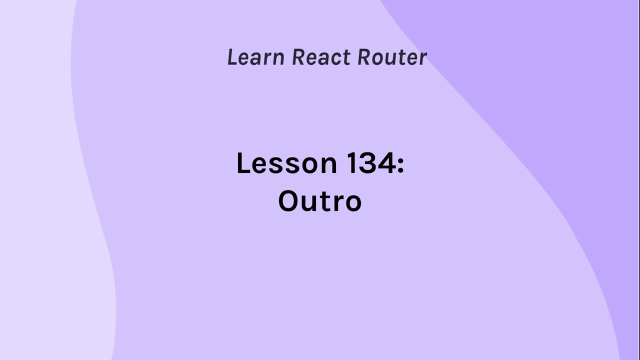 in our app At this point anyway, so it doesn't really matter. Somebody could just come up here and change the URL to instead of host vans three, they could maybe say host vans five and come to that page. But again there's no edit access, so it's not that big of a deal. 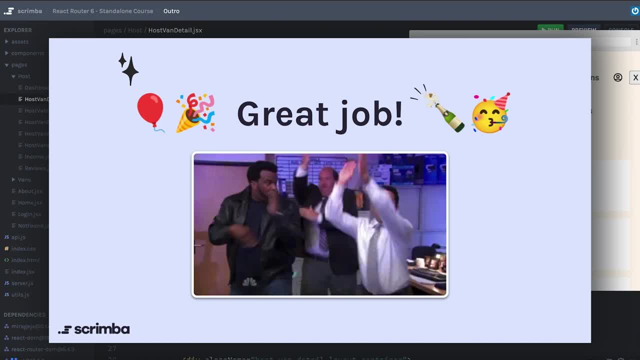 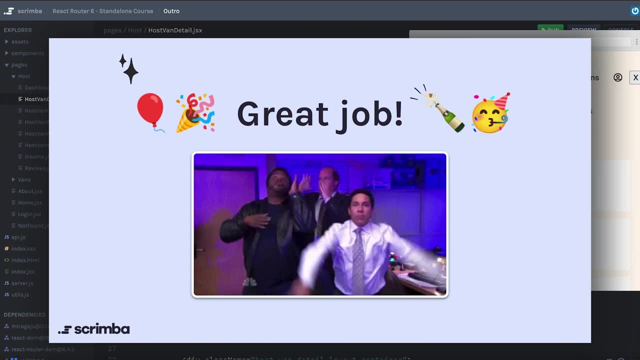 And that does it, folks. We are here at the end of the React Router course. Congratulations, Great job on all of the challenges that you did, all the quiz questions that you answered And, in the end, this amazing app that you had a chance to build by following this curriculum. 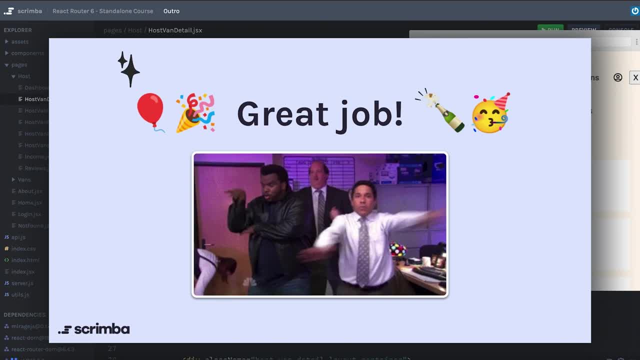 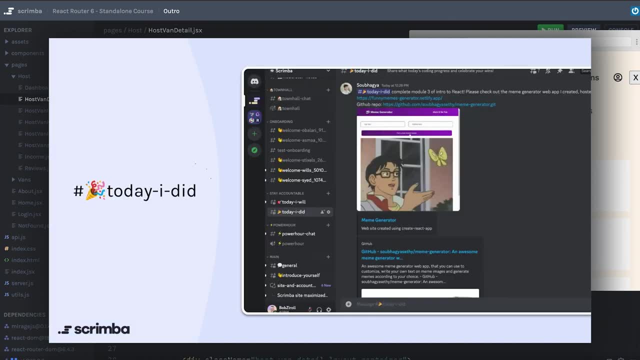 Hopefully this gives you a really great appreciation for React Router and just the concept of client side routing in general. There's a ton more that you could be learning, but I think this would be a perfect time to head over to the scrim but discord server and post something in the today I did channel. 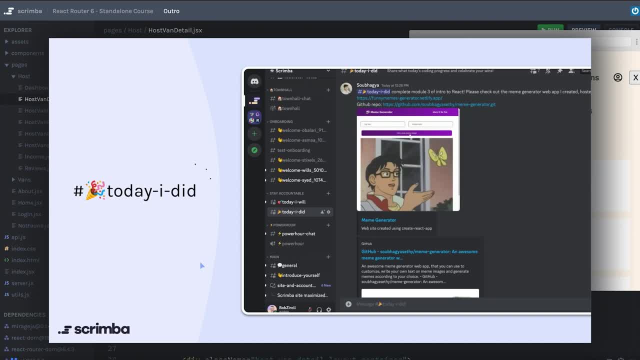 you can click the link to the screenshot here. that will take you over to the discord server and just let people know that you completed the React Router six course and that you completed all of the challenges along the way. So what comes next? Well, as I mentioned multiple times, we don't have real authentication in this app. 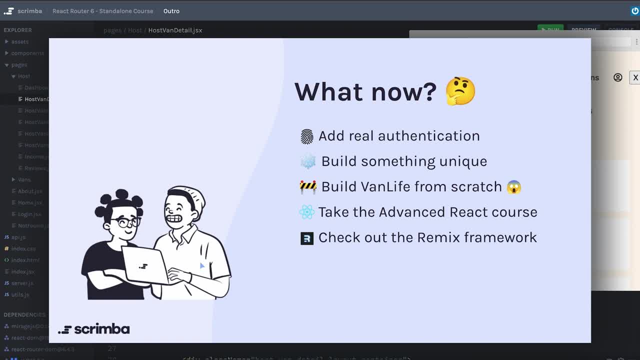 The main reason is because that would have taken us on quite a bit of a detour that I wasn't quite ready to do as a part of this curriculum, But that would be a great thing for you to spend some time on just learning how to add real authentication. 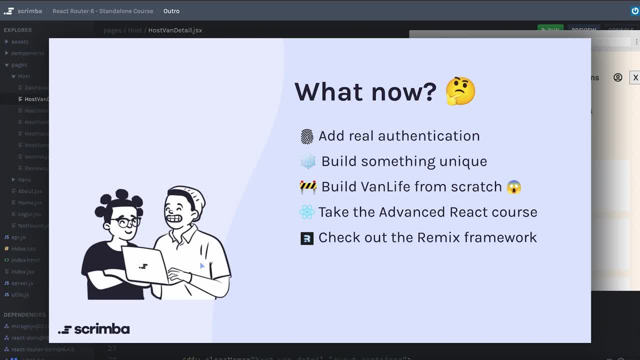 Another thing you could do is just to figure out a project that you are intrinsically interested in and build something completely unique. Now that you have the knowledge that you need to do client side routing inside of an app, the world is completely open to you. 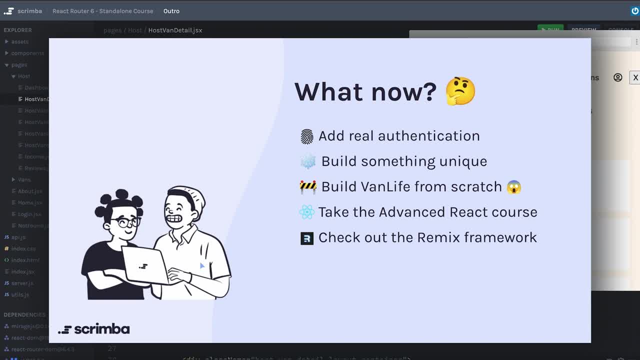 Another idea, and this is a little bit far fetched, but you could try to build this van life app again completely from scratch, entirely on your own. It might sound mundane when I say it like that, But the truth is that would be one of the best things you could do to solidify all of the information that we just learned. 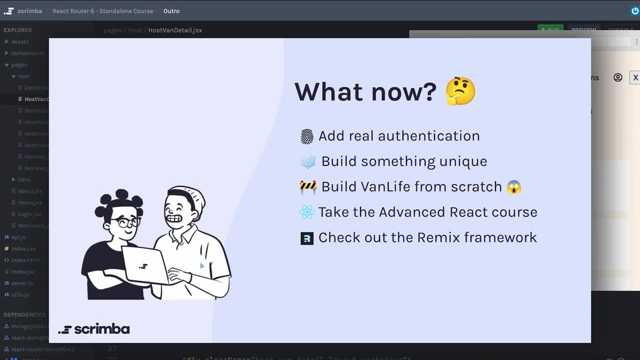 Even if you ended up building it in a fairly different way than what we did together, that's completely okay. It would be a great learning experience nonetheless. Another idea, and this is a bit of shameless self promotion, But since you have made it here to the very beginning of this video, I'm going to give you a little bit of time to think about what you're going to be doing in the next couple of weeks. And I'm going to give you a little bit of time to think about what you're going to be doing in the next couple of weeks. And I'm going to give you a little bit of time to think about what you're going to be doing in the next couple of weeks. 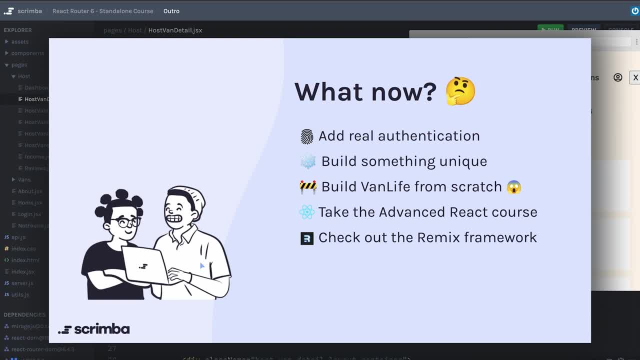 And you should've listened, as I've made it here to the very end of this course. I assume that you enjoy to some degree my teaching style And I apply all of my same pedagogy, including tons of practises, quizzes and project building over in my advanced react course on Scrimba. 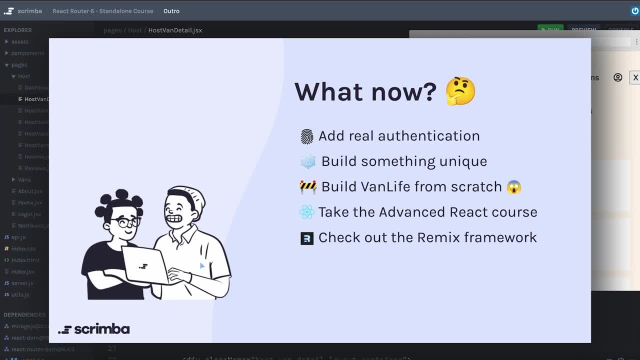 The advanced react course does require and Scrimba pro membership And it is part of the front end developer career path, which is tailored to helping people go from knowing absolutely nothing in web development all the way to being prepared for interviewing for their very first jobs. And, lastly, tips and tricks. in the end- And that's why we have connected Scrimba pro back here in塔 Dataworking to my website at traineeshipon leadingcom, And that's how you can start revising the Build your HomeOnline. 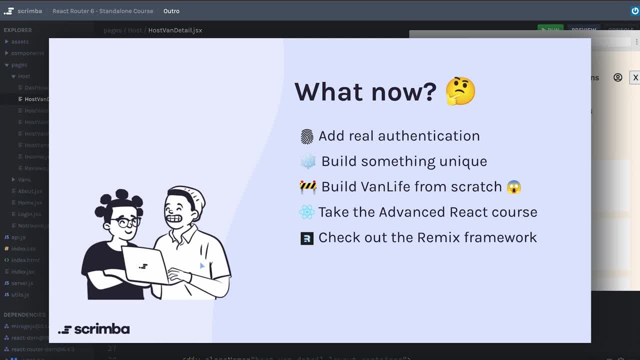 Lastly, you've heard me make the parallels a lot between React Router and the Remix Framework. I can highly recommend the Remix Framework. It's a great way to dip your toes into full stack web development. One of the greatest things I think about the Remix Framework is that their mantra. 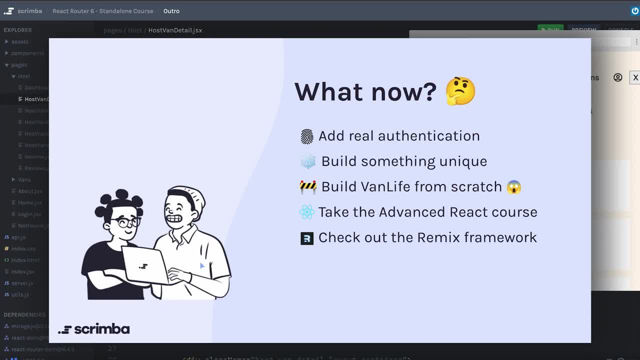 is to rely on the native web platform, And so for me personally, as I have been learning Remix, I have learned so many new things just about native web that I feel like I probably should have known at this point in my career. So feel free to check out the Remix Framework if you'd like to dive into.